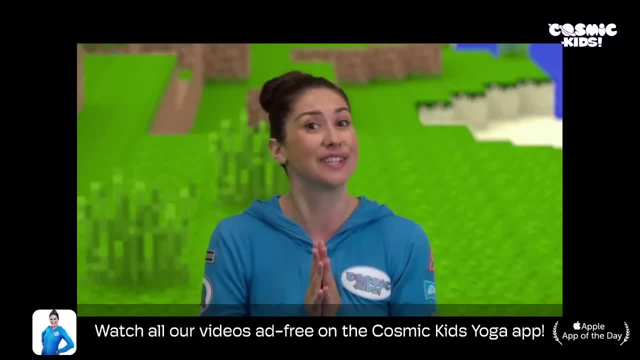 at our hearts and saying our secret yoga code word, which is namaste, Ready After three, One, two, three, Namaste There. Now we're ready to begin, and today we're in a world of blocks. This is Minecraft yoga. It's our first day here and we've got to get ready for what lies ahead. 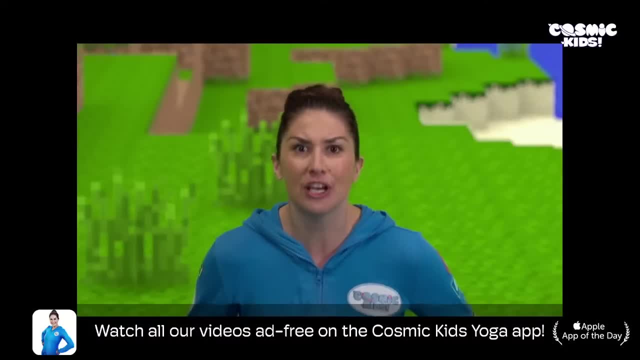 Now it's very important that we survive here in Minecraft, so we have to build a shelter, a house. Coming up to stand, jump your feet wide, take a deep breath in and out. Now we're ready to begin. Now we're in a world of blocks. This is 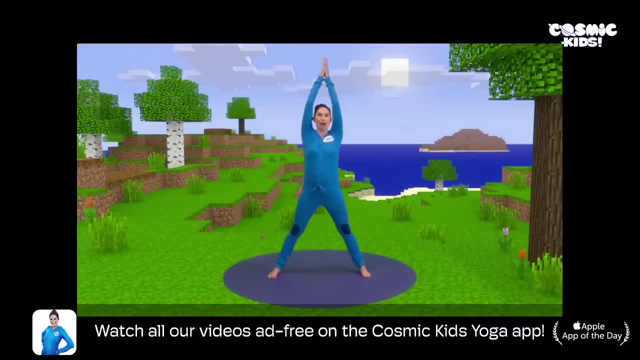 your arms wide and bring them up above your head. Coming into house pose. Very good, Now we can protect ourselves from all the mobs of monsters that spawn at night. Taking yourself all the way forward, see if you can grab hold of your ankles and then clomp them like a monster. 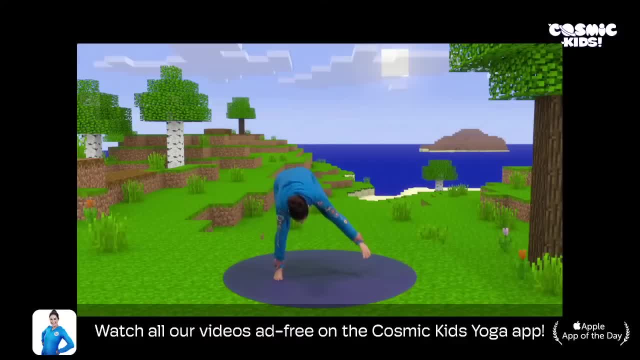 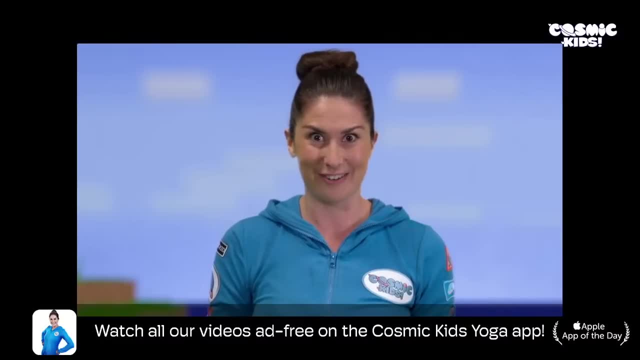 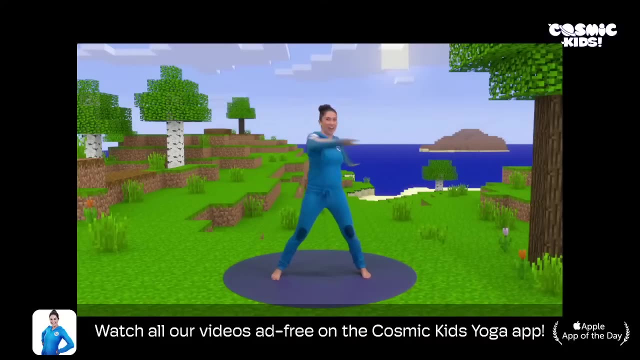 Ooh, Coming all the way up. Now, to get ready, let's spin into our Minecraft skin. Take your arms wide and begin to spin from side to side. Ooh, You can even close your eyes if you like. Wow, That's amazing. Now we jump our feet into the middle and, Oh, my goodness, I've got my 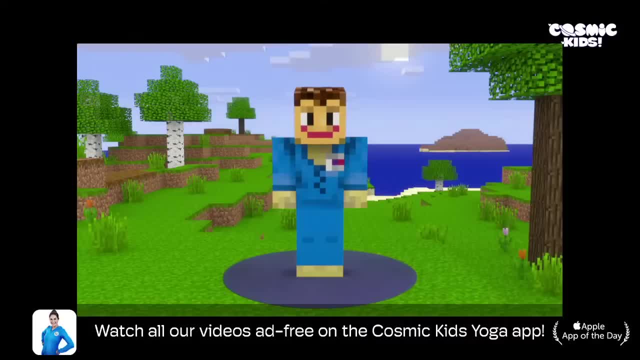 skin on. Oh, this is interesting, isn't it? I wonder how we can move. Let's lift our arms, Oh yeah, And lower them, Oh, that's fun. I wonder if we can do any yoga. Let's turn to the side. Here we go. Now let's fold all the way. 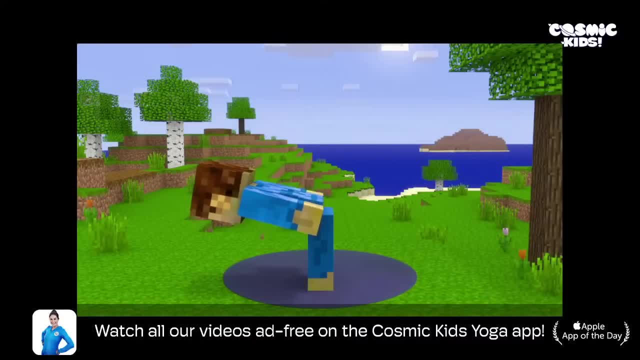 forwards. Oh, now I wonder if we can take our hands down. Oh, there we go. I wonder if we can touch our toes. Let's reach down and Oh yeah, Oh yeah, Oh, we did it And come all the way. 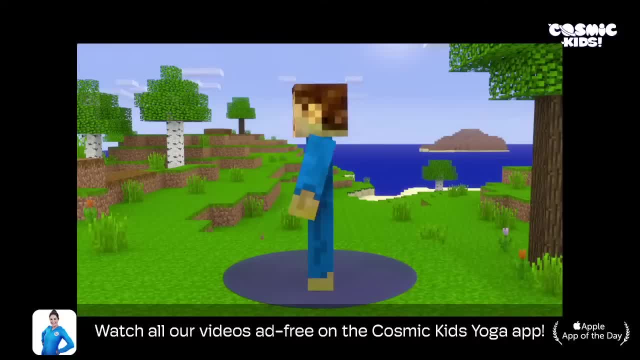 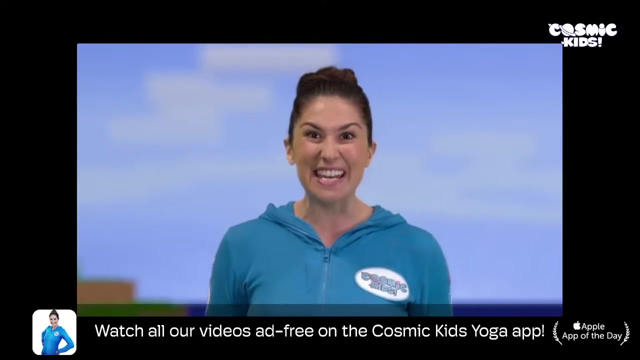 back up again, Ah, and put your arms down, Oh, and turn to the front. There we go. Hmm, It's going to be quite interesting doing yoga wearing this. Maybe we can just pretend we're wearing the skin. Let's shimmy and shake it off. Ah, that's better. Now you can see me again And I can see you We. 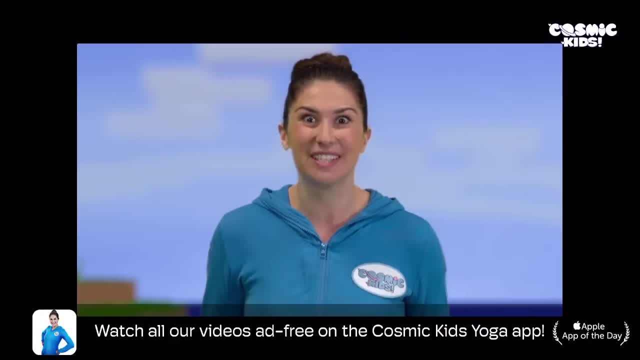 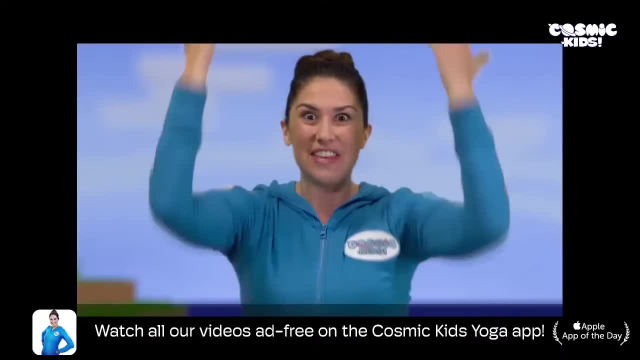 begin by looking up to the sky and seeing the sun's out. So we wave and say hello sun, Reaching all the way up and say hello sun. This is brilliant. It means we've got plenty of daylight to collect all the things we need to craft. Now let's have a 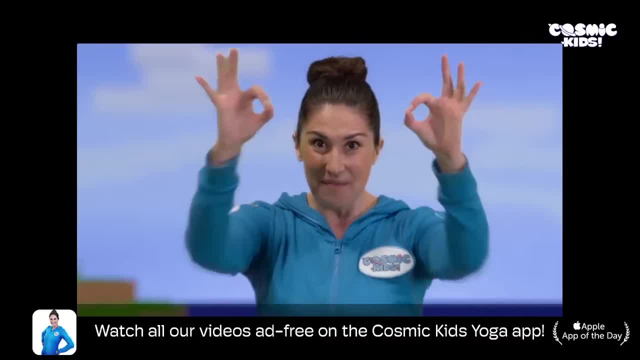 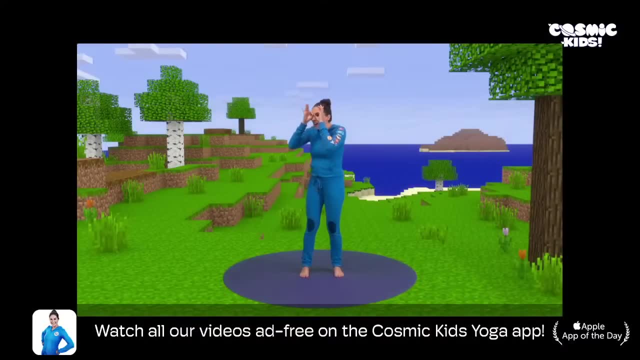 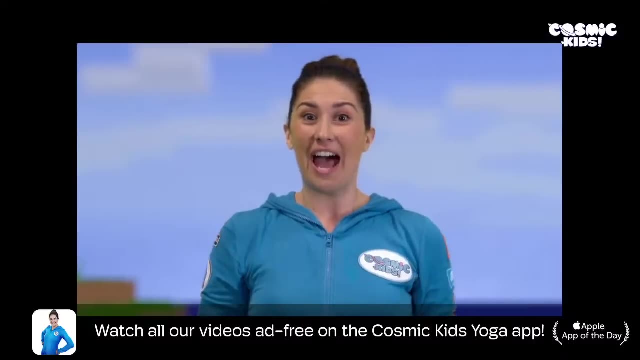 look around at where we are Joining your thumbs and fingers together. have a look through. Oh, it looks like we're on an island, surrounded by an ocean. There are trees and rocks and all sorts of things- Plenty of what we need to get crafting. We lower our hands and we 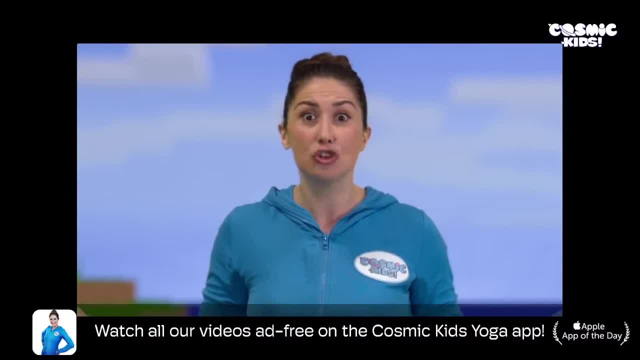 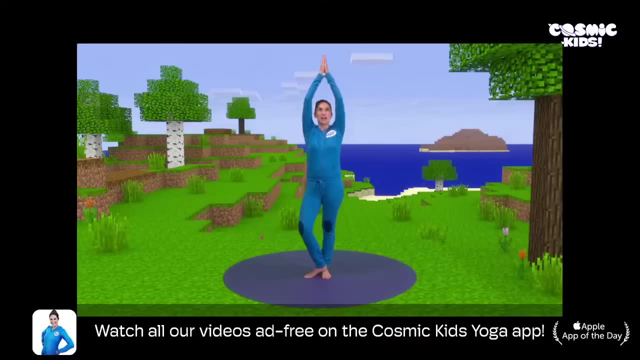 have to build a shelter, don't we? So look around and we see trees Coming into tree pose, bringing one foot on top of the other, your hands together, and grow your tree up nice and tall. Now I wonder how strong are the trees here in Minecraft? I'm going to. 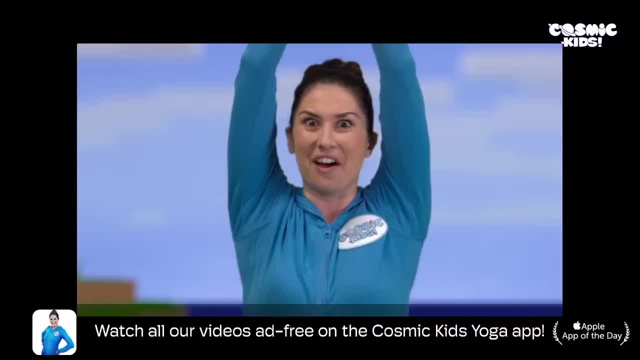 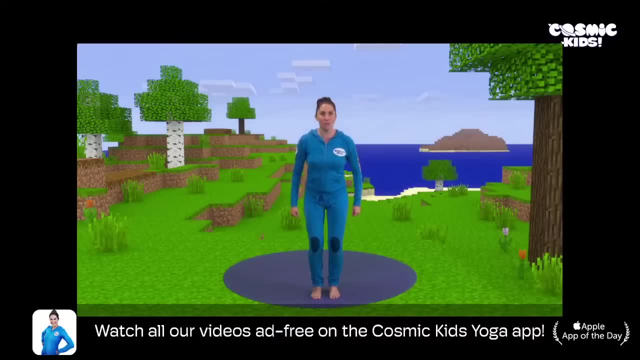 come and try and blow you down. You stay tall and strong. Here I come. Oh my goodness, you're so good at balancing. Let's try our tree on the other side. Coming to stand with the other foot on top now using your heel, balancing on your toe. 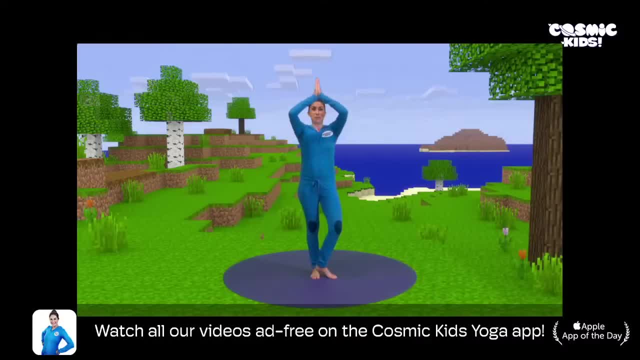 Bring your hands together. Oh, try not to wobble, and come up tall, like a very tall tree, And can you open your Minecraft tree branches? Very good, everyone. Now we've only got our bare hands to chop these trees down, So let's come into woodchopper pose. Turning to the 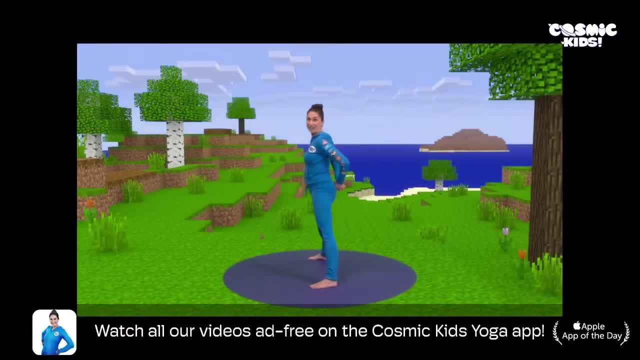 side, spread your legs nice and wide and crisscross your fingers behind your back, Stretch your arms up behind you and then fold forward as you chop. One, two, three, chop And up. One, two, three, chop And up. Last time, One, two, three, chop And all the way. 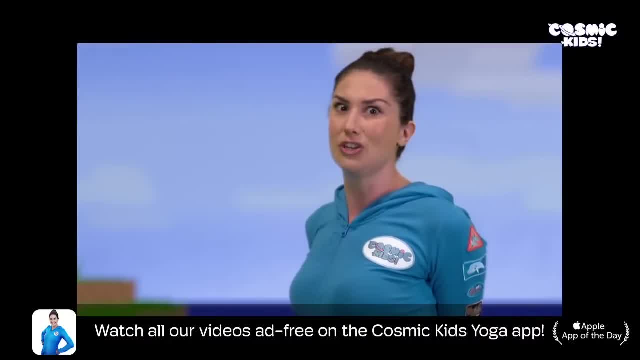 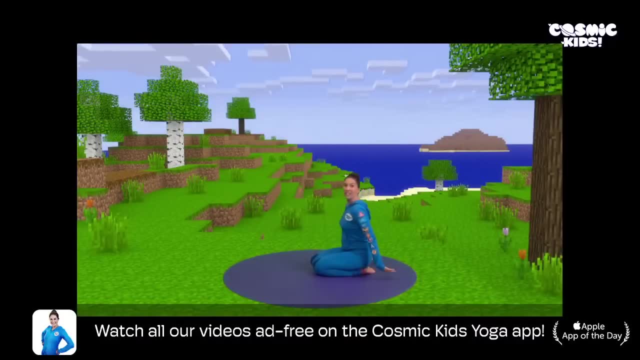 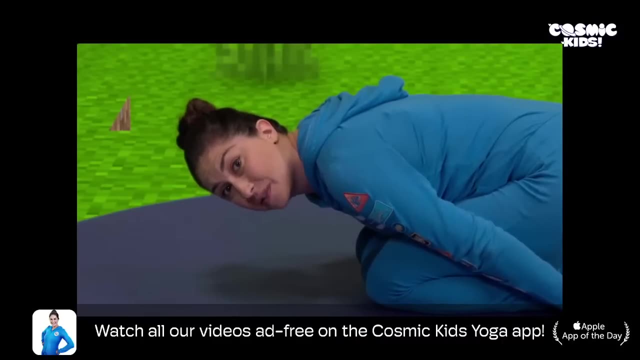 up. Very good, everyone. Now we've collected lots and lots of blocks of wood. Coming into a block of wood, pose Down onto your knees, Tuck yourself up into a tiny block shape. Ooh, brilliant. Now we need to turn these blocks into planks of wood. 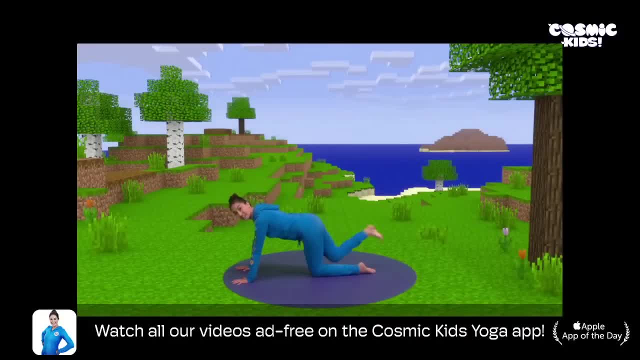 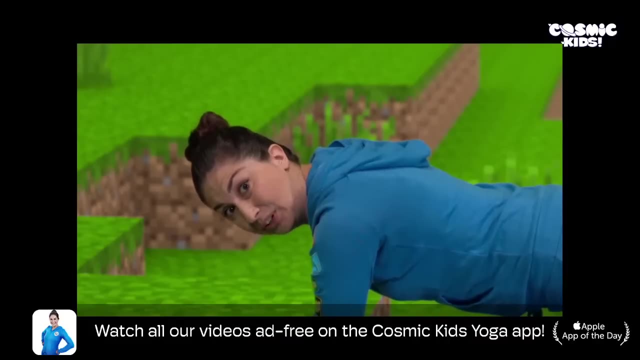 So take your hands forward, come up onto your hands and knees and stretch one foot back, two feet back and come into plank pose, Pulling your tummy nice and tight in your plank pose. Very good, Now with our planks we can make a very important thing: A crafting table. 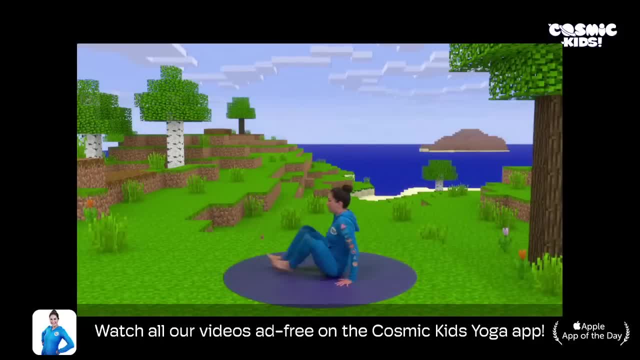 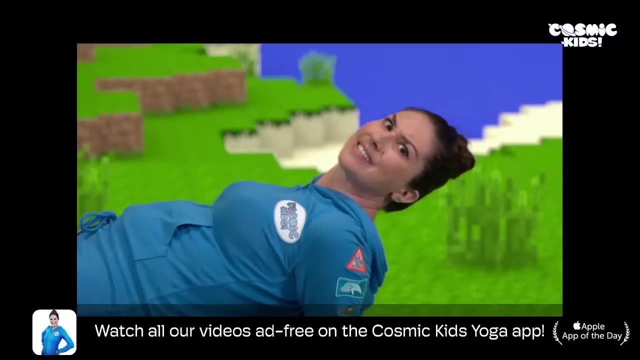 Coming into table pose, Coming to sit on your bottom with your knees bent, your feet flat and your hands behind you And lift your bottom up. coming into your crafting table pose. Very good, Now we can make all the tools we need. Let's start with a pickaxe We need. 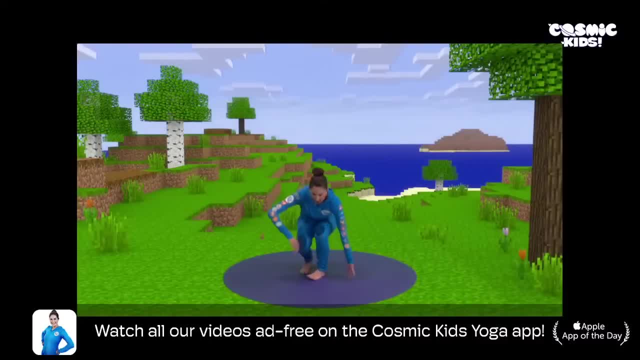 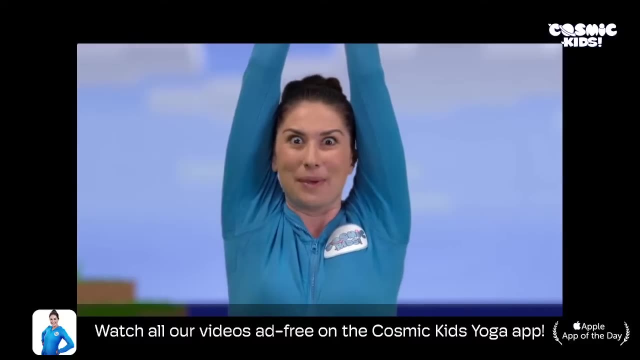 to make some sticks Coming to stand in stick pose, Standing with your toes together, Your hands up above your head, Making yourself as pointy as you can. Very good, everyone. Now we balance two planks on top of our stick to make a pickaxe in a triangle shape Coming. 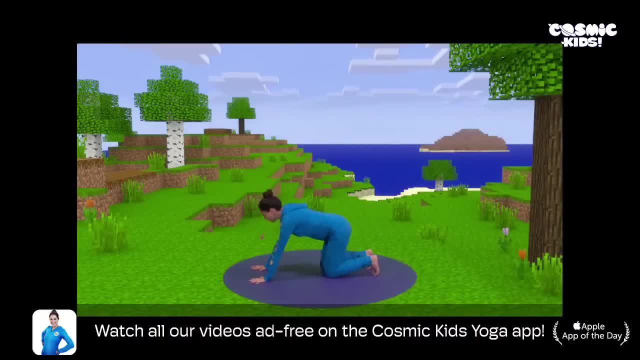 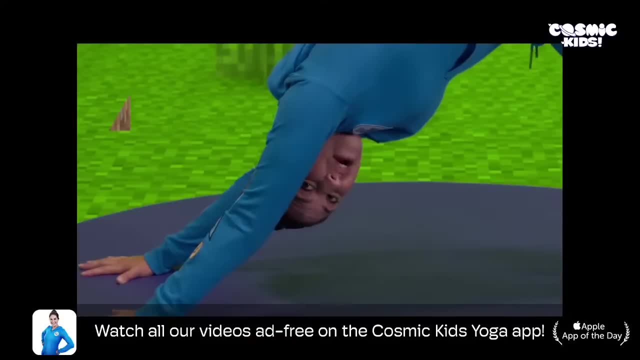 into dog pose. Onto all fours, Hands wide, Tuck your toes and lift your toes. And now we're going to make a stick. We're going to make a stick. We're going to make a stick. Lift your bottom up to the sky, Coming into your dog pose. Yay, Now we've made a pickaxe. 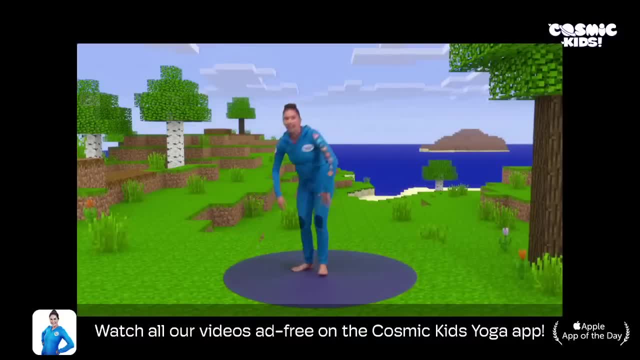 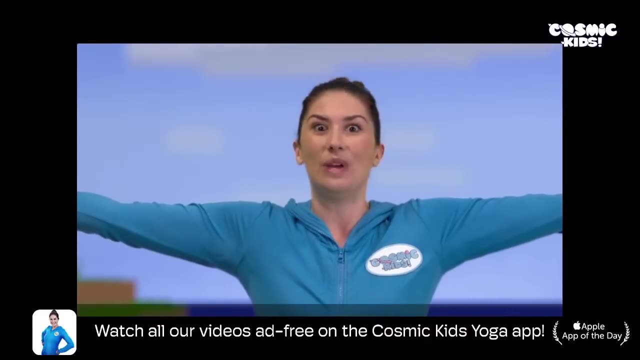 We need to go and find some coal Coming up to stand. We find a giant stone wall. Hmm, There could be some coal in here. We jump our feet wide And our arms wide, Making a giant stone wall shape. Very good, Now we've got our pickaxe, We dig at the stone wall. 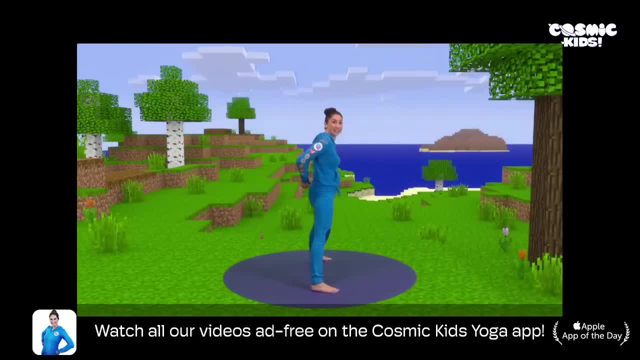 Turning to the other side. now Stretch your legs wide, Criss-cross your feet, Make your fingers stretch them out behind you And fold forward after three with a dig: One, two, three, Dig And up. And again: One, two, three, Dig And up. Last time, One, two, three, Dig. 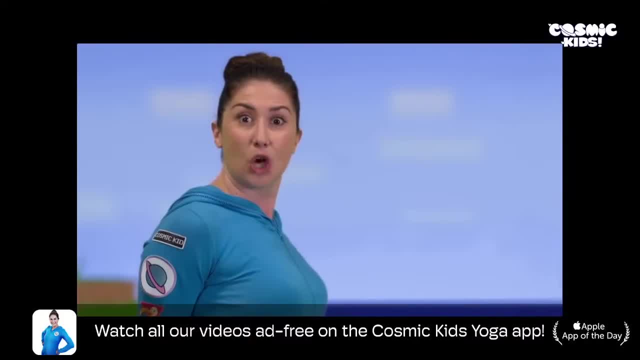 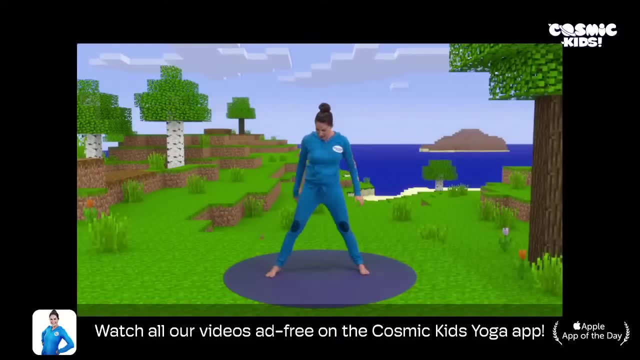 And all the way up again. Very good, We've found some coal And we've managed to dig ourselves a cave. This can be our shelter. Coming to stand with your legs wide, Making your hands above your head In your cave pose. Well done everyone. Now with our coal. 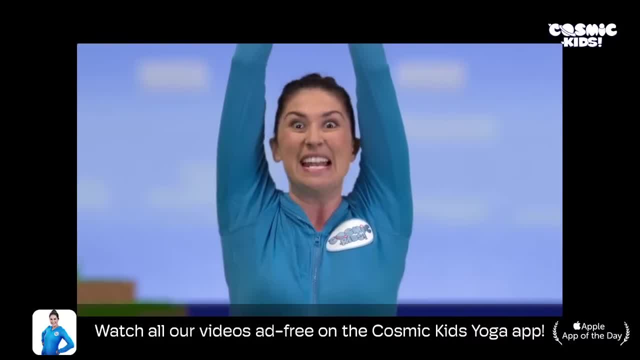 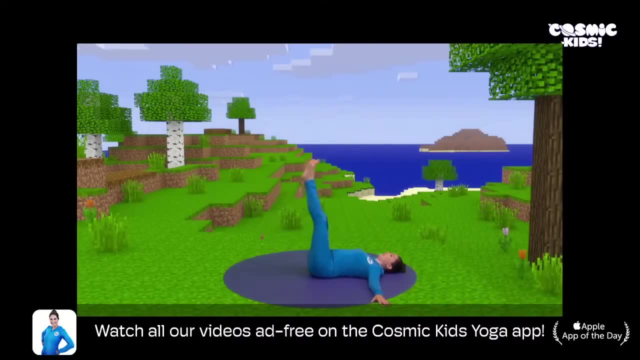 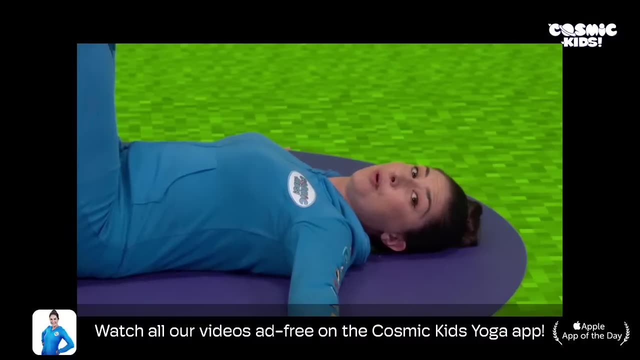 and our sticks. We're going to make some torches. Let's come into candle pose Lying down on your back, Stretch your arms out wide And lift your legs up to the sky And wiggle, waggle your toes Like flames. Very good, We've put the torches up on the walls of our cave And 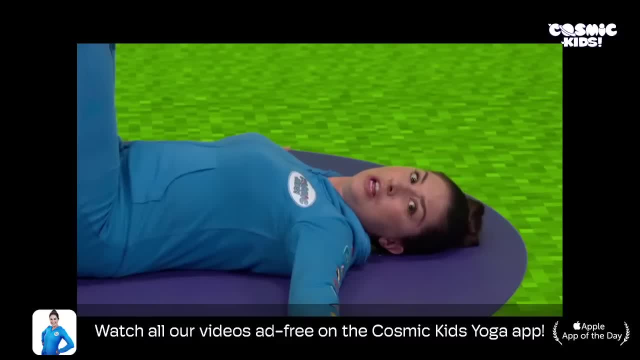 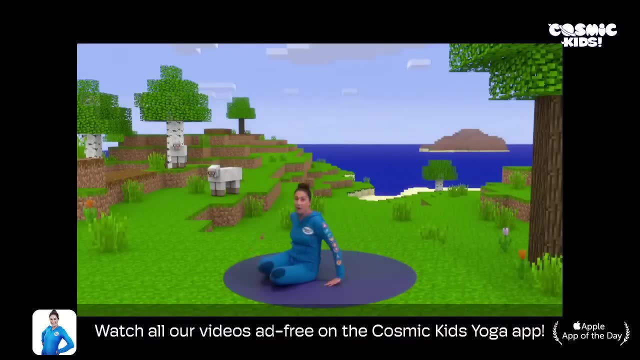 we've got light. Well done, everyone. Look outside our cave. We see some sheep Coming into sheep pose, Sitting all the way up On your hands and knees. Let's wiggle, waggle our tails And let's go. We could do. 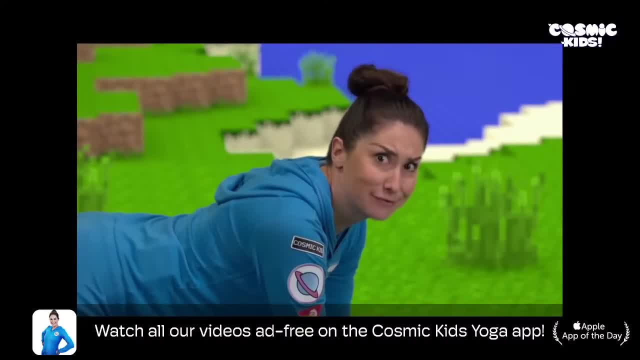 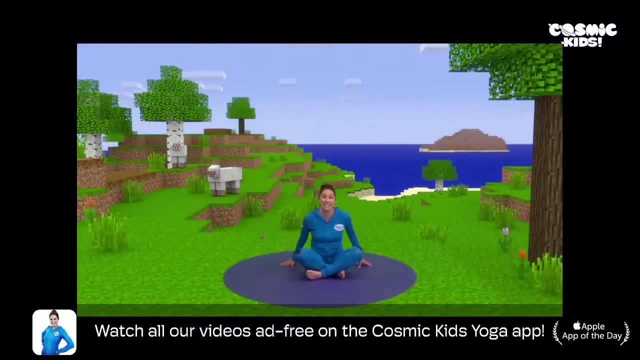 with some wool So that we can make a bed. Sleeping is very important in Minecraft. It's how we stay safe at night. We sit on our bottoms, We bring our hands together And we say bar-a-stay To thank the sheep. 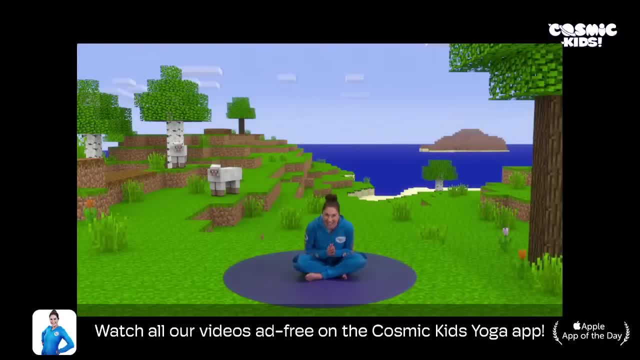 Ready Bar-a-stay- Brilliant. We take the wool And we add it to a block of wood to make a bed. Coming into bed pose. Turning to the side again, Knees bent, Feet, flat Hands behind you And lift up your bottom. Coming into bed pose: Excellent. Now we'll 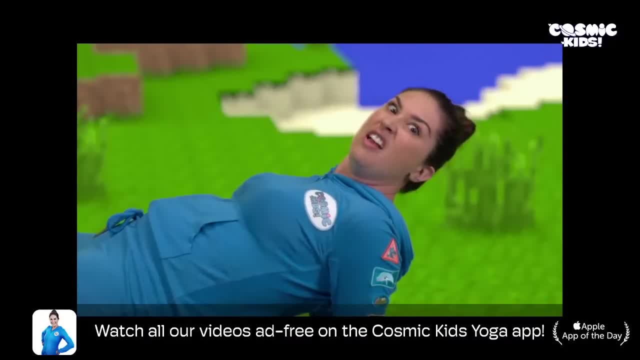 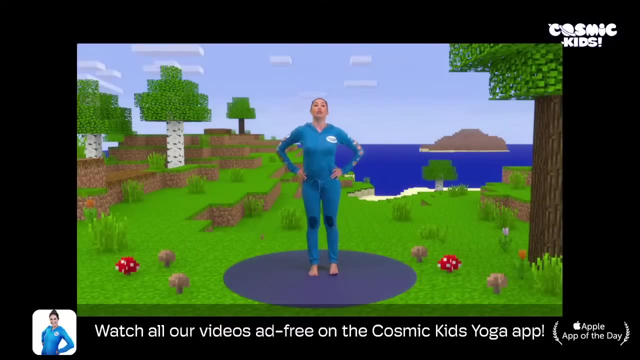 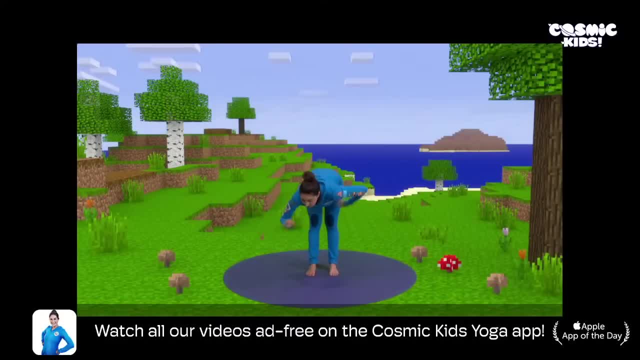 half way forwards As we pick the mushrooms, Picking them out of the ground, Collecting lots and lots and lots. Fantastic. Now we stand up tall. We need to craft a bowl So that we can put our mushrooms inside, Coming into bowl pose, Lying on your bellies Put. 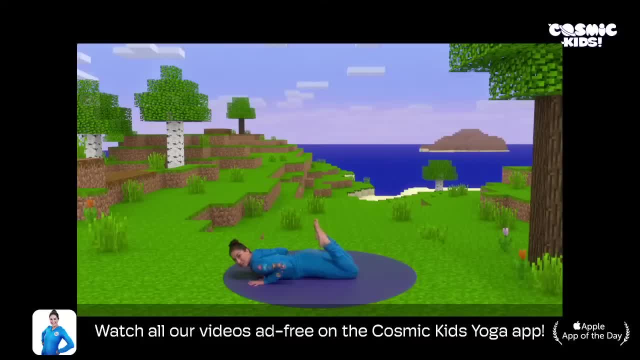 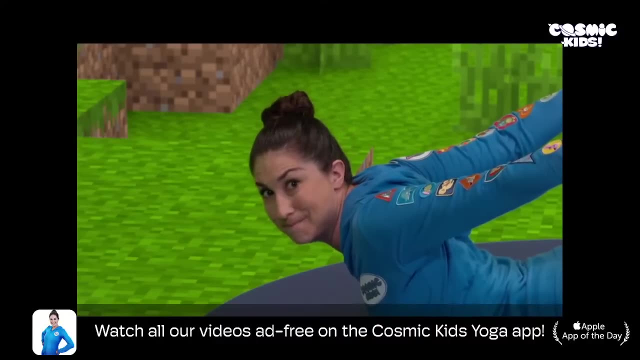 your hands under your shoulders as you bring your feet towards your bottom. Then reach around And see if you can grab your feet. Now breath in as you lift up. Very good In in your bowl pose. We put the mushrooms inside and we can make a mushroom stew Coming up. 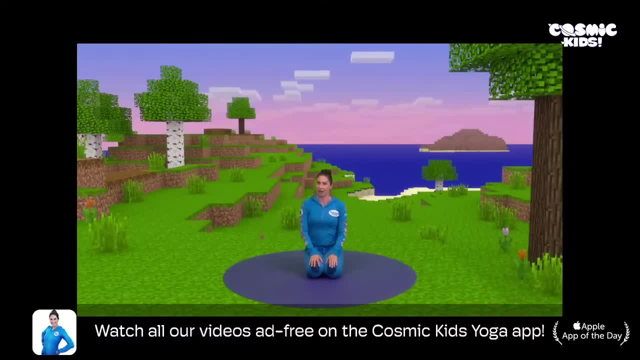 to sit. Now we need to make ourselves a door so that we're secure at night. Let's come into door, pose High up on your knees, take your leg to the side and your arm up to the sky. Let's see if it works by opening it. Very good. Now let's see if it closes. Two: 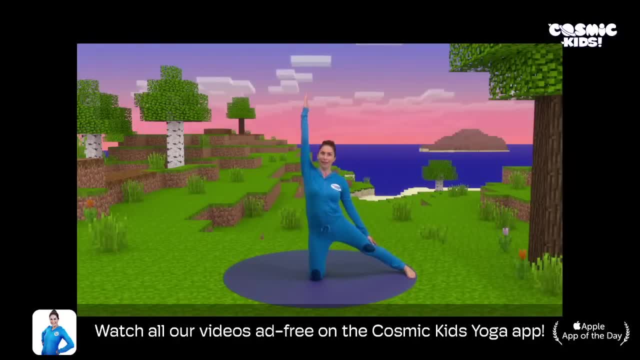 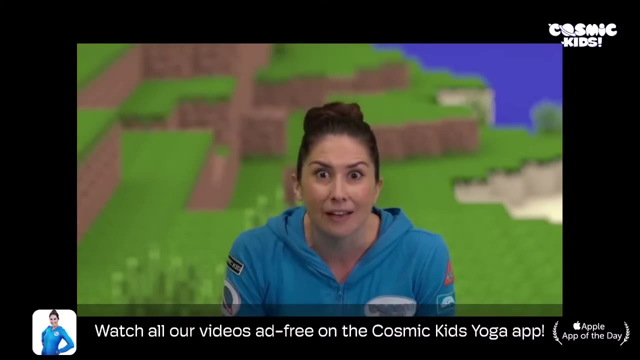 knees together, leg to the side arm, to the sky and close it. Brilliant, That's made good use of our planks. Now we're inside. We look outside and we see that the sky is turning from orange to pink to purple. It's dusk. Now we're inside, We build ourselves a chest. 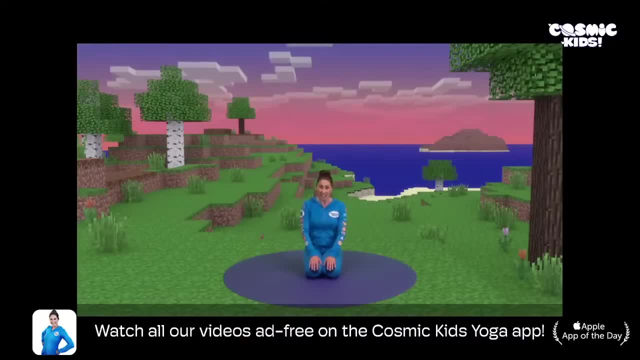 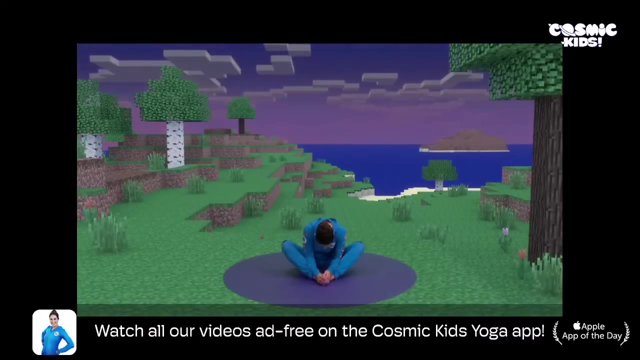 so that we can put away all the things that we've collected. Coming into chest pose: Sitting on your bottoms, joining the soles of your feet, Holding on to your toes, and close your chest down, putting your head towards your toes. Fantastic. Now we look up because outside it's night time. This is when all the mobs 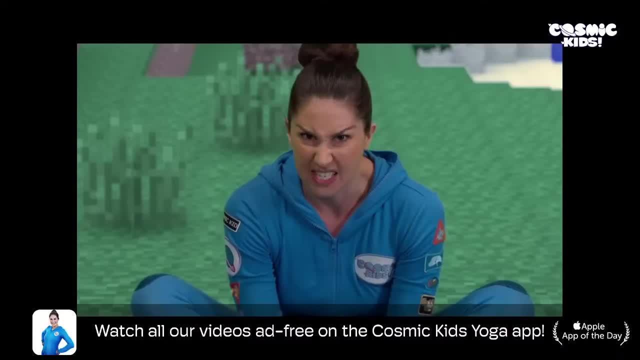 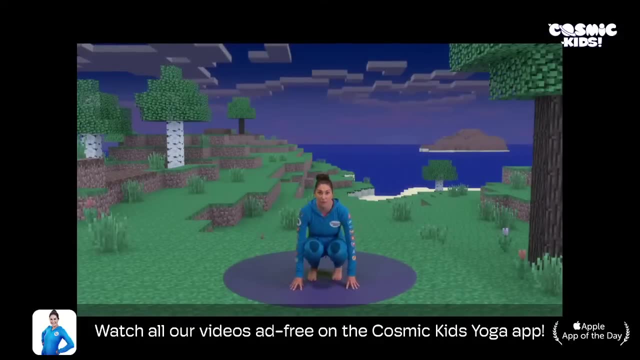 of monsters spawn. We've got to be ready for them. So let's talk about what we're going to see. There might be some creepers- Creepers- coming up to stand up on your tippy toes- everyone, because creepers like to stand on your toes. Creepers like to stand on your toes- Creepers. 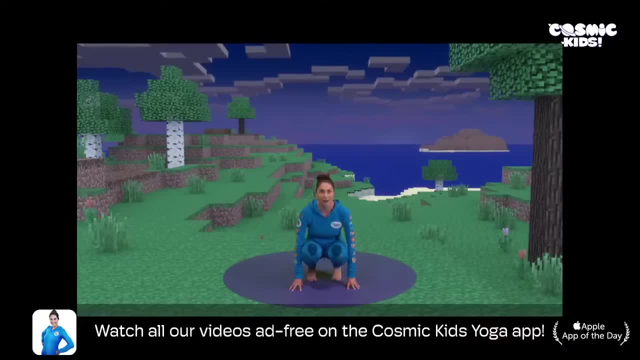 like to come up to you and blow themselves up with a kaboom. After three, let's jump and kaboom. One, two, three, kaboom. Oh, we stand up. If we see one of these, we need to run away, Run Now. there are also zombies that come out at night, Coming to stand to. 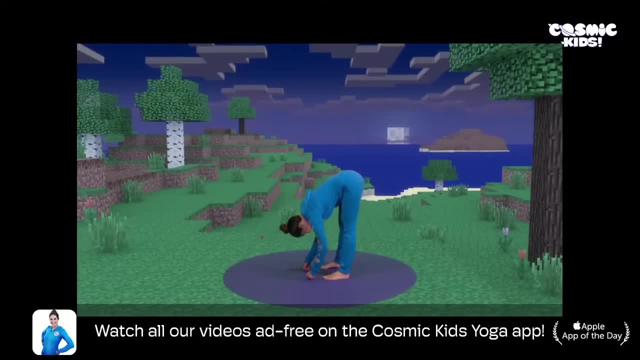 the side, roll all the way forwards and slowly roll yourself up to stand. Oh, you're going to be a zombie. Oh, and bring your arms up in front of you, Turn to the front and, like a zombie, tilt from side to side. Oh, zombies have lots of friends and they often bring. 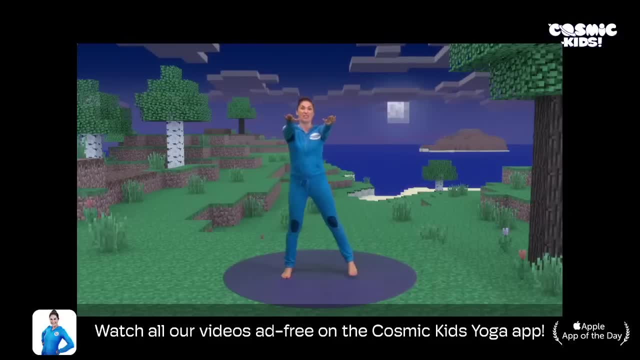 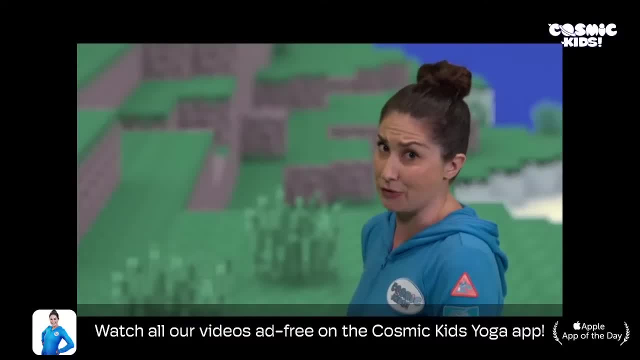 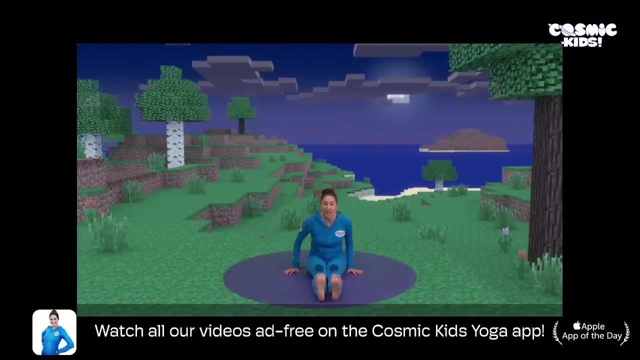 oh Now, there might often be some skeletons around And they have bows and arrows. Let's come into archer pose Sitting with your legs out long. take two fingers and put them between your big toe and your second toe. Bring your elbow back towards your ear and see if you. 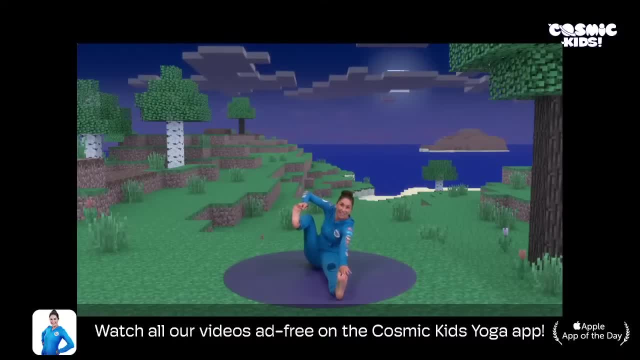 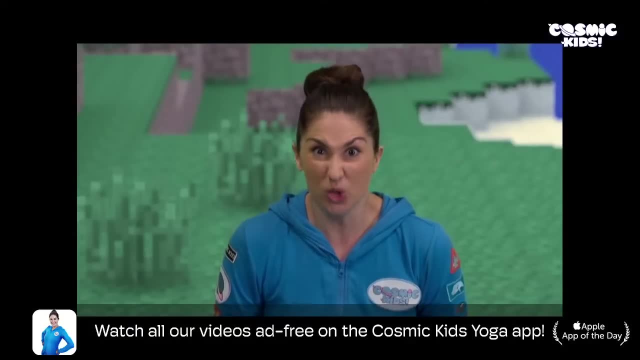 can reach forward to your other foot and fire your arrow Ready. One, two, three, pew. We better be careful. We don't want to meet any skeletons. There are also witches coming with us. There are also devils. You can't have most of them. Here's the big one, which is 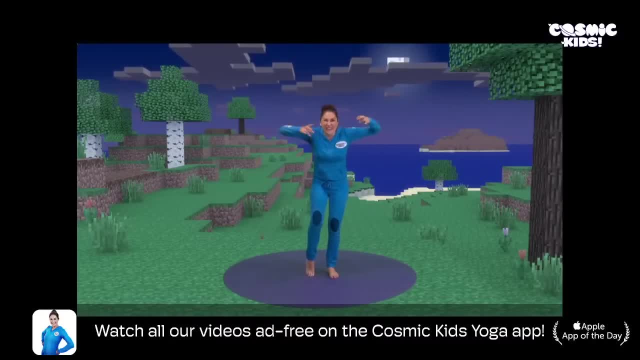 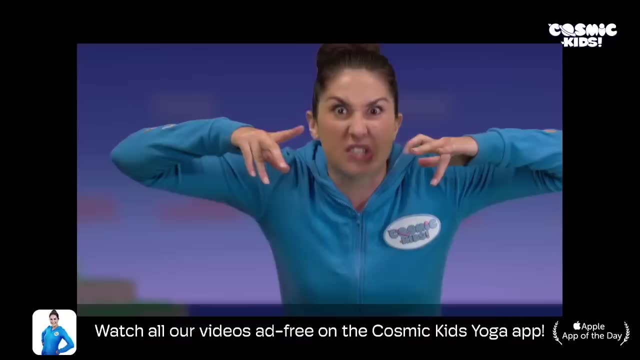 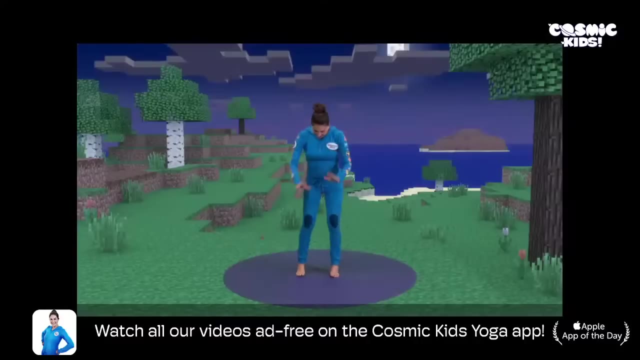 Coming into witch pose, standing up onto your craggy toes and your fingers and maybe a craggy nose. Oh, they like to cast spells and use magic and there are spiders. Let's come into spider pose, Standing with your feet just a little bit wider. 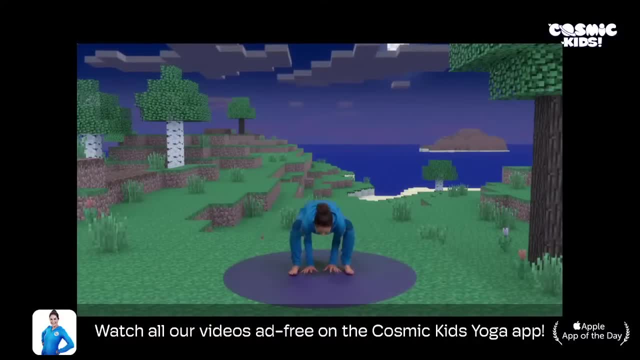 bend your knees and bring your hands down in between your feet. Now ticka, ticka, ticka, ticka your hands around to the outside and rest your feet, your legs, over the top of your arms in spider pose. Now spiders like to come in from above. 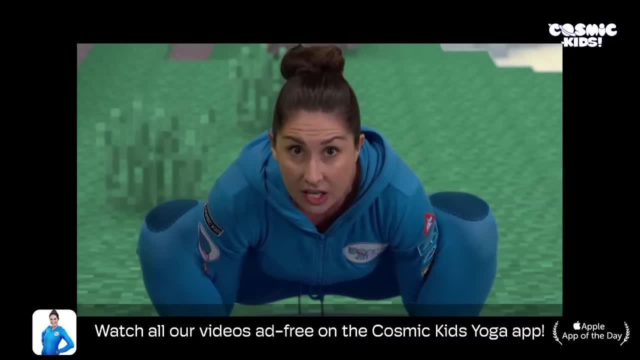 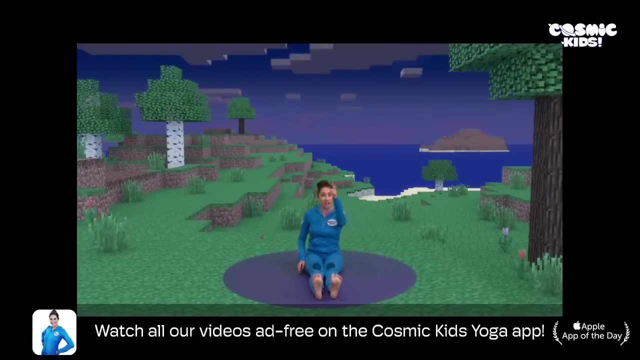 Oh no, look, one's coming in now, but there's a skeleton and he's shooting it with his bow and arrow Sitting on your bottoms, legs out long. take your other two fingers between your big toe and your second toe and bring your elbow back. 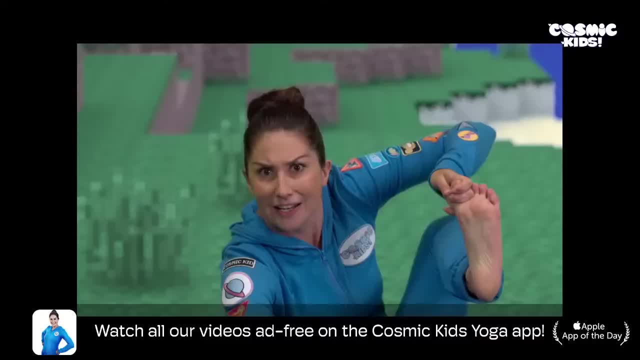 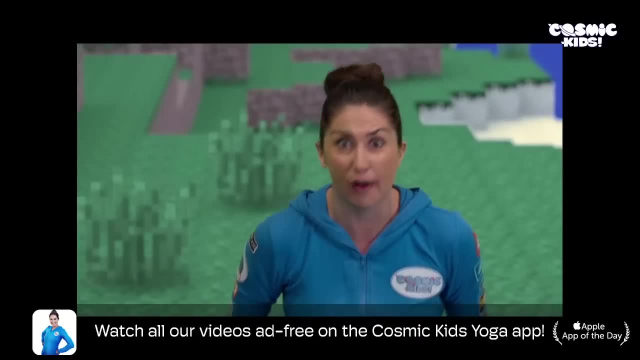 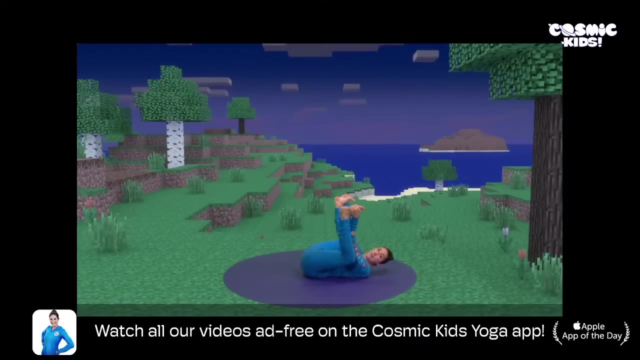 Then reach forwards and grab your other foot and watch the skeleton fire its arrow to the spider. One, two, three, Oh, the spider keels over into happy baby pose, Lying on your backs, everyone holding onto your feet, in happy baby pose. 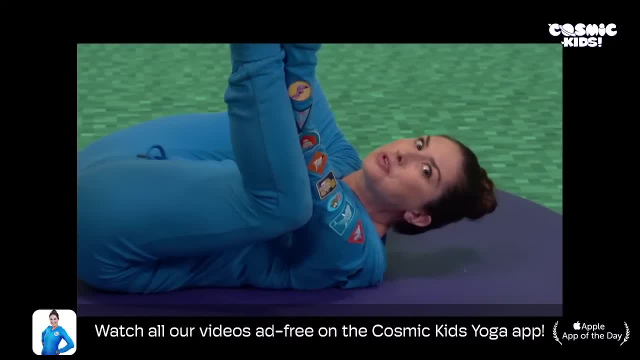 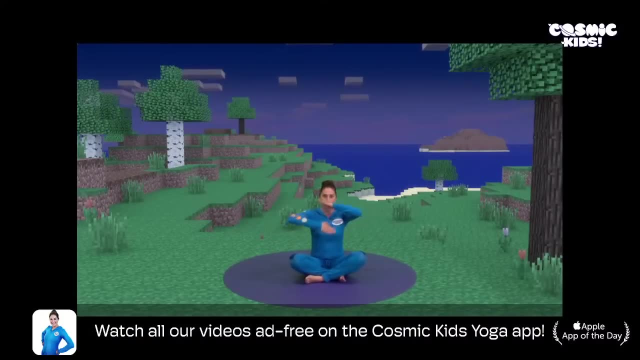 Well, this is good news. This means we've collected some string Sitting up tall crossing your legs. let's roll the string up in front of us And let's put it in our chest. Now we need to go to sleep so that we don't have any more danger tonight. 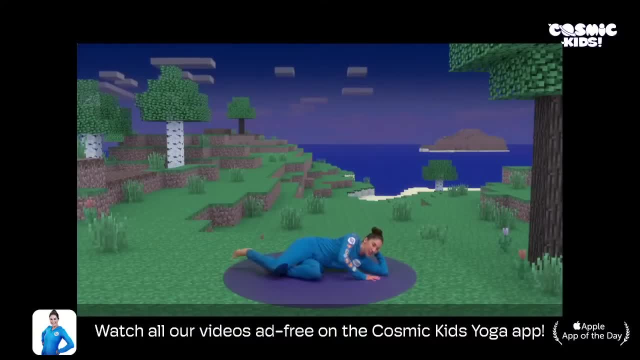 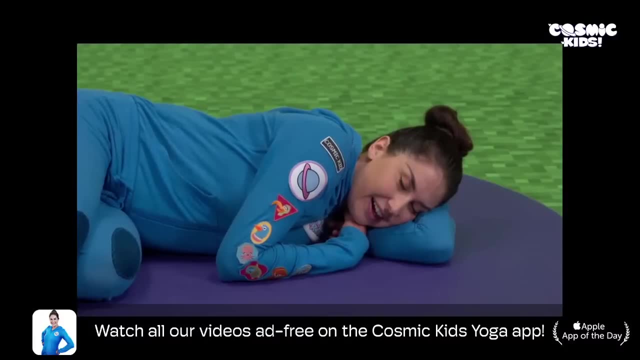 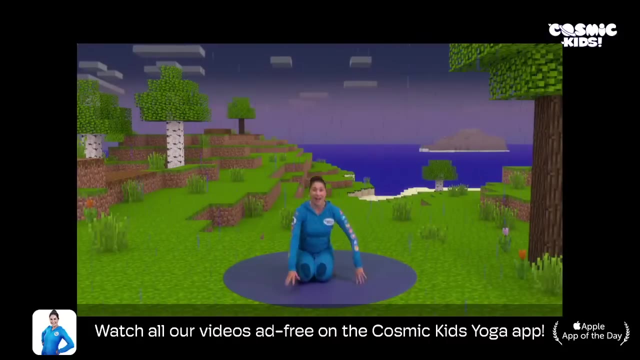 So we huddle ourselves down into a comfy position in our lovely beds and we feel safe. In the morning we wake up and it's raining, Coming up to sit on your knees. pitter patter on your faces and on your heads, Oh my goodness. 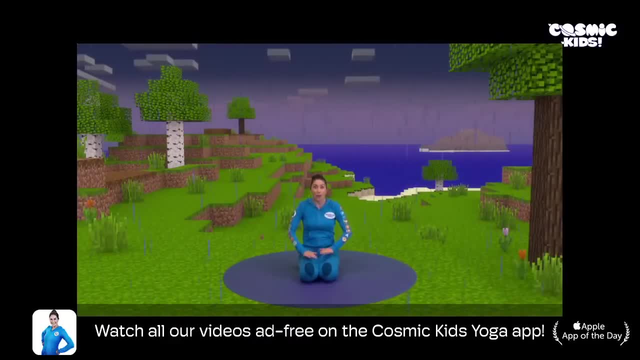 Me. This is exciting. It's daylight again, so we're safe. So we decide to build a boat. We're going to go fishing today, Sitting on your bottoms. lift up one foot, lift up two. Lift up one hand. lift up no hands. 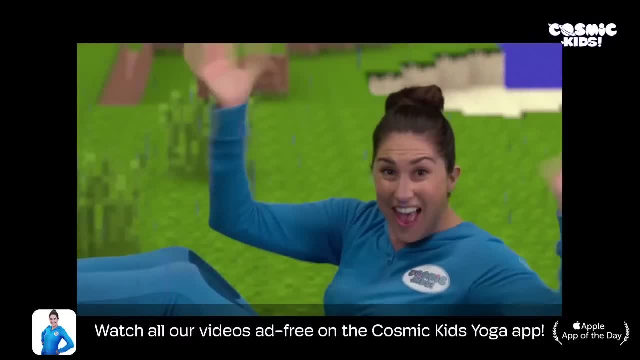 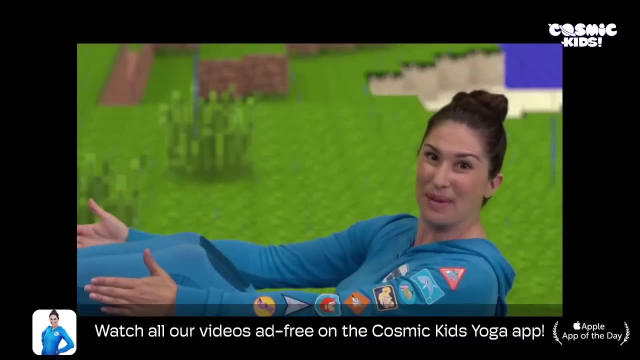 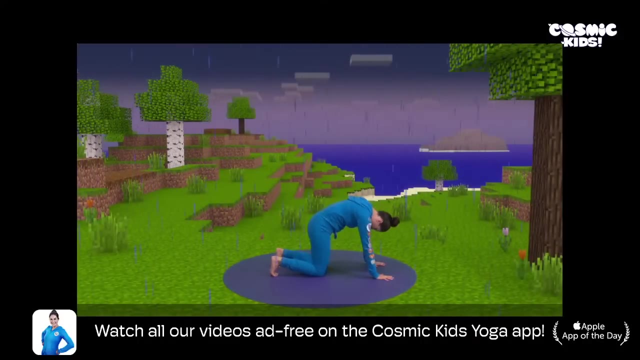 Yay, in boat pose. Give me a wave. Yay, Now, who's this coming to see us? It's our friend Stampy Cat Coming into cat pose. everyone On all fours, Fingers spread wide, tuck your toes, arch your back up and look into your belly button. 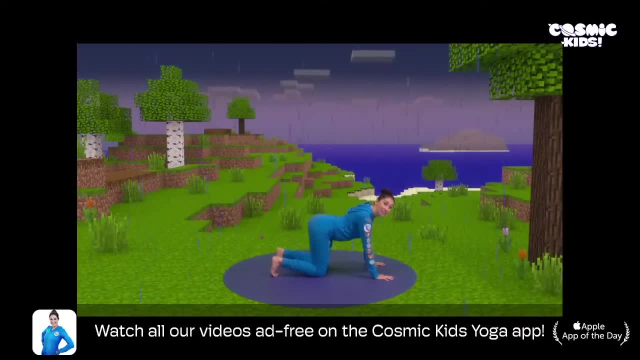 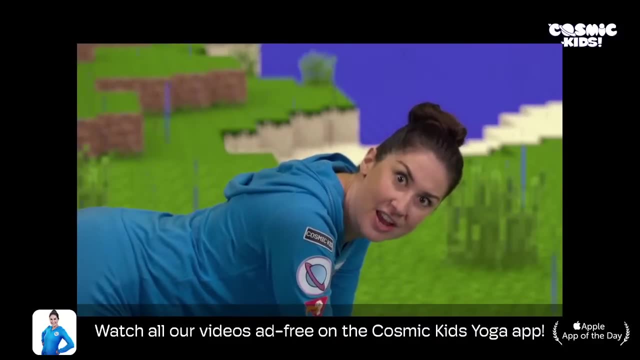 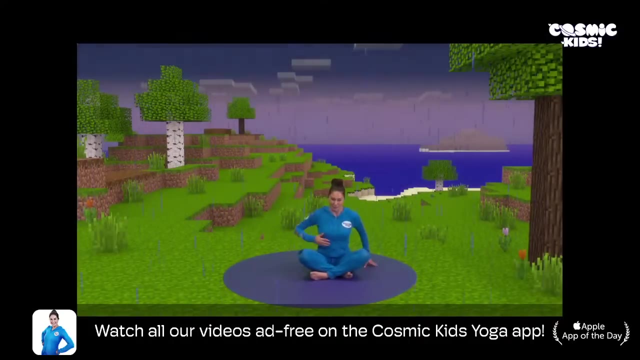 and then lower your belly down and wiggle, waggle your tail and go meow, Meow. He's brought a treat for us for breakfast: Some cake, Sitting on your bottoms, crossing your legs, rubber hand on your tummy, Pat your head at the same time as you eat your delicious cake. 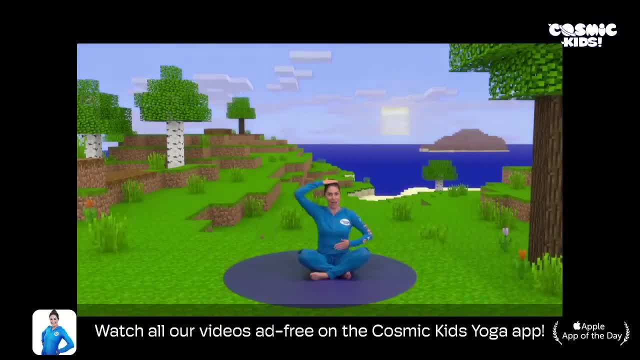 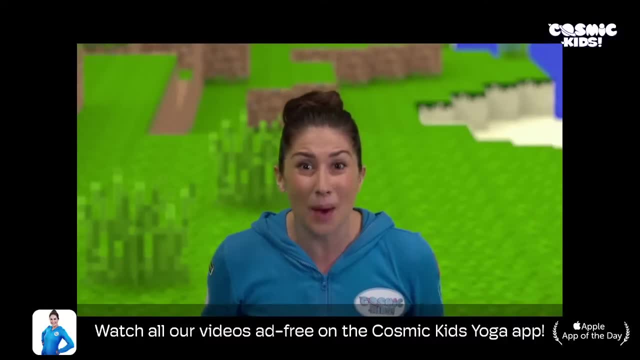 Can you do it the other way? Rub your hand and pat your head? Very good, Look, the sun's coming out and it makes a rainbow appear in the sky. Let's come into rainbow, pose High up on your knees everyone, Take your arms wide and drop down onto one side. 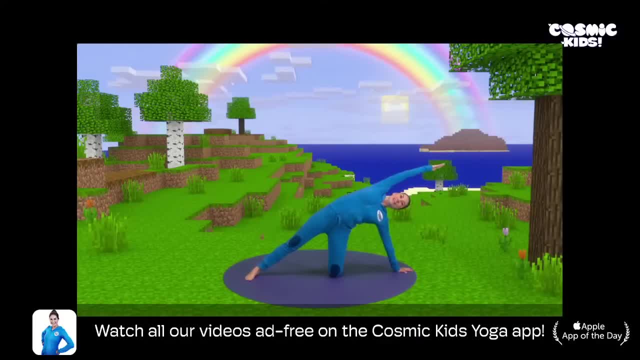 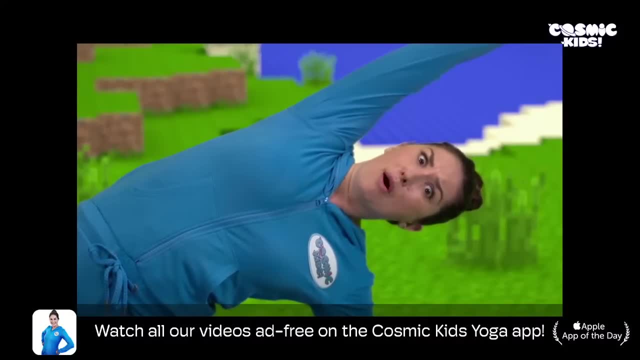 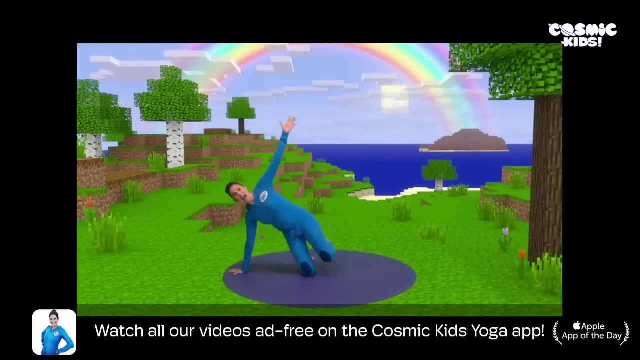 Stretch your leg out and reach your arm up and over your ear, Coming into your beautiful rainbow pose. Now we sit with Stampy and he knows an awful lot about Minecraft Coming into rainbow pose the other way, Two knees together, arms wide. drop down and stretch your leg out. 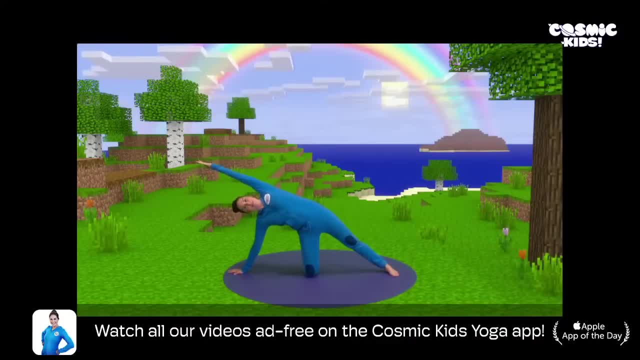 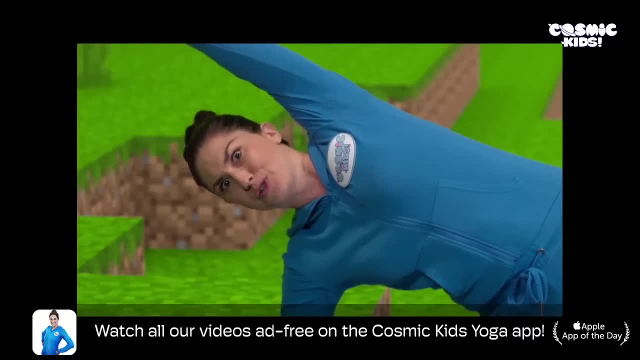 Reach your arm up and over your ear, Coming into a full rainbow. Very good, everyone We wonder whether Stampy could ever craft a yoga class into Minecraft's world. That would be funny, wouldn't it, if you were playing Minecraft and you came across a yoga class. 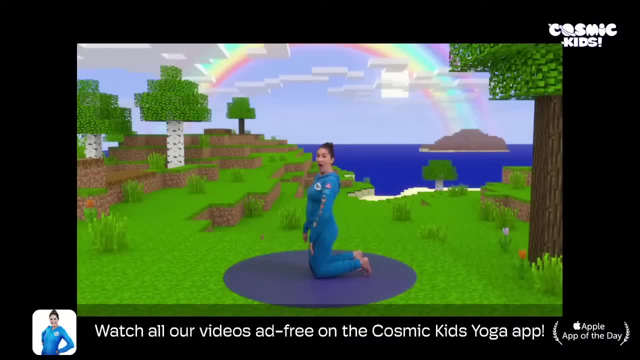 Along comes a horse Coming into horse, pose High up on your knees, Step one knee forward and lift your arms wide. Then fold forwards and lift your chest. as you go, Stampy saddles up. He lifts himself up, Turns himself round. 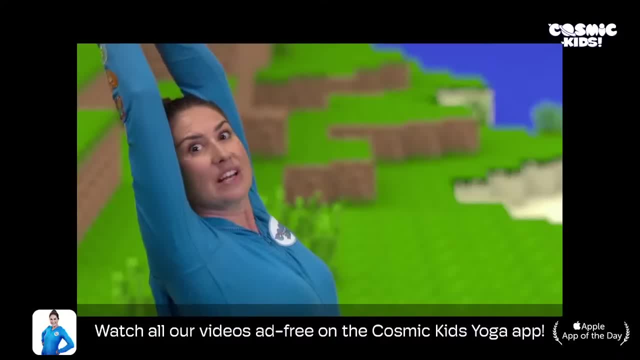 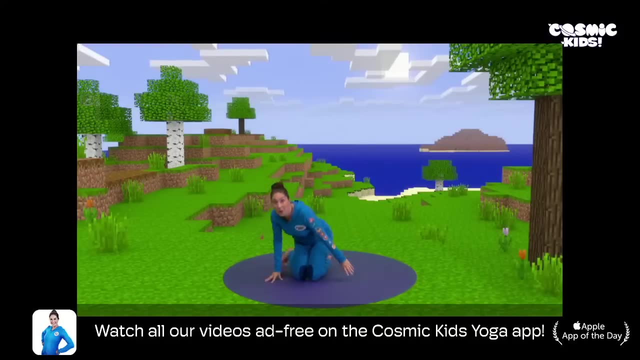 Drops down onto the other knee As he says: meow, stay And off he trots. Very good everyone. Now we better get in our boat so that we can get some fish. Sitting in your boat. pose Lifting up one leg. 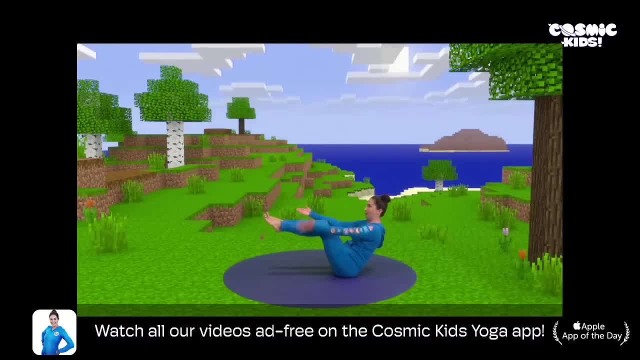 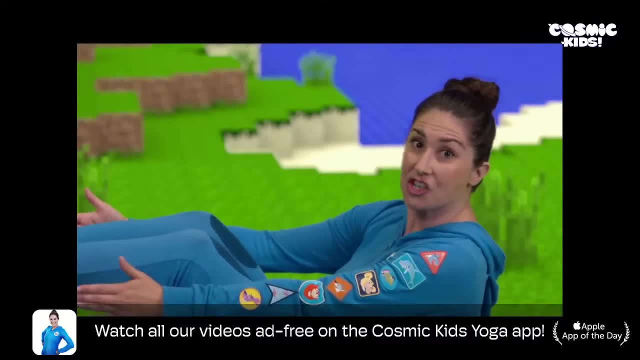 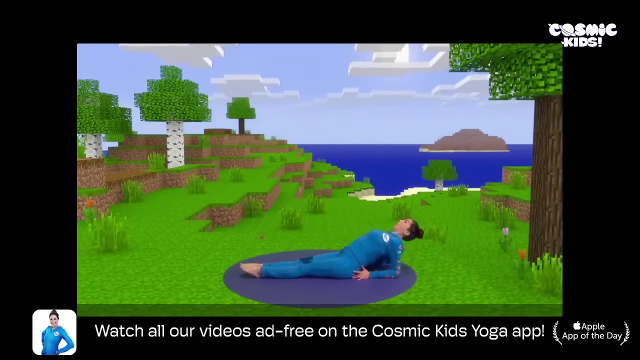 Lifting up two. Lifting up one hand, Lifting up no hands And give me a wave: Yay. Using the string from our spider, we catch a fish. Point your toes down and drop down onto your elbows. Now pop, pop, pop, pop, pop your chest to the sky. 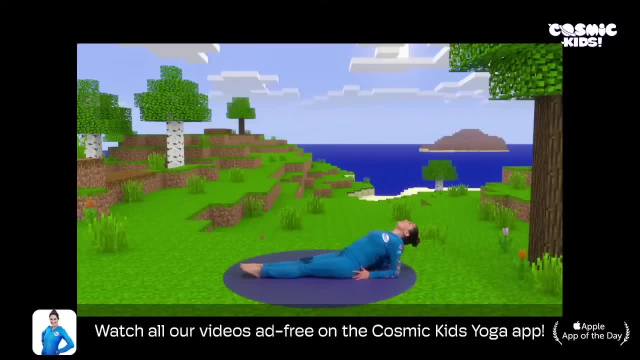 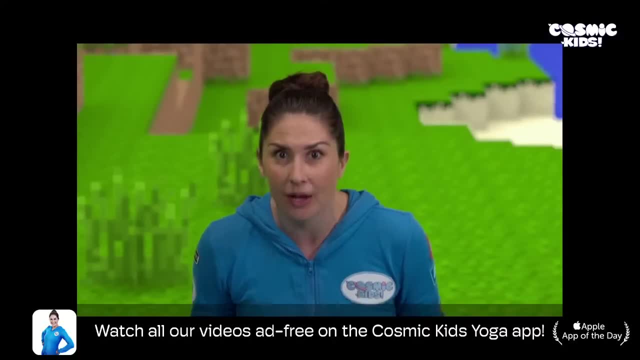 And look up to the ceiling or the sky above you Like a fish. Yay, We sit up tall. This is great news. We've got a fish for our supper. Now, back on the land, we find We're being followed by a pack of wolves. 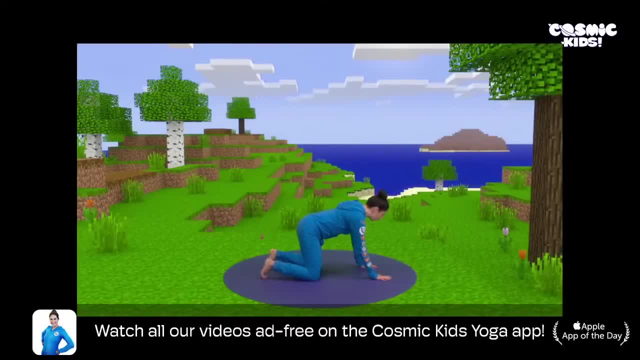 Let's come into dog pose On your hands and knees, spread your fingers wide, Tuck your toes and lift your bottom up to the sky. Coming into your dog pose Now, the wolves are our friends and they howl at the skeletons to scare them away. 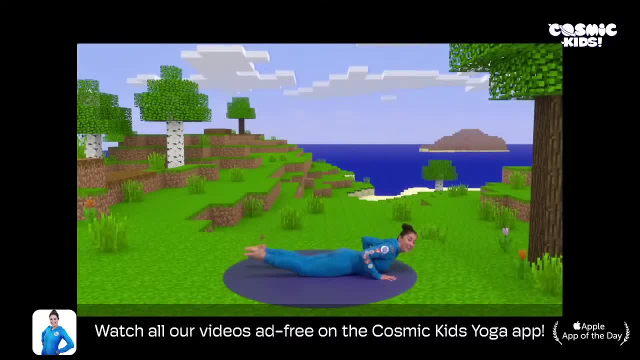 Coming all the way forward. come down onto your belly, Untuck your toes and then peel your shoulders up off the ground And see if you can make your legs really strong and lift them up too, And then look up to the sky and howl. 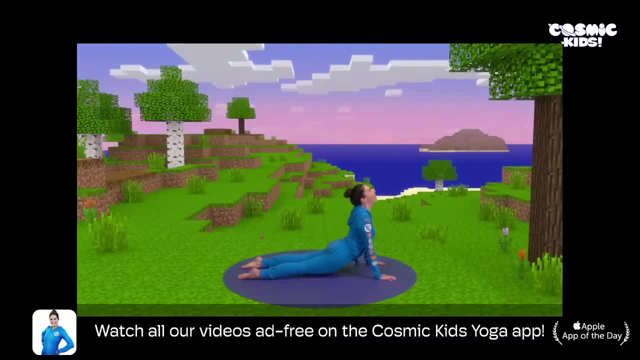 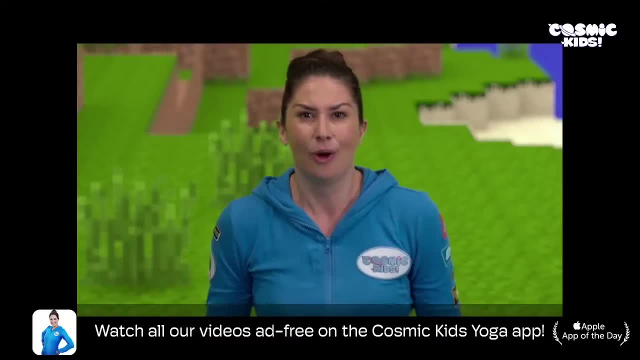 Awww, Thank you, wolves. We get back to our shelter where, after eating our fish supper, we're ready to have another sleep. We've survived our first two days and nights here in Minecraft and we feel very proud of ourselves, So we lie ourselves down. 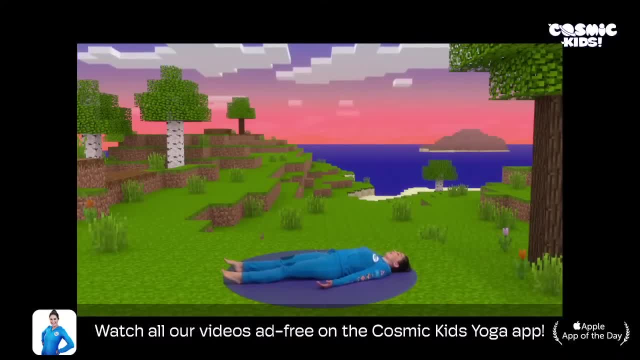 Our legs and arms long and we come to rest. What an adventure that was. It's been amazing here in Minecraft World. It makes us understand how things are made When you look around you at all the natural things in the world And how you put them together to make the tools and the things that you need. 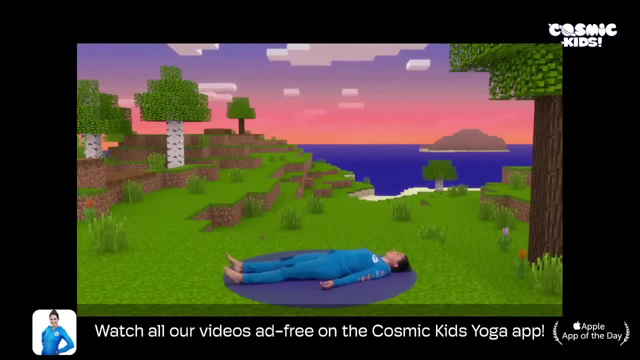 It makes us realise that we don't need very much A house, warmth, friendship, food and water, And it makes us feel really grateful for all of the other stuff that we have in real life. Maybe when we look around now we can understand how those things were made. 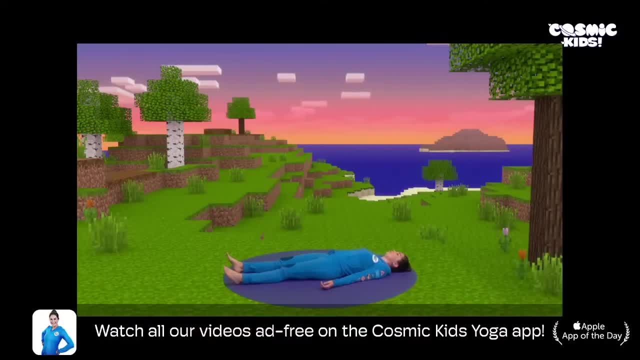 The work that went into them And we can feel very grateful, Very grateful, for all that we have. And now it's time to wake up. So we wiggle our fingers and our toes, We bring our knees into our chest And we roll over onto our side, opening our eyes. 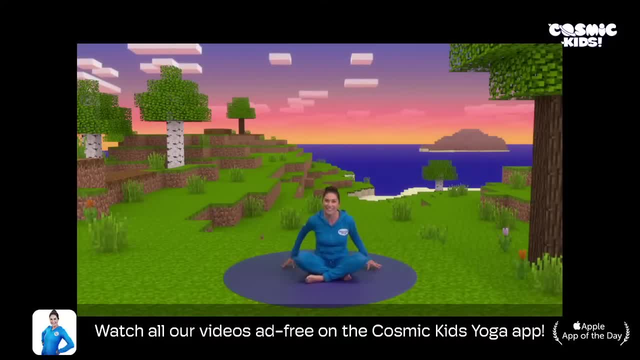 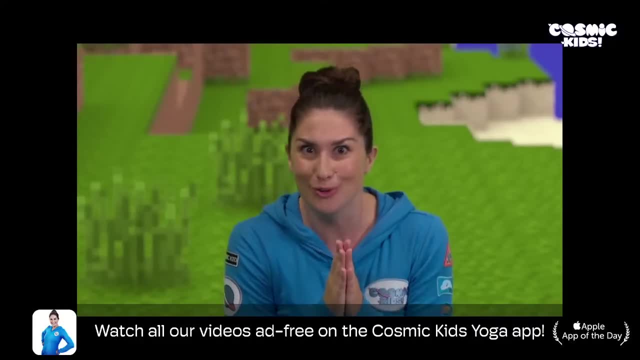 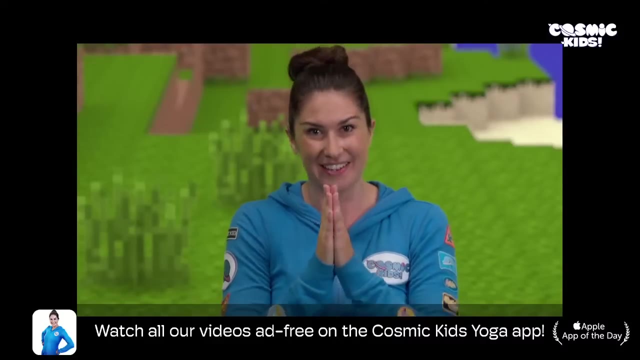 Coming up to sit with our legs crossed And our hands together at our hearts, just like we started And we finish with our secret yoga code word, which is Namaste. Ready After three. One, two, three, Namaste. 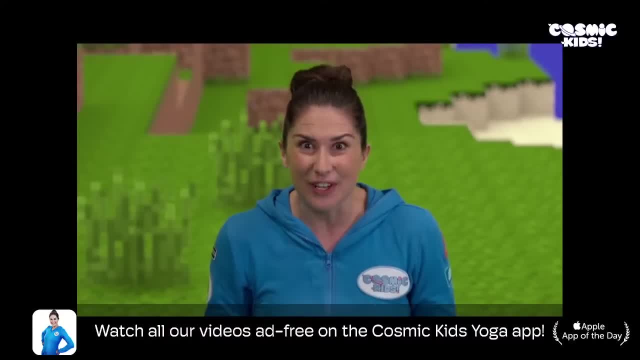 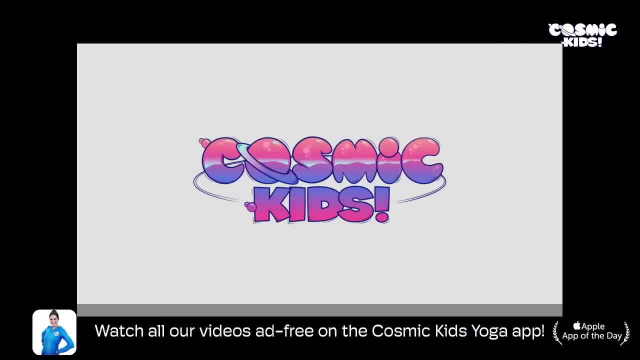 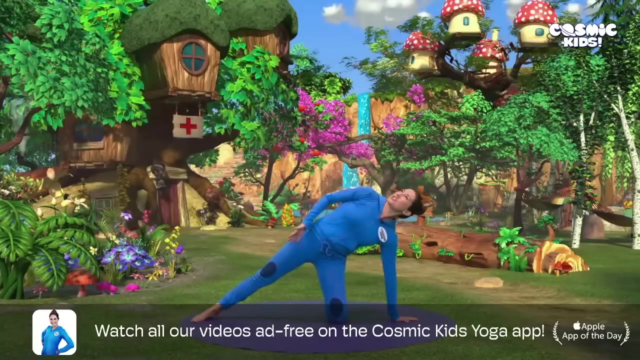 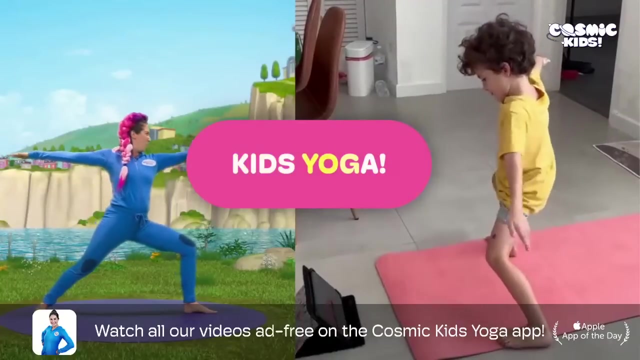 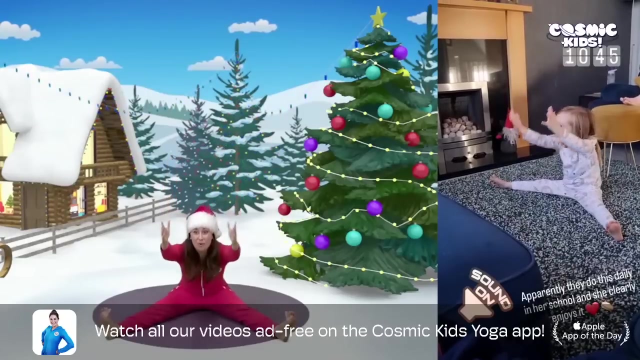 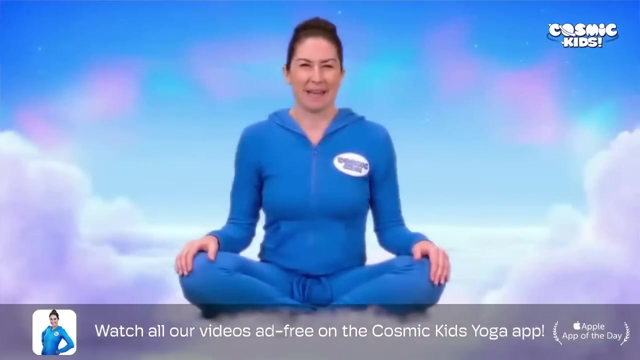 Well done everyone. That was awesome. Thanks for coming to Minecraft World with me And helping me survive my first couple of nights. You were amazing. I hope you come back soon for another Cosmic Kids adventure. Bye, bye, Bye, bye. And the best way to make the I can't thought go away is to think: oh yes, I can. 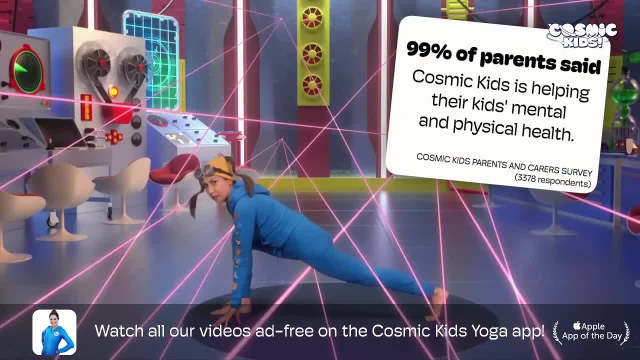 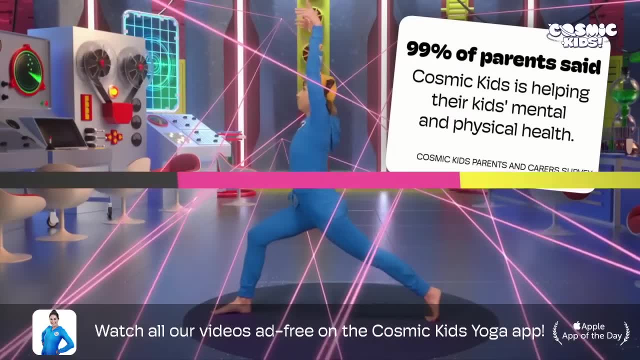 We step forward between our hands- Oh, thank goodness we do yoga Now, making our legs very strong. we lift all the way up, trying not to wobble, lifting our arms up to the sky, And then we fold all the way forwards. 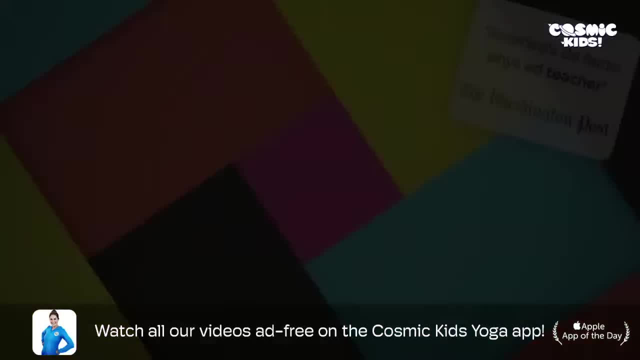 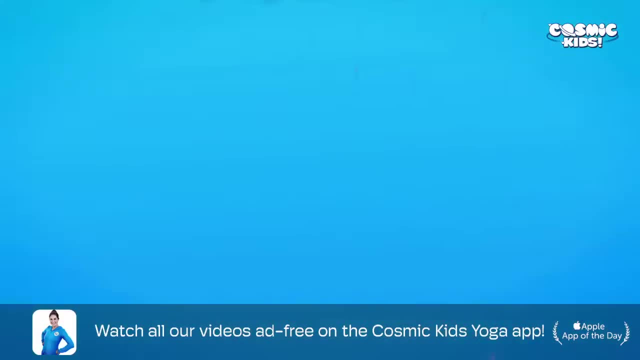 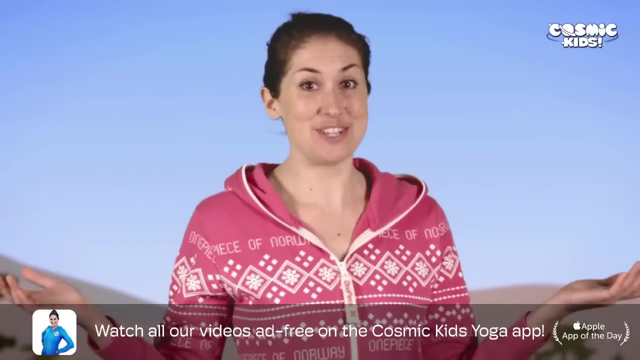 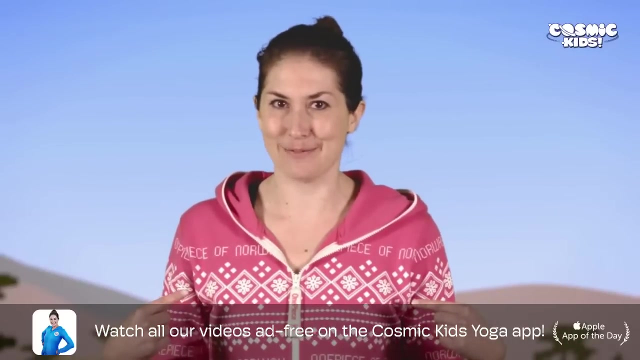 Hands come either side of our foot. Hello everyone, welcome to Cosmic Kids. I'm Jamie and this is your place for yoga stories and fun. It's easy: just copy the moves I do and enjoy the adventure. Now, we always start in the same way, and that's by sitting on our bottoms. 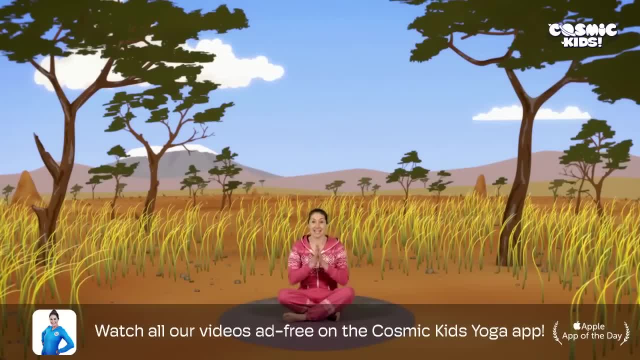 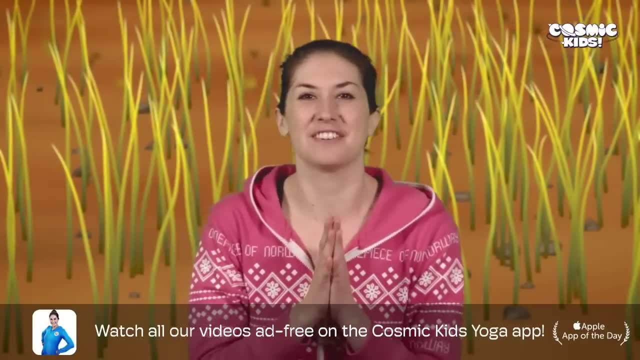 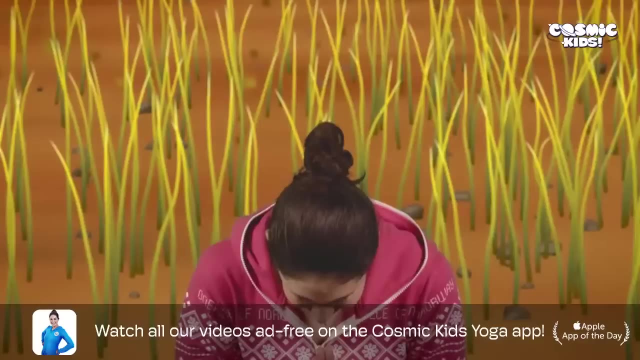 And crossing our legs and bringing our hands together at our hearts to say our secret yoga codeword, which is namaste Ready After three, One, two, three, Namaste There, Now we're ready to begin. Shall we find out who our story is about today? 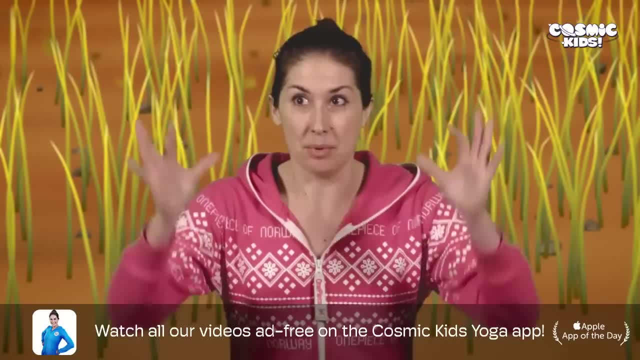 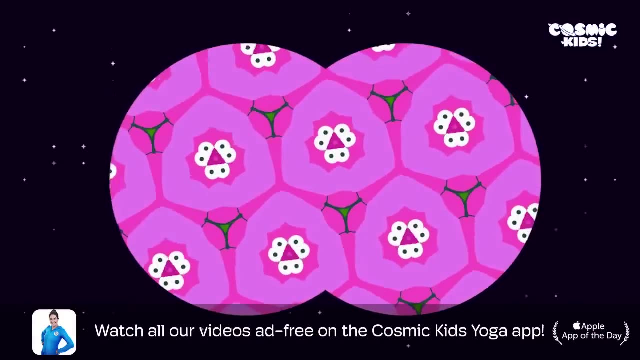 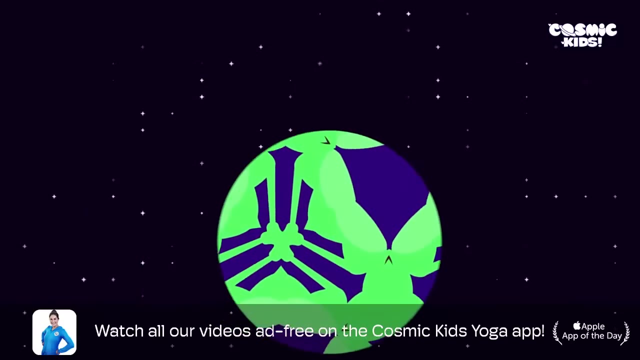 Yes, let's look through the cosmonoculars, bringing your thumbs and fingers together. Have a look through. Wow, It's beautiful. What amazing colours. Can you see the picture? What is it? It's a baby lioness. 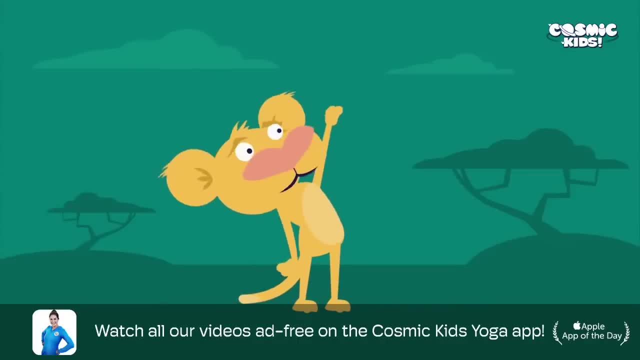 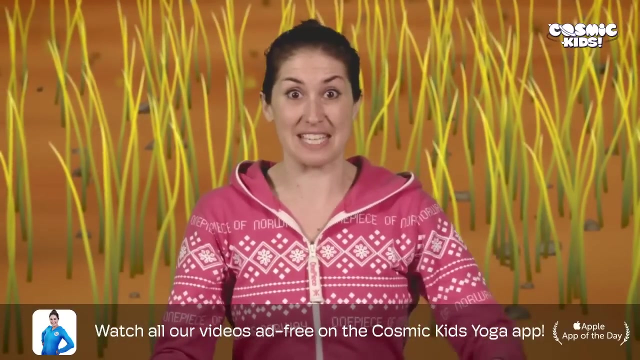 It's Lulu, the baby lioness cub. Yay, What's Lulu doing? Oh, she's doing yoga. She's doing flamingo pose. She's doing flamingo pose. This is so exciting. It means we're off to Tanzania, in Africa. 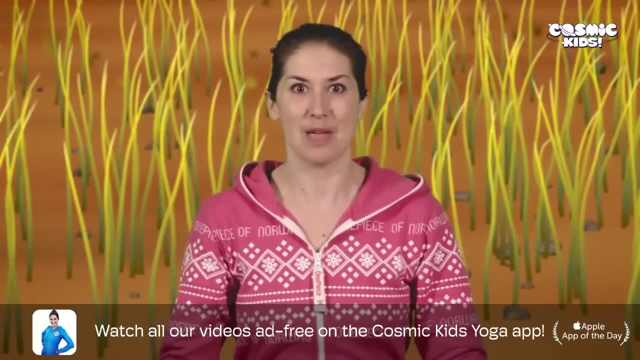 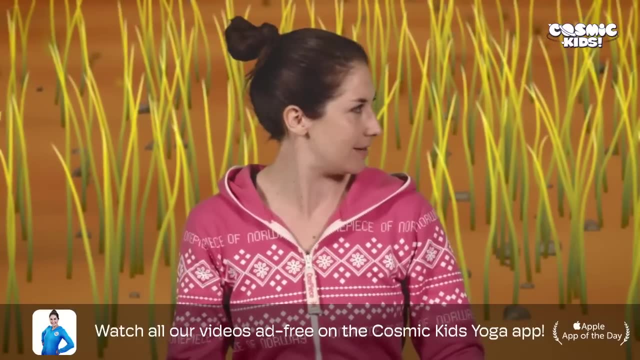 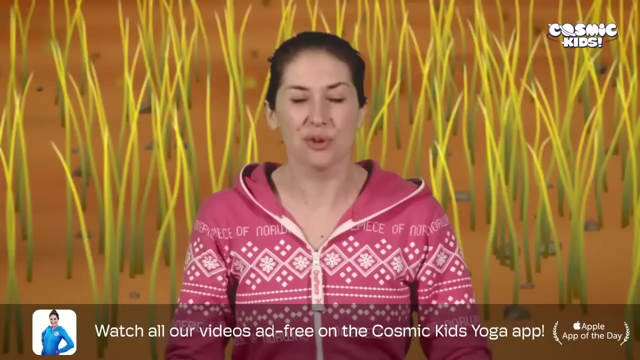 Let's get ourselves ready for our long aeroplane journey. First our necks. We look over one side and then the other. Over one side and then the other. We nod all the way forwards and all the way up, All the way forwards and all the way up. 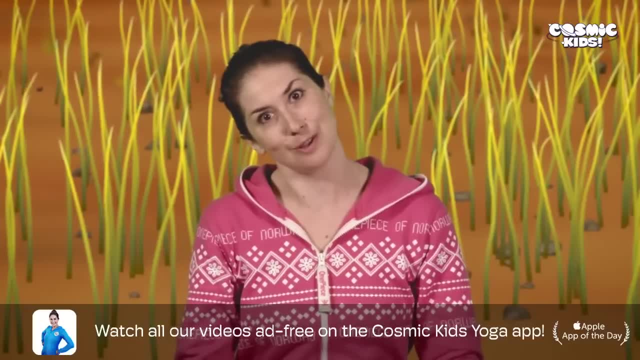 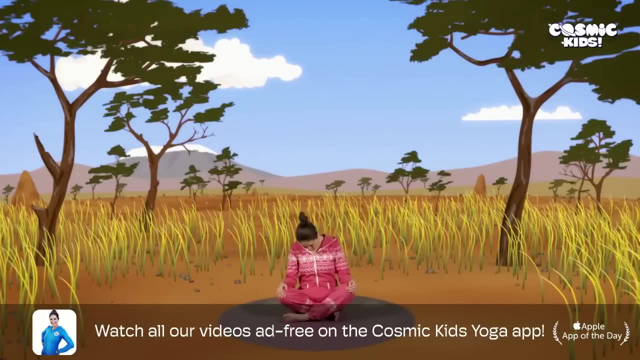 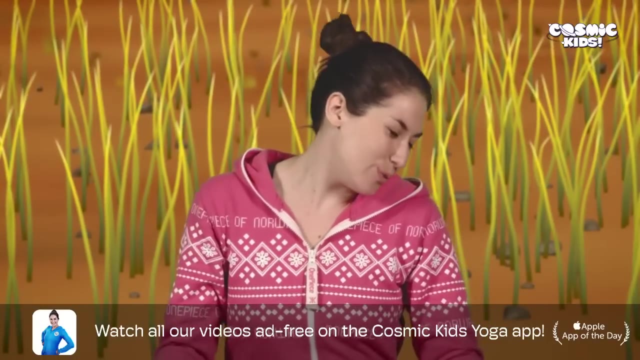 We tick our head one side and turn, Tock it to the other, Tick it and tock it, and tick it, and tock it And go all the way around like the hands of a clock, And the other way too. Oh, that feels lovely in our necks. 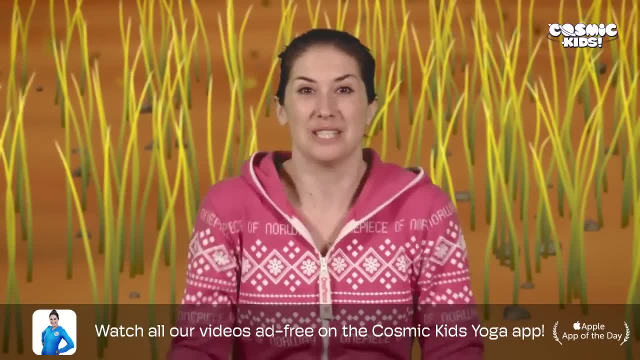 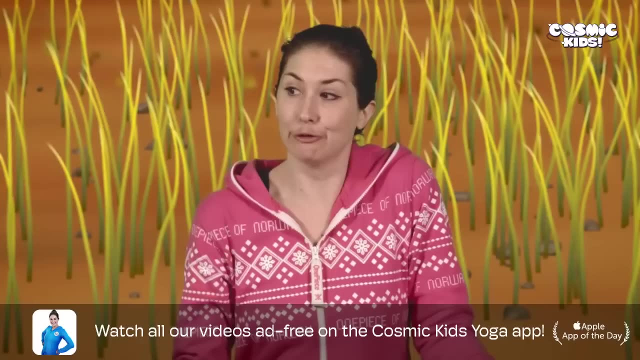 Now it's time for our shoulders. We roll our shoulders round and round. We lift them up and put them down. We lift up one, we lift up two, We put down one, we put down two. Going up up down. down. 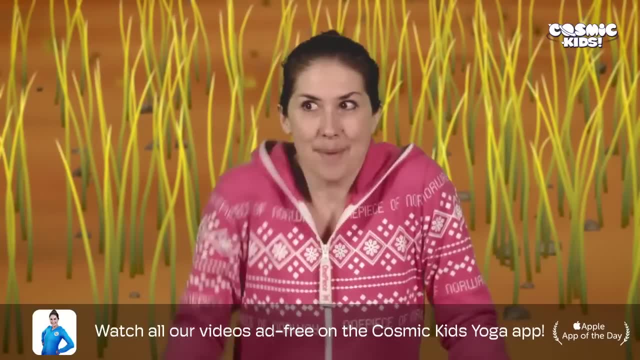 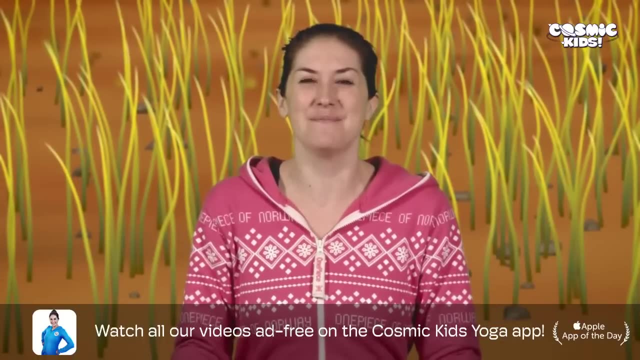 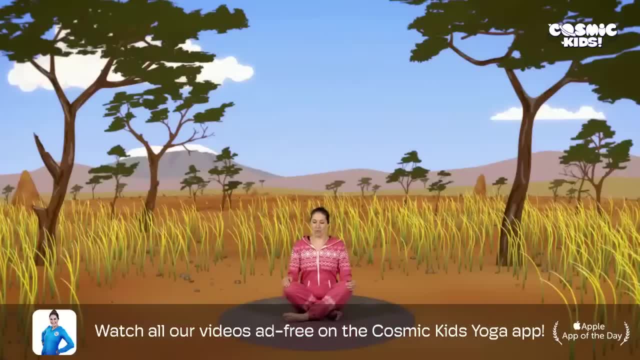 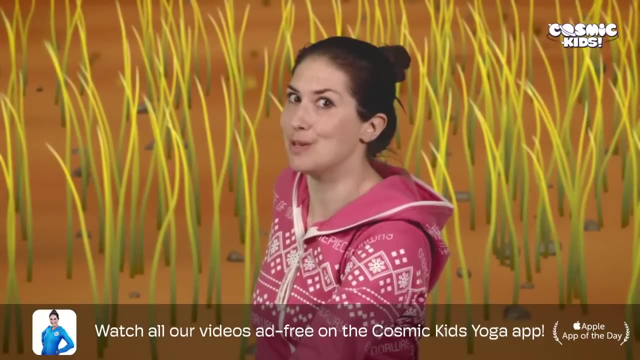 Now I think we need to pack a backpack. So we put our legs out long And we take our fingers to our toes, bending our knees a little bit to open it up. We take our arms out wide, We twist one way to get our tent because we're going to be camping. 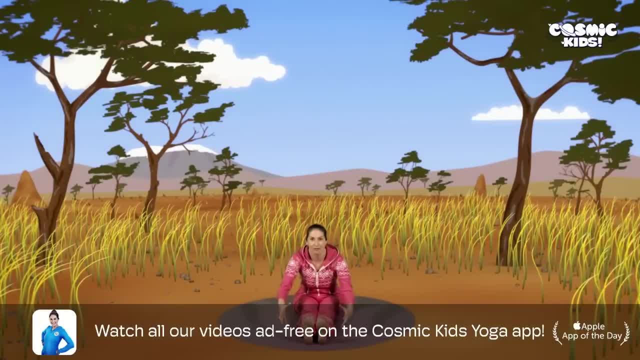 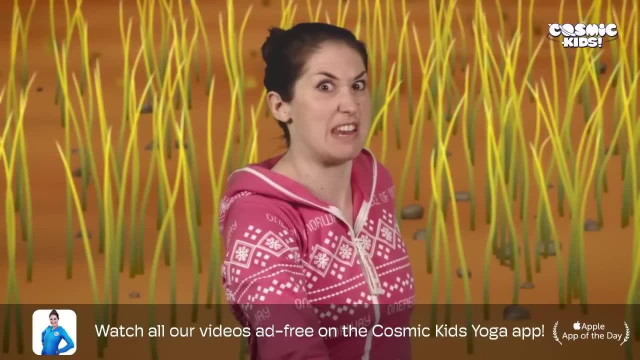 Here it goes, Plonk, Lovely. We take our arms out wide again and we twist the other way And we get our sun cream, because it's really really hot there. We take it and we check the lid's on- Lovely. 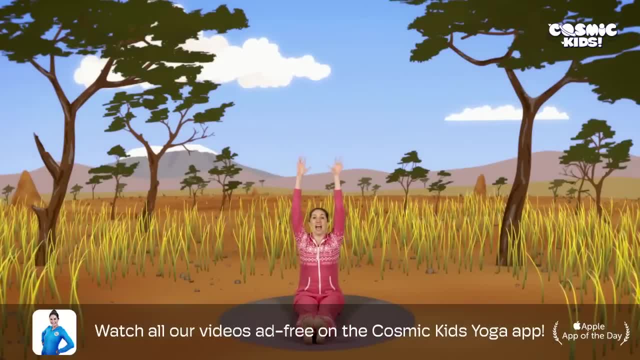 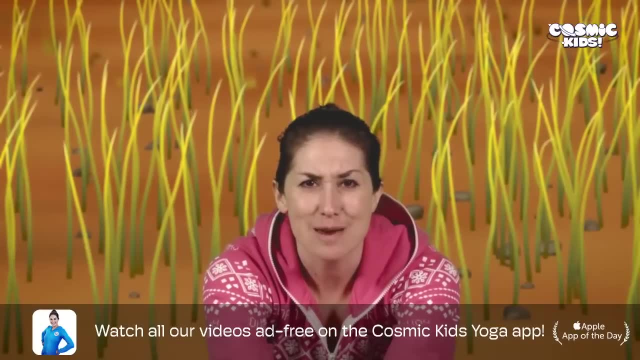 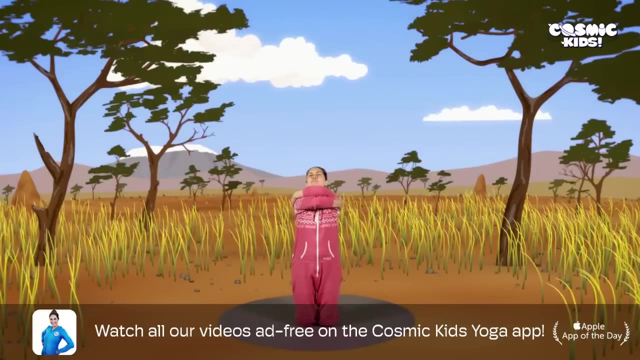 Put it in, Lift your arms up high and close your backpack. There Now we give everyone at home a great big hug, goodbye. Coming up onto our knees, we stretch out wide and we give them all a cuddle. Bye, everybody. 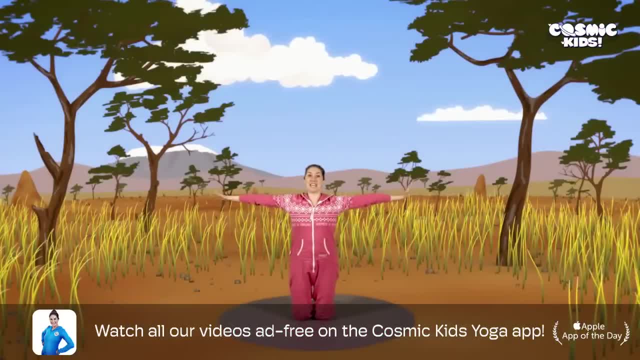 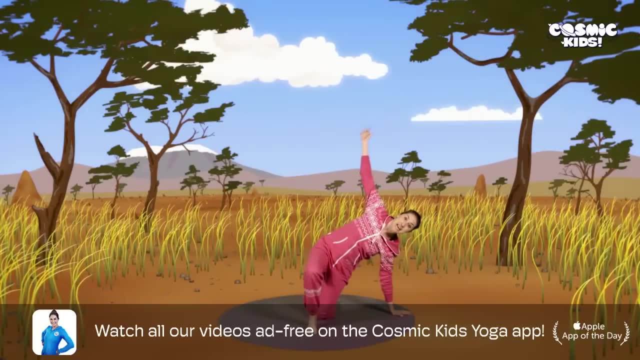 Time to catch a plane. We take our arms wide again and drop down onto one hand Wave at the sky. We bring one foot in front of our knee and stretch our back leg out. behind us Going meow, And the other side too. 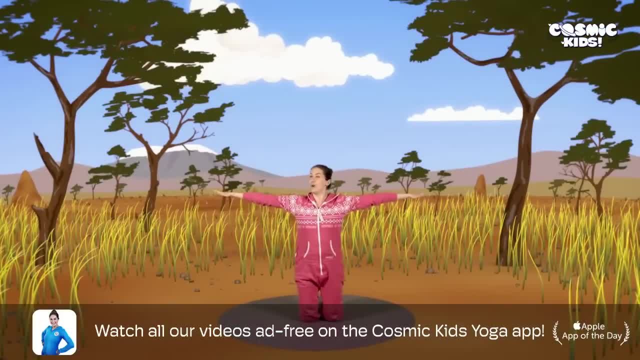 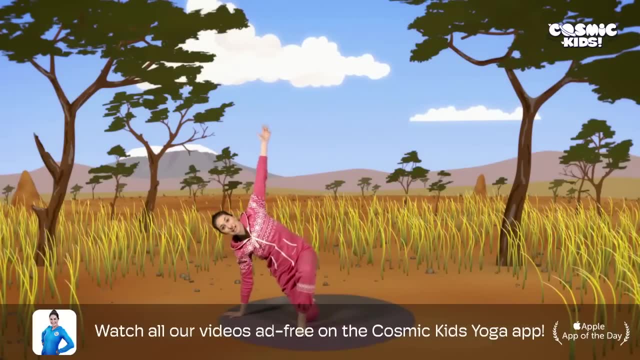 Coming back to the middle, with your knees and your arms all stretched out, We come down onto the other side, wave at the sky and bring our other foot in front of our knee and stretch our back leg out behind us, Ready Meow. 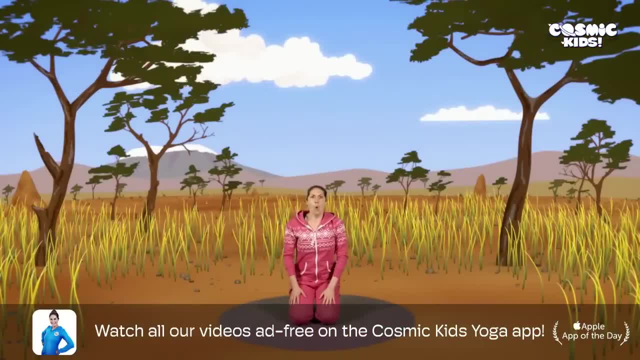 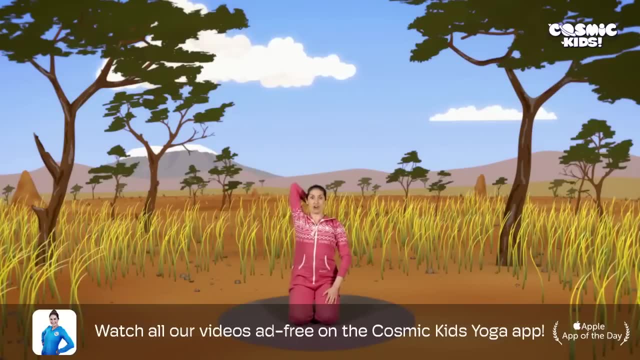 And we've arrived in Tanzania. Wow, It is hot here. So we put on our sun cream. Reach into your backpack. Ooh, ooh, ooh, Got it And stand up. Here we go, Blob, blob, blob. 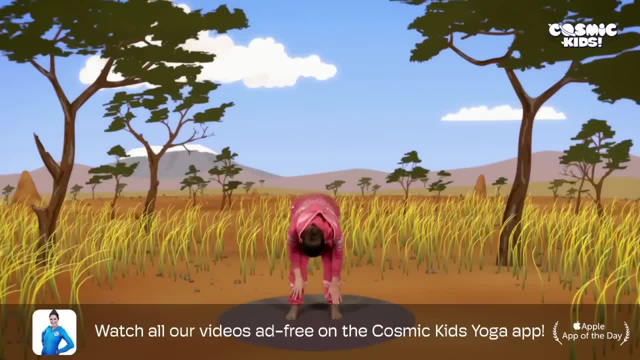 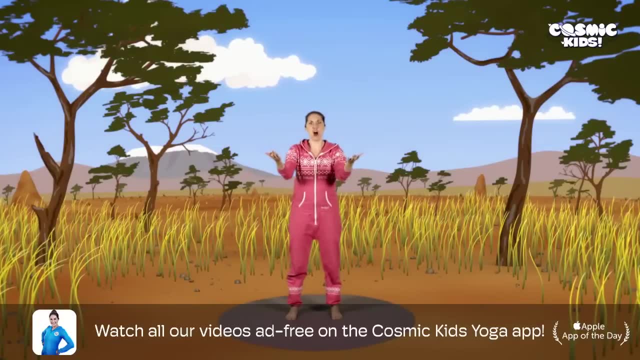 Blob, blob, blob, Rub it on your legs, All the way down on our legs. And now more Blob, blob, blob, Blob, blob, blob, Rub it on your arms. Ooh, yes, That's it. 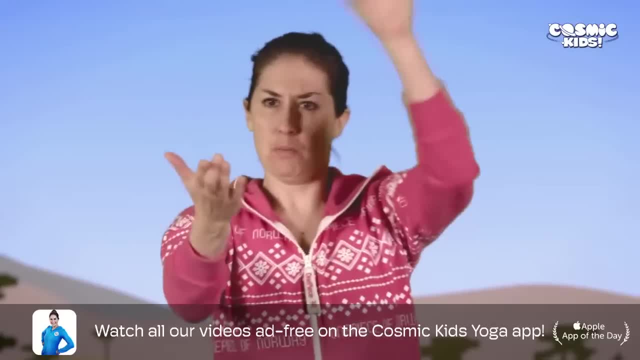 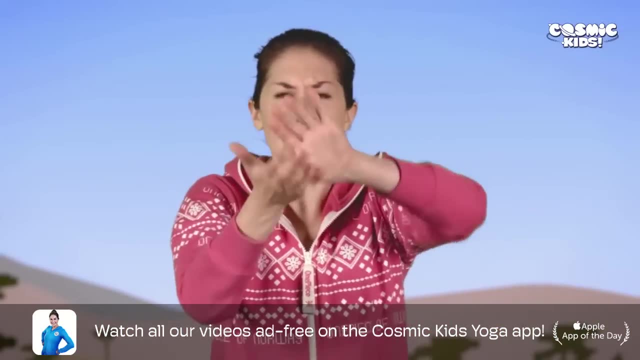 All over our arms And our bodies: Ready Blob, blob, blob, Blob, blob, blob. All over our bodies, Yes, And our faces: Ready Blob, blob, blob, Blob, blob, blob- All over our faces. 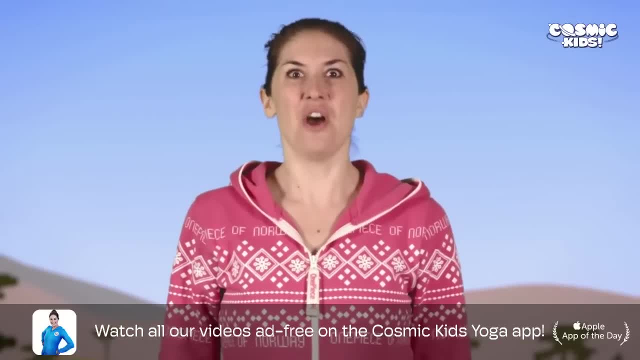 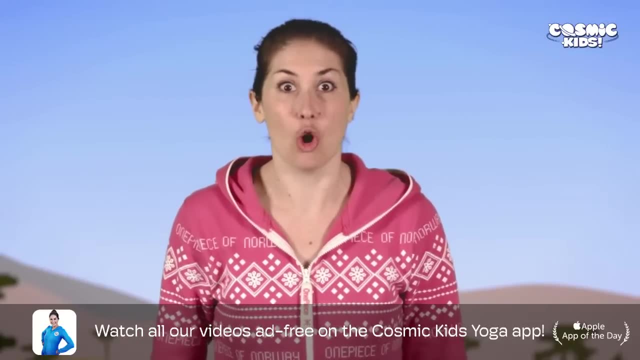 That's it. Now. we've got all our sun cream on. We are ready. But there's a clever thing we can do to cool ourselves down. Can you make your tongue into a straw by curling up the sides like this? Now suck in. 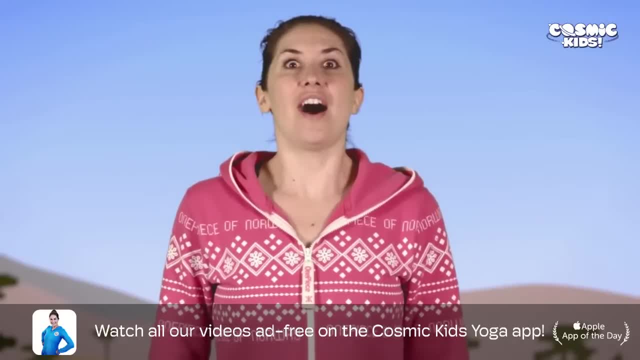 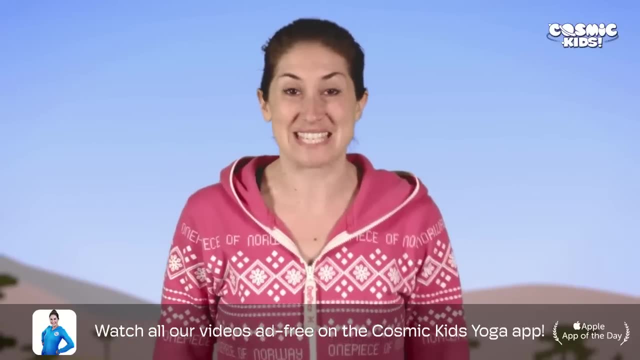 And it makes our mouth feel all cold. If we can't do that curly thing with our tongue, we can do a big smile. We can do a big smile like this And we can suck in the air through our teeth Ready. Ah, that's better. 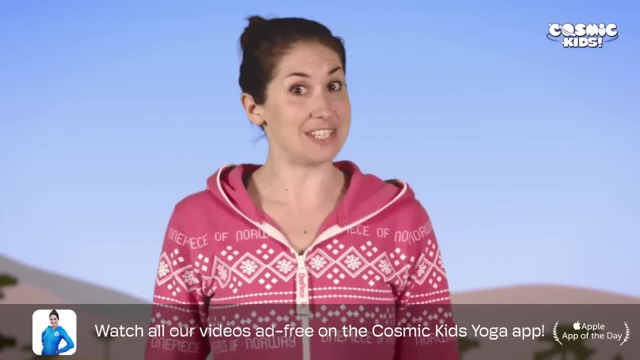 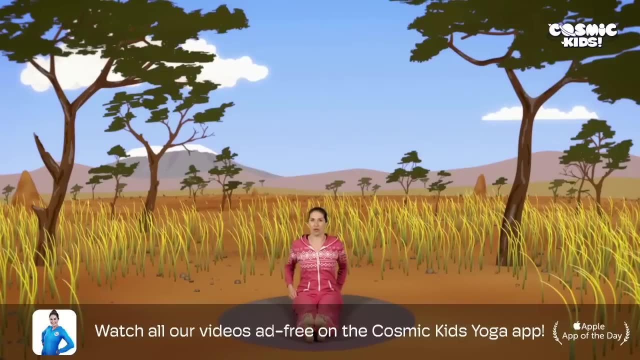 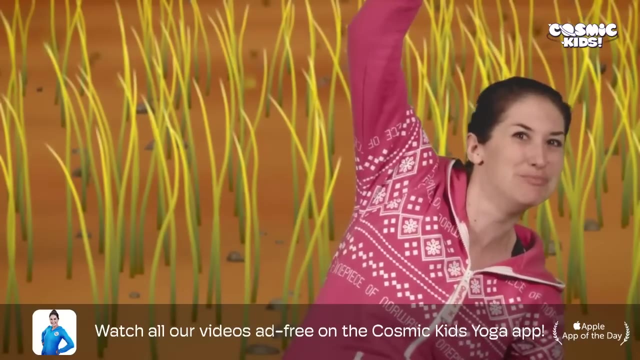 That helps us feel all lovely and cool. We get into our jeep Sitting down, take your legs out long and pop your seat belt on, Start the engine. We're going over to one side. We're going over to the other side. 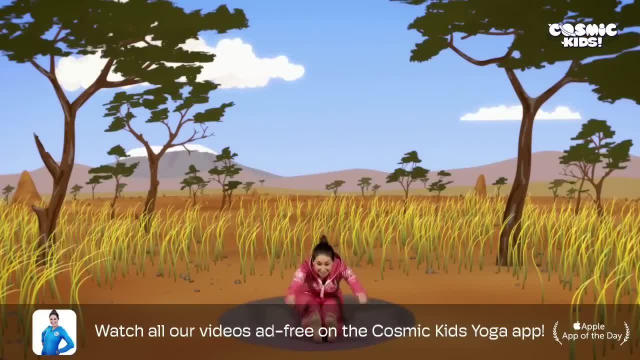 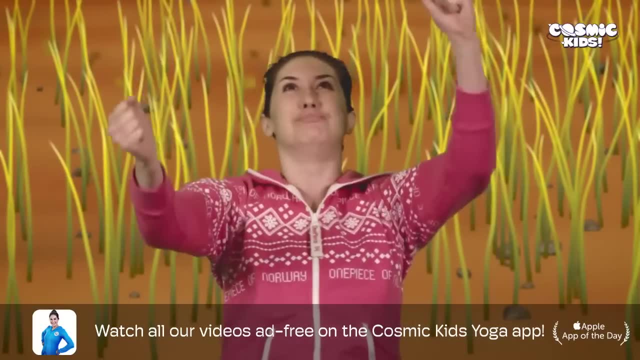 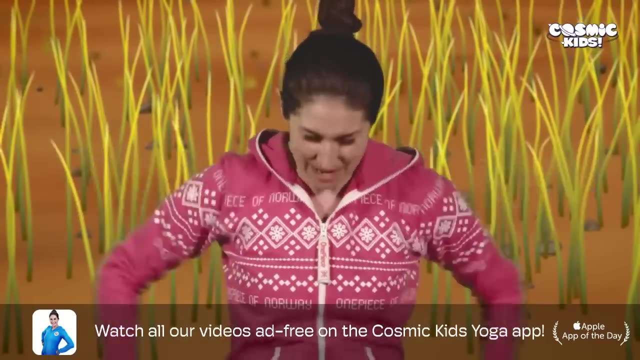 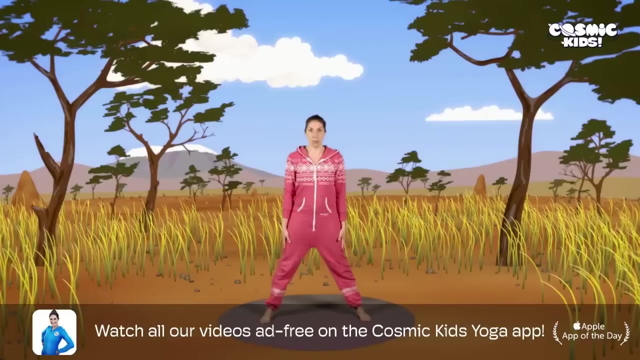 We're going down a hill. We're going up a hill. We've arrived at our campsite. Yay, Let's put up our tent. We stand up and we put up one pole, Two poles, Three poles, Four poles. 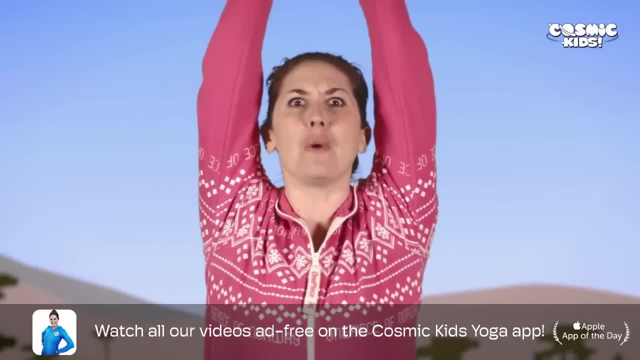 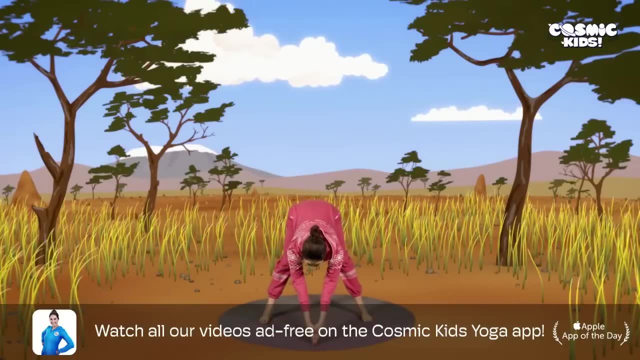 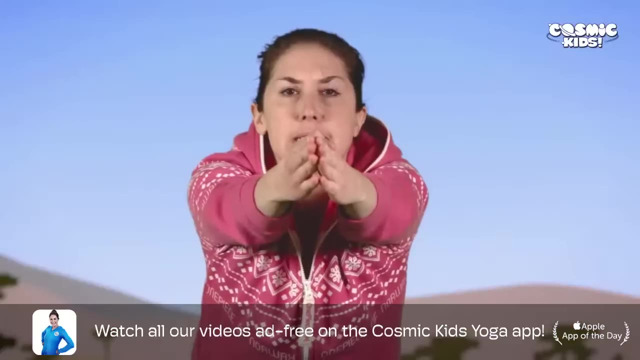 Yay, Now we check, the zip works all the way down the front. Ready, Zzzzzzzzp. Yes, Now does it go up again? Let's try Zzzzzzp. Uh-oh, It's got stuck. 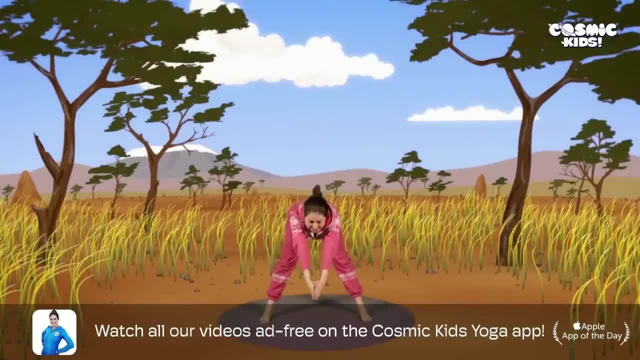 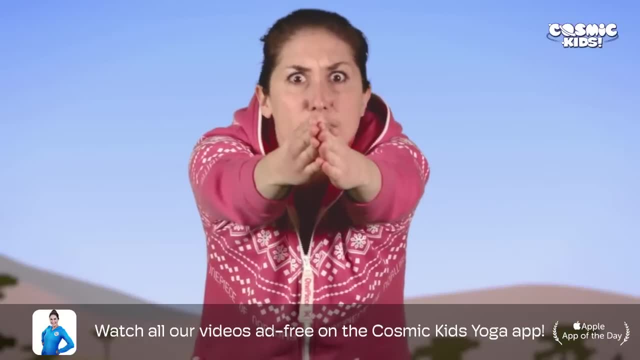 Let's go back down again, Zzzzzzp. Let's try that again, shall we? Here we go, Zzzzzzp. Oh, I don't believe it, It's got stuck again. Back down, we go, Zzzzzzp. 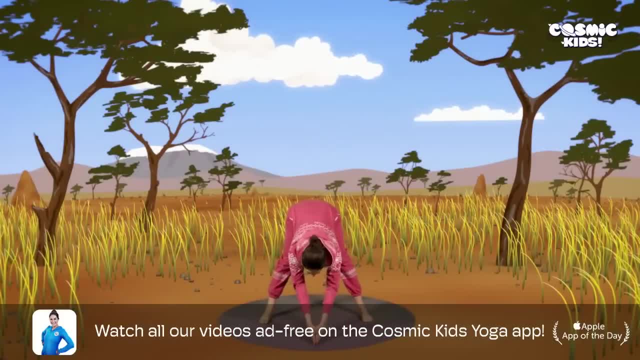 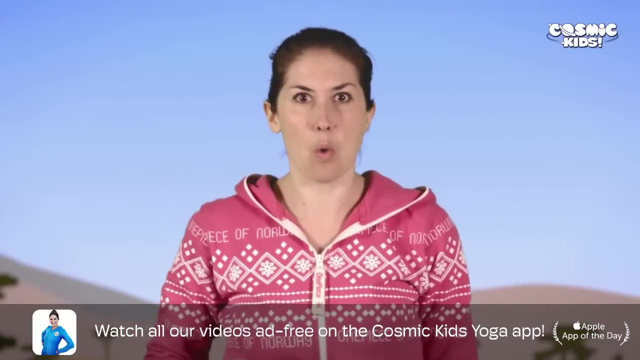 Hopefully, third time lucky, Let's try again. Zzzzzzp, Phew-ee, Thank goodness for that. Oh, but we're a bit smelly. after all of that Poo-ee, We need to give ourselves a little bit of a wash in the river. 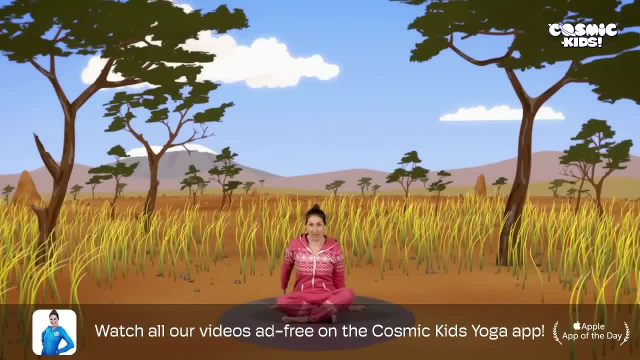 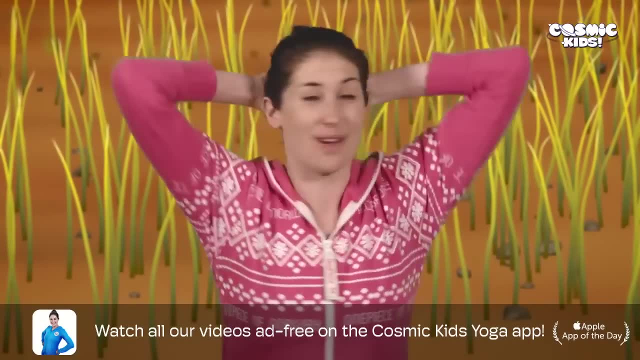 So we put our clothes in the river and we wash them like they're in a washing machine, Criss-cross your legs and criss-cross your fingers and put them behind your head. Then we go from side to side saying wishy-washy, wishy-washy, wishy-washy woo. 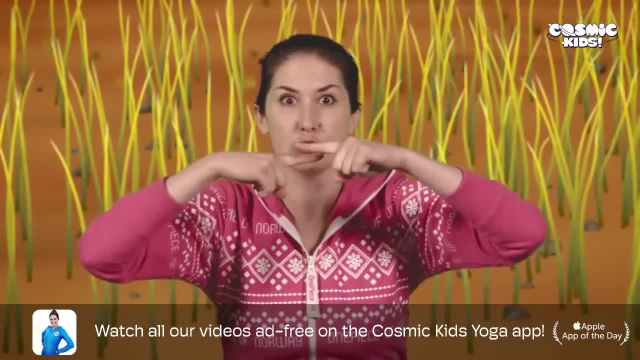 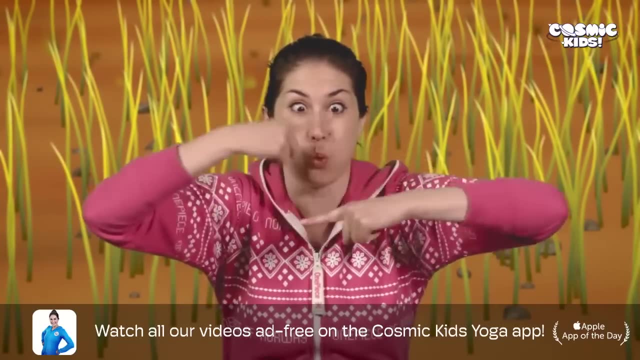 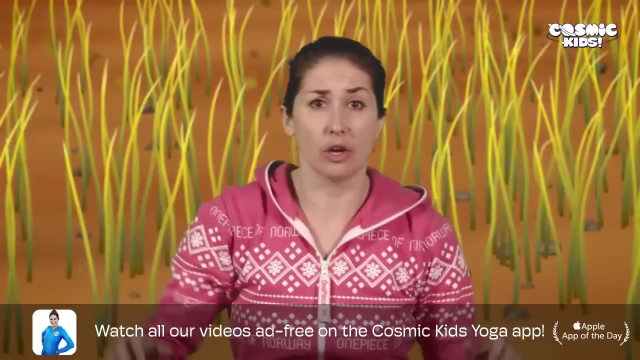 Then we dry our clothes by the campfire with tumble dryer fingers, blowing them as they go round, Ready, Yay, Oh, We're so tired, though. We want to meet Lulu first thing in the morning, So we decide to get some sleep. 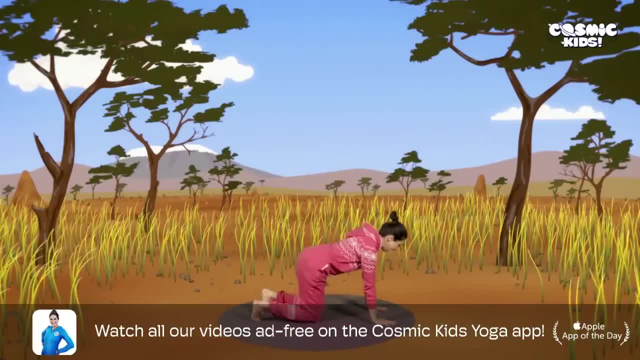 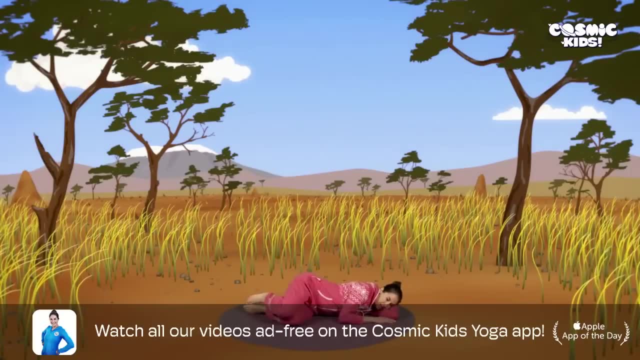 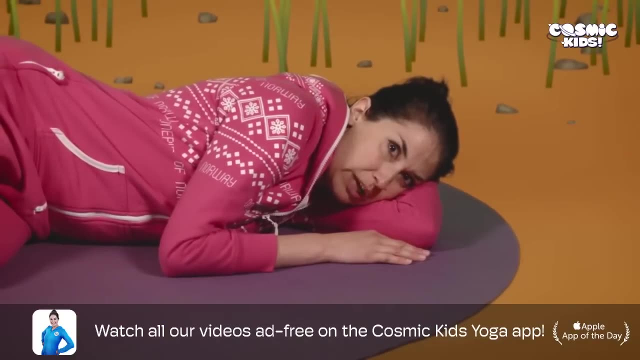 We crawl into our tents and we get all snuggled up in our sleeping bags, coming all the way down curling up. Ah, sleepy, sleepy, sleepy time. In the morning we're woken up by the sounds of the birds tweeting. 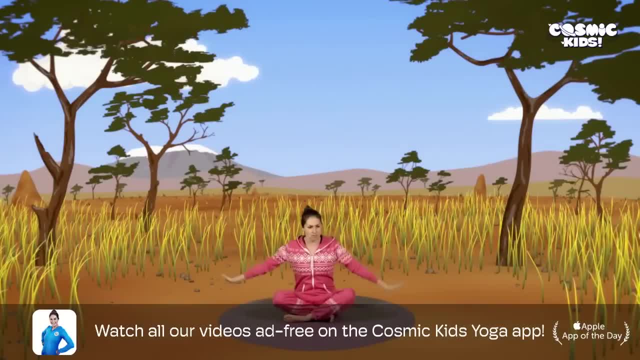 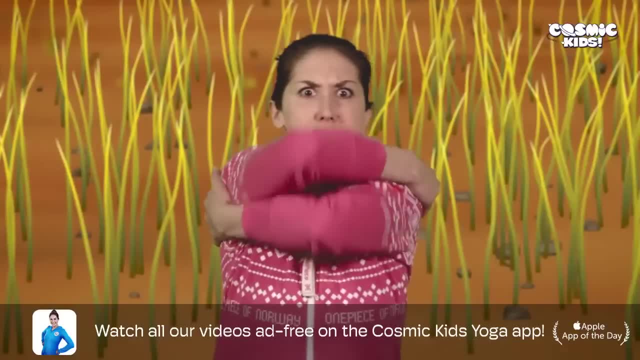 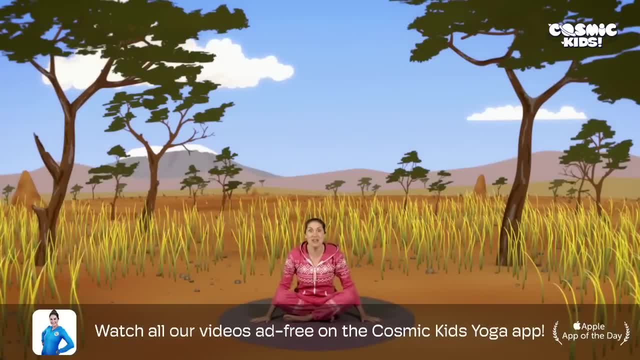 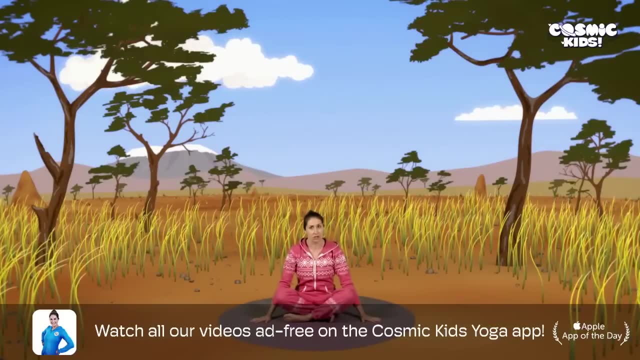 We come out of our tent to find Lulu, the baby lioness. Here she is, but she hasn't learnt how to roar yet, so she just sticks out her tongue, Coming up onto your knees. after three, we're going to stick out our tongue and do our big lion face. 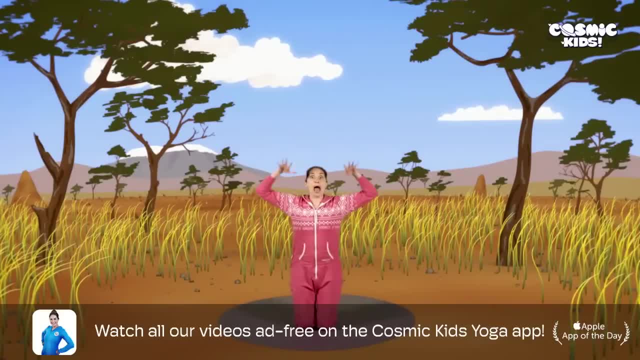 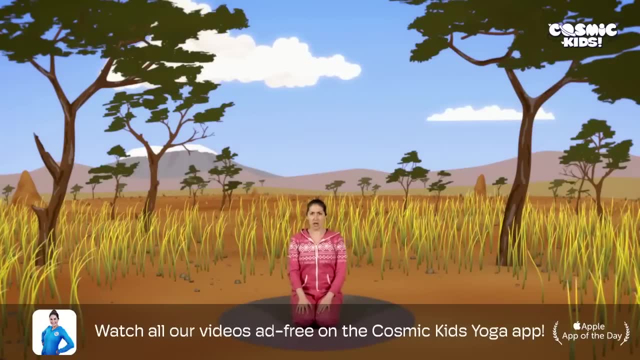 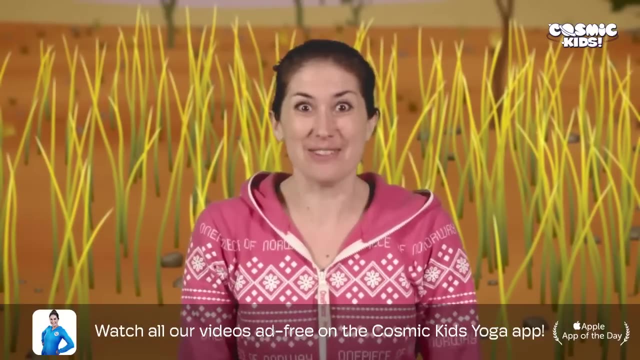 Ready. One, two, three. Everyone keeps making fun of me because I haven't learnt how to roar yet. I got really, really angry And then I came for a little walk and I found you. Maybe you can help me learn how to roar. 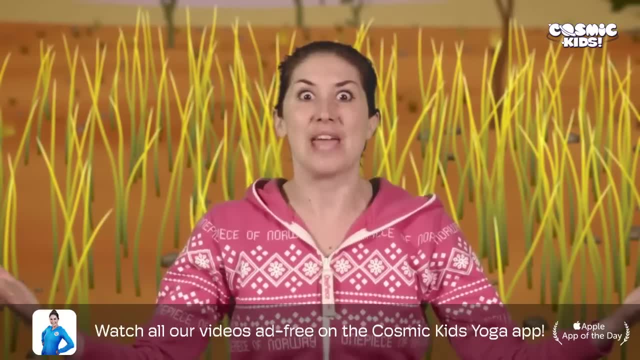 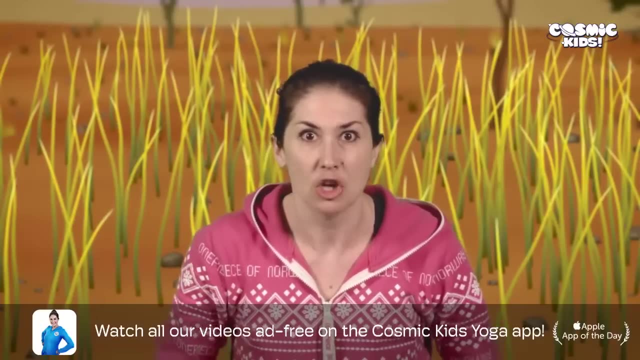 We can help, Lulu, can't we everyone? Yes, We have an idea, Lulu. we're going to climb up this tree. You're going to stay at the bottom. You get to the top. You roar as loudly as you can so we can hear you. 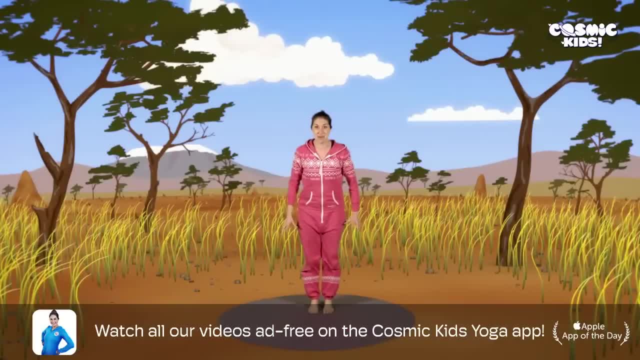 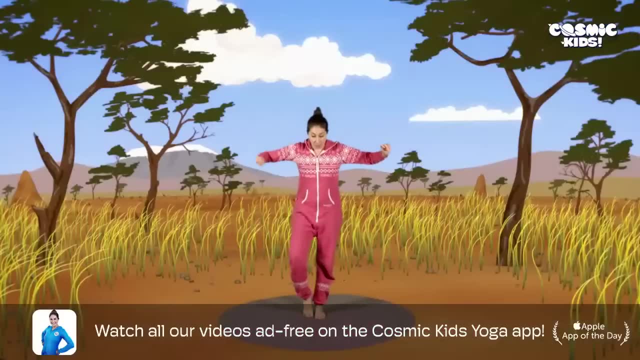 Ready, We climb up the tree, Standing up, everyone Here. we go Up, we go up, we go up, we up, we up, we go. We get to the top of the tree and we put one foot on top of the other. 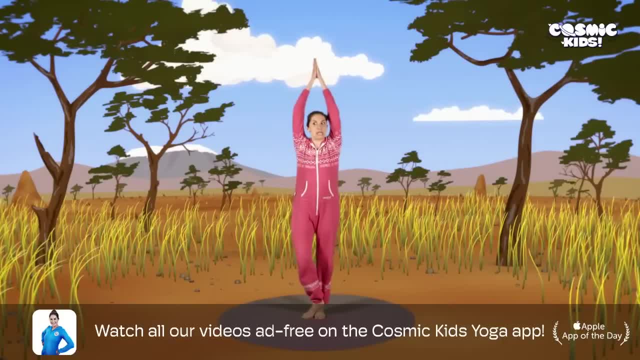 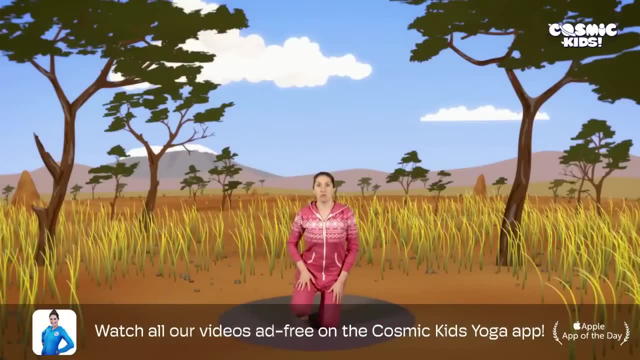 Our hands together at our hearts and we grow up tall and we listen. for Lulu, Hmm, Down at the bottom Lulu gives her roar a try. Ready One, Two, Three, Oh dear Poor Lulu, Back up the tree everyone. 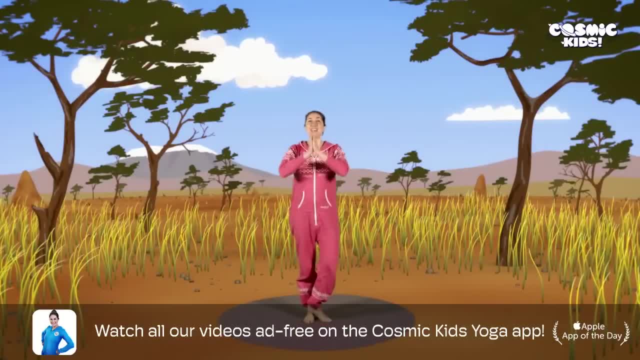 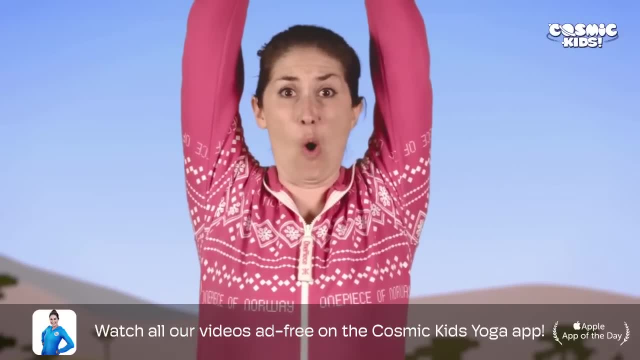 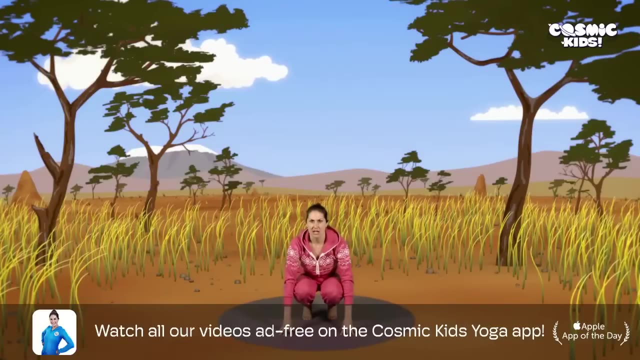 Try with the other foot now on top, Your hands together, growing up tall. We listen carefully, but it's no good. We can't hear her roar. We jump down from the tree, One, Two, Three Doing Phew. Lulu's getting really angry. 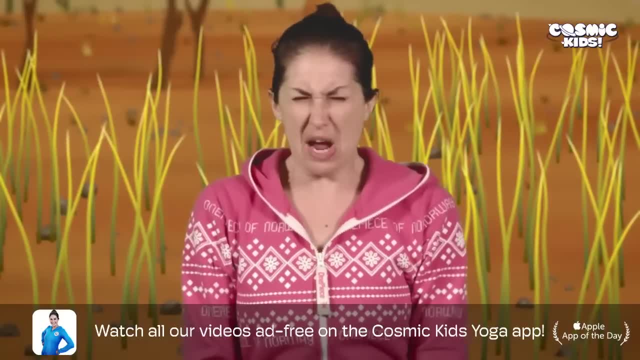 I'm never going to be able to roar. I am so, so bad at roaring. I'm going alright. Yes, Yeah, VWho doesn't know. ya, Lulu is getting really angry. I'm never going to be able to roar. 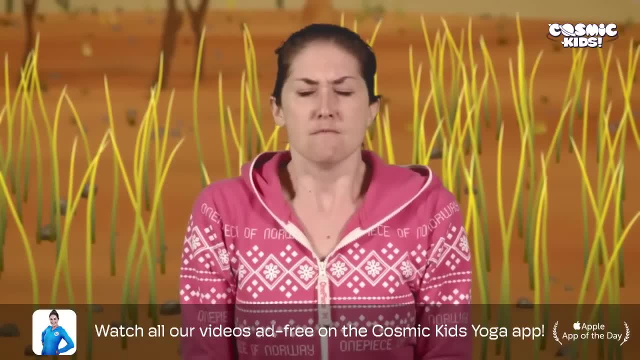 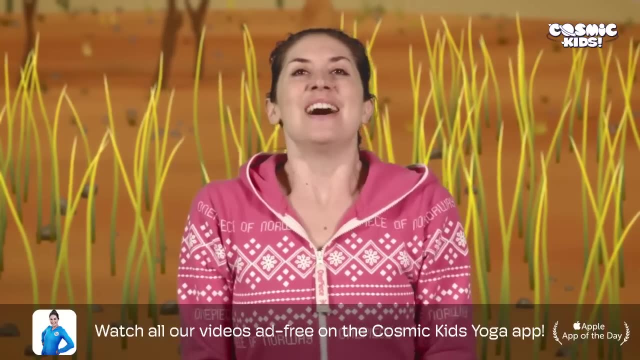 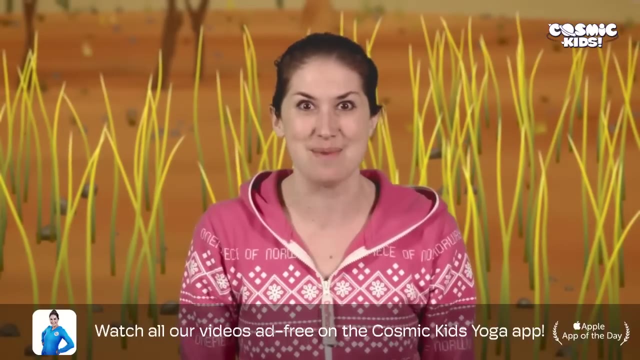 I'm so, so bad at roaring. It's horrible. But, Lulu, getting angry at yourself won't help. Let's take some deep breaths to feel better and calmer. That's better. Now you can think clearly again. Let's go see Ernie, the baby elephant at the watering hole. 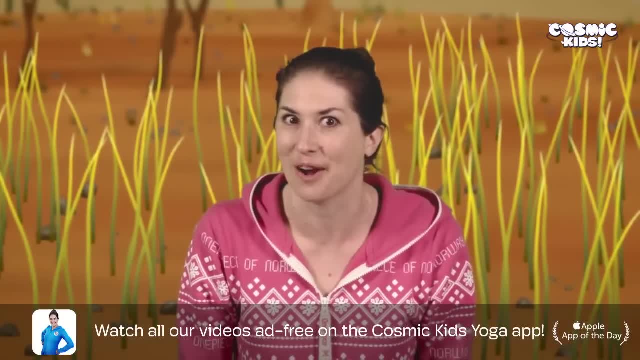 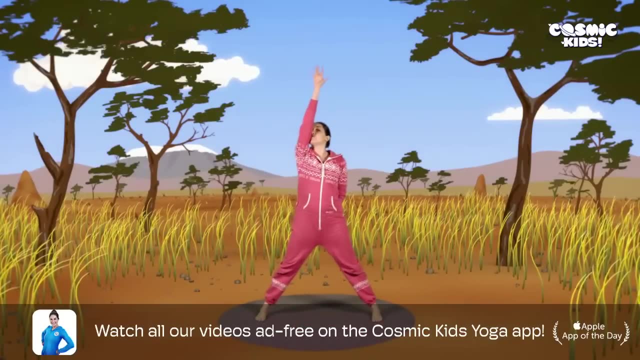 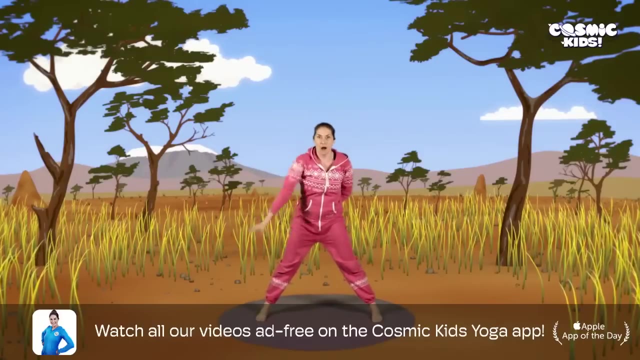 He can really make a big trumpet sound out of his trunk. Maybe he'll help. We stand up and we take our trumpety trunk out and, like Ernie, we do a big trumpety trump. Ready A-lulu. Lulu would love to be able to make a sound as big as Ernie's. 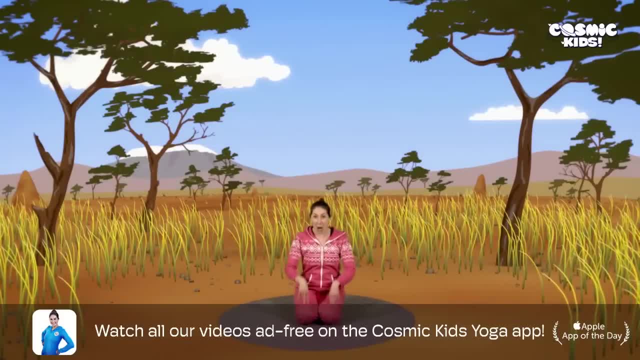 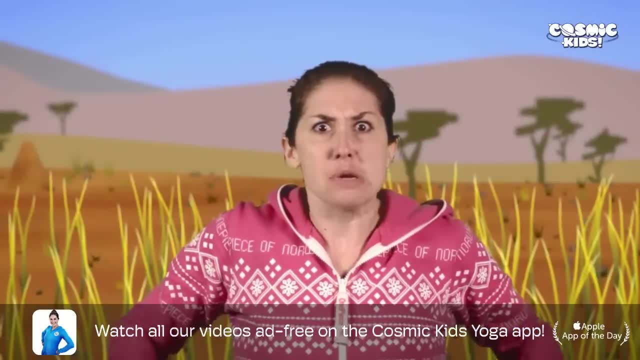 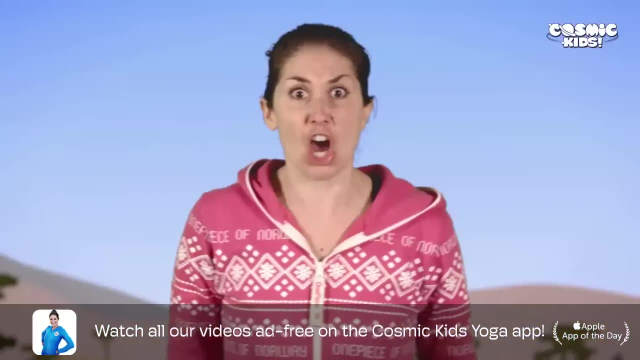 so she tries Coming down to your knees again, ready. One, two, three, But it's no good. Lulu gets so angry that Ernie can make a bigger sound than her that she ties his trunk in a knot, Arms out wide, criss-cross, one under the other. 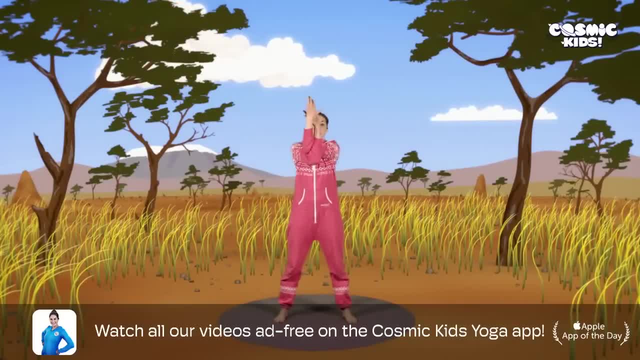 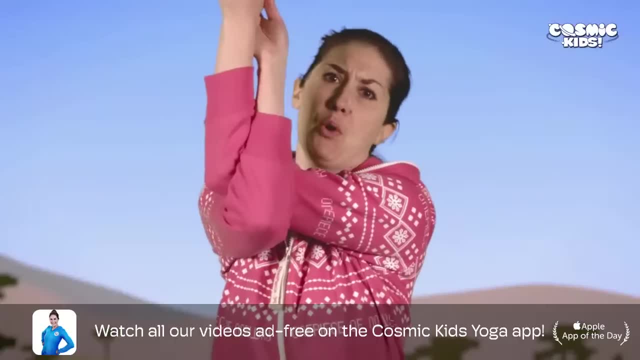 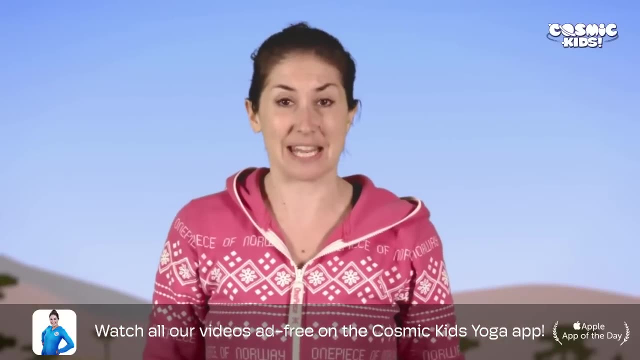 and wave with your underneath arm, Then swizzle your arms round. Ernie's trunk is in a knot. What did you do that for Poor Ernie? Lulu, you can't do that to Ernie. You need to count to ten and calm down, taking a deep breath. 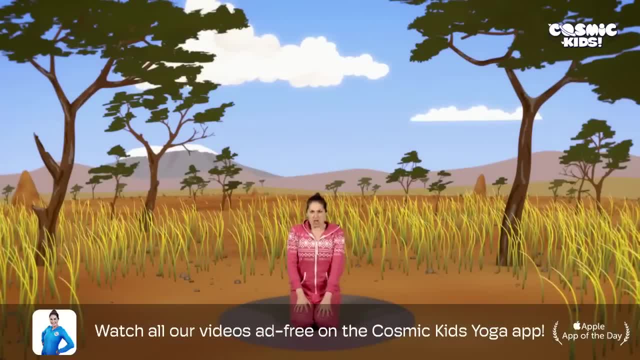 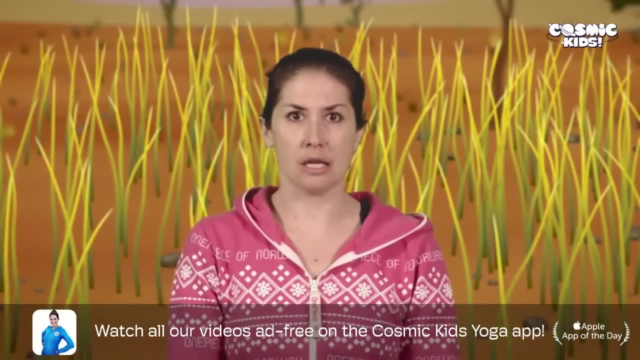 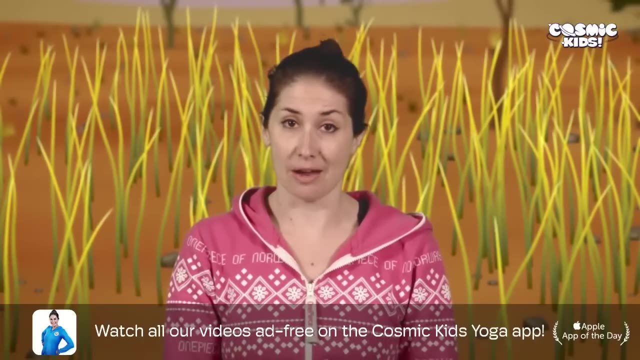 Lulu tries One, two, three, four, five, six, seven, eight, nine, ten. She unties Ernie's trunk Standing up. take your arms back into that swizzly trunk. Take your arms back into that swizzly position. 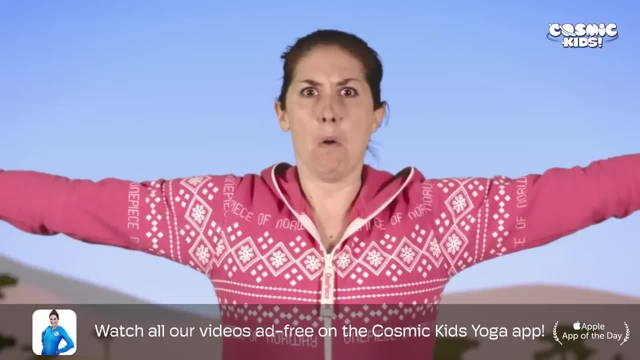 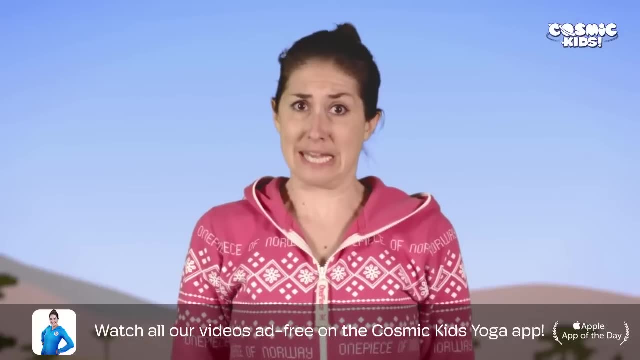 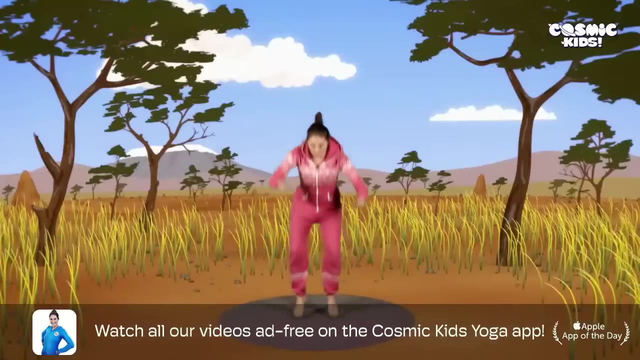 and untie them. Yes, Thanks for untying my trunk, Lulu. Lulu says sorry for being so mean and taking her anger out on poor Ernie. From the trees jumps little Mindy, the baby chimp. I couldn't help overhearing that you're having a problem with your roar. 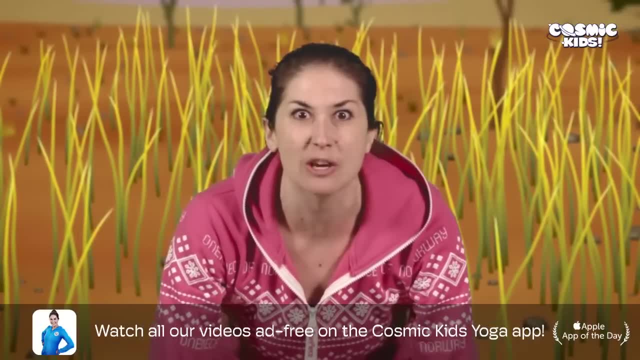 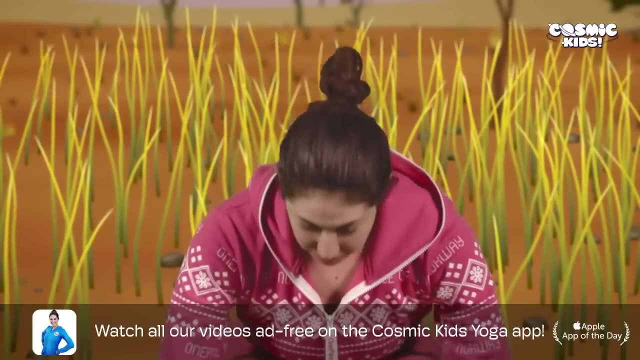 Well, what I do is I do big monkey jumps and I do a big monkey call at the top. I'll show you Three times Ready. We love monkey jumps, So we join in with Mindy, Up on your toes, ready to jump and call like a monkey. 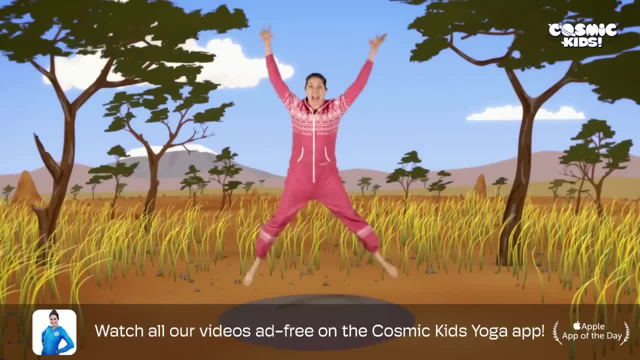 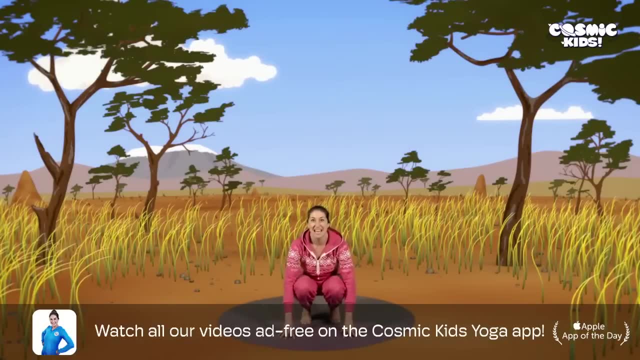 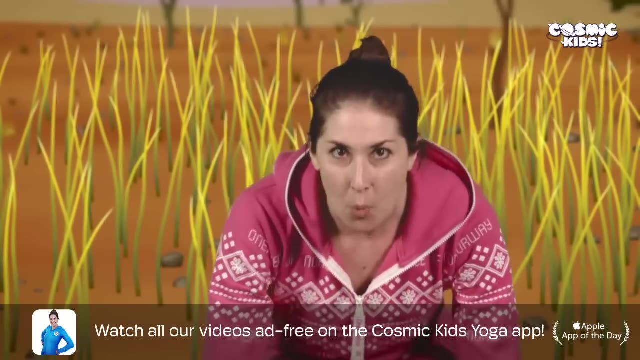 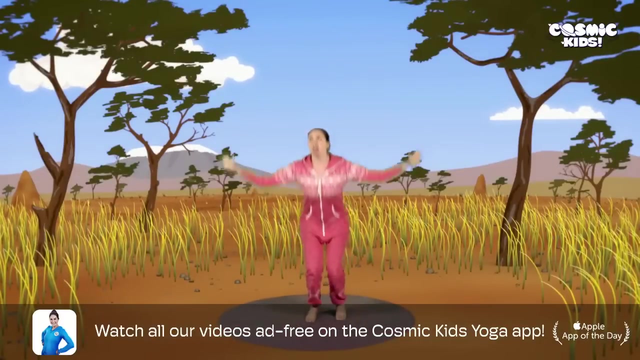 One, two, three And again. One two, three. Last time, One two, three. It's Lulu's turn. She's ready to go. One two, three. One two, three And again. 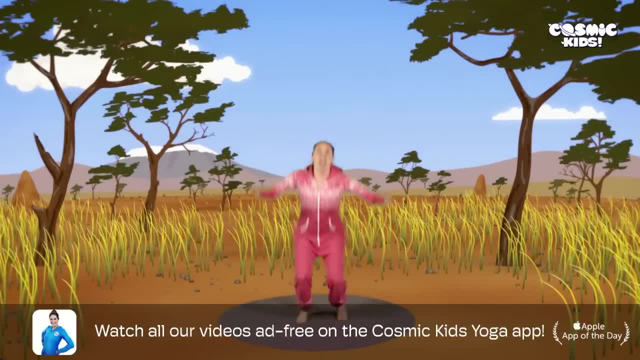 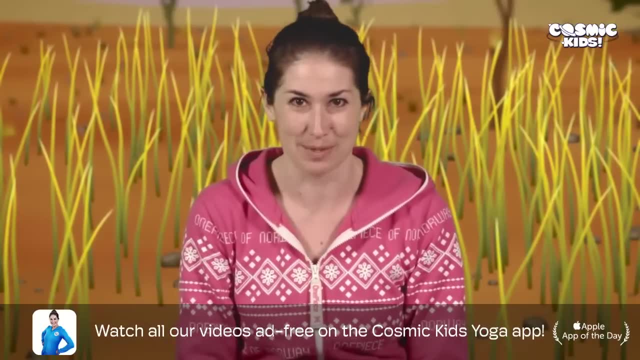 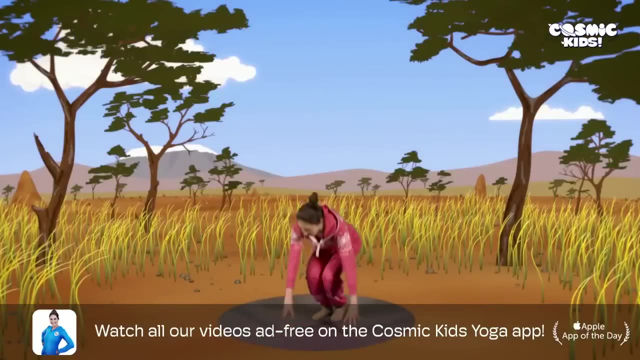 One, two, three. She's still a little bit grumpy, but at least she had fun doing the monkey jumps. All of a sudden, around the corner comes George, the baby giraffe, Standing up. put one foot forward, one foot back. 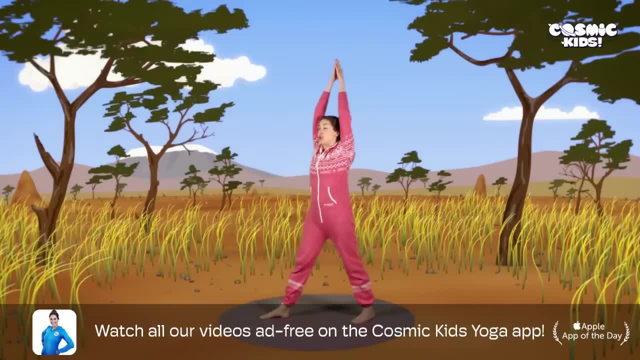 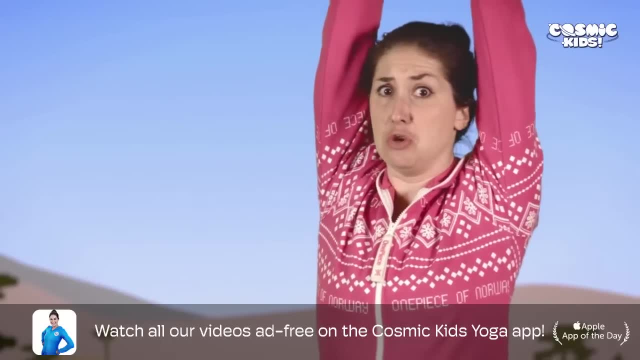 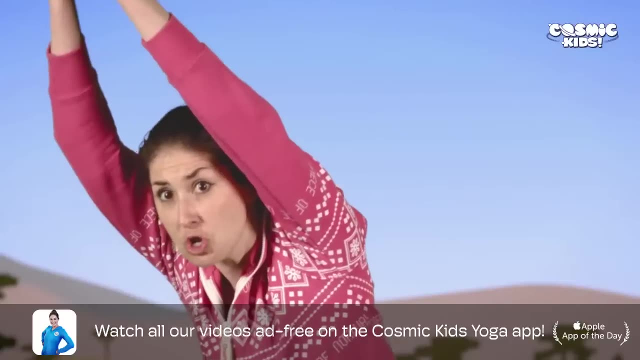 lift your arms up tall like a giraffe's neck. Now, giraffes don't make any sound, Nothing at all. And little George has something he needs to tell Lulu. Lulu, you need to warn everyone. The volcano's about to erupt. 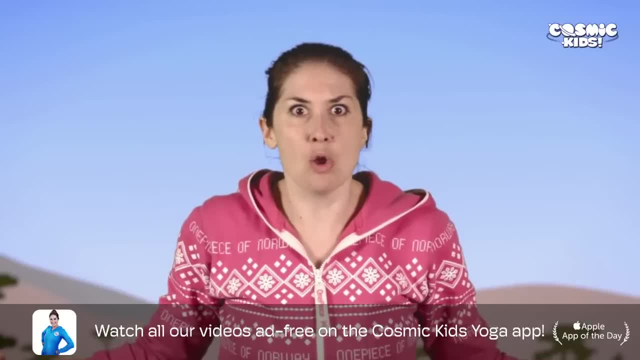 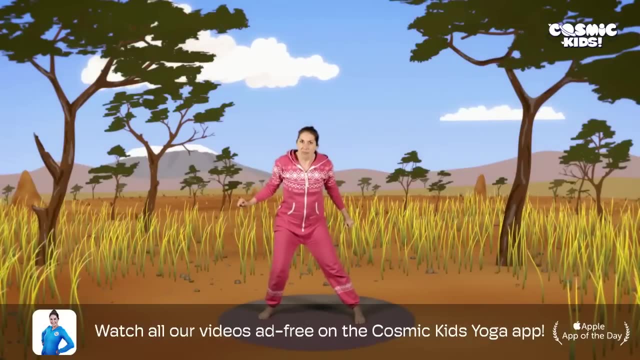 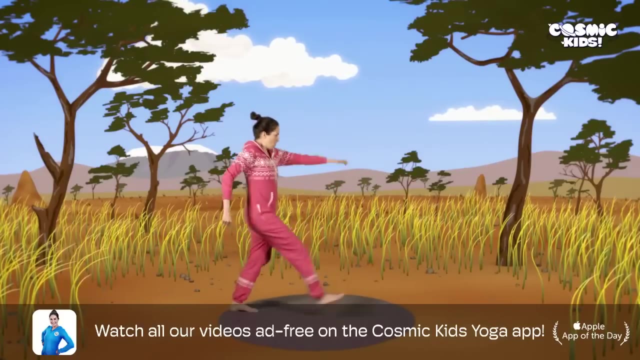 Oh no, This is Lulu's moment. She now needs to learn how to roar. She takes big, giant lion, steps up the hill Standing tall, step forward, Big step And again Big step. Lulu gets herself ready, Coming down to your knees, everyone. 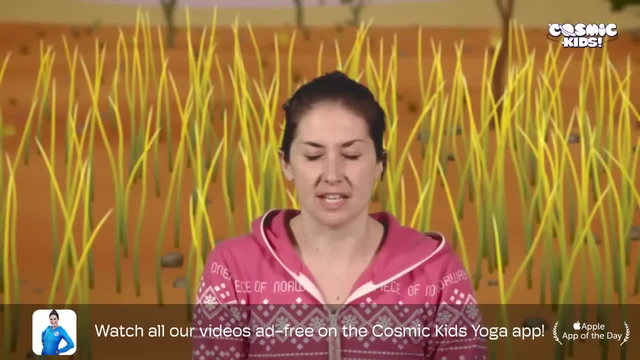 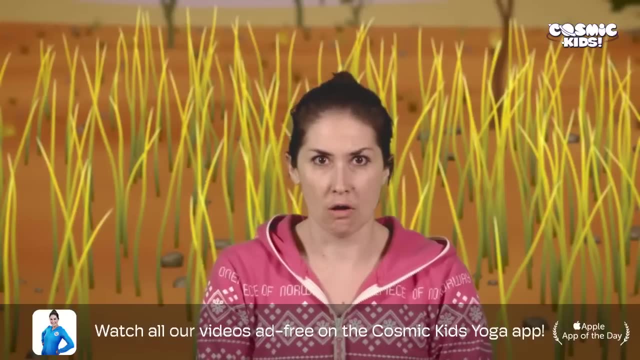 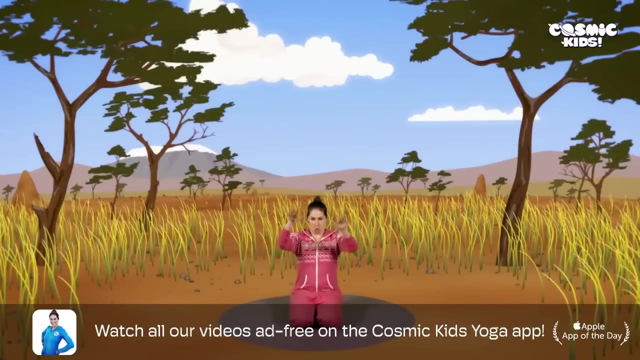 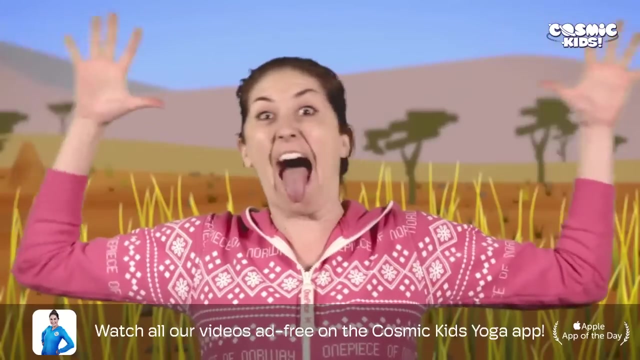 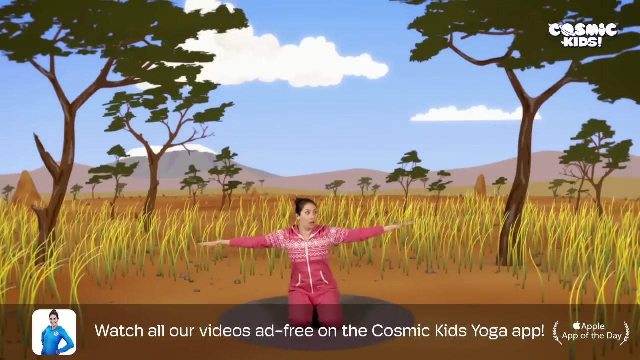 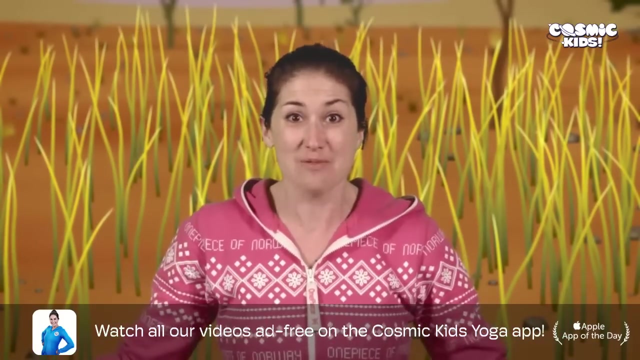 After three she takes a big deep breath And prepares for the roar of her roar In her life. One, two, three, The ground begins to rumble and shake. Lulu has done it. She managed to roar right when it counted. 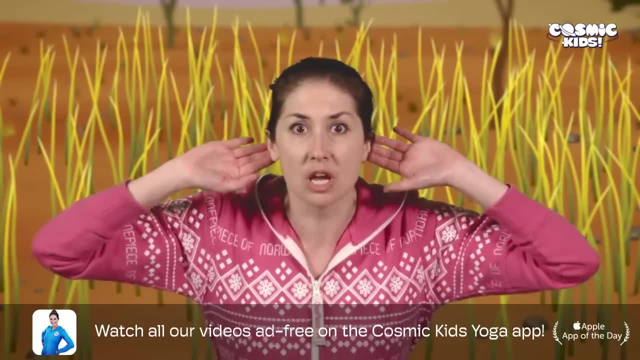 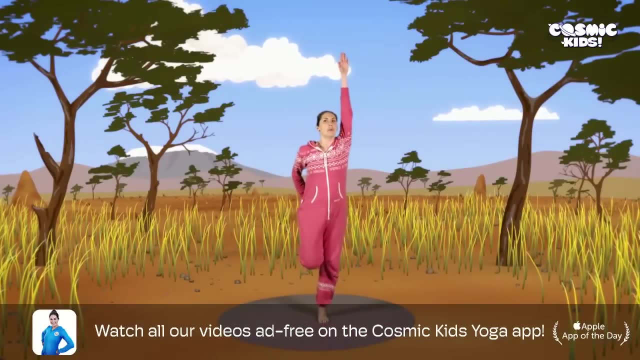 All of the animals hear her For miles around The flamingos. hear her Standing up, Reaching tall, Seeing if you can hold on to one foot And maybe hopping a bit. Was that a baby lioness? Yes, I think she was roaring about the volcano. 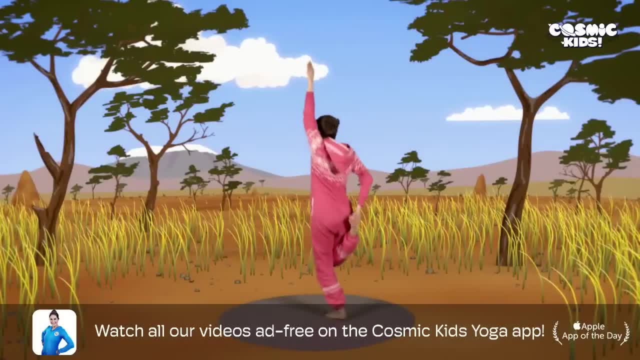 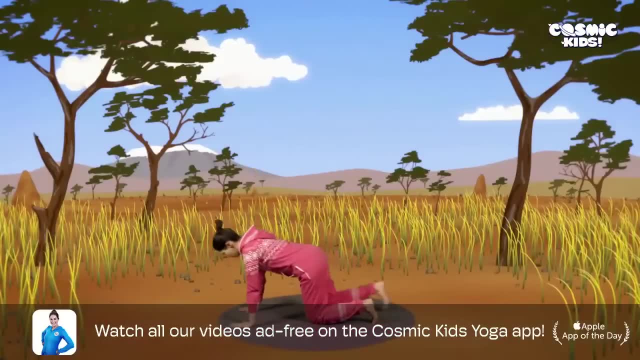 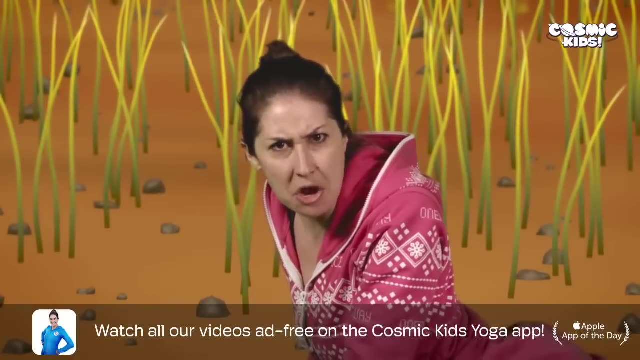 Right, Come on Off we go. Hoppity, hoppity, hop. The other animals that hear her, The snakes slithering around Coming onto our tummies. everyone Sounds like a baby lioness. She was roaring about a volcano erupting. 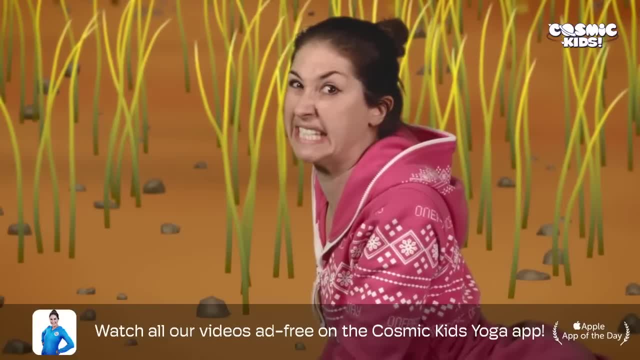 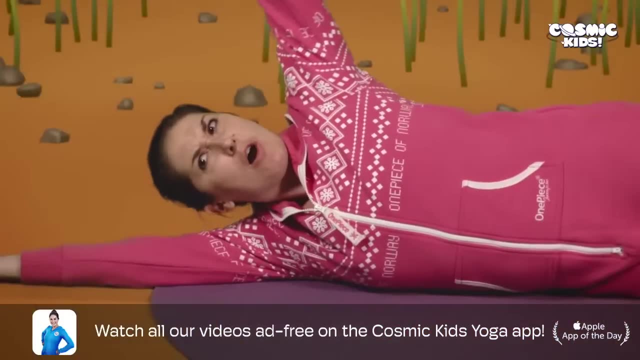 Come on, snakes, Let's slither away. The crocodiles hear her Stretching out long, Opening their jaws. Did you hear that? Yeah, I heard that. That was a baby lioness, Right? Yeah, She was roaring about some volcano. 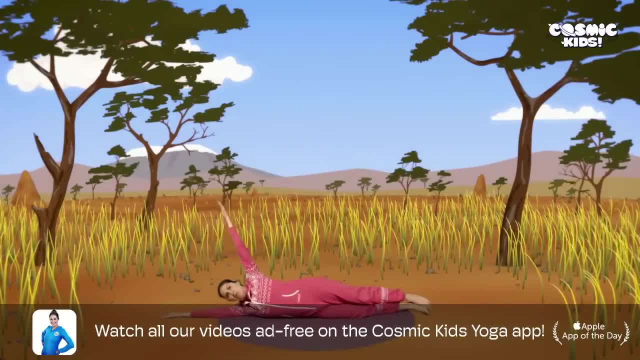 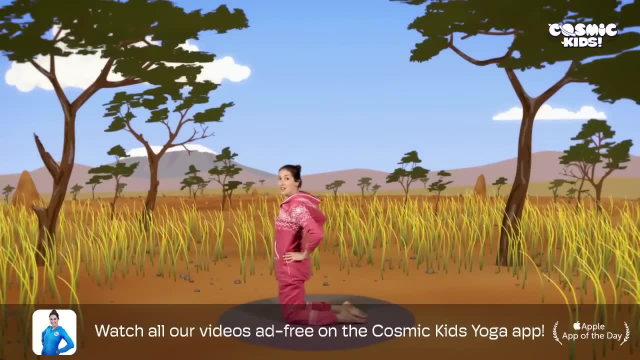 Volcano's erupting Right. Come on, Better get moving on, Go, go, go. And the camels heard her Coming back up to two knees. everyone Put your hands behind your back And press your bottom forward, Looking up to the sky. 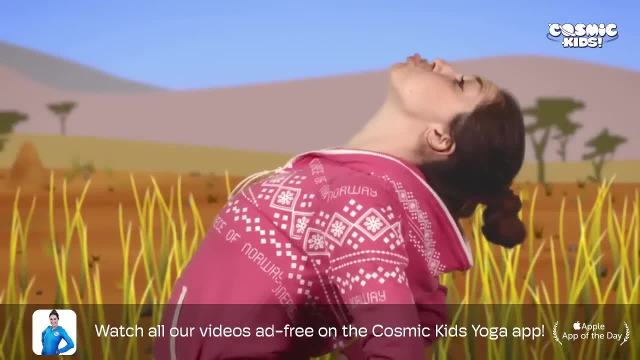 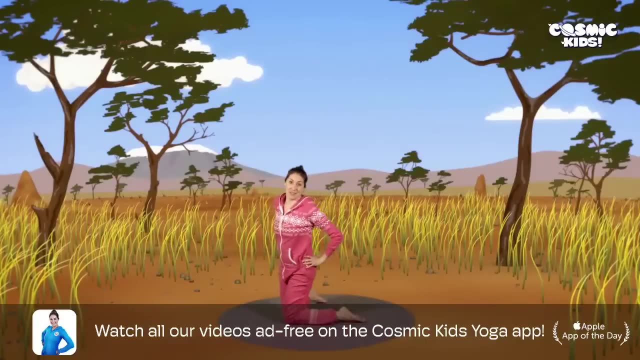 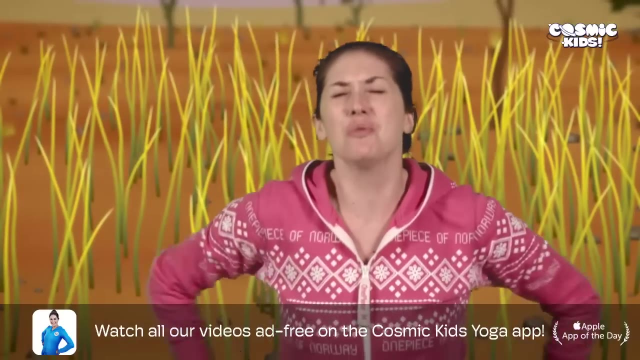 And do a big raspberry to the ceiling. Well, That's charming. of the camels, All of the animals heard little Lulu, Including her mummy, Her daddy, Her brothers And her sisters Who were so proud Of their little baby lioness cub. 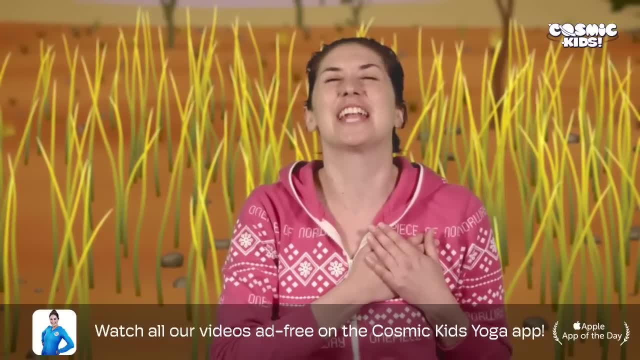 She had done it. She had learnt how to roar And, along the way, She learnt how to cope With getting frustrated And angry, Which was really good, But we'd better get out of here. Floating down towards us Is a hot air balloon. 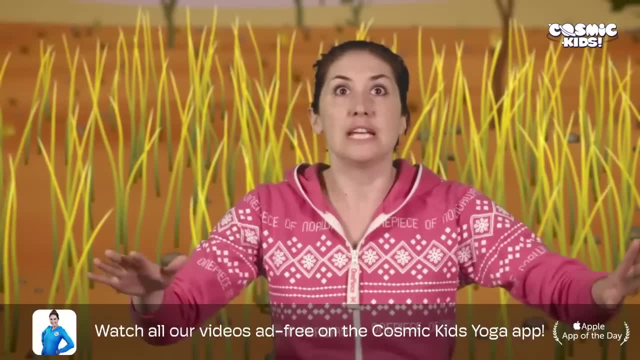 That's how we're going to get home. Yay, We cross our legs And we need to blow it up again. So it's nice and full. We bring our hands around our mouth And we blow, And we blow, And we blow. 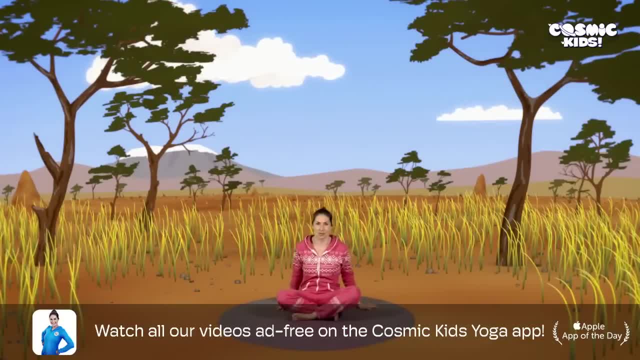 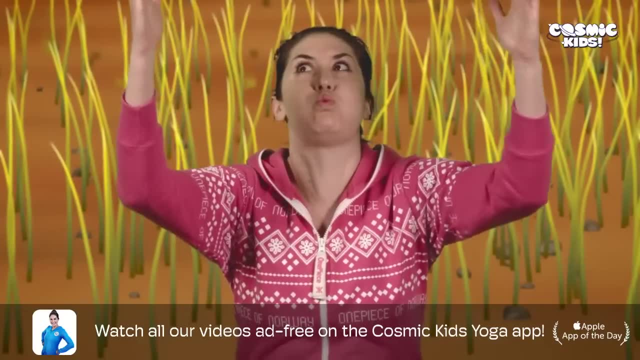 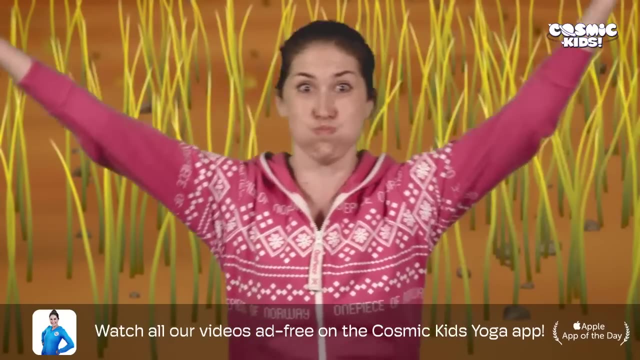 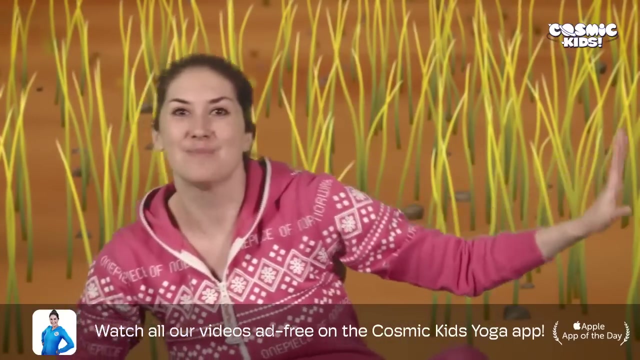 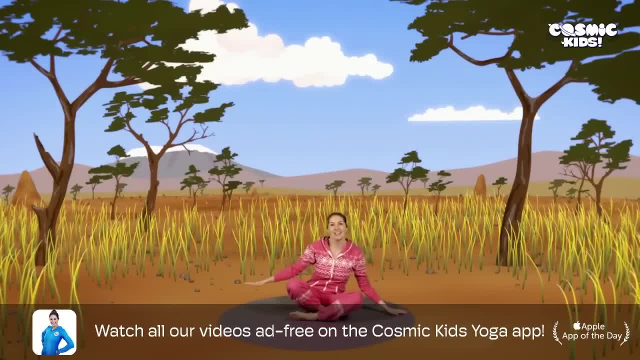 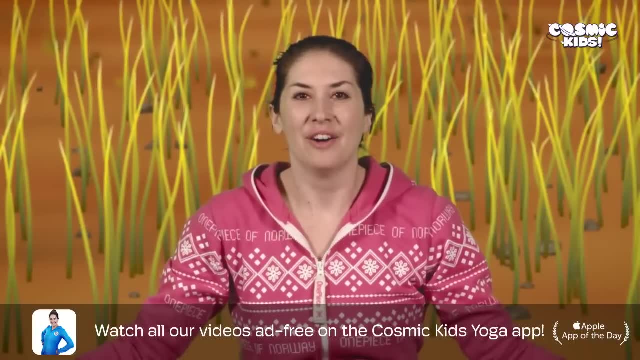 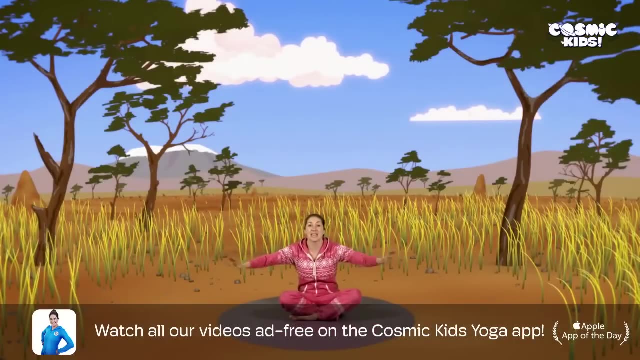 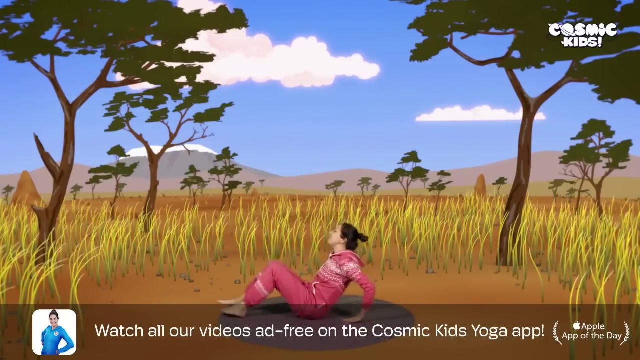 Tock Like a clock Until I find my center. Wow, Wow, we've done it. we're floating away. We wave down to Lulu and all of the other animals as they hide and prepare themselves for the volcano. We lie back in our hot air balloon feeling pleased at how we have helped Lulu today find. 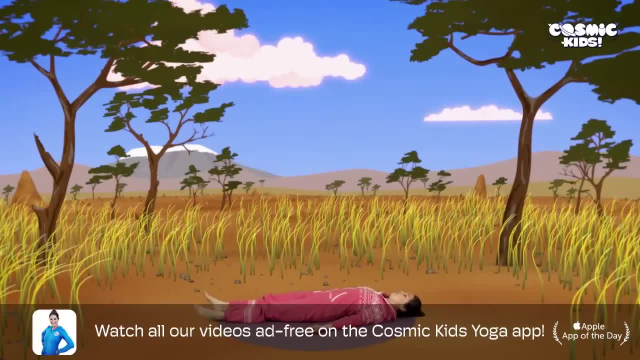 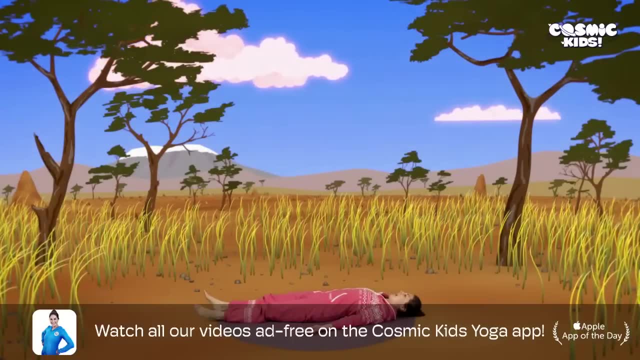 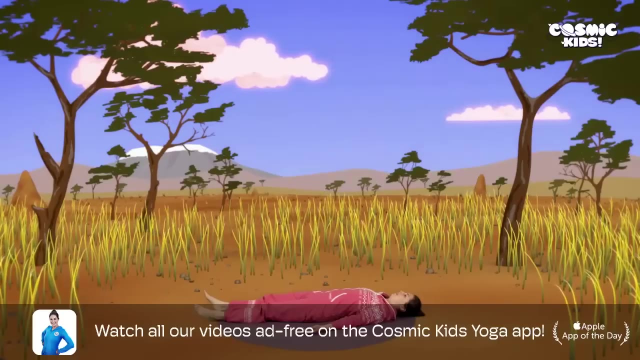 her roar. But what's more important is we've helped Lulu learn how to deal with it when she gets all frustrated and angry. Being unkind towards herself isn't going to help her, but if she can, in that moment when she's angry, breathe, breathe slowly and deeply. count to ten. maybe take a little. 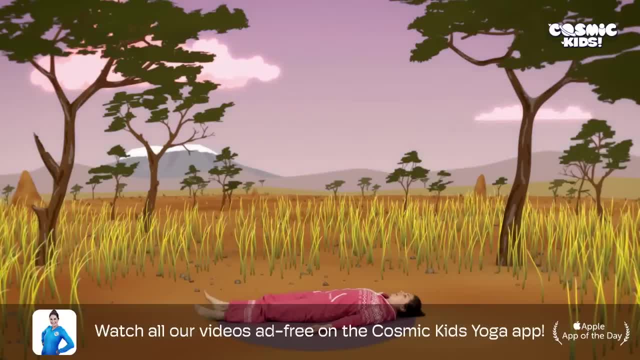 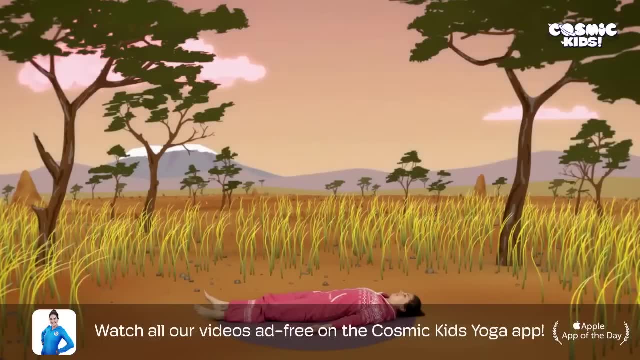 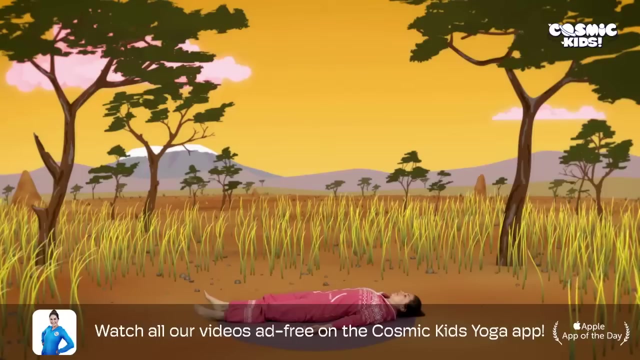 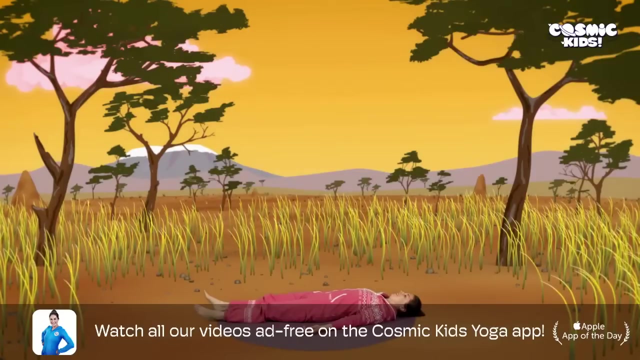 walk, if she needs to, for some fresh air. She will clear her head. Well done, Lulu. Well done for finding your voice. We've all got a voice and we all need to let it out. sometimes We relax here in our hot air balloon, but then it's time for us to wake up again. 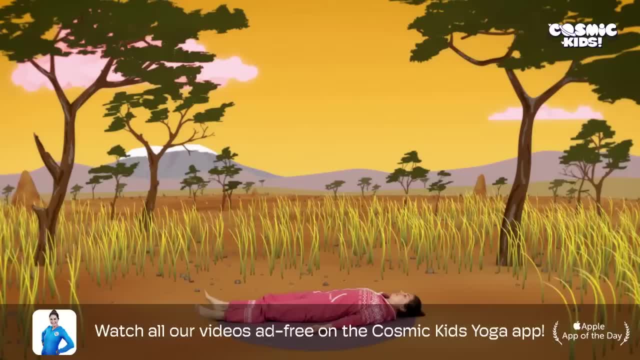 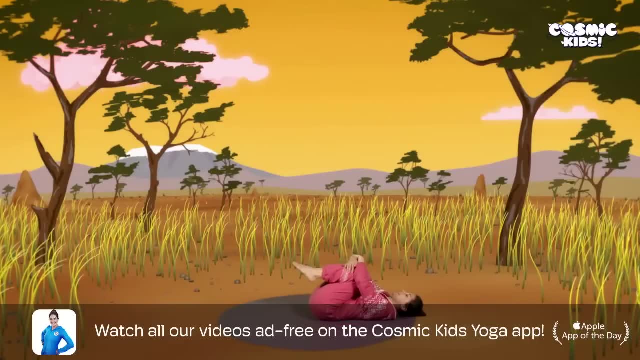 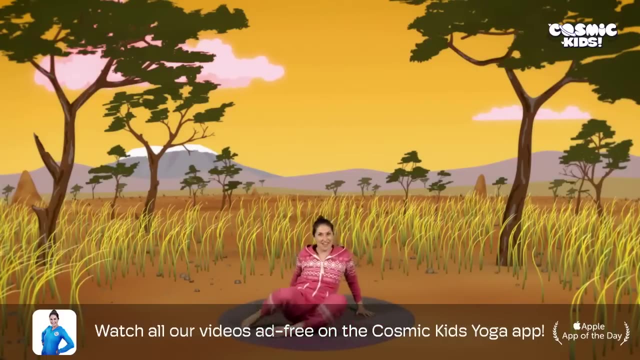 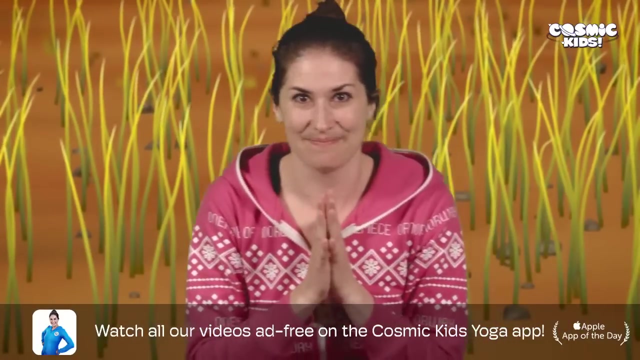 So we wiggle our fingers and our toes, We hug our knees into our chest and roll over onto our sides to come up to sitting again with our legs crossed and our hands together at our heart, just like we started. And we finish with our secret yoga code word, which is Namaste. 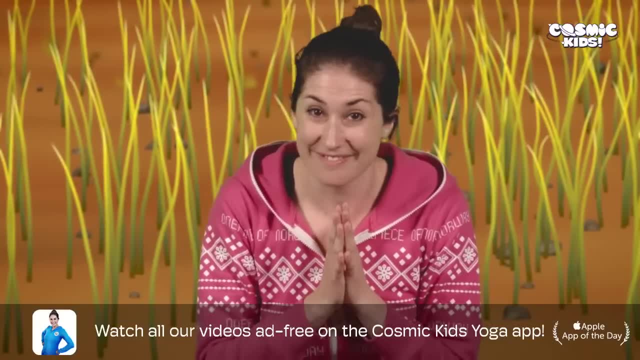 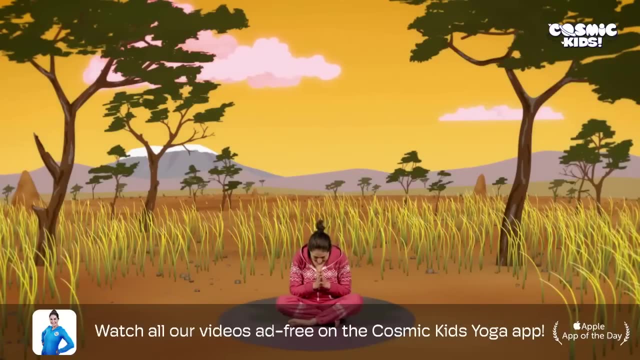 Namaste, Namaste, Namaste, Namaste. Ready One, two, three, Namaste. Well done everyone. Thanks for coming on the adventure and for helping Lulu with her anger You did so well. Come back soon for another Cosmic Kids adventure. 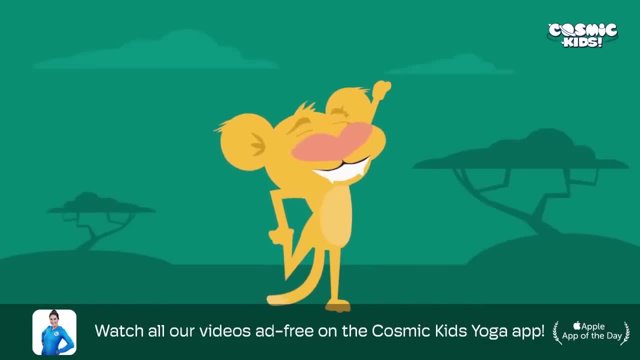 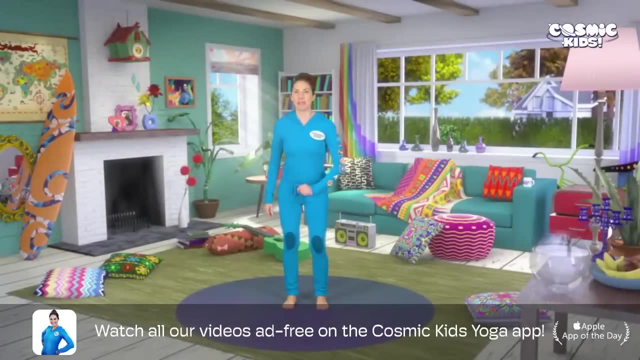 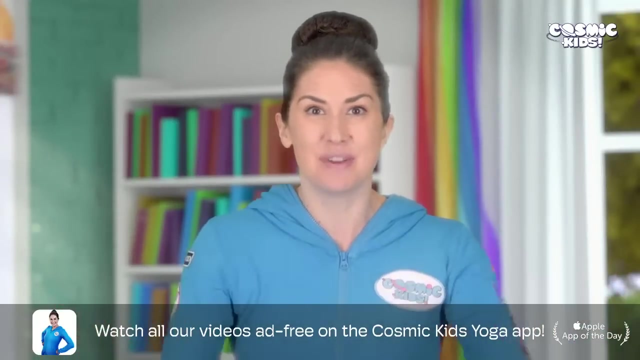 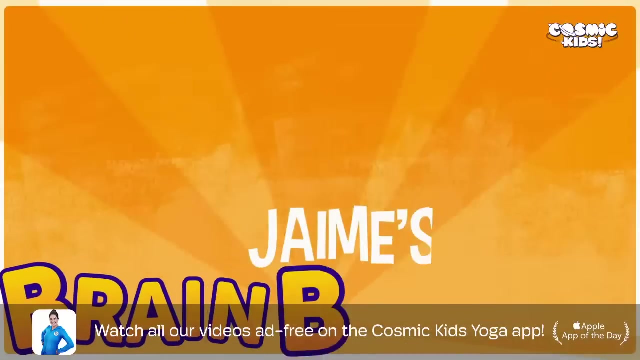 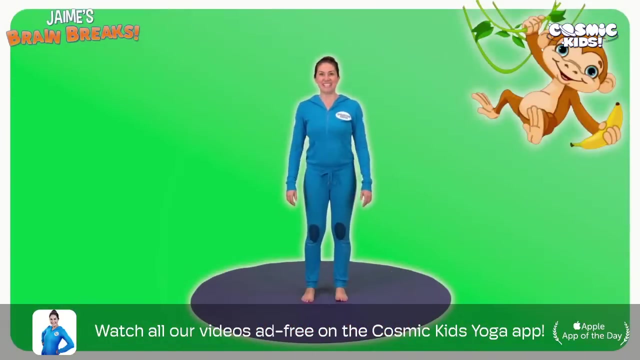 Bye-bye. Don't forget to join me on Saturday morning for Saturday morning yoga. Get everyone at home together and enjoy some family time. Remember, subscribe and hit the bell so you never miss one. I'll see you Saturday. Today we're going to do a little call and response song called Walking Through the Jungle. 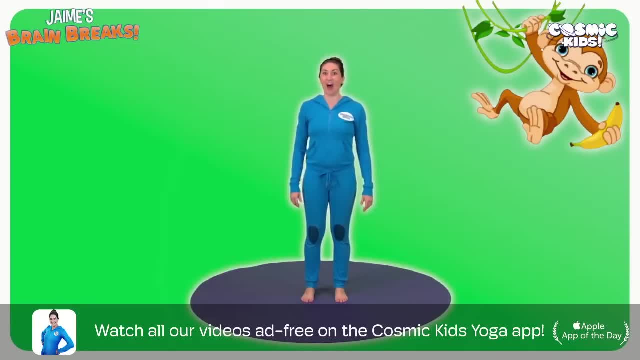 And there's lots of yoga poses to do along the way. I'll sing a line and then you sing it back. Let's go. We begin with a walk, Walking through the jungle. What can I see? I can see a lion. 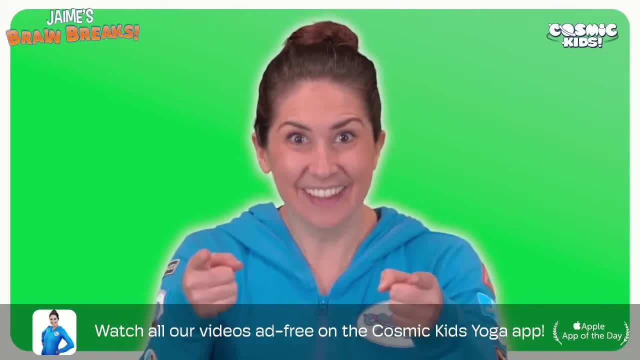 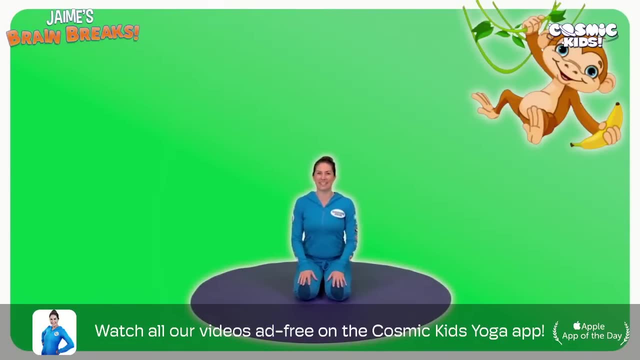 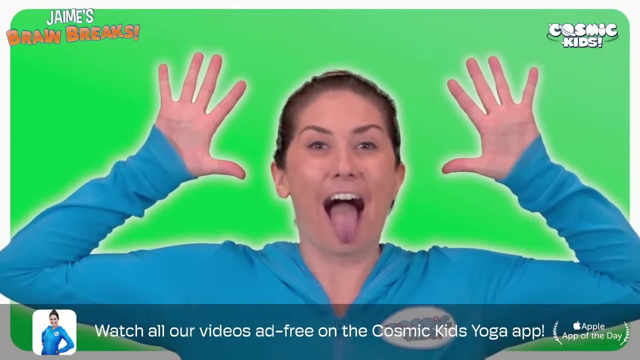 Roaring at me Coming into lion. pose everyone Down on your knees After three Big roar to the sky Ready: One, two, three Roar And let's carry on in the jungle, Coming to stand and walking. 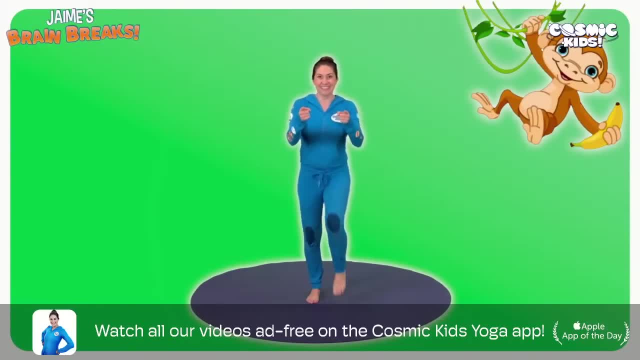 Walking through the jungle. What can I see? I can see a monkey Jumping at me. Let's do a monkey jump, coming all the way down to crouch and after three big jump in the air with a monkey. call Ready One, two, three. 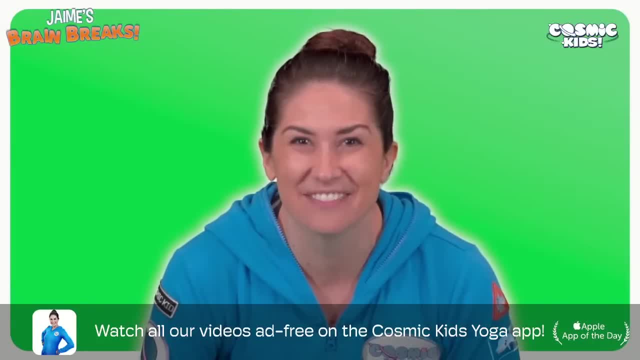 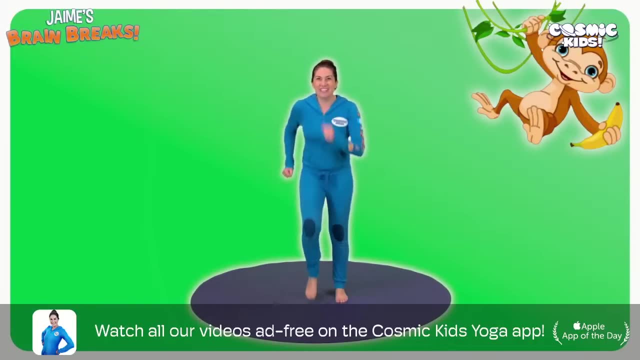 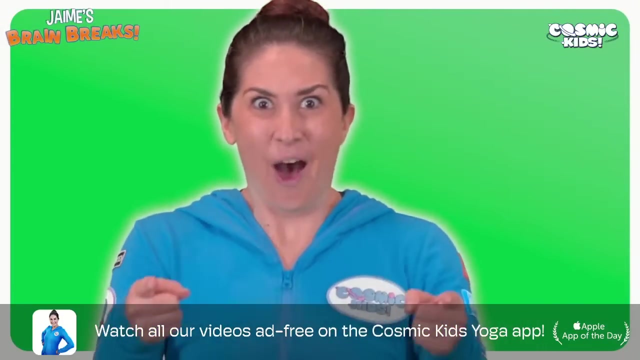 Wow, well done. everyone Coming up to stand, and let's carry on in the jungle, Walking through the jungle. What can I see? I can see an elephant. Let's carry on in the jungle. What can I see Walking through the jungle. 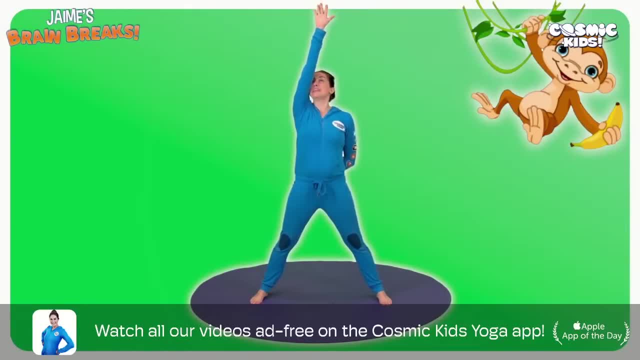 What can I see? I can see a monkey. Let's carry on Following the jumping lion. It's a monkey Way to go. Group of backpackers, everybody on your vault Watch or run Who's going to jump. Ч绢 chest. 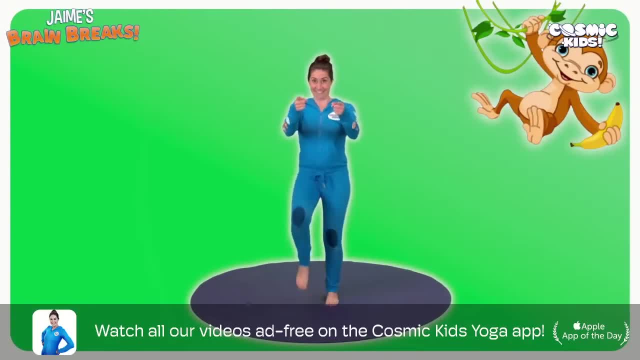 Group of backpackers. everybody on your vault, Jumping, jumping, jumping, jumping, jumping, jumping at me. what can I see? I can see a snake hissing at me, coming down to lie on your tummies. everyone into your snake, pose hands under your shoulders and wriggle, wriggle. 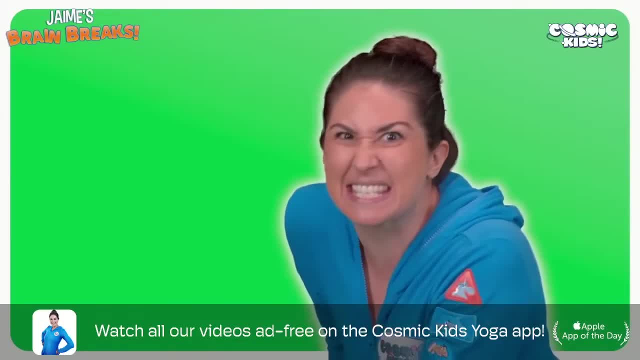 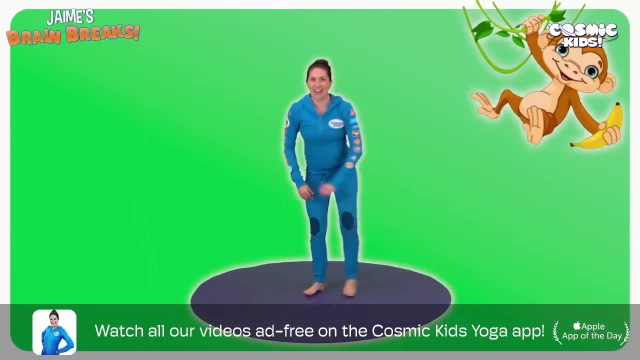 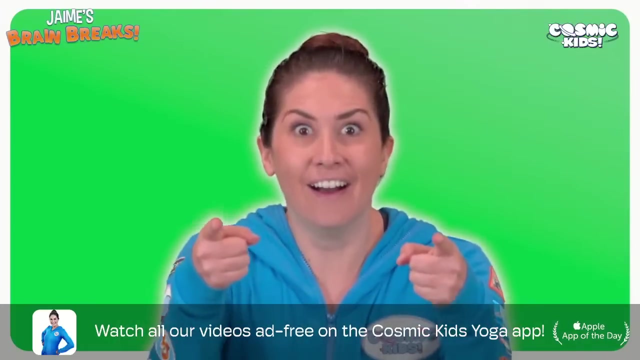 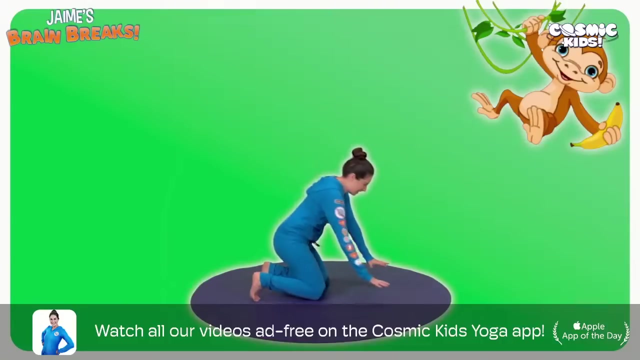 wriggle up with a nice oh well done. everyone coming up to stand again, let's carry on walking, walking through the jungle. what can I see? I can see a tiger clawing at me, coming down to lie on your tummies. on to all fours. everyone, let's try our tiger pose. reach one arm out and see if. 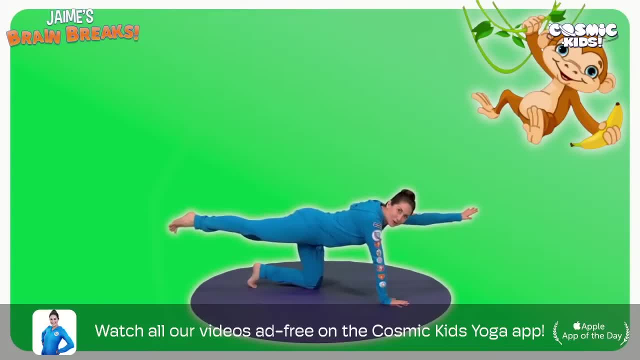 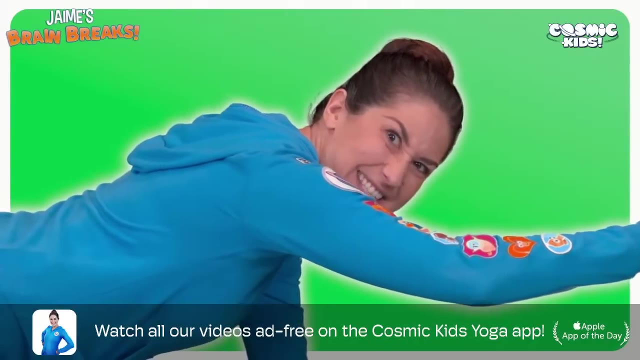 you can reach your opposite leg at the same time. oh, try not to wobble and do a big claw and the other way: hand and knee come back down, other arm goes out, other leg goes out- ready, fantastic, coming up to stand and let's carry on walking. 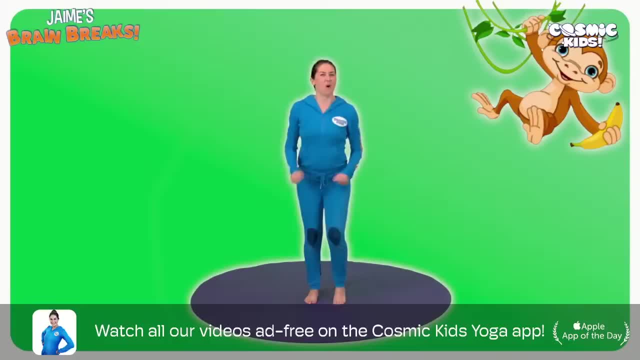 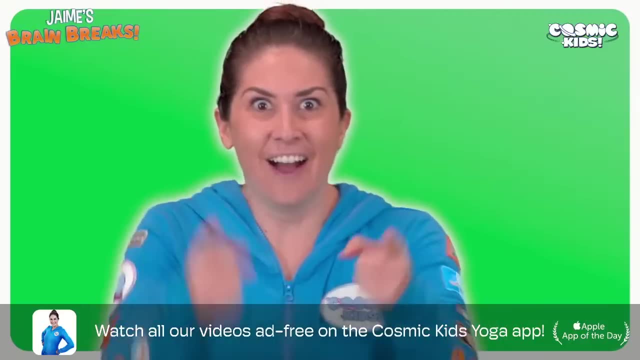 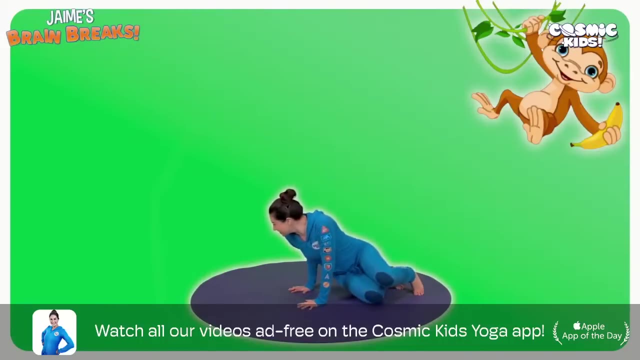 through the jungle. what can I see? 24 hours walk, what can I see? I can see a crocodile snapping at me. let's come into crocodile pose lying on our sides. everyone, make your arms as long as they'll go above your head and then use your top arm to open and close your big. 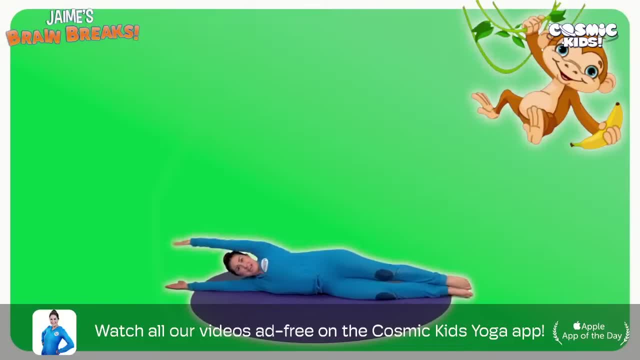 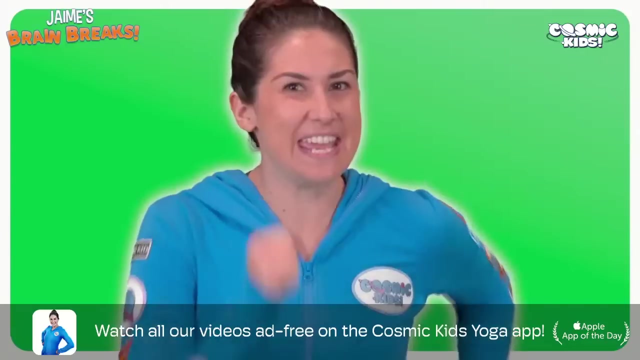 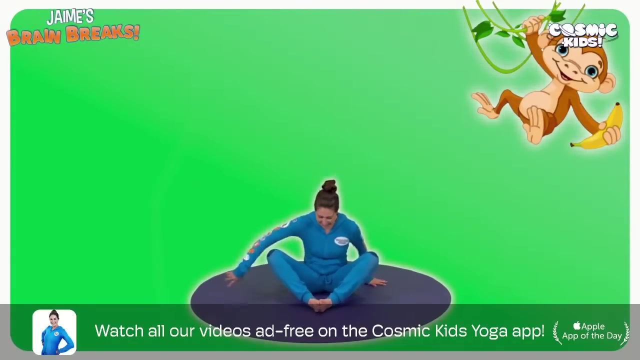 crocodile teeth. yes, snapping away. oh, my goodness me, let's carry on. through the jungle, the jungle, coming up to stand and walking, Walking through the jungle. what can I see? I can see a butterfly fluttering at me, Coming to sit on your bottoms, everyone joining the soles of your feet together. 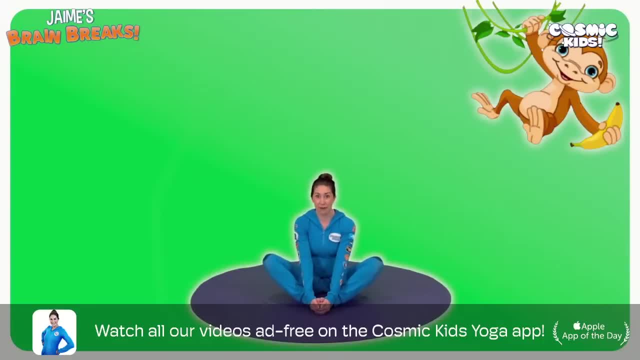 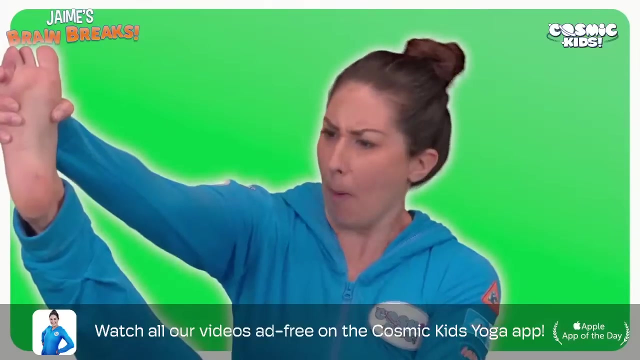 holding onto your toes so that you can stretch and flutter your butterfly wings. Now let's have a look at those beautiful butterfly colours. Let's lift up one wing Ready After three. One, two, three. Amazing, We've got pinks and oranges and reds and golds- Beautiful, Lowering that wing down. 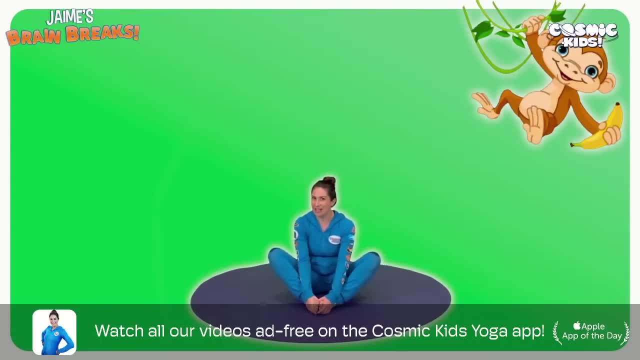 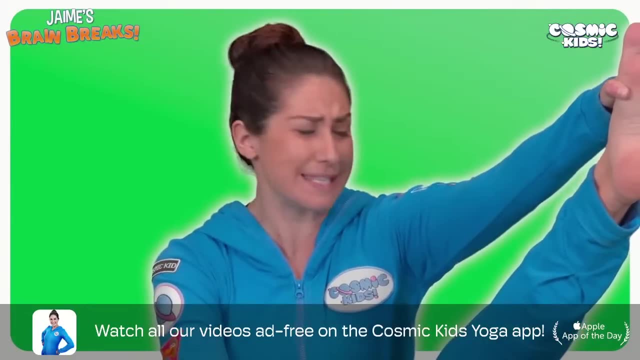 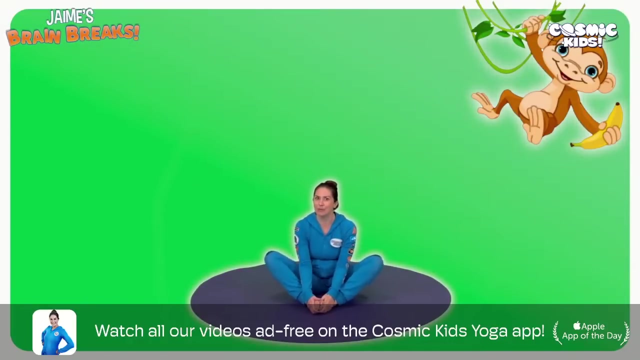 fluttering a little bit further. and then let's look under the other wing: One, two, three Amazing Blues and greens and turquoise and silver. It's gorgeous Lowering that one down, fluttering a bit further. Shall we look under both wings, both at the same time? 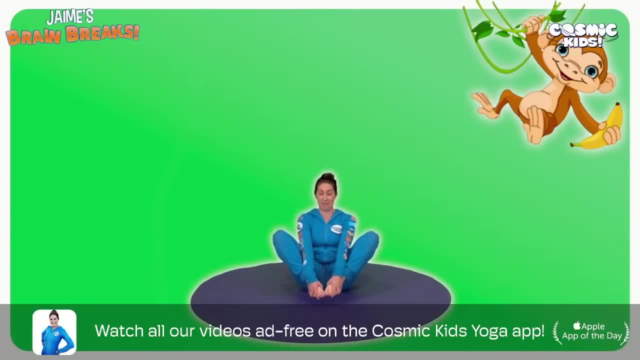 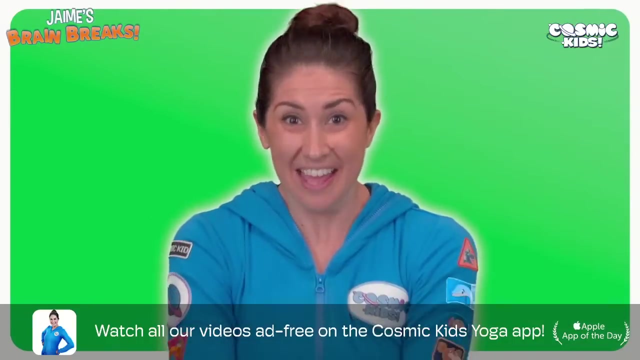 Come on, I think we should Ready After three. See if you can hold your balance. One, two, three, Amazing All the colours of the rainbow Lowering your feet back down. everyone Well done. Thanks for walking through the jungle with me. Have an amazing day. 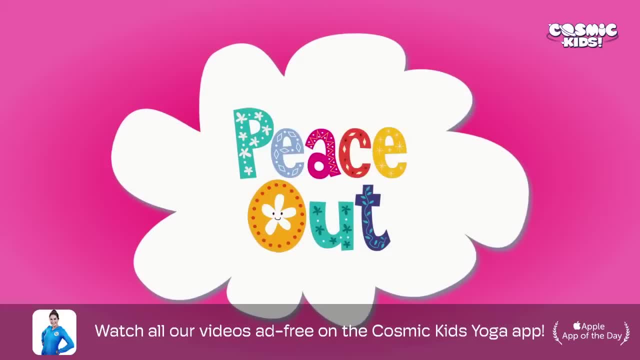 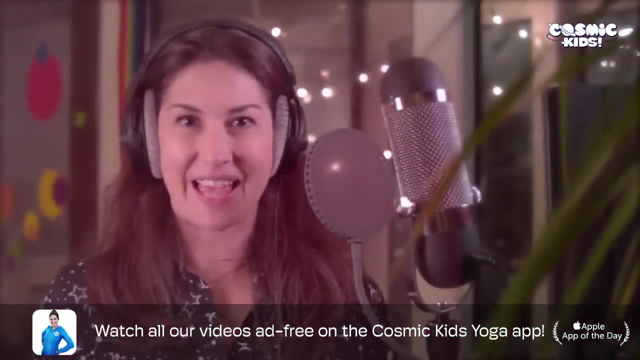 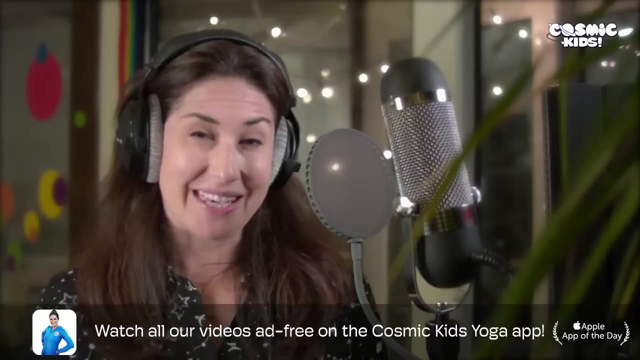 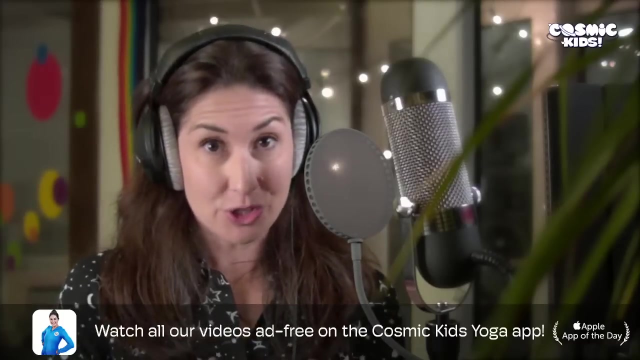 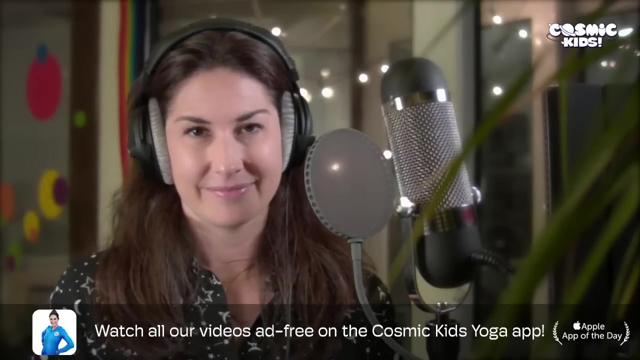 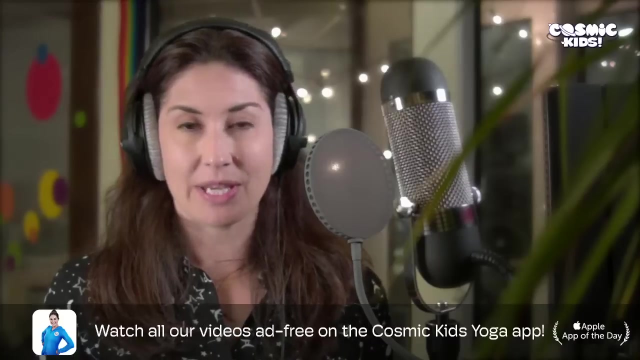 Peace out- Sleeping dragon. Hello Jamie here. Welcome to peace out. Let's begin by getting comfortable, Finding a space for ourselves To lie down or sit. You choose what works. Now give yourself some time to settle, Doing any last minute wriggles or fidgets. 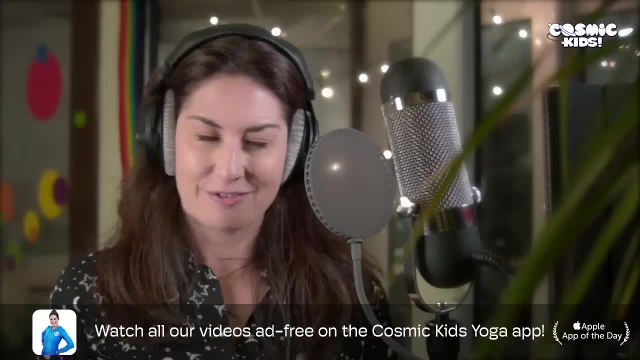 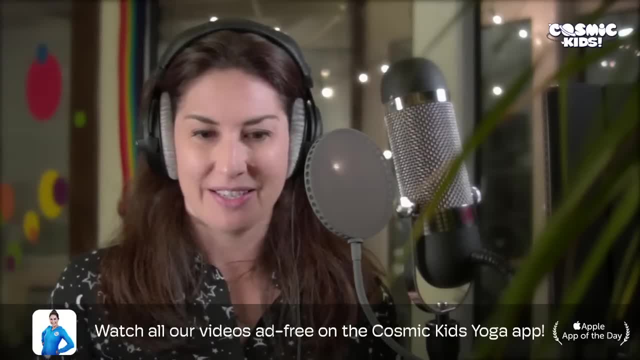 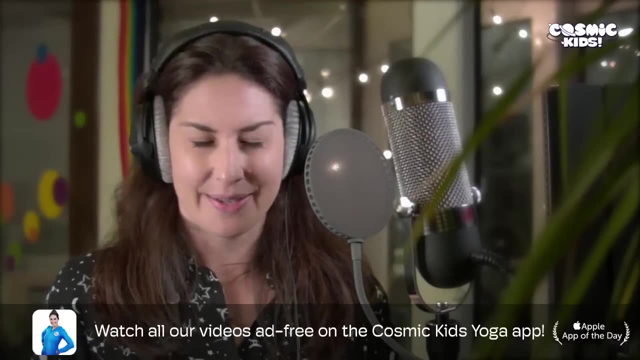 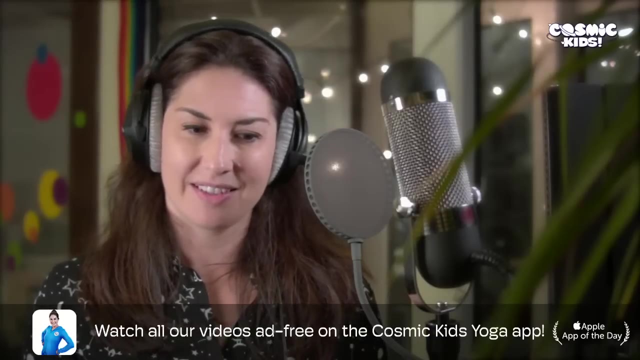 But give yourself time, Be kind to yourself. Some things take practice, Lots of practice, But the more you do it, the easier it gets. Keep your eyes open for now and see if you can notice your breathing. I find it helps to slow my breathing down, so it's easier to follow. 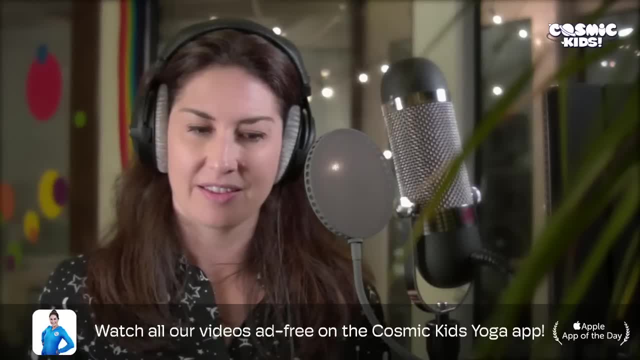 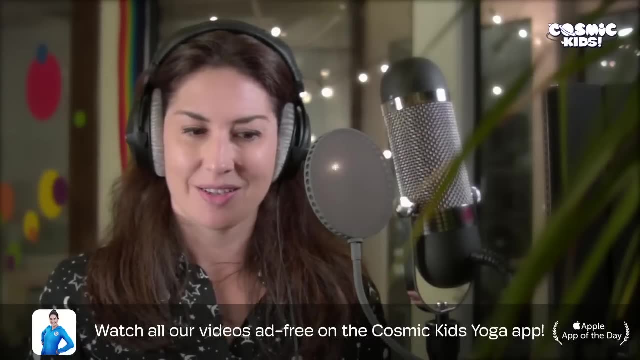 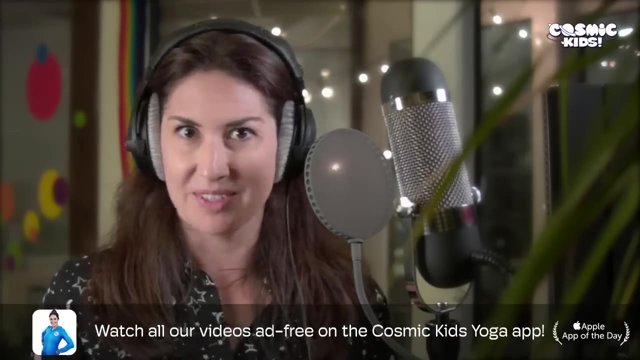 The in-breath and the out-breath. Usually I find there's a small gap between the breaths. Can you spot that too, Breathing in little gap and then out- little gap. It just happens like that without really thinking about. 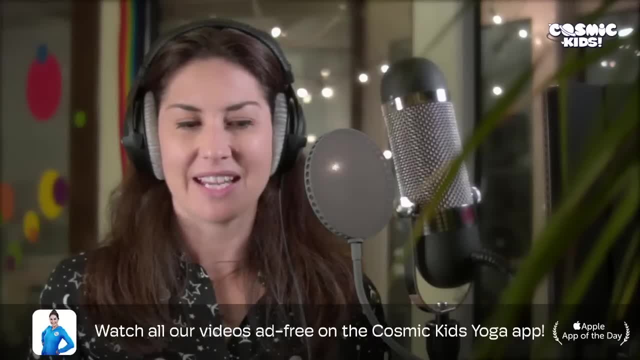 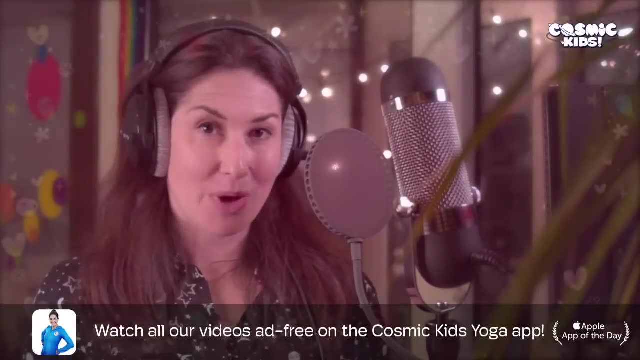 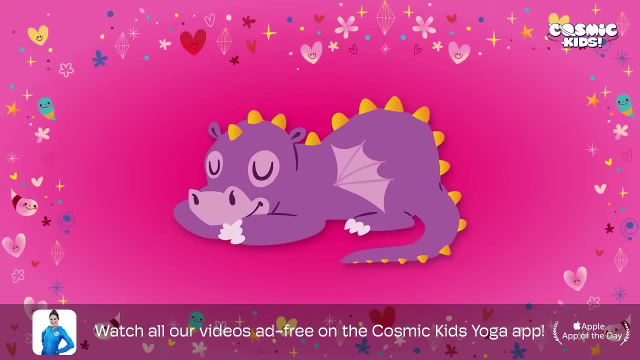 it Next time. as you breathe out, let your eyes softly close. Now your mind can make the pictures as we go on a special adventure, like in a dream. This is a story about a family of dragons. As you learn about them, maybe you'll see how life for the dragons is quite similar to the 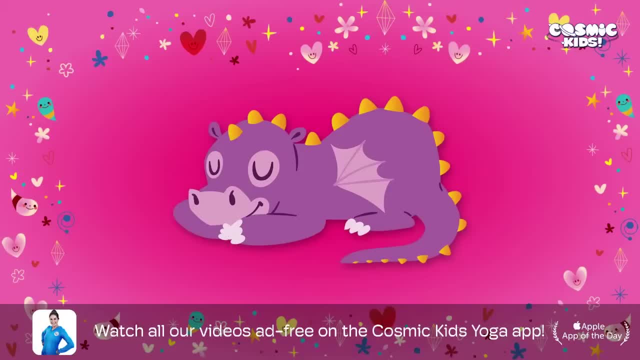 way we live. Mummy dragon was called Delilah, Daddy dragon was called Doug. and there's the baby had a little girl dragon called Dina. They lived together on a mountain covered in flowers and grass and had a lovely mossy cave where they ate together and slept. Nearby was the 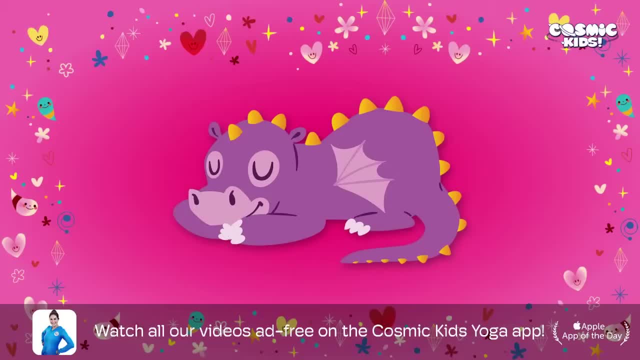 waterfall and pool where they would take a shower or bath. Every day, Mummy Delilah and Daddy Doug went out to work. They had a restaurant called The Flame Grill where they prepared delicious barbecue vegetables and toasted marshmallows for dessert. It was hugely popular. 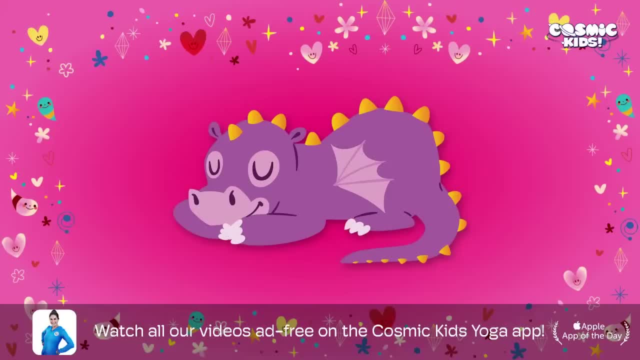 with all the dragon families in the area, so they were very busy most days, and sometimes the evenings too. Dina spent her days at dragon school practising her powers, exercising her wings, With some flying drawing cloud pictures in the sky, changing colour to camouflage herself. 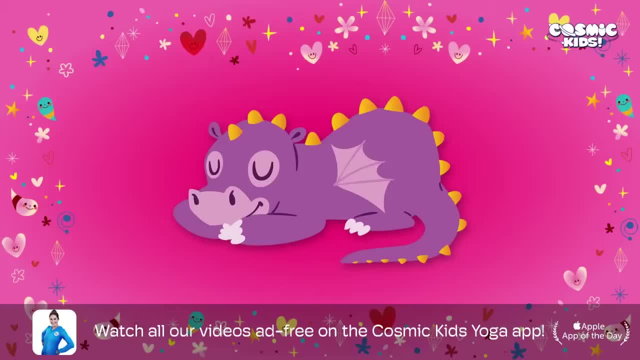 and learning how to control her fire breathing. There was so much to learn and practice. Sometimes Dina found it hard and frustrating as she just wanted to be good at everything right away. When she got angry at things not going her way, she would end up setting fire to everything. 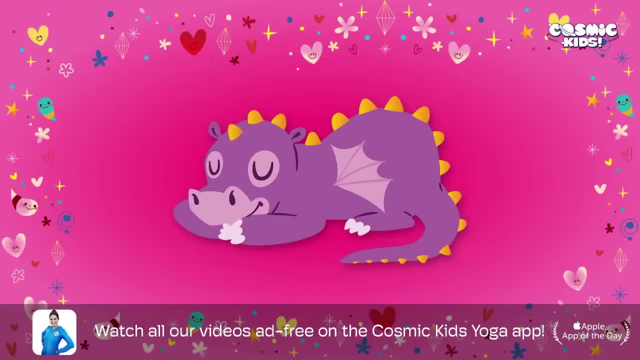 around her. That didn't help at all, And it only made her feel upset at the damage she'd caused. Dina was learning how powerful her feelings could be, But it was happening more and more often. Losing a game of Dragonopoly. 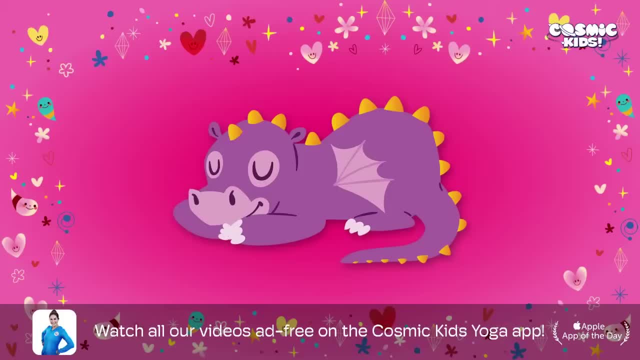 Just another day at the party. not only making her cloud picture just as she hoped, but making her bed in the morning tipped her over the edge and set fire to her pillow. All this frustration was getting her down. One day Ms Blaze, Dina's school teacher, took Dina aside after lunch. She had seen 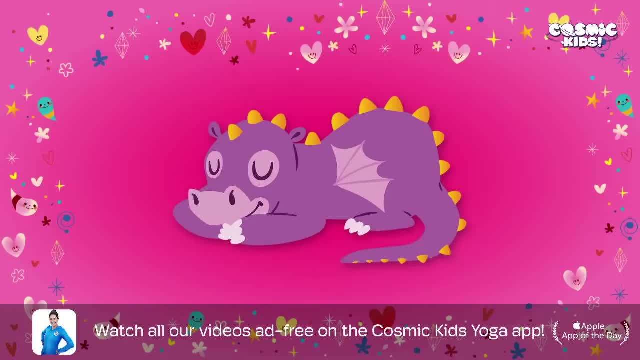 how Dina was struggling to cope with her fiery feelings and wanted to help. I went and told her that she couldn't get on with it. She said: how would I help? Did I even want to help? How could I help her? Why is this happening to me? She was like I've never seen this before. 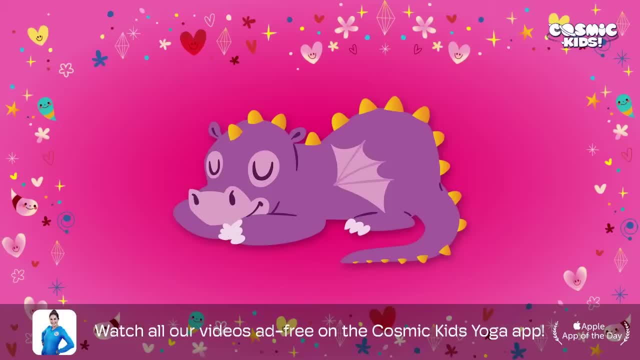 and wanted to help. Miss Blaze explained how a dragon's brain and body need time and patience to learn how to do things. She gave Dina some very special advice. The best thing a young dragon can do is learn how to use your breath to steady the fiery feelings we all have. 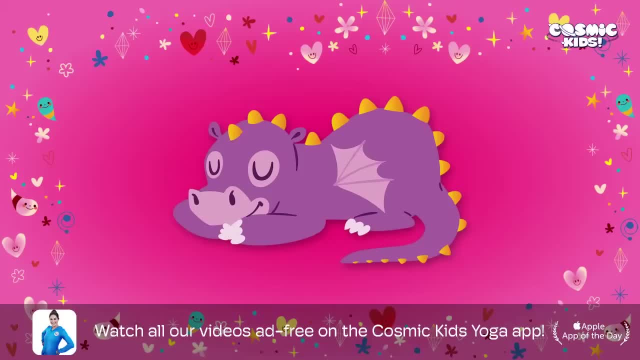 Dina decided to give it a try. Burning everything to a crisp wasn't helping and she needed to do something. So she started practising calming her breath down Every day, spending just a few moments closing her eyes, noticing her breath, the in and the out. 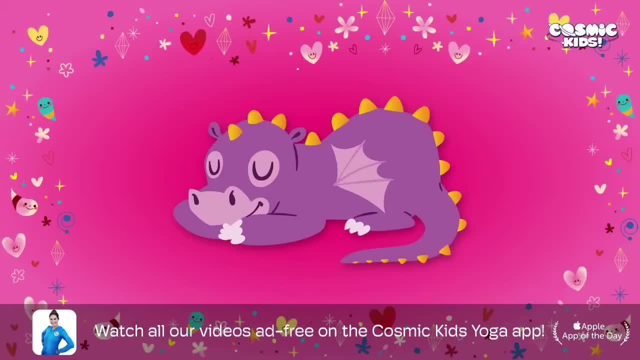 and slowing it down. After a minute or so of doing this, she felt calm. Her mind would feel clearer And on opening her eyes she felt good, like her body and mind were thanking her for being kind to herself. After a week of practising her daily breathing exercise. 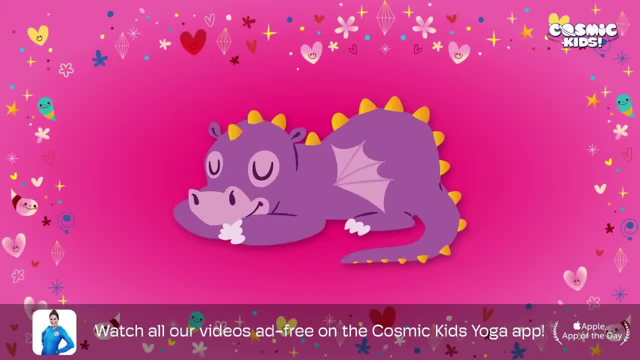 Dina's parents noticed how their daughter seemed happier, somehow calmer. They knew she'd been having trouble at school, but her frustration could send everything up in flames, and that she hadn't really been sleeping well. But something had changed. 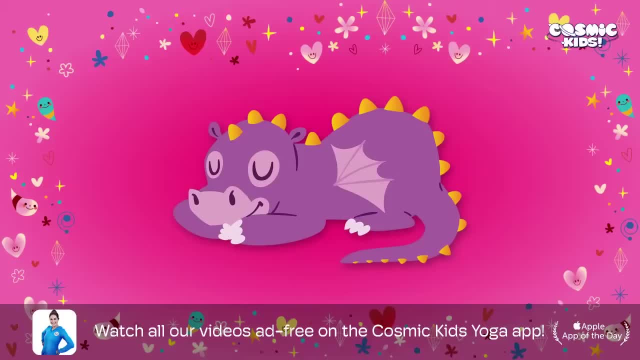 It was during bath time when Doug asked Dina how everything was going And Dina explained how she'd been learning to calm her breathing, That she was noticing when a spark of anger would appear when she found something hard, And that with the little breathing practice every day, 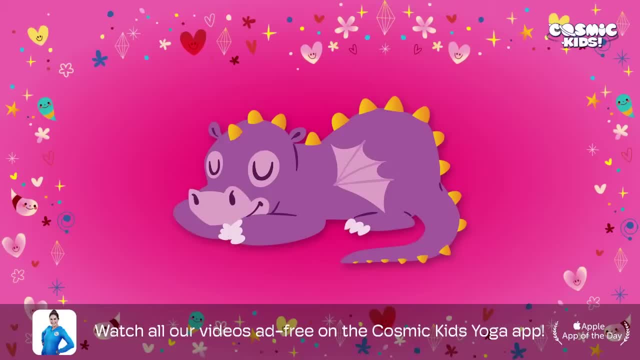 she just felt better in herself, somehow More, More in control of her feelings. Doug was so proud of his little dragon baby girl. She climbed out of the bath and he wrapped her up in a towel, hugging her tightly While she changed into her pyjamas. 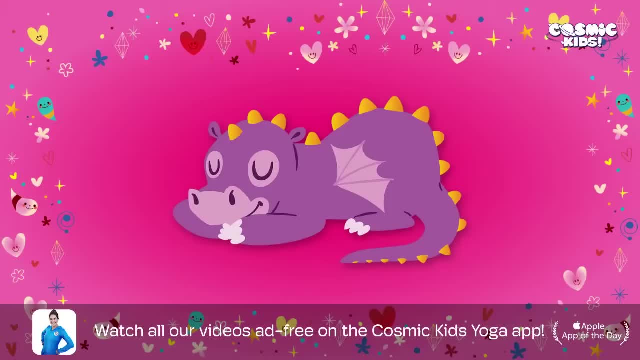 Doug quietly shared Dina's news with Dina's mummy, Delilah, who was just as proud and relieved that their daughter was going to be okay. That night, Dina snuggled up in her mossy, squishy bed. 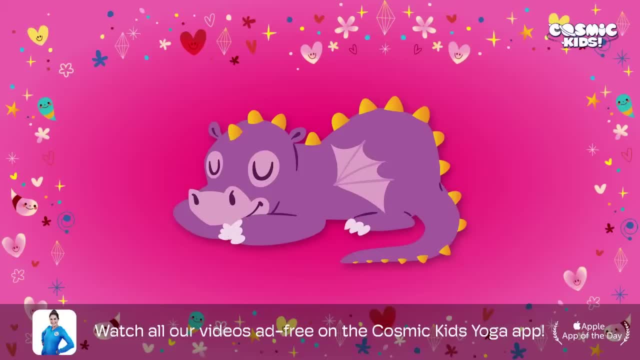 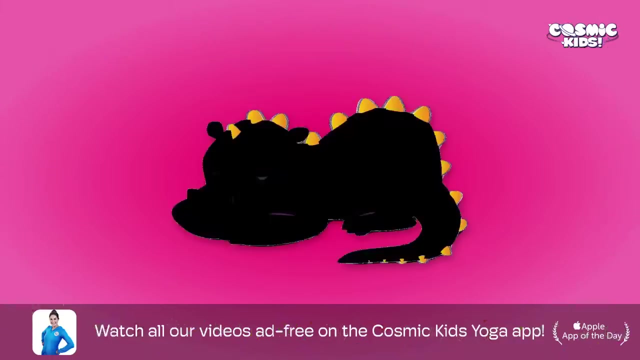 with her new pillow, feeling ready for a sleep. Nowadays, she looked forward to sleeping, as she felt stronger every day when she woke up, And that was the time she chose to do her breathing exercise Every morning. Let's find our sleeping dragon position now. 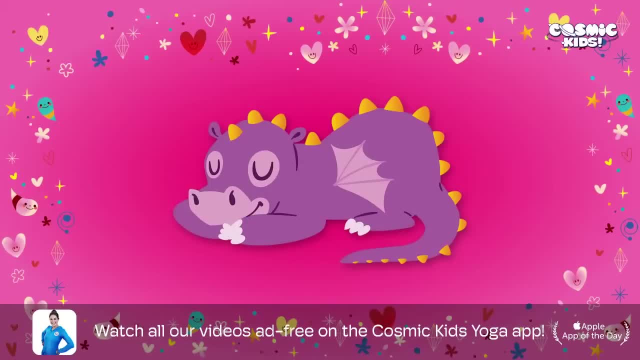 Let's find our sleeping dragon position now, With our body relaxing, Our legs, arms, Our face, Our long back And tail. if we're being dragons, Relaxing And getting heavier And heavier As sleepiness begins With each breath out. 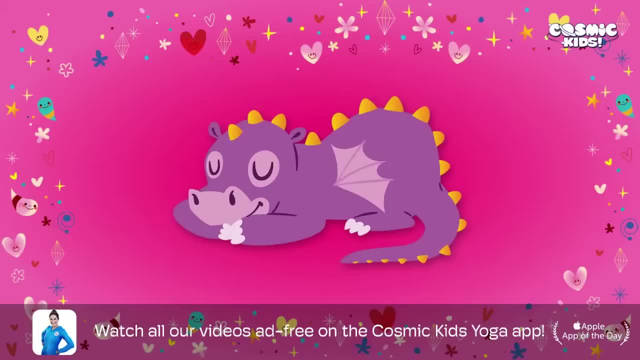 Little wisps of smoke puff from our noses. Another day, Another day, Another day. learning a bit more about ourselves comes to a close, and the night wraps us up in a cloak of stars, resting easy like a sleeping dragon, if now is sleep time. 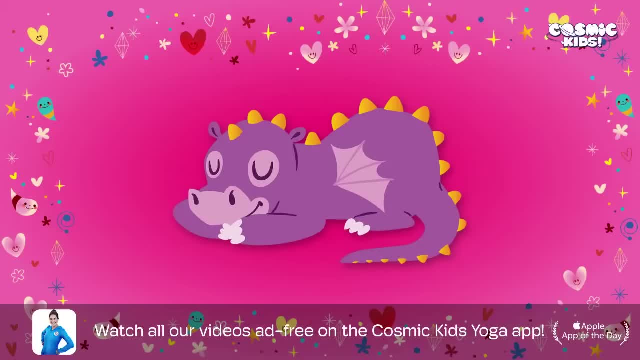 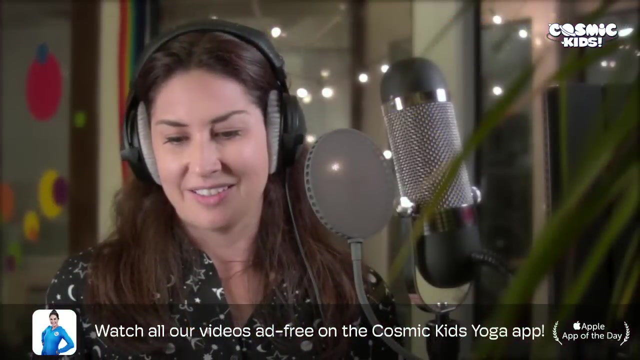 then I wish you a good night. if it's not time for bed yet, then slowly start to come back, deepening your breath, wiggling fingers and toes. take a nice big stretch and slowly gently open your eyes before you move anywhere. notice and enjoy the way you feel now. 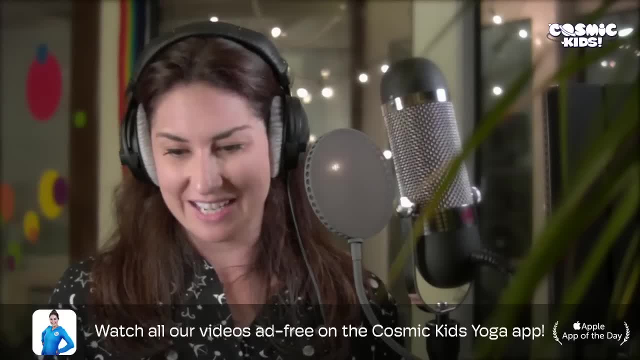 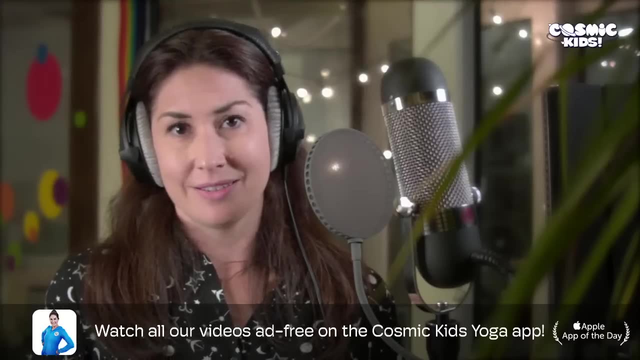 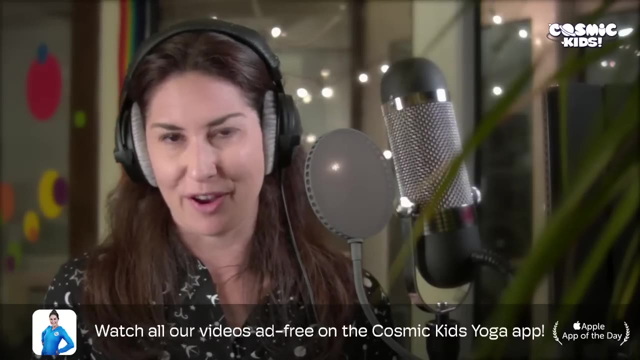 I hope you enjoyed the story of Dina the dragon and, if you notice those big angry feelings taking over sometimes, see if you can take a few deep breaths in the moment, step back from the fiery feeling and maybe even try that little daily breathing exercise that works for Dina. 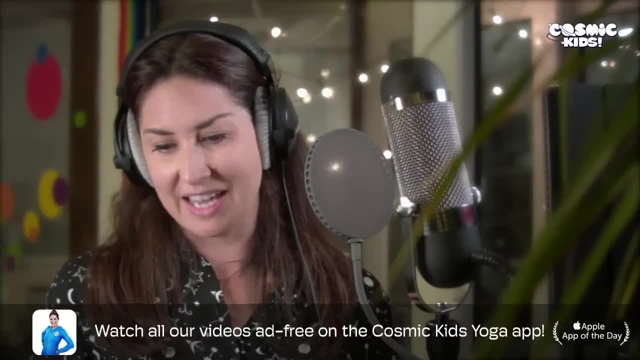 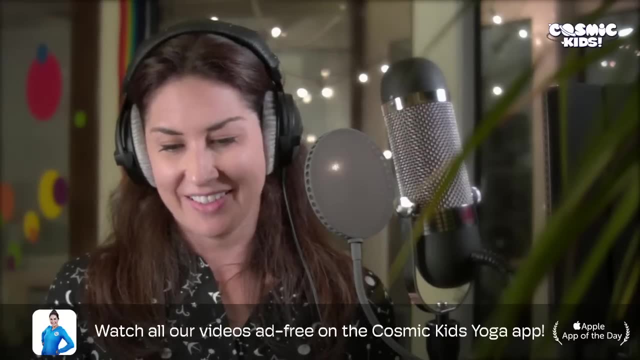 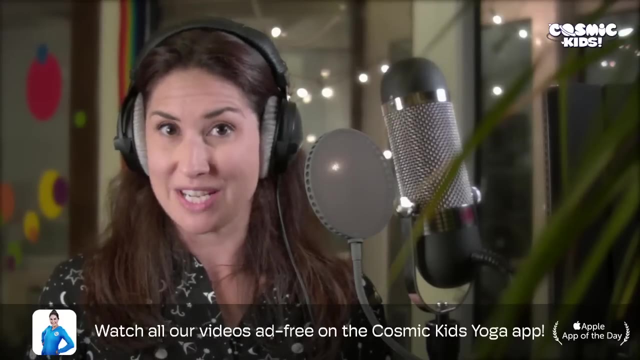 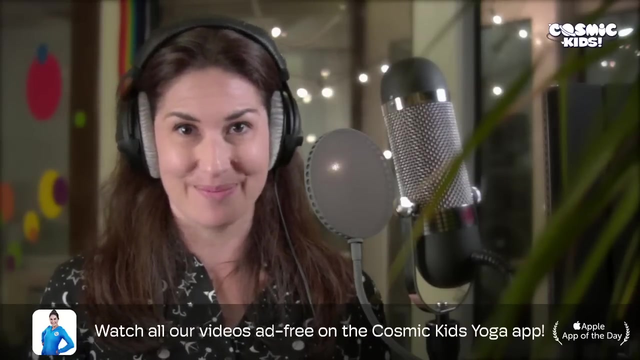 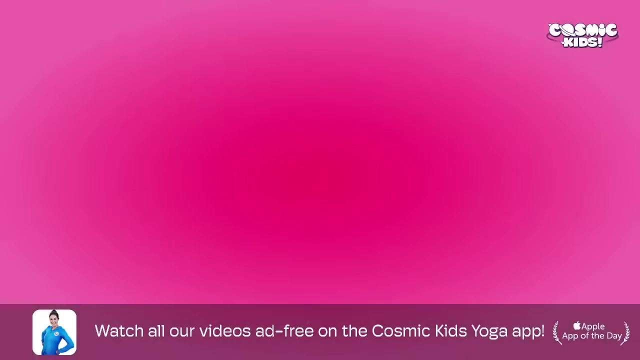 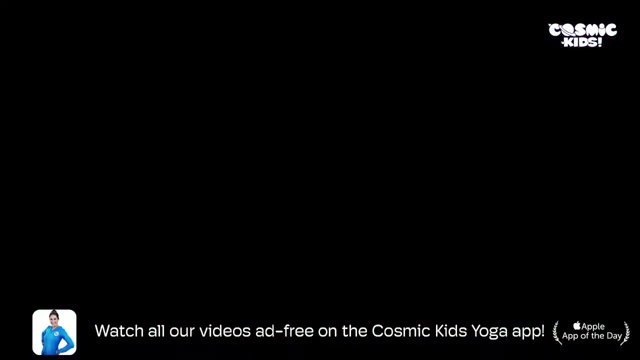 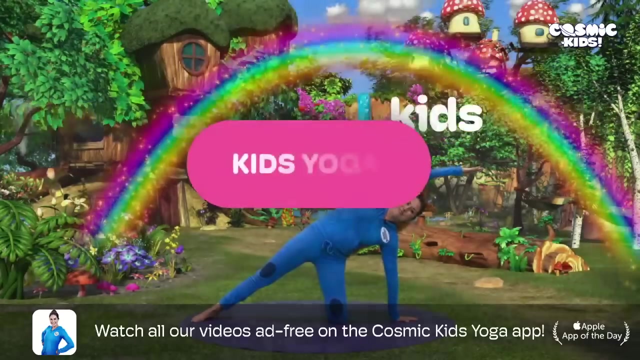 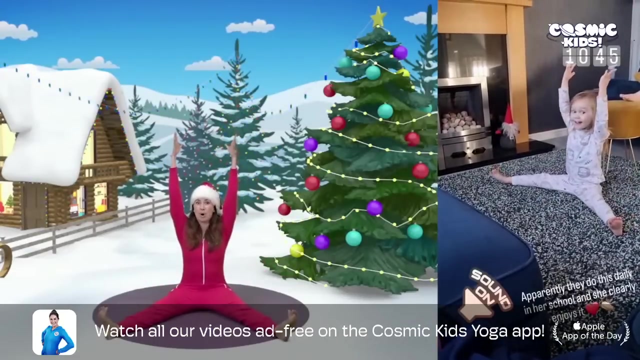 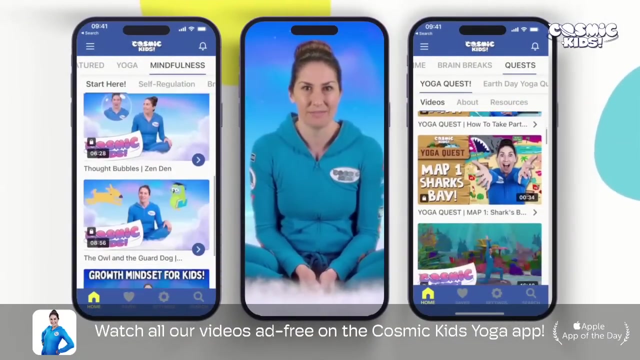 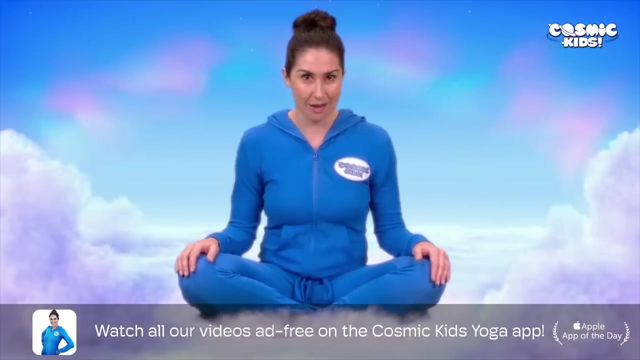 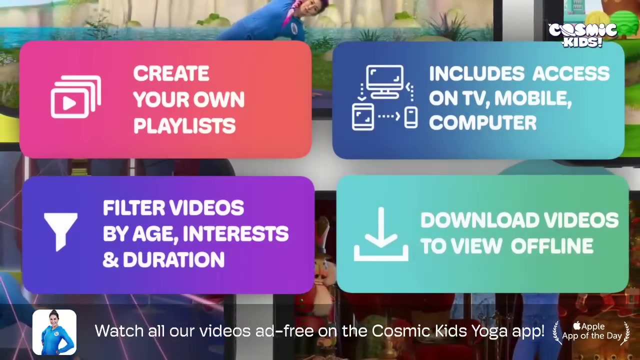 spending a few moments every day, simply closing your eyes and then and breathing just like anything. the more we do it, the more easy and natural it becomes, plus, your body and mind will love it. well, done you for spending this time. this is Jamie, saying peace out and until next time. 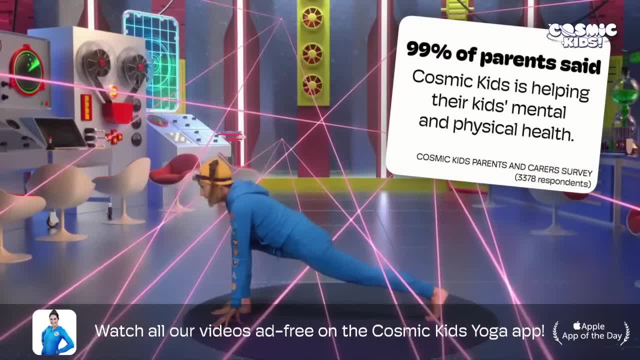 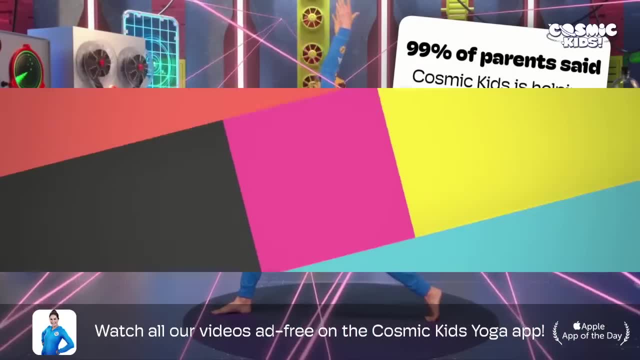 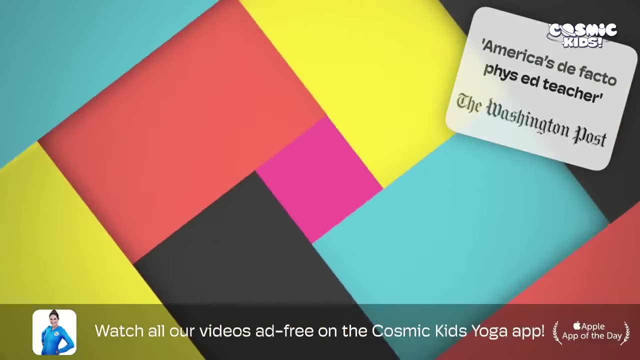 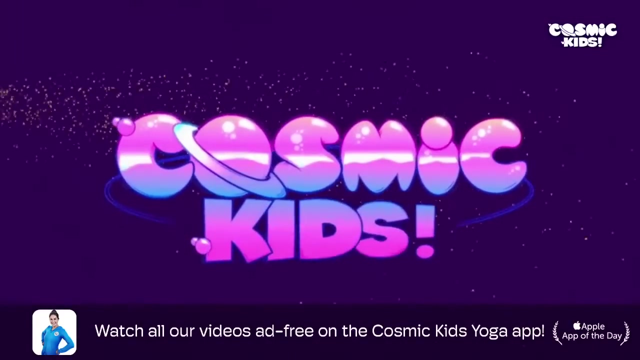 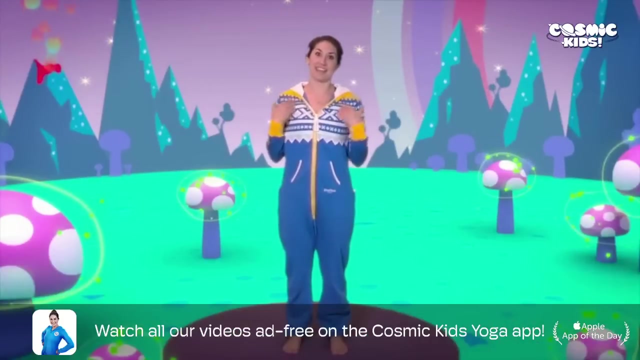 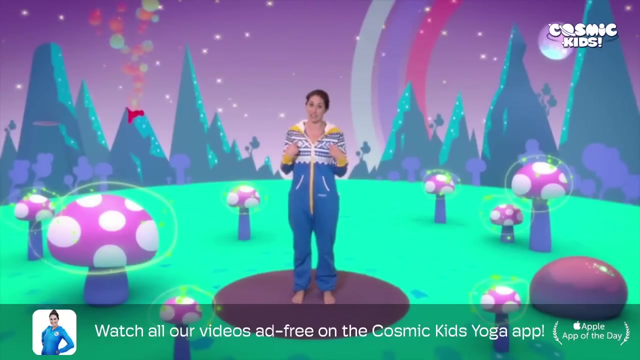 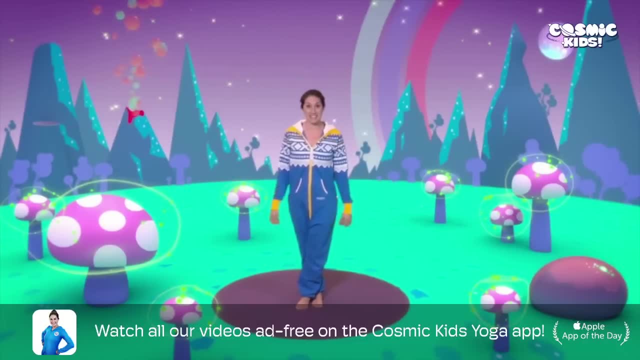 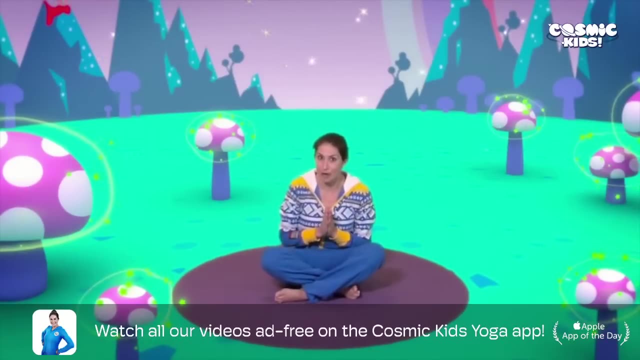 begin in the same position, and that's by crossing our legs, sitting on our bottoms and bringing our hands together at our hearts and saying our secret yoga code word, which is: Namaste Ready After three, One, two, three, Namaste There, Now we're ready to begin, and 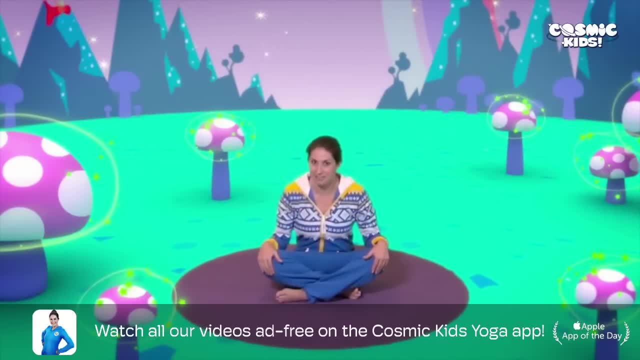 today we're off to meet Cracker, who is a dragon. So it's a story of wonder, and we've got to journey to another world, the wonderful world of Whiz. Oh, Here comes our magic carpet. Let's take our legs out super wide and our arms out wide. 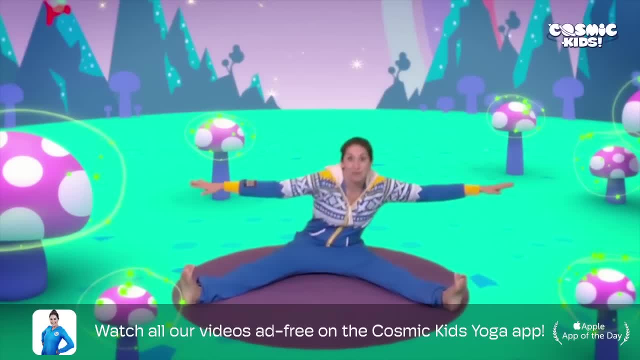 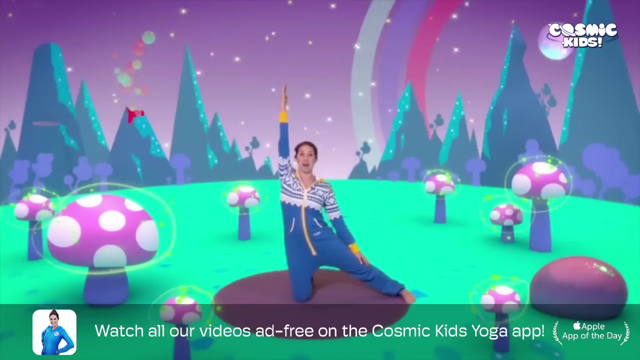 as well. We begin to go around As we take off in our magic carpet up to the sky and down through the valley. we go through a magic door, Coming up onto two knees. take your leg out to the side and lift your arm, Opening the door. we go through Bringing your knees 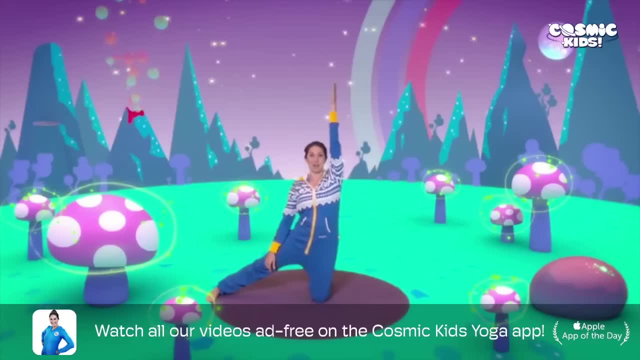 out to the other side now and your other arm to the sky. We close the door behind us. Here we are, everyone in the wonderful world of Whiz. How exciting. The trees are amazing. They're made of feathers Standing up putting one foot on top of the other. Bring your hands. 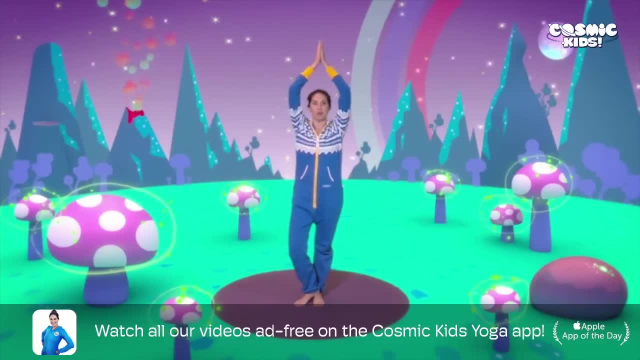 together at your heart and grow your tree up tall. Now, lots of beautiful feathery colours here. What colour is your tree? Oh, I like that colour. That's lovely. Let's swap our feet over now, Putting your other foot on top and bringing your hands together at your heart, Growing your tree up tall and. 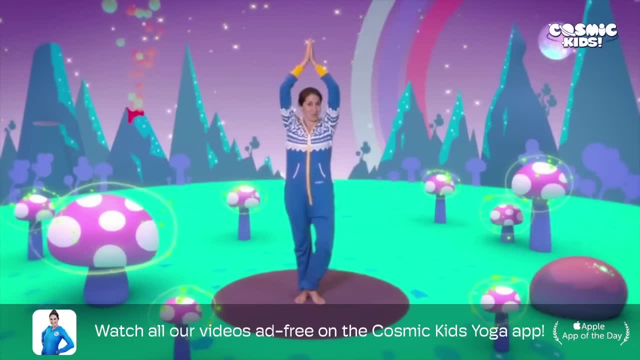 are you feeling like a strong tree today, I wonder? Let me see if I can blow you down. You stay still and I'll have a go Ready. Oh, my goodness, You're still standing up. You are a strong tree. The sky is huge in Whiz and full of the most beautiful and huge stars. Jump your feet wide. 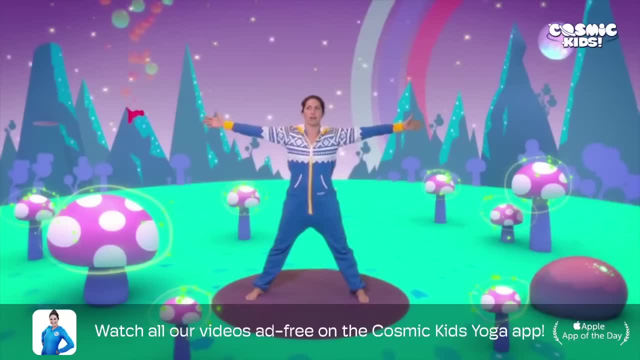 and your arms wide. We can hear something. We rub our ears. The stars are singing, Criss Cross your arms over your shoulders and Twinkle, twinkle little star. How I wonder what you are, How amazing. We're all changed. 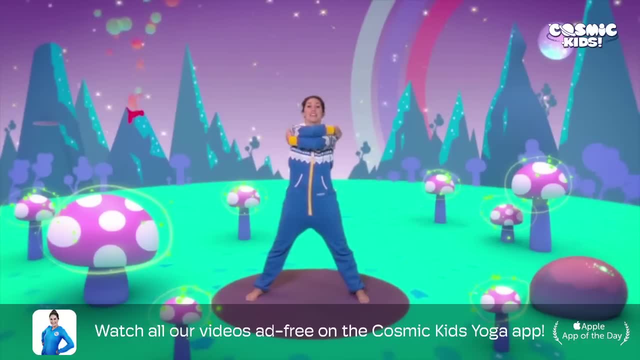 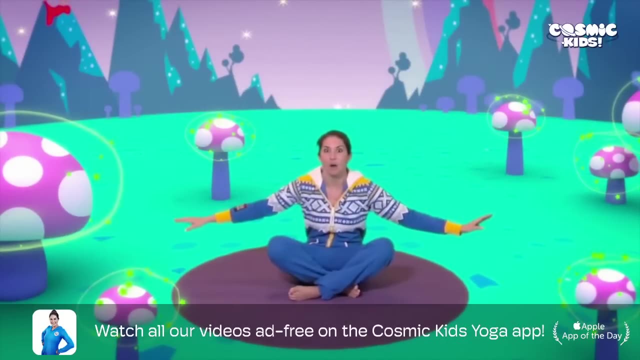 the stars singing whizz. We land cross-legged on our bottoms. Whoop, Goodness me. look at this amazing world. We hear funny footsteps, big, clumpy footsteps. Take your legs out nice and wide and hold on to your ankles- They go. 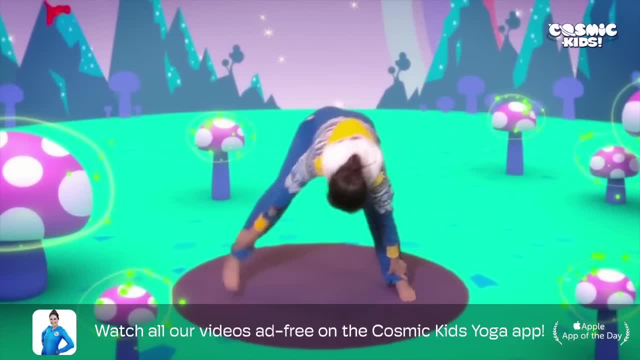 clump, clump, clump, clump, clump, clump, clump, Quick. everyone we better tuck up into a tiny little ball and hide Coming down onto your knees, tuck yourself in The footsteps, stop. just in front of us. We sit up and see the most amazing. 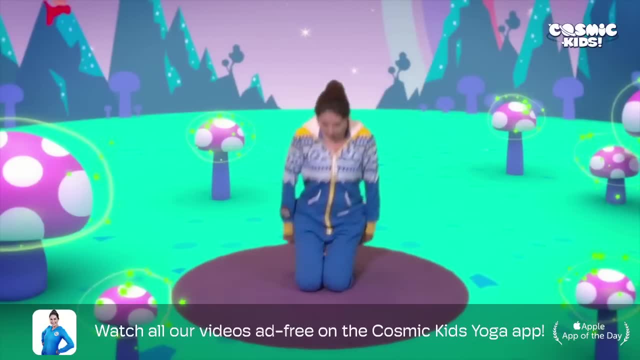 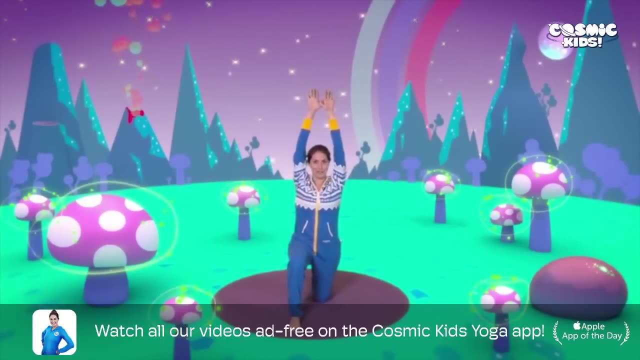 dragon in front of us, Coming up onto one knee, tie your thumbs together at the top and wiggle your fingers. The dragon bows very deeply and says: Hmm, Hello, my name is Cracker. I am the dragon of wonder Swapping your legs over now coming up with your other knee bowing again. 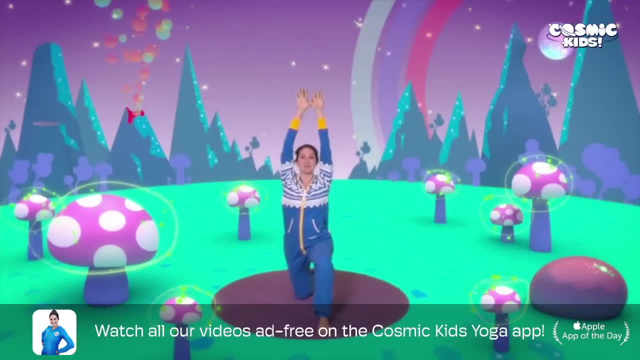 Everyone this year. I am the firework dragon and you must be my helper. Come on, we've got lots and lots of work to do. Wow, a real dragon. We can't wait, Let's get cracking. We hop onto Cracker's back. 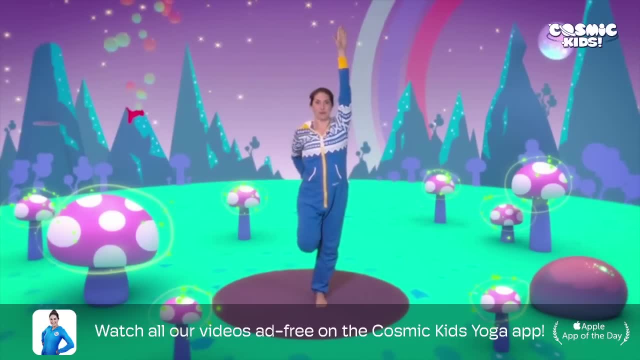 Lifting up one arm, holding onto your foot and trying not to wobble. Now we go on with the other leg, lifting up the other arm, lifting up the other foot and, yes, we're on Bending all the way forward. Cracker spreads his big, beautiful dragon wings and we're off flying. 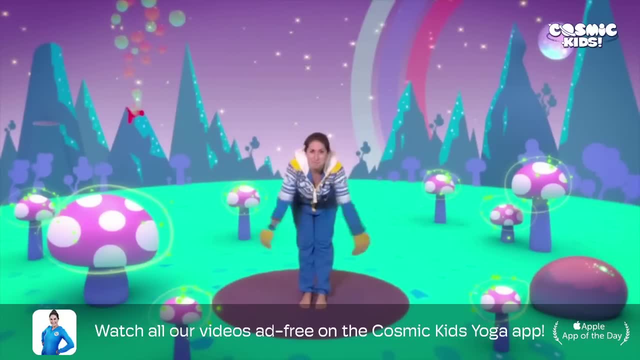 up into that beautiful star washed sky. It's amazing looking down from up here: The feathery trees, the amazing mountains. What a place, isn't it? It's a beautiful place, isn't it? It's a beautiful place, isn't it? 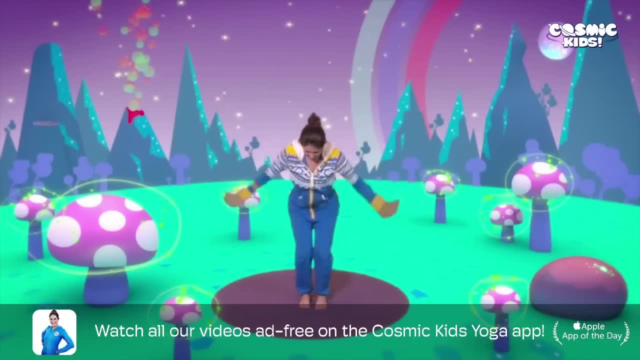 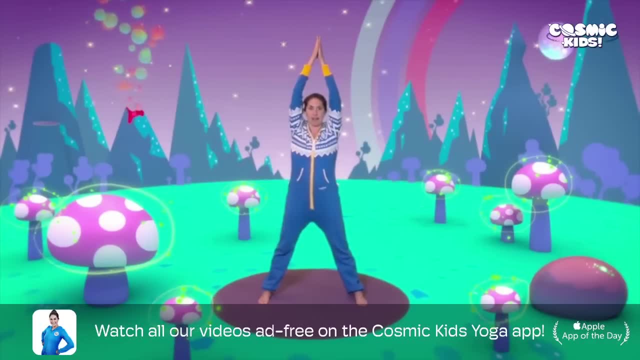 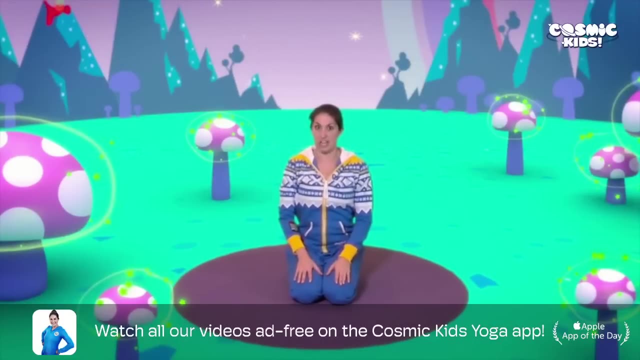 head Now. it's very dark inside this cave and full of scary shadows coming down onto your knees. Some of the shadows look like lions- One, two, three. Some of the shadows look like tigers, coming onto all fours. Claw your tigers. 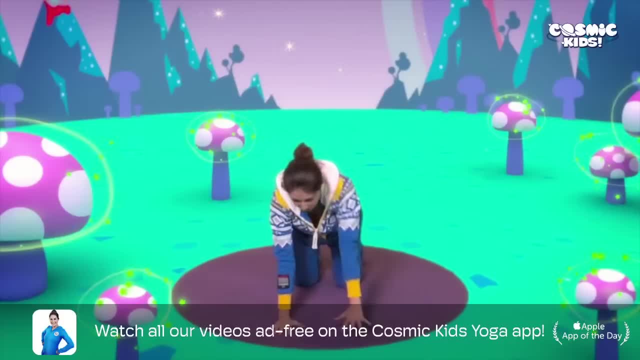 tiger paw and claw your tiger paw and swish your long tiger tail. Now, sometimes we might be afraid of the dark, but here with Cracker, we're not at all. We're really excited. and the shadows aren't scary at all, They're really interesting and amazing. Cracker explains. 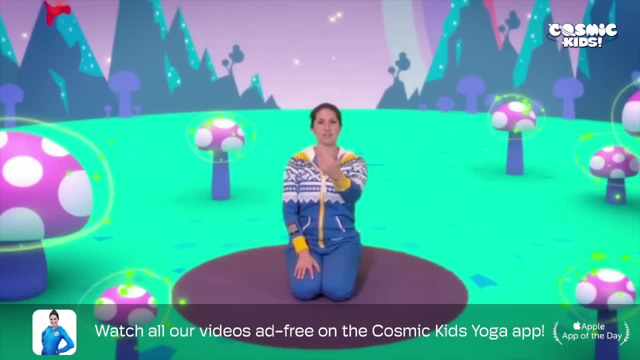 that to make the fireworks we need some ingredients. We need colours, sounds, magic and shapes. Right, we can't wait, Let's go. First stop is the Whizbang Pop Shop to get the sounds. but we've got to tiptoe through the tulips, Coming up onto your tiptoes, crouching lifting. 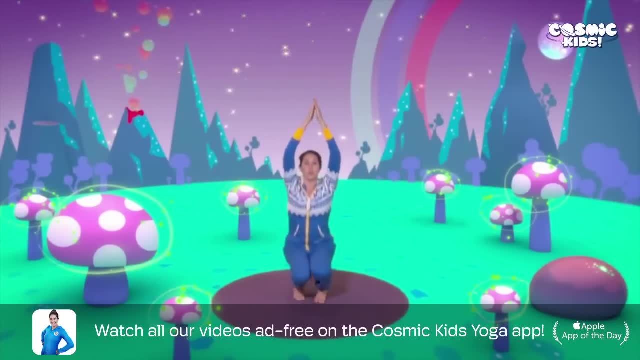 your hands above your head, Come and tiptoe through the tulips with me. We end up in the Whizbang Pop Shop, which is incredible. It's like a big, squishy, giant bouncy castle. We boing, boing, boing, boing, boing and bounce around, and all over it are floating lots of 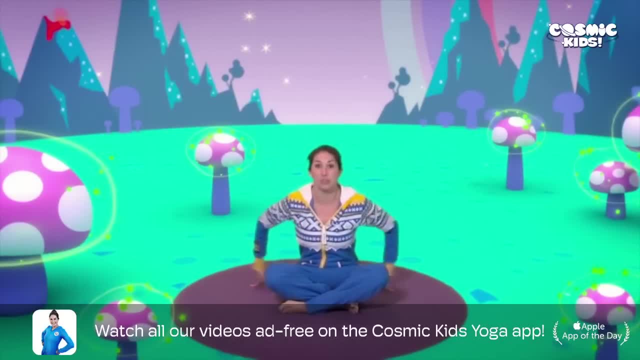 amazingly huge balloons sitting on your bottoms. Take your arms out wide and float around like a big balloon. Cracker explains that in each of the balloons is the sound for the fireworks. Wow, we can't wait to check this out. We twist this way and pop this. one Pop and it goes. 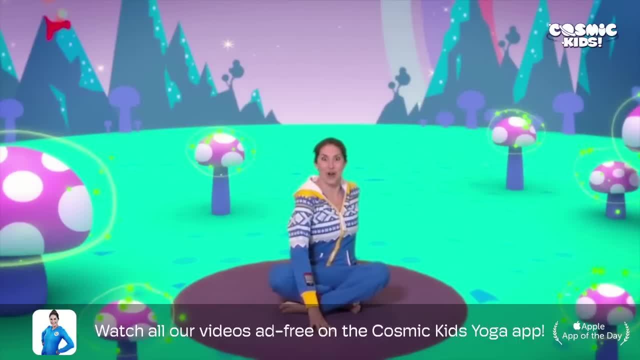 bang, Wow. Let's try another one. We twist the other way and we pop. this one Pop and it goes wee. This is incredible. We get all the sounds we need from all of these amazing balloons and we're off to the next stop, the Rainbow Roller Coaster for the colours Coming. 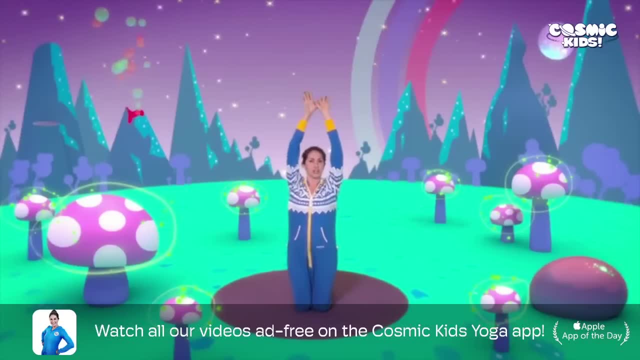 up onto your knees. Cracker says: let's get on. So we get on. We lift our arms up and pop, pop, pop, pop as the rainbow climbs up and over. And then we whoosh down really fast. We go over to one side- Wow- And over to the other side. Then Cracker shows us how. 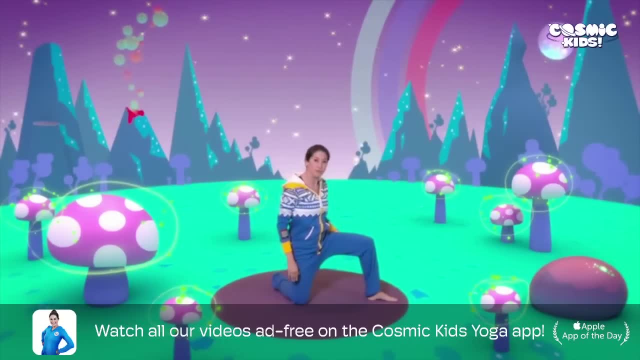 to surf on the Rainbow Roller Coaster, putting one foot forwards and one foot back, Cartwheel our arms around and whoosh, This is great fun. We even do it the other way. Whoosh, Whoosh, What a ride. At the end of the rainbow is a ginormous pot Lying on your tummies, flick. 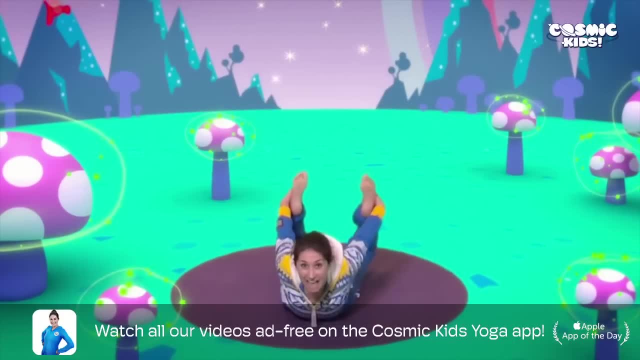 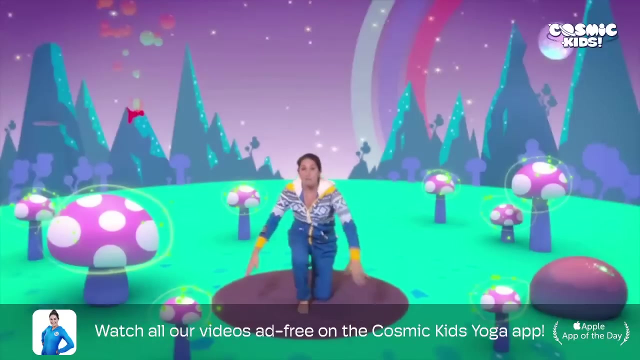 your feet towards your bottom and take hold of your ankles and lift yourself up. The pot is swirling with the most beautiful vibrant colours. We've got all the colours we need here for the fireworks. Now for the shapes: It's up on Cracker's back again and we're 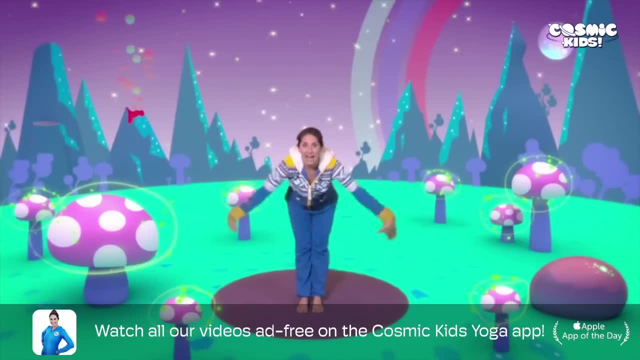 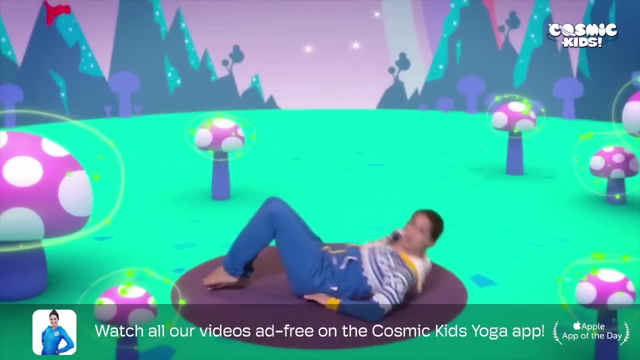 flying up into that beautiful sky towards the cloud. Now, every cloud is a different shape. Some of the clouds are like candles, All tall and straight, Lifting up your legs lying on your back. Some of the clouds are round and spinny. 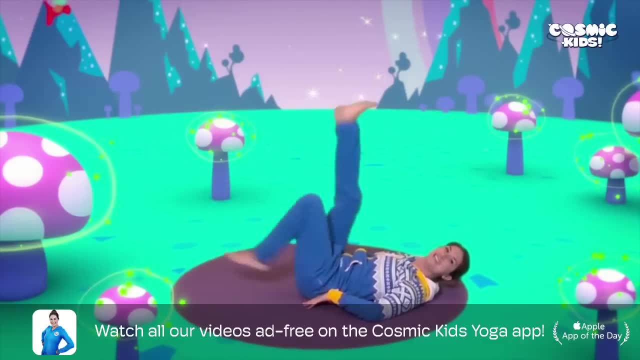 like wheels, Wheeeee, And some of the clouds go whiz, pop, whiz, pop, whiz, pop. Wow, We've got all the shapes we need here. We collect them all and off we go. We get back to Cracker's cave where we mix all the ingredients together, Taking your 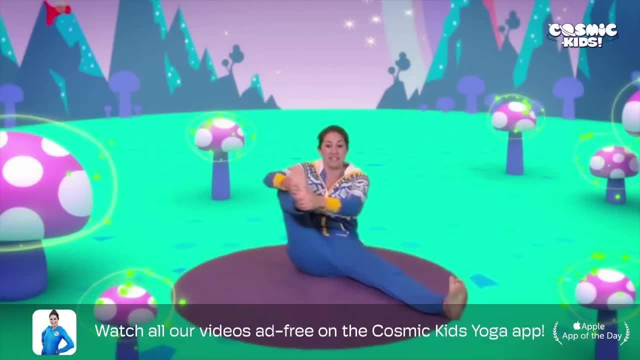 legs out wide. we take the special stick and we stir it, stir it, stir it. That's all the sounds. Now we take the other special stick and we stir in the colours, Stir it, stir it, stir it And finally, taking both together, we stir in the shapes, Stir it, stir it, stir. 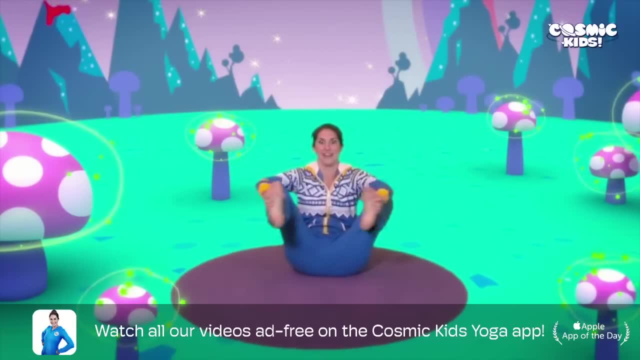 it Now for the magic Legs out wide. sprinkle in your magic and make your special firework wish. Hands together, One, two, three. Cracker breathes his fire into the fireworks. And now it's time for the big test. 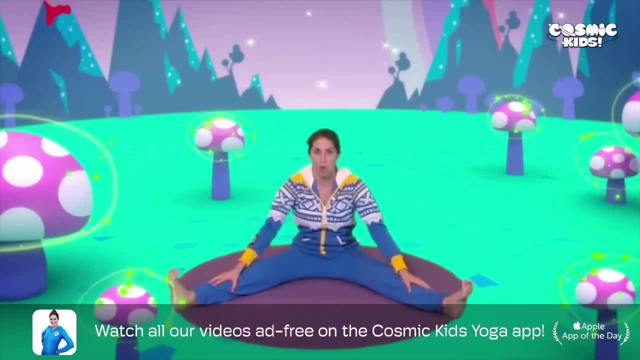 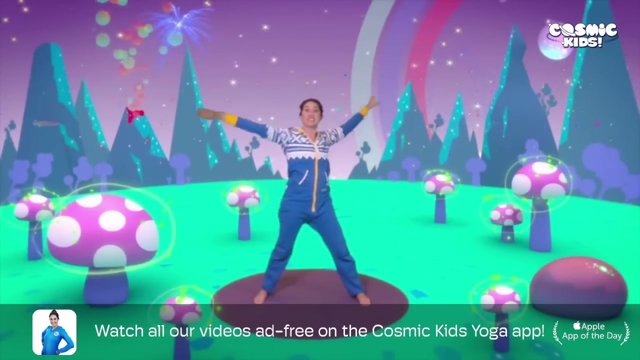 Big test everyone To see the fireworks working, Coming into a little crouched position. let's count down from five and keep very still. Five, four, three, two, one, Whoosh, Wow. The colours and the light and the sound and the shapes are amazing. We look up and we are. 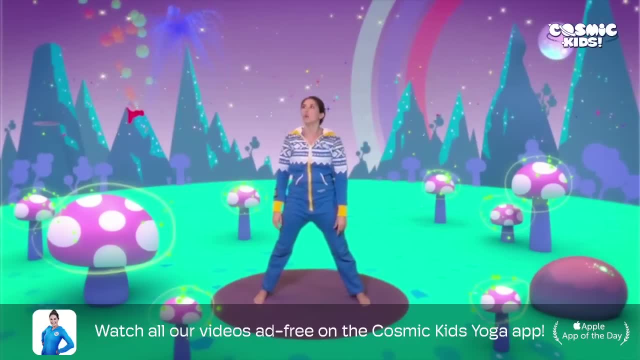 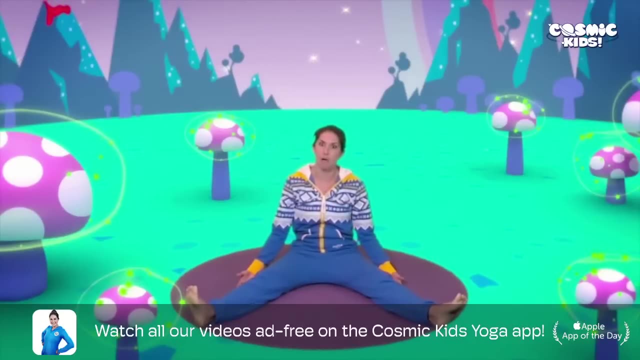 full of awe and wonder, We float back down to earth, and when we sit down on our bottoms, we find we are sat in our own beds. We're not ready to say goodbye to Wiz and Cracker, though yet, So we lie ourselves down and we close our eyes, and we are back there in. 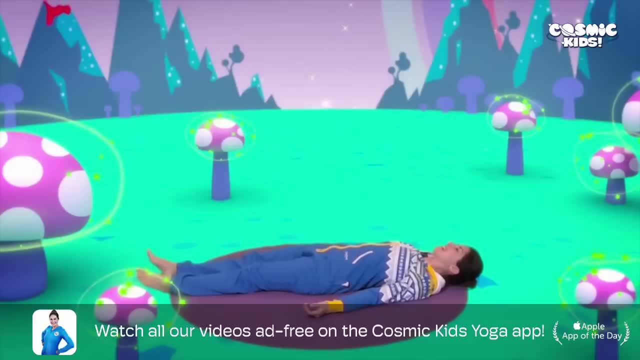 that wonderful, beautiful sky With the stars that sing, That zoom And jej, And those beautiful fireworks that fill our minds. What an amazing adventure. With every breath we glow a little bit brighter, Like a brighter firework. Thank you, cracker. What a great adventure. 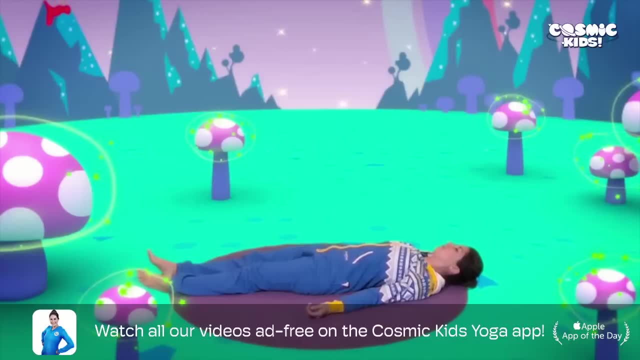 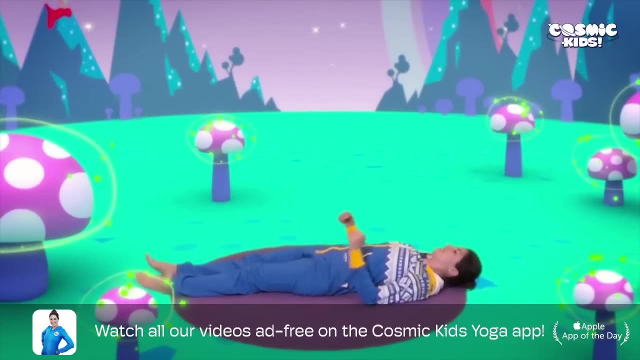 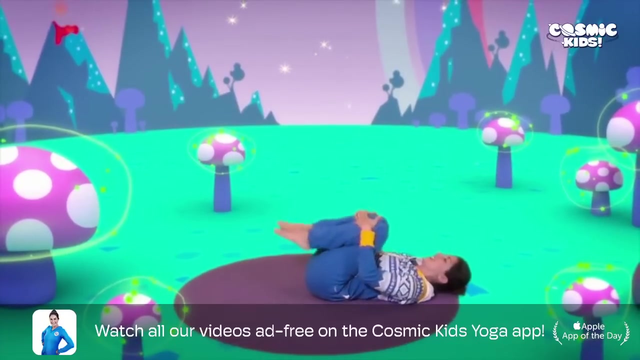 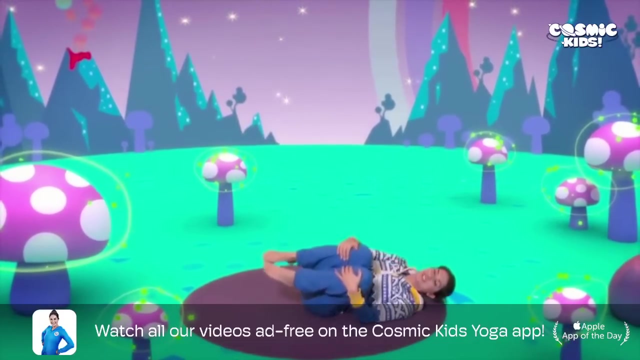 We flicker our toes, We flicker our fingers, We stretch up nice and tall And we bring our knees into our chest and have a little cuddle with them. We roll over onto our side and come up to sitting with our legs crossed. 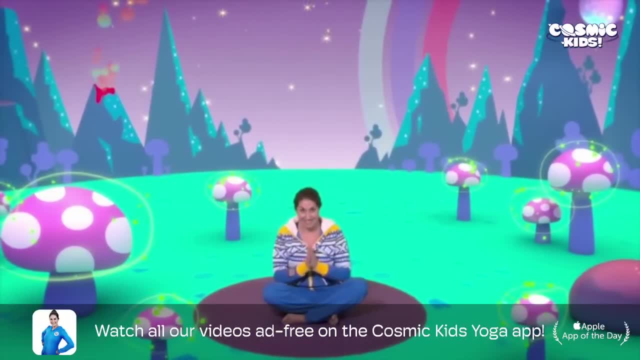 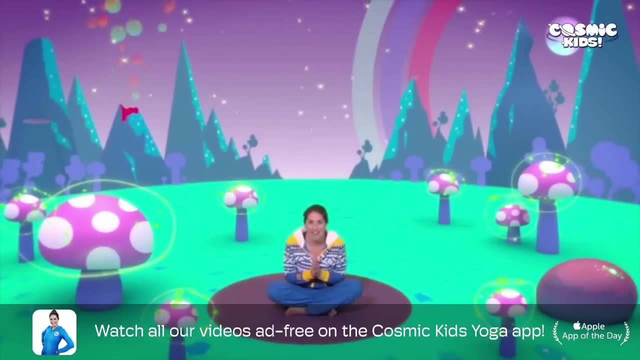 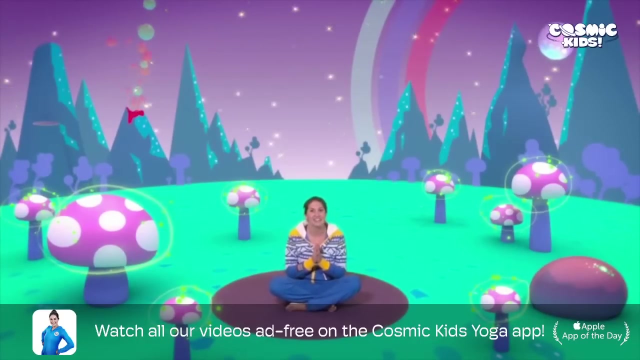 Just in the way we started With our hands together at our hearts And we finish with our special magic yoga code: word: Namaste, Ready After three. One, two, three, Namaste. Well done everyone. That was amazing. Thank you for coming to whiz with me and for meeting cracker. 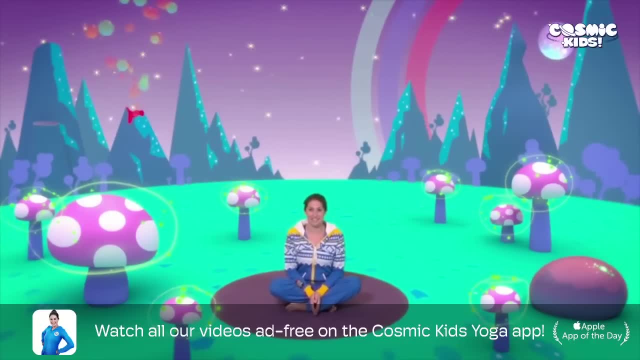 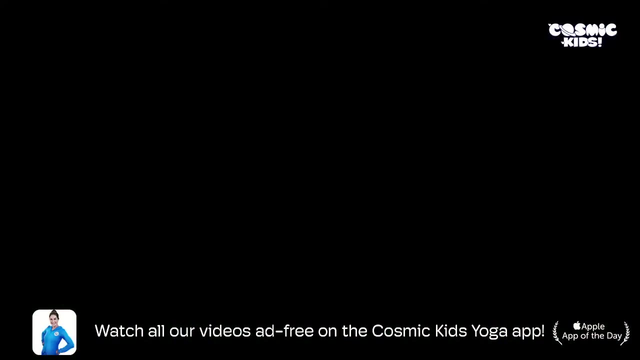 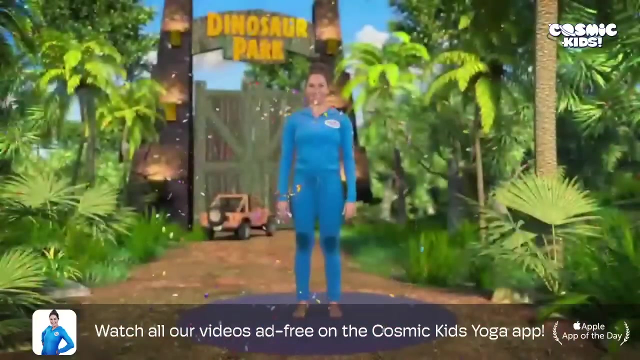 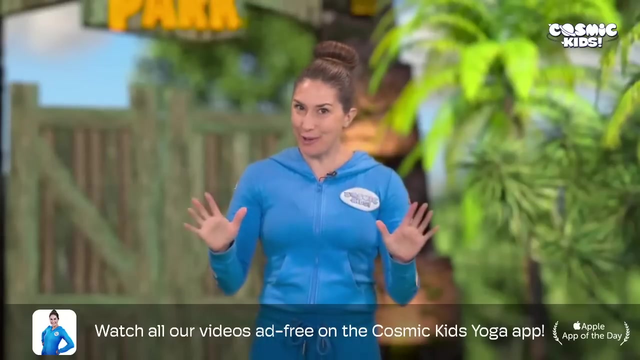 He loved it. I hope to see you again for another Cosmic Kids adventure. Bye-bye, Hello everyone. Welcome to Cosmic Kids. I'm Jamie and this is your place for yoga, stories and fun. It's easy, Just copy the moves I do. 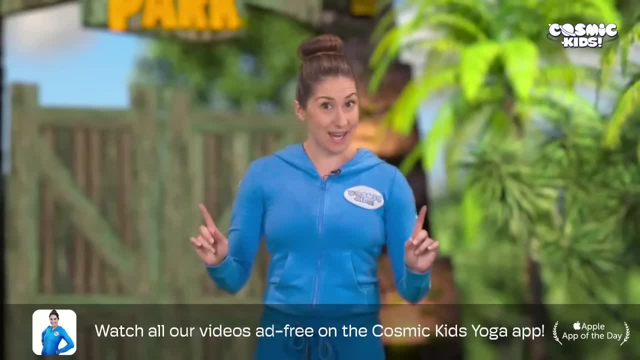 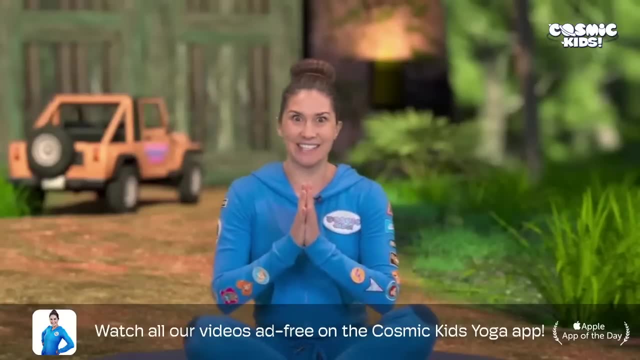 And enjoy the adventure. Now. we always start in the same way, And that's by sitting on our bottoms, crossing our legs and bringing our hands together at our hearts And today saying our secret Jurassic dinosaur yoga code word, which is Namasaurus. 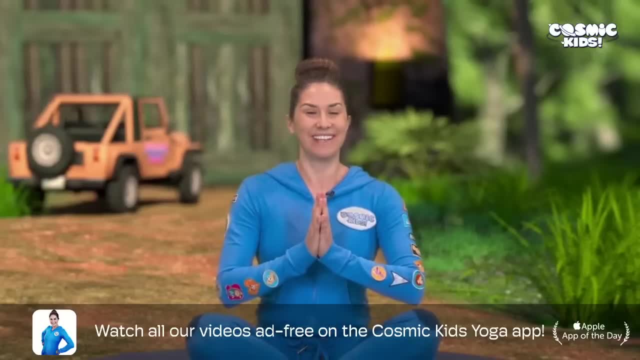 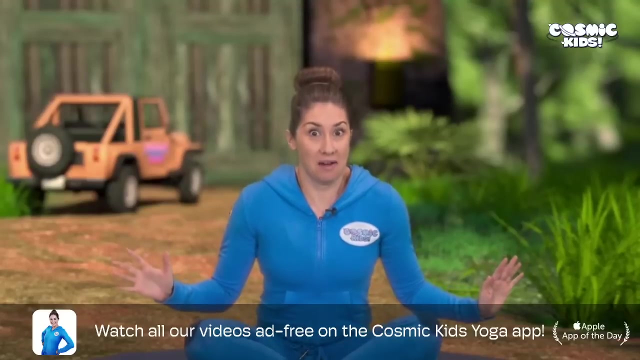 Ready After three, One, two, three Namasaurus There. Now we're ready to begin And, as you can see, we're in a rather special park today where we might meet some dinosaurs. I'm sure we'll be okay. Apparently, it's very safe. 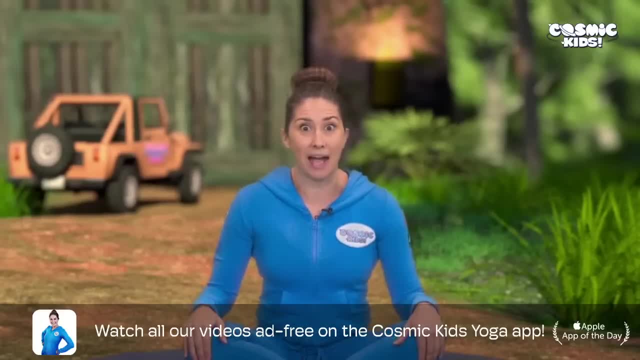 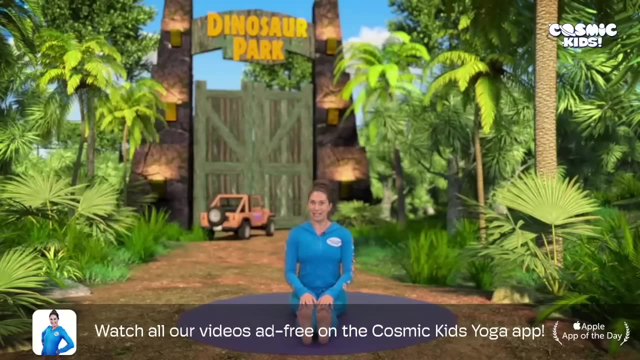 Before we go in, let's begin by packing ourselves a backpack with everything we need for our visit, Taking our legs out long in front of us, Wiggling our toes a little bit, Bending our knees and touching our toes. We open up our backpack by lifting our arms. 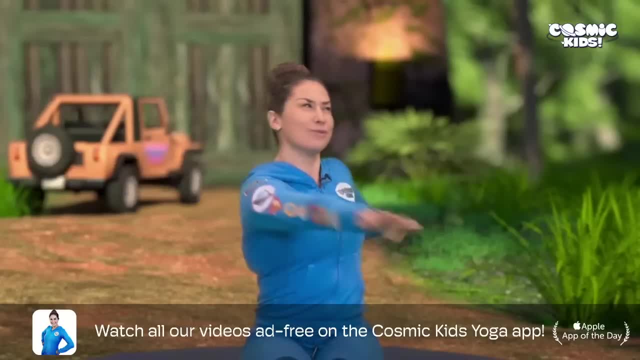 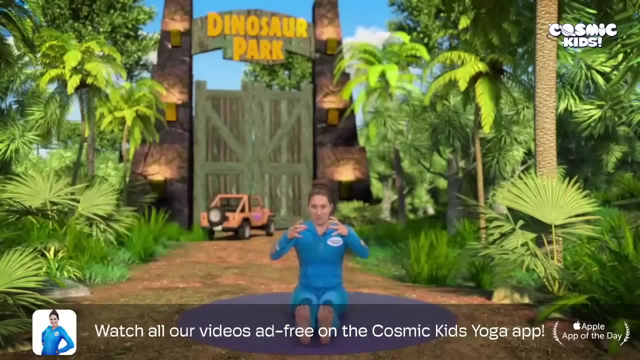 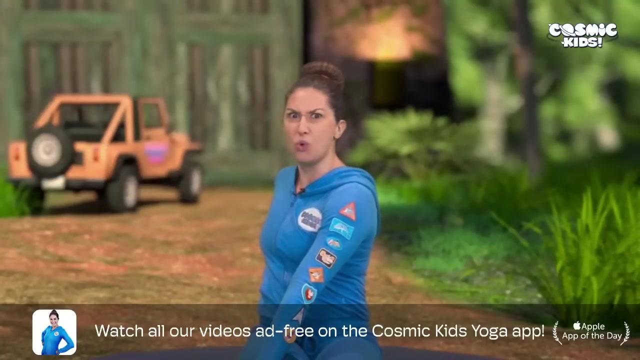 We take our arms out nice and wide and we twist one way to get ourselves some sandwiches: Getting our sandwiches, bringing them to the front and let's wrap them up. Wrap up the sandwiches and pop them in the backpack, Arms out wide again. We twist the other way now and we get ourselves something nice to drink. 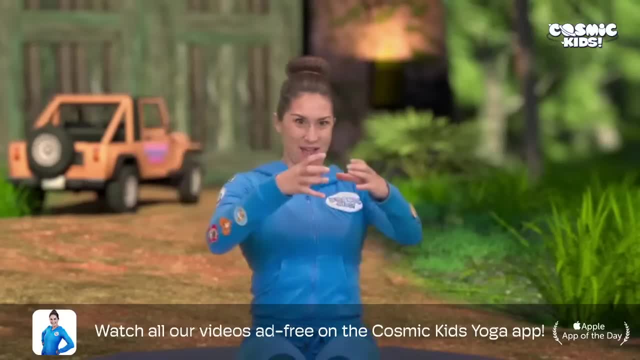 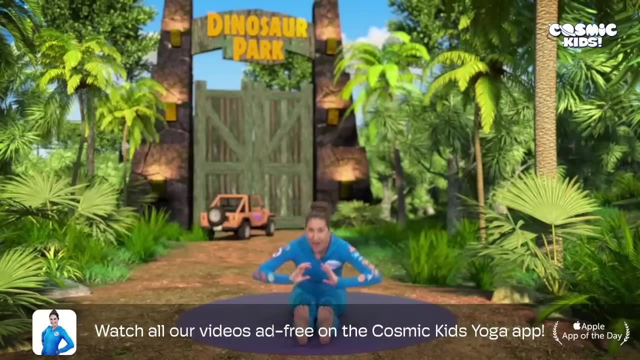 Some water. You can't go wrong with water. Get your water, Bring it to the front, Check the lids on And pop it in the backpack Arms out wide again. We twist the other way now and we get ourselves some binoculars. 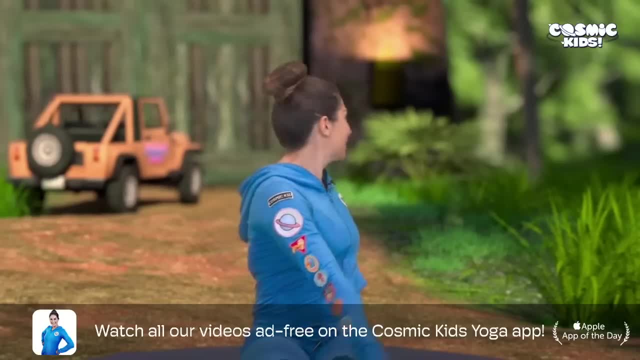 We might want to see the dinosaurs close up from far away. So we get our binoculars, Let's check they work Joining our thumbs and fingers together, Pop them on. Oh look, you're very close up when I pop these on. 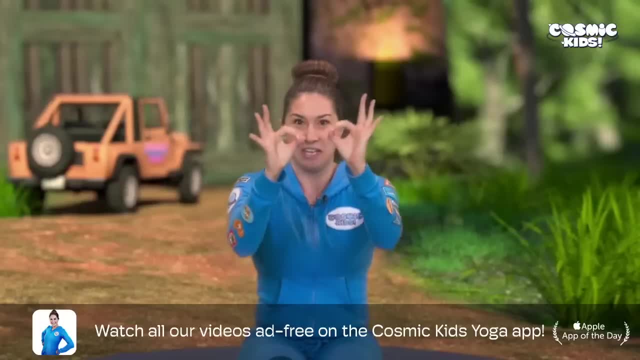 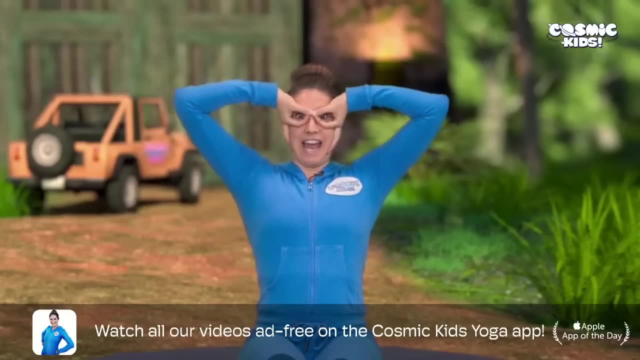 Let's see if we can put them on upside down. And what happens then? Turning our hands upside down to pop them on our face the other way. Oh, you've gone really far away. now Let's put our binoculars in our backpack. 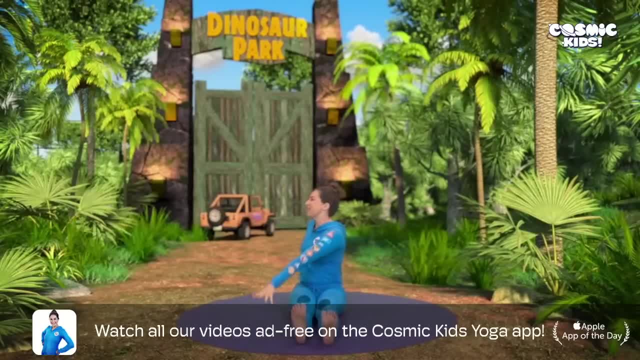 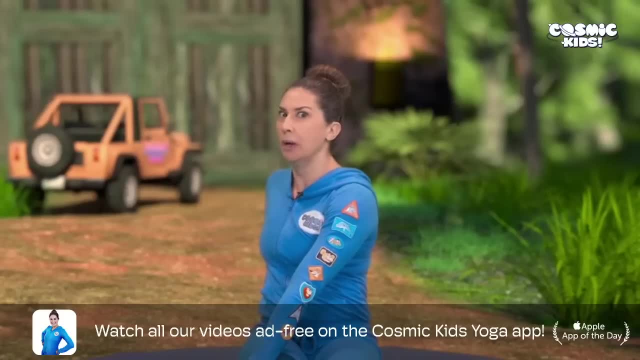 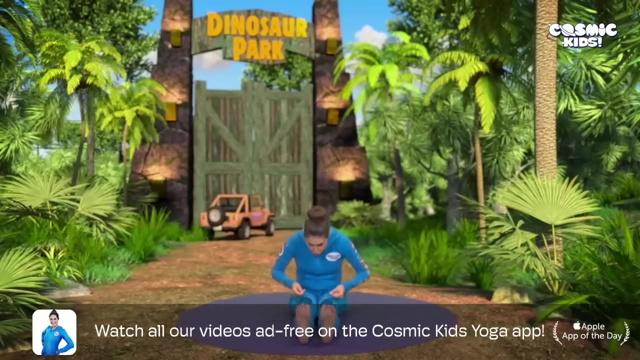 Arms out wide again, We twist the other way and let's get our emergency escape card, Just in case we want to go home quickly. Getting our emergency escape card and putting it in the little zip in the top, There we go, Reaching our arms up high, Bending our knees a little bit. 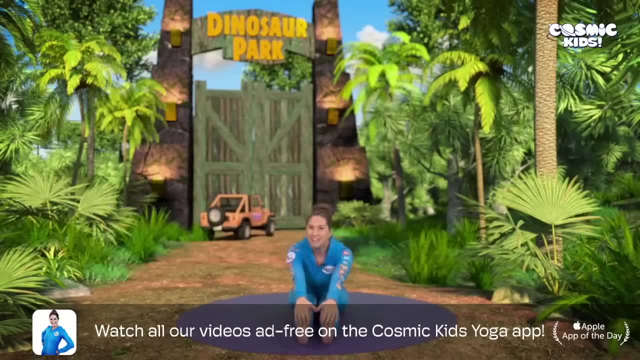 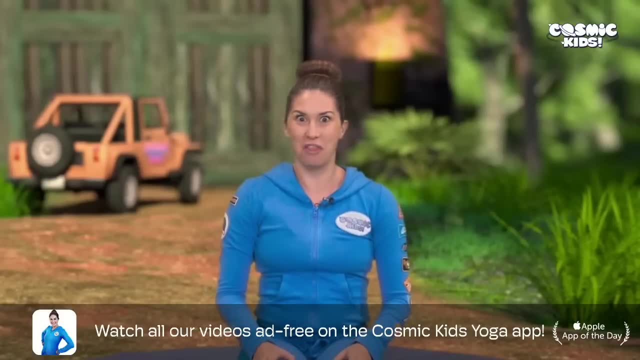 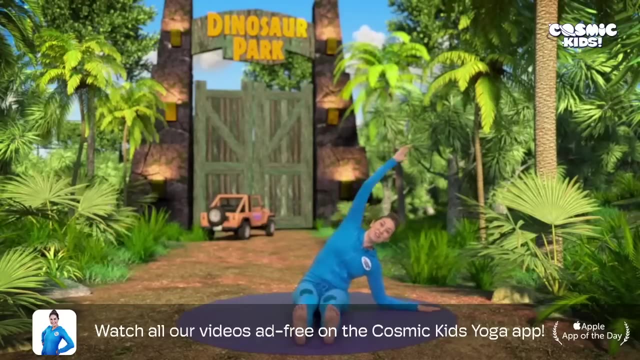 And folding forwards to close our backpack. Very good, everyone. Now let's take a ride in the Jurassic Jeep and go into the park. Let's start our engines. We're going over to one side. We're going over to the other side. 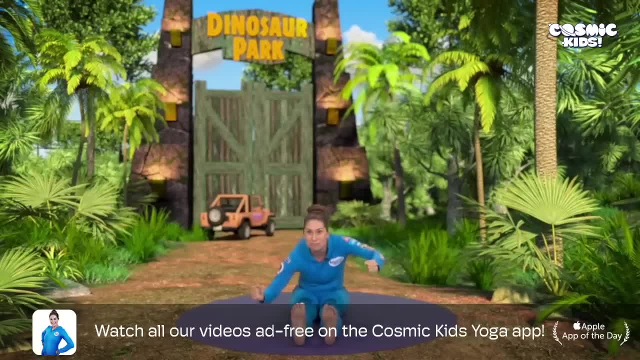 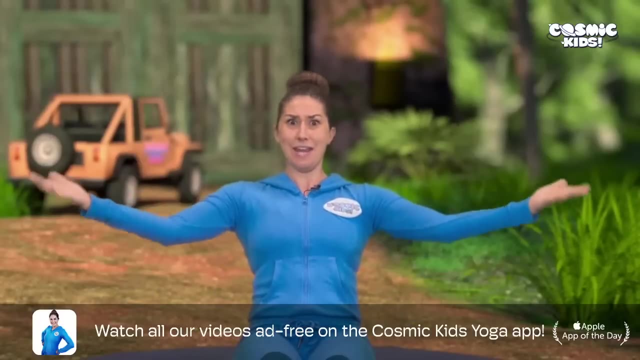 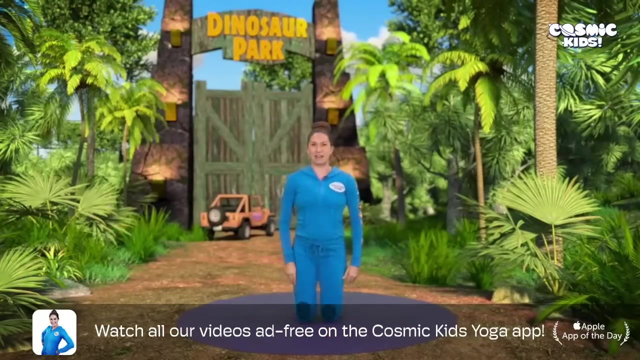 We're going down the hill, We're going up the hill, We come to a stop and we've arrived at the most majestic, enormous gates. Let's do our gate pose. Coming up onto two knees everyone. We take one leg to the side and our other arm to the sky. 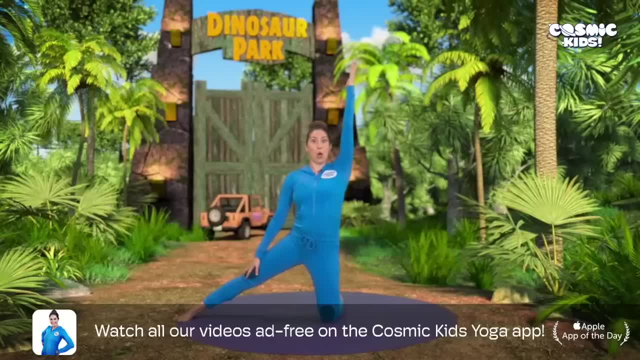 Now we open up one gate, leaning to the side, Coming all the way back to centre. Now we need to do the other side, Two knees together, Leg to the other side, Arm to the sky, And let's open up this side. 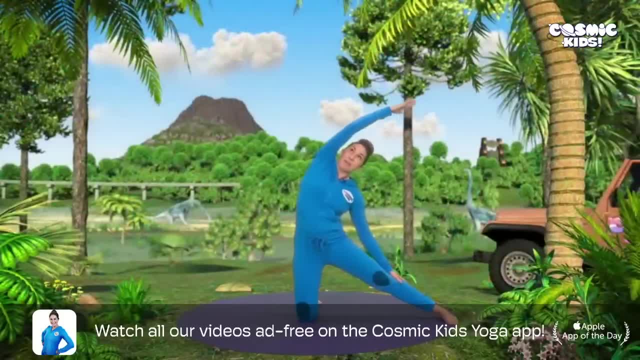 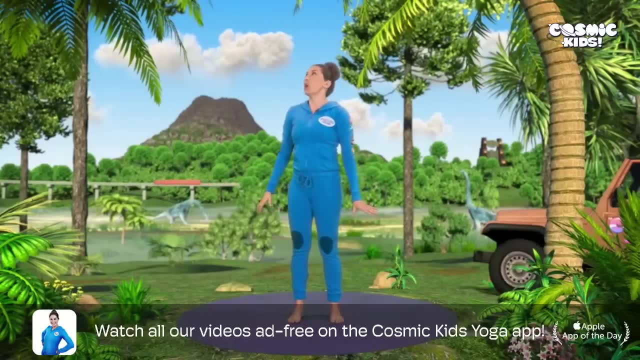 Wow, Look at it inside, Coming all the way up to centre and all the way up to stand. Wow, It's so lush and green in here. It's amazing. Can you hear that, Giving our ears a rub? Goodness me. 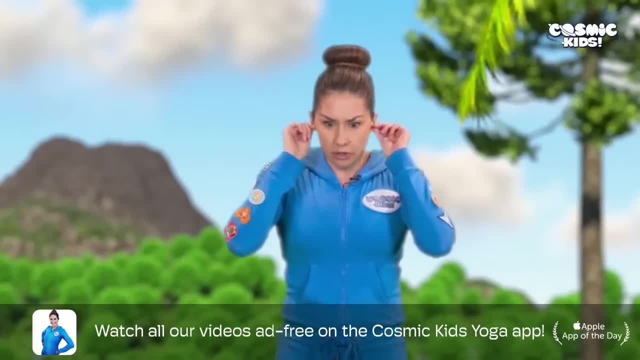 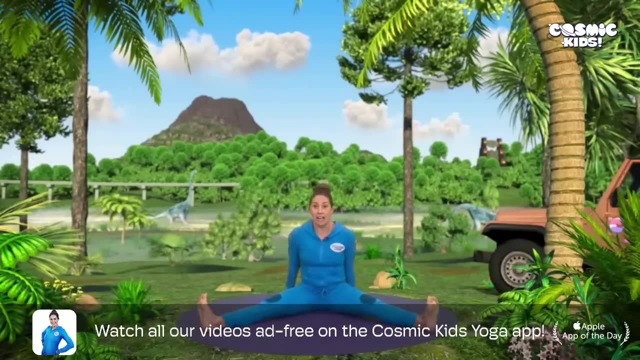 That's a funny sound. And look The ground It's beginning to rumble, Coming to sit on our bottoms, Taking our legs out wide. Our knees rumble up and down, Arms to the side. Oh, my goodness me Coming towards us. 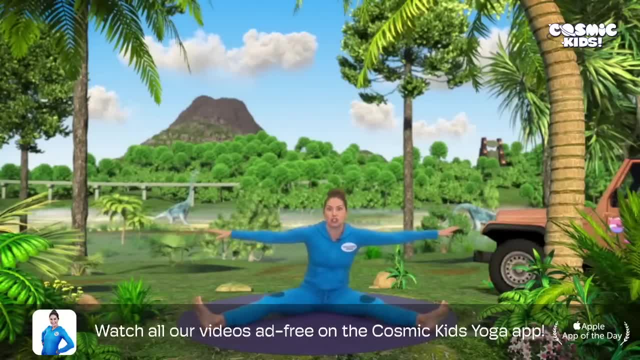 Coming towards us is a stampede of Velociraptors Folding forwards. Let's drum the ground. Here we go. Oh my goodness, I think we should probably hide- Coming up onto our knees everyone And tucking up small like a little mouse. 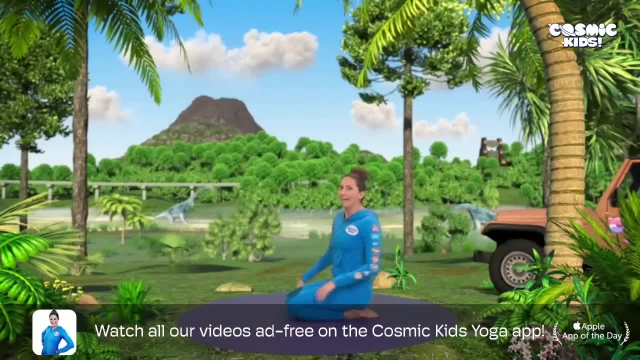 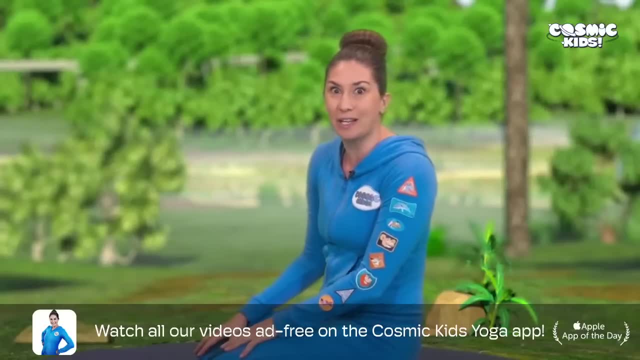 Coming all the way up to sit. Phew, I think they've gone. Well, that was exciting, wasn't it? Now let's go in and explore the park a little bit further. We go over the bridge. Let's do our bridge pose. 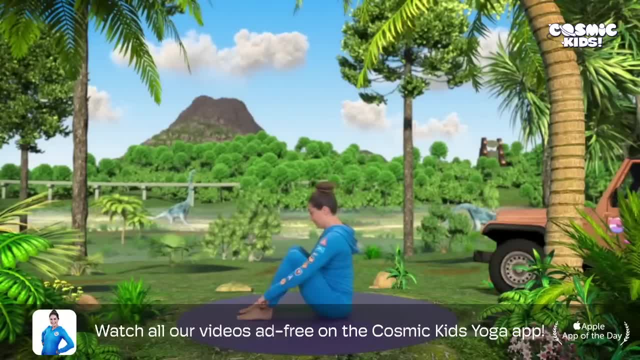 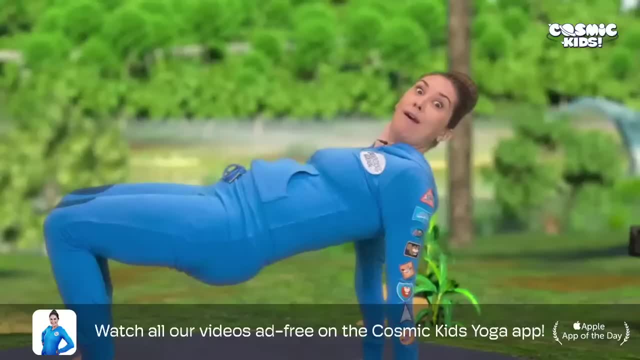 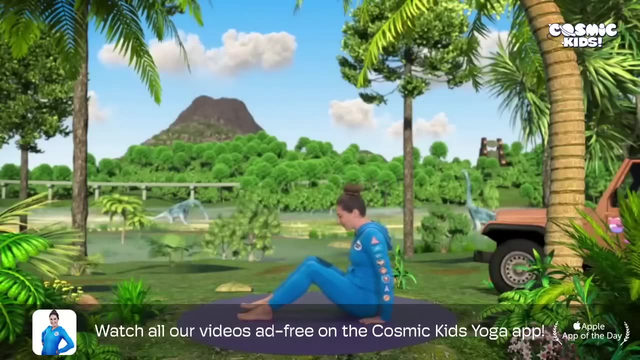 Sitting on our bottoms, Knees bent, Feet, flat Hands behind us. We lift up our hips, Coming into our bridge. pose On the other side of the bridge is a zip line. Shall, we have a go. Come on, everyone Sitting on our bottoms. 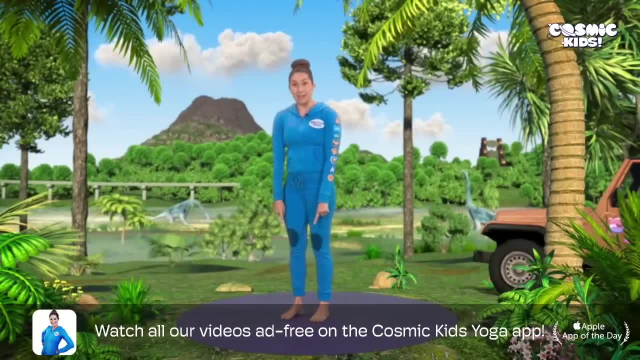 We come up to stand, We take our feet hip distance And we bend our knees. Now we sweep our arms up high, Criss-cross our fingers And hold on as we go, Whoosh And whee, All the way through the tree canopy. 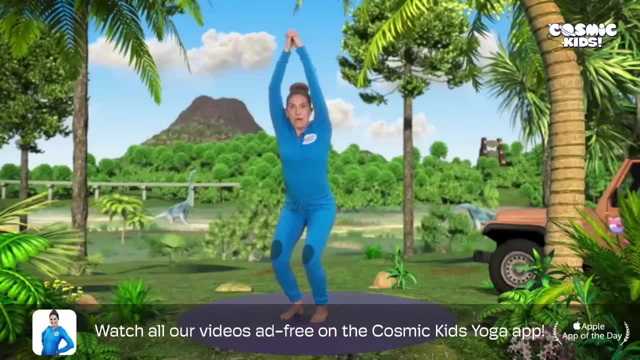 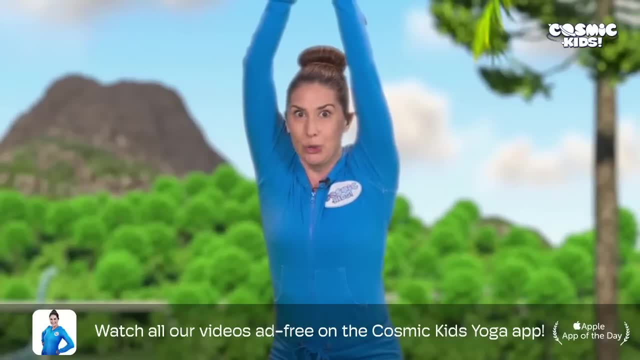 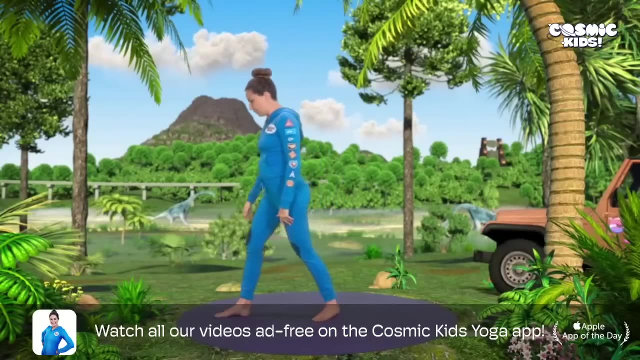 Wow, It's amazing. up here We can see a Diplodocus. My goodness me, They're absolutely huge. Let's try our Diplodocus pose Coming up to stand, Lowering our arms. We step one foot forward and one foot back. 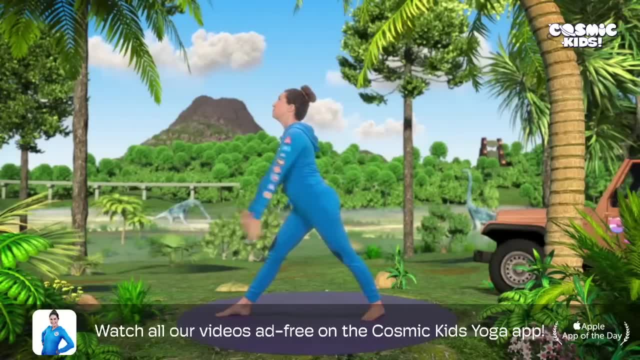 Turning our back toes out a little bit. Now we reach our arms all the way up to the sky And draw our palms together Like we're a very tall and long necked Diplodocus. Now the Diplodocus like to eat vegetables. 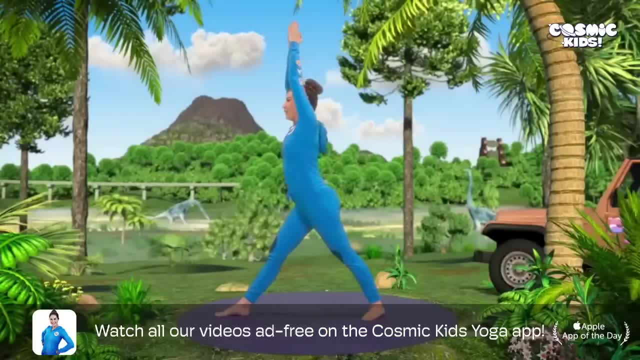 And they love munching the leaves on the trees. Let's fold all the way forwards And do some leaf munching, Munch, munch, munchity munch, Coming all the way up to stand. Let's try it on the other side. 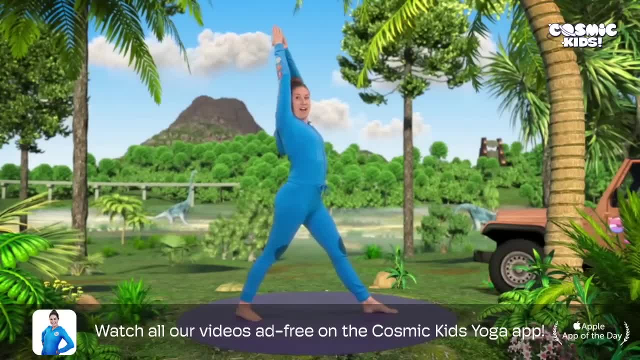 Turning to face the other way now, Reaching up high And folding all the way forwards to munch some leaves. Munch munch munch, munchity, munch munch munch, Coming all the way up to stand, Lowering our arms. 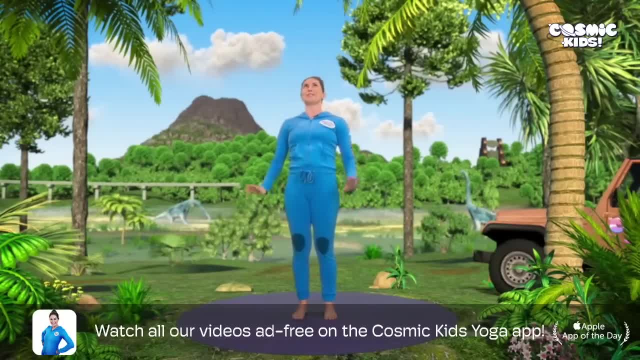 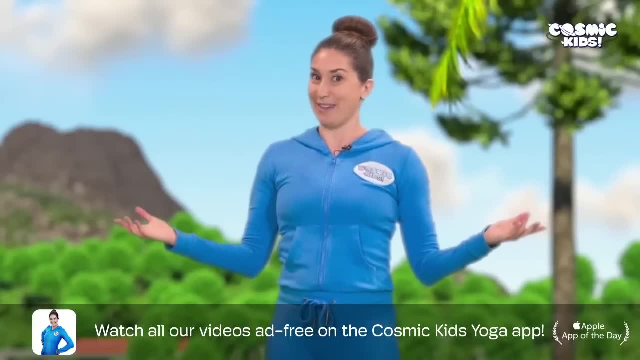 Jumping our feet together. Wow, The Diplodocus are so elegant. On the other side of the zip line, We come to the hatchery, Which is where the dinosaur eggs are. Let's try our egg pose Sitting on our bottoms. 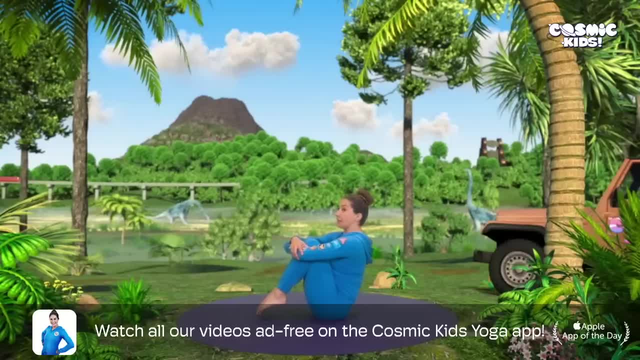 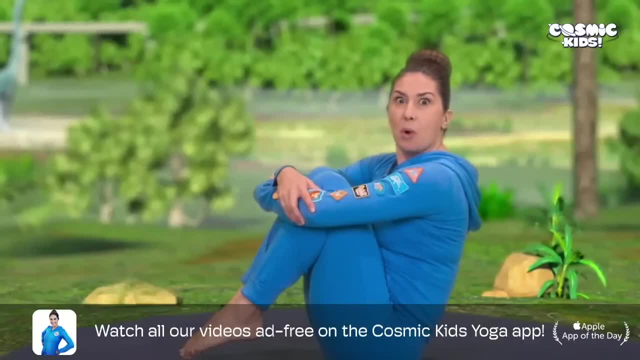 We hug our knees into our chest And we lift our toes off the ground, Balancing like a little cosmic egg. But look, Some of them are wobbling around. They're beginning to hatch, Goodness me. They're rocking backwards and forwards. 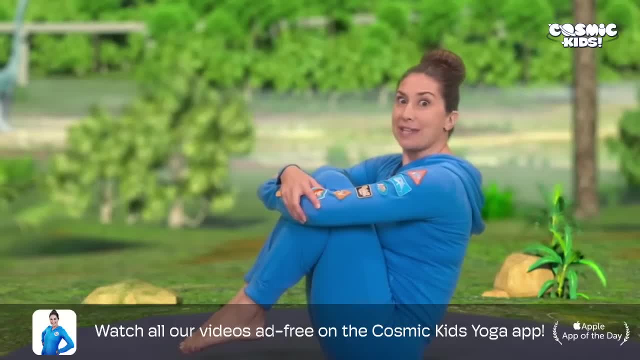 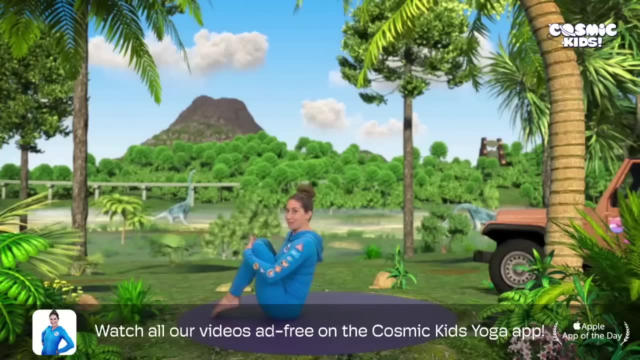 Let's rock back and forwards Like a little egg about to hatch, Sitting up tall, Hugging our knees, Holding our knees And tucking our chin After three. Let's rock all the way back And all the way up. 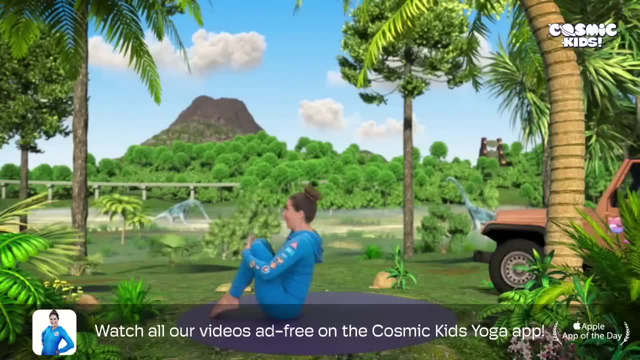 Here we go. One, Two, Three, Whoop Woo, And again One, Two, Three, Whoop Woo. Very good, It rocks all the way onto its back. Here we go, Whoop. Then it rocks onto its side. 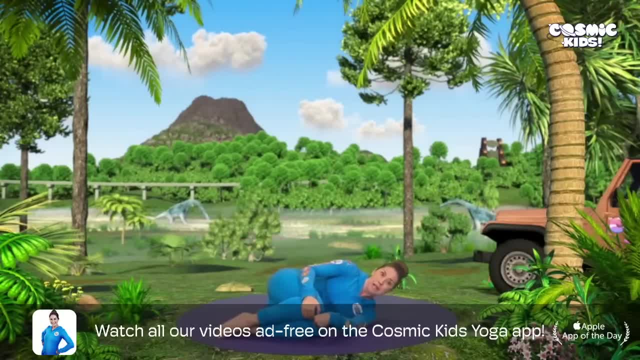 Whoop, It rolls onto its tummy, Coming onto our tummies. everyone Hands underneath our shoulders And it begins to push forwards with its nose, Cracking its shell. Wiggle, wiggle, wiggle, wiggle, wiggle, wiggle. 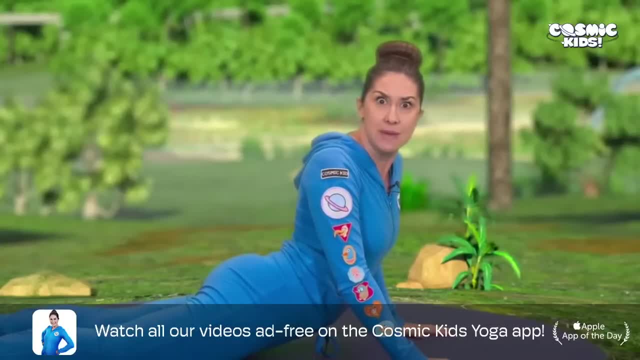 And out pops a baby Ankylosaurus. Aw, The Ankylosaurus is waiting. The ankylosaurus are a bit like a turtle, with bony plates and spikes on its back. Let's do our ankylosaurus- turtle pose. 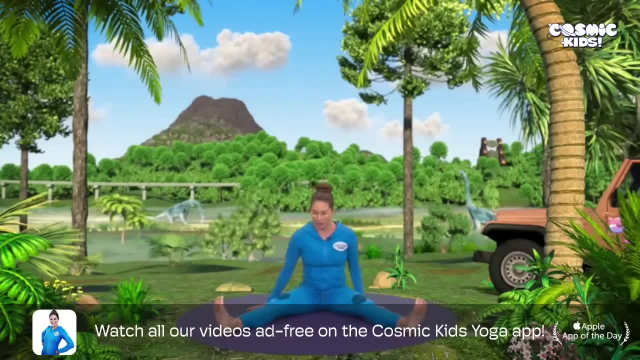 Coming to sit, we take our legs out nice and wide, bend our knees a little bit and bring our hands down in front of us. Now we slide one arm under one leg and we slide our other arm under the other leg, Coming into our turtle ankylosaurus pose. 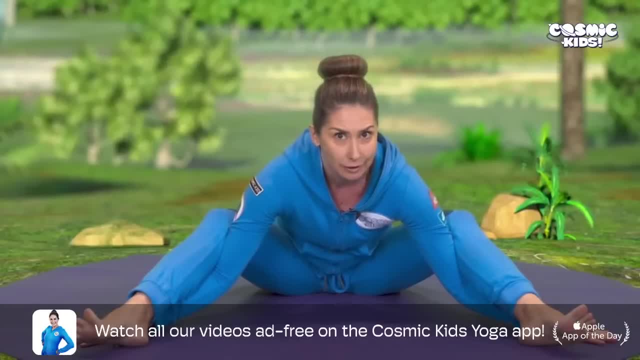 Now you have to watch out for the ankylosaurus tail. They can do a lot of damage when they swish those around. Let's try our ankylosaurus tail pose Coming all the way up to stand. we take our feet nice and wide. 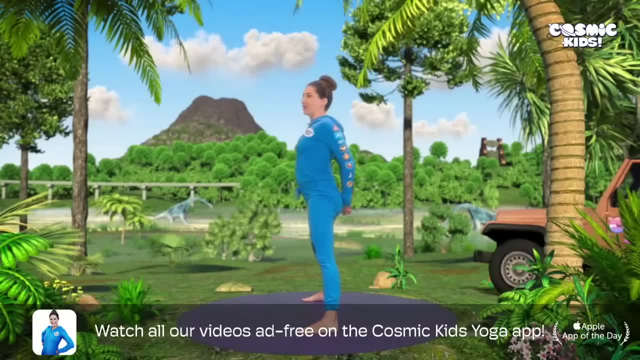 criss-cross our fingers behind our back, roll our shoulders back behind us and stretch our arms. Now, after three, we fold all the way forwards with a swoosh: Ready: One, two, three Swoosh And all the way up to stand. 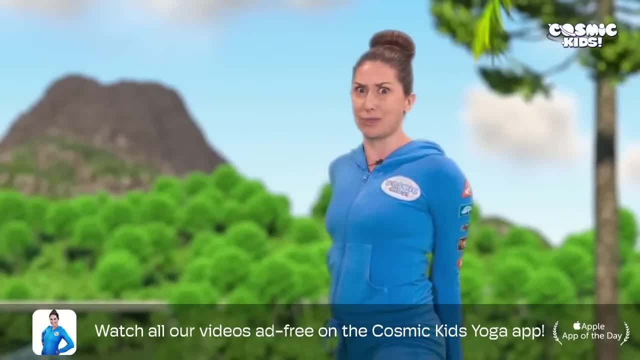 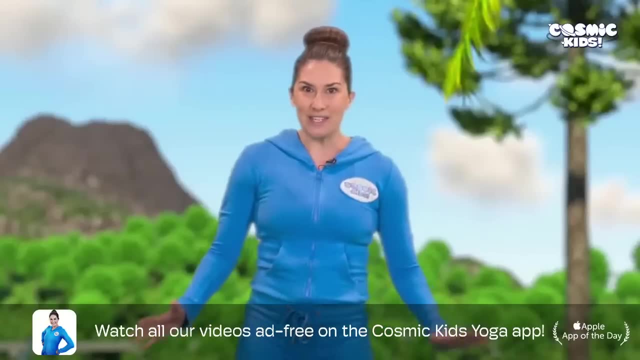 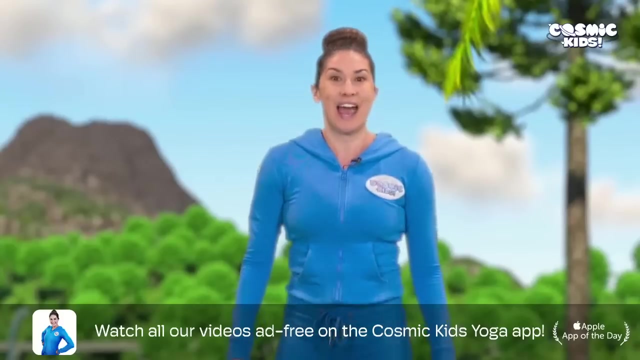 Wow, You better keep out of the way when the ankylosaurus swishes its tail around, Jumping our feet together. coming back to centre Now, why don't we be really brave and go check out some of the scarier dinosaurs? 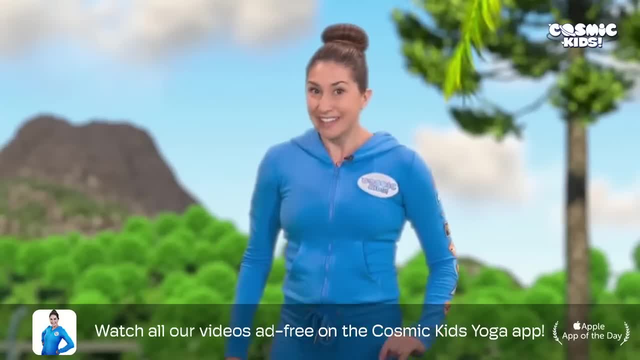 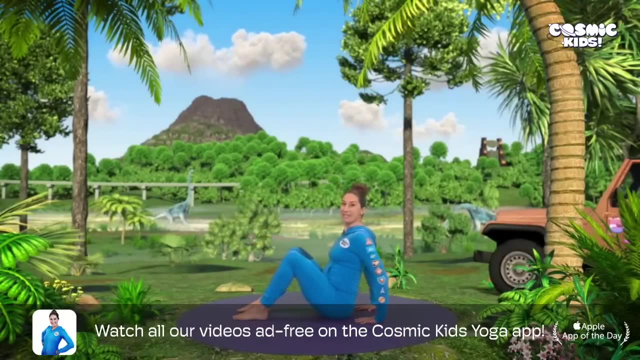 Let's get into the little raft boat. Coming into our boat pose Sitting on our bottoms, knees bent. we keep our hands behind us for balance as we lift up one foot, lift up two, lift up one hand, lift up no hands. 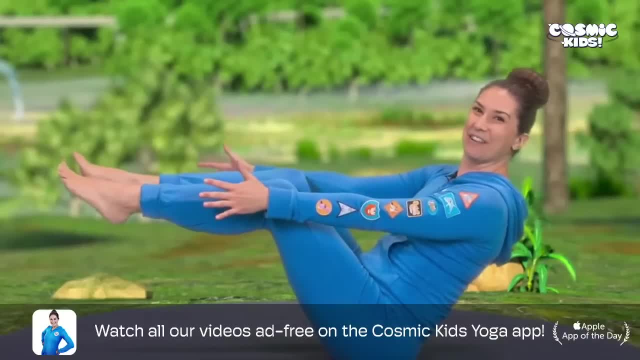 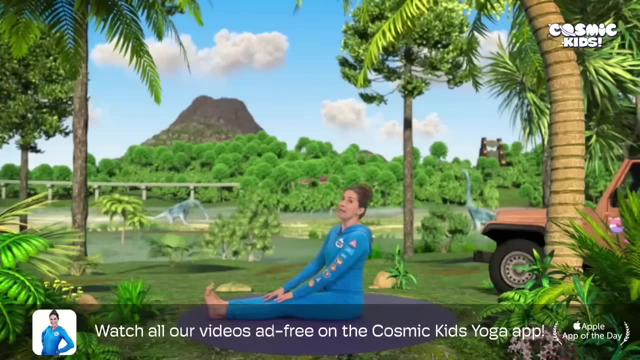 And give me a wave. Hi, Very good, everyone. Stretching our legs out forwards, we row our little raft boat down the Jurassic River, knowing that the dinosaurs are very safe in their habitats. Singing, row, row, row your boat. 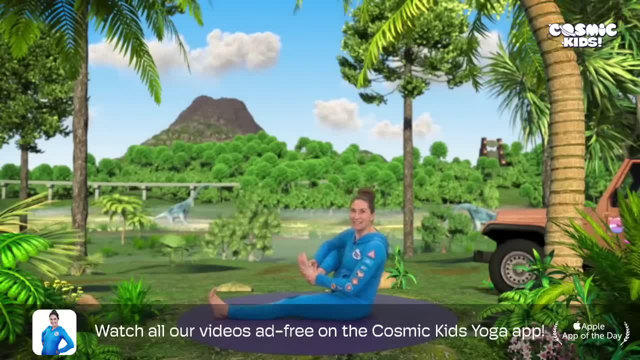 Come on, picking up one of our feet and let's row. Here we go, Row, row, row your boat gently down the stream, Merrily, merrily, merrily, merrily. life is but a dream. 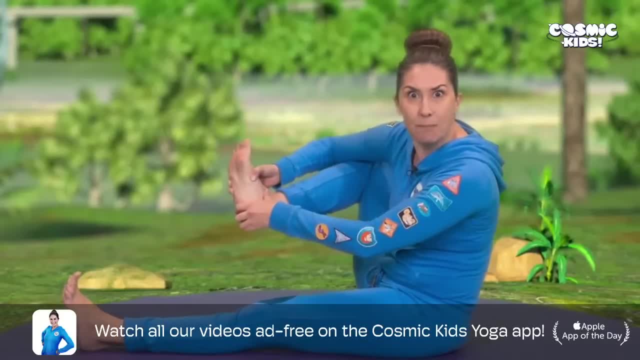 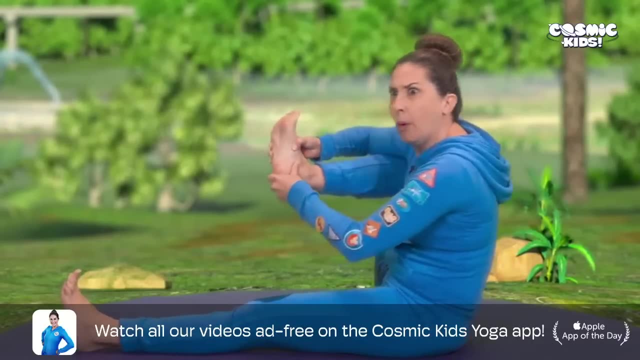 Oh, Oh look. That's the walkie-talkie from base camp. Let's answer it. Er receiving come in. we are on the raft boat, All operatives in the park. the dinosaurs have escaped, Escaped Dinosaur. 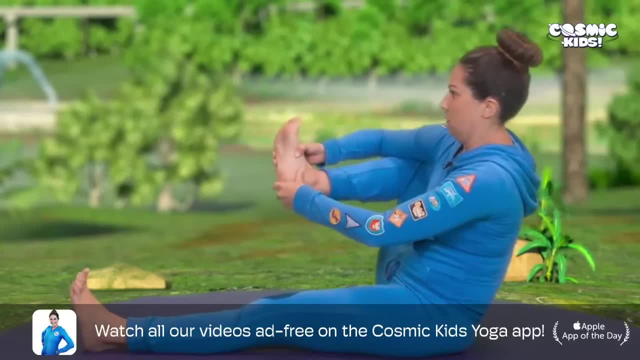 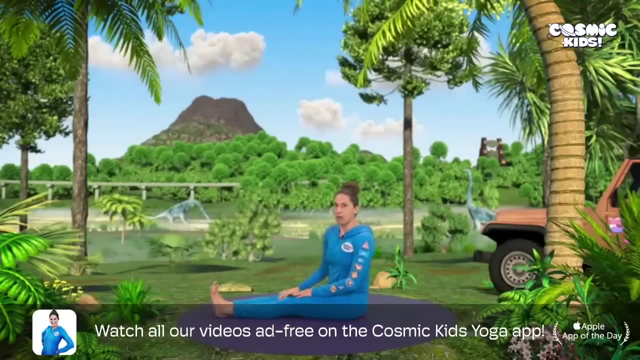 Oh, Problem, Okay, Oh, It seems to have stopped. Let's put it down. Oh dear, Maybe we should row on a little bit further. Let's pick up the other oar and stay nice and calm as we sing our row, row, row your boat song again. 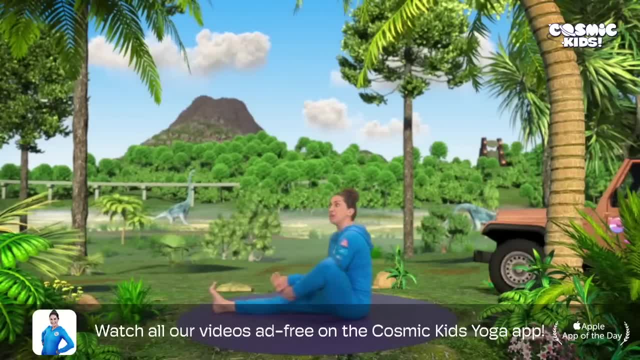 Here we go, Row row, row your boat gently down the stream, Merrily, merrily, merrily, merrily. life is but a dream. Oh, It's the walkie-talkie. again, Let's answer this one. 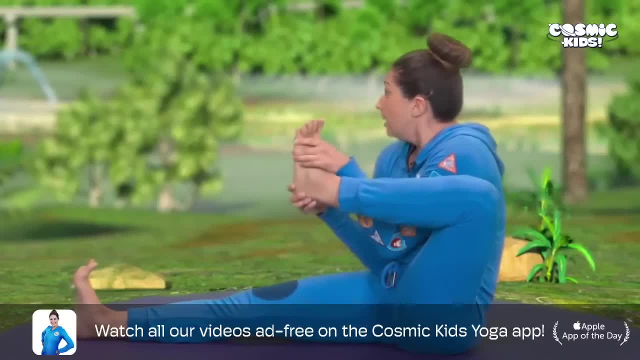 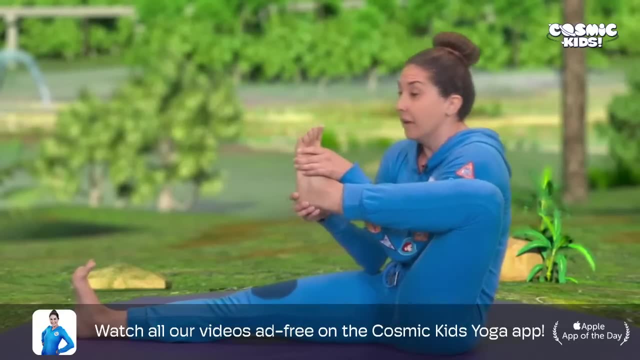 Holding it to our ear: Come in, Roger Receiving. Please make your way to the exit immediately. Exit Immediately. Oh, Okay, then Okay, Over and out, Bye. We put the walkie-talkie down, Oh. 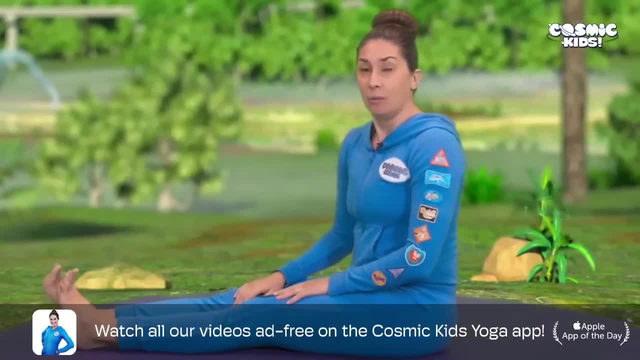 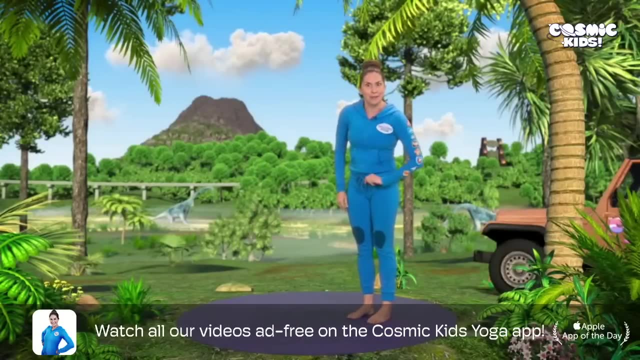 And it sounds like we need to get out of here pretty quickly. Well, we arrive at the banks of the river, Coming up to stand everyone, And we take big steps into the woods, Standing nice and tall, Here we go. 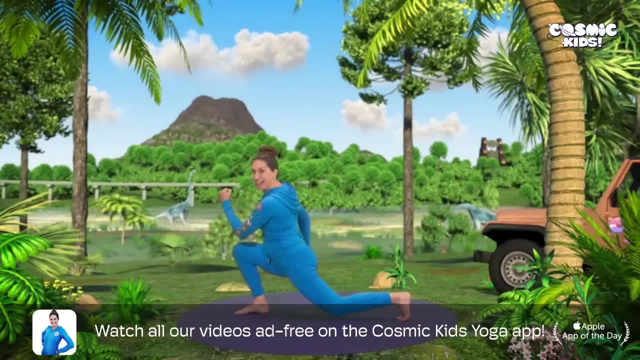 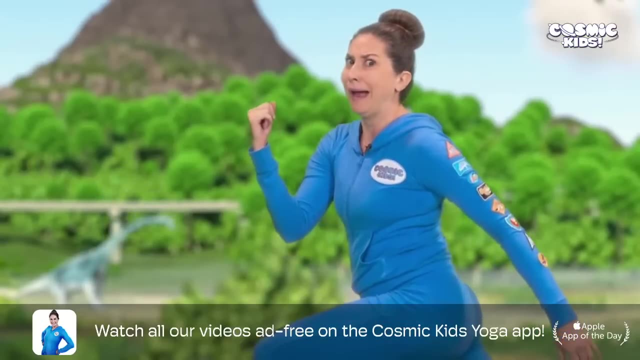 Big step And all the way back. Oh, And the other side Big step, Uh-oh, We can feel the ground trembling again, And this time it's something much bigger and much scarier. Clomping towards us is a Tyrannosaurus Rex. 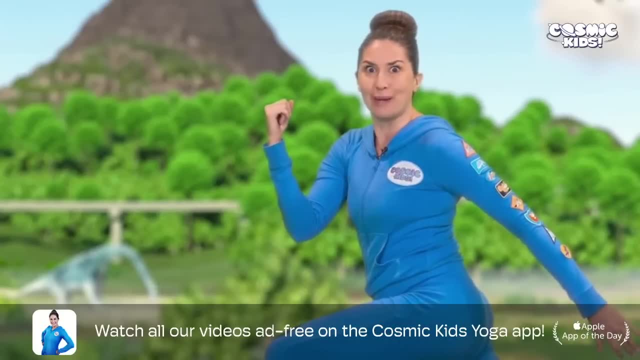 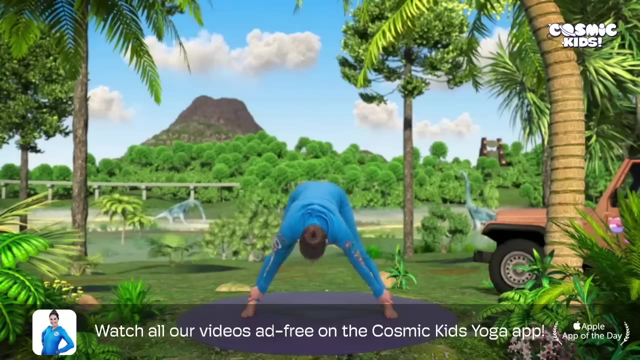 Let's do our T-Rex clomping pose. Coming up to stand Feet, nice and wide, Folding forwards to grab our ankles. We lift them up, one at a time, going clomp, clomp. Here we go, Clomp. 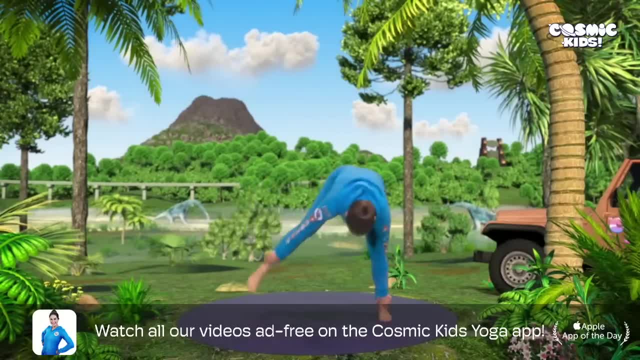 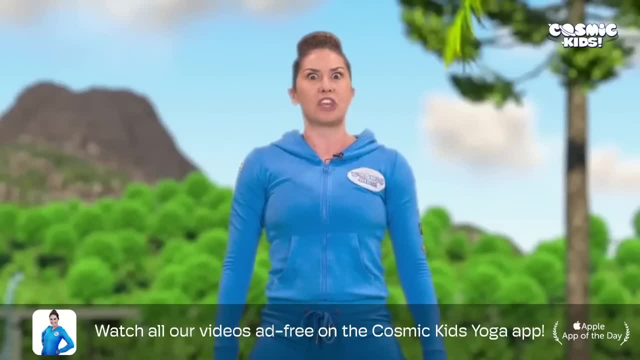 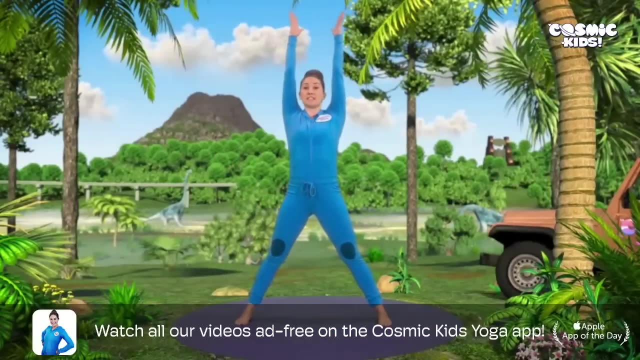 Clomp, Clomp, Clompity, clomp, Clomp, Clomp, Rolling up to stand. Okay, everyone, We've got to think quick. Let's throw our sandwiches for it, Then we can hide Reaching all the way up to the sky. 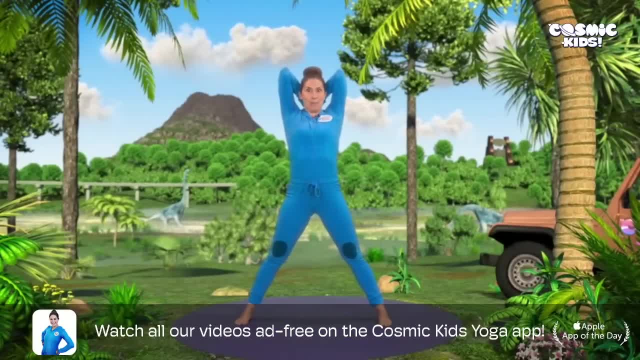 into our backpacks behind us, we grab our sandwiches and we throw them for the Tyrannosaurus Rex. Here we go, Pee-yoo. Now we need to hide, Coming down onto our knees everyone And tucking up nice and small. 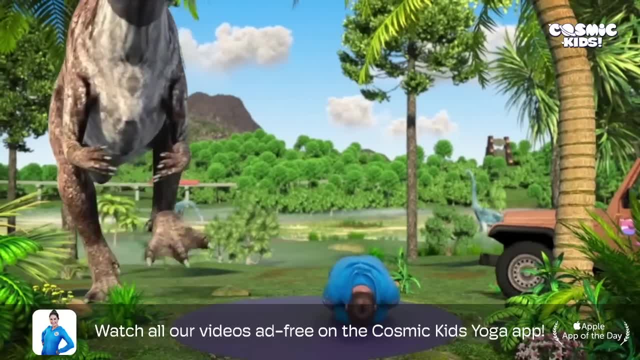 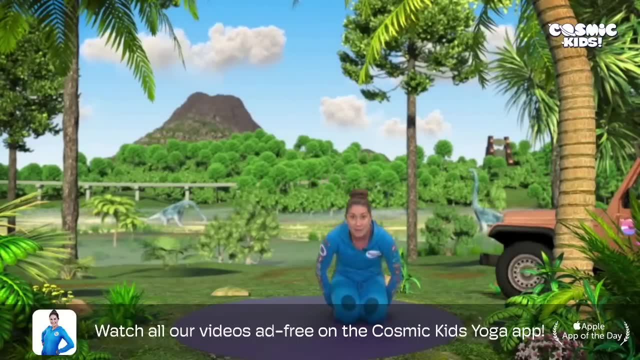 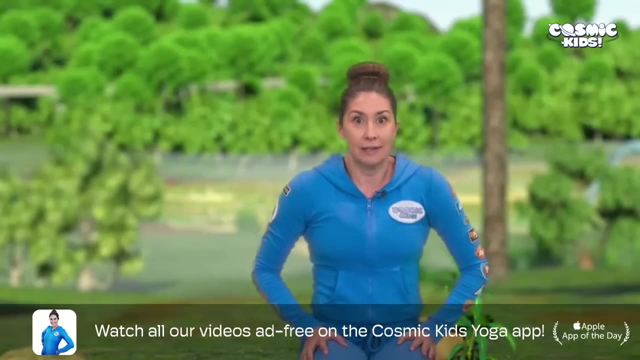 Here it comes for our sandwiches: Clomp, Clomp, Clomp, Clomp, Clomp, Clomp, Coming up to sit Pee-yoo. Well done. It clearly enjoyed our sandwiches and off it went. That's a relief. 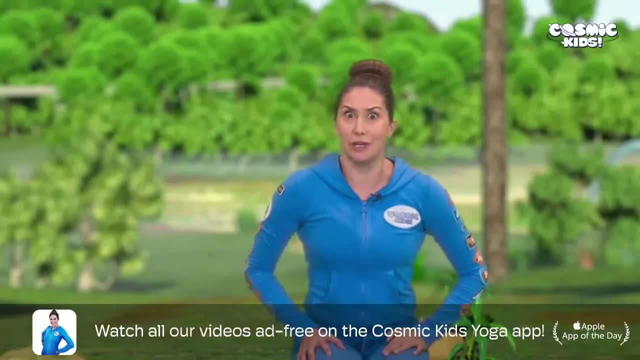 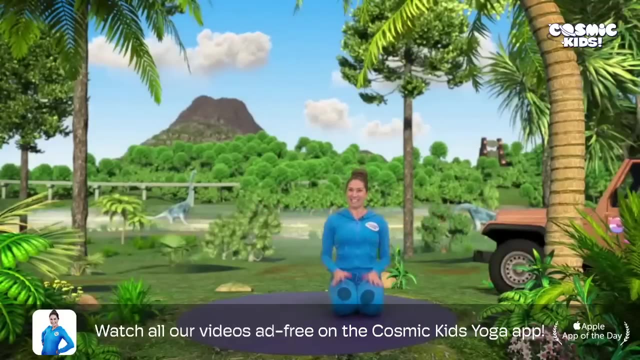 Well, I think that's about enough excitement for one day, don't you? Let's use our emergency escape card and make the podplane appear. Here it is. Let's do our podplane pose Coming up to two feet knees, we take our arms out nice and wide, we drop down onto one hand and we wave at the sky. 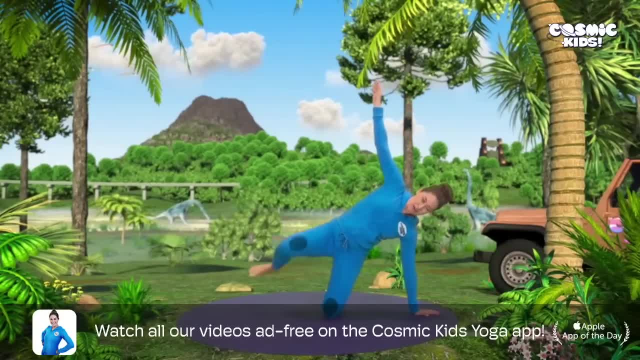 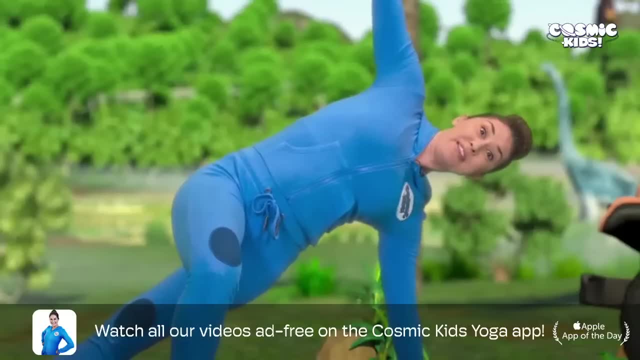 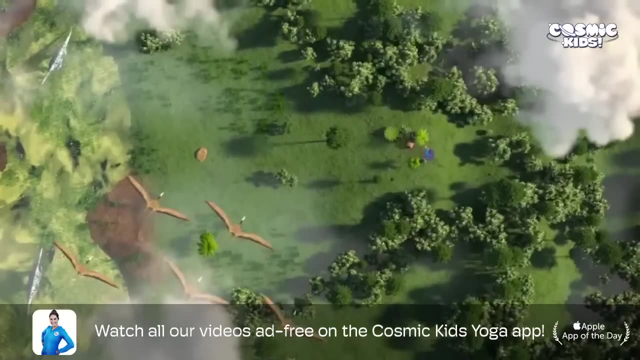 say hi sky, hi, sky. we bring one foot in front of our knee and shoot our back leg out behind us, lifting our hip and look up in the sky. we see a whole flock of pterodactyls. let's wave at the pterodactyls, hi, pterodactyls, higher. let's do our pod plane pose on the other. 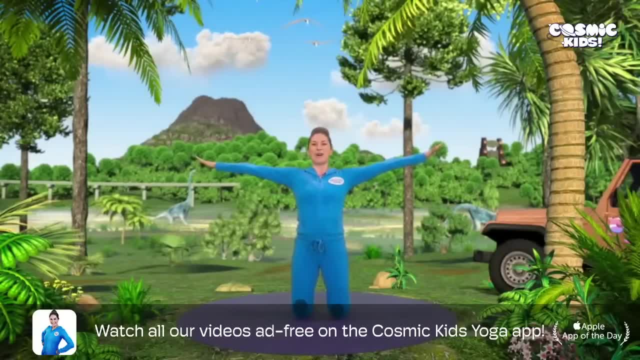 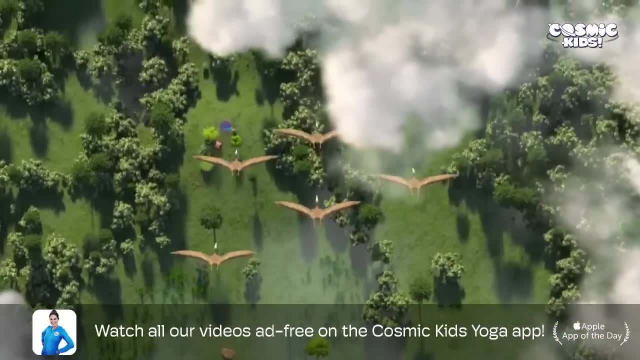 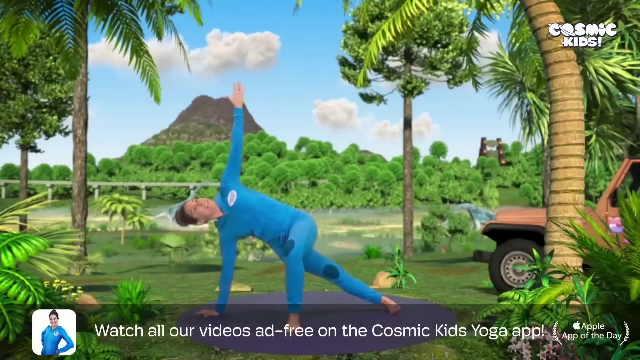 side. coming back to two knees arms wide, we drop down onto our other hand. let's give another wave to those pterodactyls, hi, pterodactyls. we bring our foot in front of our knee and shoot our back leg out behind us and lift up our hips as we go. 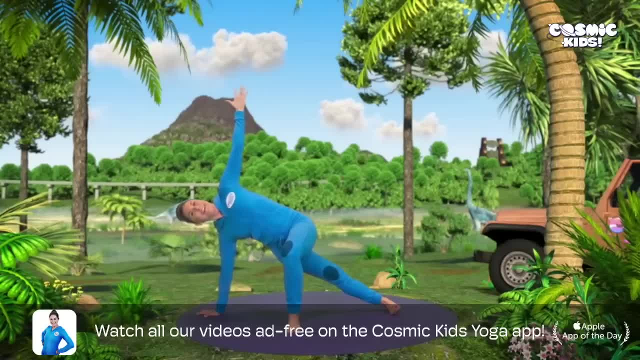 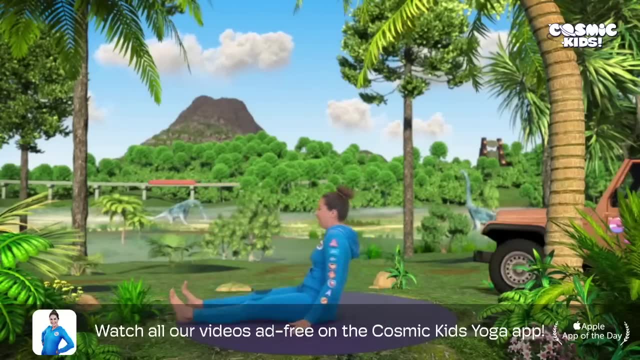 flying all the way home. we take a moment to lie back and relax in our pod plane, coming to sit on our bottoms, legs long, rolling all the way down onto our backs. ah, our pod plane will take us home, keeping us nice and safe. it's so peaceful and fresh up here in the sky. 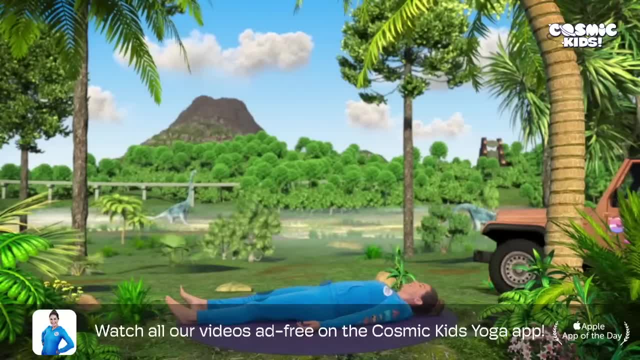 what an amazing experience, an adventure. weren't we lucky and brave to see all those amazing dinosaurs? it's very important whenever we see animals in their habitats that we treat them with respect. whether we're in a park like this, we're diving in the ocean or we're just out walking in the woods, we are peaceful and respectful. 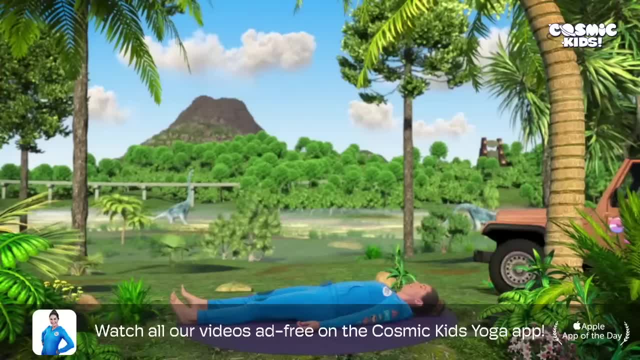 of the other creatures and animals that live there and we leave no trace. we always take our litter and our rubbish away. now we begin to wake up, wiggling our toes, wiggling our fingers, hugging our knees into our chests as we roll onto our sides. 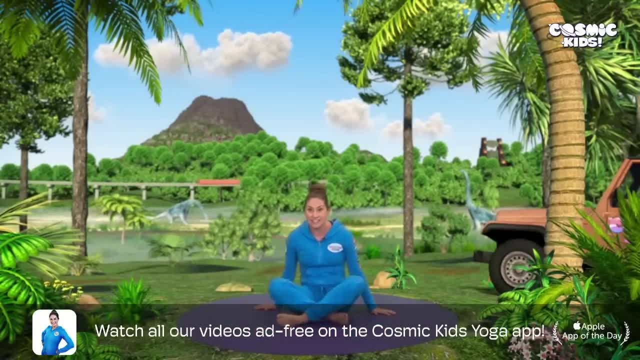 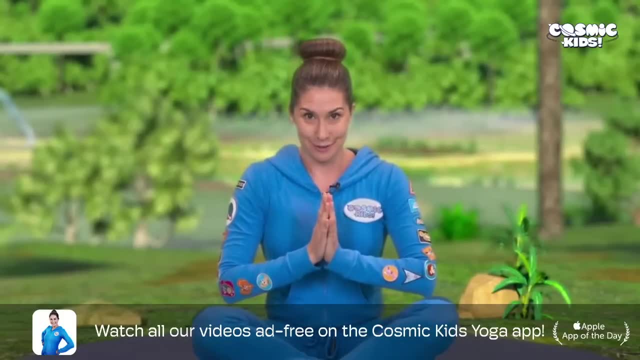 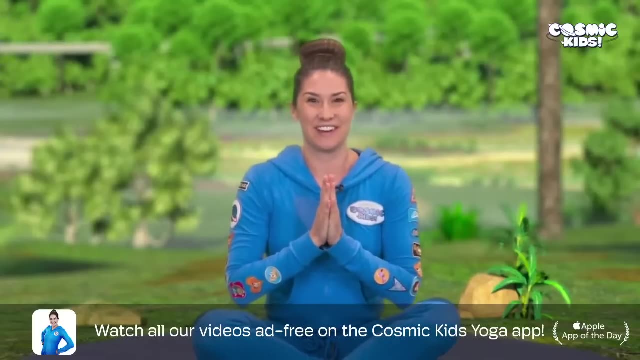 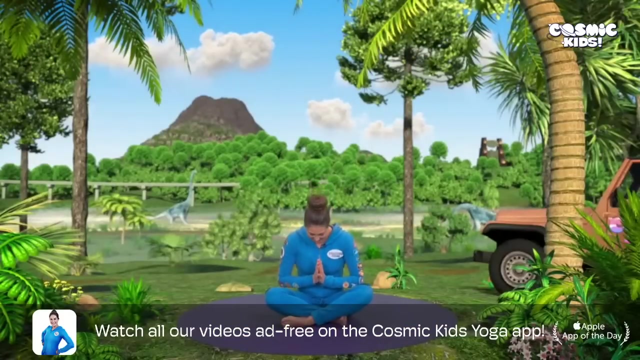 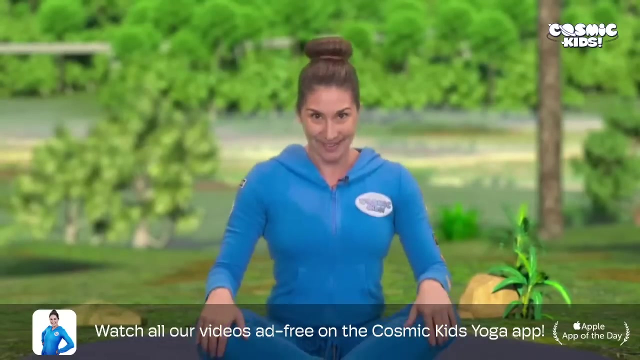 and press ourselves up to sit with our legs crossed, our hands together at our hearts. to finish just the way we started with our secret jurassic dinosaur yoga code word, which is namasaurus, ready after three: one, two, three, namasaurus. wow, you were amazing in the jurassic dinosaur yoga adventure. i hope you enjoyed it. 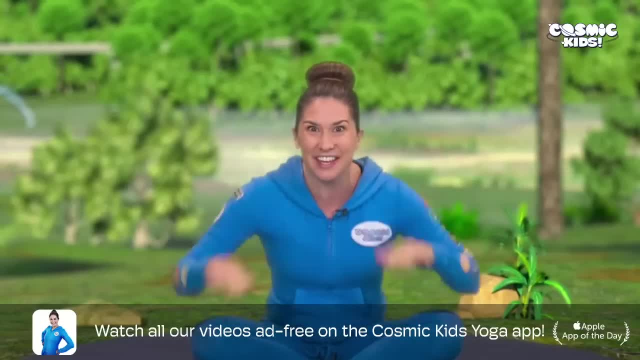 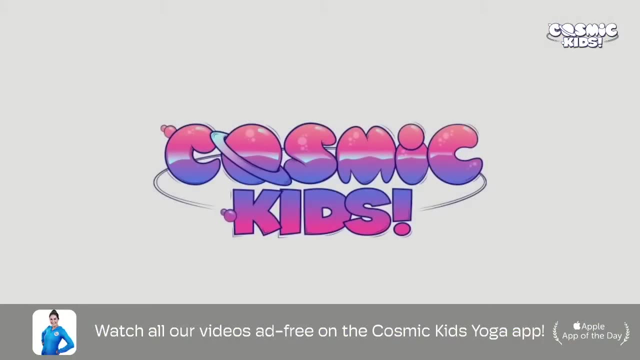 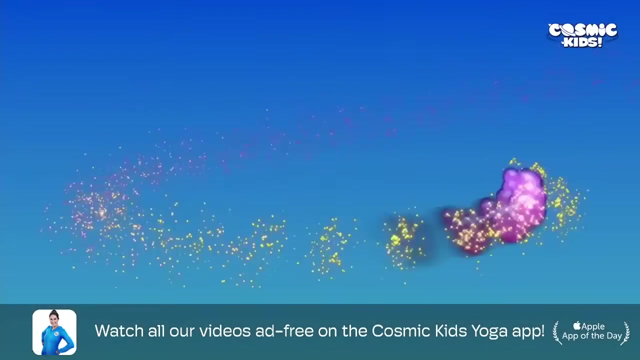 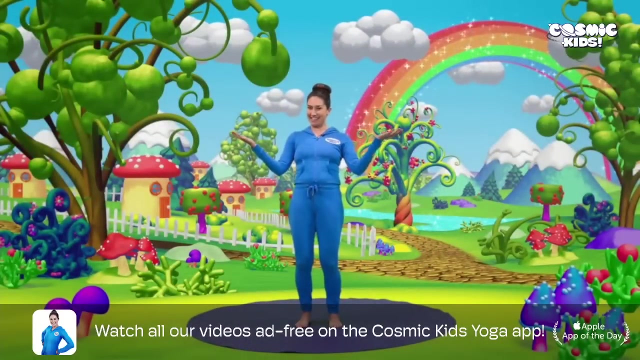 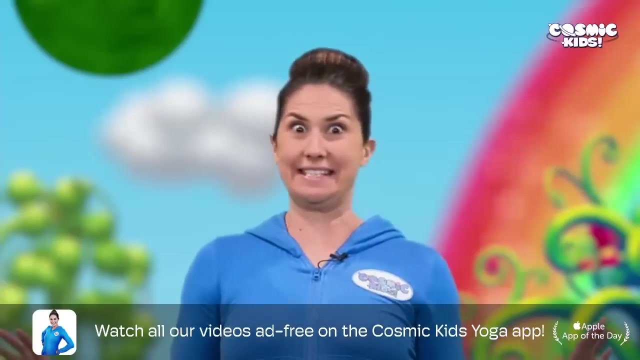 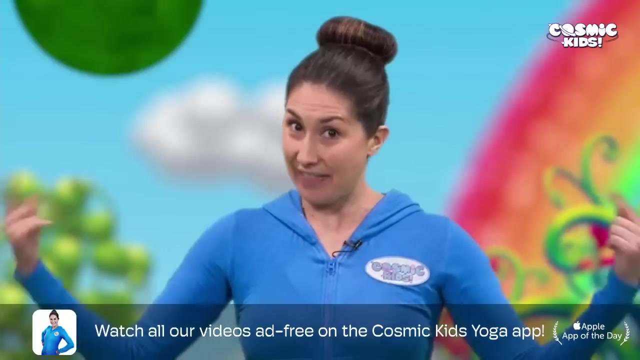 and i hope to see you again soon for another cosmic kids adventure. bye-bye, hello everyone. welcome to cosmic kids. i'm jamie and this is your place for yoga, stories and fun. it's easy: just copy the moves i do and enjoy the adventure. now we always start in the same way, and that's by sitting on our bottoms, crossing our legs. 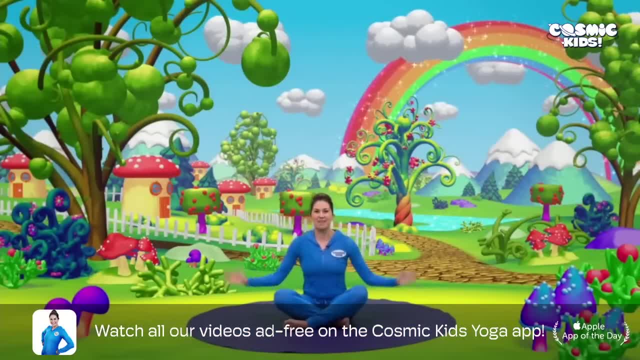 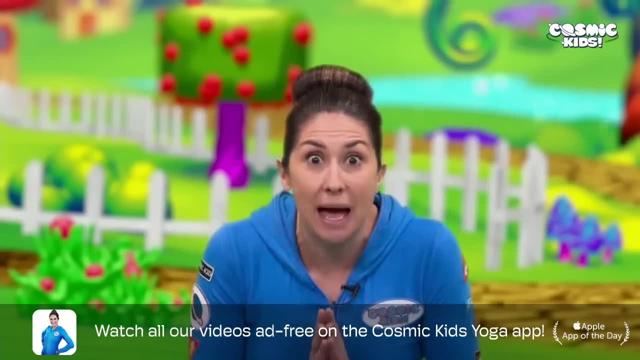 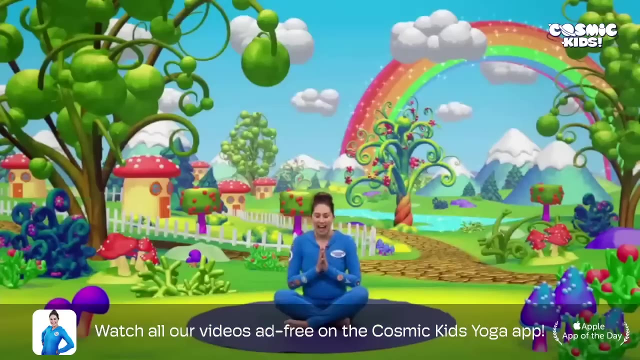 and bringing our hands to one another and in this way we're going to slouch our body straight and be able to even knead the rest of our feeteses in our pose, hands together at our hearts, and saying our secret yoga code word, which is: Namaste, Ready After three, One, two, three, Namaste, There, Now we're ready to begin. so. 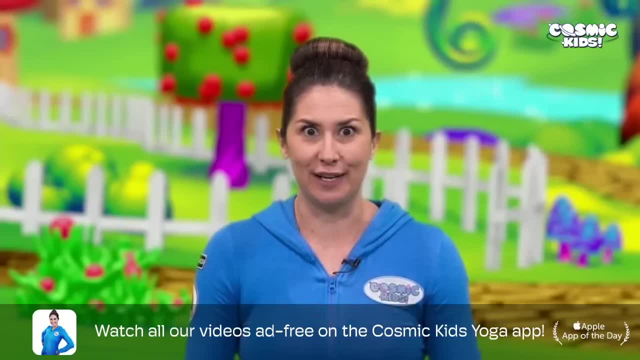 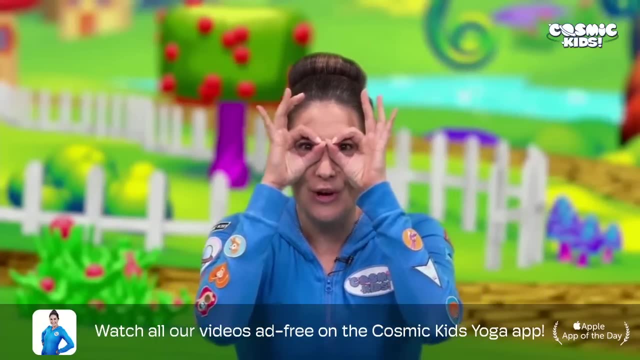 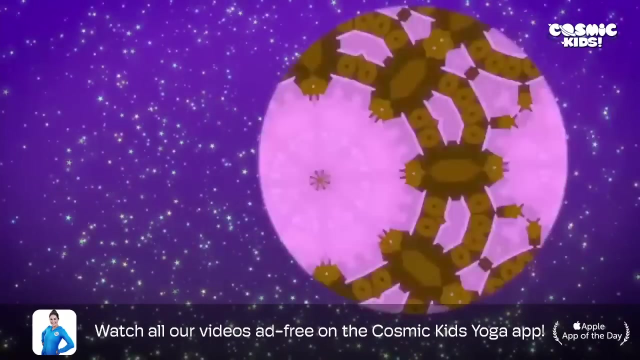 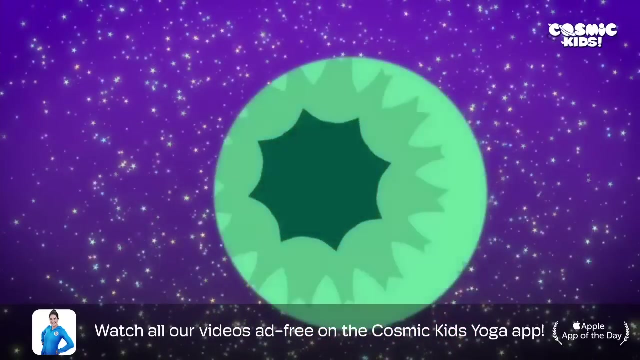 let's take a look through our cosmonoculars and find out who we're meeting today, Joining our thumbs and fingers together. have a look through. Look at those colours and those shapes, those patterns, all swirling and twirling around. Oh aren't they pretty. Can you see the picture? It's a monster, It's Biggles. the. 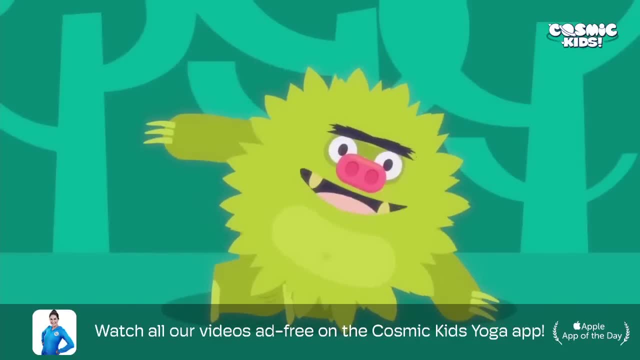 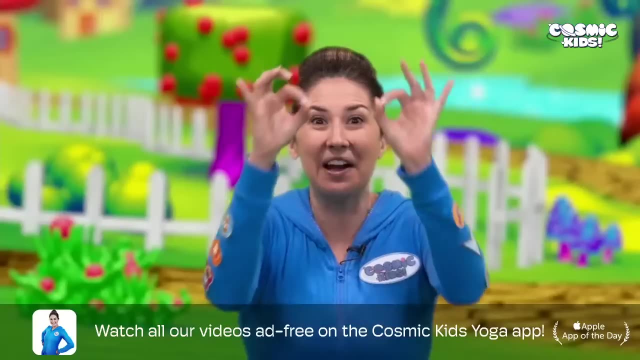 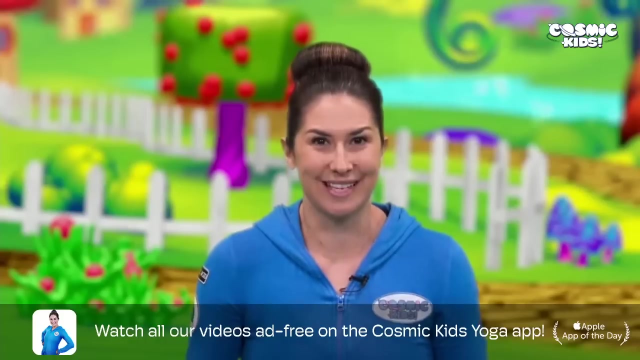 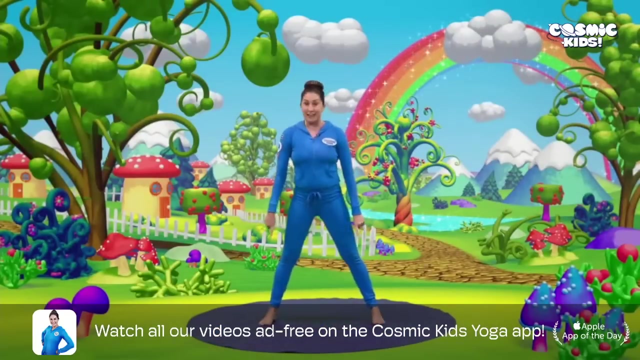 monster. Oh, what's Biggles doing. Biggles the monster, Biggles the monster, Oh, what's Biggles doing. Biggles the monster, Oh, what's Biggles doing? He's doing yoga. He's doing crocodile pose, Lowering our hands. How cool. Biggles is a very big monster. So let's begin in our clompy monster pose. Coming up to stand, we take our feet nice and wide, We fold all the way forwards to take our ankles and we lift our feet up and down as we say clomp, clomp. 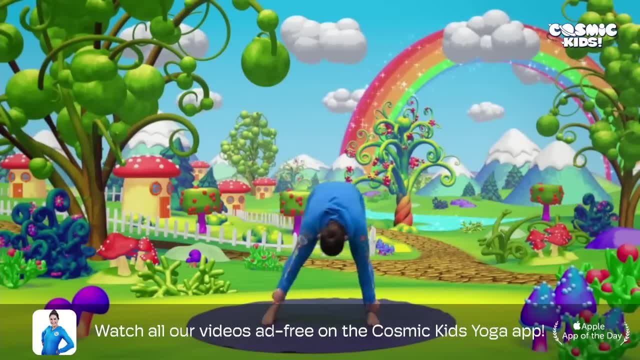 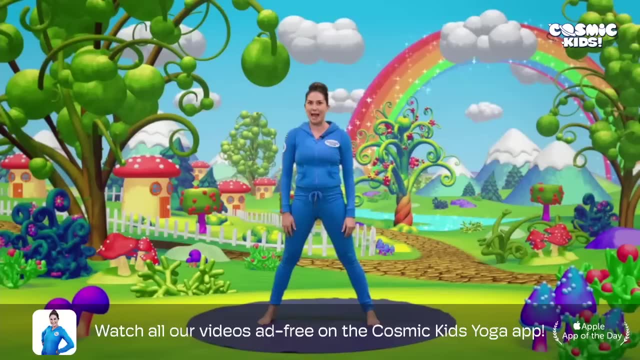 Clomp, clomp, Clomp, clomp, clompity, clomp, clomp, clomp, Rolling up to stand. Now. Biggles has spiky green hair that sticks out in all directions. Let's use our arms and legs to be our spiky green hair. Keeping our legs out wide, we stretch our arms out wide as well, and we wiggle our fingers to make extra spiky bits. He's got a big pink nose. 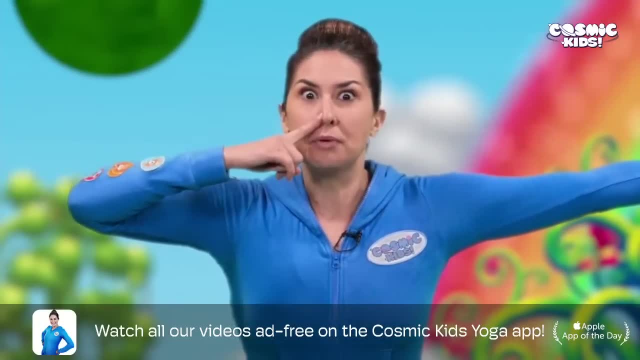 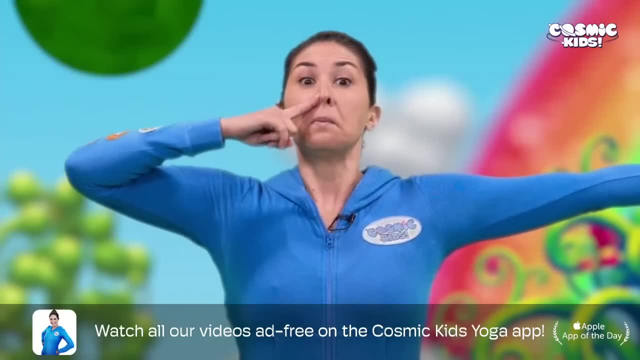 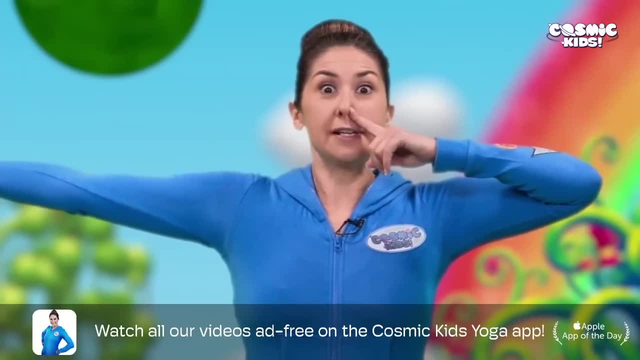 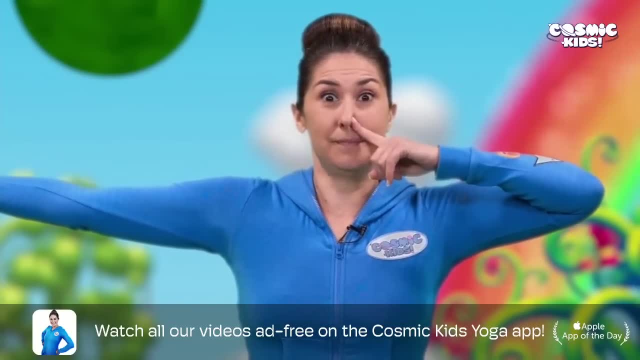 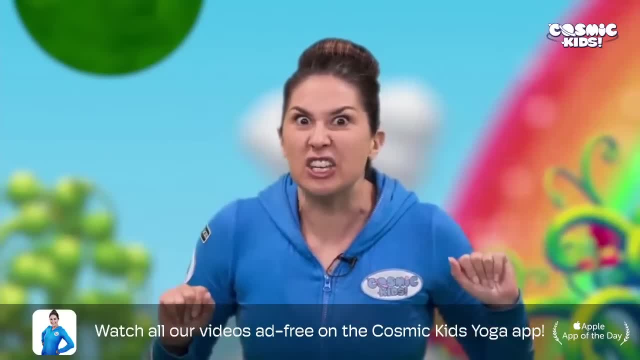 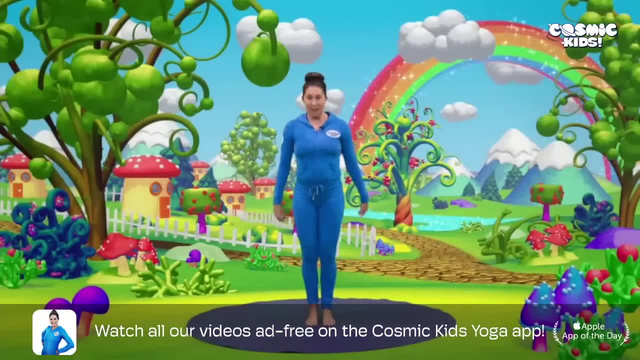 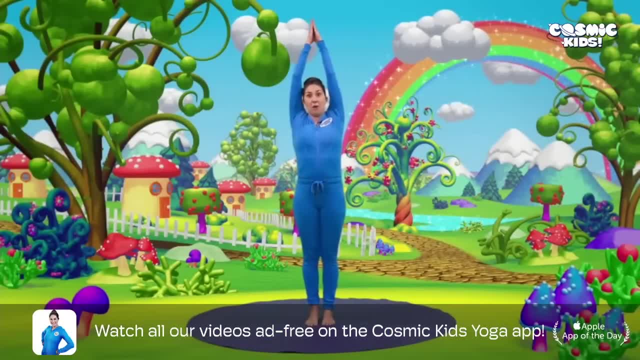 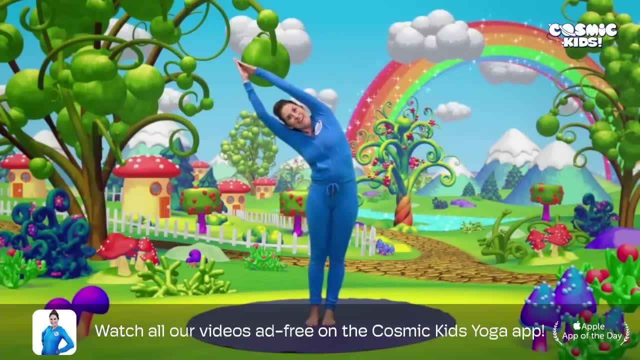 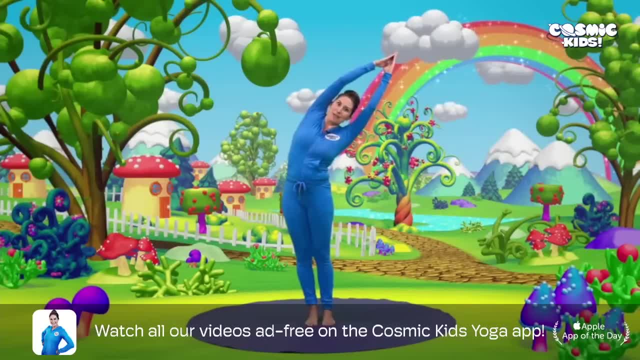 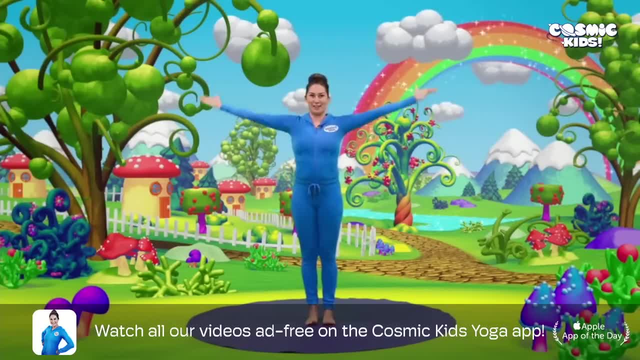 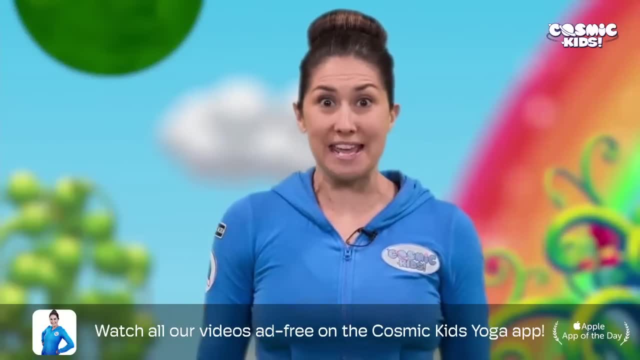 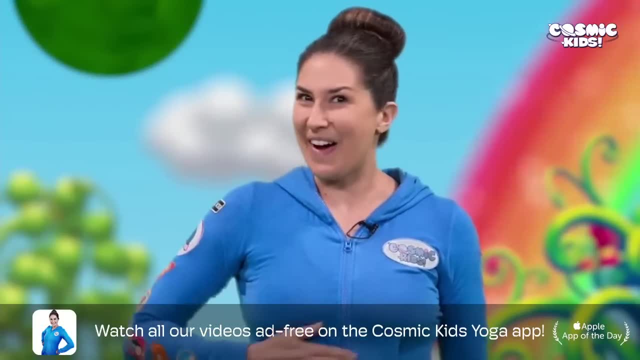 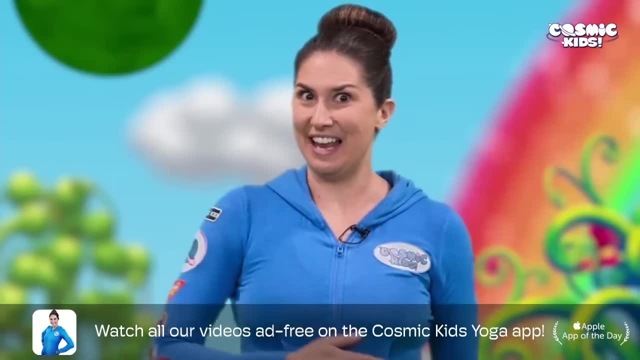 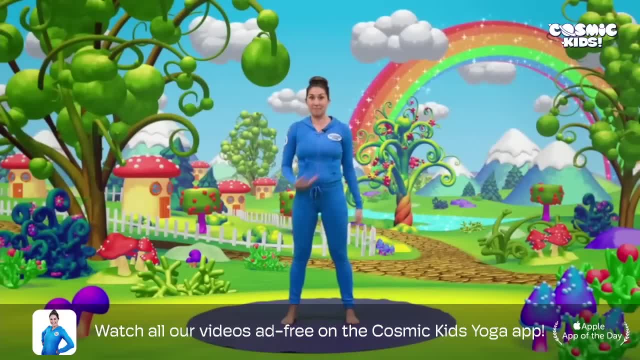 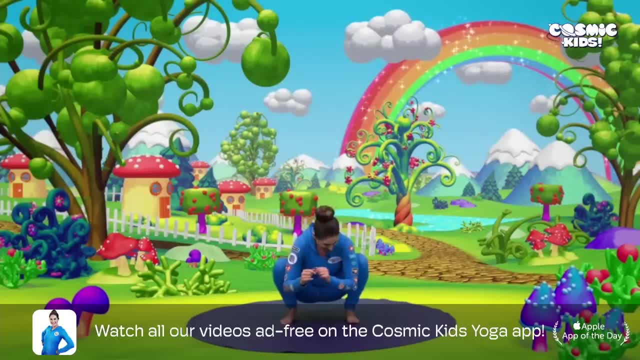 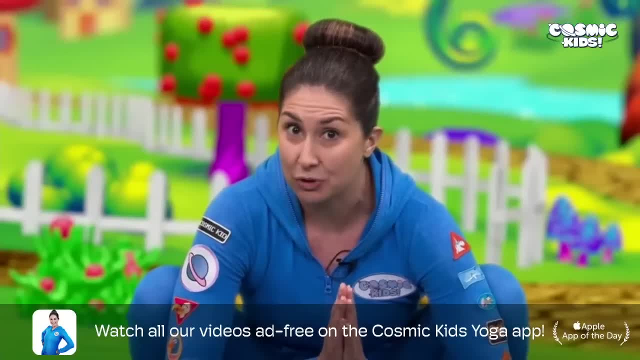 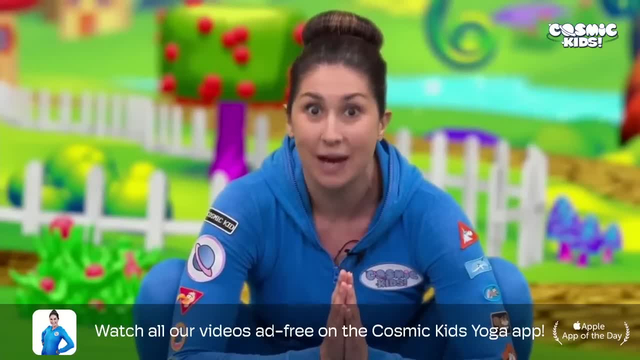 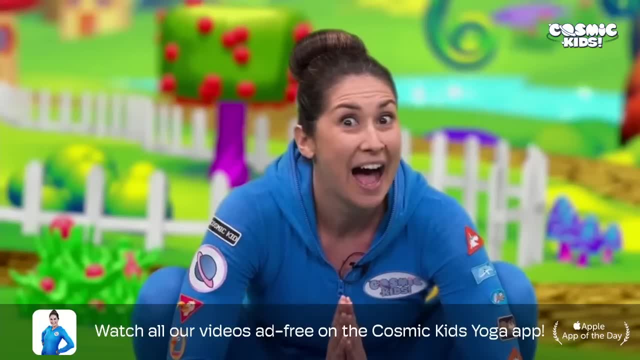 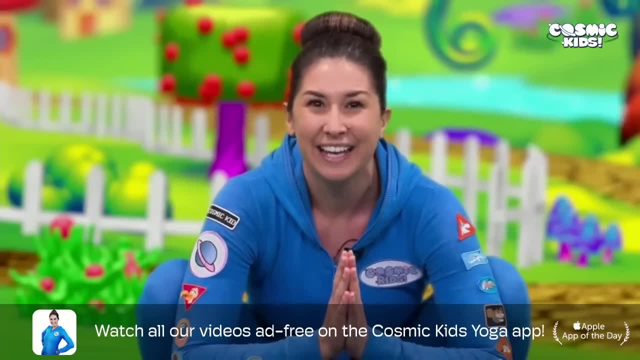 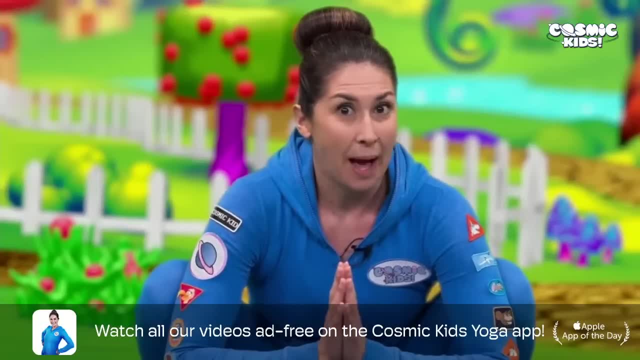 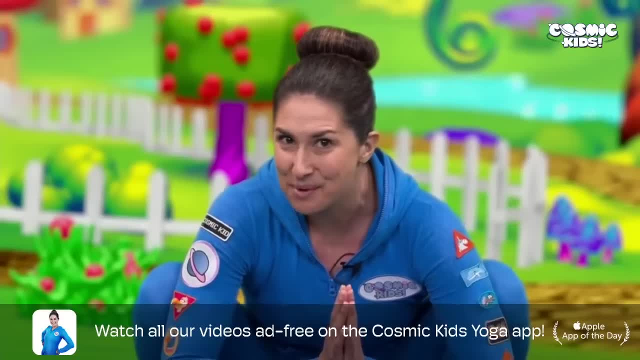 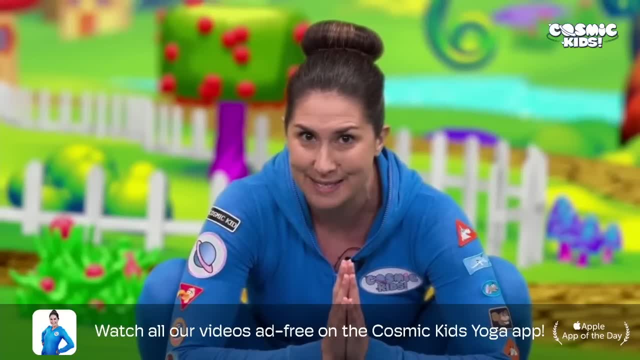 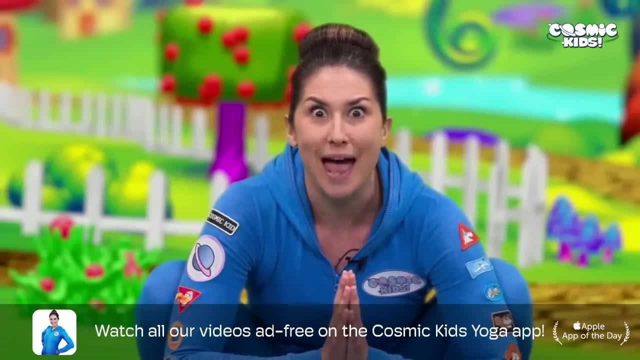 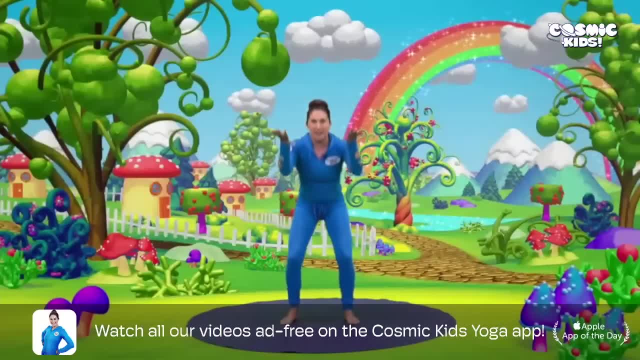 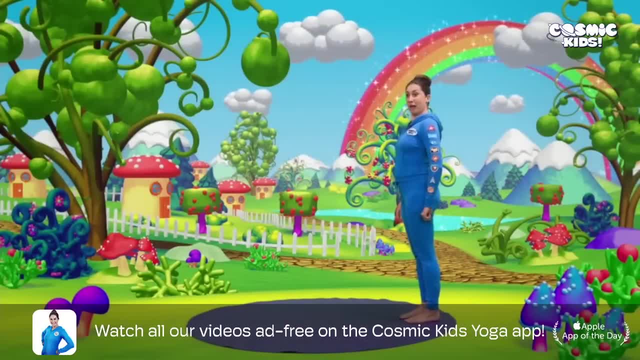 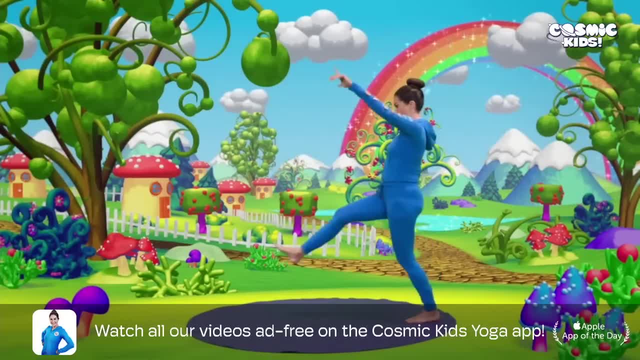 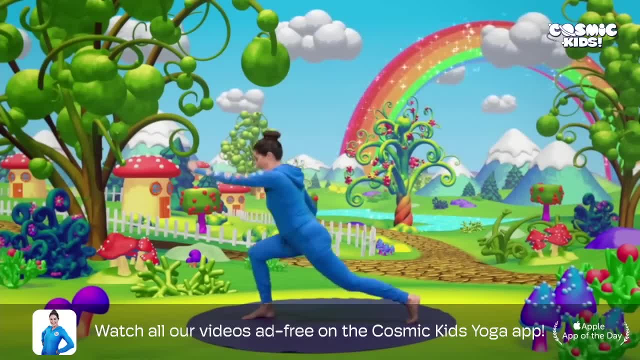 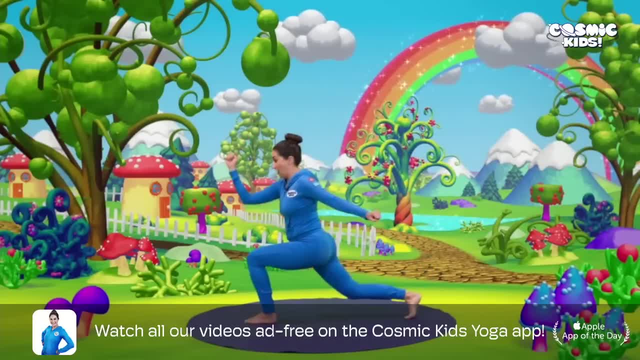 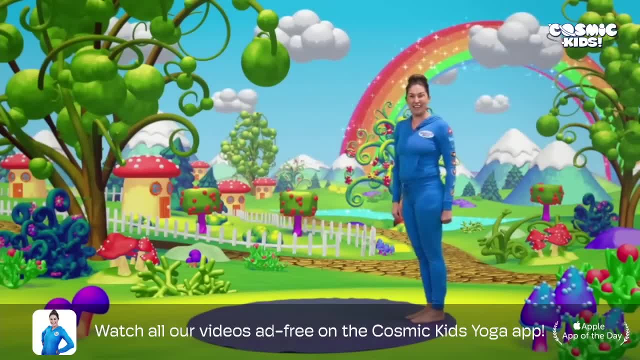 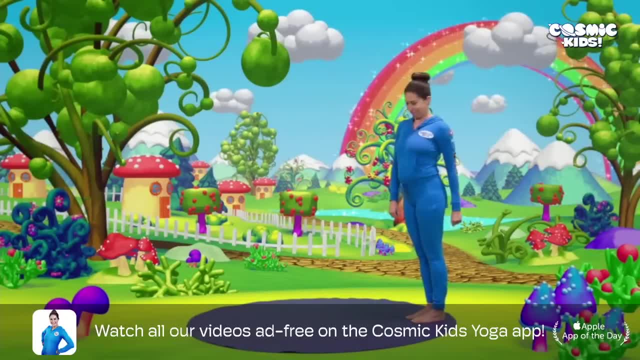 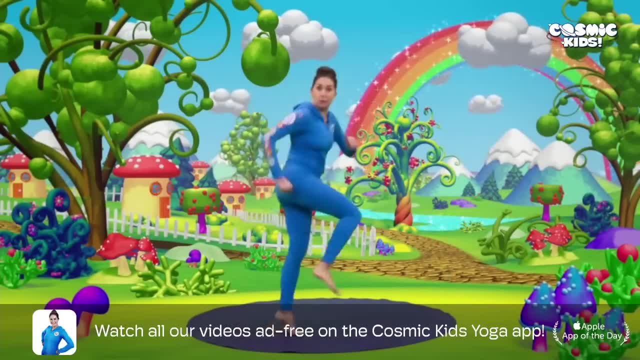 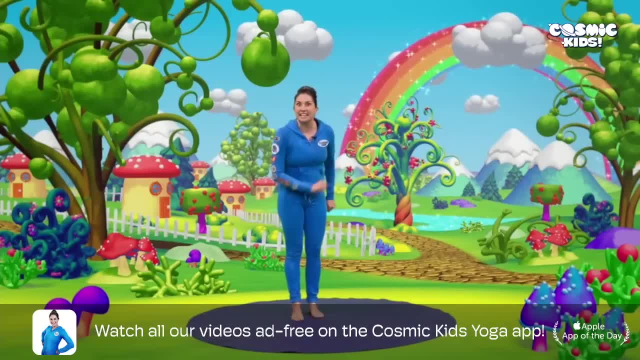 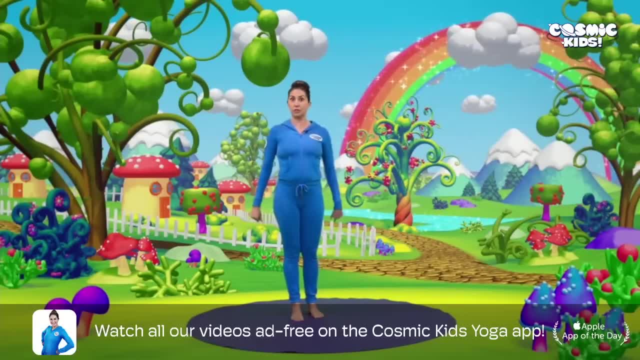 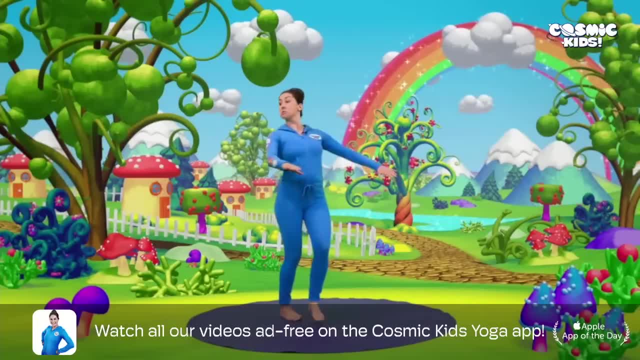 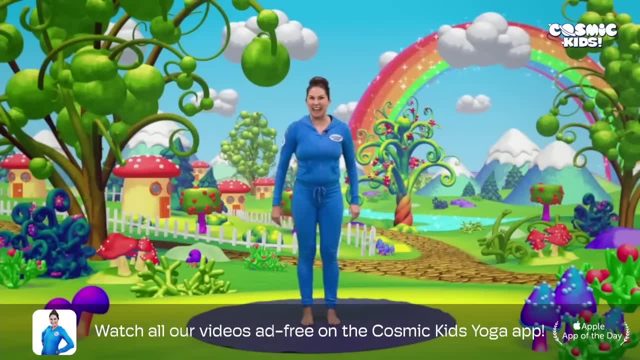 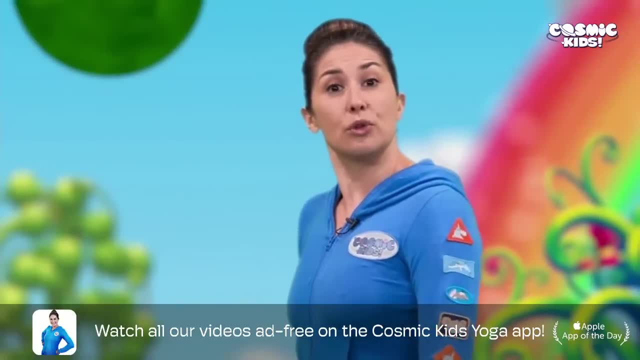 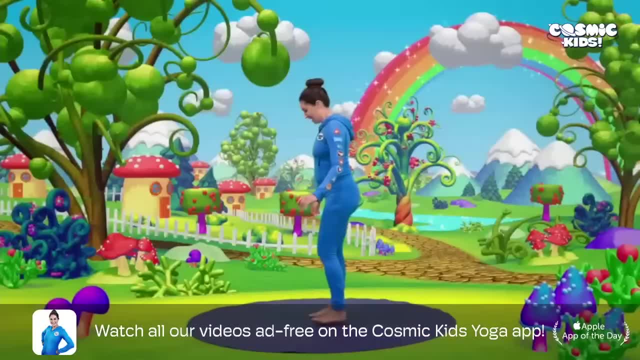 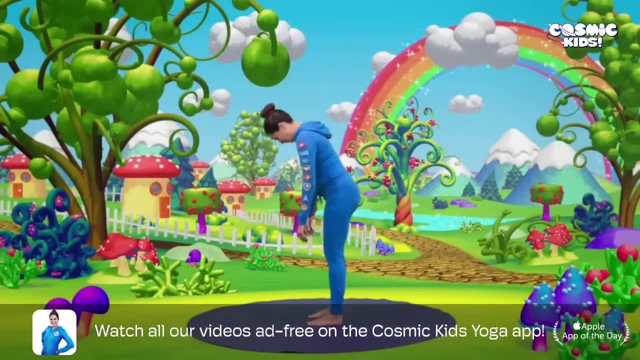 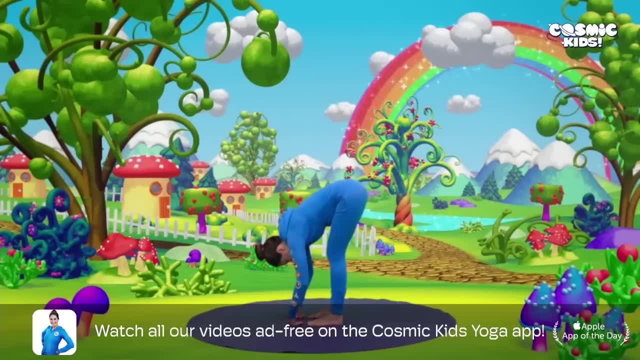 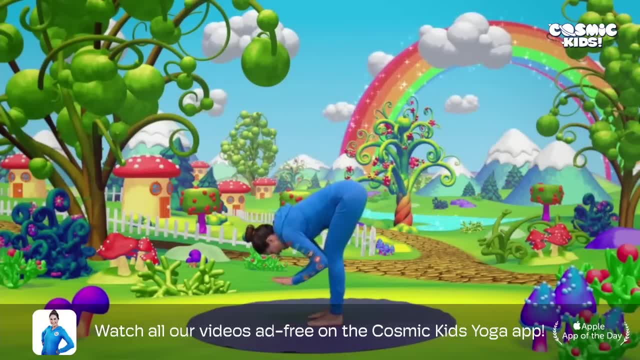 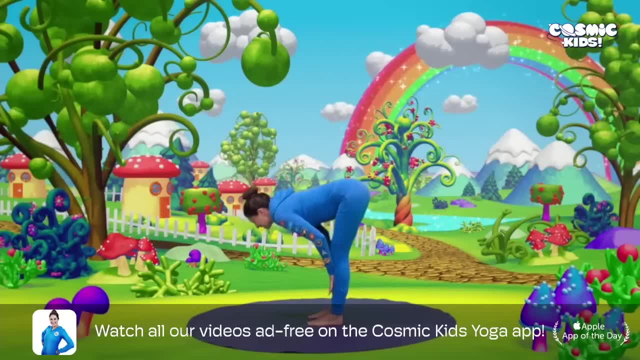 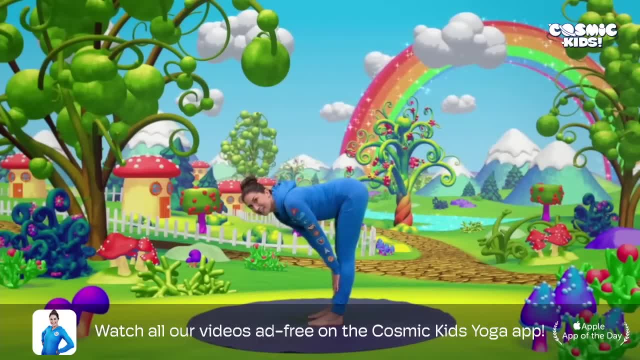 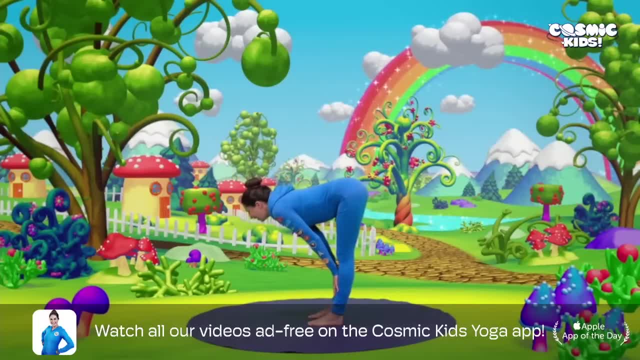 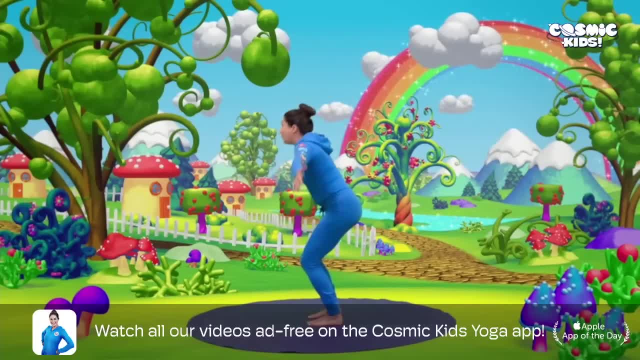 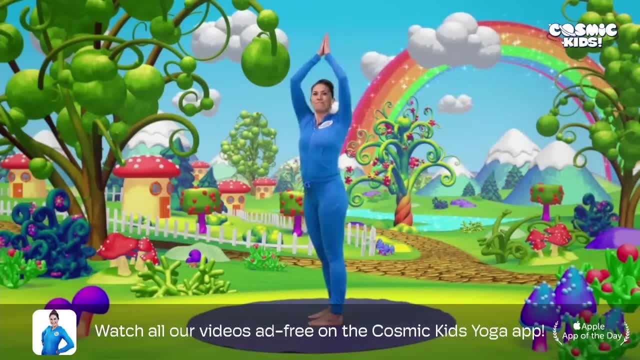 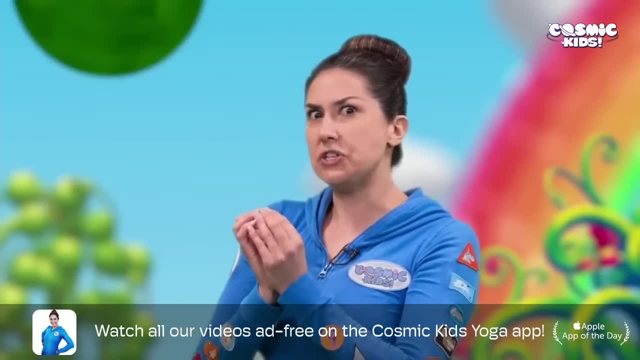 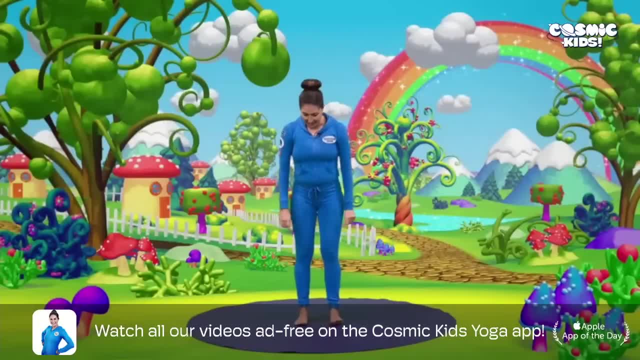 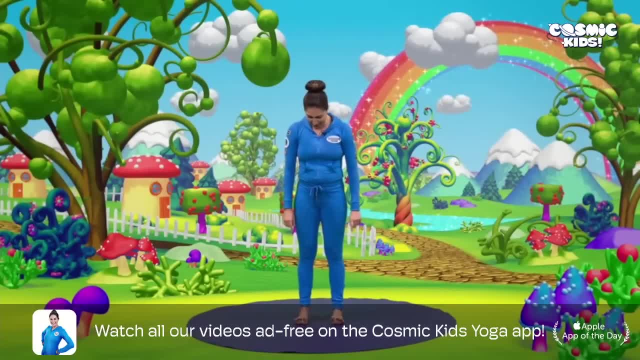 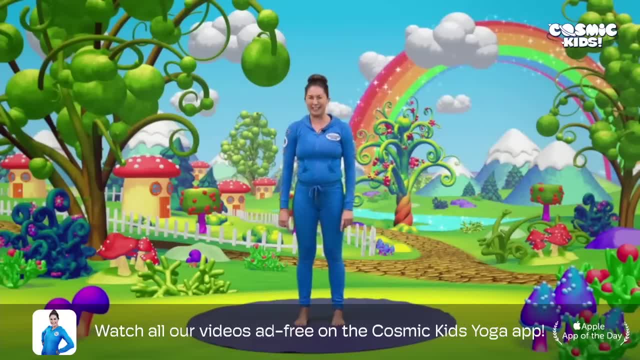 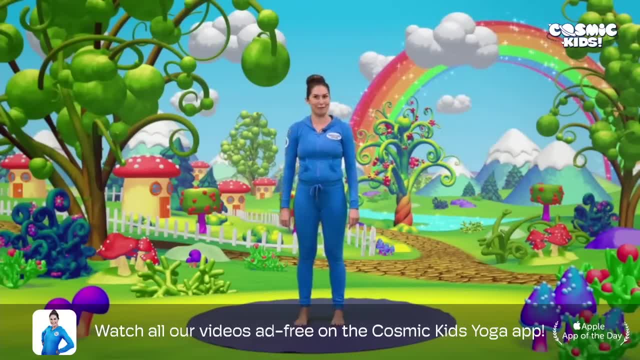 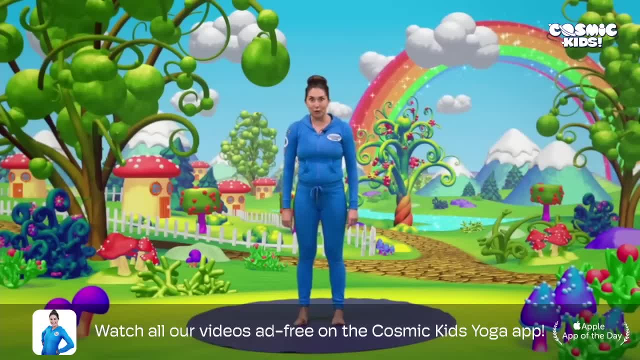 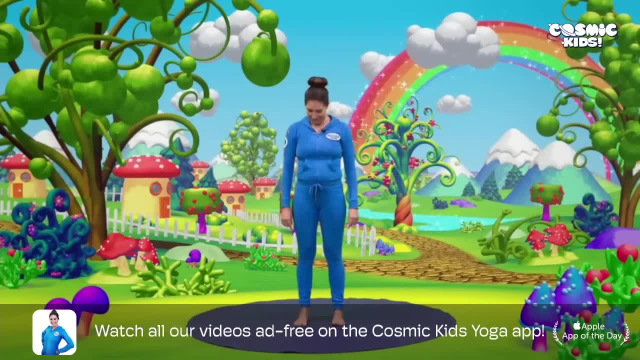 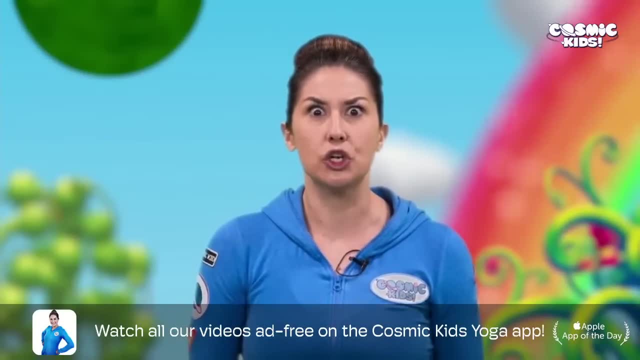 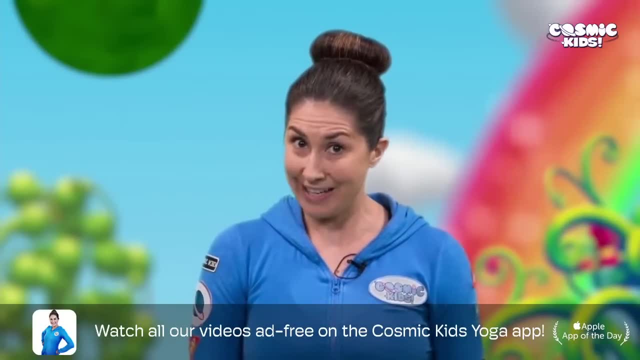 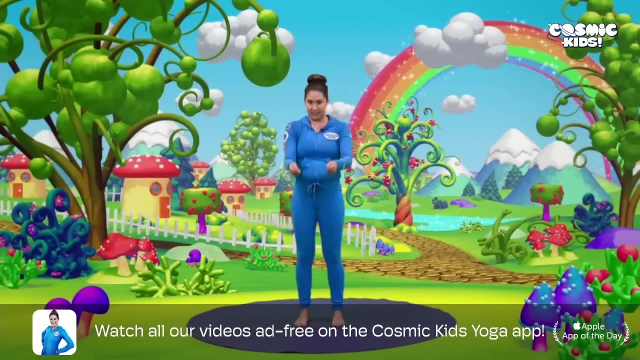 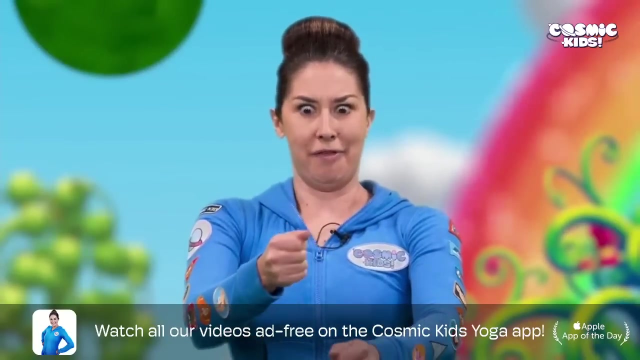 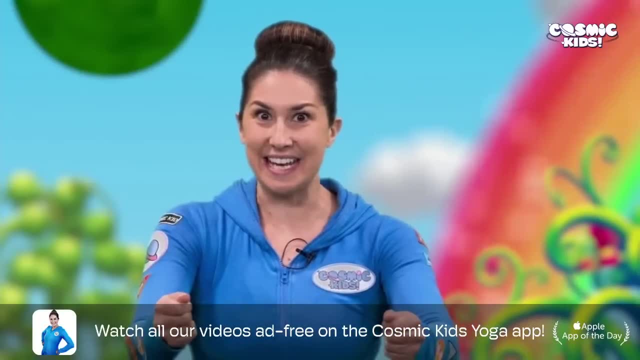 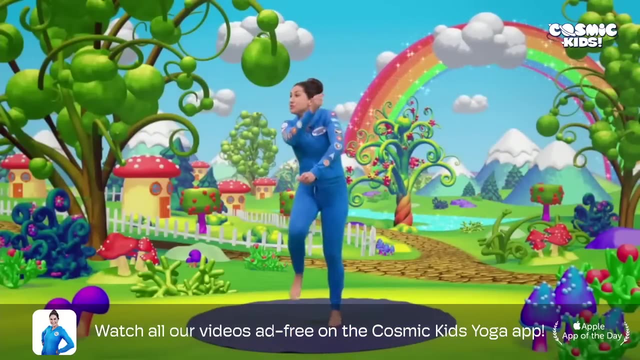 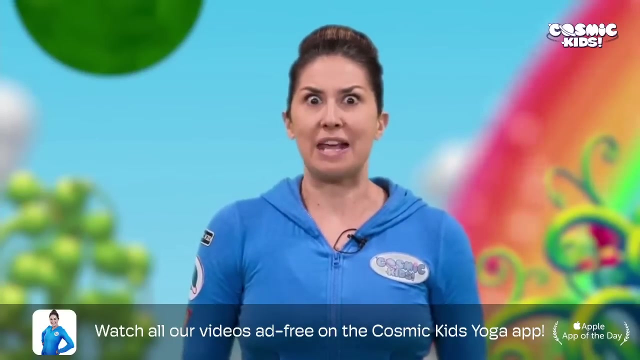 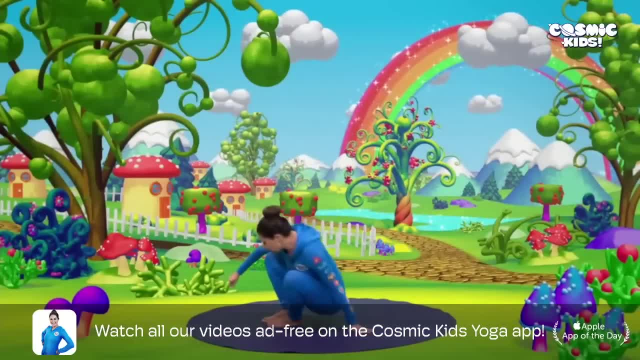 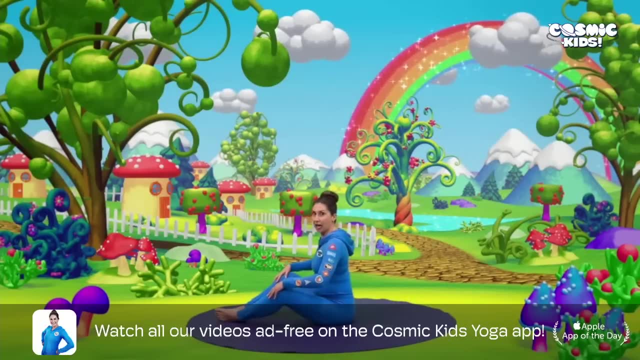 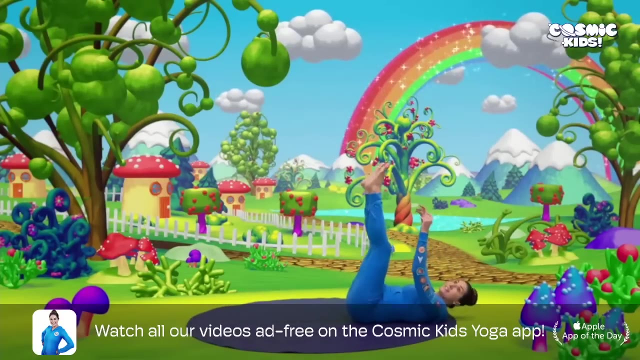 Let's make the huge hole. with our legs Sitting on our bottoms, we bring the soles of our feet together and keep our legs nice and wide, so they're in a hole shape. Biggles falls straight down, Rolling all the way onto our backs, our legs and our arms in the air. And now he's at the 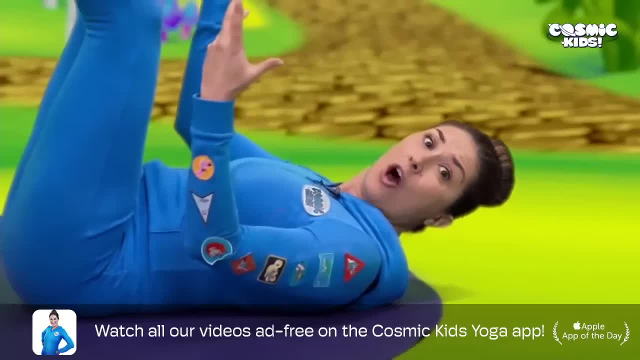 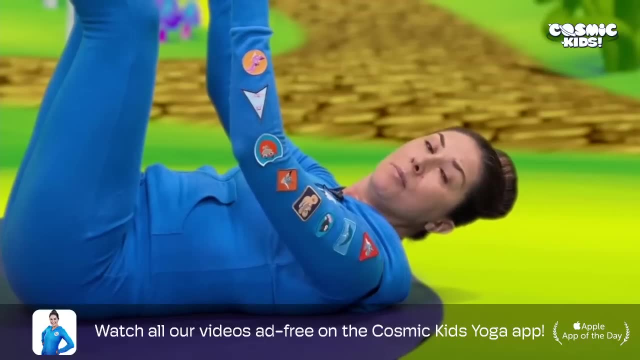 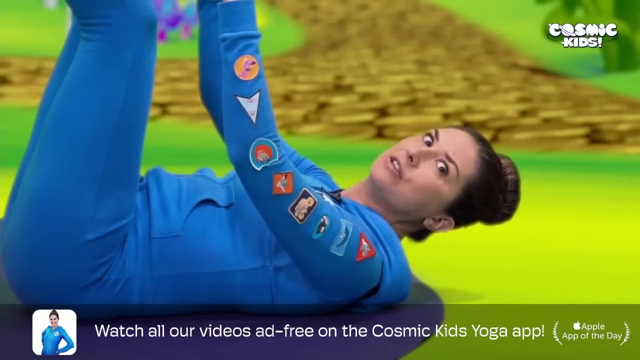 bottom of a deep, dark pit. This hole was a trap covered in branches and leaves set to capture Biggles. People from the nearby village gather round the pit. They crouch to point and shout at Biggles Coming up to our crouch position. everyone, We take our feet a little. 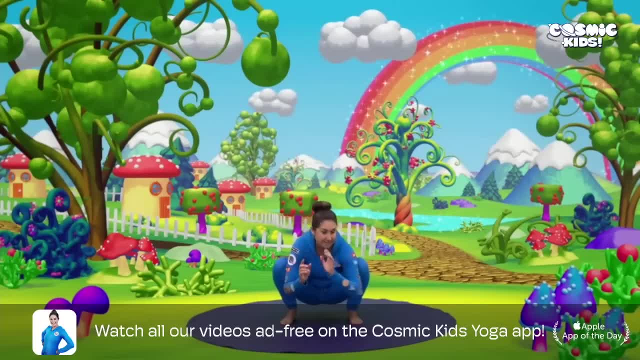 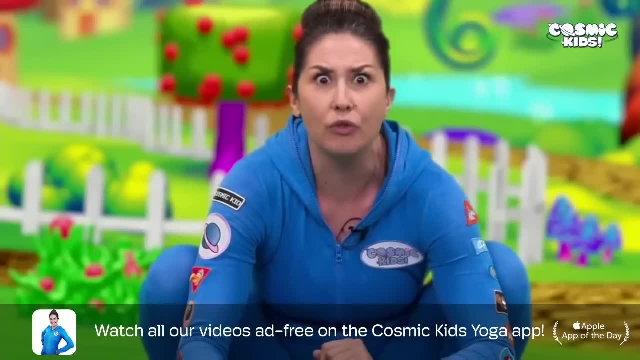 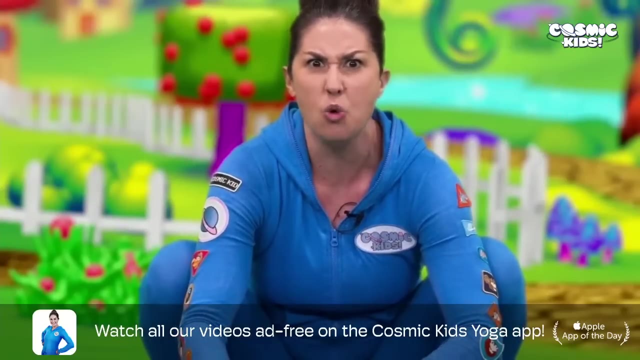 bit wide And we squat all the way down, snuggling our arms in between our legs. They're pointing and yelling at Biggles. Look, We caught the monster. Phew, He's a bit smelly, He looks a bit prickly, He's so ugly. 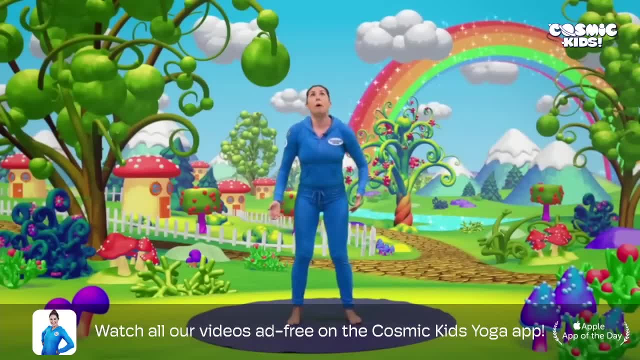 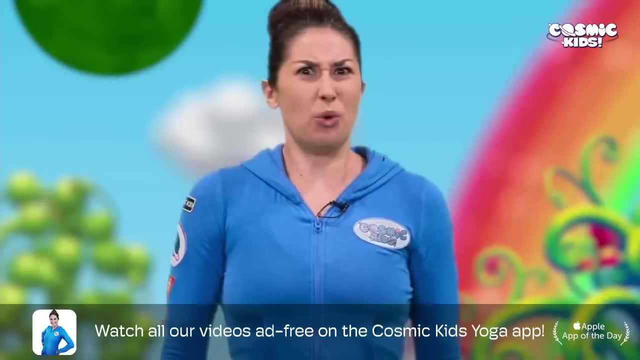 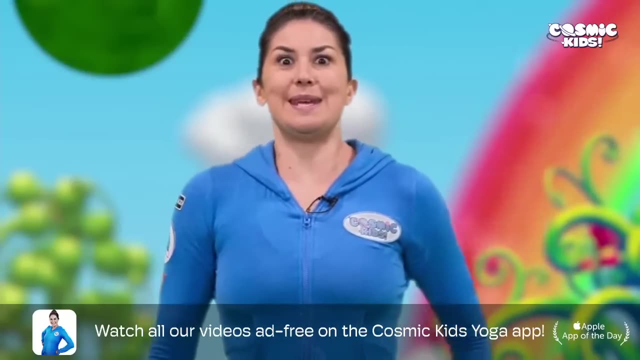 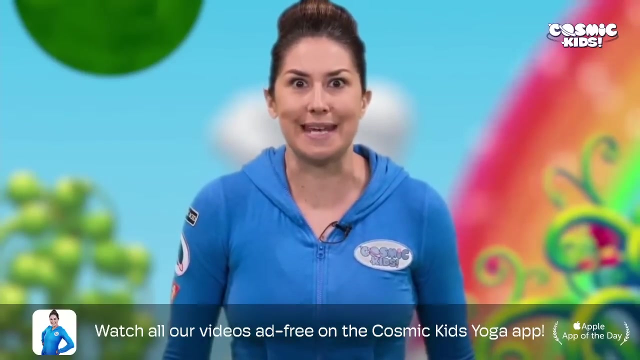 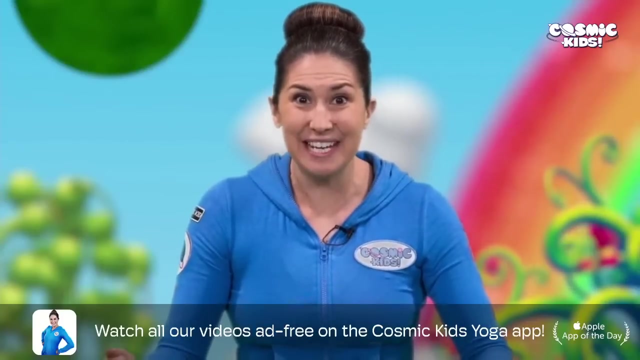 Poor Biggles stands up and he looks up at them with confused and frightened eyes. He doesn't know what to do, He doesn't understand them, So he smiles as best as he can And he says his word, Biggles, And he knocks his sticks together Just to show them how lovely that sound is. 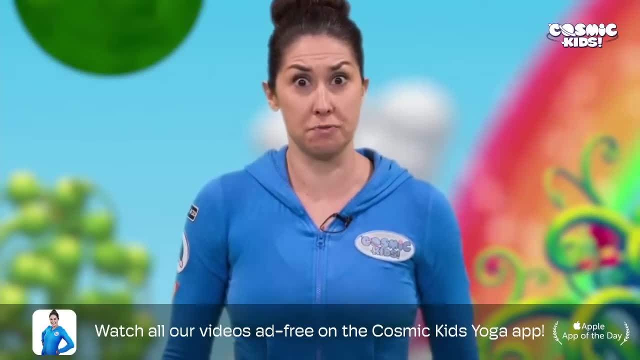 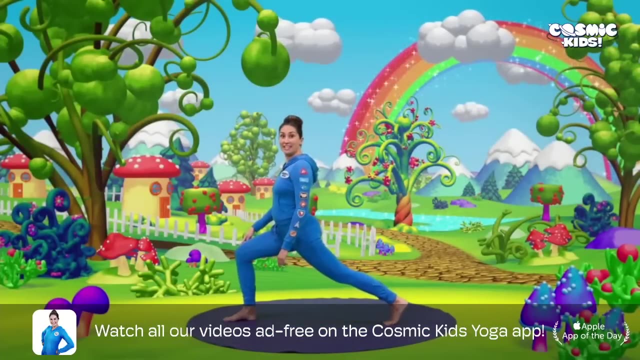 A little boy lunges and throws a rotten mango at Biggles. Turning to the side, stepping one foot forward and one foot back, we bend into our front knee. Now we stretch our arms all the way up, trying not to wobble. as we join our hands above our head, We lean all 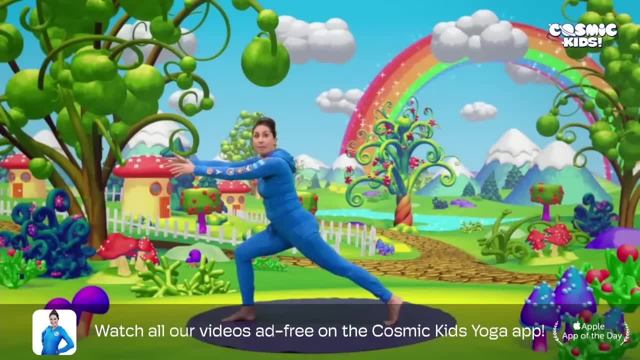 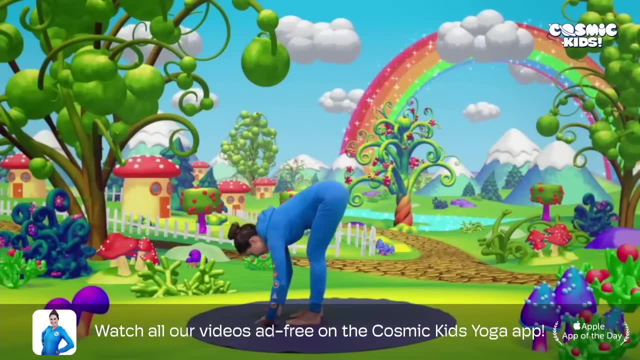 the way back and whoosh, There goes the mango. Biggles steps forwards and folds all the way down to pick the mango up, Crisscrossing our fingers, he lifts it up and he rolls it around. Biggles takes the mango out in front of his chest. He smells it. Mmm, it smells really. 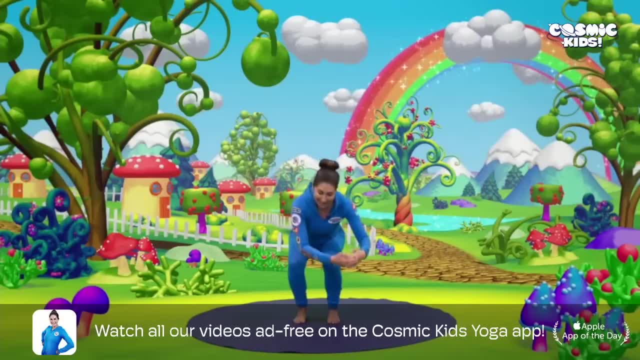 nice. So he bends very gently and he carefully places it beside him to keep it safe, Coming all the way back up to stand. Now the villagers throw even more fruit at Biggles. Let's lunge on the other side. Stepping one foot forward, one foot back, we bend into our front knee. 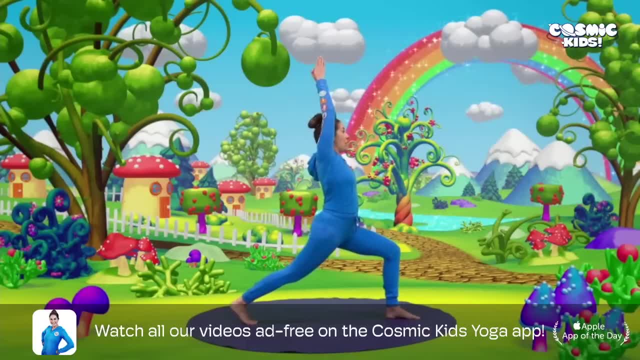 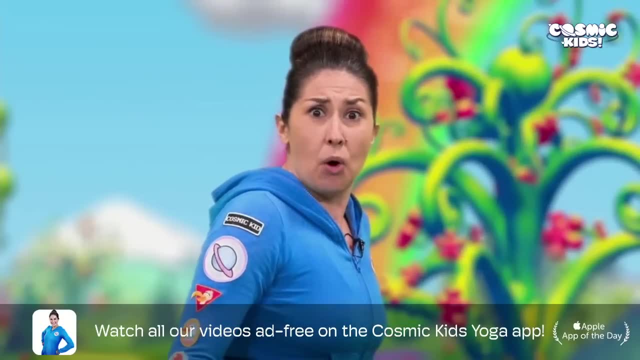 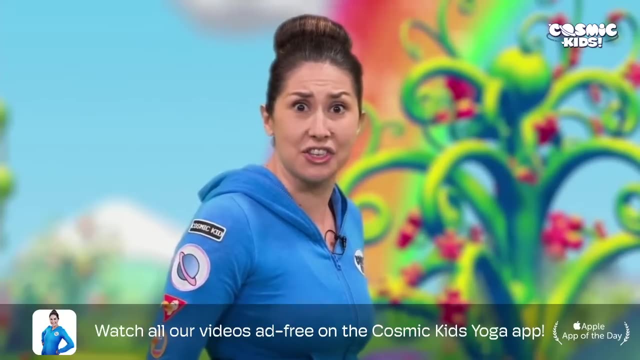 trying not to wobble as we reach our arms all the way up. We lean back and whoosh Bruised bananas and apples- Poor Biggles. But he thinks they're gifts, so he hops from side to side trying to catch them Coming up to stand. and let's hop side to side, Biggles, Biggles. 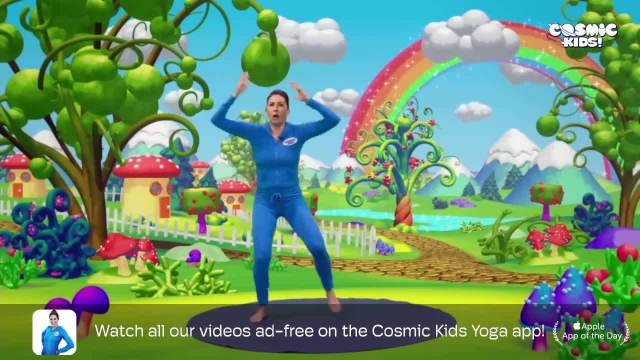 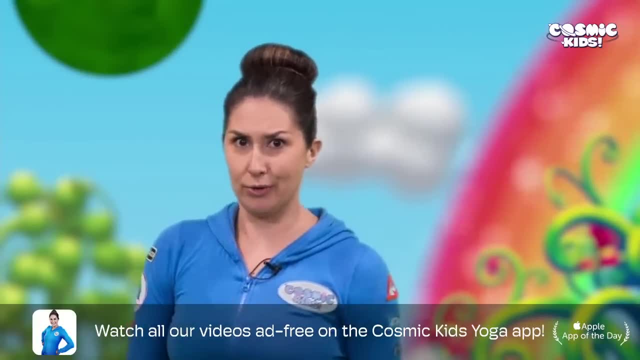 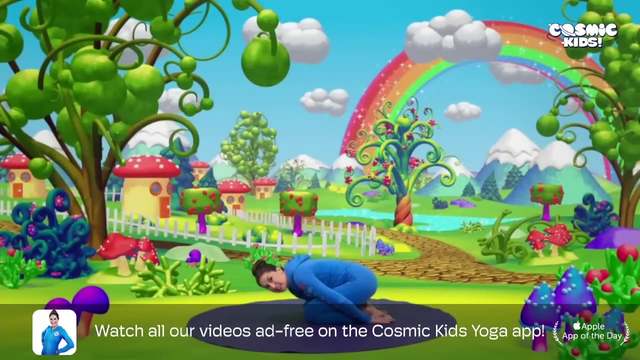 Biggles, Biggles, Biggles, Poor Biggles. They start to throw rocks at him. Let's do our rock pose. Coming down onto our knees, untucking our toes, we fold all the way forwards to make ourselves into a little round rock. 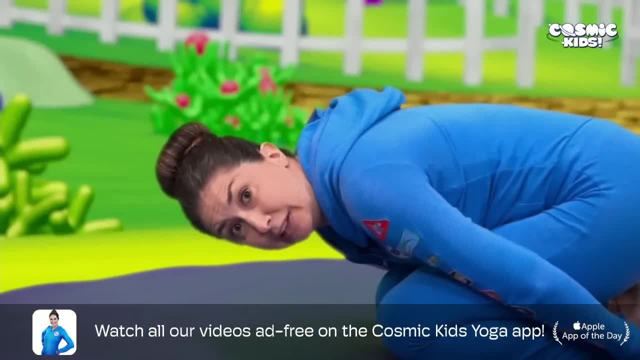 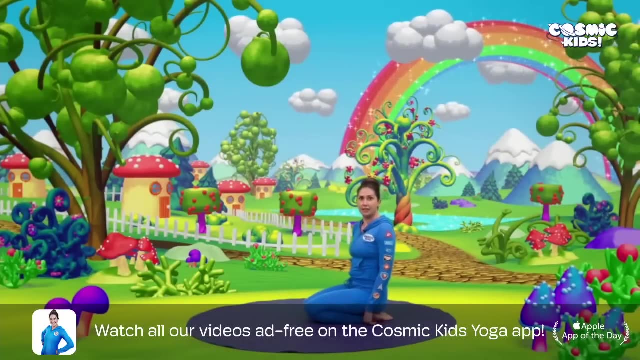 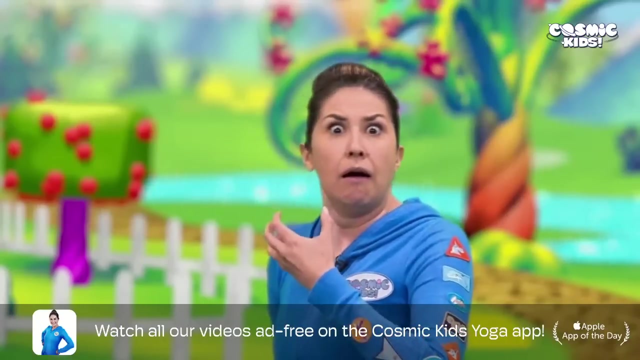 shape. Ooh, one of the rocks hits Biggles in the eye. He sits up and he blinks, He shudders the shock of it. Then he picks the rock up, He has a look at it, He rubs it on his chest and he tries to take a bite out of it. A little girl is on her. 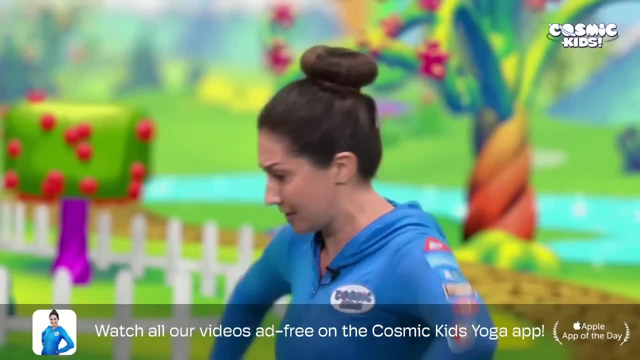 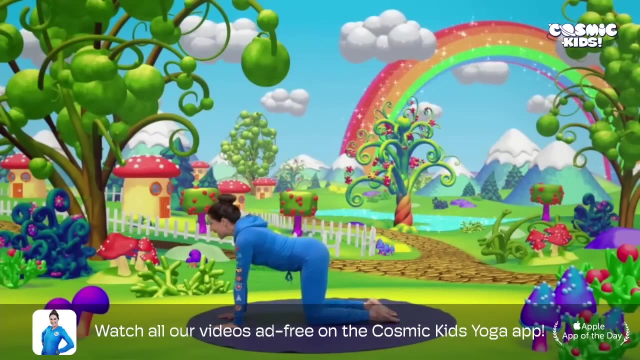 hands and knees pointing and laughing at Biggles Coming onto our hands and knees, stretching one arm forwards to look at Biggles putting that one down and the other arm forwards. She thinks he's very funny for trying to eat the rock, but she's laughing so much that 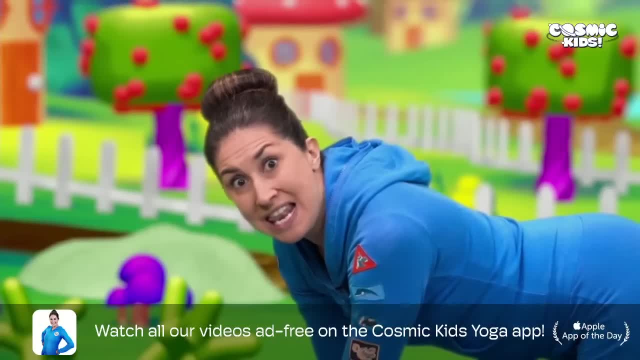 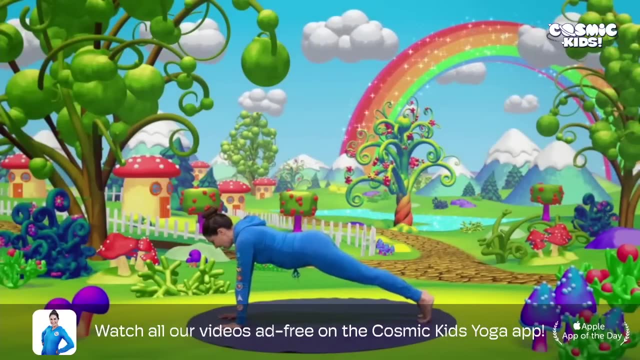 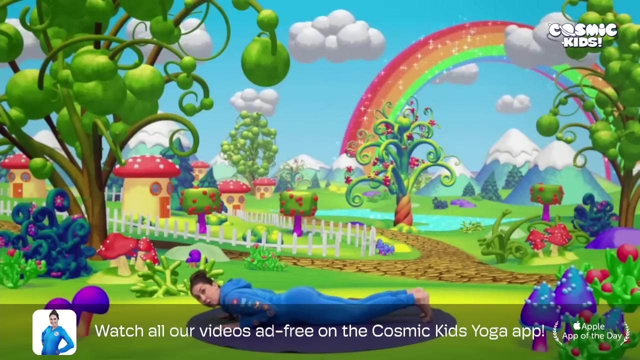 she slipped And she falls down the hole, landing on her tummy. We stretch one leg back and stretch the other leg back. Now we lower our knees and slowly lower onto our tummy. Oh no, now she's at the bottom of the hole with Biggles. 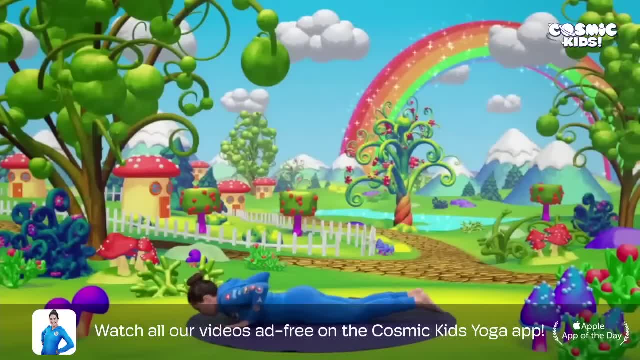 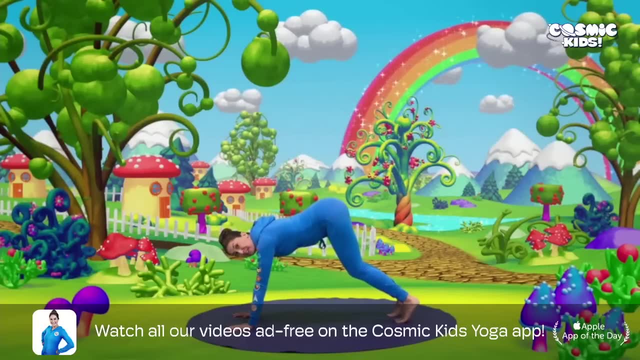 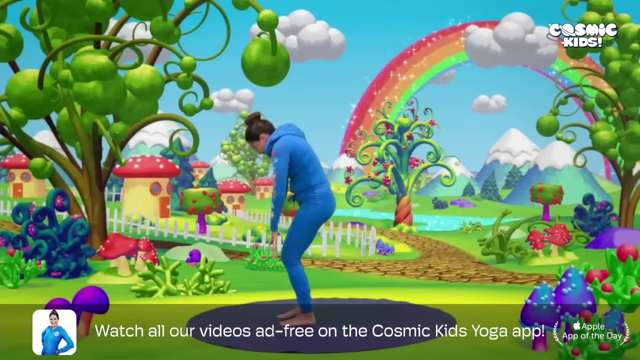 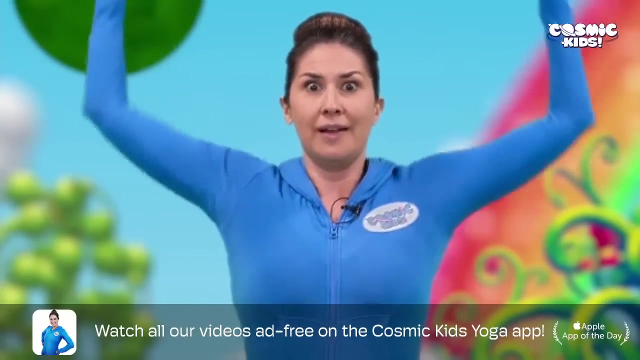 The little girl's mum jumps up and screams, Coming up onto our hands and knees, tucking our toes and pressing our hips. Now we jump our feet forwards, towards our hands, Ready, One, two, three, Boing Rolling up to stand. she reaches up: The monster has my child. What are we going to do? Everyone? 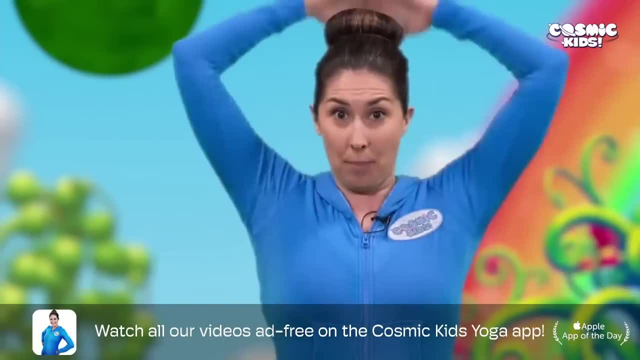 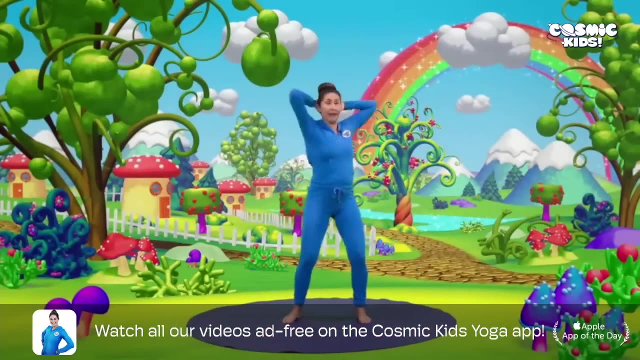 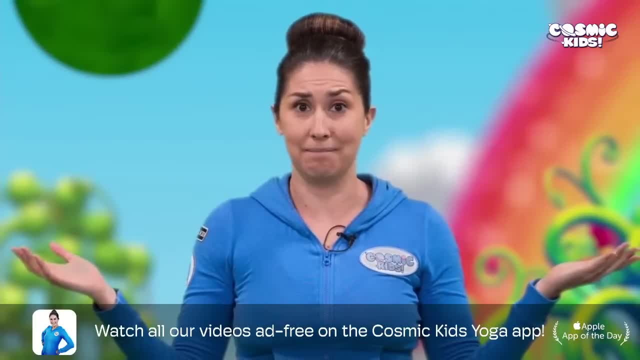 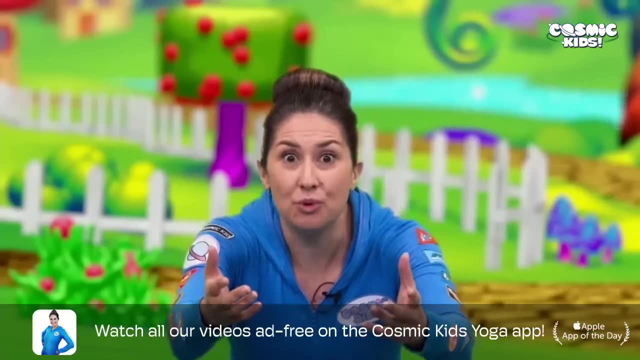 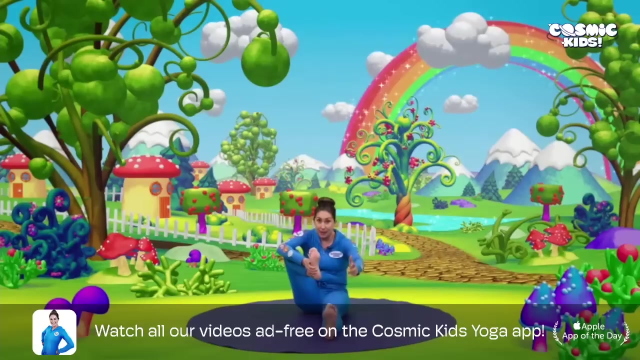 her to pieces. He'll tear her to pieces. He'll tear her to pieces. But Biggles does no such thing. He sits calmly with his legs out long in front of him And he reaches forwards towards the little girl, checking that she's OK. He picks her up. Let's pick up one of. 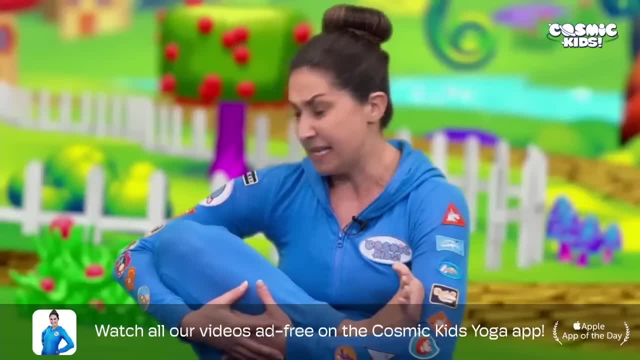 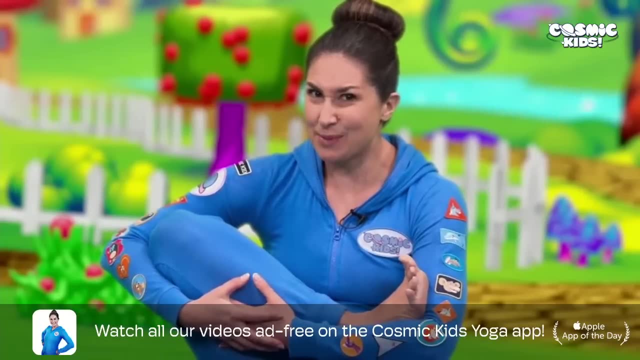 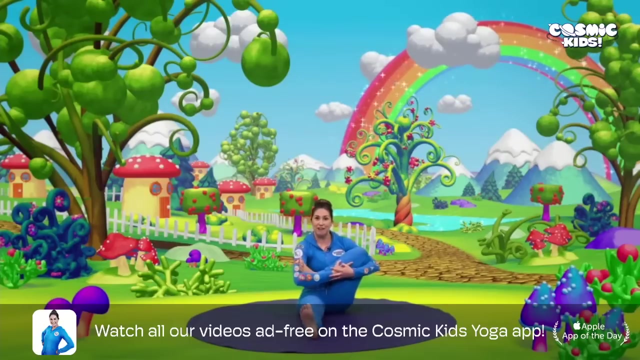 our feet and cradle it in our arms. He's a bit worried about her. That was quite a big fall, But she seems to be OK. Let's switch sides: sides, popping that foot down, picking up the other side, tucking it into our elbow and cradling on the. 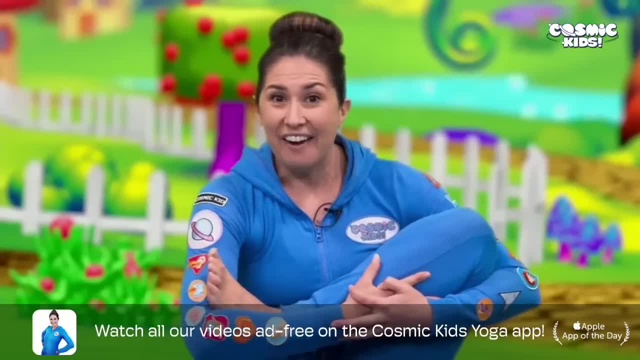 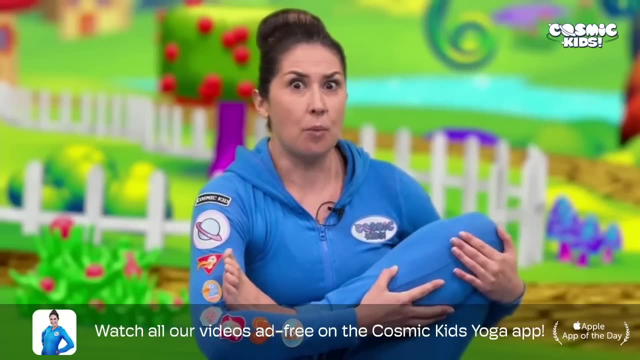 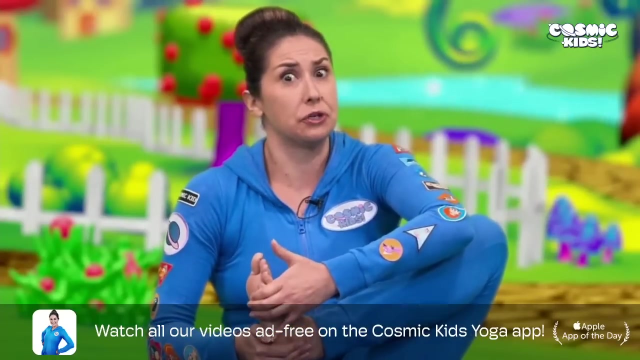 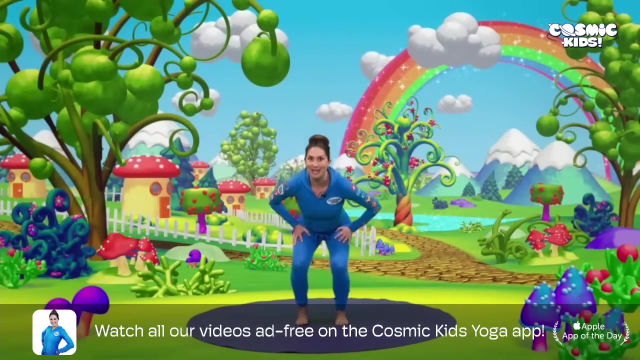 other side with his big green, hairy hands, Biggles strokes her head, checking she's okay. someone shouts down from the top of the hole: give her back. Biggles does so or tries to right away putting that foot down. we come up to stand now. we bend our knees nice and deeply reach our arms forwards. 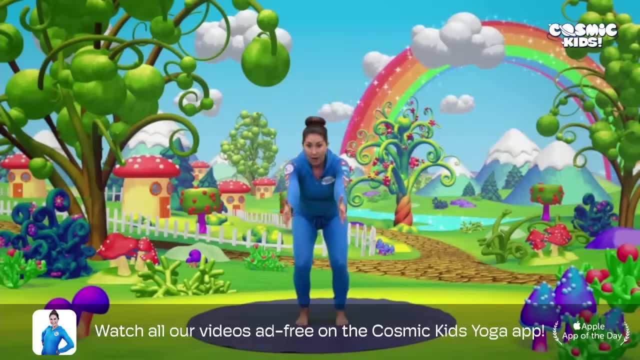 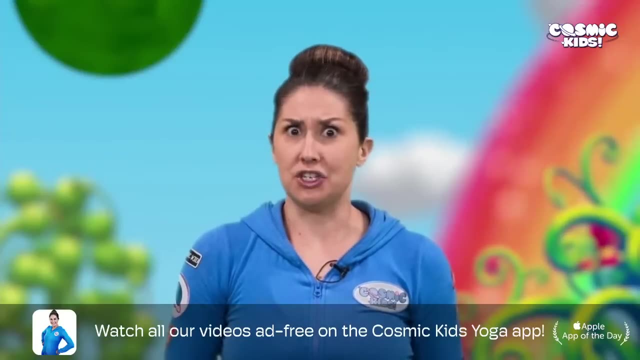 like we're holding the little girl and as we come all the way up, he lifts, lifts lips up onto his tippy toes, trying to get the little girl to the villagers at the top of the hole. coming all the way back down onto our feet, the villagers fold forwards, folding all the way down. 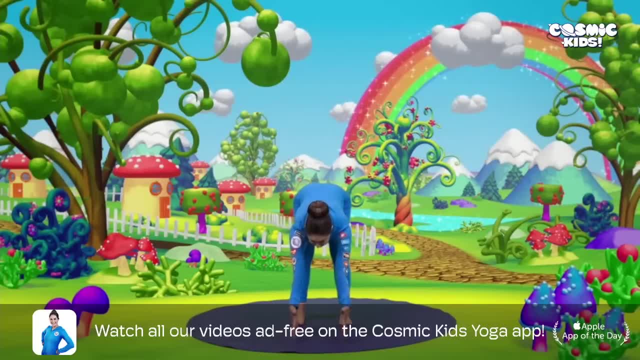 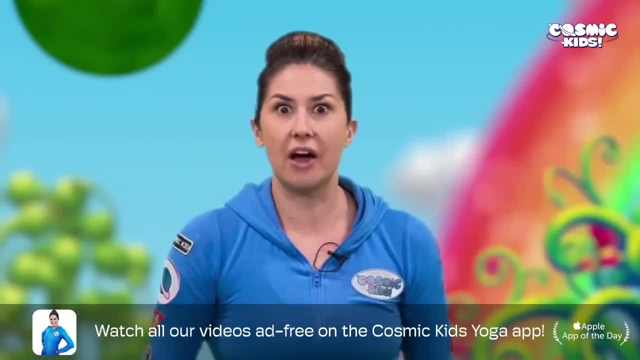 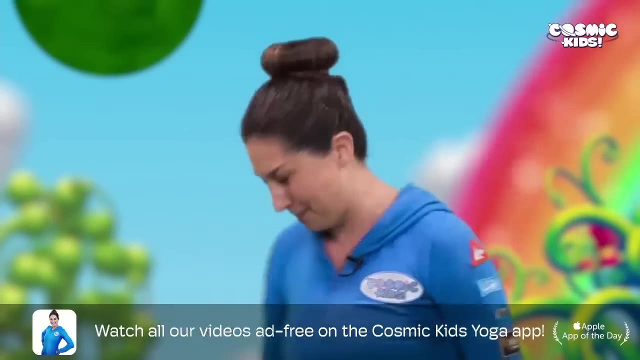 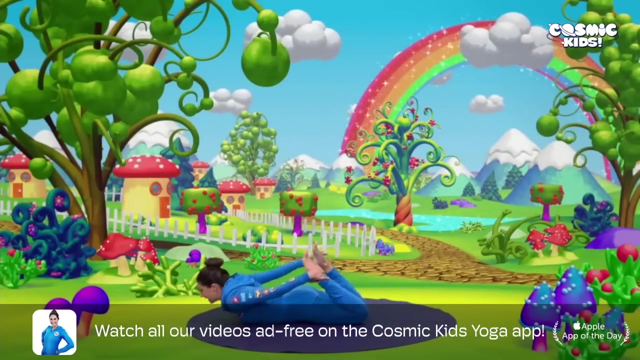 reaching down towards her to try and reach, but it's just too far rolling up to stand. next, someone has an idea: let's fetch a basket with a rope attached to it, coming into our basket pose, coming down onto our tummies, we bring our feet towards our bottoms and we reach around to take. 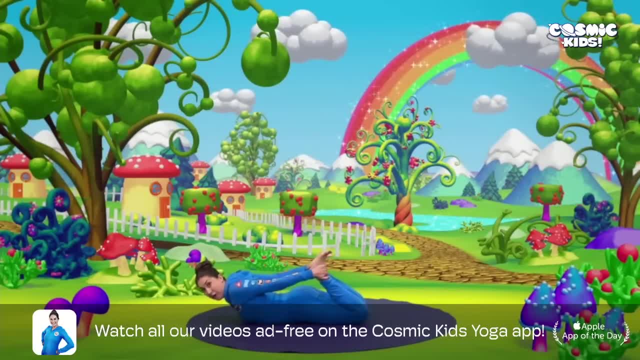 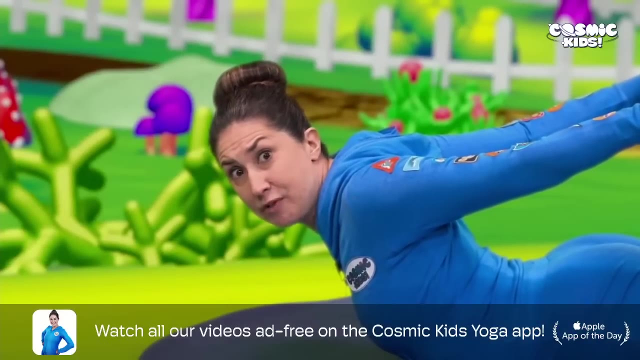 our ankles. now let's breathe in. kick our feet into our hands. here we go in our basket pose. they're going to lower it down to get the little girl out. but some are worried: what if Biggles leaves the little girl in the pit and climbs up the rope himself? but Biggles does no such thing. he carefully and gently helps the 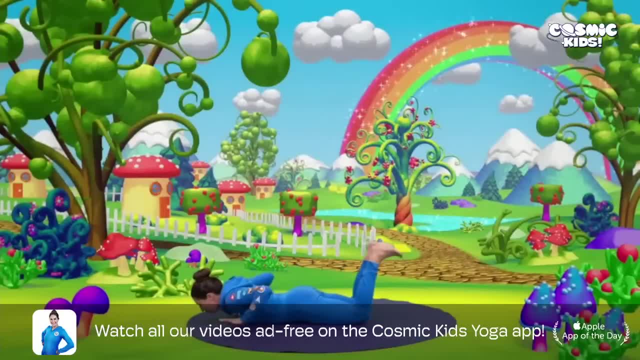 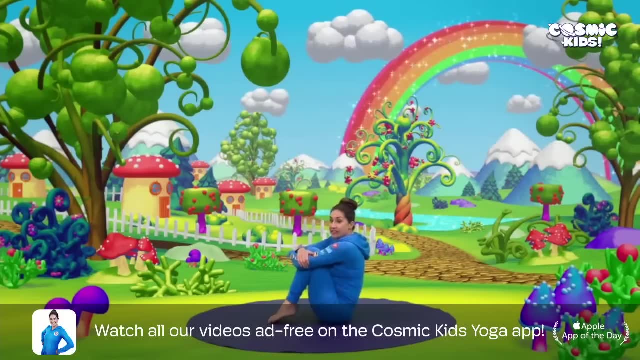 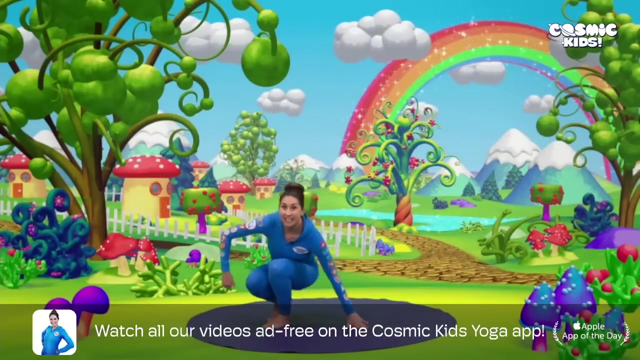 little girl into the basket, coming all the way to sit on our bottoms. we hug our knees into our chest and we push her down onto our legs and push her into the basket, wrapping her arms around her knees, and she's ready to be hoisted up to the top of the pit. now, once at the top of the hole, 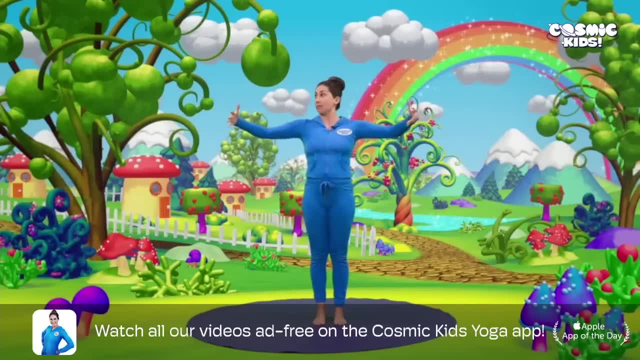 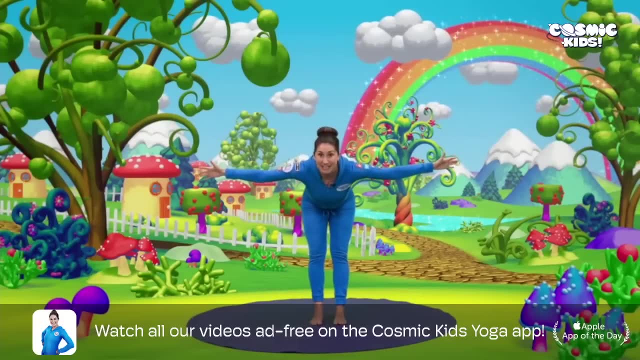 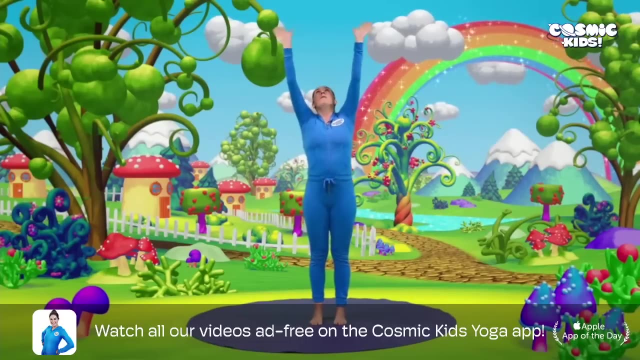 the little girl is out and she is safe. but instead of opening her arms out wide and turning to her mother, she falls all the way forwards towards Biggles. Biggles reaches all the way up at her, saying Biggles, And he plays his sticks again. 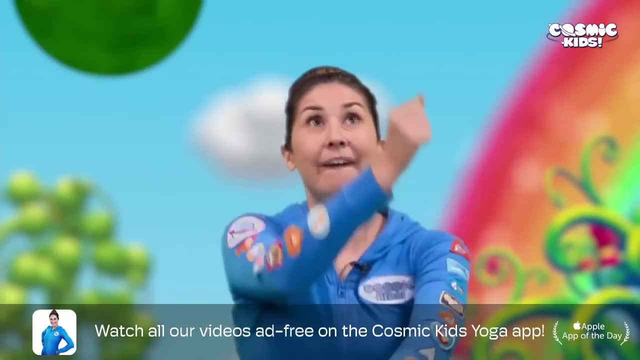 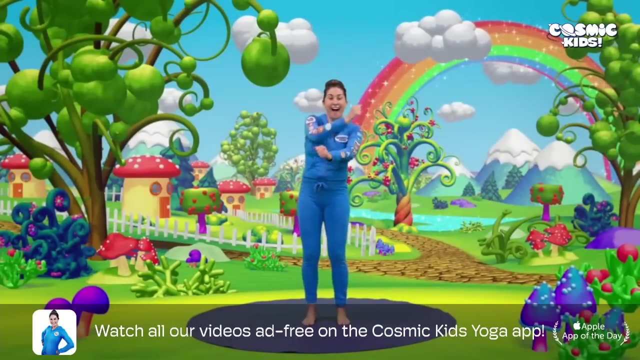 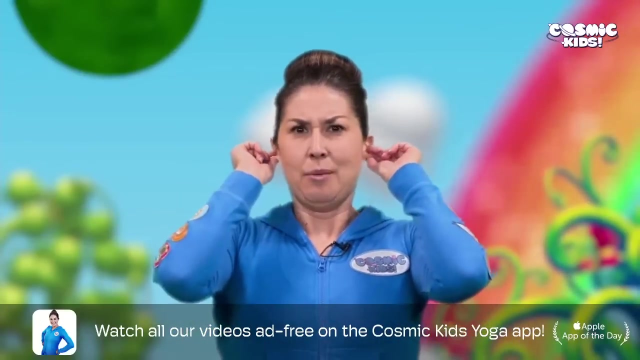 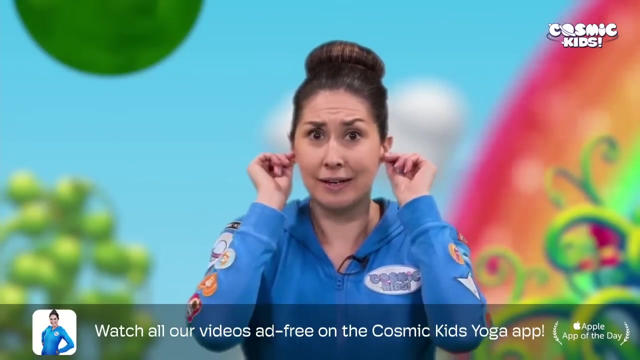 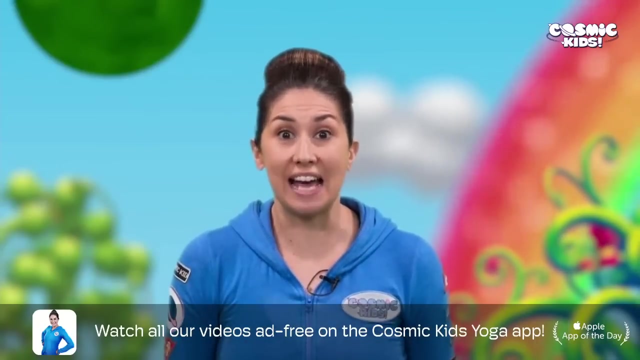 this time playing a little tune. The villagers listen, rubbing our ears. Wow, This monster is actually very clever and seems to have a kind heart. He did save the little girl. They decide to let him go. They throw a ladder down to him. 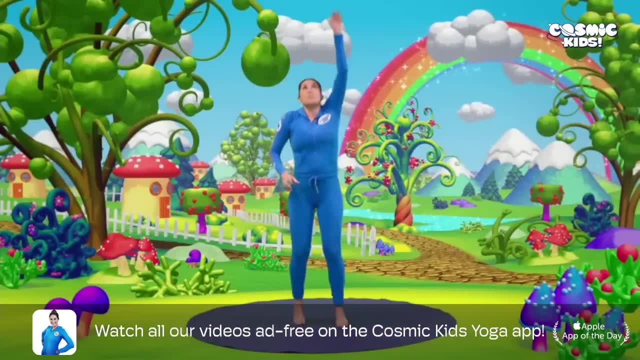 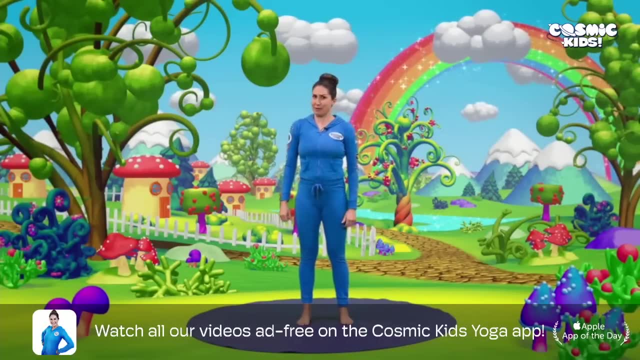 and he climbs up, Biggles, Biggles, Biggles, Biggles, Biggles, Biggles, Biggles. Once at the top, the villagers stroke Biggles. Let's stroke our arms and stroke our legs. They love his green, spiky hair. 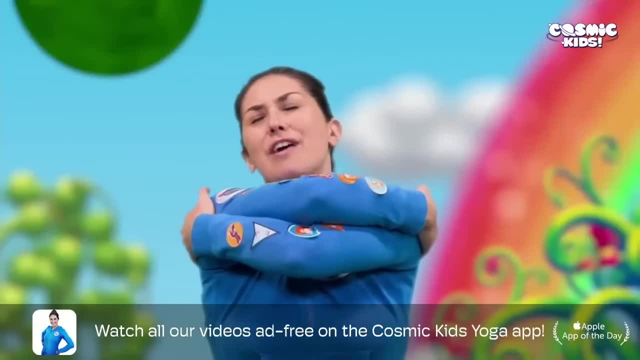 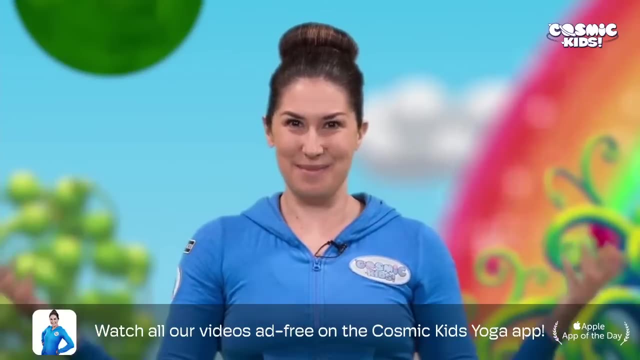 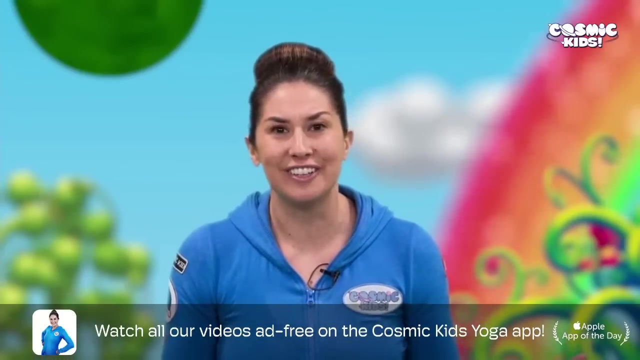 Then they give him a big hug, arms wide, wrapping our arms around. They give him lots of lovely fresh fruit to eat and they welcome him into their community. Now Biggles might look like a monster, but he's kind and thoughtful and sensitive, just like you. 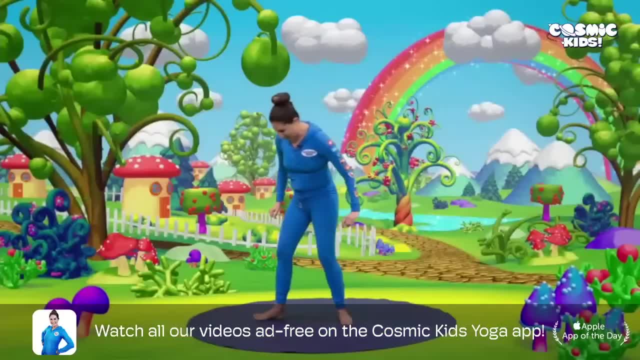 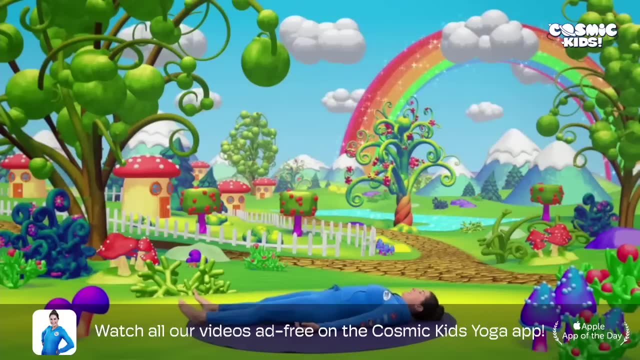 Let's spend a moment now lying down, coming to lie on our backs, legs long, arms down by our side, and take a moment to rest, relax and have a little think about our story, about Biggles the Monster. We take a big, deep breath. 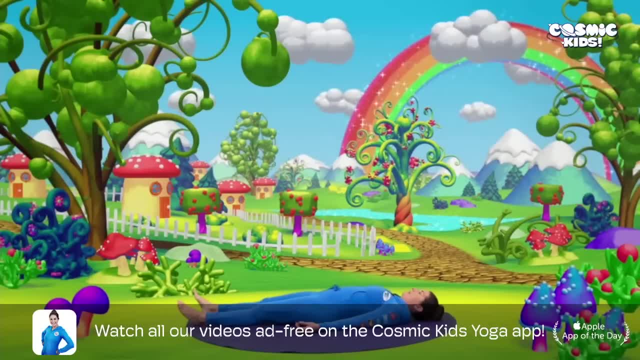 in through our nose and out through our mouth, And again in through our nose and out through our mouth. What an interesting story. Sometimes, when someone appears different to us, we might be afraid of them unsure. But as we've learnt in this story, 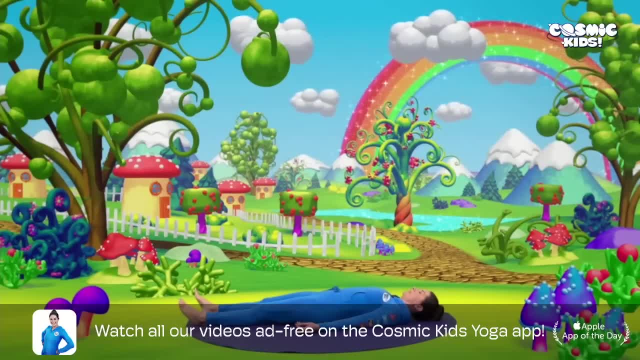 that's probably not the right thing to do. In fact, just because someone is different doesn't mean we should be unkind. It means we should be even more kind. We should get to know each other, learn to understand the world from someone else's point of view. 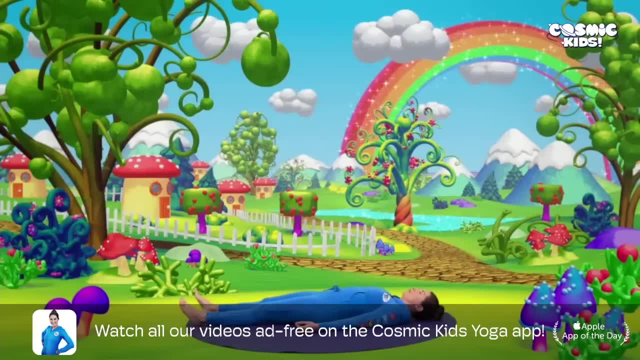 In our lives we will meet lots of different people who are very different to us. Be kind, Be thoughtful And do your best to make friends. Slowly, now we begin to wake up, Wiggling our toes and wiggling our fingers. 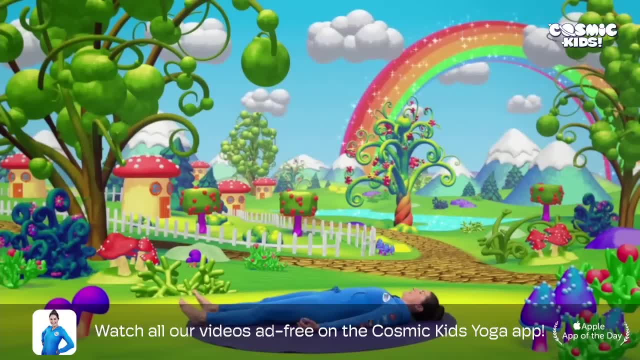 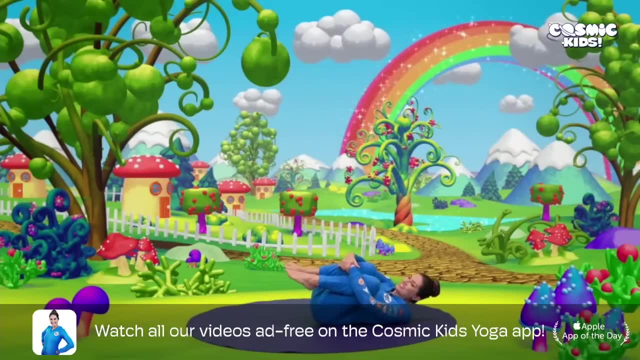 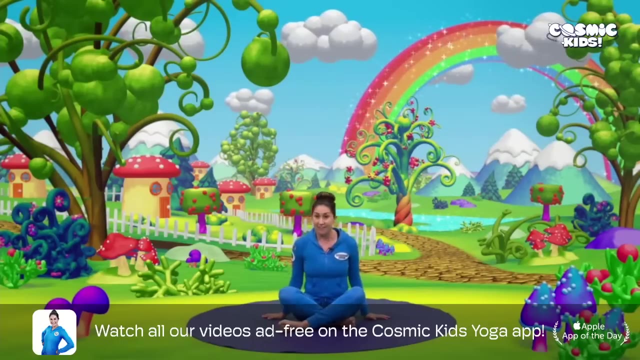 Hugging our knees into our chest and then rolling onto our sides as we open up our eyes and come to sit with our legs on our shoulders, And as we do that, we begin to wake up With our legs crossed, Finishing just the way we started. 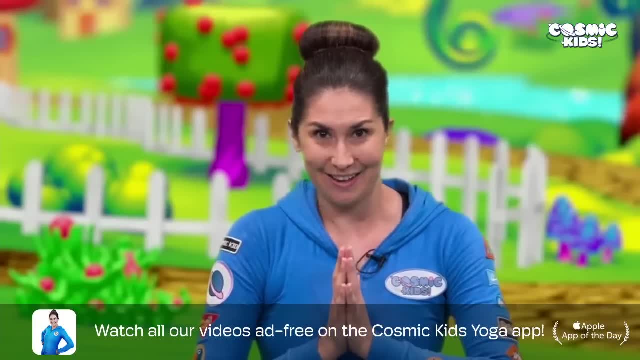 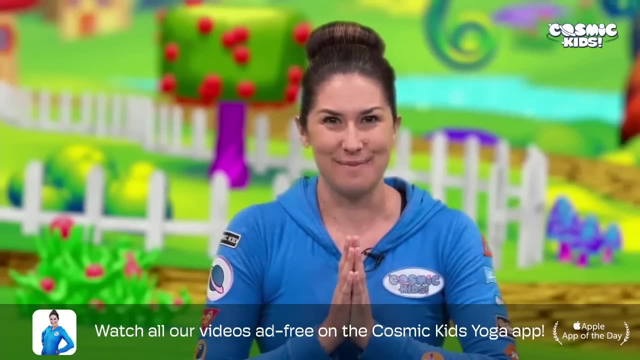 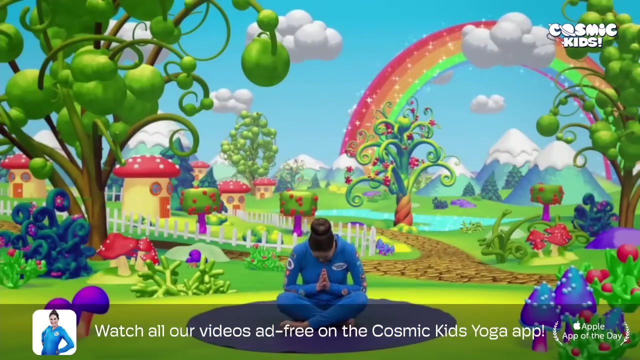 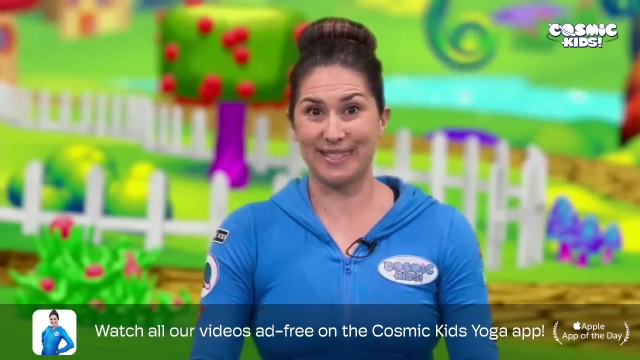 With our hands together at our hearts and our secret yoga code word, Which is Namaste: Ready After three. One, Two, Three, Namaste. Wow, You were great in the story about Biggles the Monster. I hope you enjoyed it. 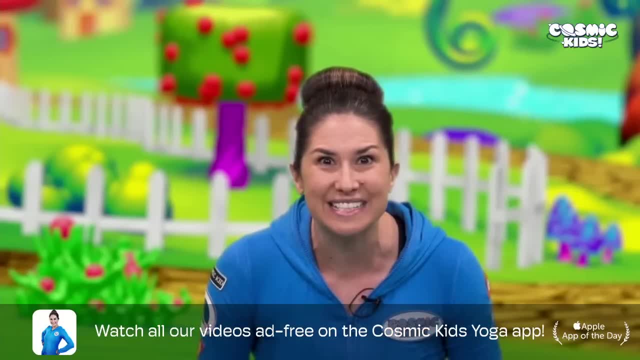 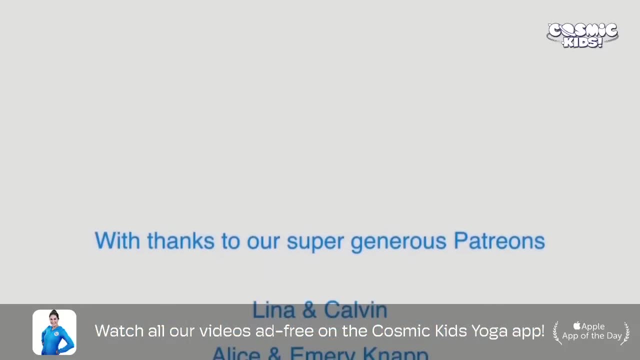 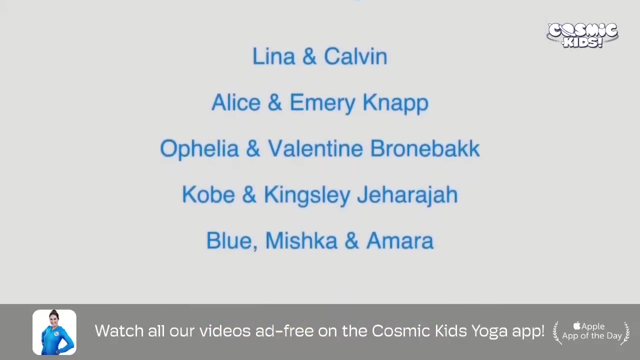 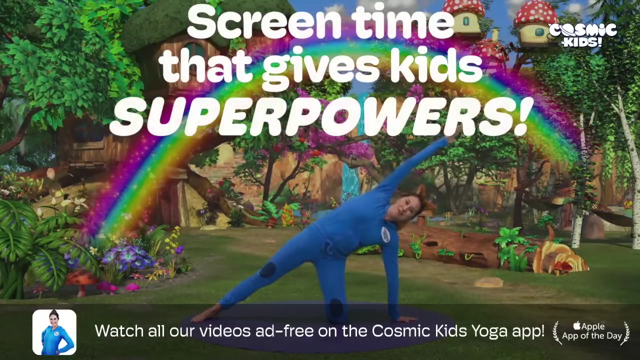 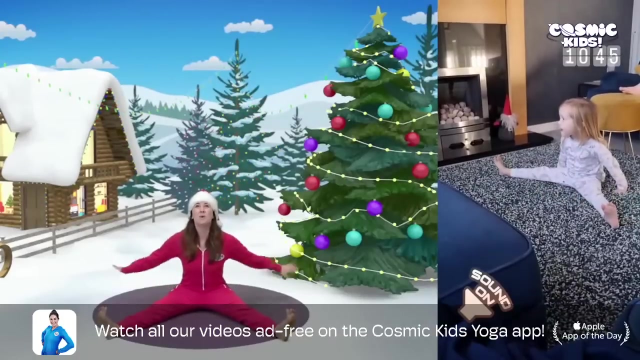 And I hope to see you again soon for another Cosmic Kids adventure. Bye, bye. Sweeping our top arm up and over, Making the most beautiful rainbow we can, Here we go, Whoosh, We take our legs out wide. We reach up very high for a big pot. 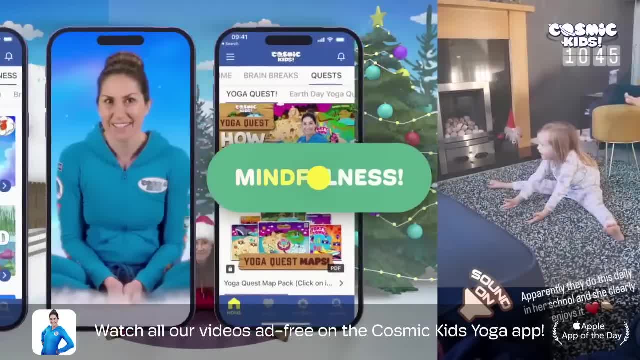 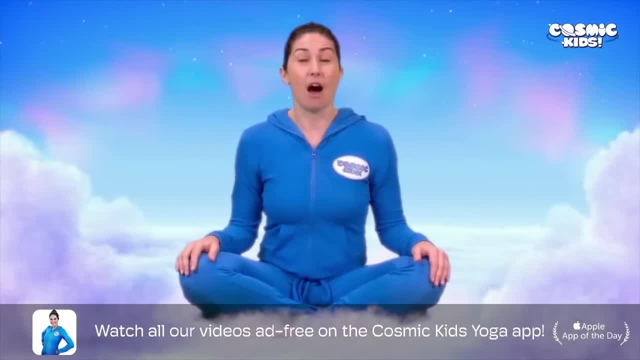 And we pop it down all the way in front of us. So what is it? What is mindfulness? How do we do it? And the best way to make the I can't thought go away is to think: oh yes, I can. 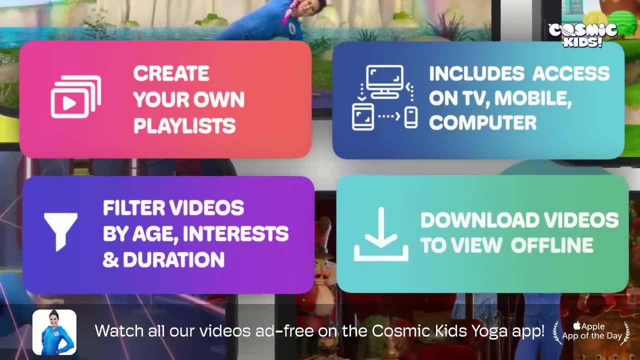 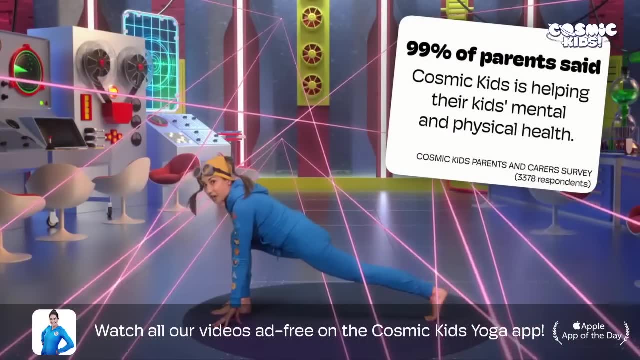 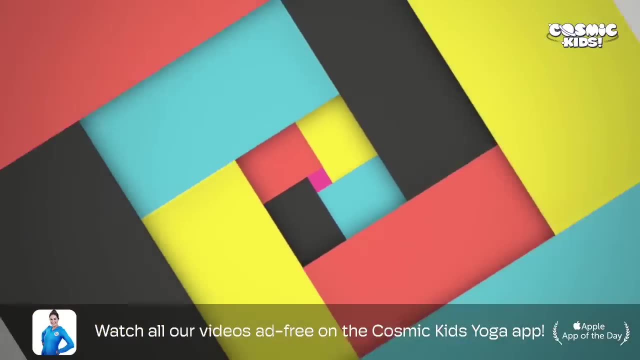 We step forward between our hands- Oh, thank goodness we do yoga Now, making our legs very strong. We lift all the way up, trying not to wobble, Lifting our arms up to the sky, And then we fold all the way forward. 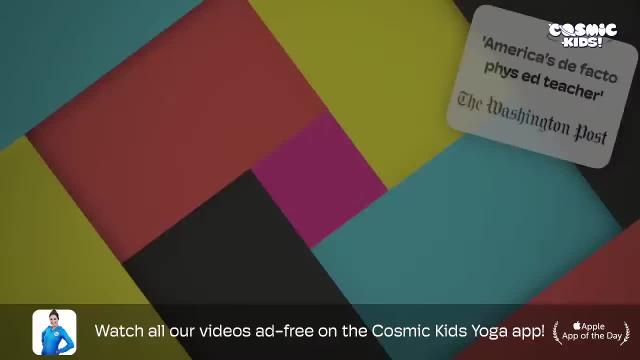 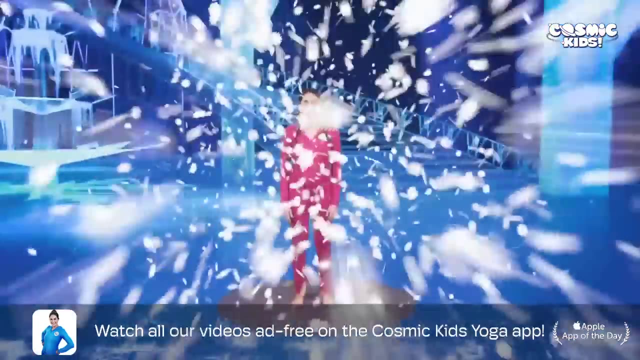 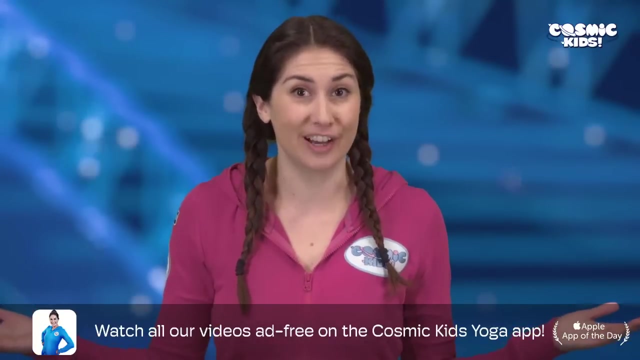 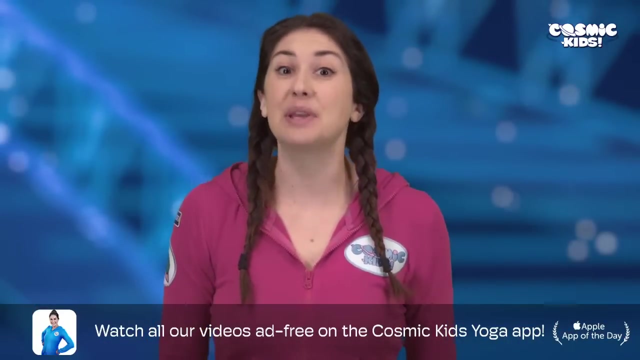 Hands come either side of our foot. Hello everyone, Welcome to Cosmic Kids. I'm Jamie and this is your place for yoga stories and fun. It's easy: Just copy the moves I do and enjoy the adventure. Now we always start in the same way. 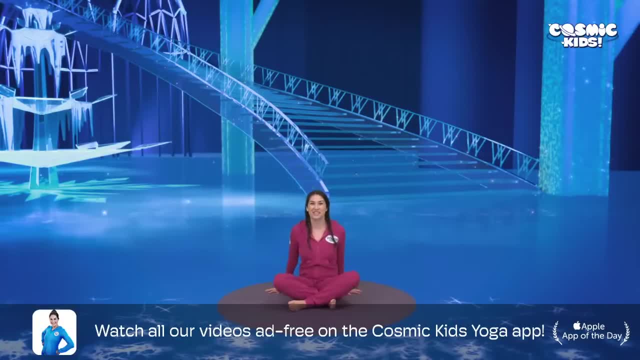 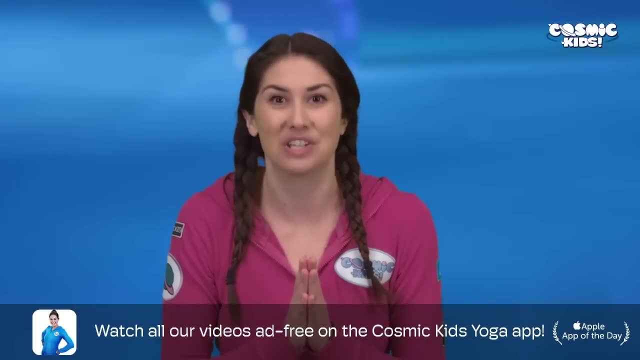 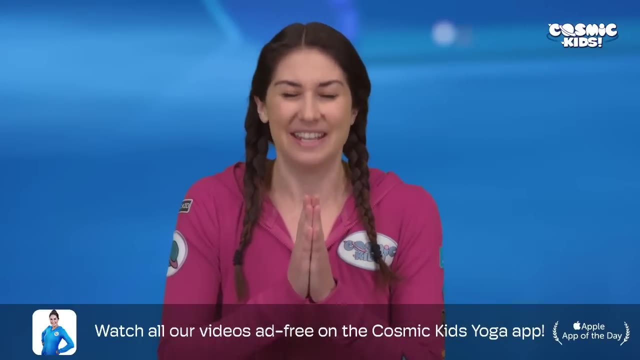 and that's by sitting on our bottoms and crossing our legs and bringing our hands together at our hearts and saying our secret yoga code word, which is Namaste Ready After three, One, two, three, Namaste There. Now we're ready to begin. 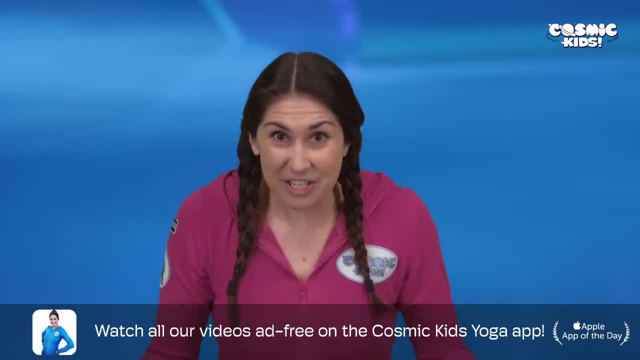 And today we've got a special episode: We're doing Disney's movie Frozen. So we're off to Arendelle to meet a pair of princesses called Elsa and Anna. Let's get ready for the snow. with a hello snow, We stand up. 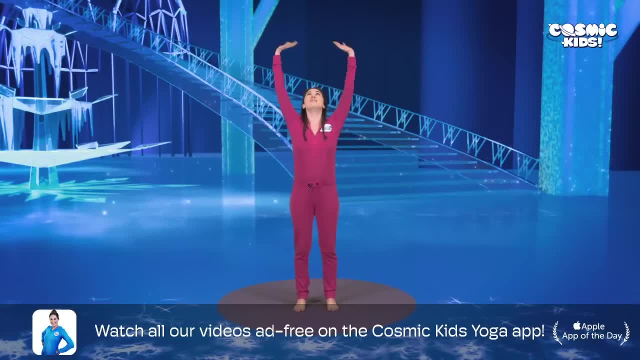 and reach up to the snow Saying hello snow. Then we fold all the way forwards, bending our knees a little bit if we need to, to say hello to the frost Ready, Hello frost. We step one leg back behind us, big, long step, and we pretend to be an ice skater. 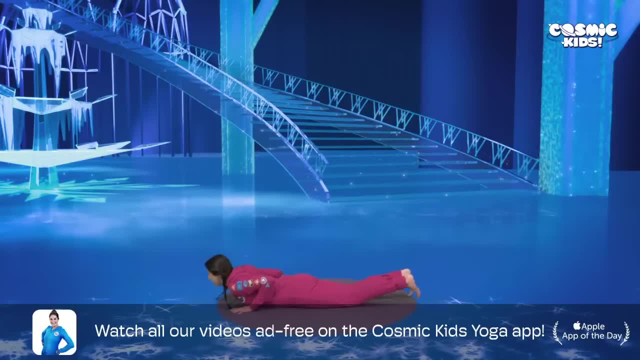 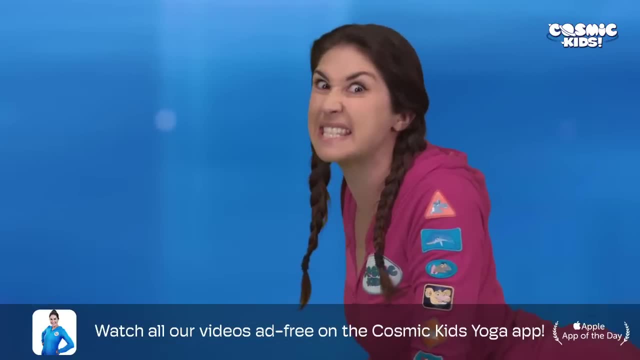 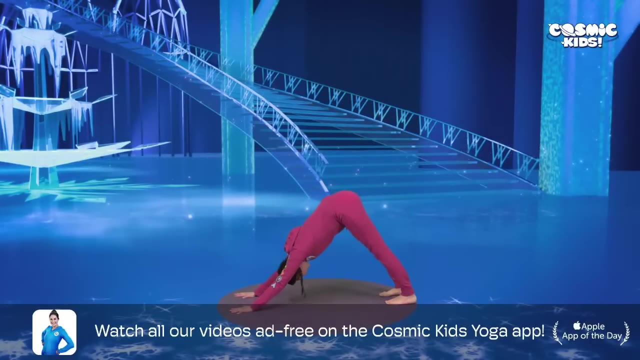 Then we step our other leg back and come down onto our bellies, where we wiggle our shoulders all the way up, pretending to be a little snow snake- Psssssss, We tuck our toes and lift our bottoms up to the sky, where we woof like a little husky dog. 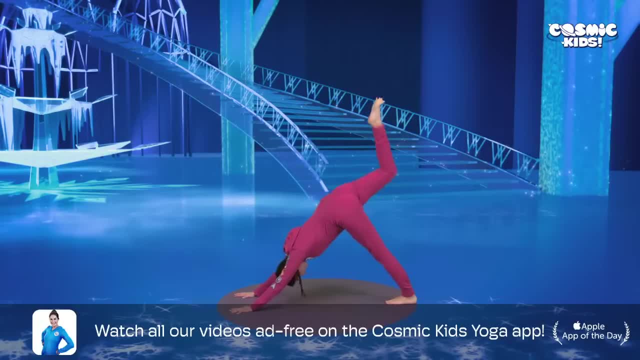 Woof, woof, woof, woof, woof. We lift up one of our legs like a happy tail and we put it between our hands, where we pretend to be an ice skater again. Whoosh, whoosh, whoosh, whoosh. 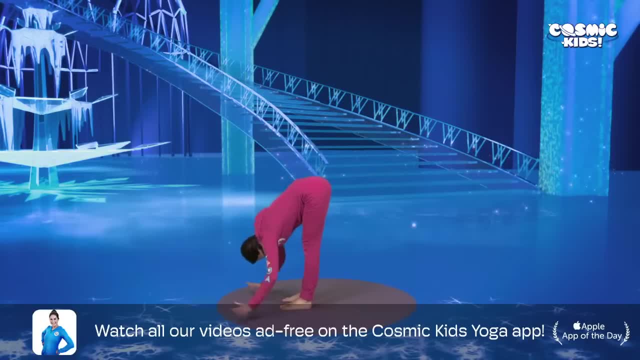 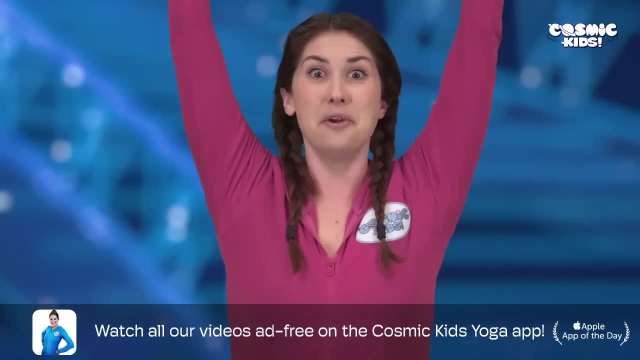 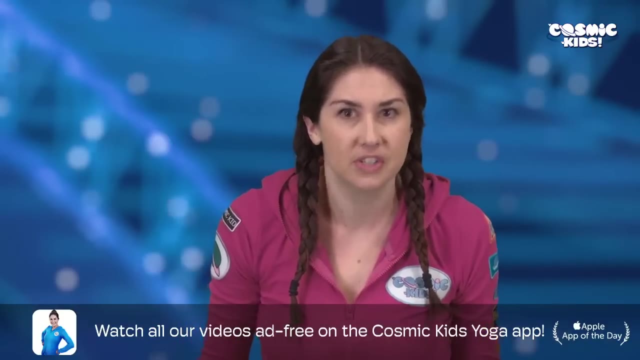 We step our other leg forwards and we say hello to the frost, Hello frost. Then we reach up to the snow and say to the snow, Hello snow. Now, Elsa was born with magical powers. Step one leg forward and one leg back. Bend your knee. 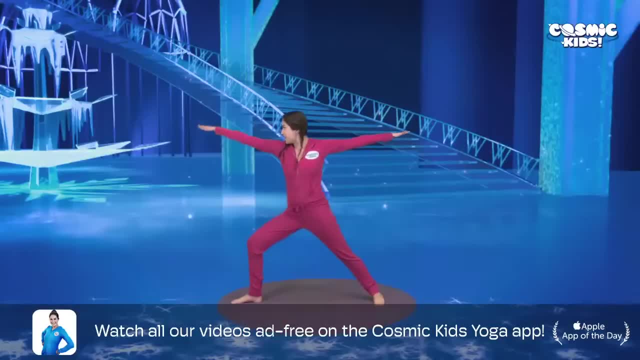 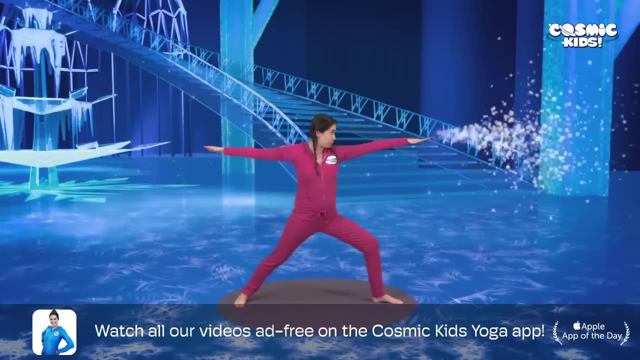 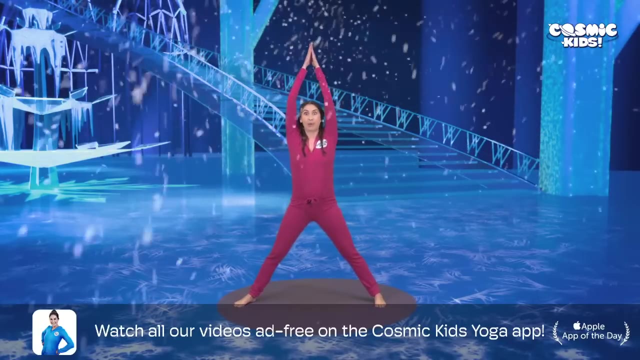 and stretch your arms, She could make ice Zooo And jump your feet the other way and frost Zooo And lift your arms above your head and snow Zooo At will. Now, Anna and Elsa were sisters, but they were also the very best of friends. 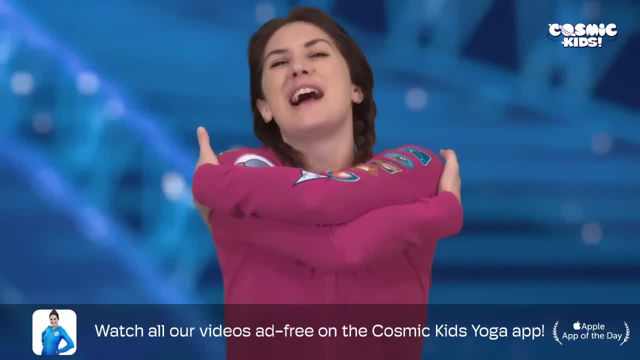 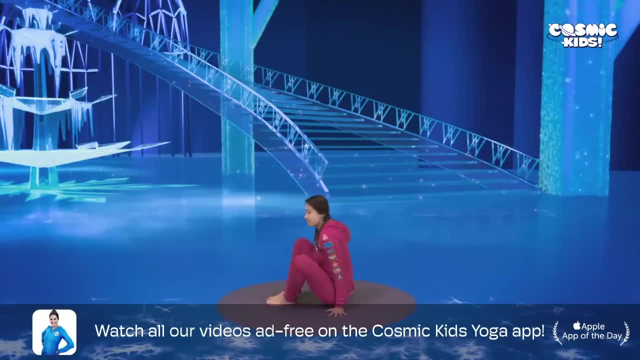 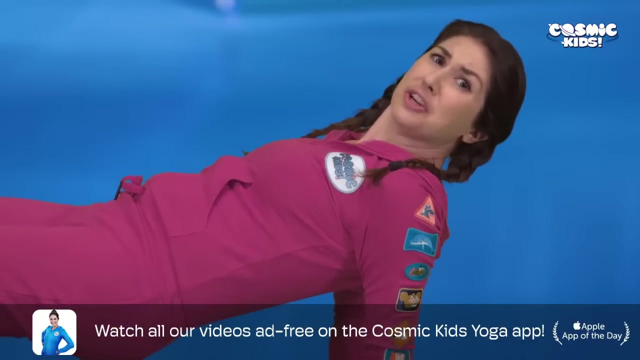 Arms wide, wrap your arms around, giving yourself a great big hug. One night the two girls were in bed Sitting on your bottoms, bend your knees, feet flat, hands behind you, Lift up your bottoms, making a bed shape. But Anna couldn't sleep. 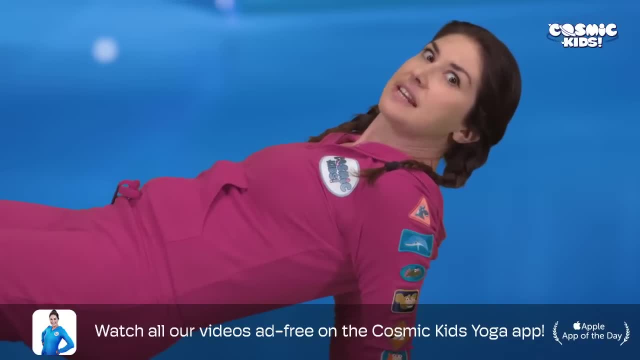 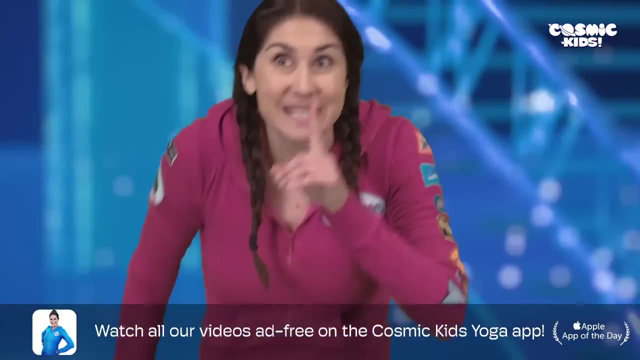 The northern lights were keeping her awake. When they woke her up, she convinces her sister to come downstairs to play The two girls tiptoe, tiptoe, tiptoe, tiptoe- quietly down the stairs where Elsa gets into position. 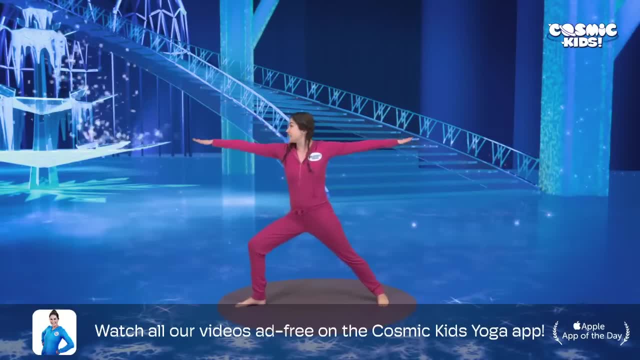 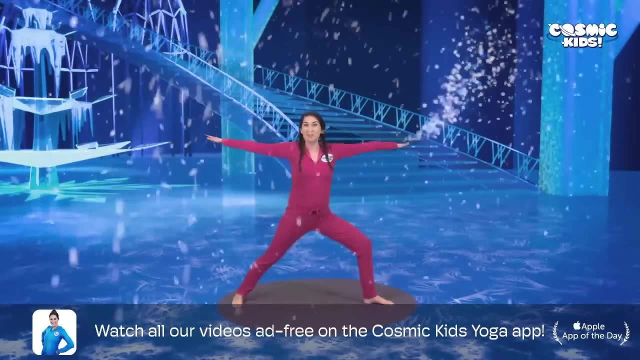 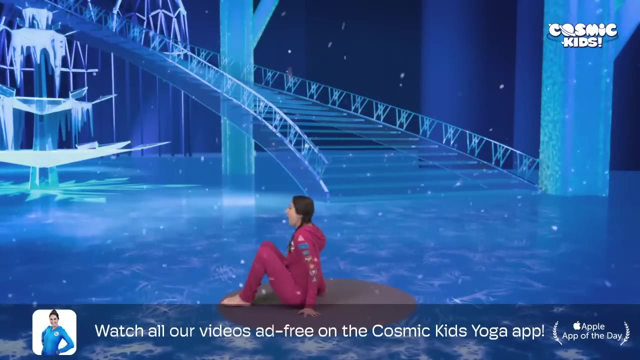 leg forward, leg back, arms stretched. She makes the whole great hall covered in ice. Jump your feet the other way, making it into a winter wonderland. The two girls decide to build a snowman. sitting on your bottoms, Hug your knees. 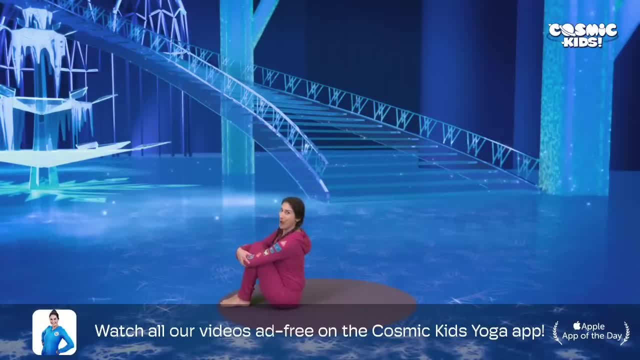 and tuck your chin in so you don't bonk your head when you roll back. They roll up a big snowball Ready All the way back, And another one for the head. Then they build him Standing up. draw your heels together. 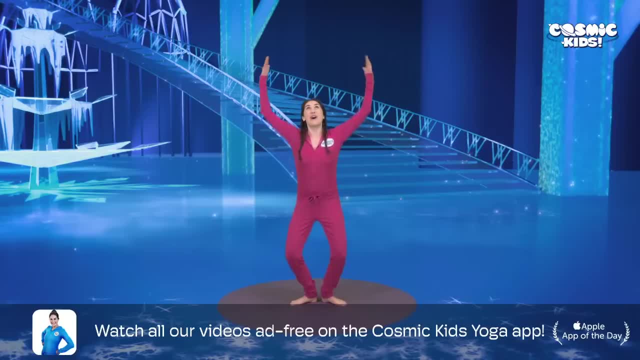 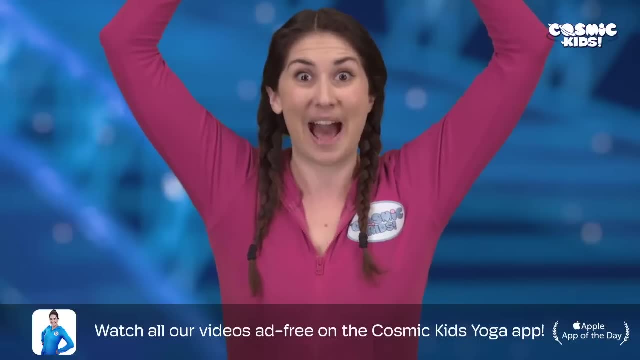 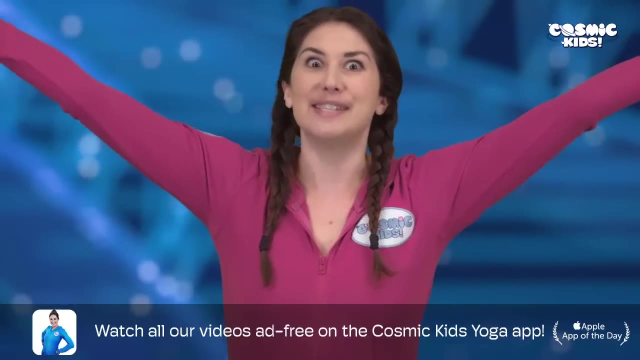 and bend your knees, Bring your arms above your head, joining your fingers over your head, making a snowman. They decide to call him Olaf And Olaf likes warm hugs. The girls have a lot of fun ice skating around the great hall. 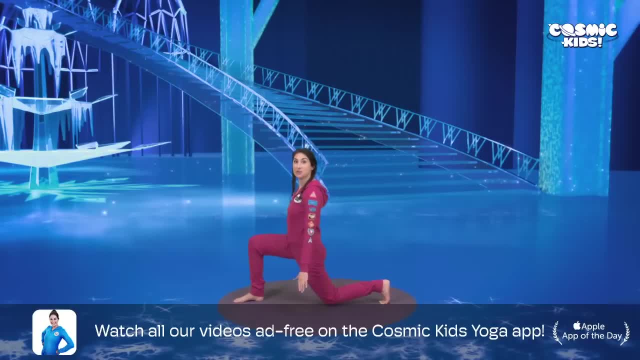 It's taking one foot forward and one foot back. Bend your knee Now. see if you can balance. Can you do the other way, Turning all the way around? drop down to your knee and try the other side. It's fun ice skating in the great hall. 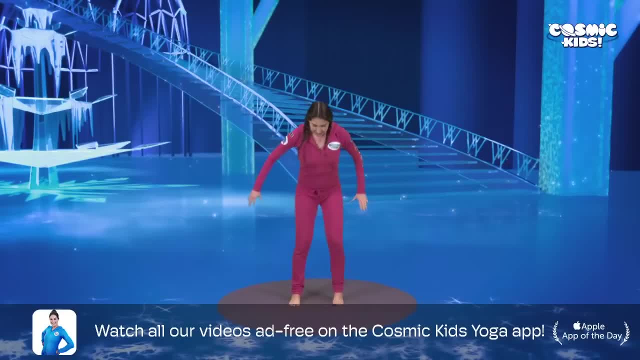 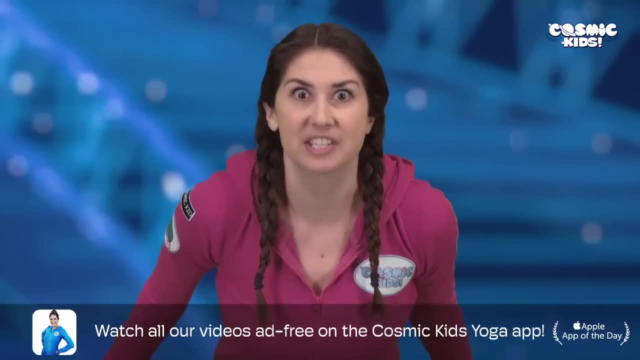 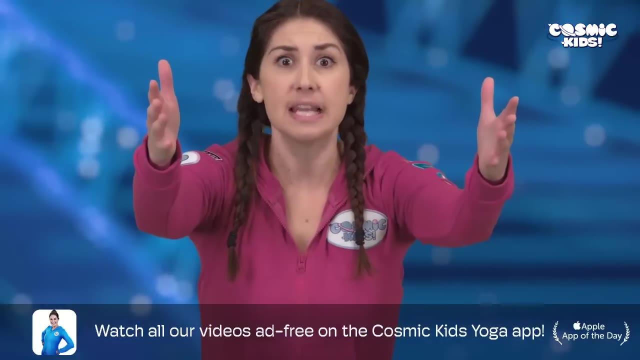 Anna loves jumping. Coming to stand in the middle, let's do a big jump: One, two, three. And Elsa uses her magic to make her jump higher: One, two, three. But oh no, Elsa slips and the magic hits Anna in the face. 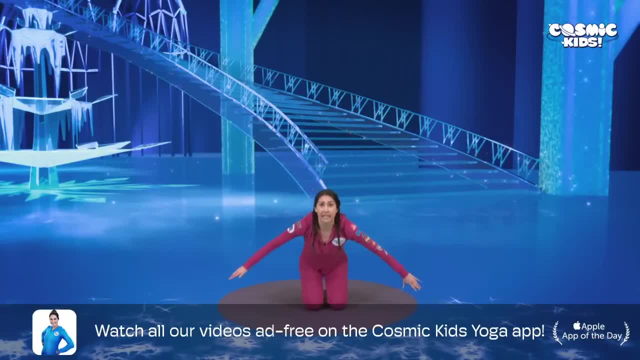 She crumples to the ground, collapsing into a snowy heap. The king and queen ride on horses to save their daughter. Put one foot forward, lifting your arms up and tuck your back toes, Swapping your legs over. now put your other foot forward. 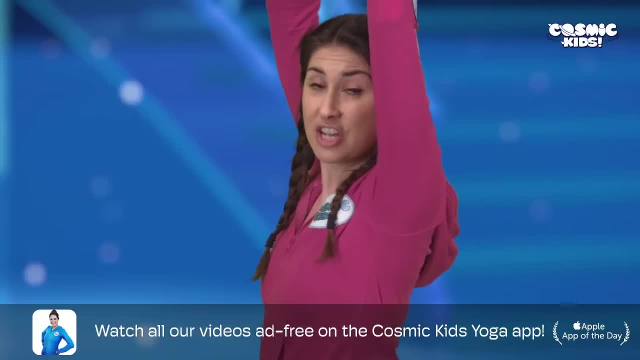 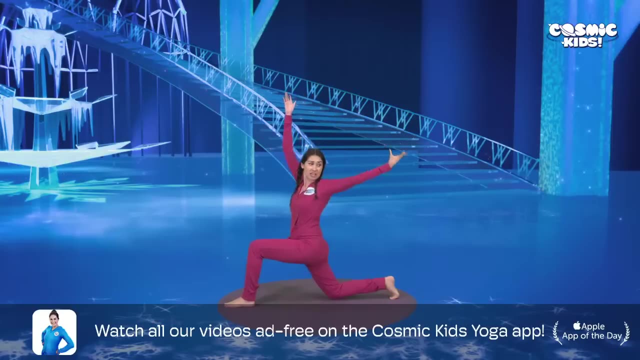 Elsa follows on behind on her horse. Tuck your back toes And because of her sadness at what she's done to her sister, she leaves behind her a trail of ice and snow. They reach the land of the trolls. Sitting on your bottoms, cross your legs. 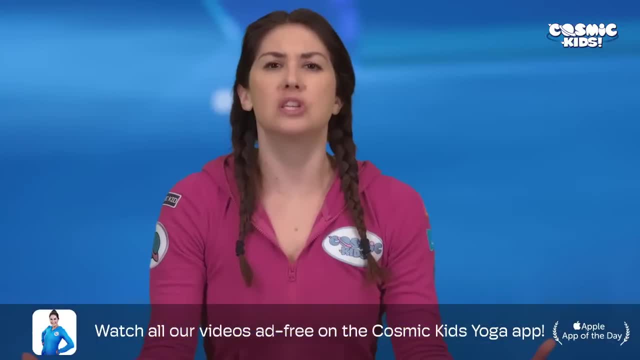 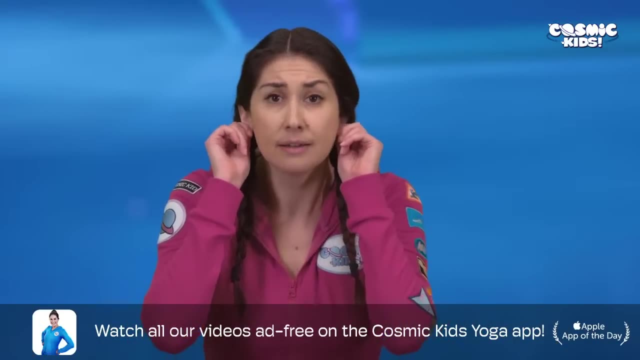 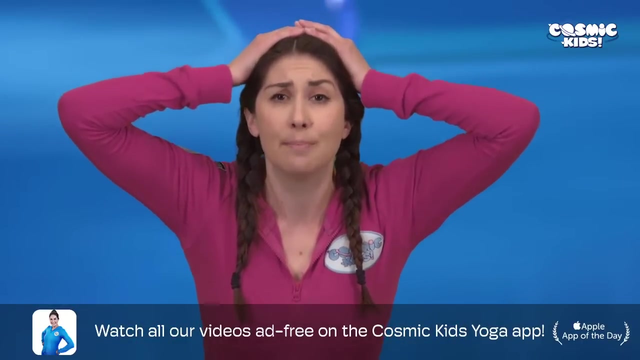 Grand Pabbie sits and uses magic to reverse the curse of Elsa's magic on Anna. He rubs her ears, He rubs her jaw And he places his hands on her head, removing from her memory all knowledge of her sister's powers, what she has done. 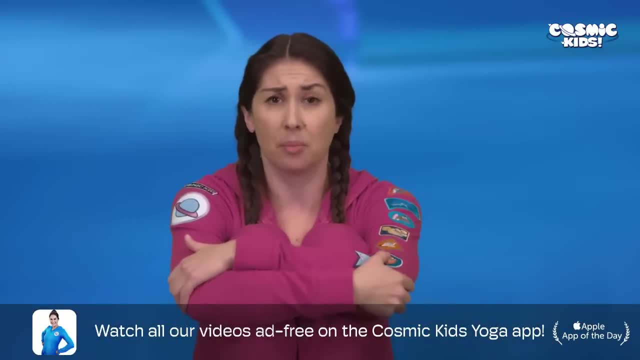 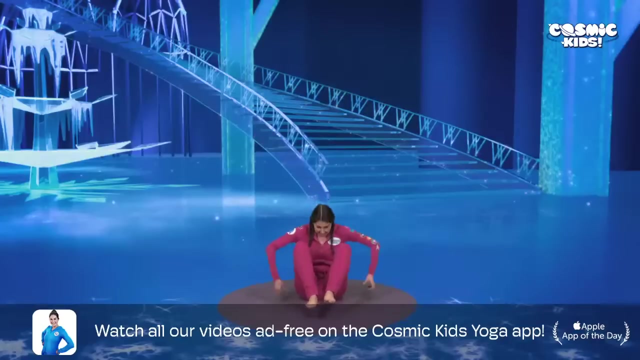 Elsa huddles herself up. She feels so bad for what she has done to her sister and promises never to let her feelings, let her powers show again. Back at the castle, she keeps herself away from her sister and her parents Standing up, take your legs wide. 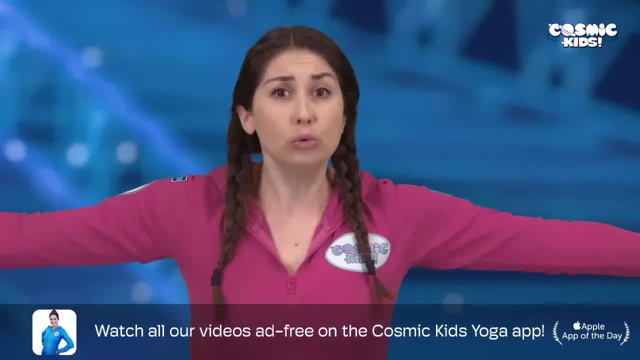 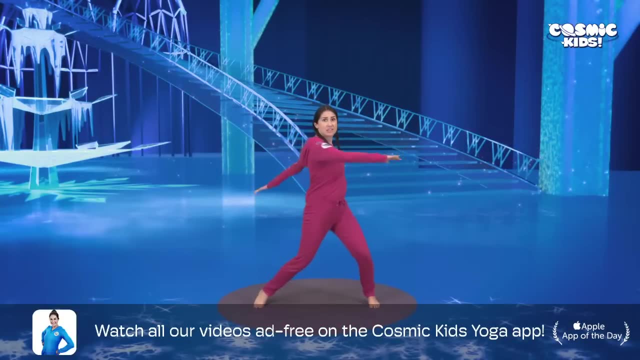 arms wide. But as she gets older, her powers get stronger. Starting to spin now, They get stronger and stronger as she grows up. She has to start wearing gloves. Take your arms wide and turn your toe to the side. Stretch out over your front leg. 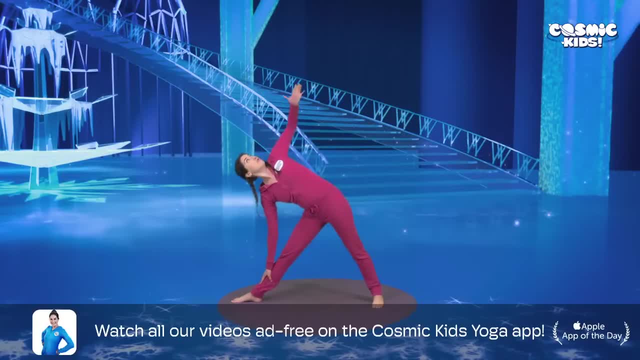 Take your hand down to your shin And reach up with your other hand, making a gloved hand, Then turning the other way. come back up to stand, Turn your toe. Turn your toe the other way, Reaching forward, touching your shin. Reach up with your other hand. 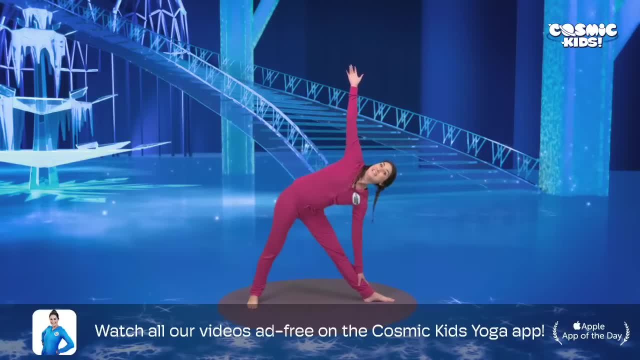 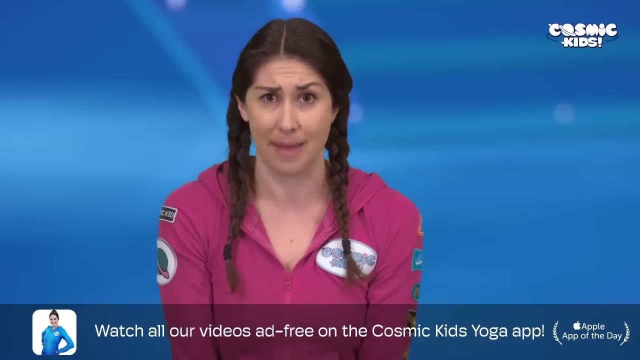 up to the sky With a gloved hand. Elsa's father teaches her a mantra: Coming down to kneel. A mantra is something you say to yourself to make your mind stronger. Elsa turns her hands over to receive the power of her mantra. 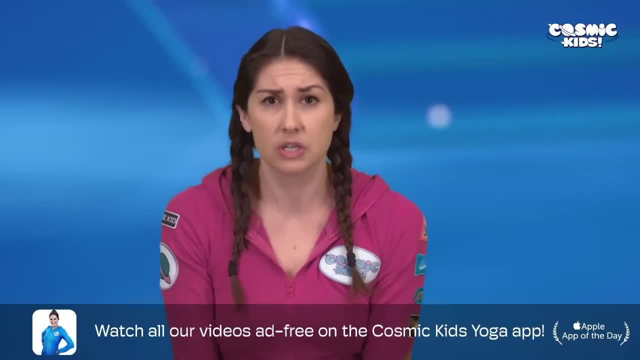 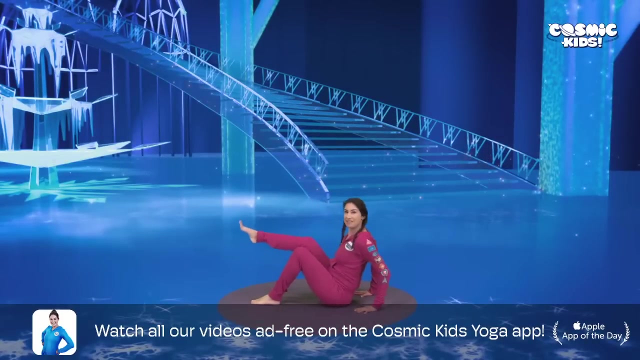 Conceal it, Don't feel it, Don't let it show, But nothing seems to stop her powers from growing stronger. Around her 18th birthday, the king and queen set sail on a boat, Sitting on your bottoms, Lift up one foot. 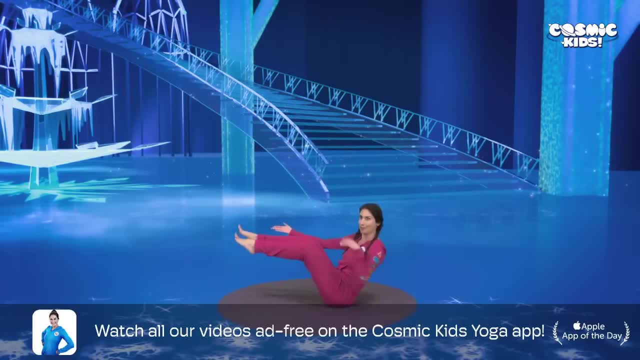 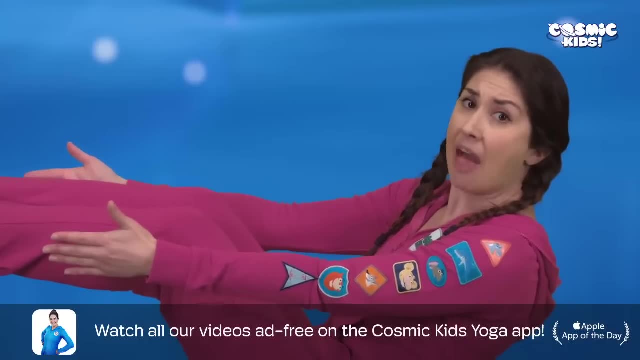 Lift up two, Lift up one hand, Lift up no hands And give me a wave: Yay, But there is a dreadful storm at sea And the boat capsizes, meaning it turns upside down. Extend your legs long, Lie back. 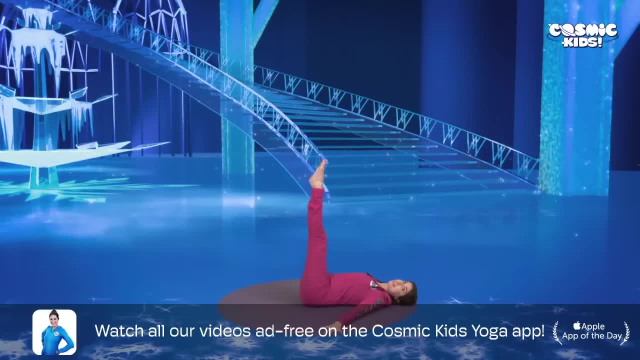 Take your arms wide And lift up your legs. Very tragically, the king and queen are killed at sea. Elsa is the next in line to the throne, Coming up to stand Using chair. pose for our throne Bending your knees and sweep your arms up high. 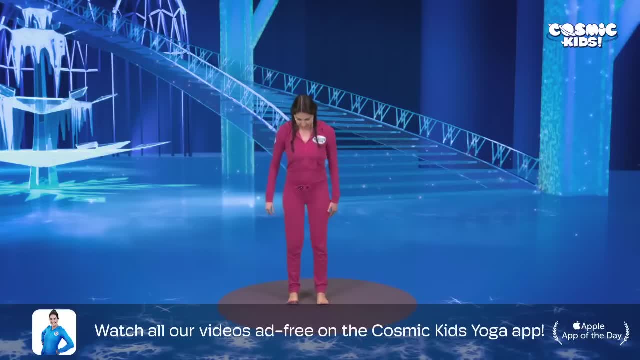 into chair pose. It's the day of the coronation And Elsa stands with her hands behind her back, Bows all the way forwards to receive the crown on her head. So they say that the crown will be lifted to the head of Elsa. 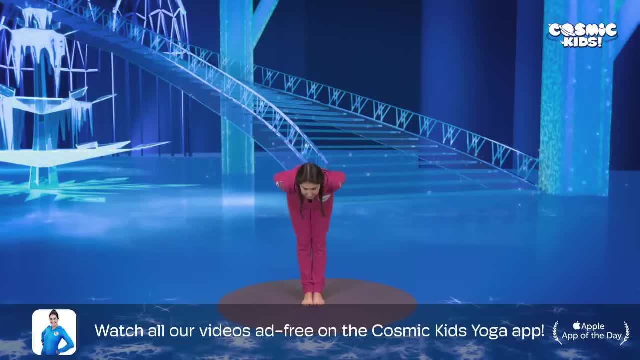 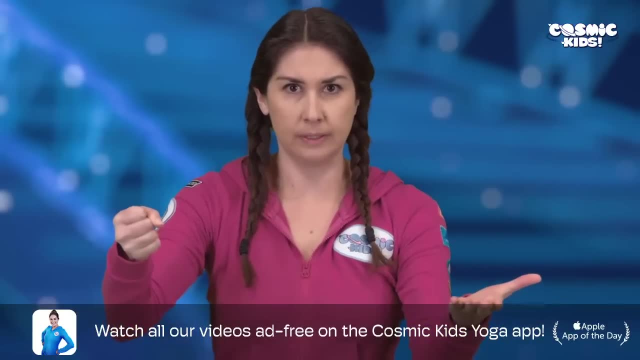 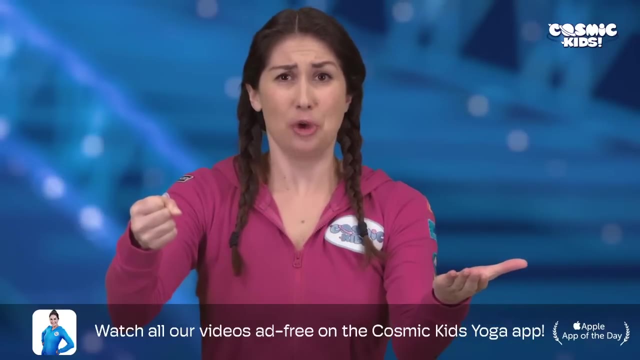 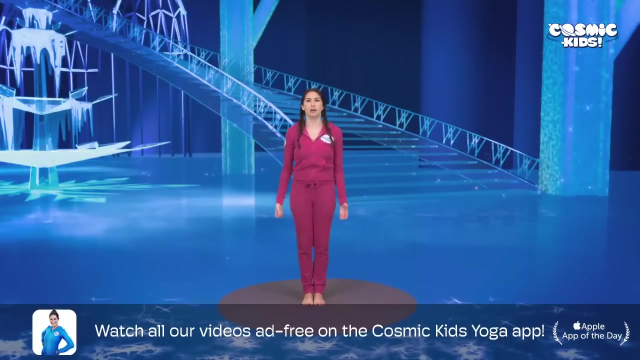 A warm and warm head. She stands up tall and, removing her gloves, holds the sceptre and the ball. She holds her breath, holding all of her powers inside. She can't let them show, not now. She holds her breath for just long enough to put them down and take a big breath out. 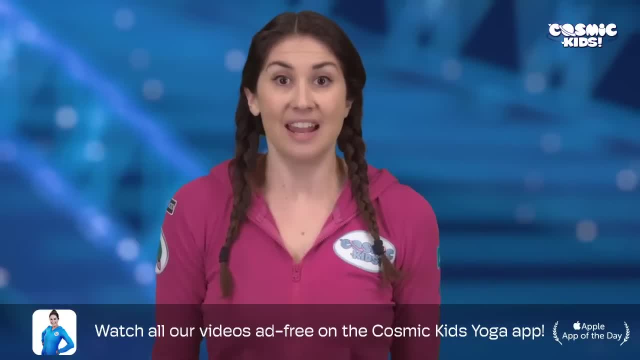 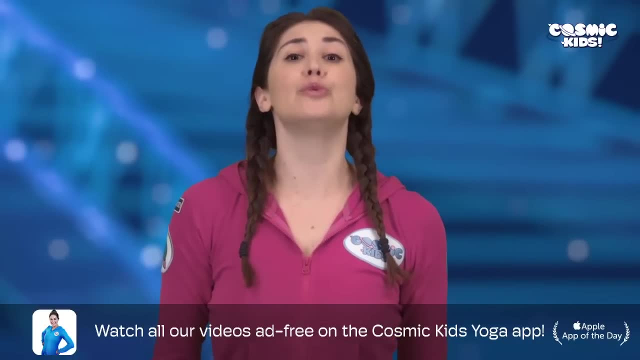 She did it. She didn't let anyone see. Later there's a party and Anna and Elsa get talking again. Along the way comes the Duke of Wesselton Turning to the side, seeing if you can hold your elbows behind your back. take one leg. 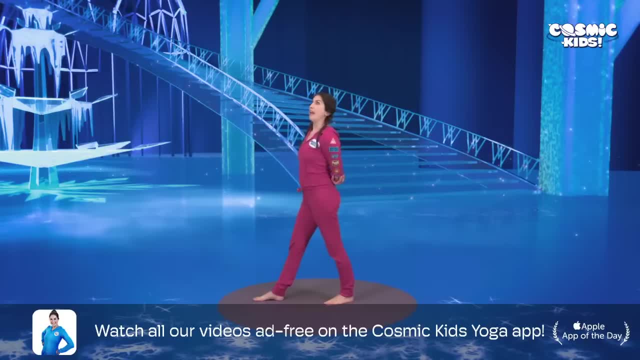 forward. He bows forward, revealing his rather funny hair. Oh hello, Queen Elsa. I wonder if I could have this dance. Well, Elsa doesn't really want to dance with him, so Anna has to instead, bringing one hand above your head for your 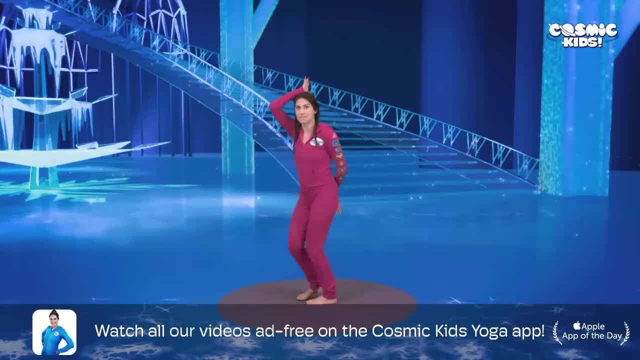 coxcomb and your other hand to your tail for your tail feather. the Duke of Wesselton moves like a chicken with the face of a monkey, coming all the way down, ready to jump like a monkey. one, two, three. Anna thinks he's rather sprightly for a man in heels standing all the way up. 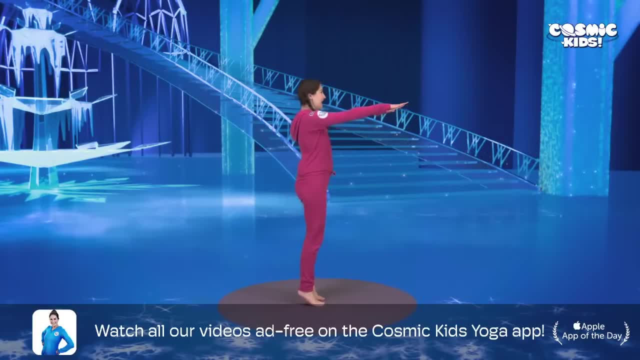 turn to the side now. lift up your arms and lift up onto your tippy, tippy tip toes, trying not to wobble. later that night Anna gets talking to Prince Hans of the Southern Isles. sitting down, take your legs around to the side in mermaid pose. take your hand onto your knee and look over your shoulder. now, Prince Hans. 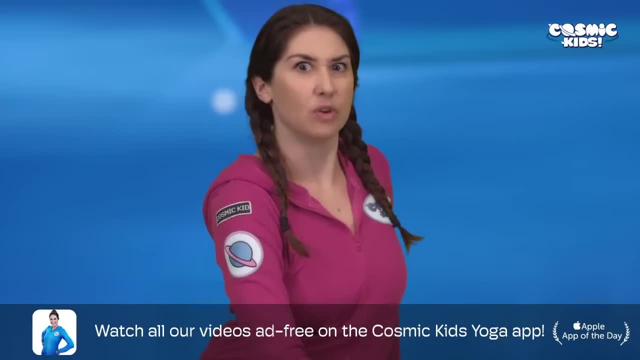 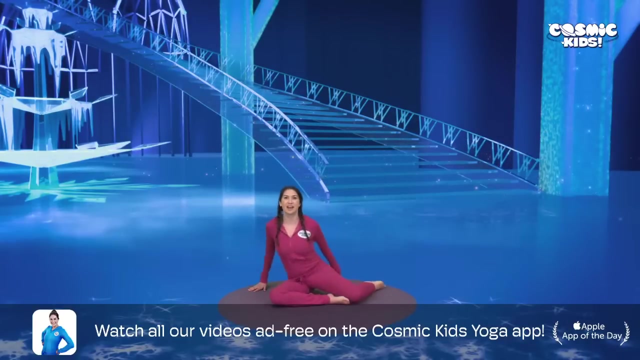 only really wants to get close to Anna because he wants to take over the throne of Arendelle. but later that night he says to Anna: can I say something crazy? will you marry me? Anna is so flattered. take your legs around to the other side, hold on to your knee, take your hand behind you, look over your shoulder, look. 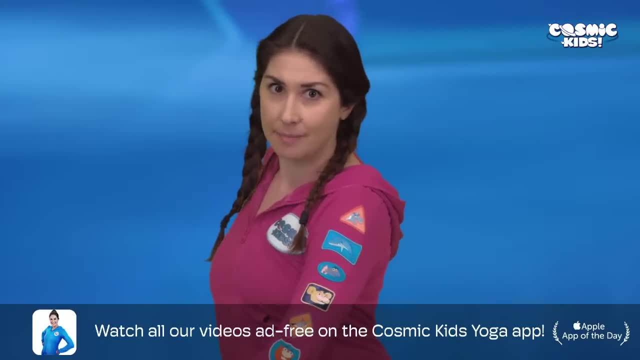 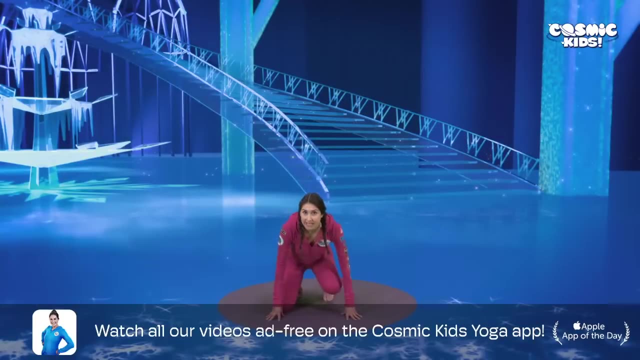 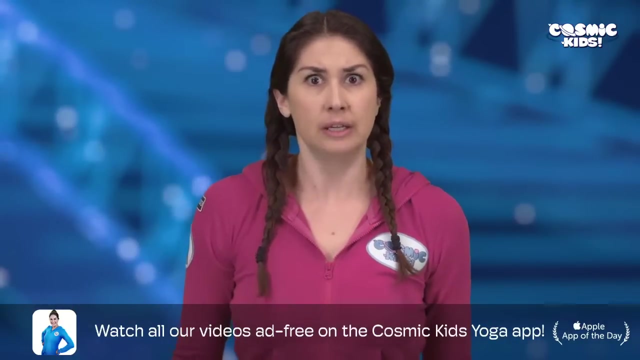 back to the front she says: can I say something crazier? yes, but Elsa, Elsa will not, cannot give her blessing. She stands, She forbids them to marry in such haste. The two girls argue And then, stepping one leg forward, one leg back, bend your knee, arms stretch. 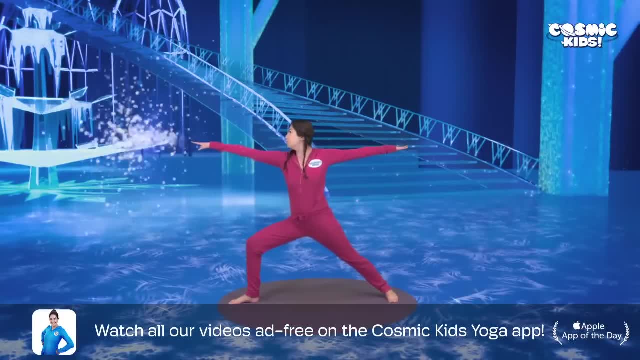 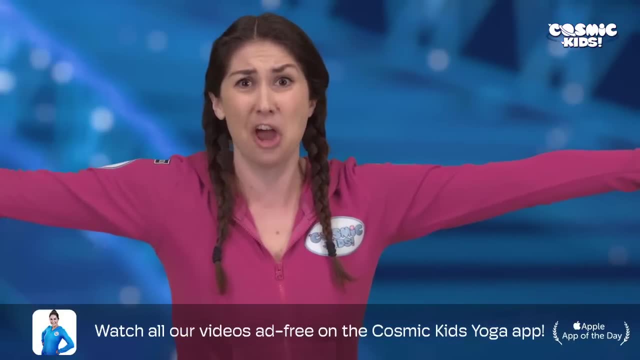 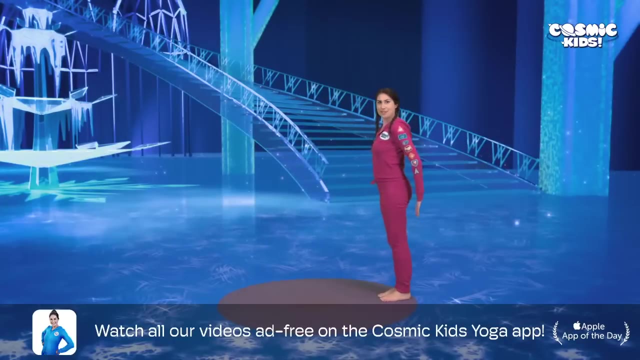 Elsa's powers are revealed. Jump your feet the other way. She covers the party in ice and frost and snow, showing everyone what she can do. Panicked, she flees up the mountain, taking big steps as she goes, Big step. 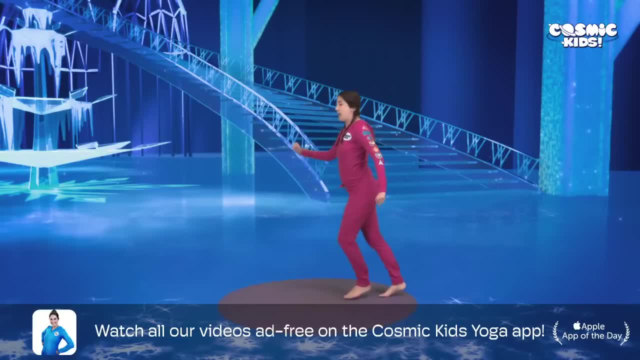 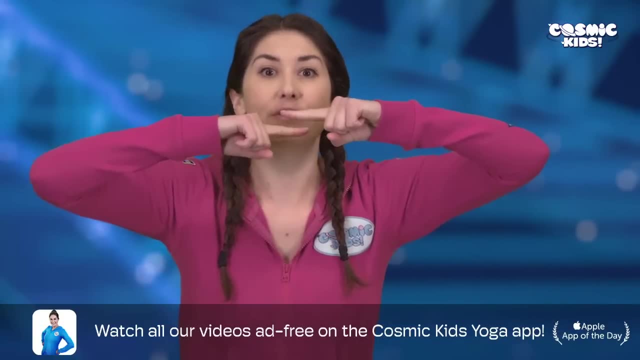 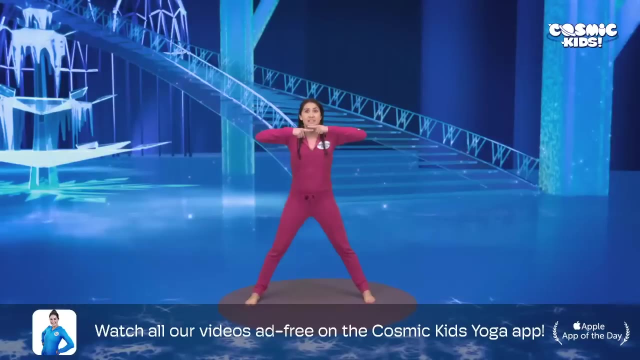 And another one Big step As she goes. the wind howls, Legs wide fingers in front of your mouth, Blow your fingers around and around. Ready An eternal winter is cast over the kingdom. At the top of the mountain, 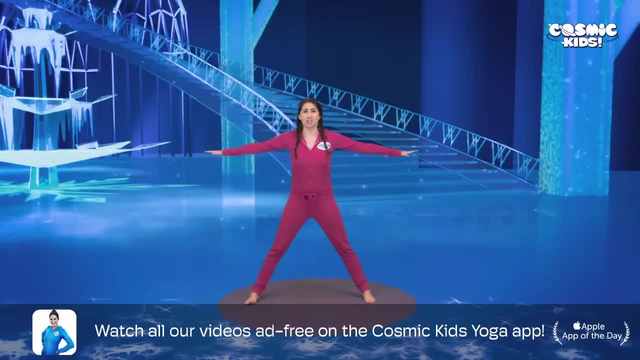 Elsa. she lets everything go. As she casts off restraint, she sings: Let it go, Let it go. Can't hold it back anymore. Let it go, Let it go, Turn away and slam the door. I don't care what they're going to say. 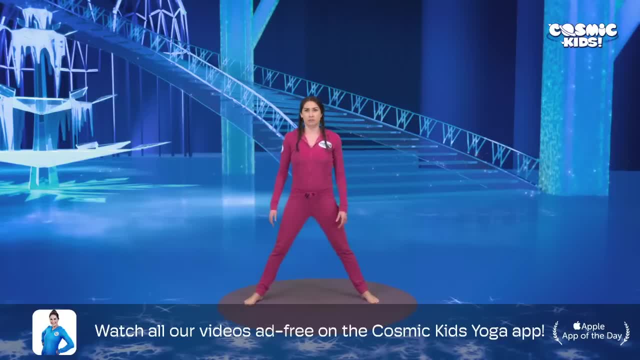 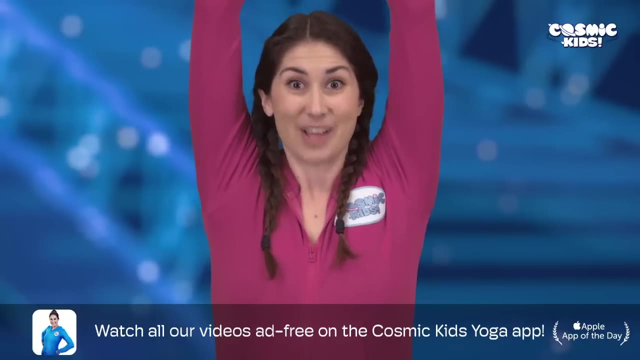 Let the storm rage on, The cold Never bothered me anyway. She builds an ice palace Arms wide. take them up and over your head, Jump your feet together, because Elsa brings back to life her and Anna's old friend, Olaf the snowman. 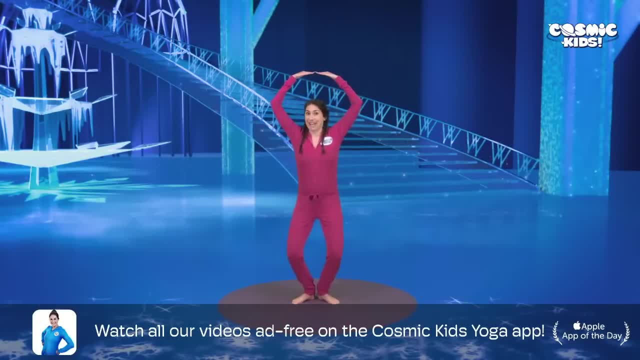 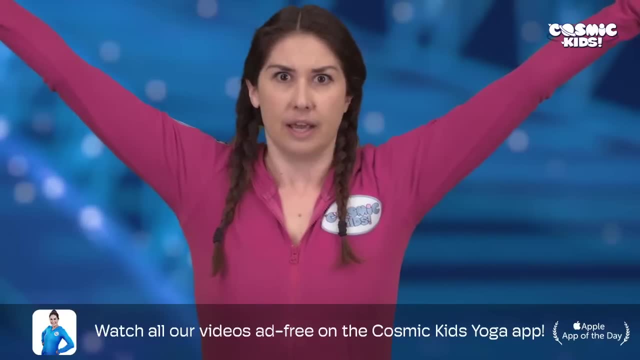 Bend your knees and join your fingers And remember. I like warm hugs. Oh, that's nice that she's got her friend up the mountain. Anna sets off in search for her sister And goes to the shops, to the store to buy supplies. 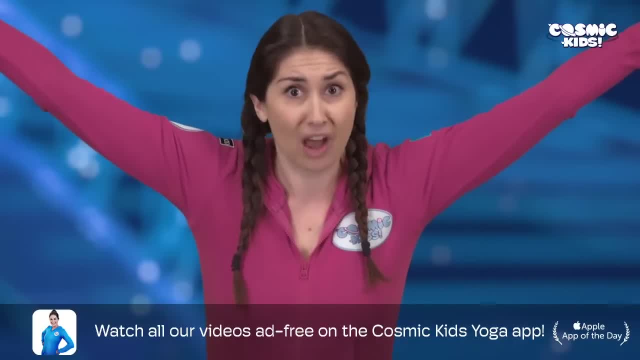 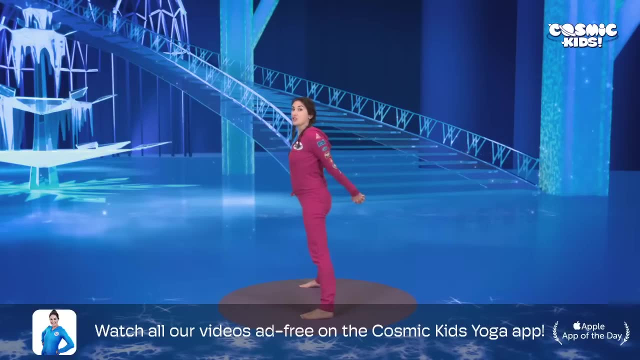 Here she meets Kristoff, the Iceman, who chops ice for a living. Turn to the side, take your legs wide, Crisscross your fingers behind your back and stretch them out. Now let's chop some ice. One, two, three chop. 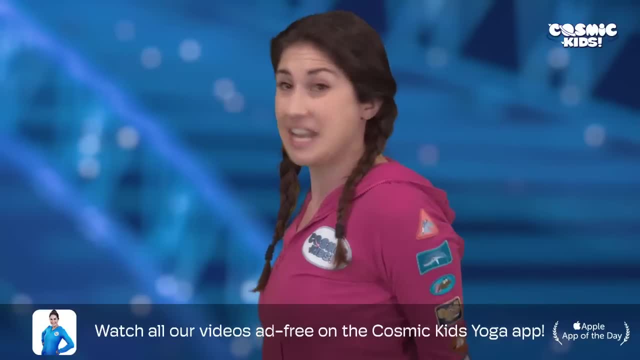 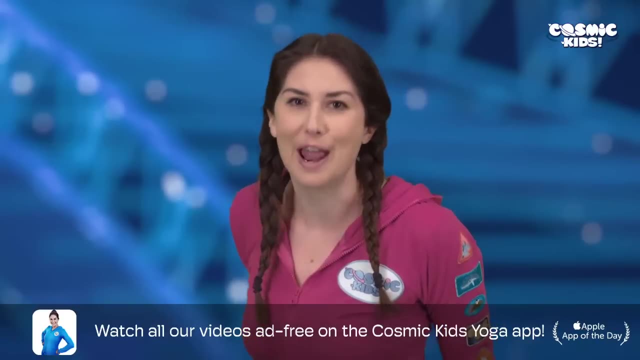 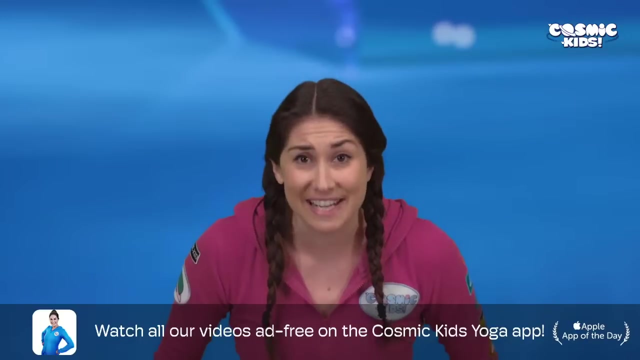 And up. One, two, three, chop And up. Now Kristoff has a rather lovely loyal friend called Sven Sitting on your bottoms, your legs out long. Sven is a reindeer. Bend your knee and take your foot over your other leg. 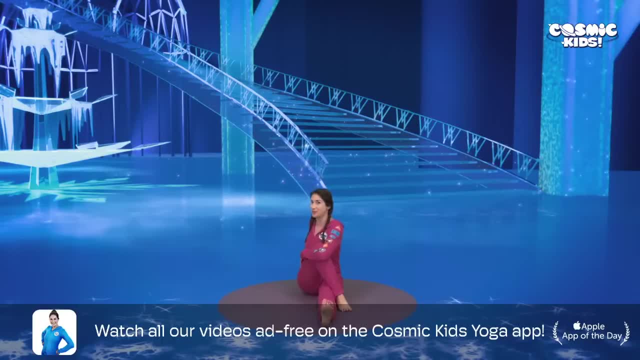 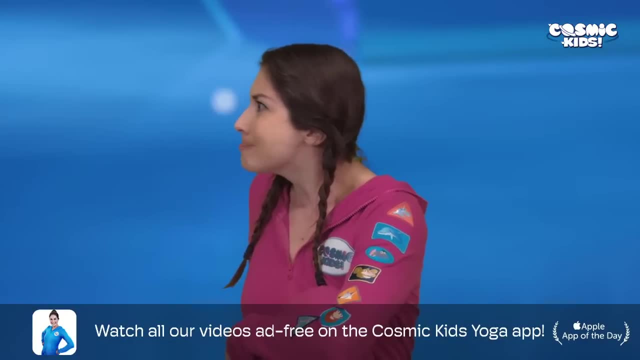 Give it a hug and stretch all the way around behind you in a twist. Now, Sven rather likes catching snowflakes with his tongue. Let's do it on the other side too. Stretch those legs long, Hug them, Put the other knee in now. 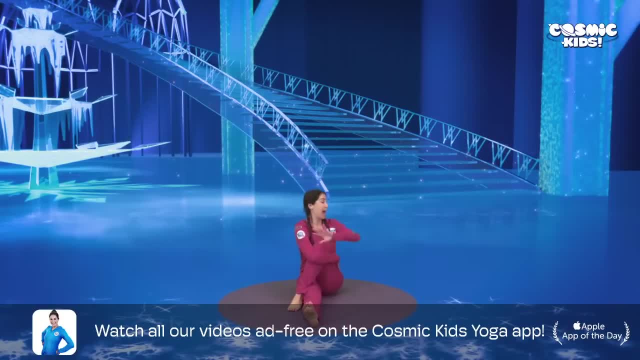 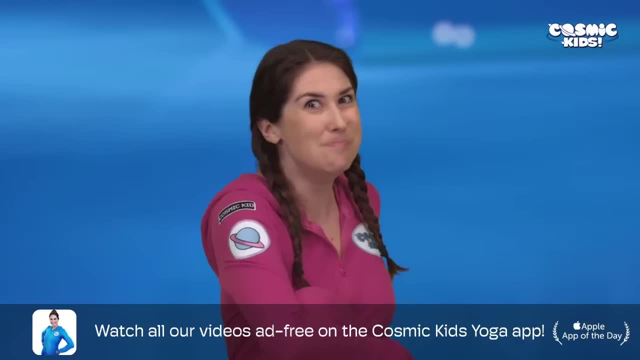 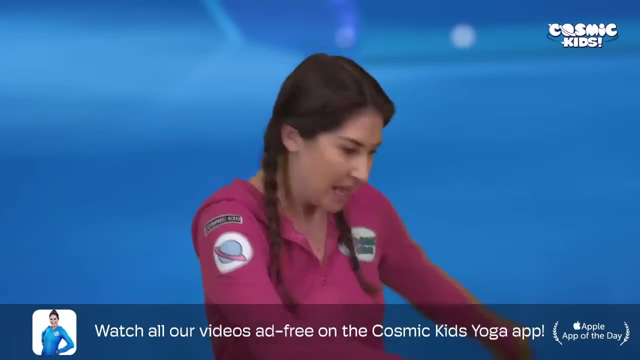 And take that foot over to the other side, Hug that knee in and twist round behind you, Catching some more snowflakes. on this side, Mmm Anna convinces Kristoff and Sven to take her up the mountain to find Elsa in their sled. 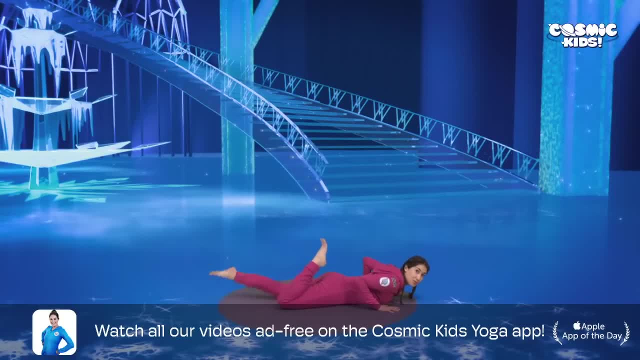 Lying on your tummies. take your feet towards your bottom and reach around and see if you can find your feet. Then you're going to smell the snow Ready Off. they go in the sled, But on the way they're attacked by wolves. 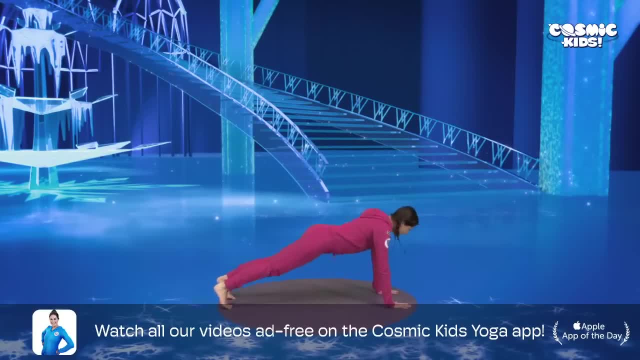 Take your hands under your shoulders, tuck your toes, lift yourself up, lift your bottom up to the sky and howl like a wolf A-woo. They manage to escape, but the sled falls down a ravine, Walking your feet towards your hands, then slowly rolling all the way up. 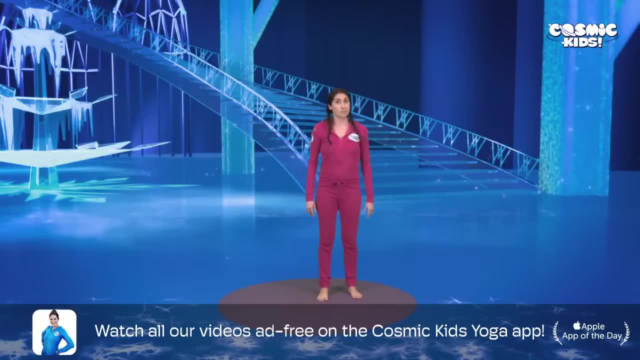 They must continue their journey on foot. They come to a magical looking forest full of trees. Bring one foot on top of the other and your hands together at your heart. Now grow your magical tree up tall. Now these trees are dangling with the most beautiful jingly, jangly icicles. 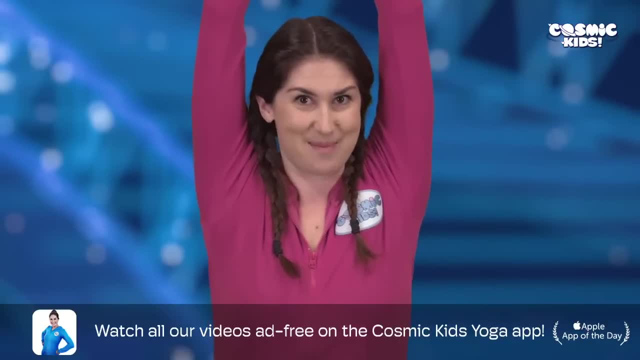 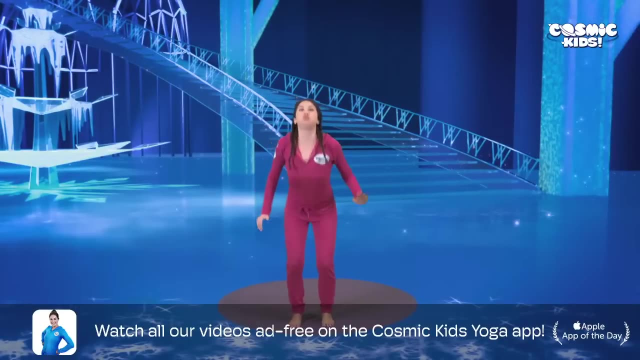 I wonder, if I blow your tree, what noise it might make. I'll have a go. You stay tall and strong, Here I come, Doop dee, doop dee, do. Wow, What a lovely sound you just made. Let's try the other side. I wonder what sound you'll make on that side. 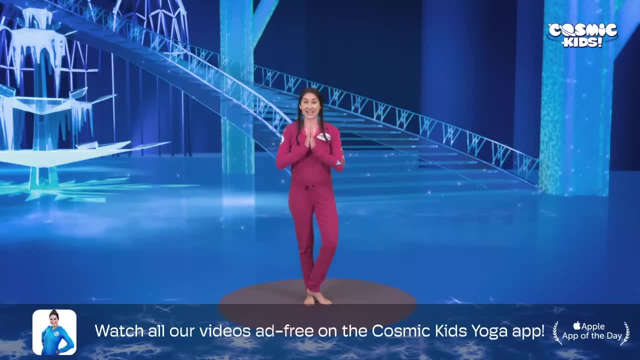 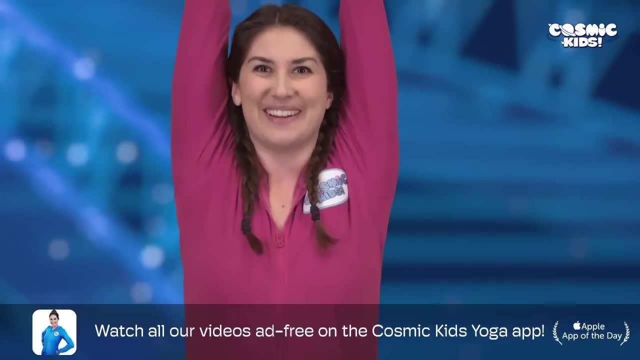 Coming back. let's bring our other foot on top now and our hands together at our hearts. Grow our trees up super duper tall. and let me try this side now. You stay tall and strong, I'll give you a blow. Ready Doop, dee, doop, dee do. 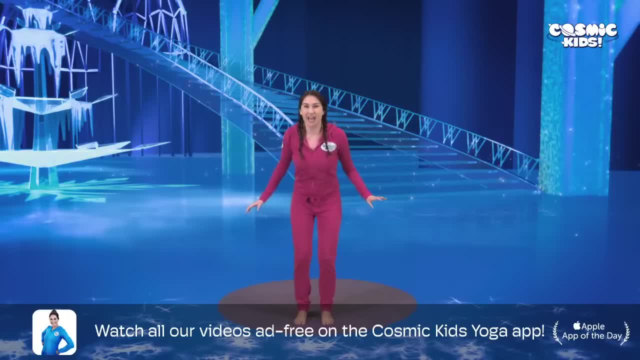 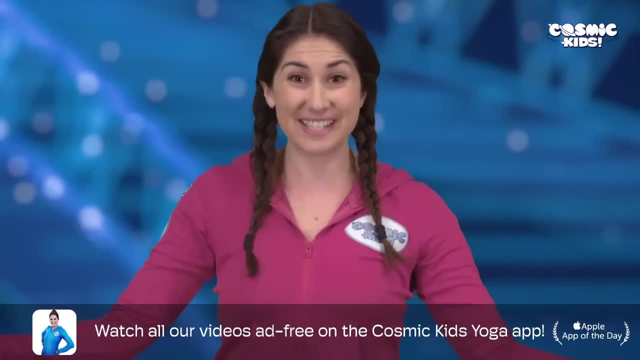 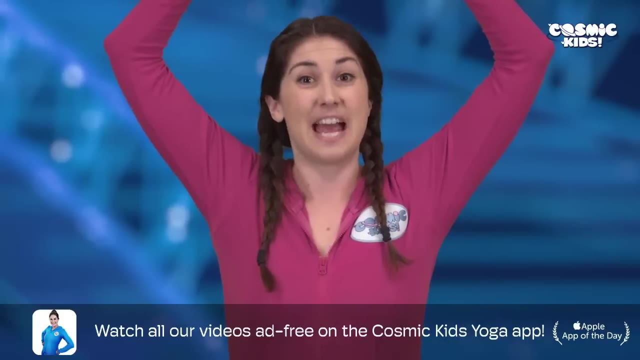 Wow, What an amazing sound that was. Now, in this magical forest, Anna, Kristoff and Sven come across Olaf the snowman, Join those heels together, bend those knees and join your hands. He introduces himself, telling them I like warm hugs. 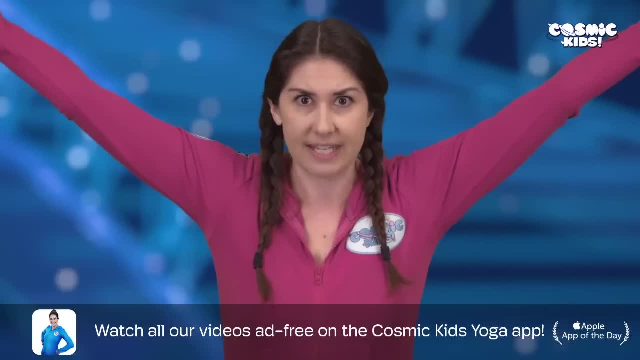 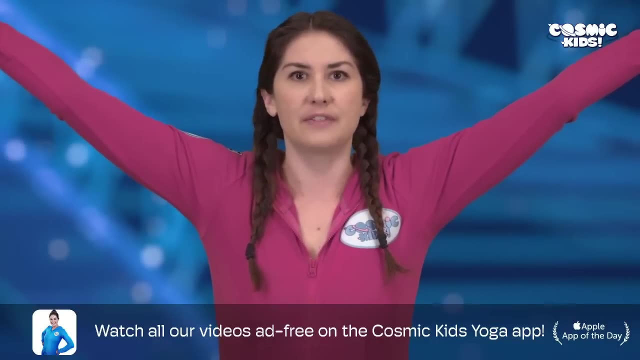 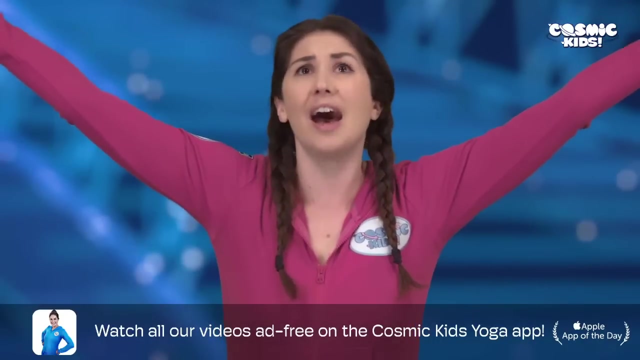 They ask if Olaf can take them up the mountain to where Elsa is hiding in her palace, Because they need her to bring back summer. At the mention of summer, Olaf says: I just don't know why. I just love the idea of summer, of sun, of all things hot. 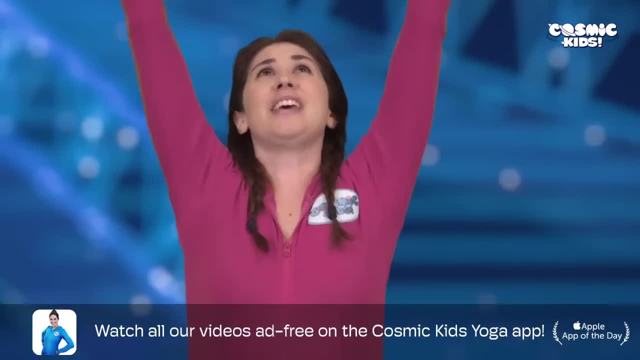 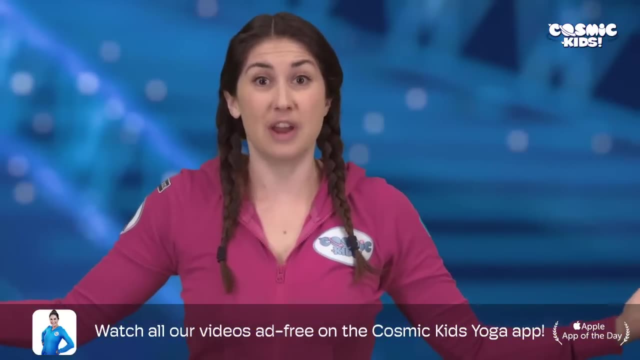 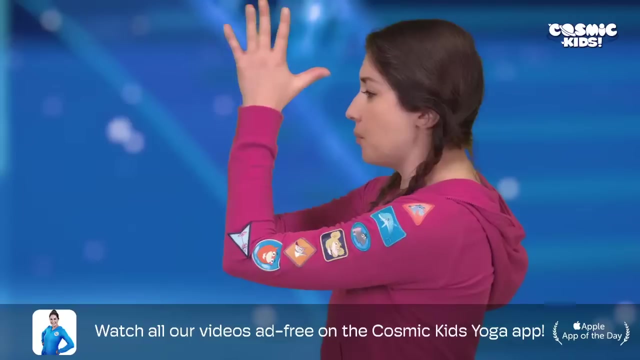 He raises his arms into the sky, as he says. in summer, He takes them up the mountain to find Elsa, where the girls reunite. Wrap your arms around yourself, Coming down onto one knee, Join your hands together and bring them in between your eyes. 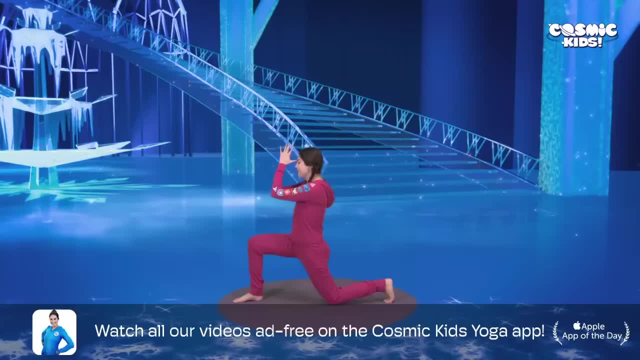 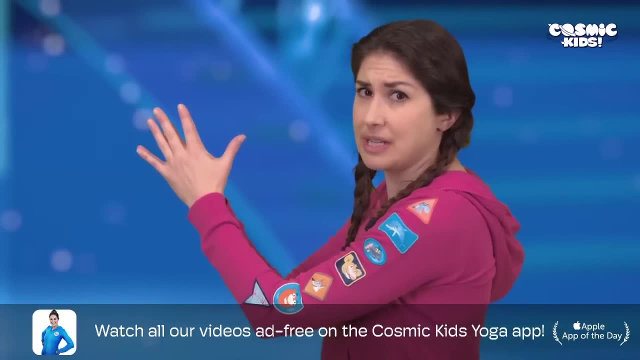 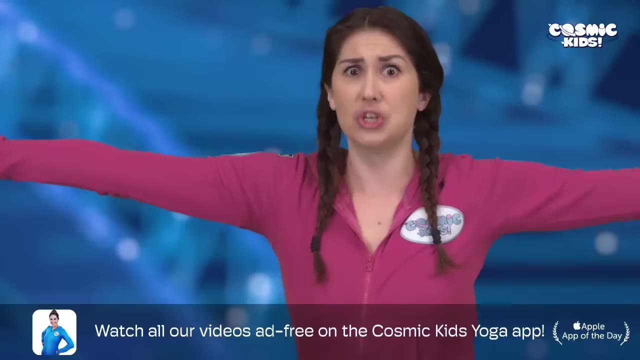 Anna begs Elsa to come back to Arendelle and to remove the curse of the winter. Elsa is terrified. she is going to show her powers And in her terror, sure enough, stretching your leg long, your arms wide, her powers do come out. 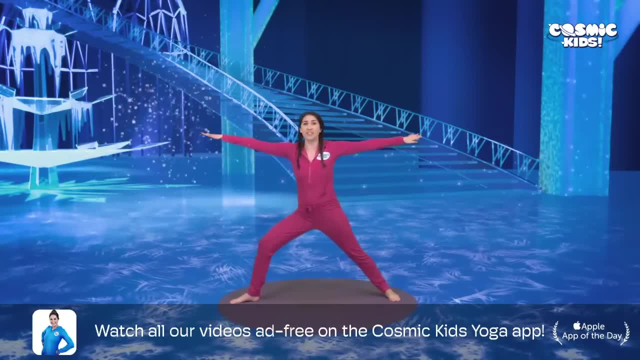 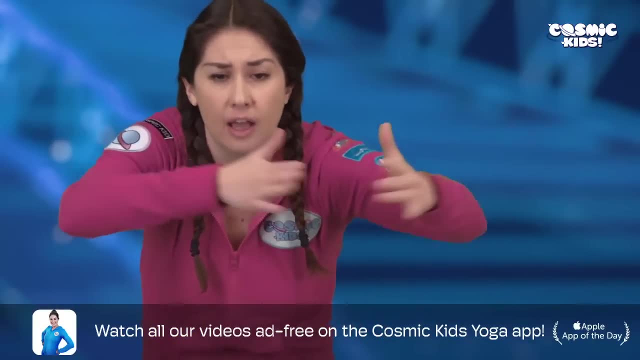 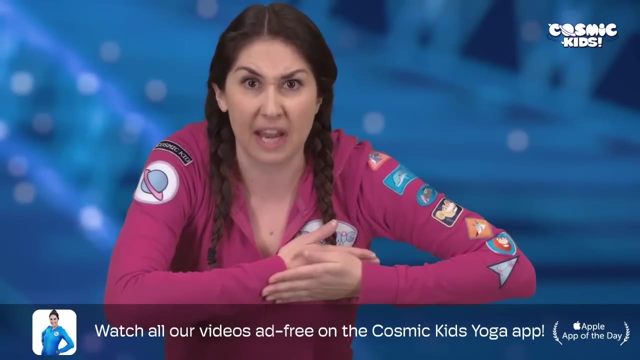 Shoo, Shoo, Shoo. Other side Jump your feet, Shoo, Shoo, Shoo. This time they hit Anna in the heart. Elsa can't believe what she's done, And so she creates a giant snow creature called Marshmallow to make them go away. 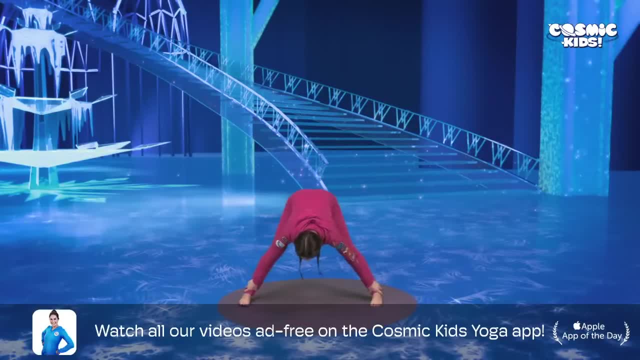 Folding all the way forwards, taking hold of your ankles. Marshmallow says: Go away. Kristoff, Sven, Anna and Olaf run. But Kristoff notices something. Jump your feet wide, Pitter-patter on your head. Anna's hair is changing colour. 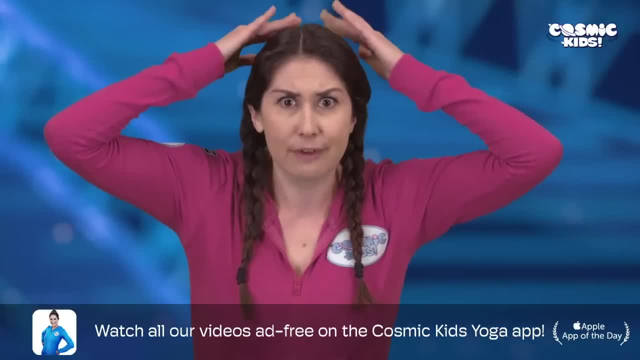 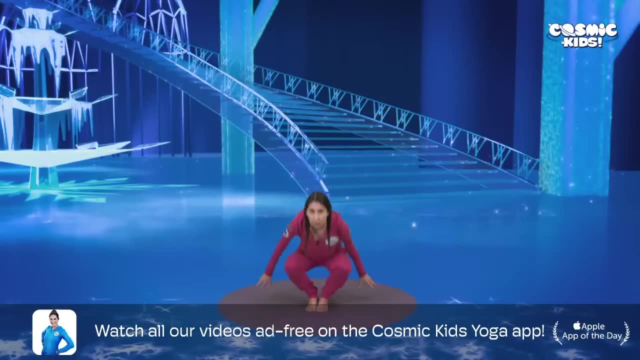 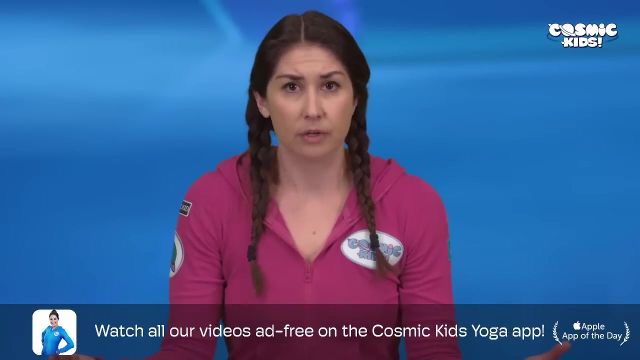 It's turning white. Something is very, very wrong. He takes them. He takes Anna to see the trolls Sitting on your bottoms, cross your legs, Where Grand Pabbie explains: Anna's heart has been frozen And only an act of true love can thaw a frozen heart. 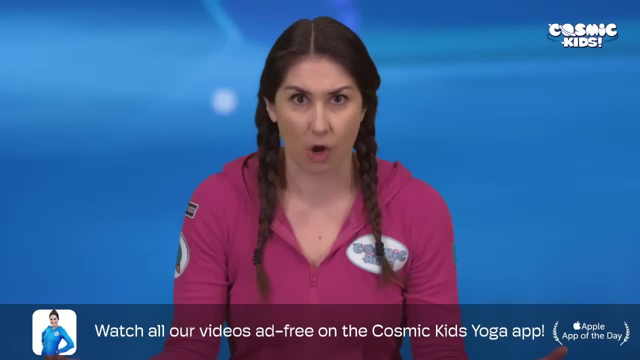 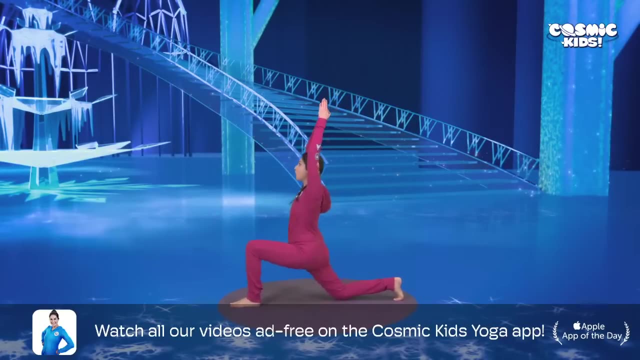 Kristoff wastes no time. He rides on Sven like a horse, Coming up one foot forward, one foot back, back toes, tucked arms up high, Swapping your legs over. now Turning your other foot forward, Tuck those back toes. 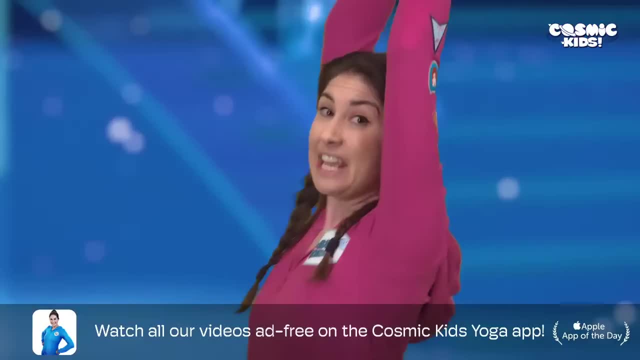 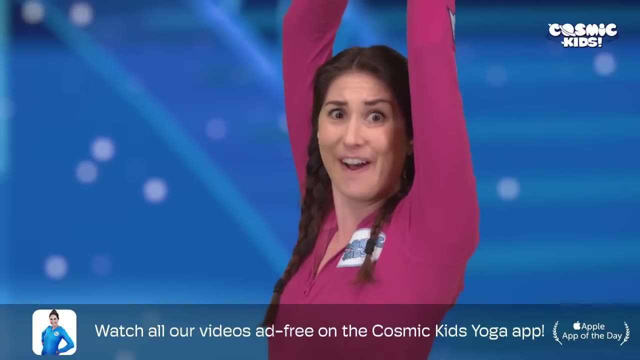 Reach up. with those hands. He rides like the wind back to Arendelle, Where Prince Hans of the Southern Isles, Anna's one true love, will be able to save her. Meanwhile, at the Ice Palace, where Elsa is legs wide arms above your head, 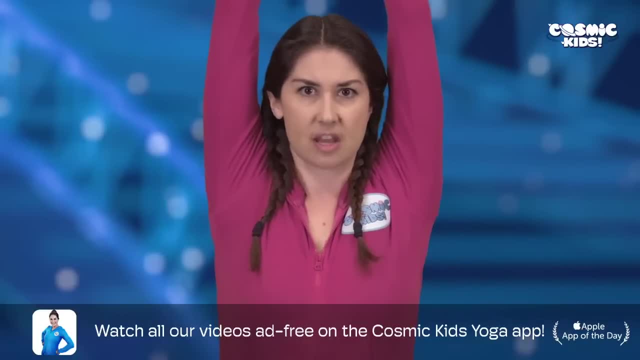 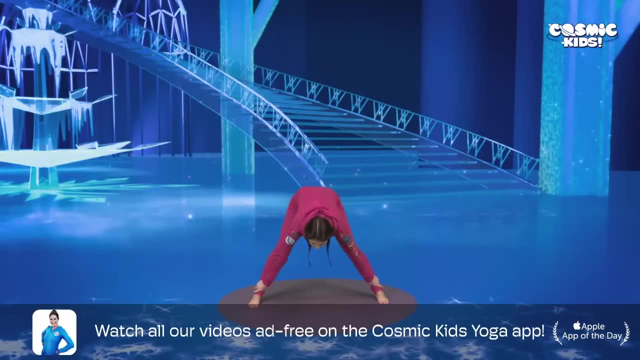 Prince Hans and the Duke's men are on their search for Anna And they've found Elsa. Elsa sets Marshmallow on them, Leaning all the way forward. he tries to fend them off, Go away, But the Duke's men have arrows and bows. 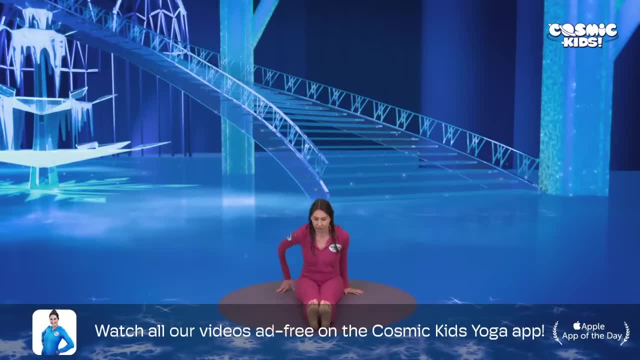 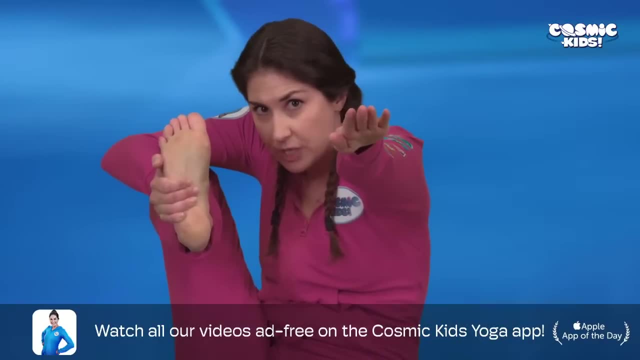 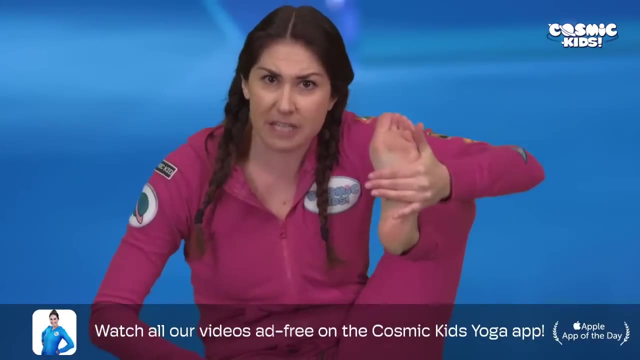 Sitting on your bottoms, legs long, They fire with their crossbows, Pulling your foot all the way back, Aiming at Elsa to try and shoot her down. One, two, three. They try on the other side as well, Lifting up your crossbow. 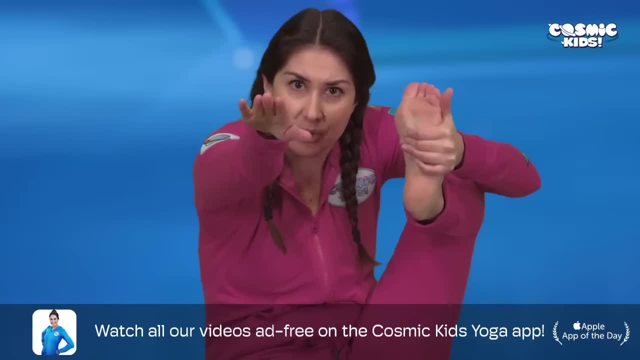 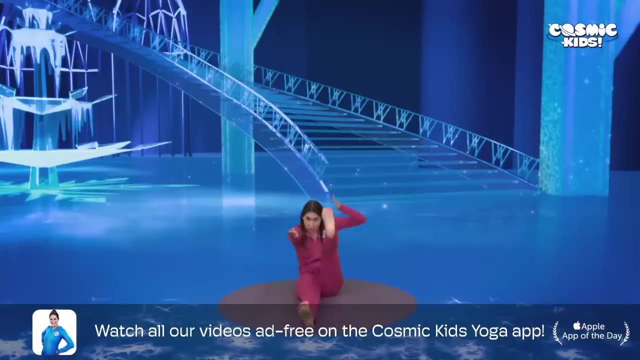 This time, though the crossbow, the arrow hits the ice chandelier right above where Elsa is standing. One, two, three. Now lying on your backs, Take your arms wide and your legs up high, Making the ice chandelier in candle pose. 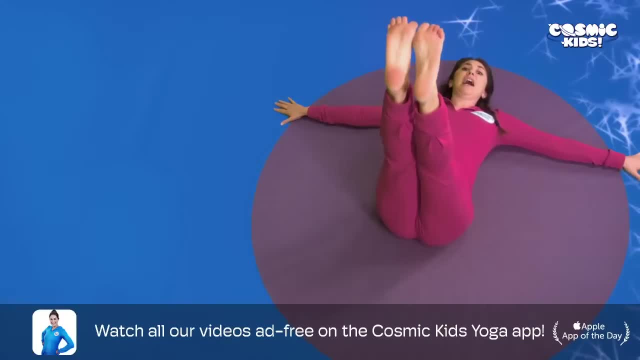 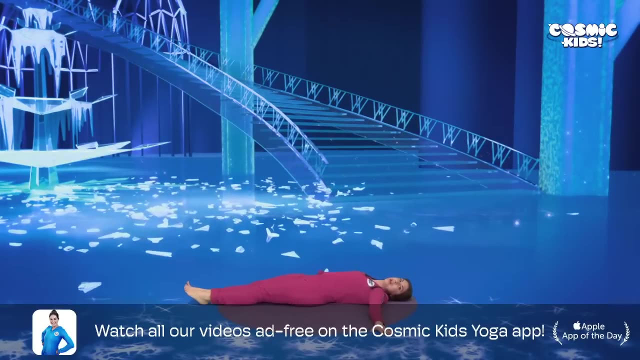 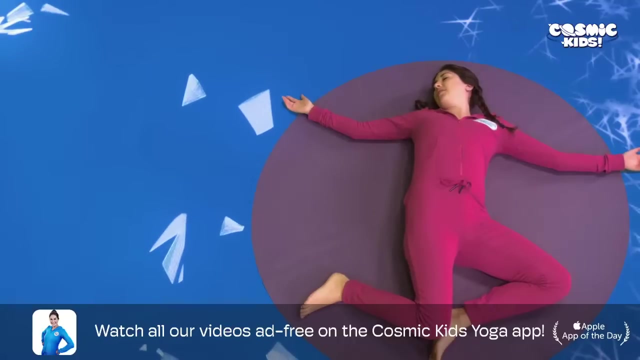 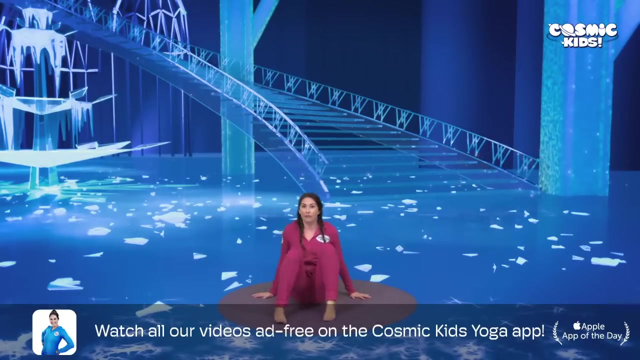 As the arrow hits the ice chandelier, it comes crashing down, Knocking Elsa unconscious. Bend your knees, turn them to the side, Turn your hands over and, taking your head in the opposite way, Prince Hans takes Elsa captive, Imprisoning her in the dungeons of the castle in Arendelle. 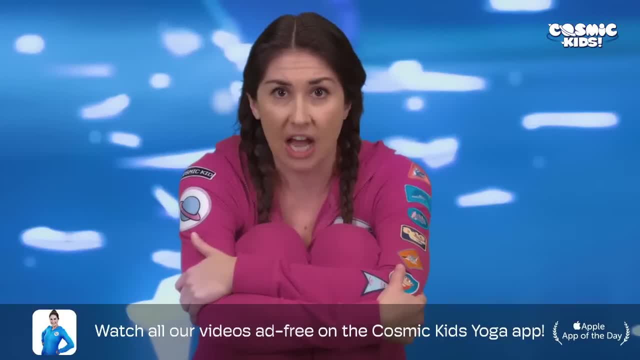 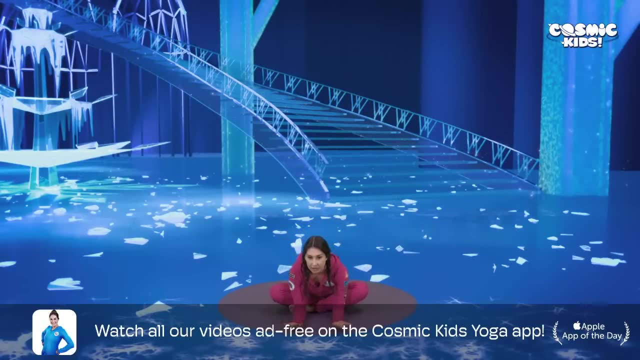 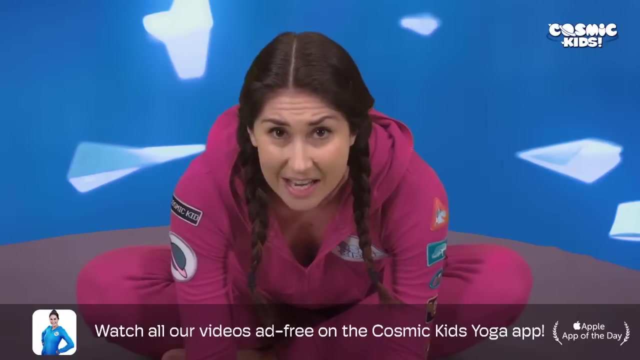 She huddles up. He then traps her hands- her hands with all that power- into metal shackles, Crossing your legs. put your hands into those metal shackles Leaning down towards your forearms. He asks: Elsa, please, please, make the winter go away. 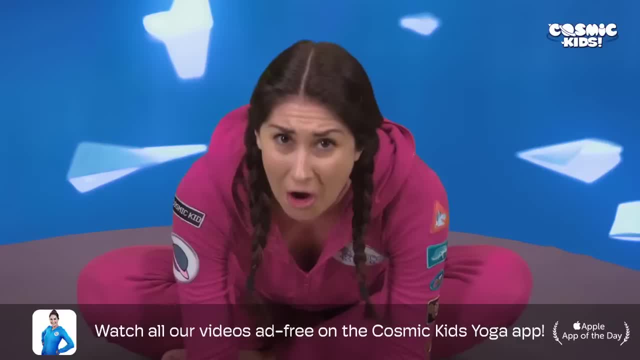 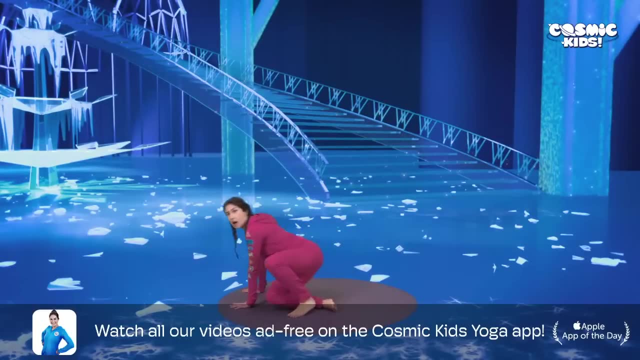 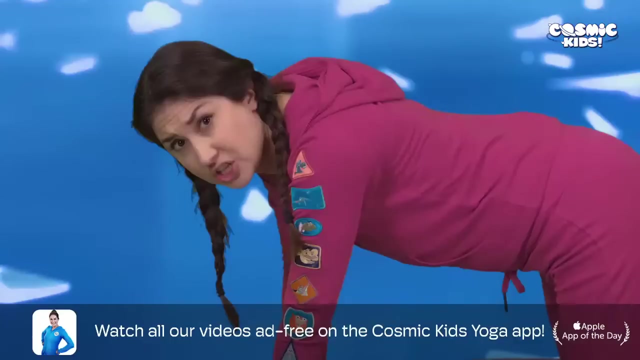 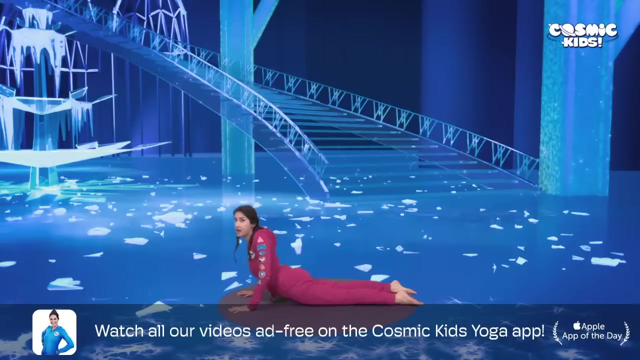 But she confesses that she won't. She confesses that she just doesn't know how Meanwhile Princess Anna, with her fast freezing heart, crawls back into the kingdom. She needs to find Prince Hans quickly before she freezes entirely. She crawls on her belly, wiggling herself into the room where Prince Hans is waiting for her. 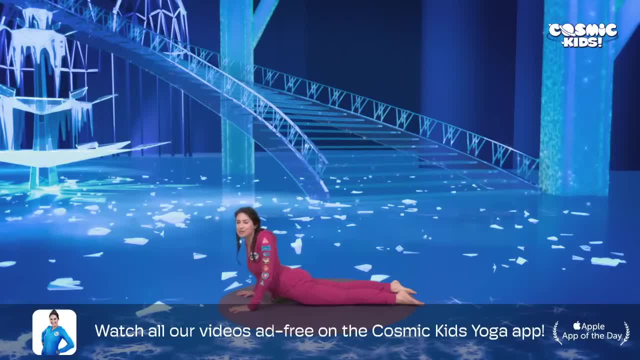 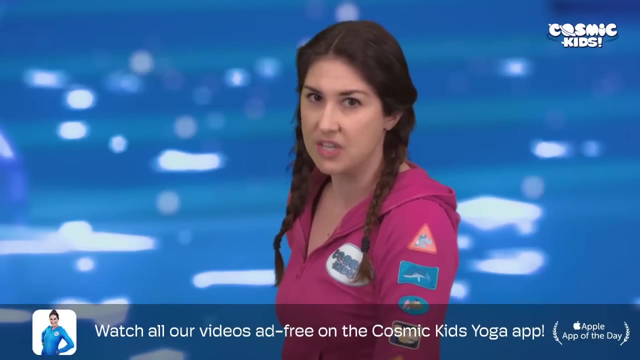 She begs him to kiss her. That true love's kiss will save her. now He sits back on his heels, kneeling up, looking at Anna, And he tells her: no, I can't kiss you because I don't love you. It won't save you. 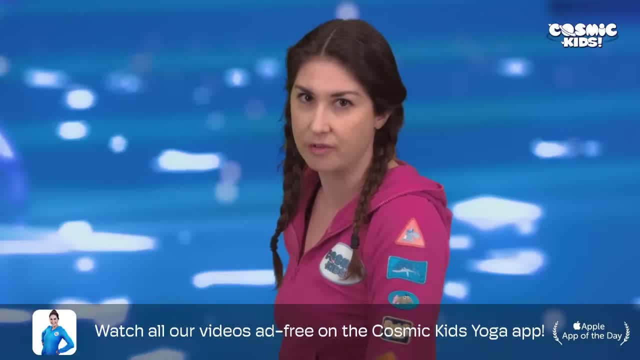 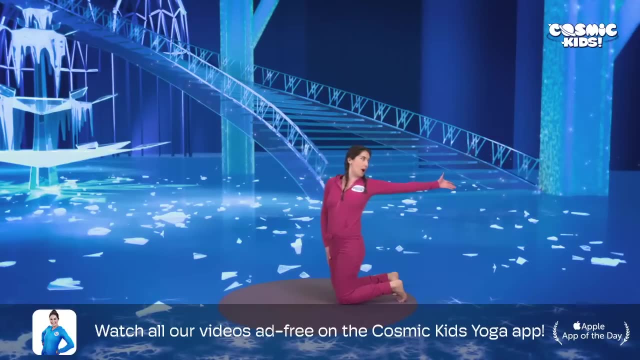 I only wanted to marry you so that I could get closer to the throne. And he puts out the fire. Come high up onto your knees and spread your arm wide behind you putting out the fire. And the other way, spread the other arm wide too. 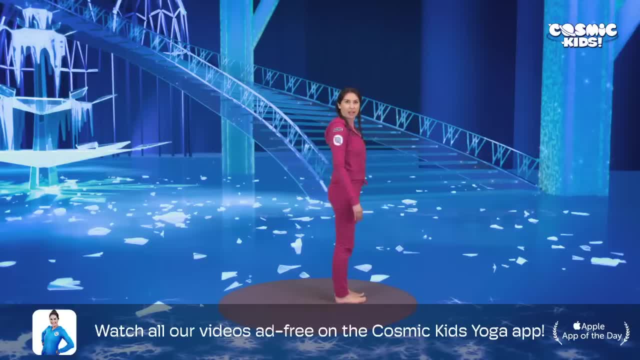 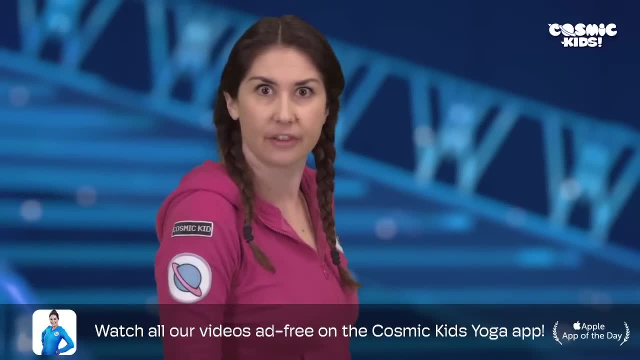 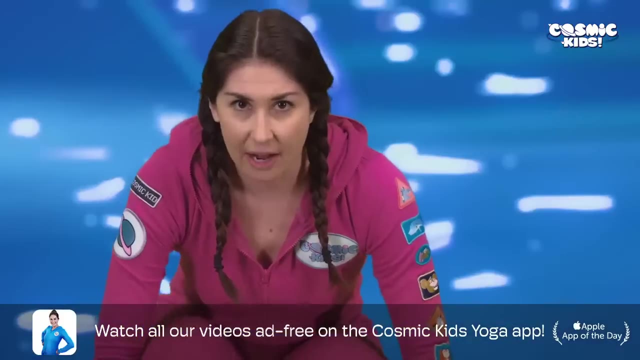 Then he stands up, turns his back, locks the door and leaves, charging Elsa with treason for Anna's death. Elsa is back in her cell And she uses every last ounce of her power to blast her way out. After three, we're going to do a big jump and a boom. 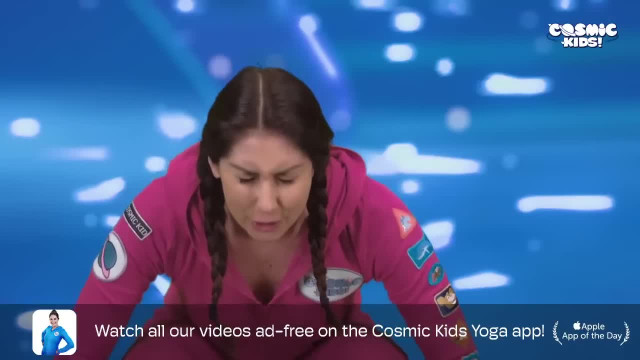 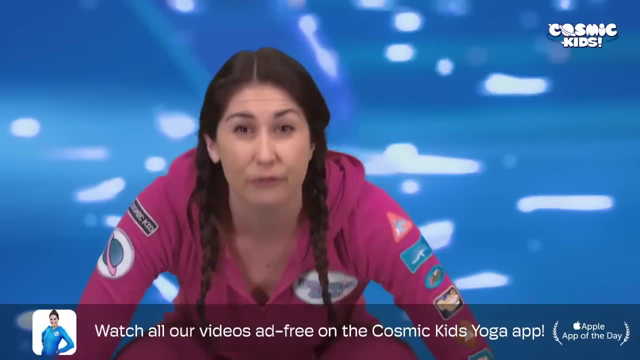 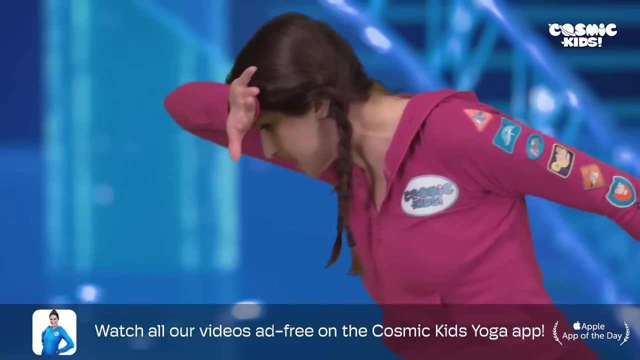 Ready Ice blast. One, two, three, Boom. Elsa escapes out onto the fjord, into the blizzard. One leg forward, bend your knee, protecting herself with her arm against the fierce, fierce snow, Turning herself the other way, turning your legs the other way. 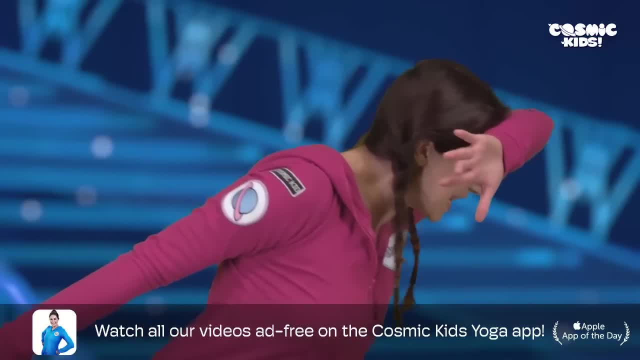 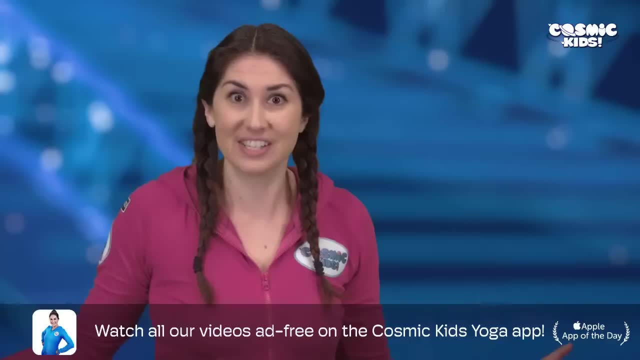 bend your front knee and put that arm in front of your head to protect yourself on the fjord. Back in the castle, Olaf finds the room where Anna is trapped. He's standing your heels together. bend your knees, hands above your head. 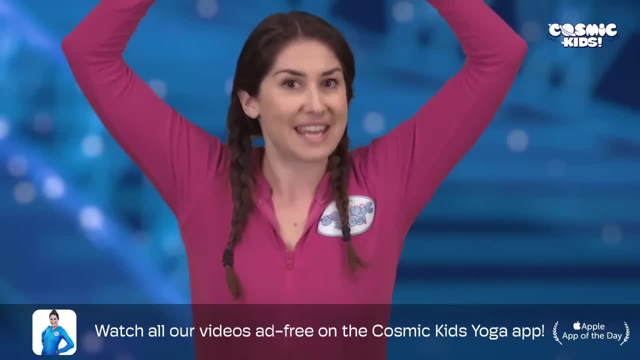 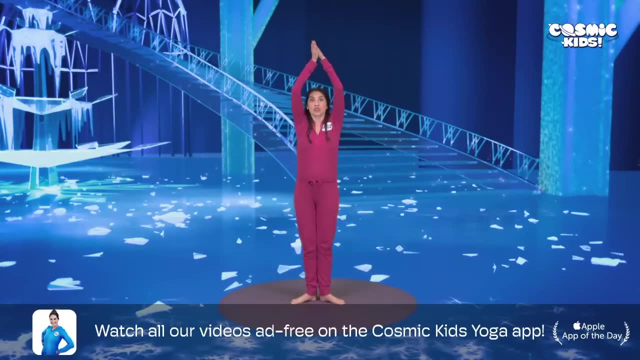 But he needs to get in. The door is locked. So he removes his carrot nose Hands in front of you and he puts it in the lock And it opens. But inside poor Anna she's freezing to death. Quickly he comes to the fire, building a lovely, lovely log fire, crossing your legs. 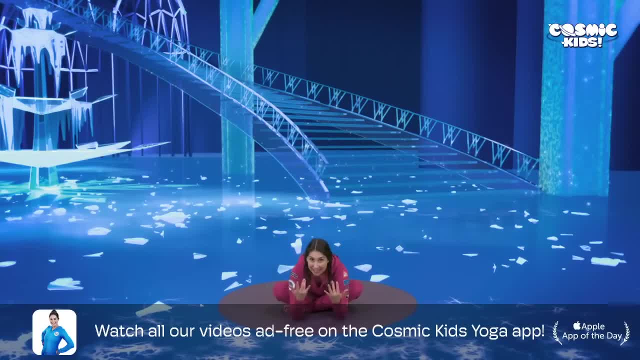 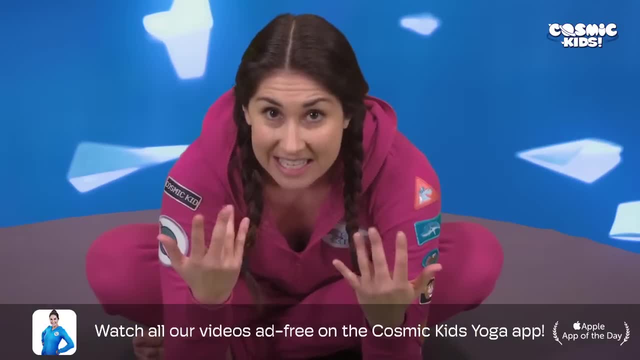 turning all the way forward and making it come to life with your fingers, like crackly flames. He nearly loses his own arm into those flames as well. He gets Anna warm and he tells her that Kristoff is in love with her and that he will be able to save her. 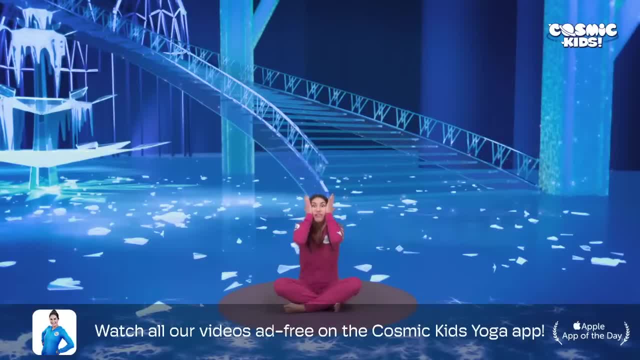 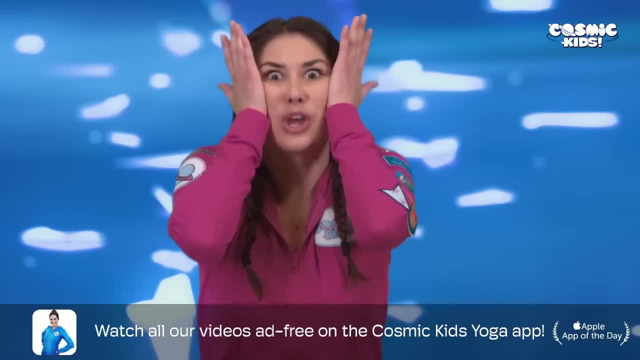 But Olaf, your face is melting. Olaf holds his face. He must get out of this warm room really fast, otherwise he'll melt entirely. The window pops open, standing all the way up, folding all the way forwards, opening the window. 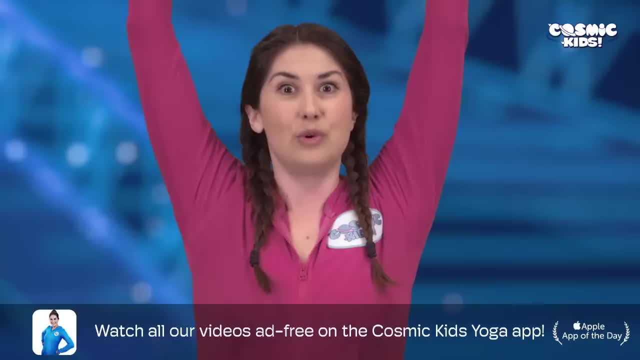 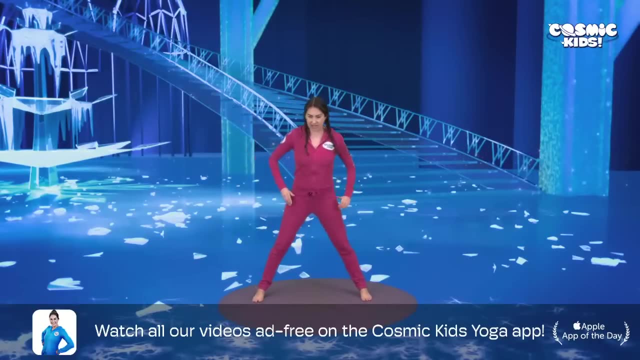 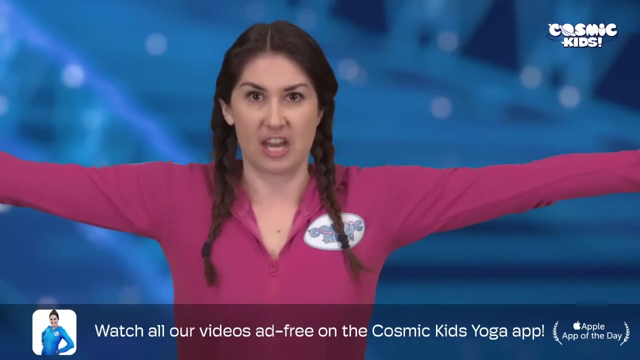 Whoop. They head out onto the fjord to find Kristoff, to save Anna. Out on the fjord, Prince Hans, standing with his legs and arms out wide, finds Queen Elsa. He tells her that she has killed her sister Anna. 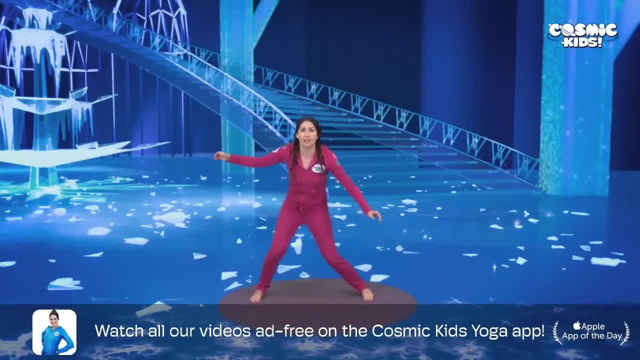 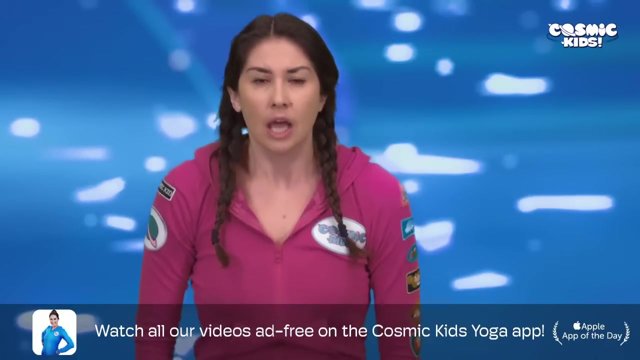 Hearing this, Elsa collapses to the ground in grief: It's all her fault, and now her sister is dead. Coming up to sit. As she does this, the whole of the winter suddenly ceases, The storm stops, And in that moment Anna and Kristoff can see each other across the fjord. 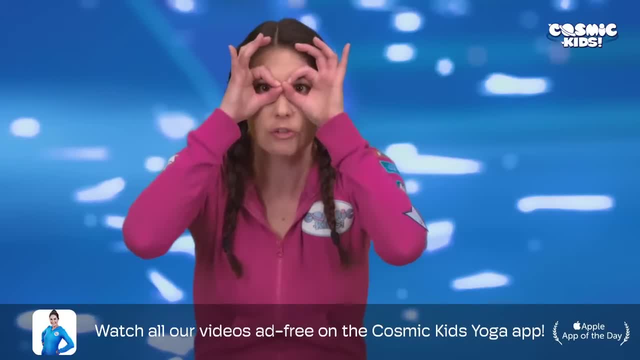 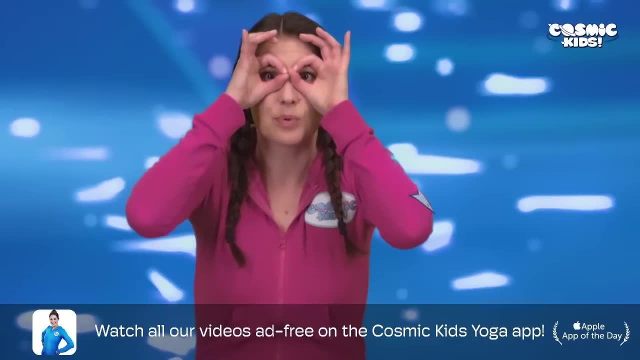 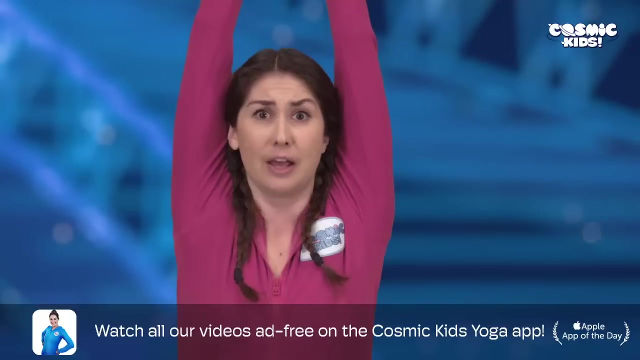 Joining your fingers and thumbs together. have a look through. They start running towards each other. But then Anna sees Prince Hans raising his sword above his head, about to bring it down on her sister Elsa. She can't let him do this. 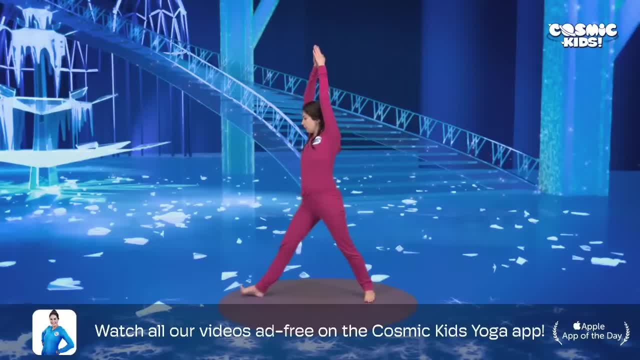 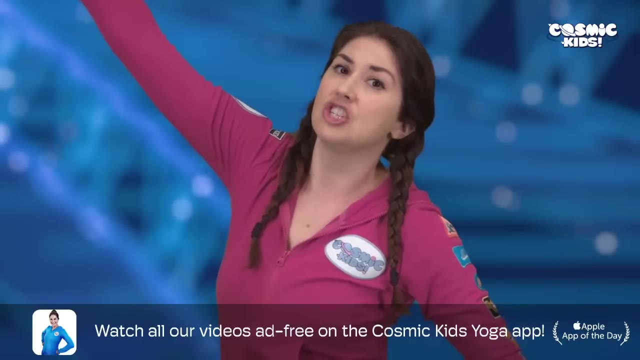 So she jumps into the way. Turn your foot to the side, Bend your back knee and protect Elsa with your hand. Reach your other hand up. She says: Stop. As she does this, she freezes entirely. In that moment the sword comes crashing down on her hand. 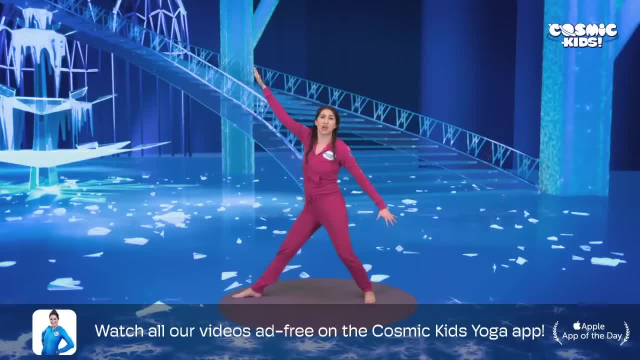 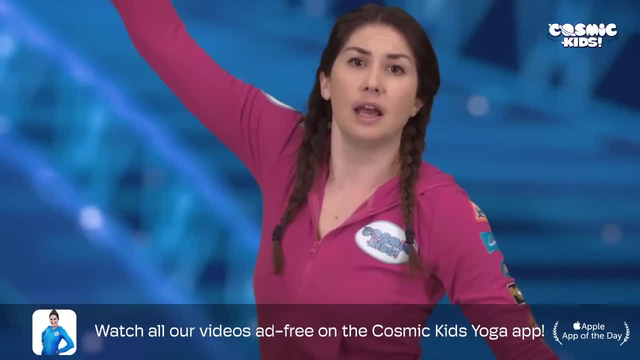 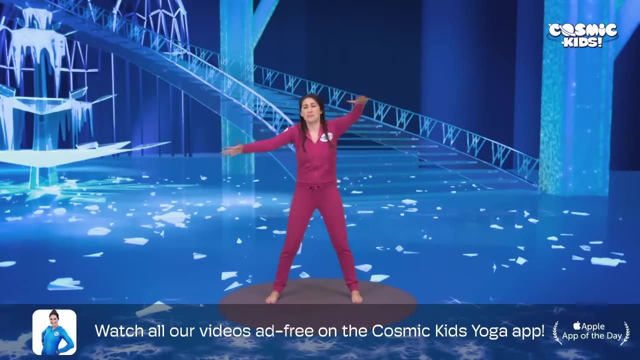 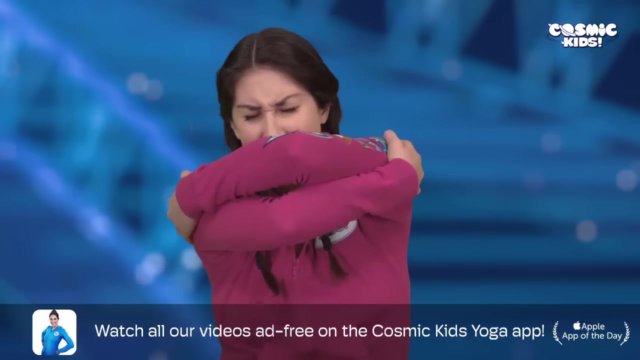 and splinters into a million smithereens. Prince Hans jumps back. Anna has frozen solid. Elsa slowly stands up to see her sister, completely frozen. She wraps her arms around her sister, crying in grief for what she has done. As she does this slowly, Anna begins to thaw. 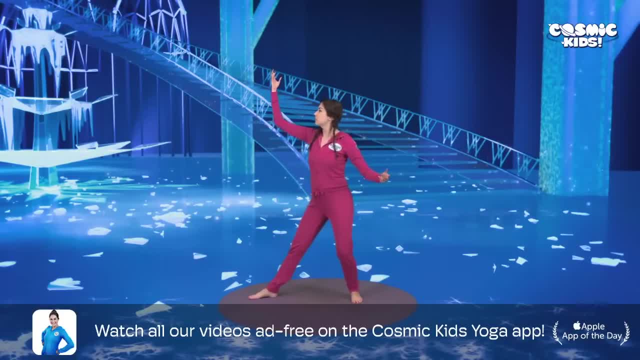 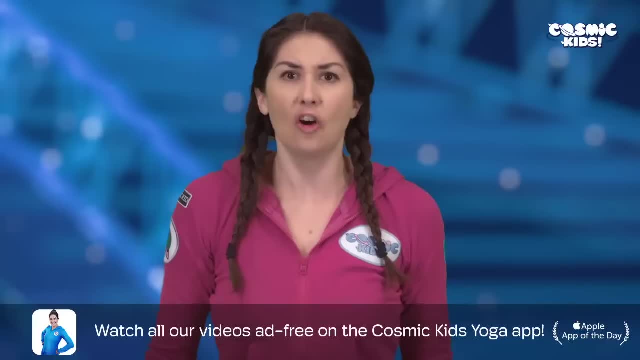 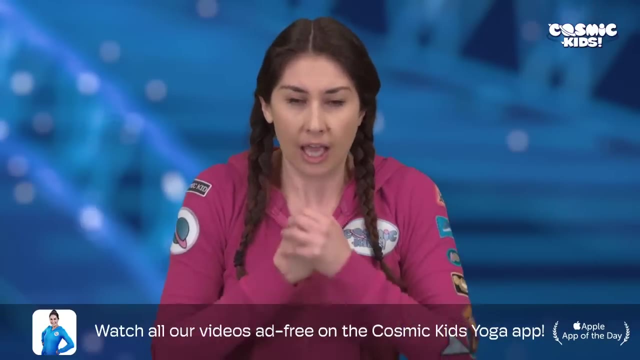 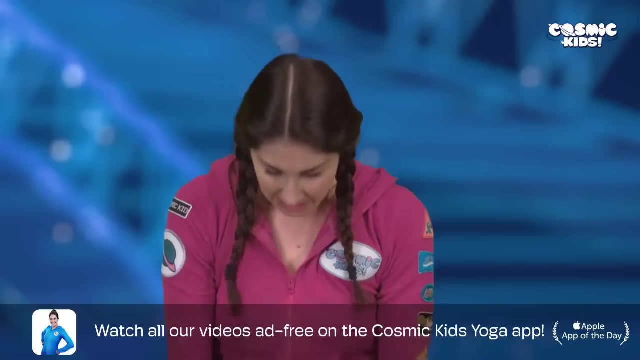 The ice starts to melt As she comes back to herself. she realises that by standing in the way of Prince Hans and protecting her sister, that was an act of true love. And in that moment, Elsa realises that love is the way to control her powers. 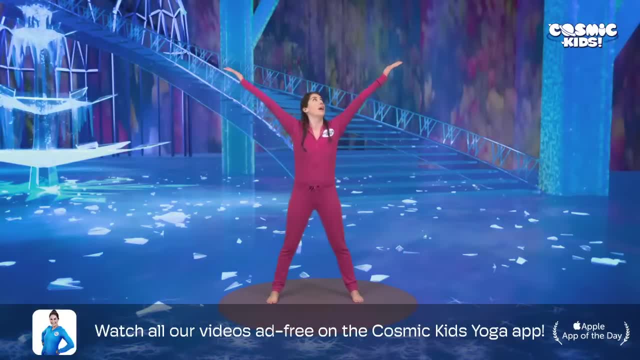 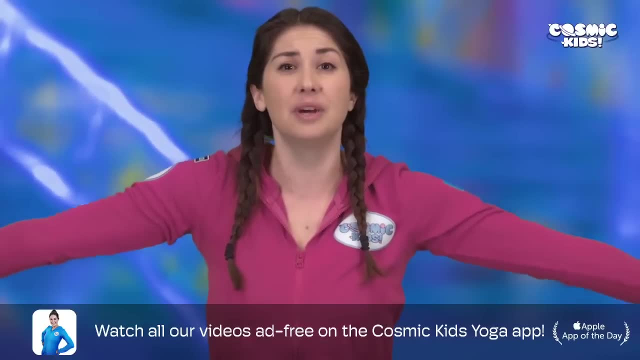 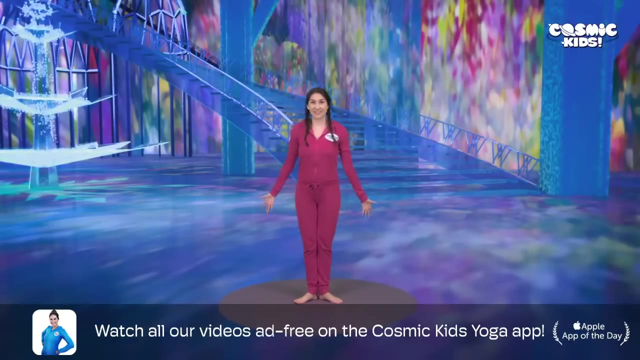 She raises her arms up to the sides And all sign of winter disappears as the sun and the spring and the summer come through. This is what she needs, Love Olaf, bringing your feet together, your heels together, bend your knees, join your fingers above your head. 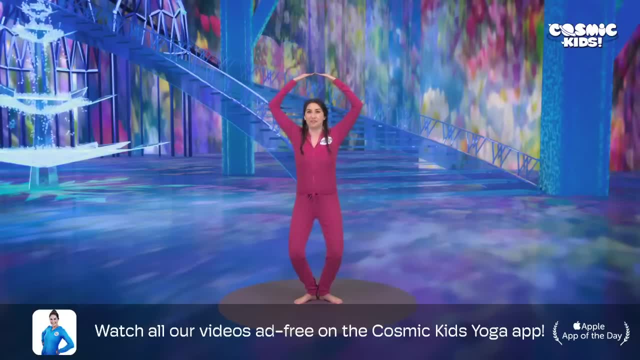 is made a little flurry, a personal flurry of snowflakes to keep him eternally in the winter. Criss-cross your fingers, take them behind your head, Flurry, flurry, flurry, flurry, flurry, flurry, flurry. Anna and Kristoff share a kiss, coming down to your knees. 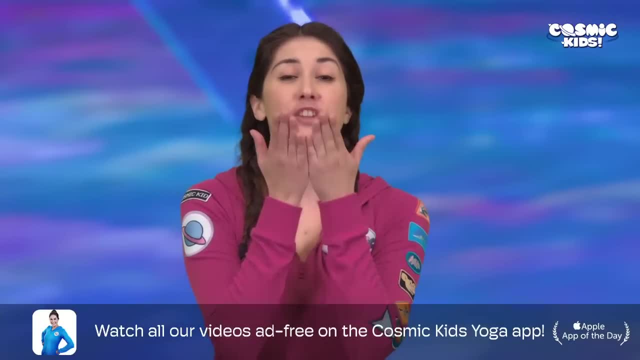 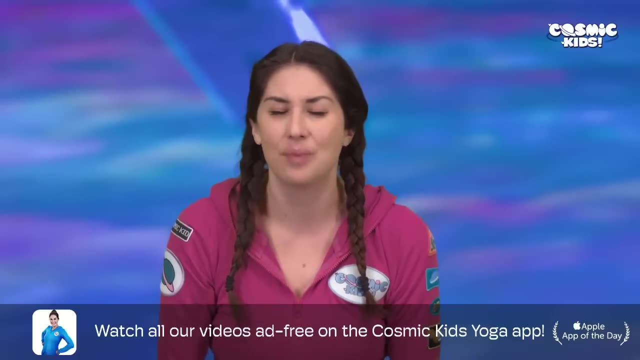 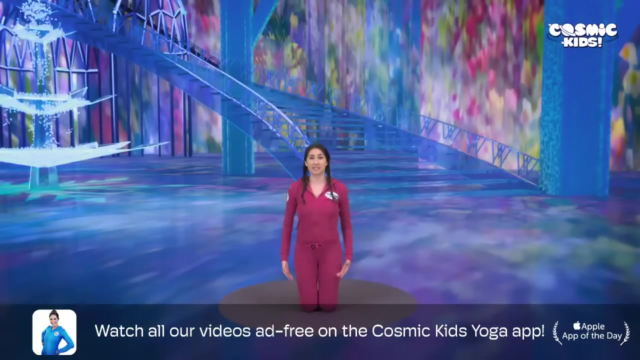 After three, one, two, three. Anna and Elsa once again are the best of friends. Arms wide, stretch them round yourself, wrapping yourself in a hug, And Elsa promises to keep the castle gates open. Leg to the side, arm up high, lean all the way over. 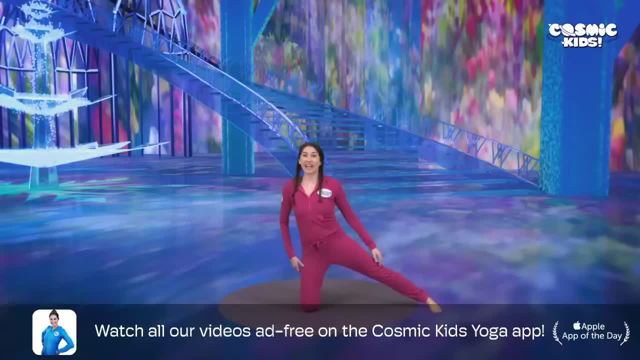 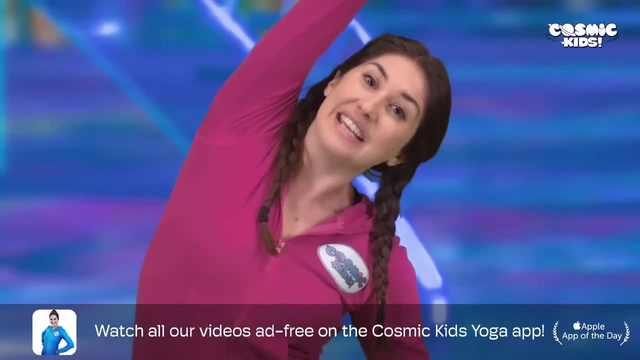 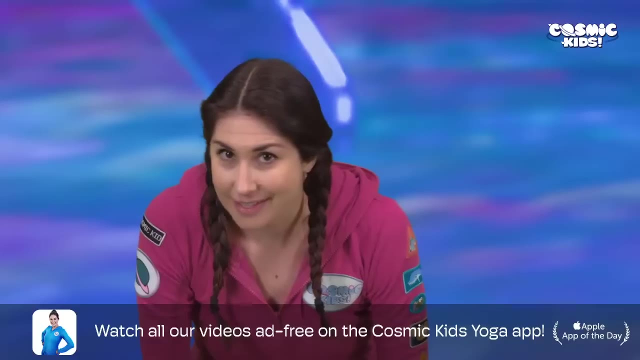 And switching sides, knees together, leg out to the other side, arm up to the sky. She will never close these gates again. Well, we're ready for a little rest and we've just, I, spied the sled. This is Kristoff's new sled, so we go and have a nice rest in it. 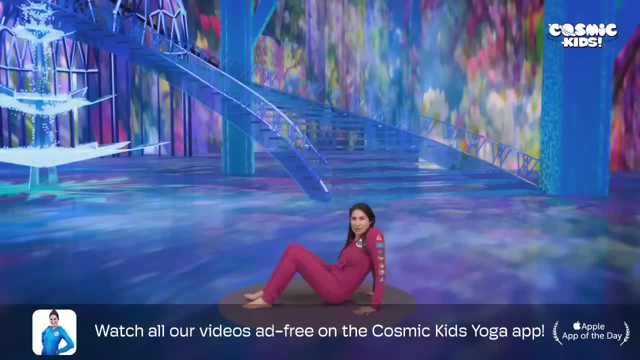 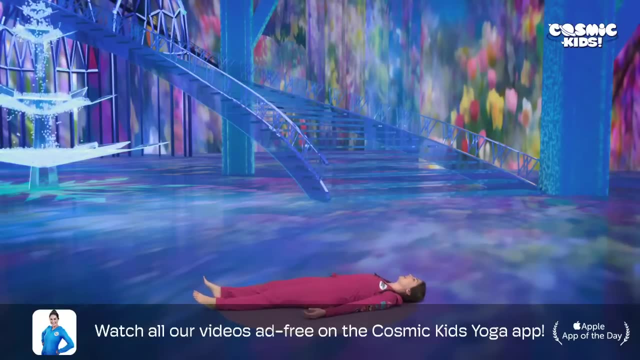 We lie down, Oh, it's so comfy and cosy. We put our bodies all the way down on the soft comfy blankets And we let our bodies go, We relax, We relax back Hearing those words of Elsa's song: Let it go. 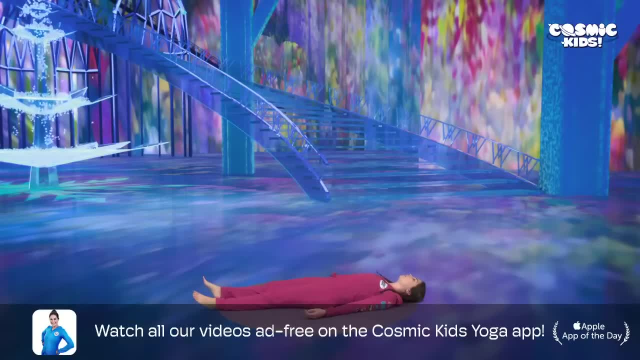 Let it go. We are one with the wind and the sky. As we lay here, we bring our hands to our heart And inside that heart we can feel the warmth, A warmth which is love, And we know the power of that love. 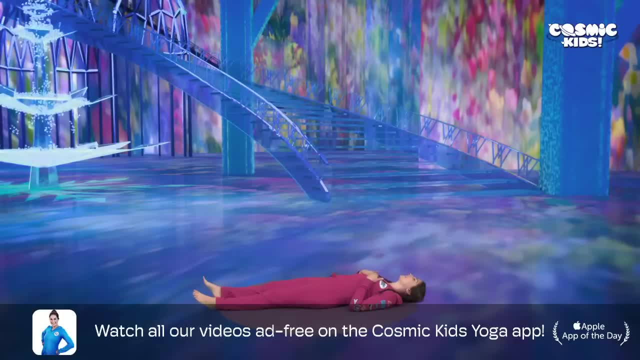 What it means to share it, How, when we share our love, we spread warmth. We spread something really special. With all that love inside, We will share with our friends and our family, With everyone. we know All the love we have And from sharing it there will be more love. 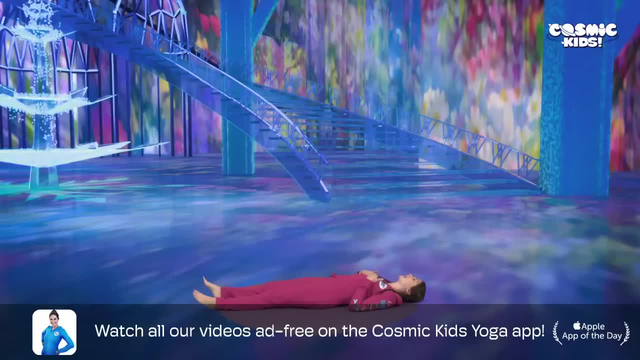 But now it's time to slowly come back. We take our arms down by our sides And wiggle our fingers and our toes to thaw them out. We stretch our arms up high above our heads and our legs long, Making ourselves into a long popsicle shape. 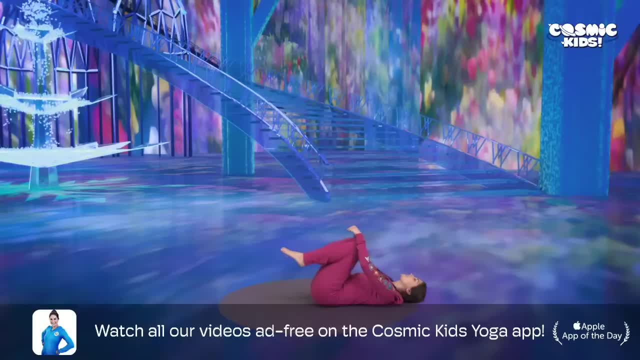 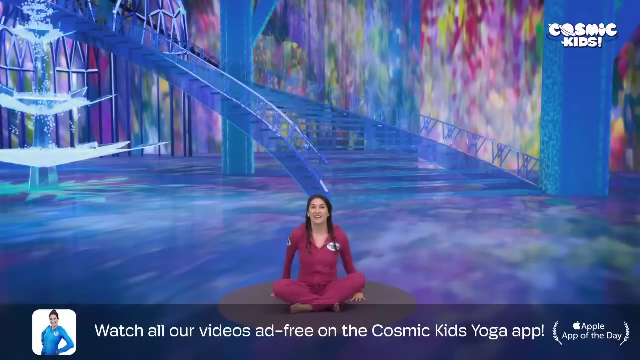 Then we draw our knees into our chest, Hugging them in tightly And rolling over like a little snowball. Then we come up to sit And we cross our legs, Bringing our hands together at our hearts, And we finish just the way we started. 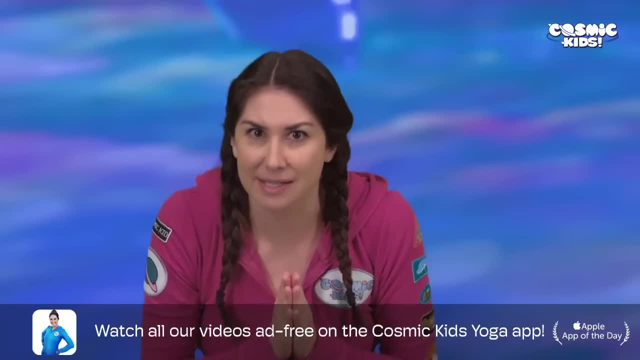 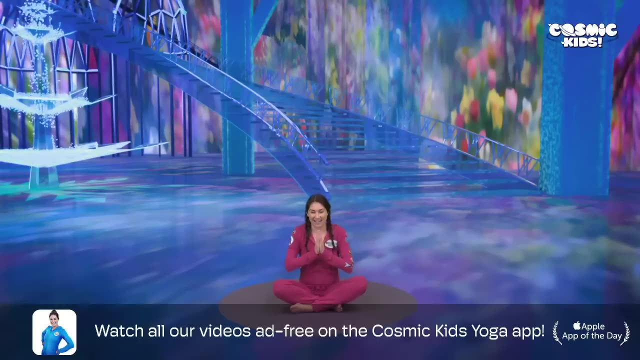 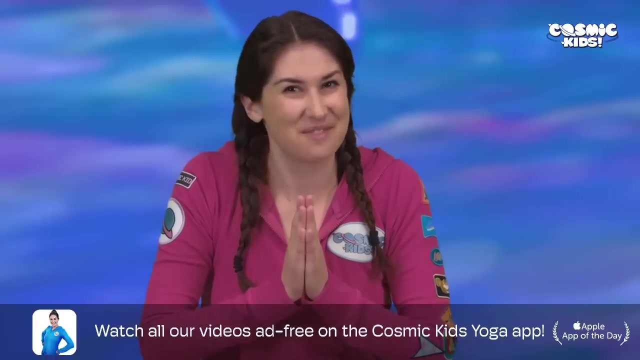 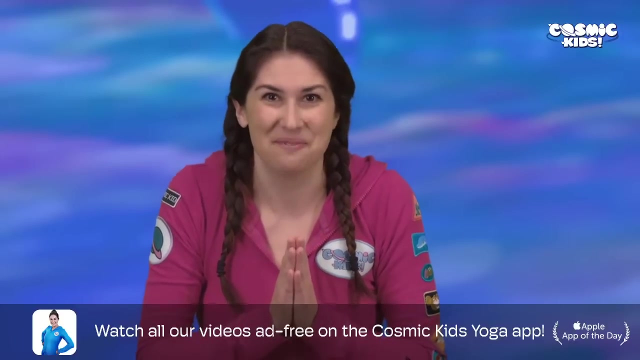 With our secret yoga code word Which is Namaste, Ready After three. One, Two, Three, Namaste There. Well done everyone. That was amazing. I loved doing the story of Frozen with you. I hope you enjoyed it too. 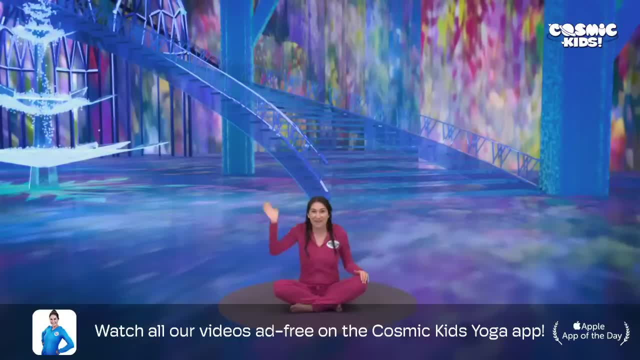 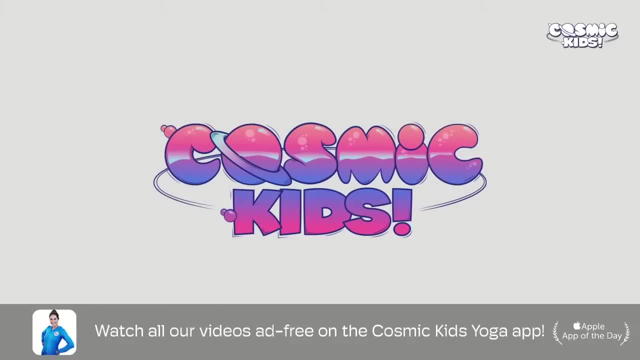 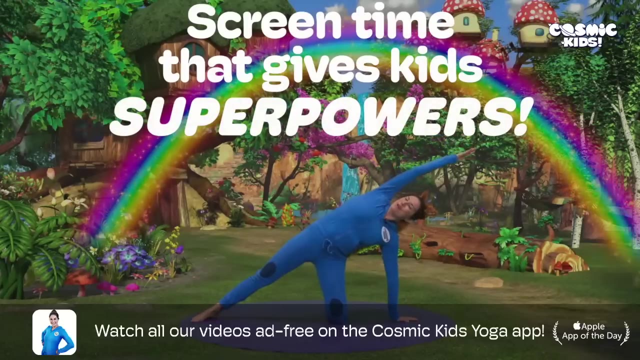 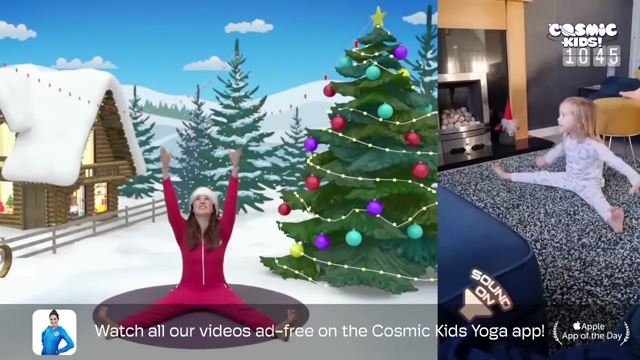 I'll see you again soon for another Cosmic Kids adventure. Bye, bye. Sweeping our top arm up and over, Making the most beautiful rainbow we can, Here we go, Whoosh, We take our legs out wide. We reach up very high for a big pot. 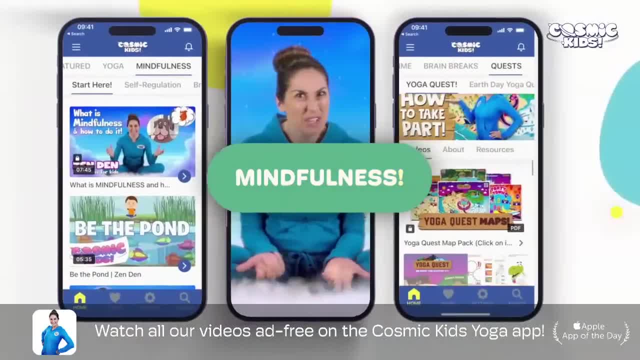 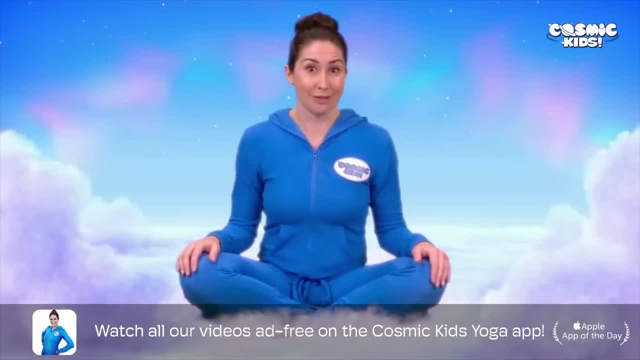 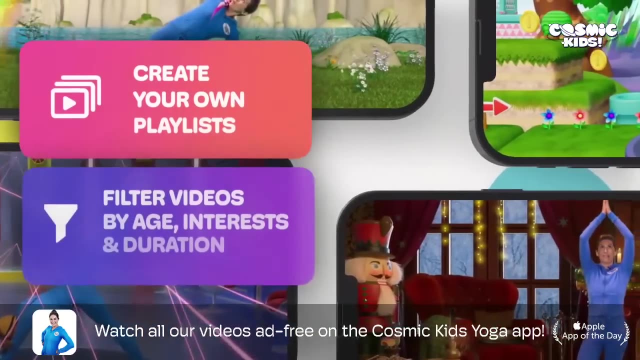 And we pop it down all the way in front of us. So what is it? What is mindfulness? How do we do it? And the best way to make the I can't thought go away Is to think: Oh yes, I can. 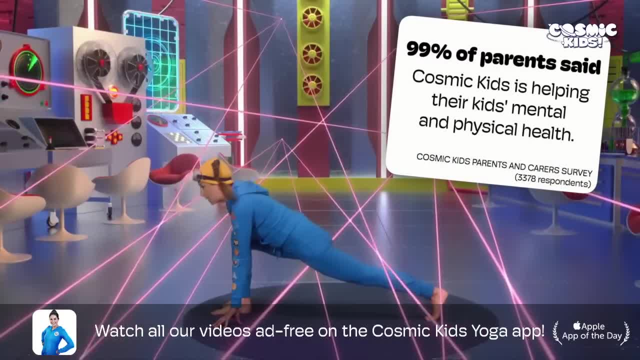 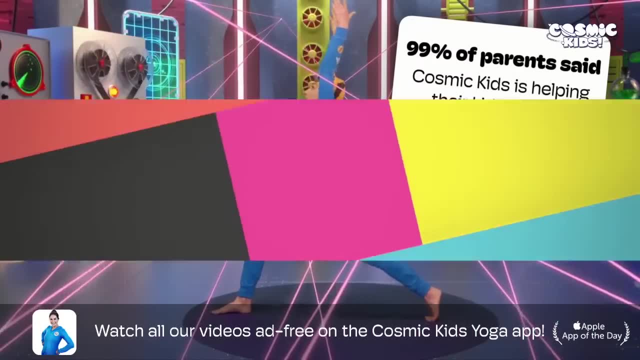 We step forward between our hands- Oh, thank goodness we do yoga Now, making our legs very strong. We lift all the way up, Trying not to wobble, Lifting our arms up to the sky, And then we fold all the way forwards. 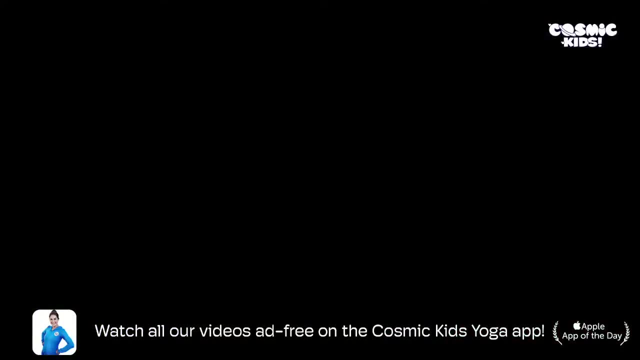 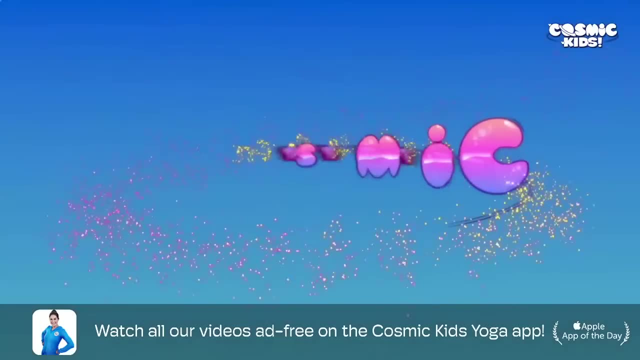 Hands come either side of our foot And we can make the I can't thought go away. And this is the physical act. What is it? How about we do the I can't thought go away? We step forward between our hands, Making the most beautiful rainbow. 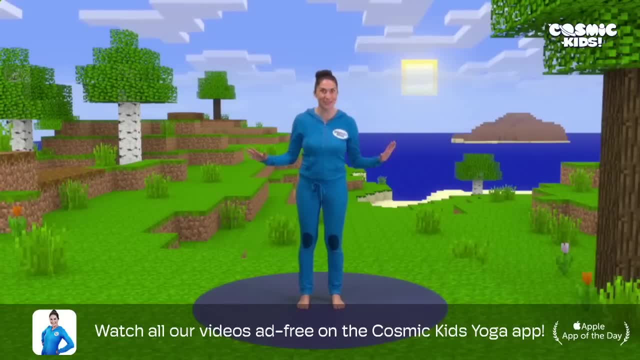 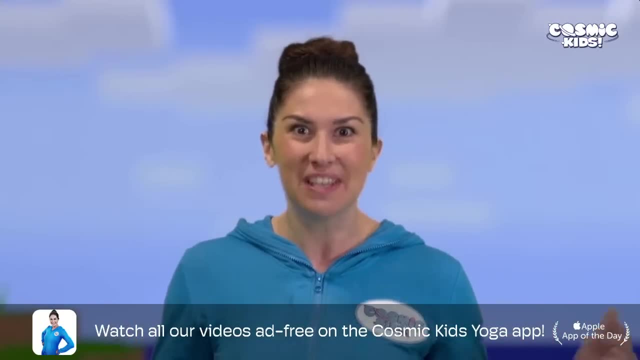 And we pop it down all the way in front of us. So what is it? We do yoga, Making the most beautiful rainbow, And the best way to make the I can't thought go away Is to think: How about we take our legs out wide? 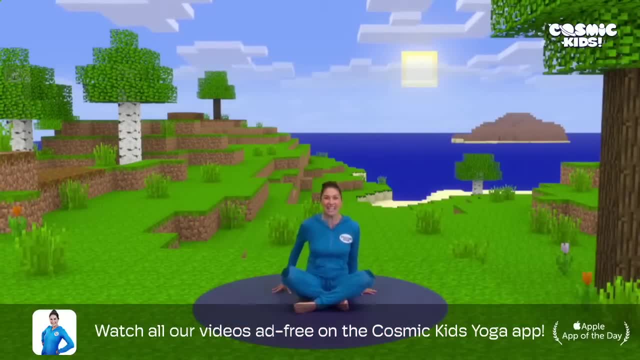 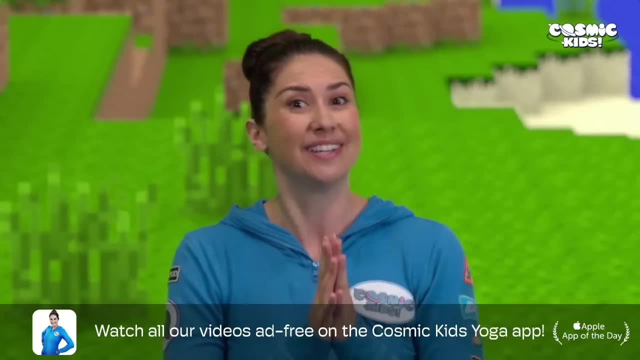 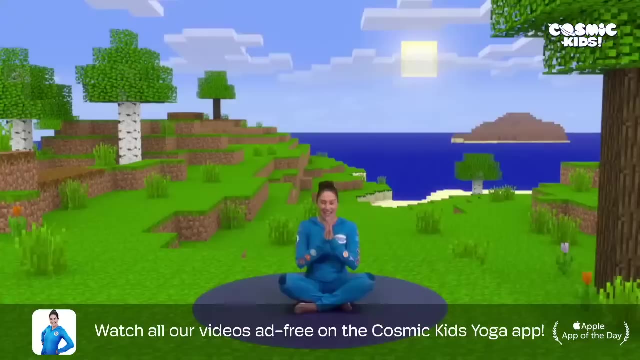 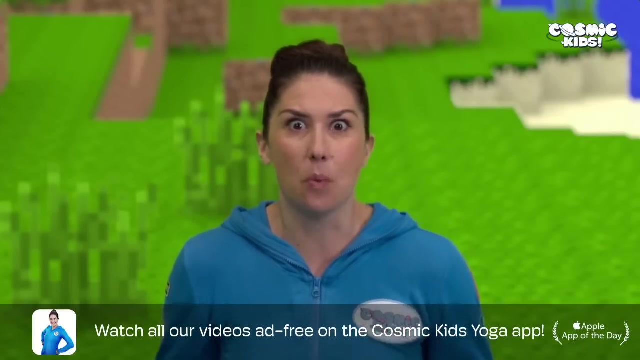 And we pop it down to the sky, Trying not to wobble, And we stop everything but our legs. What is it? hands together at our hearts and saying our secret yoga code word which is namaste, Ready After three, One, two, three, Namaste. There, Now we're ready to begin And today we're 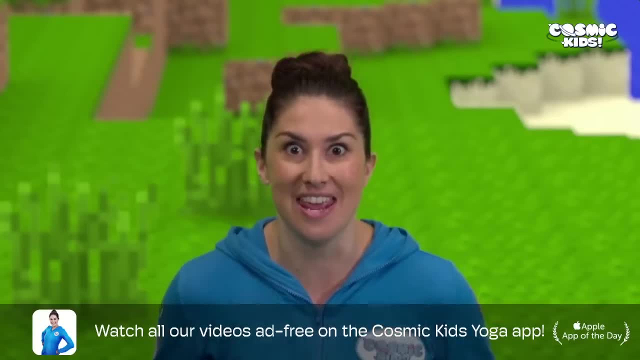 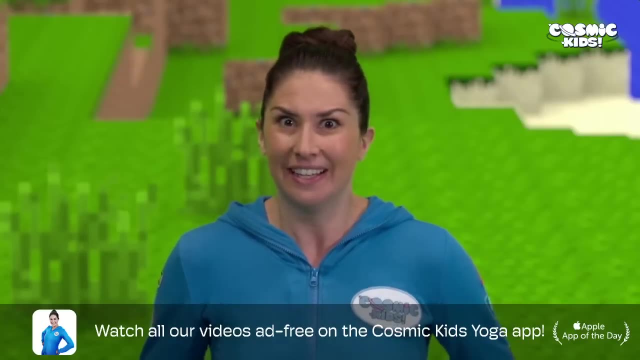 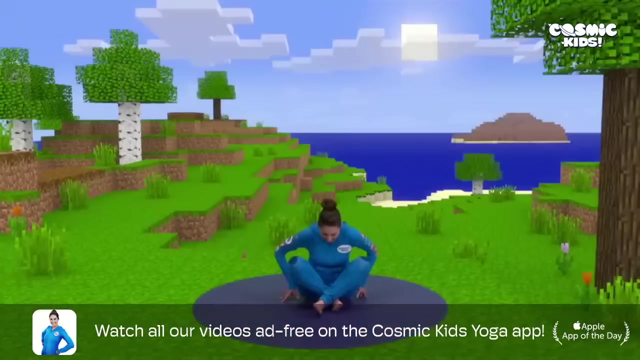 in a world of blocks. This is Minecraft yoga. It's our first day here and we've got to get ready for what lies ahead Now. it's very important that we survive here in Minecraft, so we have to build a shelter, a house. Coming up to stand, jump your feet wide, take your 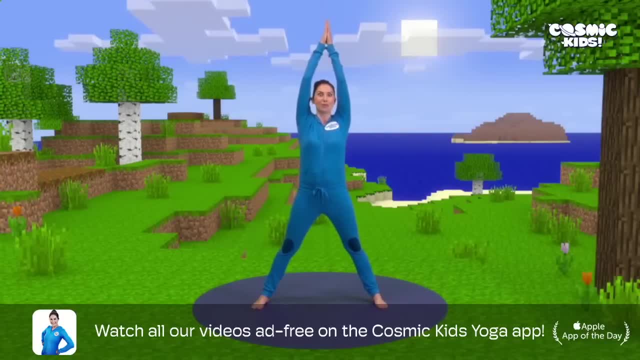 arms wide and bring them up above your head. Coming into house pose: Very good, Now we can protect ourselves from all the mobs of monsters that spawn at night. Taking yourself all the way forward, see if you can grab hold of your ankles and then clomp them like a. 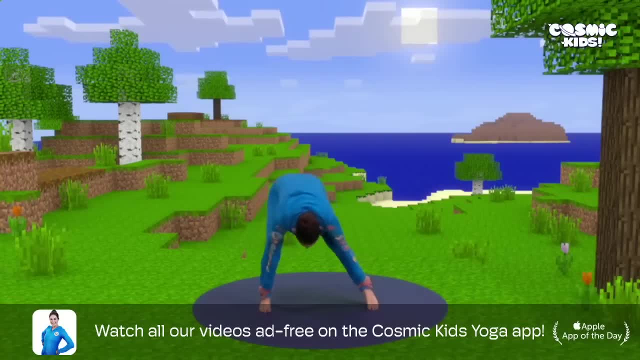 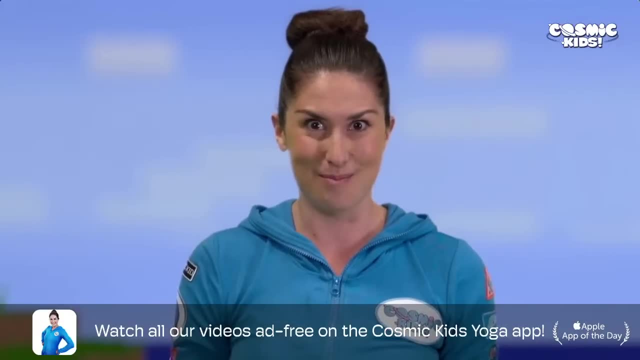 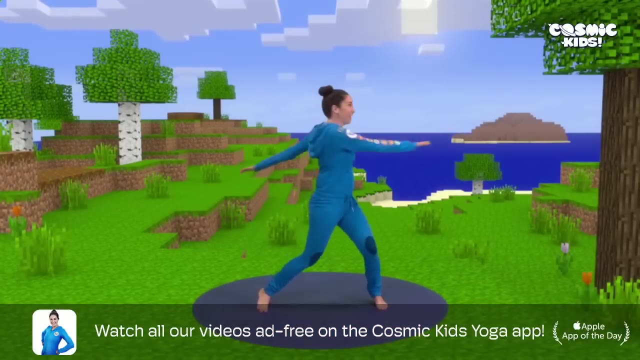 monster Coming all the way up. Now to get ready, let's spin into our Minecraft skin, Take your arms wide and begin to spin from side to side. Oh, you can even close your eyes if you like. Wow, that's amazing. Now we jump our feet into the middle and, oh, my goodness, I've got. 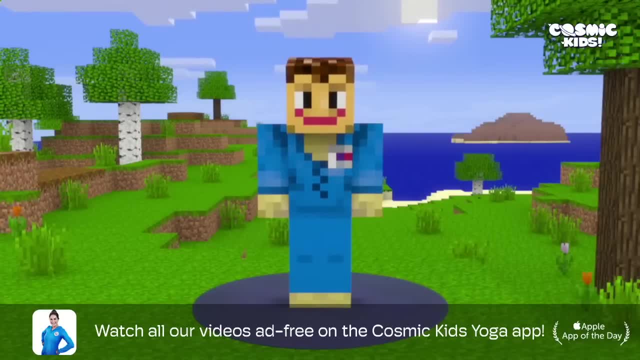 my skin on. Oh, this is interesting, isn't it? I wonder how we can move. Let's lift our arms, Oh yeah, and lower them, Oh, that's fun. I wonder if we can do any yoga. Let's turn to the side. 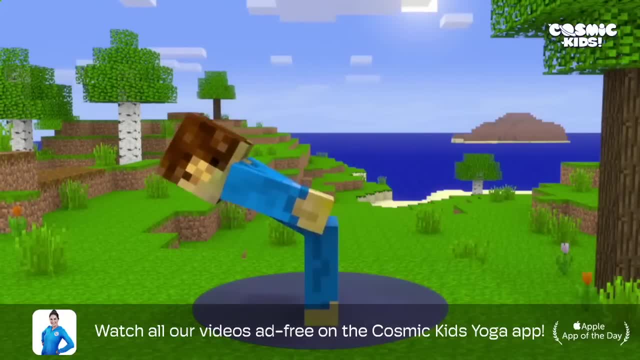 Here we go. Now let's fold all the way forwards. Oh, now I wonder if we can take our hands down. Oh, there we go. I wonder if we can touch our toes. Let's reach down, and oh yeah, oh yeah. 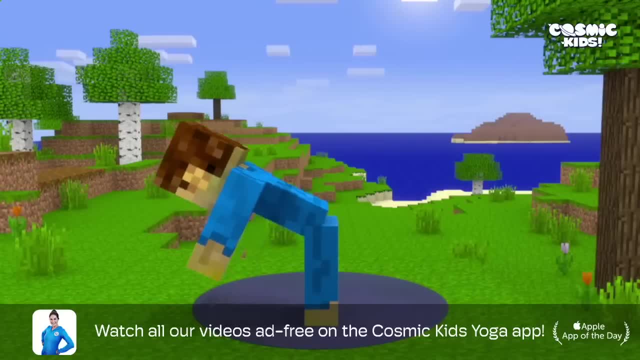 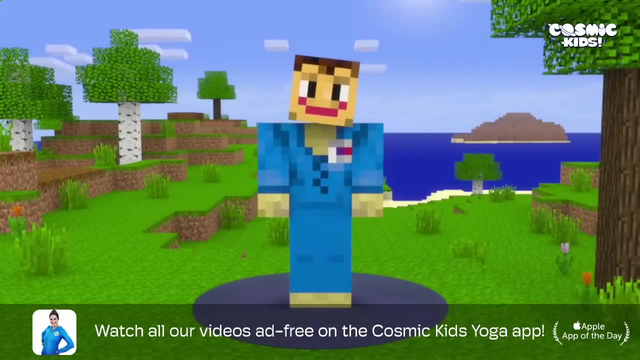 Oh, we did it. And come all the way back up again. Ah, and put your arms down. Oh, and turn to the front. There we go. Hmm, it's going to be quite interesting doing yoga wearing this. Maybe we can just pretend we're wearing the skin. Let's shimmy and shake it off. 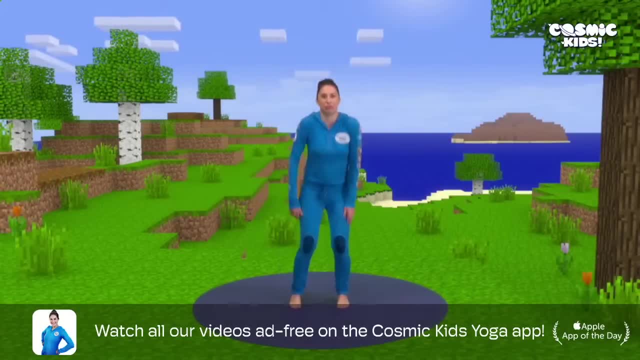 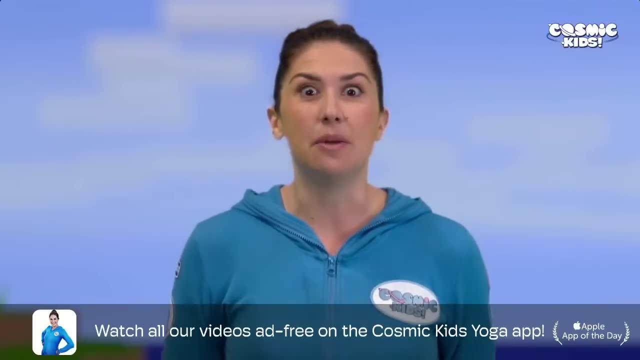 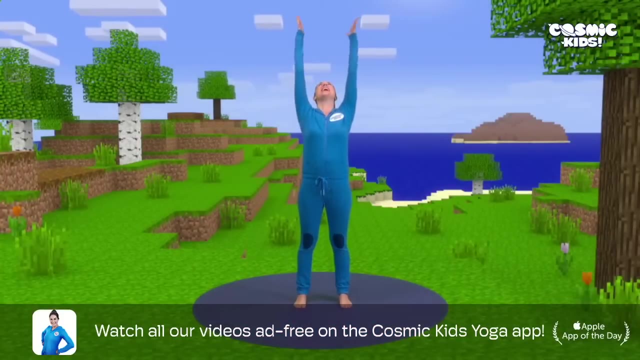 Ah, that's better. Now you can see me again and I can see you. We begin by looking at the sky. We're looking up to the sky and seeing the sun's out, So we wave and say hello sun. reaching all the way up and say hello sun. This is brilliant. It means we've got plenty. 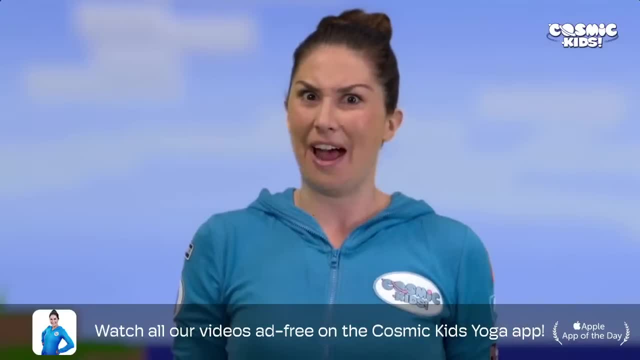 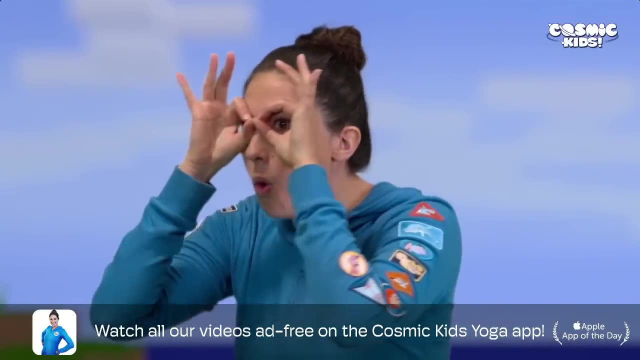 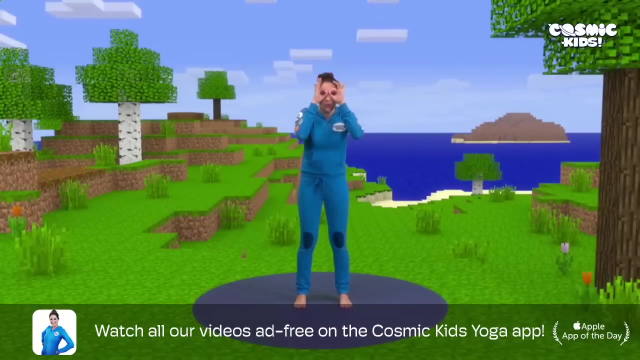 of daylight to collect all the things we need to craft. Now let's have a look around at where we are Joining your thumbs and fingers together. have a look through. Oh, it looks like we're on an island surrounded by an ocean. There are trees and rocks and all sorts of things. 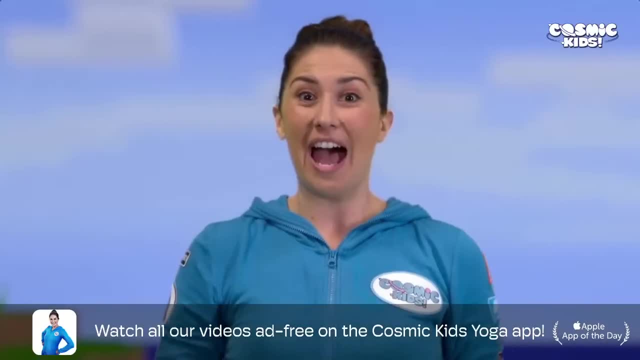 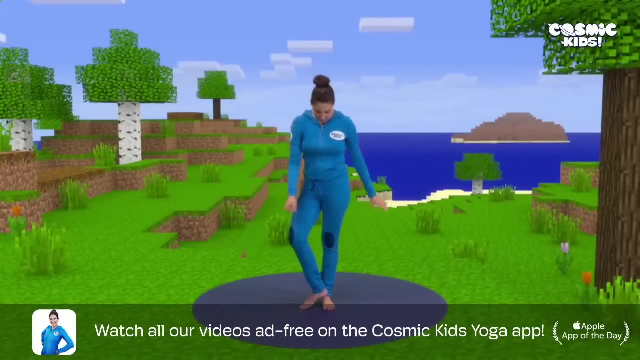 Plenty of what we need to get crafting. We lower our hands and we have to build a shelter, don't we? So look around and we see trees Coming into tree pose, bringing one foot on top of the other, your hands together, and grow your tree up nice and tall. Now I wonder: 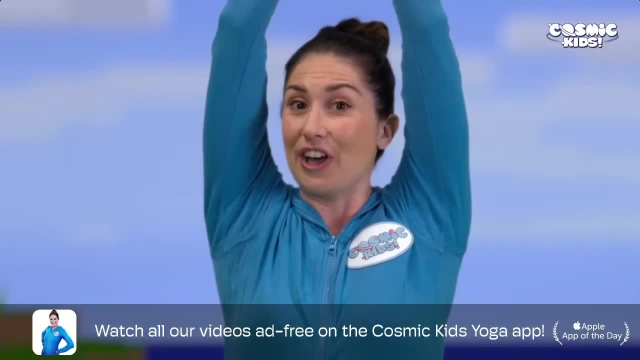 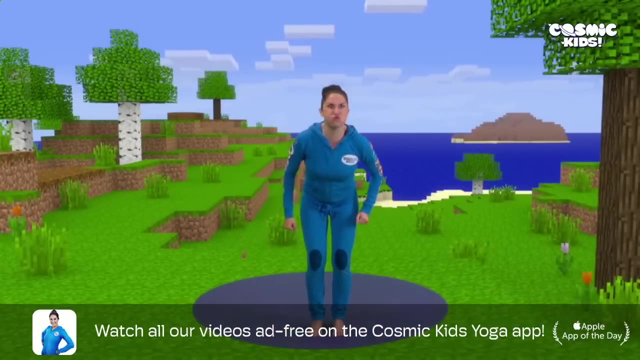 how strong are the trees here in Minecraft? I'm going to come and try and blow you down. You stay tall and strong. Here I come, Doop dee, doop, dee doo. Oh my God, Oh my God, Oh my goodness, You're so good at balancing, Let's try our tree on the other side Coming. 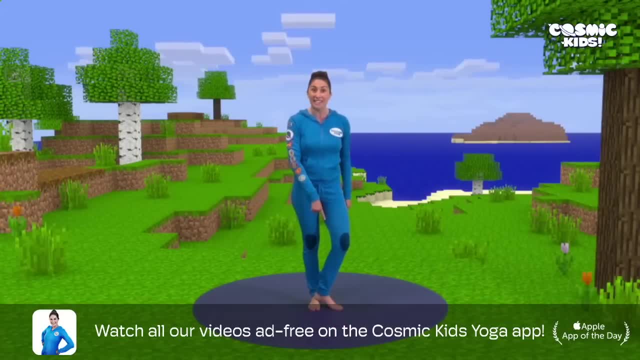 to stand with the other foot on top now, using your heel, balancing on your toe. Bring your hands together. Oh, try not to wobble and come up tall, like a very tall tree, And can you open your Minecraft tree branches? Very good, everyone, Now we've only got our bare. 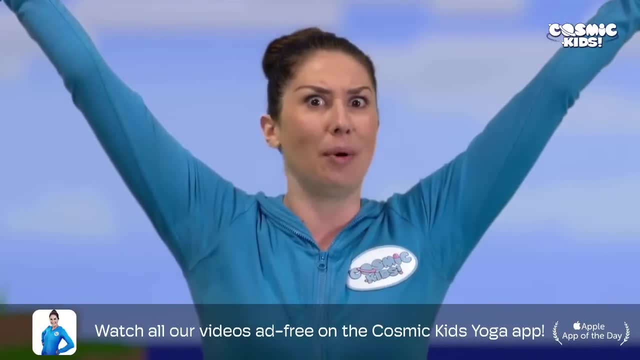 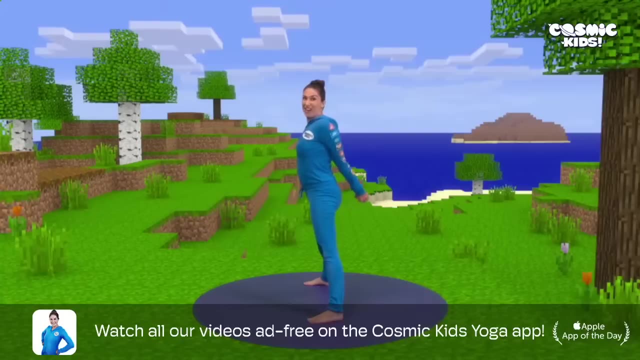 hands to chop these trees down. So let's come into woodchopper pose, Turning to the side, spread your legs nice and wide and crystal Squash your fingers behind your back, Stretch your arms up behind you and then fold forward as you chop. One, two, three chop And up. One, two, three chop And up. Last time. 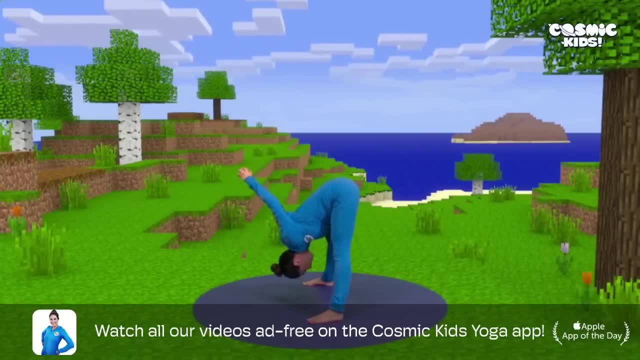 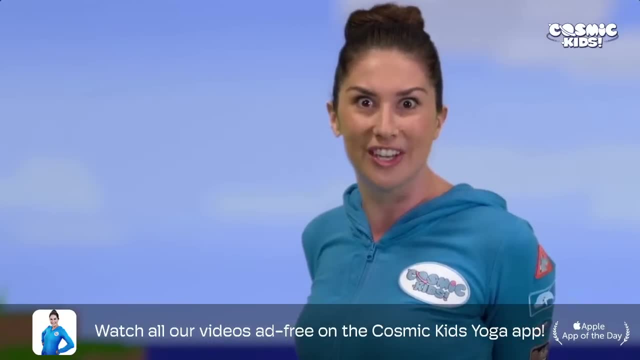 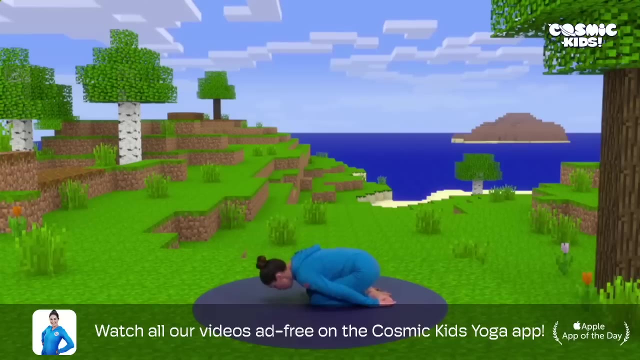 One, two, three chop And all the way up. Very good, everyone. Now we've collected lots and lots of blocks of wood. Coming into a block of wood, pose down onto your knees, tuck yourself up into a tiny block shape. brilliant. now we need to. 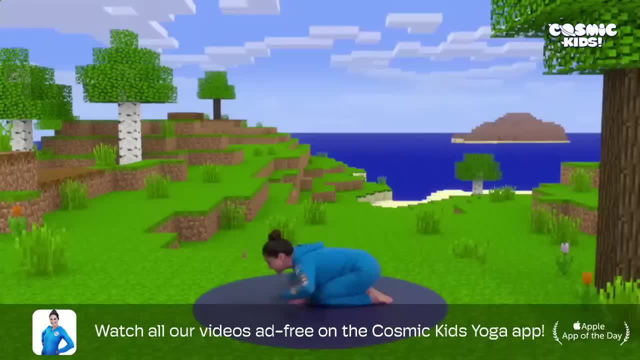 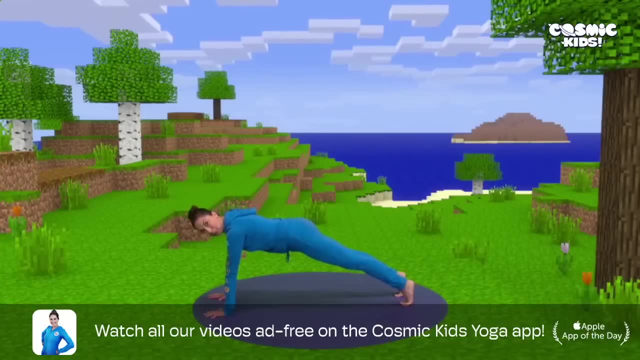 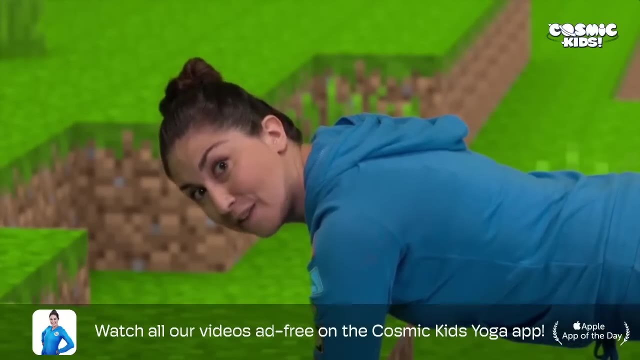 turn these blocks into planks of wood. so take your hands forward, come up onto your hands and knees and stretch one foot back, two feet back and come into plank pose, pulling your tummy nice and tight in your plank pose. very good, now with our planks we can make a very 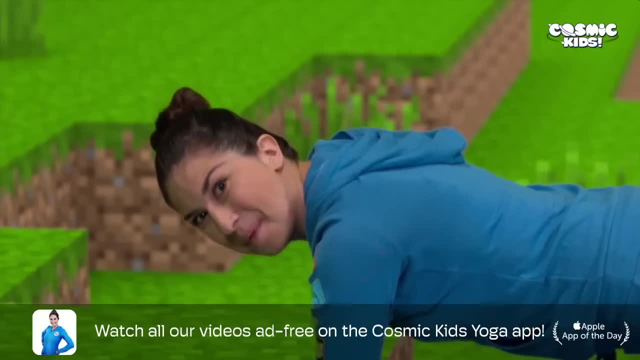 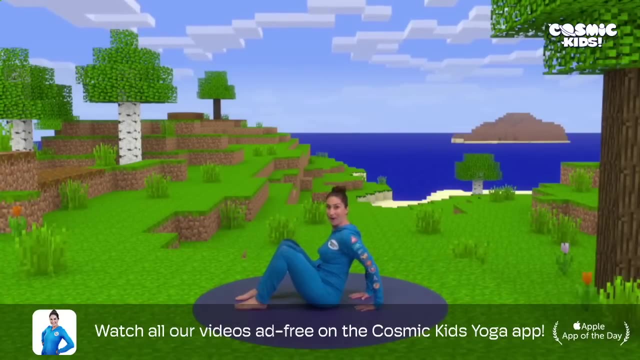 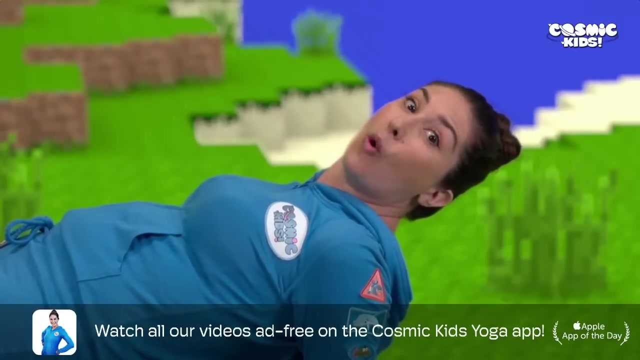 important thing, a crafting table coming into table pose. coming to sit on your bottom with your knees bent, your feet flat and your hands behind you and lift your bottom up coming into your crafting table pose. very good, now we can make all the tools we need. let's start. 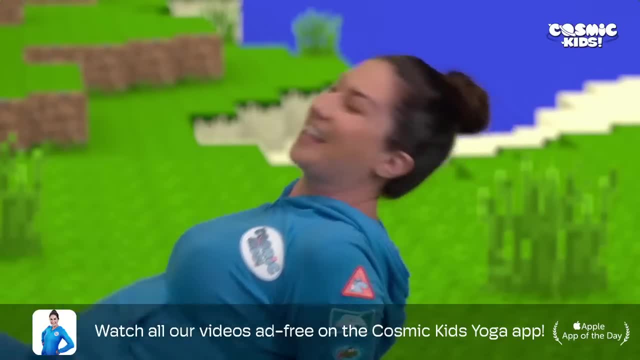 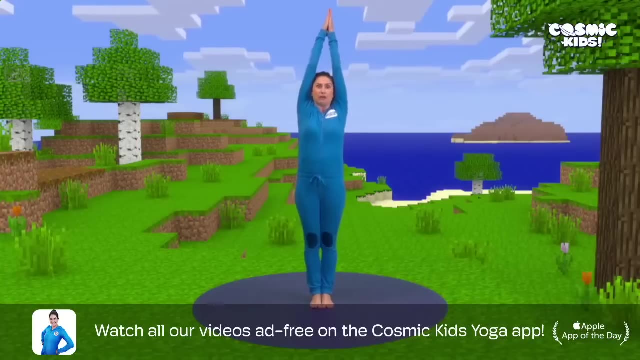 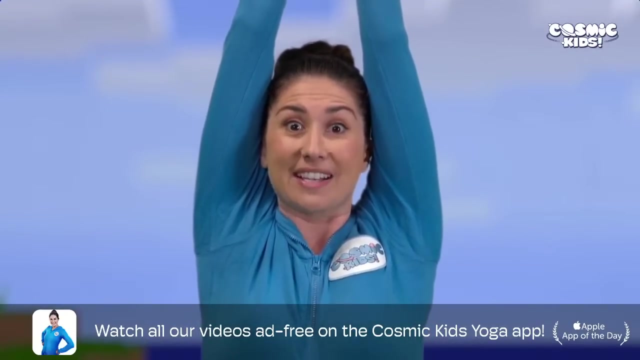 with a pickaxe. we need to make some sticks coming to stand in stick pose. standing with your toes together, your hands up above your head, making yourself as pointy as you can. very good, everyone. now we balance two planks on top of our stick to make a pickaxe in a triangle shape coming into dog pose onto all fours. 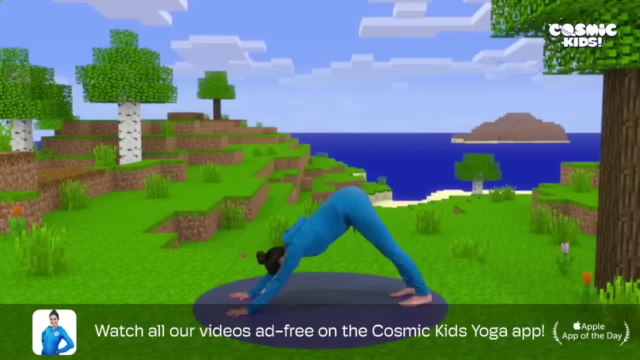 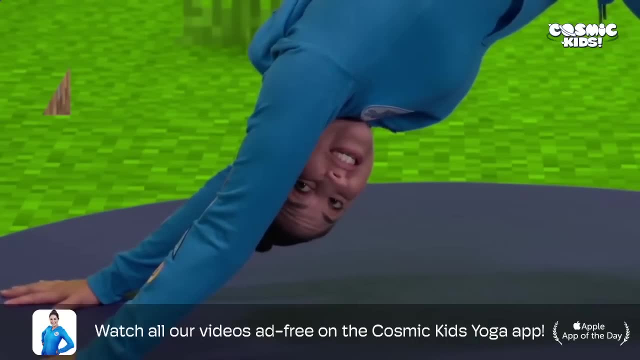 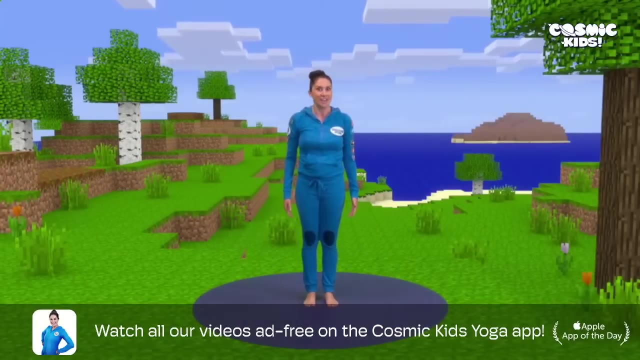 hands wide, tuck your toes and lift your bottom up to the sky, coming into your dog pose. yay, now we've made a pickaxe. we need to go and find some coal coming up to stand. we find a giant stone wall. hmm, there could be some coal in here. we jump our feet wide and our 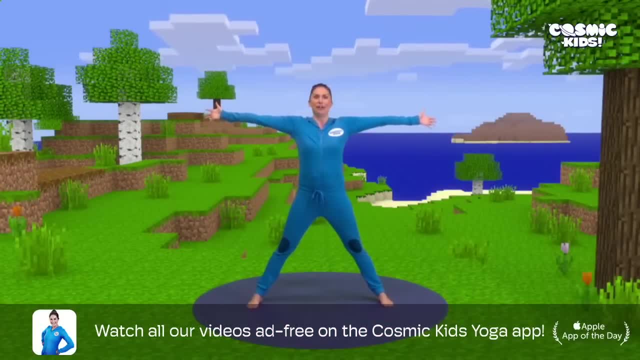 arms wide, making a giant stone wall shape. very good, now we've got our pickaxe, we dig at the stone wall. turning to the other side, now stretch your legs wide, criss-cross your fingers, stretch them out behind you and fold forward after three with a dig: one, two, three, 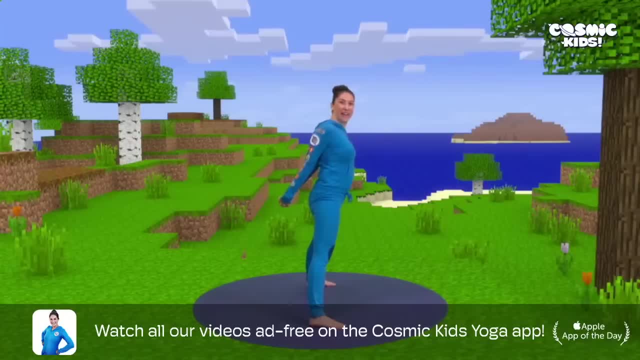 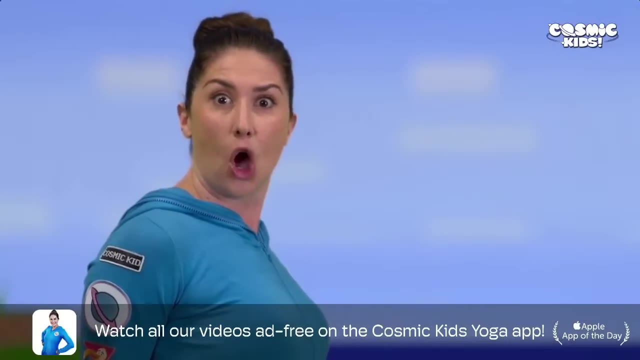 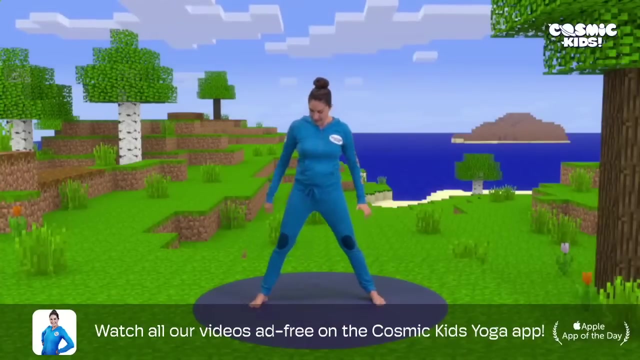 dig and up and again. one, two, three, dig and up. last time, one, two, three dig and all the way up again. very good, we've found some coal and we've managed to dig ourselves a cave. this can be our shelter, coming to stand with your legs wide and your hands above your head in your cave pose. well done everyone. 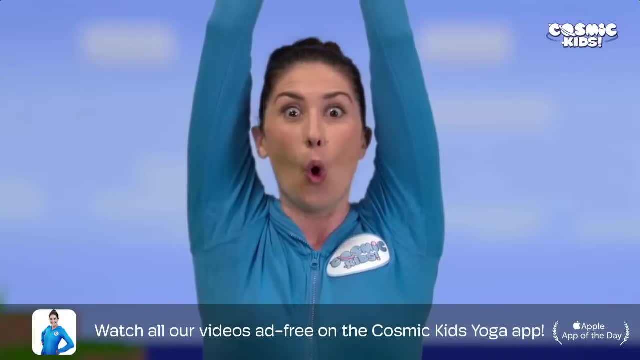 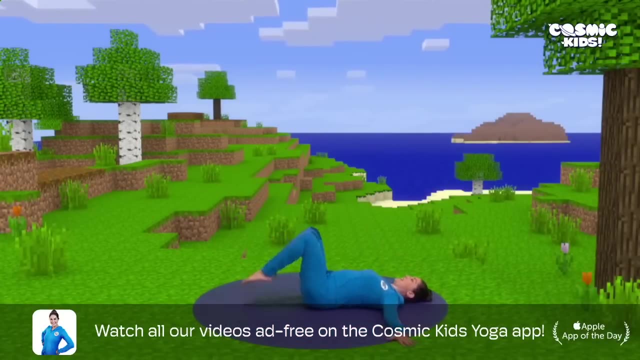 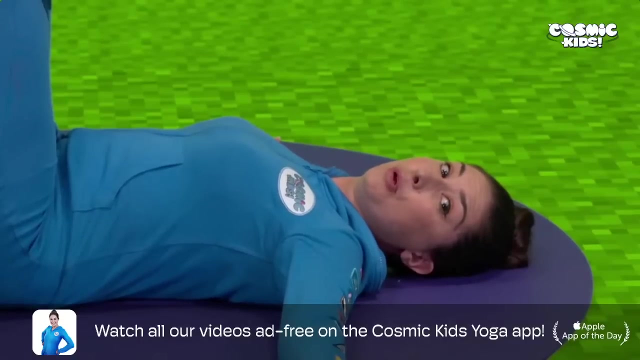 now, with our coal and our sticks, we're going to make some torches. let's come into candle pose Lying down on your back, stretch your arms out wide and lift your legs up to the sky and wiggle, waggle your toes like flames. Very good, We've put the torches up on the 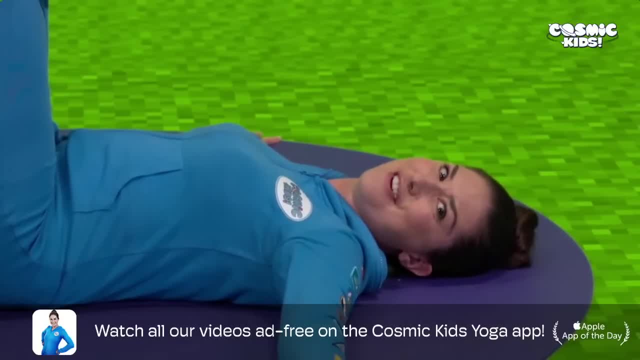 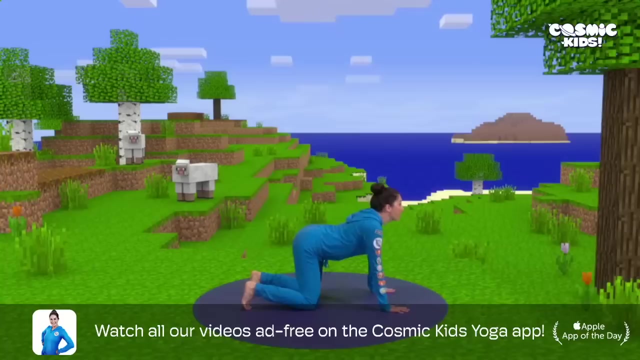 walls of our cave and we've got light. Well done, everyone. Now look outside our cave. We see some sheep coming into sheep pose, Sitting all the way up on your hands and knees. let's wiggle, waggle our tails and let's go. We could do with some wool so that we can. 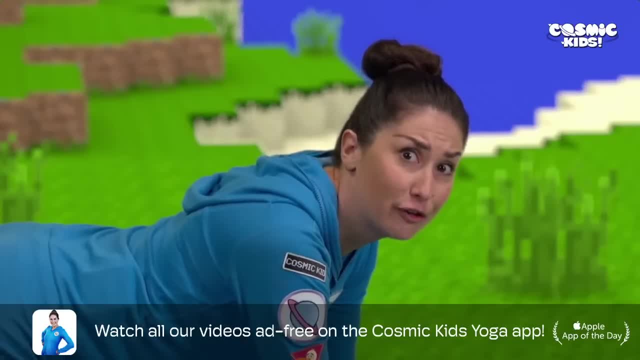 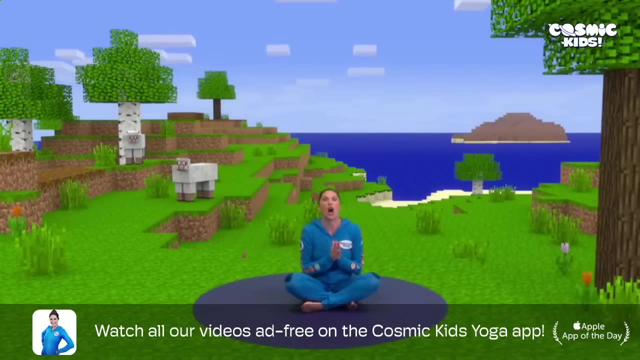 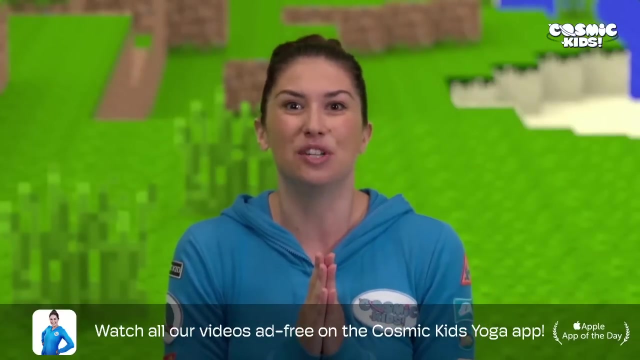 make a bed. Sleeping is very important in Minecraft. It's how we stay safe at night. We sit on our bottoms, we bring our hands together and we say: bar a stay to thank the sheep Ready. Bar a stay, Brilliant. We take the wool and we add it to a block of wood. 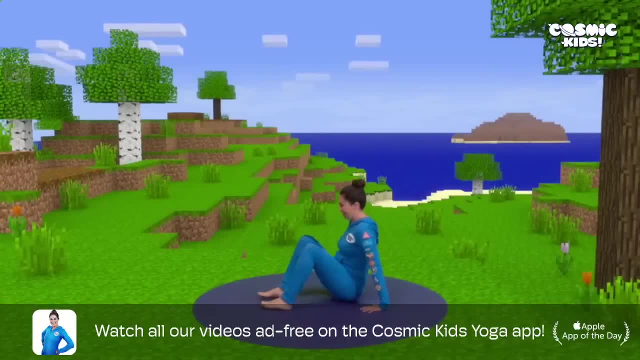 to make a bed. Coming into bed pose. Turning to the side again, Knees, bent, feet, flat hands behind you and lift up your bottom. Coming into bed pose: Excellent, Now we'll be safe at night. Look outside, everyone There. 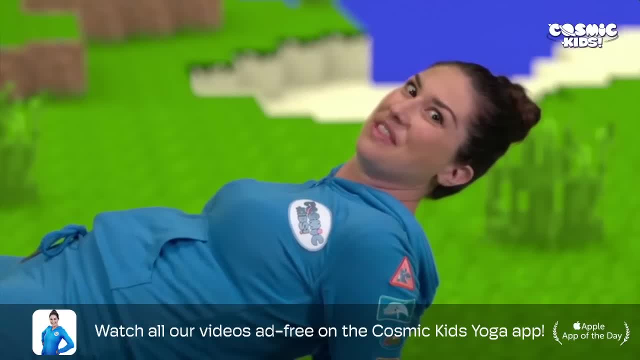 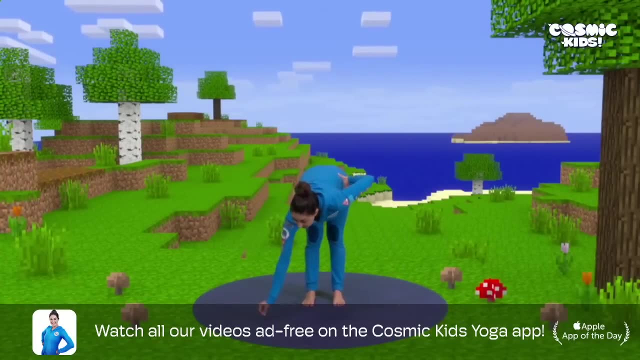 are some mushrooms, We can get some dinner with them. We come up to stand and we fold halfway forwards as we pick the mushrooms, Picking them out of the ground, collecting lots and lots and lots. Fantastic. Now we stand up tall. We need to craft a bowl so that we can put our mushrooms inside. 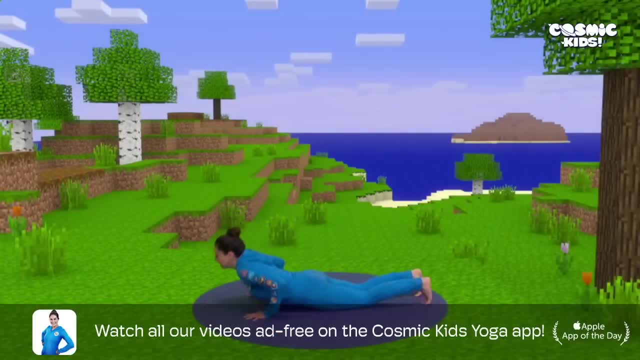 Coming into bowl pose, Lying on your bellies, put your hands under your shoulders as you bring your feet towards your bottom. Then reach around and see if you can grab your feet Now breathe in as you lift up. Very good, In your bowl pose we put the mushrooms. 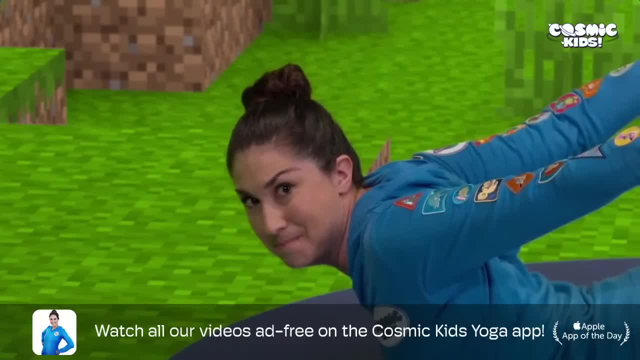 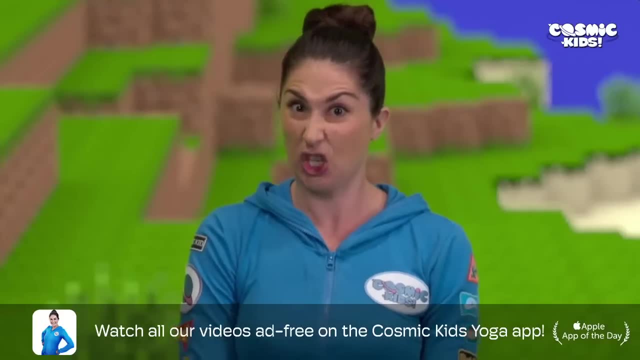 inside and we can make a mushroom stew. Coming up to sit. Now we stand up tall. We need to craft a bowl so that we can put our mushrooms inside. Coming to bed pose. We need to make ourselves a door so that we are secure at night. Let's 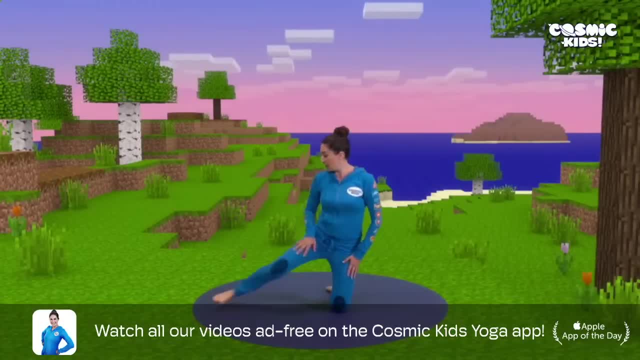 come into door, pose High up on your knees, take your leg to the side and your arm up to the sky. Let's see if it works by opening it. Very good. Now let's see if it closes Two knees together: leg to the side, arm to the sky and close it. Brilliant, That's made. 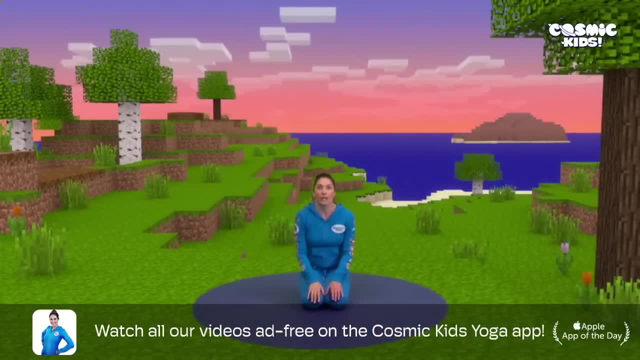 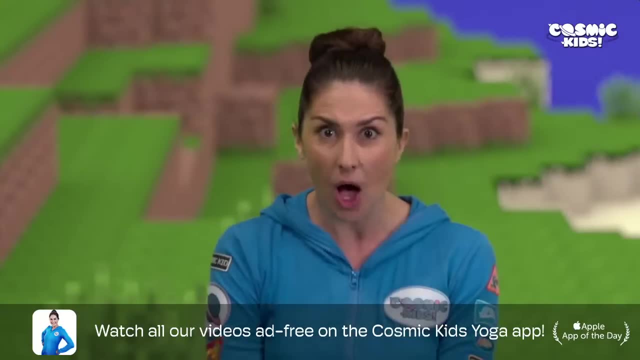 good use of our planks. Now we're inside, outside, and we see that the sky is turning from orange to pink, to purple. It's dusk. Now we're inside, we build ourselves a chest so that we can put away all the things that. 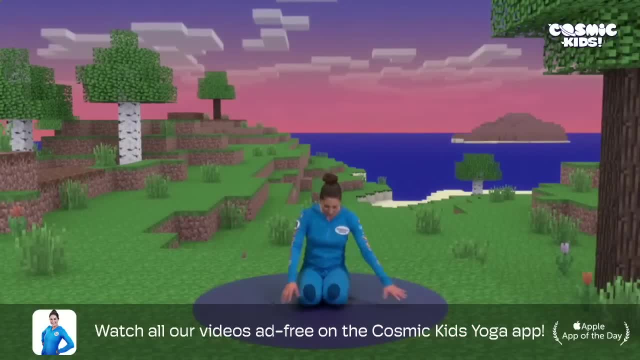 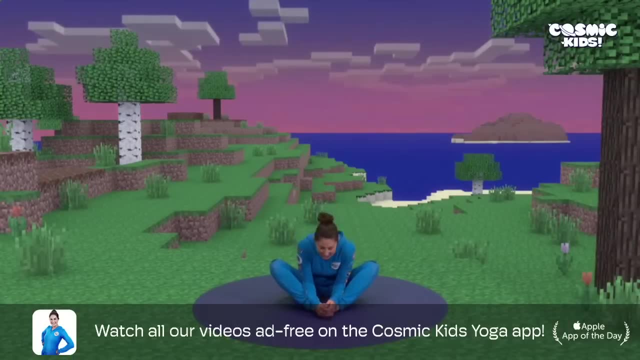 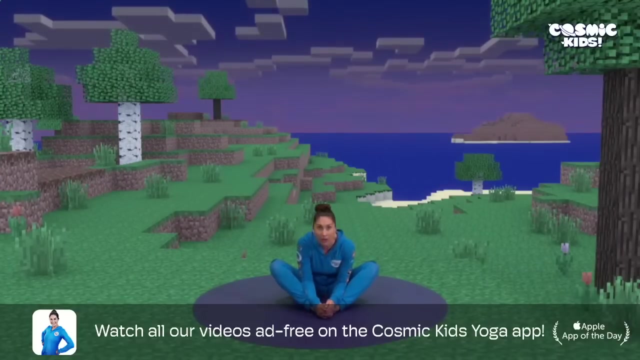 we've collected. Coming into chest pose, sitting on your bottoms, joining the soles of your feet together, holding onto your toes, and close your chest down, putting your head towards your toes. Fantastic. Now we look up because outside it's night time. This is when all 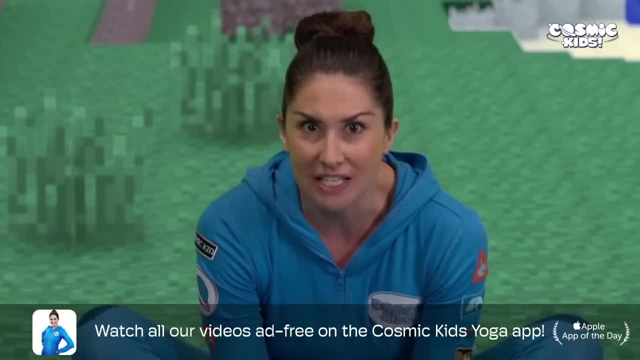 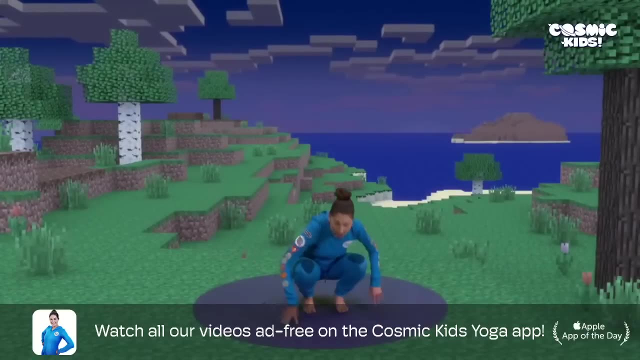 the mobs of monsters spawn. We've got to be ready for them. so let's talk about what we're going to see. There might be some creepers- Creepers- coming up to stand up on your tippy toes- everyone- because creepers like to come up to you and blow themselves up with a kaboom. 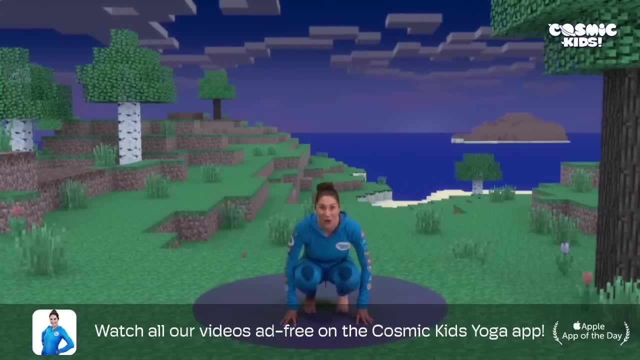 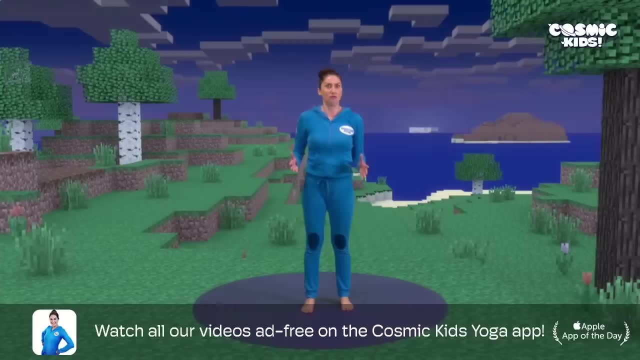 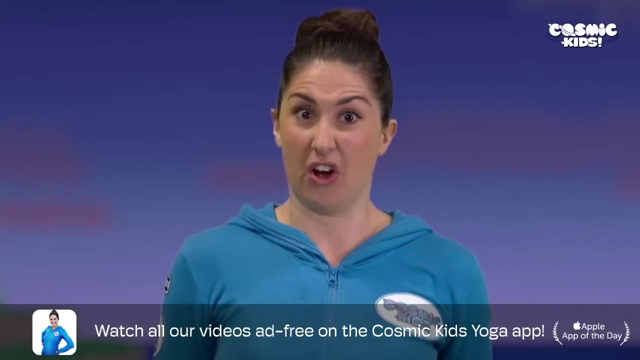 After three, let's jump and kaboom. One, two, three, Kaboom, We stand up. If we see one of these, we need to run away, Run Now. there are also zombies that come out at night, Coming to stand to the side, roll all. 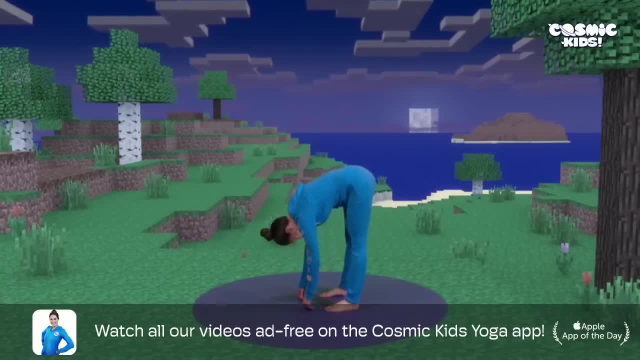 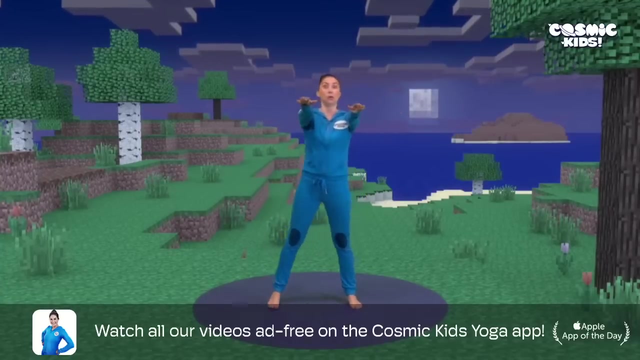 the way forwards and slowly roll yourself up to stand And bring your arms up in front of you, Turn to the front And, like a zombie, tilt from side to side. ooooh, Zombies have lots of friends and they often bring them with them, so we need to hide like little mice if we see the zombies Coming. 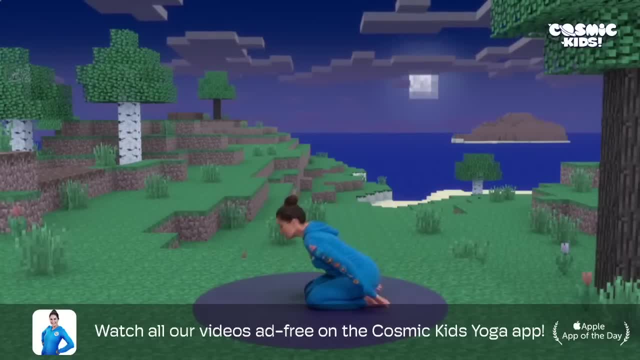 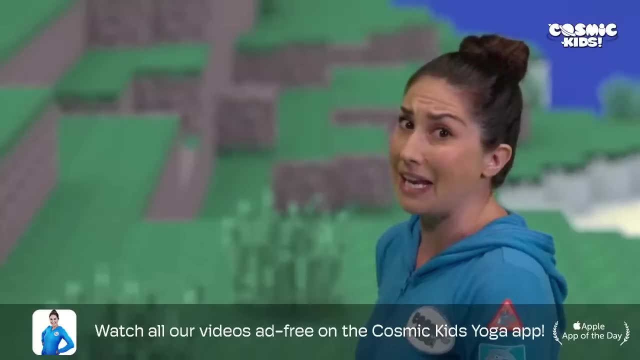 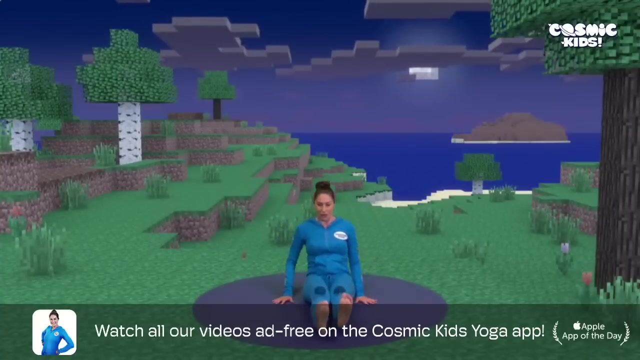 into mouse pose on your knees. Tuck yourself up into a tiny little ball. Coming up to sit again Now, there might often be some skeletons around and they have bows and arrows. Let's come into archer pose, Sitting with your legs out long. Take two fingers and put them. 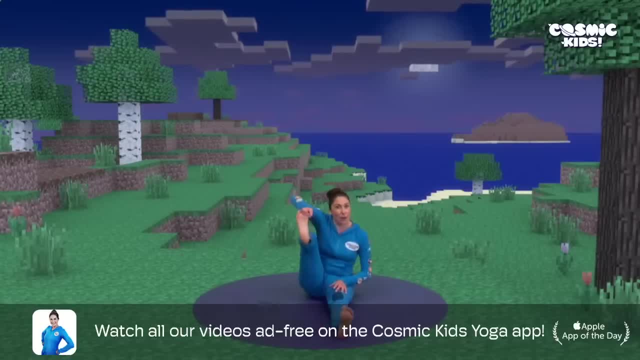 between your big toe and your second toe. Bring your elbow back towards your ear and see if you can reach forward to your other foot and fire your arrow Ready: One, two, three Pew. We better be careful. We don't want to meet any skeletons. There are also. 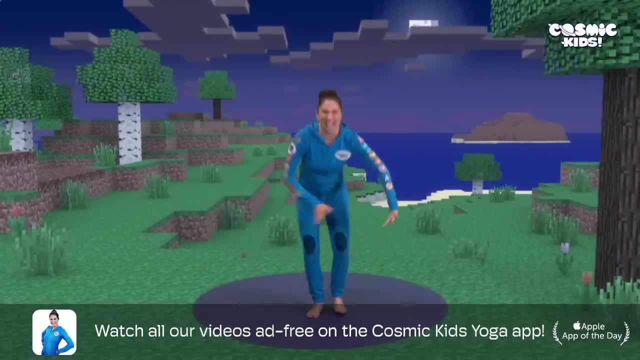 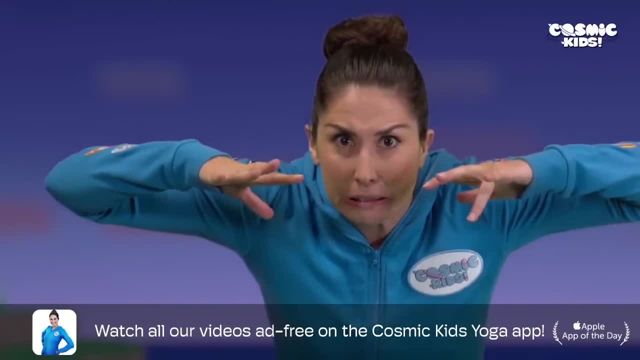 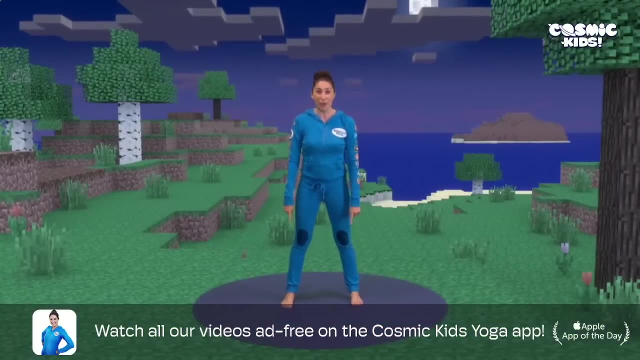 like to cast spells and use magic. Whew, And there are spiders. Let's come into spider pose, Standing with your feet just a little bit wider, bend your knees and bring your hands down in between your feet. Now ticka, ticka, ticka, ticka. 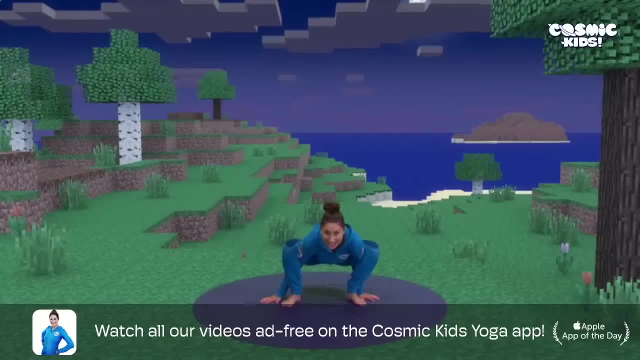 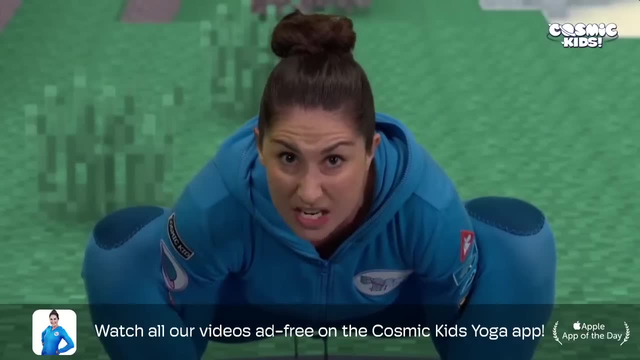 your hands round to the outside and rest your feet, your legs, over the top of your arms in spider pose. Now, spiders like to come in from above. Oh no, Look, One's coming in, but there's a skeleton and he's shooting it with his bow and arrow. 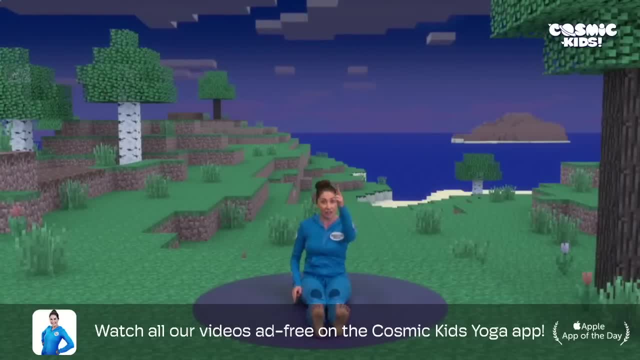 sitting on your bottoms, legs out long. take your other two fingers between your big toe and your second toe and bring your elbow back. then reach forwards and grab your other foot and watch the skeleton fire its arrow to the spider. one, two, three pew. 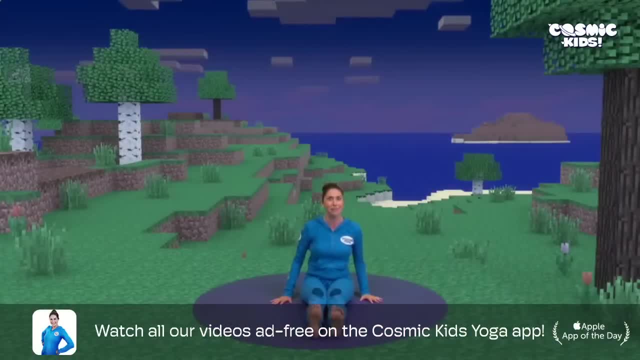 the spider keels over into happy baby pose, lying on your backs, everyone holding onto your feet in happy baby pose. well, this is good news. this means we've collected some string, sitting up tall crossing your legs. let's roll the string up in front of us. 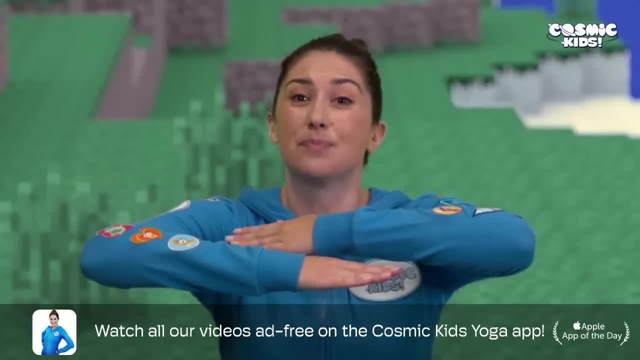 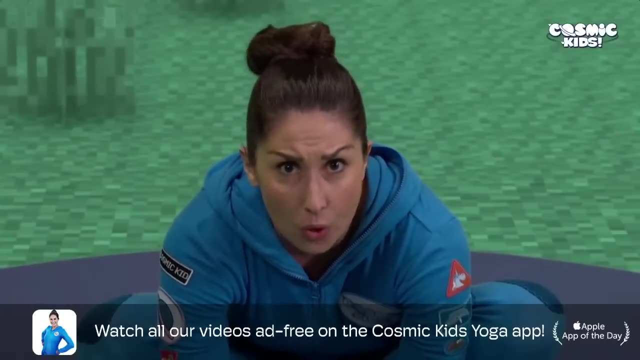 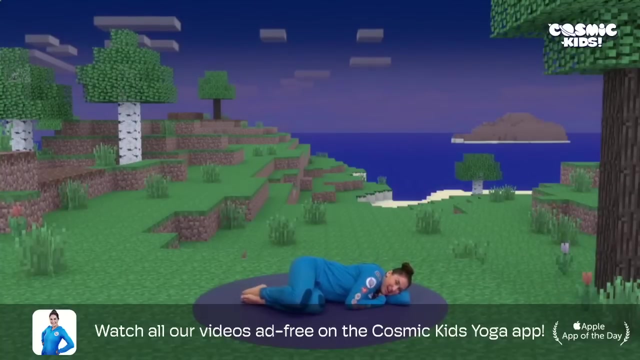 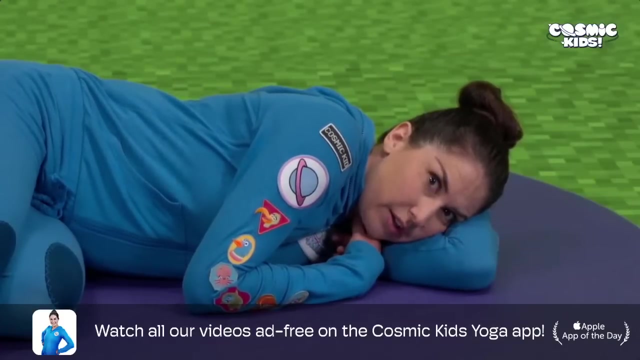 and let's put it in our chest. now we need to go to sleep so that we don't have any more danger tonight. so we huddle ourselves down in our bed into a comfy position- ah, in our lovely beds- and we feel safe. ah, in the morning we wake up and it's raining. 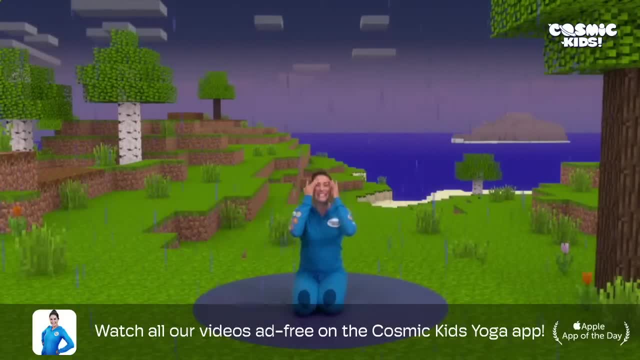 coming up to sit on your knees. pitter patter on your faces and on your heads. oh, my goodness me. this is exciting. it's daylight again, so we're safe. so we decide to build a boat. we're going to go fishing today, sitting on your bottoms. lift up one foot. 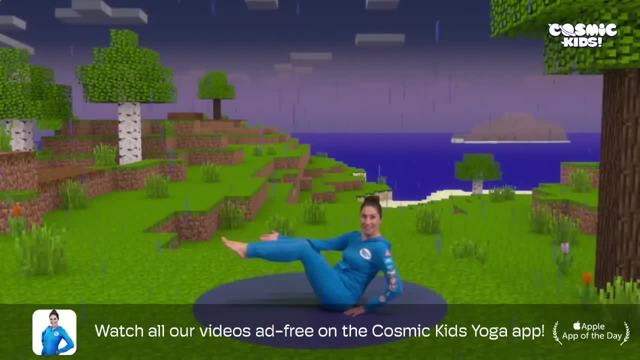 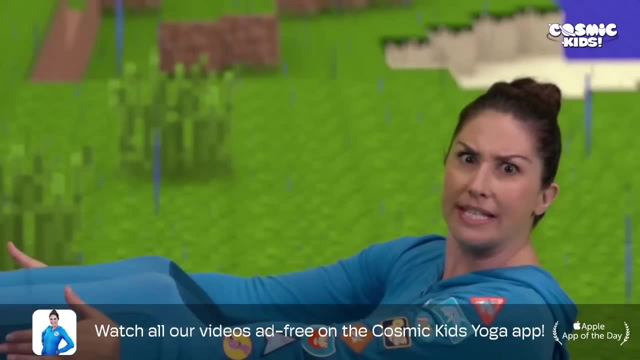 lift up two. lift up one hand. lift up no hands. yay, in boat pose. give me a wave. yay, now who's this coming to see us? it's our friend stampy cat coming into cat pose. everyone on all fours fingers spread wide, tuck your toes, arch your back up. 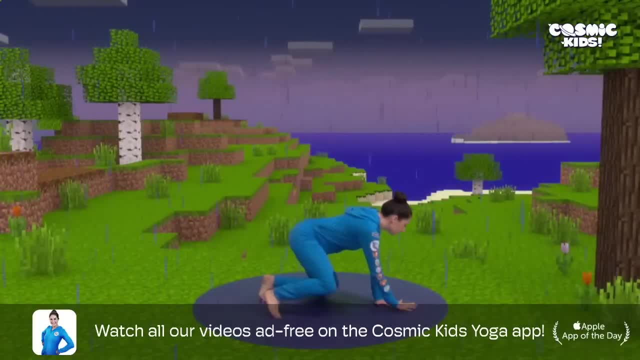 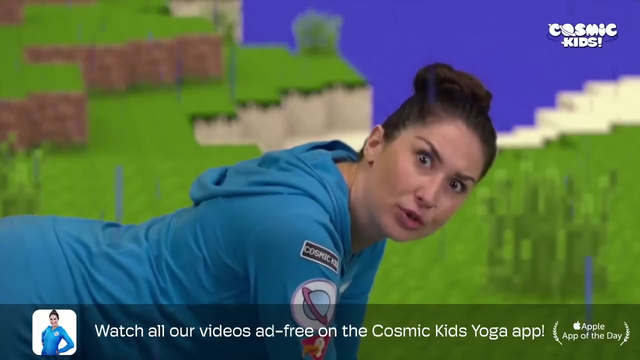 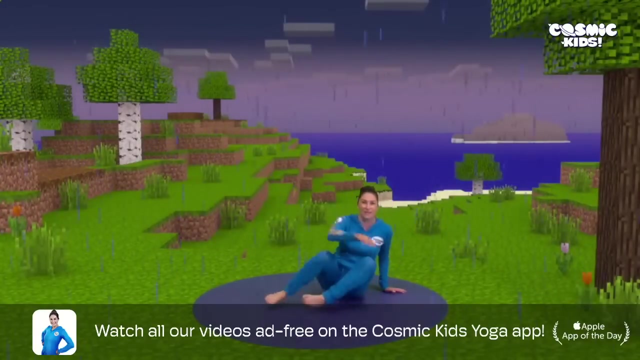 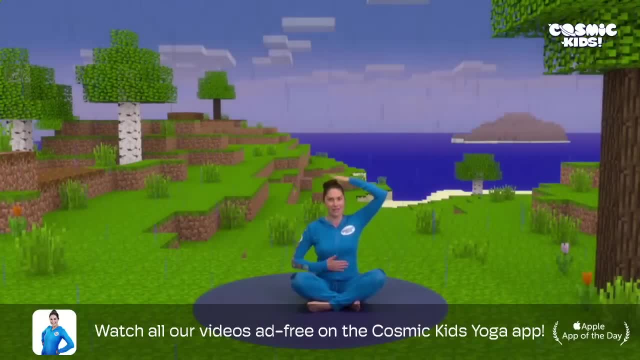 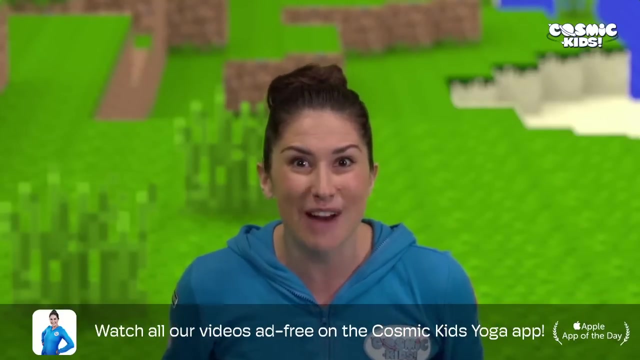 who can't swim. what's so funny? what's so funny, what's so beautiful? what a sad. what an odd, but so sad, really cute, so cute, so helpless, unbig, watchful. maybe the animal does it. what's theieren которая sky? let's come into rainbow. pose high up on your knees, everyone, take your arms wide and drop down. 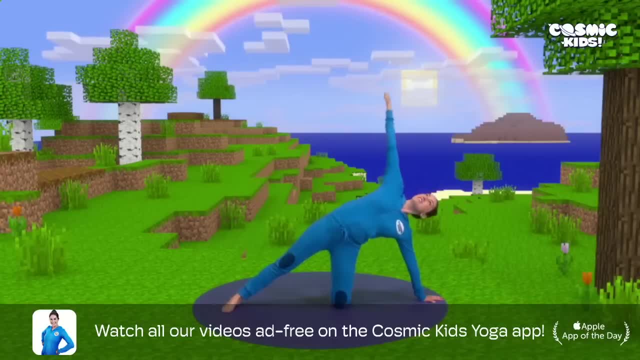 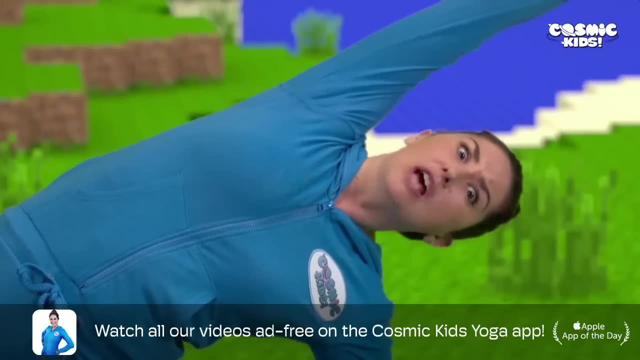 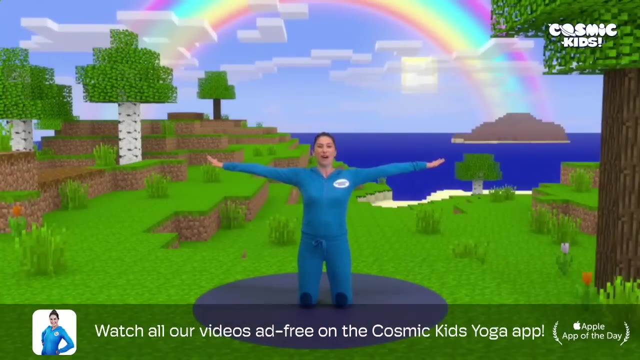 onto one side, stretch your leg out and reach your arm up and over your ear, coming into your beautiful rainbow pose. now we sit with stampy and he knows an awful lot about minecraft- coming into rainbow pose the other way, two knees together, arms wide, drop down and stretch your leg out, reach your arm. 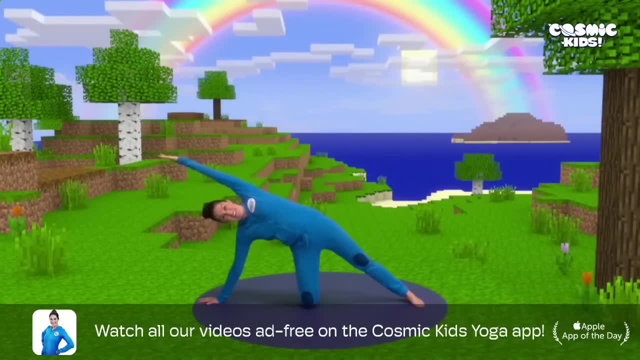 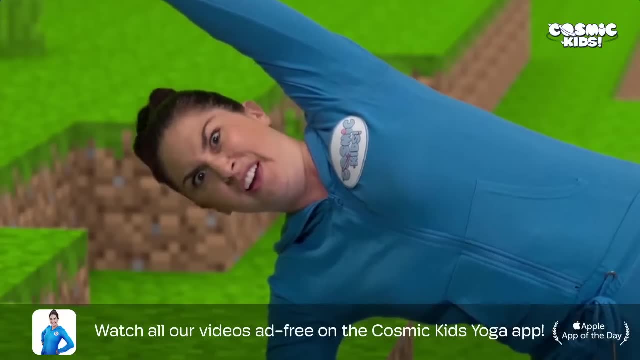 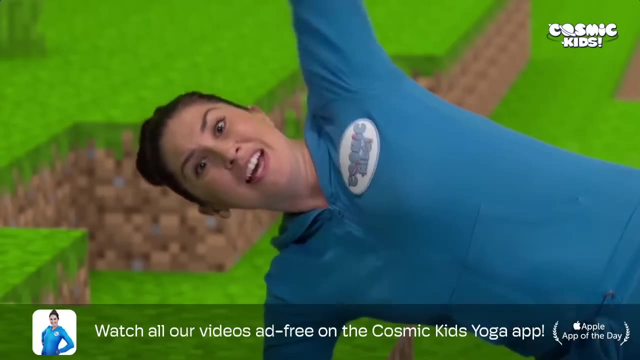 up and over your ear coming into a full rainbow. very good, everyone we wonder whether stampy could ever craft a yoga class into minecraft's world. that would be funny, wouldn't it, if you were playing minecraft and you came across a yoga class. along comes a horse coming into horse pose high up on 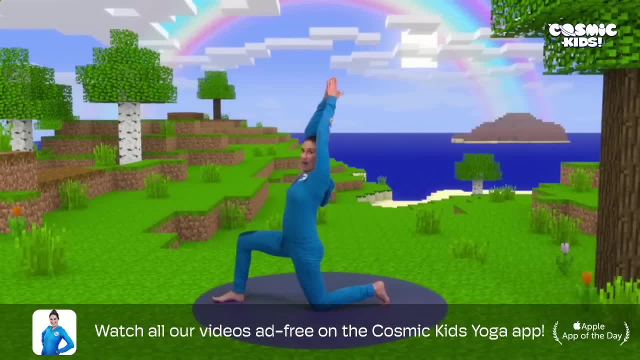 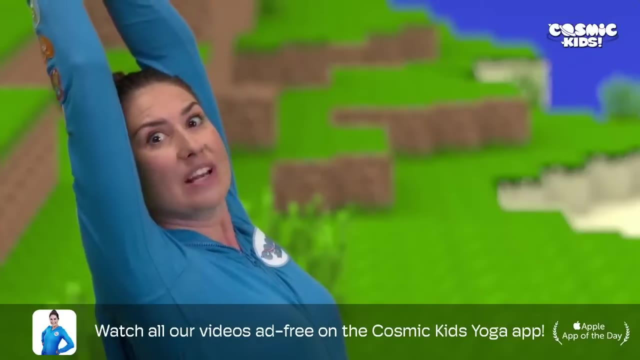 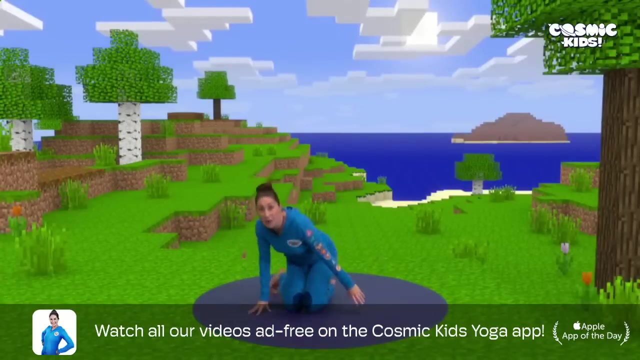 your knees, step one knee forward and lift your arms up, then fold forwards and lift your chest as you go, stampy, sad up. he lifts himself up, turns himself round, drops down onto the other knee, as he says, and off he trots. very good everyone. now we better get in our boat so that we can get some fish. 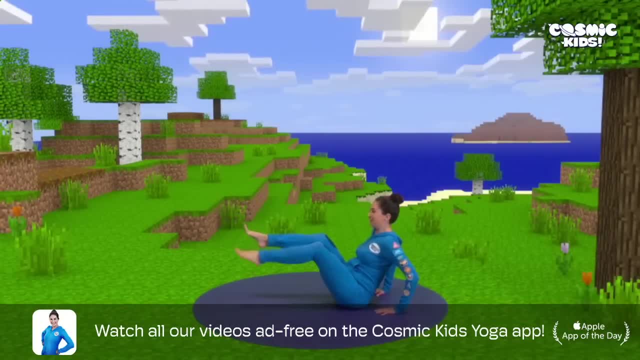 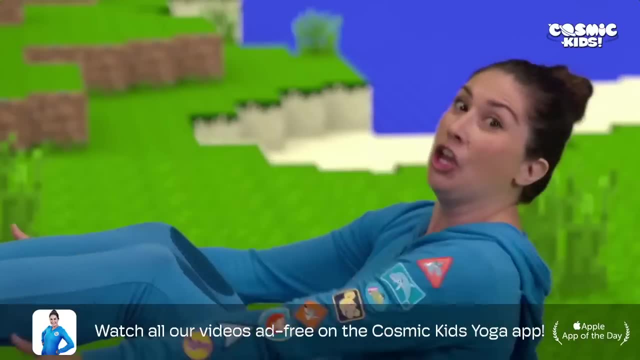 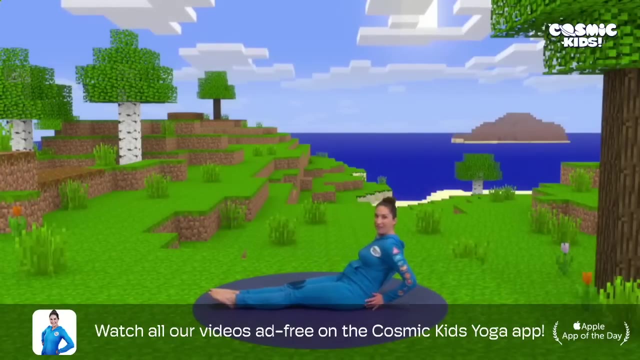 sitting in your boat pose, lifting up one leg, lifting up two, lifting up one hand, lifting up no hands. and give me a wave: yay. using the string from our spider, we catch a fish. point your toes down and drop down onto your elbows. now pop, pop, pop, pop, pop your chest to the sky. 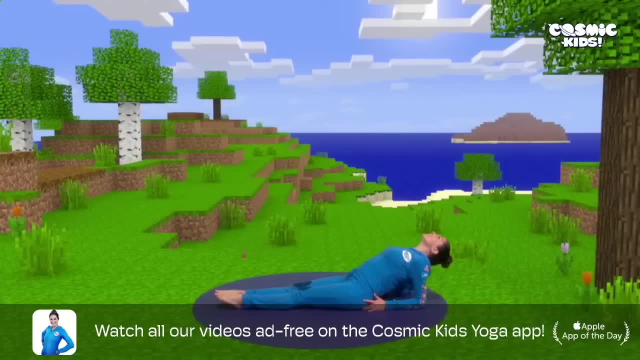 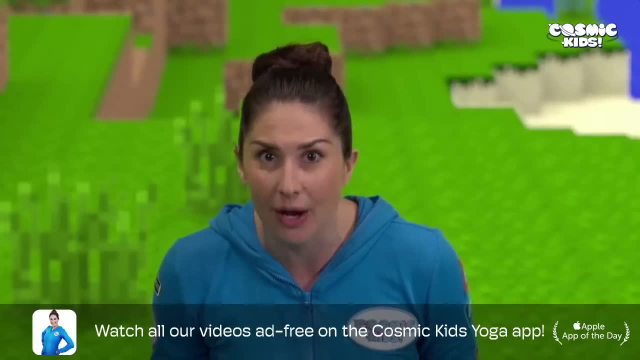 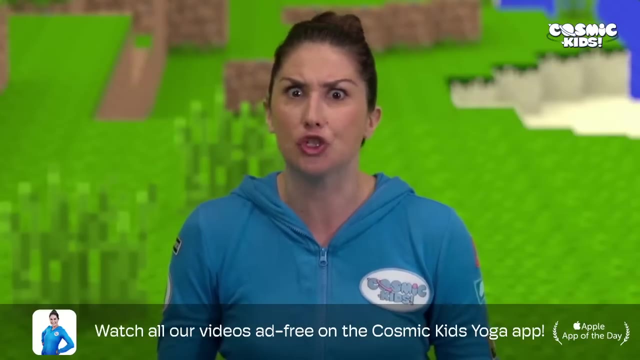 and look up to the ceiling or the sky above you, like a fish. yay, we sit up tall. this is great news. we've got a fish for our supper. now, back on the land, we find we're being followed by a pack of wolves. let's come into dog pose on your hands and knees, spread your fingers wide, tuck your toes in. 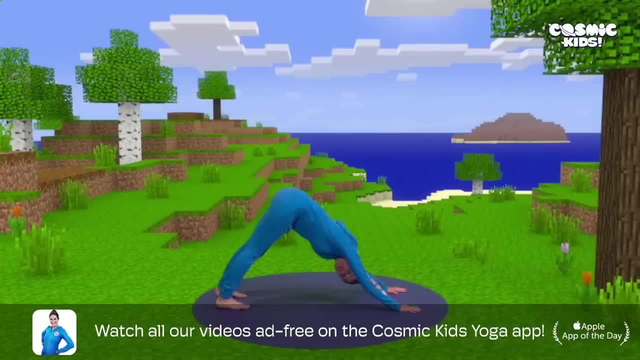 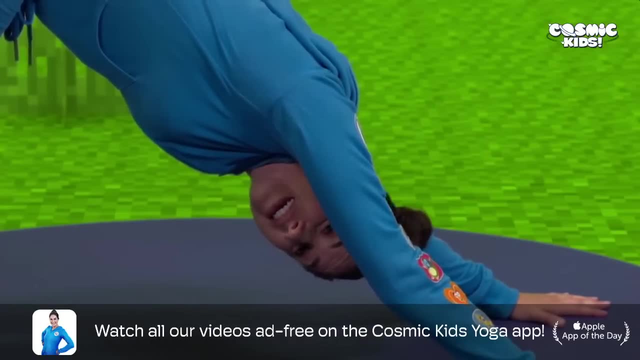 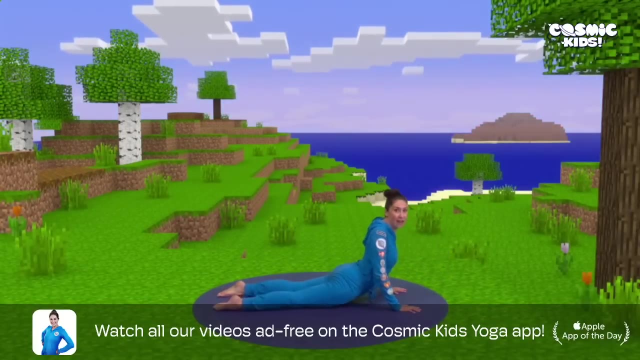 your toes and lift your bottom up to the sky, coming into your dog pose. now the wolves are our friends and they howl at the skeletons to scare them away coming all the way forward. come down onto your belly, untuck your toes and then peel your shoulders up off the ground and see if you can make your. 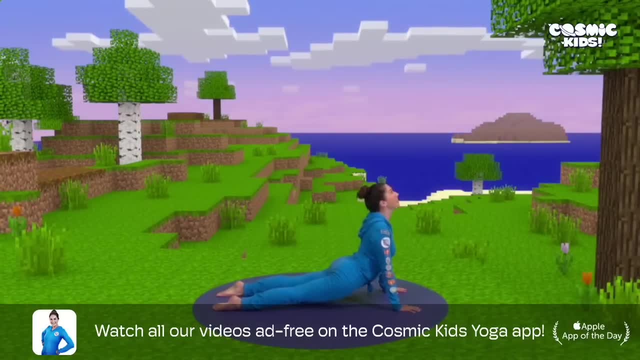 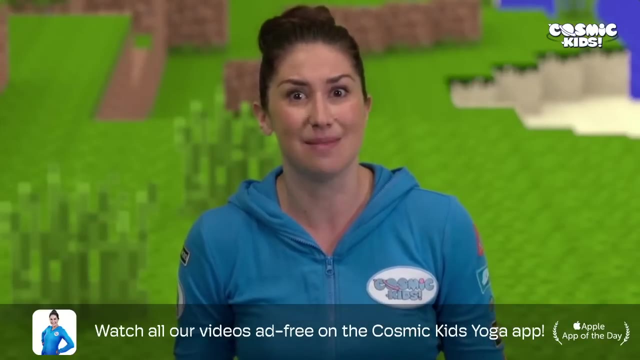 legs really strong and lift them up too, and then look up to the sky and howl: oh, thank you, wolves. we get back to our shelter where, after eating our fish supper, we're ready to have another sleep. we've survived our first two days and nights here in minecraft and we feel very proud of ourselves. 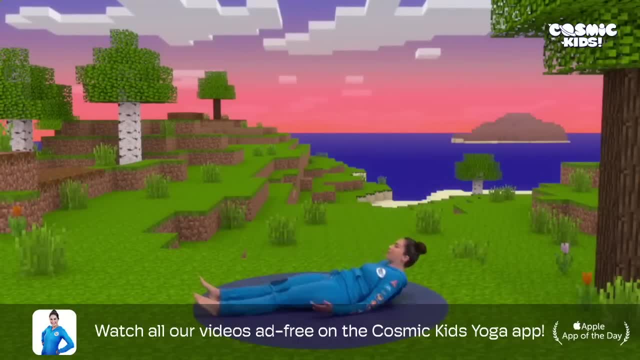 so we lie ourselves down our legs and arms long and we come to rest. what an adventure that was. it's been amazing here in minecraft world. it makes us understand how things are made when you look around you at all the natural things in the world and how you put them together to make the tools and the things that you need. 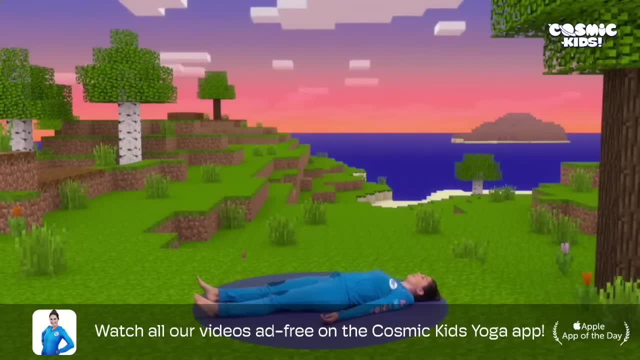 it makes us realize that we don't need very much a house- warmth, friendship, food and water- and it makes us feel really grateful for the other stuff that we have in real life. maybe when we look around now we can understand how those things were made, the work that went into them, and we can feel very grateful. 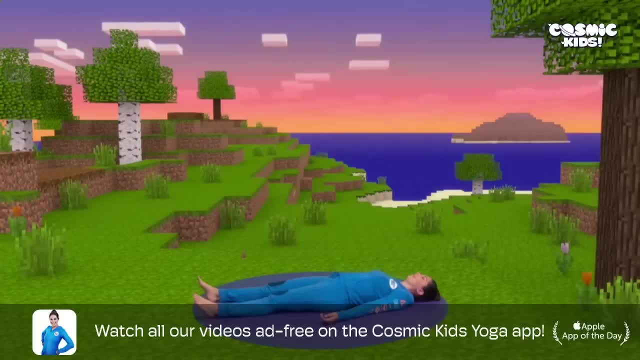 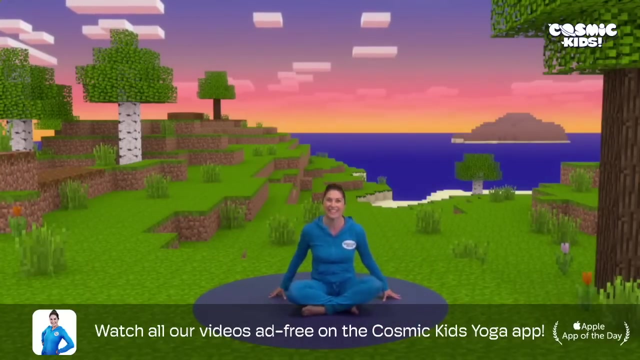 very grateful for all that we have, and now it's time to wake up. so we wiggle up our fingers and our toes, we bring our knees into our chest and we roll over onto our side, opening our eyes, coming up to sit with our legs crossed and our hands together at our hearts, just like we started. 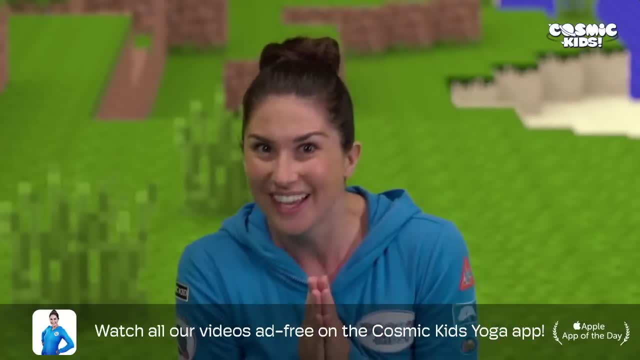 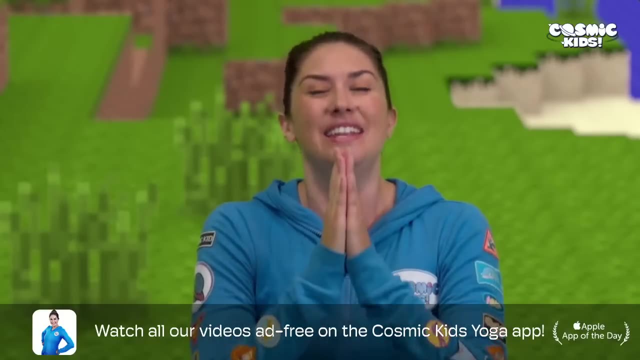 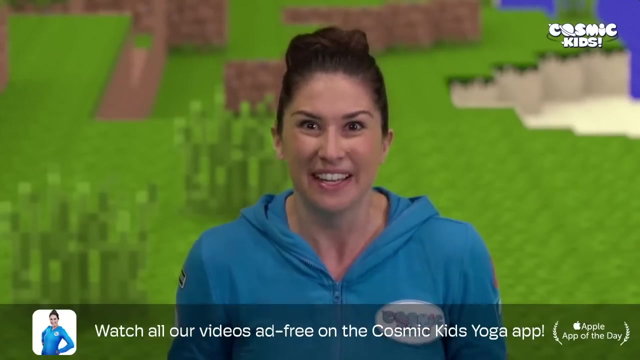 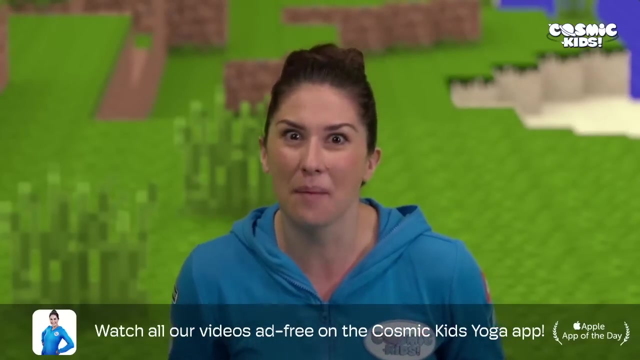 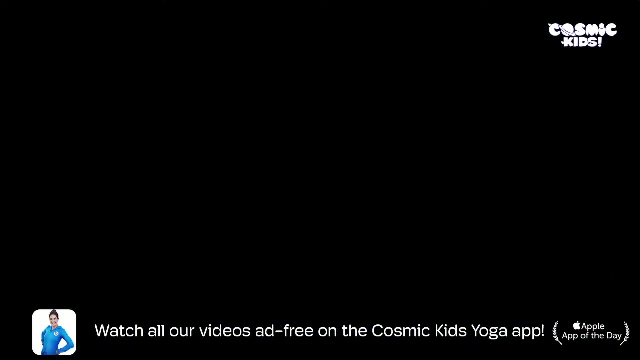 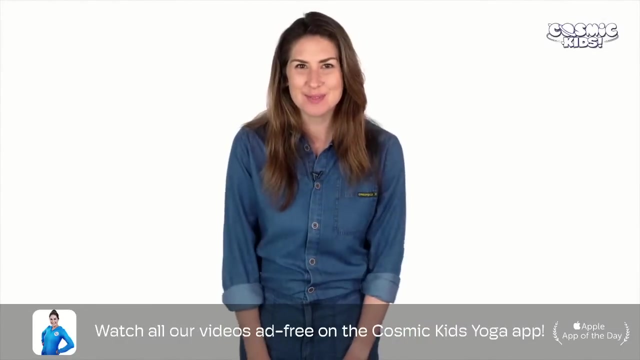 and we finish with our secret yoga code word, which is namaste, ready after three, one, two, three, namaste. now we can everyone. we are safe and sound. namaste, namaste, namaste, namaste, namaste. well done everyone. that was awesome. thanks for coming to minecraft world with me and helping me survive my first couple of nights. you were amazing. i hope you cum back soon for another cosmic kids adventure. bye-bye. 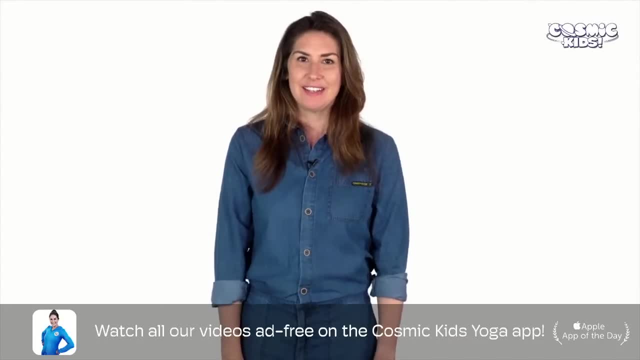 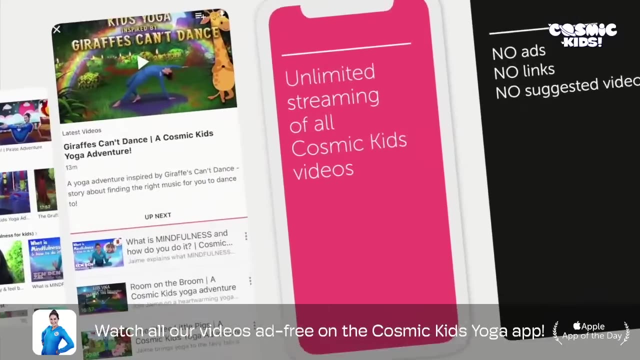 app the safest place to view our videos. This is basically our very own walled garden. It gives you unlimited streaming of all our videos and we make sure there are no ads, no funny links and no suggested videos. To sign up head to. 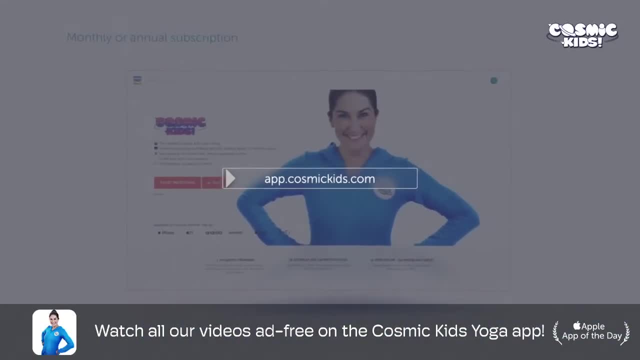 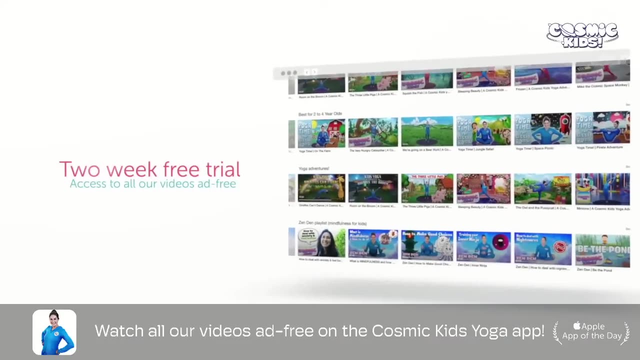 appcosmickidscom. pick a monthly or an annual subscription and then you get a two-week free trial to see if you like it. Every single video we've ever made is on there, and all our new and future videos too. We organize all our videos. 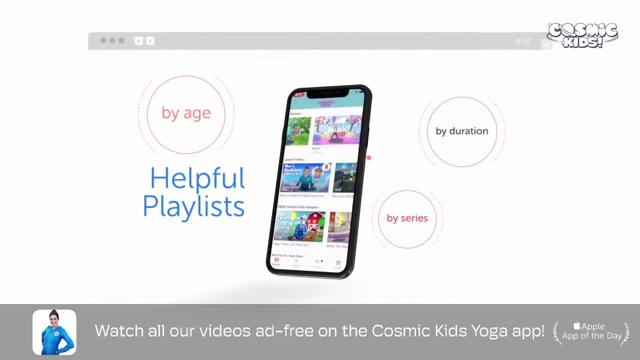 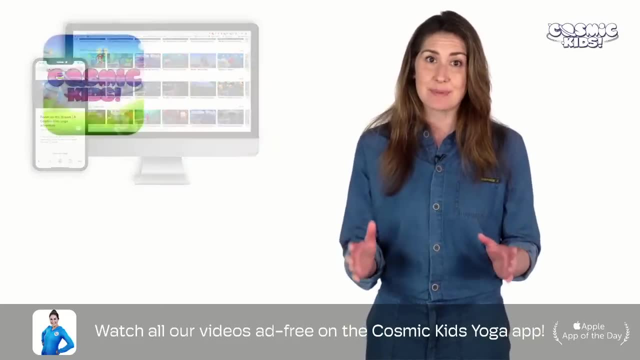 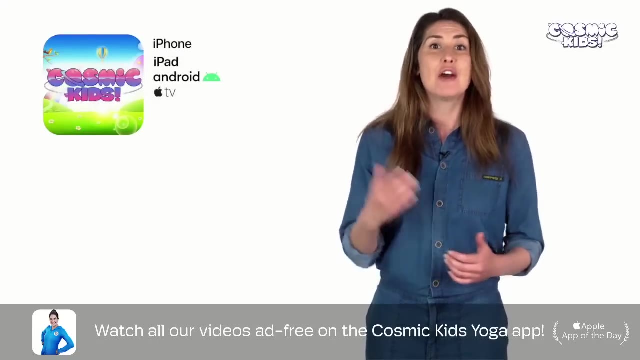 into helpful playlists, making it super easy to find your way around. You can watch it on your computer or phone using your web browser or by downloading any of the apps which are included in your subscription, and we have these apps for iPhone, iPad, Android, Apple TV, Roku and Amazon Fire TV. You can view the videos. 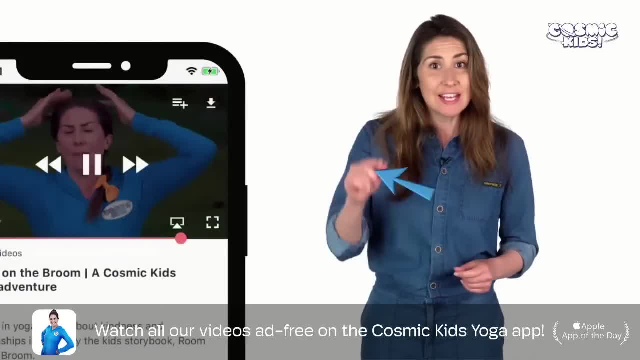 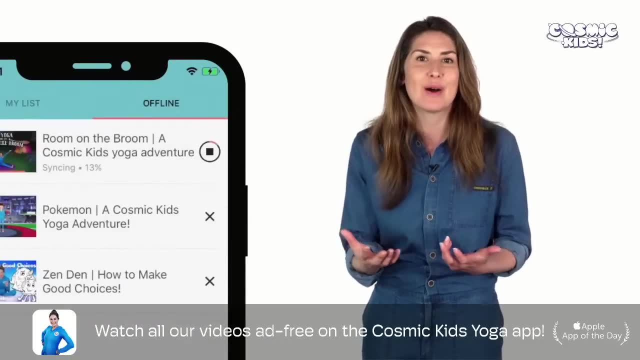 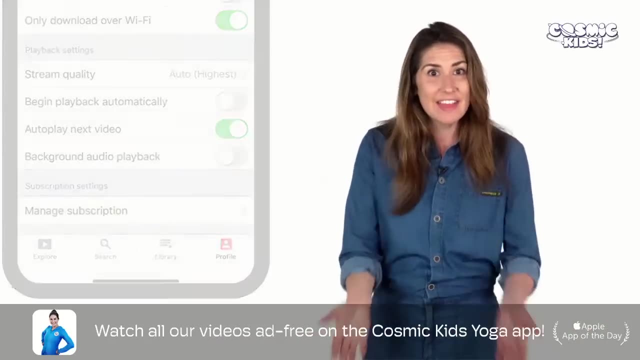 offline on phones and tablets. Just click to download the video to your watch later playlist and watch it whenever you want. This is perfect if you want the peace of mind that your kids aren't connected to the internet. You can also autoplay your favorite videos back-to-back: Just set the. 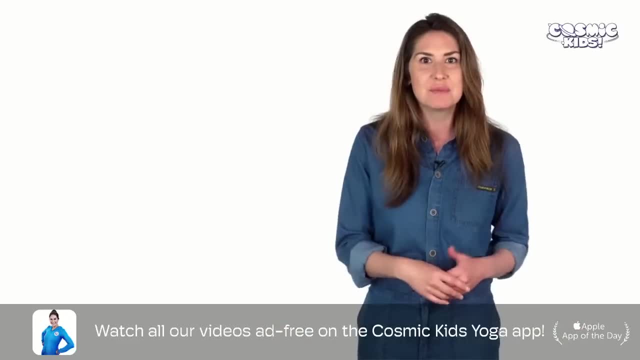 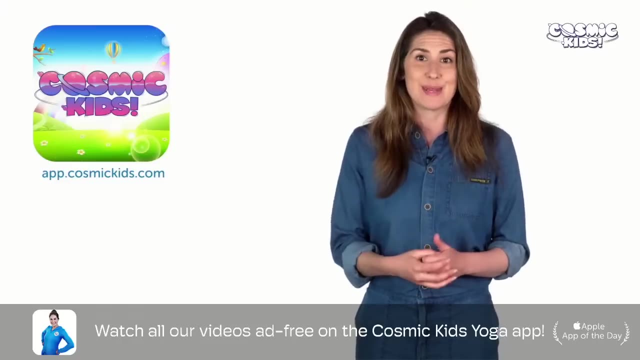 kids up with a marathon Cosmic Kids session and you can leave them to it. I hope that you love what we're doing with Cosmic Kids and this has helped you understand a little more about the Cosmic Kids app. It is the safest place to view our content and the best way to support. 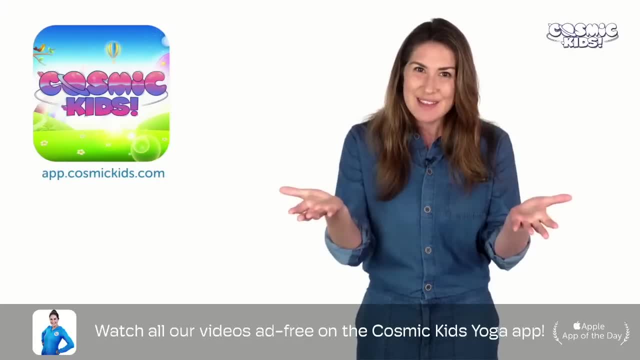 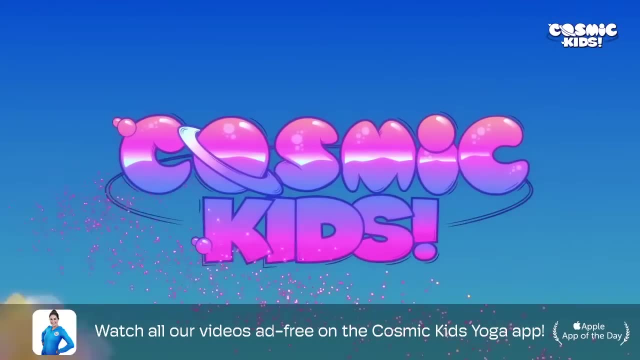 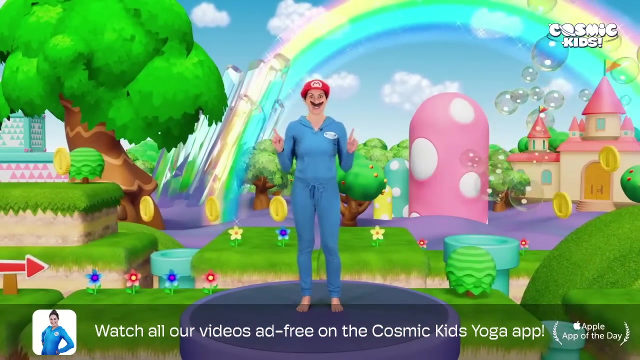 us too, Wishing you all the best from the team here at Cosmic Kids. Bye, bye, Hello everyone. Welcome to Cosmic Kids. I'm Jamie and this is your place for yoga stories and fun. It's easy: Just copy the moves I do and enjoy the adventure Now. 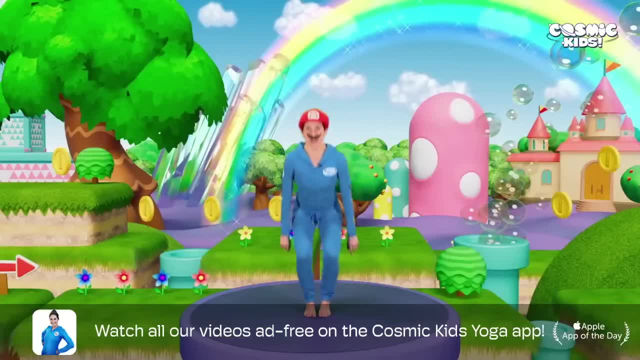 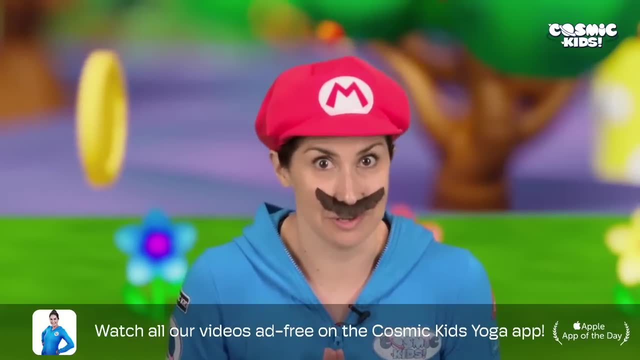 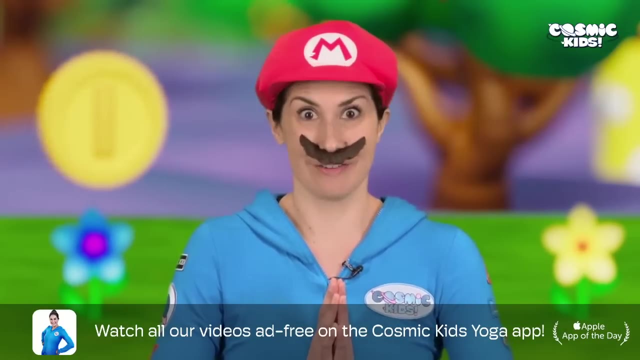 we always start in the same way, and that's by sitting on our bottoms, crossing our legs and bringing our hands together at our hearts and saying our secret yoga code word, which is namaste, Ready After three, One, two, three, Namaste. There, Now we're ready to. 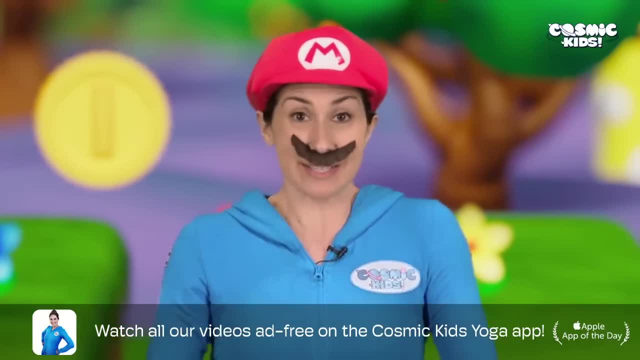 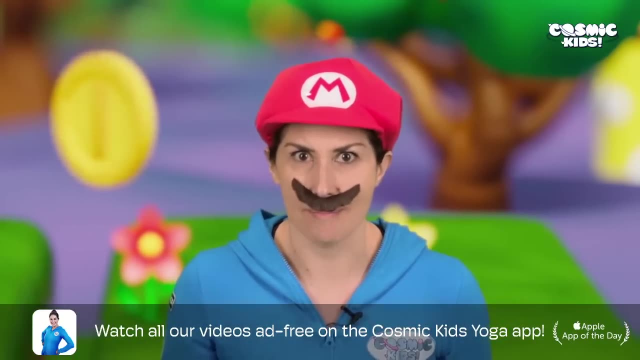 begin, and today we've got a special adventure based on Super Mario, which is why I'm wearing my red cap and my moustache. Let's begin with a Mario pose. We come up, we go up and then we go down. We walk up and then we go down. This is a 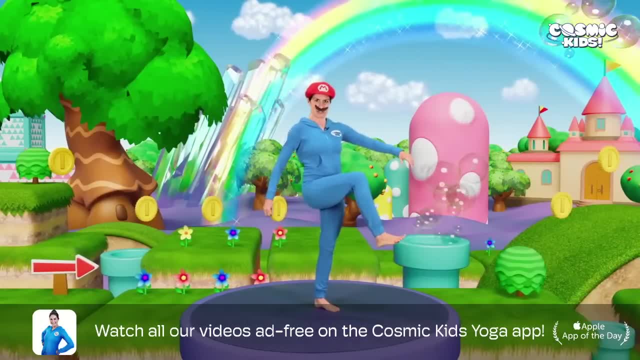 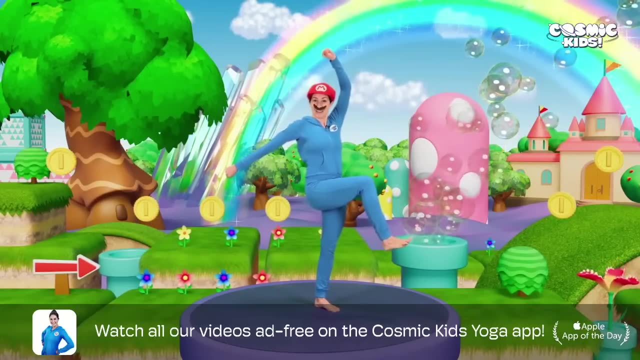 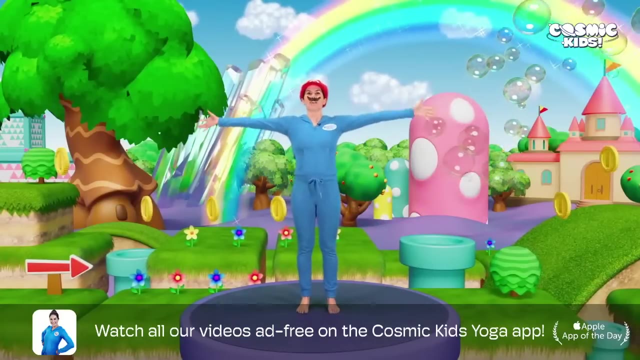 up to stand and we take one leg up in front of us. we take our arm up over our head, our other arm behind, and we say, wahoo, very good everyone. now Mario lives in the mushroom kingdom with his brother, Luigi. let's stand tall, take our arms wide and give Luigi a big hug, wrapping him up. let's. 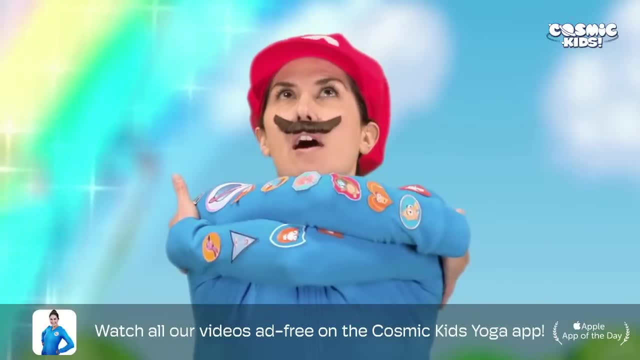 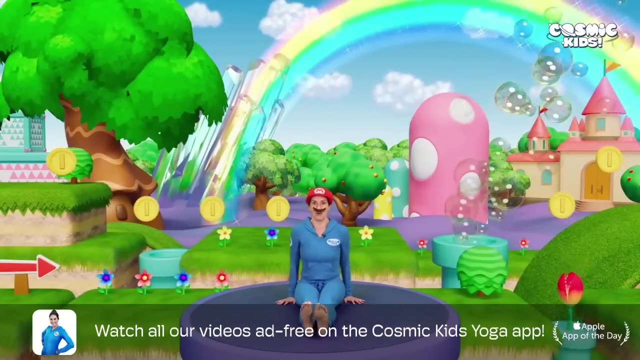 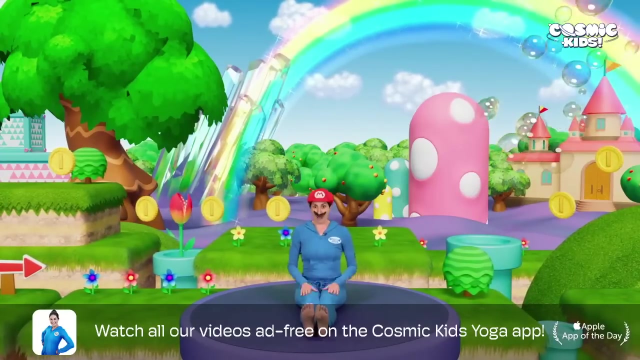 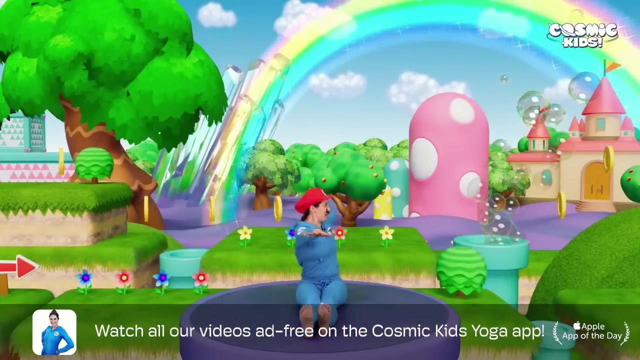 go, Luigi. now. Mario and Luigi love to eat pizza, so let's make one. we sit down on our bottoms and take our legs out long. now we need to lay out the base. let's pat it down. now it needs some tomato sauce, so let's take our arms out wide, we twist all the way around to one side and we get our tomato. 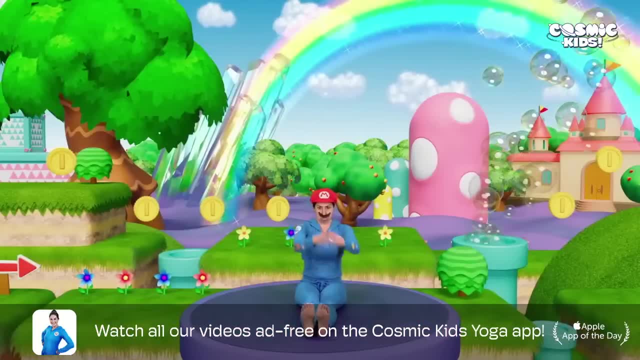 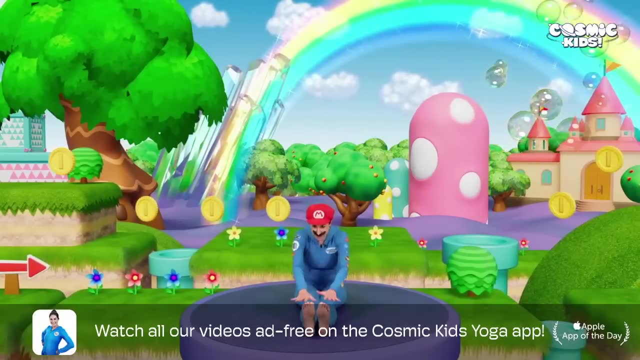 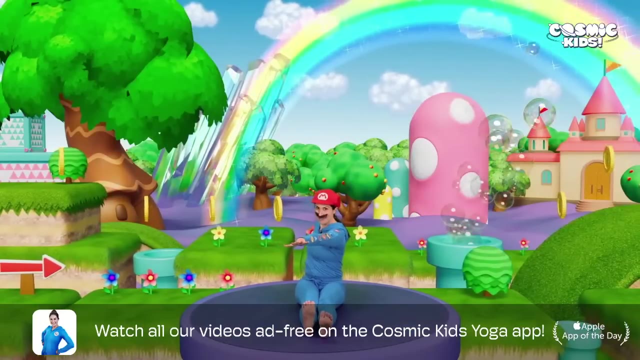 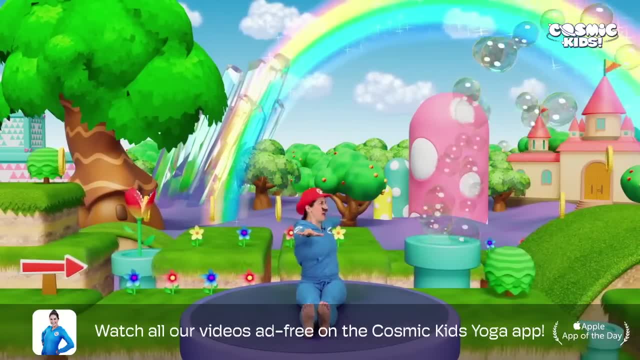 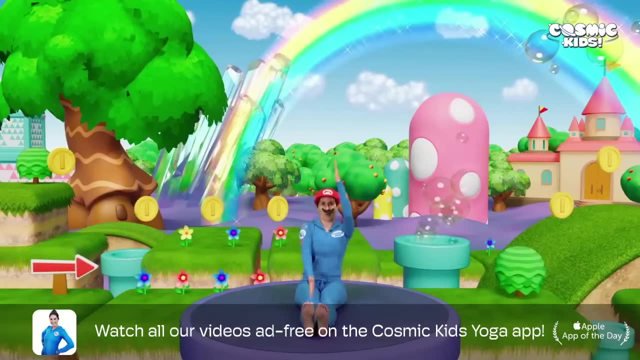 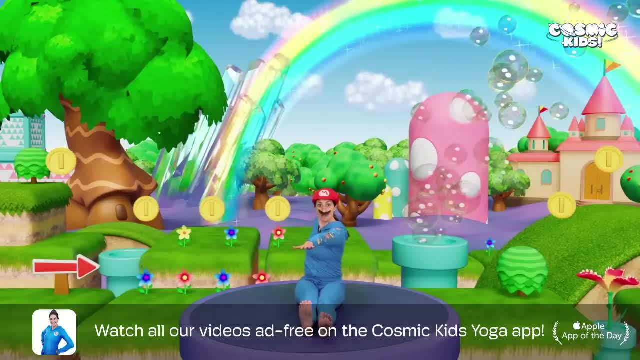 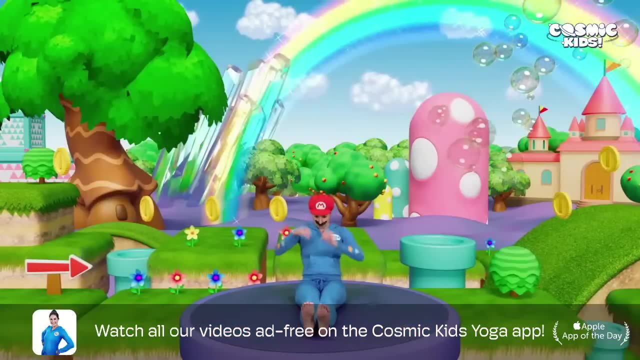 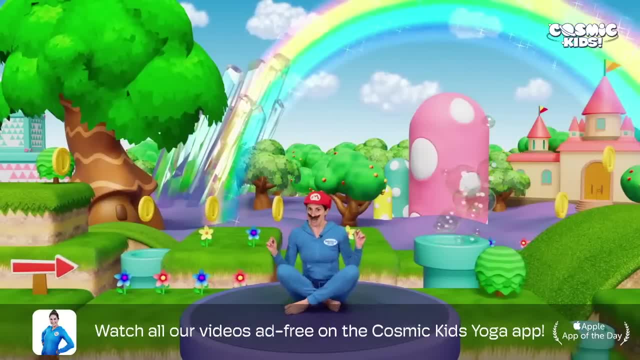 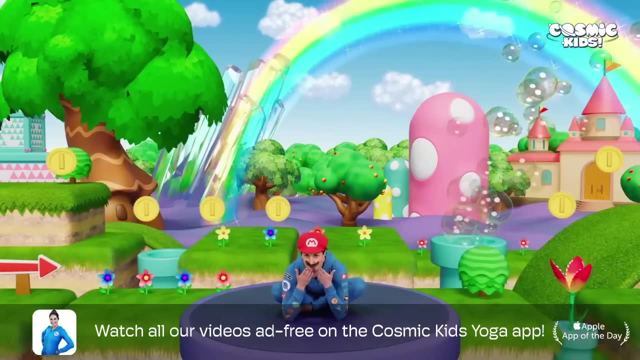 Oh delicious. Now it cooks, And after it's ready, we cross our legs, We fold all the way forwards onto our elbows and we gobble it all up. Mmm, ooh, hoo-hoo, That was delicious. 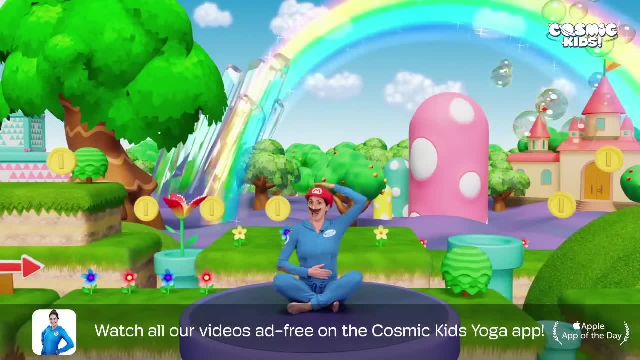 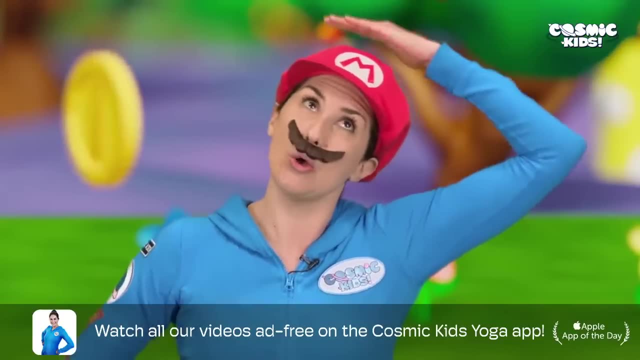 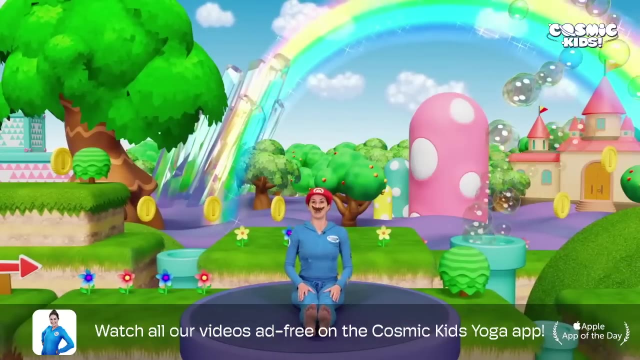 We rub our hand on our tummy and we pat our heads at the same time. Now Mario and Luigi have lots of friends in the Mushroom Kingdom: There's Toad and Toadette, Oh, and Princess Peach. Let's do our Princess Peach pose, Taking our legs out long. we swish them round one way. 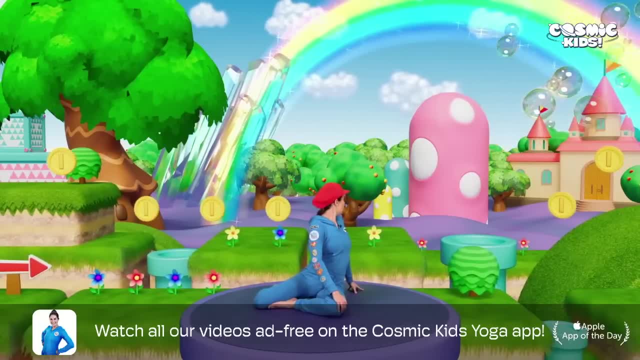 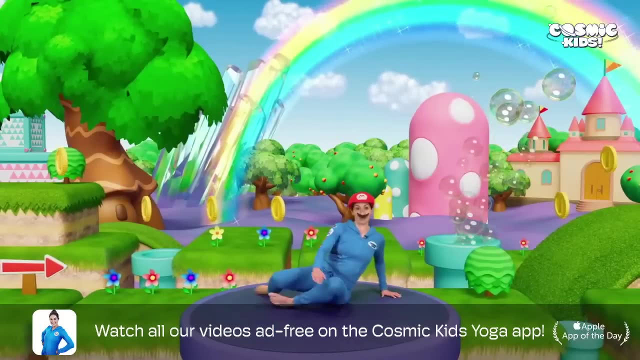 We bring one hand on our knee, one hand behind. We look over our shoulder, We look back to the front and we say hurrah for our hero Mario. Then we swish our legs round the other way, Take our hand onto our knee, our other hand behind. 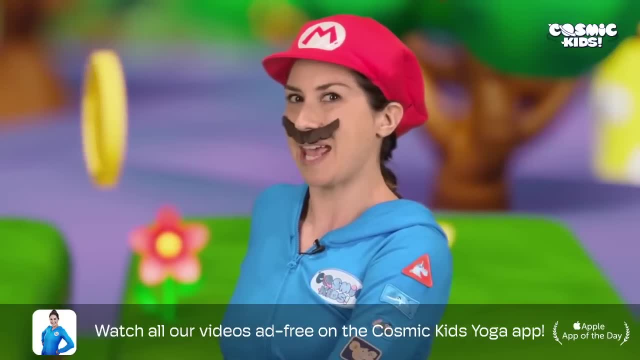 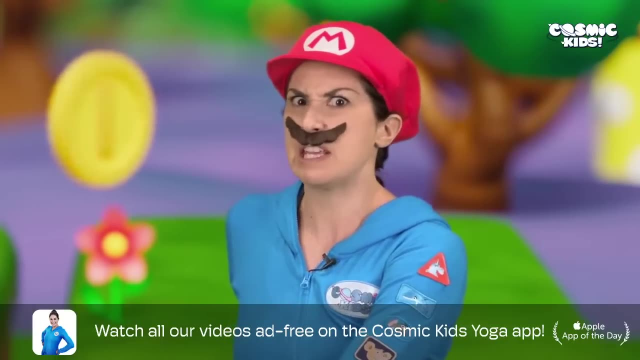 Look over our shoulder, look back to the front and we say hurrah for our hero Luigi. Now their big enemy is Bowser, a very greedy and mean turtle with spikes on his shell. Let's do our Bowser turtle pose. 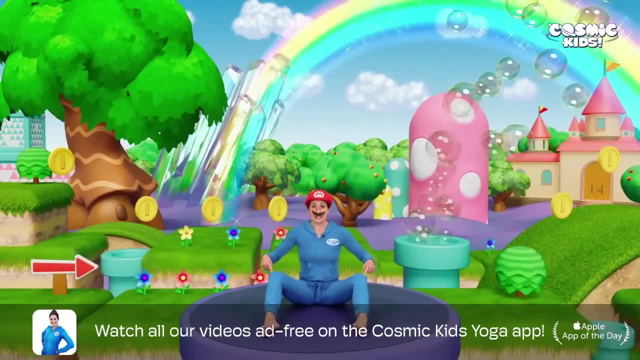 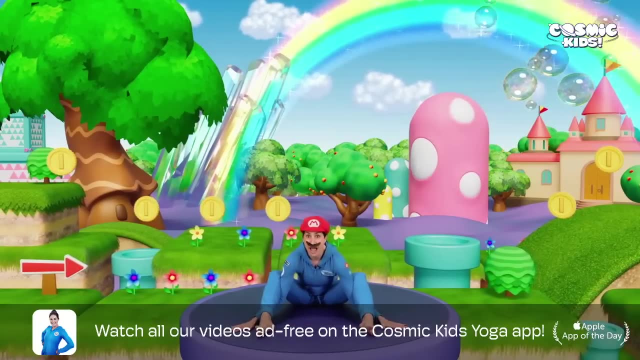 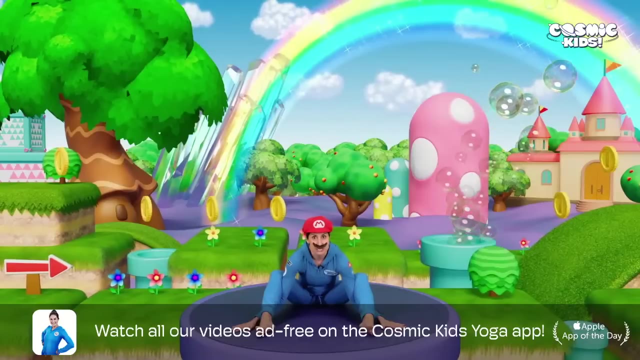 Sitting with our legs out A little bit wide and with our knees nice and bent. We bring our hands down in front of us and we slide them underneath our legs, coming into our Bowser turtle pose. All Bowser wants to do is rule over all the kingdoms, and Princess Peach keeps getting in his way. 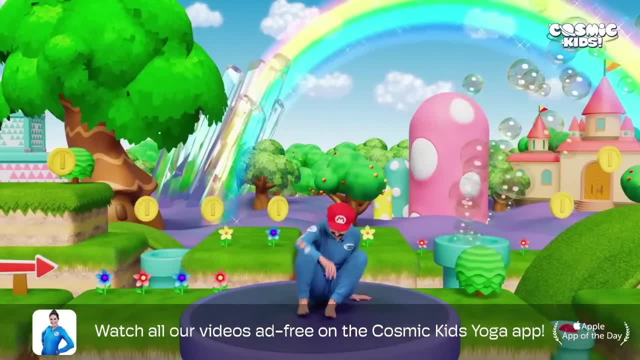 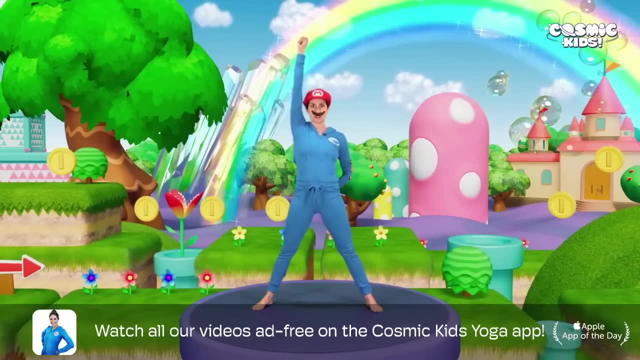 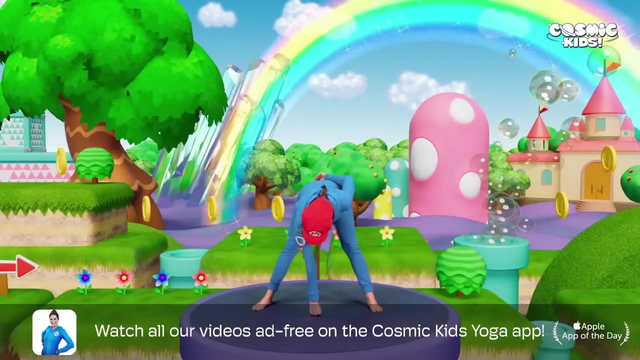 And this time he's attacked again, Coming up to stand with our legs wide, we raise our arm all the way up, making it into a fist. He's attacked Peach's castle with a giant machine arm folding all the way forwards to go. boom, rolling up to stand. 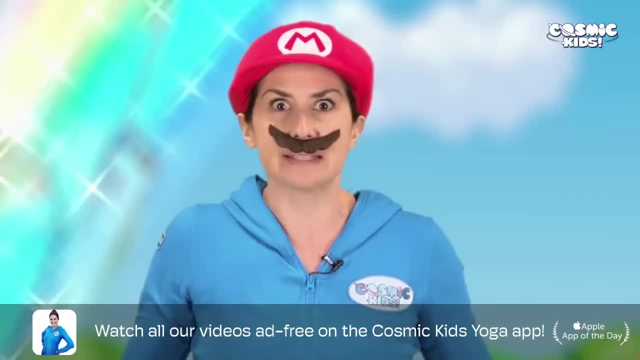 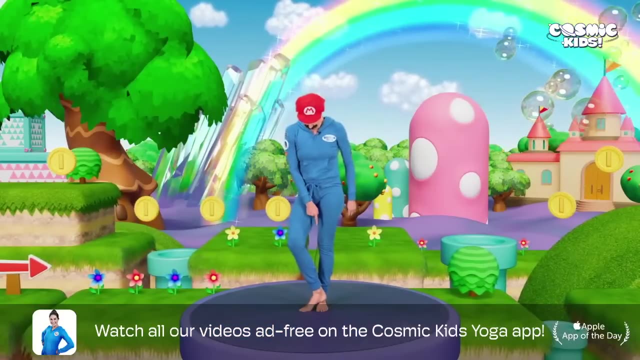 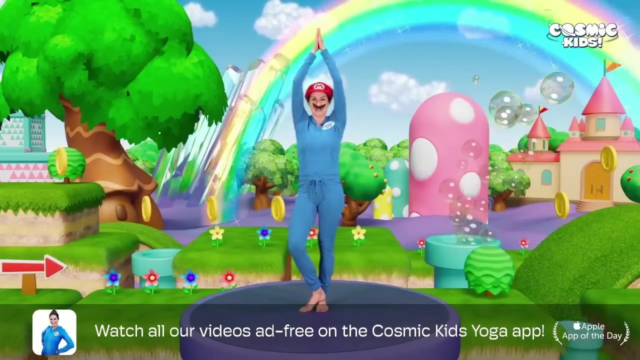 It sends Mario flying. He lands in an acorn tree. Let's do a tree pose. Standing with our feet together, we bring one foot on top of the other, using our heel and our hands together at our hearts. Now we grow, grow, grow, grow, grow up nice and tall and we open our branches wide. 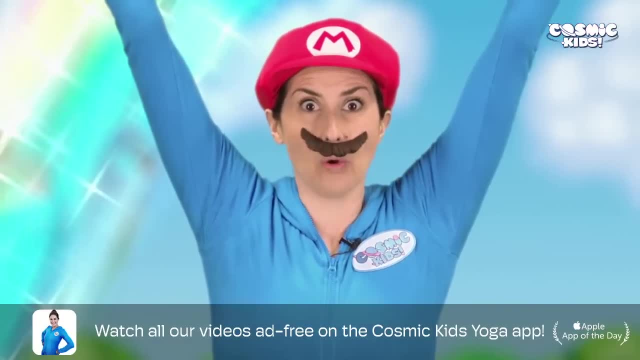 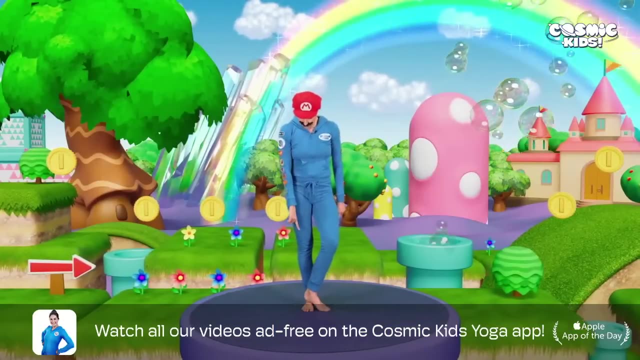 Wow, He's so far away in the acorn plains. Let's see if we can do our tree pose on the other side, Bringing our feet back together, putting our other foot on top now, using our heel hands together. we grow, grow, grow up nice and tall. 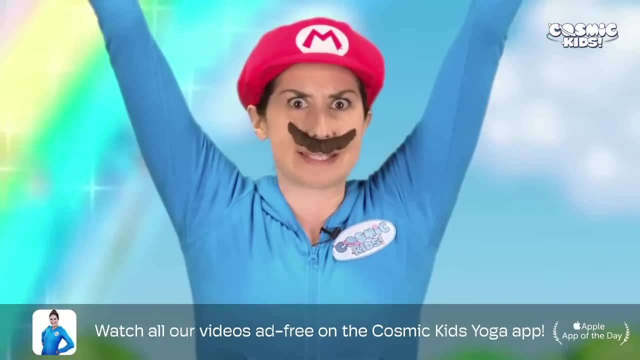 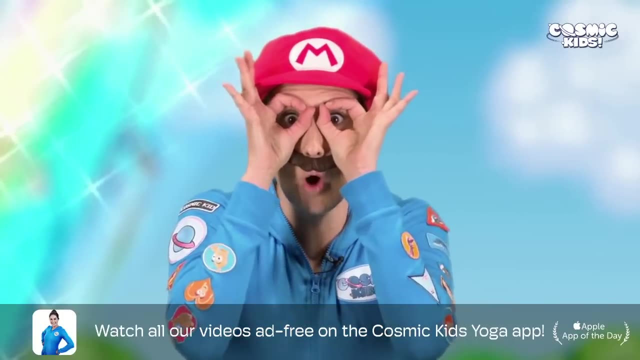 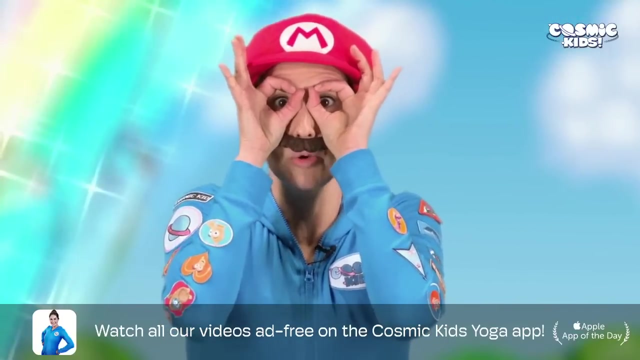 Open those branches Now let's see if we can see Peach's castle. using our cosmonoculars, Joining our thumbs and fingers together, have a look through. Oh, look, there it is On the horizon And it's surrounded by black smoke, which means Bowser has taken over and Princess Peach is trapped. 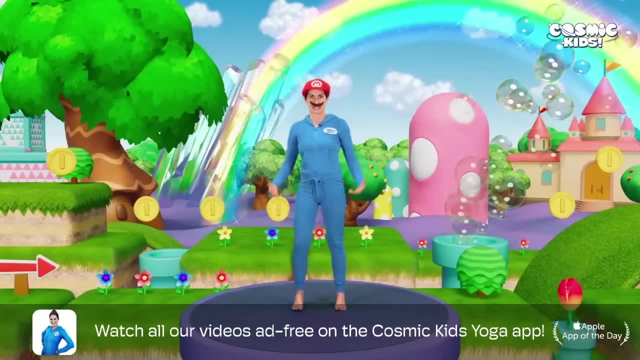 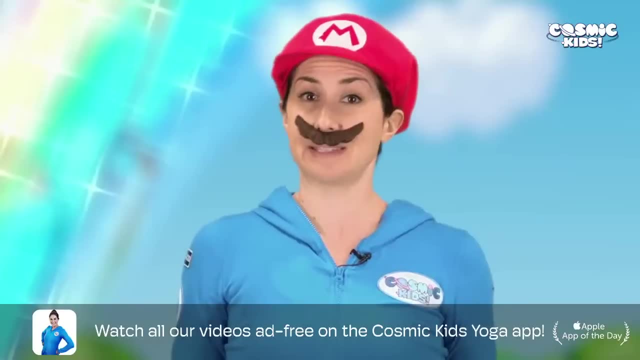 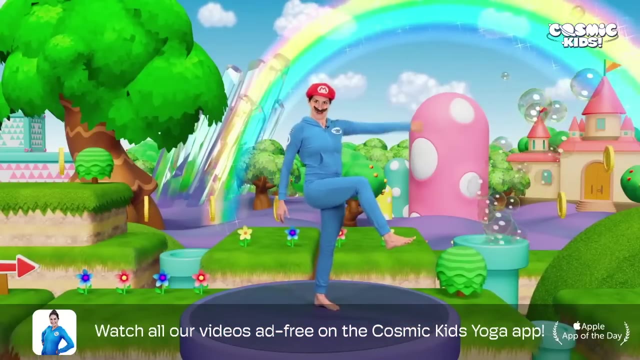 Lowering our hands all the way down. we stand tall. Mario must be determined and courageous to save Princess Peach. And today we will be Mario. Let's do our Mario pose again. We take our leg up, lift our arm, arm behind and we say let's-a go. 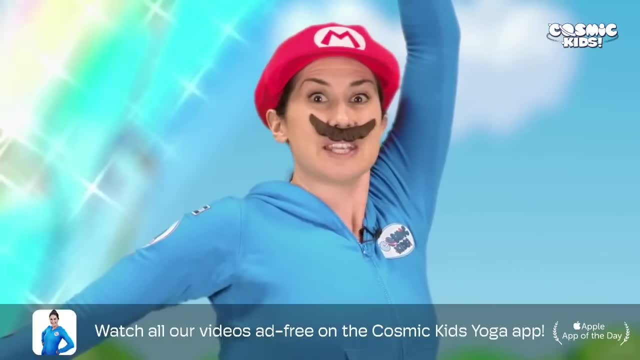 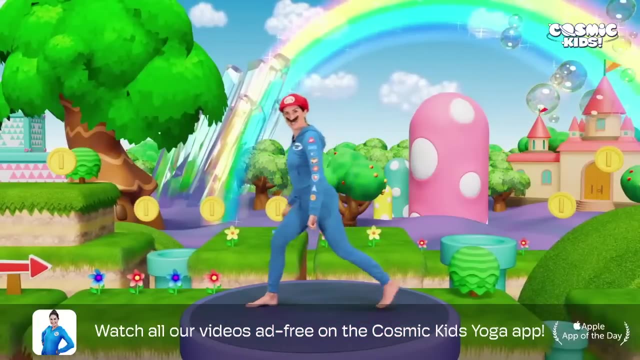 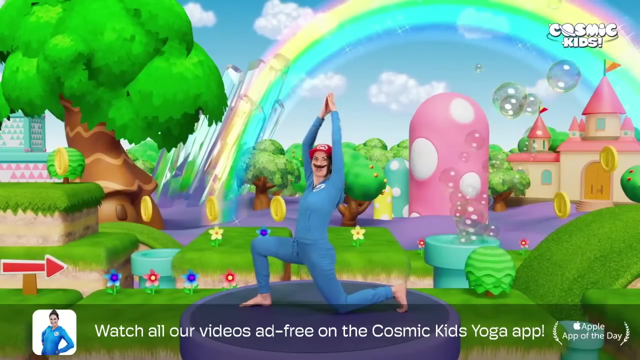 Now off we go into the world riding on our Yoshi the dinosaur. Let's do riding Yoshi pose Coming down onto one knee hands to our heart. we lift them up above our head. Now Yoshi sticks his tongue out and in. 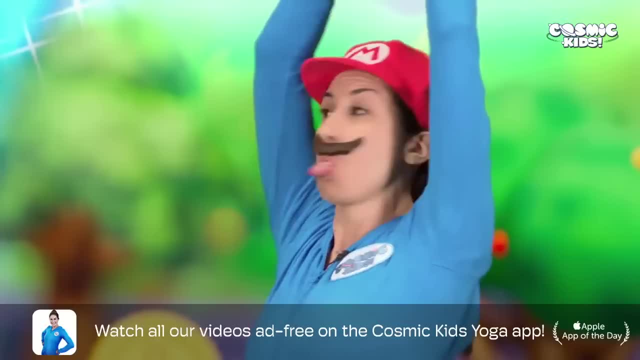 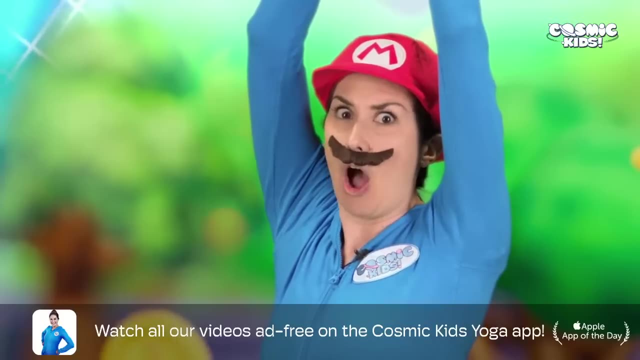 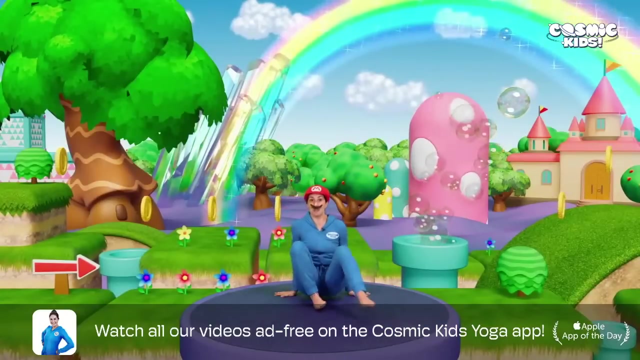 Let's have a go. Very good, everyone. Now, Yoshi can only get us so far. before we need to get higher in the sky, And for this we need a pink baby Yoshi who blows up like a balloon, Coming to sit on our bottoms with our legs crossed, we cup our hands around our mouth and take a big breath in through our nose. 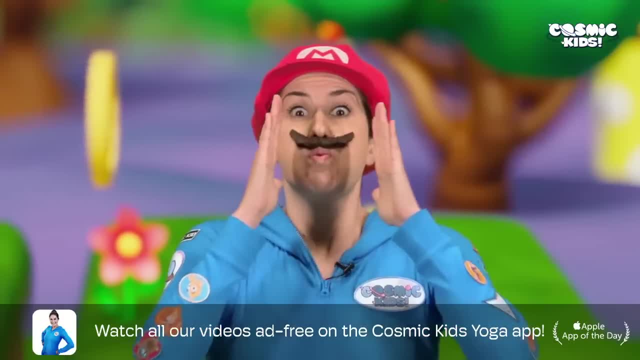 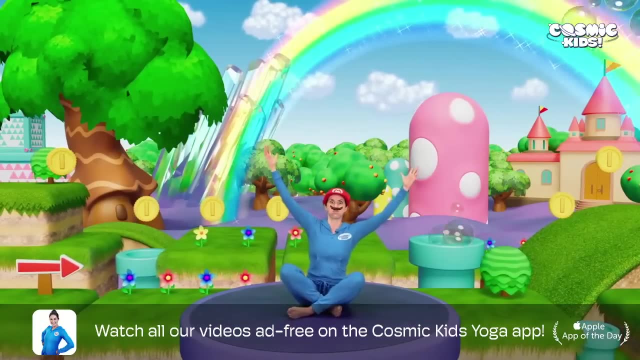 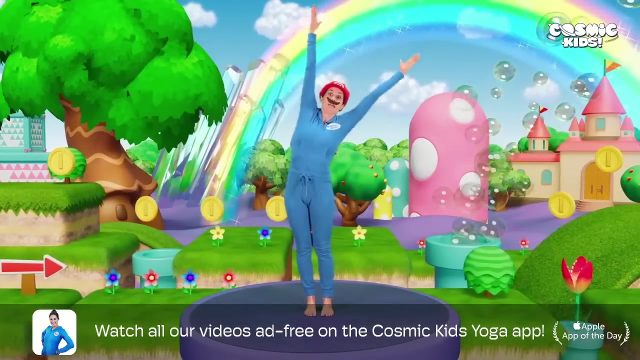 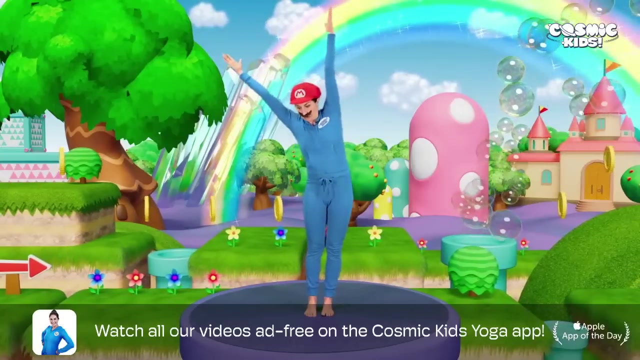 Ready. And now we blow. Wow, we've blown up our pink baby Yoshi. We stand on up, Reach up with our hands And we hold on as we float up, up, up in through the sky, through the clouds. Oh, we have to be careful. 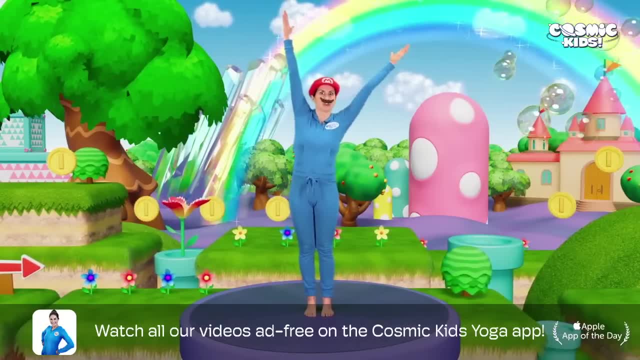 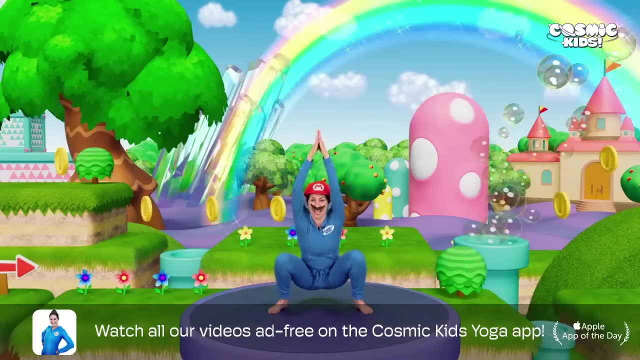 Down below are the piranha plants popping out of the pipes. Taking our feet a little bit wider, we bend our knees all the way down, Join our hands together over our heads. Now we slowly, slowly, slowly rise all the way up. 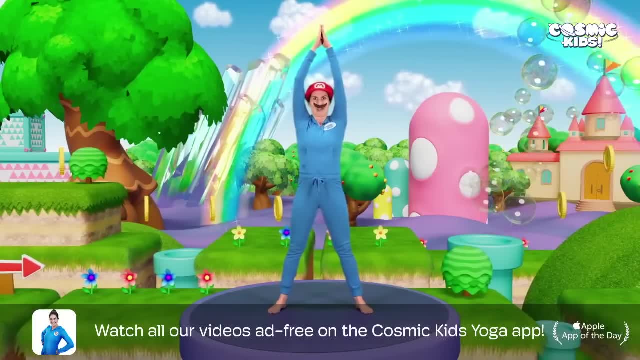 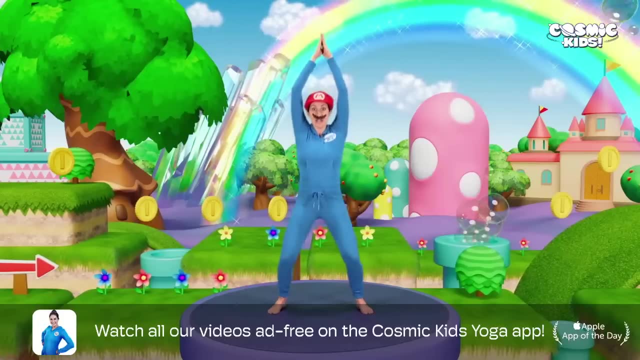 And we go, snap, snap, snap like a piranha plant. Now let's jump down onto the platform After three, One, two, three, Boing, boing, Wow, Here we are on the ground And we have to be very careful for the goombas. 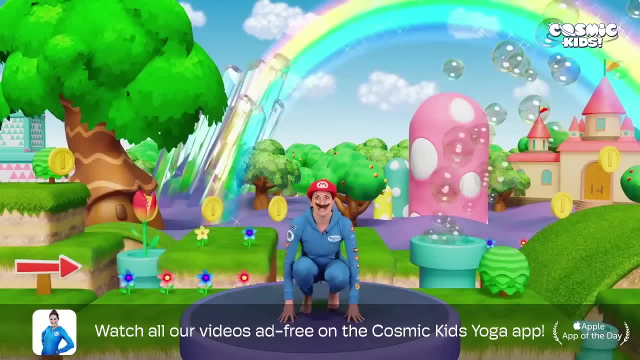 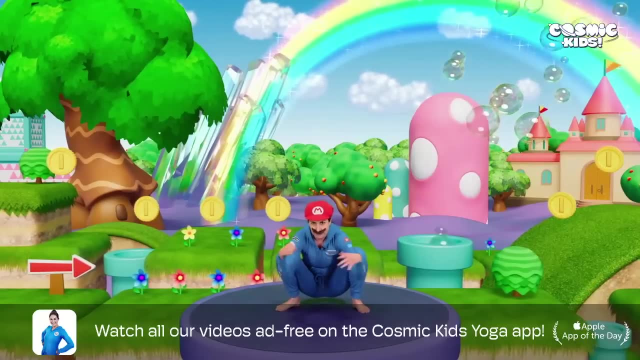 These are the little brown mushrooms with mean faces. Let's do our goomba pose: Coming into a squat position, snuggling our arms in, making a fist, holding it with our other hand and doing our meanest goomba face. Mmm, 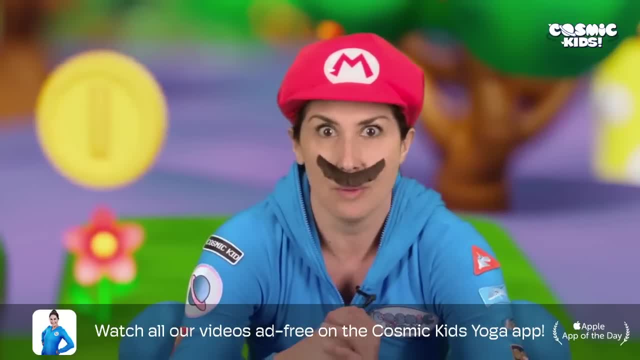 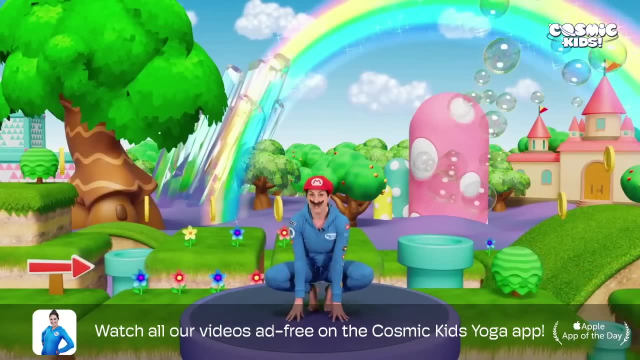 We have to squash these. We have to squash these guys and jump on them like a frog. Let's do our frog hop pose Coming up onto our tippy toes, knees wide onto our fingers for balance. After three, let's do a big jump. 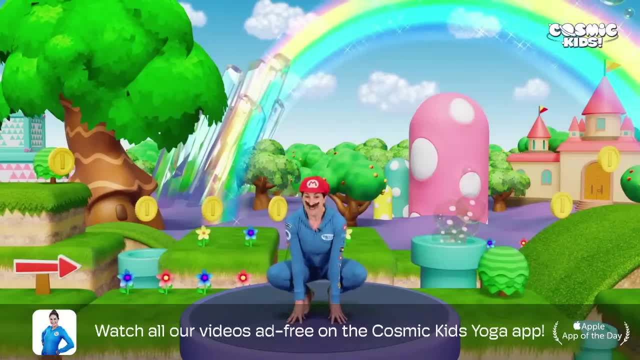 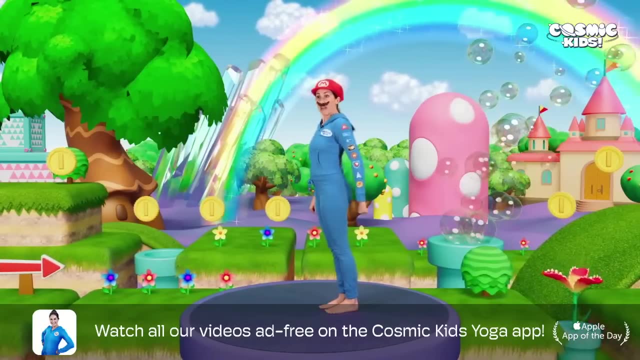 Ready. One, two, three, Wahoo. Very good everyone. We squashed them Coming up to stand. Now off we go running through the levels. Run, run, run, run, run, run run. 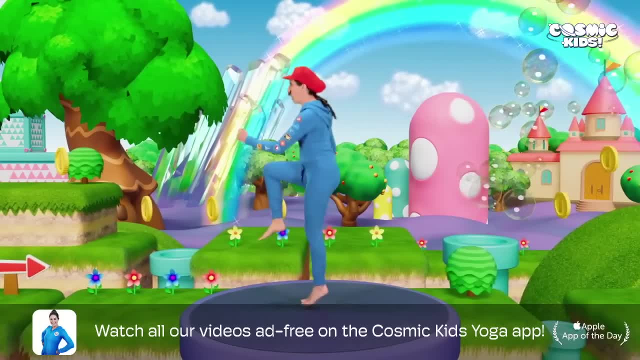 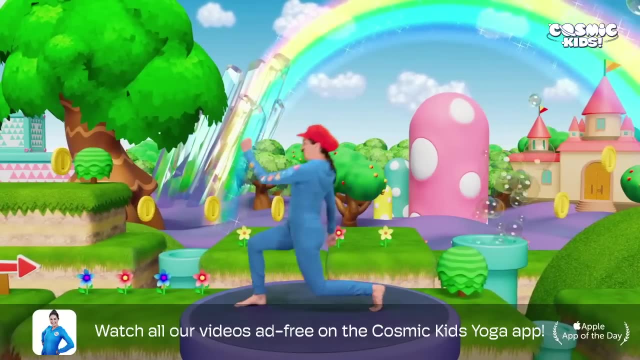 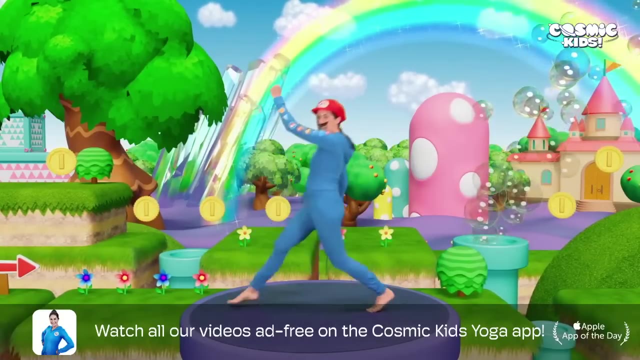 We do some hopping, Hop, hop, hop hop And the other leg, Hop, hop, hop, hop hop. We take some big steps, Ready, Big step across the platforms. Big step, Two more Big step. 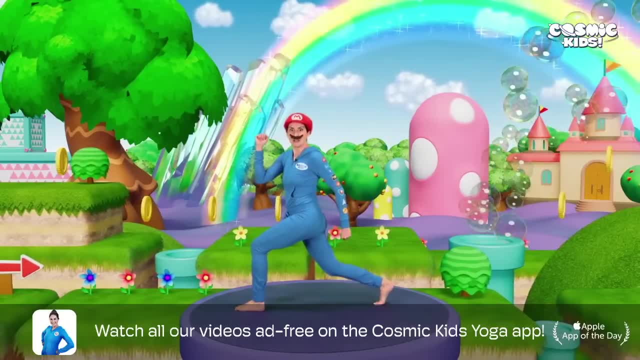 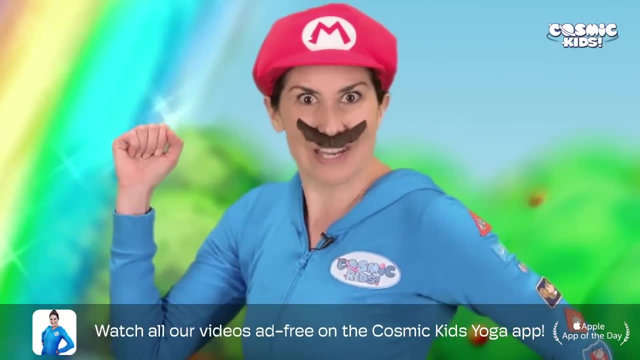 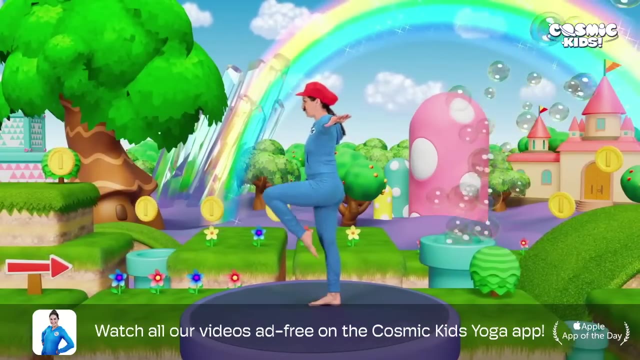 Last time Big step, And we find lots of things which give us special powers. The super acorn turns us into flying squirrel, Mario. Let's do our flying squirrel pose. Coming up to stand, we take our arms wide, we lift up our leg and we send it all the way. 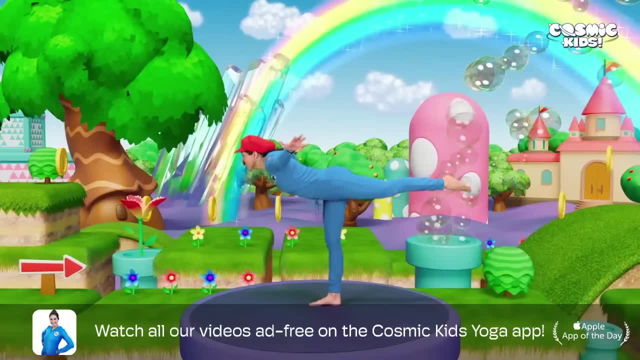 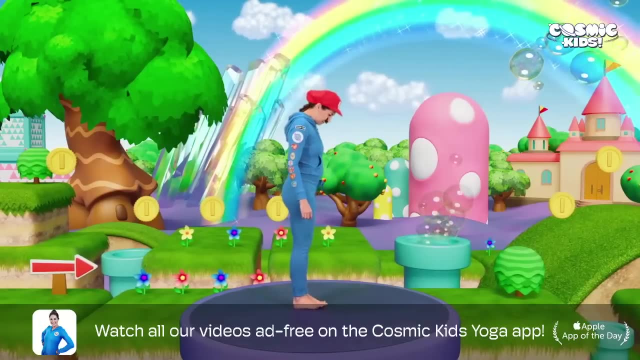 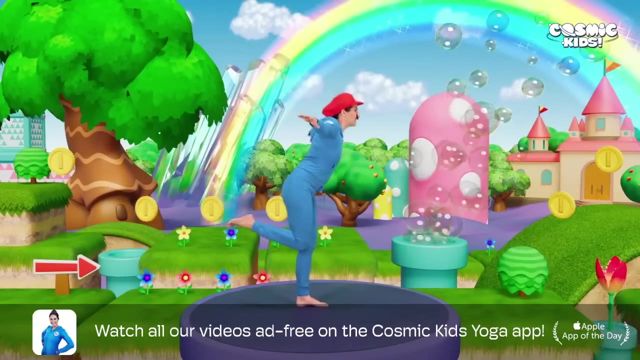 back behind us in our flying squirrel pose, Wahoo Coming back to stand. let's try it on the other side, Turning to face the other way, finding a spot to focus on. we take our arms wide, lift up our foot and send it all the way back behind us, making our legs as strong as they can. 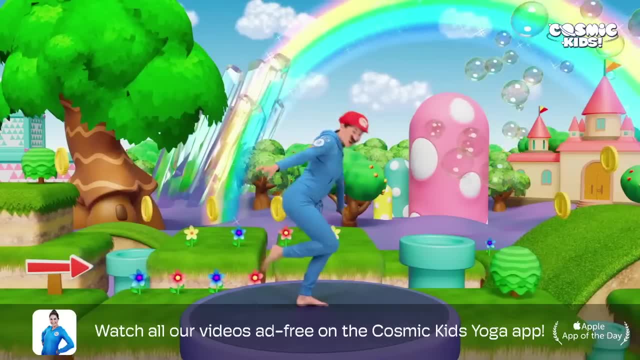 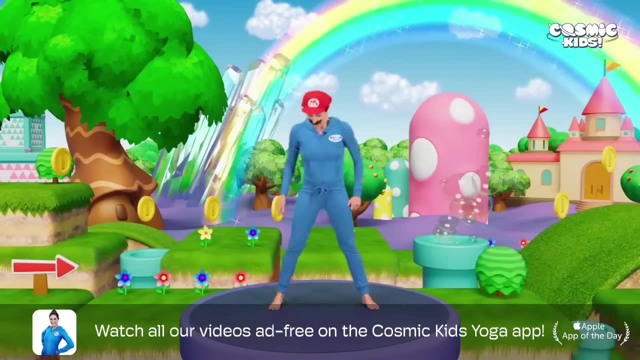 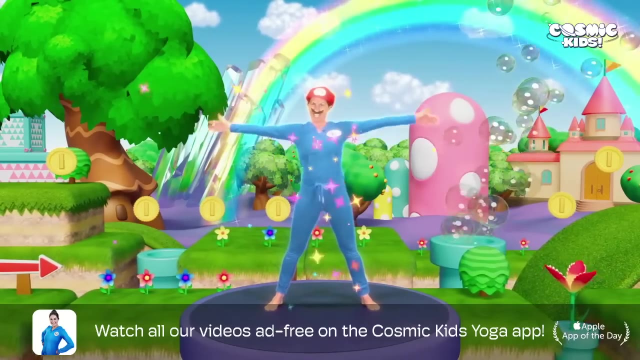 be Wahoo. Coming up to stand the super star makes us invincible. Let's do our star pose: Feet nice and wide, arms wide And flickering our fingers as we go, zooming through the levels: Invincible. This is amazing. 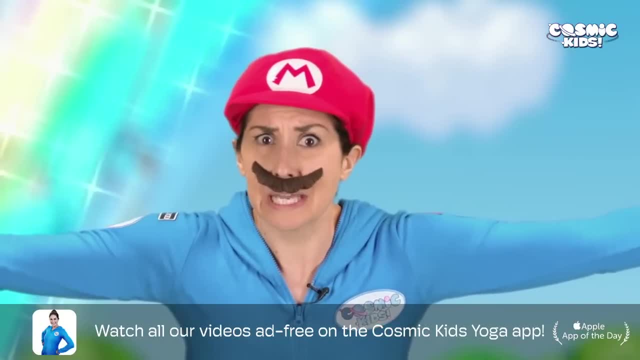 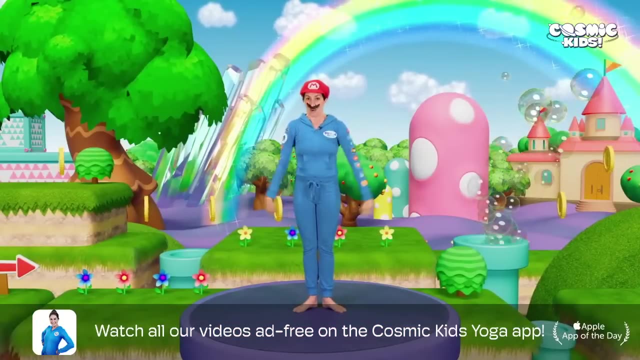 We also find a penguin suit, And can you guess what that turns us into? Yes, Penguin Mario, Jumping your feet together, toes out wide arms to the side and let's waddle around. Waddle, waddle, waddle, waddle, waddle, waddle, waddle. 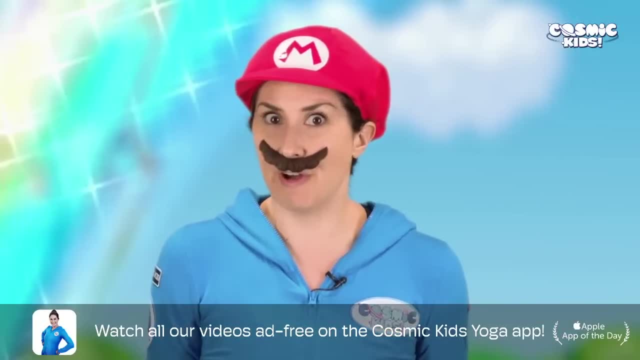 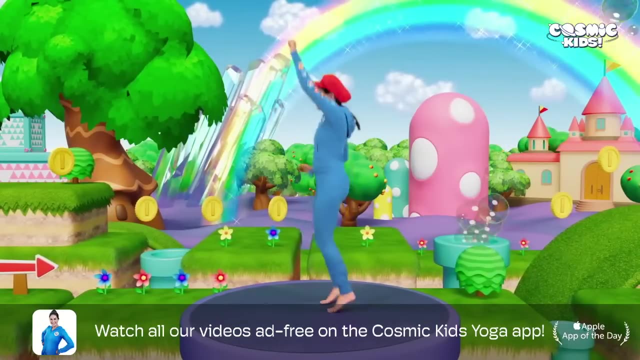 Off. we go through the levels some more. We climb up some vines and beanstalks. Here we go Up, we go up, we go up, we up, we up, we go Up, we go up, we go up, we up, we up, we go. 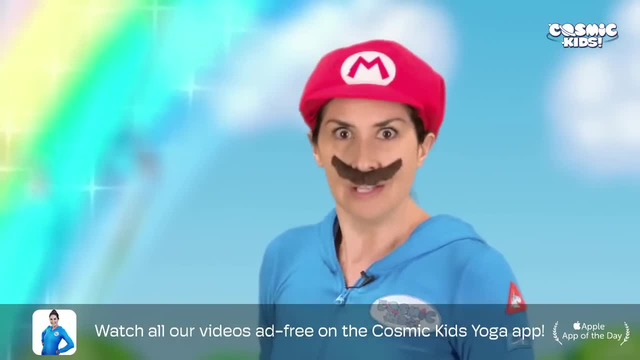 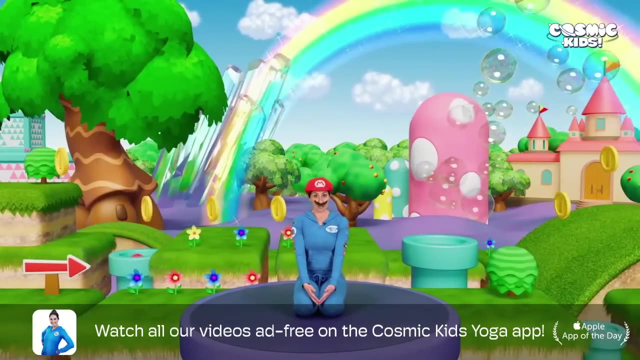 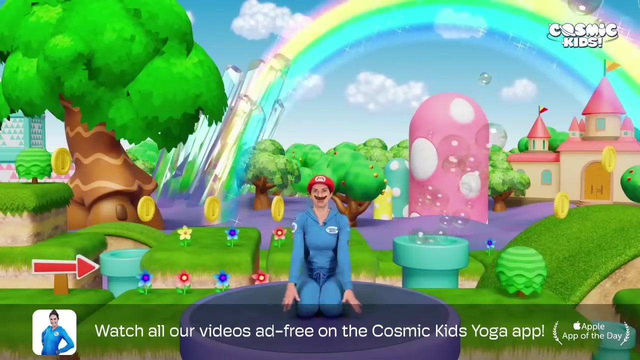 We head through Iggy's volcanic castle, Let's do our volcano pose: Coming down onto our knees, Hands down in front of us. We lift all the way up as we breathe in And we blow to the sky, Ready And again breathing in, lifting up. 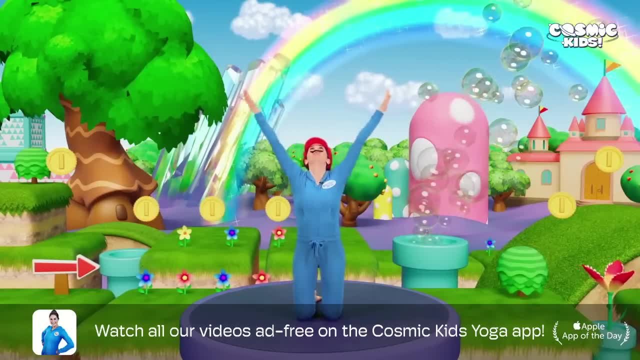 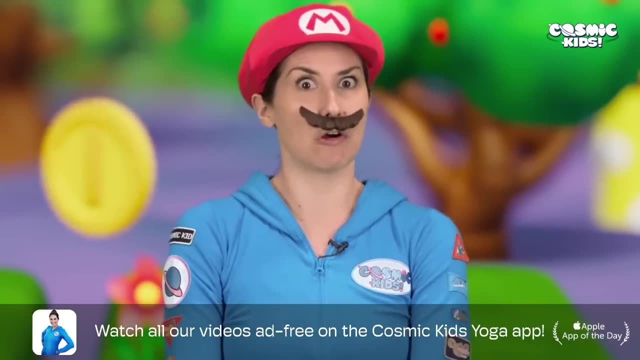 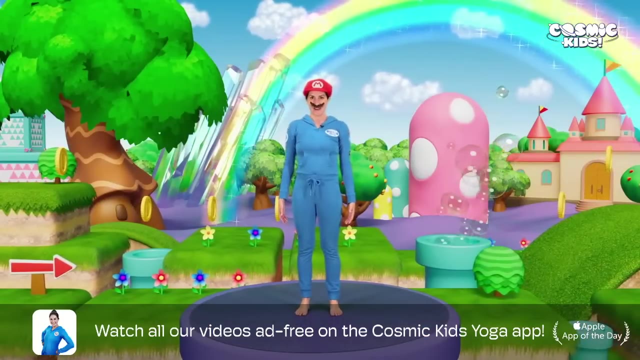 And blowing out to the sky. as we lower down, We even face the fuzzy cliff top mountains in the rock candy mines. Coming up to stand And let's do our mountain pose, Feet hip distance apart, Arms down by our sides, Standing as still and powerful as a mountain. 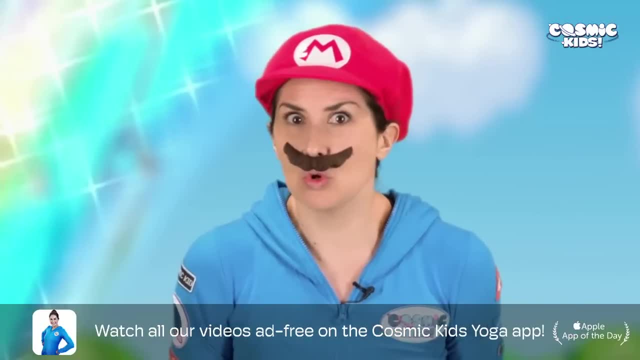 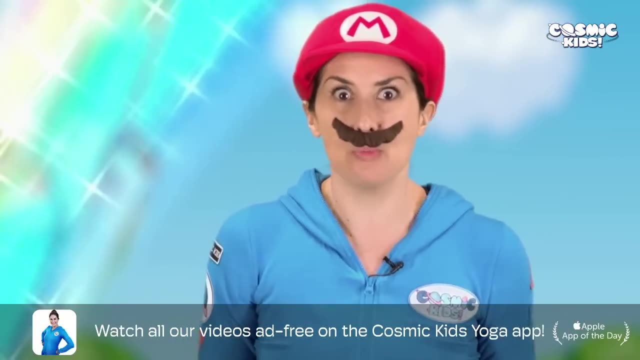 Wow, well done everyone. In the sparkling waters we discover a shipwreck, A boat that sunk to the bottom of the ocean. Let's do our boat pose Sitting on our bottoms. we lift up one foot, Lift up two. 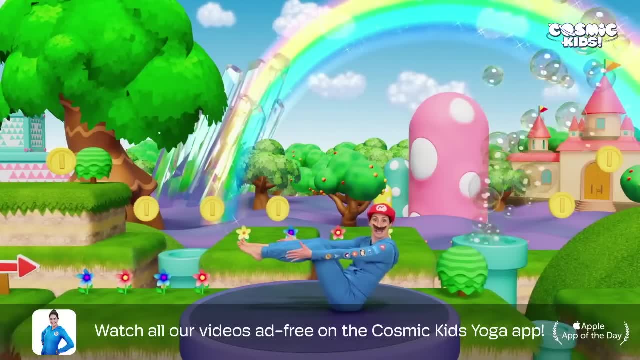 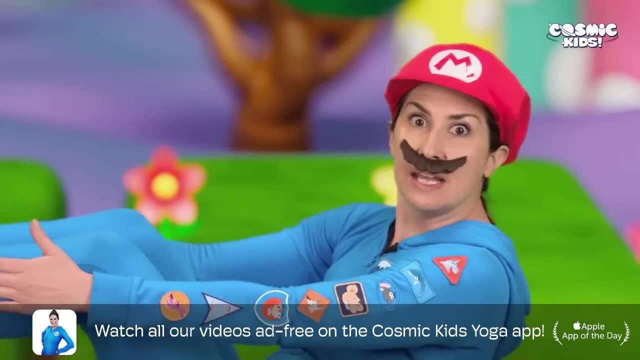 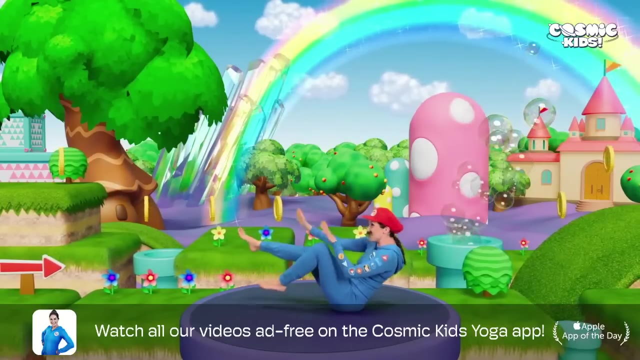 Lift up one hand, Lift up no hands And give me a wave. Now this shipwreck is haunted. It's full of boos, Little ghosts. Let's wiggle our arms and our legs around going, And there are skeleton chief cheeps. 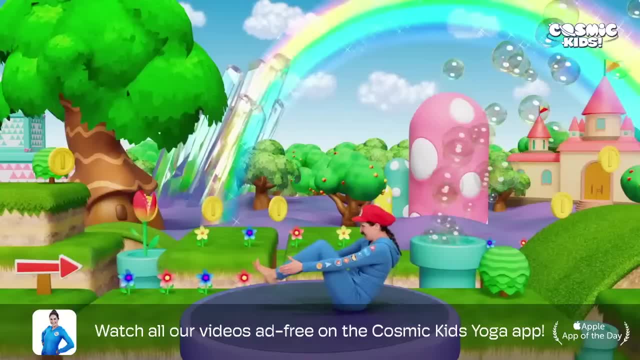 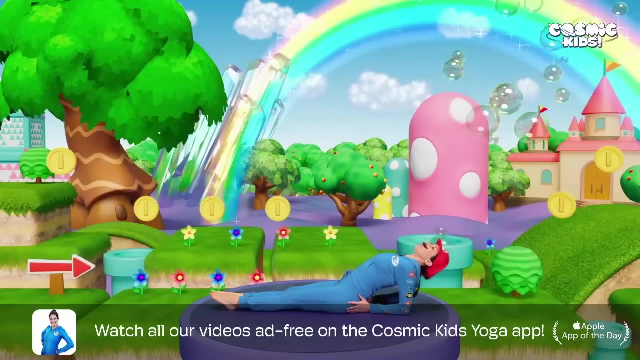 Fish bones. Let's do our fish pose, Sitting with our legs out long, Pointing our toes, We drop down onto our elbows And we pop, pop, pop, pop, pop our chest to the sky, Looking up and back behind us. 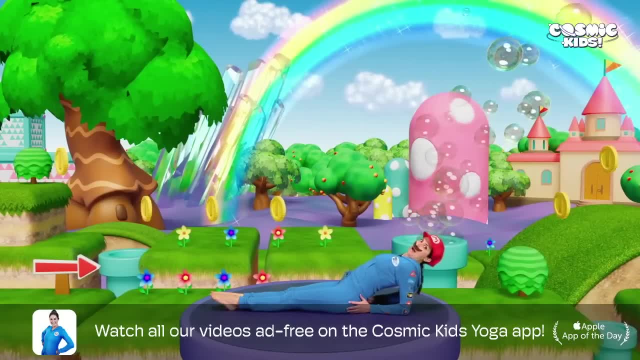 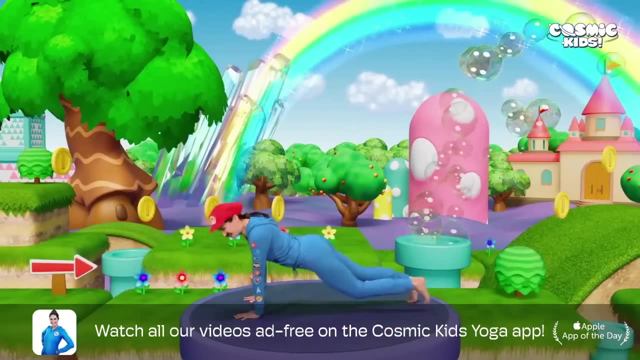 Like a skeleton: cheep, cheep Woo. Now we need to travel through these underwater worlds, So let's swim. We come onto our tummies And we use our arms and our legs, Raising our legs up and lifting our arms. 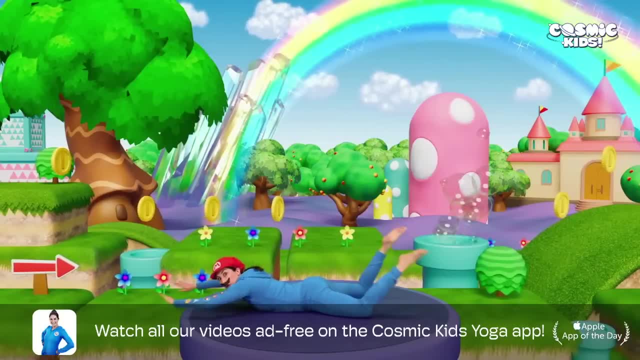 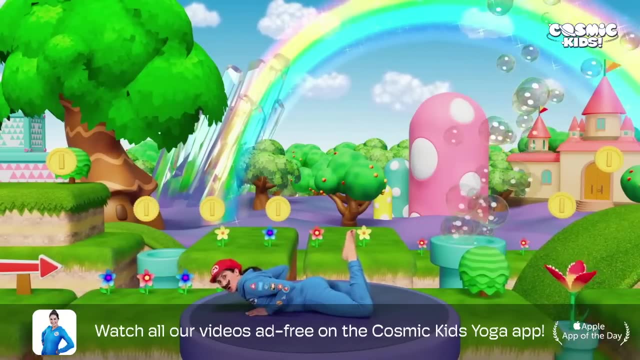 As we swim through the underwater worlds. Uh-oh, Swimming towards us are some bullet bills Which look a bit like Sharks. Let's do our shark bullet bill pose, Stretching our legs behind us, Criss-crossing our fingers behind our back. 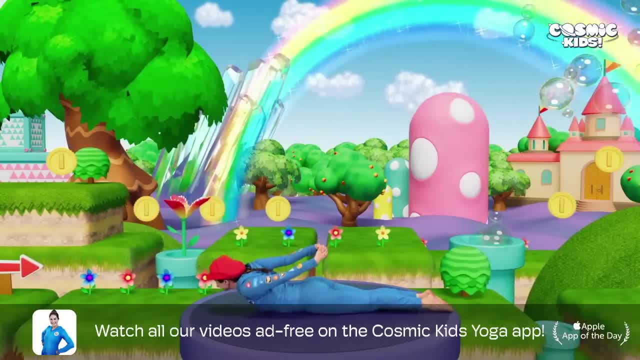 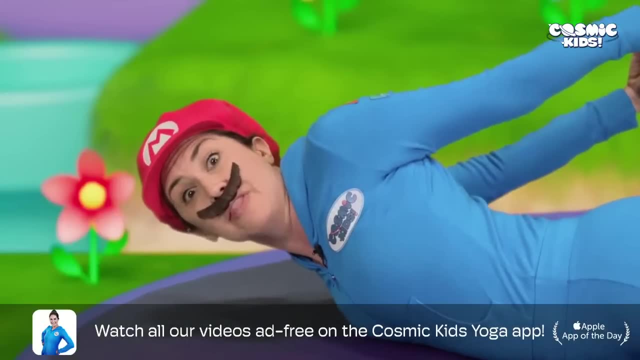 We lift up our shark fin And we loll from side to side, Going doo-doo-doo, Doo-doo-doo, Doo-doo-doo, Doo-doo-doo. The bullet bills and the torpedo teds swim right by. 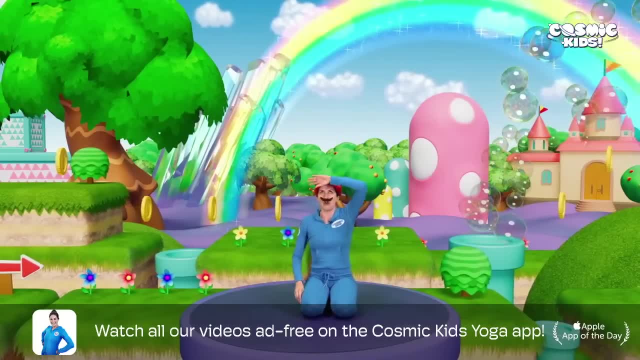 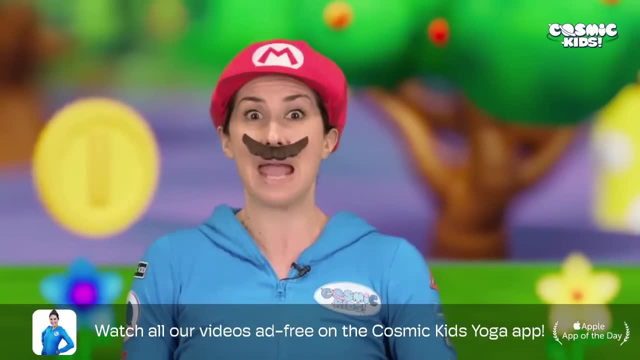 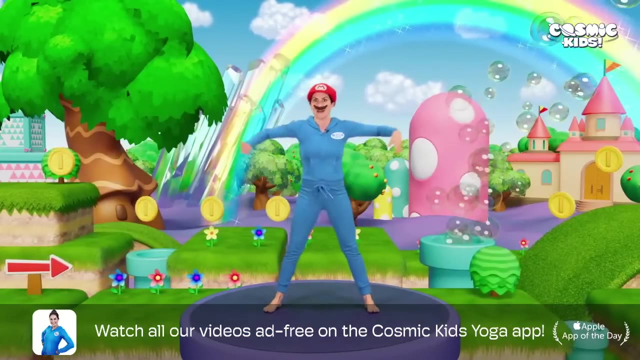 Coming up to sit. We say for you Now, after those we come to Peaches Castle. We have made it, But it's surrounded by a tornado Coming up to stand, everyone Feet wide, Arms wide. We spin side to side. 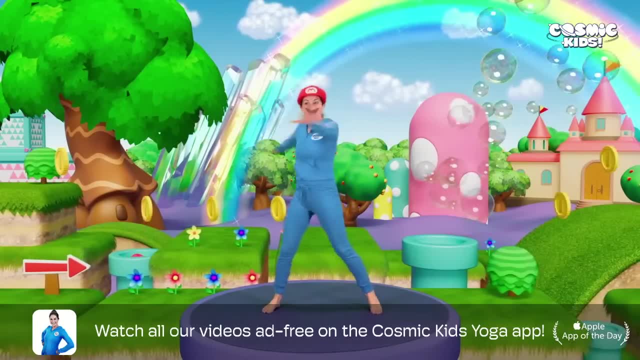 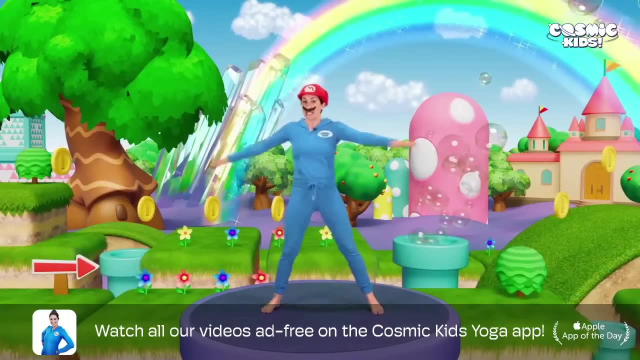 It's a tornado of black smoke. It's black magic Made by Magi Cooper, Who has also turned Bowser into Super Bowser. He's now as big as a dragon And he breathes fire. Let's do our dragon pose. 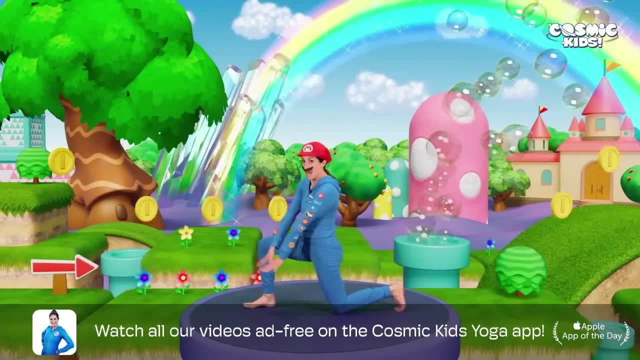 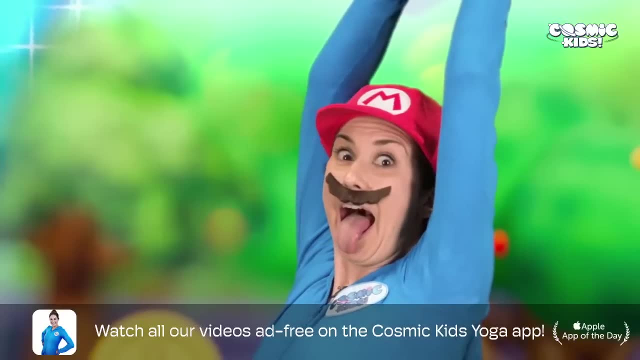 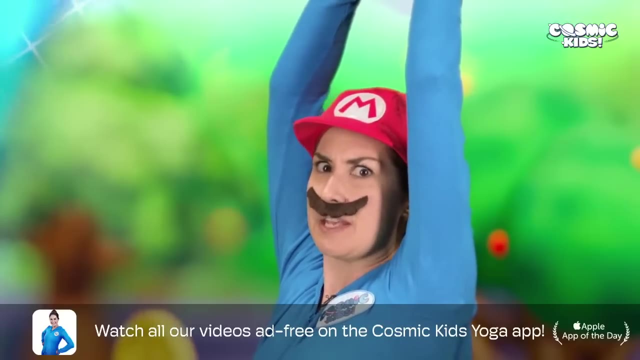 Coming down onto one knee, Criss-crossing our thumbs And lifting them up above our head. Now let's stick out our tongues as we breathe some fire. We need to rescue Peach. We've come all this way. Let's use all the skills we've learned and defeat Bowser. 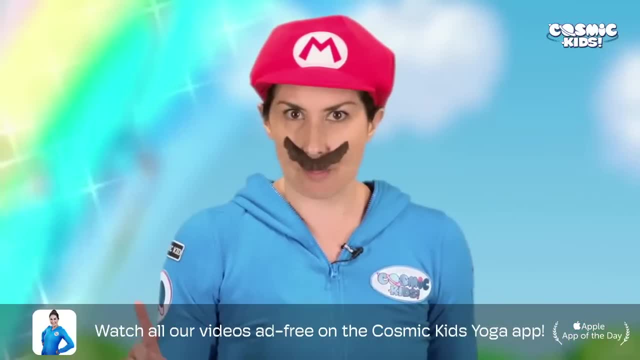 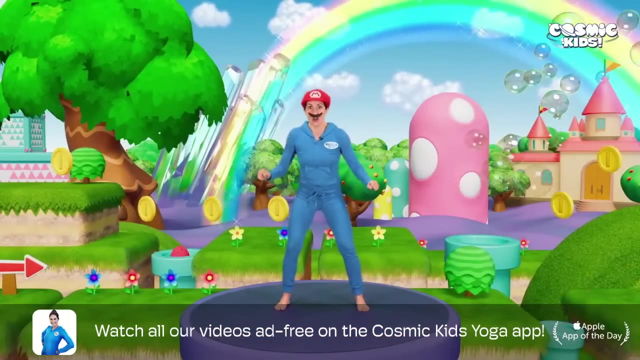 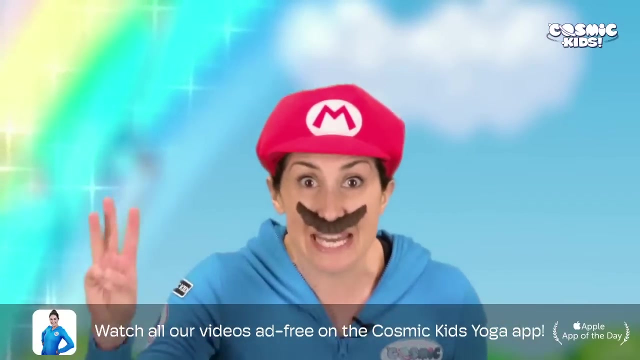 We come up to stand First. we need to jump on him three times. After three, let's do three jumps Ready: One, Two, Three, Boing, Boing, Boing. Very good, everyone Next. we need to duck down three times. 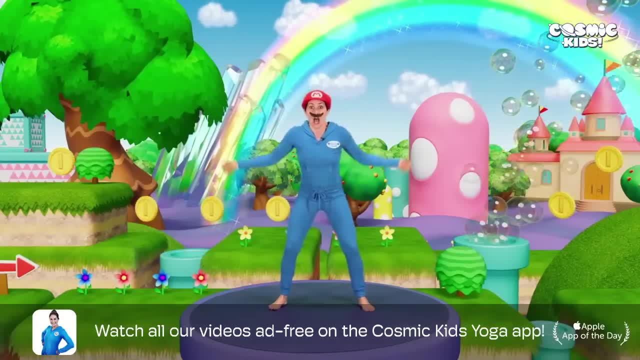 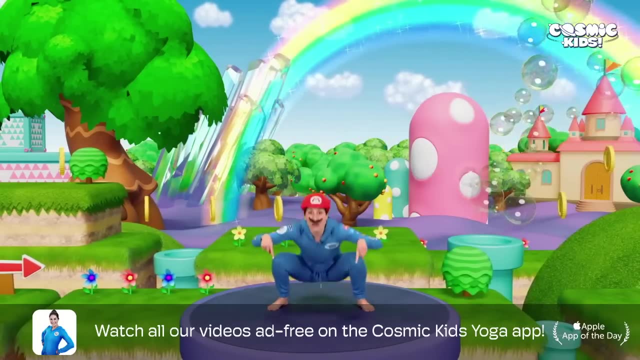 After three: One, Two, Three Ducking all the way down And up, And again All the way down And up. Last time All the way down And up. Wow, We're nearly there. Next we get into Bowser Junior's clown car. 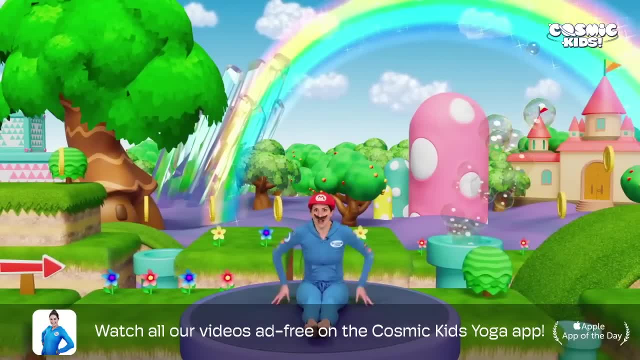 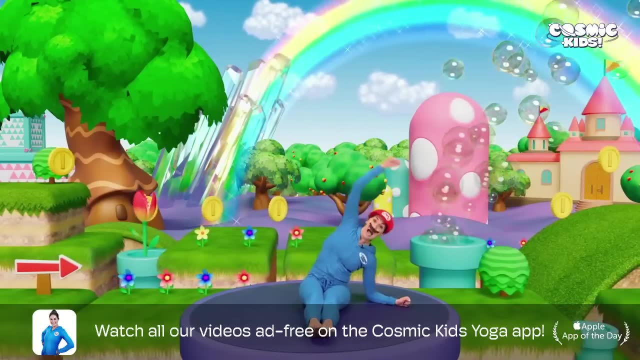 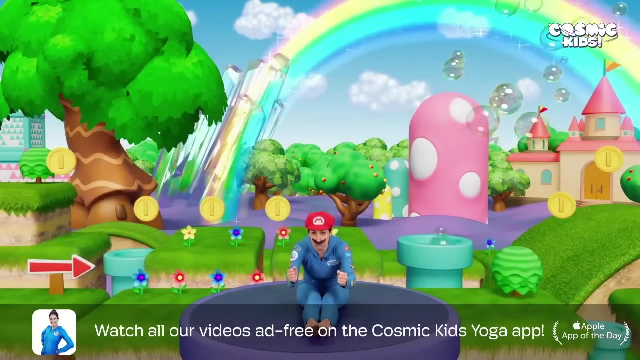 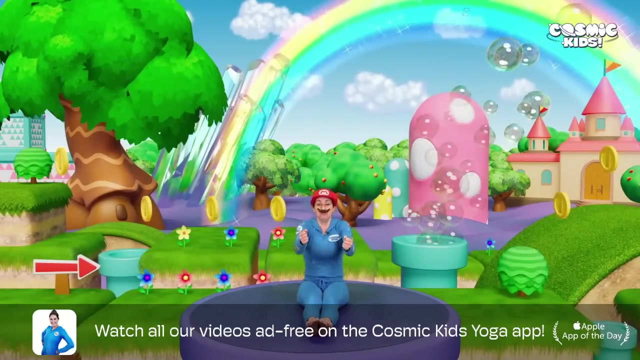 Sitting on our bottoms, Legs out long, Holding onto the steering wheel. We're going over one way And the other way. We go all the way forwards, All the way back, And now we slam forwards into Bowser Bof. 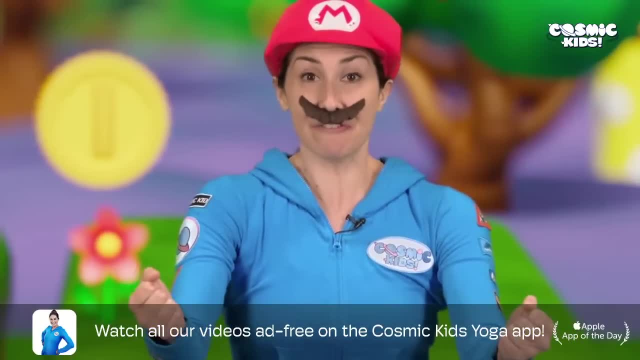 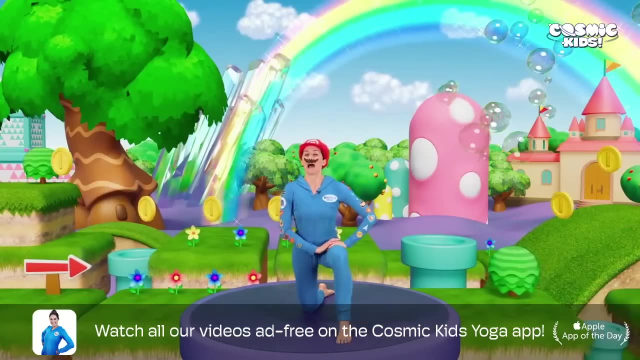 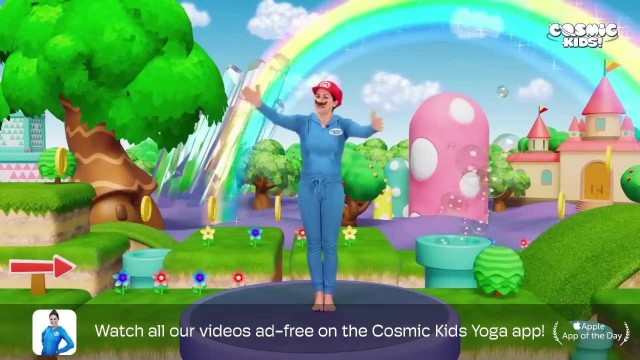 We've boffed Bowser And we've defeated him. Princess Peach is here. She is free. We come up onto one knee And we bow down towards her. Princess Peach has a stand up, She opens her arms wide And she gives us a ginormous cuddle. 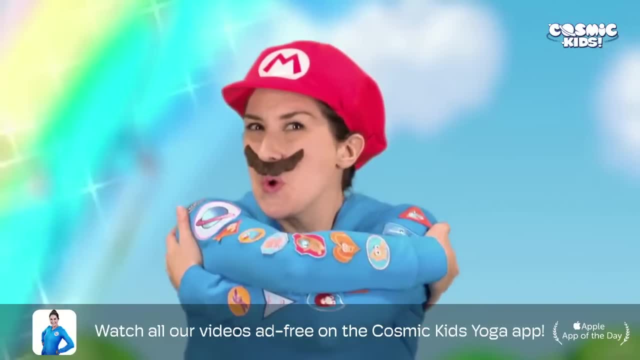 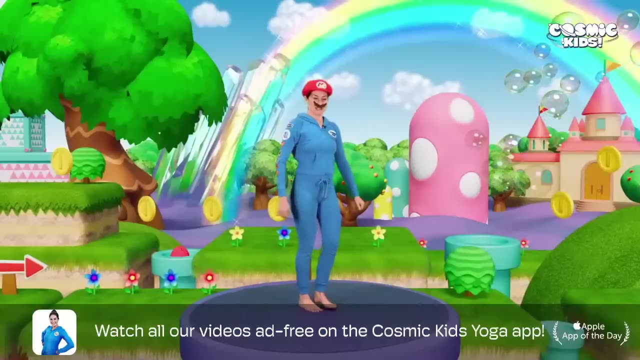 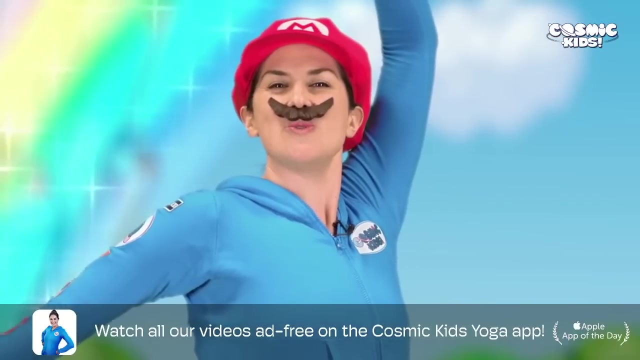 And a kiss. Ooh, It's been so exciting being Mario. Let's finish with a final Mario pose. We take our leg up, We lift up our arm, Take our arm behind us And we say: wahoo, Very good everyone. 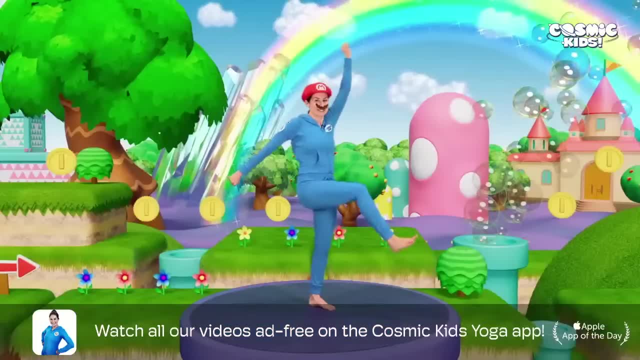 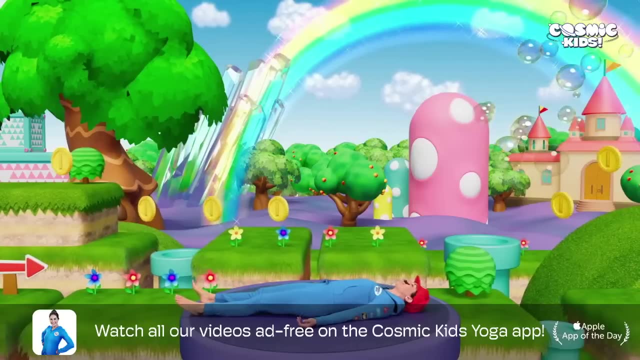 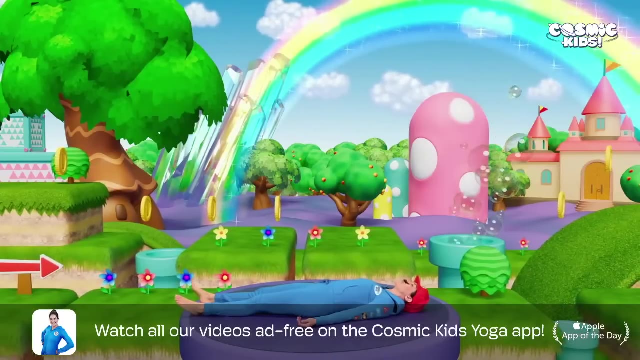 Let's take a moment now to lie down and relax. Coming onto our backs, Making our legs and arms long, Ah, It's lovely just to stop for a moment After such an amazing adventure. It's so much fun. Super Mario, Such a fun game. 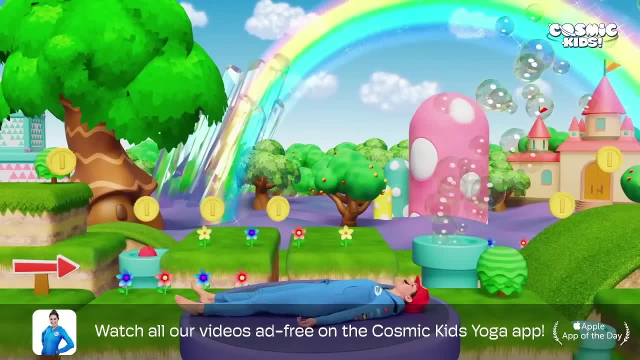 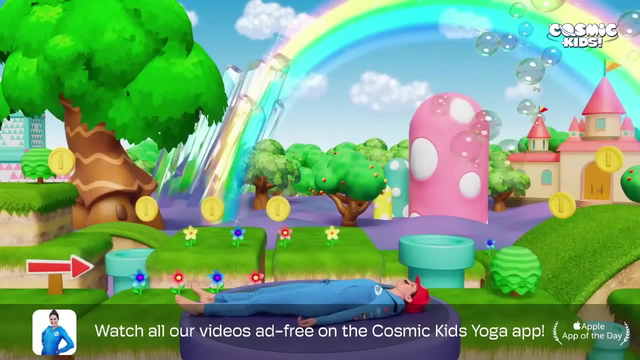 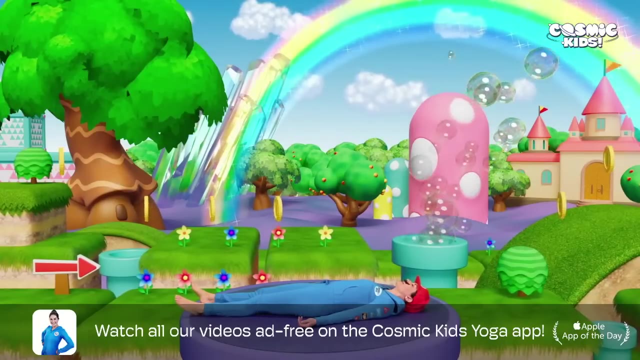 Mario has to be determined, Brave to face all those enemies And strange places. We feel very proud to have been Mario today: All the things that we learnt along the way That kept us moving forward And every time we made a mistake. 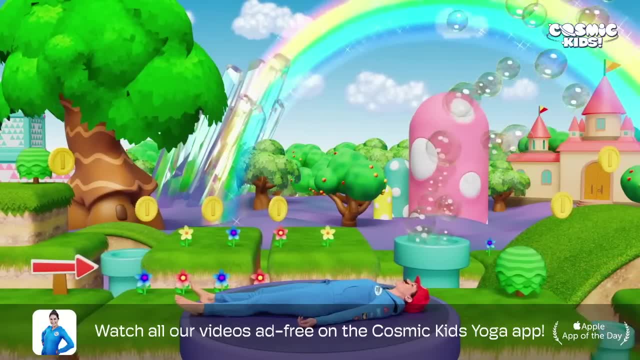 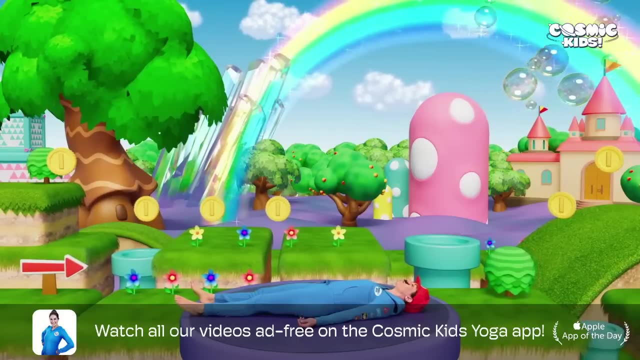 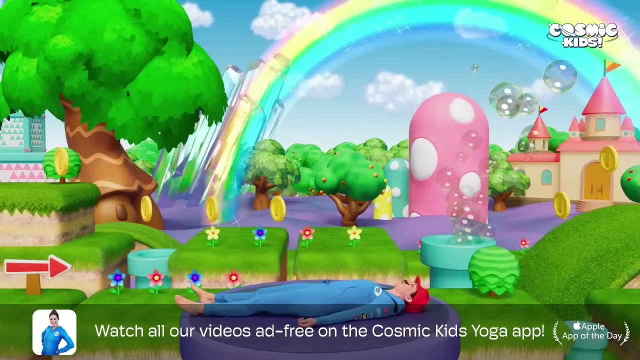 We learnt from it. This is why making mistakes is actually quite a good thing, Because when we make them, We can notice what went wrong And we can know what to do different next time. That's how we learn. It's how we improve. 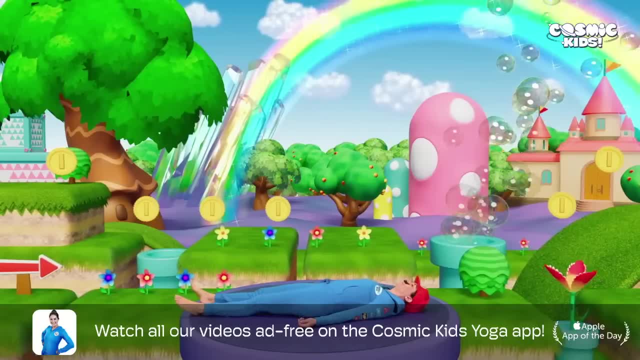 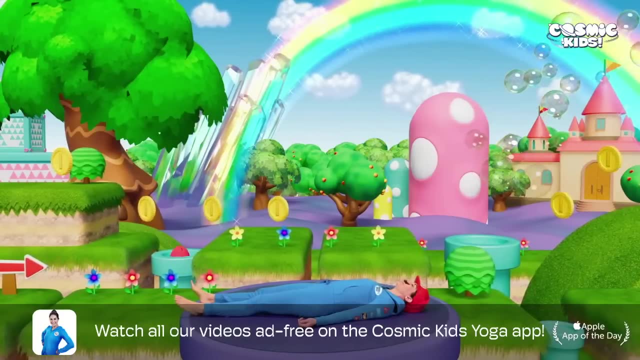 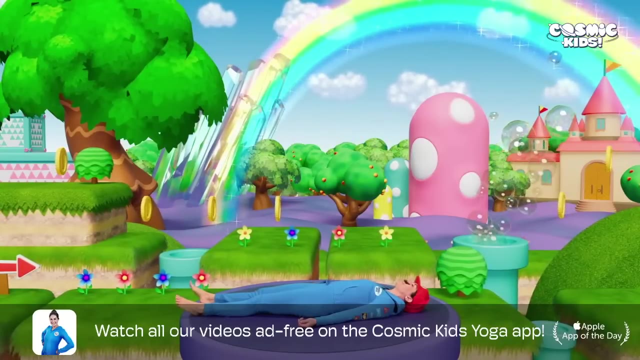 And it's how we get better. So Now we take a moment just to rest And enjoy this stillness. Slowly we begin to wake up, Wiggling our toes, Wiggling our fingers, We hug our knees into our chest. 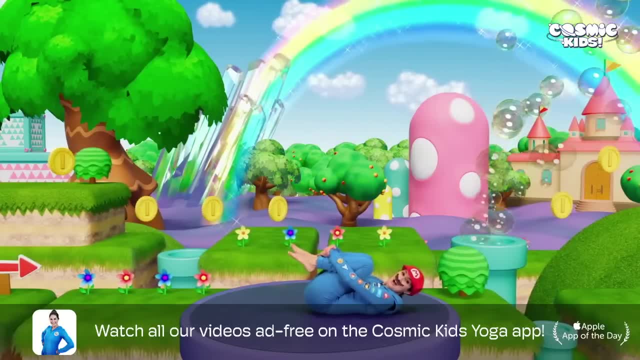 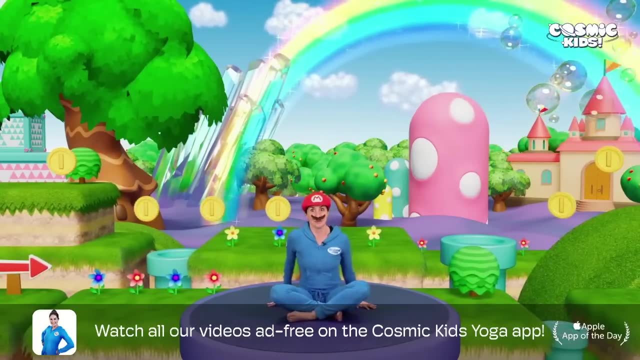 And we open up our eyes. We roll onto our sides And press ourselves up to sit And we finish just the way we started With our secret yoga code word: Let's bring our hands together at our hearts After three One: 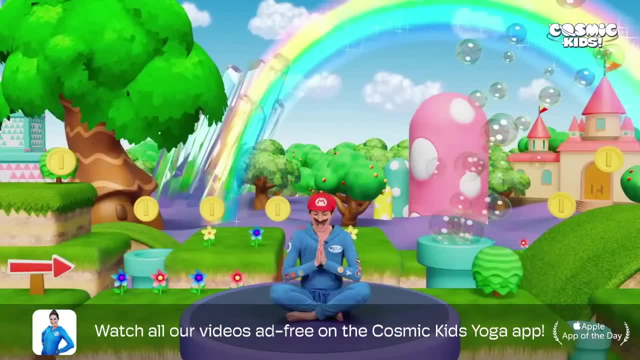 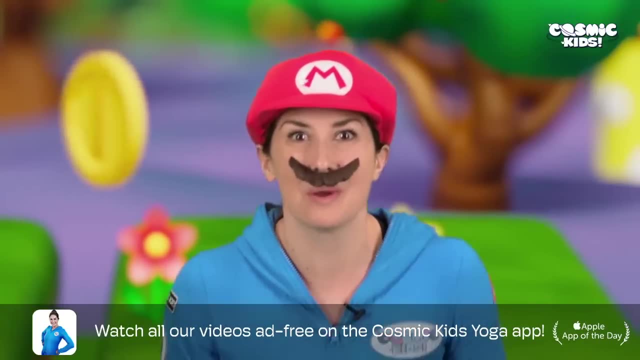 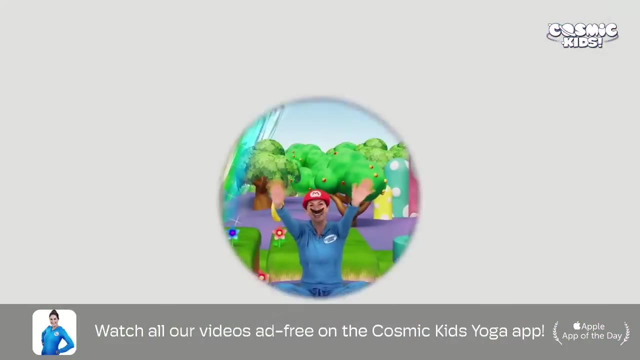 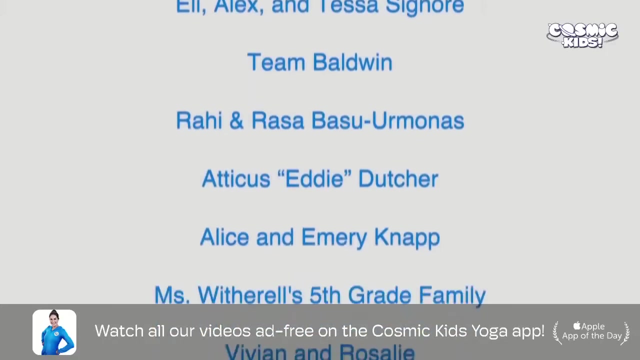 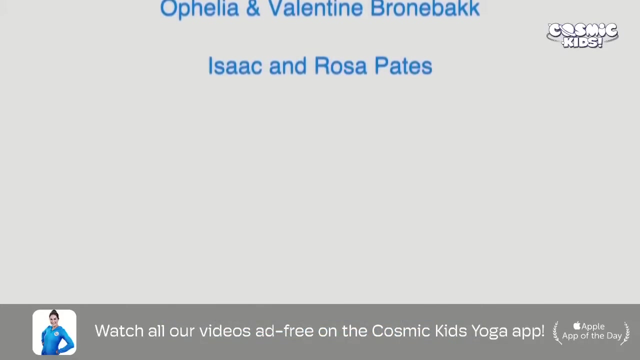 Two, Three, Namaste. Wow, Well done everyone. You were great in the Super Mario adventure. I hope you enjoyed it And I hope to see you again soon For another Cosmic Kids adventure. Bye, bye, I'm here to talk about our app. 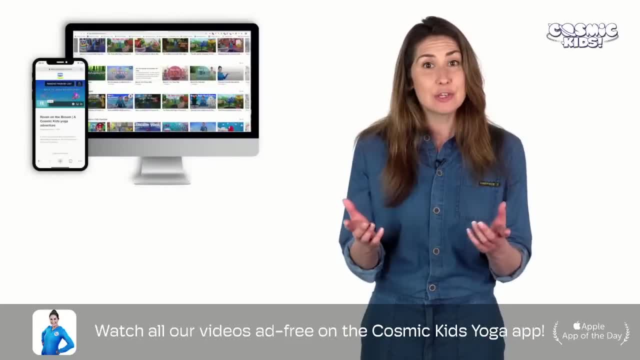 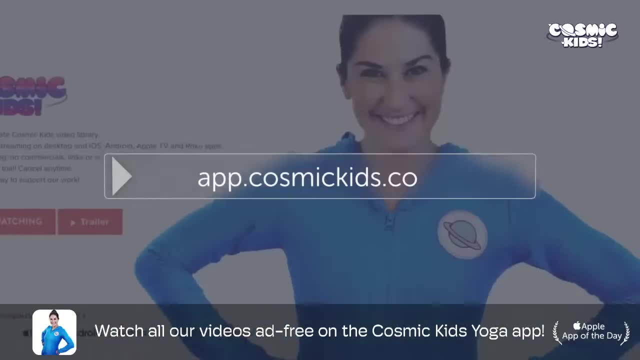 You can watch it on your computer or phone Using your web browser Or by downloading any of the apps Which are included in your subscription. To sign up, Head to appcosmickidscom, Pick a monthly or an annual subscription. 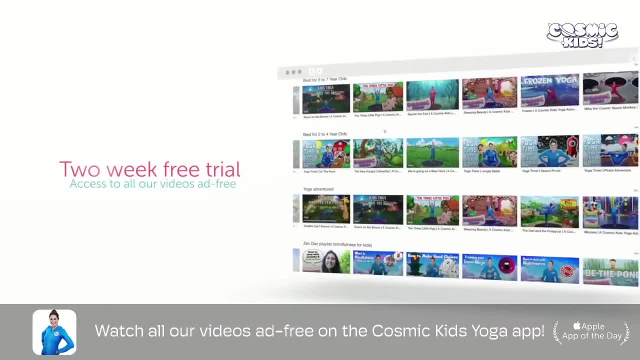 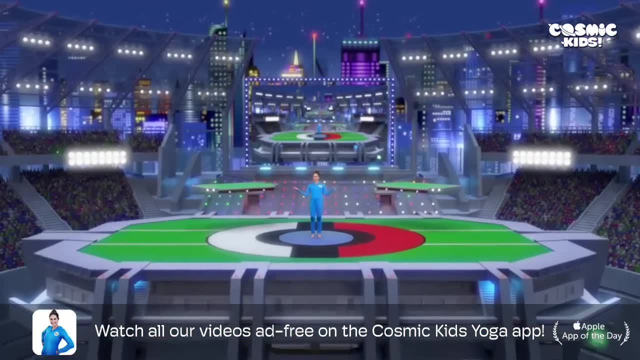 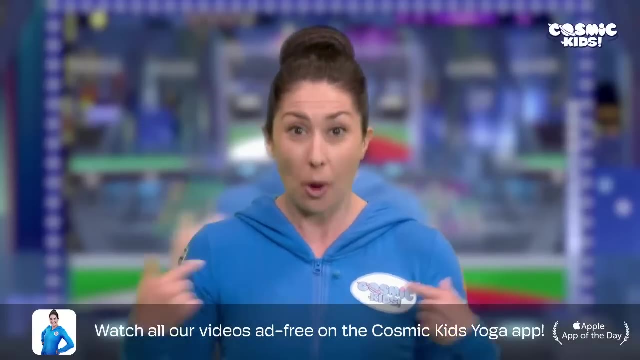 And then you get a two week free trial To see if you like it. Hello everyone, Welcome to Cosmic Kids. I'm Jamie And this is your place For yoga Stories And fun. It's easy, Just copy the moves I do. 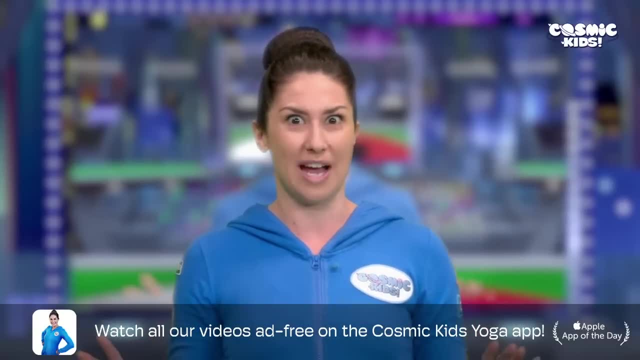 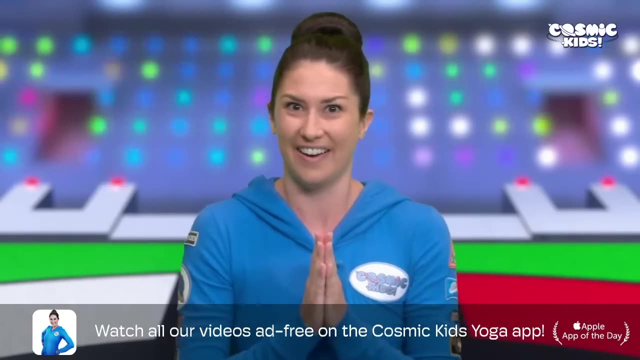 And enjoy the adventure Now. we always start in the same way, And that's by sitting on our bottoms, Crossing our legs And bringing our hands together at our hearts And saying our secret yoga code word, Which is Namaste Ready. 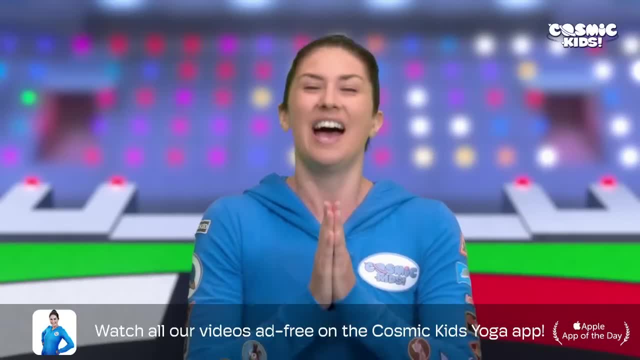 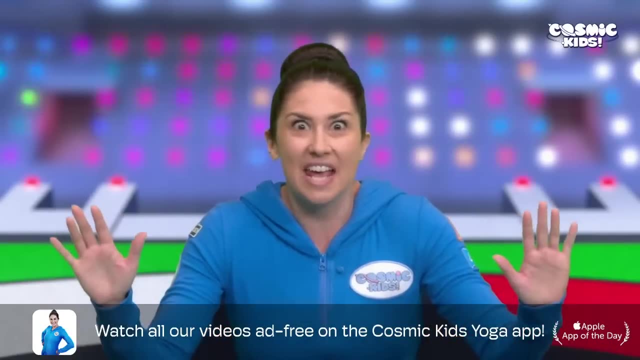 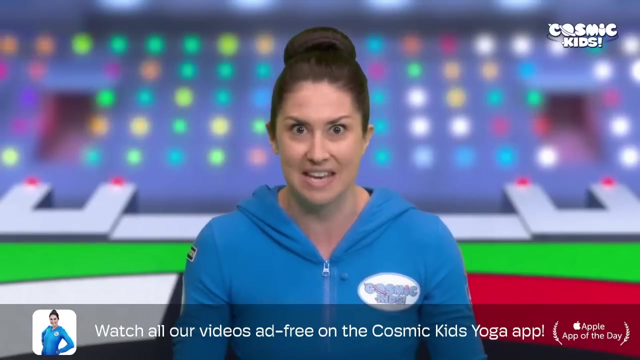 After three, One, Two, Three, Namaste There. Now we're ready to begin, And today we've got a special Pokemon adventure. Yes, Our journey to become a Pokemon master begins now. Now, the idea is to catch and train as many Pokemon as we can. 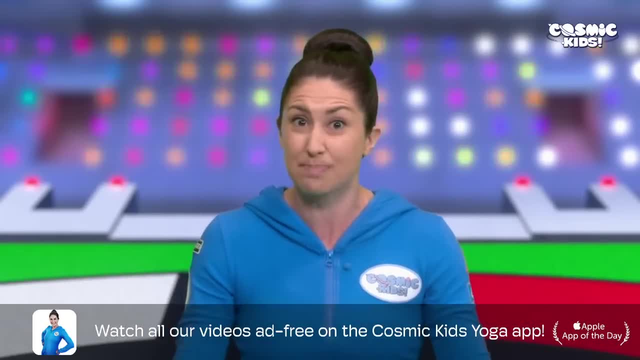 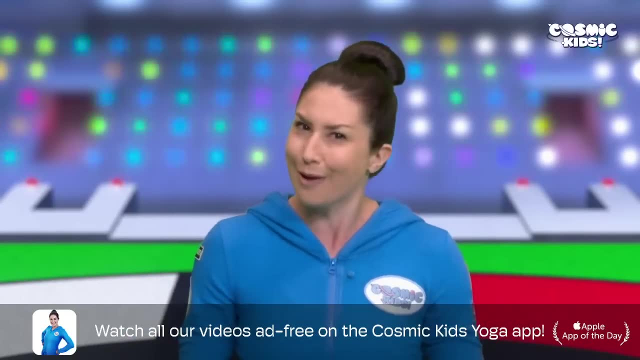 And today we're going to try and do our first battle in a gym. We're going to learn a lot along the way About our strengths and weaknesses And how to stay calm when we're faced with a challenge. Come on up to stand. 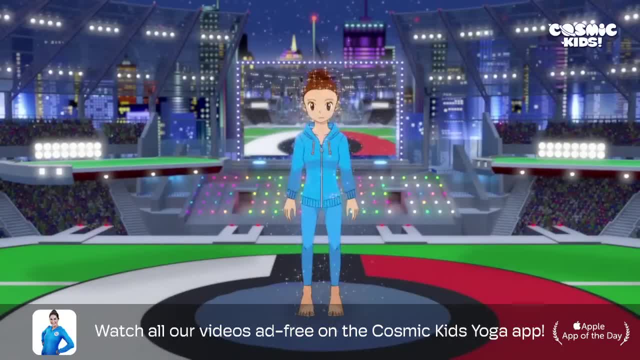 And let's get started. Oh, This is strange. I seem to have turned into a cartoon, Like the Pokemon cartoon. I'm not sure I can do yoga like this. I need to stay calm. I wonder if you can help me. 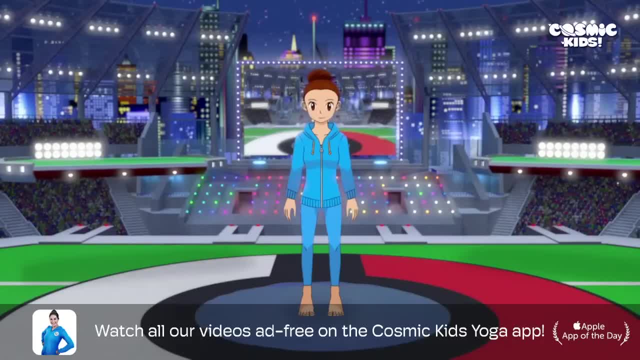 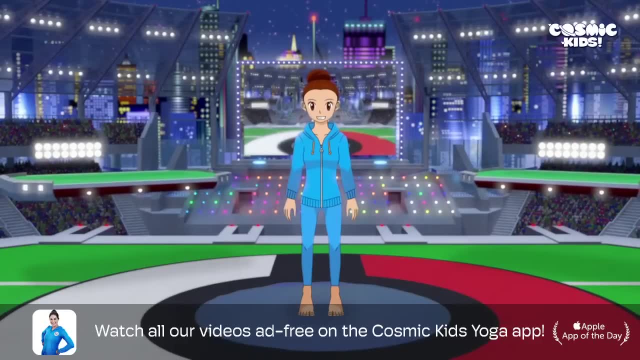 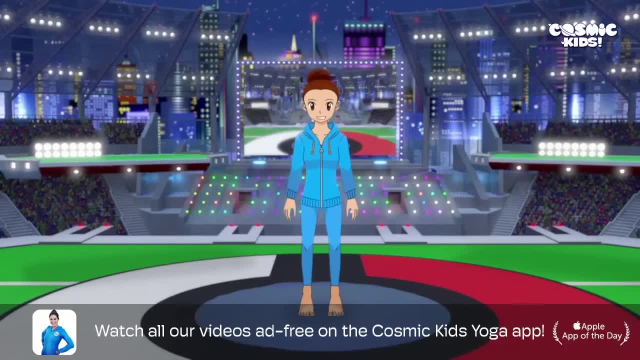 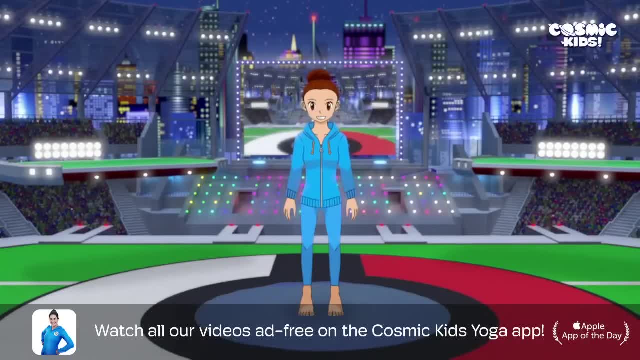 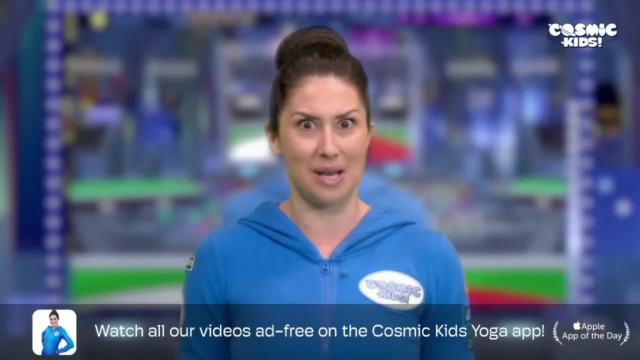 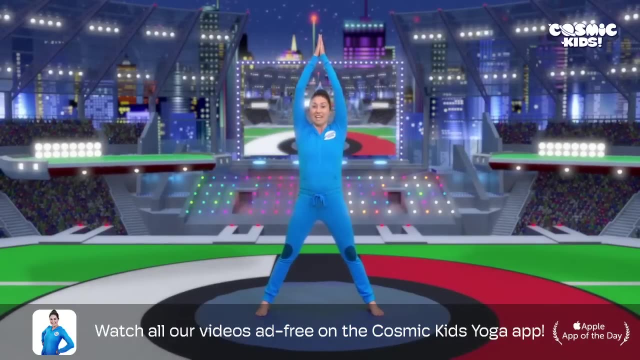 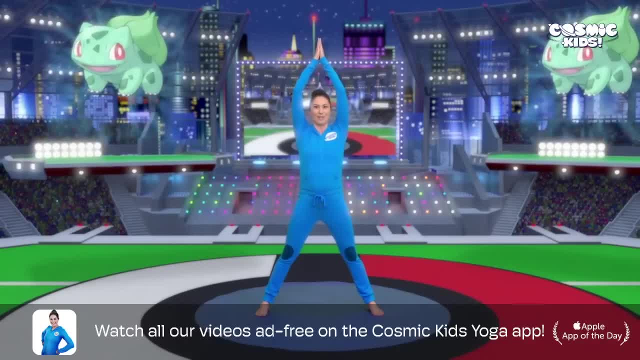 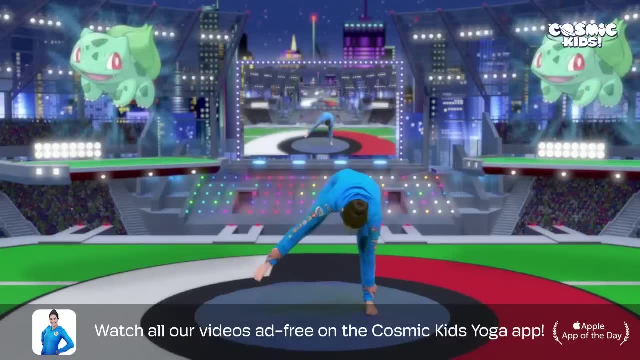 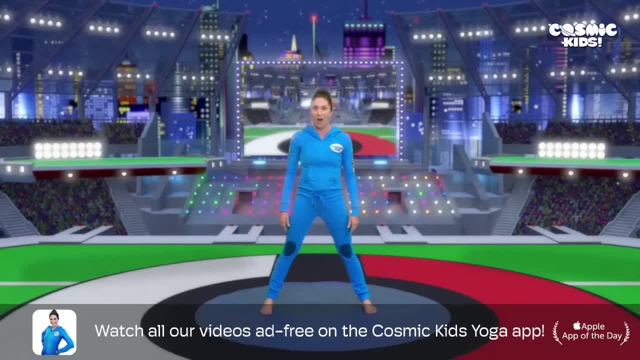 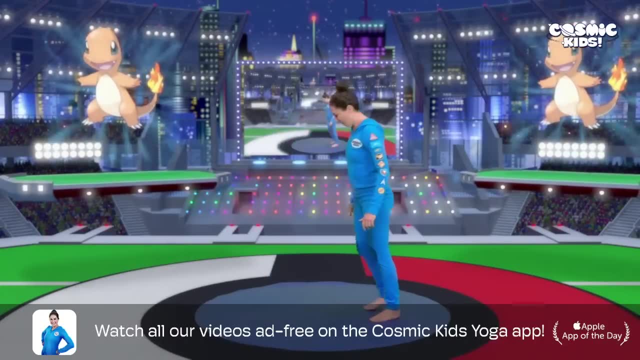 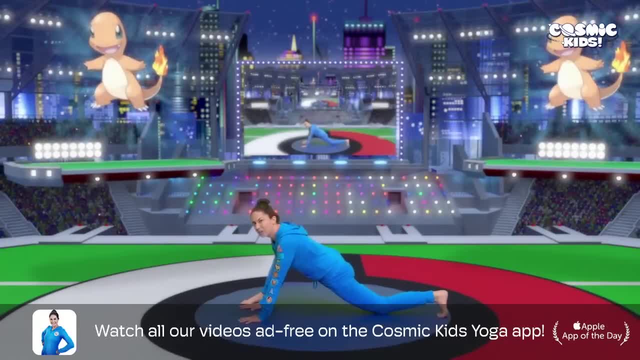 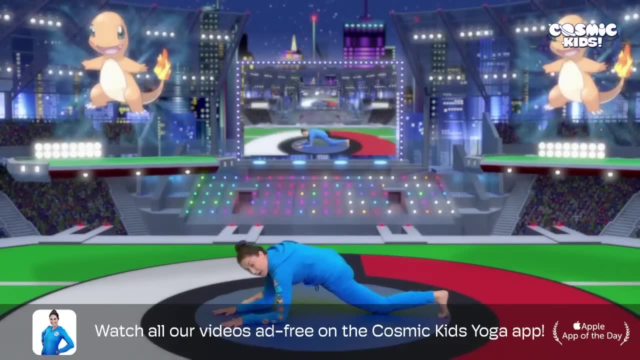 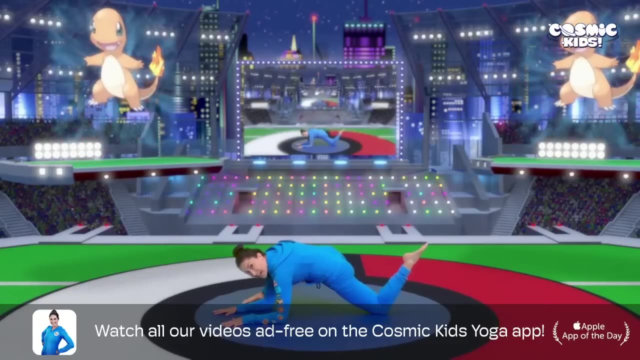 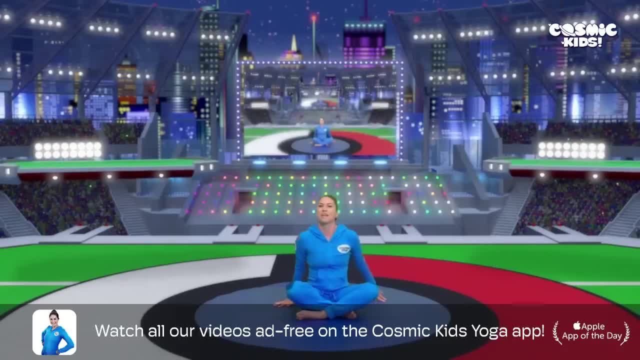 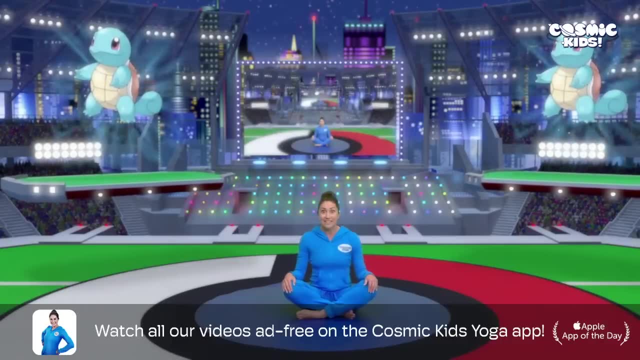 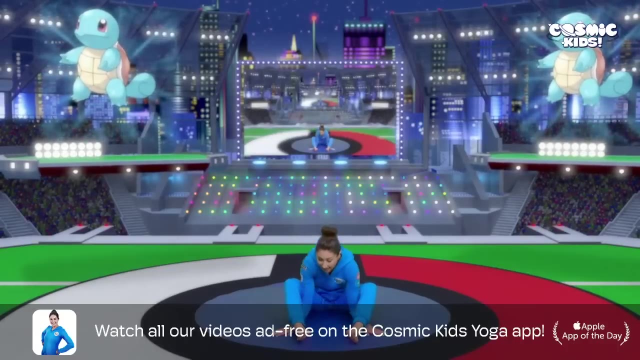 Coming back to sit with our legs crossed. Our third choice of starter Pokemon is Squirtle, a turtle-like Pokemon Coming into turtle pose, Taking our feet out in front of us. we keep our knees bent. We put our hands down and slide them underneath our legs like two little turtle flippers. 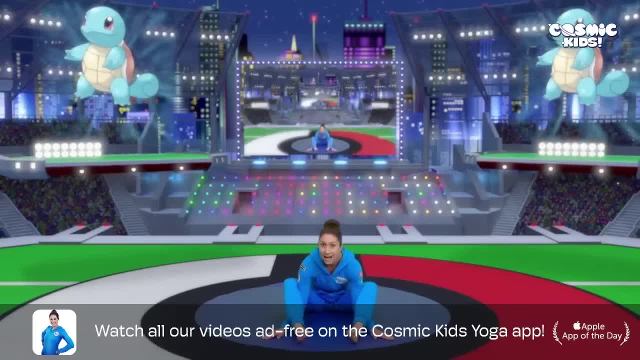 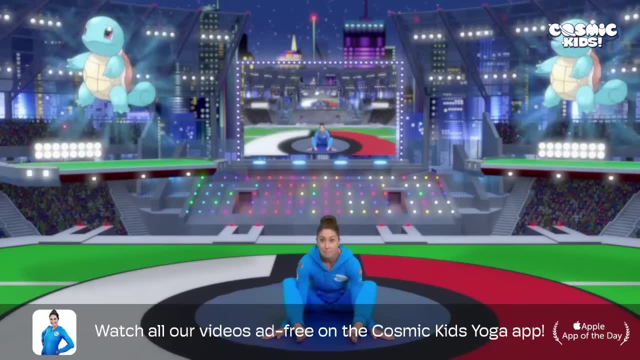 Squirtle can go very fast through the water thanks to its shell, And it can blast water from its mouth. Let's have a try by breathing in through our nose and blowing out of our mouth. Wow, We've soaked everything For our adventure. today, we decide to choose Squirtle. 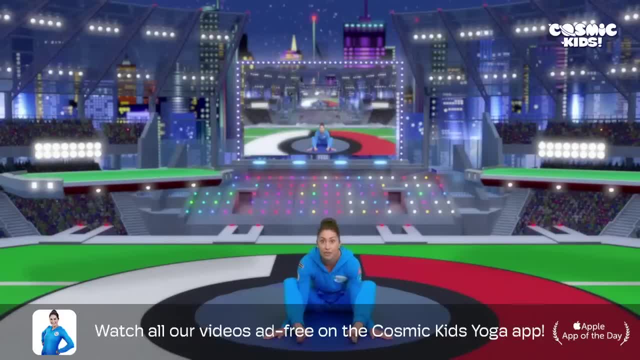 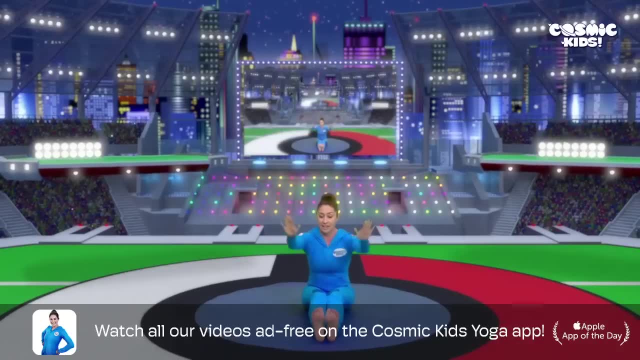 as our starter Pokemon. Now it's time to pack a bag with all the things we need to be Pokemon trainers. Sitting with our legs out long in front of us, we bend our knees a little bit to touch our toes. Now we open up our bag by lifting our arms. 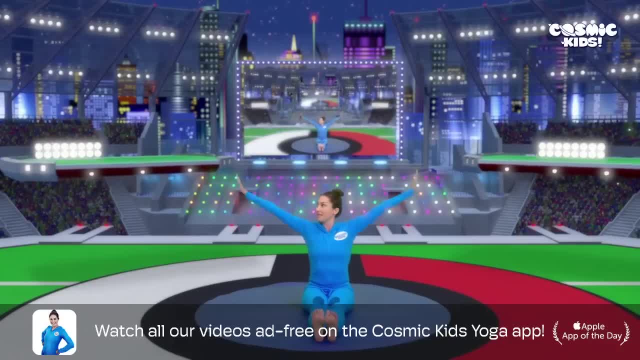 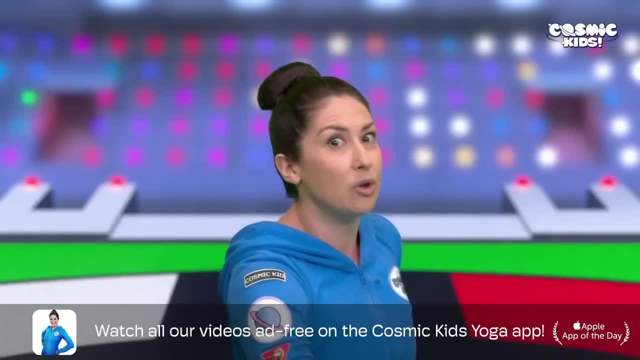 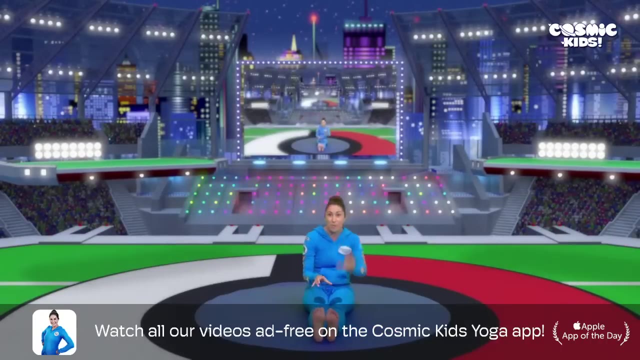 Here we go, We take our arms out nice and wide and we twist one way to get some Pokeballs. We need Pokeballs to catch all the Pokemon. when we find them, Here we go, Let's put them in the bag. Pokeballs, Pokeballs, Pokeballs, Pokeballs. 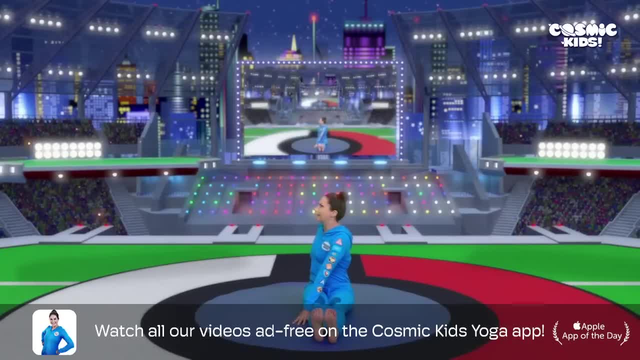 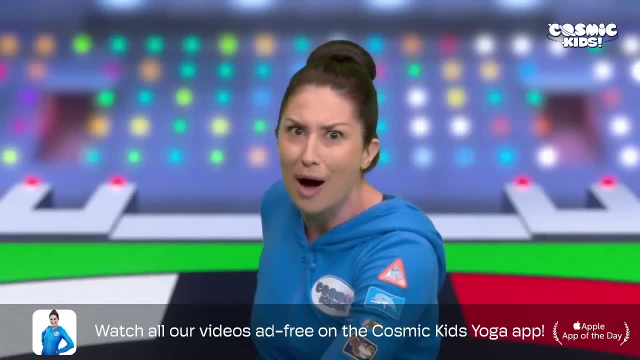 Arms out wide again, We twist to the other side to get a Pokeflute. We need a Pokeflute. if we find any sleepy Pokemon and need to wake them up, Let's put it in the bag. Here we go: Pokeflute, Pokeflute, Pokeflute, Pokeflute. 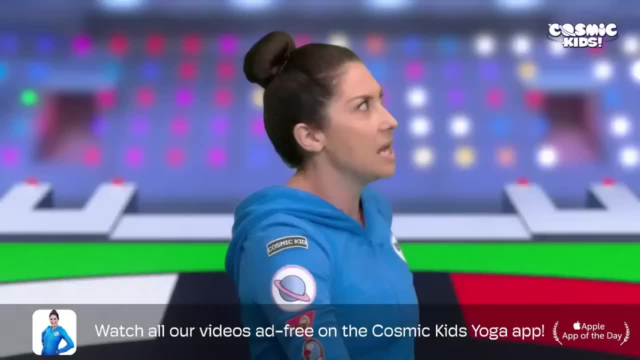 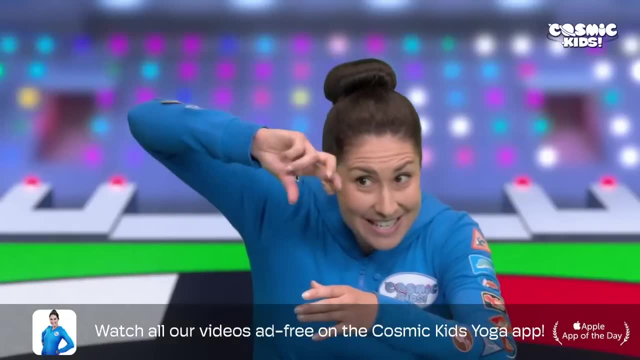 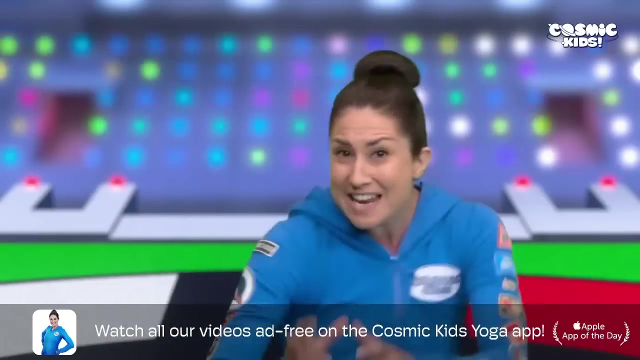 Arms out wide again, We twist to the back and we get some Lemonade, Very good for restoring our health. Here's the Lemonade. Let's check the lids on And put it in the bag: Lemonade, Lemonade. We love lovely Lemonade. 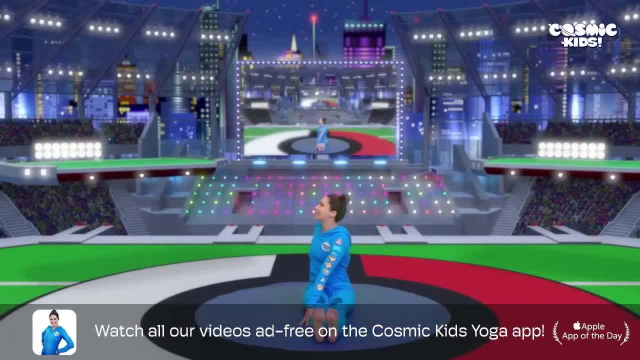 Arms out wide again. We twist to the other side and we get some Nuggets, Honey and Berries. Very useful. Here we go, Let's put them in the bag. Nuggets, Honey and Berries. Nuggets, Honey and Berries. 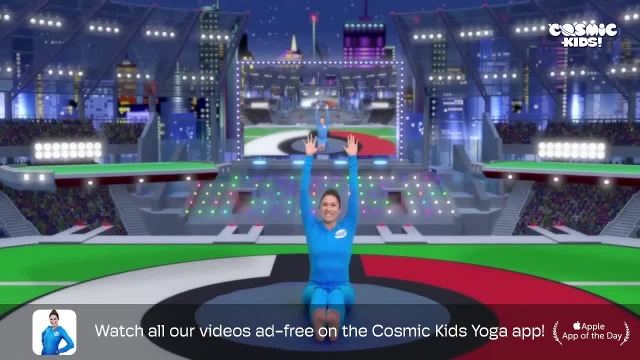 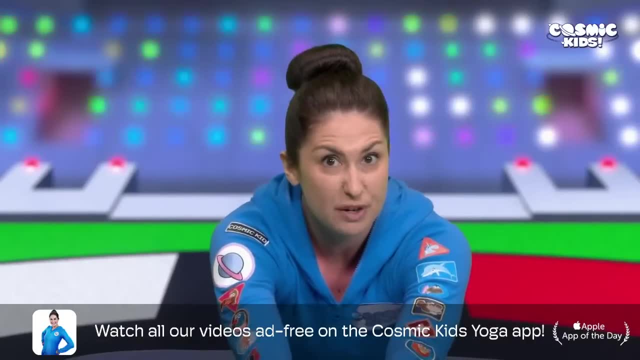 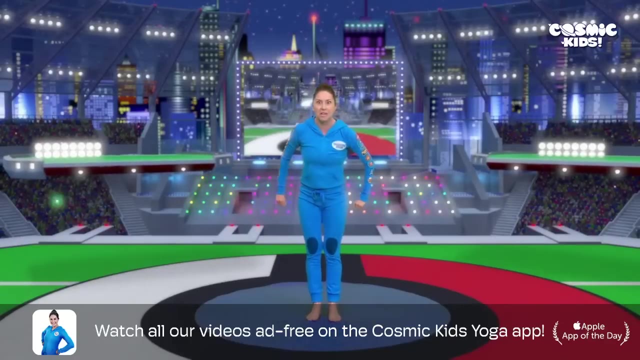 Lifting our arms all the way up, we bend our knees And we close our bag. Now our first stop is the Viridian Forest, which is a maze of trees. Let's come up to stand and do our tree pose, Bringing one foot on top of the other. we use our heel and we bring our hands together at our hearts. 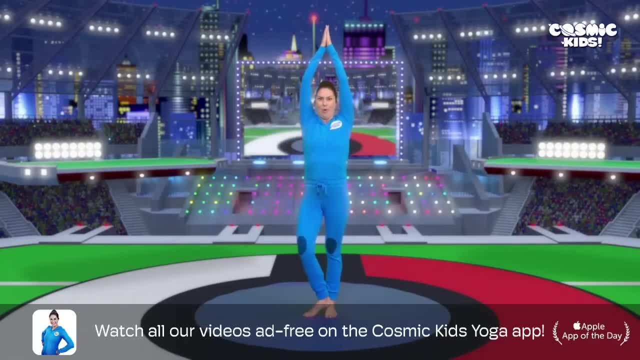 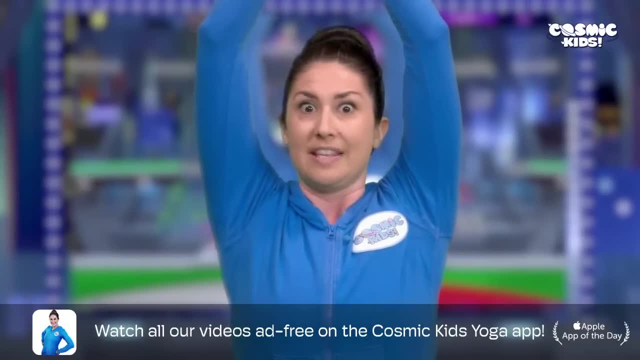 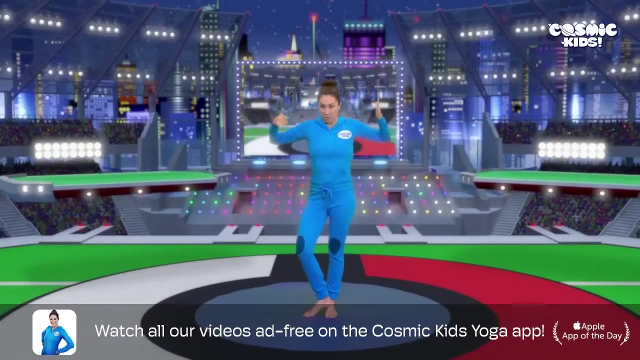 We grow our tree up, nice and tall. Oh, very good, everyone. Now we need to make these trees into honey trees By covering them in honey. This way we can attract hungry Pokemon. So let's take that honey and slather it all over our trunks while we stay in our tree pose. 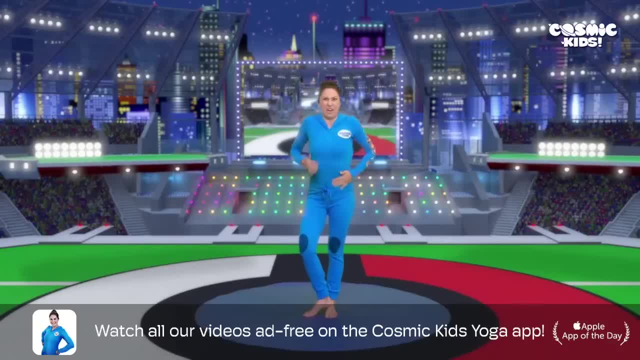 Try not to wobble. Rub it on our trunks, On the front and the back All the way down our legs A bit wobbly, And on our arms. We're doing very well, But we're very sticky now. 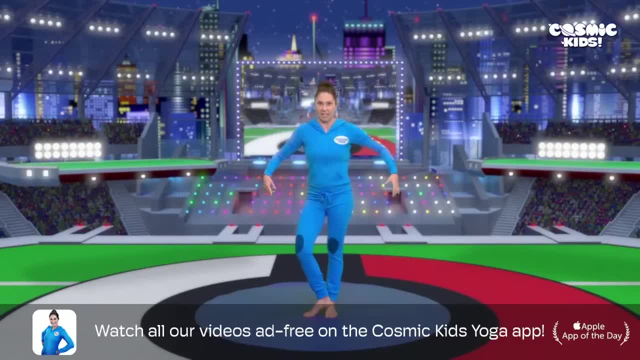 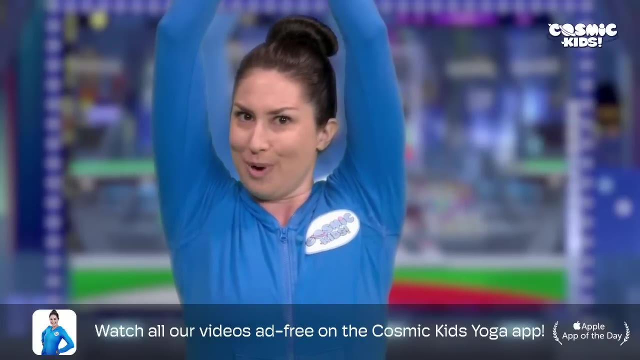 Let's try and do our tree pose on the other side. See if you can unstick your foot Yuck. And let's put the other one on Hands together. Grow up tall Now I wonder how strong are you? honey trees today. 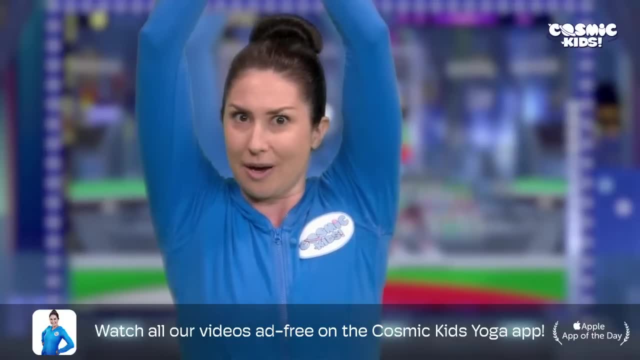 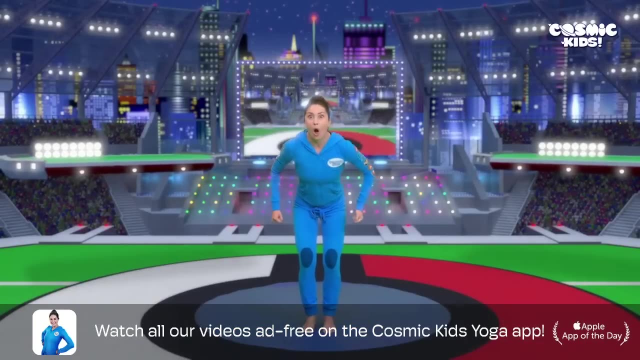 Let me see You stay tall and strong and I'm going to come and try and blow you down. Here I come. Oh my goodness, You are super strong. today Must be all that honey. Now it might be a bit of a wait before we get a hungry Pokemon. 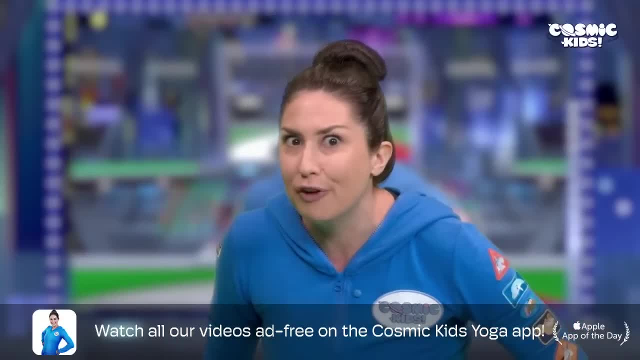 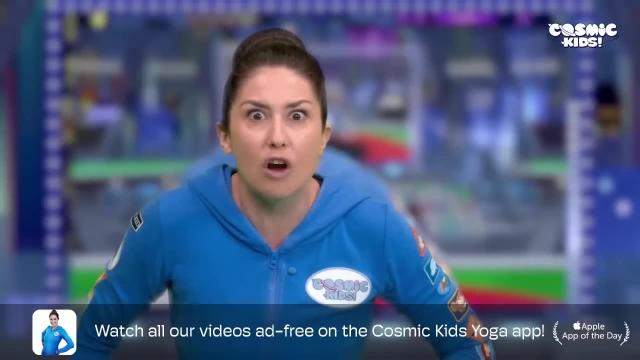 So let's tiptoe away and see what else we can find. And we go, tiptoe, tiptoe, tiptoe, tiptoe. We come to some long grass. This is a great spot for finding wild Pokemon. 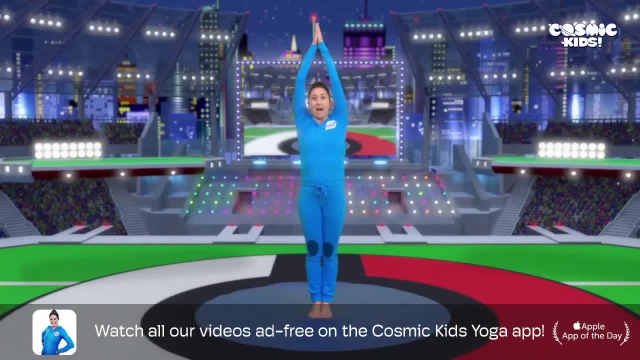 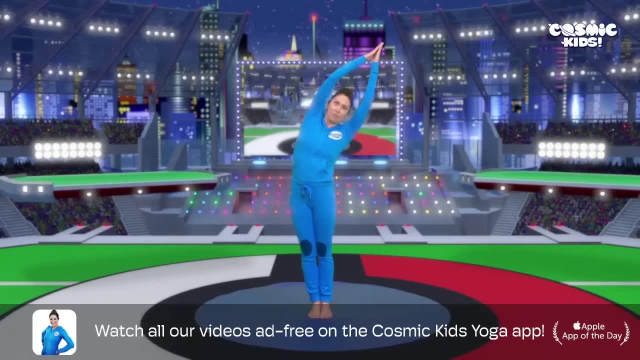 Bringing our feet together, We reach our arms up above our head And we lean over one way like a blade of grass, And over the other way like a blade of grass Or a banana. Look In the grass: we spot a wild Pikachu. 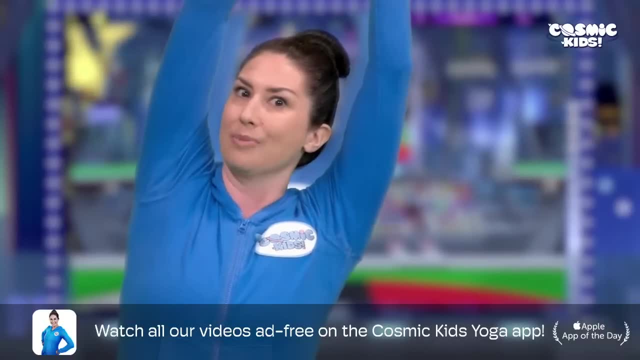 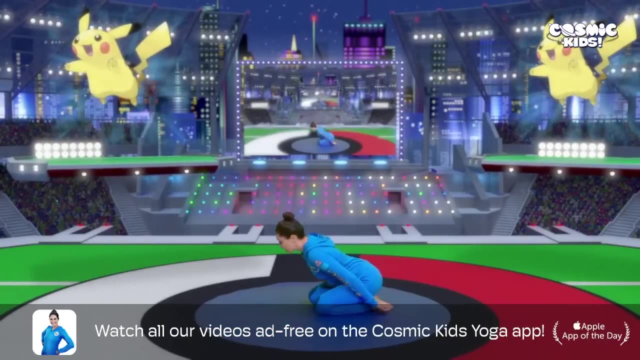 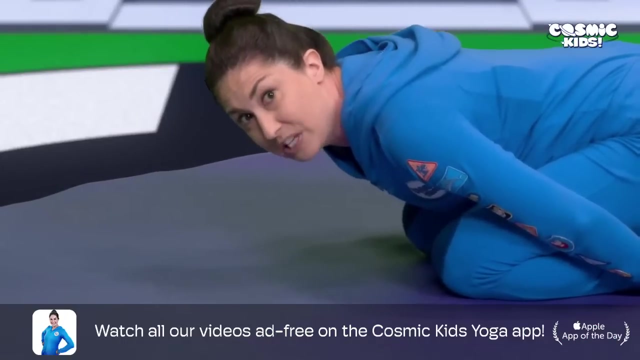 Pikachu is a yellow mouse type Pokemon Coming into mouse pose, Down onto our knees. We fold our body all the way forward as we say Pikachu. We need to hold Pikachu in place, So we use our squirtle and its rain dance move. 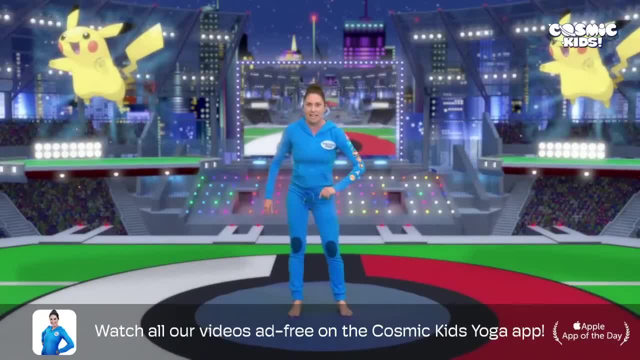 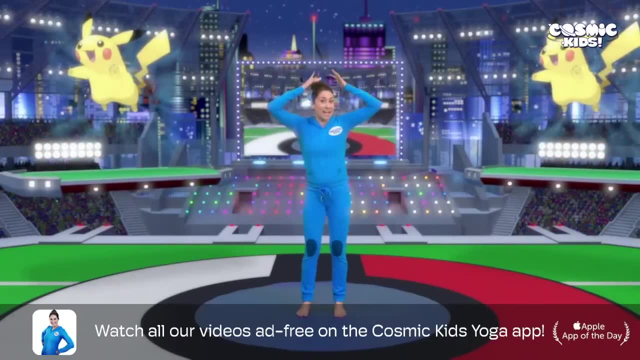 Coming up to stand, Let's do our rain dance move, Using our fingers to pitter patter, Here we go: Rain, rain, rain on my head, head, head, Rain, rain, rain on my face, face, face. 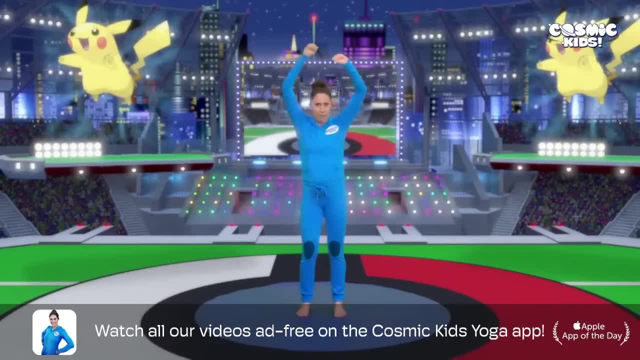 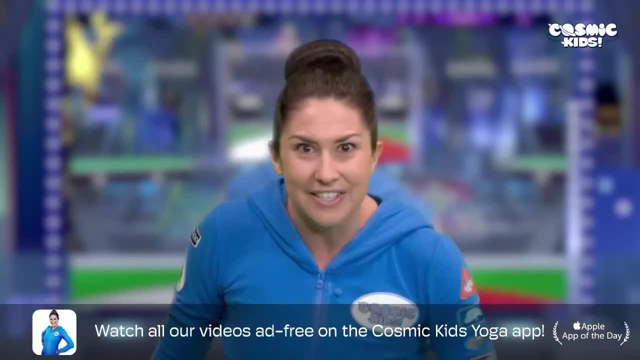 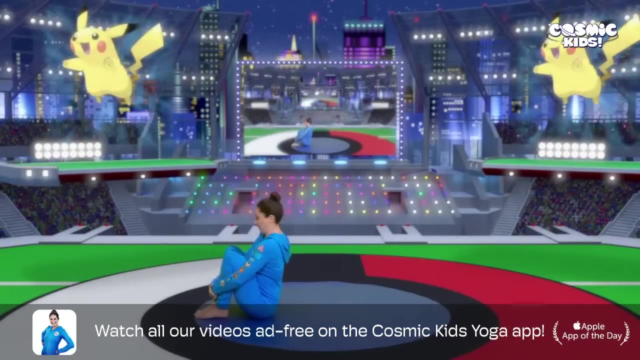 Rain, rain, rain on my bum, bum, bum, Raining all day long. Yes, It worked. Pikachu is stunned. Time to roll a Pokeball and catch it Sitting on our bottoms. We hug our knees in tight. We tuck our chin like we're squashing a tomato. 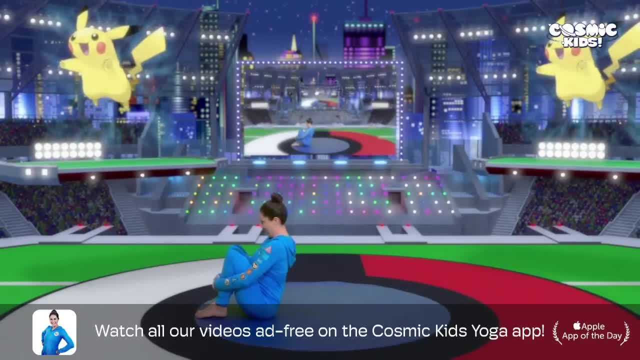 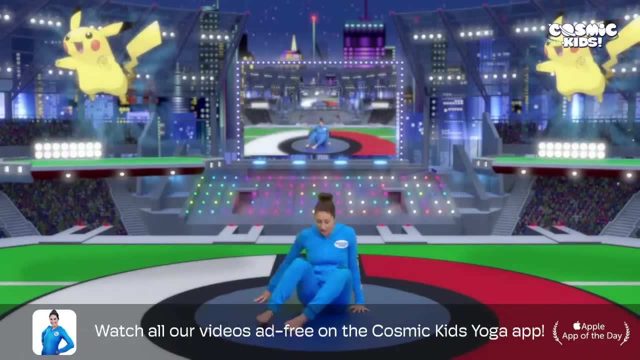 And then we rock all the way back and all the way up, Ready After three, One, Two, Three, Whoop, Woo. We sit up nice and tall With our legs crossed. Bring one hand to our tummy, One hand to our back. 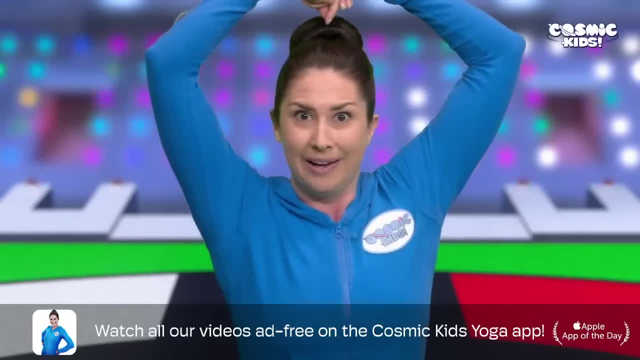 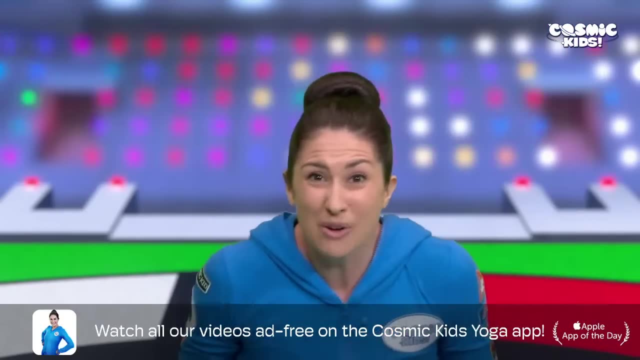 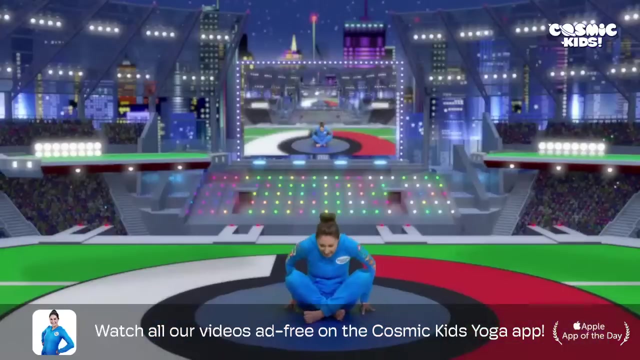 We zip ourselves up And we give a silent celebrationary cheer to the sky. We caught our first Pokemon, Brilliant. Now I wonder if our honey trees have worked. Let's tiptoe back into the forest. We come to stand. 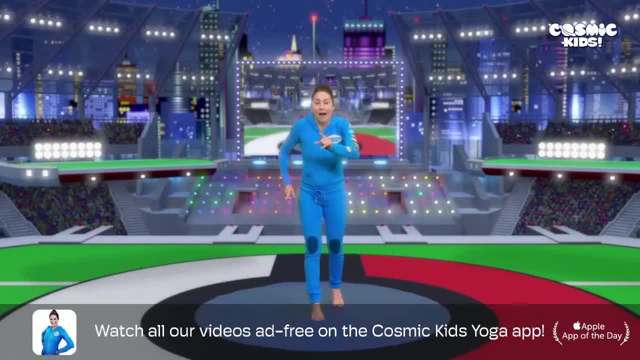 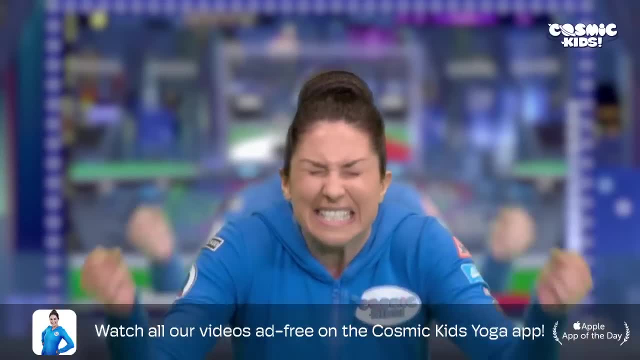 Shh Shh Shh. There At the bottom of the honey tree is a sleepy snoozy, snorey Snorlax. Now we need to wake this Snorlax up using our Pokeflute. 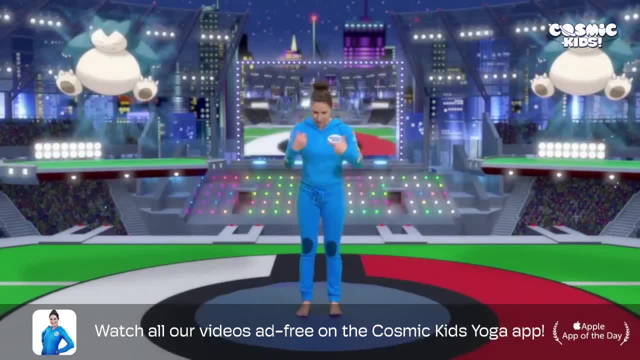 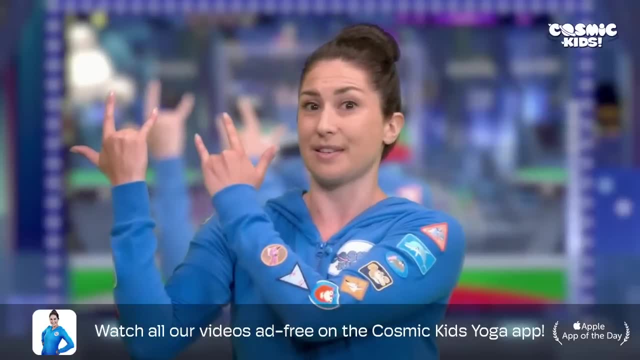 Let's do our Pokeflute pose, Standing with our hands up, Standing with our hands in front of us, We bring our third and fourth finger into our palms, We bring our hands up to the side of our face And we turn our outer hand round. 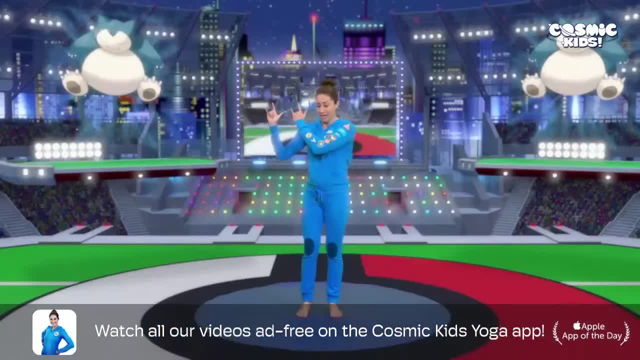 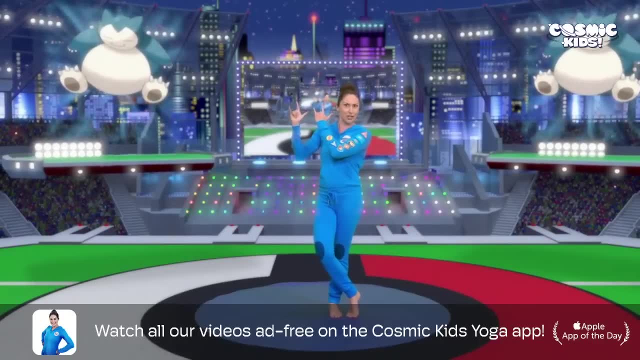 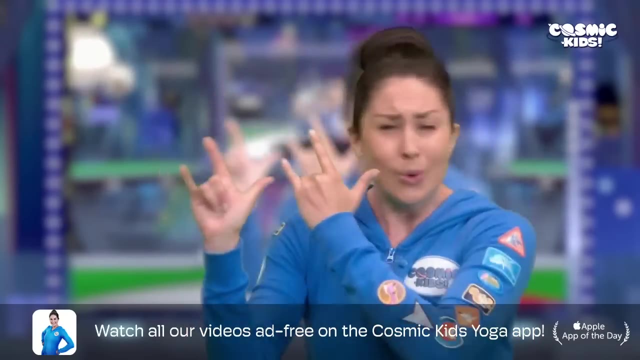 Now we're very good at playing the Pokeflute. So we cross one leg over the other And we balance on our toes. Yes, Now we play our Snorlax tune. Here we go, Let's try our Pokeflute pose on the other side. 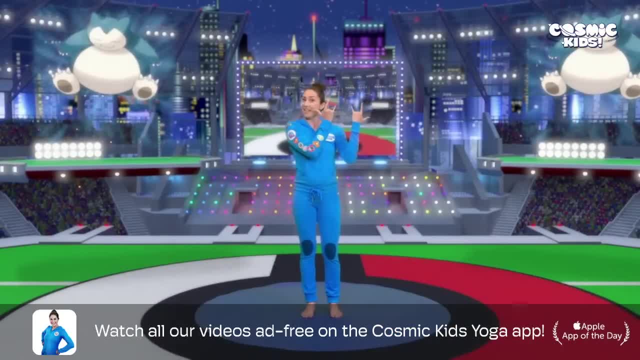 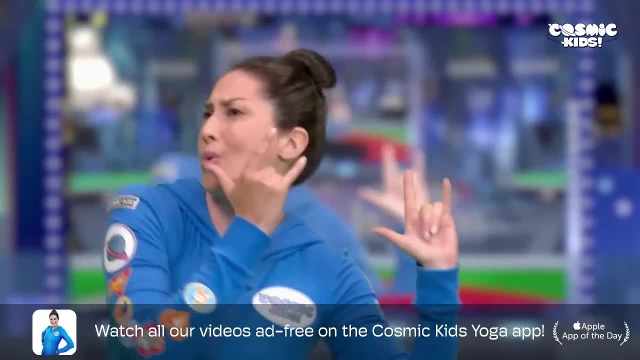 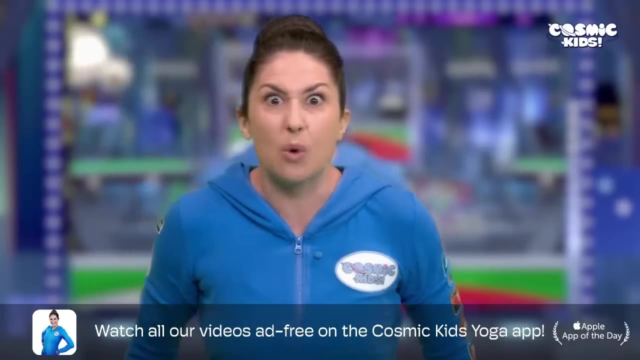 Uncrossing our legs. we bring our hands to the other side, Turning our outer hand round. We cross our other leg over now And play a little bit more. It's worked. The Snorlax is awake. Time to roll a Pokeball and catch it. 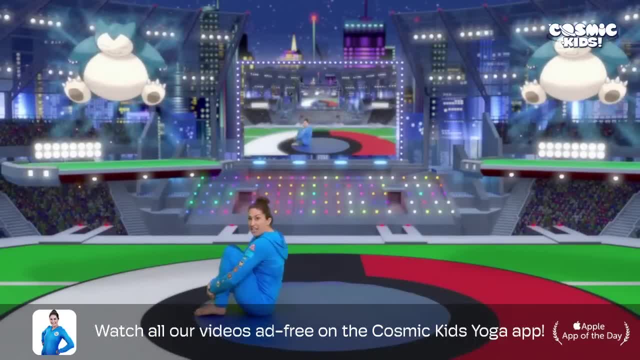 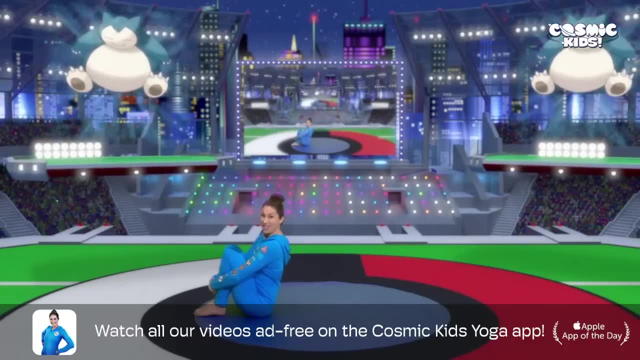 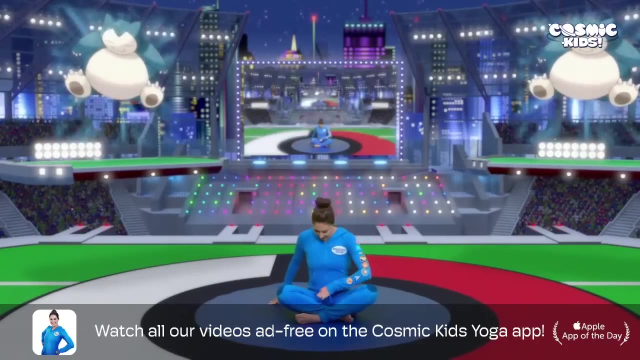 Sitting on our bottoms, Hugging our knees, Squashing a tomato. After three, let's rock all the way back and all the way up. One, Two, Three. We sit up tall with our legs crossed, One hand to our tummy. 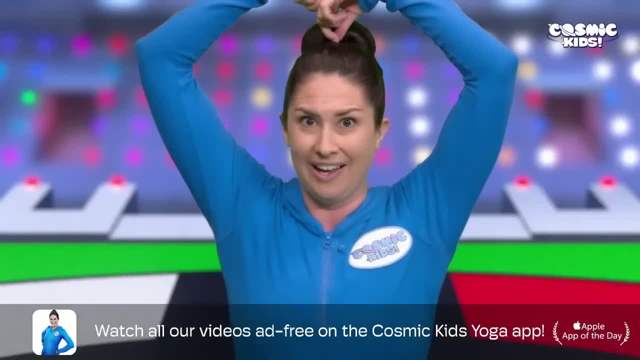 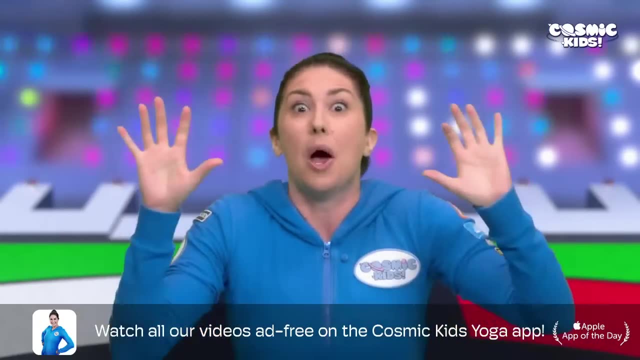 One hand to our back, Zip up nice and tall And a silent celebratory cheer to the sky. We've caught a Snorlax and a Pikachu. We're doing great, We're doing awfully well, We're on a roll. 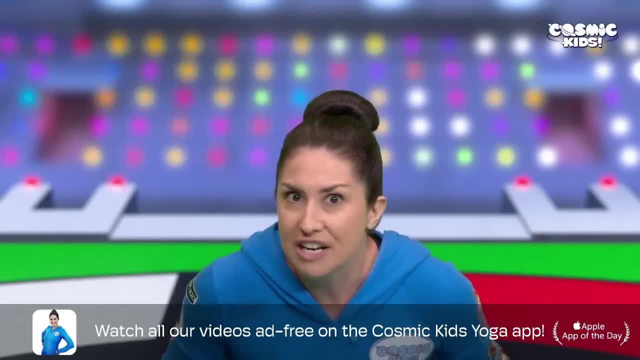 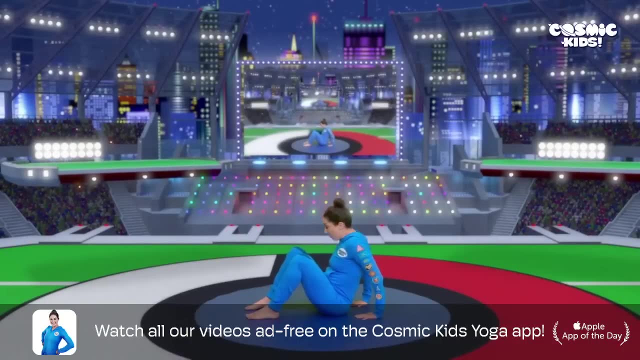 Let's go catch some more. We head over Nugget bridge Coming into our bridge pose Sitting on our bottoms, Knees bent, Feet, flat Hands behind us. We lift up our hips Coming into our bridge pose. Oh look. 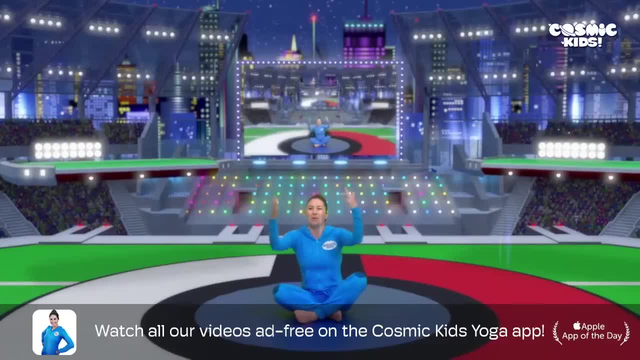 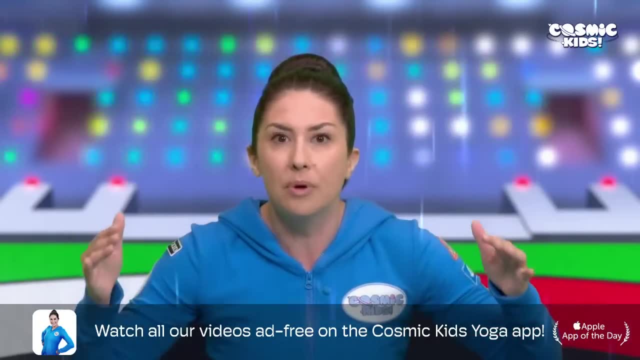 It's started to rain. Sitting with our legs crossed, We use our fingers to pitter-patter on our faces and our heads And- oh, look, On the bridge, all left by itself is a Pokemon. It's Charmander. 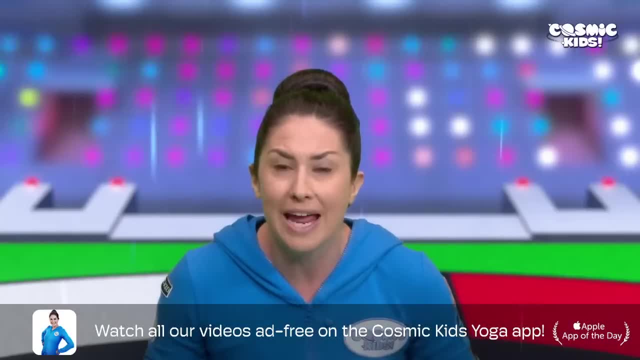 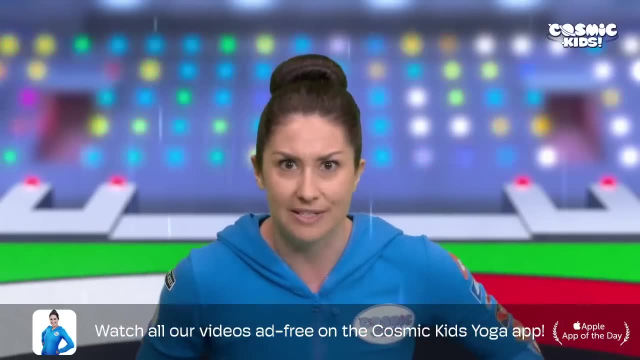 The lizard fire type Pokemon, Remember, with the flame. Oh, it doesn't do very well in the rain. Its flame has nearly gone out. We need to rescue it, So we take it into a cave. Coming into our cave, dog pose. 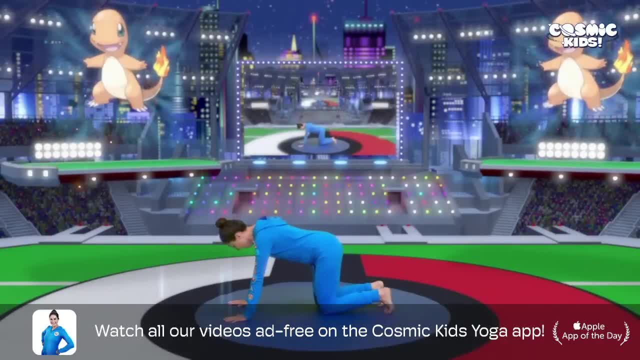 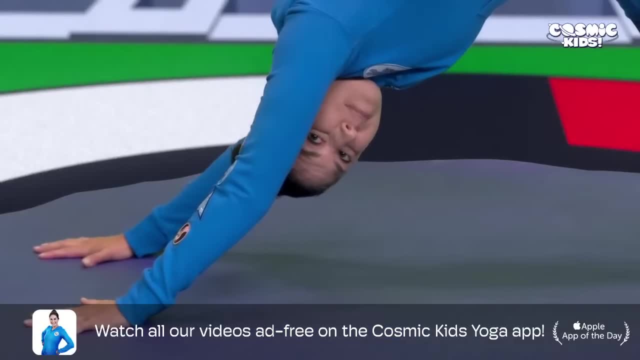 Onto our hands and knees, We tuck our toes and we press our hips up to the sky. Now let's mix up some medicine And help Charmander get better. Sitting on our bottoms, with our legs out wide, We take hold of one stirring stick. 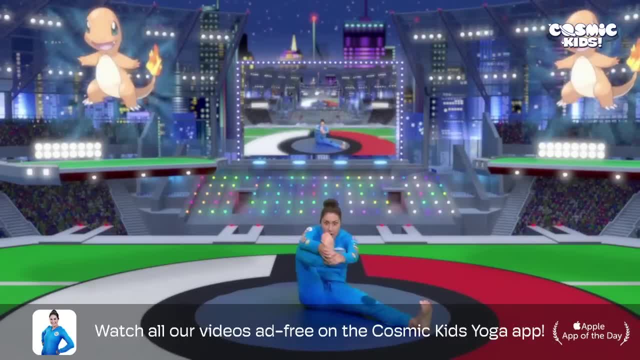 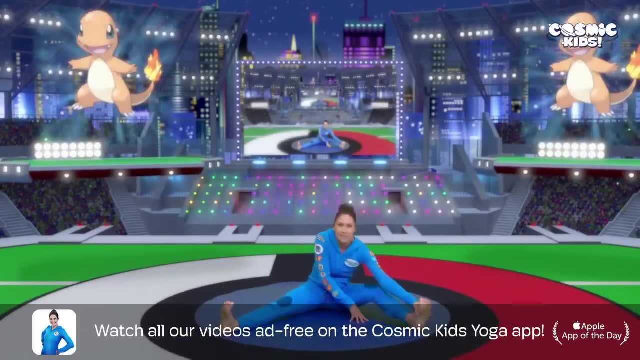 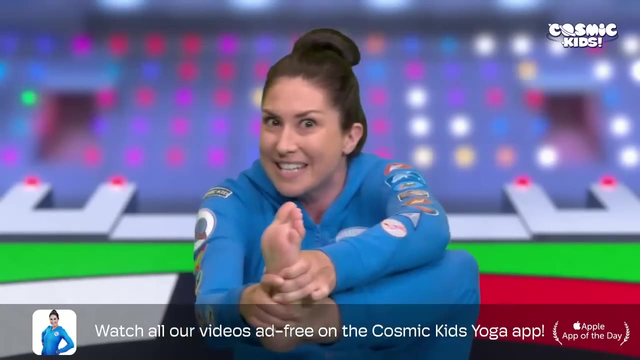 And we mix up the medicine, Stir it, stir it, stir it, Popping that, stirring, stick down. We lift up the other one And we stir it some more. Stir it, stir it, stir it, Pop it down. Now we need to rock this little Charmander to heaven. 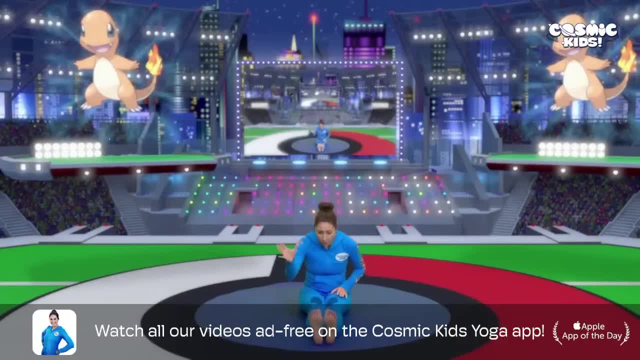 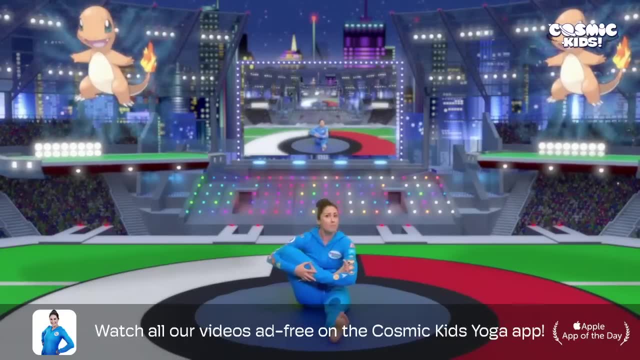 Bringing our feet in front of us. We pick it up And put it in the crook of our elbow And hold it, Cradling it. Rock the Charmander, Rock the Charmander. We put the little Charmander down. 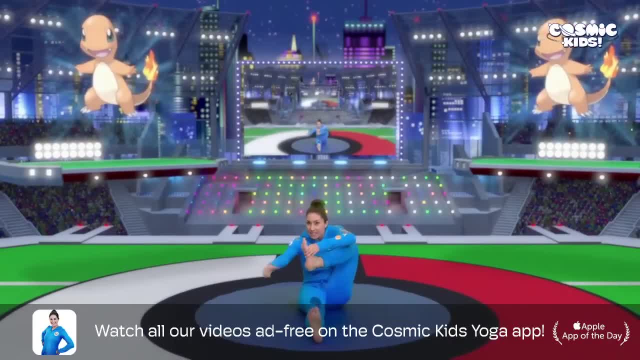 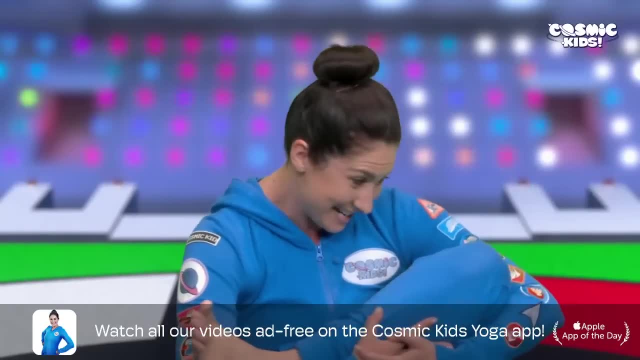 And we pick it up on the other side By putting it in the crook of our elbow, Wrapping it up, And we rock the Charmander, Rock the Charmander. It gets better. The flame has come back Ow. 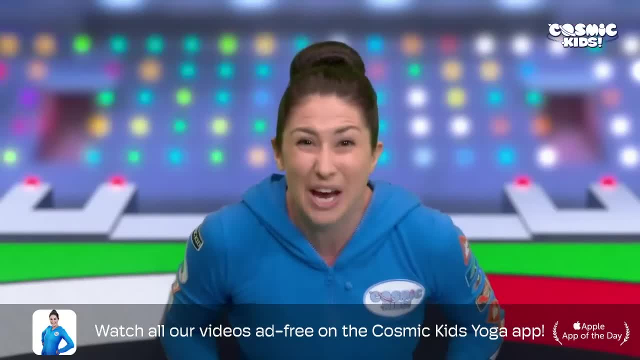 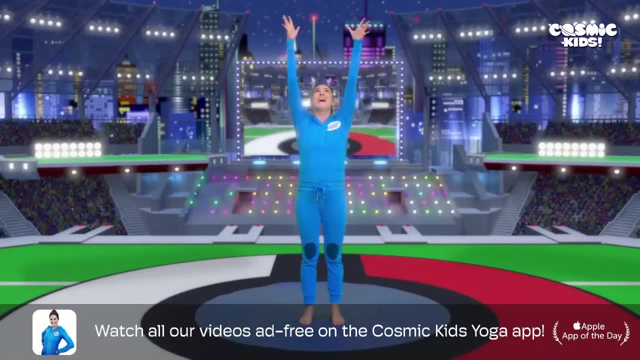 And it agrees to join our team. Woohoo, We're doing so well. And look, The sun's come out. So we come up to stand, We reach up to the sun, We wave at the sun And we say: 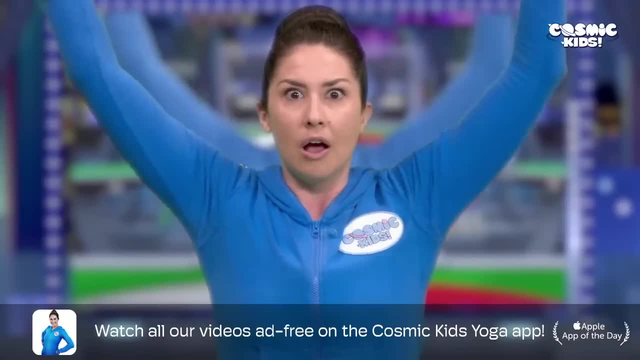 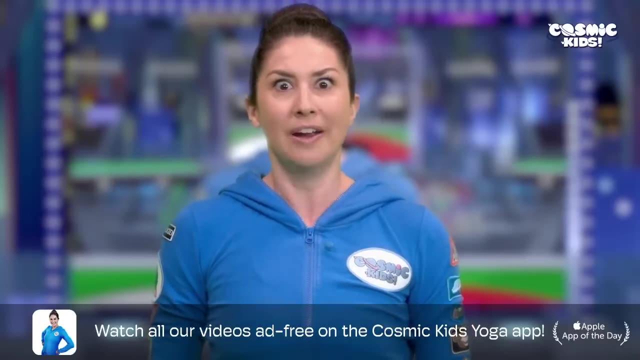 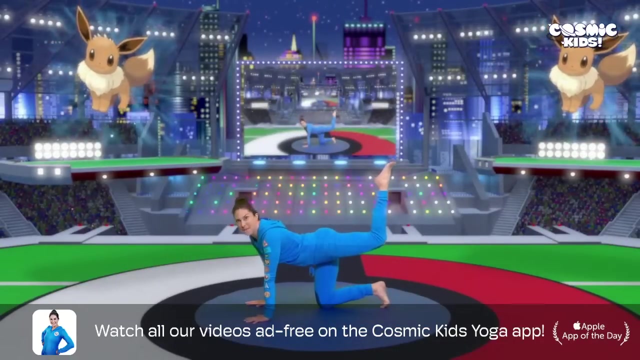 Hello sun. Look There On a ledge We spot an Eevee, A fox-like Pokemon Coming into our fox, pose Onto our hands and knees. We press one foot up to the sky Like a big, bushy fox tail. 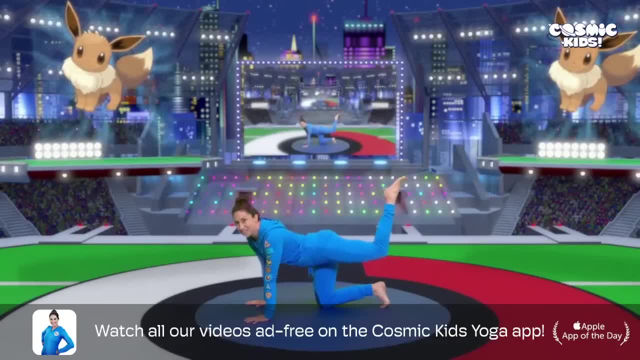 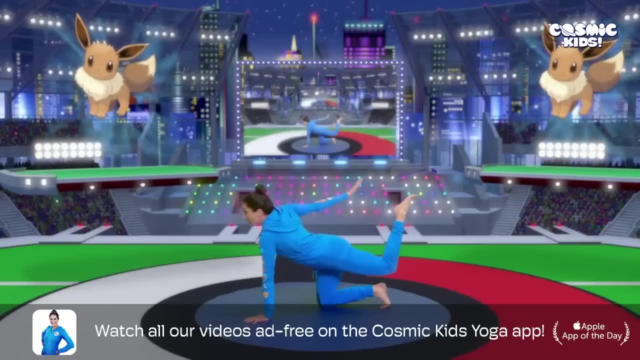 But look, Eevee is dancing. Let's do a dancing fox pose. We reach our opposite hand forward. Try not to wobble As we sweep it back behind us, To catch our foot behind us And kick our foot into our hand. 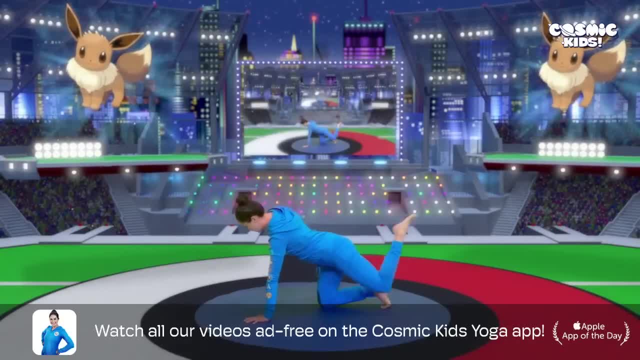 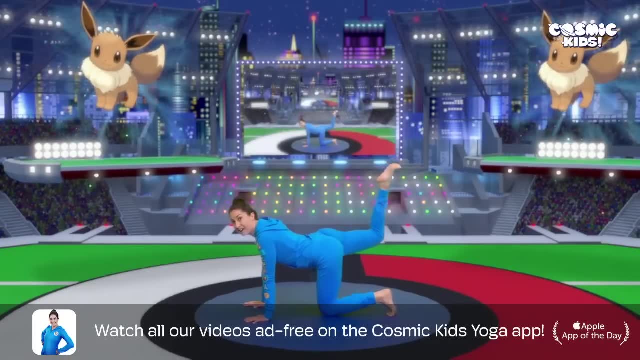 Coming into our dancing fox pose. We bring our hand and our knee back down And we try our dancing fox. on the other side. We press the other foot up to the sky, Reach forward with our arm, Try not to wobble. We sweep it round to catch our foot. 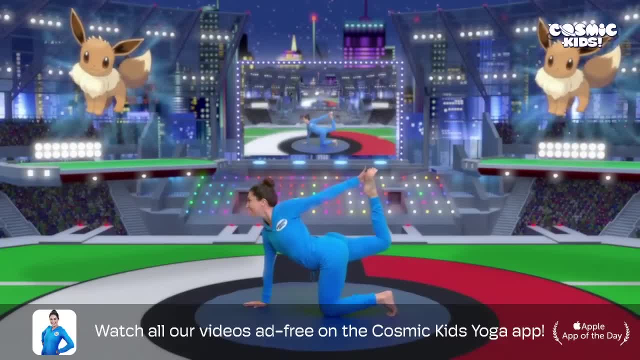 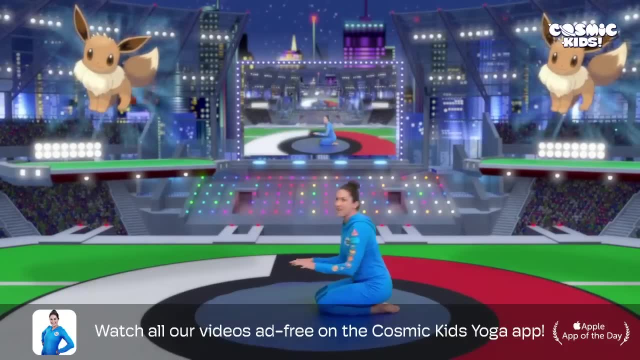 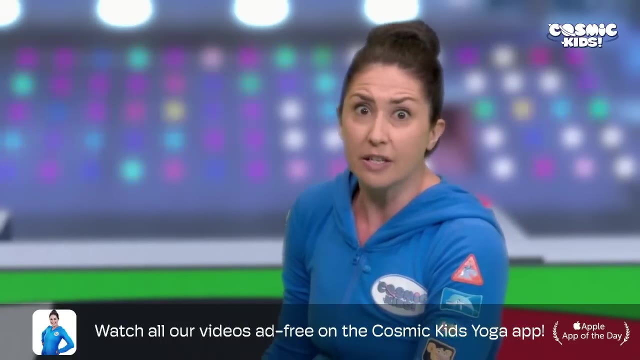 Kick our foot into our hand, Lift our chest up high. Yay, Dancing fox pose, Sitting all the way back on your heels. We would so love to catch an Eevee, But it sees us, It gets frightened And it runs away. 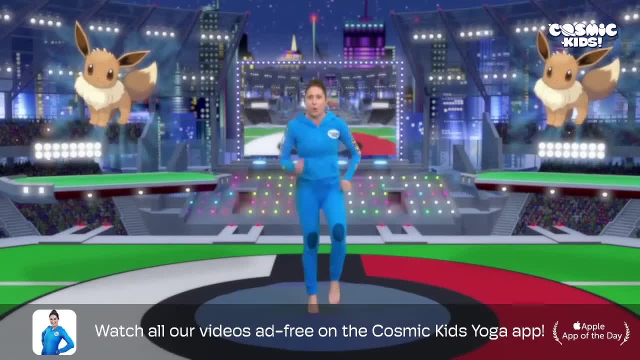 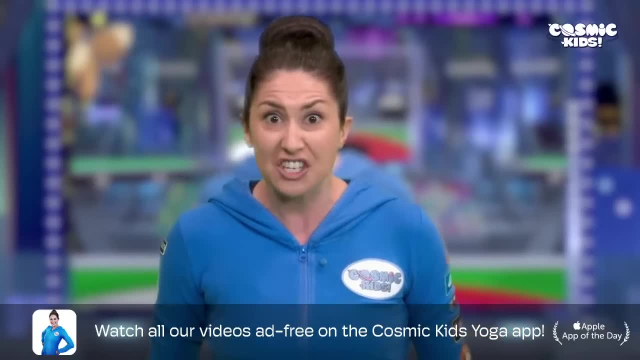 Coming up to stand. everyone We follow. We really want her. We really want to find it Just in time to see Team Rocket. The bad guys Catch Eevee in a net. Jump your feet wide, Arms wide- Oh no. 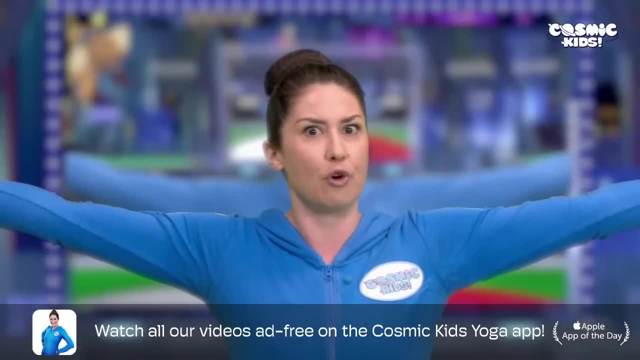 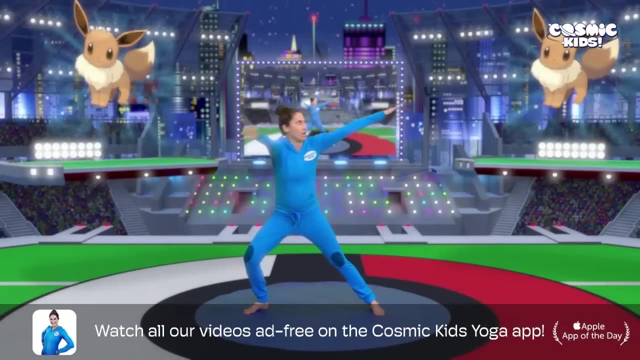 We need to rescue her. There's only one thing for it. We use our Pikachu And it's thunderbolt move. Bending into one of your knees, We sweep our arms up to the sky, We draw our top elbow down And we shade our eyes from the thunderbolt power. 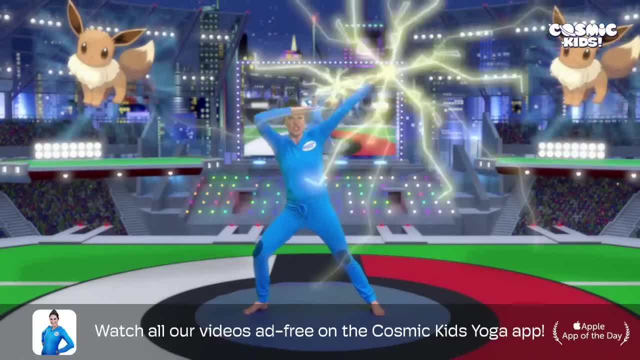 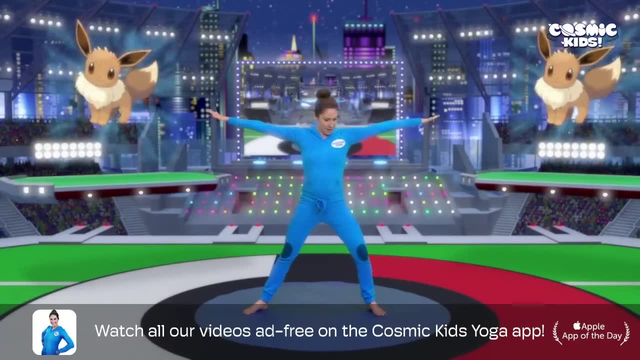 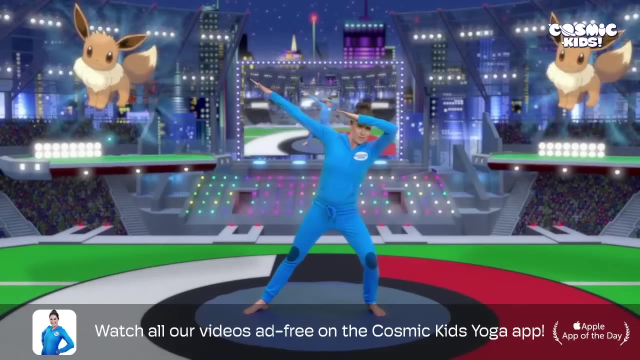 As we say, Pikachu, Let's do it on the other side, Arms out wide, Bending into the other knee, Sweeping your arms up to the sky, Drawing your elbow all the way back, Shading those eyes from the thunderbolt power. 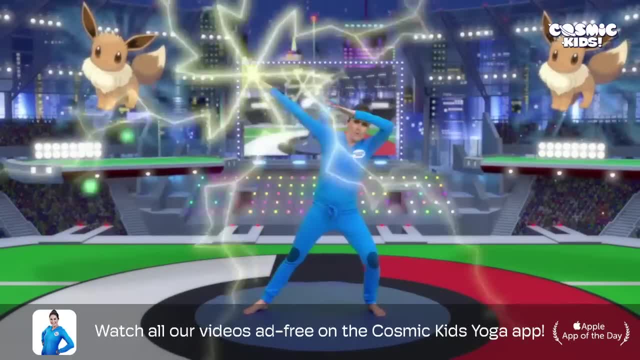 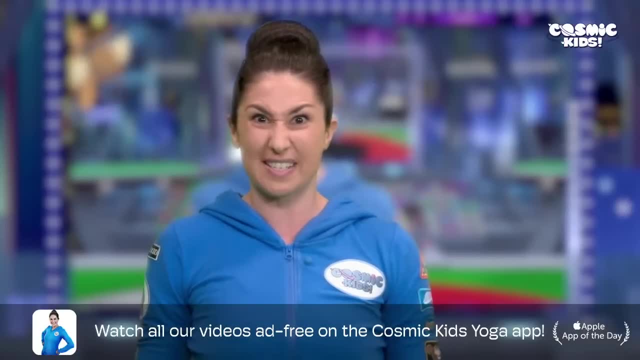 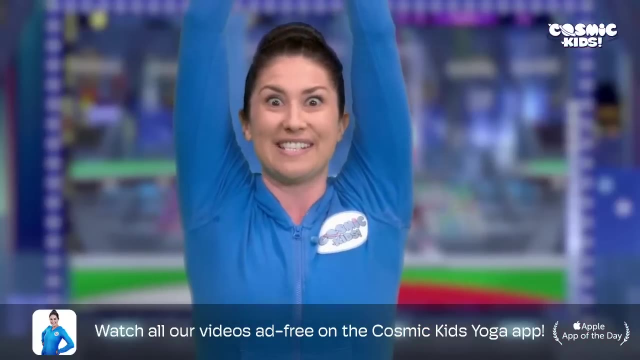 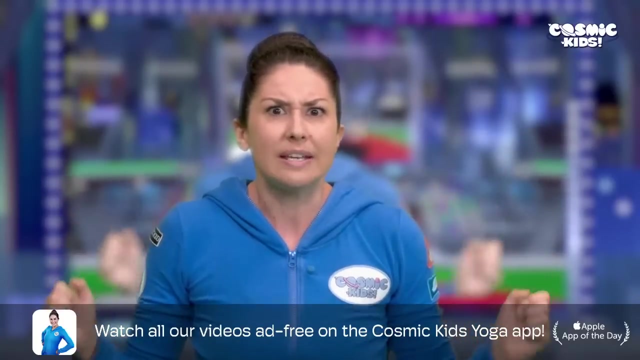 Pikachu, It's worked And Team Rocket blast off into the sky, Reaching your arms all the way up. And whoosh, Eevee is now free And agrees to join our team. Woohoo, Oh, We can see something. 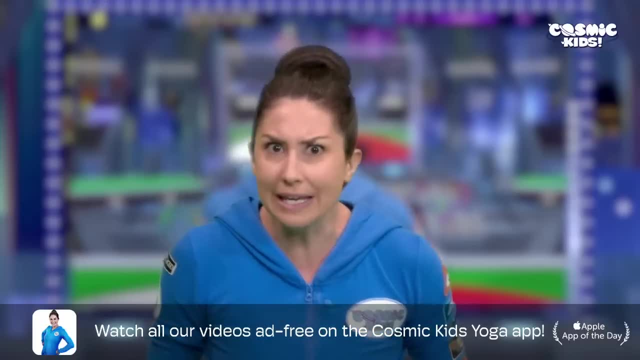 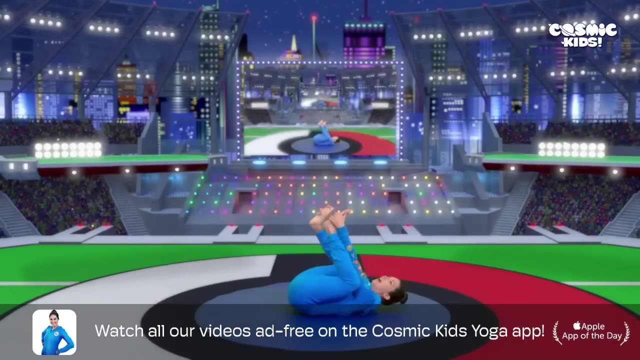 Jiggling And wriggling And giggling In the long grass. Coming down to lie on our backs, We hold onto our feet In our happy baby pose, Wriggling And jiggling And giggling. 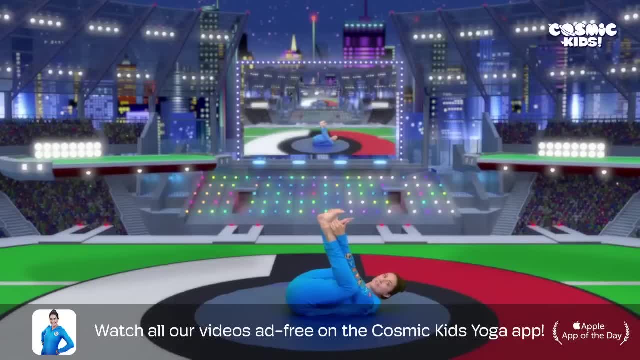 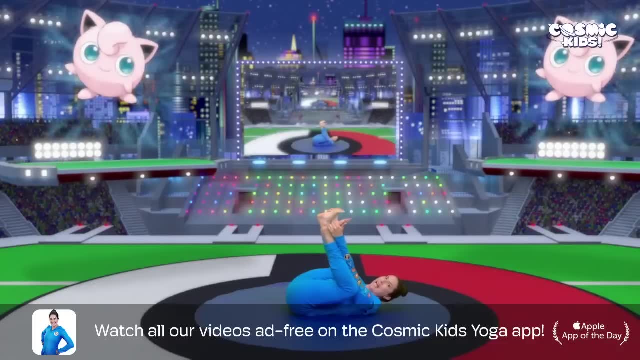 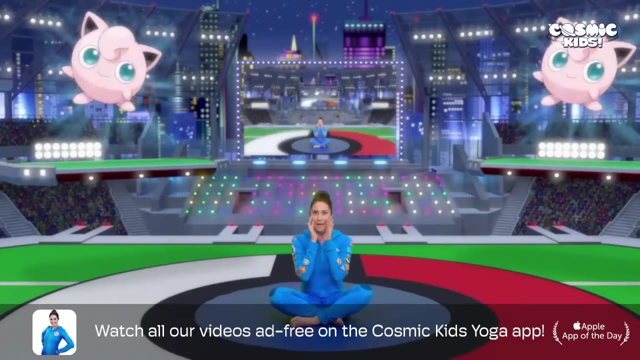 Hee, Look, We've spotted it: It's a Jigglypuff. A Jigglypuff is a balloon-like Pokemon And it's pink, Filled with air, Sitting up. We cross our legs, We cup our hands around our mouth. 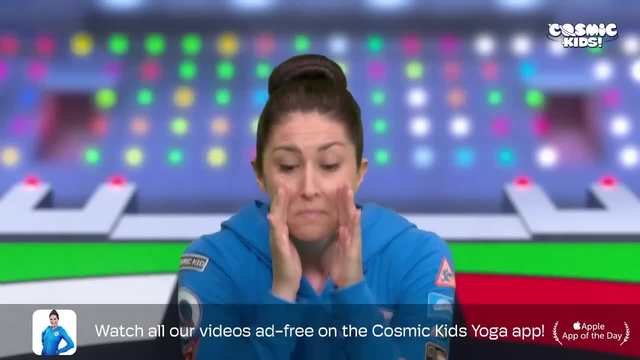 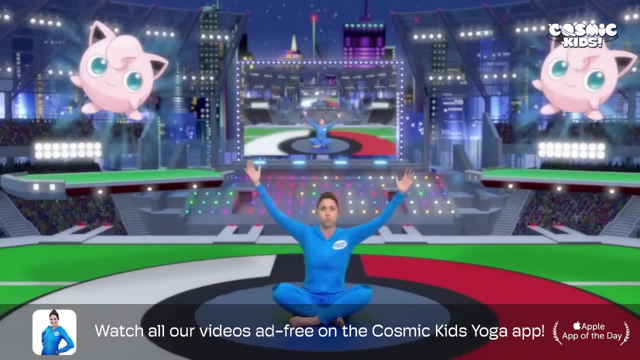 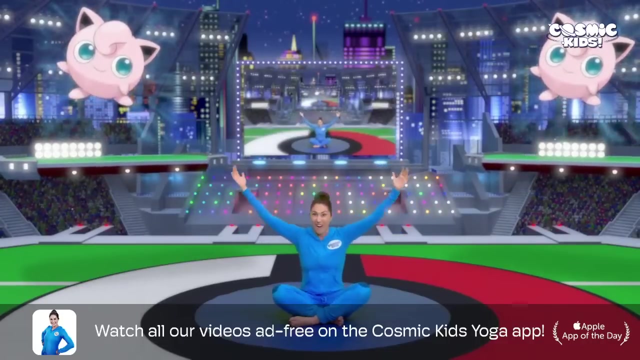 And we blow up our Jigglypuff Ready, Breathing in, And blow Woo, Wee, Wewe, wewe, wee Aa. Jigglypuff has the most enormous eyes, Which it uses to mesmerise its opponents. 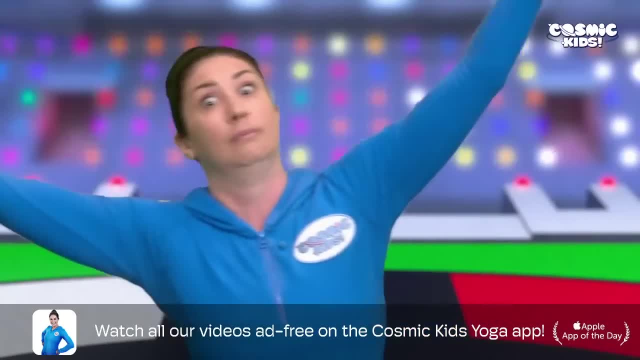 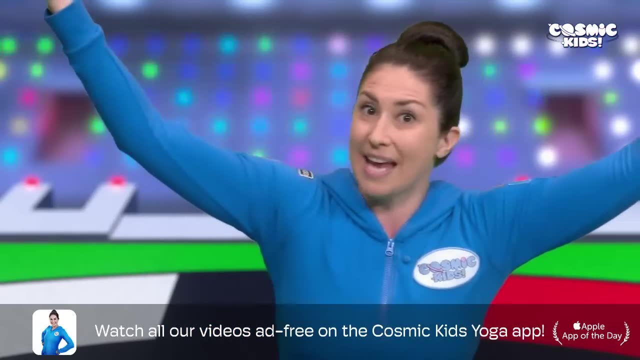 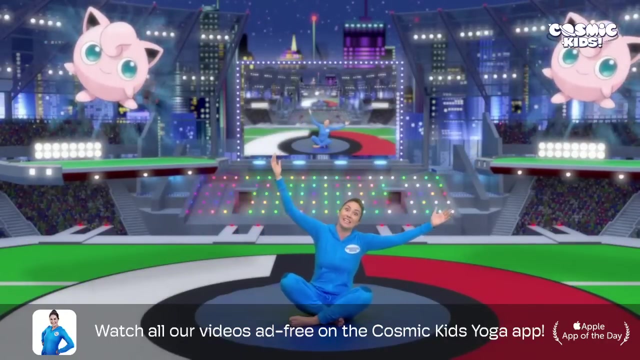 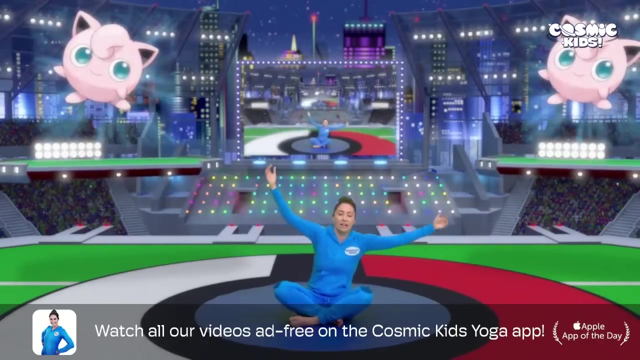 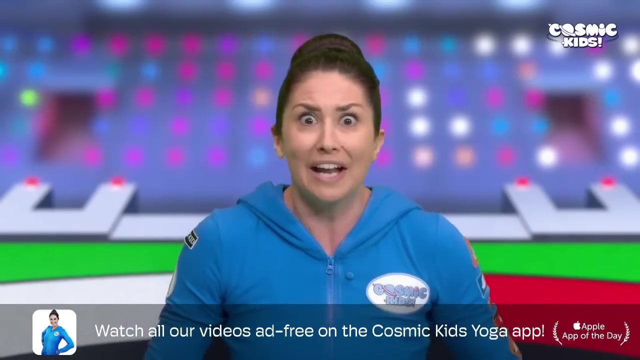 Let's see how big we can make our eyes. Very good, everyone, Your eyes are huge. It also uses a lullaby To send its opponents to sleep: Jigglypuff, Jigglypuff, Oh, we can't go to sleep. we can't go to sleep. we need to roll a poke ball and catch it sitting. 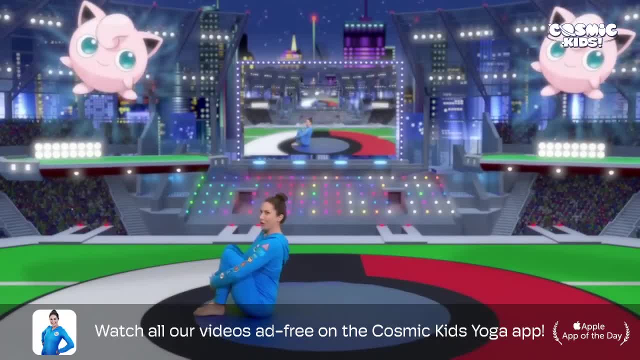 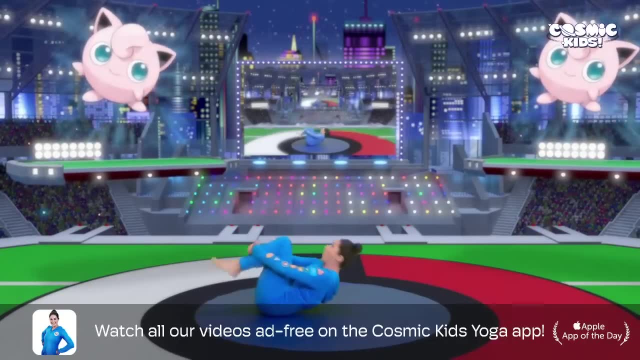 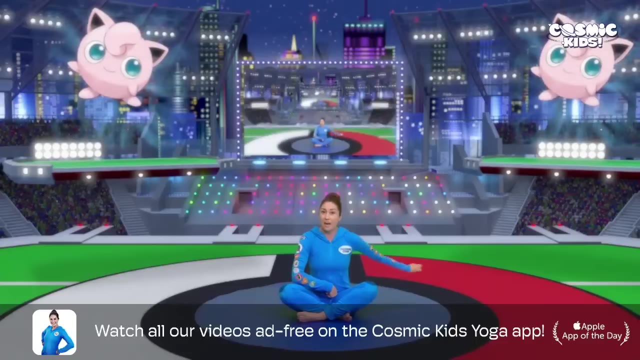 up, nice and tall, we hug our knees, we tuck our chin and we rock all the way back and all the way up. here we go after three, one, two, three. we cross our legs, we zip up our poke ball- hand to our tummy, hand to our back, and a silent 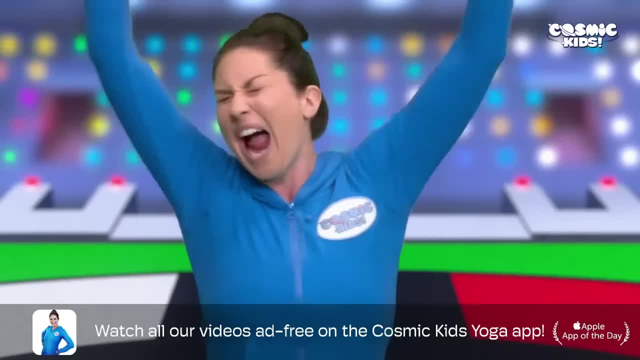 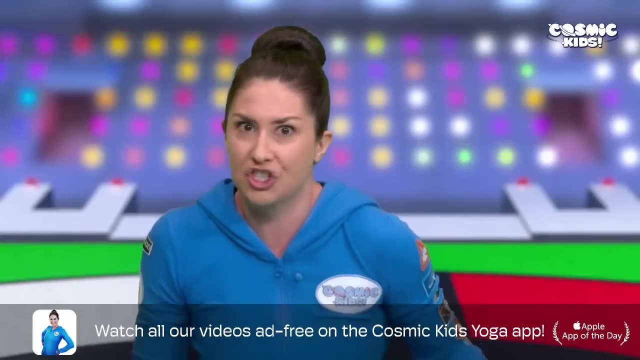 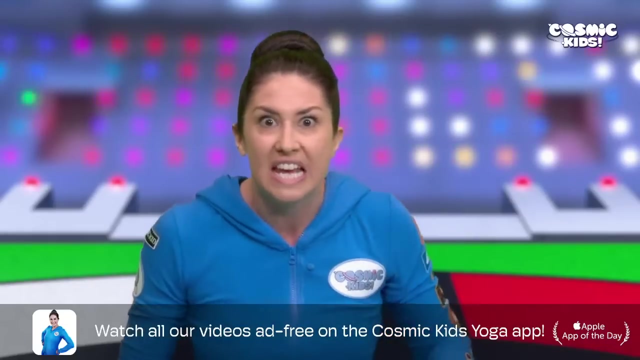 celebratory cheer to the sky. we're doing so well collecting all of these amazing Pokemon. we're nearly ready for our first gym at the pewter city. we're on our way there and just outside the city we find ourselves in a secret house. coming into house. 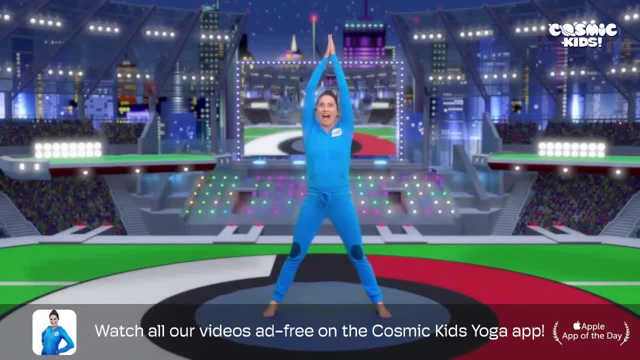 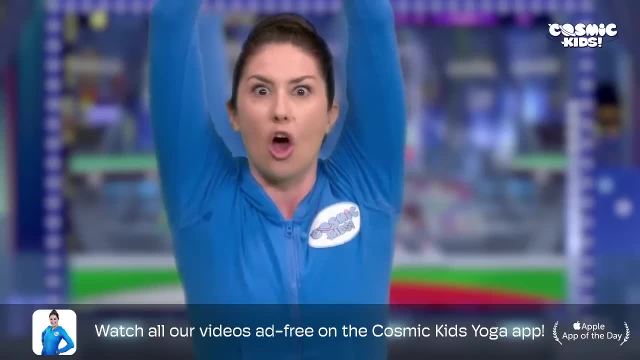 pose: Jump your feet, wide arms, wide hands above your head. In the secret house we are taught a new special move: Surf. Yes, let's do our surfer pose, Turning your foot out to the side, bending into your knee. 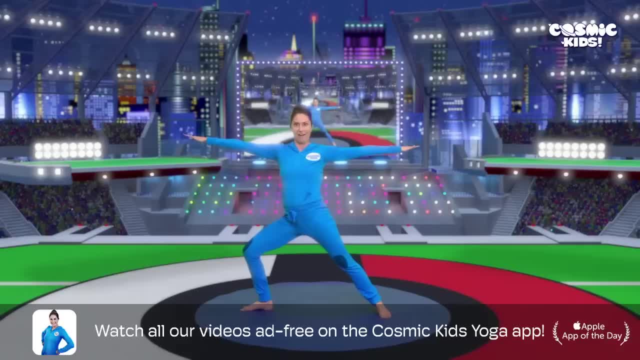 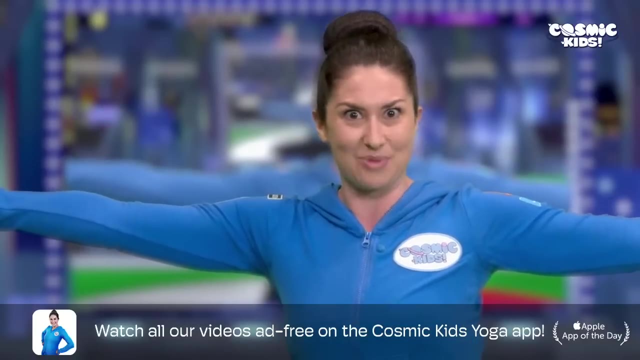 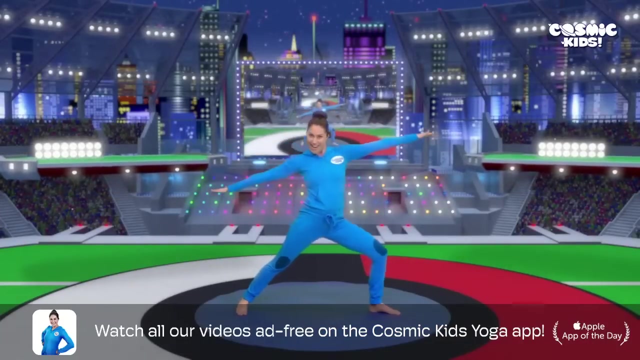 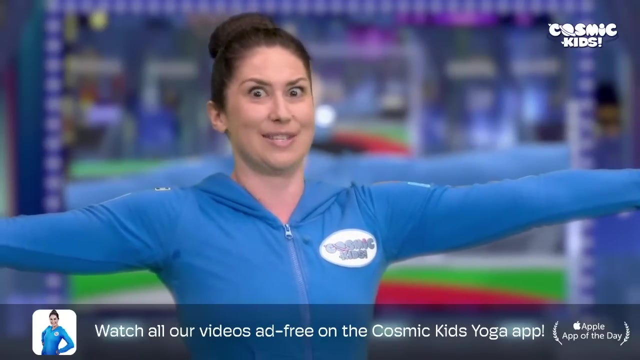 we open our arms wide and we are surfing. We teach all of our Pokemon team how to surf as well, So now we can cross water and catch water Pokemon. Let's jump and surf the other way. This is awesome. Our first water Pokemon that we catch is a Wooper. 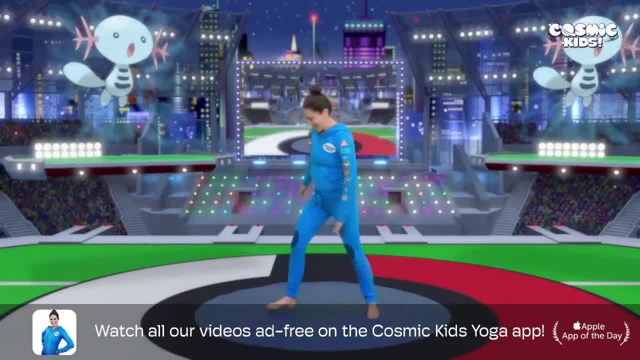 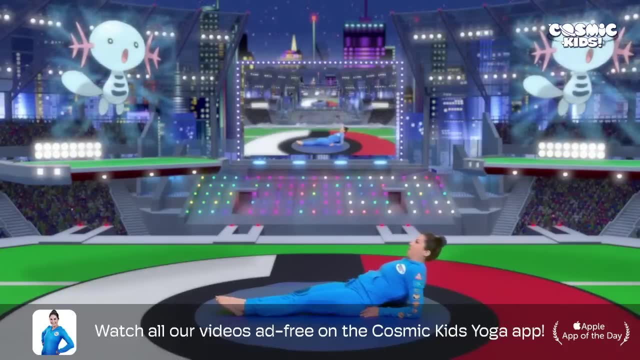 a fish-like Pokemon Coming into fish pose, Sitting on our bottoms, our legs out long. We point our toes and come down onto our elbows. We pop, pop, pop our chest to the sky, looking all the way up and back behind us like a fish. 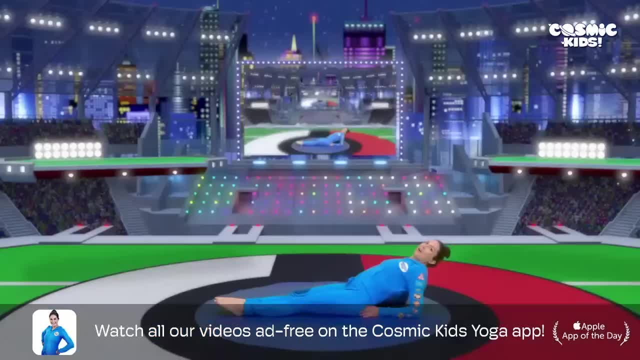 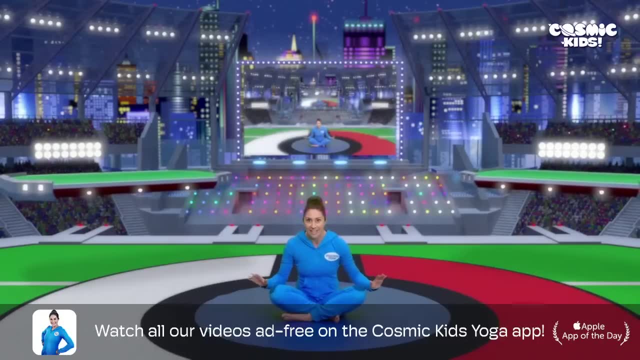 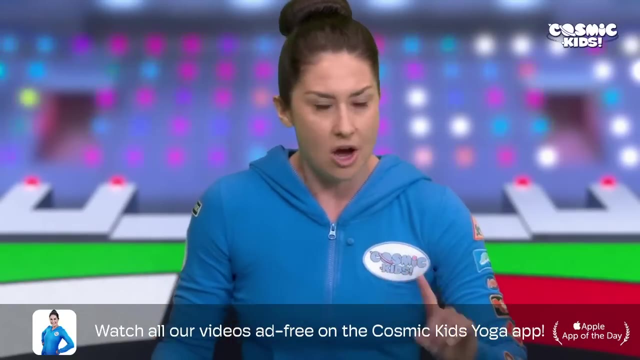 Oh wow, our team is pretty strong now. We sit up tall because we are readier than ever for our first gym battle with Brock and his Pokemon. Now, Brock's Pokemon at the Pewter City Gym are all rock types, So we know which ones have the strength to beat Brock's Pokemon. 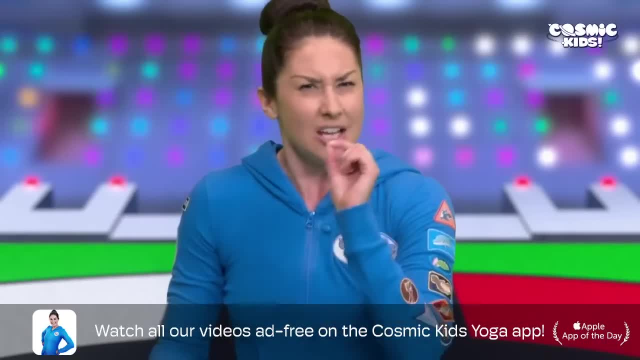 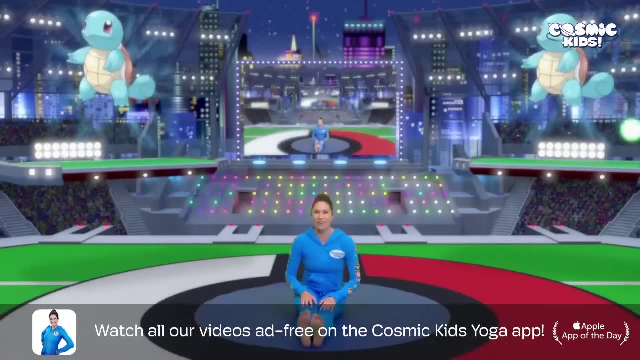 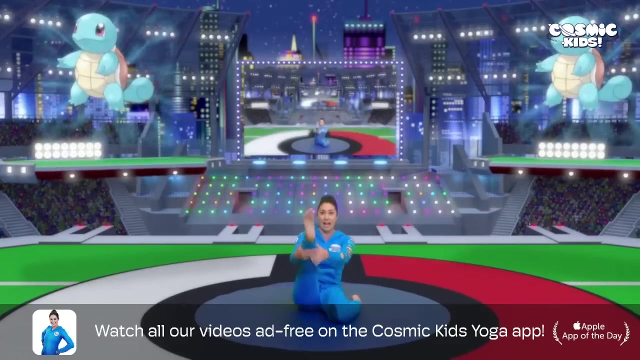 It's our water types. So we send in Squirtle to battle with its water gun, hose, pose, move, Let's try. it Legs out long in front of us. We sweep one leg back behind us, pointing our toes backwards. We lift up our front leg, pointing our hose, our water gun, to the sky. 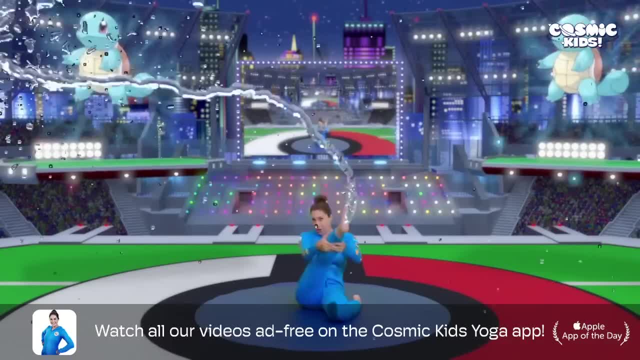 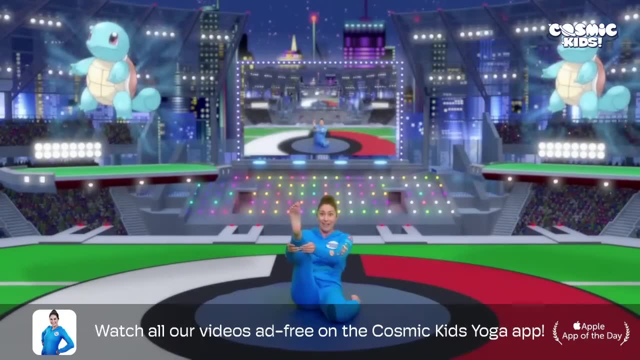 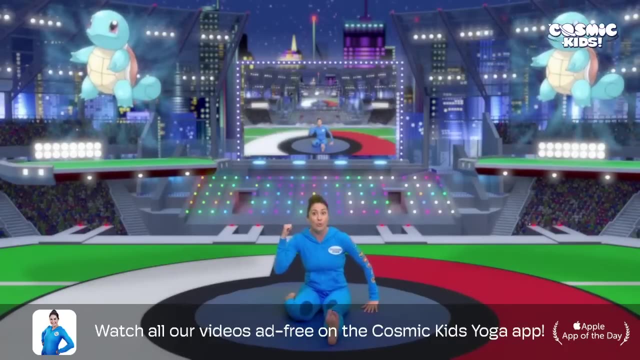 And we spray Sweeping. Let's try it on the other side: Lowering our leg down, bringing our other foot forward, we sweep our other leg back behind us, pointing our toes all the way back. Now we lift up our other leg and let's do a bit more of that water gun hose pose. 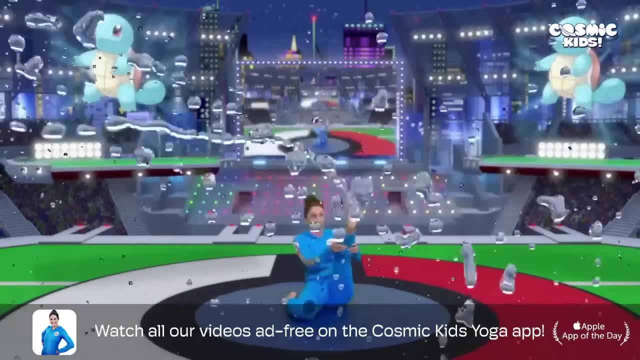 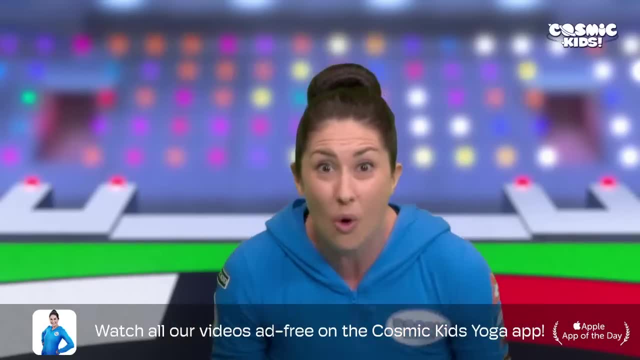 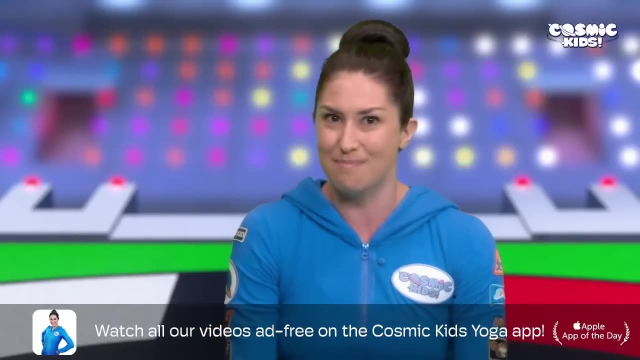 Here we go And lowering it down. We've nearly finished. We've nearly beaten all of Brock's Pokemon. We should try one more thing, though: Wooper. Wooper's special move is the Mud Shot, which means it can shoot blobs of mud at its opponents. 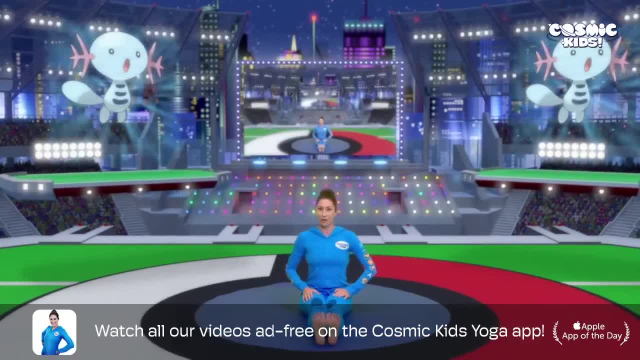 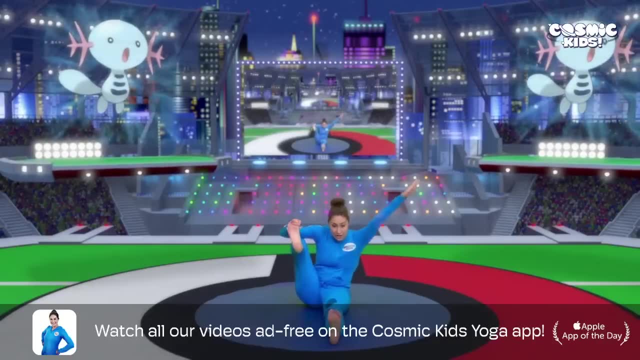 Let's do the Mud Shot pose. Sitting with our legs out long, we take two fingers between our big toe and our second toe, We draw our knee all the way back and we reach forward with our other arm to take aim. Now we get ready to fire our blob of mud. 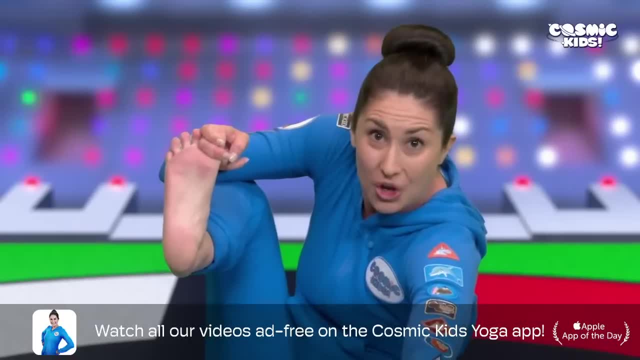 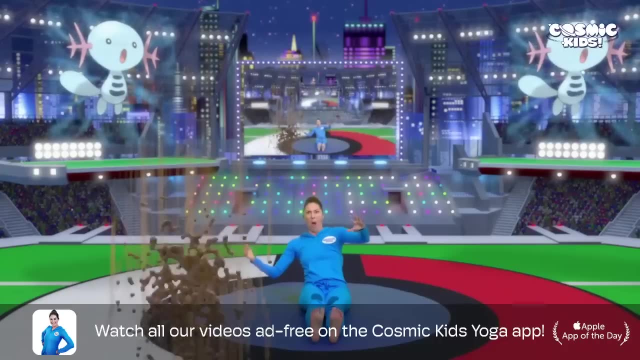 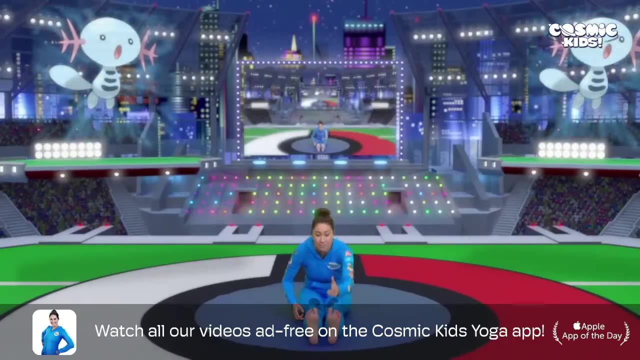 After three, let's fire One, two, three Fire. Oh, that was amazing. Let's try it on the other side. Bring two fingers down between our big toe and our second toe. Draw our knee all the way back. 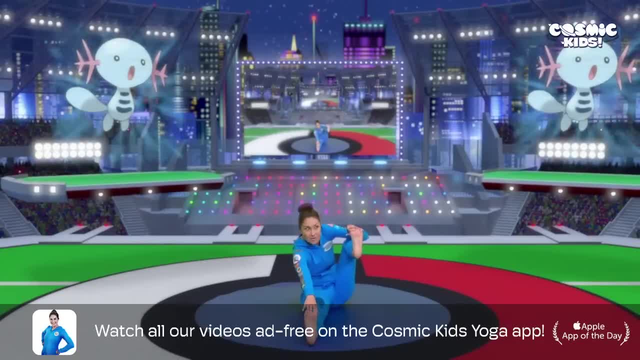 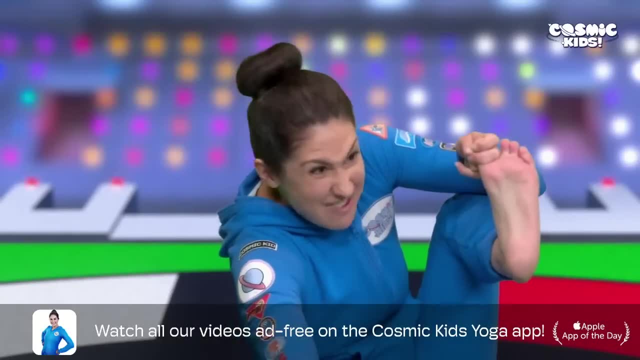 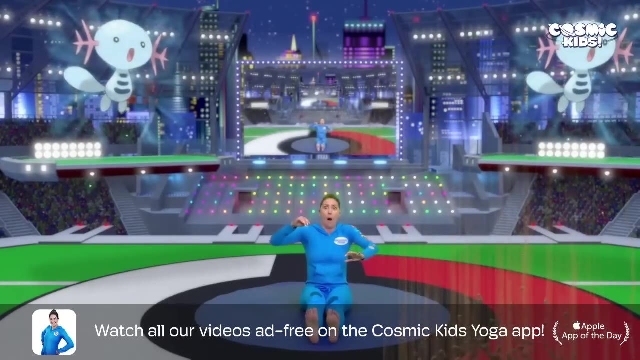 We reach forward to take aim, putting our fingers on our toes, and after three we fire another big blob of mud. Here we go, One, two, three, Fire, Mmmmmm. Oh Wow, We've done it. 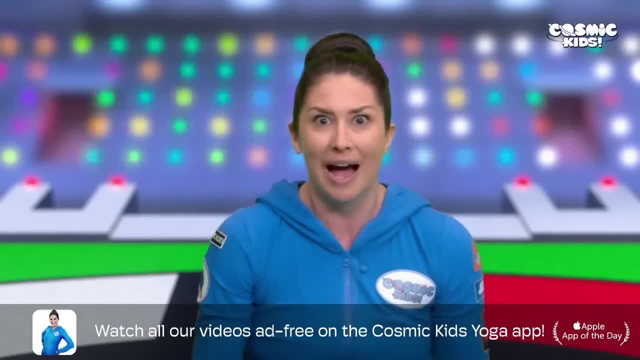 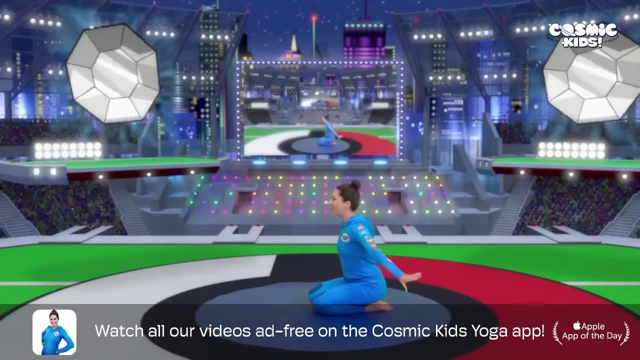 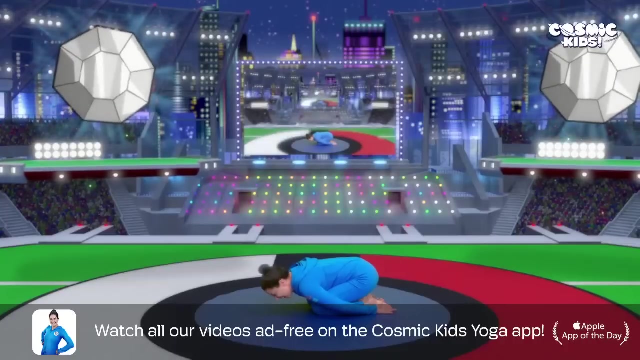 We've defeated Brock and all of his Pokémon and won our first badge, the Boulder Badge. coming into Boulder, Pose Onto our knees, we fold our body all the way forwards, coming into our amazing, brilliant Boulder shape, Ta-da Coming up to sit. 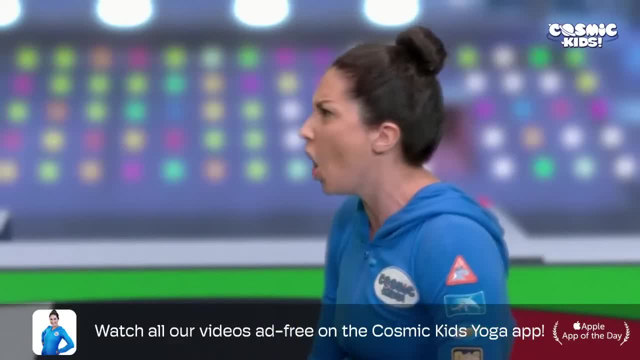 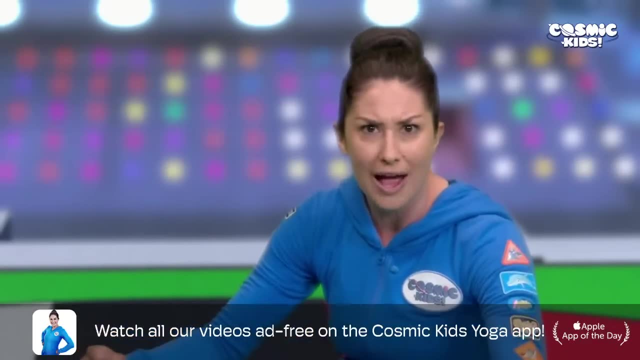 Wow, everyone, We've done it. We've collected loads of Pokémon and we've beaten Brock in our first gym. But we need to rest and recover now restore our health. So we take our team of Pokémon for a well-earned rest at the Pokémon Centre. 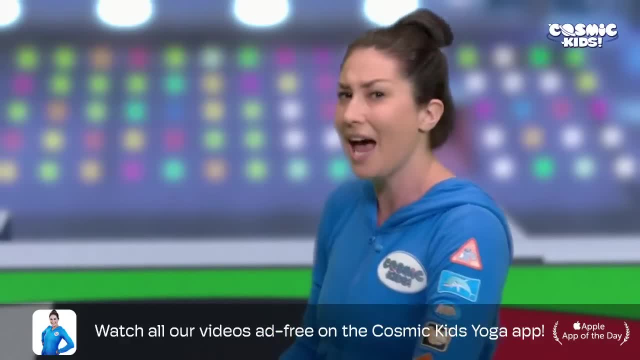 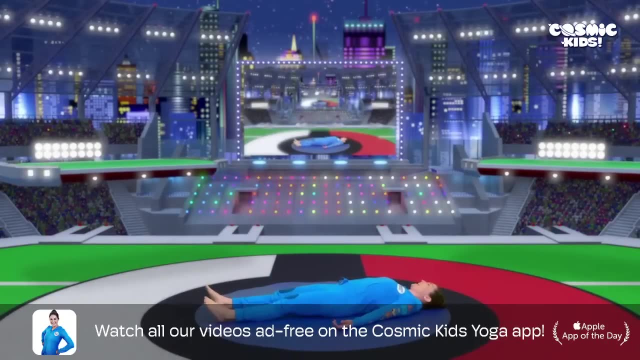 and we release our Jigglypuff to sing its little lullaby to help us relax. Lying on our backs, taking our legs and arms long, we rest our bodies down, Letting ourselves breathe slowly As we lay here. 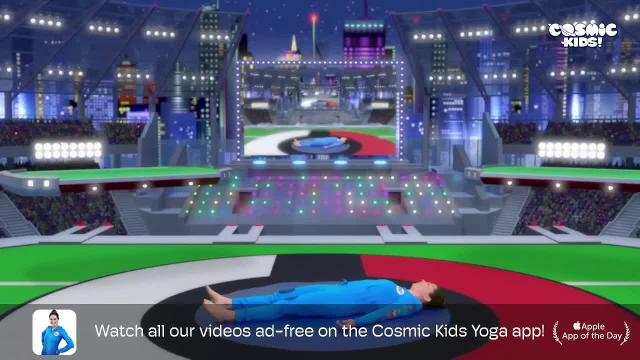 we think about our awesome team of Pokémon and how we are so strong when we work in a team, how we can recognise our strengths and those strengths of our team members, And working together gives us so much more power, helps us achieve so much more. 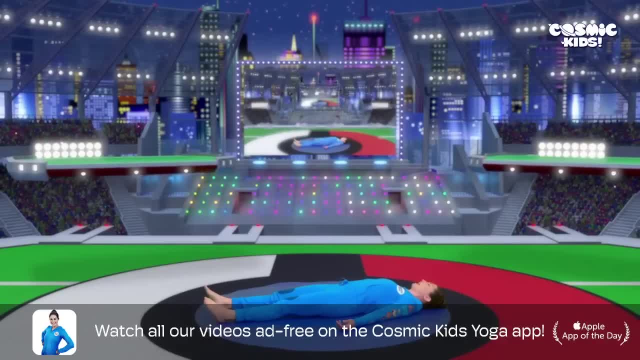 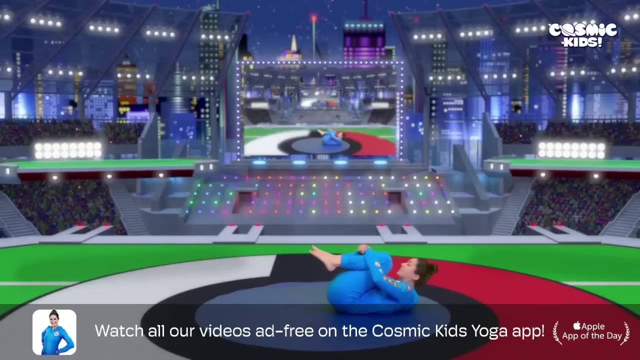 And even when we fail, we can learn, we can practise and get better and come back even stronger. Now it's time to wake up. So we wiggle our fingers and our toes, We hug our knees into our chest, giving them a little kiss. 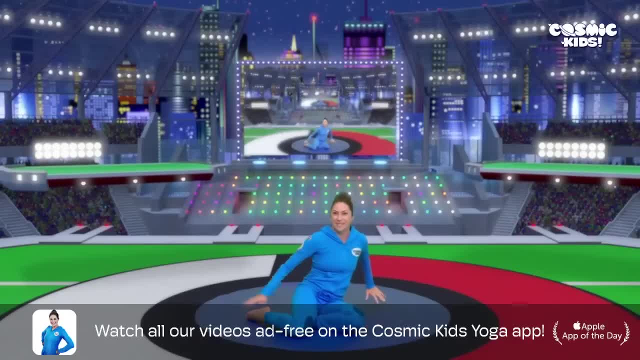 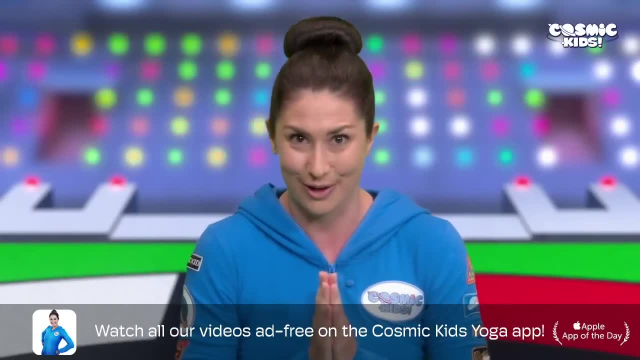 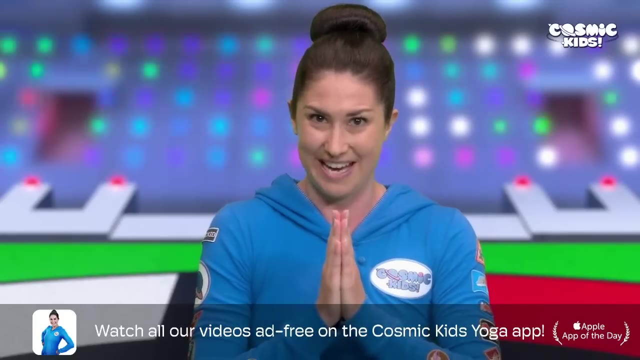 We roll over onto our side and press ourselves up to sit, bringing our hands together at our hearts and finishing just the way we started with our secret yoga code word which is Namaste, Ready After three. One, two, three. 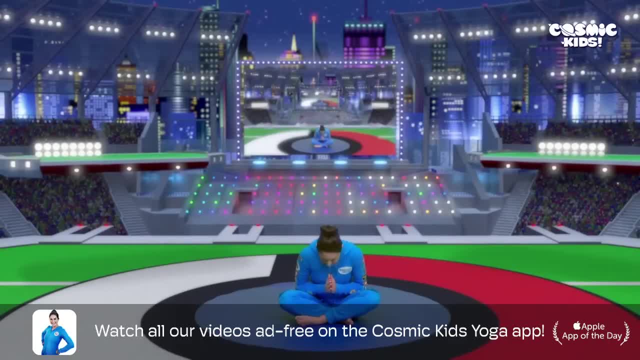 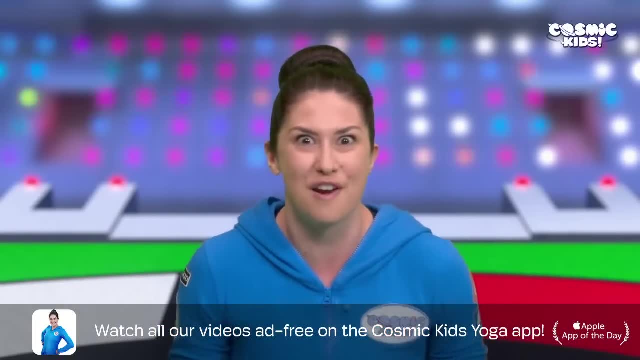 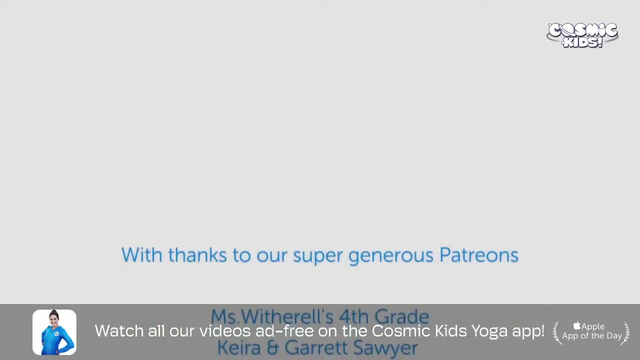 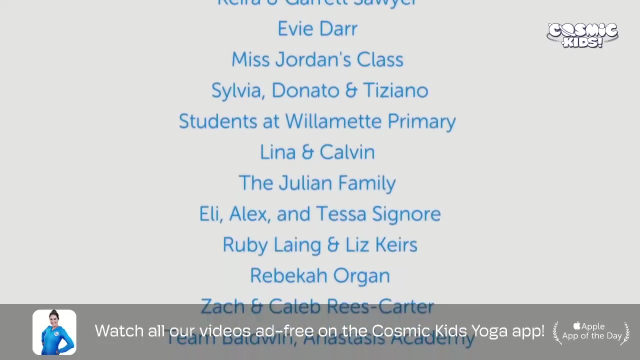 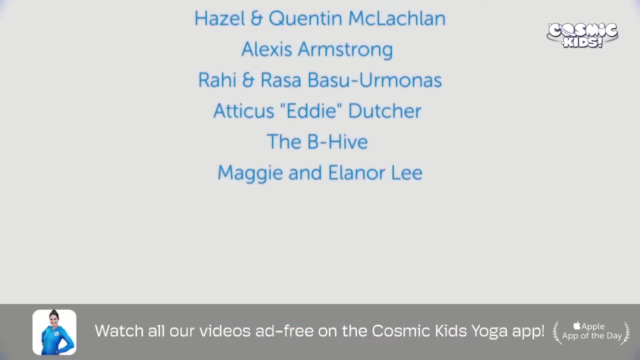 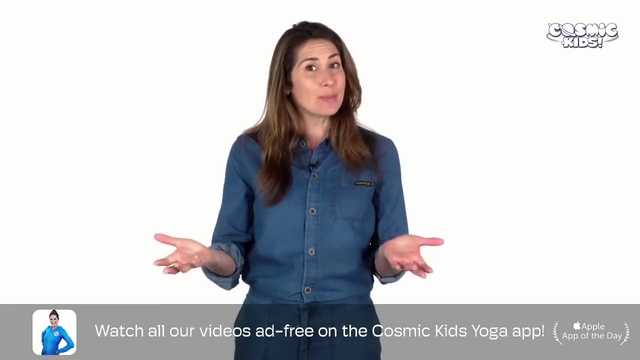 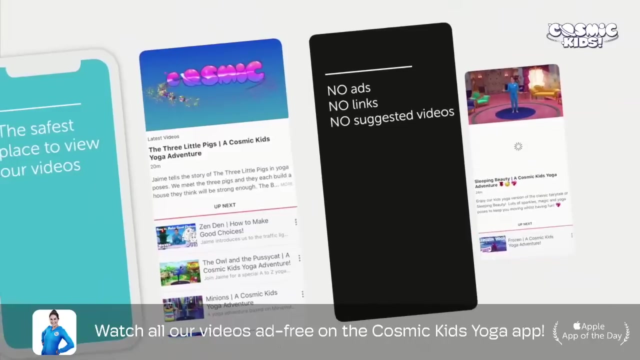 Namaste. Wow, well done everyone. That was awesome. I hope you enjoyed the Pokémon adventure and you come back soon for another Cosmic Kids adventure. Bye-bye. Captions by Red Bee Media. Copyright Australian Broadcasting Corporation. Head to appcosmickidscom. 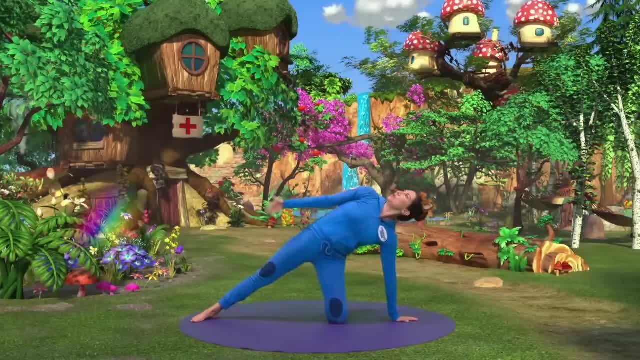 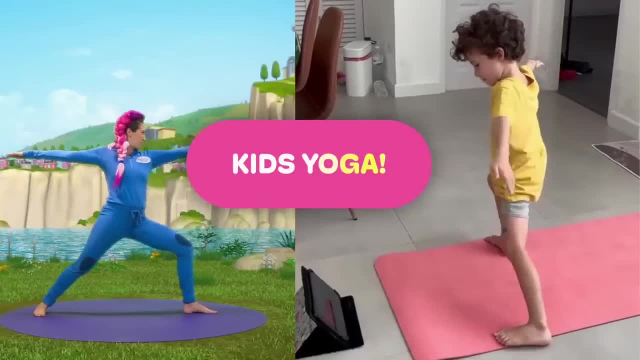 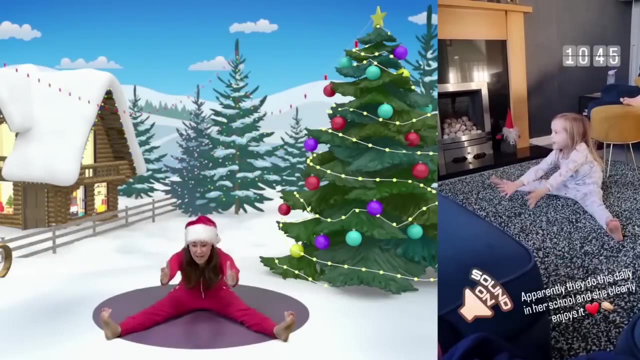 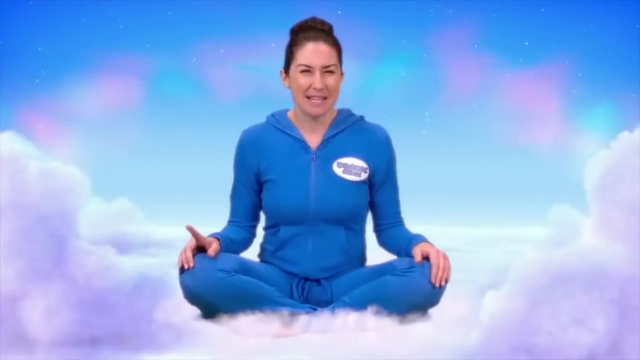 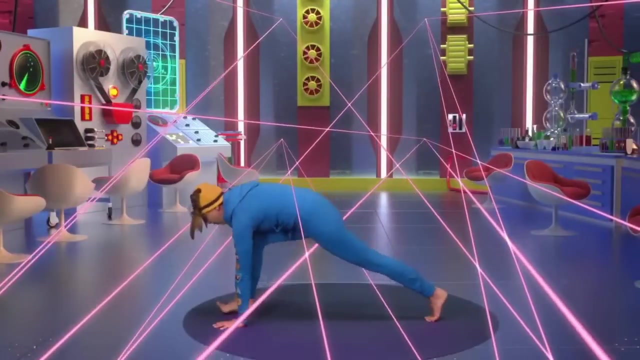 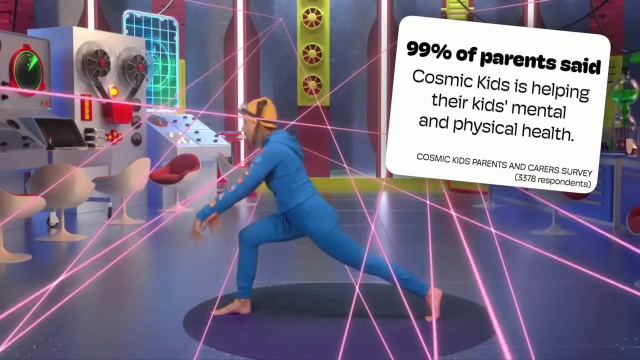 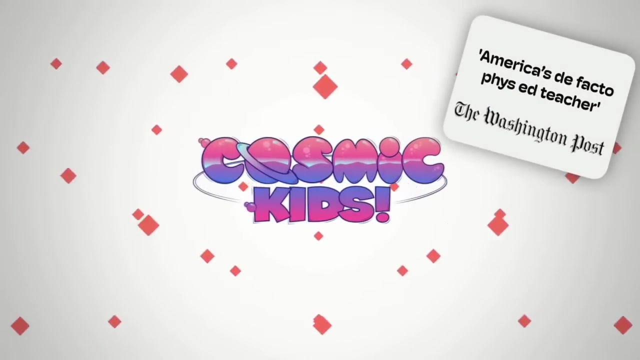 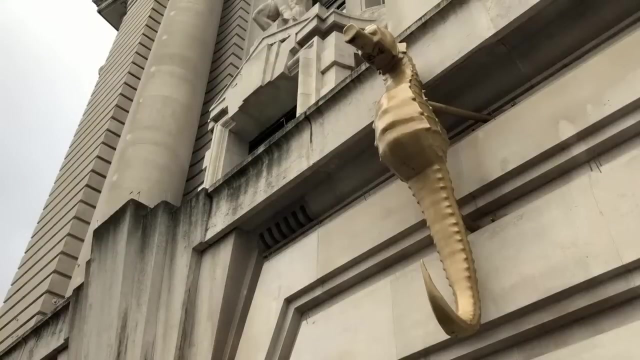 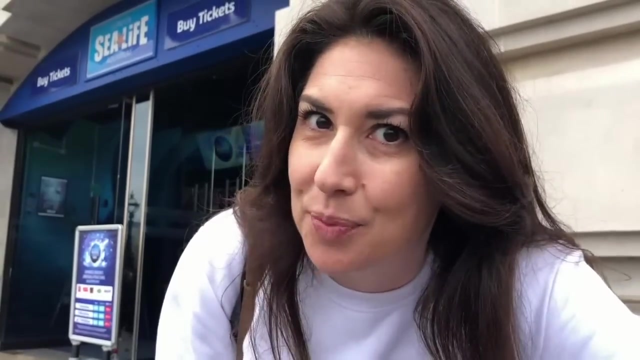 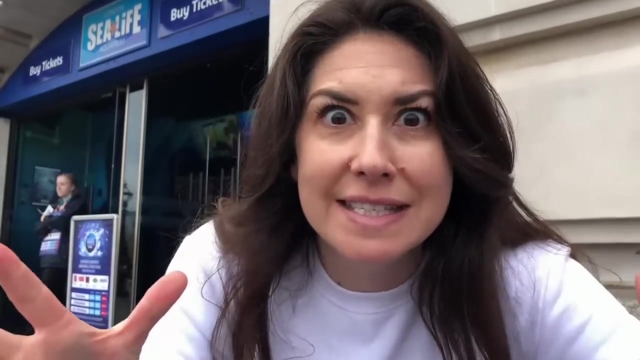 Pick a month, Go away Is to think: Oh, yes, I can. Welcome to London, to the Sea Life London Aquarium, where we are here to bring you a very exciting mix of yoga videos, Yoga videos that are all based around the ocean and sea life. 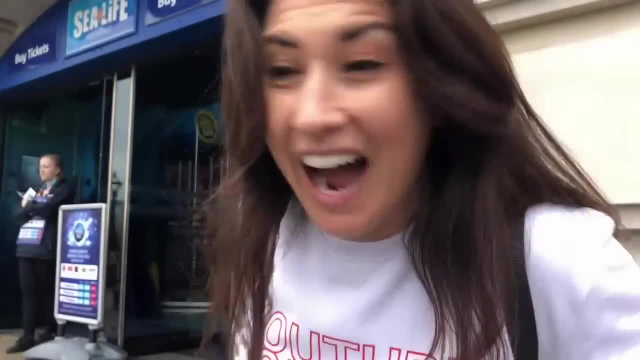 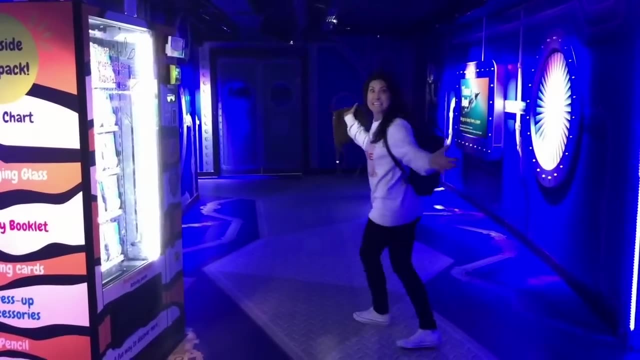 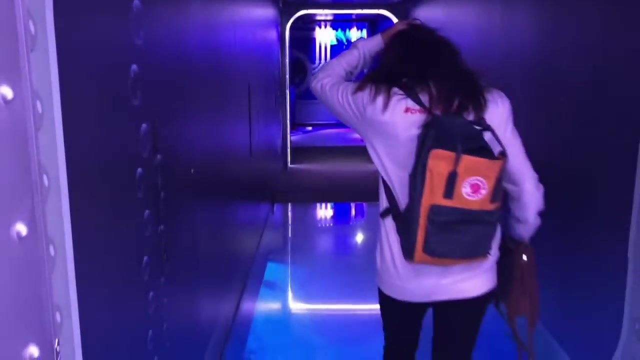 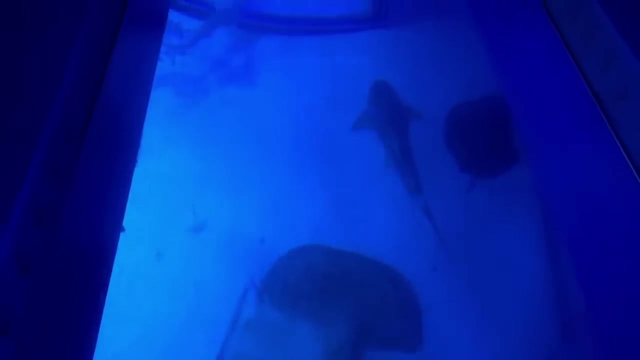 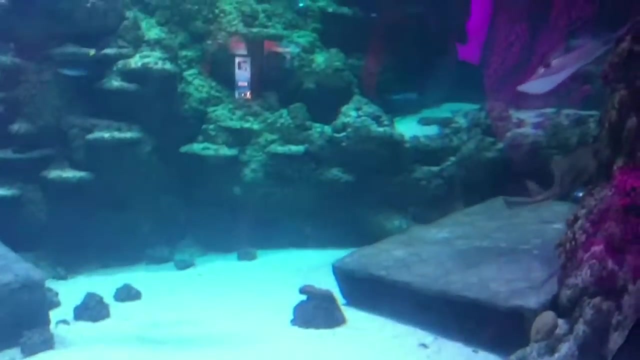 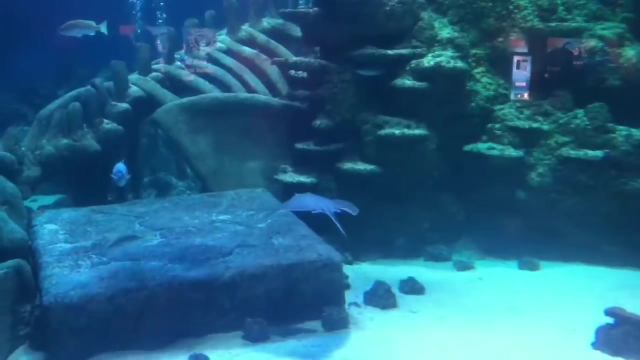 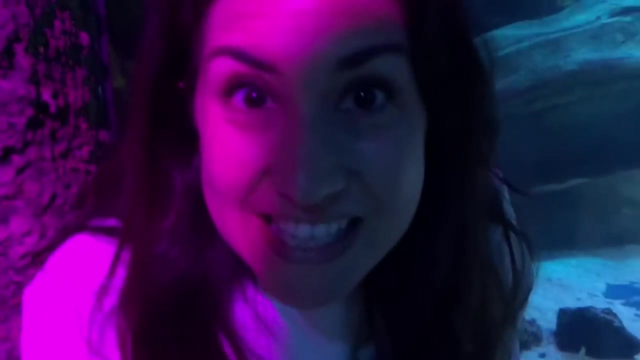 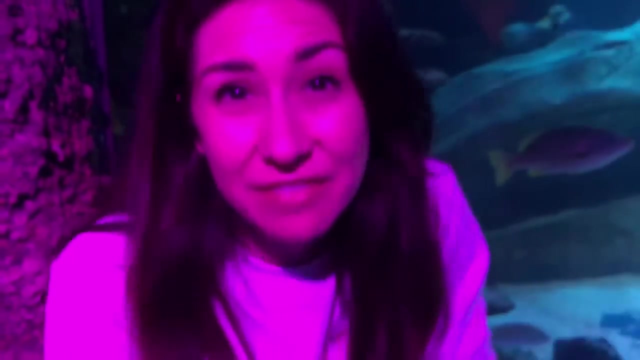 So let's go on in and see what we see. Captions by Red Bee Media. Copyright- Australian Broadcasting Corporation. Look, I am here in the Sea Life Aquarium in London. It's beautiful, full of amazing fish and sea life. It's incredible. 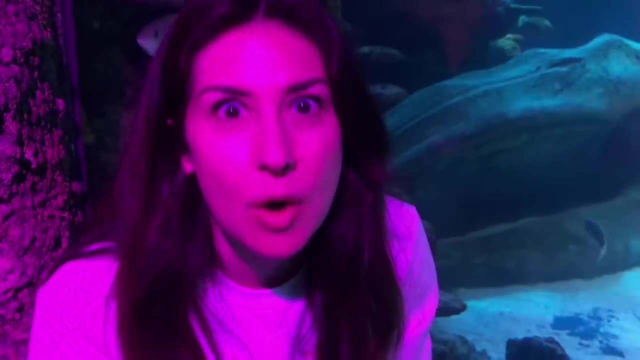 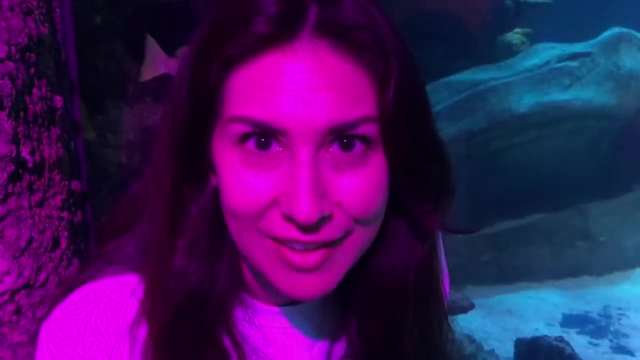 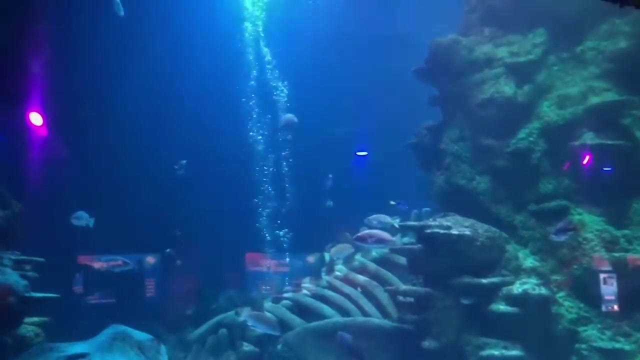 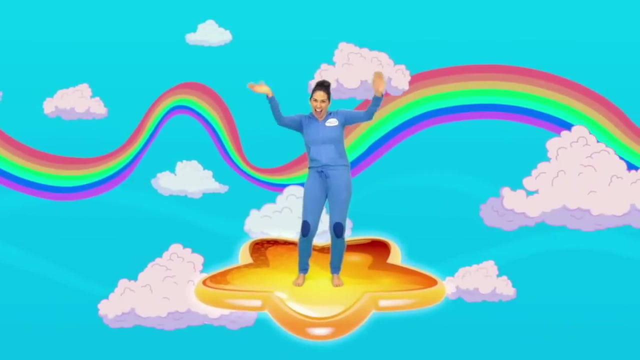 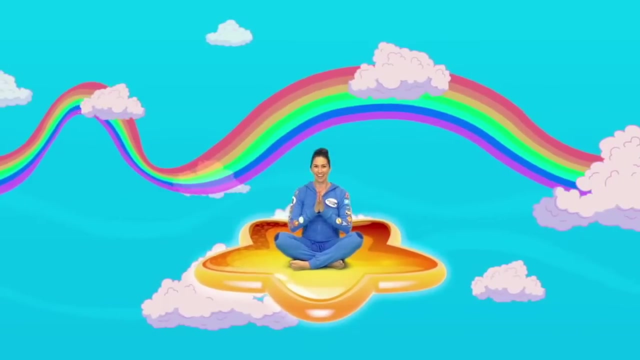 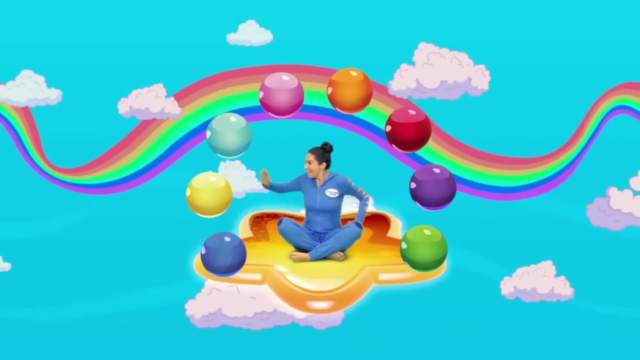 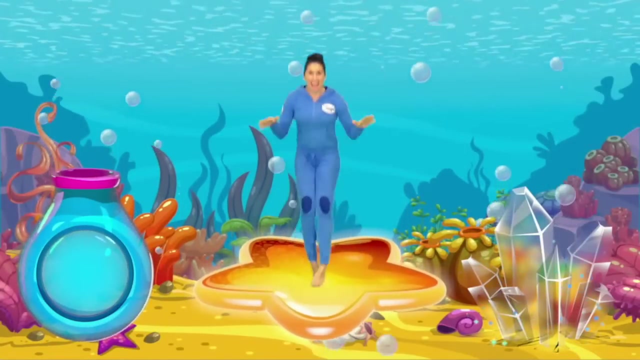 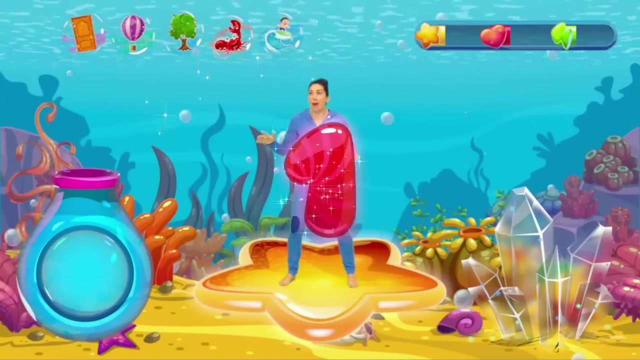 Now we're going to begin by getting ourselves warmed up with a wonderful super yoga game. Yes, it's the underwater party, And make sure you do that. Disco Carrot. I can't wait to see you afterwards. Super yoga Three, two, one go. 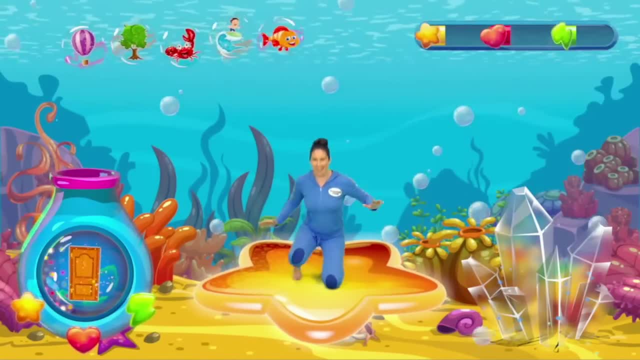 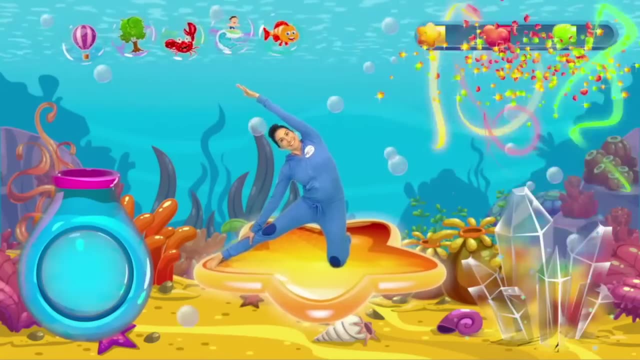 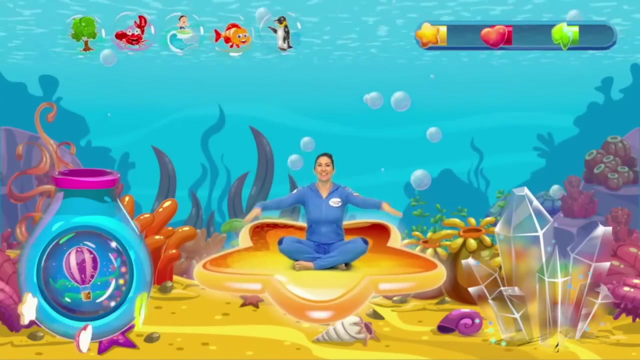 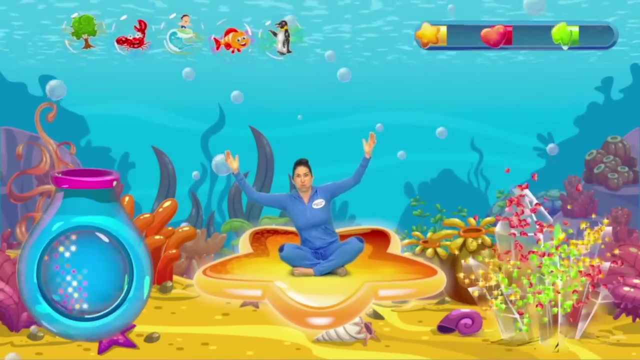 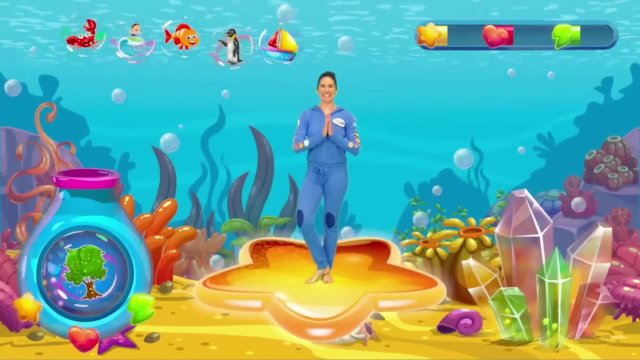 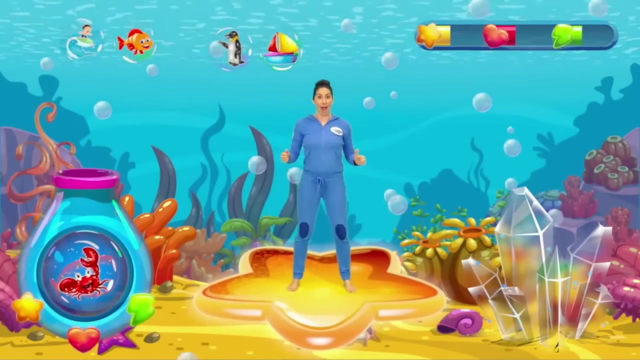 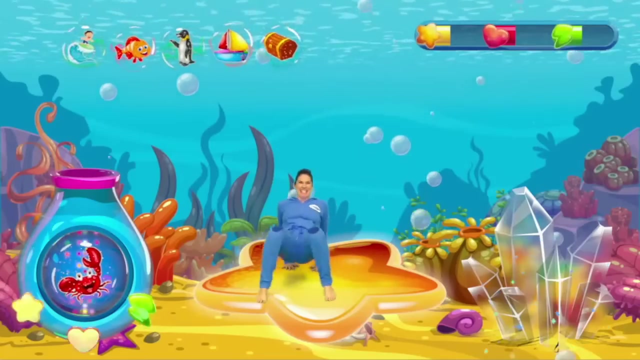 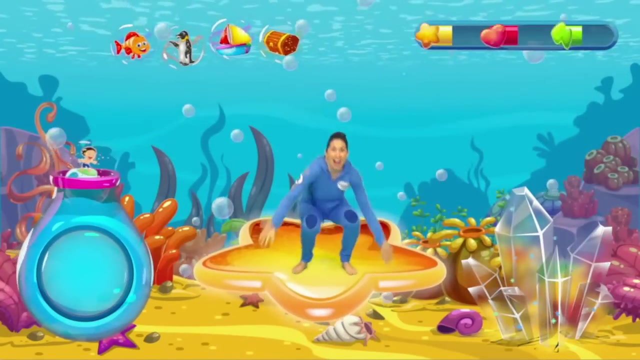 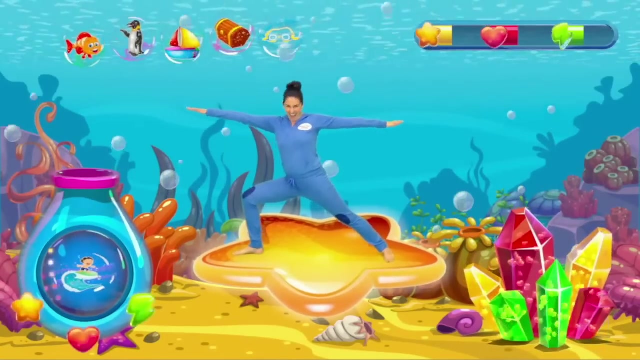 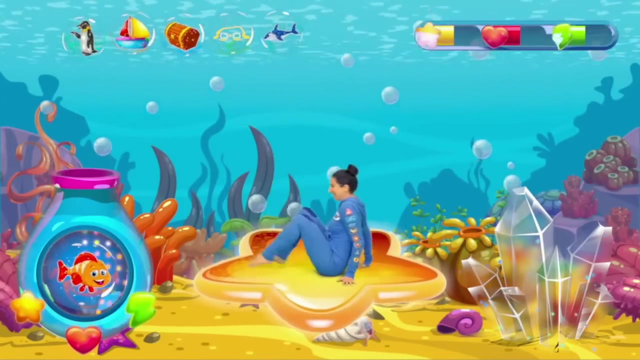 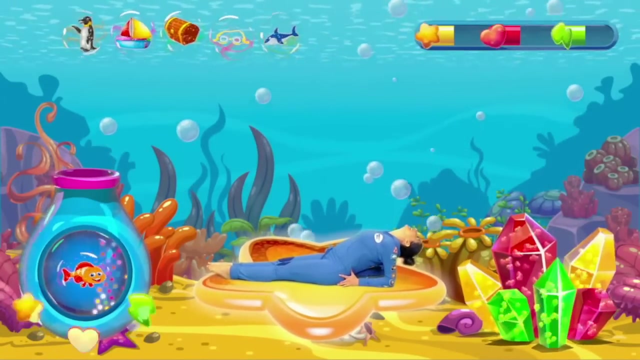 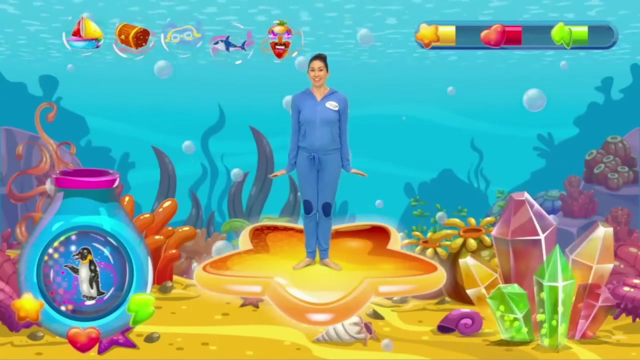 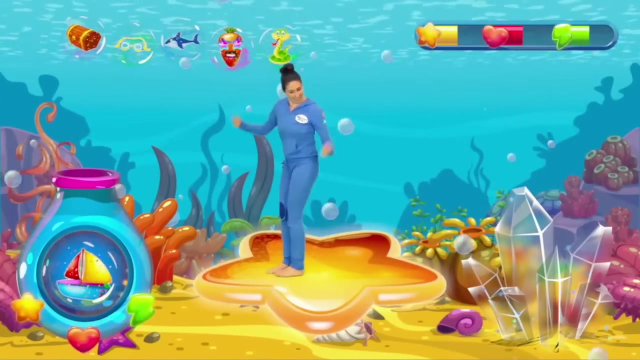 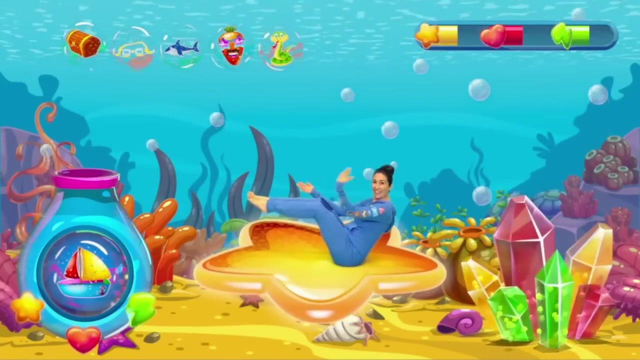 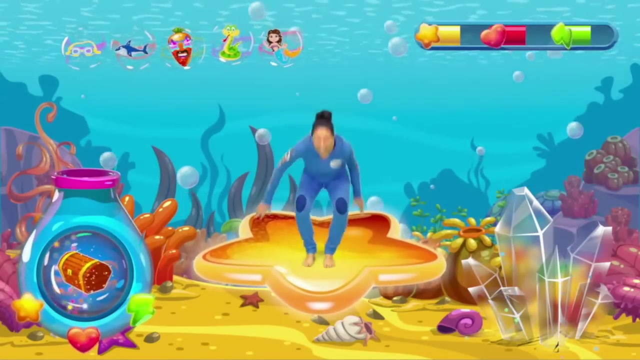 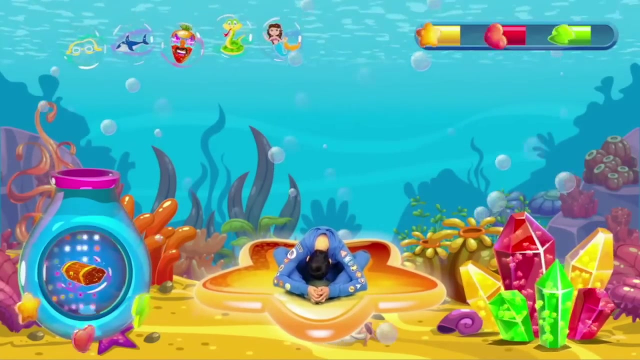 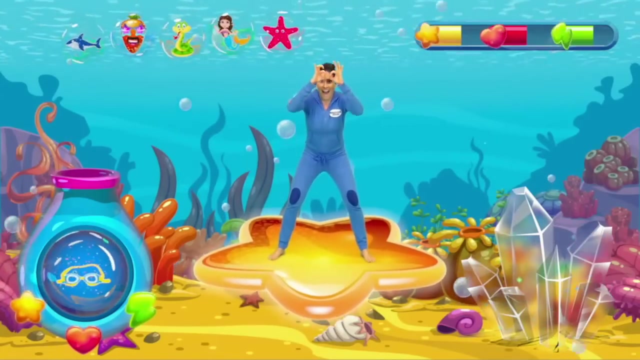 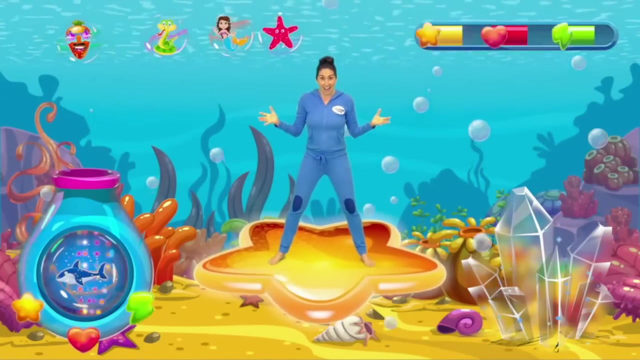 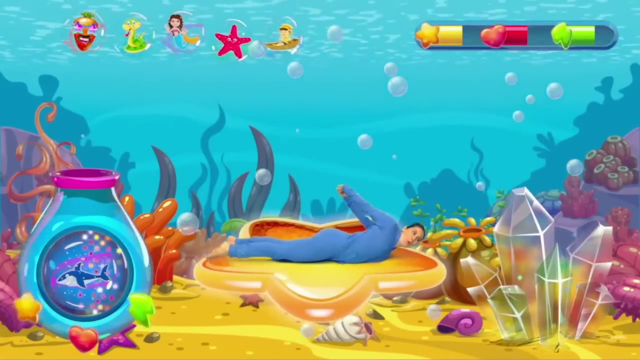 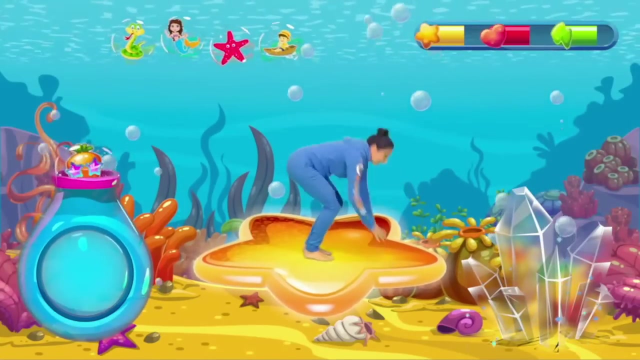 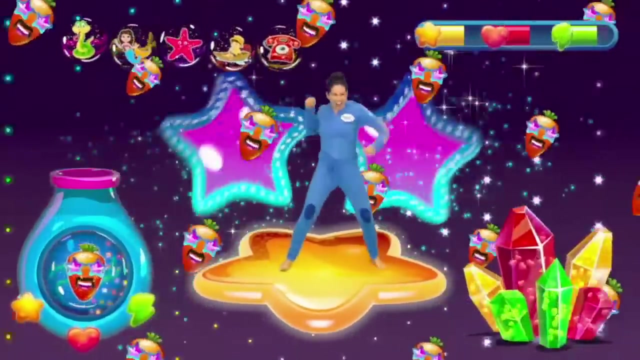 Door pose. Hot air balloon pose. Tree pose. Crab pose. Surfer pose. Fish pose. Penguin pose. Boat pose. Treasure chest pose, Cosmic Oculus. Cosmic Oculus Sharp pose. Look out, It's the disco time. It's time for a party. Time for a party. 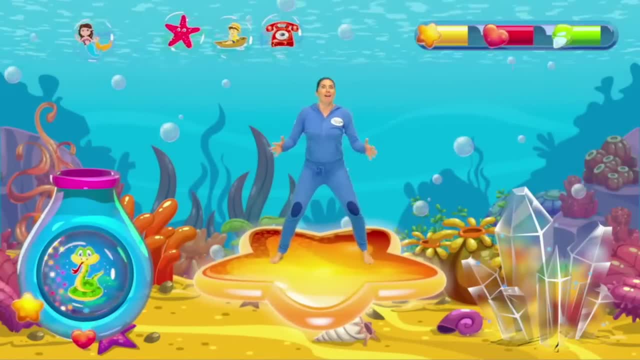 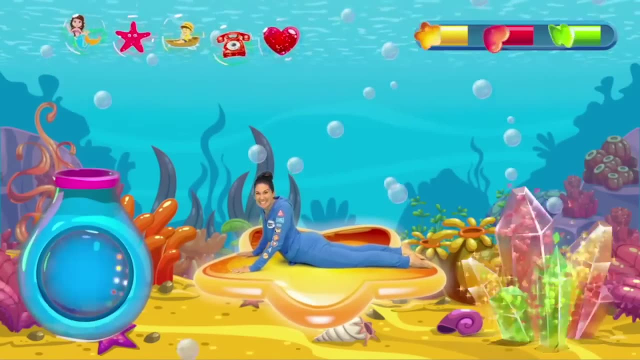 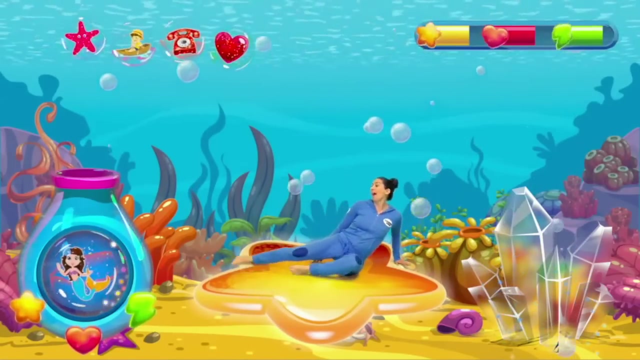 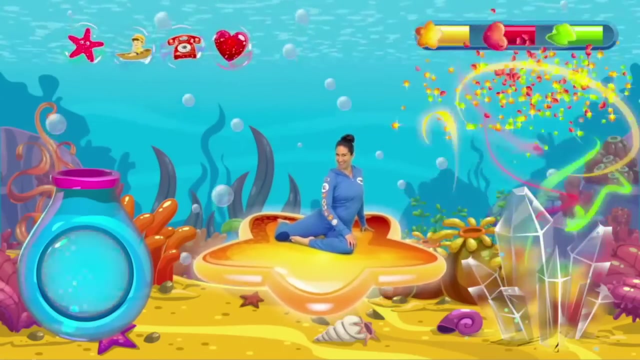 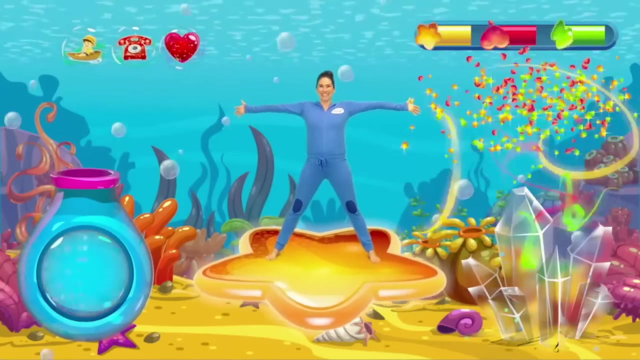 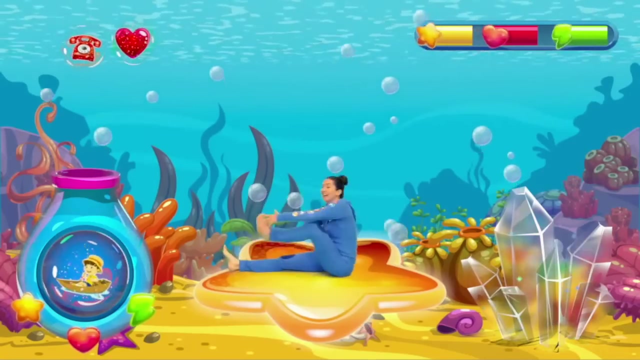 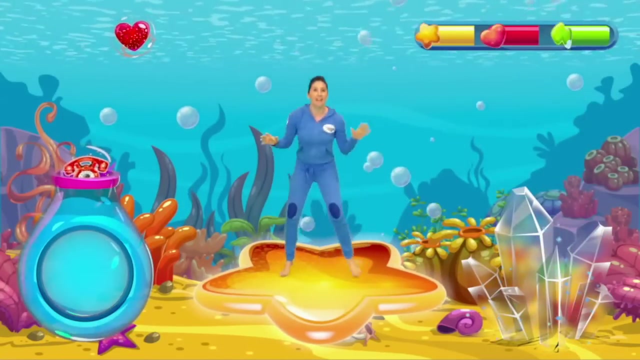 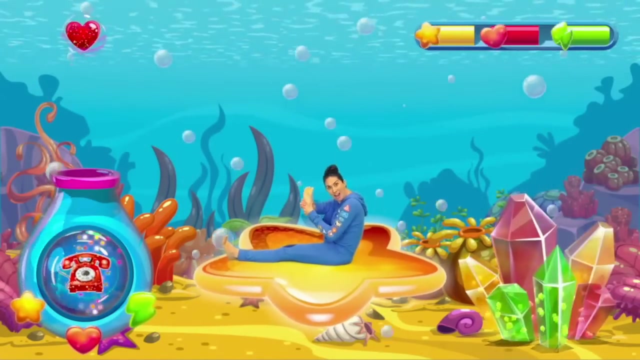 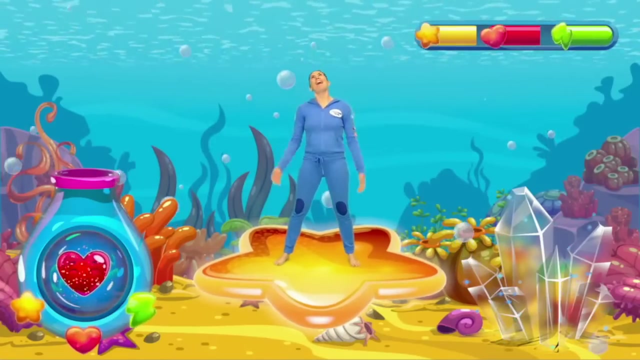 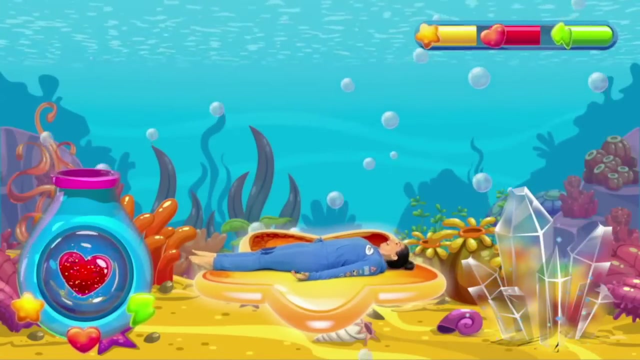 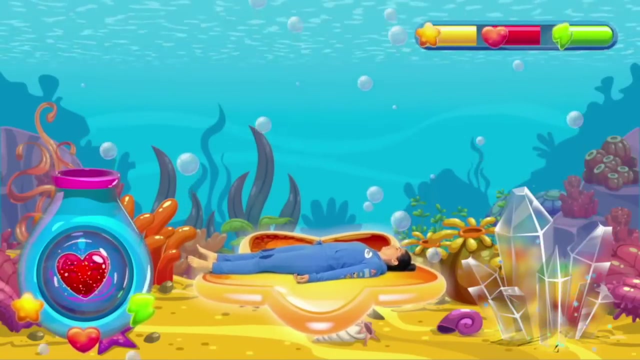 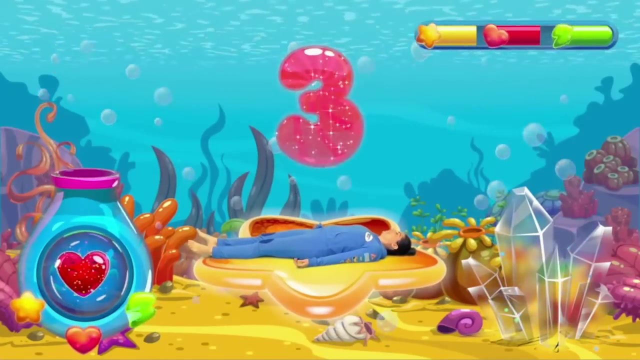 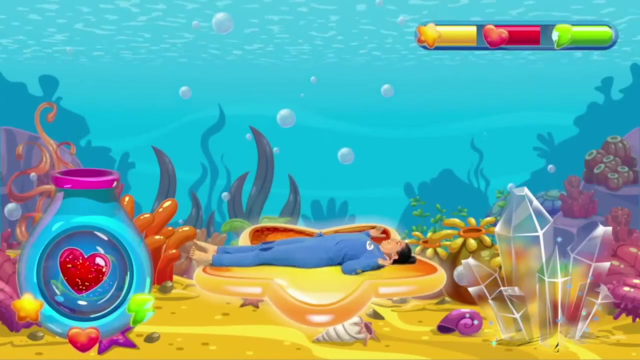 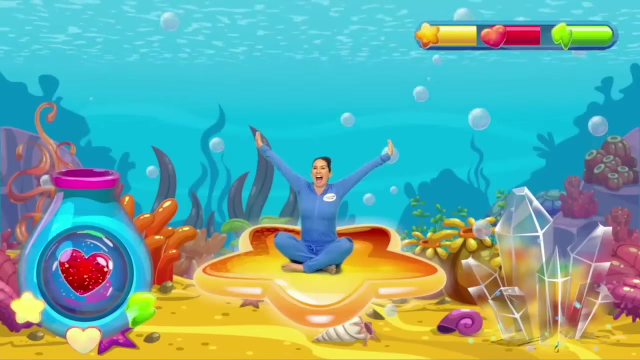 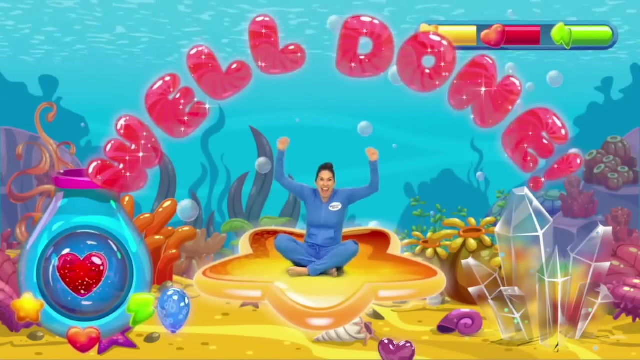 Snake pose. Mermaid pose. Ooh la la Starfish pose. Marine pose. Telephone pose 10, 9,, 8,, 7,, 6,, 5,, 4,, 3,, 2, 1. Mermaid pose. Mermaid pose. 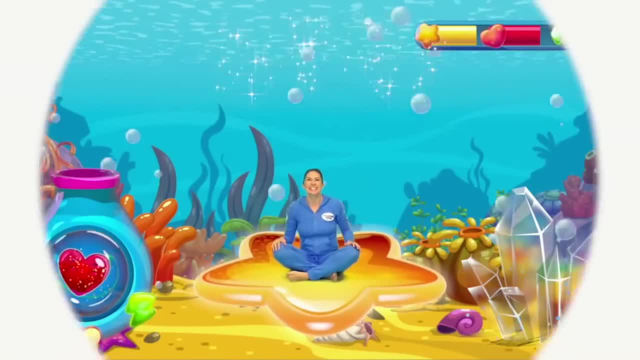 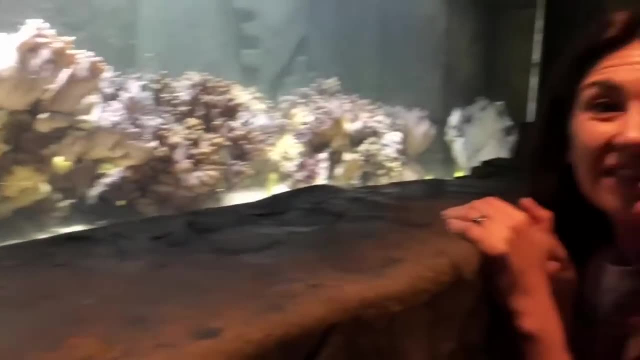 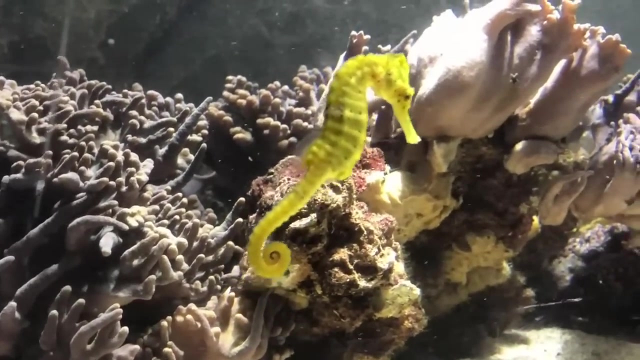 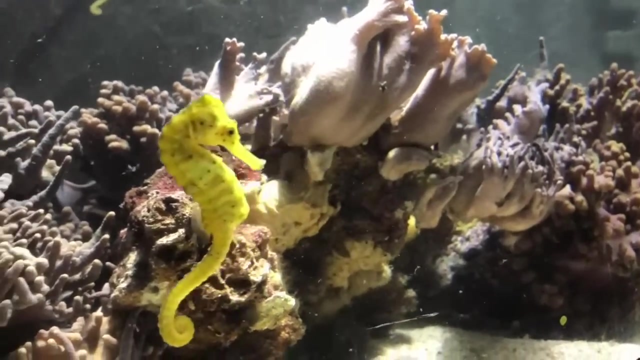 Mermaid pose. Look, we're here with the sea horses. Aren't they amazing? Look at the way they swim standing up. They're so, so sweet. Now we have a very special yoga adventure, all about a yellow seahorse just like this one. 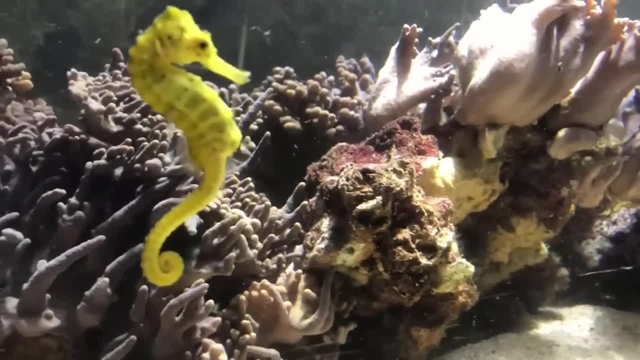 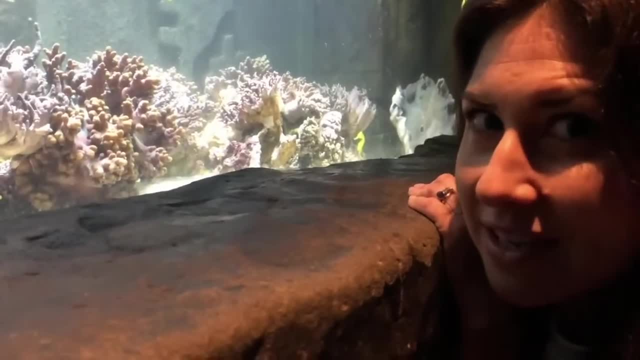 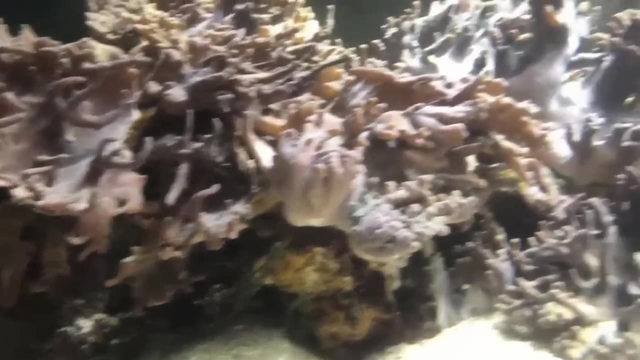 And his name is Norris. Let's go and do that adventure now And I'll see you afterwards to say goodbye with some of the amazing, amazing sharks. My name is Norris and my tiny little fellow- My nose is so long and my body is so yellow. 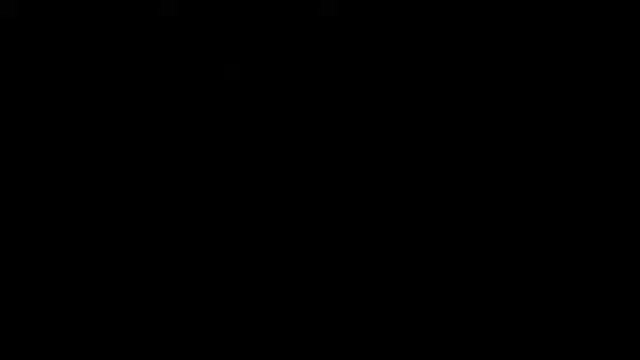 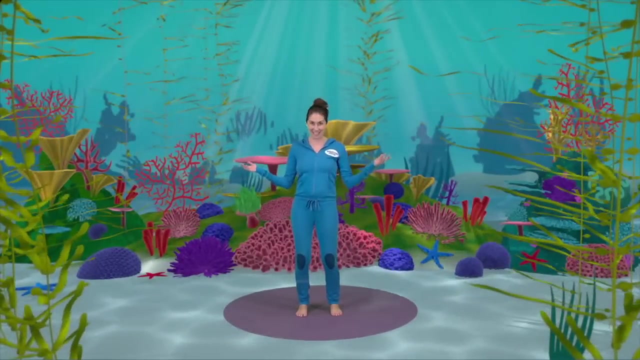 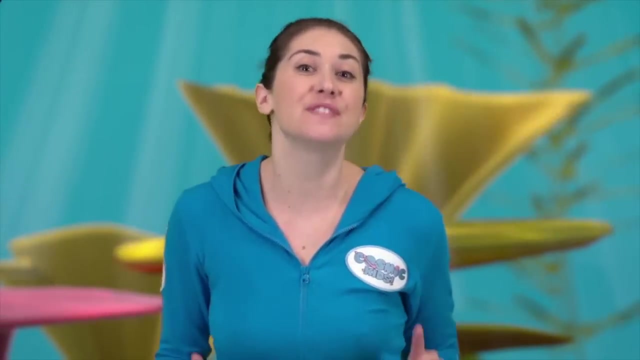 I rock like a rocking horse gliding through the sea Music. Hello everyone, Welcome to Cosmic Kids. I'm Jamie and this is your place for yoga stories and fun. It's easy: Just copy the moves I do and enjoy the adventure. 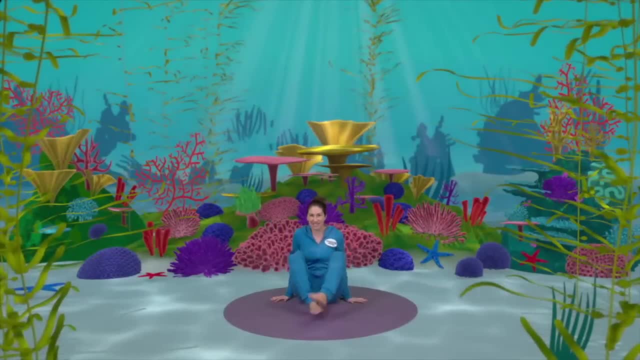 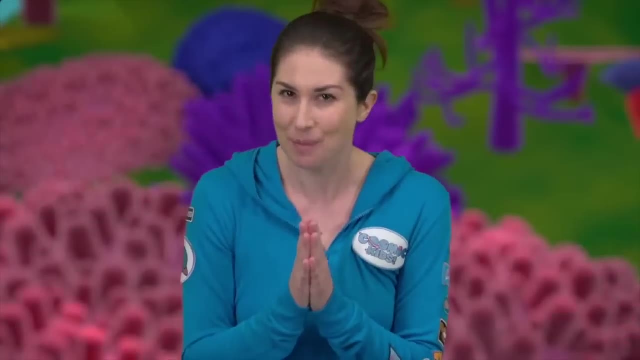 Now we always start in the same way and that's by sitting on our bottoms and crossing our legs And bringing our hands together at our hearts And saying our secret yoga code word, which is Namaste, Ready After three: One, two, three. 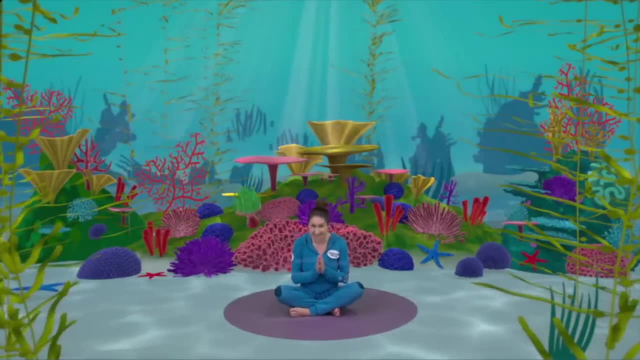 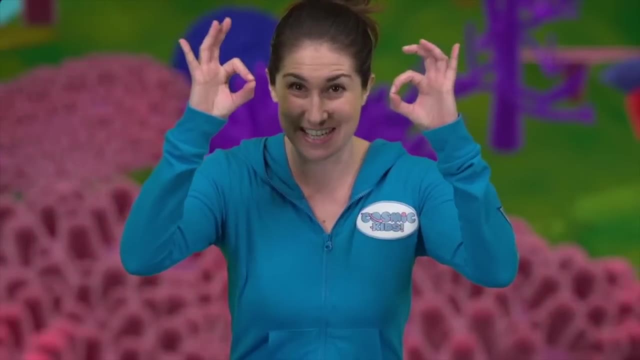 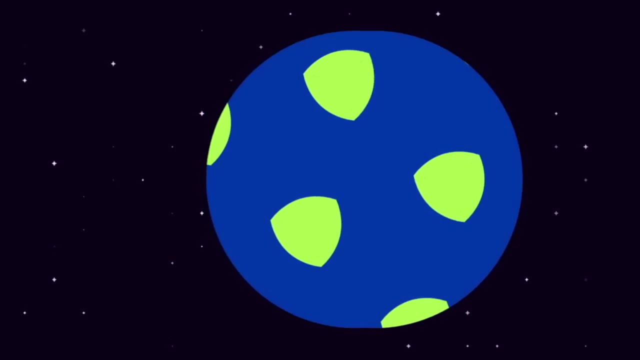 Namaste. There. Now we're ready to begin. So let's take a look through the cosmonoculars, joining our thumbs and fingers together to have a look through. Oh, look at those colours. Yes, Yes, they're so beautiful and bright and colourful. 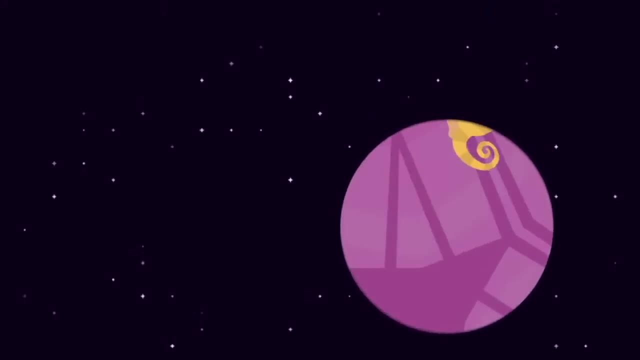 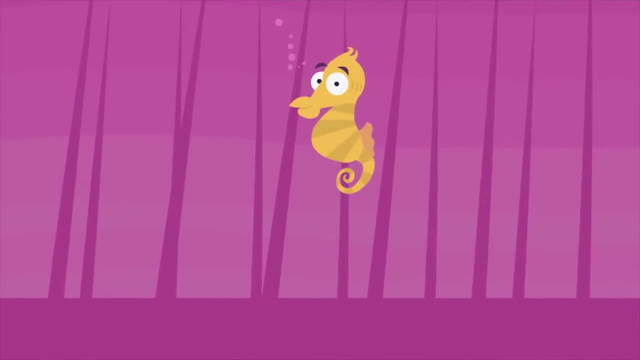 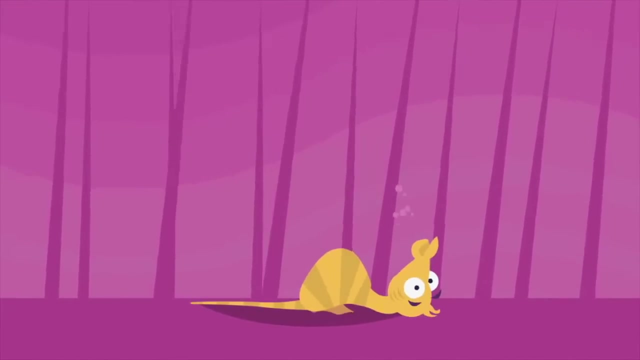 Oh, can you see it? Can you see the? Yes, It's a seahorse, It's a baby seahorse, It's Norris, the baby seahorse. Oh, what's Norris doing? He's doing yoga, He's doing fish pose. 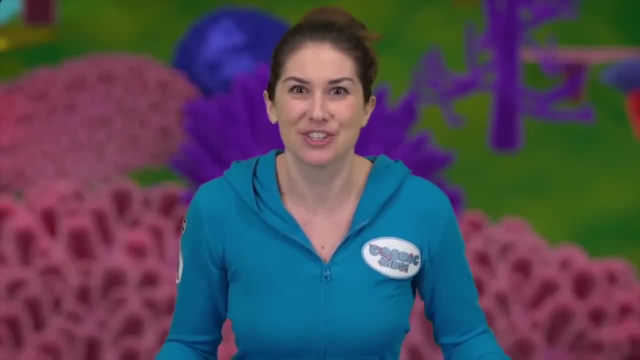 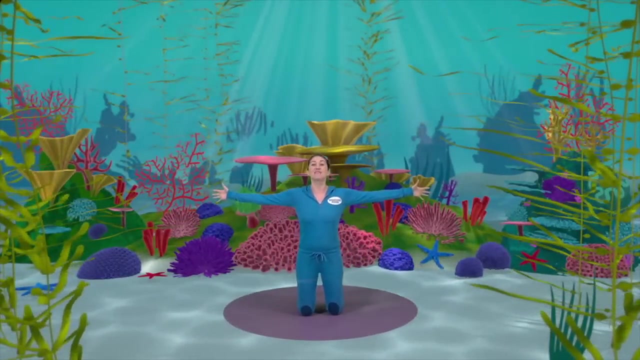 This is very exciting. Let's not beat around the bush. Let's get right to it and go and find Norris. Come to your knees, everybody, Take your arms out wide And give everyone at home a great big hug. Bye, Oh hello. 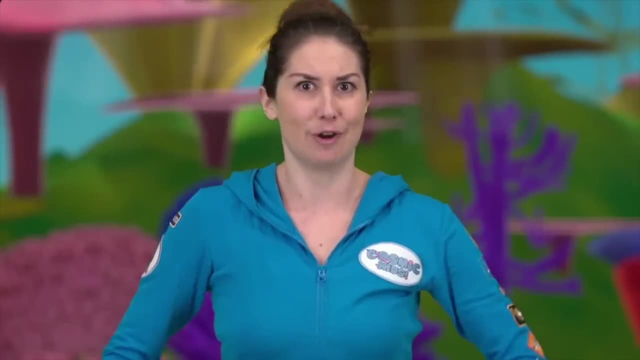 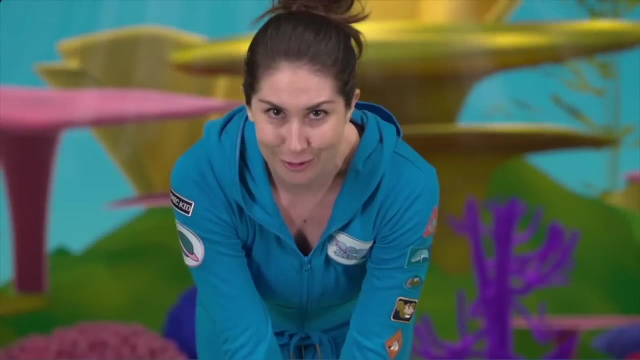 Who's this that's just landed on the window sill. It's a rather magical looking bird Standing up, folding forward. take your wings down Now. this magical looking bird has rather big blue webbed feet. It's a blue footed booby. 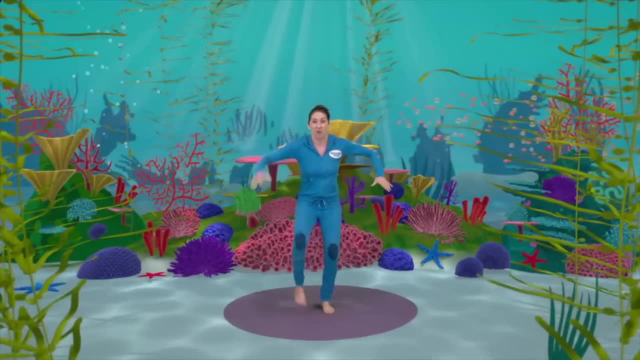 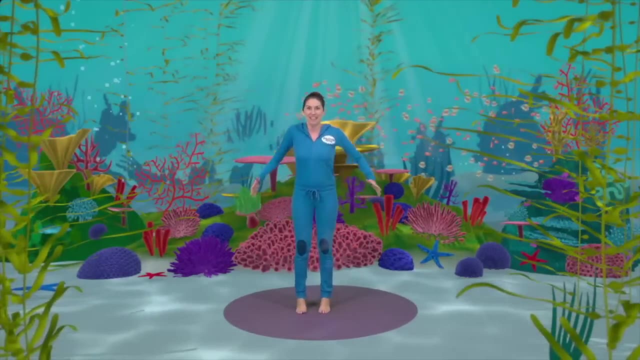 And he does a funny dance. Hello, hello, I'm Bez the booby bird. Yes, I am. I love to do my dancing. Oh, this is great. We get on the back of Bez, Taking our wings down low. 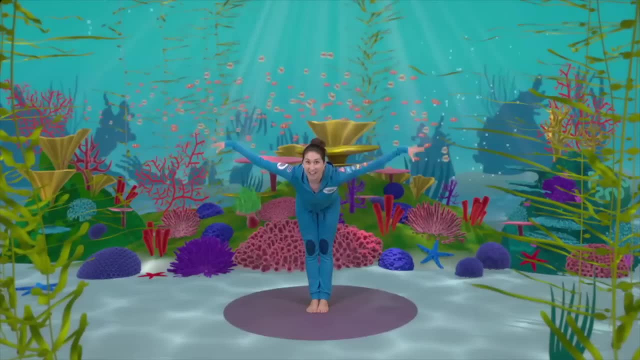 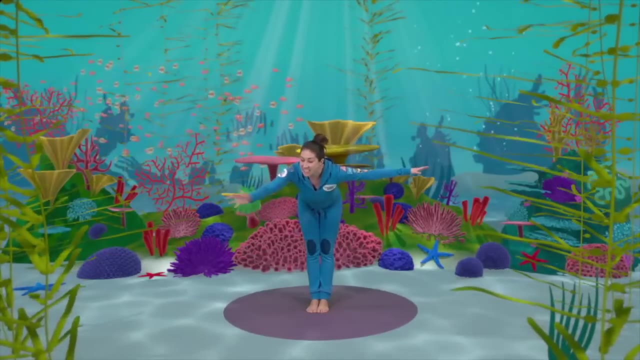 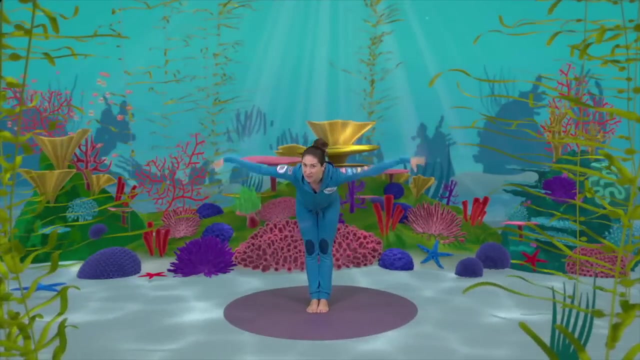 And he swoops them up. Off we go, everyone. We're flying out over the trees and the hills. We wave down to our friends, Hi friends. And down we come Towards the beach Where we're going to hopefully meet Norris, the baby seahorse. 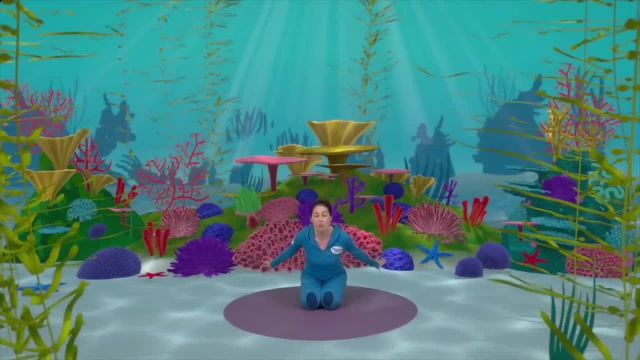 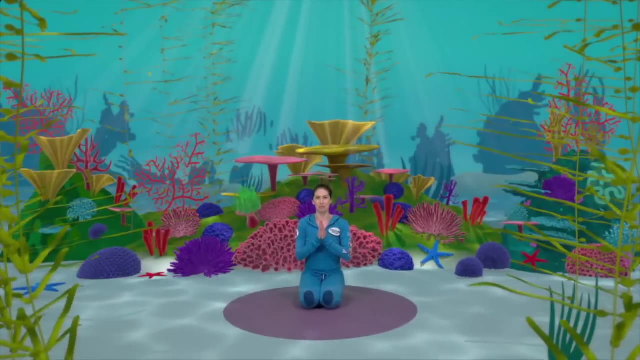 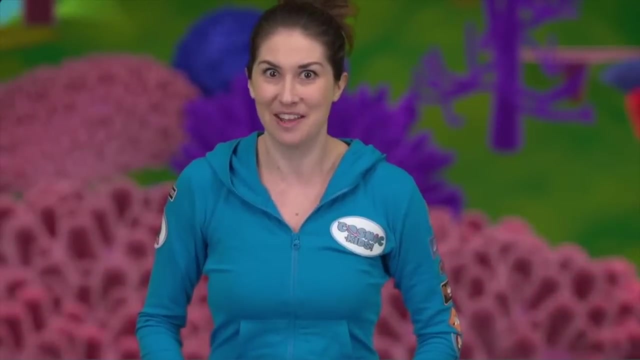 We land in a little landing ball. Oooh, We sit up tall And we say namaste to Bez, The blue footed booby bird, Namaste. Now to continue our journey. We pick up a lift with Popcorn the dolphin. 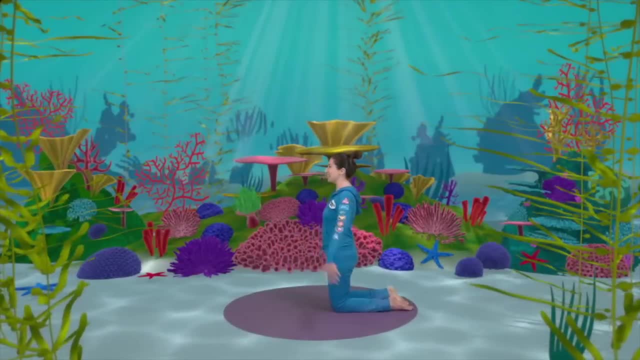 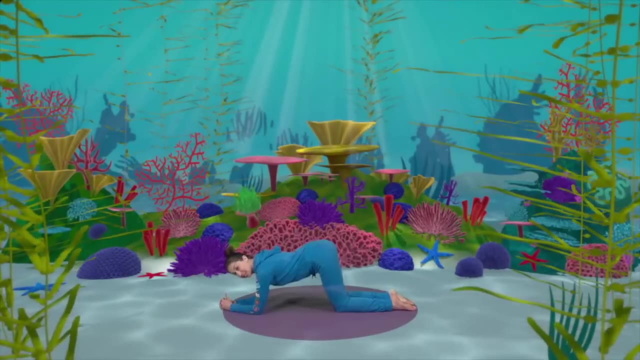 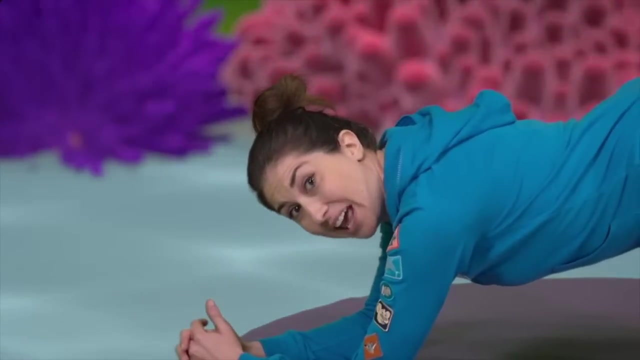 Who's riding the waves? Coming up onto your knees? Cross your fingers, Drop down onto your elbows. Now dive forward and backwards, making your dolphin clicky noises. She drops us off in the kelp garden, Turning over, Lying on your back. 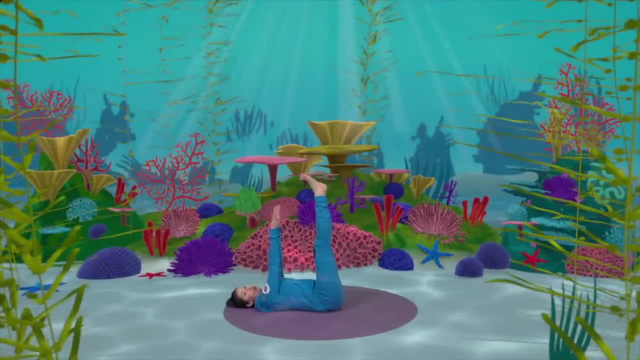 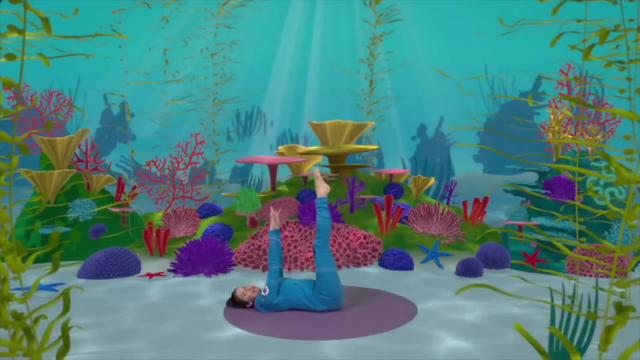 The kelp garden is long, long strands and fronds of seaweed That stretch right from the bottom of the ocean Right to the top. Now we need to swim, So we come over onto our tummies And we swim. 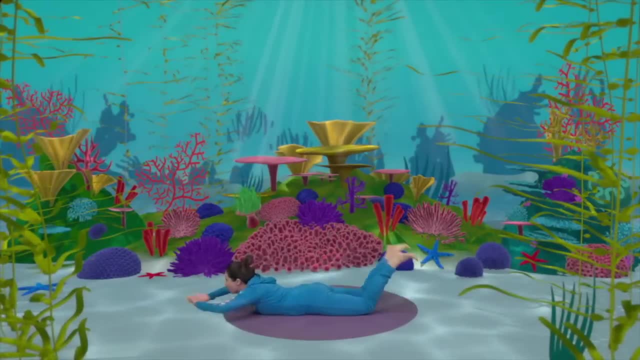 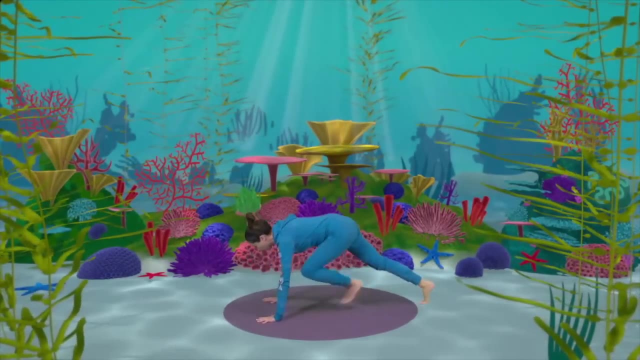 Using big strokes with our arms and our legs, We part the seaweed And we come to Norris, the baby seahorse's house, Standing all the way up, Take your feet wide, Take your arms wide And lift them up above your head. 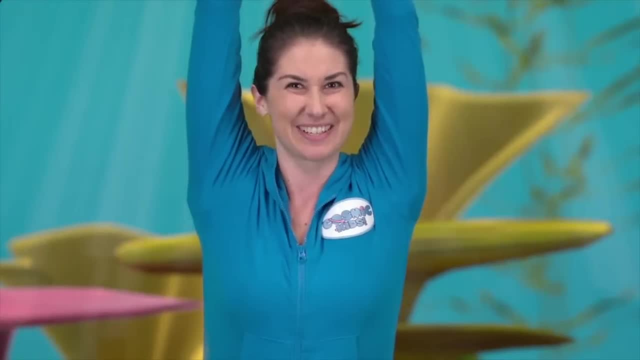 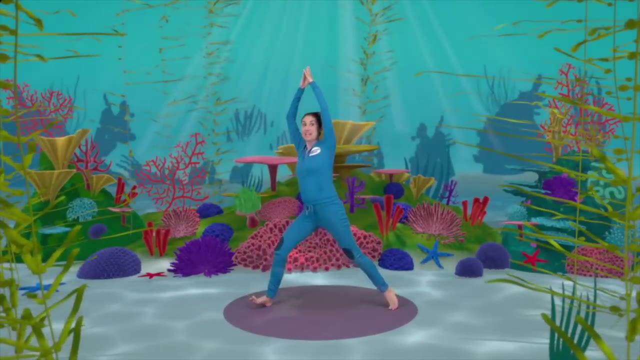 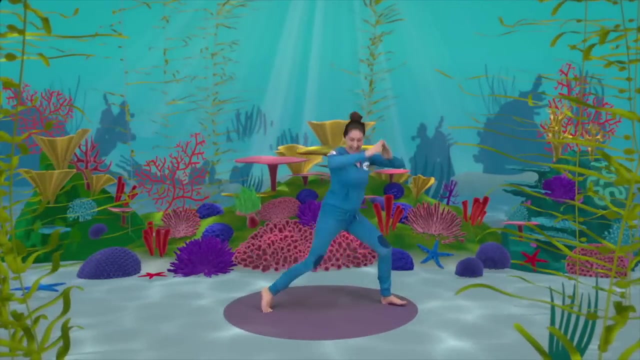 Coming into house pose And here's Norris, the baby seahorse, Coming down onto one knee. He does a little Knee. Now lift up that back knee, Turn yourself around And drop down onto the other knee, Knee, Standing all the way up. 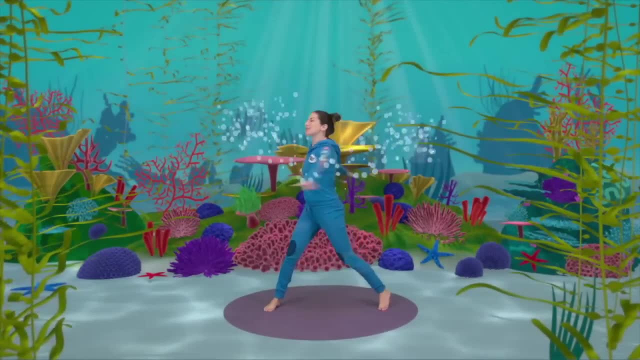 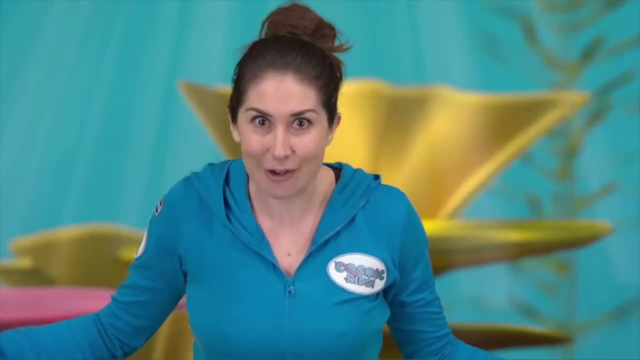 Arms wide Because we're such good friends with Norris. We do a twirl up in a flurry of bubbles. Norris is so excited Because today he got invited to join the best fish in the sea club. He's never heard of it before. 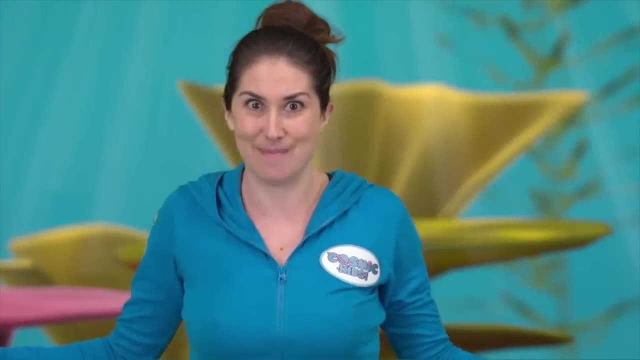 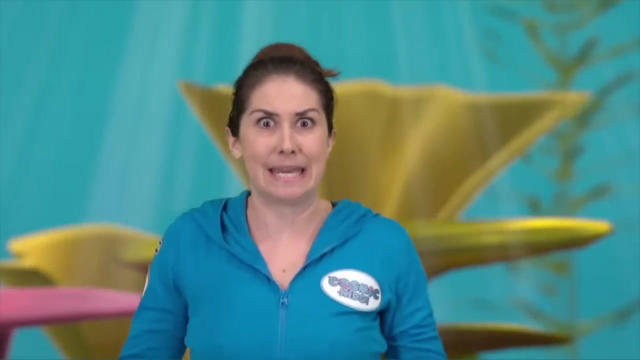 But it's called best fish in the sea club, So it must be the best, Right? He's got his first meet up today at the coral reef cafe. He's so excited He sings a little song. We join in with the actions. 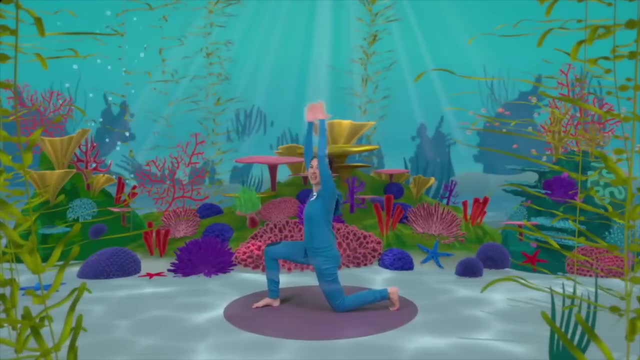 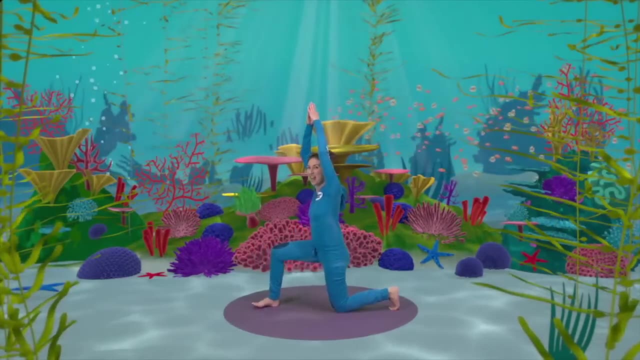 Ready, Come down to one knee. My name is Norris, I'm a tiny little fella, But my nose is long And my body is so yellow. I rock like a rocking horse, Gliding through the sea. And I tell you now. 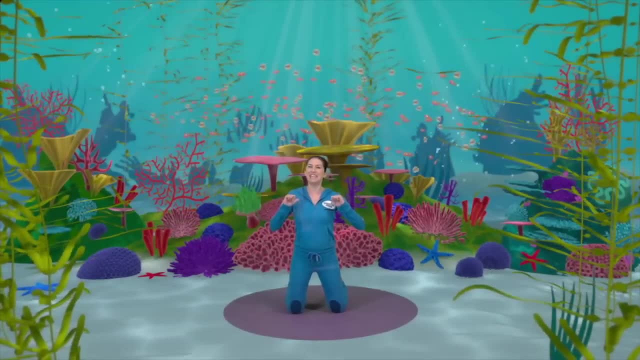 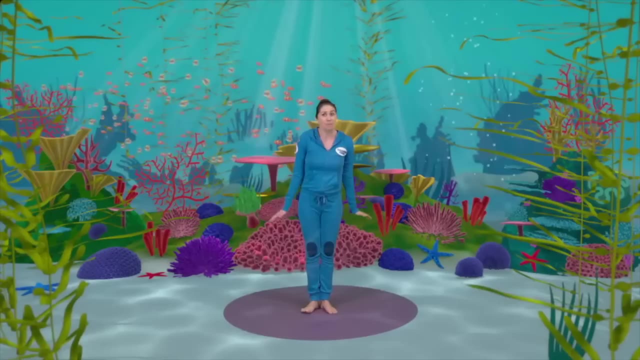 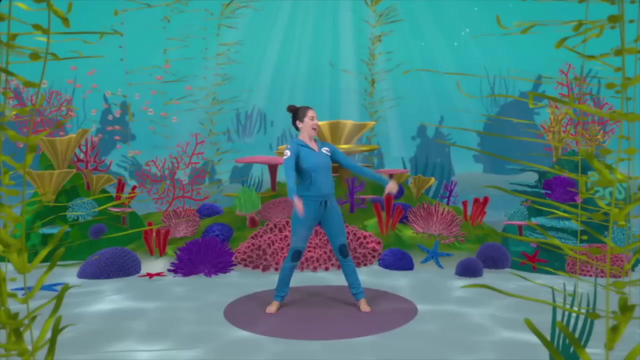 That I love being me Standing up. I swim standing up And I may be slow, But that never stops me having a go. I'm the best baby sea horse you ever did see. Like I said before, I love being me. 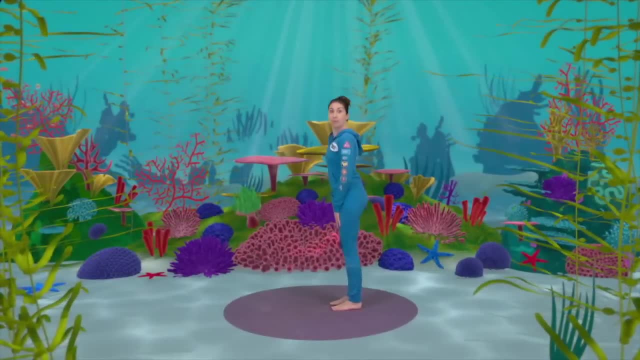 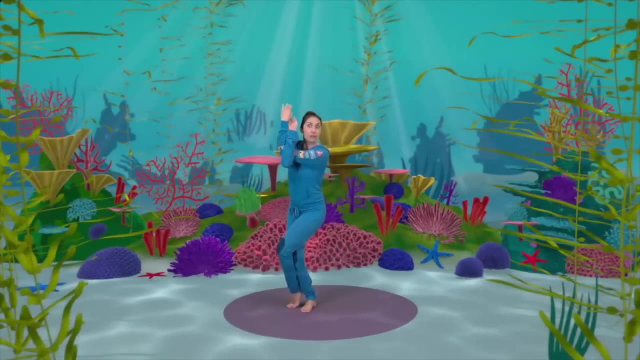 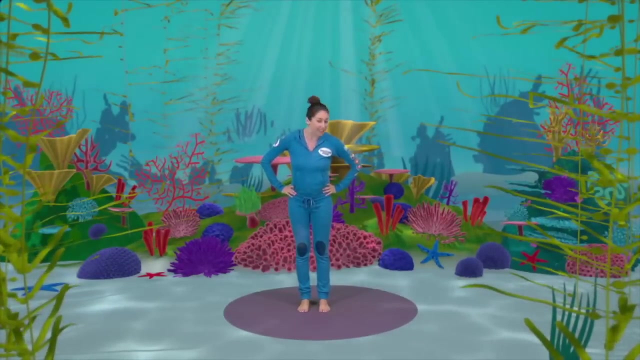 My tummy's round And I bob up and down And I'm made out of bony rings. I like to hold onto a seaweed frond And take a rest frequently. I can wiggle my nose around and around. I look with my eyes both up and down. 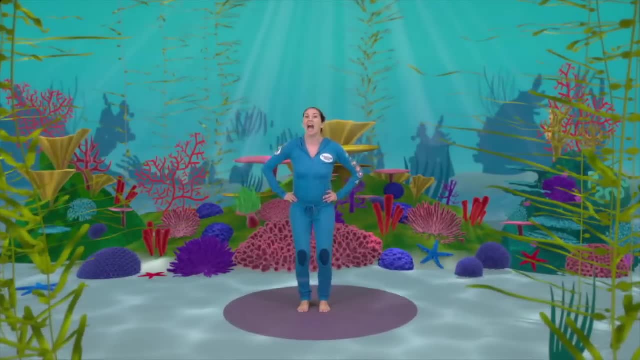 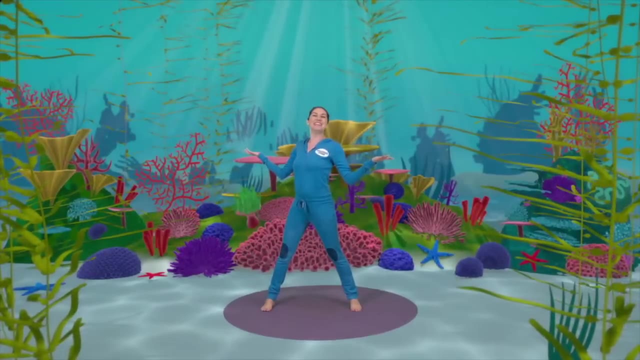 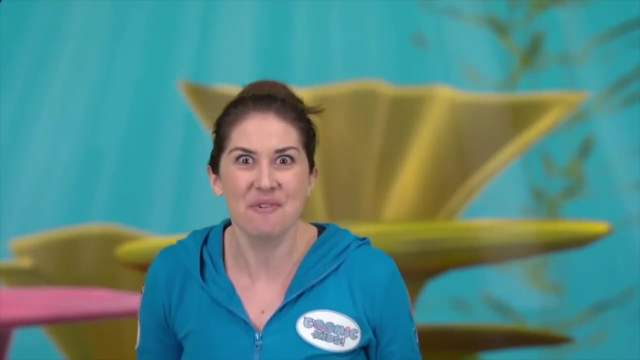 I'm a bright spark. clever lad diddly-dee, I'll tell you again: I love being me, I love being me, I love being me. That's right. Wow, What a great song, Norris. But, Norris, we'd better go, because time's running out. 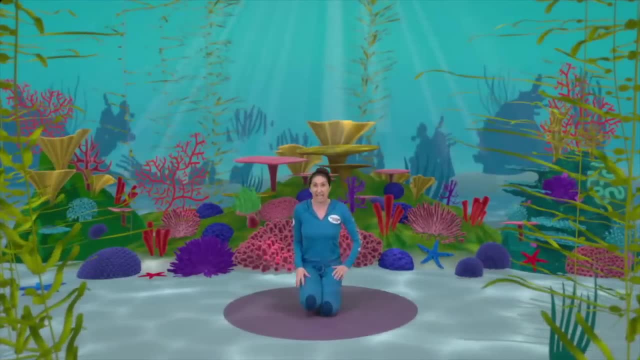 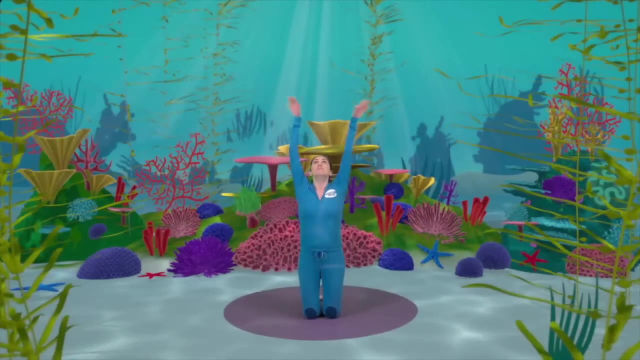 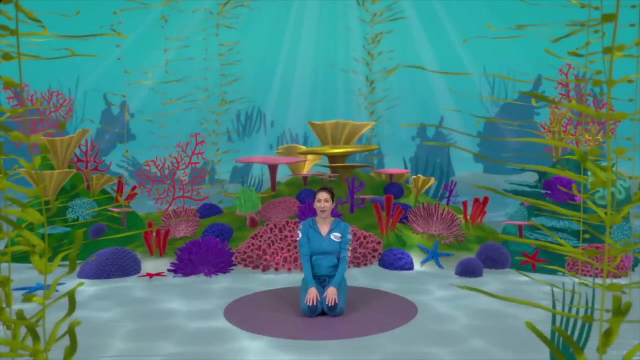 and we know you're a little bit of a slow swimmer, so come down to your knees, let's go. Come down to your knees. everyone hands down swimming up, slowly breathing in. On our way to the Coral Reef Cafe, we pass Mimi the Mermaid. 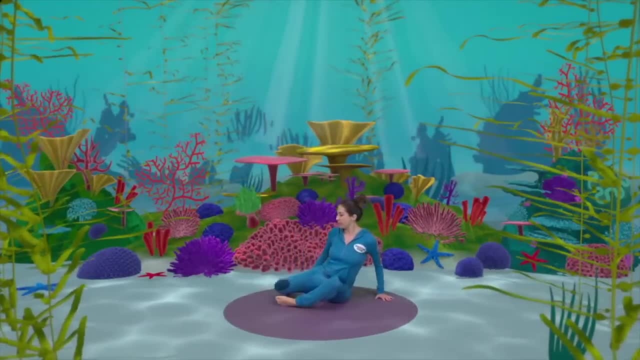 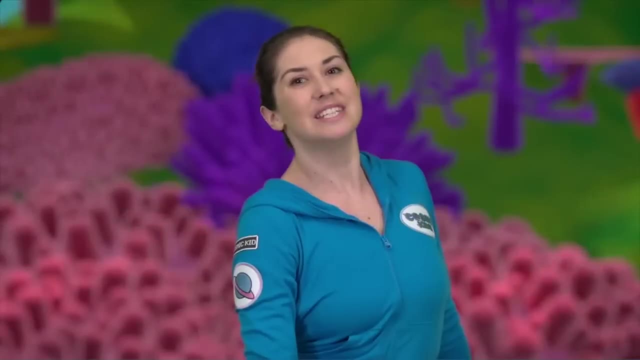 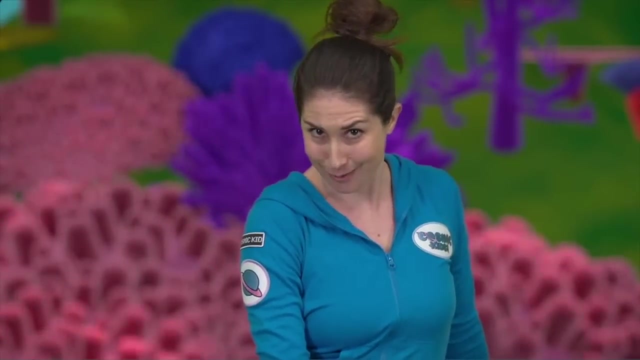 sitting with your legs out long, swish your tail around to one side, put one hand on your fishy knee, your other hand behind you, look behind you and look forward. she says to Norris: Bonne chance, petit Norris, which means good luck, little Norris in French. 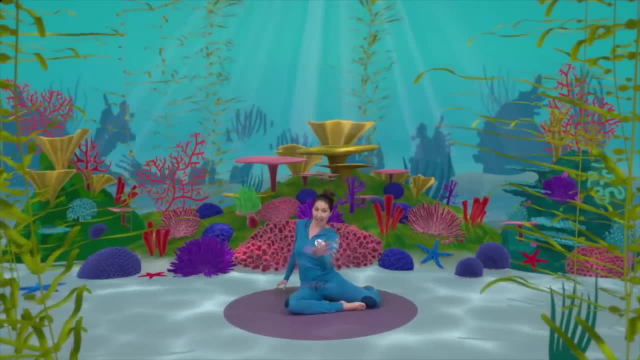 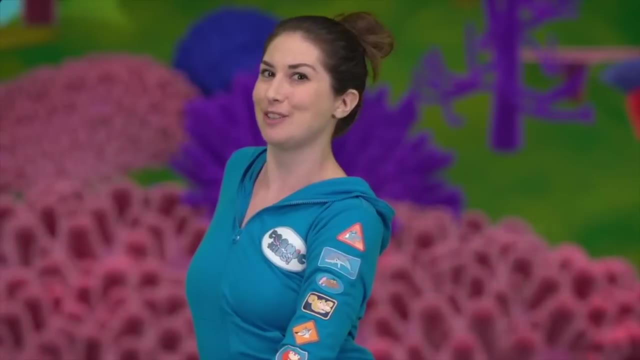 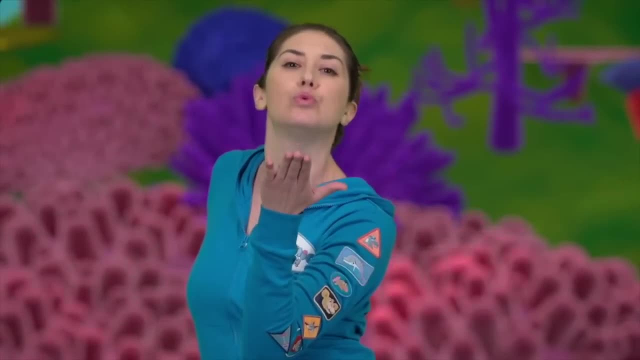 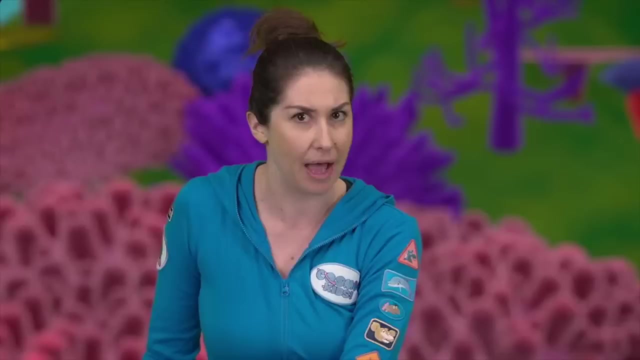 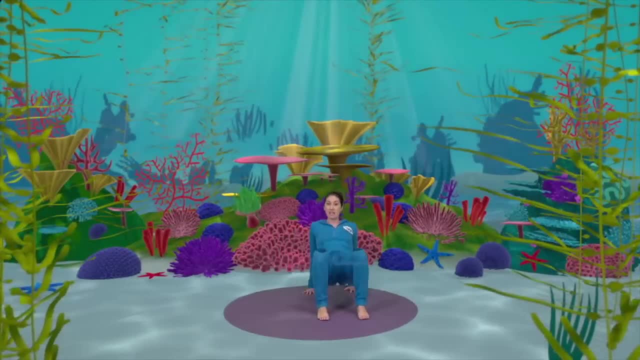 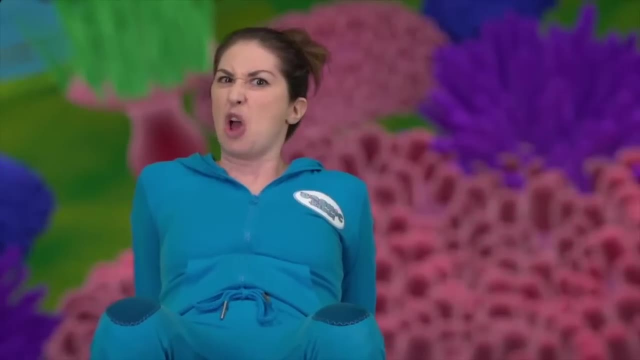 coming up, bent knees, hands behind you, lift up your bottom now. digger, digger, ready. Digger, digger, digger, digger. Oi, you big nose. You can't join the best fish in the sea club, your nose is too big. Then he digger diggers the other way. 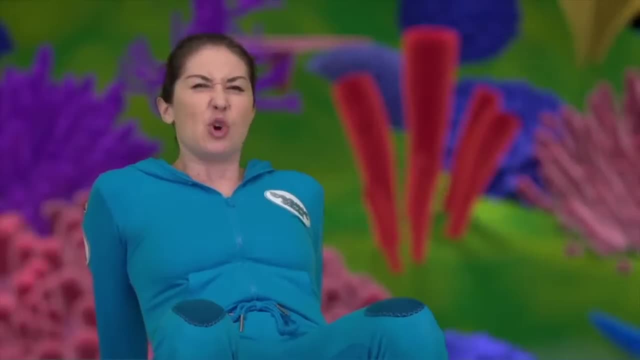 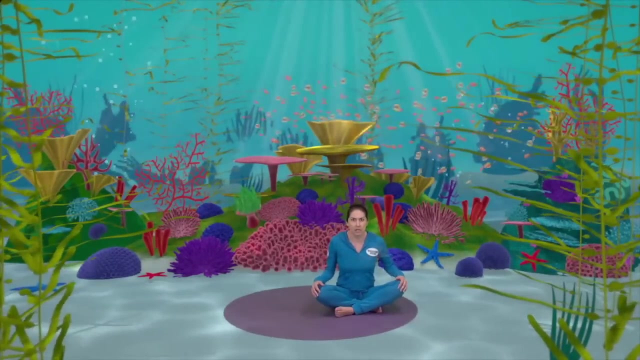 Digger, digger, digger, digger, And if you join, I'm gonna pinch you on the nose with my crab claws. Yeah, Oh, poor Norris. He's feeling a bit upset by that, but he doesn't want to say anything. He doesn't want to upset anyone, so he. 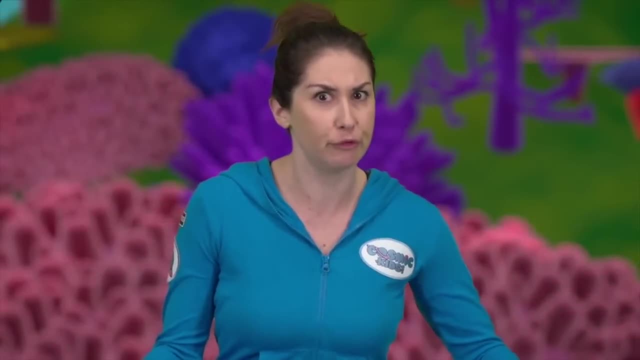 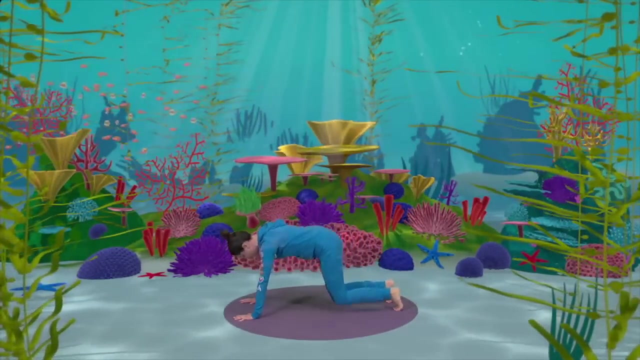 carries on. Then overcome a pair of wolf fish coming into your dog. pose Hands down, tuck your toes. lift your bottoms to the sky. Come all the way down to your knees. Untuck your toes, Lift up your chest. Alright, Boney, you want. 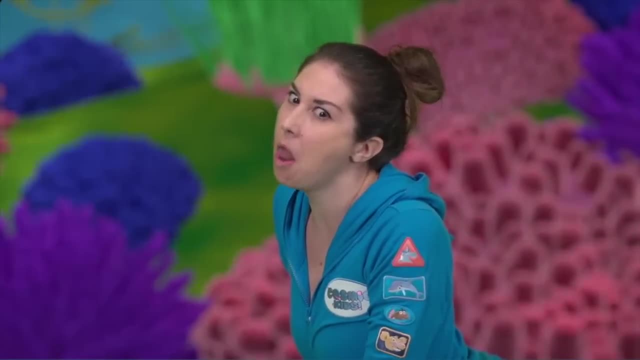 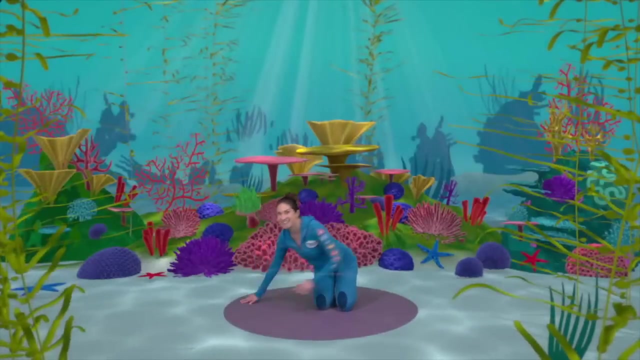 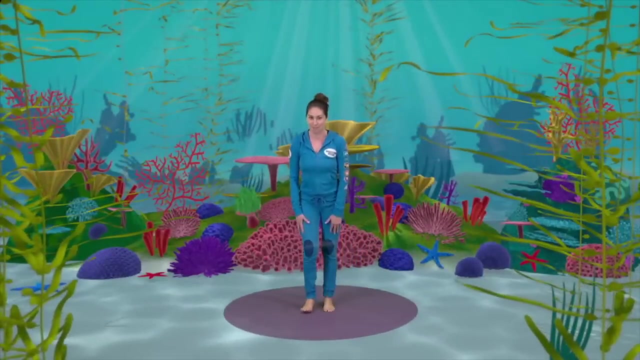 to join the best fish in the sea club, do you? Well, you can, if you can, show us a tree pose. Oh, Norris is quite pleased that they've asked him to show a tree pose. He's rather good at tree pose. He stands up and shows them. I put my foot on. 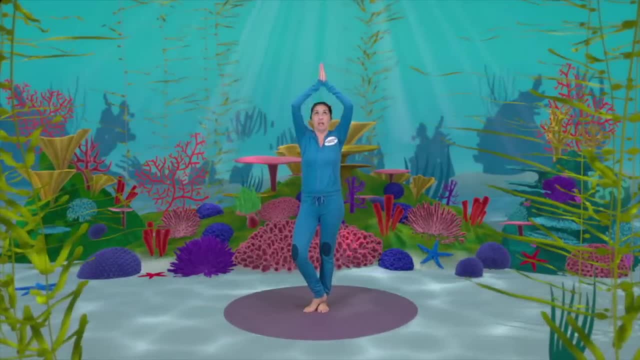 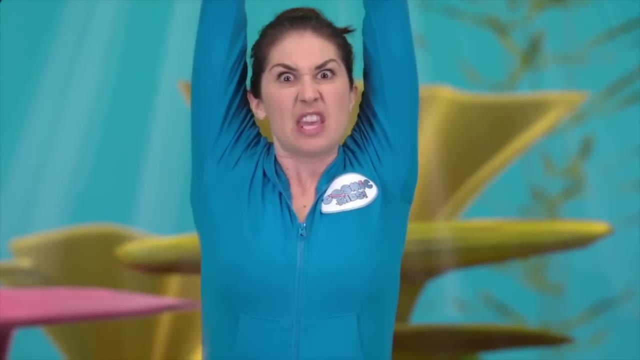 there. I put my foot on there. I put my foot on there. I put Finn's here. I grow my tree There. there's my tree pose. Norris is great at tree pose. He even shows them on the other side, just to show he can do it on that side as well. 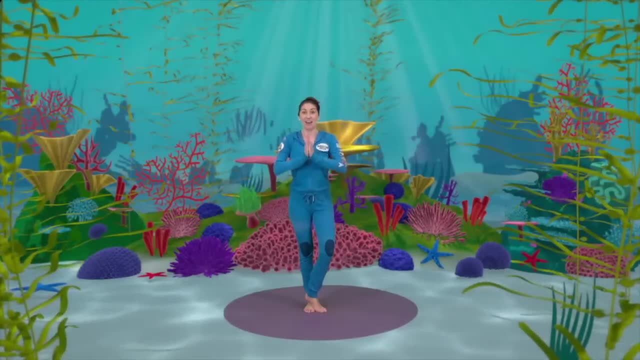 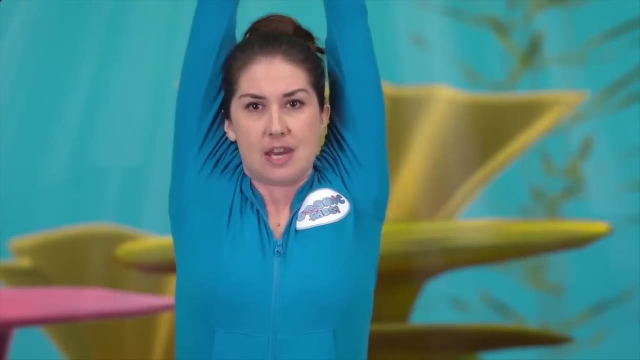 Swapping our legs over. now put your other foot on top hands together. grow up tall. Yep, you see I can do the tree pose. doing it. yep, The wolf fish seem to make a fool out of Norris. 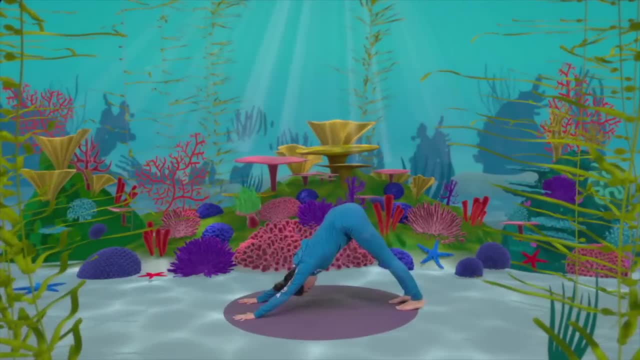 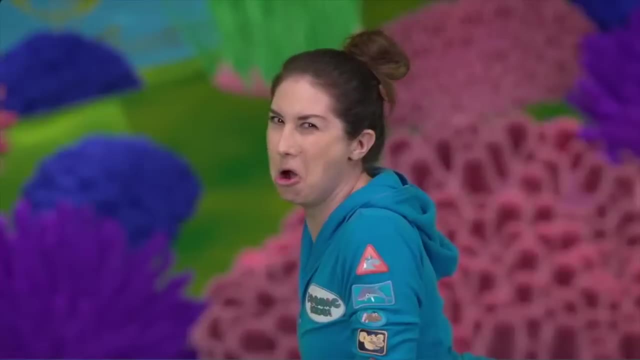 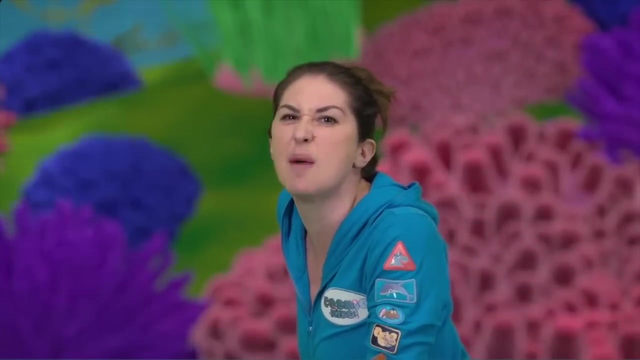 Coming back into your dog pose, lifting your bottom to the sky, dropping down to your knees, untucking your toes all the way to your belly and press up. Only joking, Boney, You can't join the best fish in the sea club because you've got a big, silly round tummy. 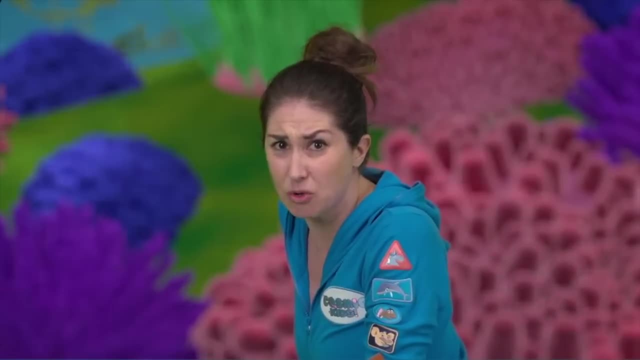 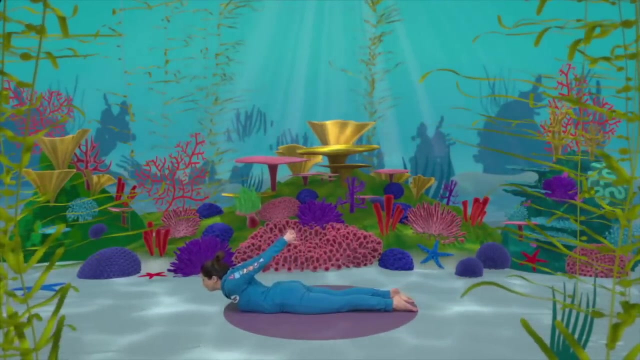 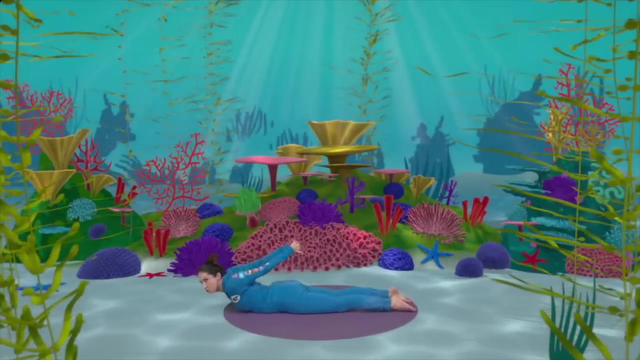 Oh, poor Norris. This is not very nice at all, And over now is swimming a shark. Crisscross your fingers behind your back, Lift up your shark fin. She's swimming right towards Norris. Excuse me, My name's Shona. I'm a shark. 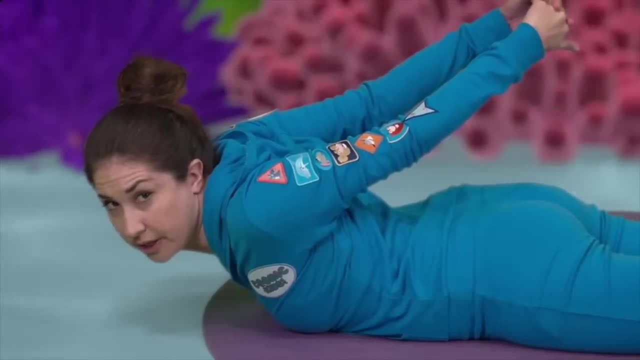 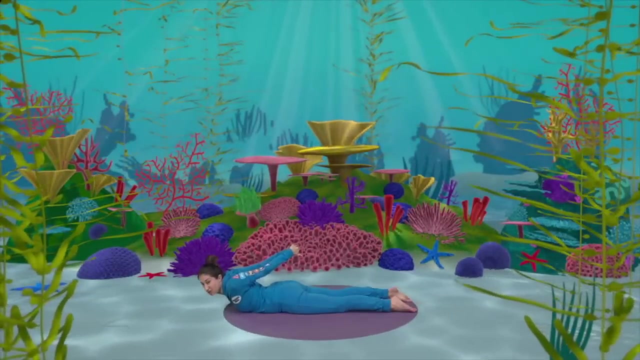 I just wanted to let you know that apparently you can't join the best fish in the sea club because apparently you're a really slow swimmer. That's what the crab and wolf fish said. so sorry, I'm just telling you, See, ya. 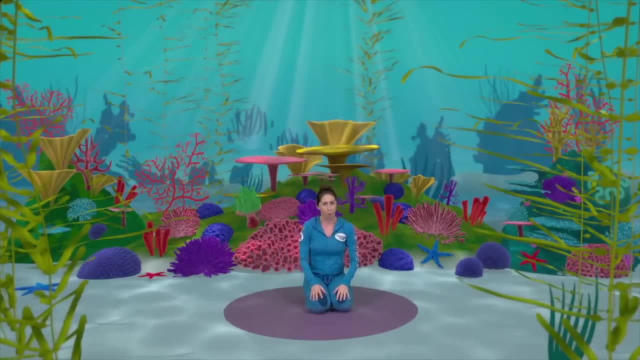 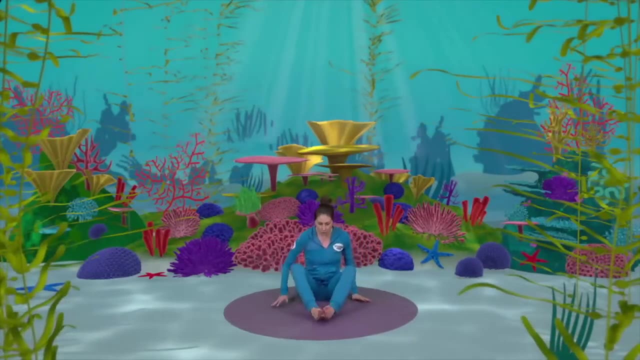 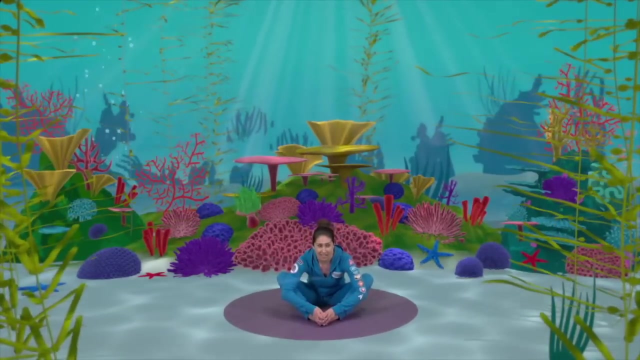 Oh, this is awful. We take Norris for a little bit of a rest. in an oyster shell, Sitting on your bottoms, join the soles of your feet together, Holding onto your toes folding down. This isn't the best fish in the sea club. 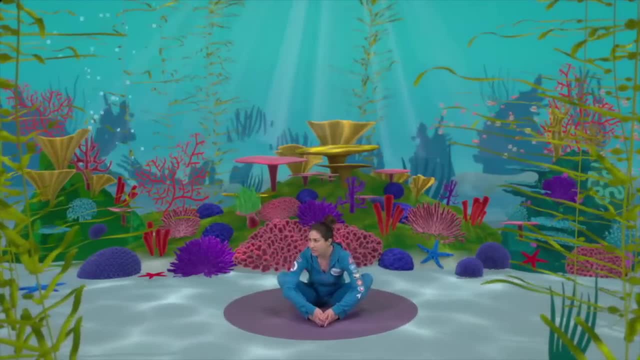 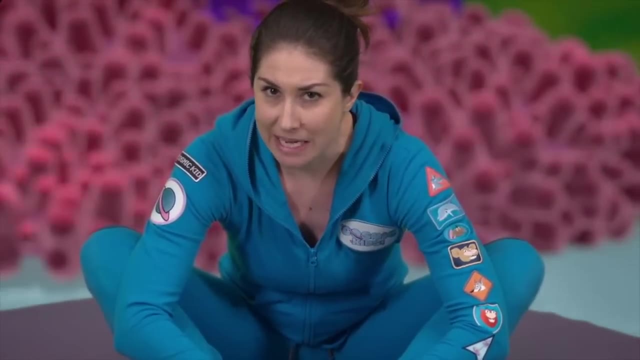 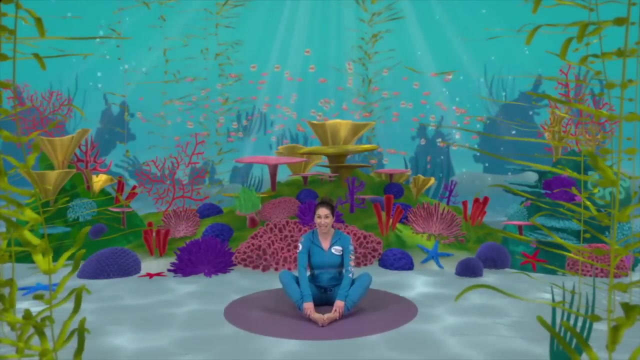 This is the worst fish in the sea club. All of these horrible creatures are bullying Norris. That's not right. Hmm, When this happens, we need to speak to a wise grown-up friend. And here come just the people we need. It's Tommy, the bedtime turtle. 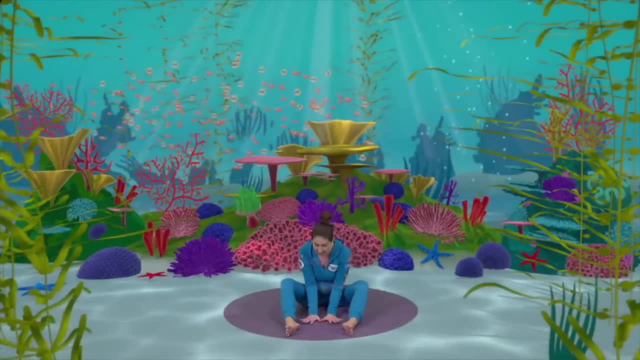 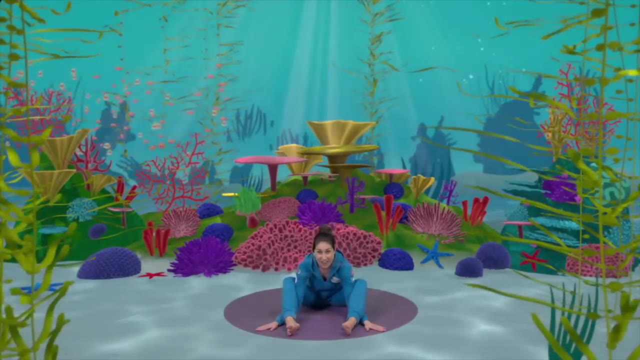 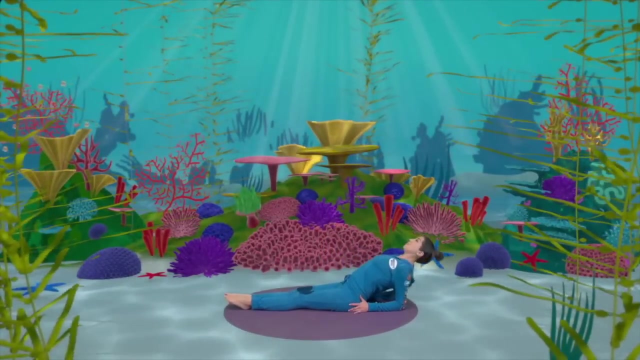 Take your legs out, wide bent knees, hands down underneath, making your flippers like a turtle, And with him is our very good friend. Squish the fish, Pointing your toes long, come down onto your elbows Now, pop, pop, pop, pop, pop your chest to the sky. 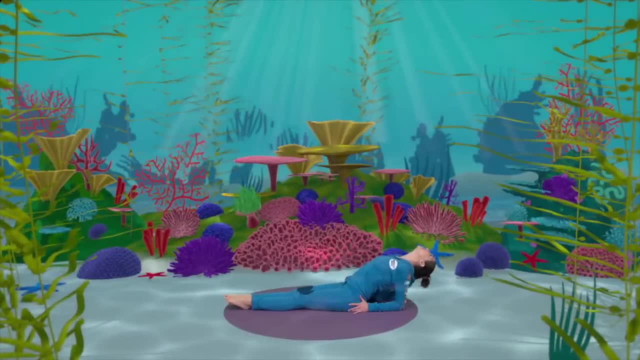 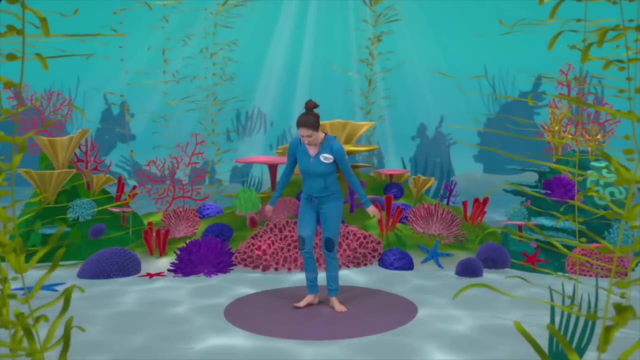 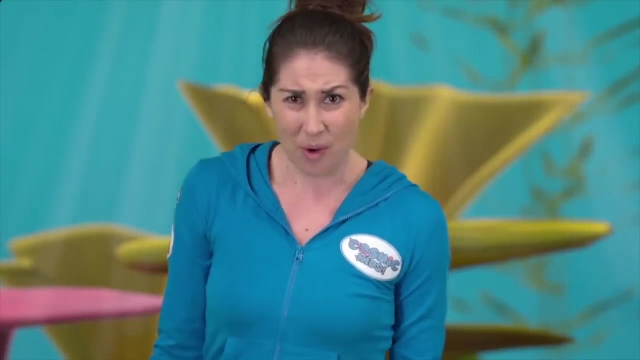 Looking up to the ceiling and all the way back behind you. But Squish, as usual, is using his tail as a surfboard Standing up, So he looks a bit like a penguin. Hey, dude Norris, why the long face? What's going on? 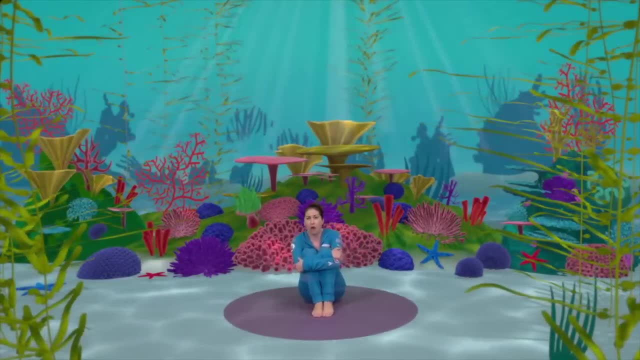 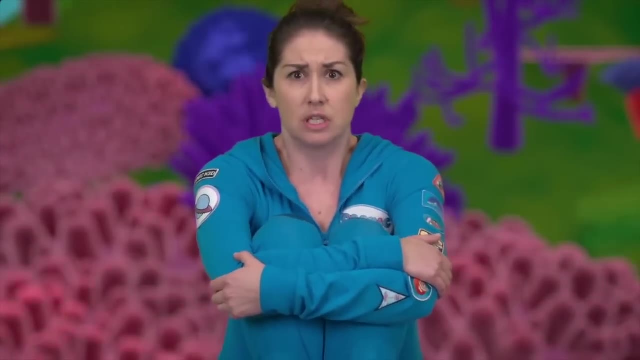 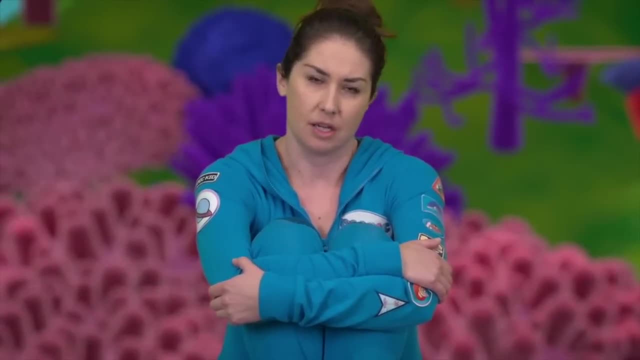 But they said I can't because my nose is too long and my tummy's round and I'm not very strong at my swimming. Tommy the Bedtime Turtle thinks this is awful: Taking your legs out, bend your knees, hands down, making your flippers. 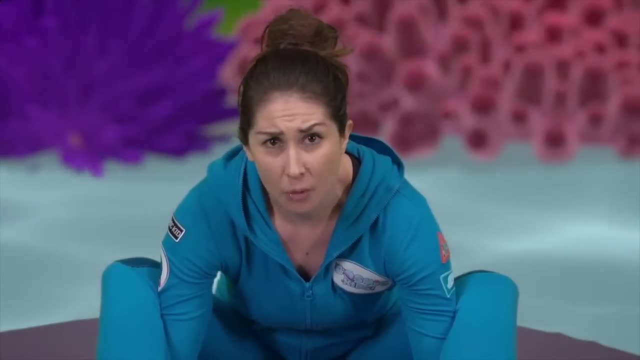 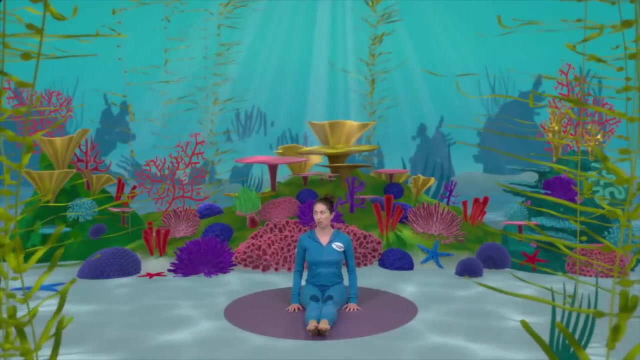 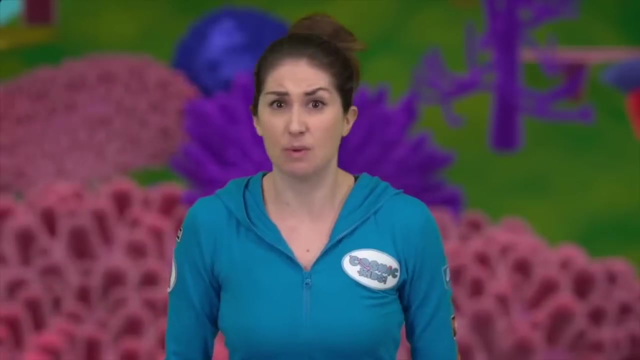 Oh, Norris, you're a wonderful sea horse. What do you think about this? Norris sits up. He unravels his tail sitting up tall. Well, I quite like my nose and my tummy And I don't like swimming fast, because if I swim fast I get all tired and stressed out. 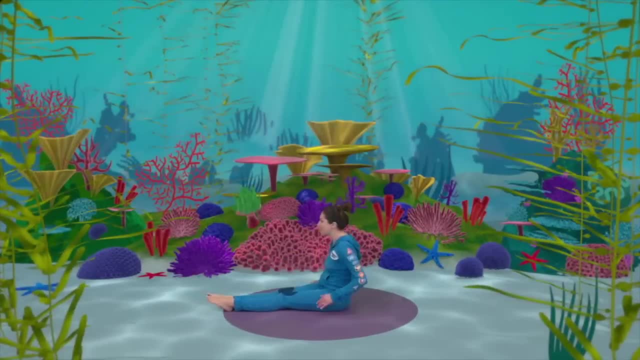 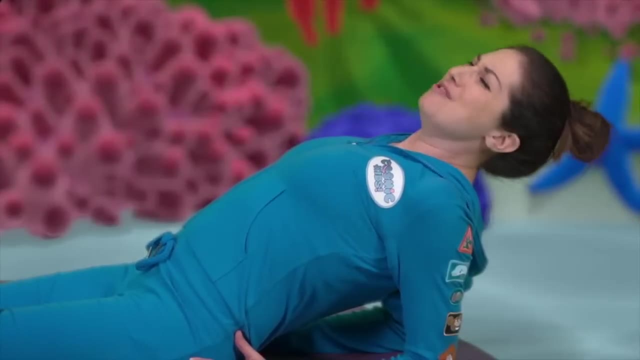 Squish reclines in his fish pose. coming back down to your elbows, point those toes. pop, pop, pop your chest to the sky. Dude, you know it. you don't need to be in this club. best fish in the sea club, it's not at all. why don't you start your own? 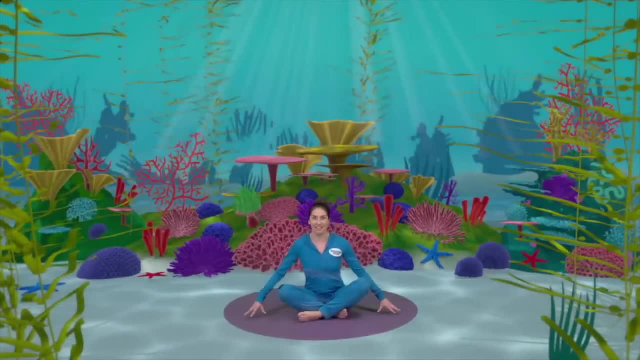 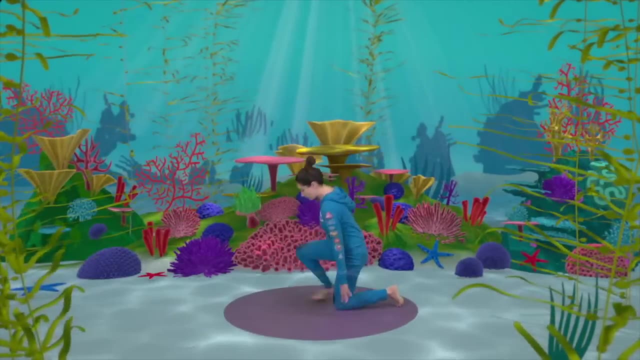 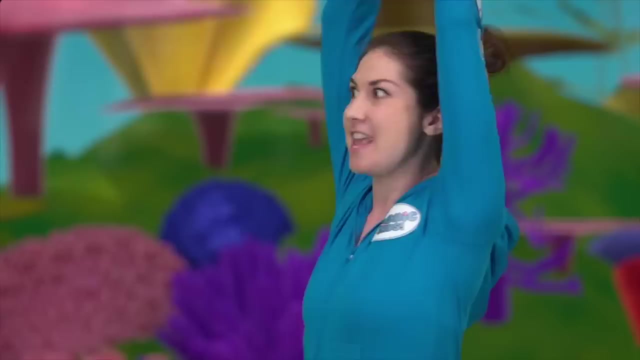 club At this Norris gets excited. yeah, I'm gonna start me own club, coming back onto one knee into your horse pose lifting your hands above your head. Yes, I'm going to start it and I'm going to call it the I love being me club and 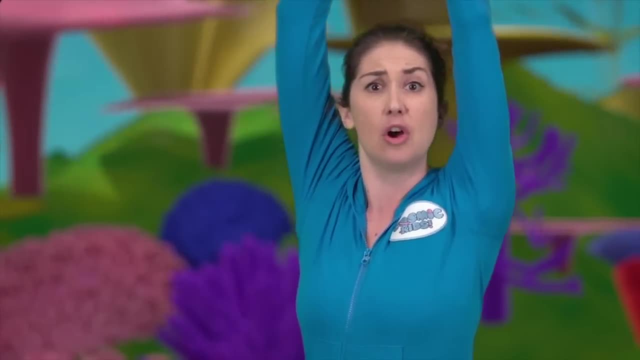 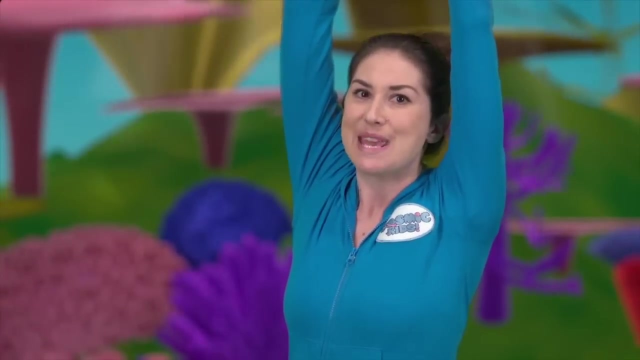 anyone can join, whether they've got a long nose or a short nose, or a little tummy or a big tummy, or whether a fast or a slow swimmer. you just got to be nice in the I love being me club. Norris was over the moon, but coming over was. 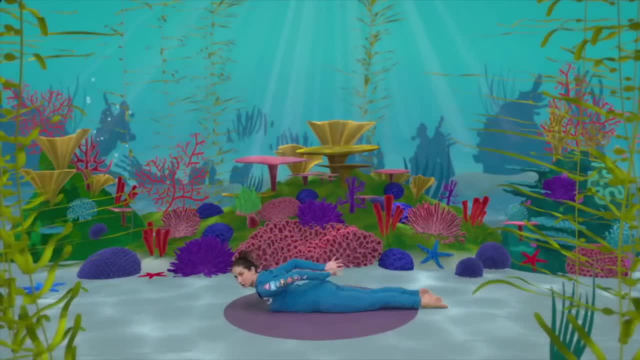 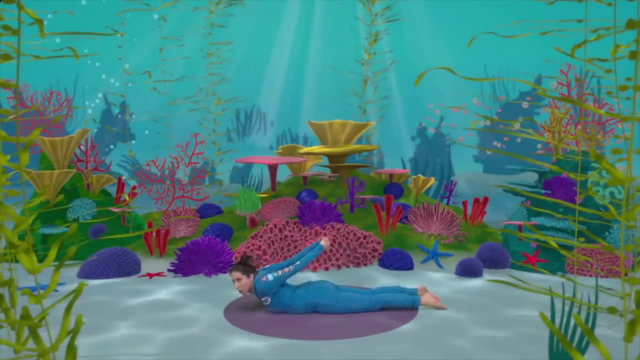 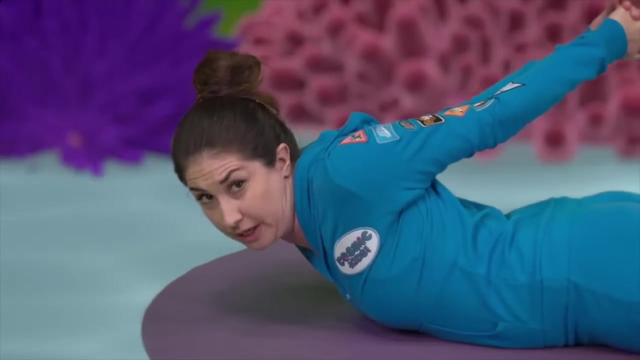 Shona the shark Coming back onto your belly, crisscross your fingers, making your shark fin lift it up. Excuse me, is Shona again? Yeah, I'm a shark. I just wanted to ask: could I join the I love being me club, because I'm just really fed up of being in the other club. they kept. 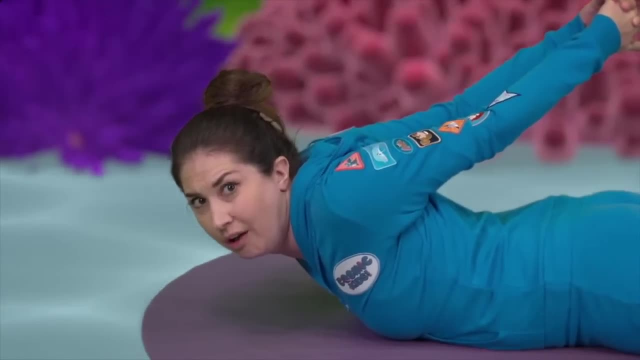 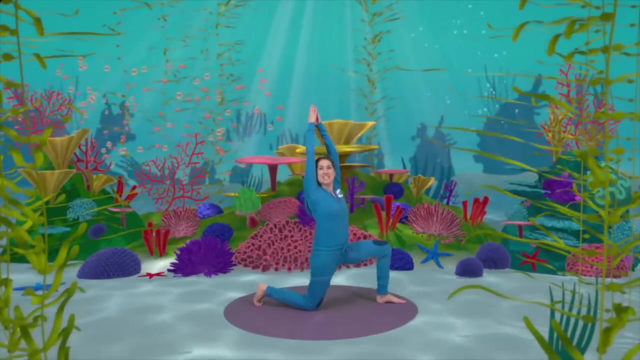 telling me what to do and what to say, and I didn't like it at all. Norris is delighted Coming on to the other knee now, lifting yourself up, arms up and above your head. Yes, Shona, you can join. you're very welcome, Soon. all of the 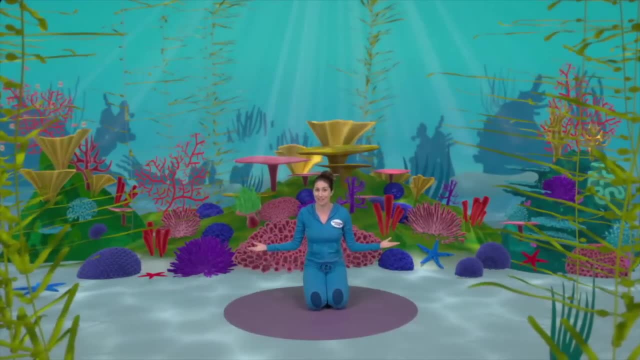 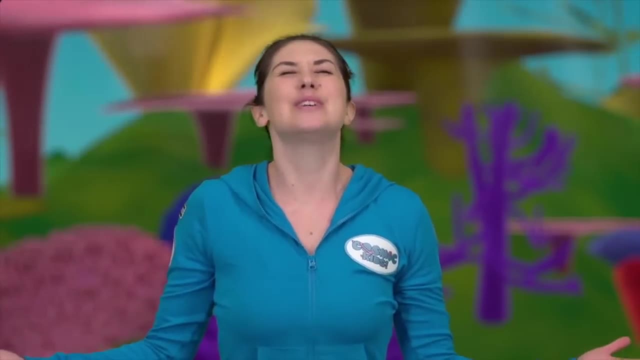 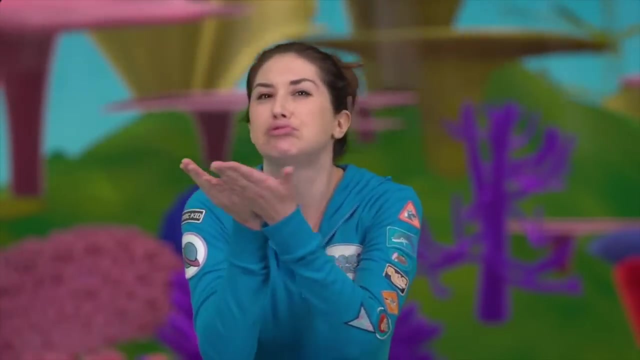 animals and creatures from the best fish in the sea club started to join Norris's- I love being me club. He'd done it, he'd started his own club and he was delighted It was time for us to go. so we blow our bubbly kisses to all of our 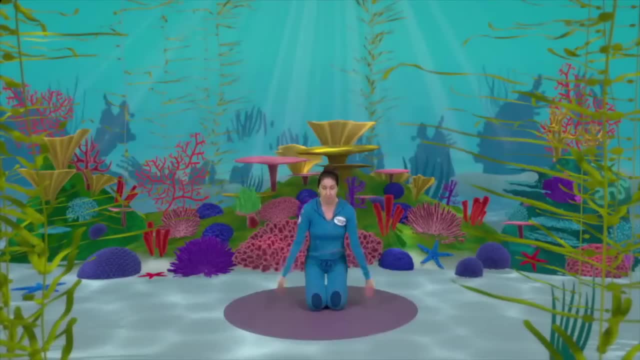 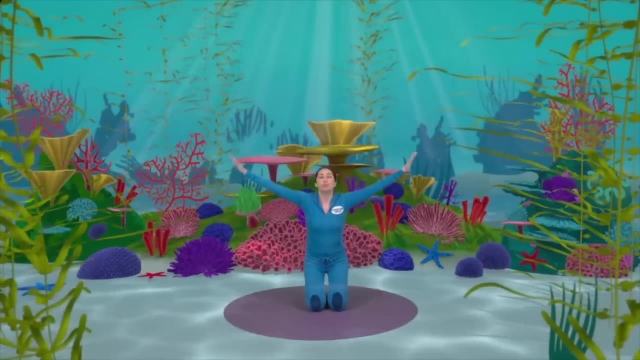 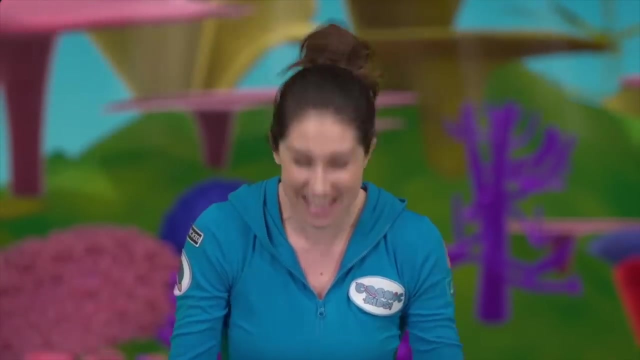 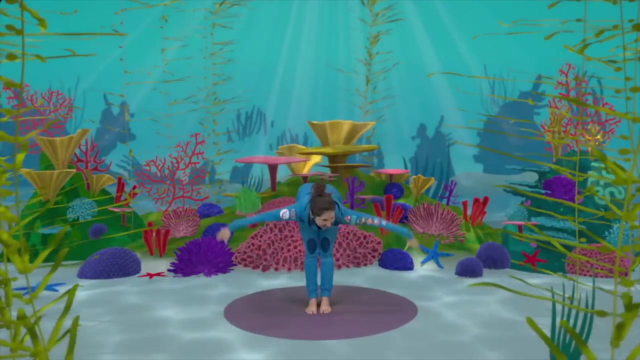 friends and we swim up back to the surface of the sea. When we get there, we find our friend Bez, the blue-footed booby, standing up. we bow all the way forward, taking our wings down, and then we swoop them up and high. We're off, being transported back to our house, back. 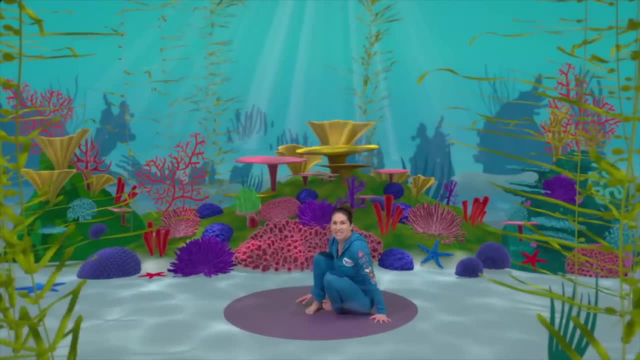 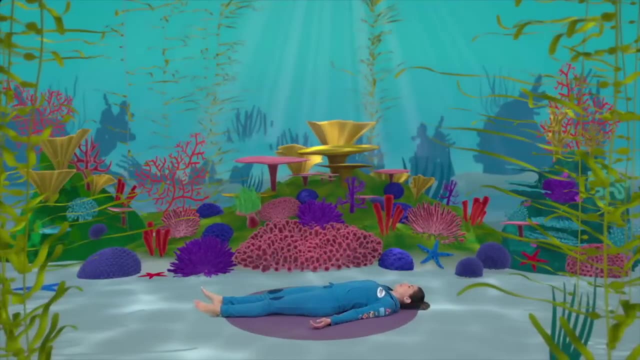 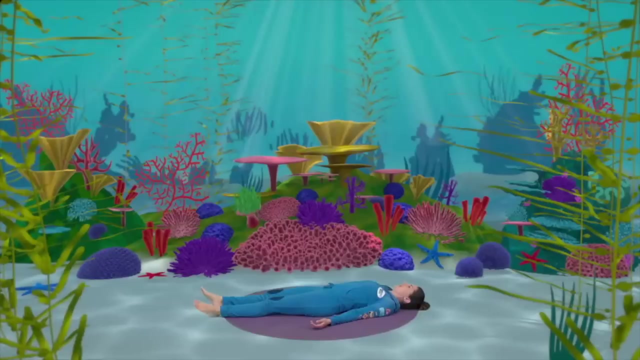 to the warmth. We lie down on Bez's back in all of his feathers and let our bodies rest and relax for a moment as we think about the story we've just done with Norris, How he went through some really awful things- Bullying, Saying, 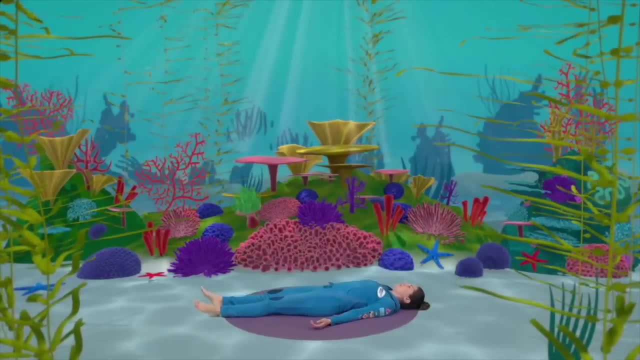 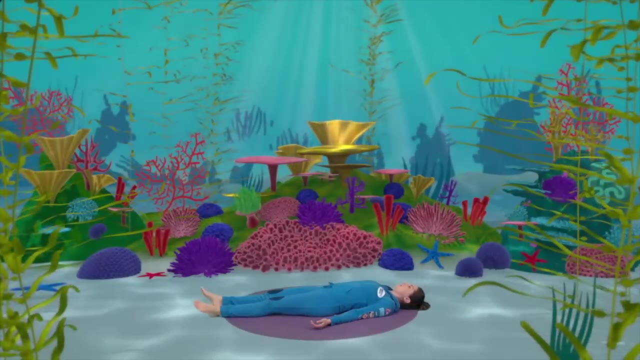 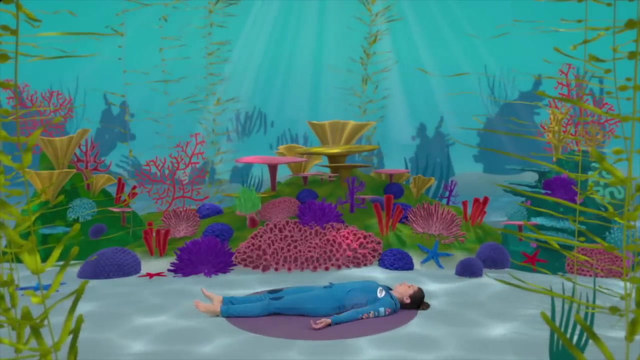 those things is never okay. Or getting someone else to say nasty things about you is never okay, And if it happens- and it might happen to a friend- you might see it happening. you must always go and tell a grown-up And you don't need to worry about being a tell-tale. 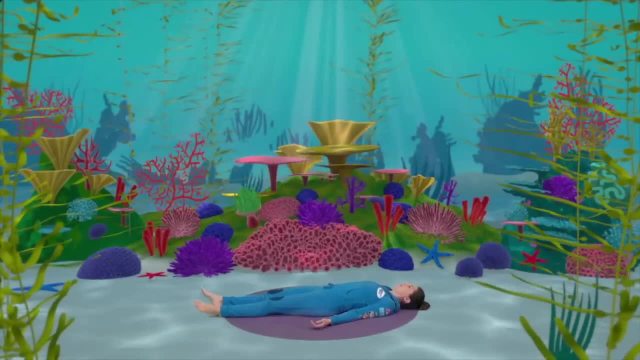 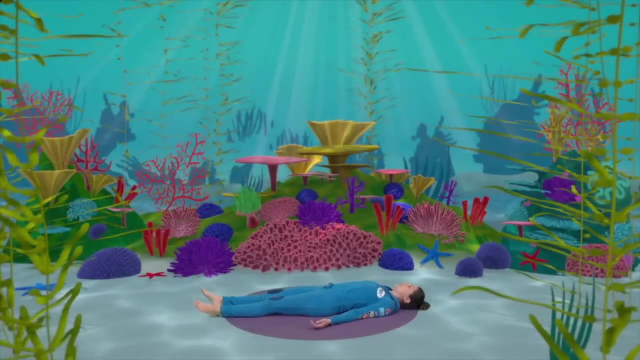 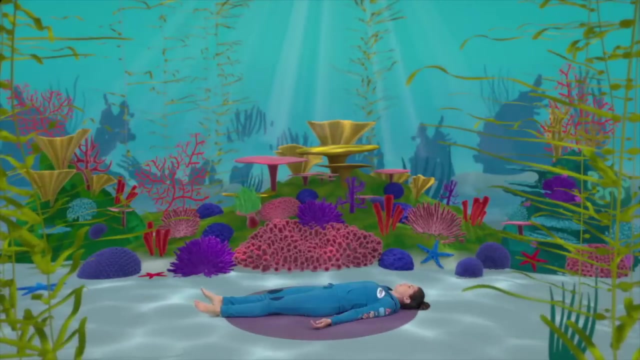 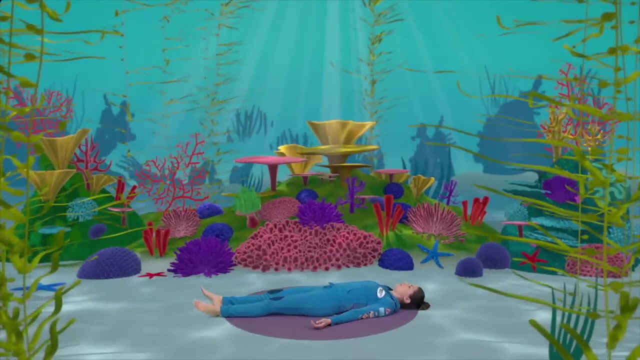 at all. You're not. You're helping, Because that bully probably needs some help too. They sometimes do these things because they feel weak inside, So they need to feel more powerful by saying these things about others to make them look weak. But it's not okay, And we must always go and tell a grown-up when it happens. We 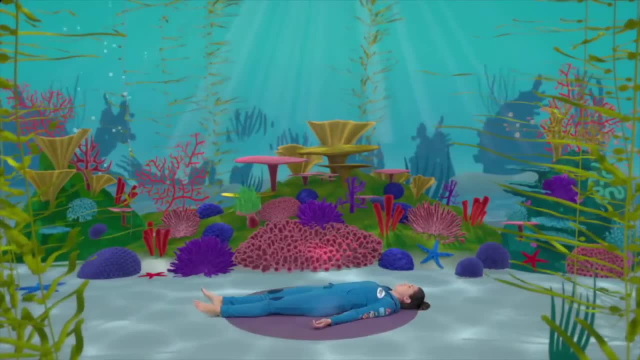 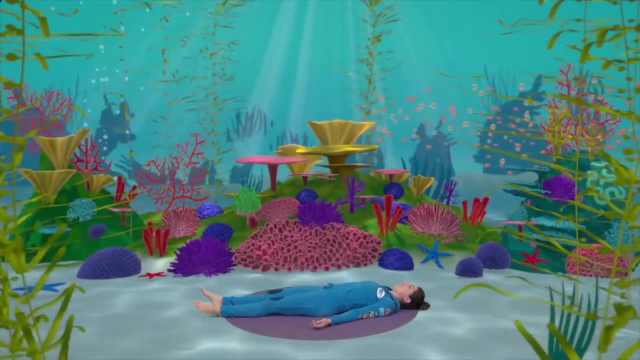 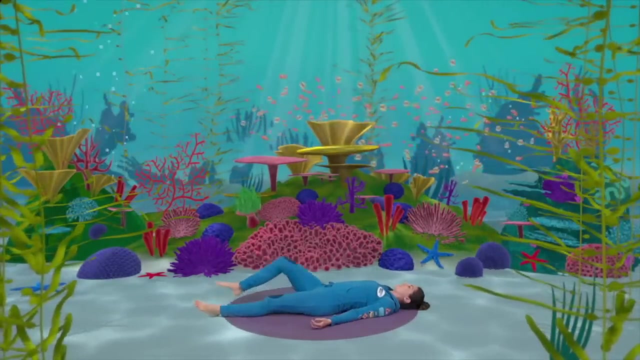 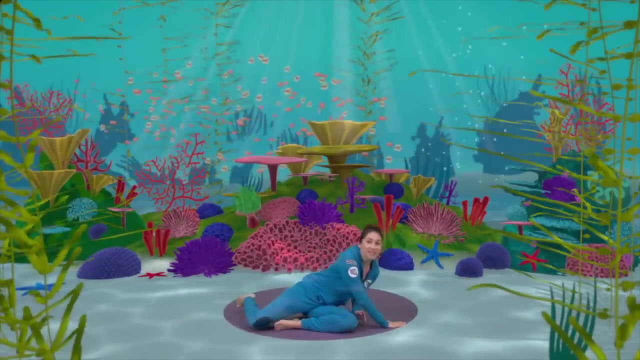 rest back in this peaceful time. So pleased for Norris. We love the I Love Being Me Club. What a fun thing. But now we wiggle our fingers and our toes, We bring our knees up to our chest And we roll over onto our sides, Slowly coming up to sit With our legs crossed And our hands. 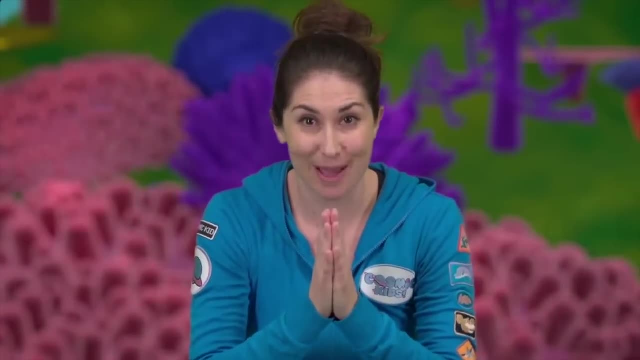 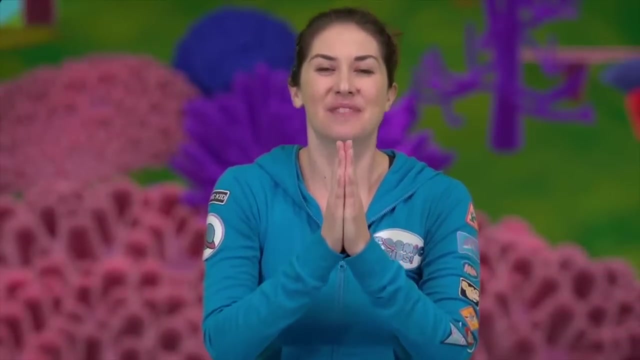 together at our hearts And we finish just the way we started with our secret yoga code word, Which is: Namaste, Ready After three, One, Two, Three, One, Two, Three, One, Two, Three, Namaste. 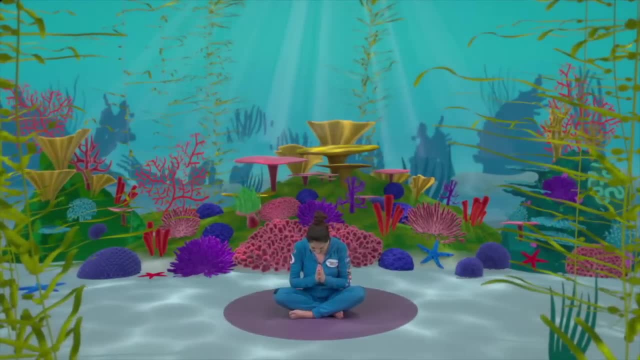 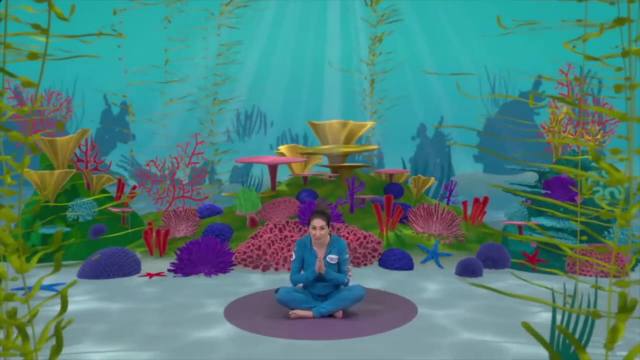 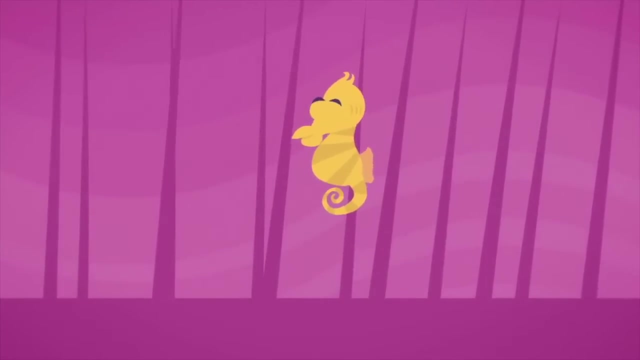 Namaste, Namaste, Namaste. Well done everyone. Thanks for coming on the Norris the Baby Seahorse Adventure with me. You were great. I hope you enjoyed it And I hope to see you soon for another Cosmic Kids Adventure. Bye, bye. 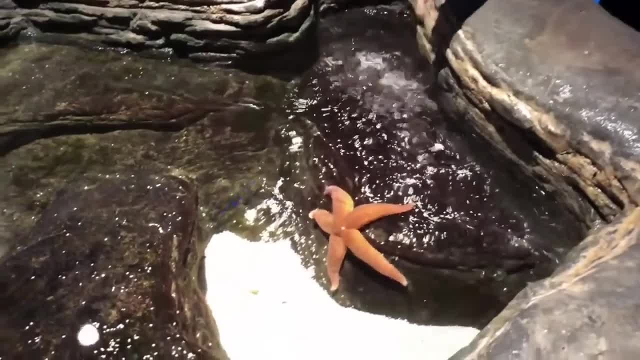 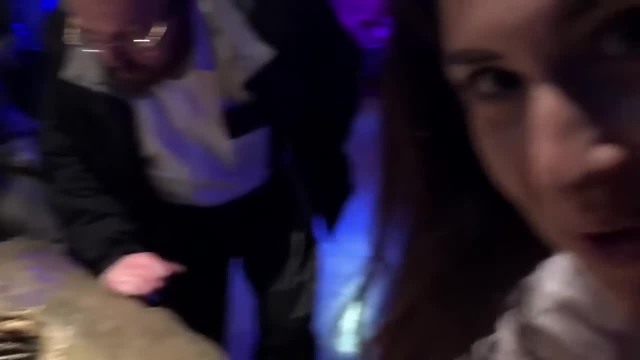 So I'm here, We're here. We're here with a starfish, a real-life starfish. Hi, can you guys cut the starfish for me? Let's pop a little finger in there, Give him a stroke. 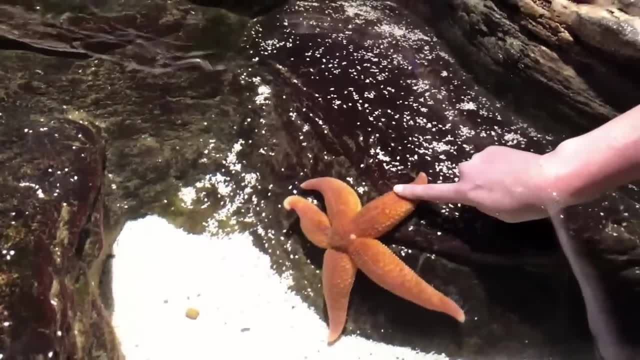 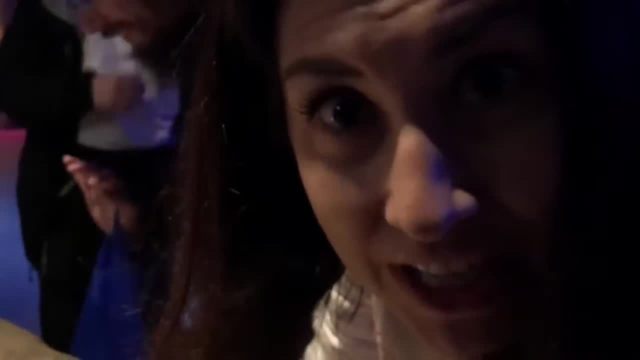 Oh, really, Yeah, Oh wow, What an amazing being, So cool. Now we've got a special video all about a starfish. It's a peace out, so let's go and enjoy that now, and I'll see you afterwards. 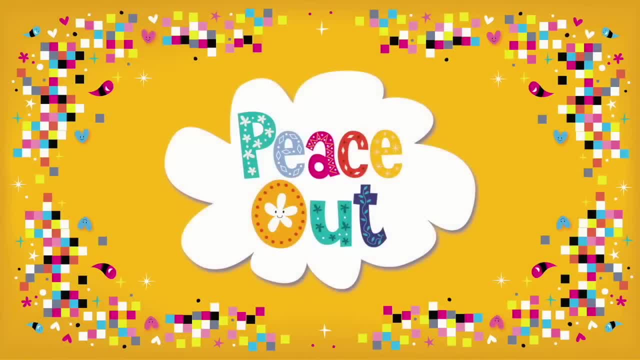 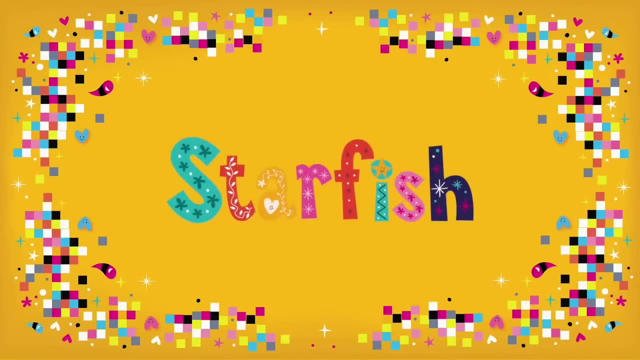 Peace out Starfish. Hello, Jamie here, Welcome to Peace Out. First, find yourself a space on the floor to lie down, big enough so you can have your legs and arms stretched out in a star shape. To start off, just be in a relaxed star shape. 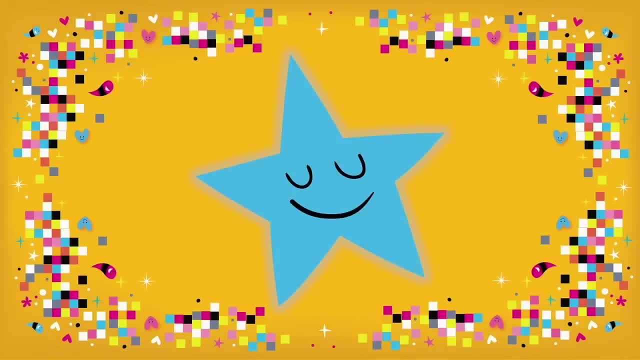 Get settled and do any last fidgets you need to do to feel happy and comfortable here. Take a couple of nice deep breaths in through your nose and out through your mouth. in through your mouth, in through your mouth, in through your nose. 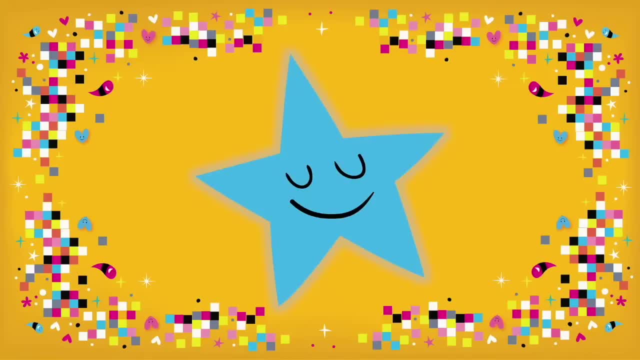 and out through your mouth And with this next breath out, let your eyes gently close. Well done, Now you're settled. You're ready to be a starfish. Can you imagine a starfish with five points coming out from the top of its head? 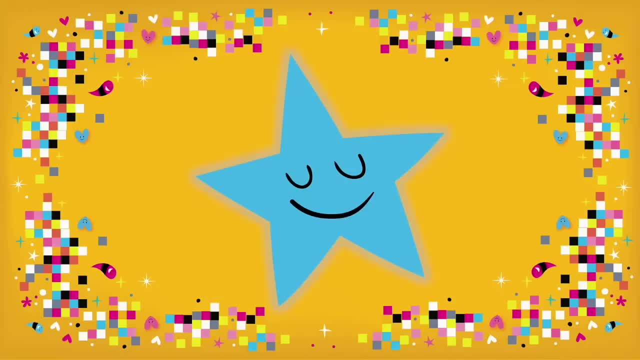 And a starfish with five points coming out from its centre. Choose what colour you'd like it to be. Starfish can be all sorts of colours, So make it the colour you'd like. You can make it patterned too, if you like. 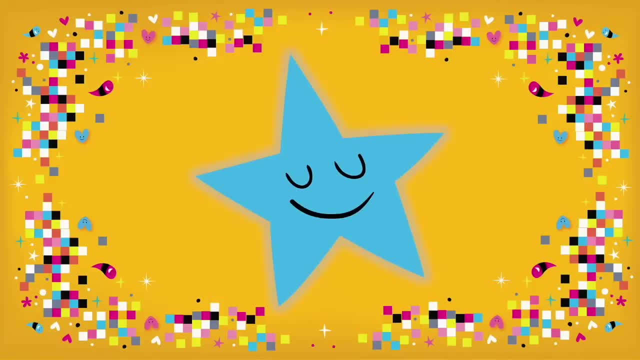 Spotty or stripy, Maybe even sparkly with glitter. Good job, What a great starfish you have there, And I hope you enjoyed this video. If you enjoyed it, please leave a like And leave a comment if you have any questions. 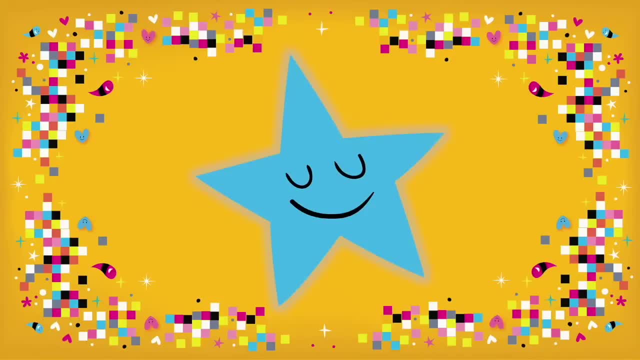 And if you liked the video, please feel free to leave a comment down below. And if you enjoyed the video, please leave a comment down below. I'd love to hear from you. If you've got any questions, please let me know in the comments. 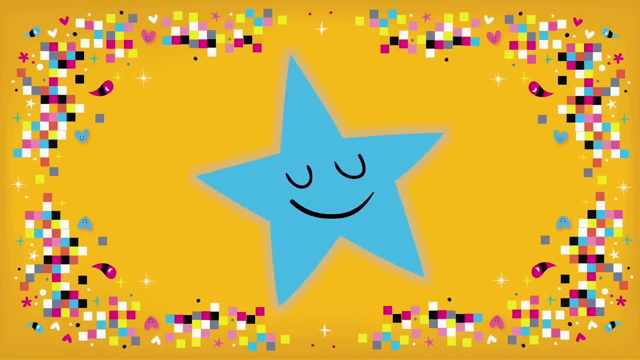 And I'll see you next time. Bye, that on too. That's it. Starfish are amazing creatures. Everything happens in the middle of their body. Their mouth is in the middle, their tummy is in the middle and they breathe. 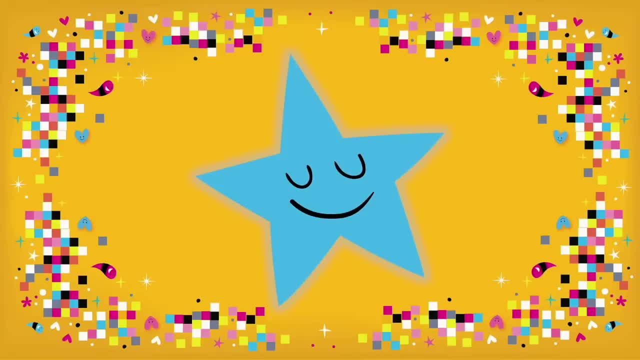 from the middle as well. Just like a starfish, we can breathe from our middles too, when we want to. Let's try starfish breathing and see if we can make our breath go from our middle and reach right to the end of our star points. Start by breathing out all the air. 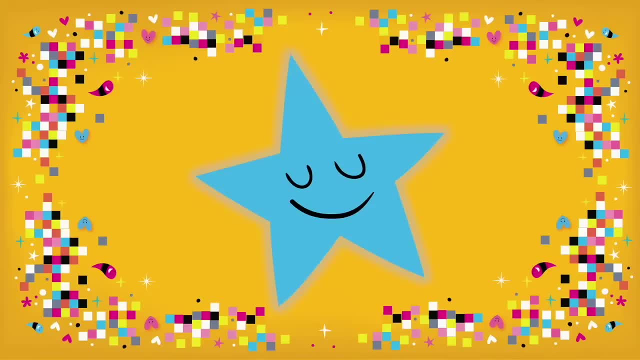 inside you, so you're completely empty. Now start to breathe in and notice as your middle starts to fill. Now start to breathe in and notice as your middle starts to fill. Your breath also spreads and starts to stretch the five points of your star right out Your. 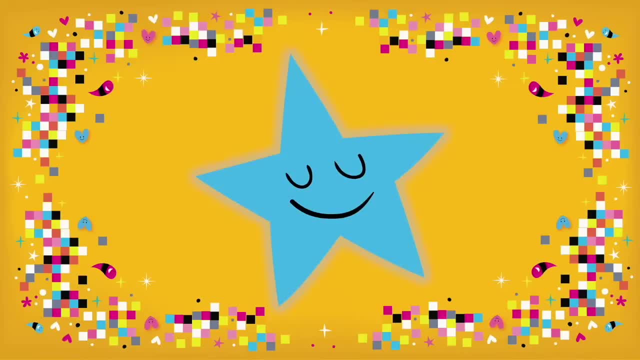 arms and legs, stretching out your head and neck, stretching up And now breathe out, relaxing your body as the breath leaves and your tummy goes down. Try it again, breathing in deep and slowly The breath, stretching the five points of your star right to your fingers. 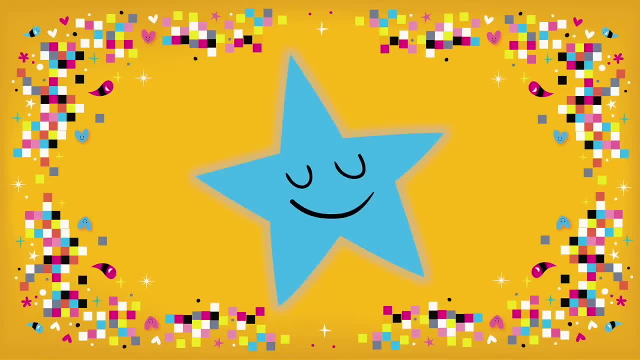 toes and up to the top of your head And relax, letting it all go. Your star points spread but nice and floppy. One more big starfish breath from your middle, Breathe in, filling all the way up, stretching to the ends of your star shape. Stretch, stretch, stretch And relax, Letting it all go Well. 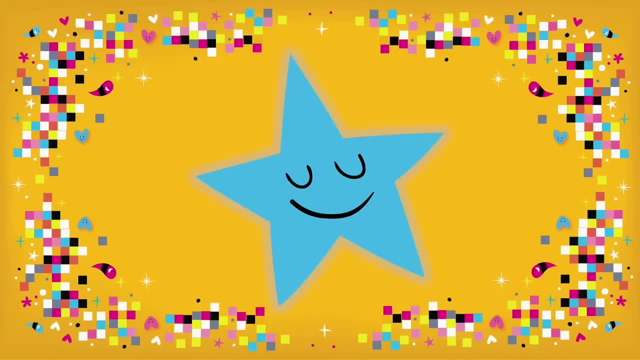 done. You've done some great starfish breathing And your body has had a good stretch too. Enjoy letting your breath be normal again And notice the restful, calm feeling that has come from this lovely stretching and breathing. It's quite nice being a starfish, isn't? 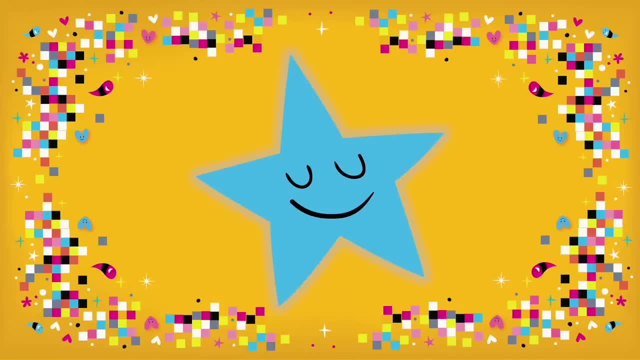 it. Now we come back, Hear the sounds around you, Slowly start to wiggle your fingers and toes And roll your wrists and ankles around in a circle. That's it. Roll over onto your side And push yourself up To sit, Open your eyes And take a moment to be pleased with yourself For doing something. 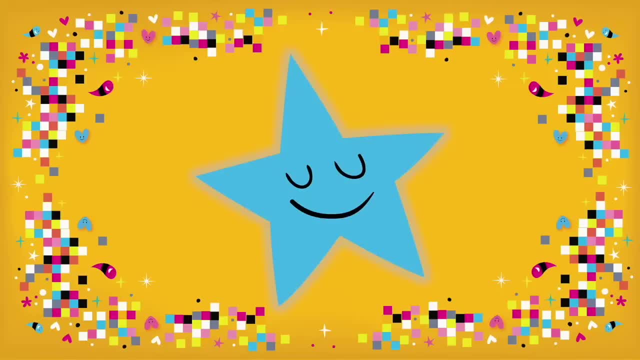 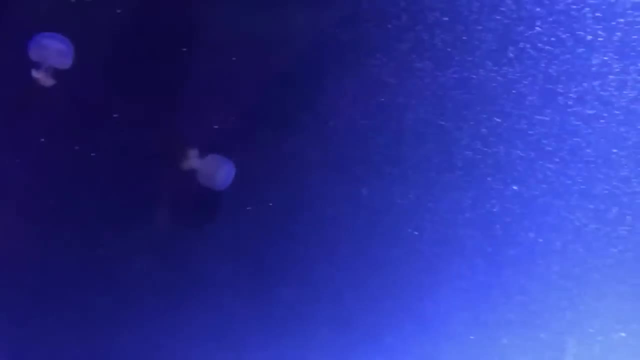 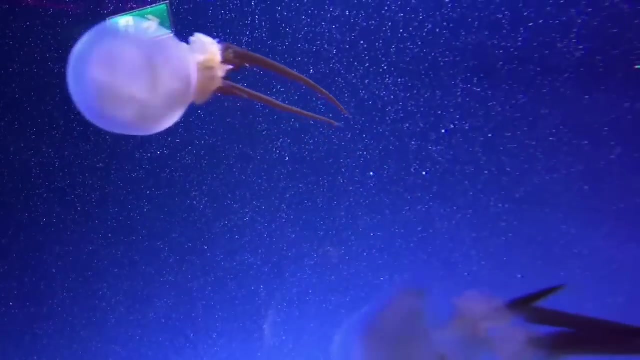 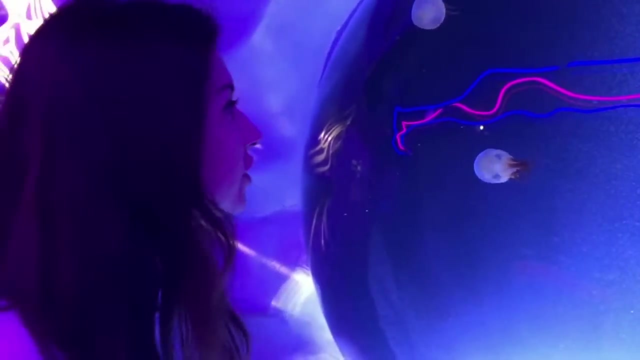 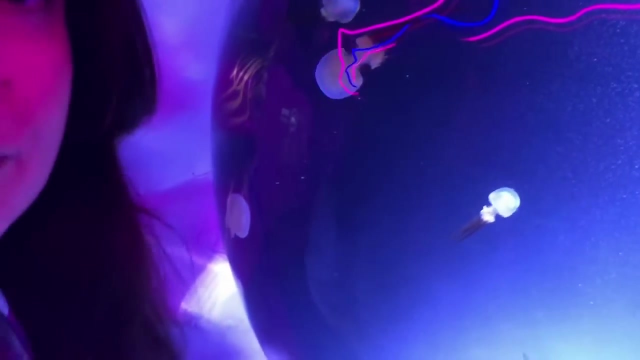 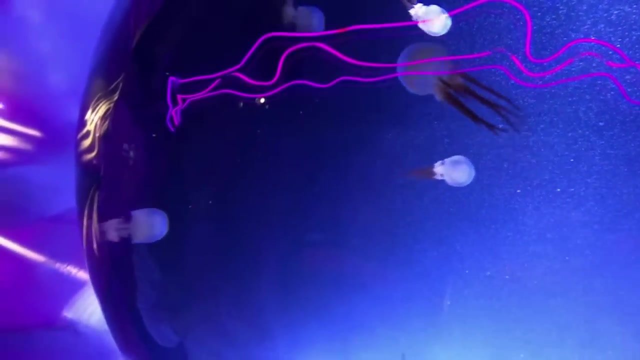 good for yourself, For your body and mind. I hope to see you soon. This is Jamie Saying peace out. Look at these amazing jellyfish- It's like it's flashing, Like mushrooms floating through the water. These amazing tentacles, Starfish and jellyfish. 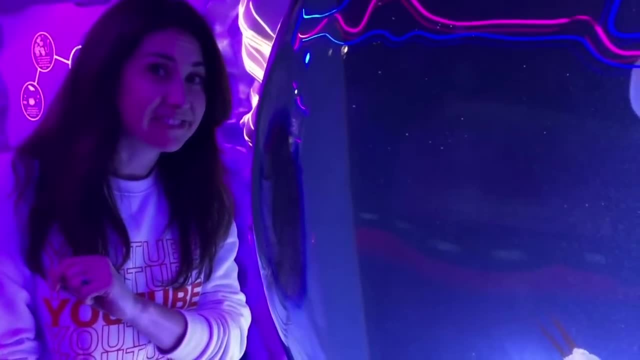 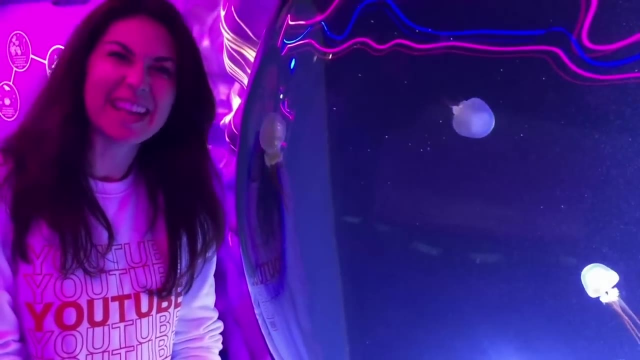 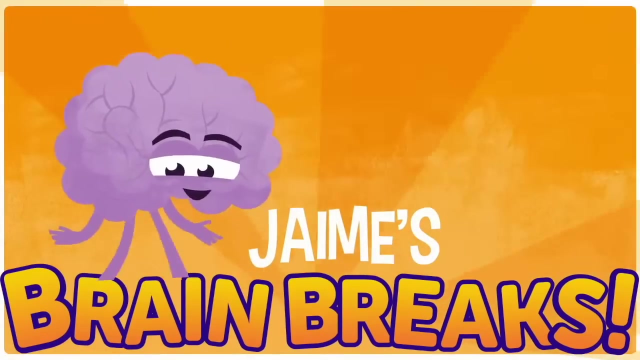 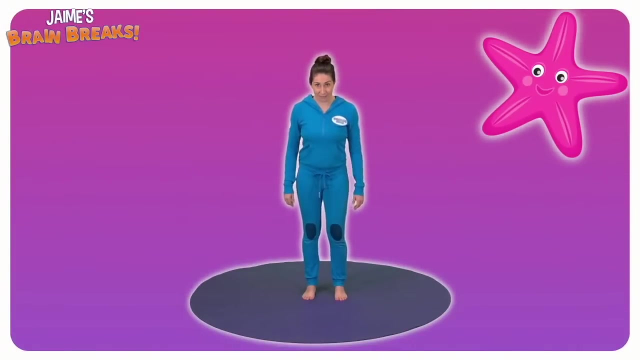 Now that's a really good brain break And we really, really enjoy being starfish and jellyfish in it, So maybe we should enjoy that. Let's go and enjoy that brain break now. Today we go deep sea core diving to meet a jellyfish and a starfish. Now these creatures- 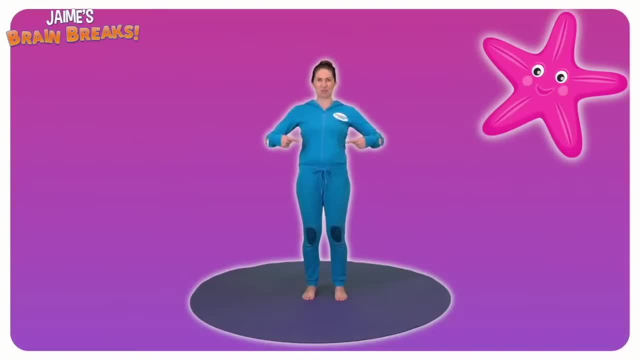 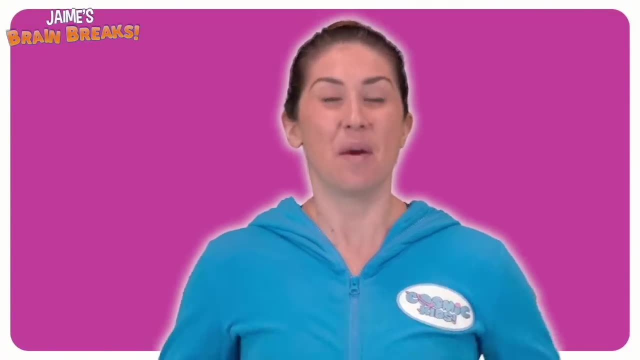 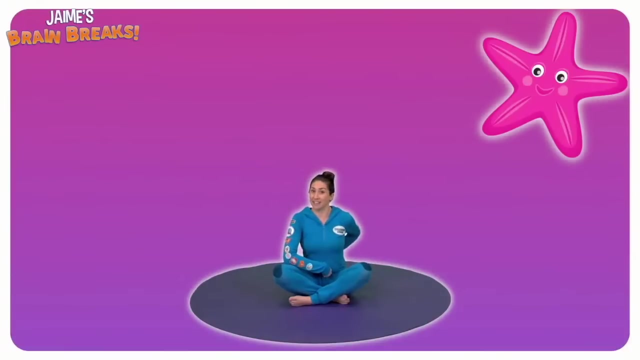 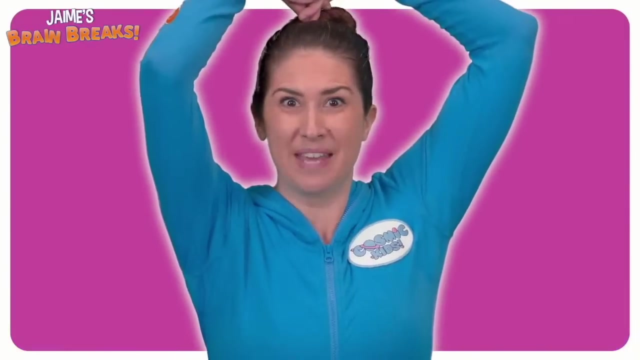 do everything from their middle, their core. We are going to start with a re-lapse Right from where we started. here we go Now. I just want to clean up our hands and the body. You are really branching out more than ever 來. 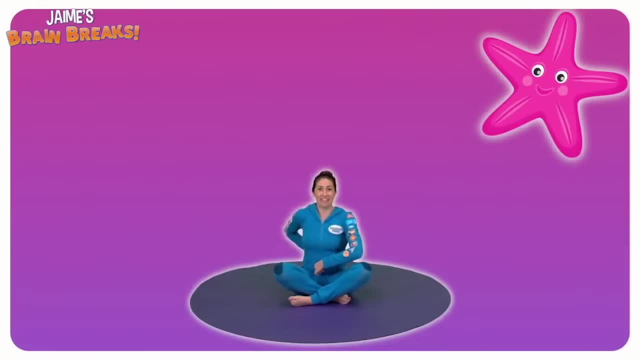 Now you are doing the vår, Let's get into this. Whoa, Whoa, whoa, Whoa, whoa, whoa. There you go. So we have our slipped setup. Let's do the laughed first ones, I would love. and your other finger to the base of your spine and zip up and give a silent 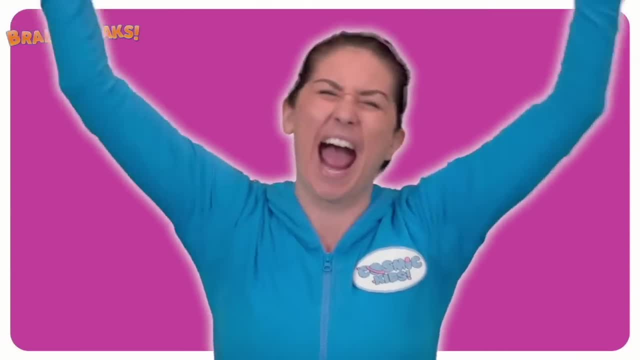 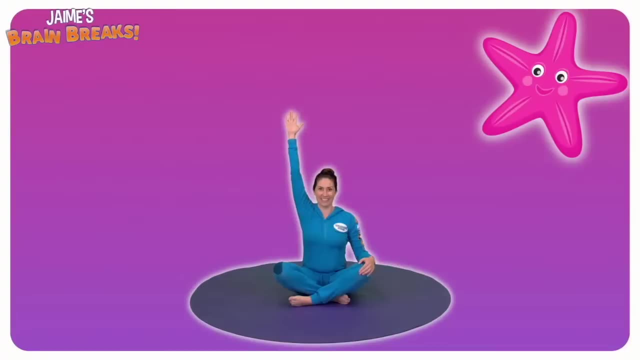 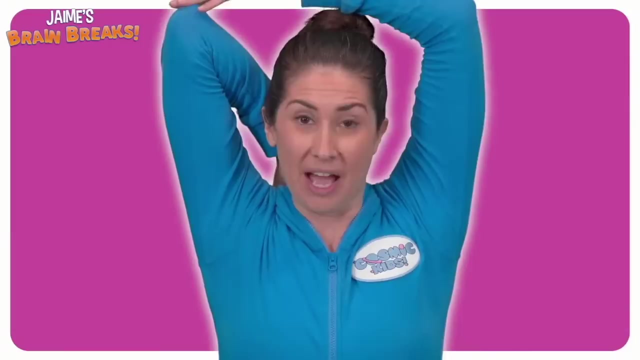 cheer to the sky, Fantastic. Now let's get our scuba tank in place. We reach up with one hand and we pop it down on our backs. We can't quite reach, so we take our other arm over the top and press our elbow down a little bit so that we can. 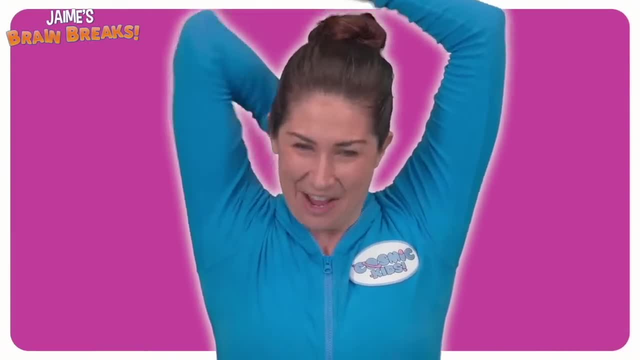 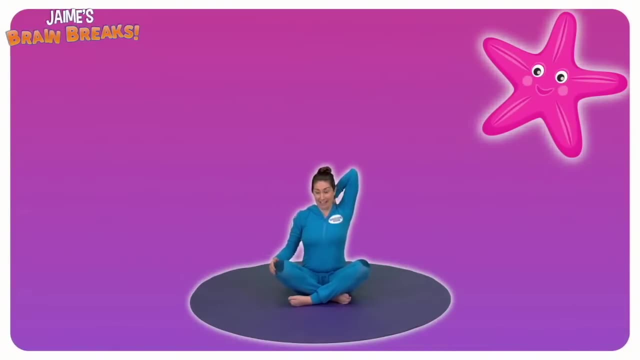 check that the tank is secure. There it is. We release our arms. Now we need to check that it's on. So we reach our other arm up and we pop that down into our back and then we take our other arm over the top to press our elbow down a little. 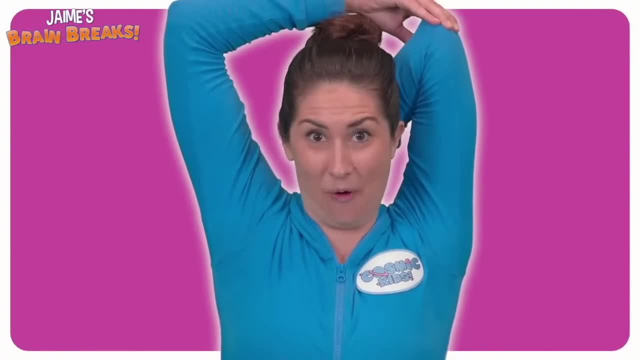 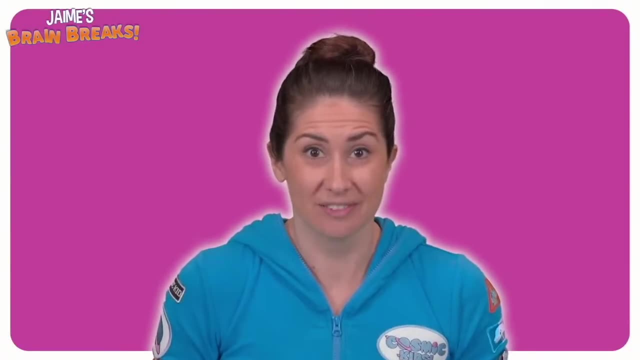 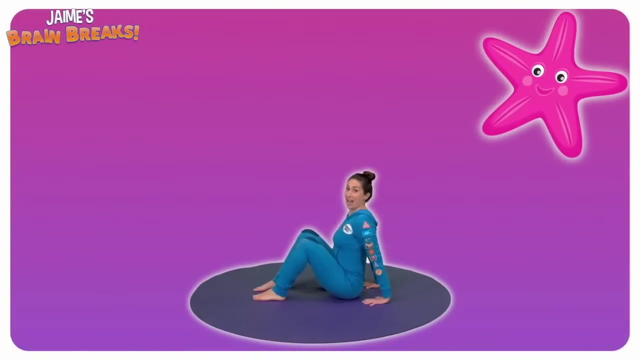 bit further. Yep, there we go. Oxygen tap on Fantastic Now lowering our arms. To get to the deep sea, we need to take a boat, So let's come into boat pose, Turn yourself to the side and get yourself nice and strong and stable by using your hands behind you to hold yourself up. Now lift. 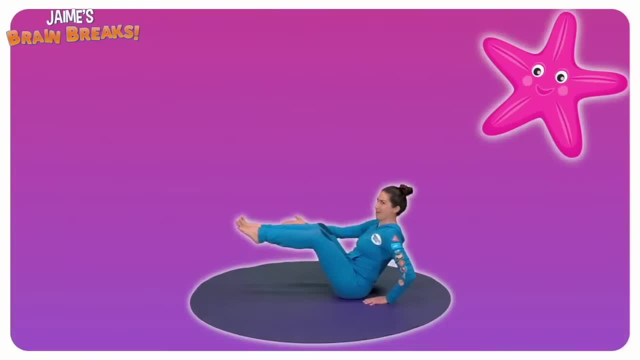 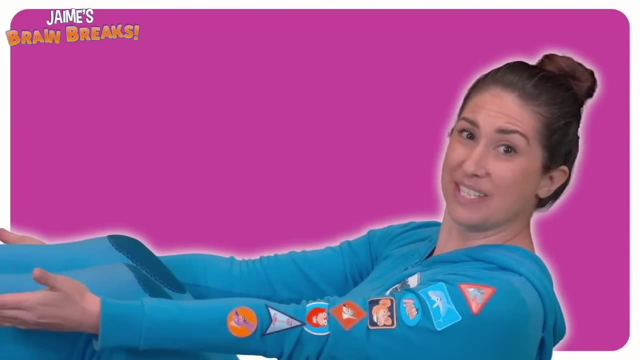 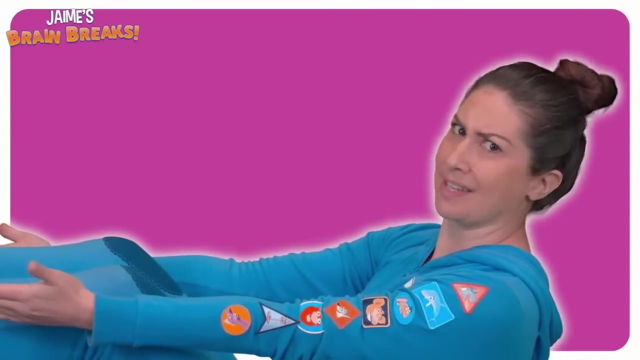 up one foot, Lift up two. Lift up one hand, Lift up no hands. Wow, we're already using our cores as we go in our boat. Yay, Now to get into the water when we're diving, we have to rock and roll off the side backwards. Let's practice that a couple. 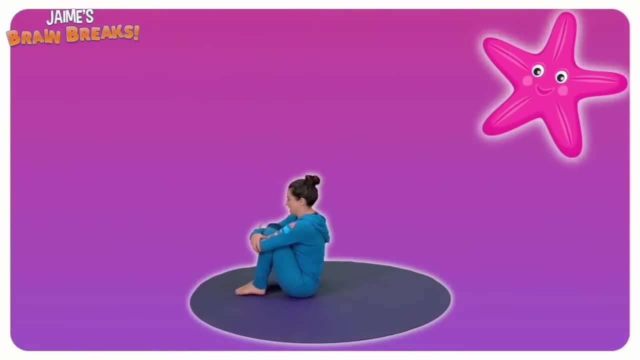 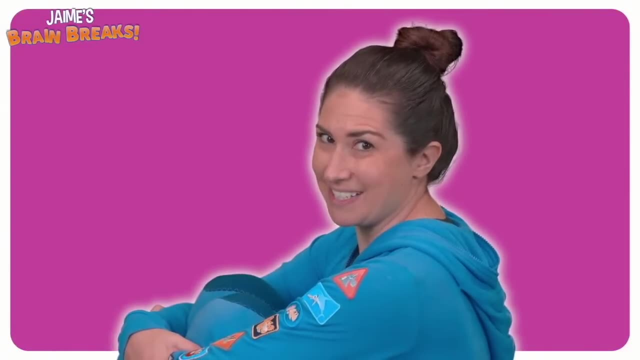 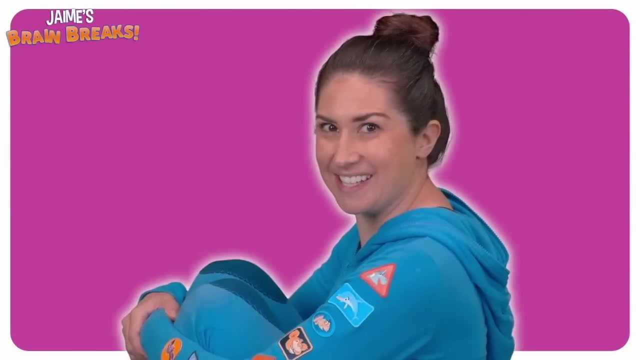 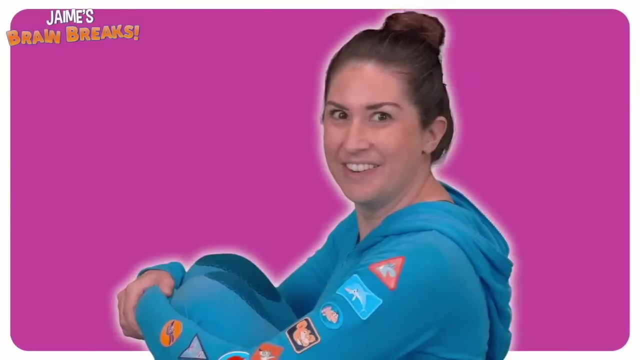 of times Sitting up, nice and tall, hug your knees and tuck your chin in like you're squashing a turtle. Now we're going to rock all the way back and all the way back to sit Ready. One, two, three, Nice. Let's do that again. One, two, three, Nice. Now this. 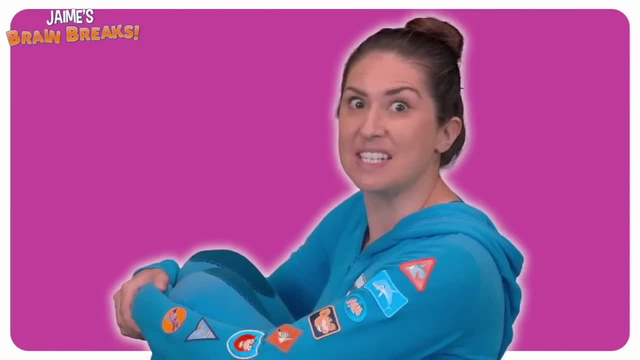 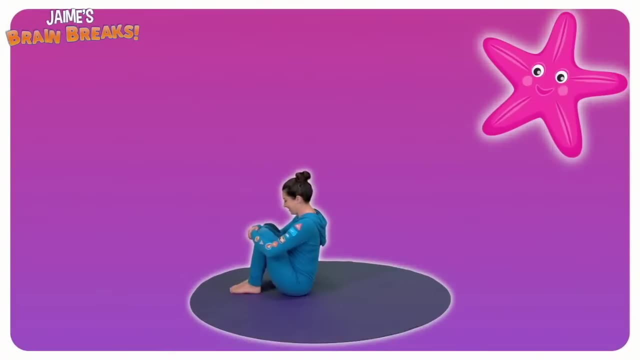 time. I wonder if you can rock all the way up to stand by kicking your legs as you rock forwards. Let's try, Ready. Tuck your chin in One, two, three, Whoop, Kick your legs And up. Yay, We did it. Coming to stand, everyone, We reach our. 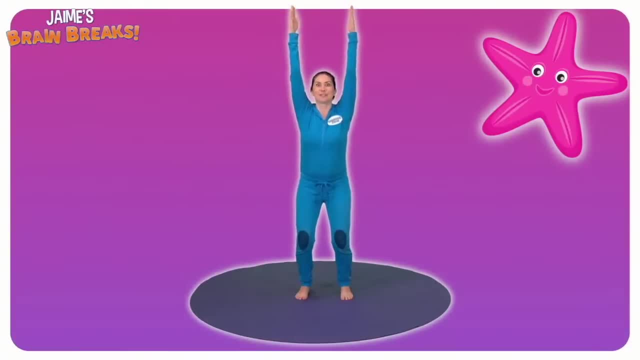 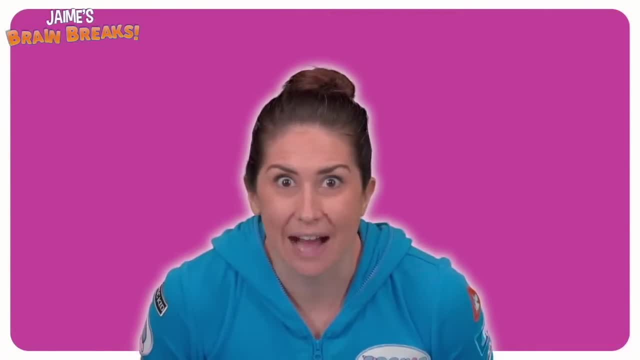 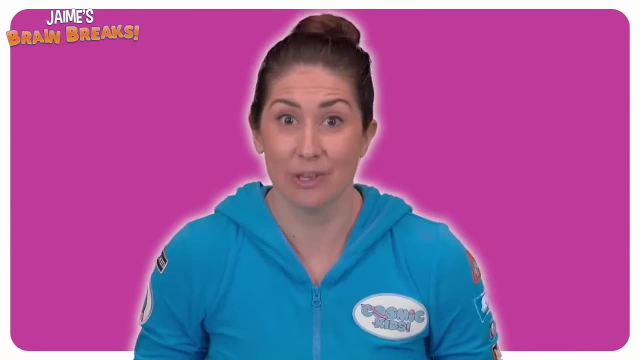 Wow, We've made it all the way down to the bottom of the seabed. Now let's check our scuba breaths. We're gonna use our legs to auch ach, ach, ach, ach. going to breathe and see if you can hear your breath like a whisper at the back of your throat. 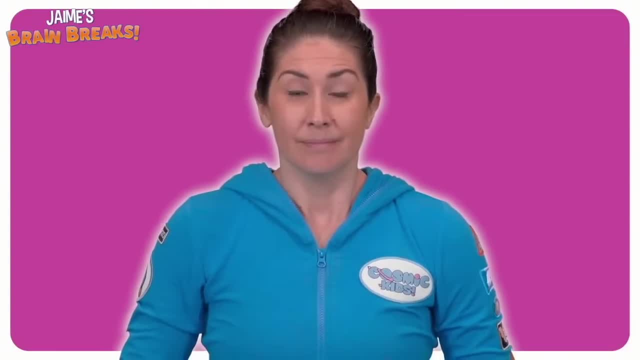 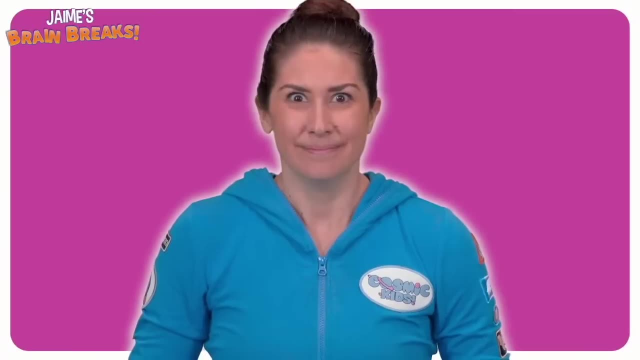 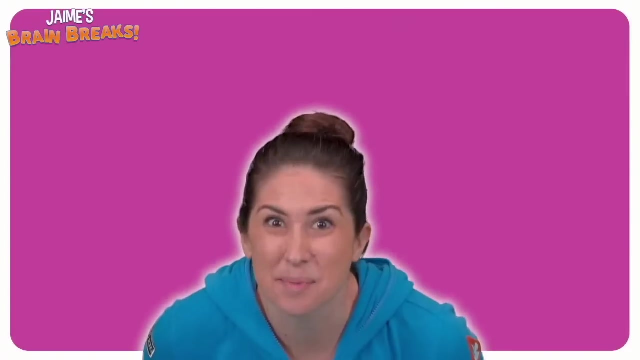 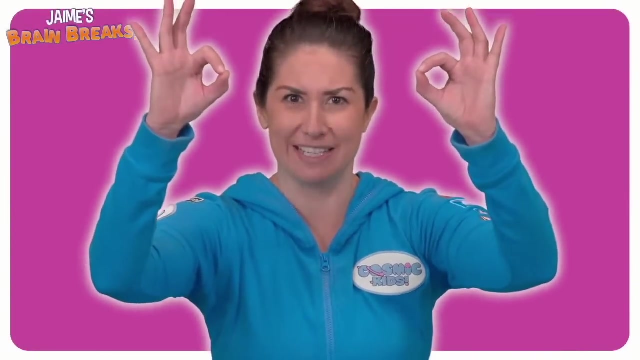 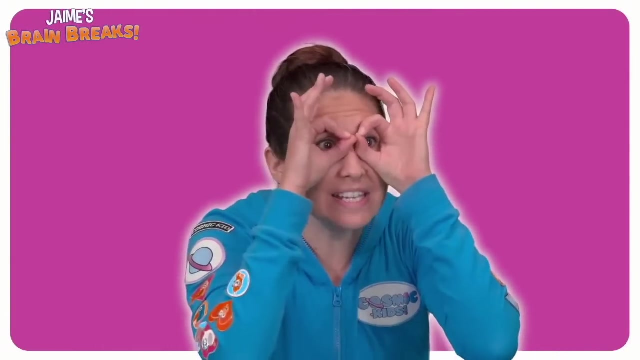 like this And again. Wow, amazing scuba breaths everyone. Now we're here, let's have a look around. Let's look through our sea goggles. Joining your thumbs and fingers together, have a look through There. look, we can see a jellyfish coming up to stand. everyone, Take your feet nice and wide. 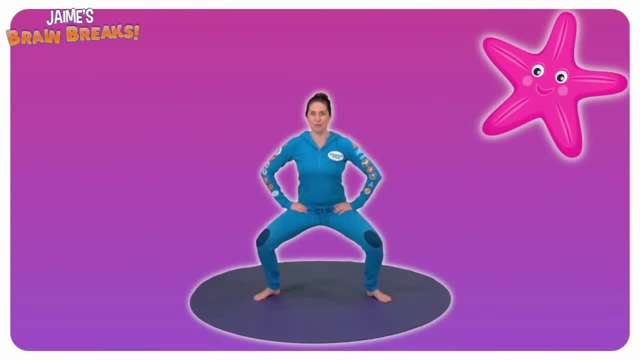 and point your toes out to the side. Now bend your knees, bring your hands up and join your fingers above your head. As the jellyfish moves up, it opens its head and spreads its tentacles wide. Then it becomes a jellyfish. 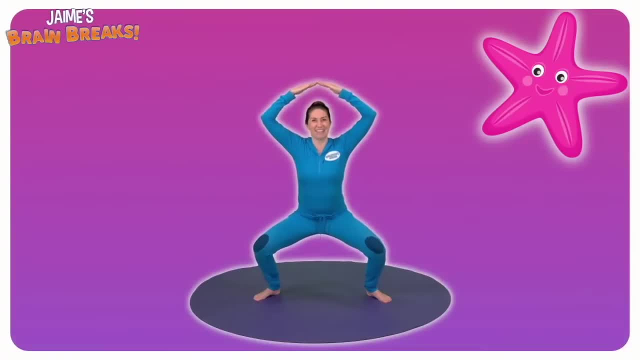 Now bend your knees, bring your arms up and join your fingers above your head As the jellyfish floats and closes back down, bending our knees again. It presses up, opens out, stretching its tentacles, and then lowers back down as it closes everything down. 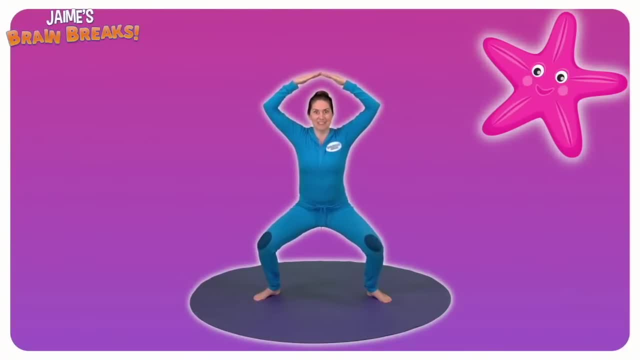 to float. We watch it bob through the seaweed coming into seaweed pose Lying on our backs, we lift our legs up to the sky and our arms up to the sky. Now see if you can very slowly begin to move your arms and your legs like you're. 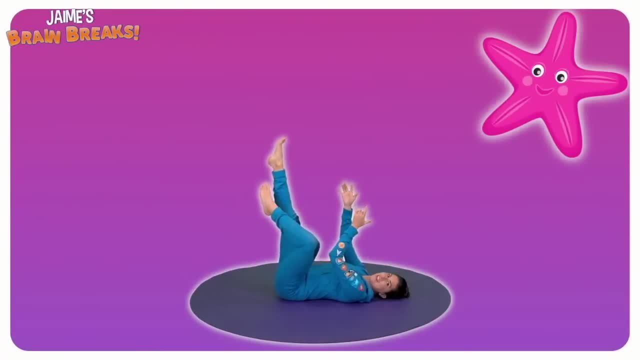 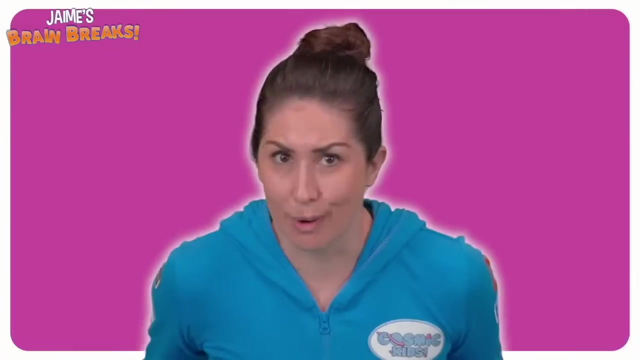 seaweed flowing in the water Almost like it's slow motion- Amazing. We have to be very slow and controlled to do this. Now cross your shins and come back up to sit by rocking all the way up, Sitting in the middle. I think it's time to look through our sea goggles again, but this time we're 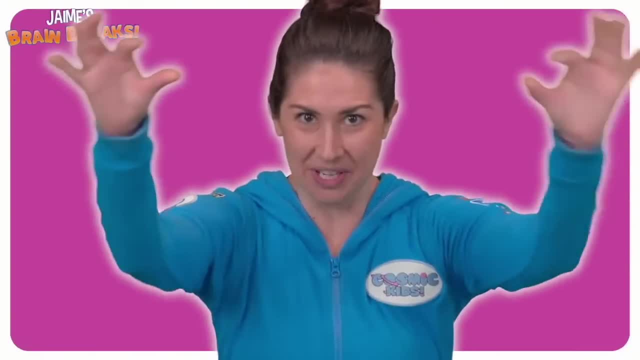 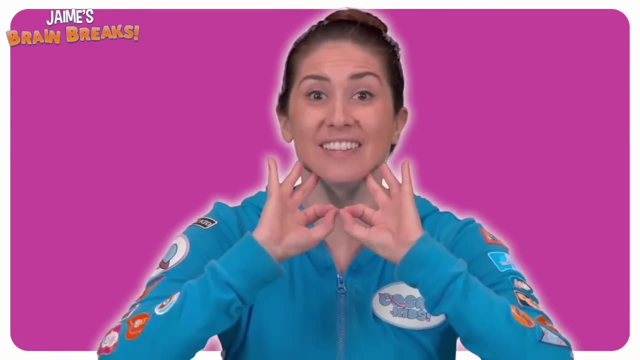 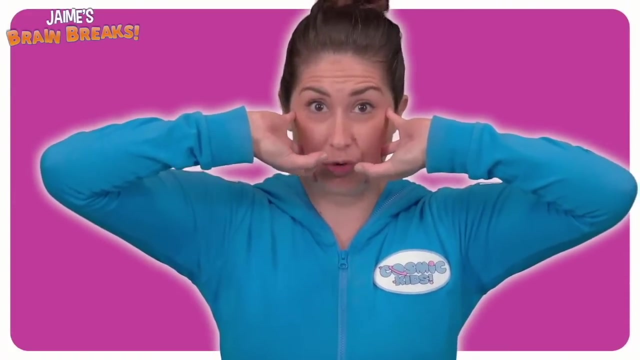 going to look through them the upside down way, Joining your thumbs and fingers together. take these three fingers and put them under your chin, just like that. Yes, now bring your other fingers up a bit higher and bring your pinky finger, your little finger, up to where your cheek joins your jaw. Now lift up your 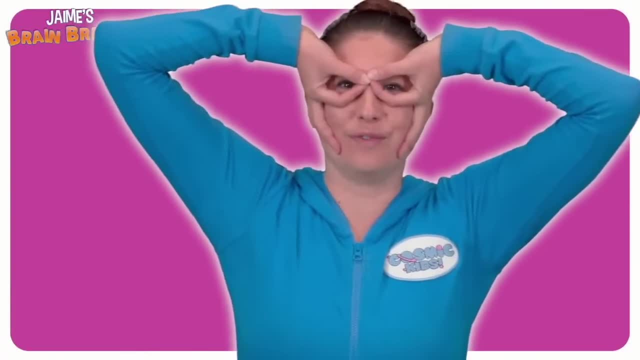 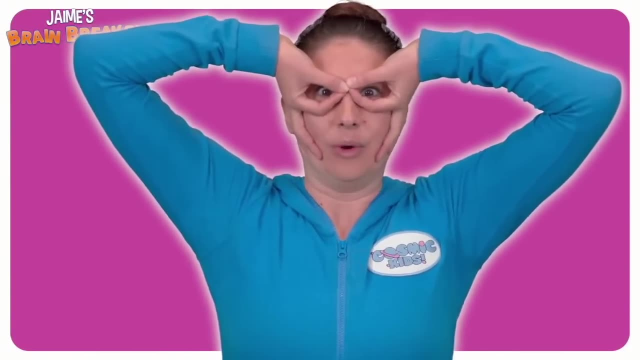 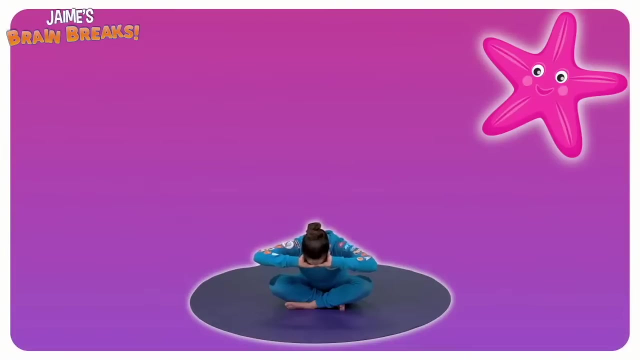 elbows and stretch those holes of your sea goggles over your eyes. Oh, now we're looking through them upside down. That's really cool. Now let's have a look. what's on the sea bed Folding all the way forwards? we have a look. Wow, we can see a. 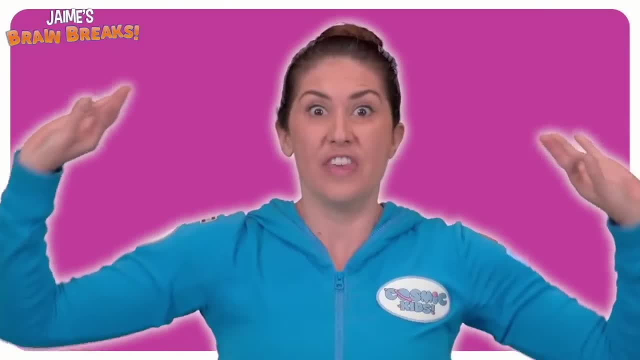 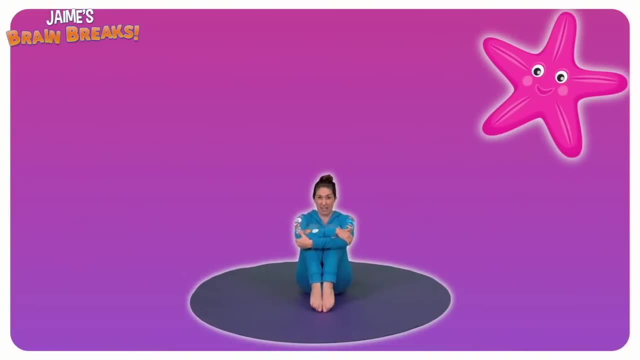 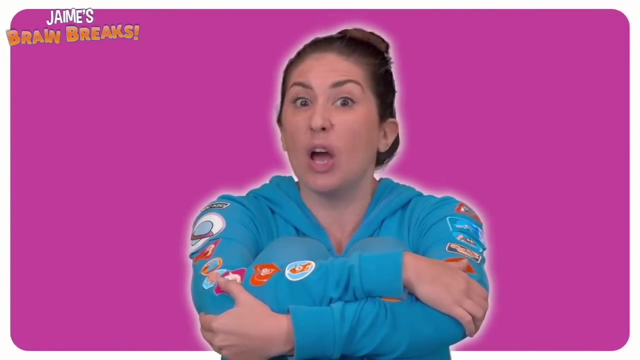 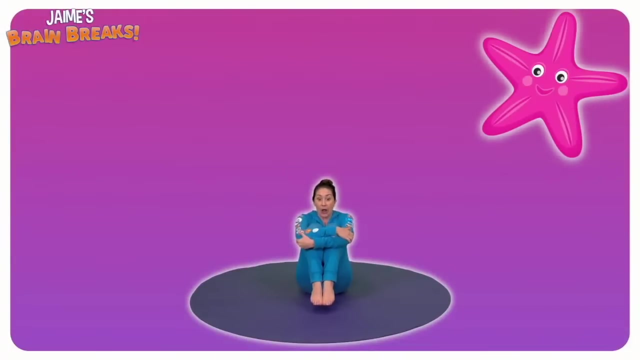 starfish sitting up everyone. This is super cool, but it's seen us and it's scrunched itself up. Hug your knees in nice and tight everyone and tuck your chin in, seeing if you can balance your toes off the ground. If we're very quiet it might open up again. Look there it goes. Slowly, start to open up. 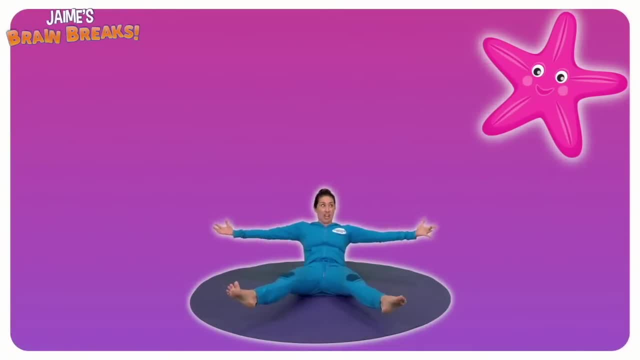 Your points. like you're a starfish, Your arms and legs go as wide and as straight as they can be. Boy, oh boy, you've got to have a strong core to do this pose, don't you See if you can hold it a bit longer. Oh no, it's seen us again and scrunched itself up. 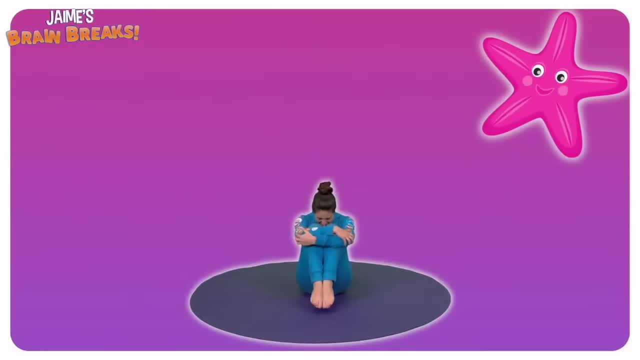 Huddle yourself all the way back in everyone. Oh, I think we better leave this starfish in peace. Let's swim up, Coming onto your knees everyone. Bring your hands in between your knees As you breathe, in use your scuba breaths and 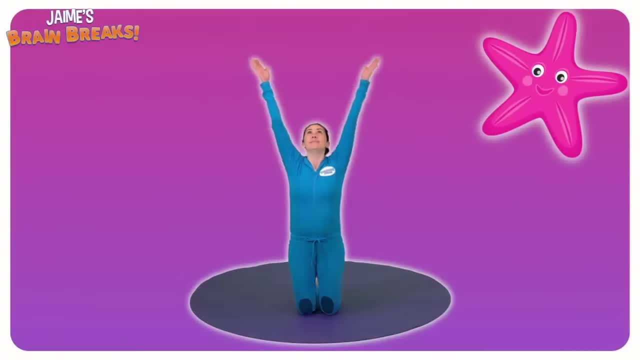 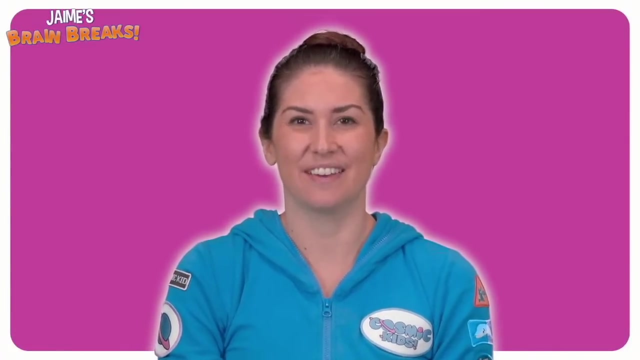 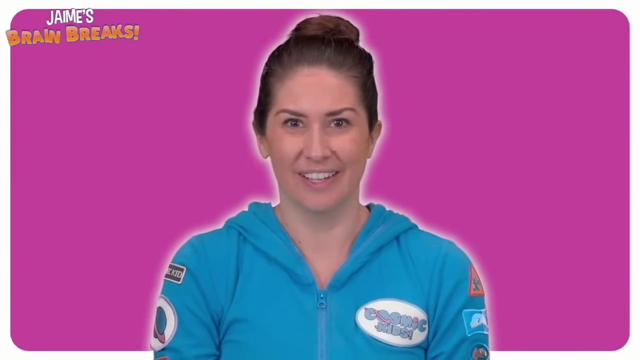 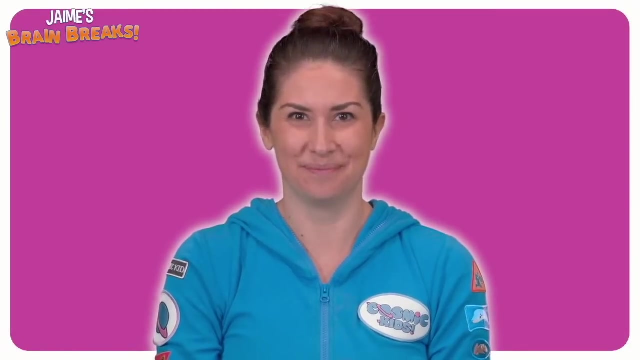 lift up Ready and lower down One more time And lower down. We sit back in our boat, allowing ourselves to float along the water, thinking about those incredible creatures, how they use their core. They're so strong and it helps us feel strong and powerful, ready to stand tall. Have a 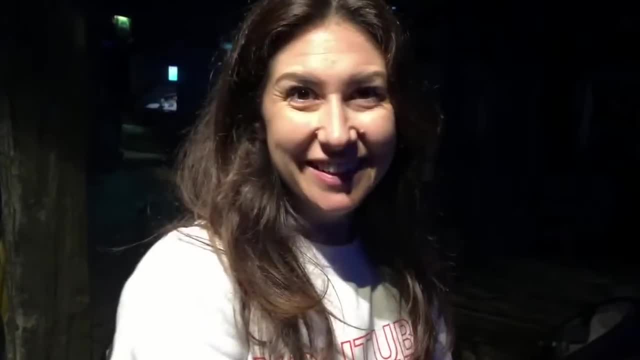 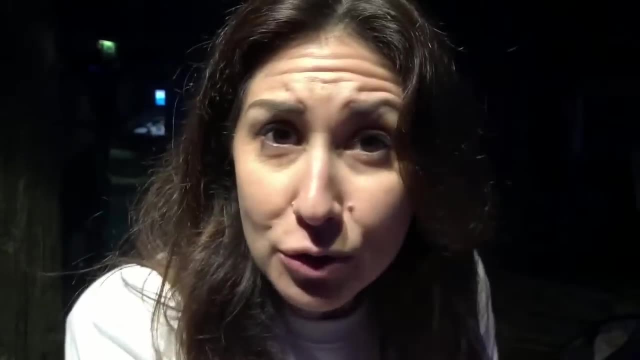 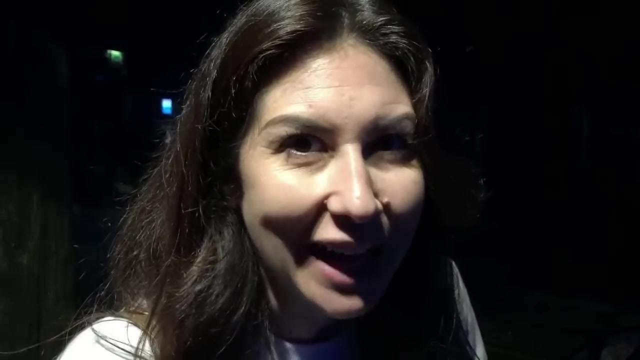 brilliant day. So here we are at an amazing shark tank. These sharks are the most beautiful creatures. They're so graceful with their teeth And I wanted to finish our little underwater mix with these guys because they're pretty spectacular. You've been awesome on our ocean mix and I hope you've enjoyed it. 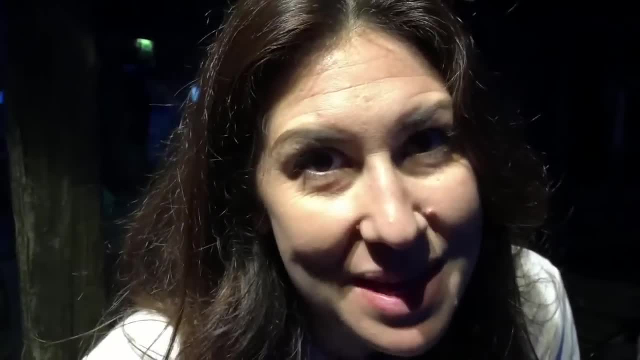 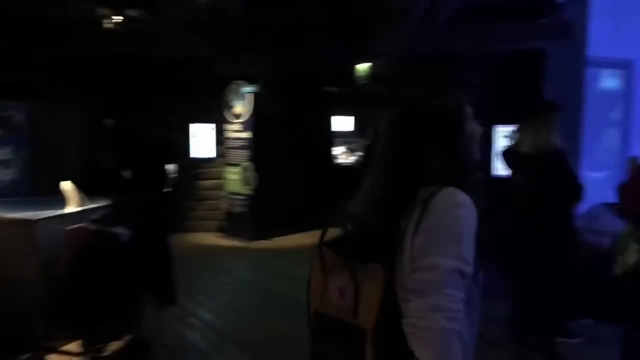 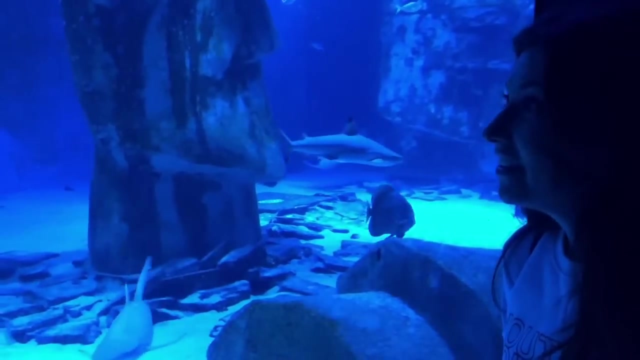 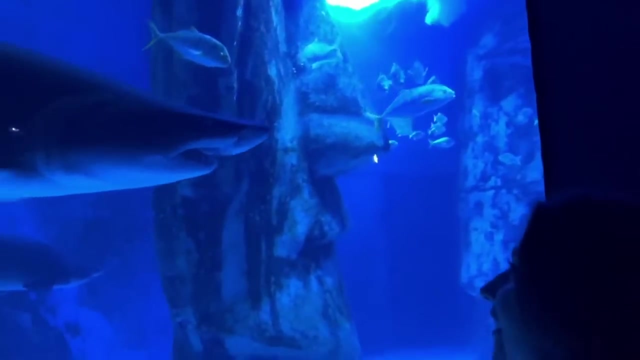 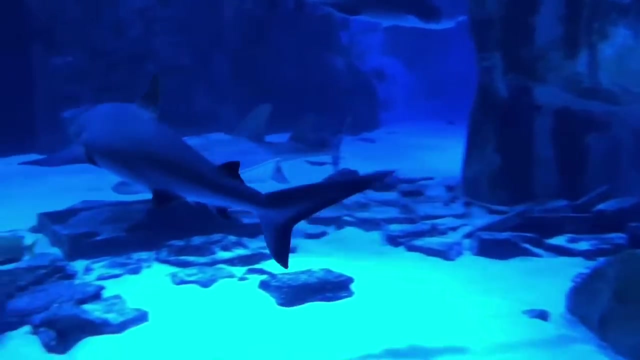 Now don't forget to subscribe and hit the bell so you never miss another video. Namaste everyone, Bye. Wow, These amazing sharks, And this one coming right towards us. now, Here he comes. Wow, Look at those teeth, They're so sleek. 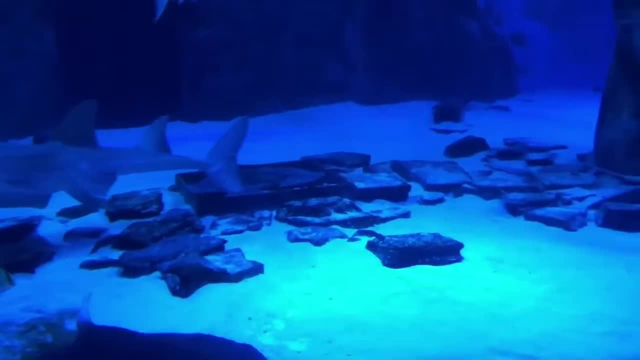 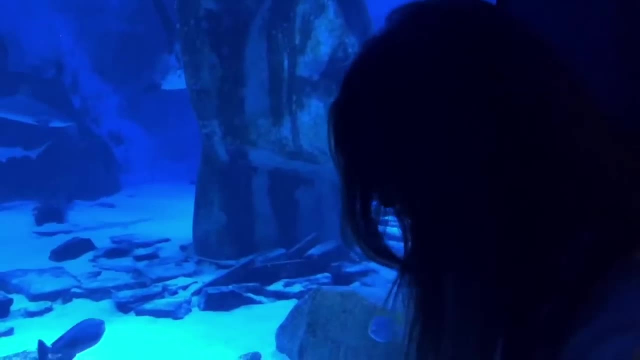 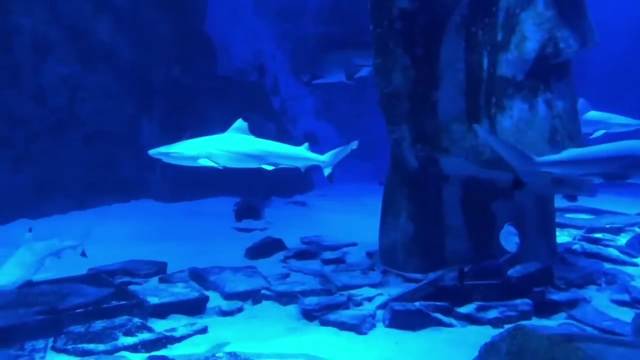 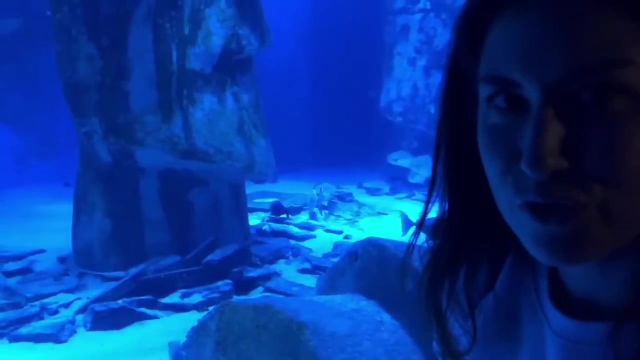 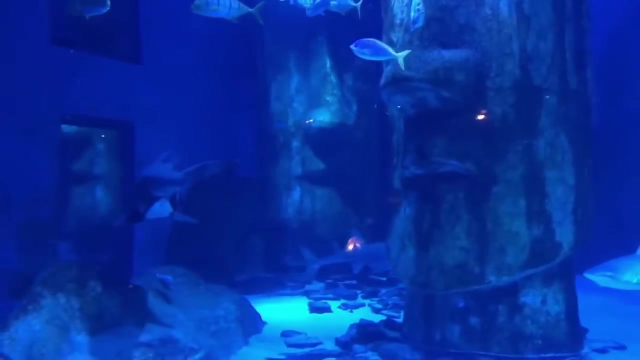 Look at this stingray. Wow, This is coming to shuffle up and have a bite And have a look, Say hello, Amazing reef shark. Look at that black tip. Hello, Hello, Hello, Hello, Hello, Hello, Hello. 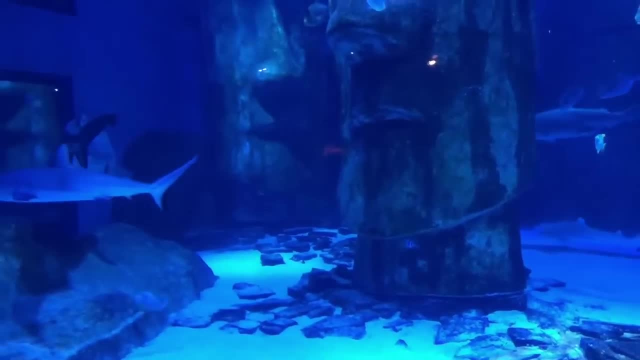 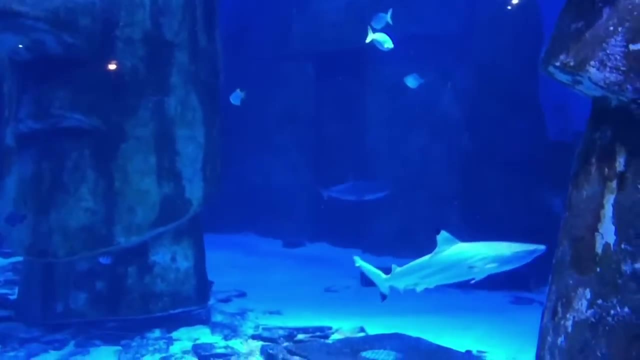 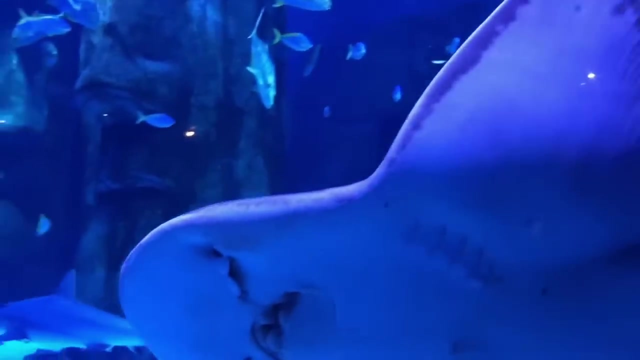 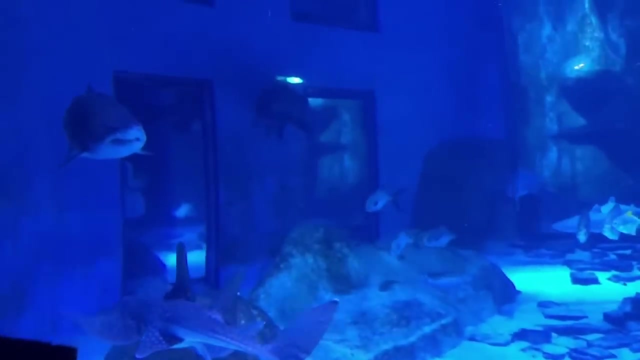 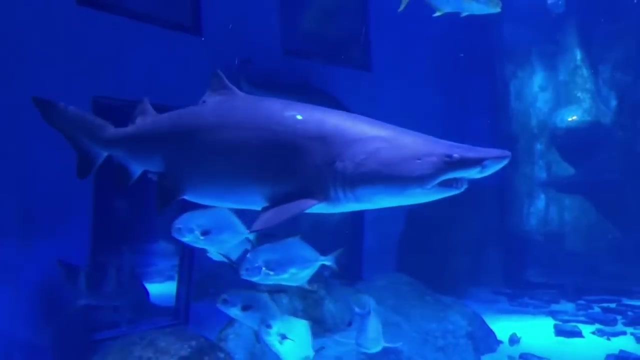 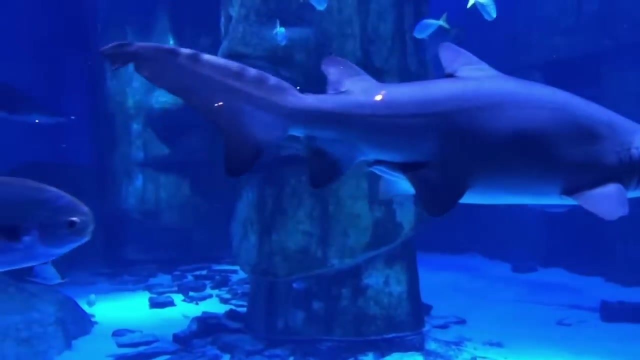 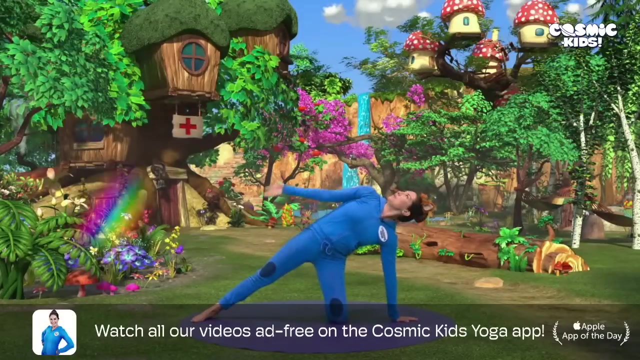 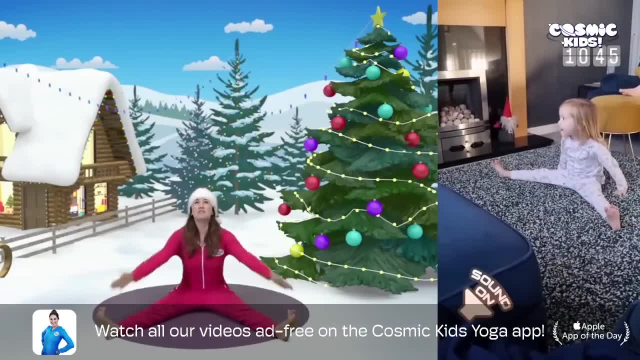 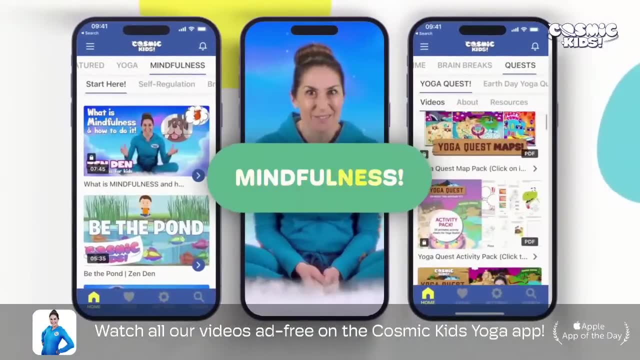 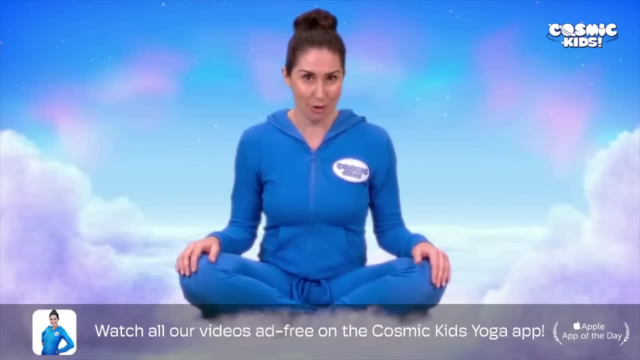 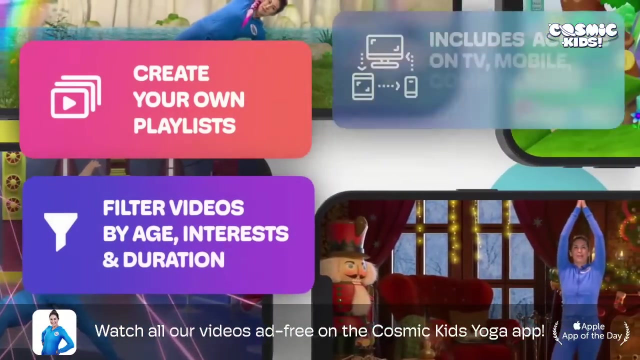 we take our legs out wide, we reach up very high for a big pot and we pop it down all the way in front of us. so what is it? what is mindfulness? how do we do it? and the best way to make the I can't thought go away is to think: oh, yes, I, can we step forward between our hands? oh, thank goodness. 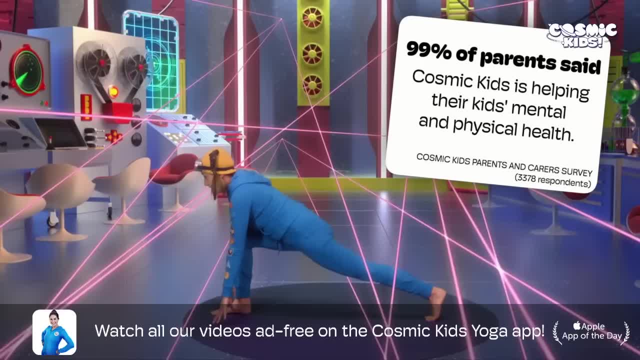 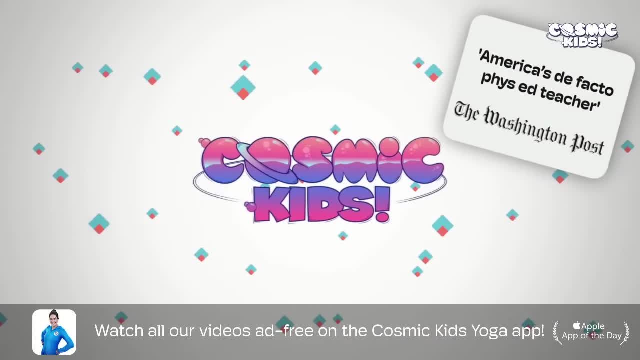 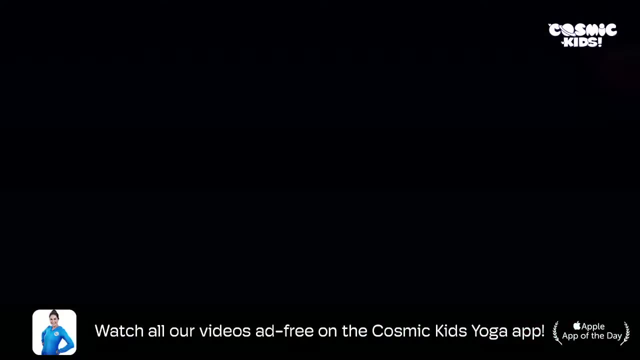 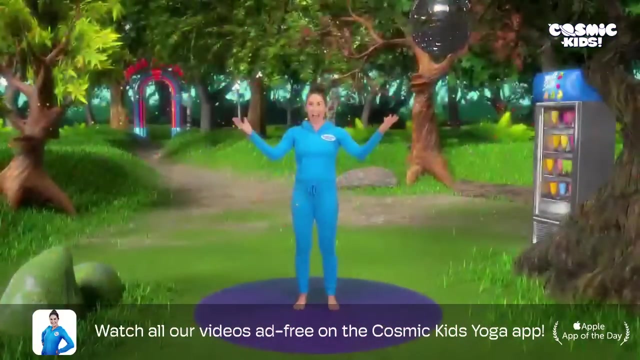 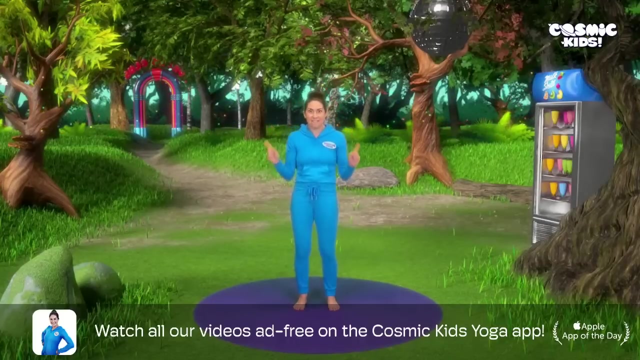 we do yoga now, making our legs very strong. we lift all the way up, trying not to wobble, lift our arms up to the sky and then we fold all the way forwards. hands come either side of our foot. hello everyone, welcome to cosmic kids. i'm jamie and this is your place for yoga, stories and fun. 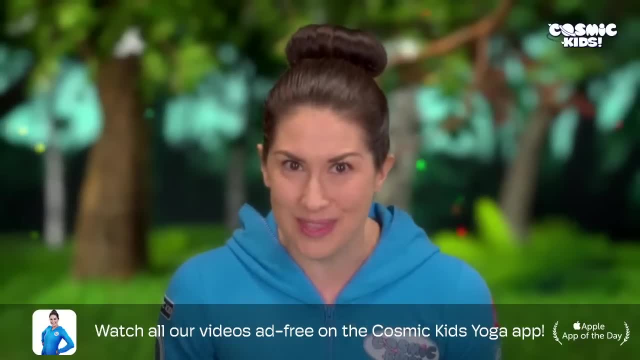 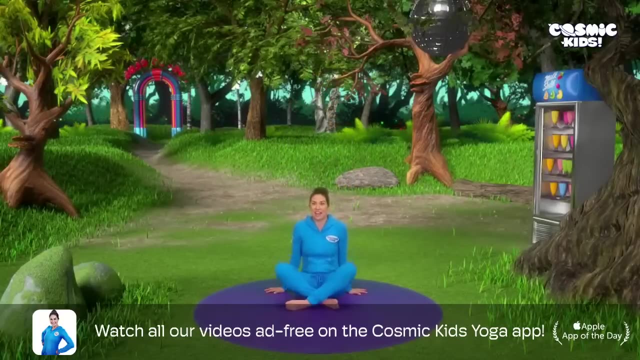 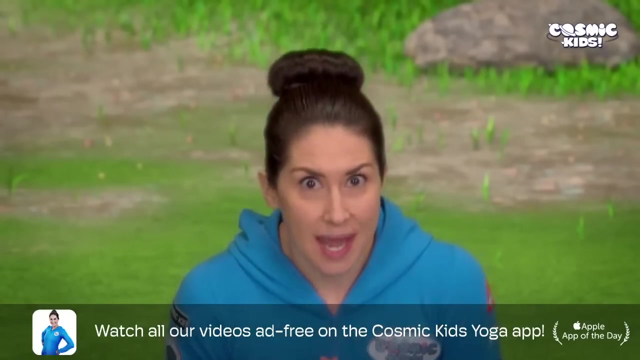 it's easy: just copy the moves i do and enjoy the adventure. now. we always start in the same way, and that's by sitting on our bottoms, crossing our legs and bringing our hands together at our hearts and saying our secret yoga code word, which is namaste. ready after three. one, two, three. 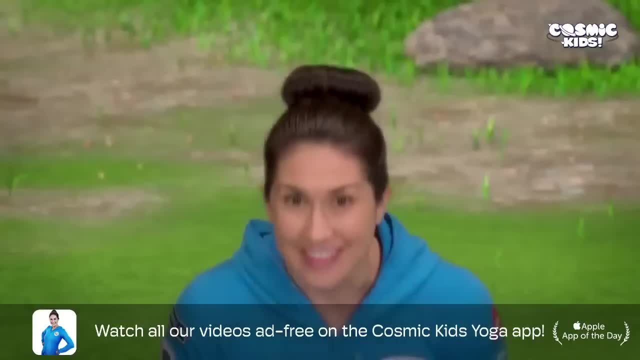 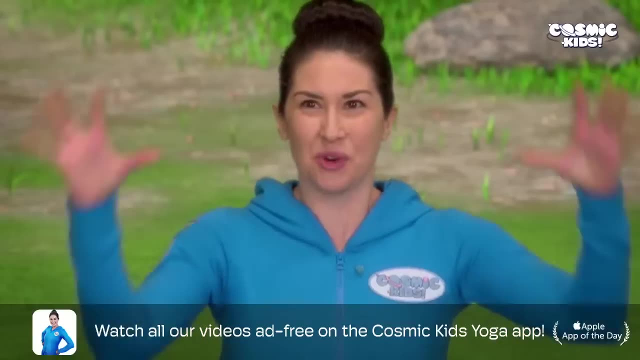 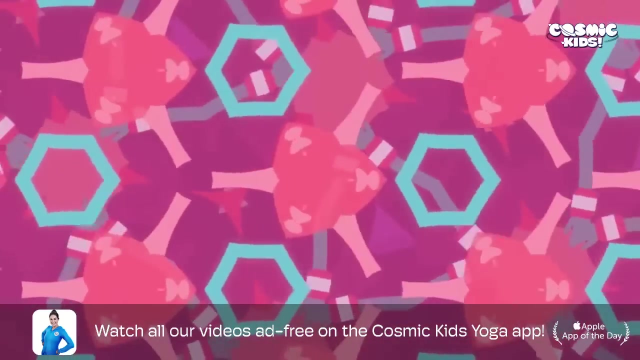 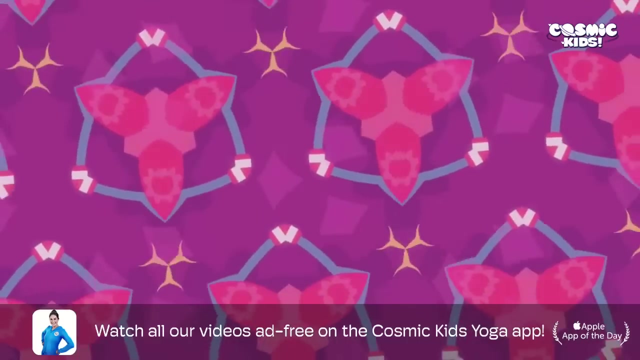 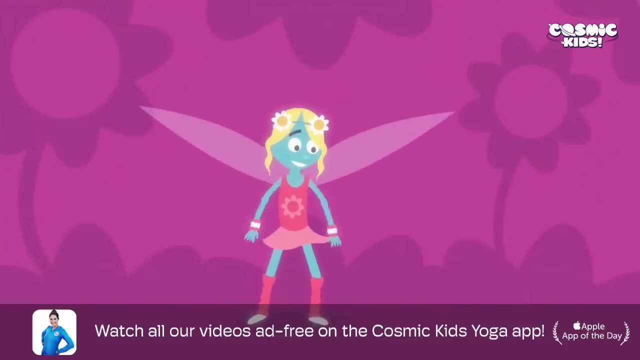 namaste there. now let's have a look through our cosmonoculars and find out who we're meeting today. joining our thumbs and fingers together, we have a look through. oh, look at the colors, look at the shapes, the patterns, all going round and round. can you see it? the picture? it's a fairy, it's fairy floss. oh, what's fairy floss doing? oh, of. 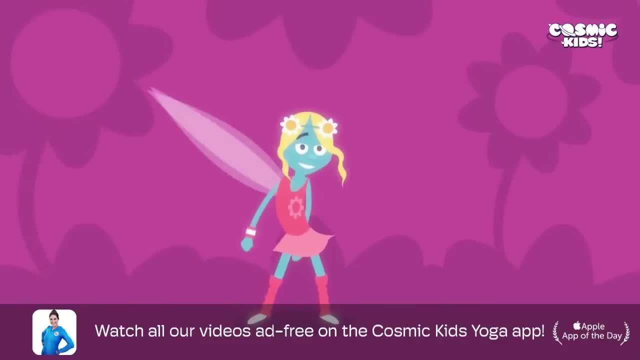 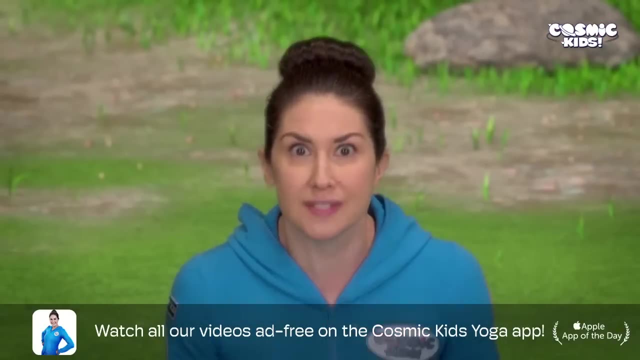 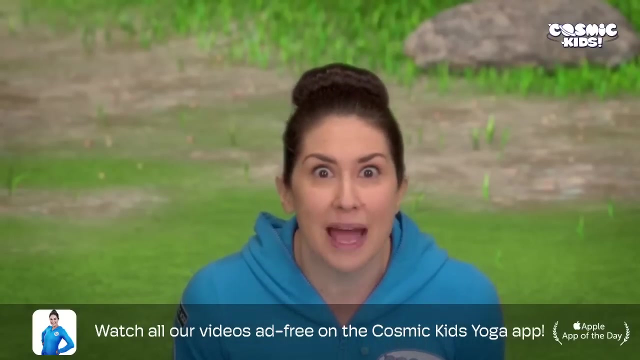 course. look, she's doing the floss dance, lowering our hands all the way down. how exciting: we're off to meet fairy floss, a real life fairy. now, fairy floss lives in pixie patch, which is home to a community of magical folk who love nature and the simple things in life mostly. 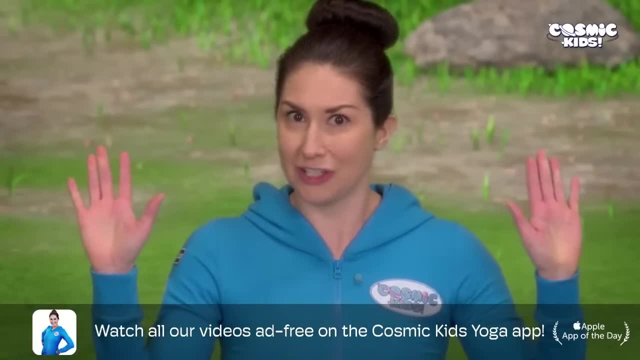 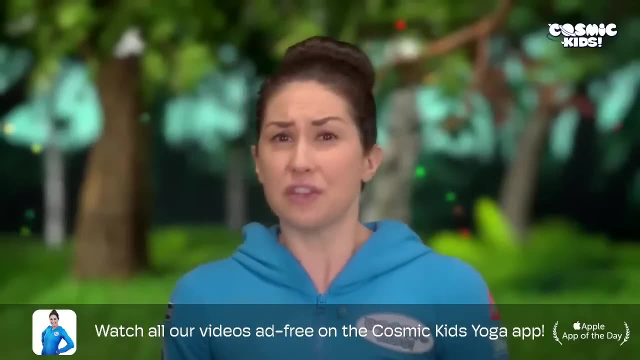 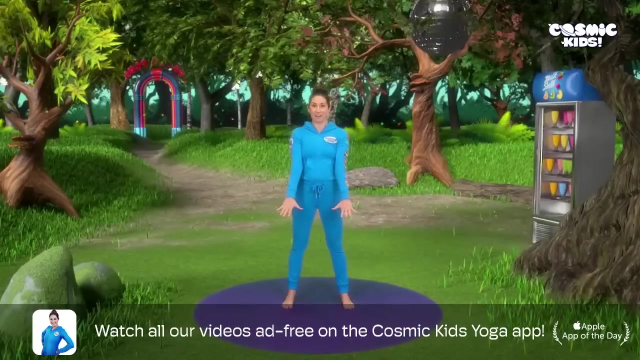 dancing. let's come up to stand without touching our hands on the floor ready. well done everyone. now fairy floss, as you've already guessed, loves one dance in particular: the floss. let's try it. we take our arms down in front of us and make our hands into fists. 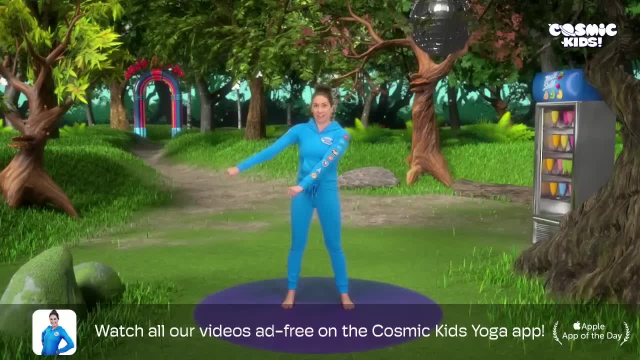 now we count: one to the side, two to the other side and through front and back. let's do that again: one to the side, two to the other side, and through front and back. and again: one is the hour now and front and back. two is the hour then, back. 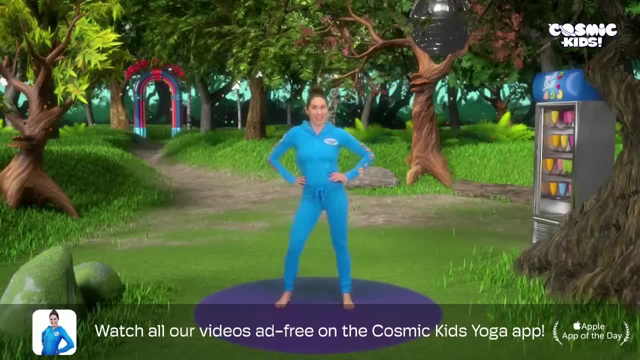 one, two through, and one again, one, two through, one, two through, one, two through. yay, We've got the arms. now let's try the hips. let's bring our hands onto our waist and our hips go side to side. we can add a little bend of the knee as well to help. yay, now we're going to try and put the arms and. 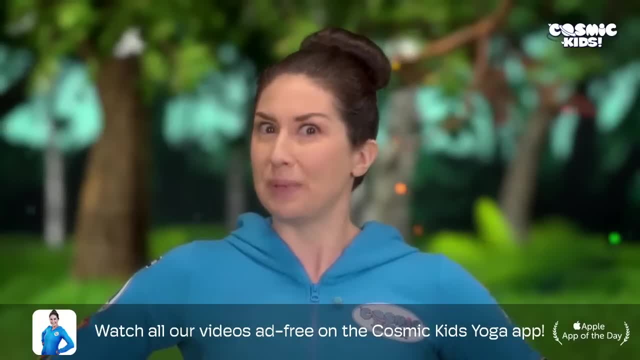 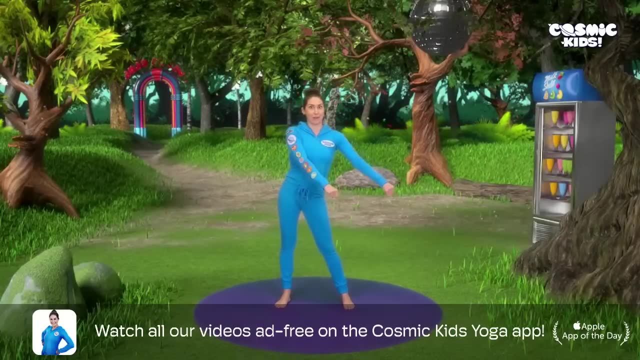 the hips together. we're going to step up and we're going to touch back. hold your toes together أن we're going to start slowly and build up speed, taking our arms down hands into fists. Now, our arms go one way as our hips go the other. Here we go: One, two through And again One. 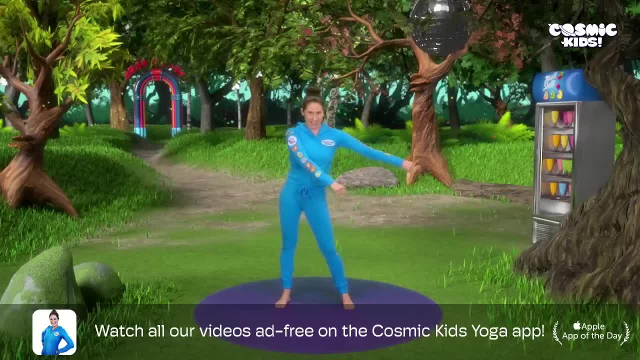 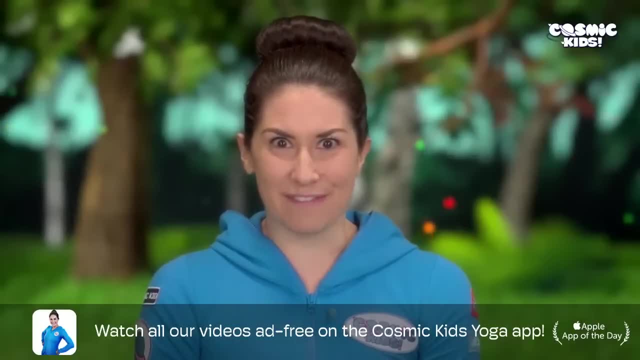 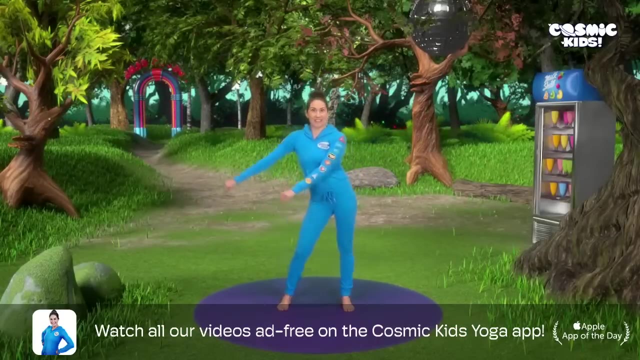 two through. Yay, Here we go. One two through, One, two through. Let's try a little bit faster. Here we go One two through, One two through, One two through. We're getting. 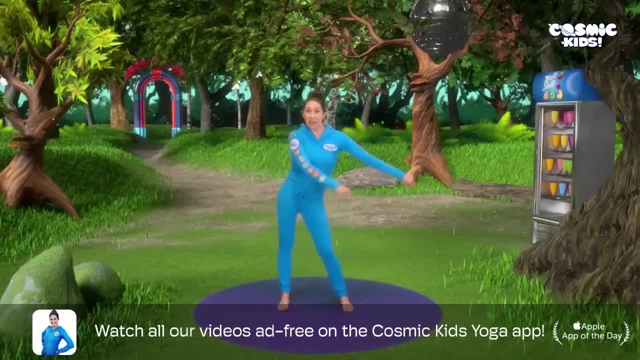 it. That's it. We're getting it. Keep going. And we are flossing: Fairy floss, do-do-do-do-do fairy floss, do-do-do-do-do fairy floss, do-do-do-do-do fairy floss, Woo-hoo Now. 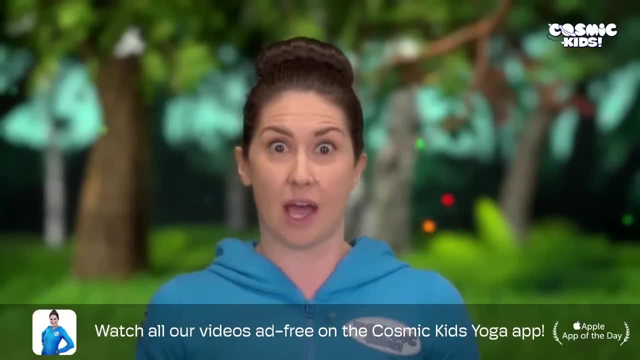 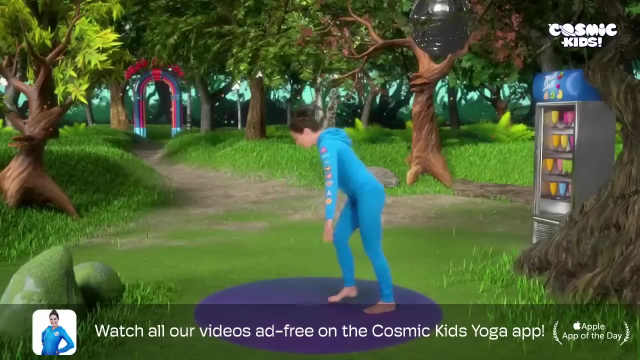 every week, Fairy Floss arranges a big dance meet-up at the brilliant, brilliant Bubble Club. The Bubble Club is a place to dance, to laugh and to drink milkshakes And it's run by none other than Wonky, who is a worm coming into our worm pose. We lie. 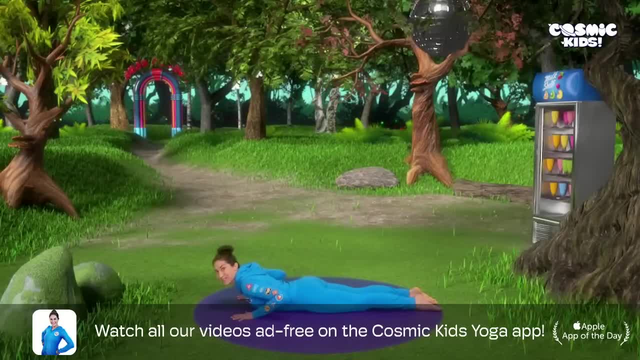 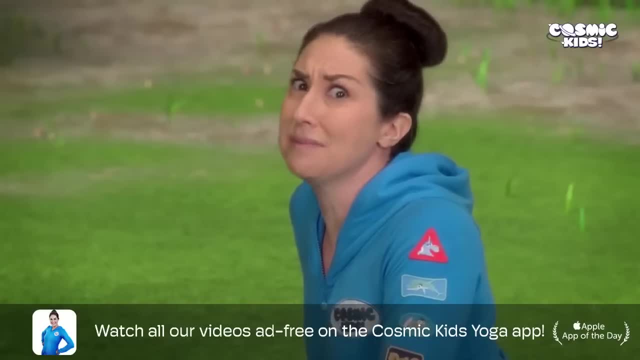 down on our tummies and we bring our hands under our shoulders and we wiggle, wiggle, wiggle, wiggle all the way up like a worm. Now Wonky makes a mean milkshake. He's also got his own special dance move known as Wonky's Wiggle. 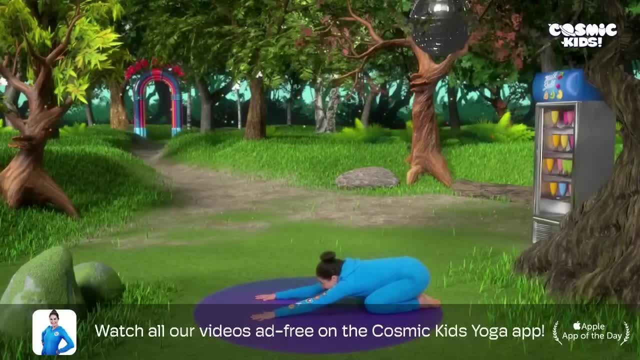 Let's try it. We sit back on our heels, then we slide our body through and we wiggle on up like a worm. And again, Sit back on our heels, slide our body through and wiggle on up like a worm. 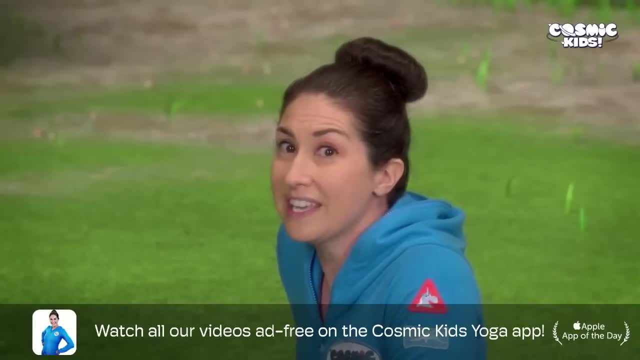 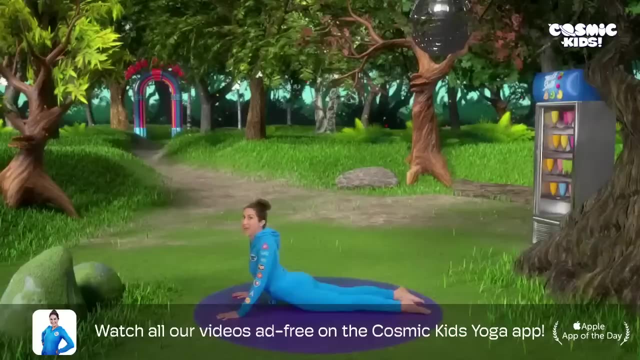 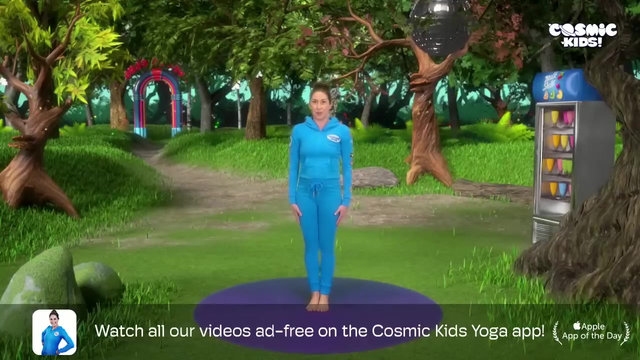 Very good. everyone Now working alongside Wonky is Dez. Dez is a carrot, a disco carrot. He's also a keen gardener. coming up to stand in our carrot pose, We bring our feet together and our arms down by our side. We go all the way around. 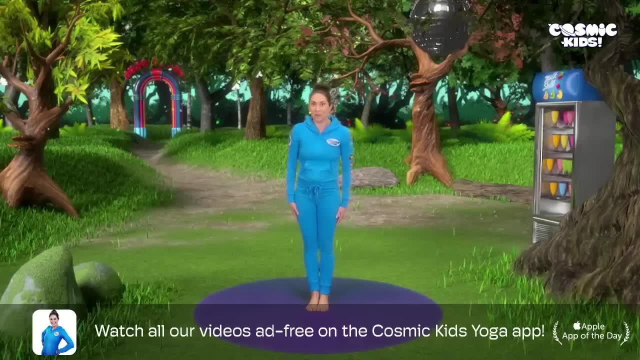 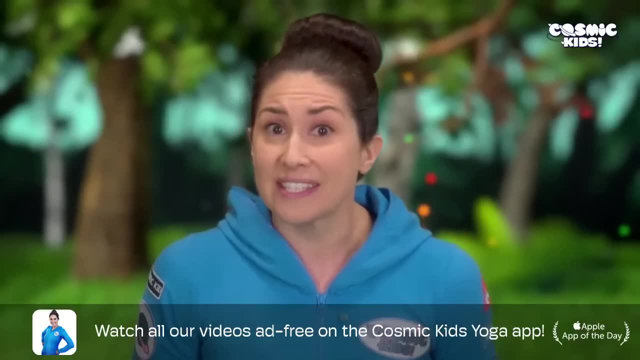 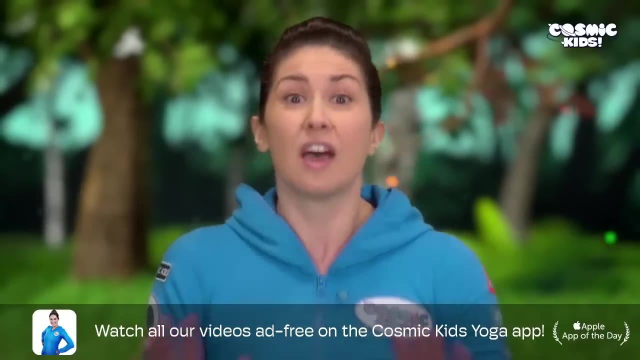 one way, Yeah, And all the way around the other, Yeah. Now Dez has one job at the Bubble Club and that is to turn on the great big giant glitter ball. That's it Now. every week, Fairy Floss flies all over the neighbourhood like a bird, inviting everyone to the dance. 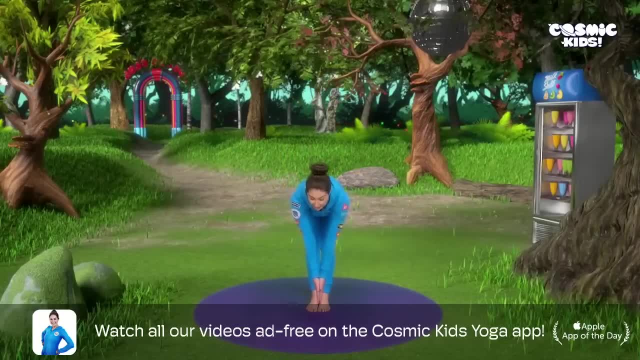 meet Folding all the way forwards. Hands come down, we lift and lower our arms as we fly like a bird. She never misses anyone out, even inviting Nicodemia the witch, who can't bear dancing, Rolling up to stand coming. 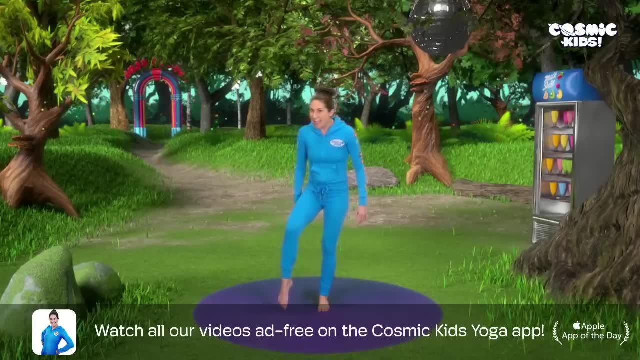 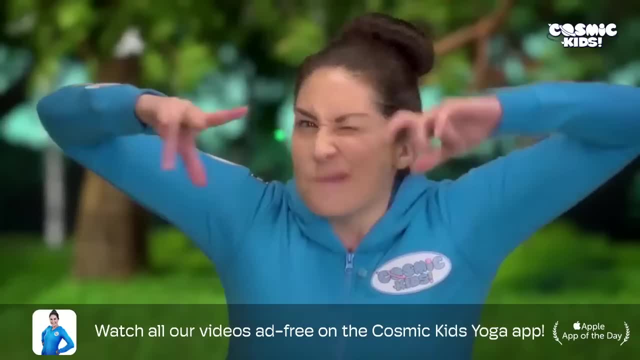 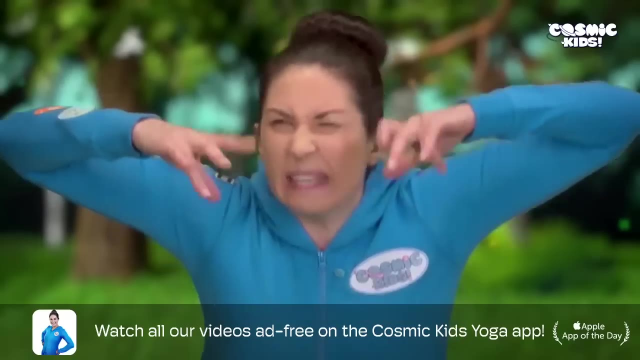 into our witch pose. We stand on one leg using our toe for a bit of balance. We make our fingers all craggy, lift up our elbows, maybe close one eye, and we stick out our tongue. All this dancing making everyone feel good. If only there a way I could make. 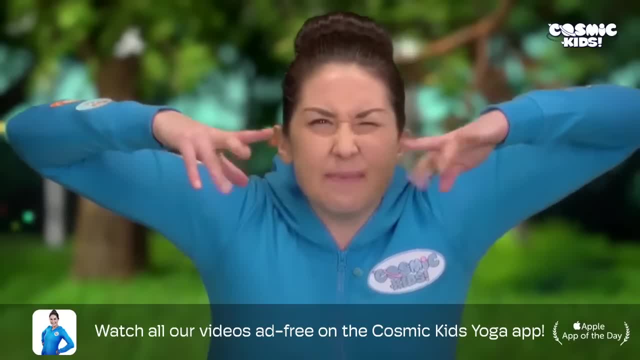 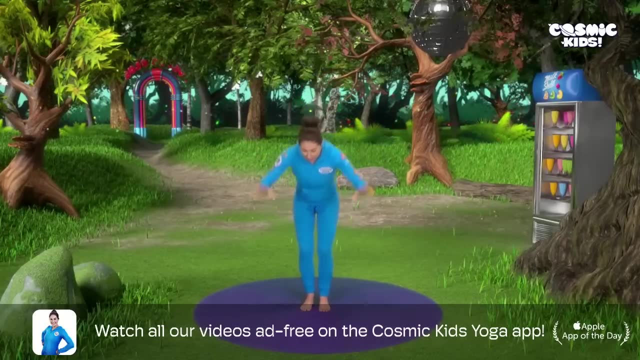 it stop. Fungus. where is my spell book? Fungus is a frog coming into our frog pose. We crouch all the way down, take our knees wide and we use our fingers like little froggy finger pads for balance. Now, Fungus the frog. 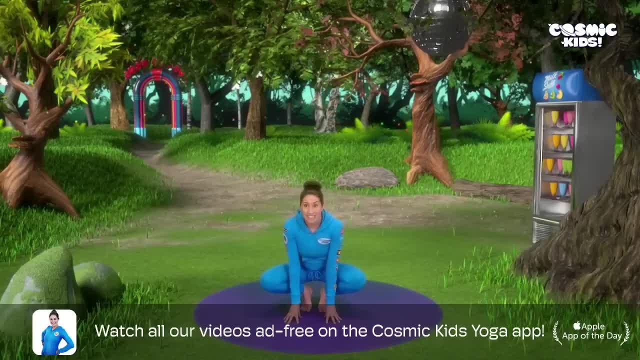 has been servant to Nicodemia since he was a tiny tadpole. He hops all over the cottage looking for the spell book. After three, let's do a hop and a ribbit Ready, One, two, three Ribbit. 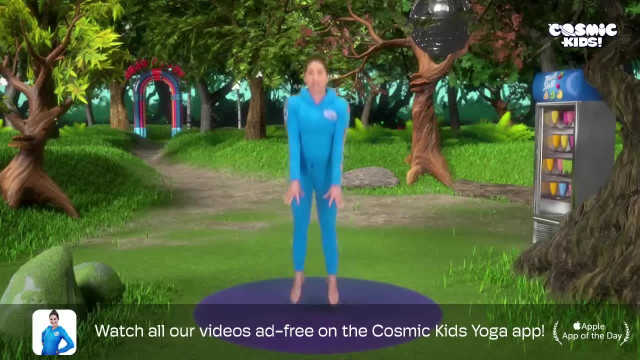 And again One, two, three Ribbit. I found it, milady. Just then, Fairy Floss arrives with their invitations for the dance meet-up. Coming down onto our knees, Nicodemia opens the door, Taking our leg to the side. 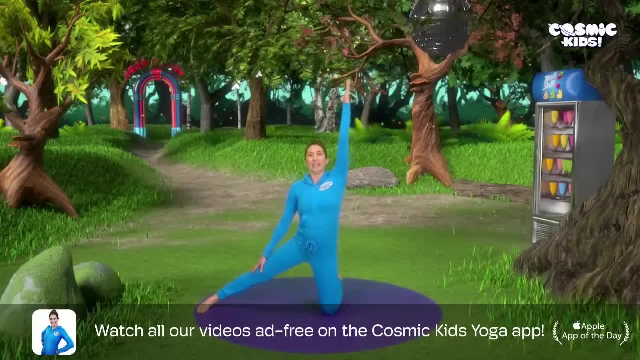 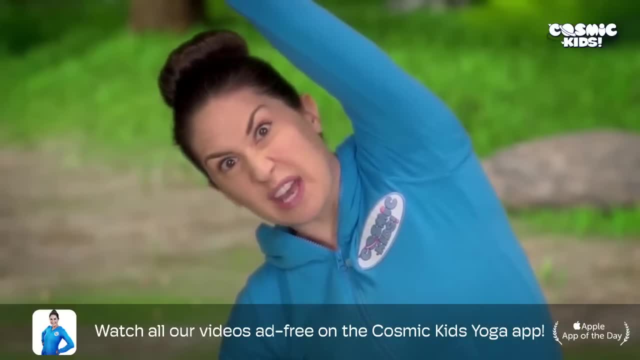 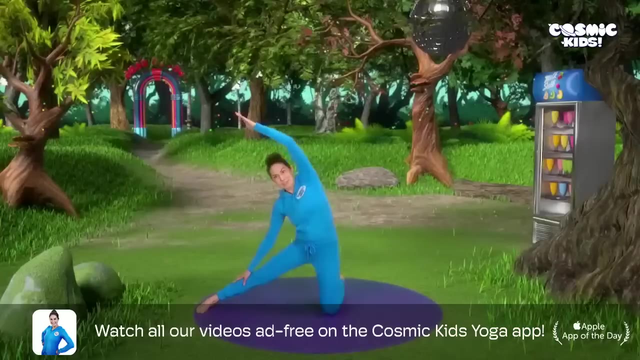 our arm up to the sky. we open the door, going Eeeeee. She stares at Fairy Floss with her grumpy witch face. What do you want, Fairy, Not put off? Fairy Floss stands and smiles Coming up to stand. 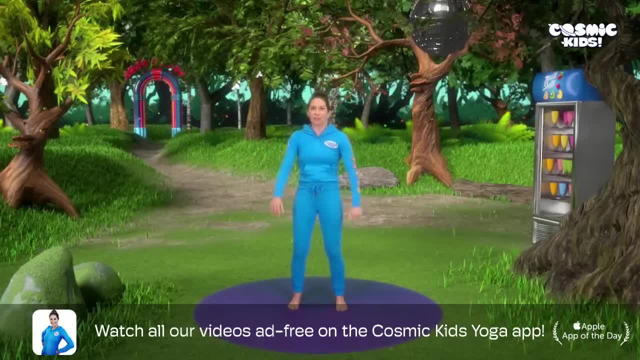 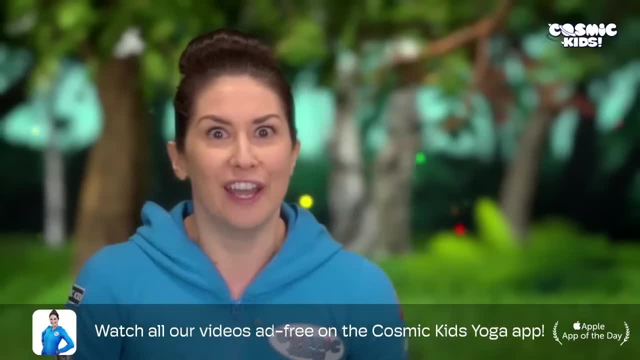 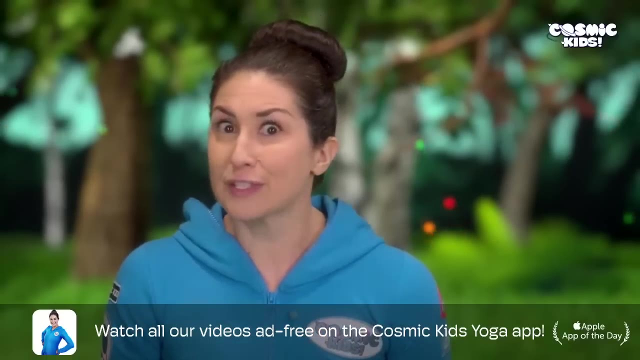 Hello, Just popping round to offer you both an invitation to the dance meet-up, To the dance meet at the Bubble Club tomorrow, And to suggest some dance moves that could be fun to try. Nicodemia stares unimpressed. Fairy Floss continues. 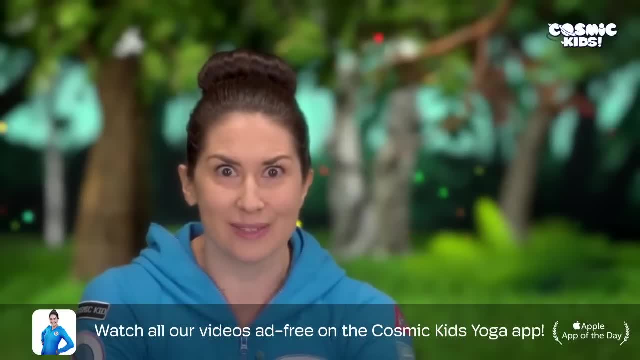 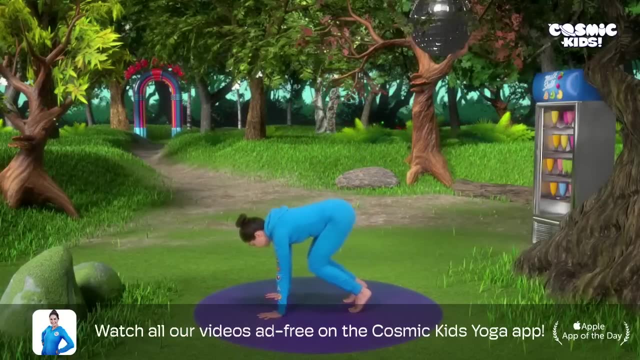 Right now I am loving the bunny bounce. Let's give that a try. You come all the way down, put your hands flat, stay high on your tiptoes and lift up your hips. Then you do a little hop Ready: One, two, three. 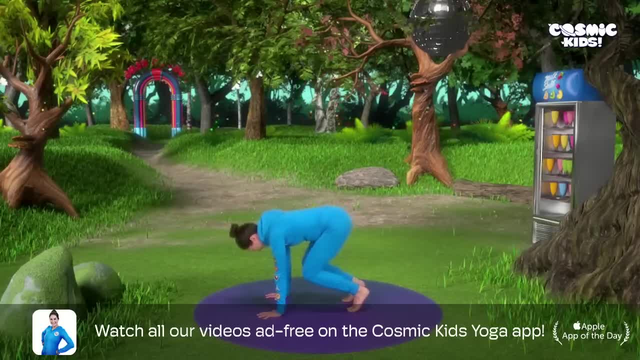 Hoppity, hoppity, Hoppity, hoppity, And again One, two, three, Hoppity, hoppity, hop, No, Okay. Well, there's also the washing machine move where you sit on your bottom with your legs crossed. 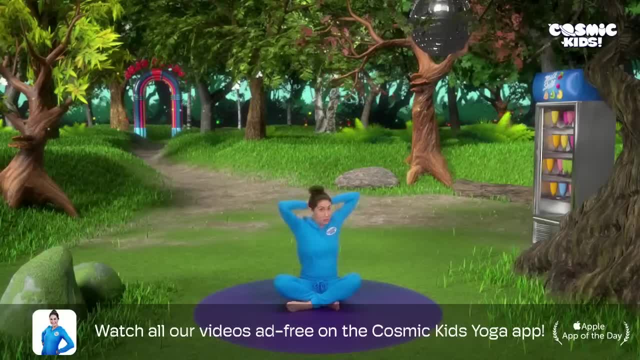 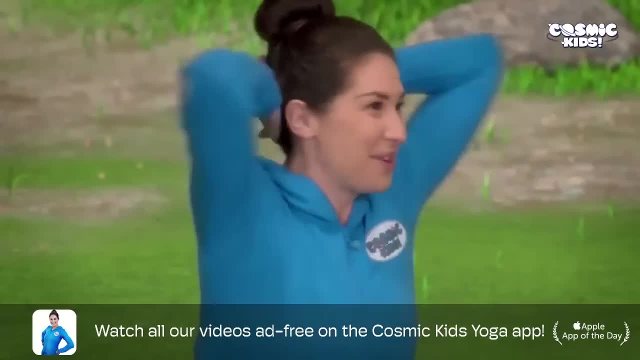 criss-cross your fingers, put them behind your head, and then you twist from side to side, saying: Whisher washer wisher, washer, wisher, washer woo. Whisher washer wisher, washer, wisher, washer woo. 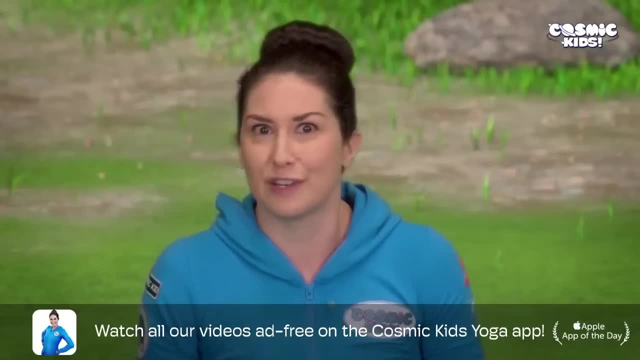 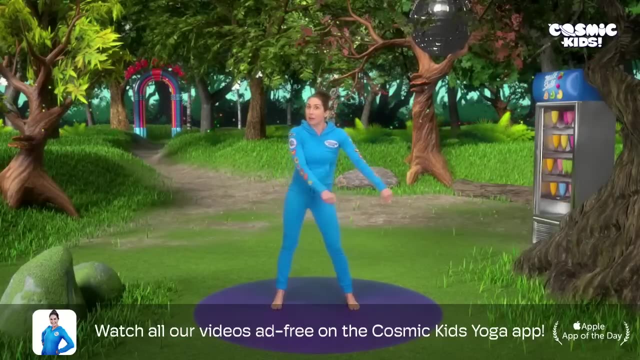 No, Okay. Well, there's also my favourite dance move, the Floss. Let's give that a go. You come up to stand legs a little bit wide Now your arms go the opposite way to your hips. Here we go. 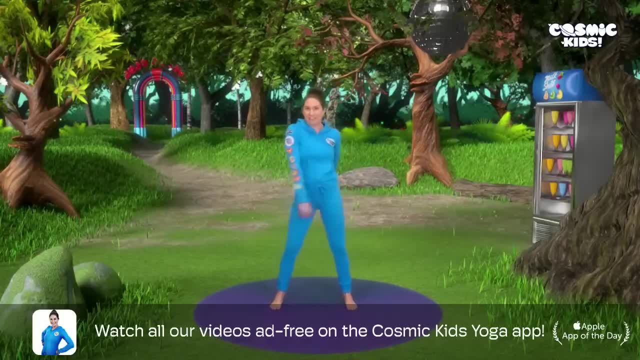 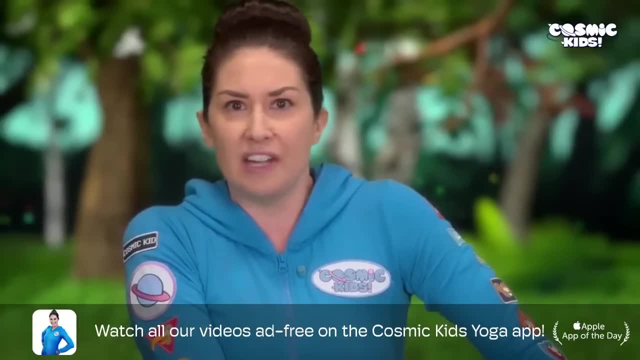 Fairy Floss- do-do-do-do-do-do. Fairy Floss- do-do-do-do-do-do. Fairy Floss- do-do-do-do-do-do. Fairy Floss. Nicodemia can't bear anymore and she slams the door in Fairy Floss's face. 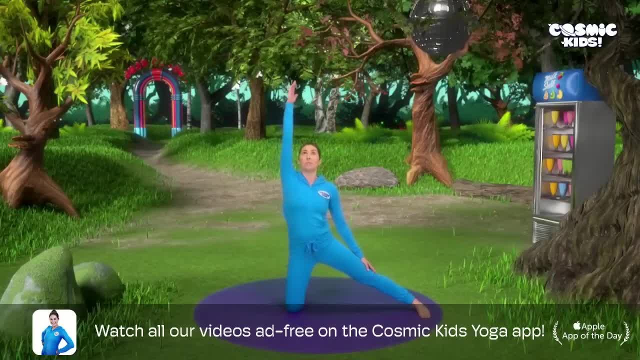 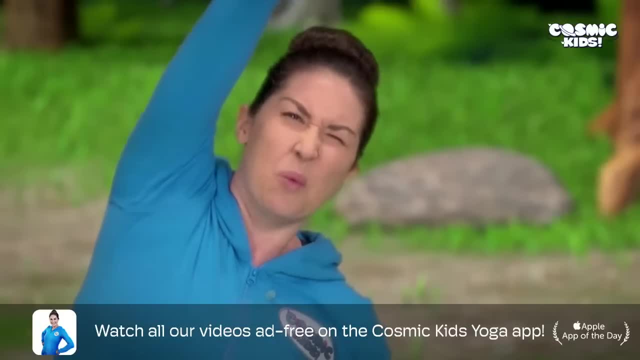 Coming down onto our knees, leg to the side, arms to the skull and Salaam. It's time to put an end to all this dancing once and for all. That night, Nicodemia rides on her broomstick, Coming into our broomstick pose. 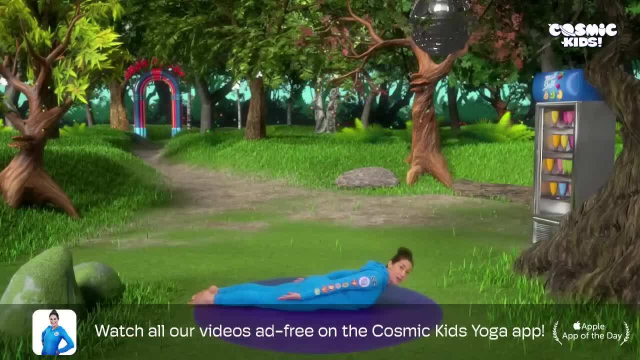 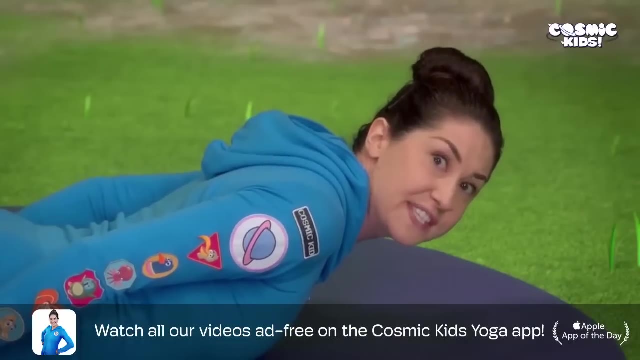 we lie on our tummies, our arms down by our sides, we lift up our chest, lift up our feet and we fly going whoosh Through the night sky straight for the bubble. When she arrives, Nicodemia turns herself magically. 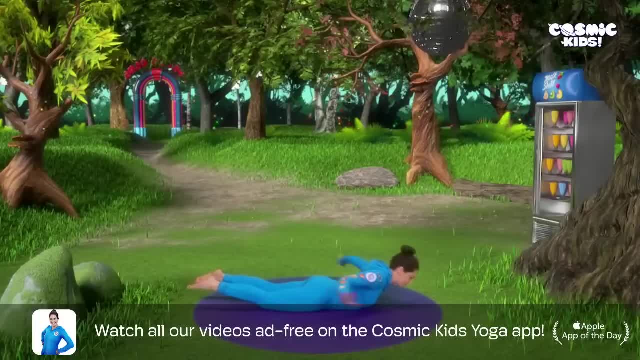 into a cat, Coming into our cat pose up onto our hands and knees, we tuck our toes and we arch our back looking into our tummy. Then we dip our tummy down and we wiggle-waggle our tail, saying: 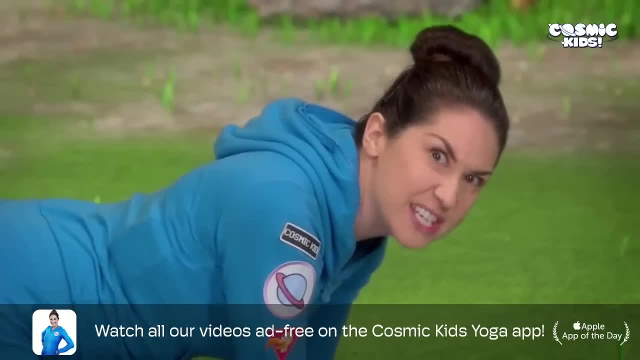 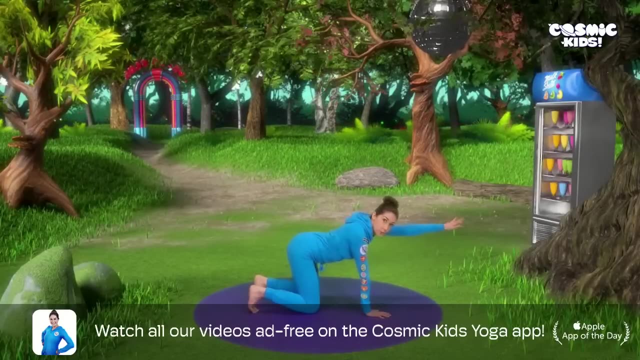 Meow Quietly. she slips in through the cat flap, reaching in with one paw, reaching in with two, reaching in with three paws, reaching in with four. Then she rolls herself back up to her normal witchy self, walking your hands all the way back. 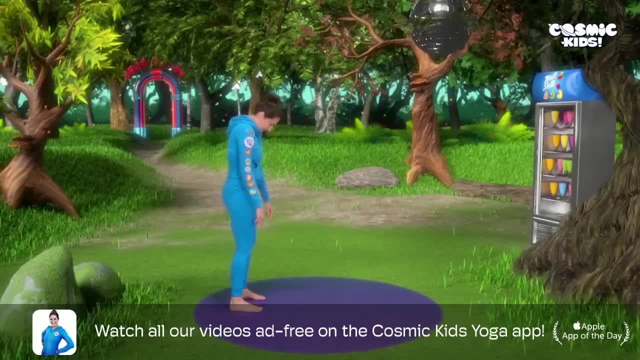 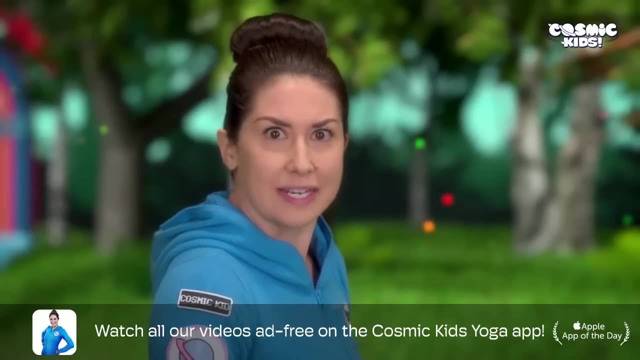 and rolling up to stand, keeping your knees bent, head to come up last. Then she takes out her wand and she points it straight up at the giant glitter ball, Stepping one foot forward, one foot back, bending into our front knee. 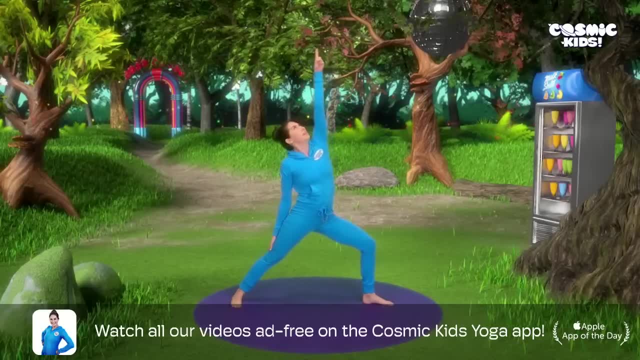 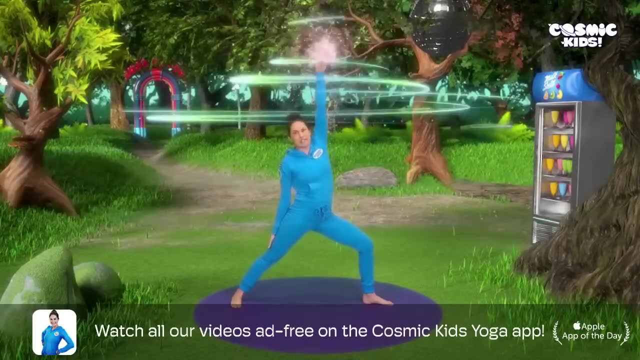 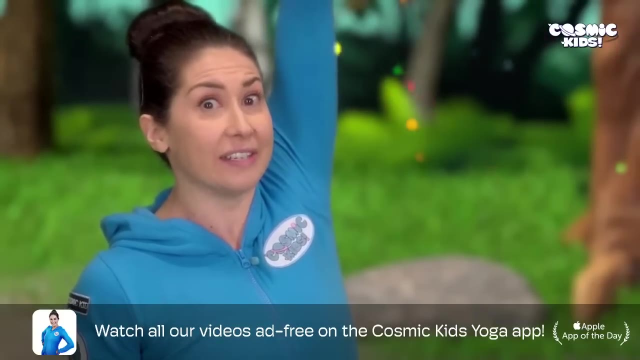 stretching our top arm all the way up, making our finger a point like we're holding a wand, Then she encants her spell, She turns, and she does it on the other side, turning to face the other way, bending into our front knee. 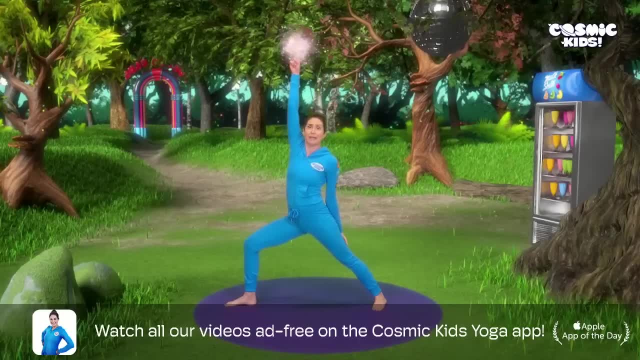 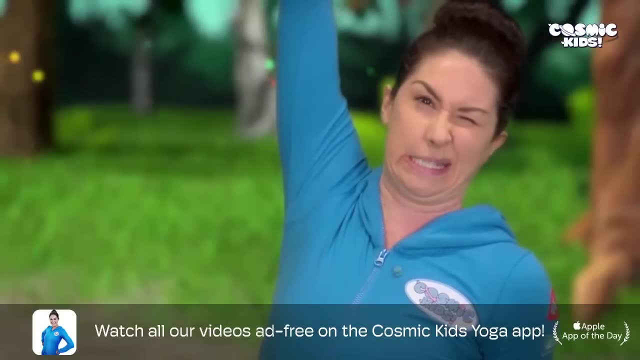 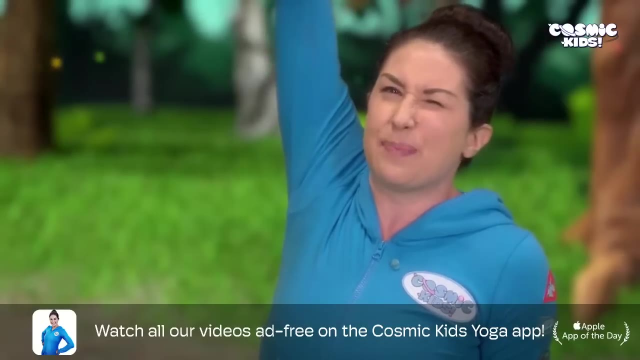 reaching our arm all the way up, She encants her spell again. Now, when they all start dancing and their precious glitter ball begins to spin, they will all turn to stone And with that she disappears in a puff of smoke, coming all the way down to crouch. 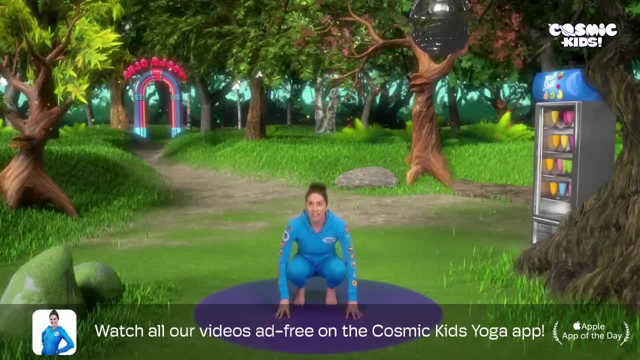 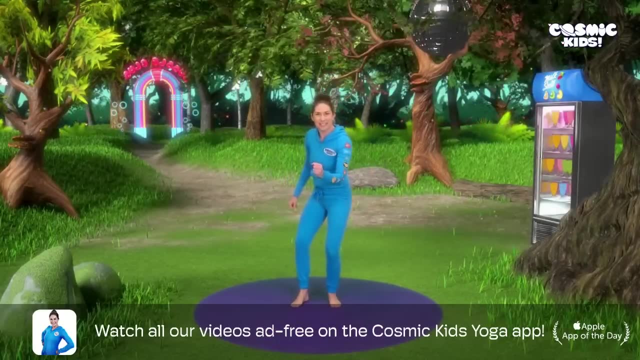 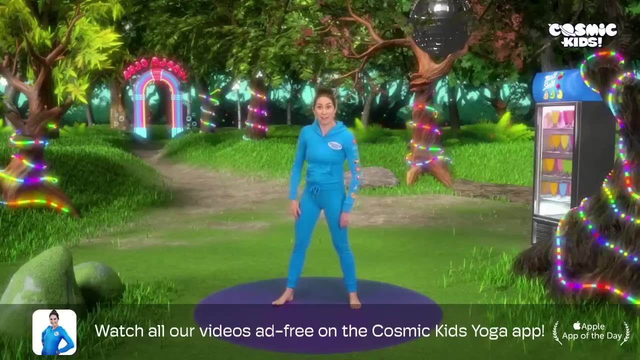 After three big jump and a puff: One, two, three puff. The next day is the dance meet, The music starts and the dancing begins. It's led by Fairy Floss doing her favourite dance, the floss. 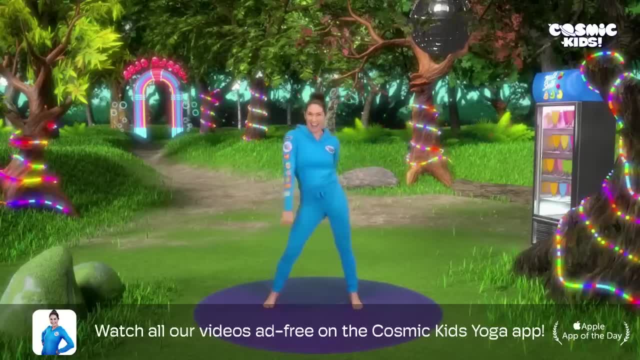 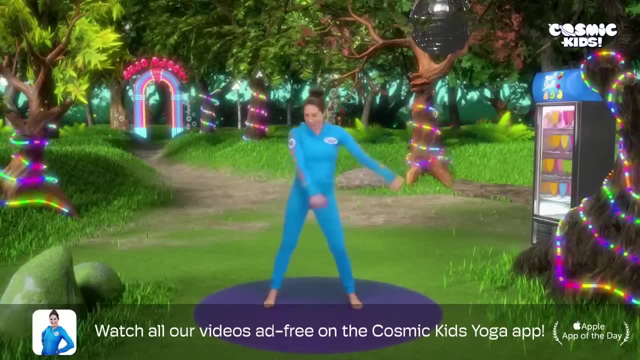 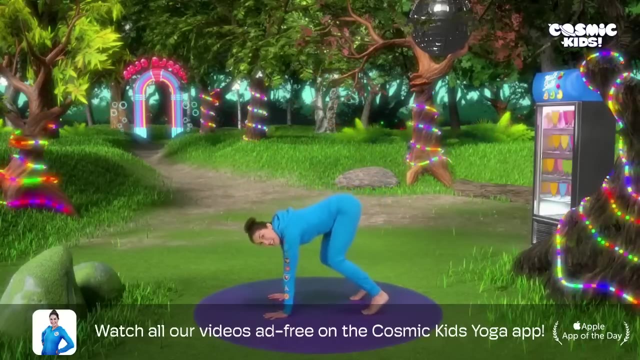 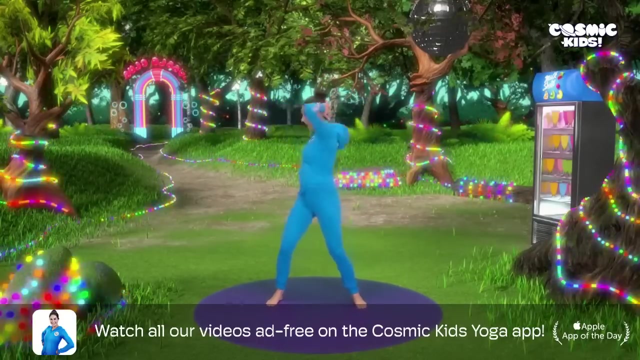 Here we go. everyone, Yeah, Give it some floss. everyone. She does some bunny bouncing. Ready to hop? Here we go, Hop And again Hop. Last time, Hop, Coming all the way up Washing machine And a knee cross. 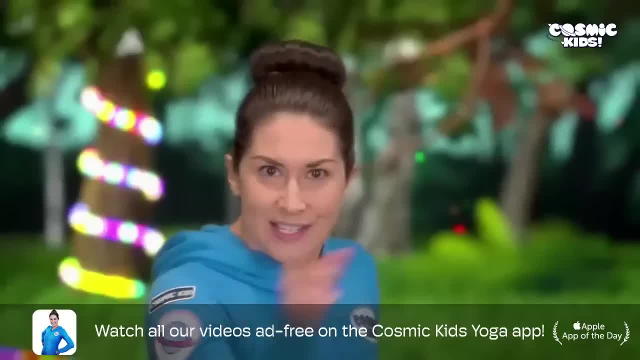 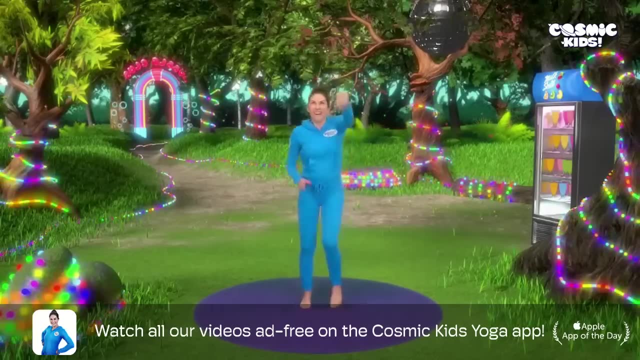 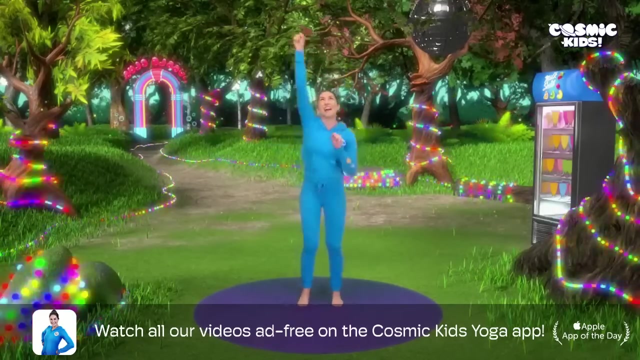 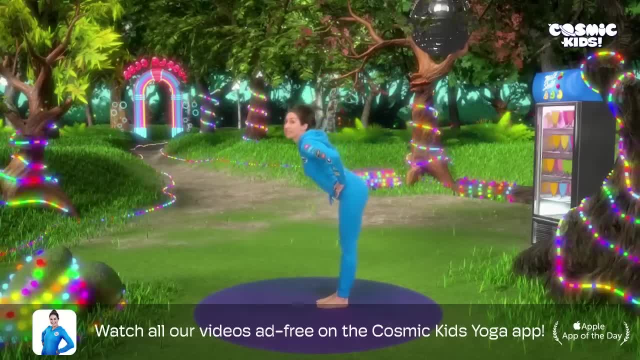 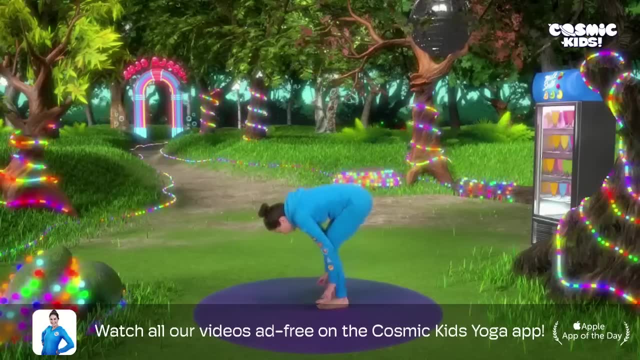 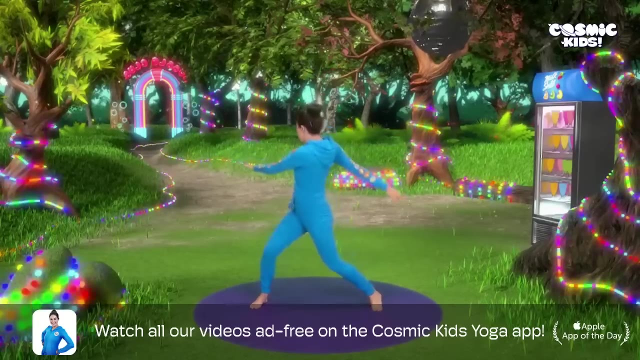 He turns to the side, folds his little carrot body in half and he presses go on. the big green go button Rolling up to stand, the glitter ball begins to spin, Taking our legs wide, arms wide, and we spin As soon as it does. 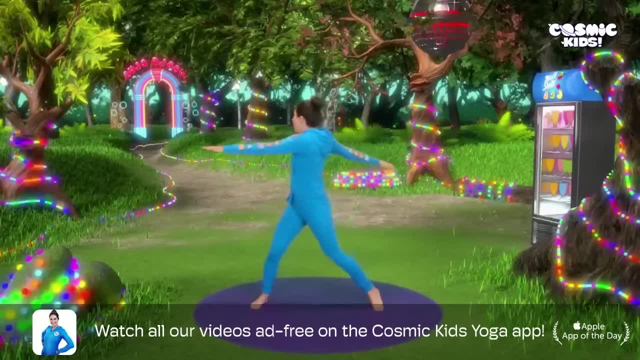 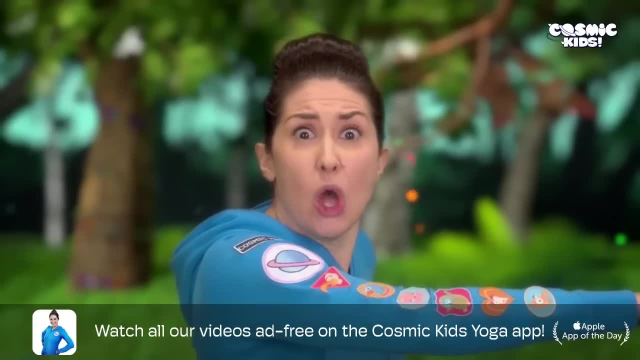 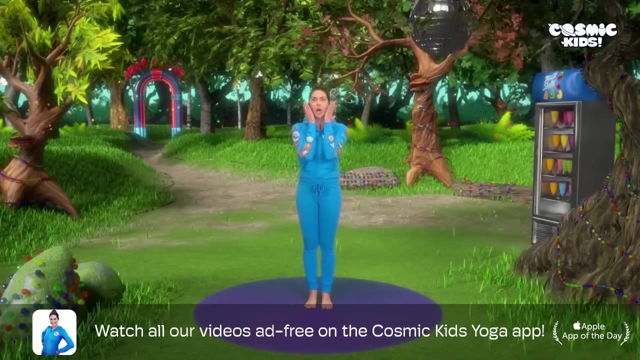 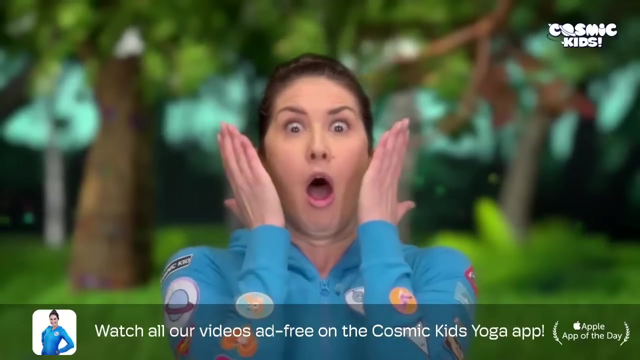 Nicodemus' spell is activated. Everyone freezes because everyone has turned to stone. Jump your feet together, hold onto your face, Dez. the disco carrot is horrified, Oh no. And then he spots someone hopping out of the bubble club. It's Fungus the frog. 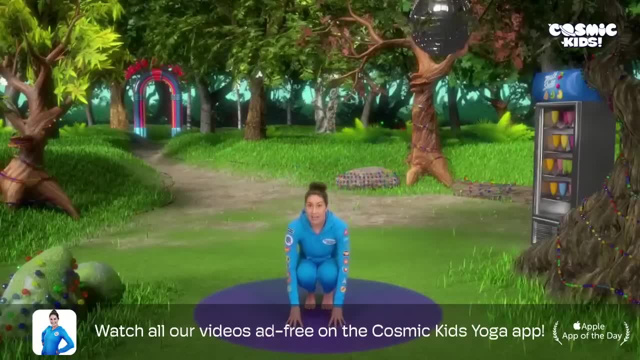 Coming into our frog pose, Crouching all the way down knees, come wide balancing with our froggy fingertips. After three, let's do a hop and a ribbit. One, two, three, Ribbit And again One, two, three. 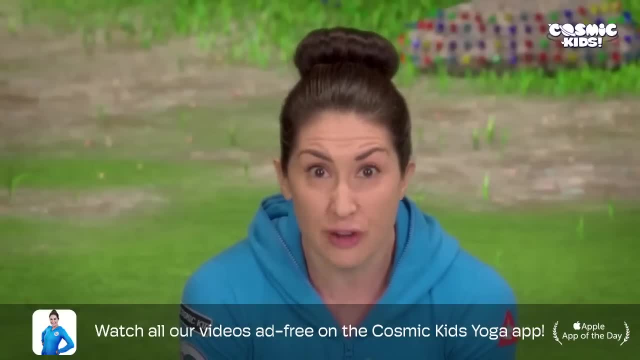 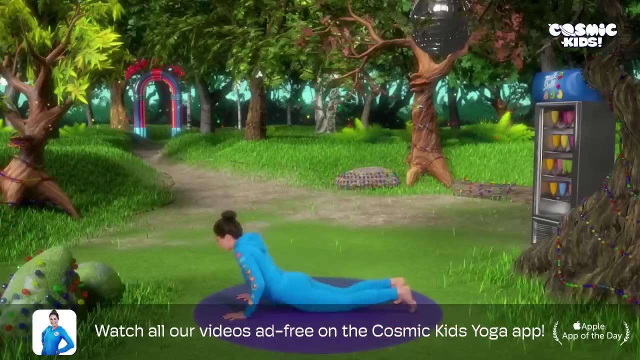 Ribbit Wonky the worm comes out of the fridge and he sees him too Coming into our wonky the worm pose Lying on our tummies, hands under our shoulders, Wiggle, wiggle, wiggle, wiggle all the way up. 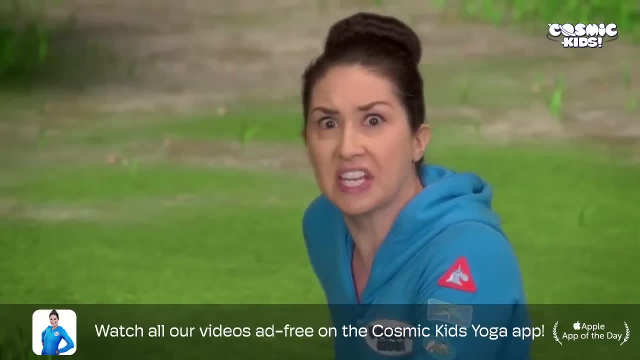 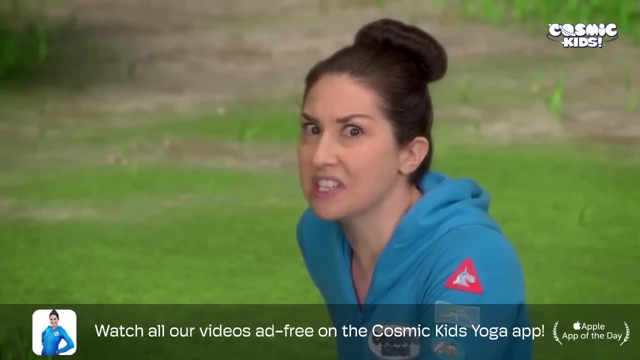 Now we know who's behind this, Dez: It was Nicodemia. We've got to find out how to break the spell, And so Wonky and Dez go to Nicodemia's cottage, Coming to sit on our heels When they arrive. 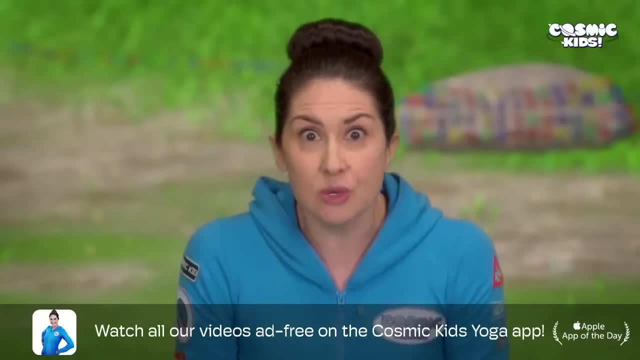 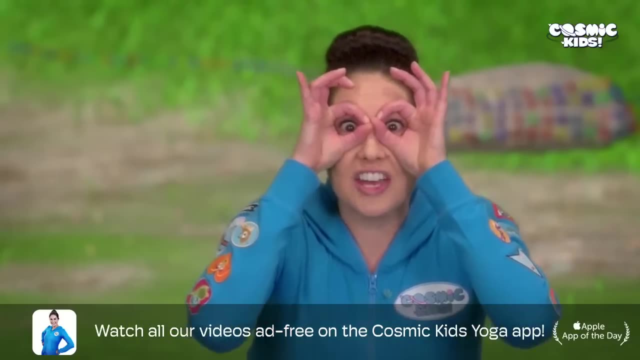 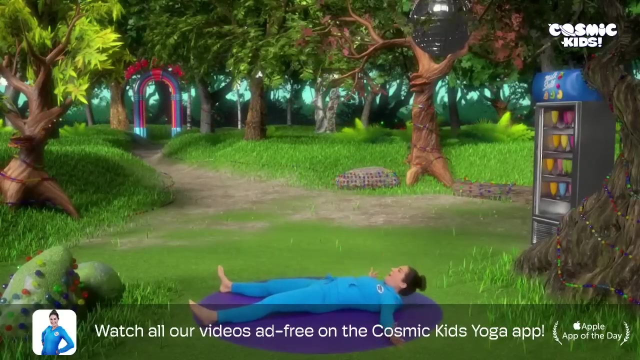 Wonky and Dez peep in through the window using their cosmonoculars, Joining our thumbs and fingers together. Have a look through. There she is Lying on the couch, Coming to lie down everyone. Legs wide, arms wide. 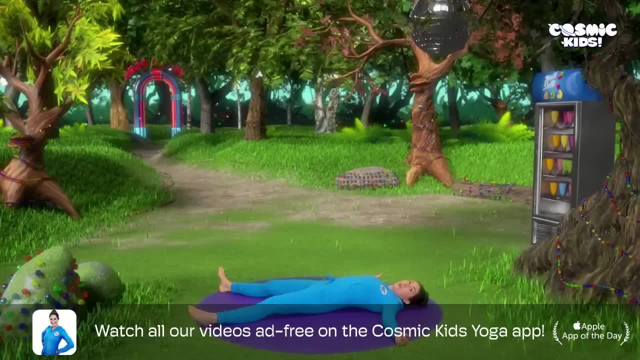 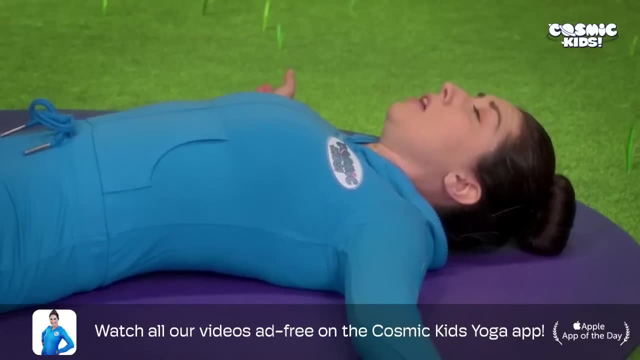 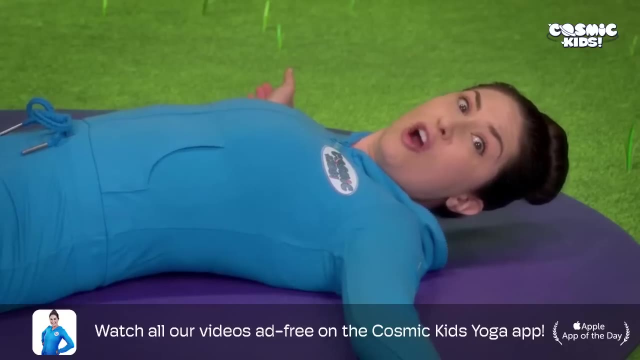 She's asleep And she's snoring loudly Like a witch. In the corner in his frog basket is Fungus the frog. He's also lying asleep, But with his legs in the air, Lifting our legs up. 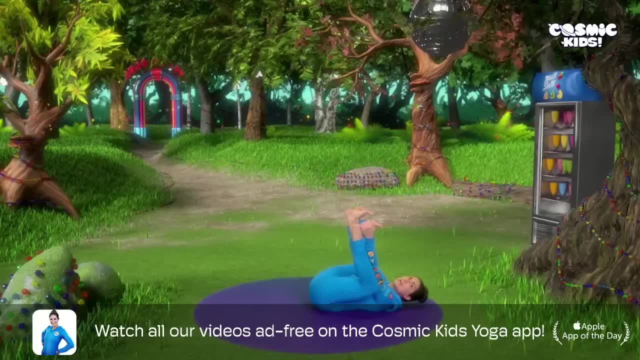 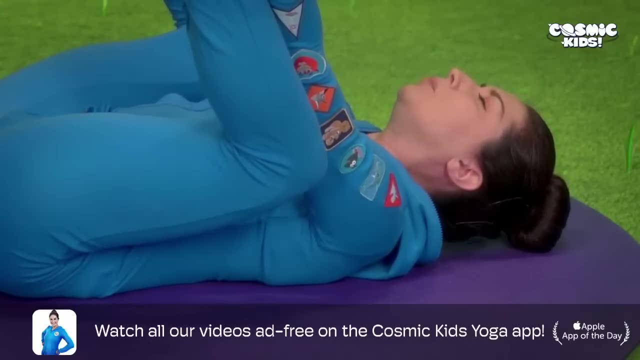 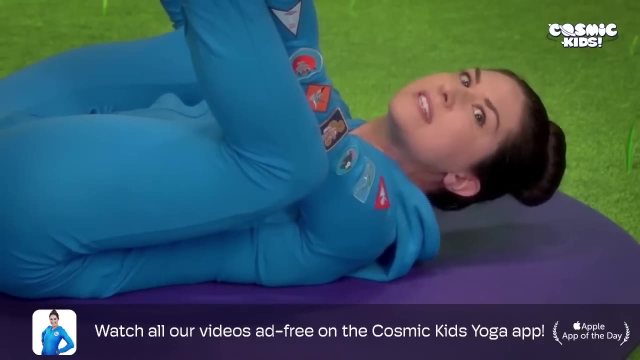 Holding onto the soles of our feet. He's also snoring loudly, But like a frog, Ribbit. Ribbit Dez keeps a lookout And does a bit of weeding in the garden While Wonky wiggles inside. 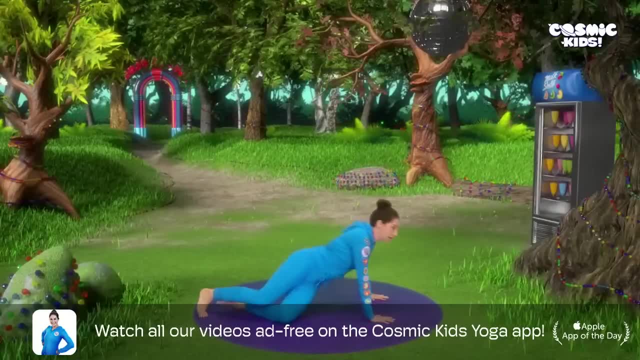 Bravely Coming onto our tummies. everyone Hands under our shoulders. Let's wiggle in, Wiggle, Wiggle, Wiggle, Wiggle, Wiggle, Wiggle. He finds Nicodemia's spell book Coming into our book pose. 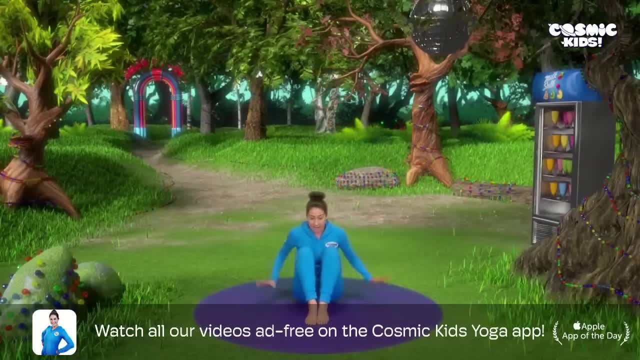 Sitting on our bottoms, Knees bent, Feet, flat Hands on our knees. The book is still open, Lowering our knees down to the side. The page is titled How to Stop Dancing. Wonky reads down the spell And at the bottom is a note that says: 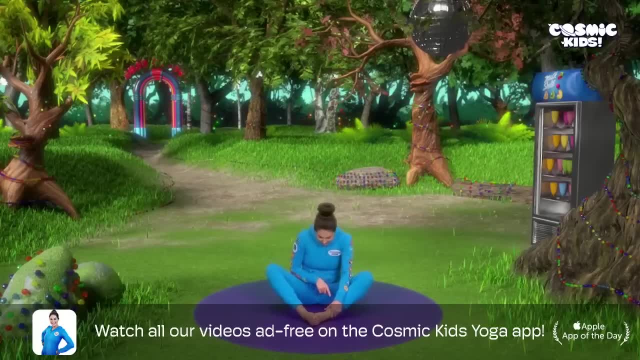 How to break this spell. It reads: Find as many people not under the spell To dance, dance, dance Until they hear a bell. When the spell is broken, A new curse shall begin For the one who cast it: To forever dance like a chicken. 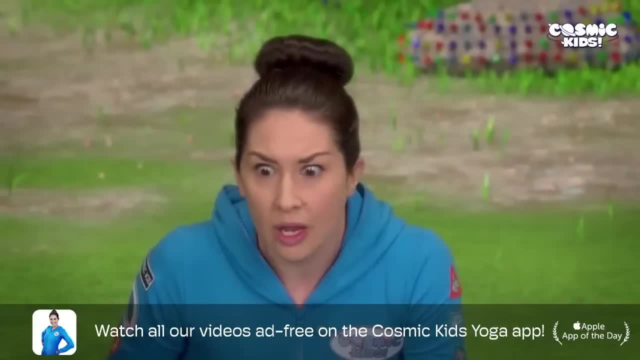 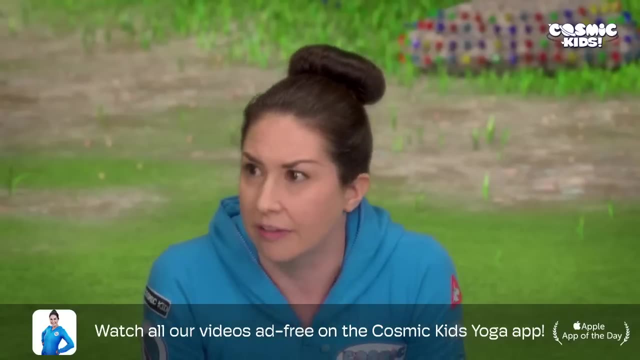 Chicken. It says chicken, So so this means, When the spell is broken, Nicodemia will forever dance like a chicken. Well, that is something Wonky quietly, silently, wiggles out, Trying not to disturb Nicodemia and fungus. 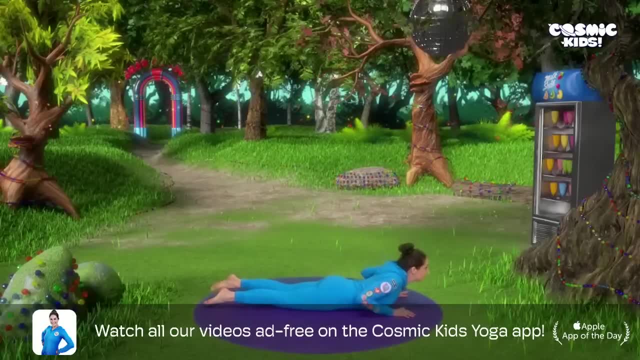 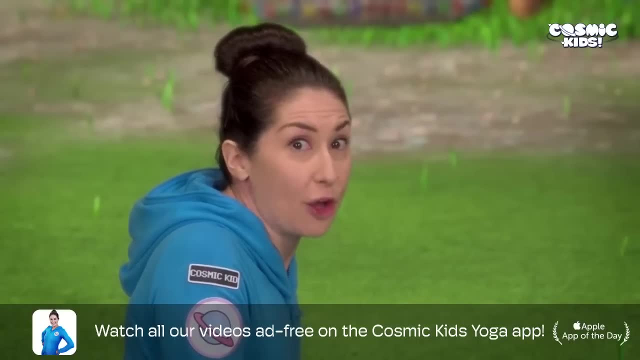 Coming back onto our tummies, Hands under our shoulders, Wiggle, Wiggle, Wiggle, Wiggle, Wiggle, Wiggle. Back at the bubble club. Wonky and Des start phoning round Everyone they know Sitting on our bottoms. 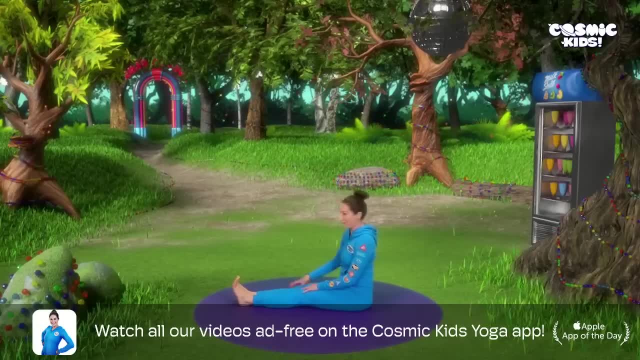 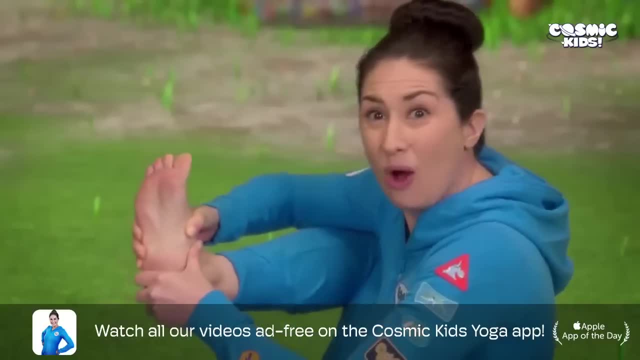 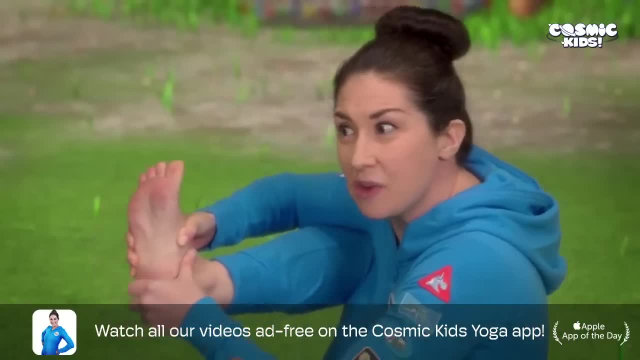 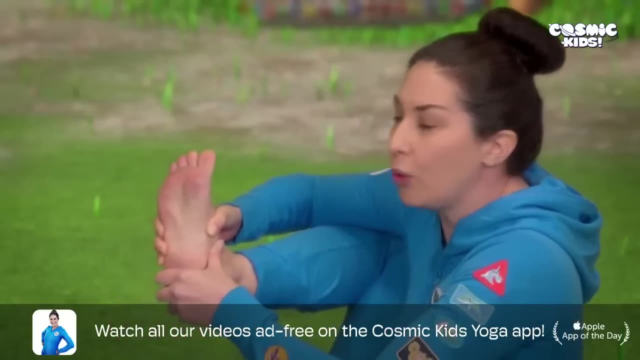 How are you? Oh good, How are all the gnomes? Yeah, they all, okay, Excellent, Look, we've got a favour to ask. Would you mind gathering as many gnomes as you can? Yeah, all your gnome friends. 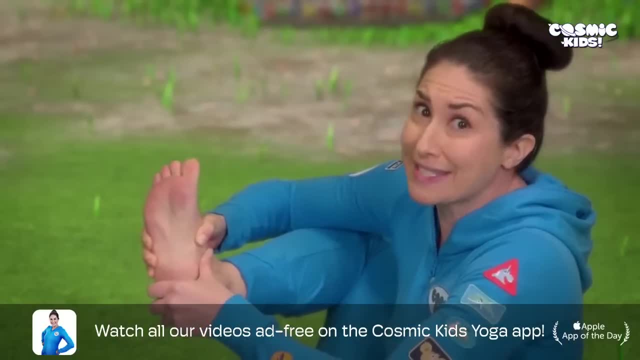 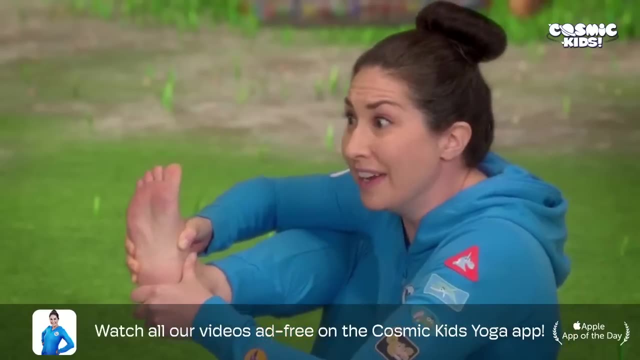 Bring them to the bubble club, Because we need you to dance. Yeah, we've got to break this spell. Nicodemia, she's turned everyone to stone. I know it's awful. Oh, you'll come, Yeah, And you'll bring them all. 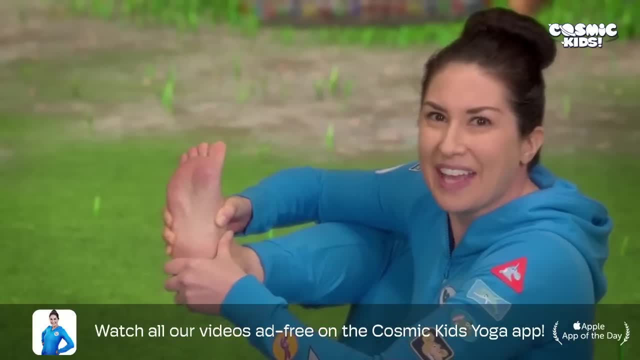 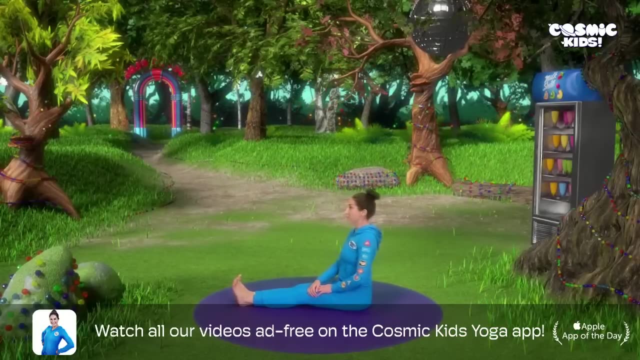 Oh brilliant, you're a star, Bob. We'll see you in a minute. Okay, bye. They put the phone down and the next thing we know our telephone is ringing, Ring, ring, ring, ring. Let's answer it. 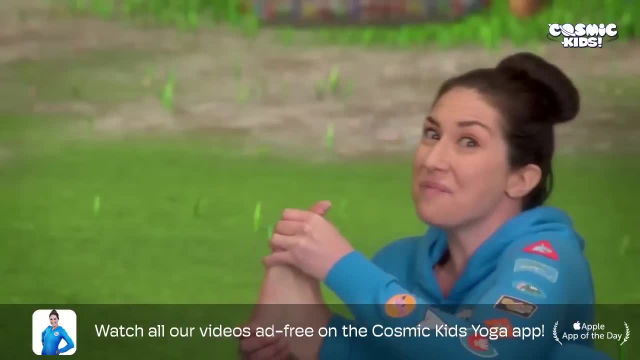 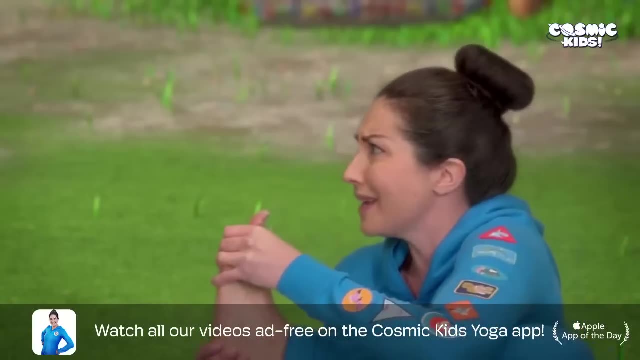 We pick up the phone. Hello Cosmic Kids here, How can I help you? Oh, hi Wonky, Hi Des. Yeah, we heard all about it. Dreadful business, Nicodemia, turning everyone to stone, Awful. 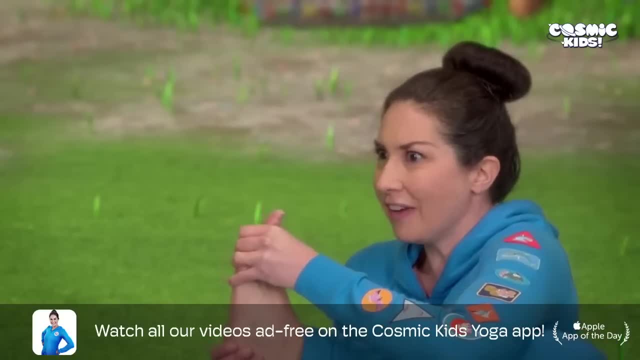 Yeah, we can do that. We can come to the Bubble Club. Yeah, we can dance. Yeah, Cosmic Kids are awesome at dancing. Easy, Yeah, okay, we'll be there in a minute. All right, Wonky Bye. 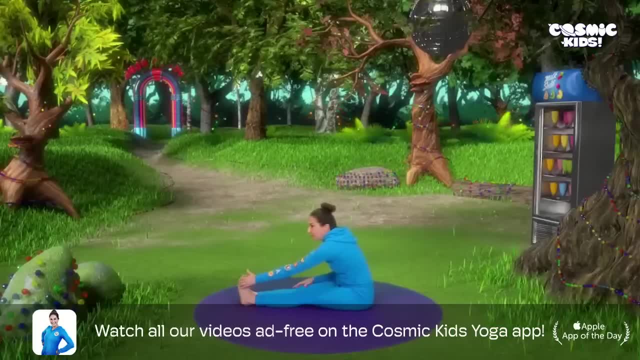 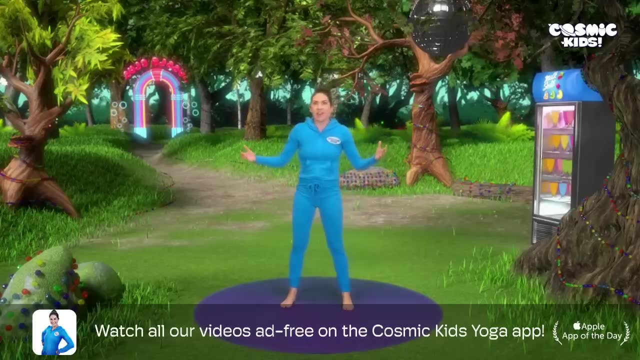 Oh, yeah, yeah, love you too, Des. Okay, bye, Bye. We put the phone down and we get ourselves down to the Bubble Club, Coming up to stand everyone. When we get there, the place is packed full of. 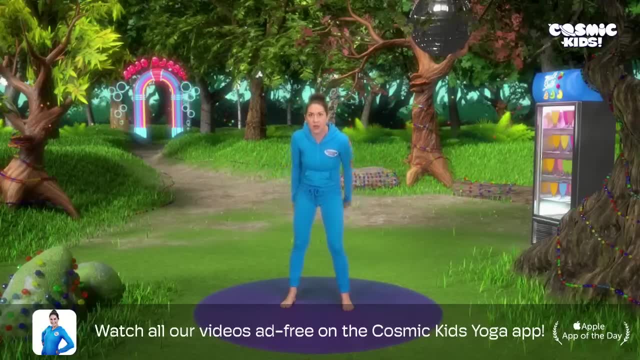 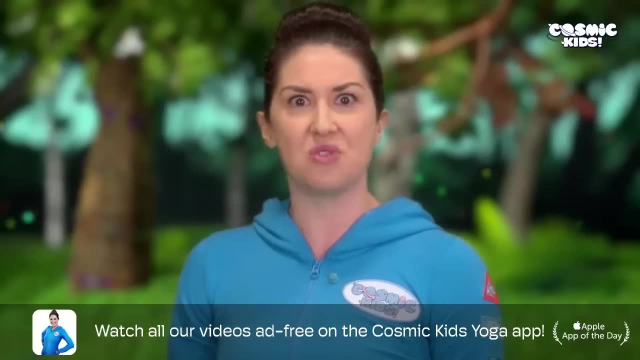 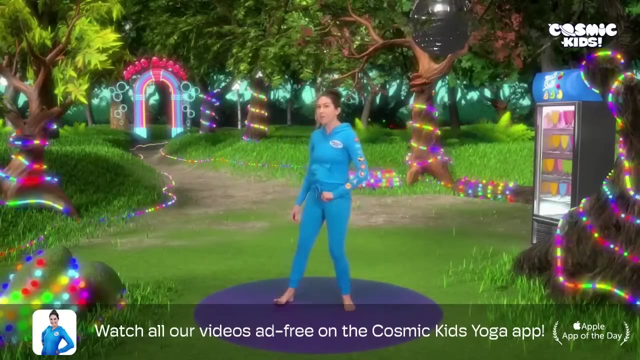 of people and thousands of gnomes. It's time to unfreeze our frozen friends and start the dancing. Wonky cues the music and the dancing begins. We dance in slow motion, starting with a slow motion floss dance. Are we ready? 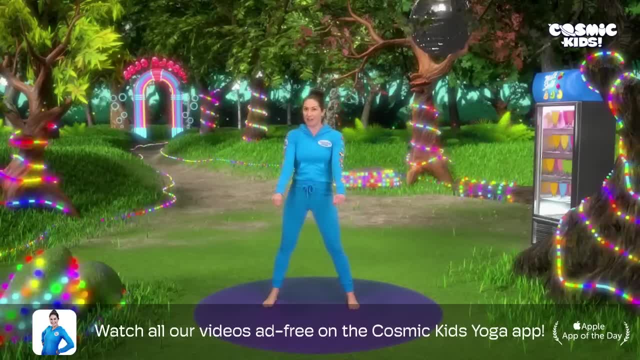 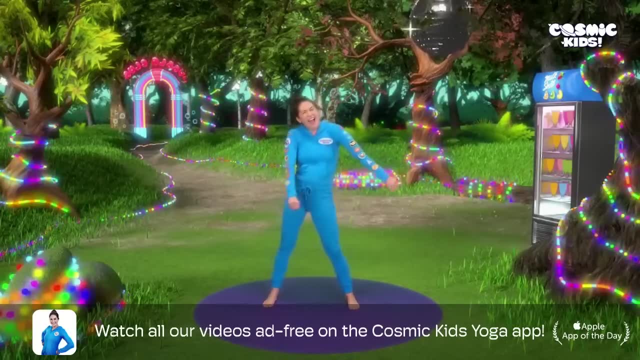 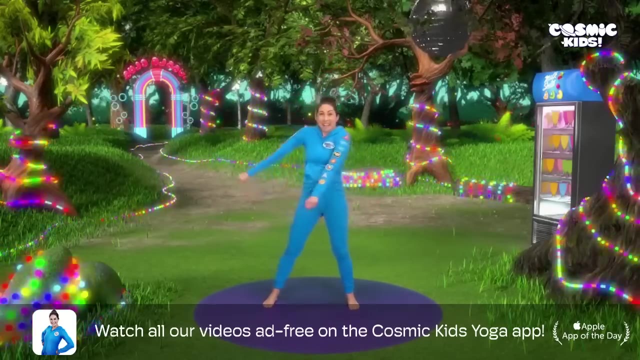 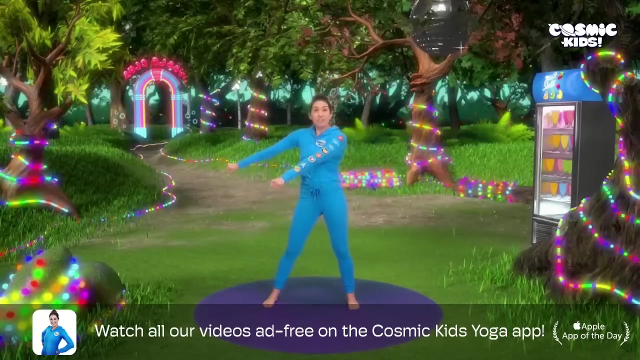 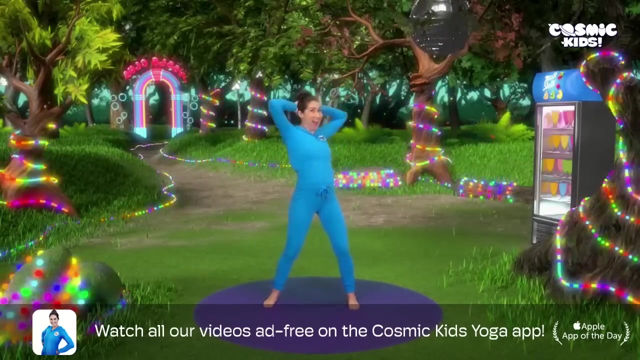 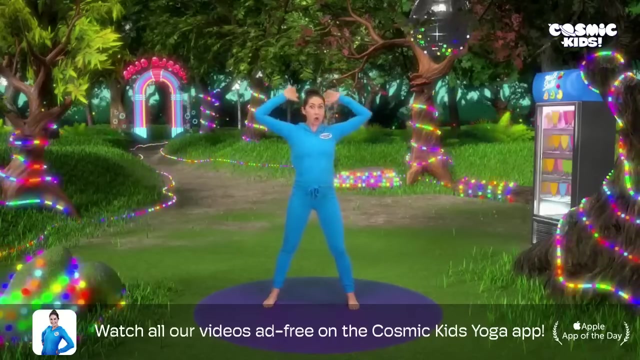 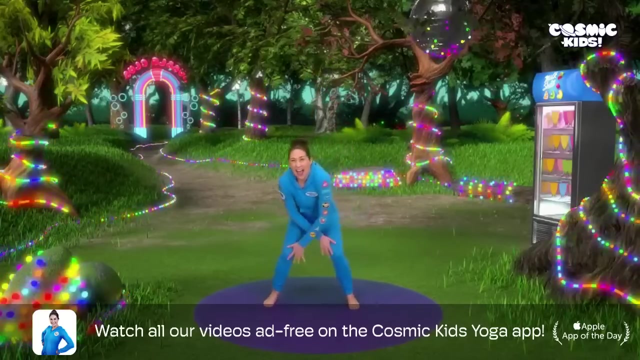 Arms down opposite way, with arms and hips. Here we go, Ready, We do slow-mo washing machine. We do slow-mo washing machine. We do slow-mo washing machine. We do slow-mo knee cross, Slow-mo bunny bounce. 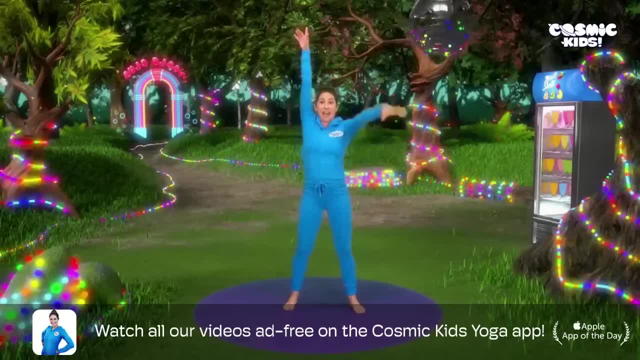 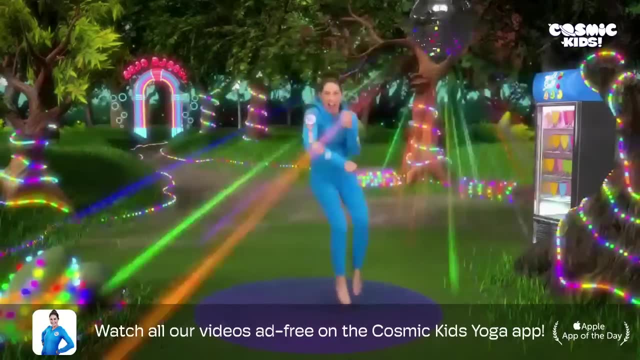 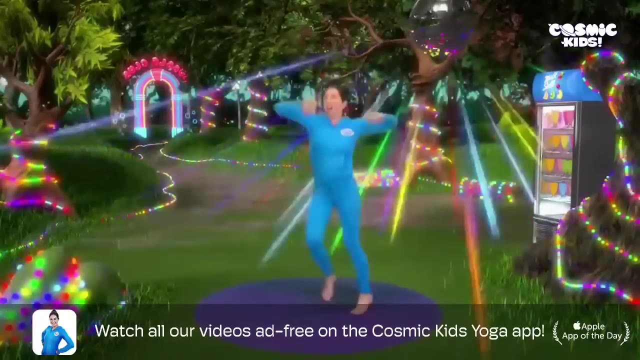 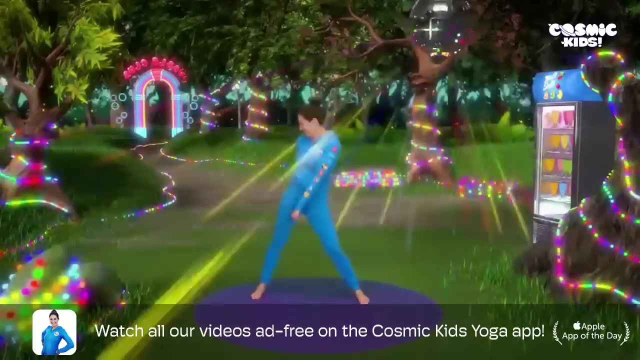 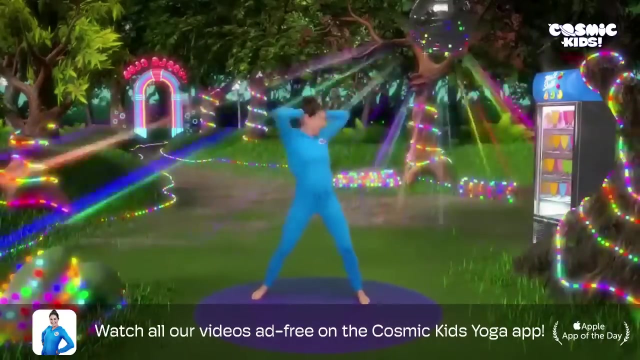 Then we stand up, put our hands in the air and we dance. Here we go Ten or ten seconds. Let's do it Part of it again. We keep dancing, everyone, until we hear the bell. You know what to do. 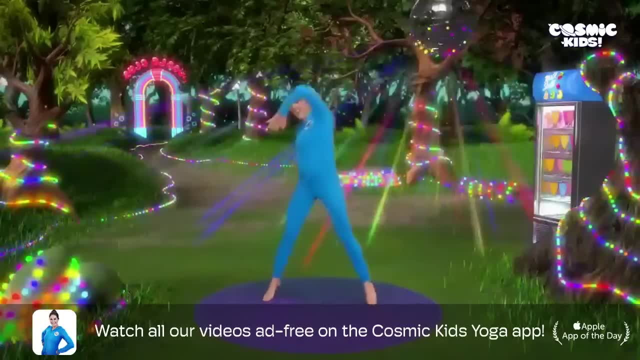 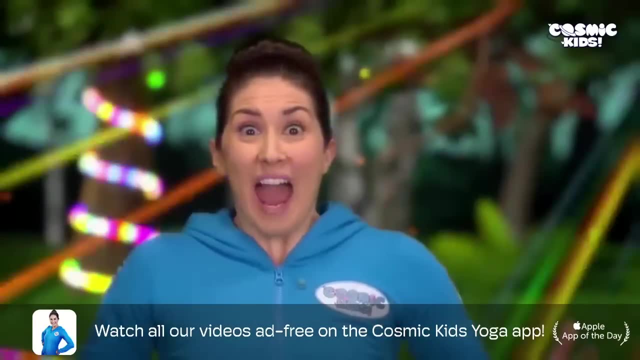 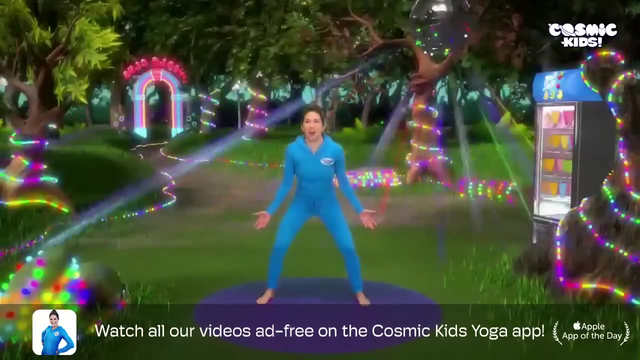 Keep dancing, We keep dancing, everyone, until we hear the bell. did you hear it? yes, we heard the bell. it's worked. everyone who was frozen is dancing again. fairy floss comes running over and she gives us a ginormous hug, reaching our arms wide. 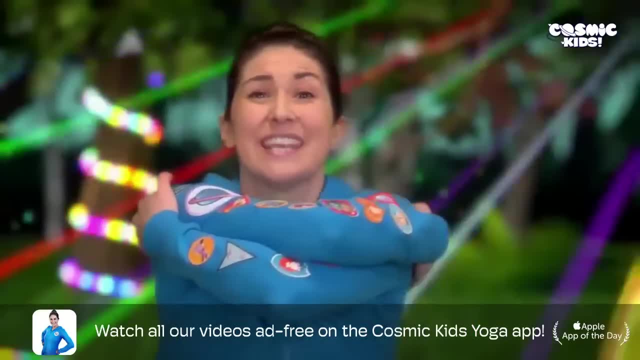 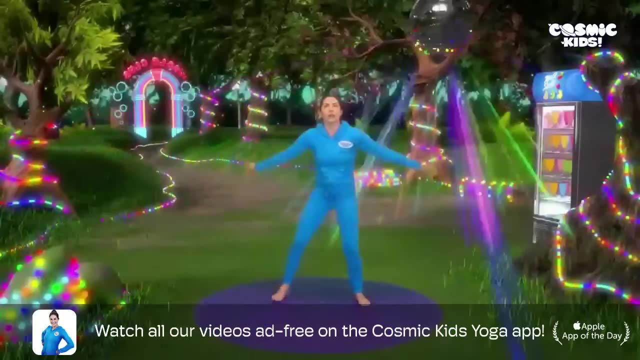 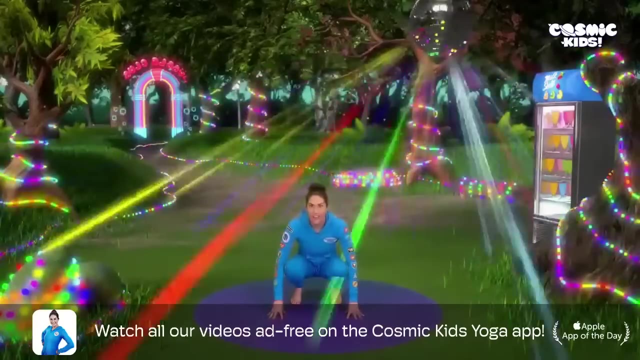 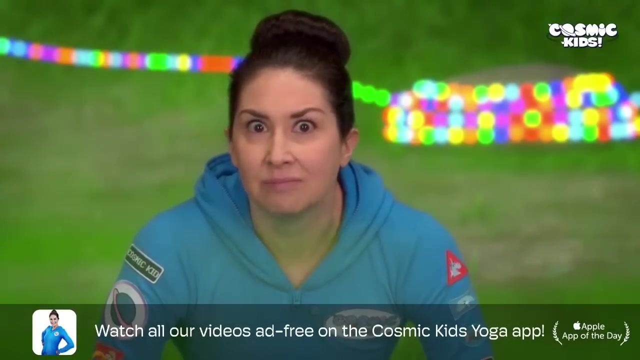 wrapping us up. oh, you've done it, cosmic kids, you saved us with a dance. all of a sudden, there is a puff of green smoke coming all the way down to crouch. after three, let's do a big jump and a puff: one, two, three. appearing before us in the mist is nicodemia the witch, coming up to stand in our witch pose. 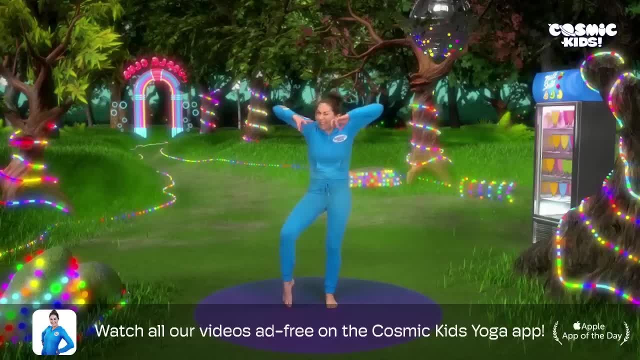 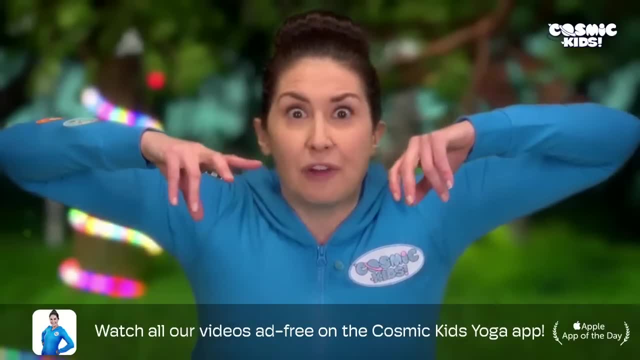 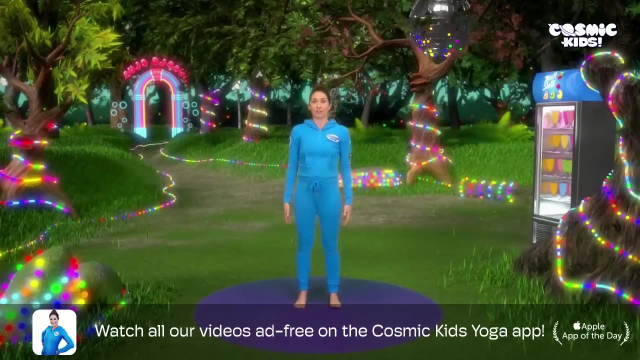 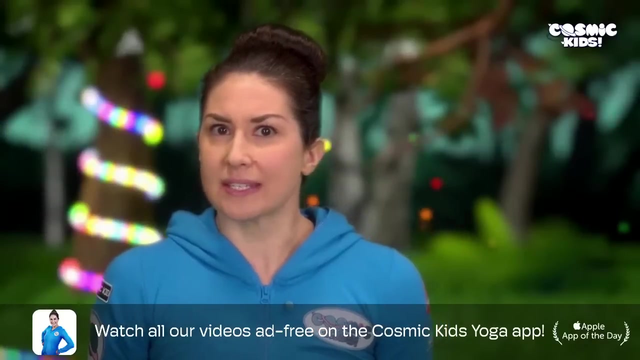 onto one leg, craggy fingers lifting our elbows, closing our eye and sticking out our tongue. everyone stops as still as mountains to stare, standing with our feet, hip distance apart, arms down by our sides, shocked to see her here for the first time. but as the music starts again, 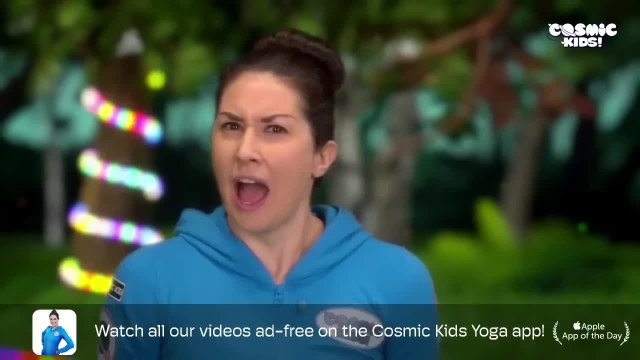 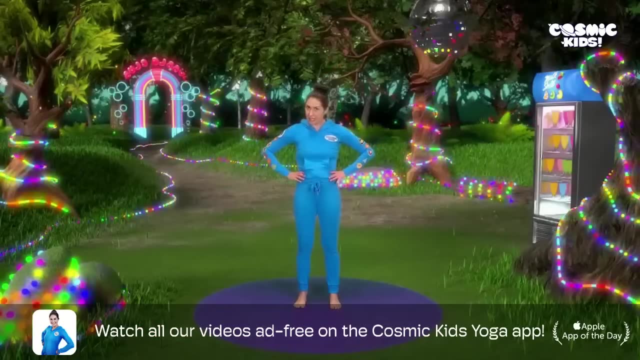 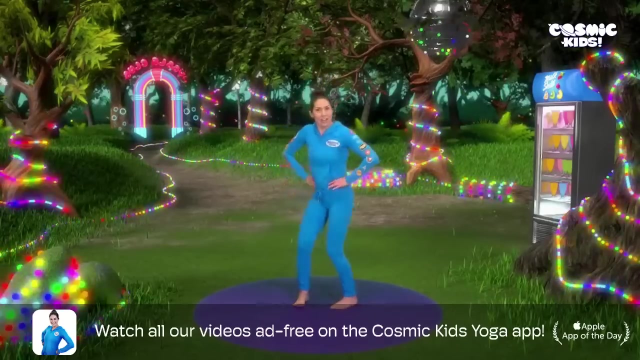 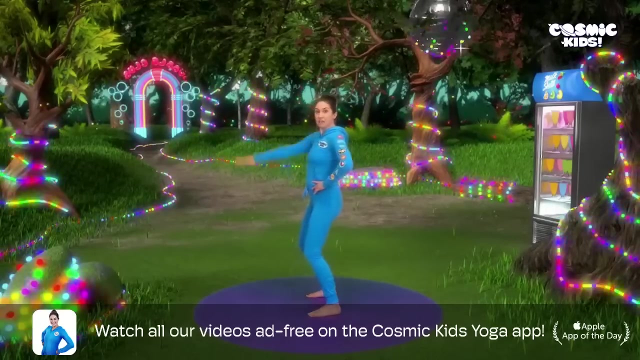 nicodemia begins to dance unlike anyone could ever have imagined. just like a chicken. she puts her hands on her hips and she clucks her wings bye. she digs her head forward and back. she even makes a comb on her head and a little tail feather with her hand. 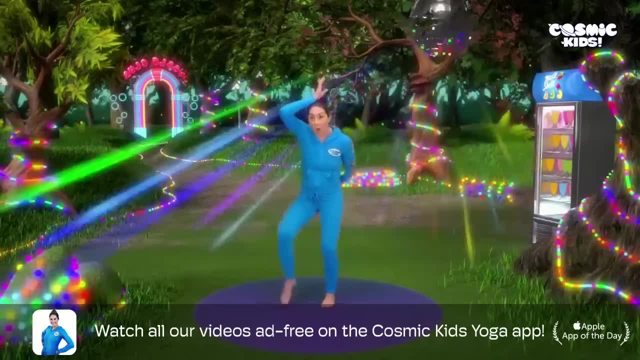 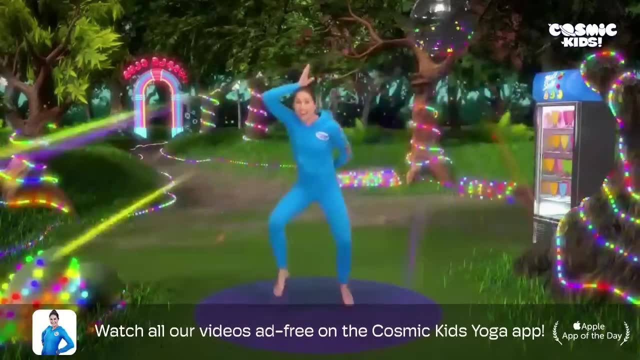 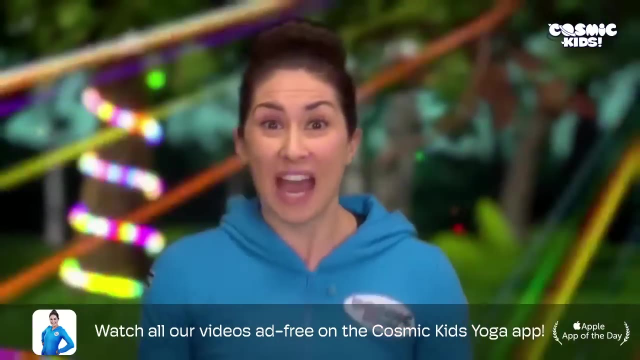 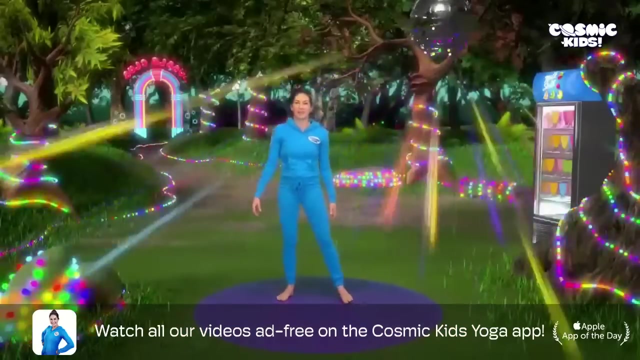 and she kicks her legs up high to the side. nicodemia is having fun. she is loving the dance, and so is everyone else, as we all join in dancing together. as we look around, we take a moment to step back, and we take this moment to lie ourselves all the way. 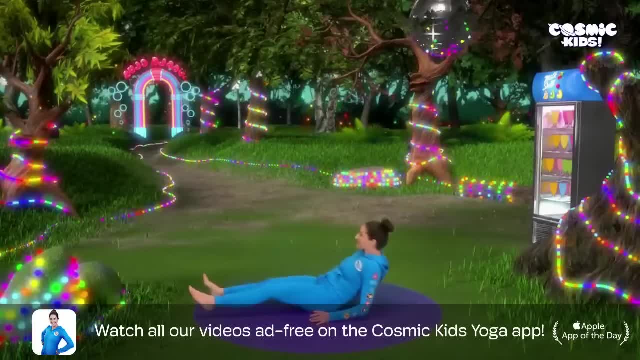 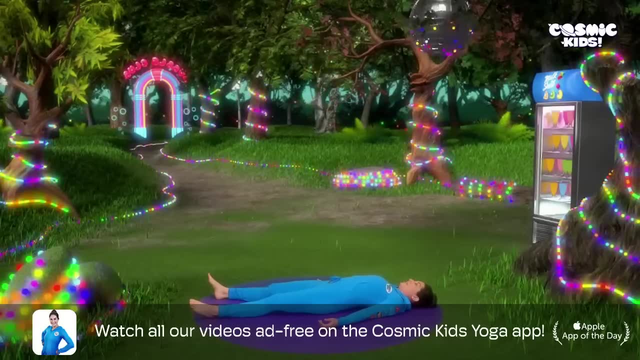 down on the ground, we stretch our legs long and our arms long, and we let our bodies rest, allowing our breath to come back to normal. wow, it's amazing, Isn't it? we've been dancing all morning. Let's take a deep breath, a few breaths, a few breaths. 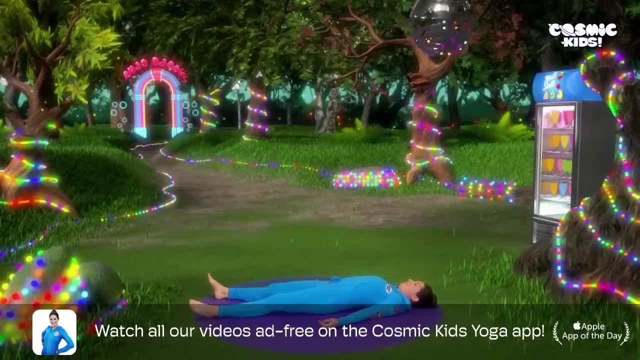 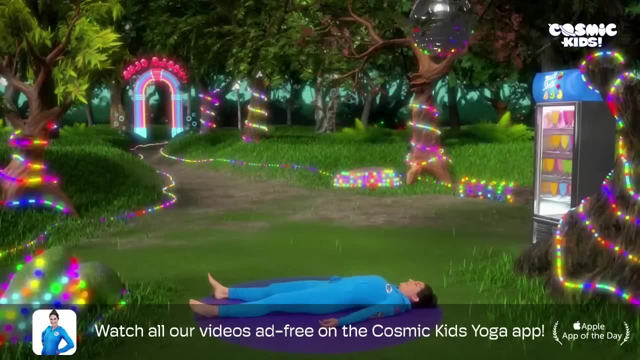 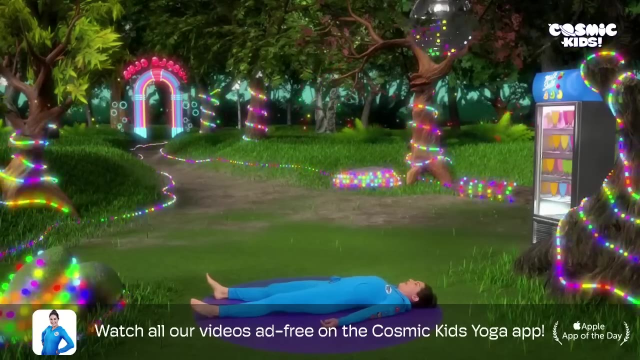 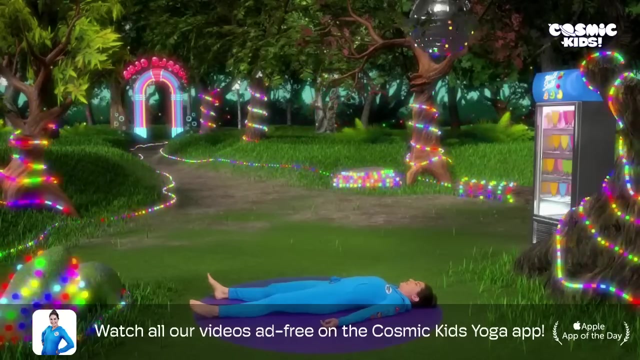 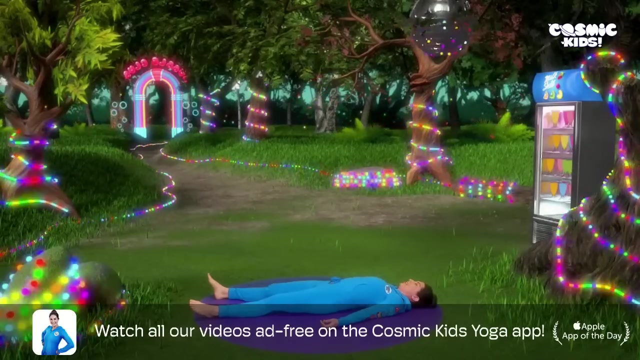 Wow, It's amazing, isn't it amazing, just to notice how you feel in your body after you've been dancing. You feel so alive, so strong, so free. Dancing is like a magic power that can transform the way you feel, Whenever you feel- sad or worried or cold. if you dance, you transform your body, You make 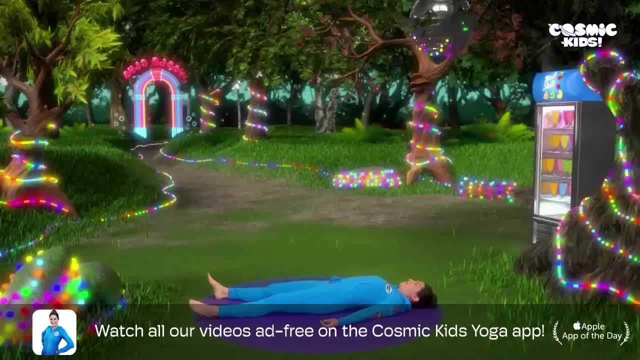 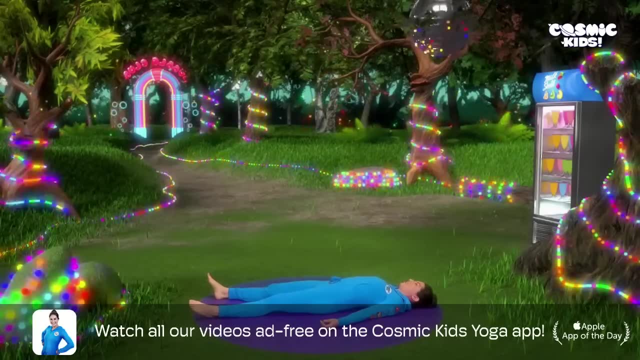 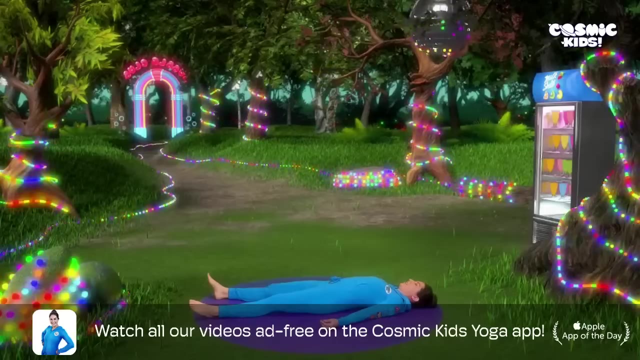 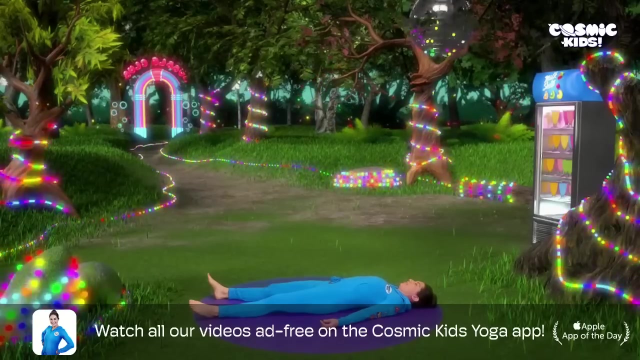 yourself feel good. It's a powerful thing like that, And when we dance together, when we dance with others, something very special happens. We create an amazing bond, a bond of trust, a connection. When we trust those around us enough to dance freely, when we feel that safe, we are stronger. 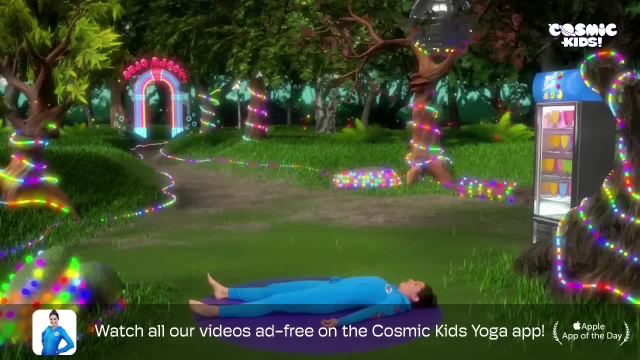 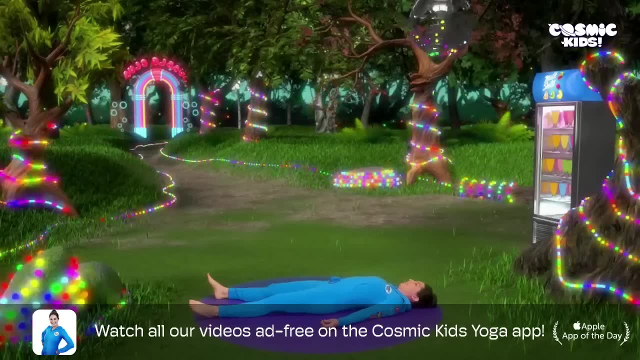 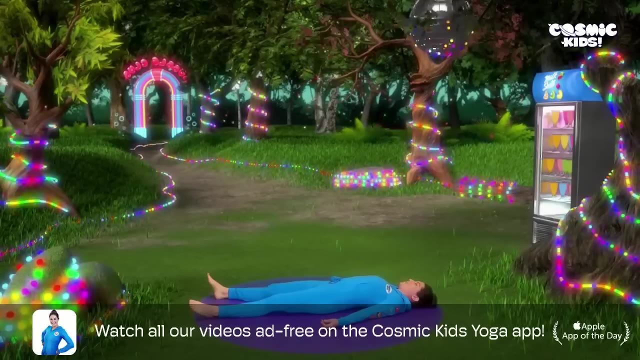 than ever. We are open, we are free, We are able to learn and ready to listen, ready to receive Dance. whenever you can And when you get a moment to share dance with someone else, do it. You will only grow. 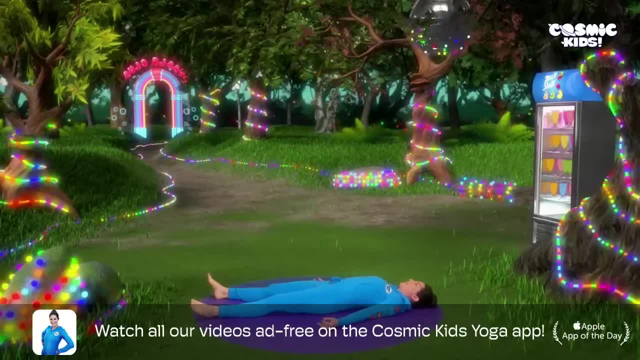 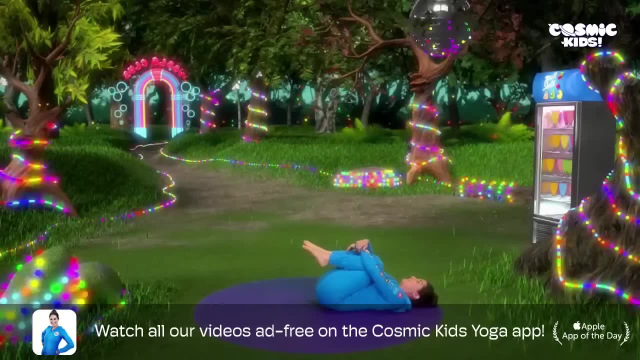 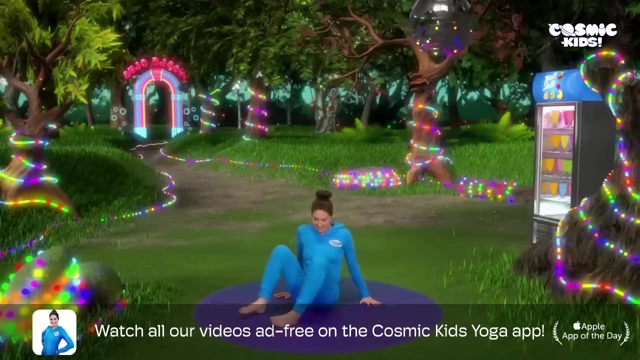 Slowly now we begin to wiggle our fingers and wiggle our toes. We hug our knees into our chest, giving them a nice big squeeze, And then we roll onto our side, opening our eyes, to press ourselves up to sit, We cross our 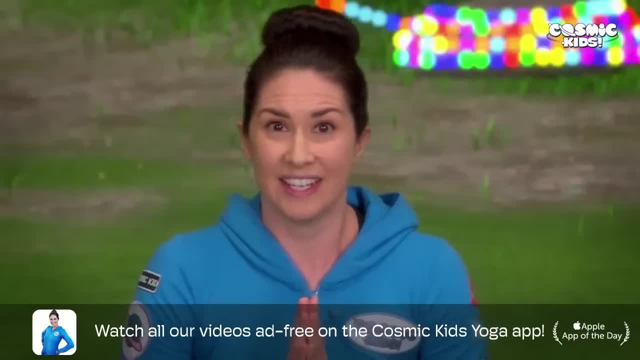 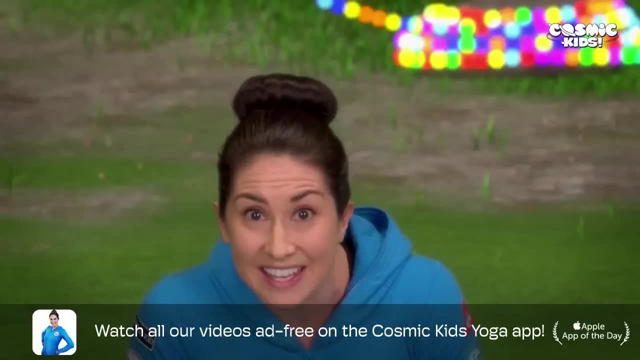 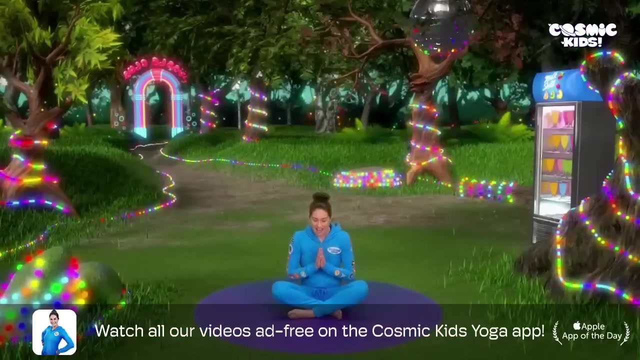 legs and we bring our hands together at our hearts And we finish just the way we started with our secret yoga code: word Namaste, Ready After three. One, two, three, Namaste, Wow, Well done, everyone That was. 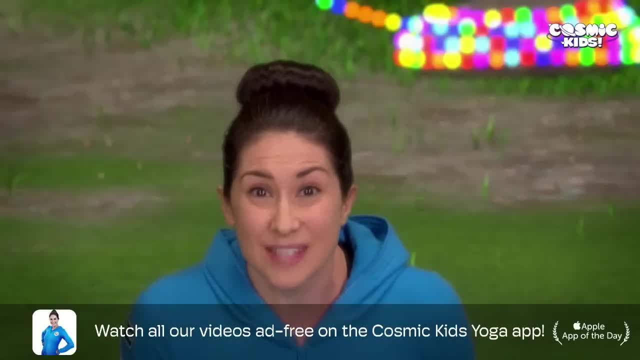 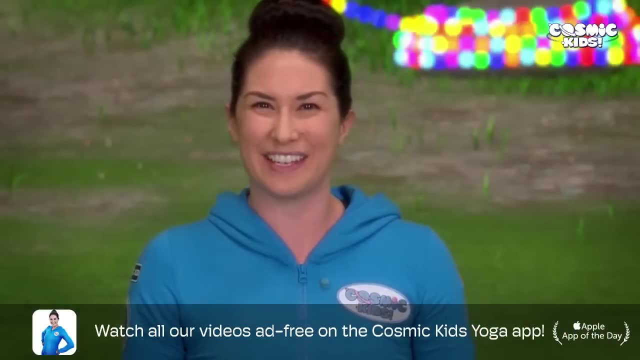 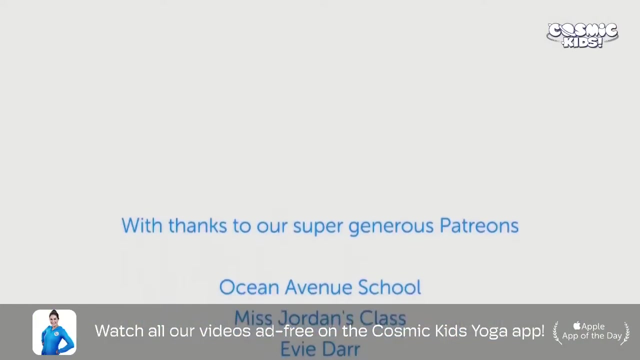 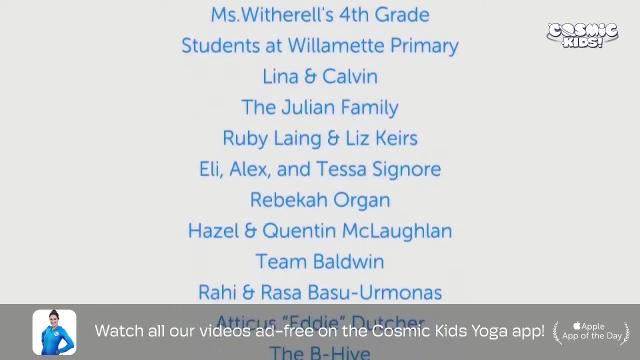 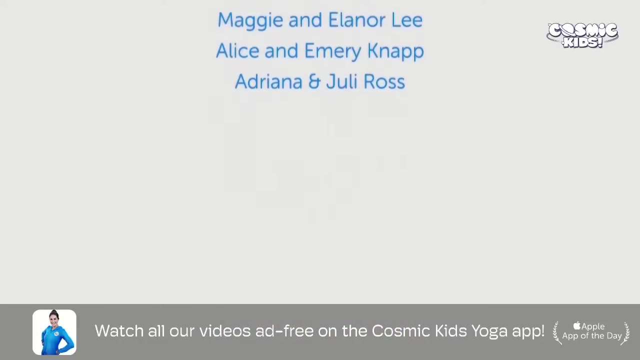 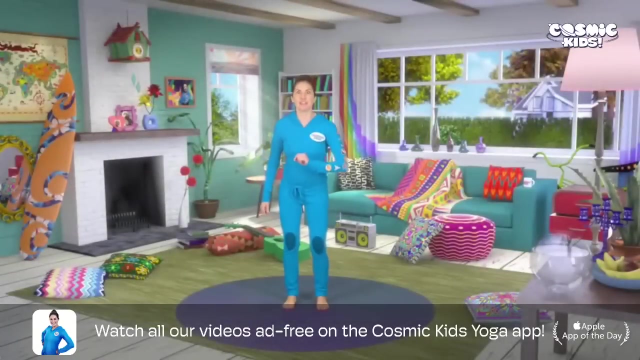 amazing. You were brilliant at dancing. Thank you so so much. I hope you enjoyed the Fairy Floss adventure and I hope to see you again soon for another Cosmic Kids adventure. Bye-bye, Don't forget to join me on Saturday morning for Saturday morning yoga. Get everyone at home. 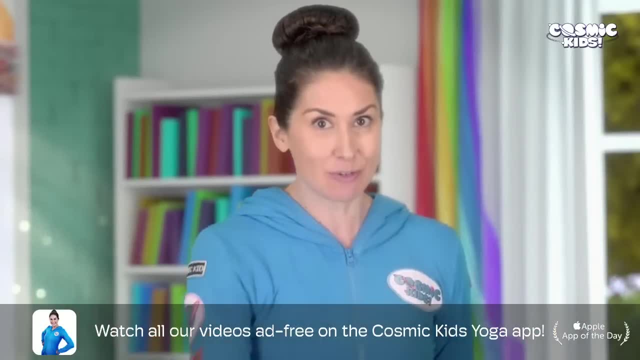 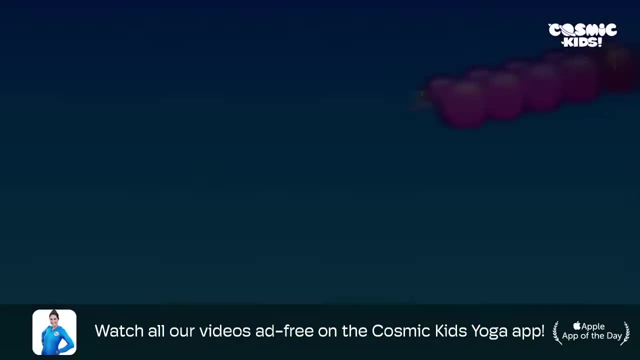 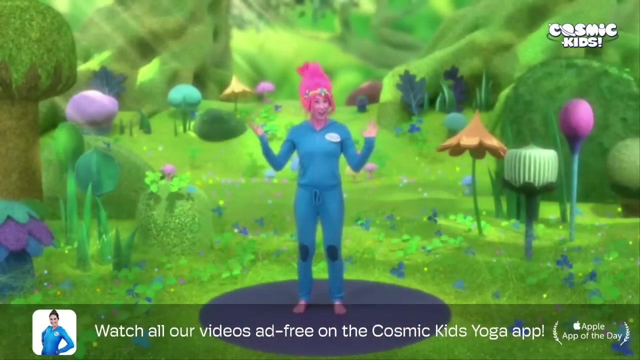 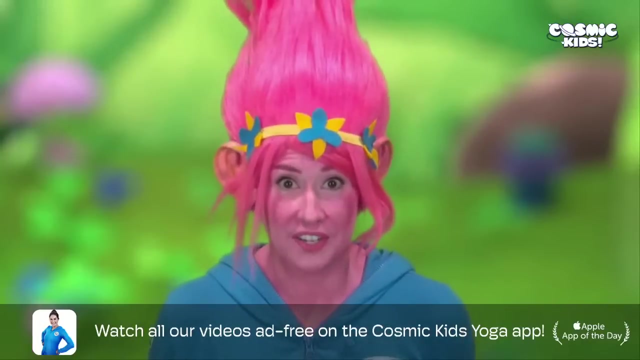 together and enjoy some family time. Remember, subscribe and hit the bell so you never miss one. I'll see you Saturday. Hello everyone, Welcome to Cosmic Kids. I'm Jamie and this is your place for yoga stories and fun. It's easy: Just copy the moves I do and enjoy the adventure. Now we always 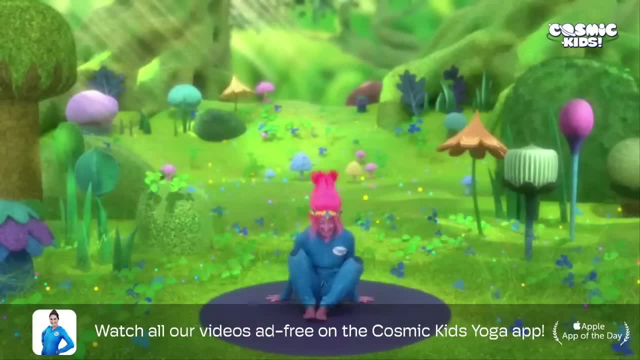 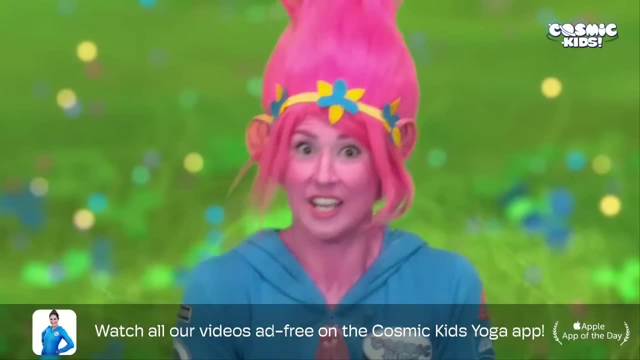 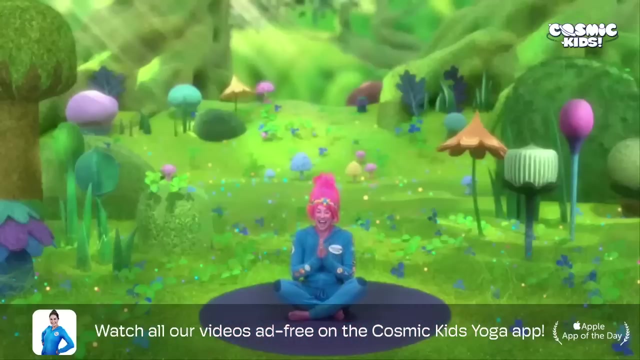 start in the same way, and that's by sitting on our bottoms, crossing our legs And bringing our hands together at our hearts and saying our secret yoga code word, which is namaste Ready After three, One, two, three, Namaste There, Now we're ready to. 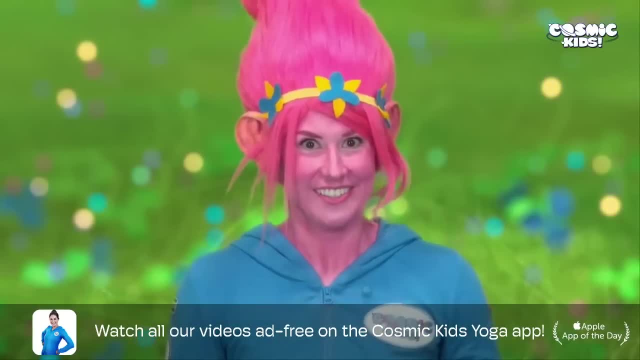 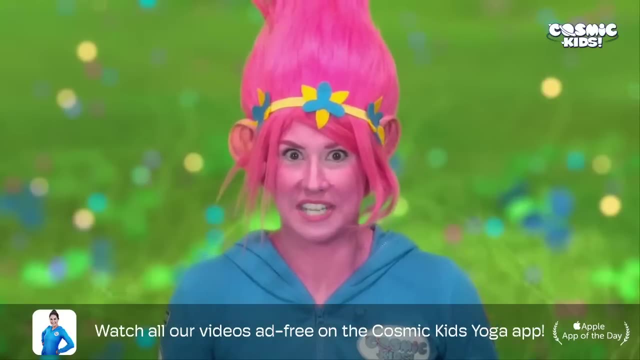 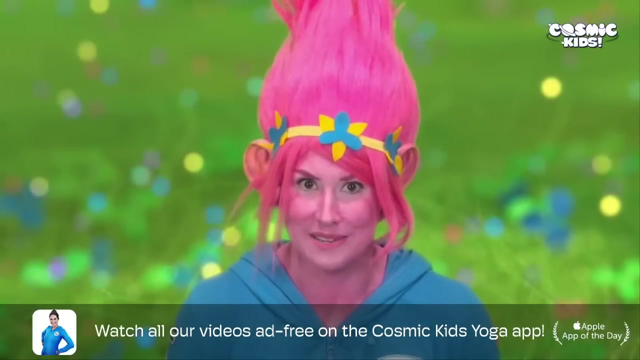 begin, And today we've got a special adventure inspired by the Dreamworks movie Trolls. That's why I've got my pink poppy hair and my pink poppy body. Very exciting. Now our story is. our story begins 20 years ago In the happy forest, in the happy tree. So let's come up. 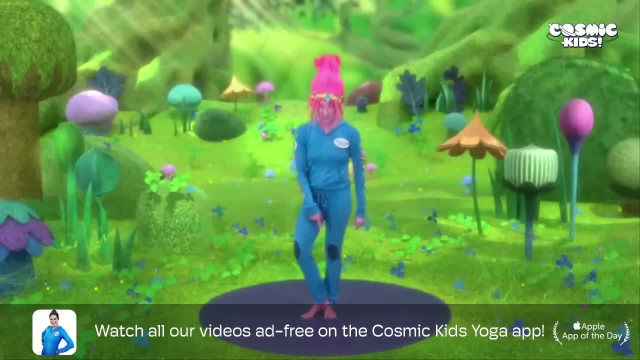 to stand and do our tree pose, Bringing one foot on top of the other, our hands together at our hearts. Let's grow our tree up, nice and tall, and open our branches And let's sparkle our fingers because we're a very happy tree. Yes, Now can we do our tree pose. 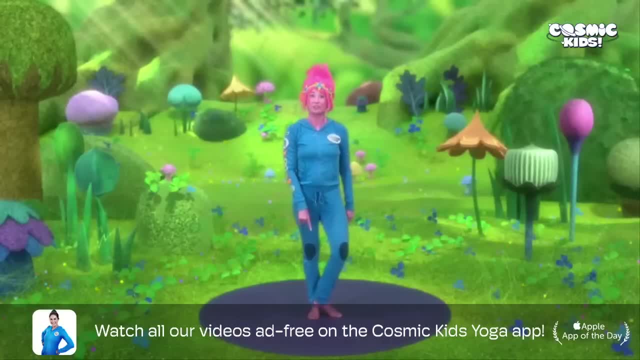 on the other side. Let's try. Bring your other foot on top now using your heel. Bring your hands together at your heart and grow your tree out. All right, Okay, now I'll show you some chair work If we start Say your theme here. for me it's a press when And 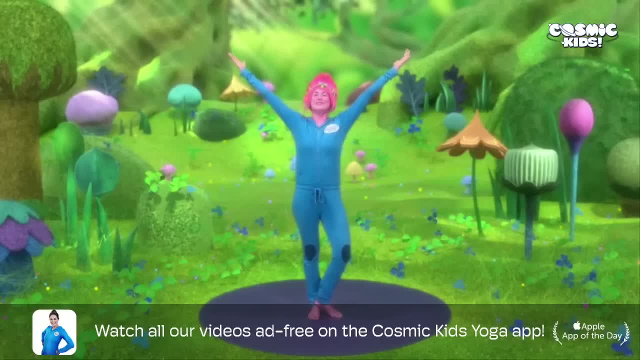 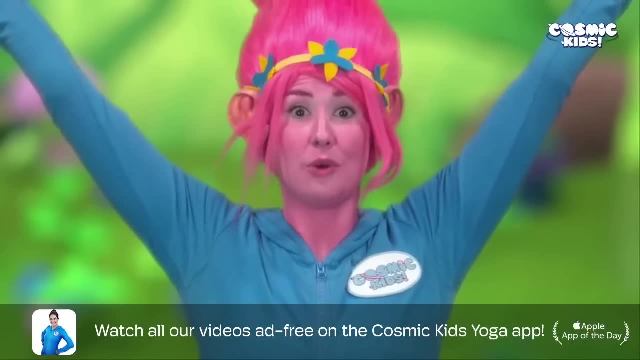 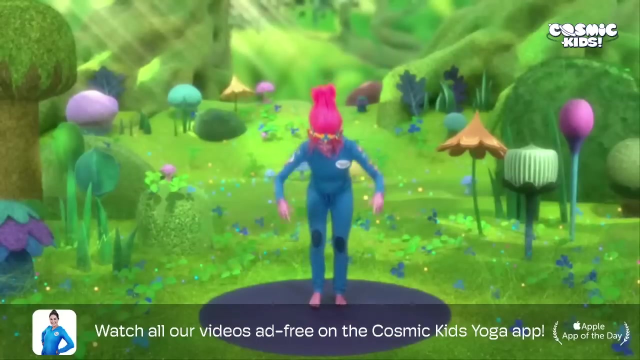 up, nice and tall, opening your branches wide, sparkling your fingers and how about a big smile? yay, we're happy. trees now living in the tree were trolls, tiny creatures with big, colorful hair. let's come into our troll hero pose coming down onto our knees. now take your hands forwards, take. 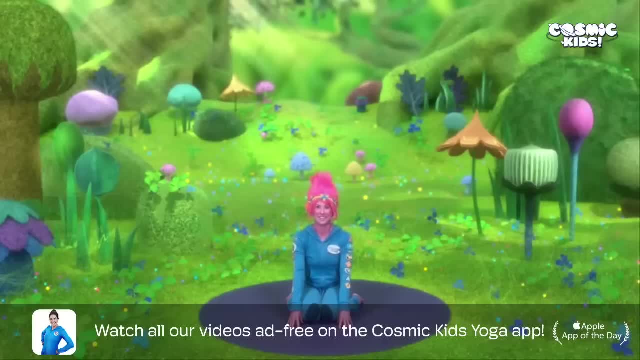 your feet wide and snuggle your bottom down in between your ankles. yes, crisscross your fingers, turn them inside out and lift your arms above your head, coming into your troll hero pose. now, if that's a bit ouchy on your knees, you can lift your bottom, scoop your feet underneath and sit. 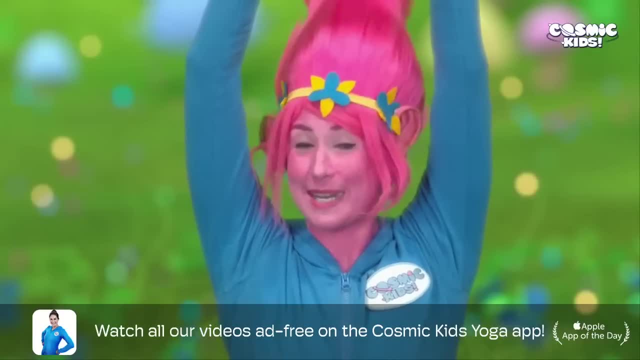 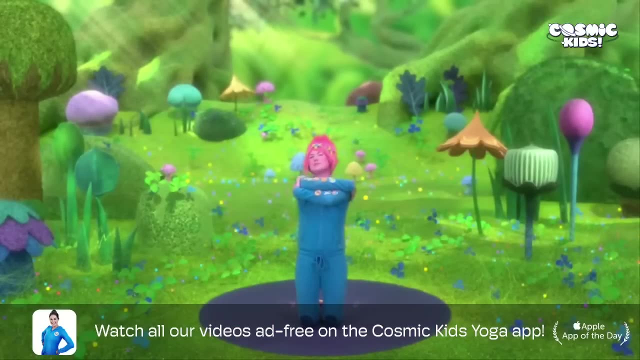 back on your heels. yes now the trolls love to sing, to dance and to hug. let's come up into a hug pose, sitting up tall arms wide. wrap yourself up in a big, beautiful hog. oh, it's wonderful life for the trolls was full of glitter showers. let's come into our glitter shower pose. 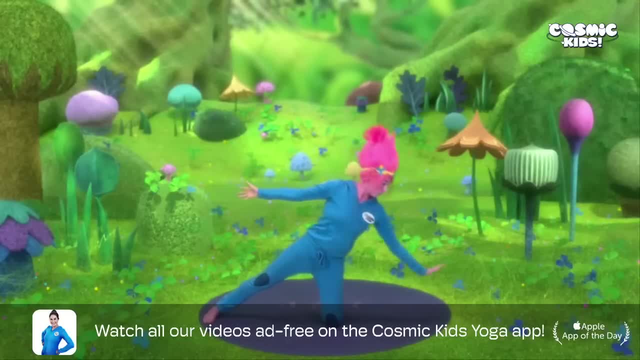 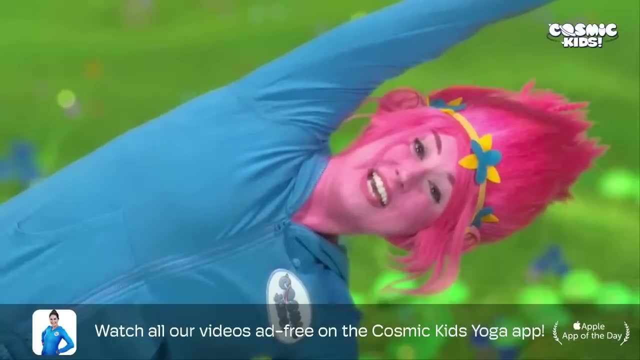 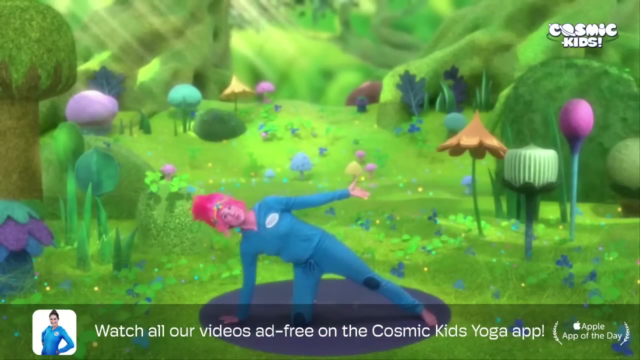 taking your arms wide. take your foot to the side and drop down onto one of your hands and sweep your arm up and over your ear- yes, making a glitter shower appear. it was also full of rainbows. coming back to two knees, arms wide, leg to the side, drop down onto one hand and sweep a big, beautiful. 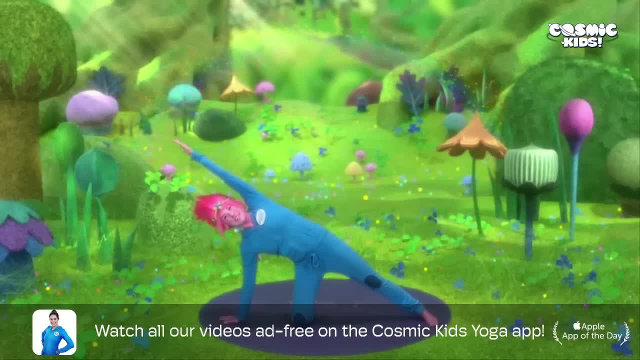 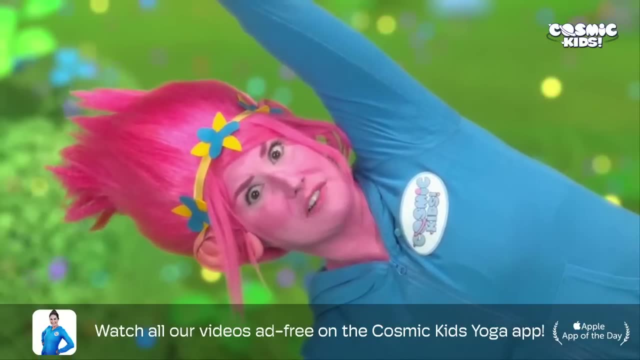 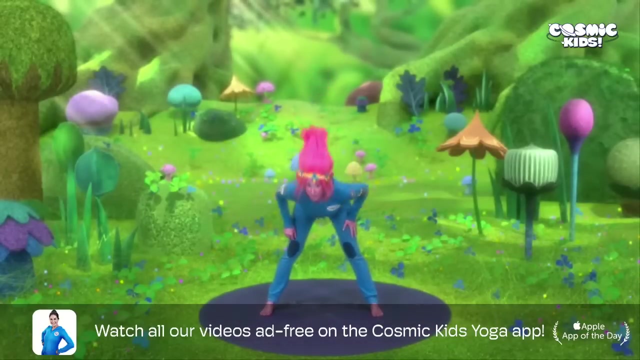 arcing rainbow over your head. wow, how lovely now the bergens were. the exact opposite of the trolls, always feeling sad and clomping heavily around bergentown. coming up to stand in our clompy bergen pose, feet nice and wide, fold your body forwards, holding onto your ankles, and let's clomp. here we go: clomp, clomp, clomp, clomp, clomp, clomp. 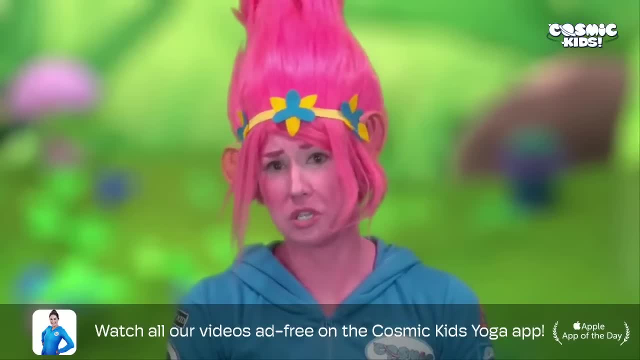 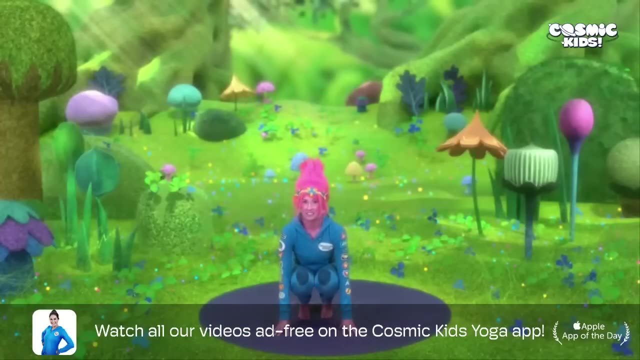 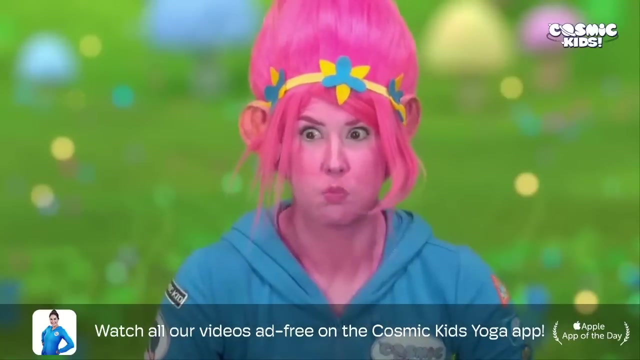 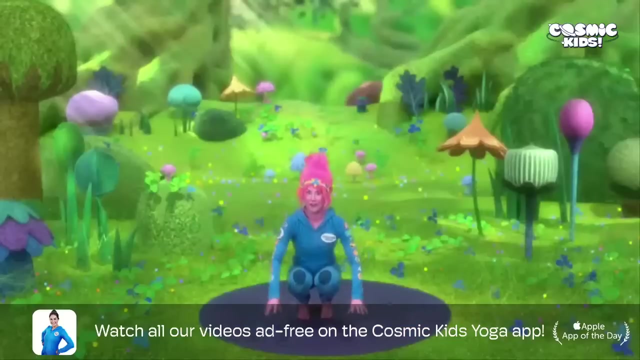 rolling up to stand, oh, to be happy like a troll. that's all they wanted. then one day coming down to crouch fingers to balance a bergen ate a troll if you can balance with your fingers off and gobble a troll. it made him smile and then it made him jump for joy with a big woohoo. 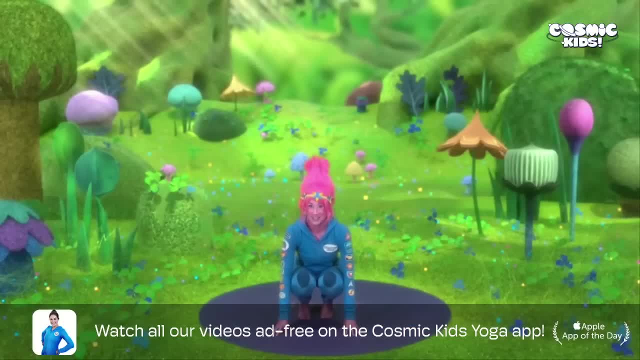 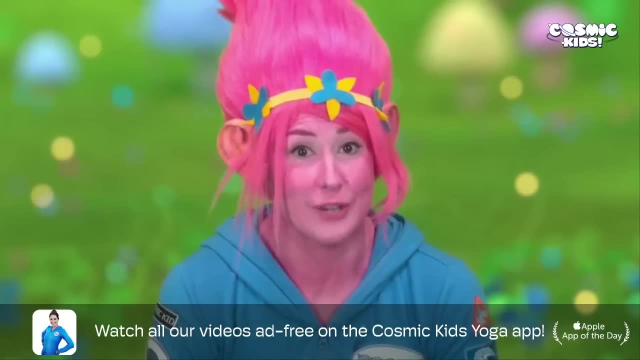 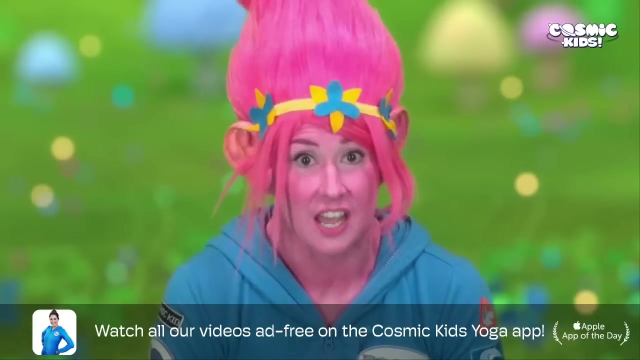 after three, let's do a big woohoo, jump in the air. one, two, three. so this is the secret to happiness: eating trolls. and so they hold a festival each year, trollstice, where they feast on trolls. to be happy for one day. one trollstice, the young bergen prince, prince. 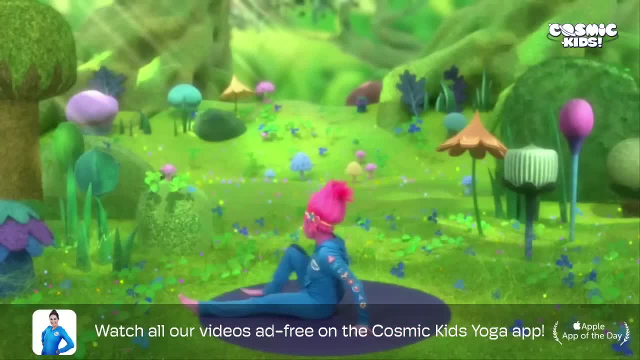 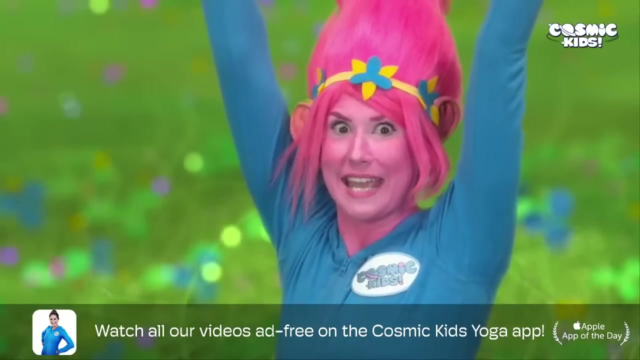 gristle is lying in his bed. coming to lie on our beds, everyone legs out long arms down by our sides and closing our eyes. it was time to wake up, so we open our eyes. he sits all the way up and he stretches excitedly. today is the day he gets to eat his first troll, and no ordinary troll, princess. 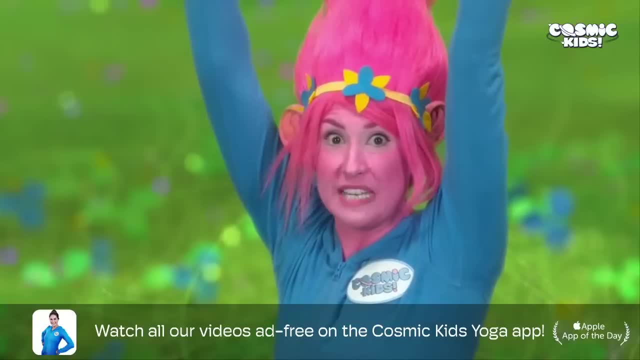 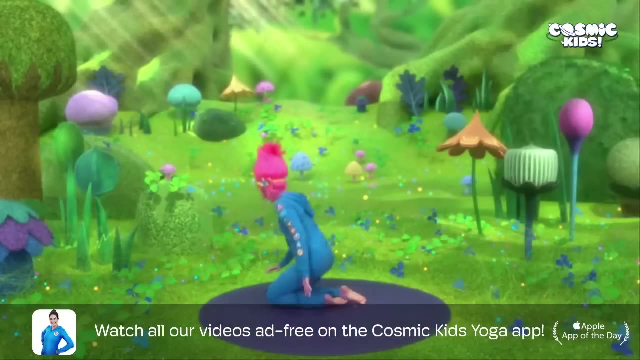 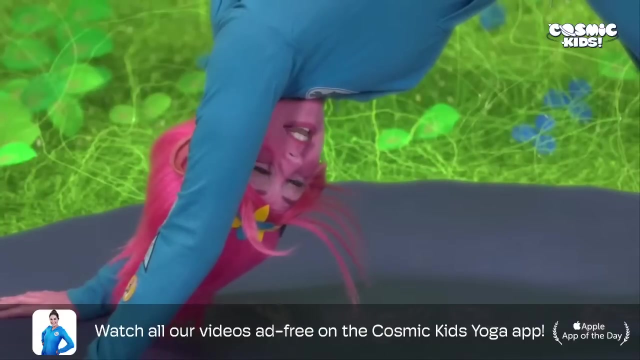 poppy, the special baby troll. but come feast time, all the trolls escape down the secret tunnels, pose onto our hands and our knees, tuck your toes and lift your hips all the way up to the sky. ah, they're escaping, and the bergens reach down after them with their hands, coming onto all fours. 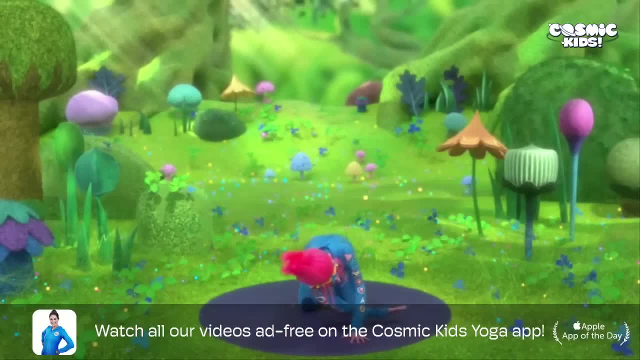 again, everyone. now scoot your hand through the gap between your arm and your leg and see if you can rest on your shoulder reaching for a troll. ah, coming all the way back up. let's do that on the other side. scoot your hand all the way through the gap and reach for a troll, because it's time for 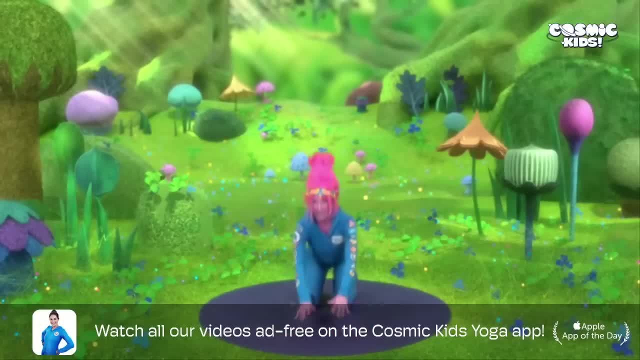 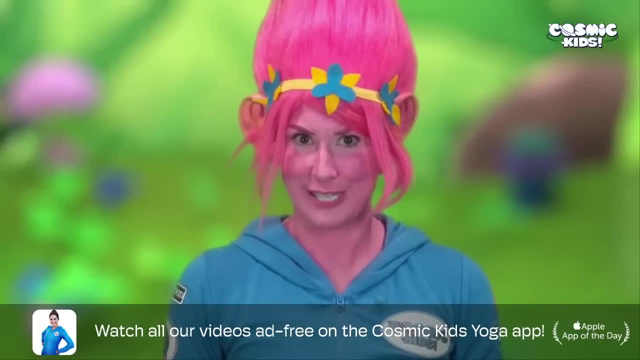 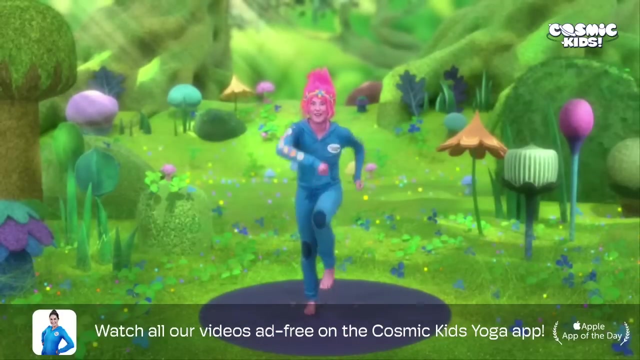 the other way. Nope, they can't get them Coming all the way up to stand. That's because the troll king, King Peppy, marches. his people to safety, Let's march, He chants. No troll left behind, No troll left behind, No troll left behind. Back in the Bergen Palace, the 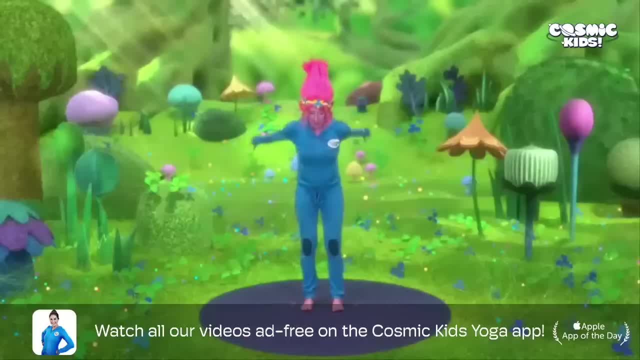 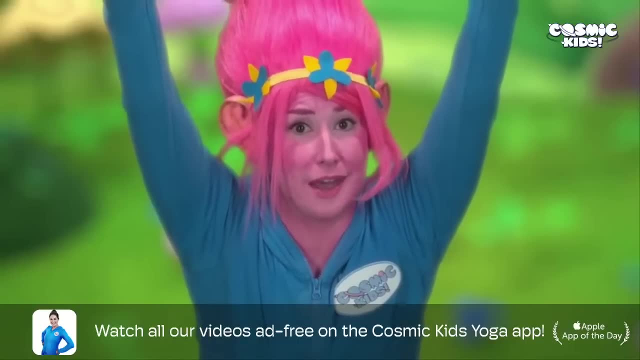 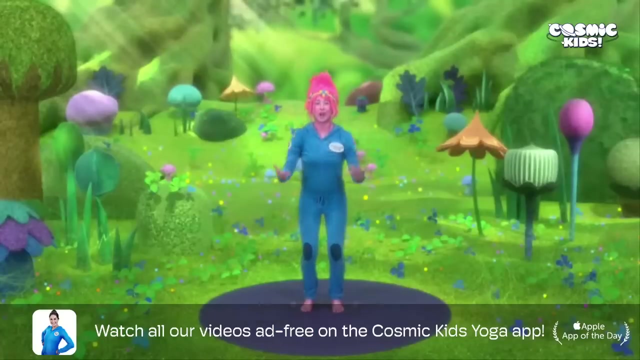 king, King Gristle sits sadly in his throne, Bending your knees, sweeping your arms up either side of your ears. coming into your throne pose, He tells his young son that he will never be happy And he banishes Chef for letting the trolls escape Coming up to 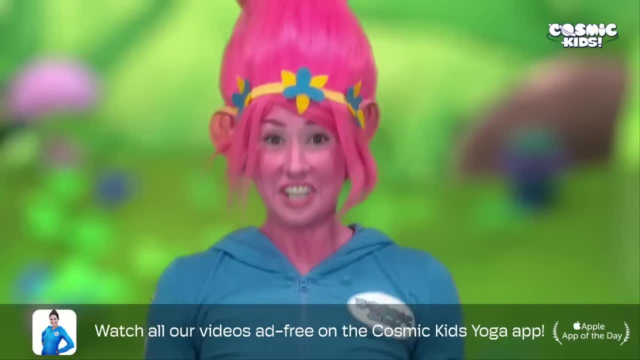 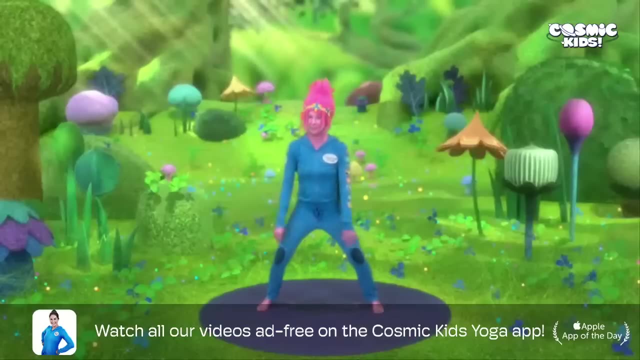 stand. Now, 20 years later, in the new troll kingdom, Princess Poppy decides it's time for a party. Jumping her feet wide, taking her arms wide, she begins the spin And she sings, inviting Everybody: move your hair and feel united. Branch. the grey troll crouches down going. 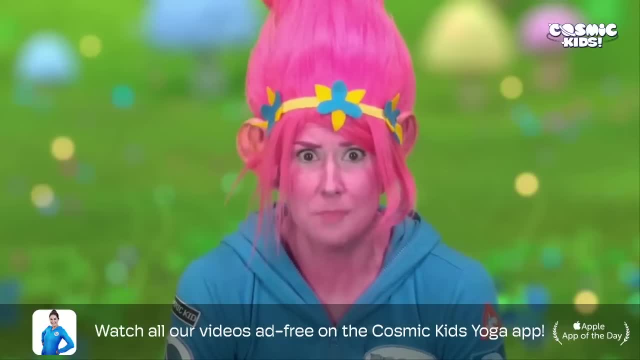 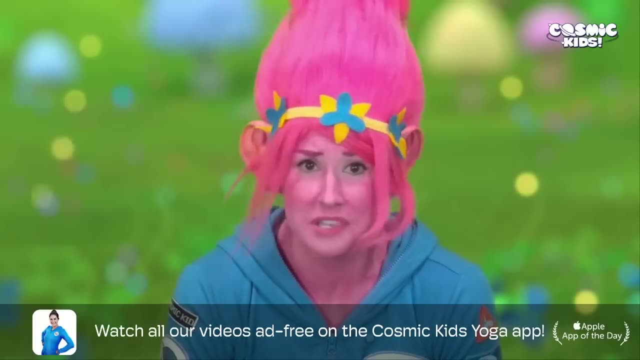 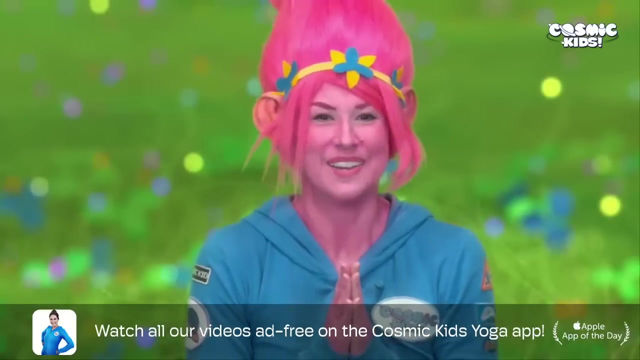 shhh, Too much noise and the Bergens will hear. You'll lead them straight to us. And then Creek, the yogi troll, arrives with a namaste Sitting on your bottoms, crossing your legs. Bring your hands together. After three, let's do a namaste: One, two, three. 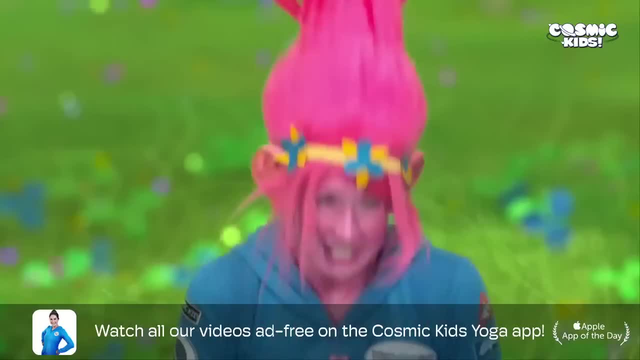 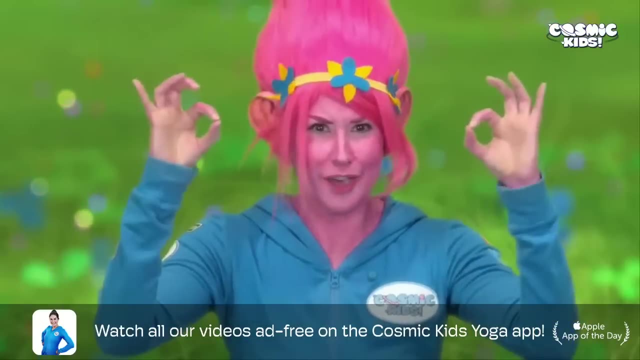 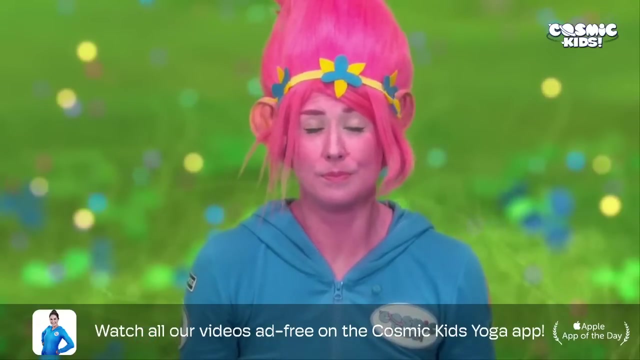 Namasteing. He encourages Branch to channel the positive energy And together we do an om Just to do that, Bringing our thumbs and fingers together, resting them on our knees And let's om, Ommmmmmm, Opening our eyes Bing. 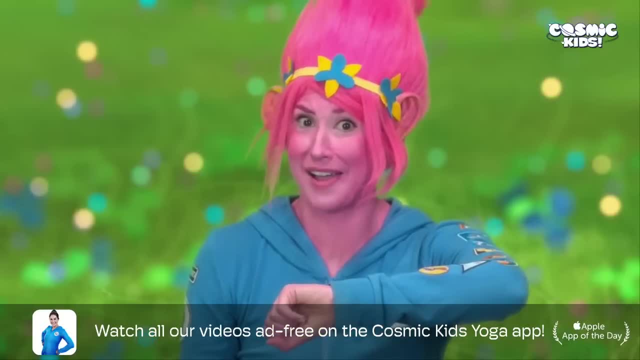 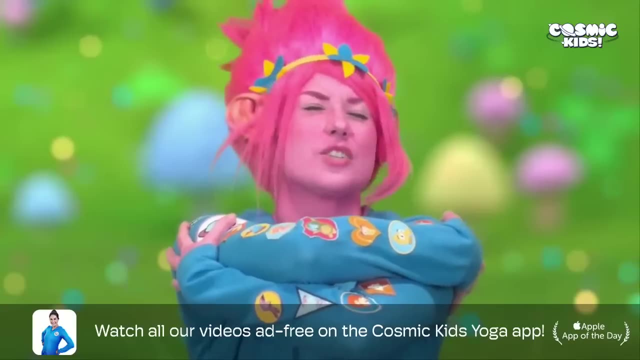 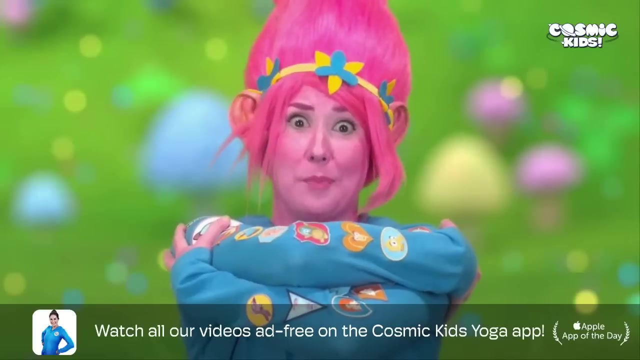 Oh, look at the time- It's hug time- Coming up onto our knees, arms wide, let's hug. Oh, wrap it in. Oh, yes, I could squeeze you forever. Now, despite Branch's warnings, the party happens. There are glitter, cannons popping. 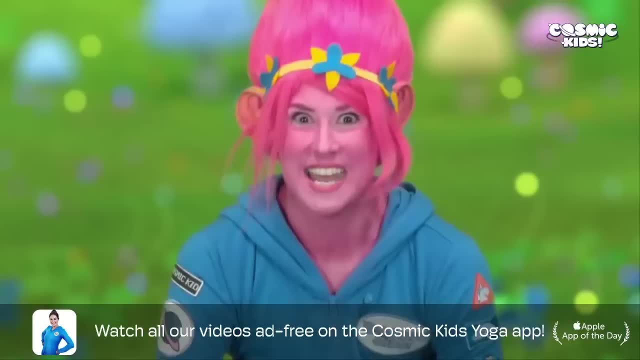 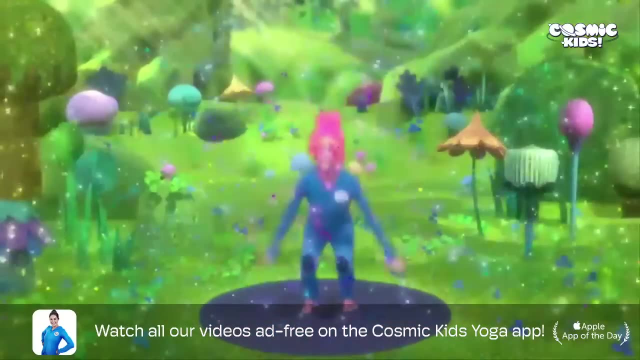 Let's come into our glitter cannon. pose Up onto our tippy toes. Now we're going to jump in the air after three with a big pop of glitter. One, two, three pop, Yay, There's jumping to the music. 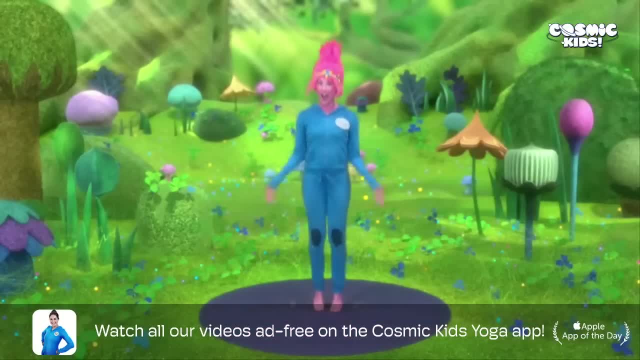 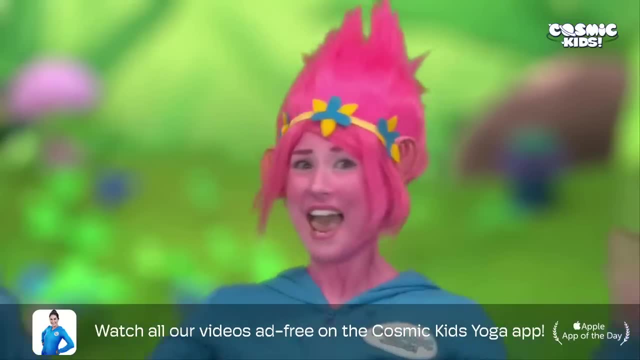 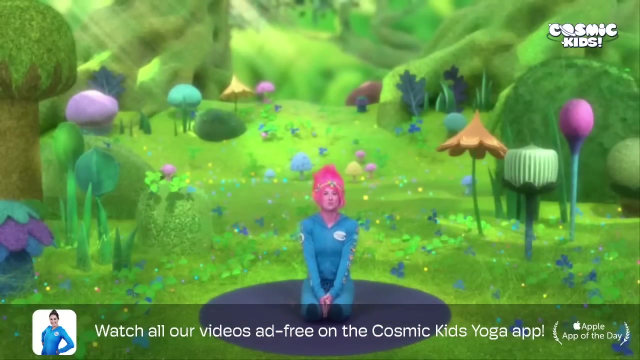 Coming up to stand and let's jump And there are light volcanoes exploding everywhere Coming into volcano. pose Down onto our knees, bringing your hands down in between your knees. We're going to breathe in as we lift up. Here we go. 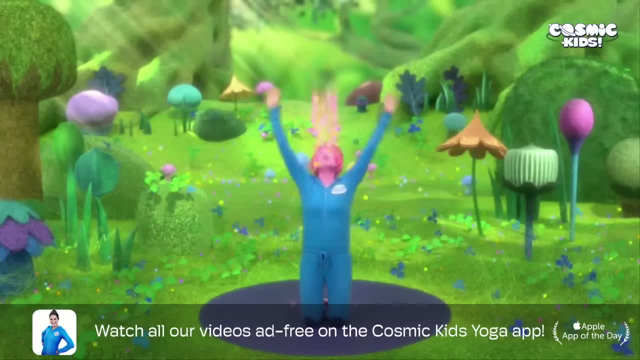 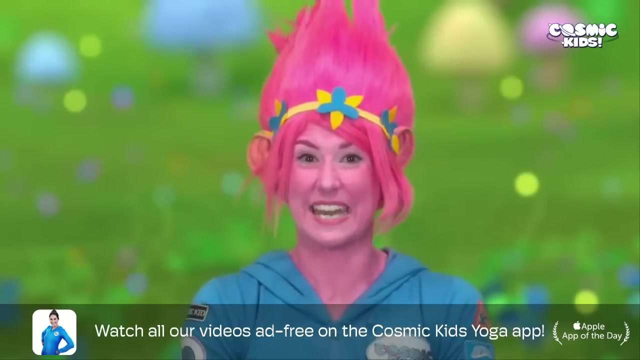 And then we're going to blow a light volcano to the sky, Breathing in, lift up And whoosh a light volcano to the sky. Let's do a few little ones. It's amazing, Wow, it's amazing. It is loud, so loud that the Bergen chef hears them. 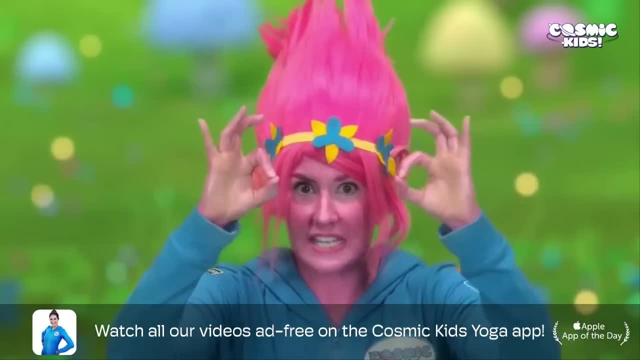 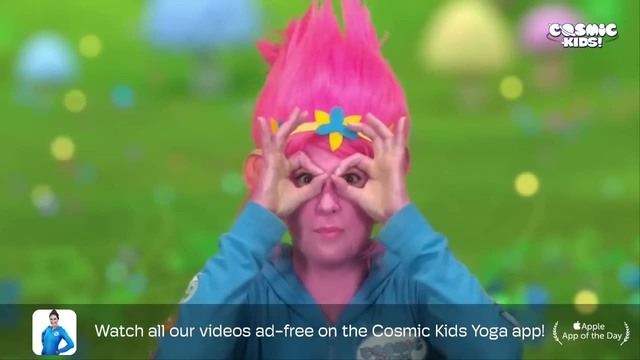 She looks through her cosmonoculars, Joining your thumbs and fingers together. everyone, Have a look through. There they are the trolls. She sees them Lowering her hands. Here she comes, taking big steps, Coming up to stand everyone. 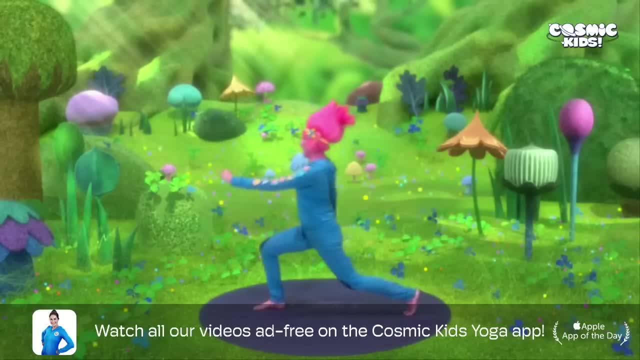 Let's take a big step forwards. Here we go, Big step. she reaches all the way forwards to grab a handful of trolls. Then she steps all the way back to put them in her pouch. Then she steps forward on the other leg, big step. 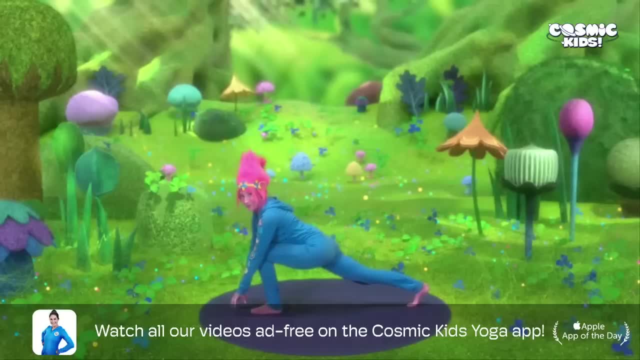 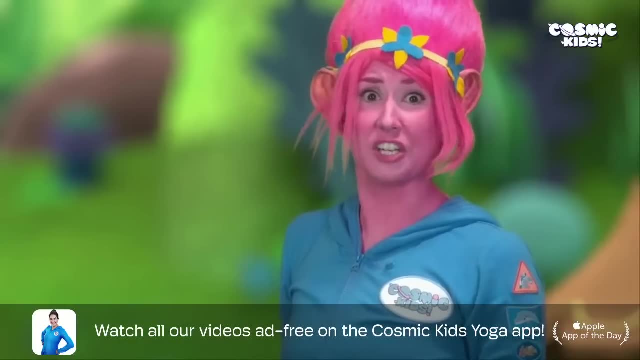 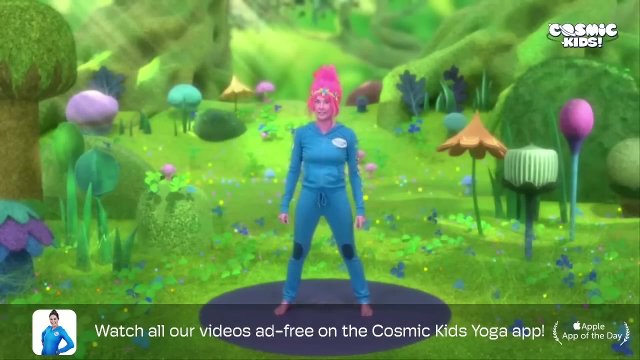 She reaches all the way in to grab those trolls and she steps all the way back to put them in her pouch. Oh no, the trolls run in all directions. Help King Peppy and Poppy hide, coming into hiding, pose Down onto our knees, untuck our toes, folding our heads all the way forwards to be very 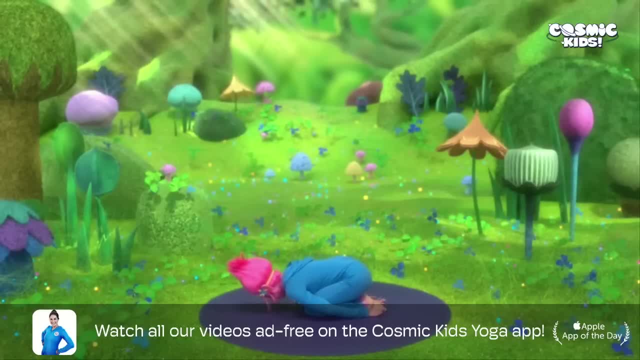 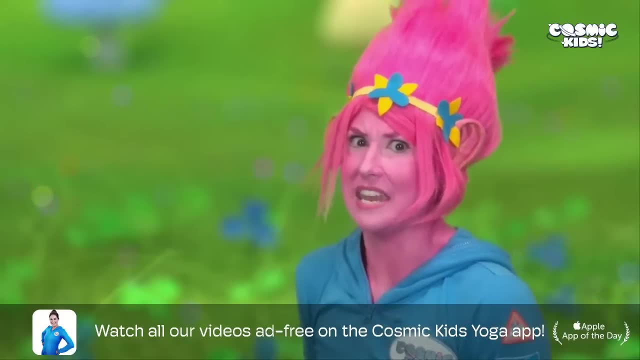 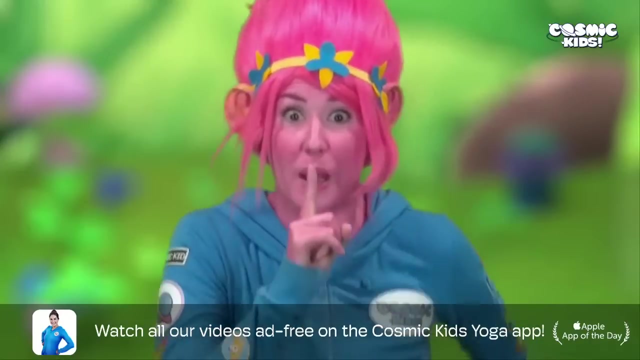 quiet as we hide under our hair. coming up to sit When the coast is clear, Poppy decides she needs to save everyone and she gets up quietly. She tiptoes down To branch the grey troll's bunker. She asks for his help, but he doesn't want to. 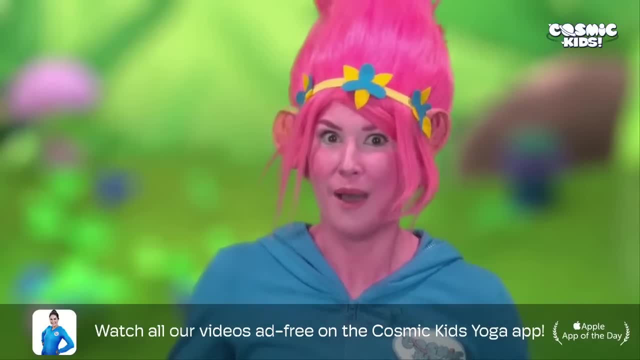 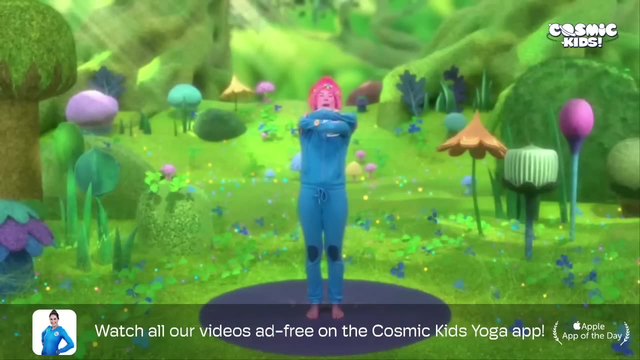 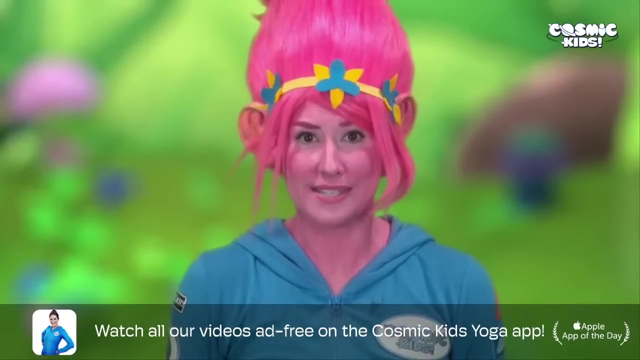 And so Poppy brings all the other trolls down to hide with him. Just in time for ding, hug time. Arms wide, wrap yourself up in that big beautiful troll hug, Luring your arms all the way to the side. And so Poppy sets out on her journey alone. 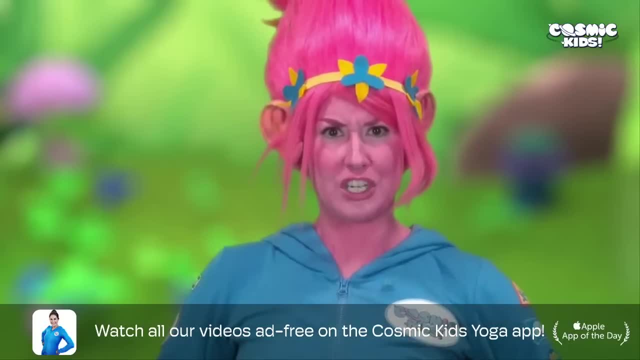 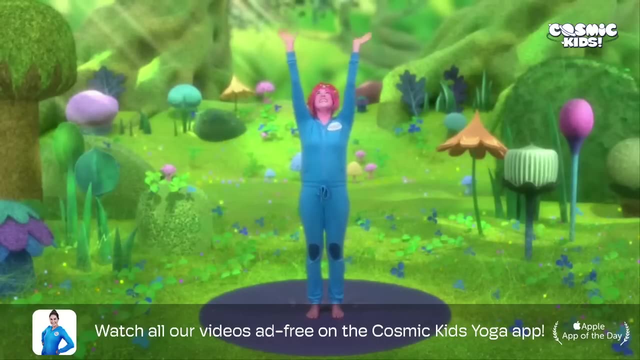 Into the scary forest To feel brave. she sings about the sunshine Reaching up to the sun. give it a wave and say hello sun. She sings about the butterflies coming to sit in butterfly pose, Soles of your feet together, holding onto your feet and fluttering your butterfly wings. 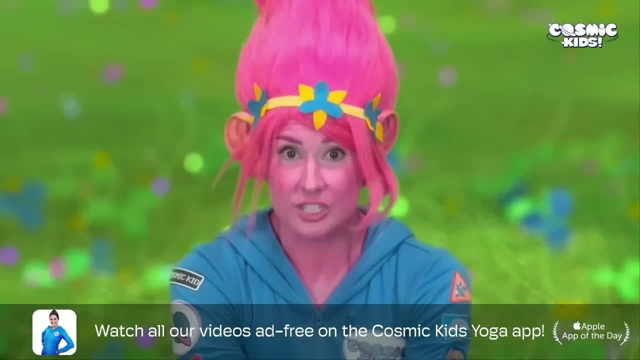 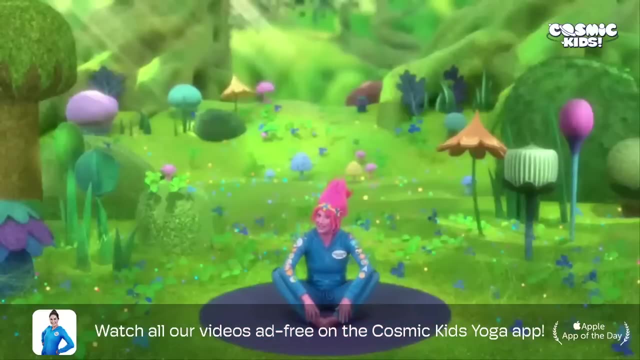 Yes, lovely, Even getting soaked by the rain, Using your fingers to pitter, patter your head and your face all the way round. Maybe your legs, yes, And she gets chased by the wiggly wormy monsters Coming into our wiggly wormy monster pose. 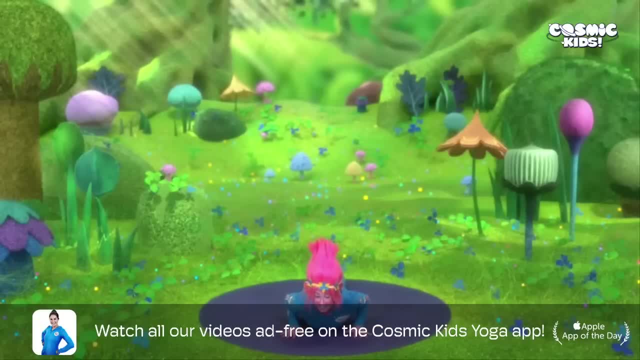 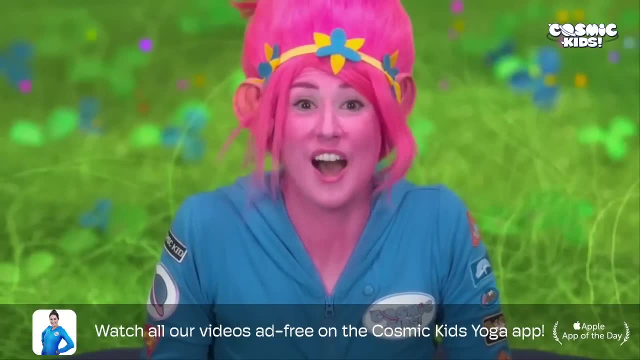 Onto our tummies. everyone Hands underneath your shoulders Now wiggle, wiggle, wiggle, wiggle all the way up, Making yourself into a wiggly wormy monster. She sings: I'm not giving up today. 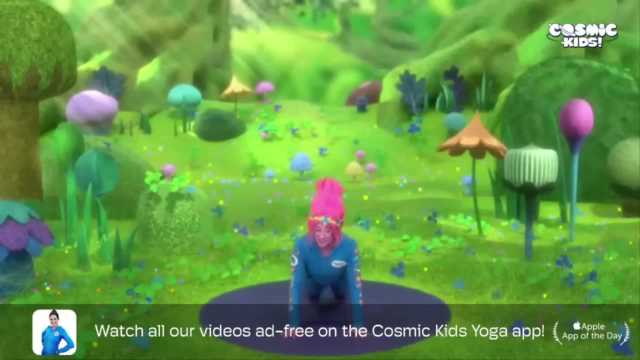 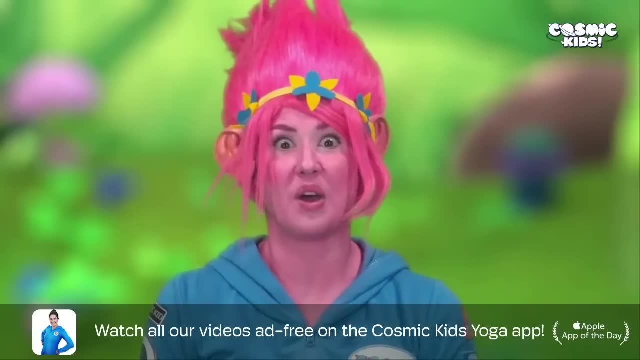 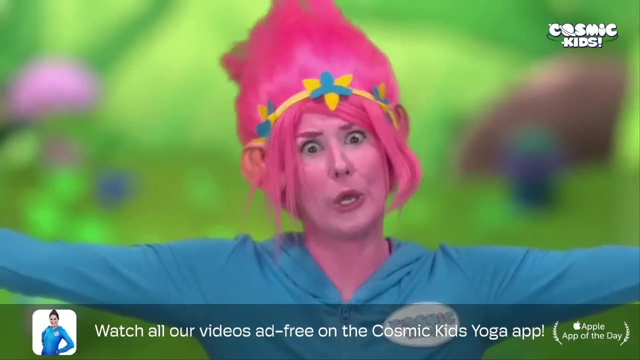 And about getting up again, Tucking your toes up onto all fours, Walking your feet forwards and rolling up to stand. Then comes the spider's web: Jump your feet wide, take your arms wide, Oh no, she gets wrapped up in a sticky cocoon. 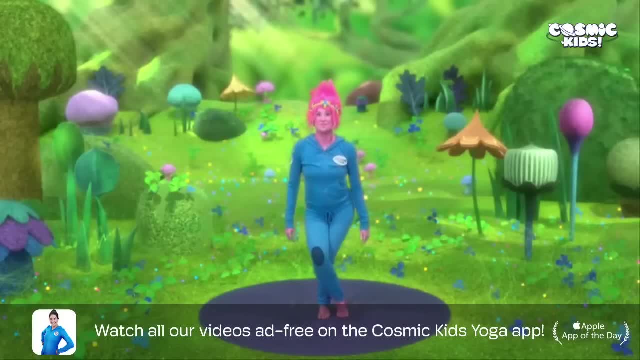 Bringing your feet together now, crossing one leg over the other and bending your knees Arms wide. scissor your arms Wave with your underneath arm and twizzle them round, Sitting yourself down a little bit lower. Oh no, she's in a real sticky cocoon. 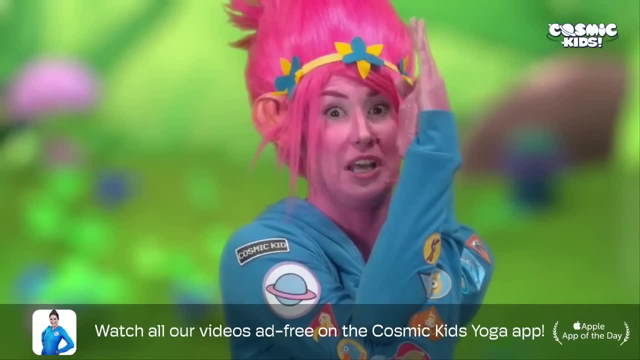 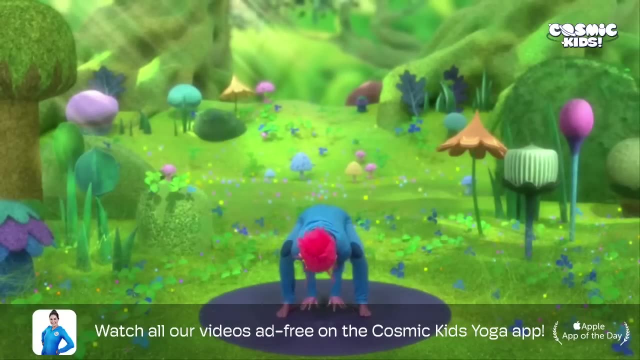 And here come the spiders scuttling along to gobble her up, Taking your feet wide, coming into spider pose, Bending your knees, hands going between your feet. Now ticker, ticker, ticker your fingers round the back to the outsides of your feet. 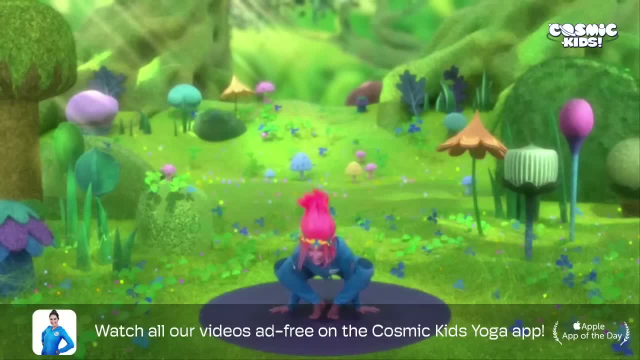 And walk your feet all the way in Coming into your spider pose. Oh no, but just in the nick of time, Who should appear but Branch the grey troll Using his hair like a warrior to shoo them away, Coming up to stand into our warrior pose. 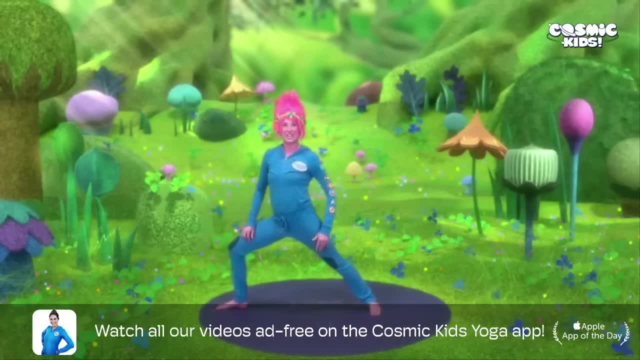 One foot forward, one foot back. Bend your knee, sweep your arms up high And open them wide. Let's shoo those spiders. Shoo And jump the other way. Shoo Branch has decided he will help Poppy. 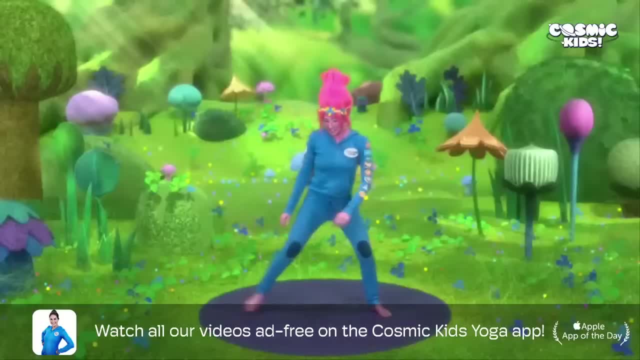 Together. that night they make a campfire, Sitting on our bottoms with our legs crossed, Bringing our elbows forward and wiggling our fingers like they're the flames of the fire Crackling away. It's time to go to sleep, And so Branch and Poppy lie down. 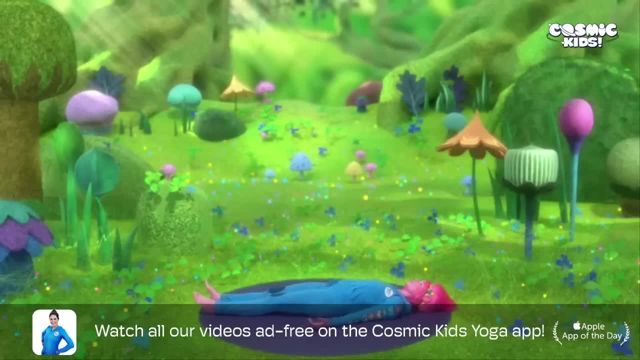 Lying down with your legs long and your arms down by your sides. Poppy can't really get to sleep, And she looks up at the starlit sky. She sings, Stars shining bright above me. Branch rolls over, Taking your arms wide. 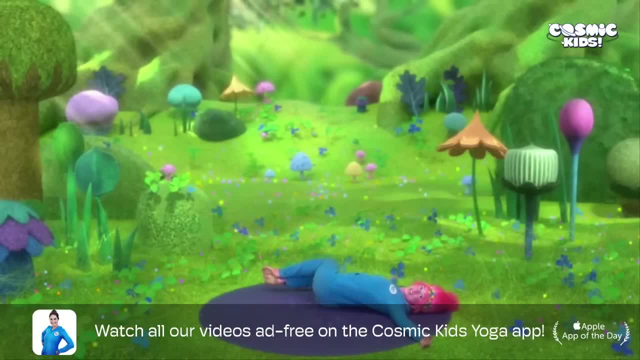 Bringing up your knees, Taking them over one way And your head over to the other. He looks at Poppy and he goes Shoo. Then he rolls over the other side, Lifting up your knees, Going to the other side and your head to the other side. 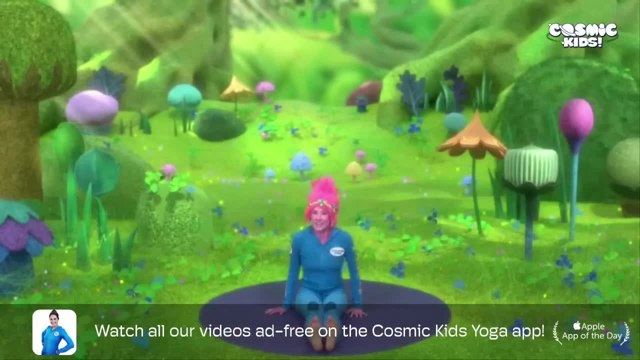 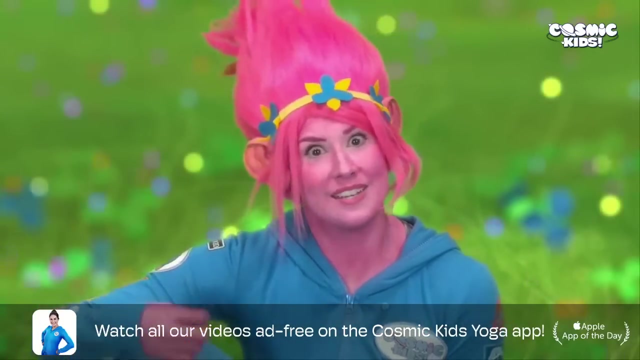 Poppy sits up And she takes out a ukulele, Taking hold of your foot, Bringing it to your body And strumming it like a ukulele. She begins to sing to Branch: Hello, darkness, my old friend Branch sits up. 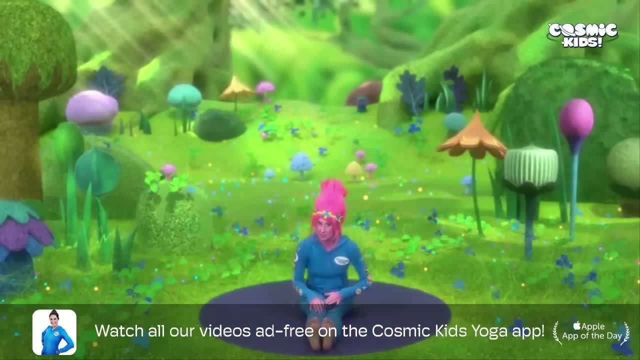 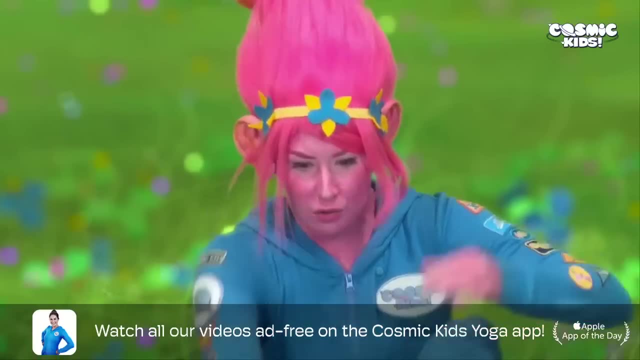 Poppy puts the ukulele down, Branch picks the ukulele up, Picking up the other foot, And he's going to play it, But before he does He throws it on the fire. Oh, Now, the next day they arrive at the secret tunnels. 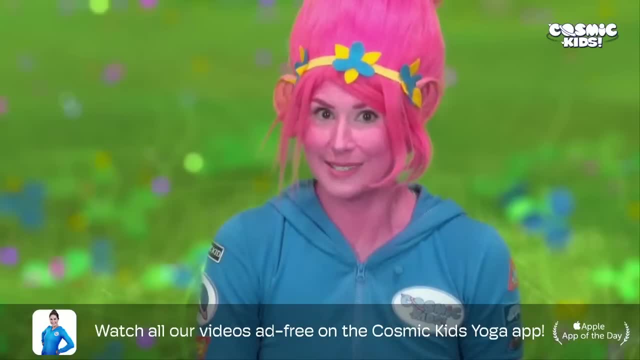 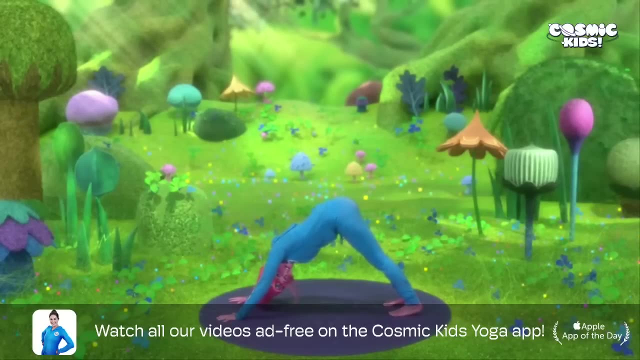 Which take them down to Burgantown. Let's come into our secret tunnel, pose Onto our hands and our knees, Tuck your toes and lift your bottoms to the sky. There are so many holes to choose from. Which one will lead them there? 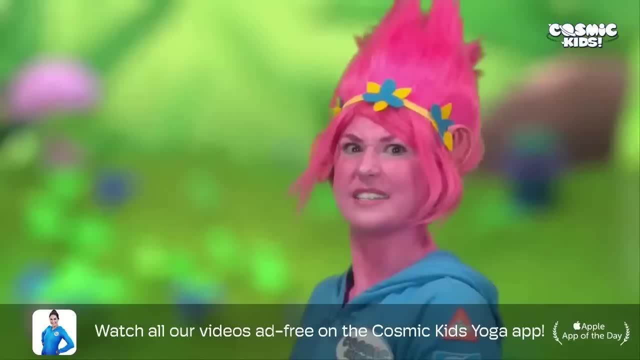 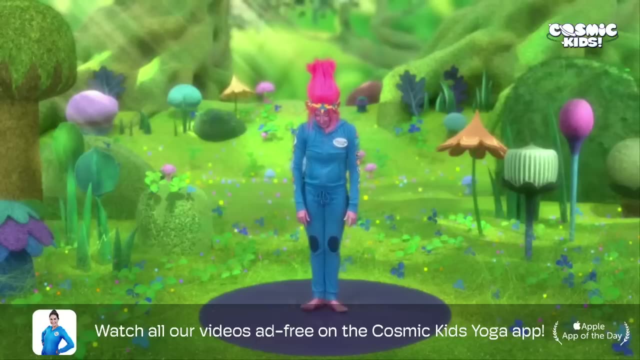 Walking your feet all the way forwards, Rolling up to stand, And then Cloud Guy arrives. Coming into Cloud Guy pose, Bringing your feet together And turning your toes out to make them a V shape, Cupping your hands around your mouth. And we're going to do a big blow. 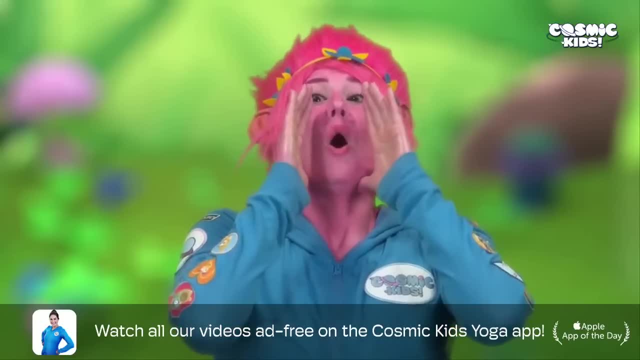 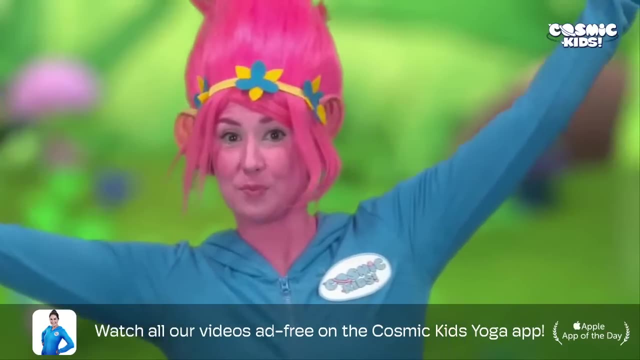 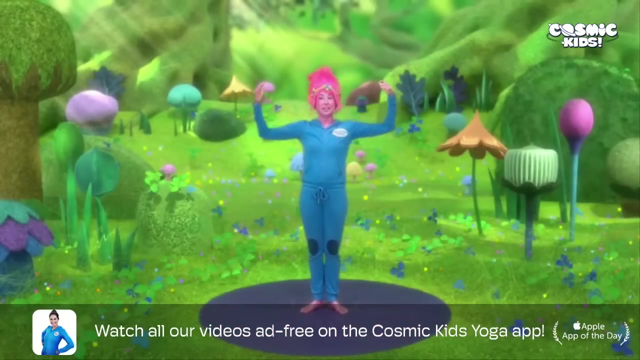 To blow up a big puffy, fluffy cloud. Here we go. Cloud Guy tells Poppy and Branch That one of the holes will lead to Burgantown, The other hole will lead to certain death. And then he opens his arms wide. 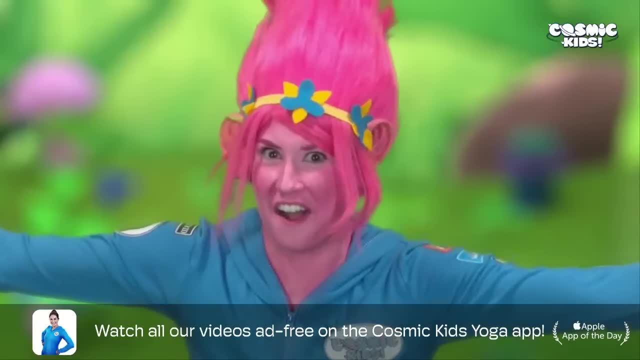 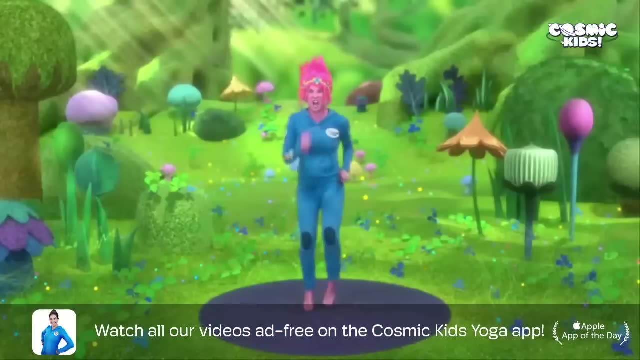 And he invites little Branchy Wanchy in for a huggy wuggy. Branch has had enough of hugging And he chases after Cloud Guy Come back. He dives down one of the holes after him, Reaching your arms all the way up. 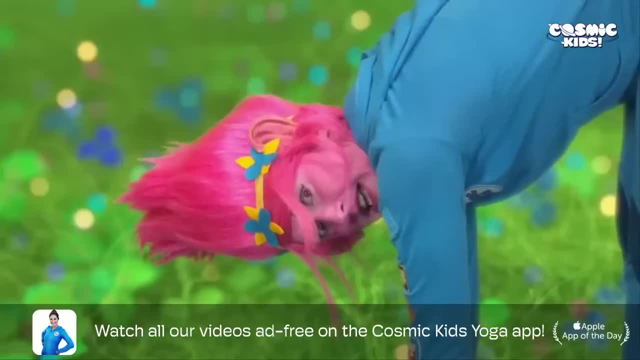 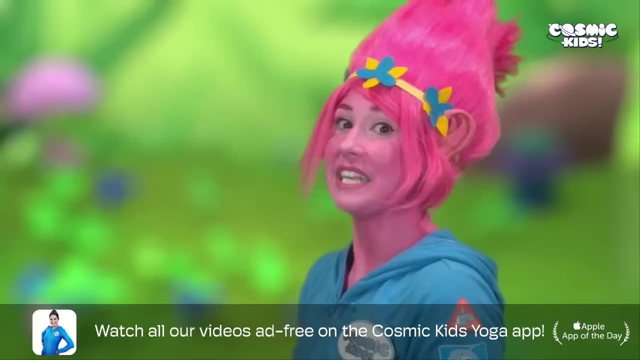 And folding all the way forwards, Following Cloud Guy down the hole. Luckily it leads them to Burgantown, Rolling all the way up to stand Now sitting in the palace is the young Burgon King, King Gristle, Coming into throne pose. 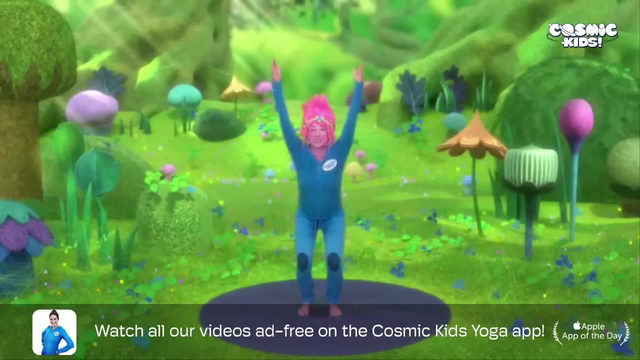 Feet hip distance. Bend your knees, Sweep your arms up by your ears And sit yourself down like you're sitting on a throne. He's with his pet crocodile Barnabus, Coming into crocodile pose, Lying on our sides, Arms long above our heads. 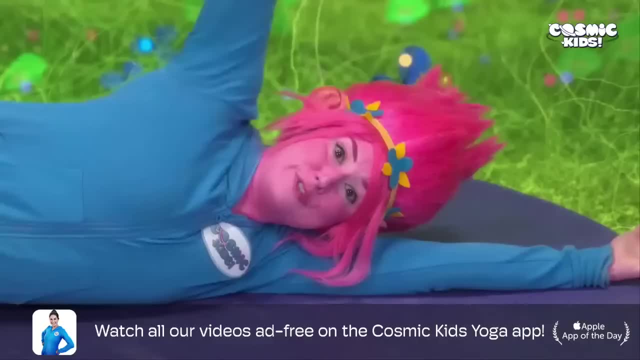 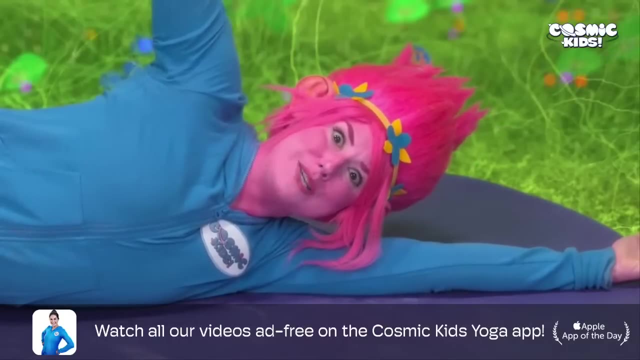 And then opening and closing your jaws By lifting and lowering your arms. Very good, everyone In comes. Chef, Looking very proud and pleased with herself Coming up to stand, She puts her hands on her hips And she tells King Gristle: 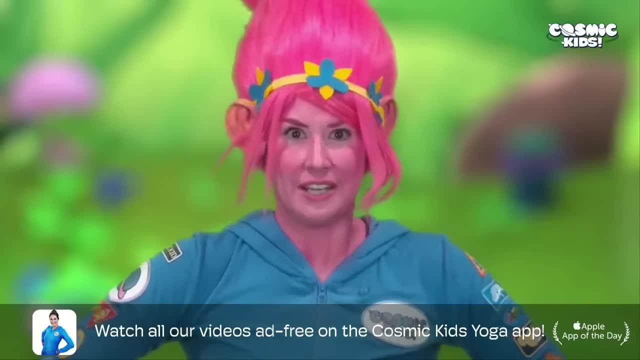 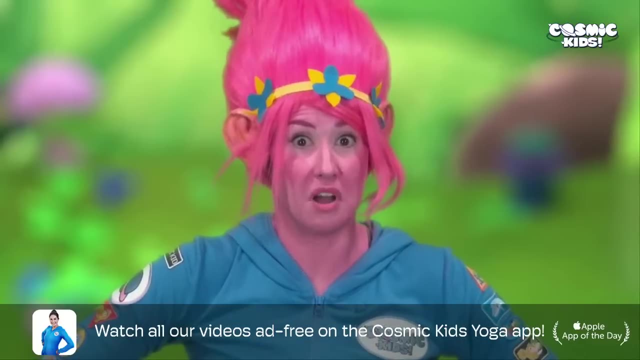 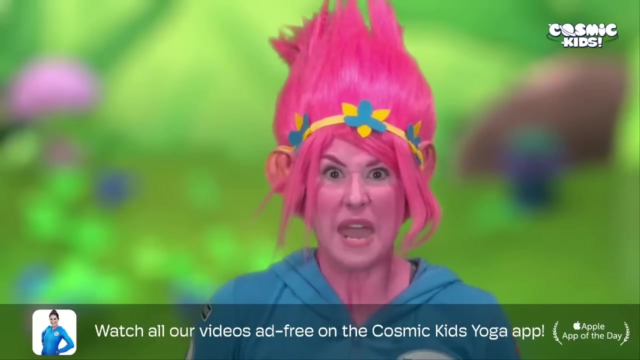 That she has captured the trolls And it is time for trollstice again. Just at that moment, Poppy and Branch tiptoe into the palace, Just in time, Just in time to see Chef Making a sandwich wrap Out of their friend. 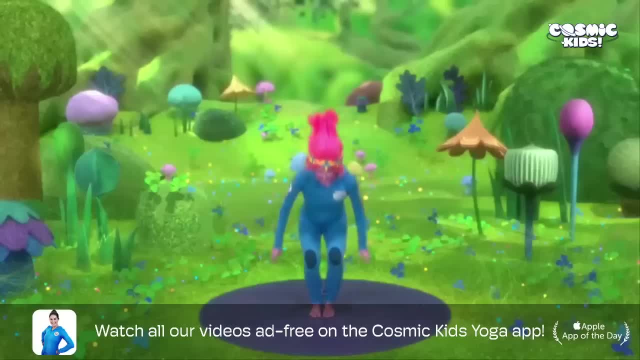 Creek. the Yogi Troll Coming into sandwich pose Sitting on our bottoms, Legs out long. Chef rolls out the wrap. Let's rub our legs. Here we go. Roll out the wrap. Roll out the wrap. She takes her arms wide. 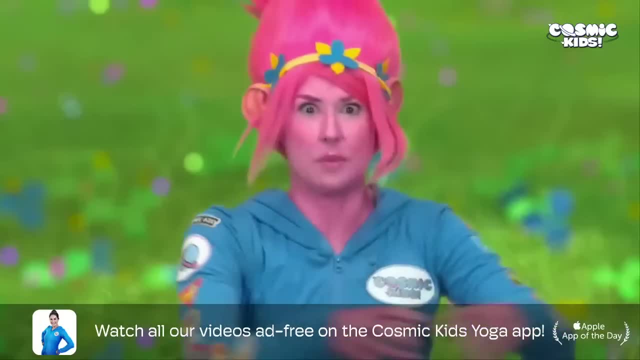 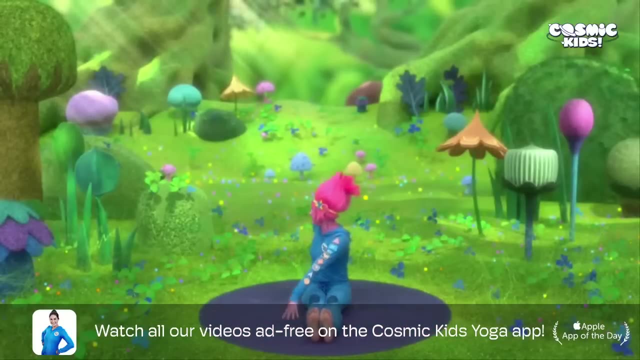 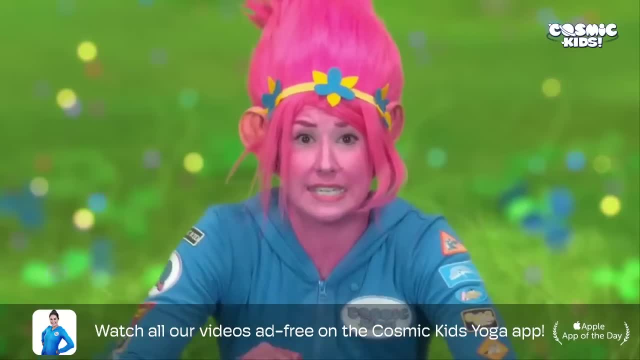 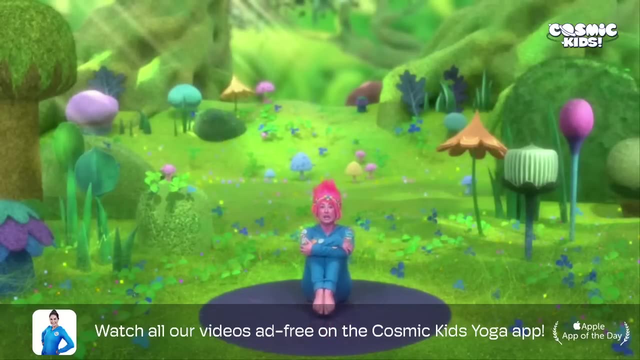 Here we go: Lettuce, Lettuce, Lettuce, Lettuce. Then she rolls the wrap up Arms wide. Now see if you can bring your knees all the way in Lifting your feet, Hugging them in. 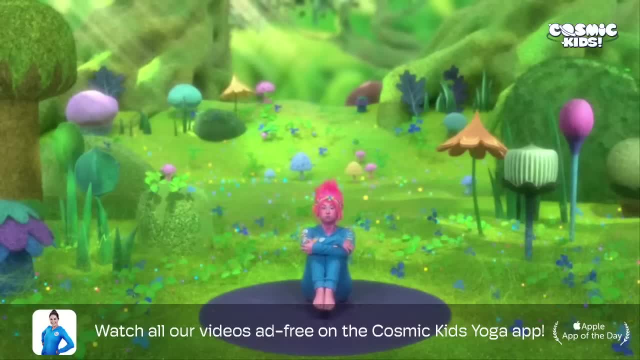 She shoves the whole lot into King Gristle's mouth, But before he can swallow, She slams the door. Coming into door, pose Up onto two knees, Leg to the side, Arm to the sky, And let's slam it this way. 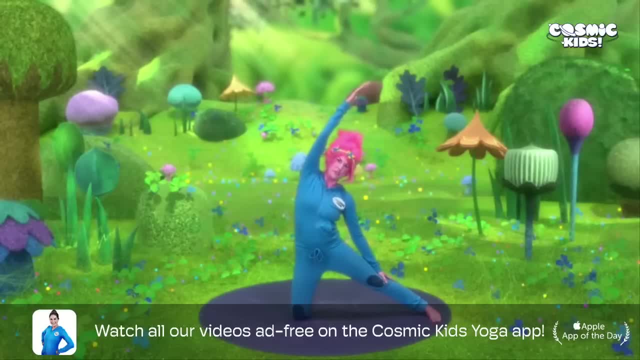 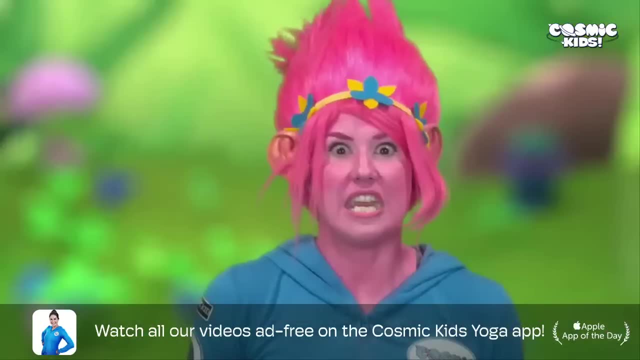 Salaam Poppy feels sure Creek must still be alive, But first she needs to save the others. Coming up to stand, She and Branch jump onto the apron strings of Bridget, The Bergen scullery maid, Bringing your feet together. 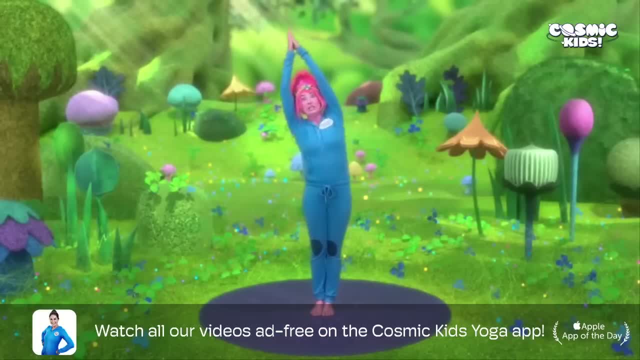 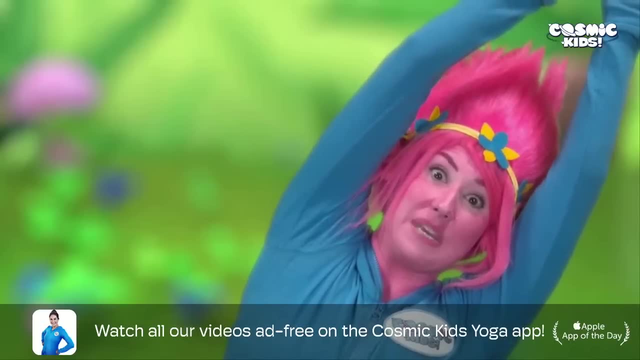 Taking your hands up above your head, Bringing your hands to touch. Now lean over one way, Holding on tight to those apron strings, And lean over the other way. Bridget's taking them into her room to guard the trolls And when she gets there, 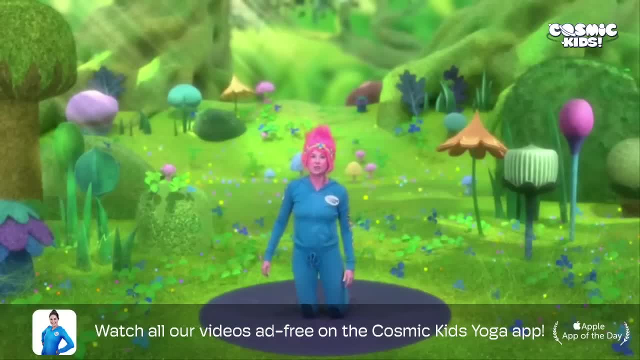 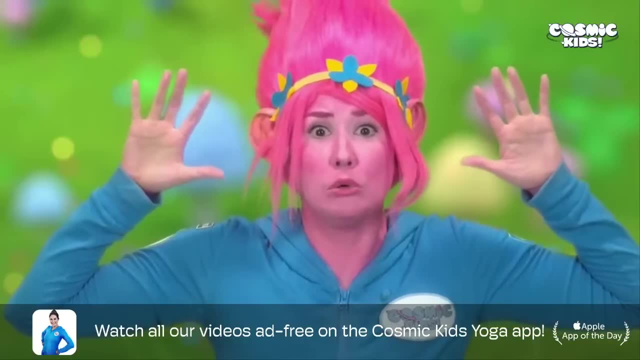 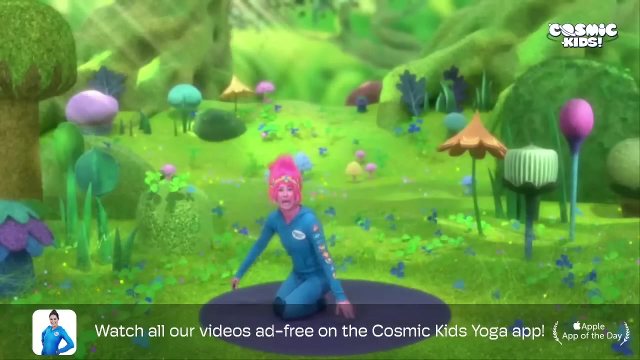 She comes to her knees And she sings a song About her secret love of King Gristle, Bringing your hands up, Hello, Is it me you're looking for? And she lies down on her bed feeling sad: Arms down, Legs down. 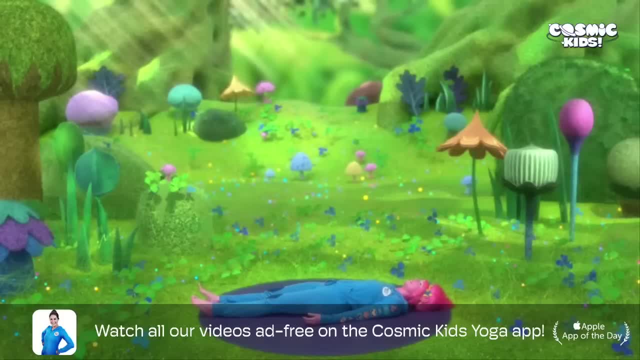 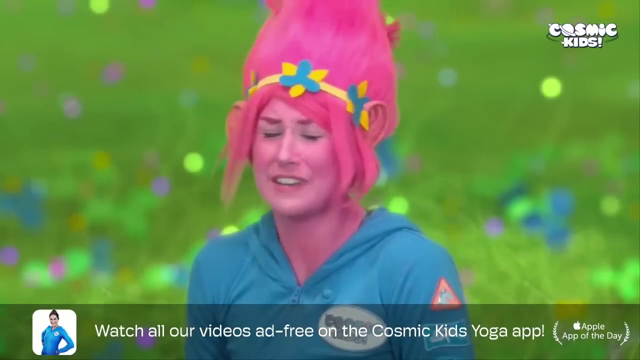 Crying And sleeping, Whistling, Opening your eyes, Coming up to sit- Oh, this is so sweet. Poppy thinks Bridget's in love with King Gristle- Oh, that's the loveliest thing, But she needs to save her friends. 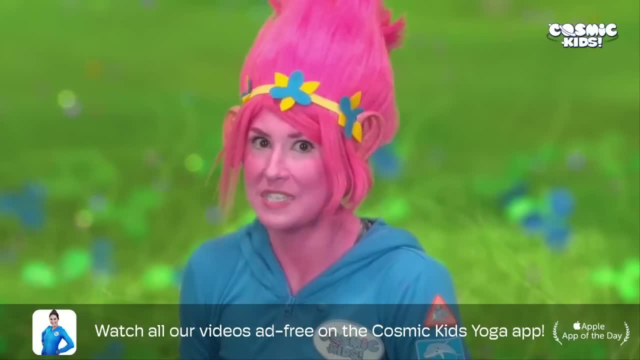 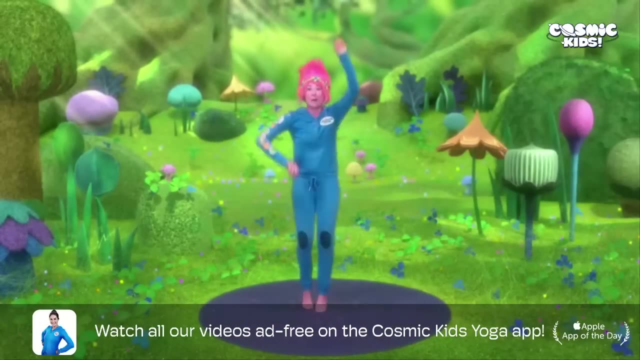 So she and Branch climb silently up to where they're kept in the cage, Coming up to stand. Let's climb silently Up, we go Up, we go Up, we up, we up, we go. When they get to the top, 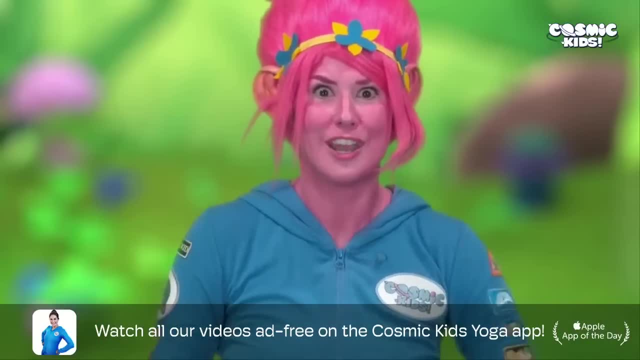 The trolls are so happy To see Poppy and Branch. They do a happy dance And they sing about having a party again. Celebrate good times, Come on, But we need to be quiet. So we crouch down And we. 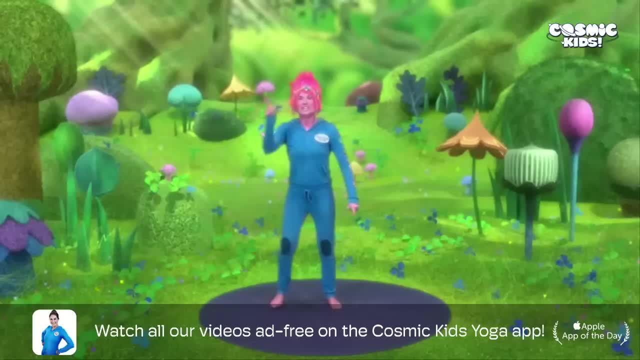 Shhh, Now they're free from the cage. It's time to save Creek, But just as they're escaping, Bridget jumps up in star pose. Stop, Poppy needs to make a deal with Bridget, And so sits calmly with her legs crossed. 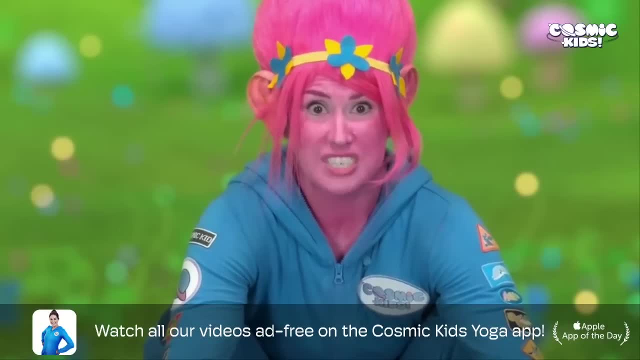 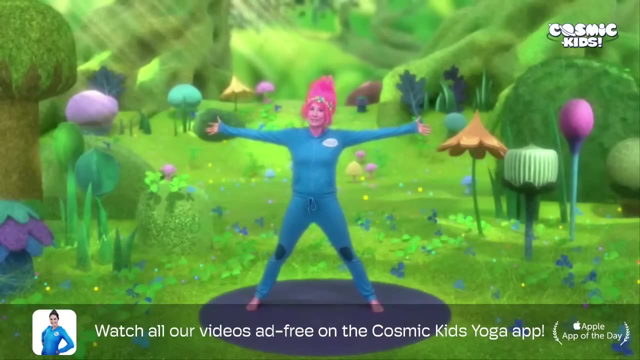 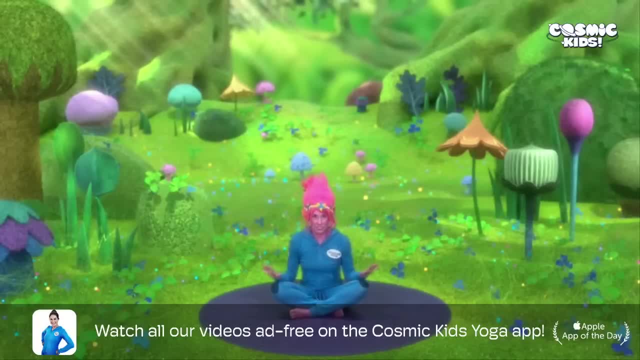 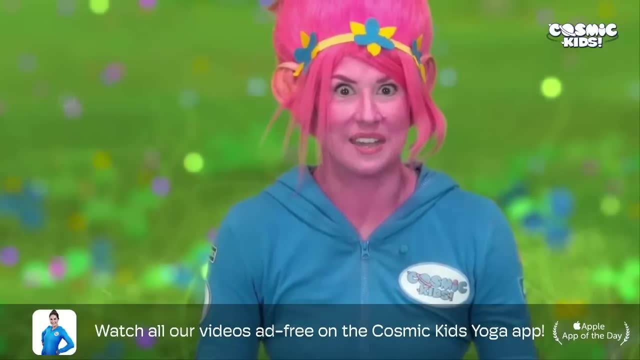 She gets this lovely córnel in family with her legs crossed. She suggests to Bridget That she and the trolls Will turn her into A total Babe So that she can get a date with the king Coming into total babe pose. 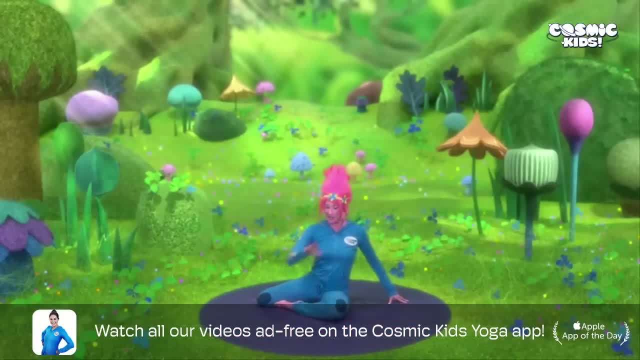 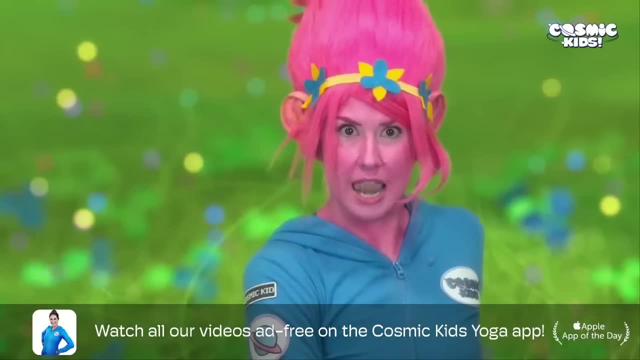 Taking your legs out long, Sweeping them around one way, Putting your hand on your knee, Your other hand behind you, Looking over your shoulder, Back to the front, And going: oh la la, Then let's do it on the other side. 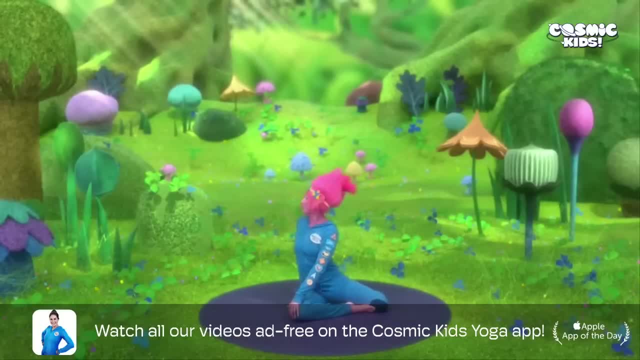 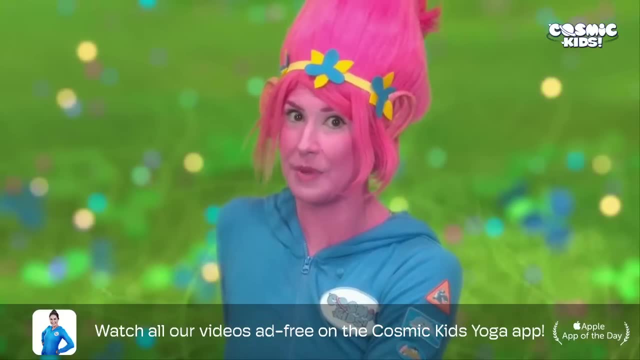 Sweeping your legs round the other way, Hand on your knee, Hand behind your lap, you looking over your shoulder, looking back to the front and ooh la la. In return, they ask Bridget to help them get Creek, the yogi troll, back. After some convincing Bridget, 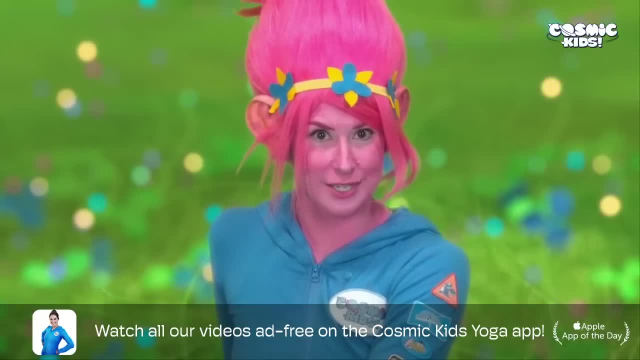 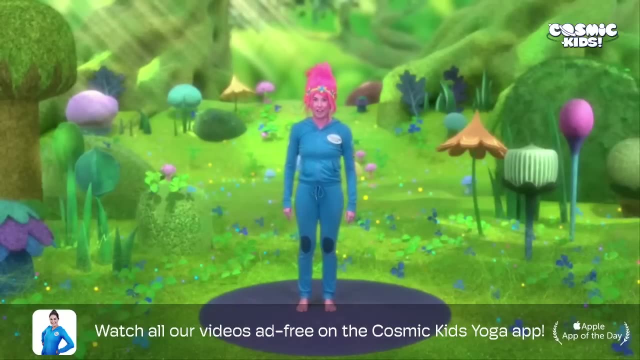 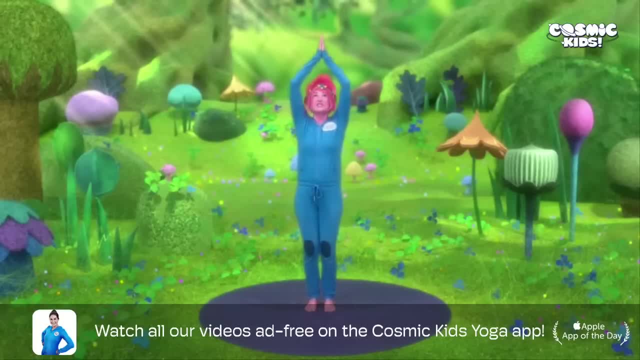 her head, bringing your hands above your head, palms to touch, stretch your arms up high, like your hair's grown very long and they're opening it wide, making that big, beautiful rainbow coloured hair. From here, the trolls can give Bridget the word she needs, because 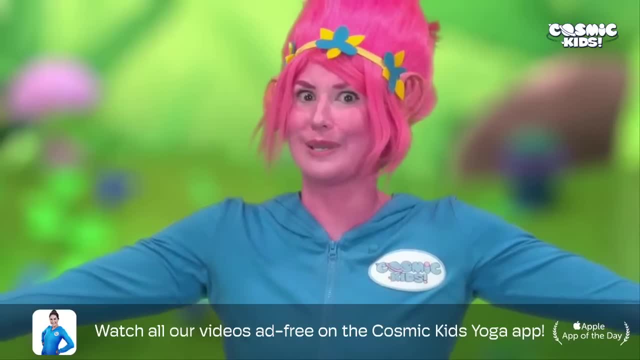 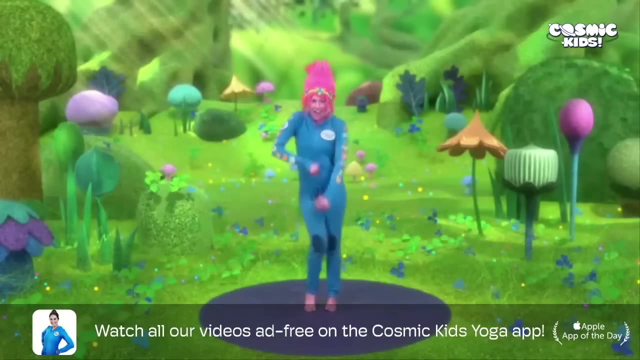 they're standing on her head just in case she gets stuck. when she's talking to King Gristle, Bridget steps out feeling rather awesome and confident: I'm coming out, I'm coming out. I want the world to know. Got to let it show When King Gristle sees lady. 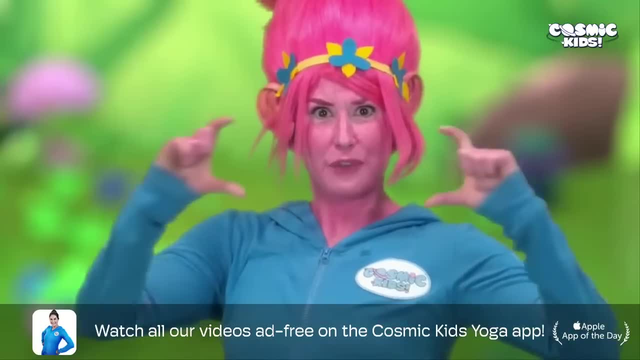 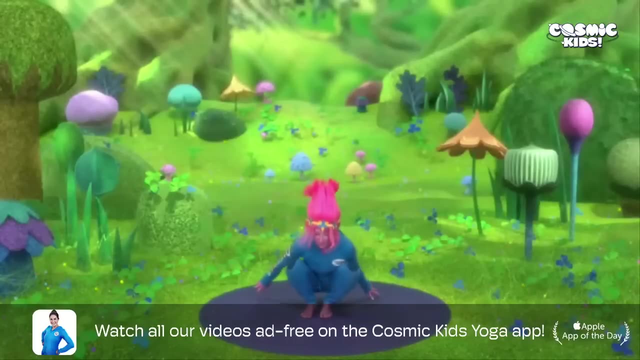 glitter, sparkles. he is in love Seeing if you can make a heart shape with your fingers, Oh yes, together they go and eat some pizza. Sitting on our bottoms, crossing our legs, we rub a hand on our tummies and we pat our heads at the same time. Isn't this amazing? They 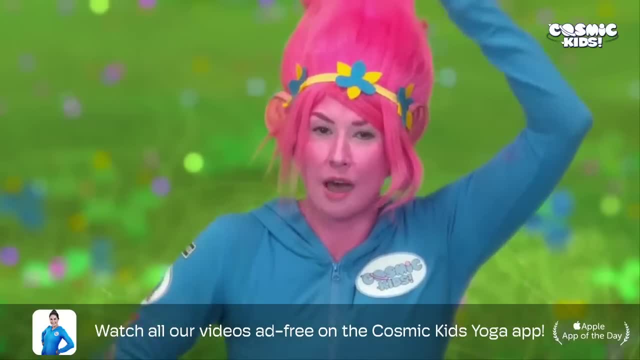 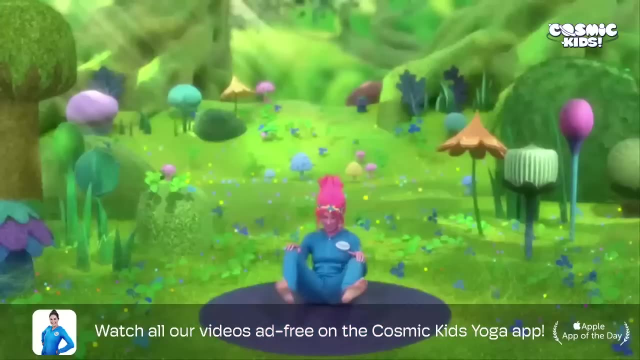 are happy without eating trolls. King Gristle decides to eat to show Lady Glitter Sparkles his gem locket. Coming into our gem locket, pose soles of your feet together, holding onto your feet now, folding your head all the way forwards. 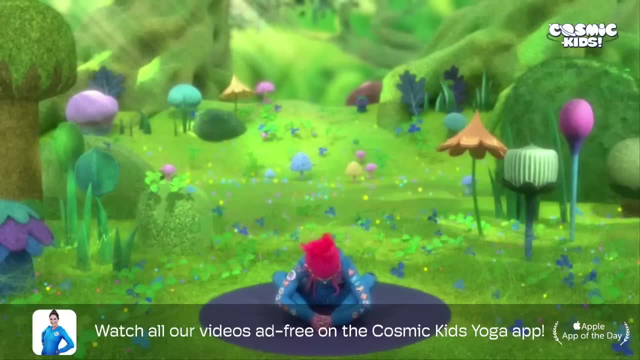 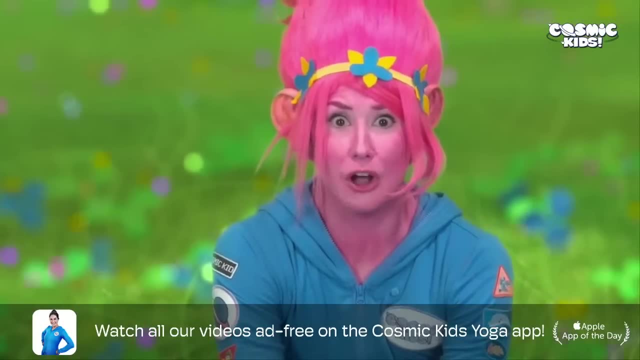 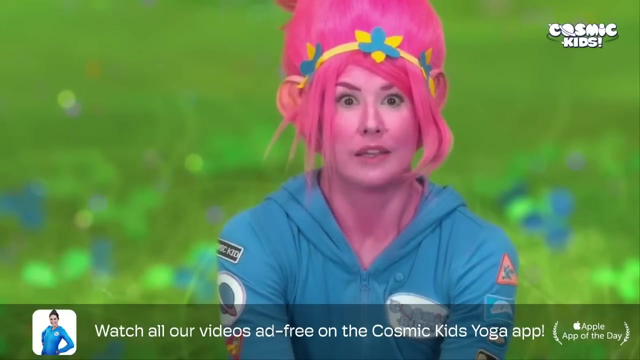 We're going to lift up our head after three to open it up. One, two, three, Whoop. Inside is Creek, the yogi troll. He's alive. Even Mr Dinkle said something. Oh, snap King Gristle asks Lady Glitter Sparkles. 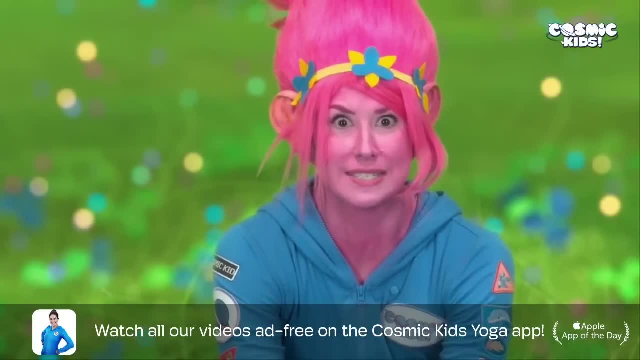 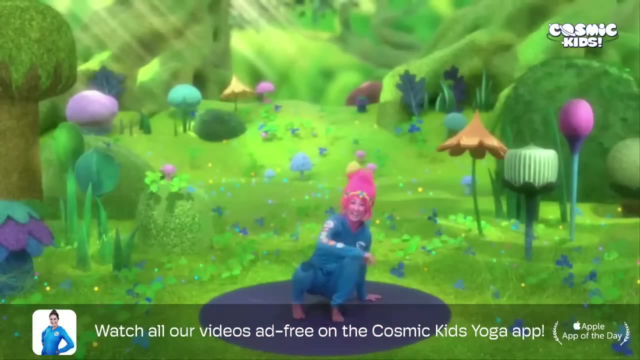 whether she will be his plus one for Trollstice And she says yes. Now they go roller skating. Coming into roller skating, pose up to stand, everyone turning to the side. Now we're going to lift up one of our legs and take our arms wide to take our leg all the way back behind us. 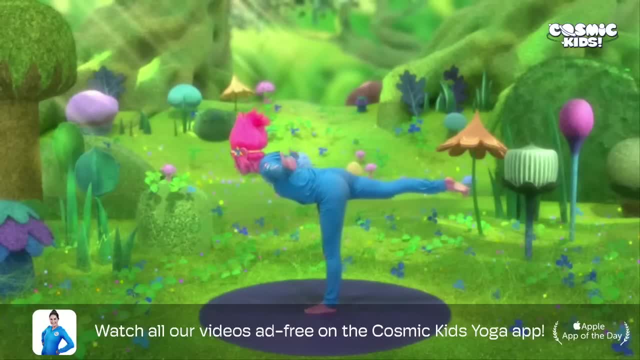 in our roller skating pose. Woo-hoo Coming up to stand. Should we try that on the other side? Yes, I think we should, Standing nice and tall, lifting up one of your legs Now, arms wide, taking it all the way back behind you. 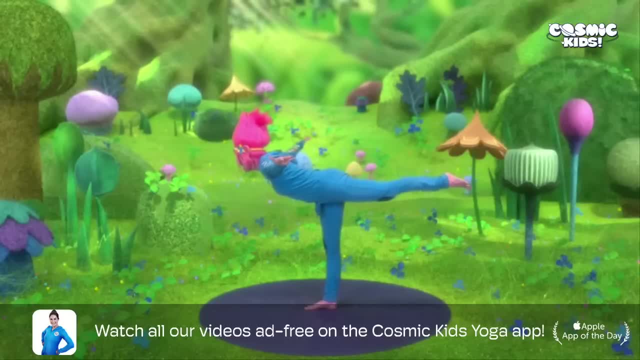 nice and strong. We're roller skating, Coming up to stand. They're having such a wonderful time. And then Chef arrives. She has her hands on her hips and she folds halfway forwards to get a closer look at Lady Glitter Sparkles. 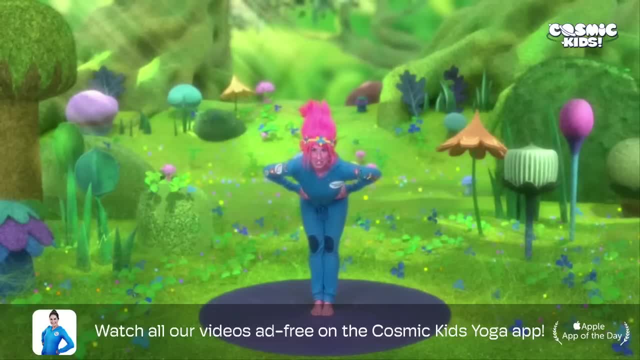 Mm-hmm, She recognises that it's Bridget and Bridget knows she needs to be there. She knows she needs to be there. She knows she needs to be there, She knows she needs to get out of there, Coming up to stand, putting one foot forward, one foot back. 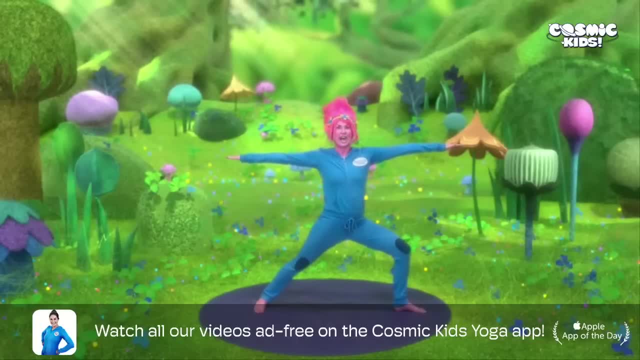 Bend your knee arms wide. She skates as fast as she can, Whoosh, But she leaves a roller skate behind. Coming to stand, King Gristle is delighted. Folding all the way forwards, he scoops up the precious roller skate. 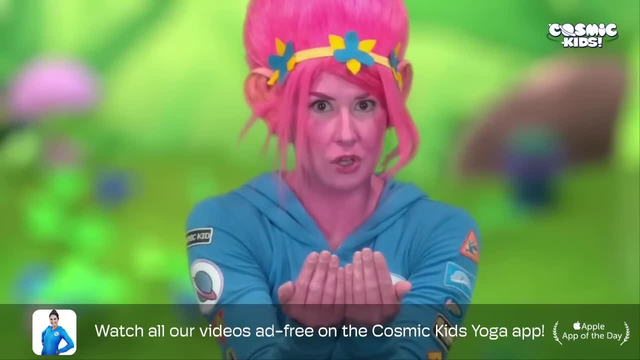 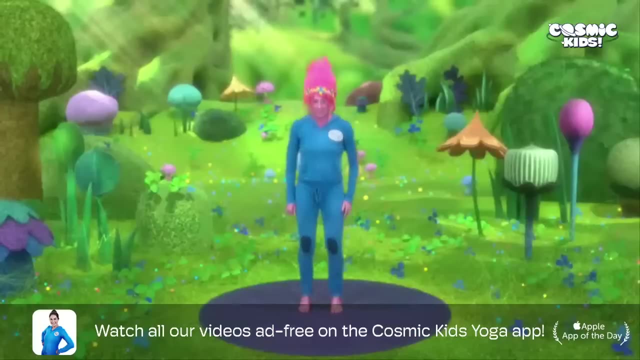 Will she be his Cinderella and come to Trolstice? He hopes so. He decides he needs to get back. He has to get fit, and so he starts exercising. Jump your feet wide, take your arms wide. Let's do some windmill pose. 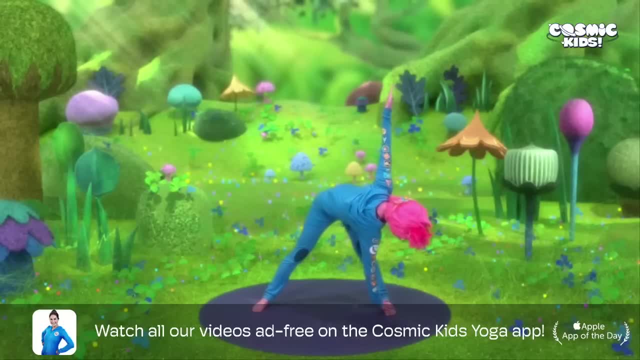 Take your hand across to your opposite foot and reach your top arm up to the sky. Now let's switch sides. Take the other hand across and your other arm to the sky. Now let's see if we can do eight switching sides. Here we go. 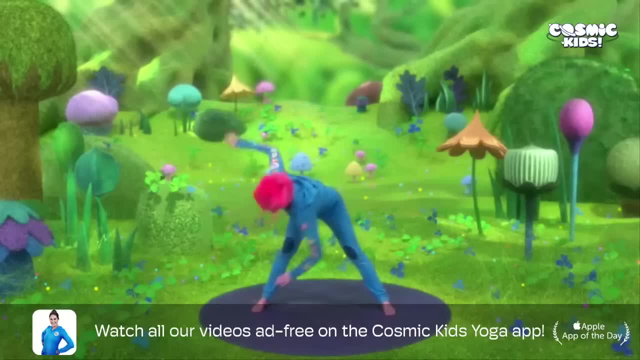 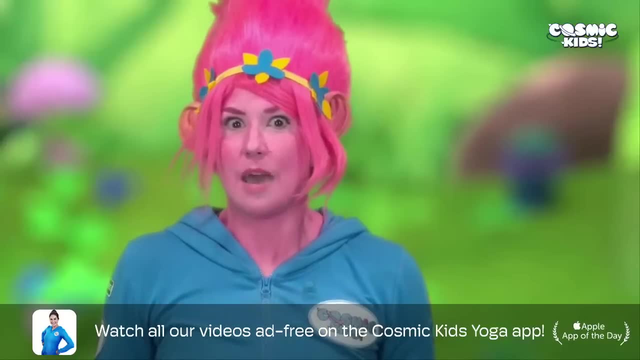 And one and two and three and four and five and six and seven and eight, Rolling up to stand. This is their moment. The trolls wiggle in under the rug, Coming onto your tummies everyone. 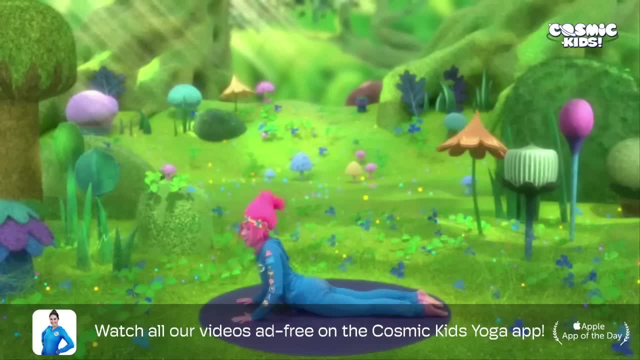 Hands underneath your shoulders and let's wiggle, wiggle, wiggle, wiggle under the rug. They're looking for the gem locket with Creek inside. There it is Lying all the way down, reaching forward with your arms to grab it. 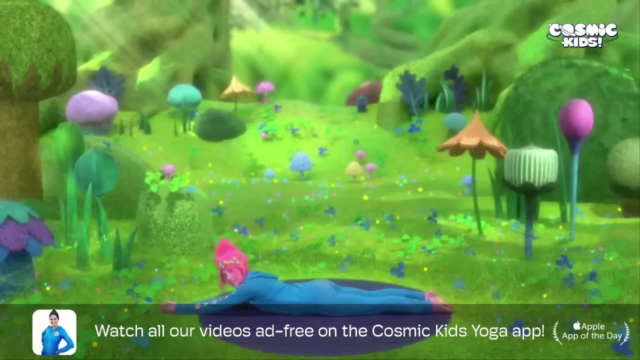 They've got it. But just as they do, Barnabus the crocodile sees them Rolling onto your side and opening and closing your crocodile jaw. Oh no, he's chasing them. The trolls jump on the roller skate, Sitting up legs out long, and they drive it out of there. 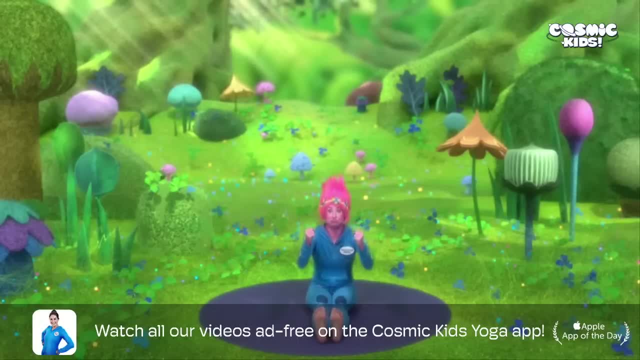 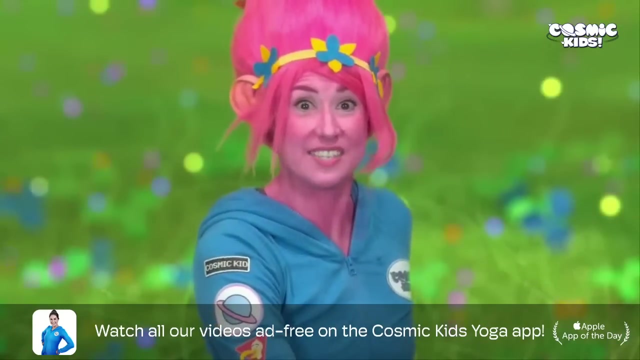 Holding onto the laces. they go forwards really fast. Then they sit up really tall And Guy Diamond, the wonderful glitter troll, twists to the side and he blows Barnabus with his glitter And the other side, turning to the other side, blows some more glitter. 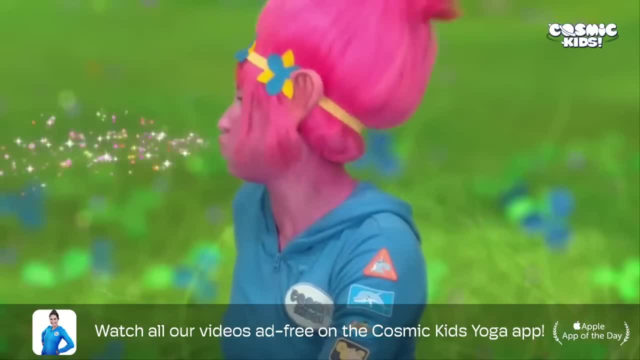 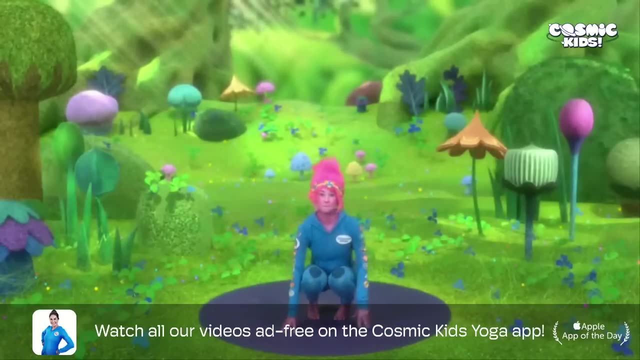 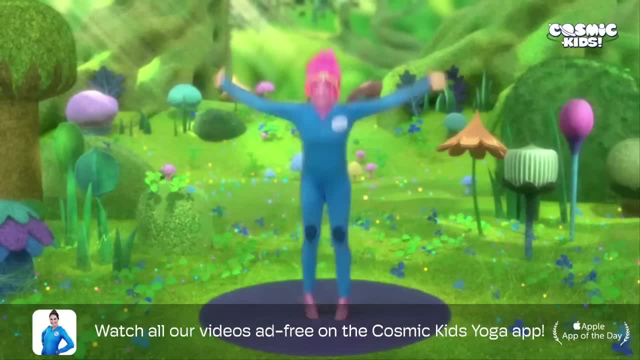 After three, let's jump in the air like with a locket. One, two, three, whee. It pops open, sitting on our bottoms, soles of the feet together, bringing your head all the way forwards. After three, lifting it up: one, two, three, whoop. 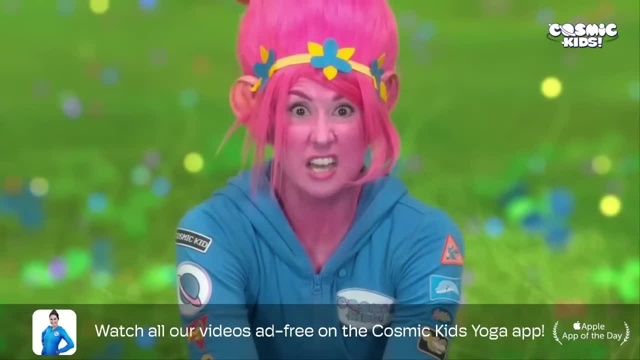 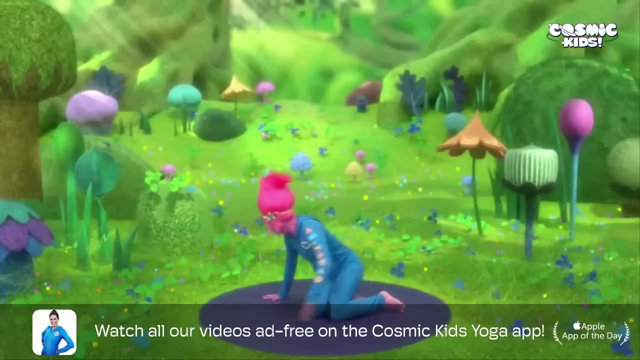 But Creek isn't there. He's disappeared. Just at that moment, Chef arrives And she puts down a grill. thenhaft, She twists down and balls him. a confetti Got up and haunts him. for all those bars cage on top of them, all coming onto our hands and our knees, tucking our toes and lifting our 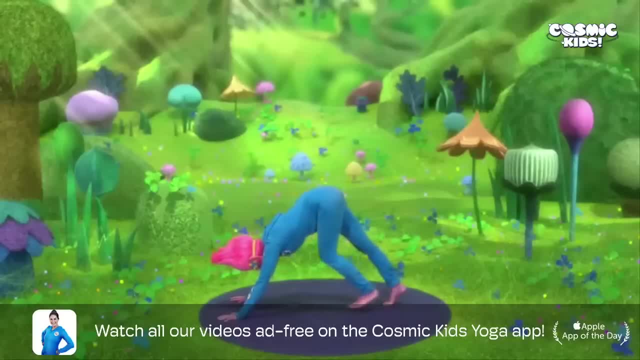 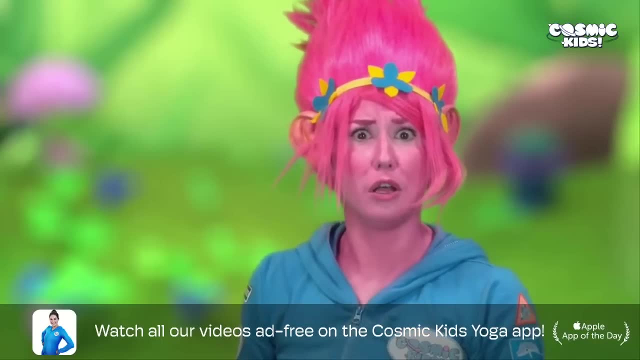 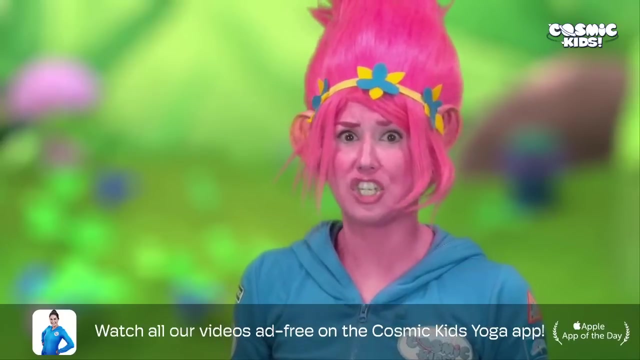 bottoms to the sky. but who's this appearing walking your feet all the way forwards, rolling up to stand. it's creak. the yogi troll. he's sold them out. he's agreed that he will ring poppy's cowbell three times and lead chef to where all the other trolls are hiding. take your feet wide. 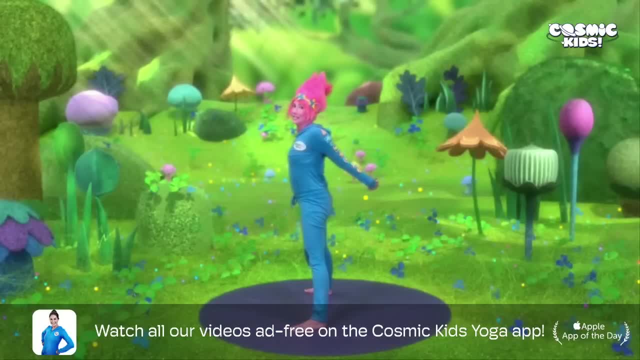 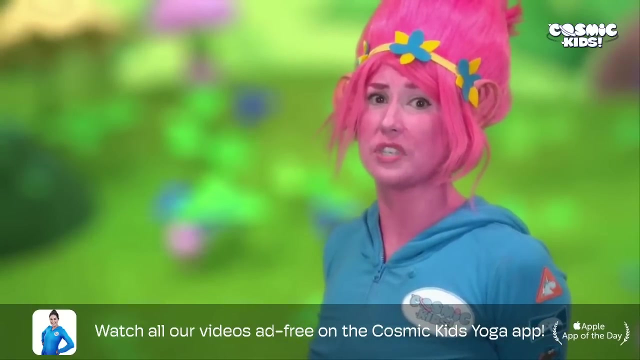 crisscross your fingers behind your back, stretch your arms out. now, after three, let's fold forward and ring poppy's cowbell. one, two, three and up. one, two, three and up. last time. one, two, three and up. this is so. there'll be enough trolls for trollstice. come the day of trollstice. 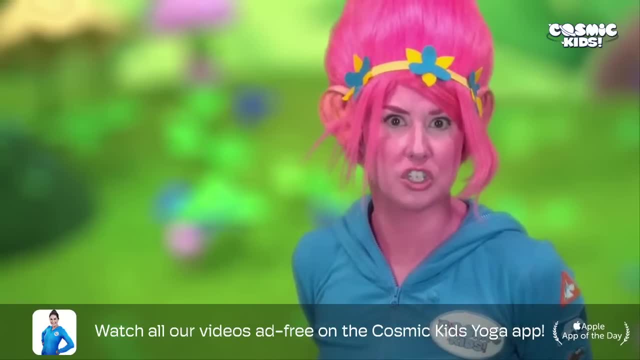 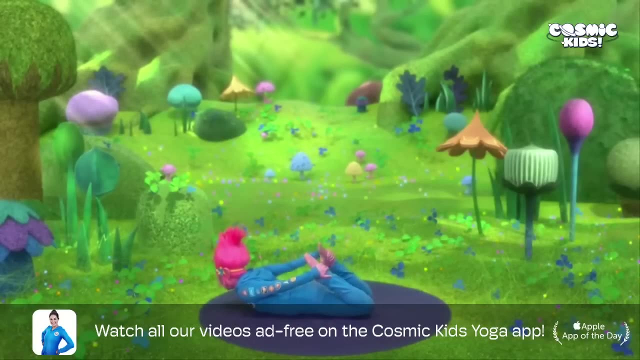 chef puts all the trolls into one ginormous pot. coming into pot pose, lying on our tummies, everyone bring your feet towards your bottom, reach round to grab your ankles and kick your feet into your hands, lifting yourself up into your pot pose. poppies feeling sad. 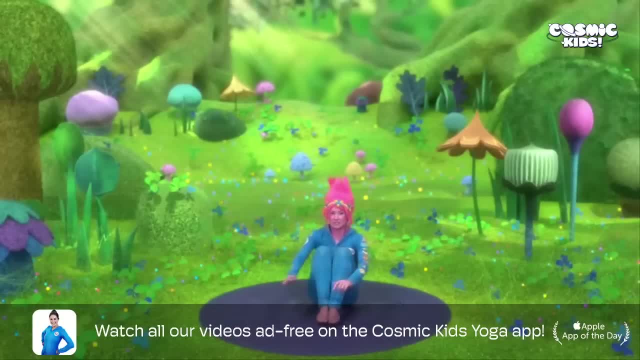 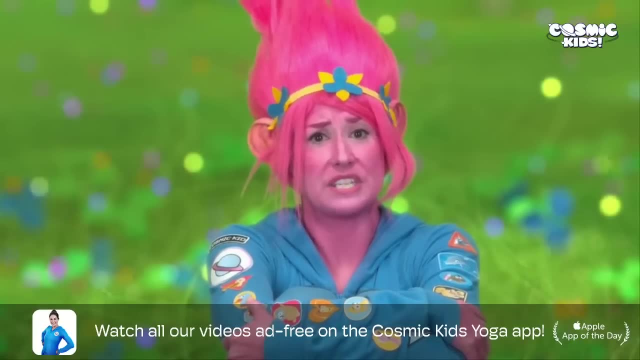 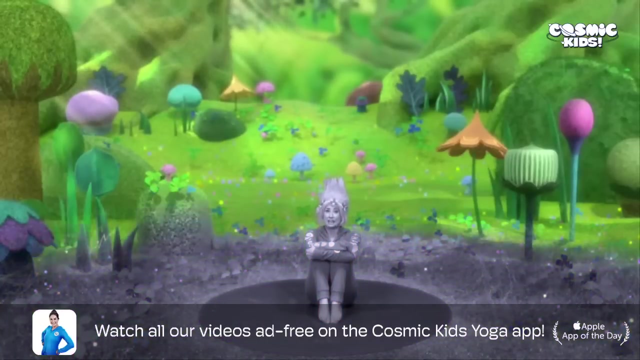 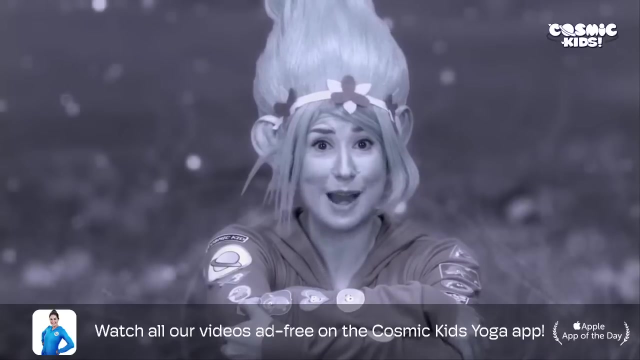 sitting up. she hugs her knees. she feels like she's let everyone down. she feels like she's let everyone down and all of the positivity and hope leaves her. her color drains away and she is left gray. it then drains away from all the other trolls. then, for the first time since losing his grandma, branch comes forwards. 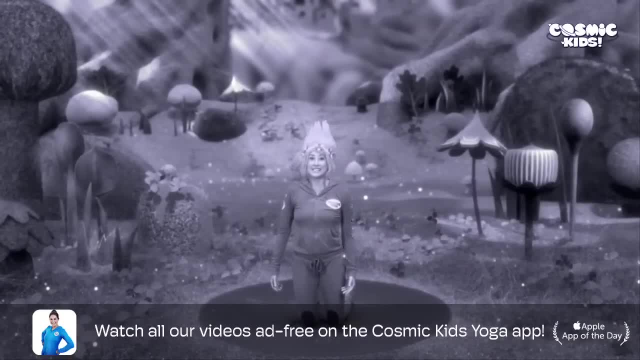 coming up onto our knees everyone. he sings to poppy. he tells her that he thinks her true colors are beautiful like a rainbow. let's do our rainbow. pose arms wide, leg to the side, drop down onto one hand and sit down on your knees and let go of your knees and let go of your knees and. 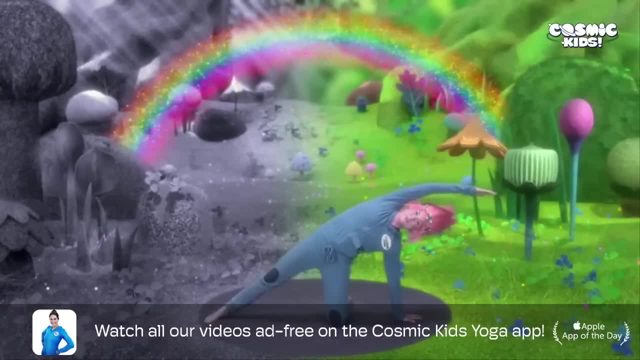 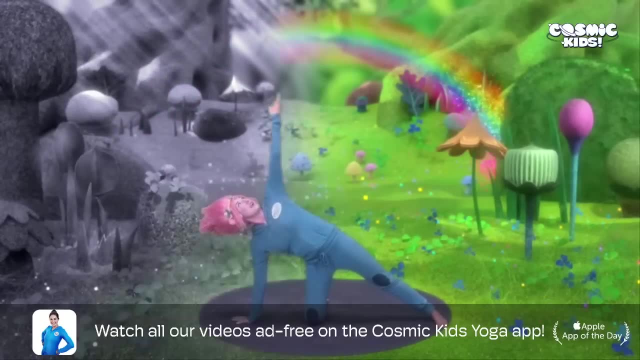 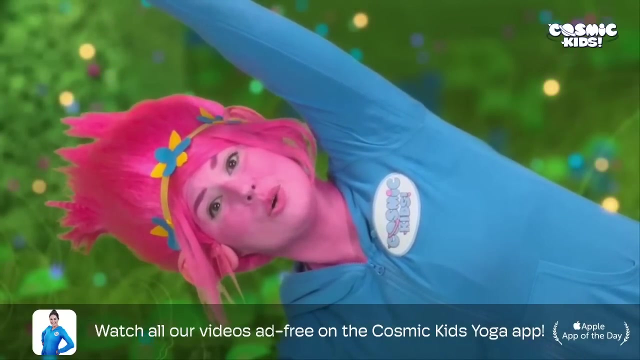 sweep your arm up and over your ear, making your big, beautiful rainbow coming to two knees again. arms wide, leg to the side. drop down onto one side and sweep your rainbow up the other way. he sings to poppy and that's why I love you, poppy. 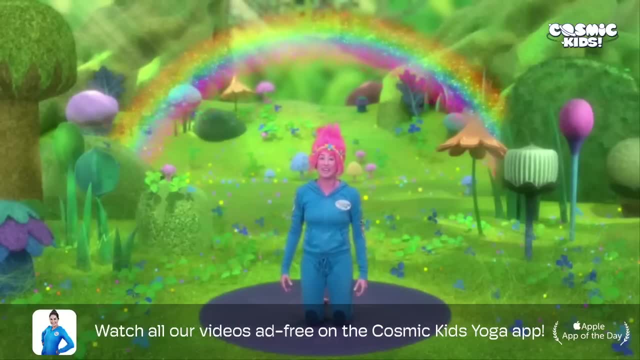 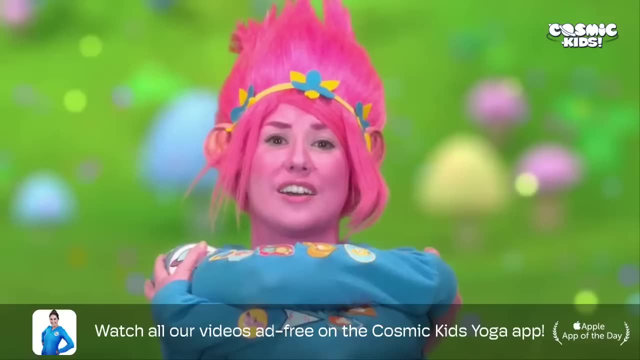 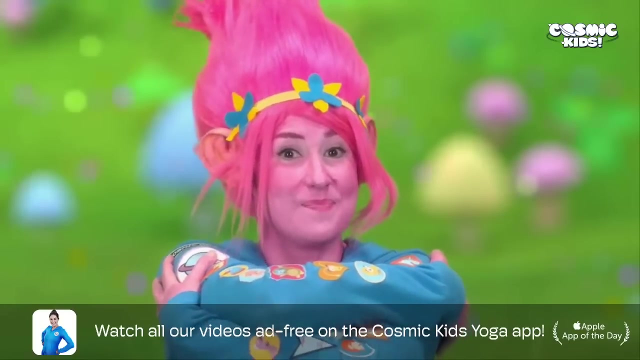 comes up. hearing this, hearing this hope again brings hope flooding back to her and she and branch open their arms wide and share a big, wonderful hug. all of the color comes back to the rest of the trolls and to branch: isn't grey but is blue. now the lid of the pot gets opened. sitting on your 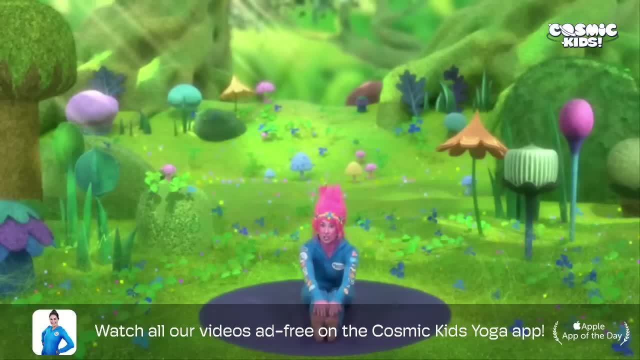 bottoms, legs out long, bending our knees, touching our toes. after three, let's lift our arms up to open the pot. 1, 2, 3. it's Bridgette. einfach, she's letting them all escape. she wants to thank poppy for helping her find her. тому I взглядachte перемешать vais ущипатьה. 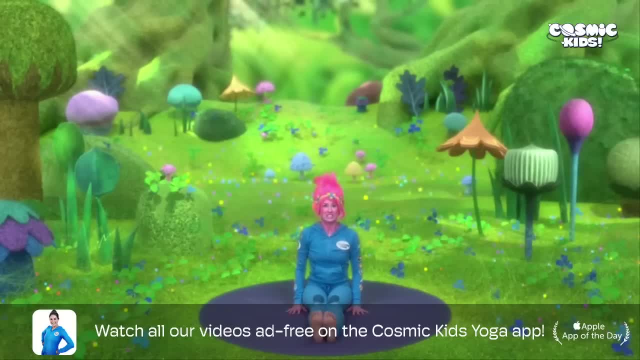 true happiness. But now Bridget is in some serious trouble for letting the trolls escape, Coming up to stand one foot forward, one foot back. Poppy's not going to leave Bridget, nor are the other trolls, and they whoosh in on the. 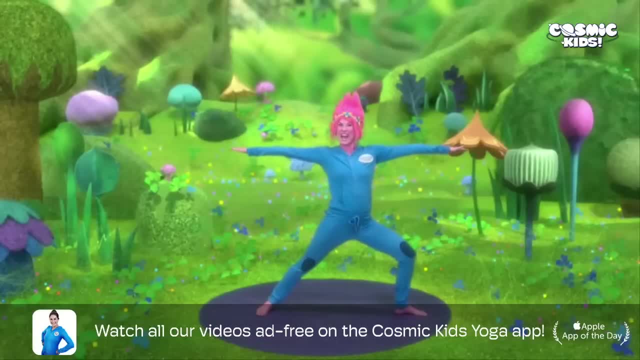 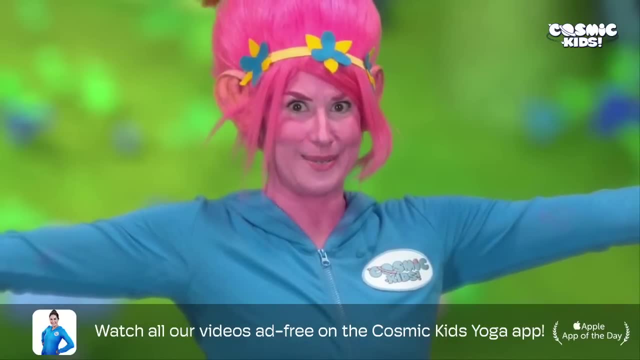 roller skate to save her. Sweep your arms up, bend your knee and let's whoosh, Whoosh- They jump back on Bridget's head, turning her back into Lady Glitter Sparkles. Hands together above your head, sweep your arms up and open them wide, King. 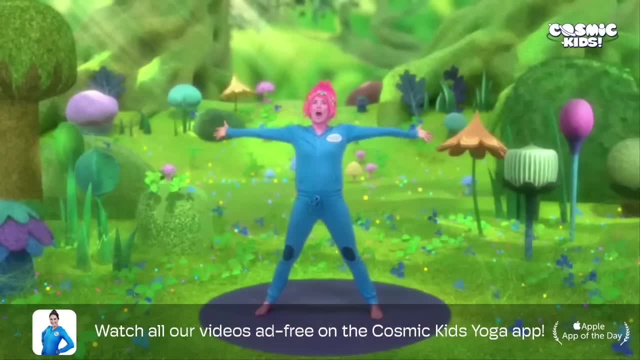 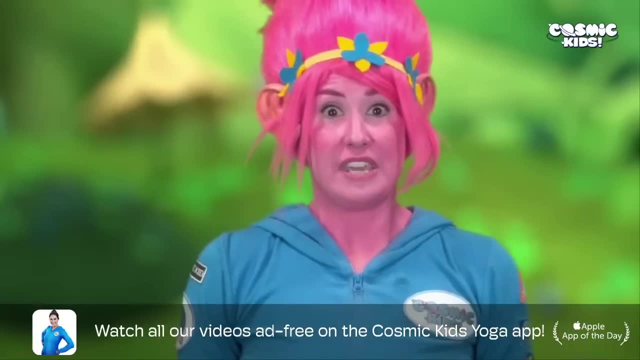 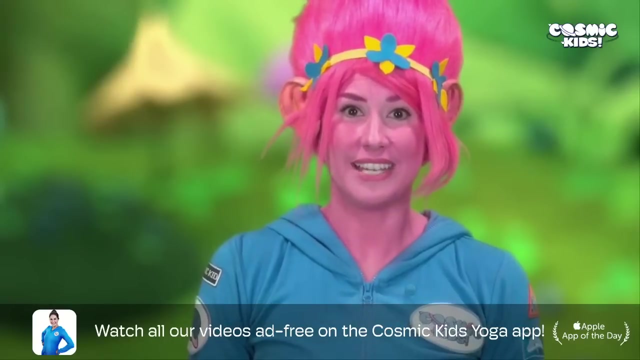 Gristle is delighted and stands in star pose to protect his Lady. Glitter Sparkles Poppy steps forwards, She reveals herself and she explains: You don't need to eat trolls to find happiness. It's in each and every one of us. We just need to find it. Look at King Gristle and Bridget. They had a. 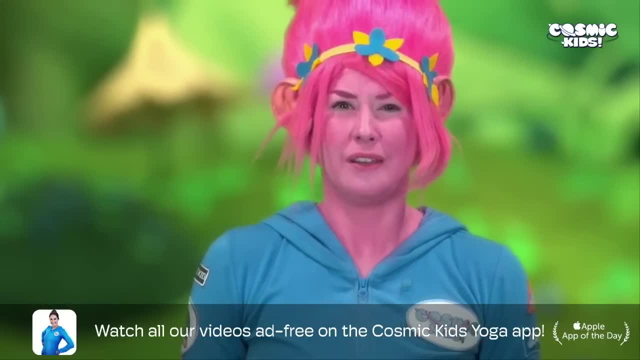 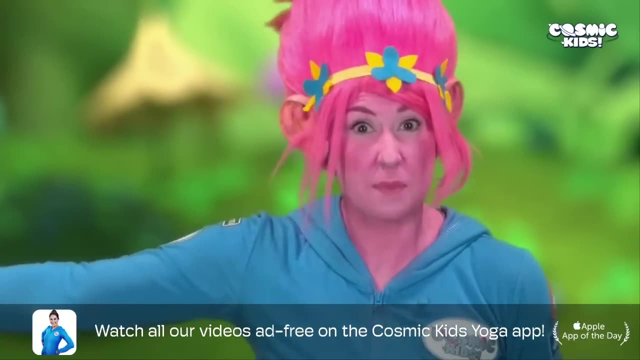 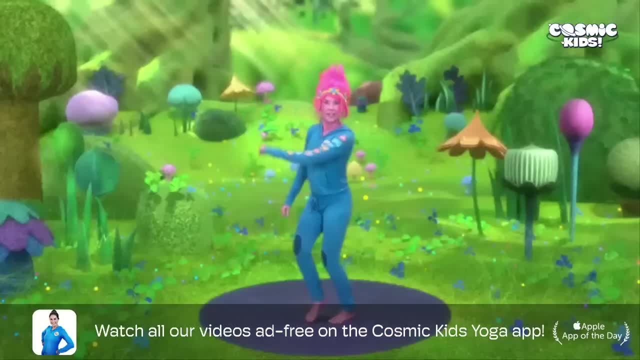 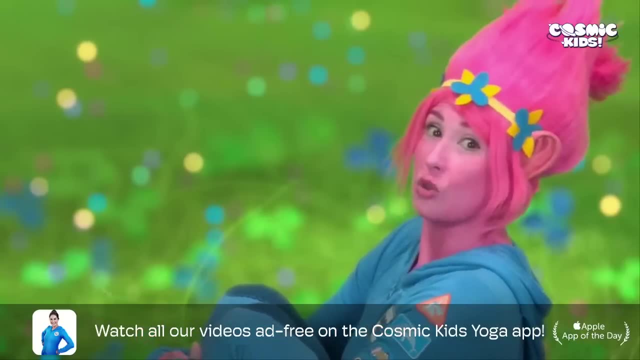 palace, rolling down the hill in a burning hot pot, Coming into our roly-poly burning hot pot pose, Sitting on our bottoms, hugging our knees. Now we're going to tuck our chin and rock all the way back and all the way up After three. 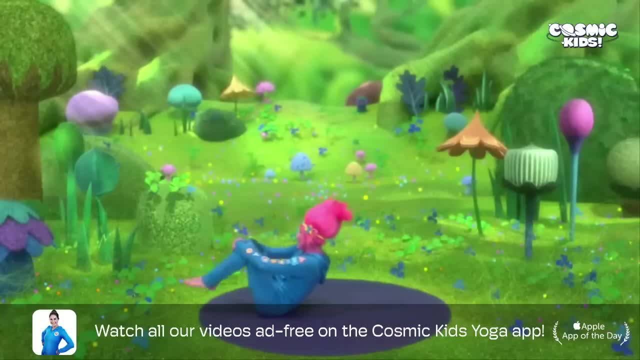 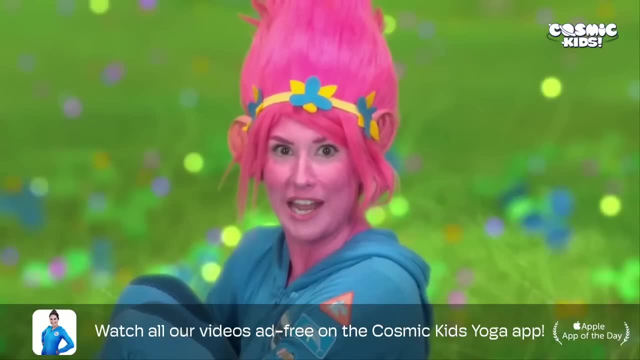 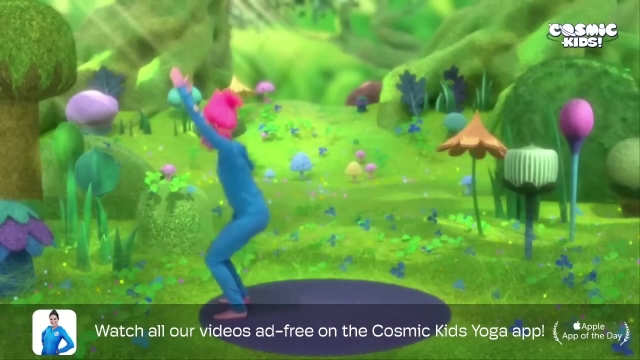 One, two, three, Whoop Whee. One, two, three, Whoop Whee. Now, this last time, can we rock all the way up to stand? Let's try Ready. One, two, three, Whoop, Kick your legs and up we go. Yay, From that day on, Bergentown blooms again. 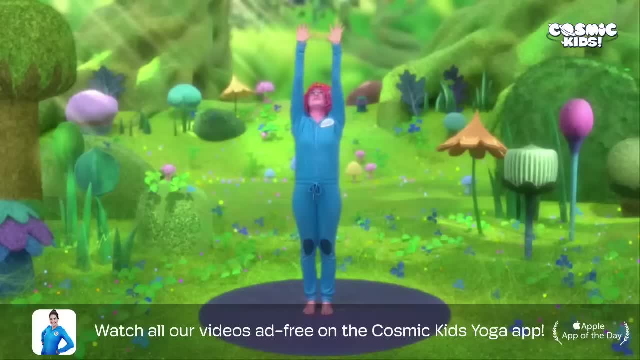 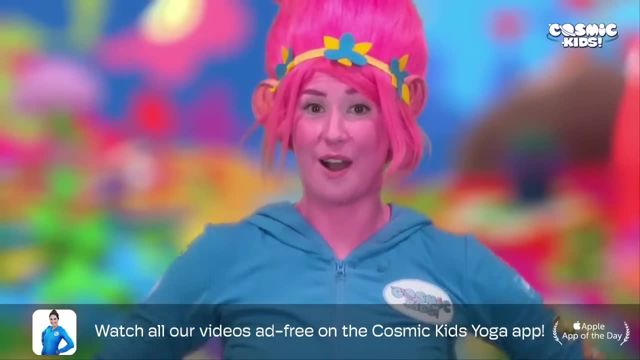 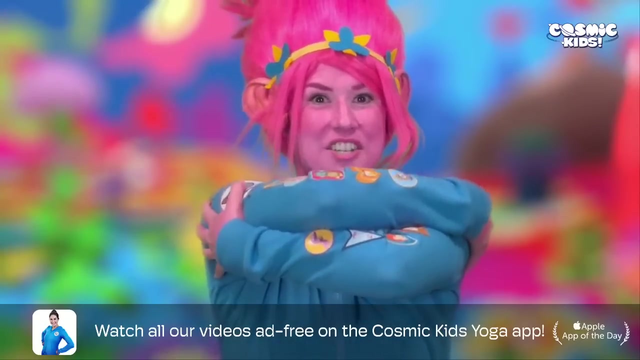 Bringing your hands together. Grow your arms up nice and tall and open your arms, spreading beautiful rainbow colours all over. Branch and Poppy share a big hug, Arms wide, Wrap yourself up in that wonderful hug and Poppy is now the queen. She makes a new law: that hug time is all the 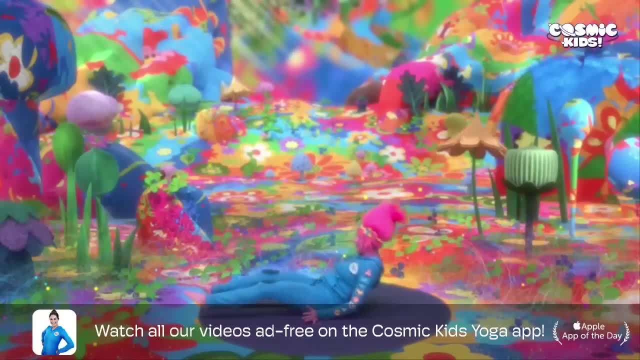 time, Coming down to lie in our relaxation pose, Our legs long and our arms down by our sides. We close our eyes and let ourselves relax here for a few moments, Enjoying this peace and this calm, Letting all of the glitter and the 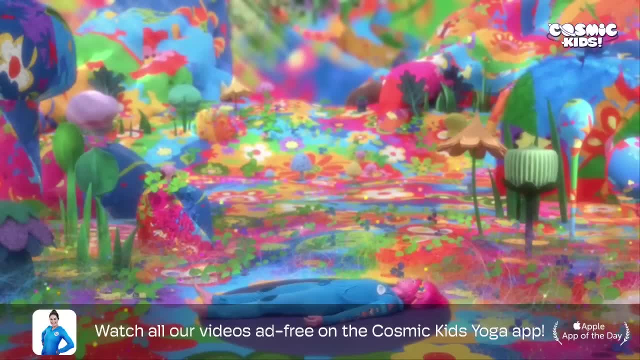 sparkle settle in our hearts. So often we look for happiness outside of ourselves To things that we own, Things that we buy Stuff, When actually real happiness lives inside each and every one of us. We just have to find it And the time that we share with loved ones, friends and families. 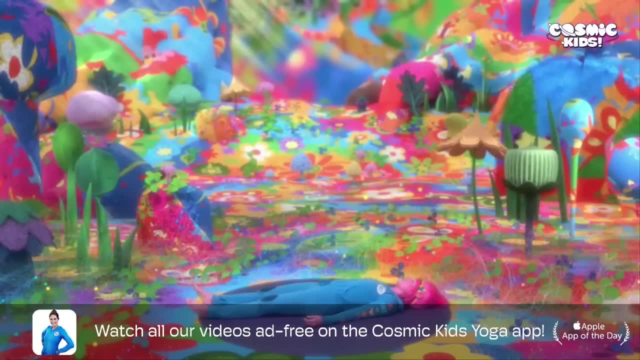 We can double, triple and maybe even quadruple our happiness by sharing just that special time with them, And the happiness we feel from a hug is so special and so strong. Look for the happiness in the little things in life, And that means life will be full of glitter, showers and rainbows. 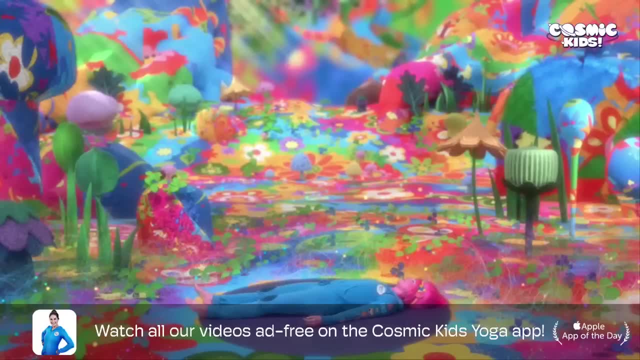 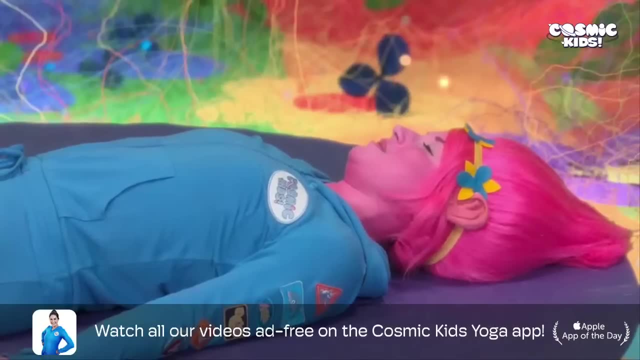 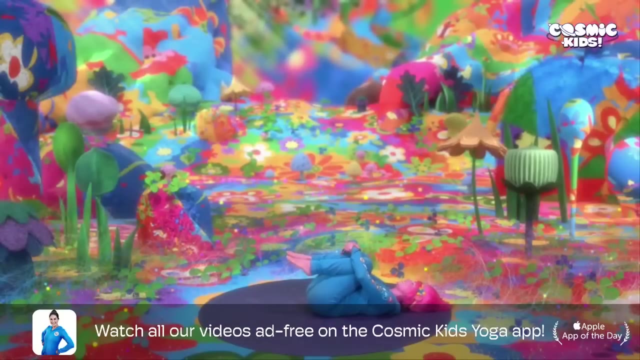 just as it is for the trolls. And now it's time to wake up. We wiggle our fingers and our toes, We bring our knees into our chests and give them a nice hug. We roll onto our sides, pushing ourselves up to sit. 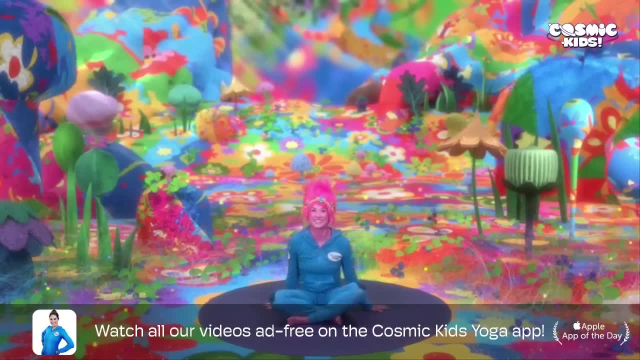 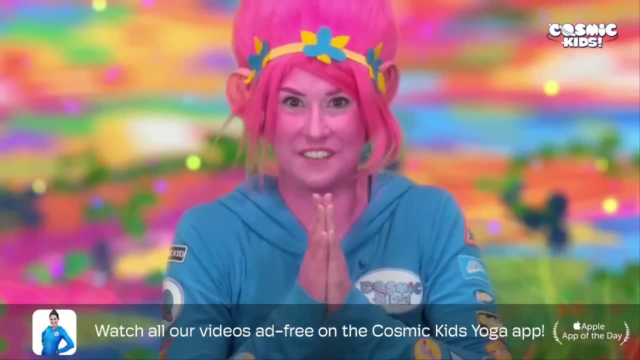 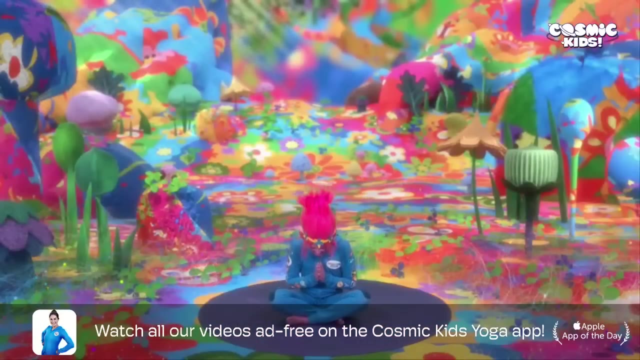 opening our eyes and crossing our legs. We finish just the way we started: with a namaste. So we bring our hands together at our hearts And after three, let's say it together: One, two, three, Namaste, Wow, well done everyone. 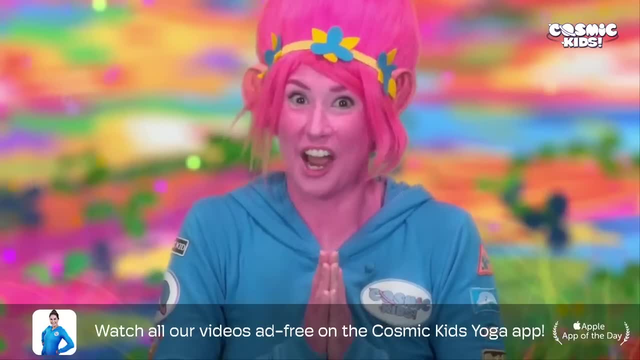 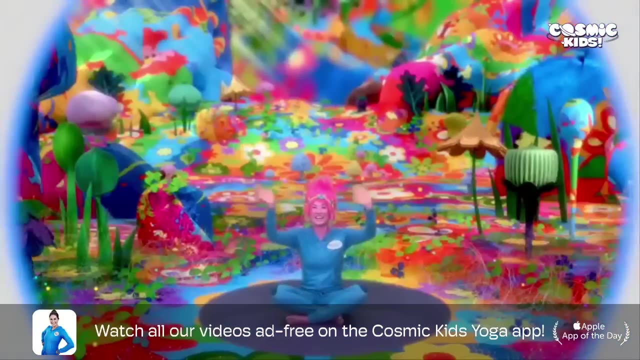 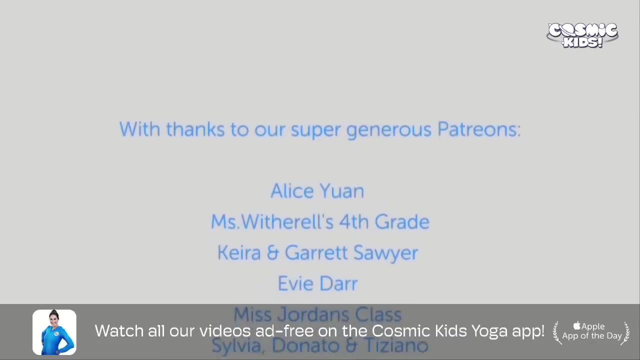 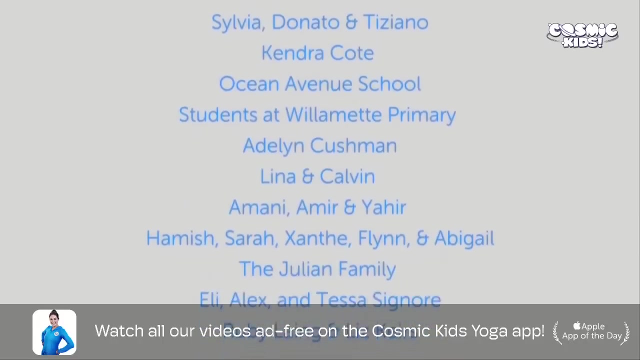 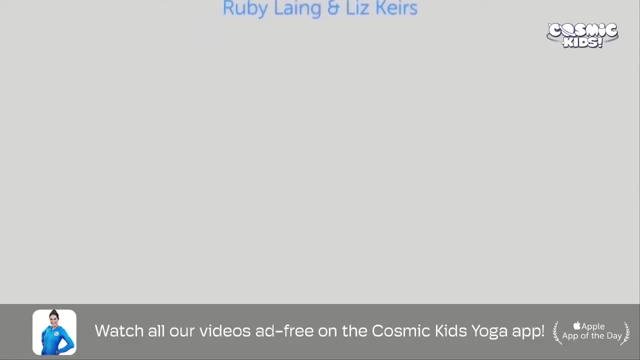 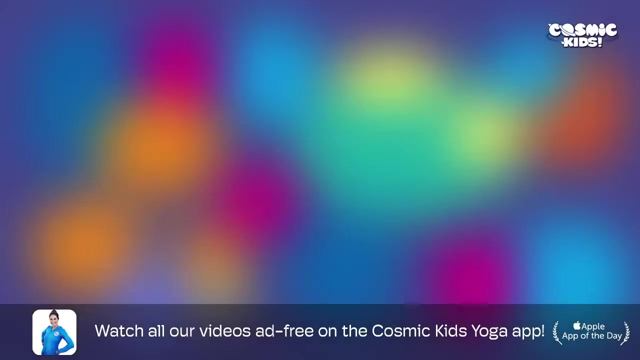 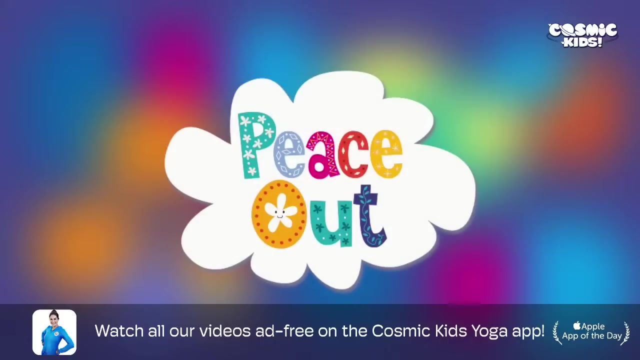 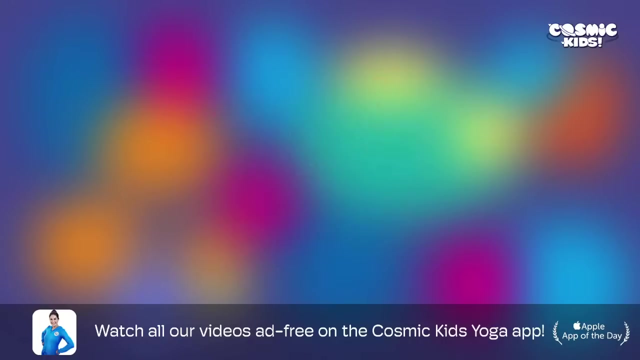 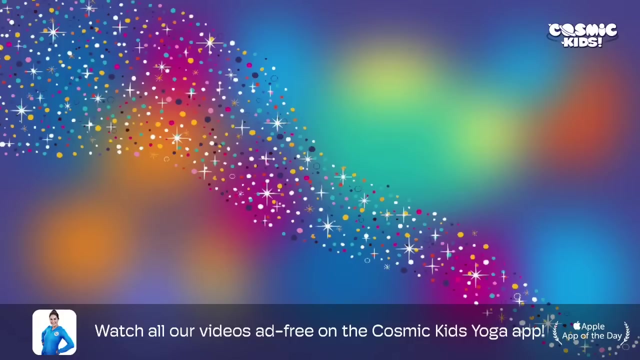 That was super cool. You were amazing. I hope you enjoyed the trolls adventure And I'll see you again soon for another Cosmic Kids adventure. Bye-bye, Peace out. Tickle pixie. Hello Jamie here, Welcome to peace out. 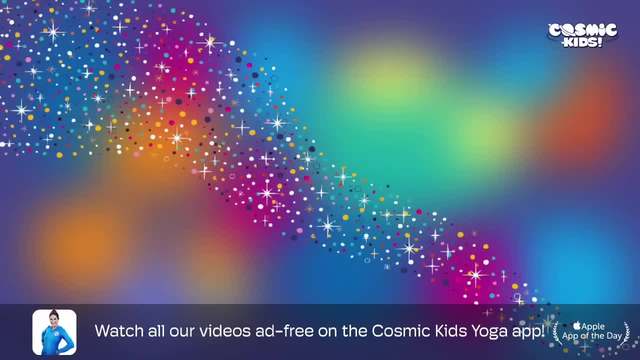 It's time to turn the light on in your imagination and enjoy your amazing mind. So do what you need to do to get lovely and comfy, Find a space and lie down On your back, with your arms down by your sides or on your tummy. 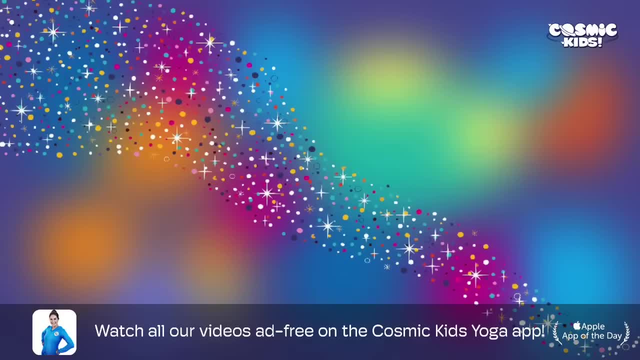 making a pillow with your hands to rest on. You decide which feels most comfortable. Now get settled. Do a wriggle and a fidget to make sure your body feels really happy and comfy. You don't need to be a superman. 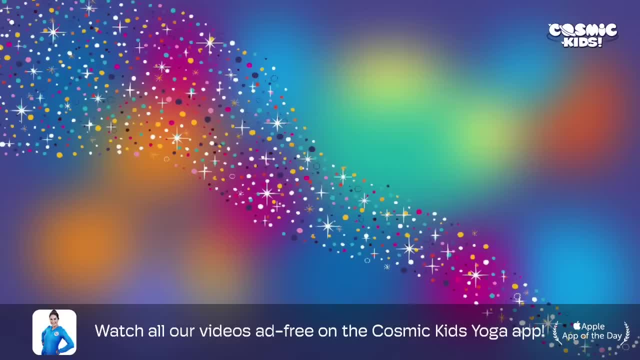 You don't need to be a superwoman. You don't need to be a superman. You don't need to be a superwoman, You don't have to be completely still. You can breathe and blink as normal. Just see if you can keep your body nice and still. 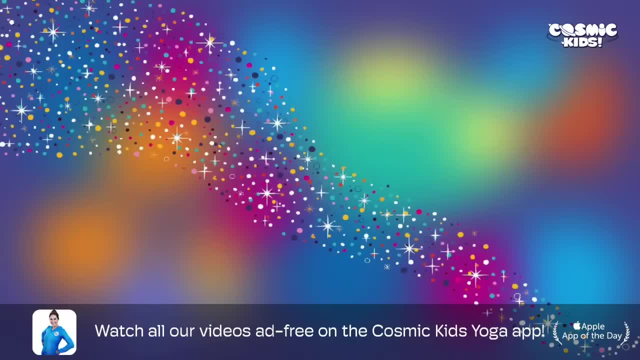 Your eyes are open. Now that you're still, can you notice your breathing? Maybe you can feel it a little bit in your chest, maybe your tummy, at your nose and mouth Can you hear it too. It might be very, very quiet. 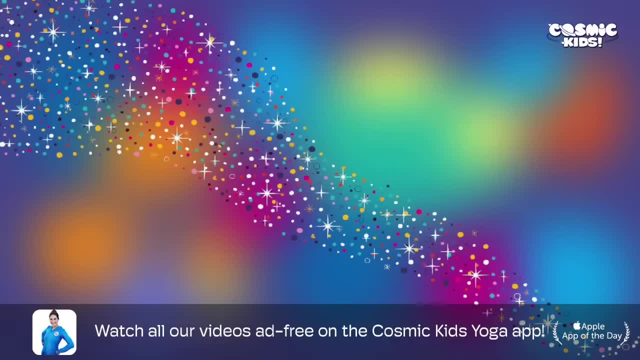 like a tiny whisper sound. See if you can hear it. I'll be quiet, so you can try. I'll be quiet, so you can try. That's it. Gentle breaths coming in through your nose and out through your mouth, In through your nose. 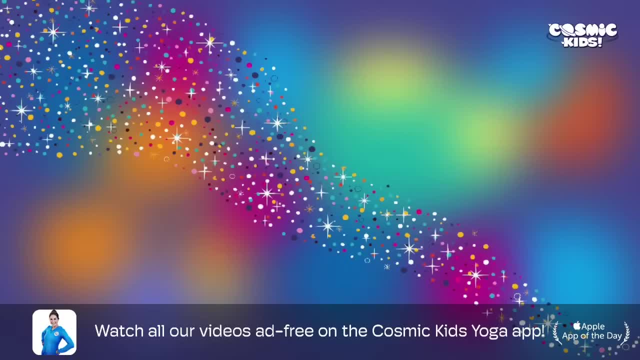 and out through your mouth. This next time, as you breathe out, let your eyelids softly close. Well done. Now you have a big blank screen in your mind. See if you can imagine a little pixie standing right in the middle of it. 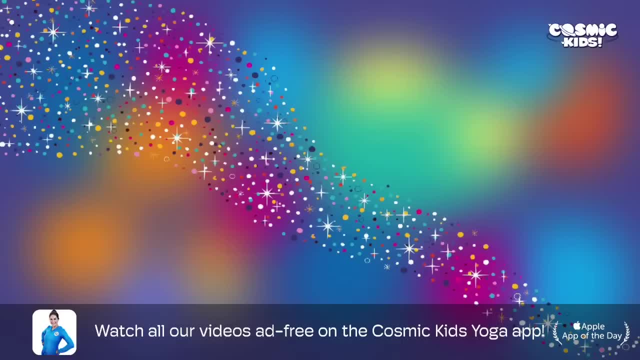 That's right, a pixie, A small, fairy-like creature. Think about how it looks. Does it have wings? What colour are its eyes? What's it wearing? It may be a girl pixie or a boy pixie, or an animal pixie. 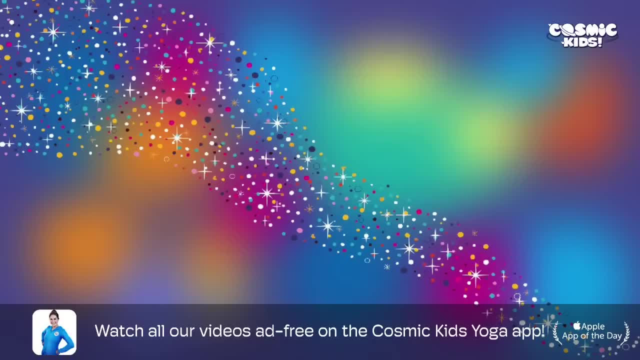 You decide how your pixie looks. One important thing, though, is that this friendly pixie- it's a good one. This pixie loves using pixie dust for tickling, Not the kind of wriggling, giggling and jiggling tickles. 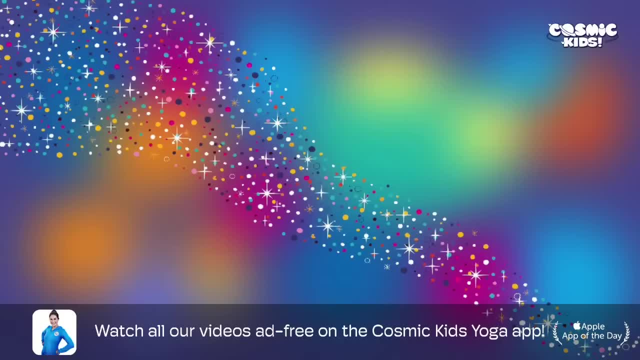 Just a light, fuzzy tickle, That kind of feel nice and relaxing. The tickle pixie sprinkles magic pixie dust on our body and we feel it because of the slight tickly feeling that happens where it's been sprinkled. Let's see if we can notice the feeling when the tickle pixie. 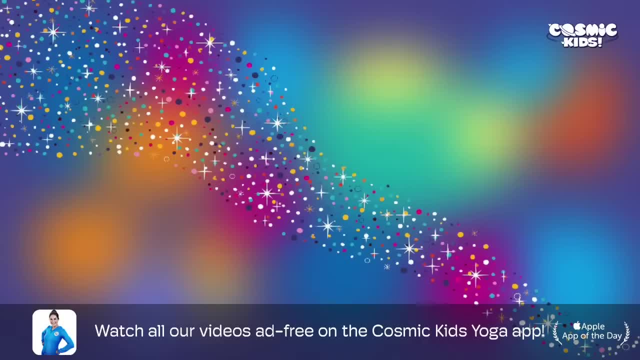 sprinkles the magic pixie dust on us, Ready. Okay, Let's be as still as we can and see if we can feel the little tickles. Here we go. The tickle pixie starts by sprinkling our feet. There's already a tickle pixie on our feet. 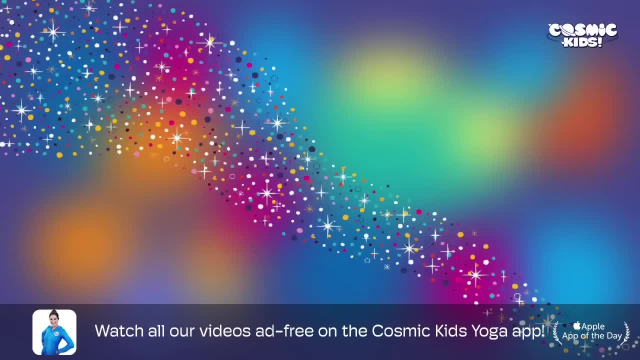 There's already a tickle pixie on our feet. There's already a little tingle in our toes. Can you feel it? A slight fizzy feeling. It's moving all the way up through our feet and around our ankles. The pixie moves up, sprinkling the magic dust on our legs. 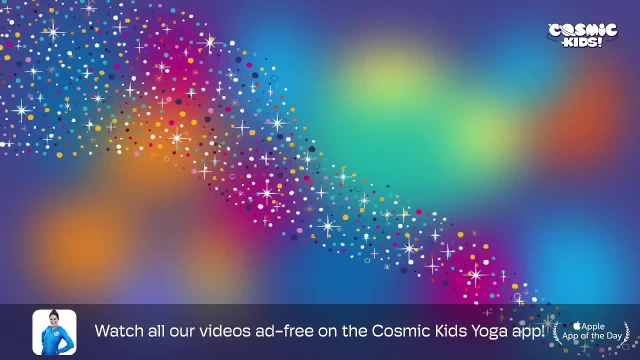 Ah, now the warm, tickly tingles are happening in our legs, moving up over our knees and into the tops of our legs. They feel all warm and sparkly. We begin to smile as we notice the tickly feelings. Now the pixie sprinkles the magic. 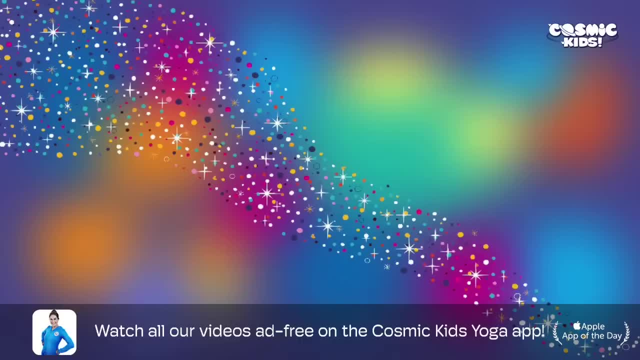 tickle dust over the middle of our body, our hips, on our tummy and up across our chest. Ah, now the pixie sprinkles, the magic tickle dust over the middle of our body. our body feels the fuzzy tickles, like we are full of twinkle lights. 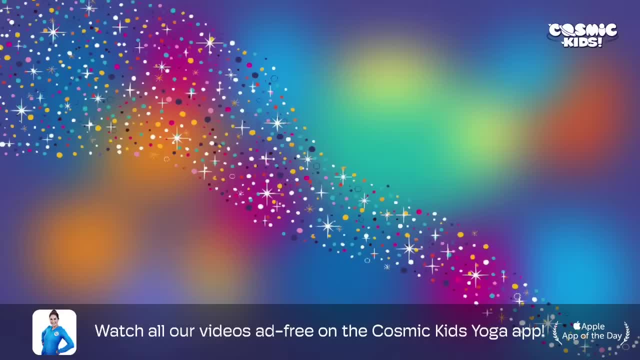 The tickle pixie carries on with the sprinkling. Now we feel the tickles travel all the way down our arms right to the very ends of our fingertips And now coming back up our arms again and over our shoulders. Now the fizzy feelings. 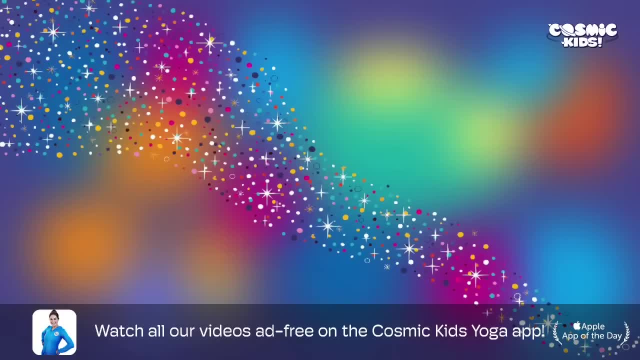 tingles through our neck and up into our head. We feel our face tingle with the tickly dust. It may even make our nose wiggle. Wow, what a magic feeling. Our whole body is tingling with sparkling, tickle pixie dust. 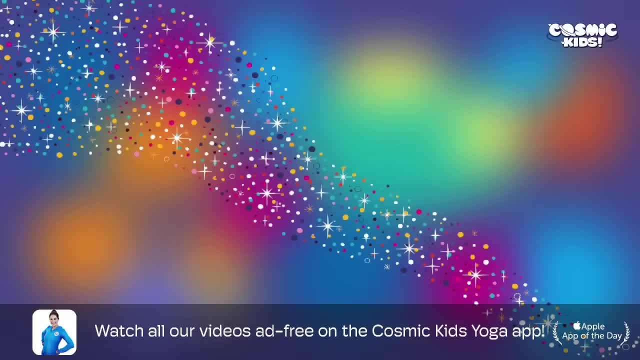 We feel fizzy and sparkly all over. The tickle pixie has done its job. You see it in your mind, smile at you And blow you a sparkly pixie dust. kiss goodbye. It disappears in a puff of magic dust. 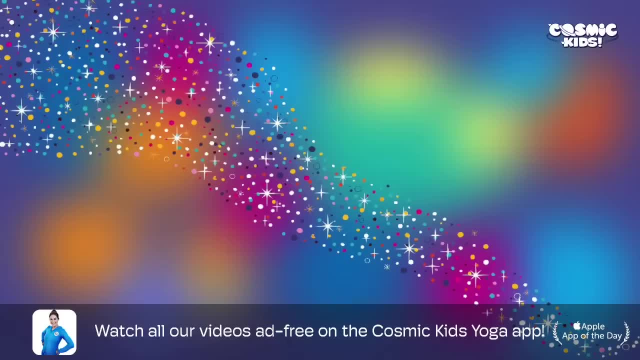 And the screen in your mind is once again blank. You smile, feeling happy that your body has felt the magic of the pixie dust and, without saying the words, you think: a big thank you to your little pixie. It's time to return now. We come back slowly. 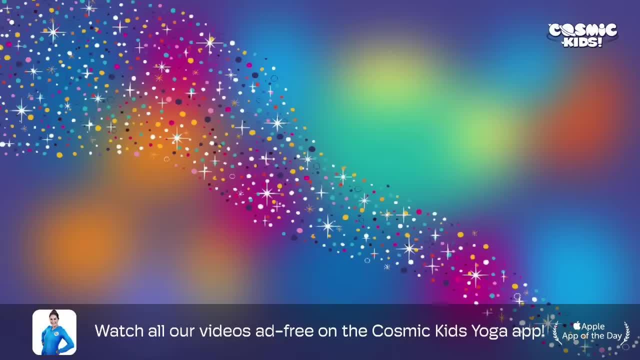 See if you can notice the sounds around. you Feel where your body meets the ground. Have a good stretch making your body long like spaghetti. Take a nice big breath in, Let your stretch relax and sigh out of your mouth. Gently open your eyes and now just say: 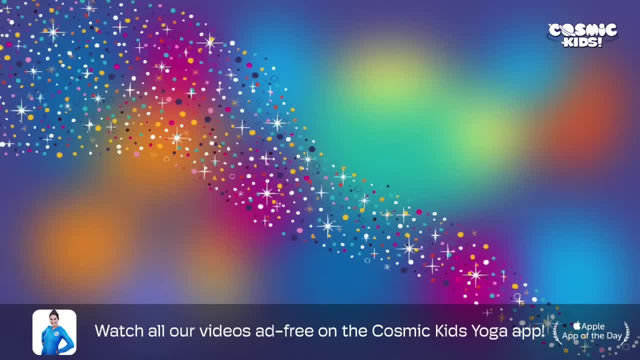 Sit or lie where you are for a minute. How was that? Having the pixie dust sprinkled all over you? Maybe you can still feel it a little. Well done for giving yourself this time to stop breathe and feel your body, from top to toe, tingly with magical, sparkling pixie dust. 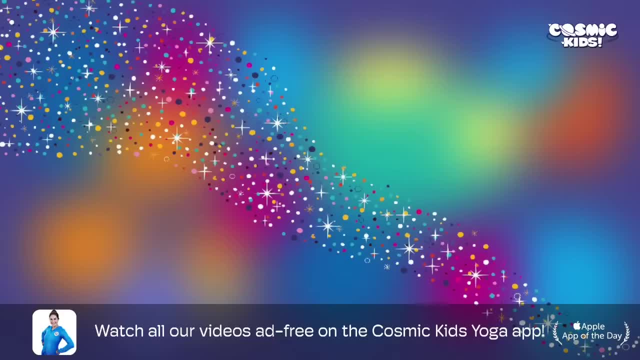 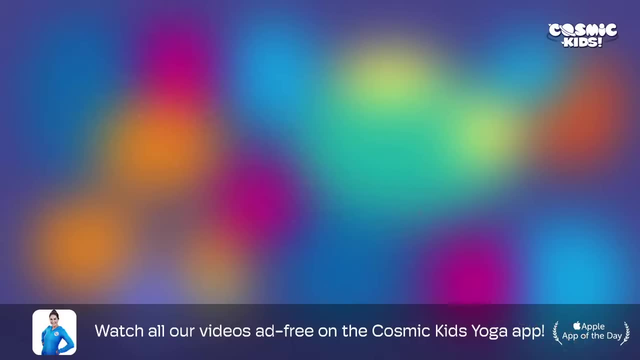 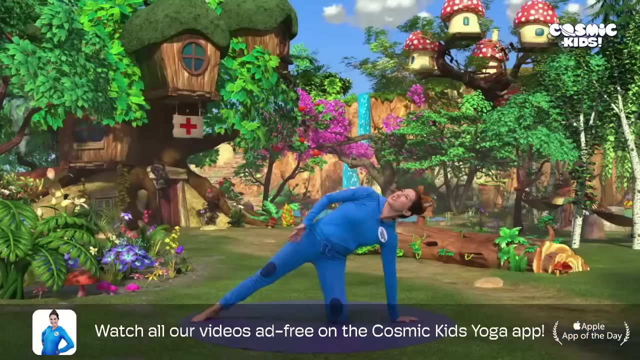 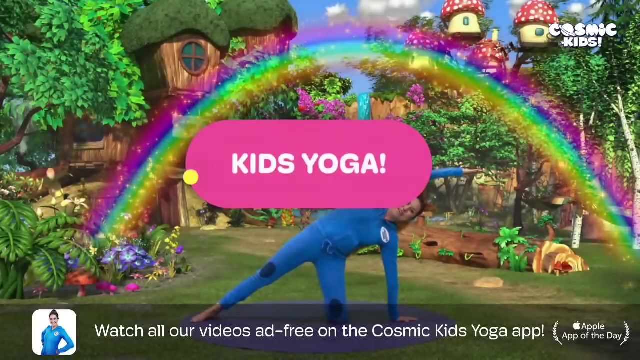 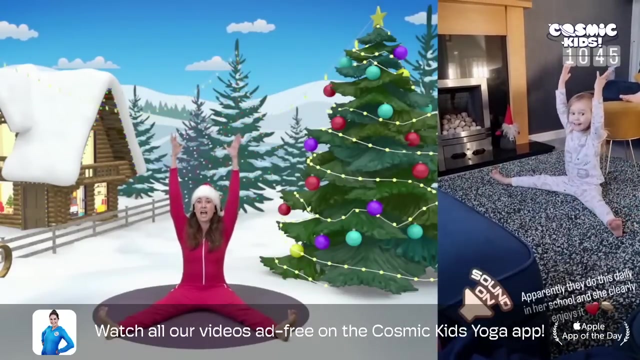 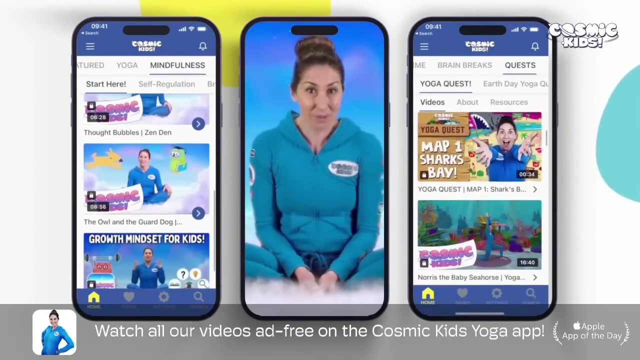 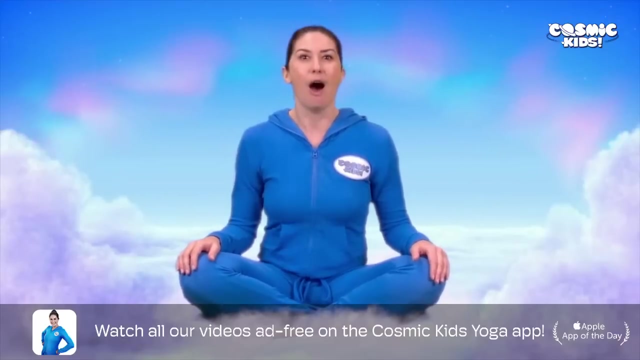 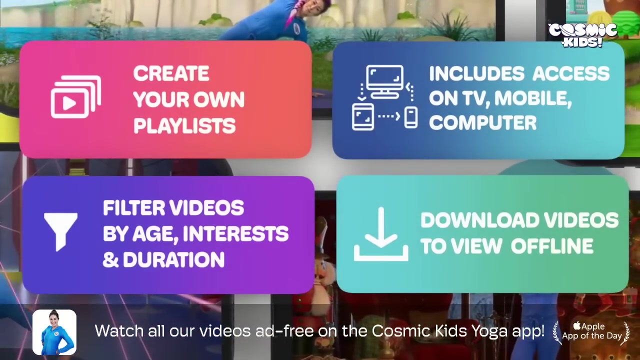 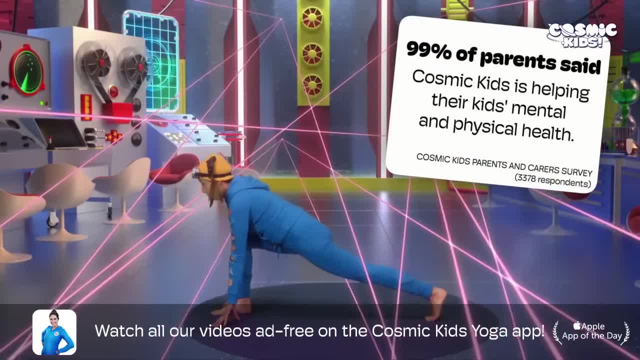 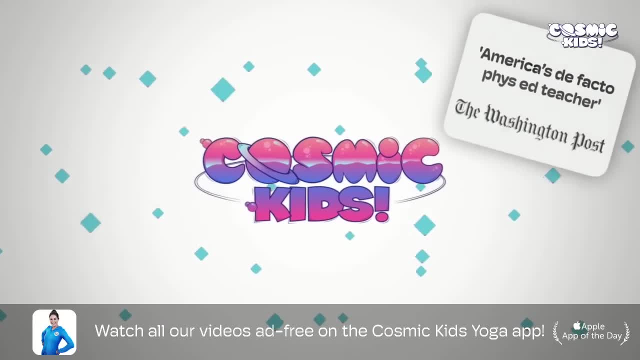 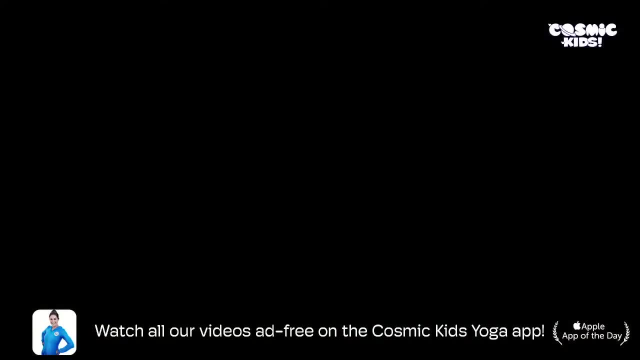 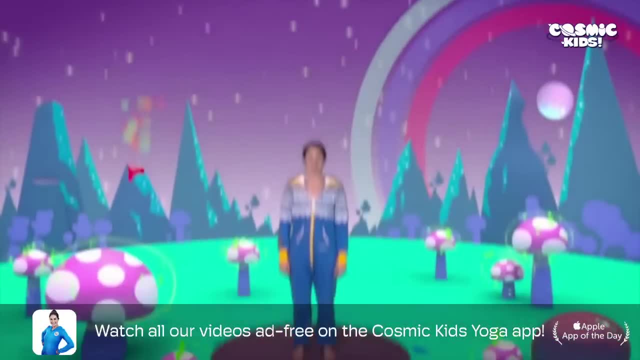 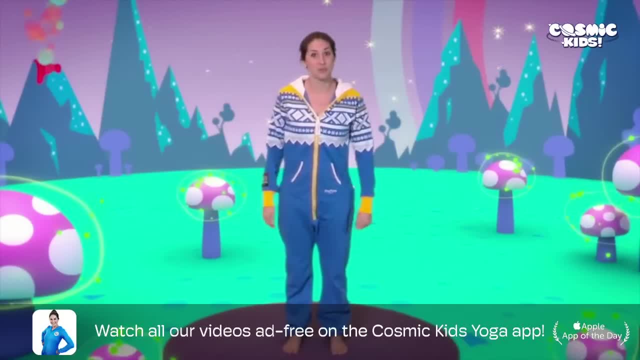 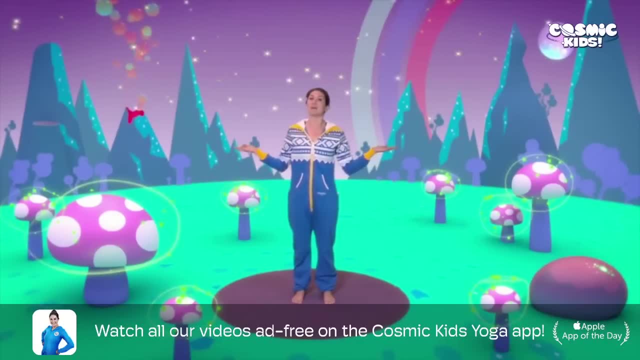 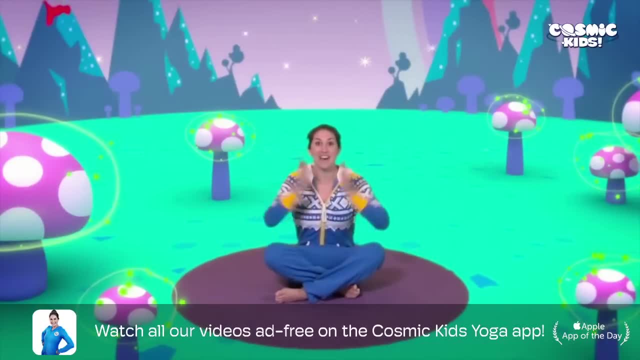 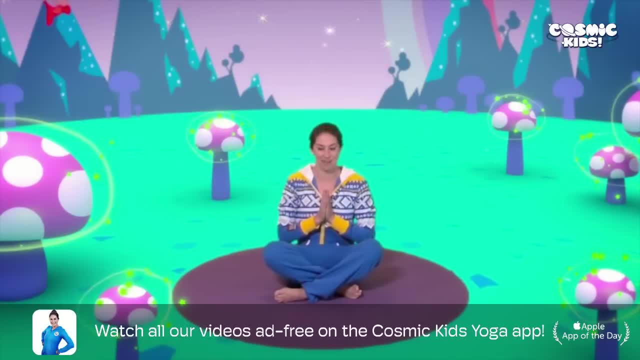 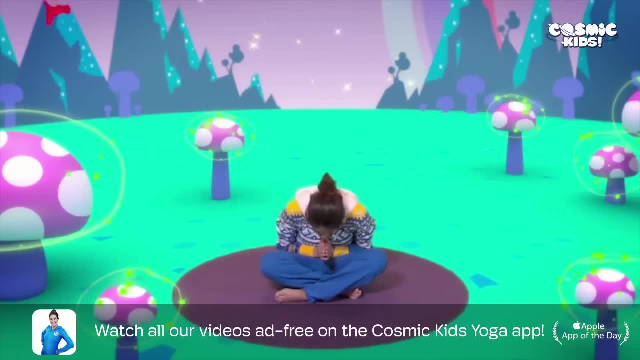 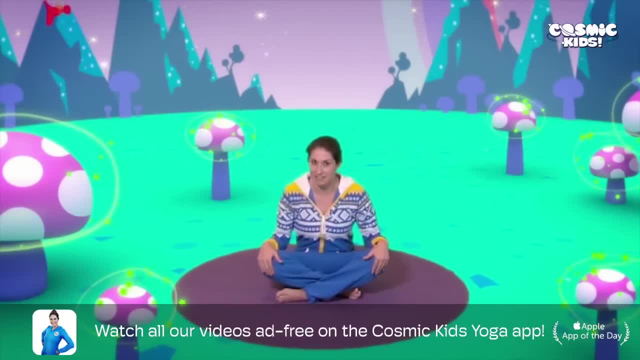 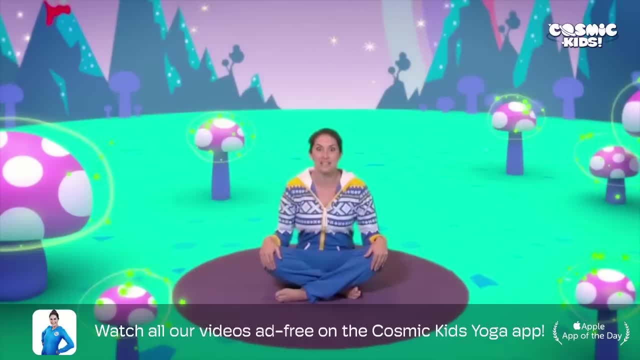 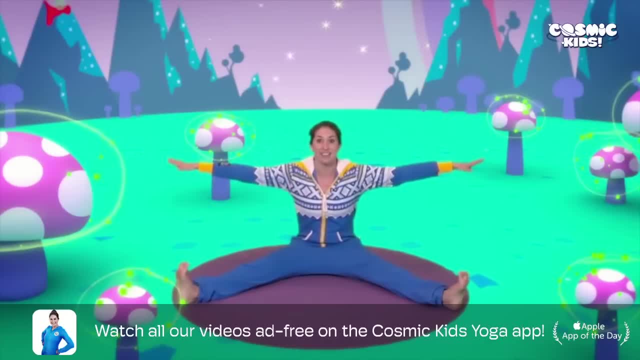 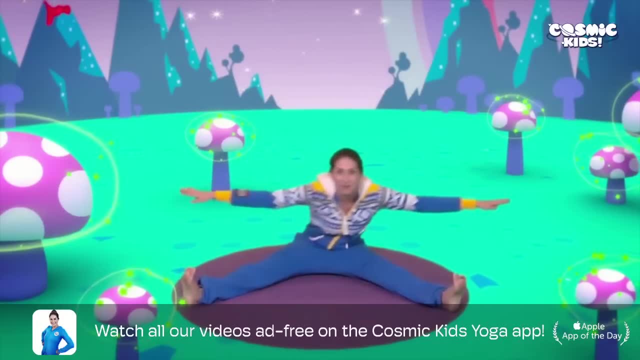 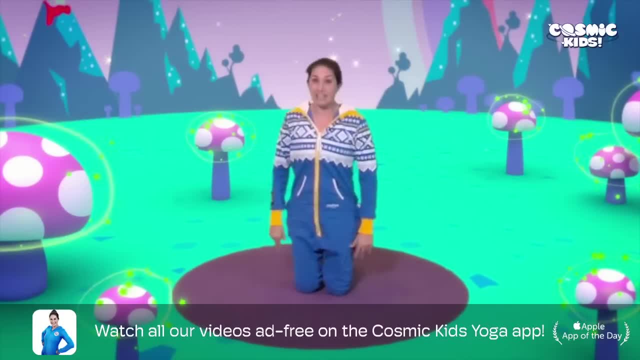 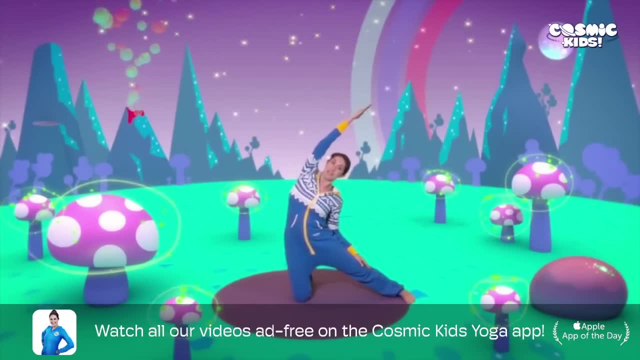 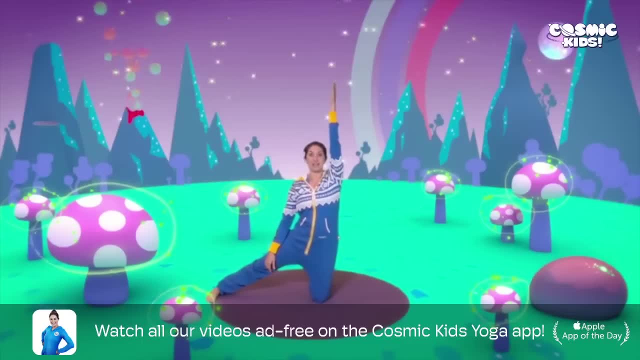 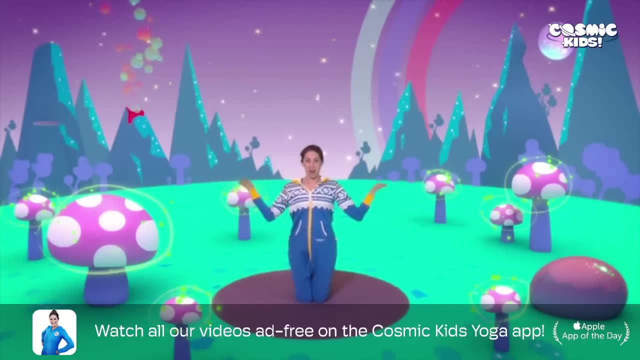 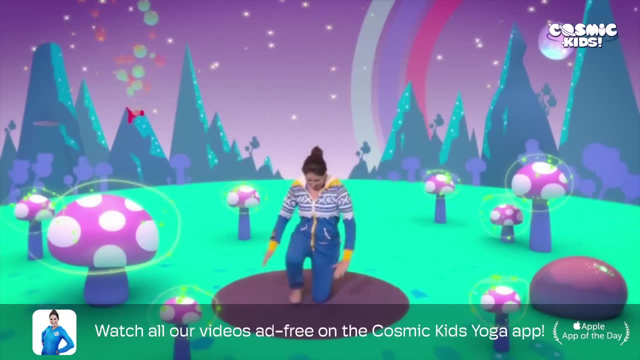 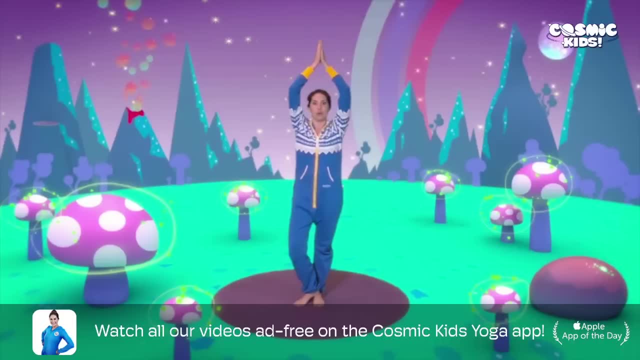 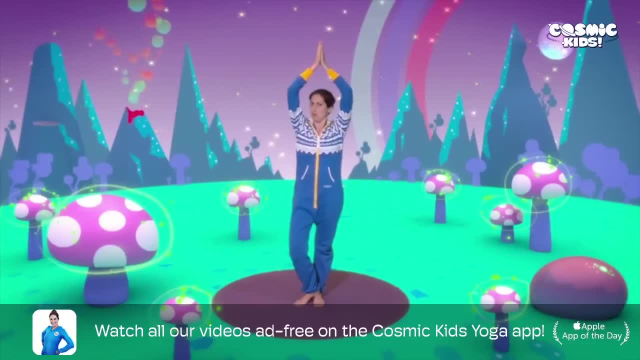 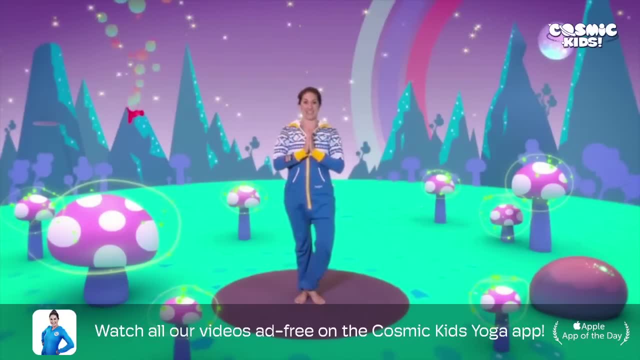 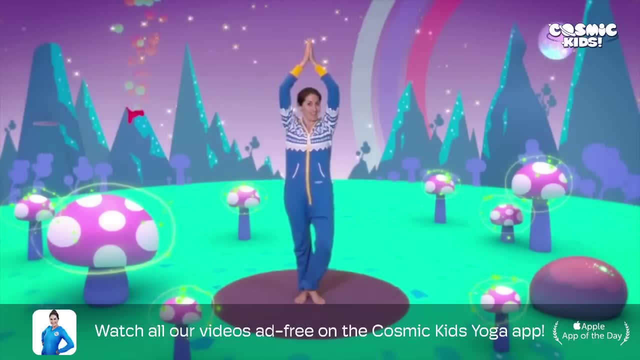 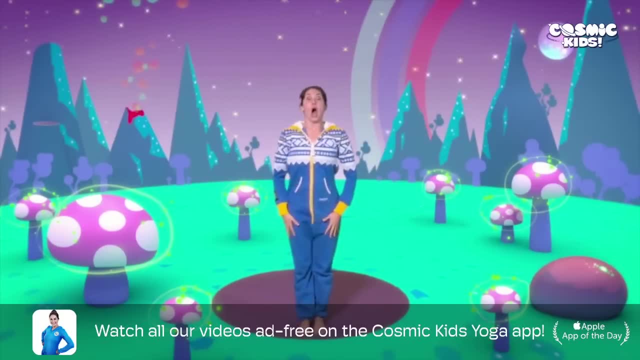 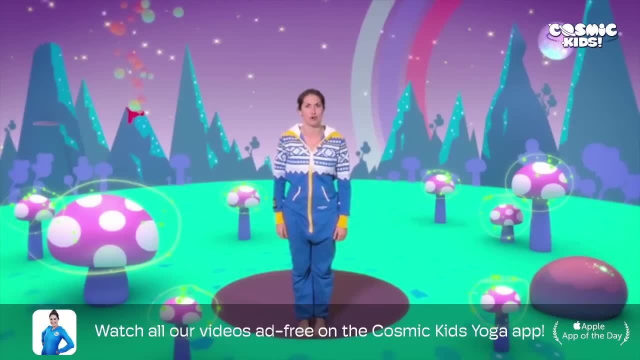 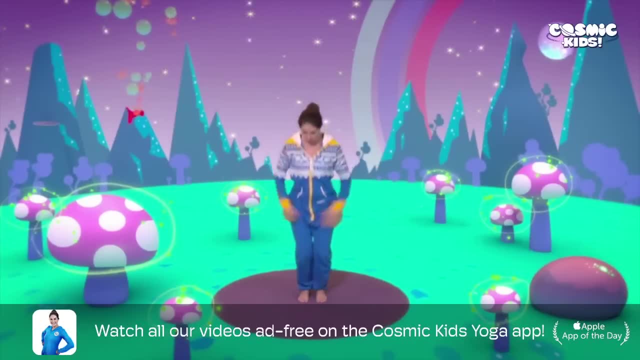 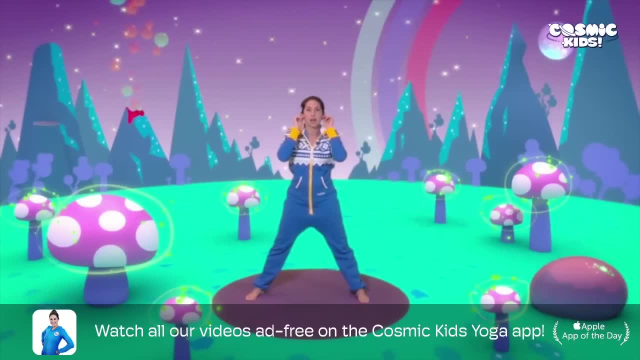 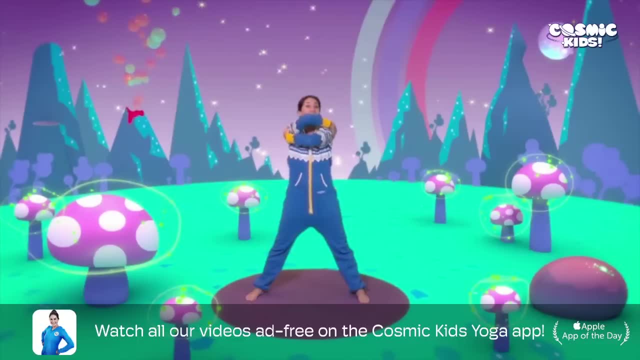 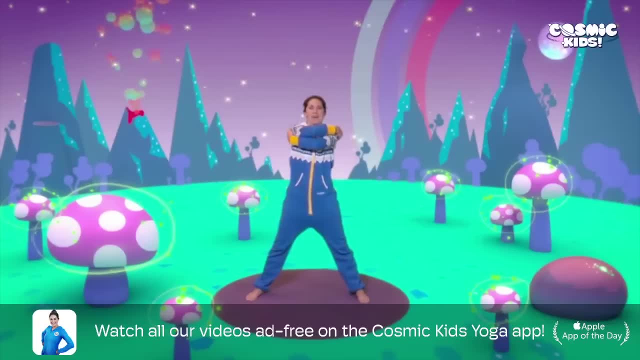 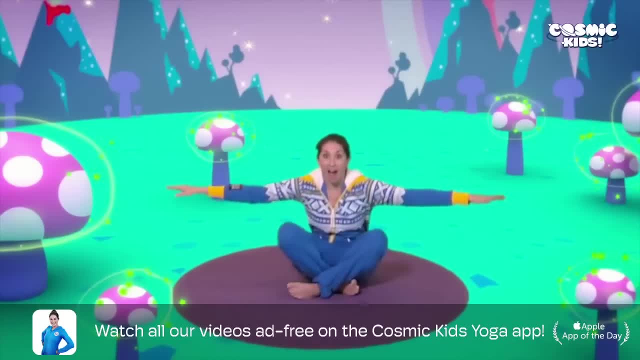 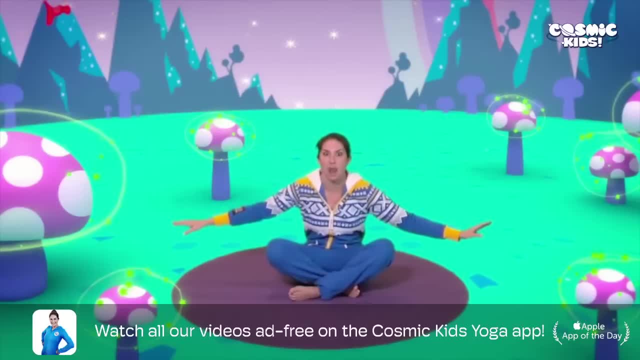 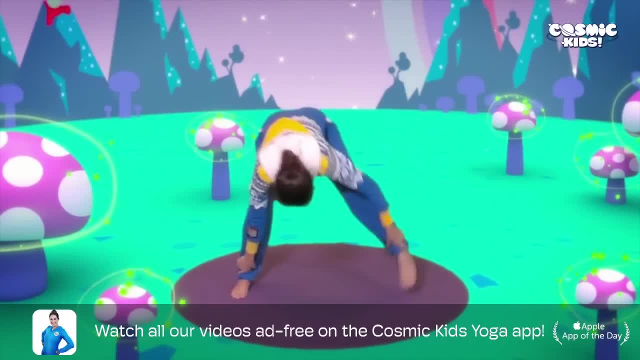 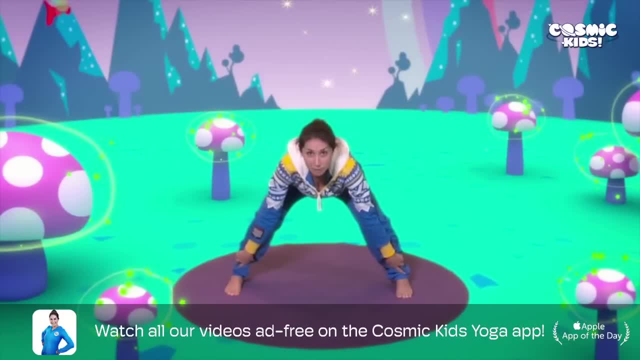 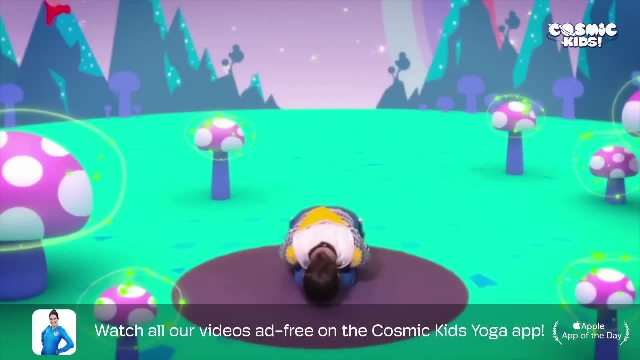 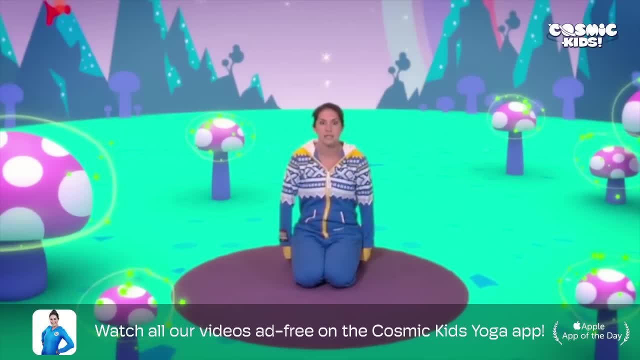 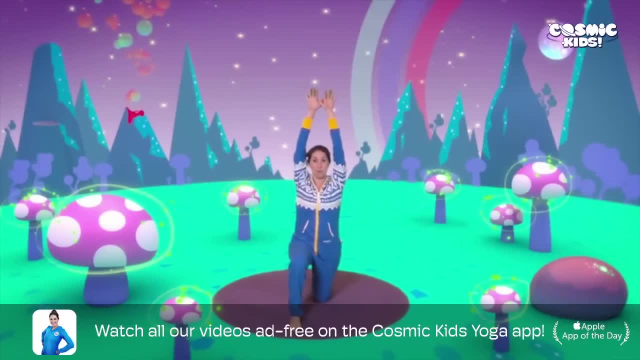 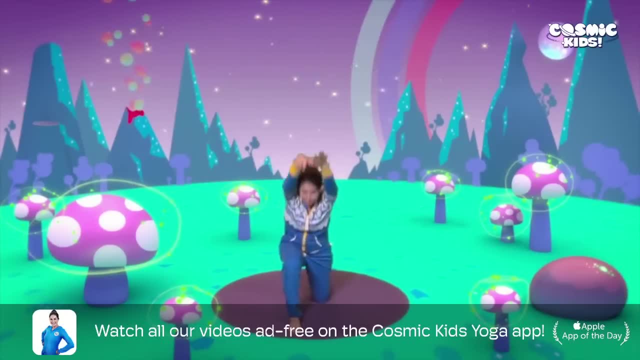 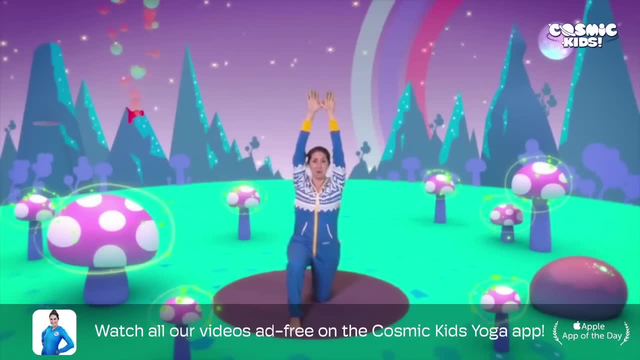 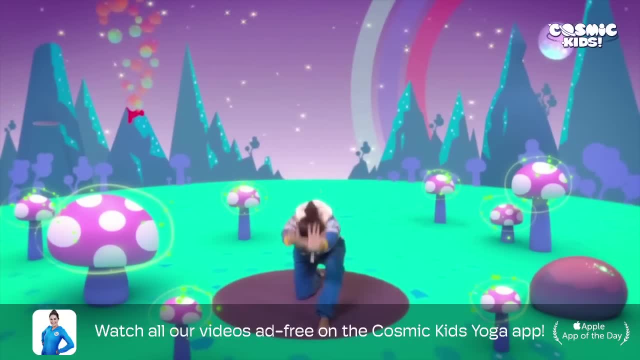 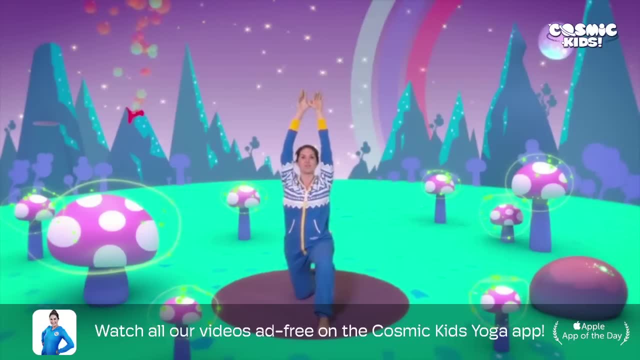 Subtitles by the Amaraorg community. And you must be my helper. Come on, we've got lots and lots of work to do. Wow, a real dragon. We can't wait, Let's get cracking. We hop onto Cracker's back. 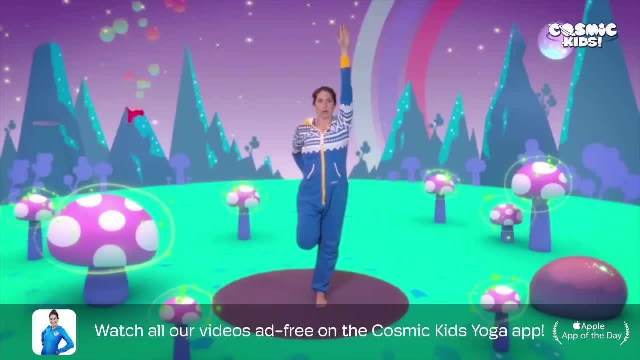 lifting up one arm, holding onto your foot and trying not to wobble. Now we go on with the other leg, lifting up the other arm, lifting up the other foot and, yes, we're on Bending all the way forward. 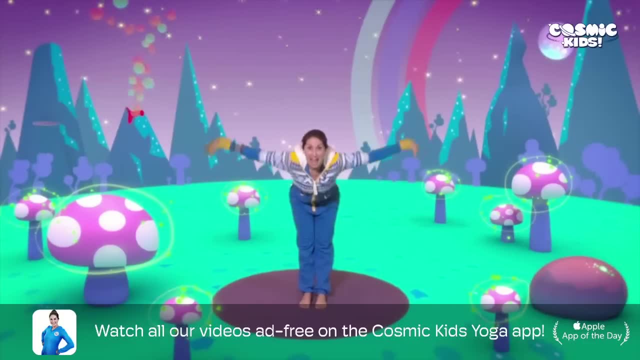 Cracker spreads his big, beautiful dragon wings and we're off flying up into that beautiful star-washed sky. It's amazing looking down from up here: The feathery trees, the amazing mountains. What a place We come to Cracker's cave. 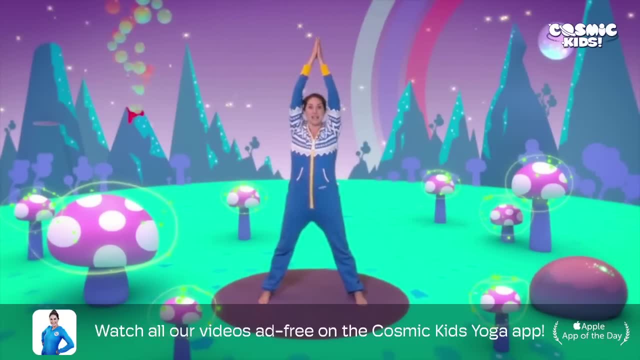 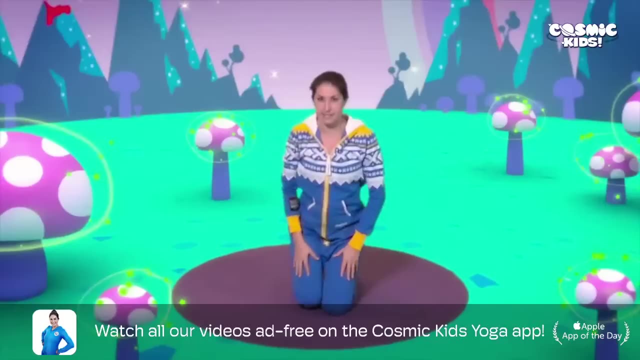 Jump your feet wide and bring your hands up above your head. Now it's very dark inside this cave and full of scary shadows Coming down onto your knees. some of the shadows look like lions. One, two, three, Rawr. 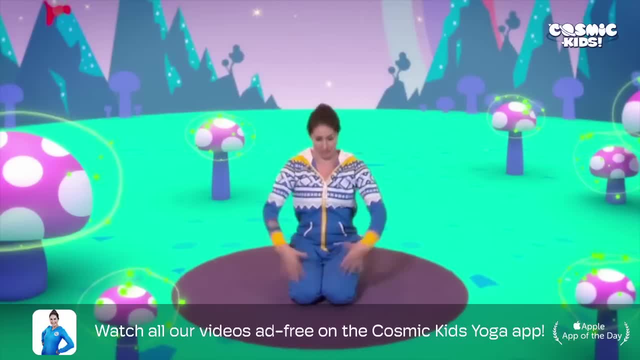 Some of the shadows look like tigers Coming onto all fours. claw your tiger paw and claw your tiger paw and swish your long tiger tail. Now, sometimes we might be afraid of the dark, but here, with Cracker, we're not at all. 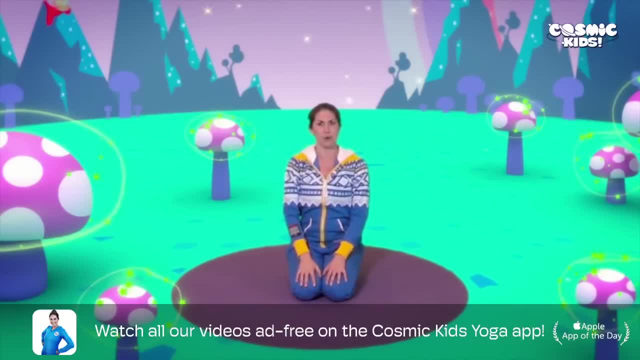 We're really excited. and the shadows aren't scary at all. They're really interesting and amazing. Cracker explains that to make the fireworks we need some ingredients. We need colours, sounds, magic and shapes. Right, we can't wait. 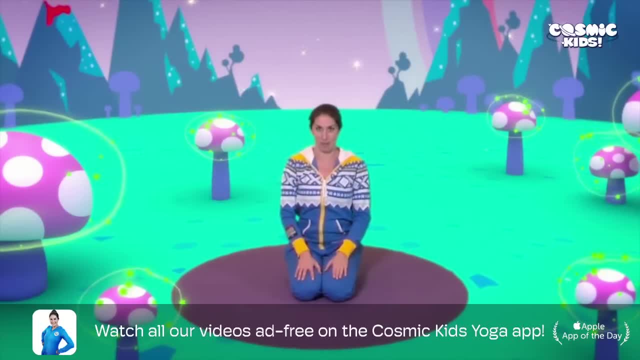 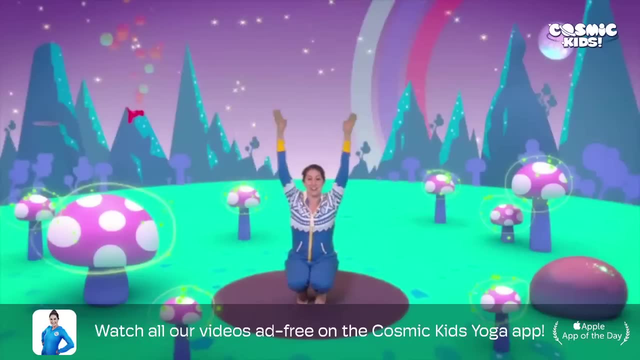 Let's go. First stop is the Whizbang Pop Shop to get the sounds, but we've got to tiptoe through the tulips. Coming up onto your tiptoes, crouching, lifting your hands above your head, Come and tiptoe. 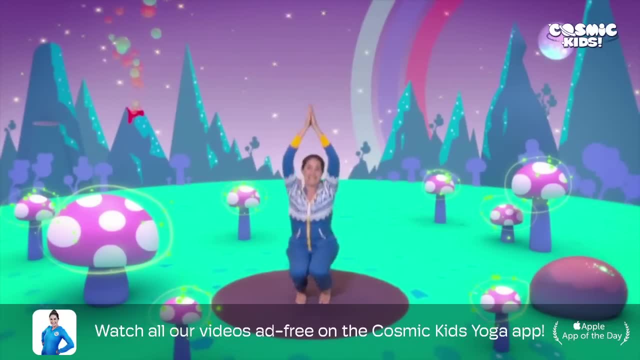 through the tulips. Come and tiptoe through the tulips With me. We end up in the Whizbang Pop Shop, which is incredible. It's like a big, squishy, giant bouncy castle And we boing, boing, boing, boing, boing, boing. 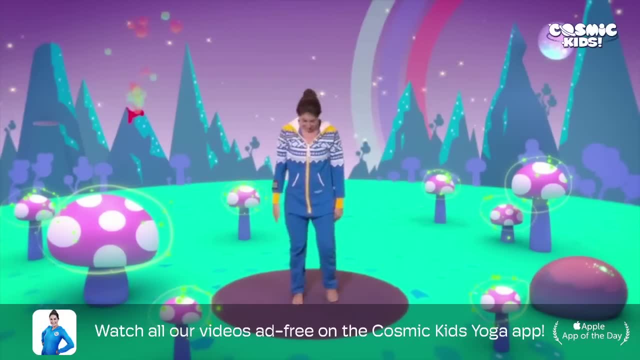 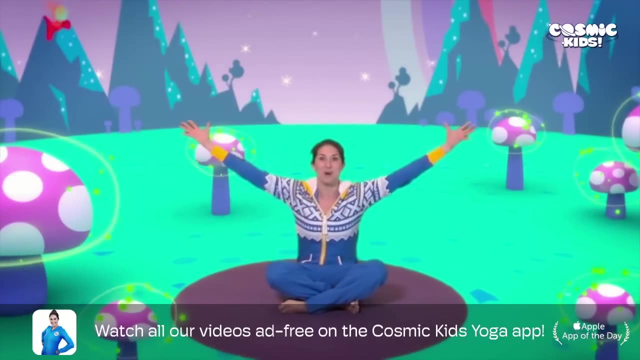 boing and bounce around, And all over it are floating lots of amazingly huge balloons. sitting on your bottoms, Take your arms out wide and float around like a big balloon. big balloon. Cracker explains that in each of the balloons is the sound for 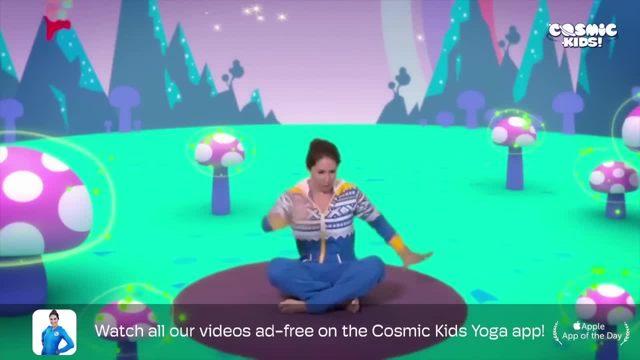 the fireworks. Wow, We can't wait to check this out. We twist this way and pop this one, and it goes bang. Wow, Let's try another one. We twist the other way and we pop this one, and it goes- whee. This is incredible. We get all the sounds we need. 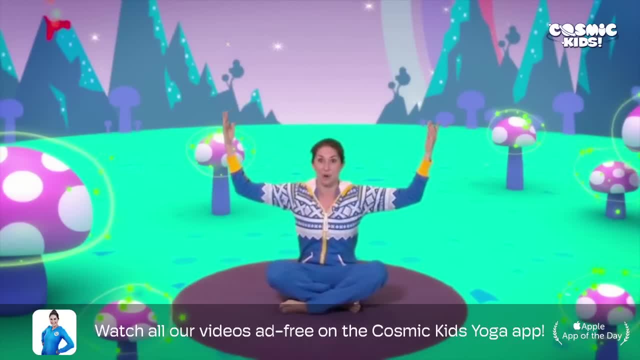 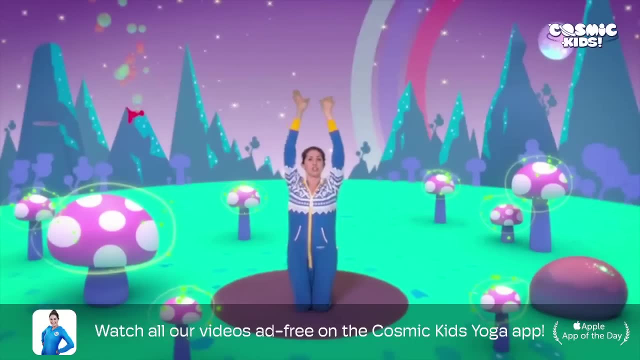 from all of these amazing balloons and we're off to the next stop, The rainbow roller coaster for the colours Coming up onto your knees. Cracker says let's get on. So we get on. We lift our arms up, up, up, up up as the rainbow climbs up and over, and then we. 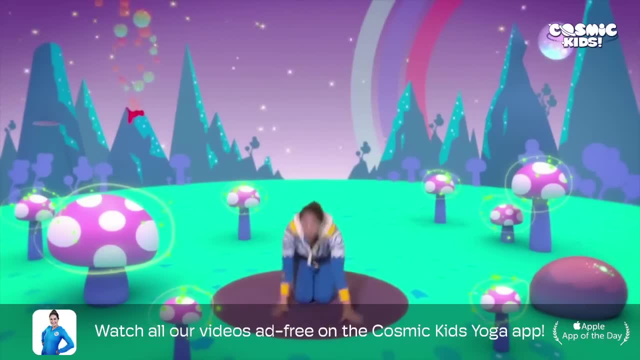 whoosh down really fast. We go over to one side- Wow- And over to the other side. Then Cracker shows us how to surf, Surf on the rainbow roller coaster, putting one foot in forwards and one foot back, Cartwheel our arms around and whoosh. 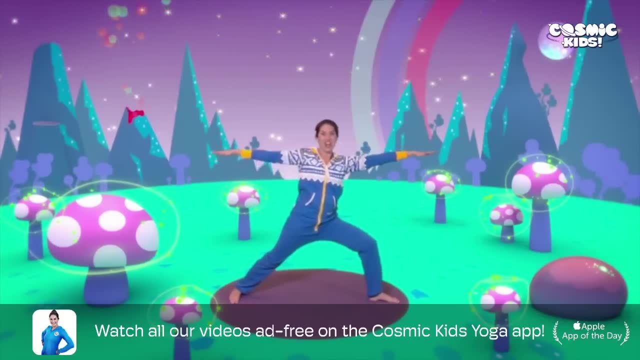 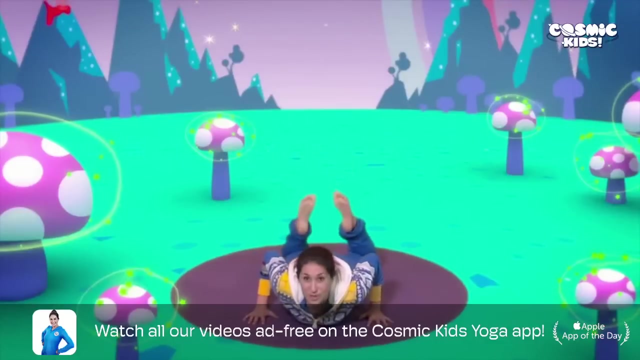 This is great fun. We even do it the other way. Whoosh, What a ride. At the end of the rainbow is a ginourmous pot Lying on your tummies. flick your feet towards your bottom and take hold of your ankles and lift yourself up. The pot is swirling with the most beautiful 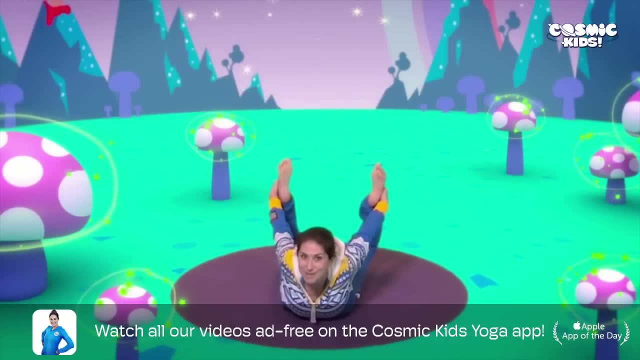 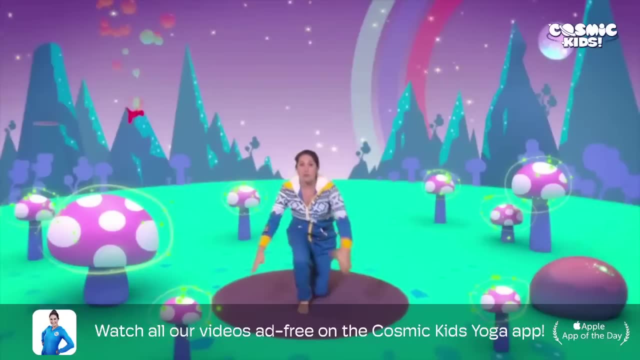 beautiful, vibrant colours. We've got all the colours we need here for the fireworks. Now for the shapes. It's up on Cracker's back again and we're flying up into that beautiful sky towards the cloud. Now, every cloud is a different shape. Some of the clouds: 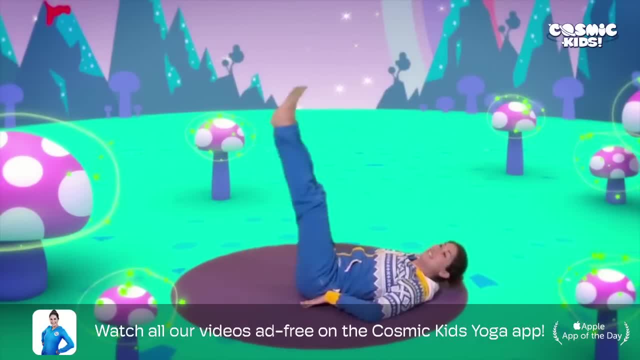 are like candles, all tall and straight, lifting up your legs, lying on your back. Some of the clouds are round and spinny, like wheels, Wheeeee. And some of the clouds go whiz, pop, whiz, pop, whiz, pop. Wow, we've got all the shapes we need here. We collect them all and 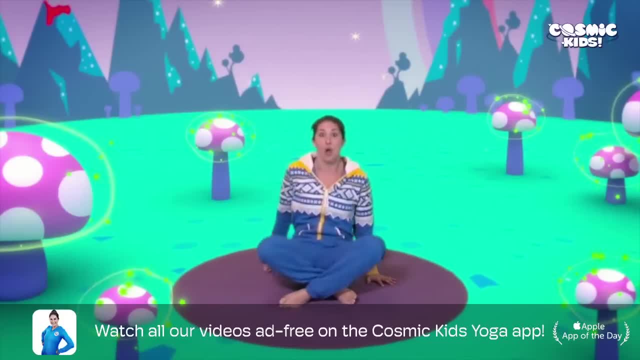 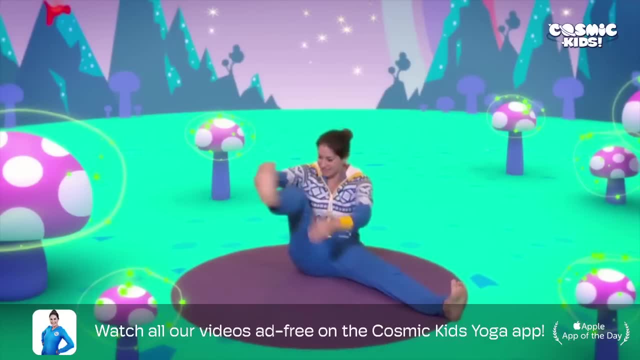 That's all the sounds. Now we take the other special stick and we stir in the colours. Stir it, stir it, stir it And finally, taking both together, we stir in the shapes, Stir it, stir it, stir it. 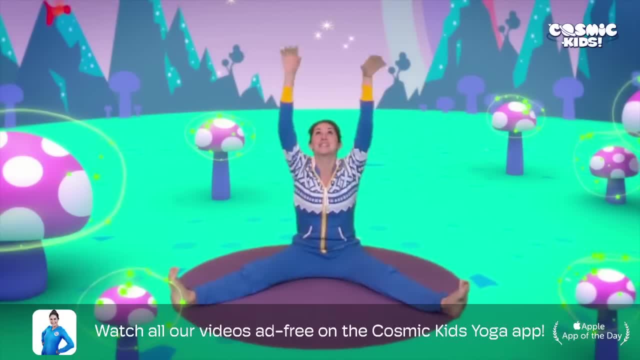 Now for the magic Legs out wide. sprinkle in your magic and make your special firework wish. Hands together, One, two, three. Cracker breathes his fire into the fireworks. And now it's time for the big test: everyone to see the fireworks working, Coming into. 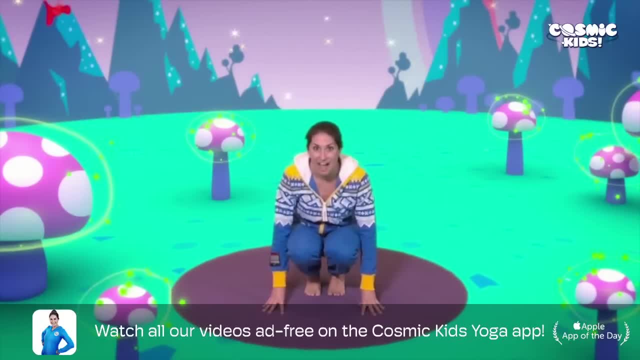 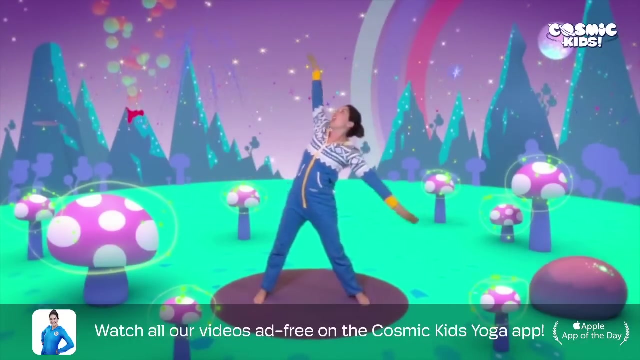 a little crouch position. let's count down from five and keep very still. Five, six, five, four, three, two, one, Whoosh, Wow. The colours and the light and the sound and the shapes are amazing. We look. 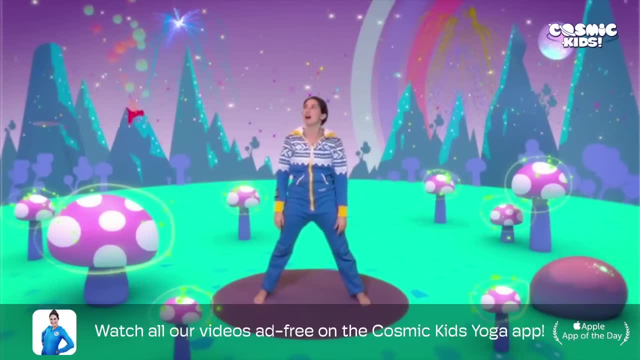 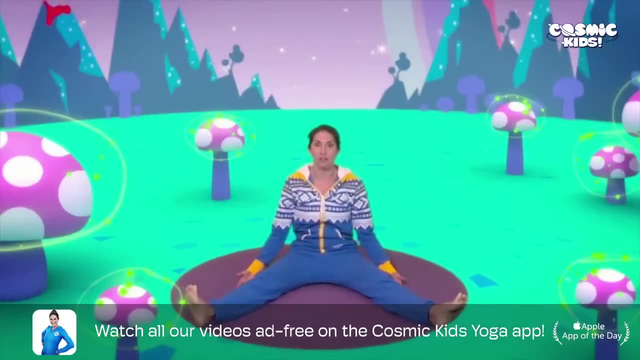 up and we are full of awe and wonder. We float back down to earth And when we sit down on our bottoms we find we're sat in our own bed. We're sitting on our own bed. We're sitting on our own bed. 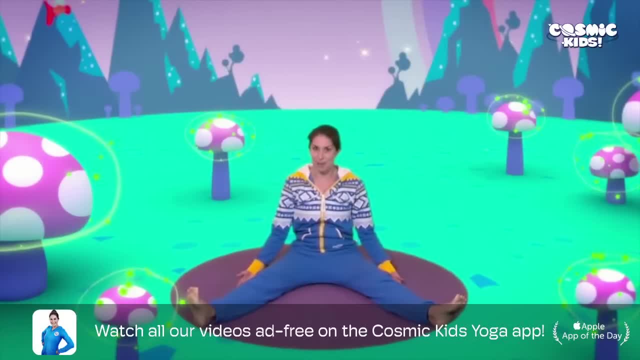 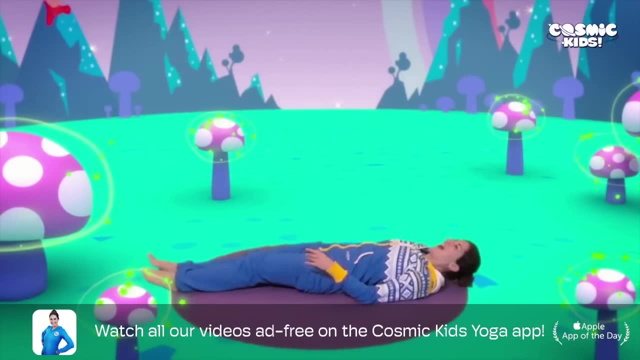 We're not ready to say goodbye to Whiz and Cracker, though, yet, So we lie ourselves down and we close our eyes and we're back there in that wonderful, beautiful sky, with the stars that sing, that zoom, and those beautiful fireworks that fill our minds. What an amazing. 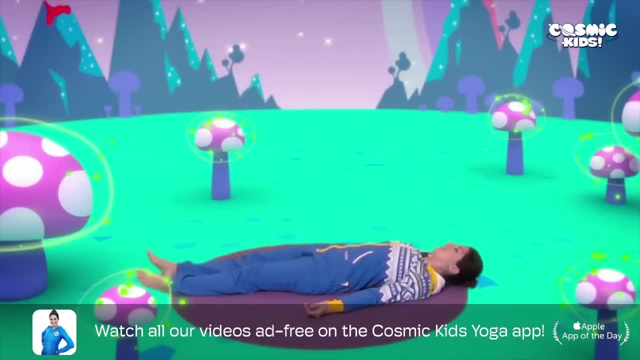 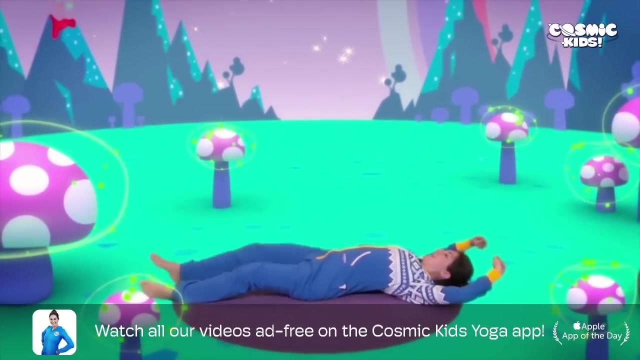 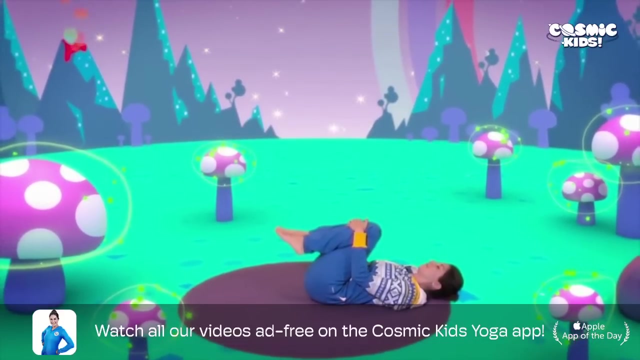 adventure. With every breath we glow a little bit brighter, Like a brighter firework. Thank you, cracker. What a great adventure. We flicker our toes, We flicker our fingers, We stretch up nice and tall And we bring our knees into our chest and have a little cuddle with them. 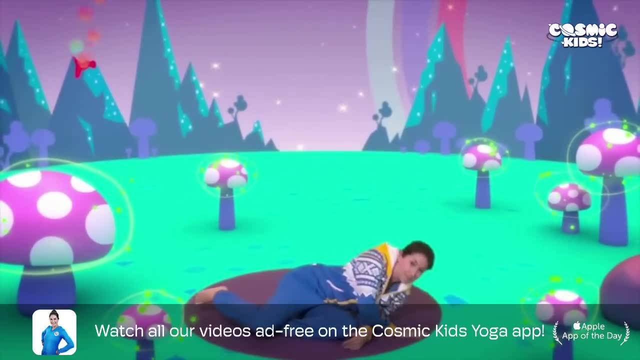 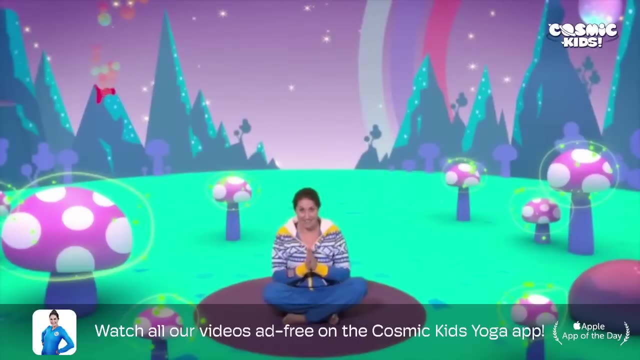 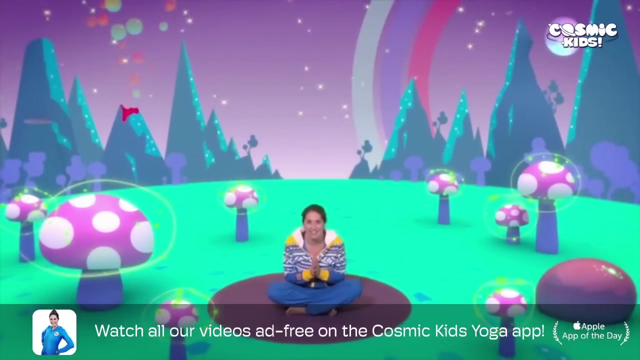 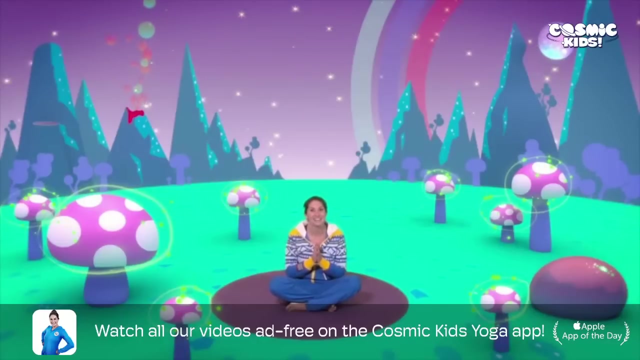 We roll over onto our side and come up to sitting with our legs crossed, Just in the way we started, With our hands together at our hearts, And we finish with our special magic yoga code word: Namaste, Ready After three. One, two, three, Namaste. 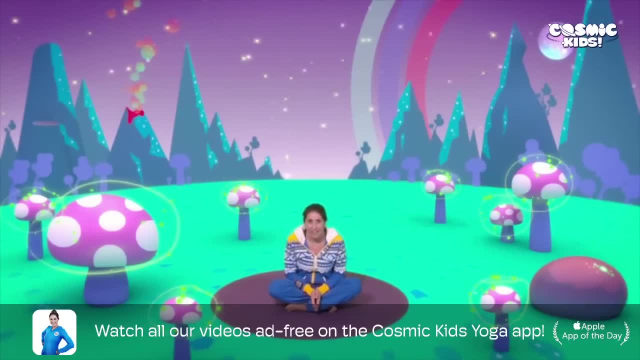 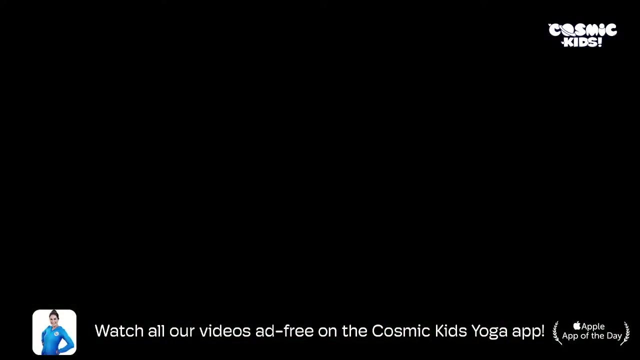 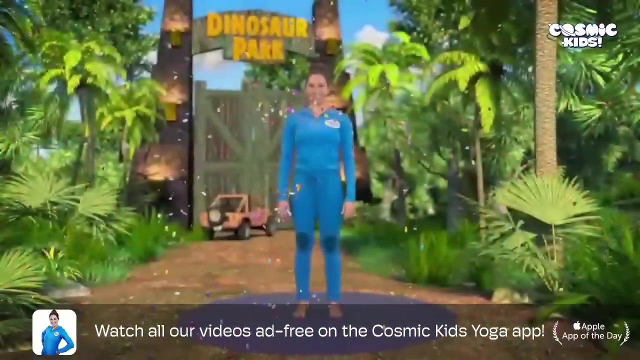 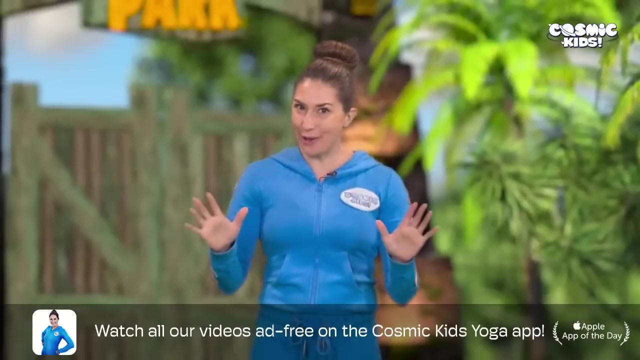 Well done everyone. That was amazing. Thank you for coming to Whiz with me and for meeting Cracker. He loved it. I hope to see you again for another Cosmic Kids adventure. Bye, bye, Hello everyone. Welcome to Cosmic Kids. I'm Jamie and this is your place for yoga. 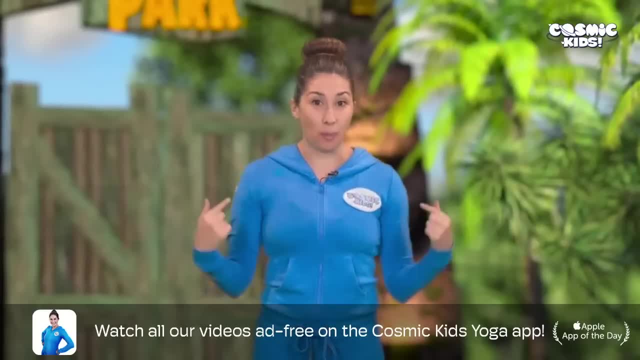 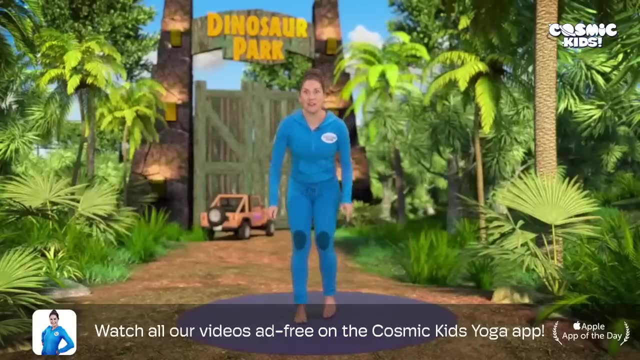 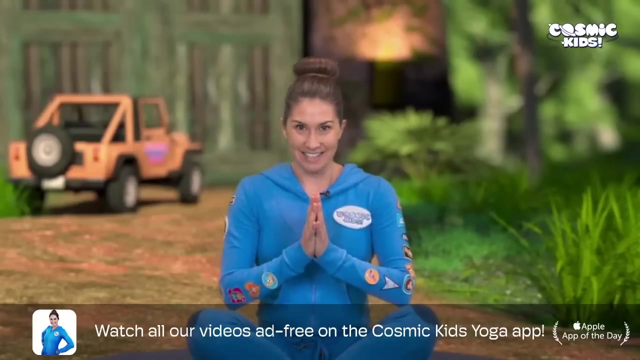 stories and fun. It's easy: Just copy the moves I do and enjoy the adventure. Now, we always start in the same way And that's by sitting on our bottoms, crossing our legs and bringing our hands together at our hearts And today saying our secret Jurassic dinosaur yoga code word which is Namasaurus Ready. 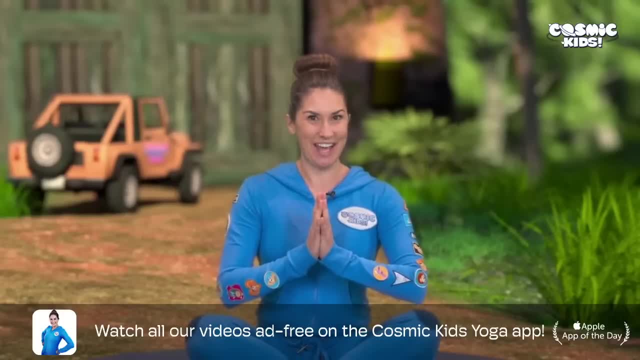 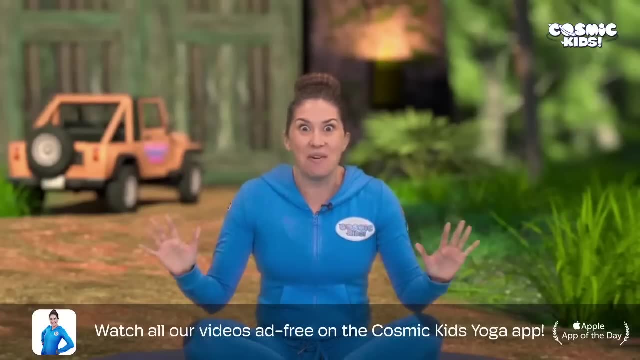 After three, One, two, three Namasaurus There. Now we're ready to begin And, as you can see, we're in a rather special park today where we might meet some dinosaurs. I'm sure we'll be okay. Apparently, it's very safe. Before we go in, let's begin by 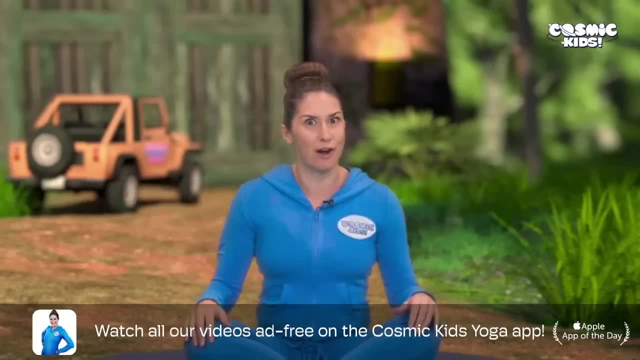 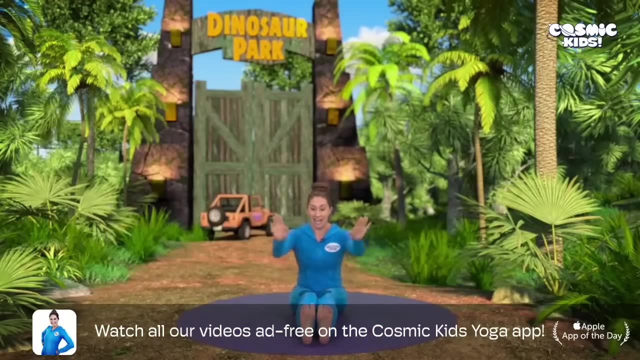 packing ourselves a backpack with everything we need for our visit, Taking our legs out long in front of us, wiggling our toes a little bit, bending our knees and touching our toes. We open up our backpack by lifting our arms. We take our arms out nice and wide and we 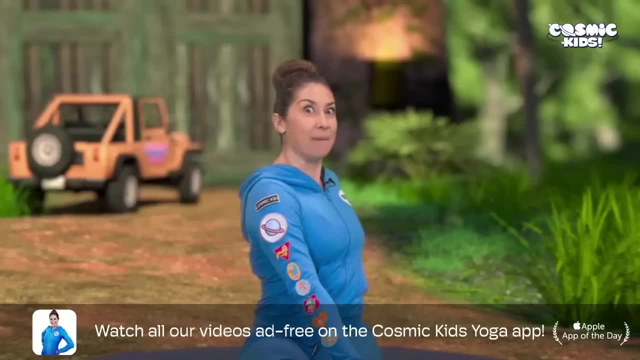 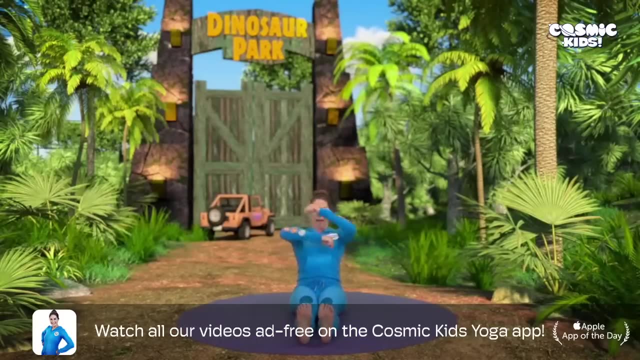 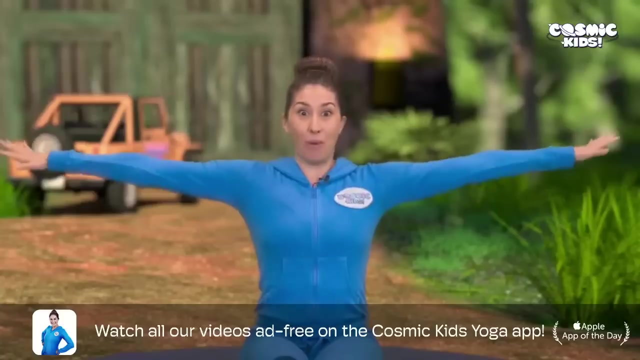 twist one way to get ourselves somewhere. We're going to start with some sandwiches, Getting our sandwiches, bringing them to the front and let's wrap them up. Wrap up the sandwiches and pop them in the backpack Arms out wide again. We twist the other way now and we get ourselves something nice to drink. 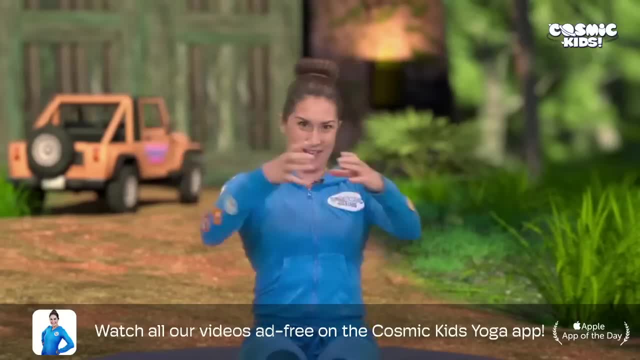 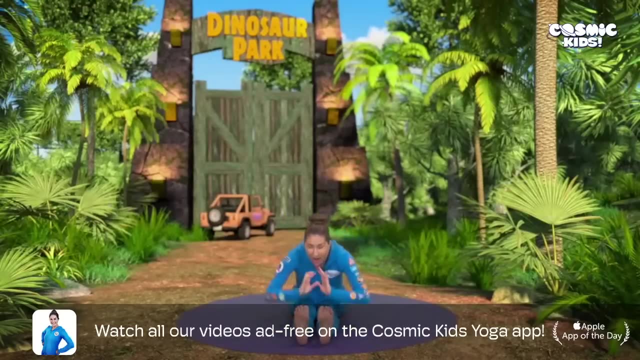 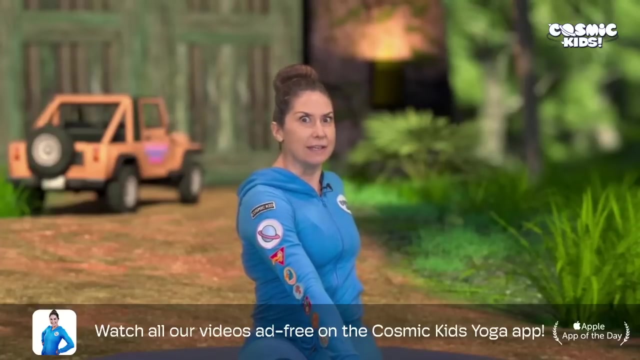 Some water. You can't go wrong with water. Get your water, bring it to the front, check the lids on and pop it in the backpack. We twist the other way now and we get ourselves some binoculars. We might want to see the dinosaurs. 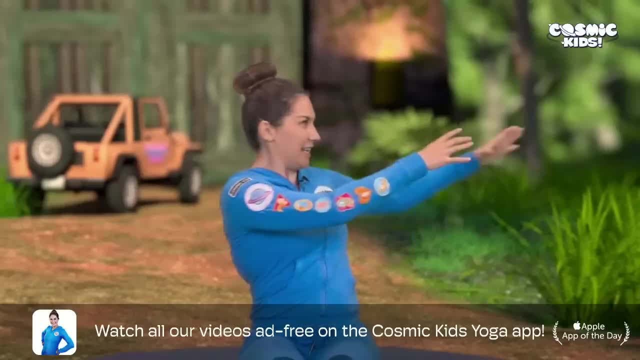 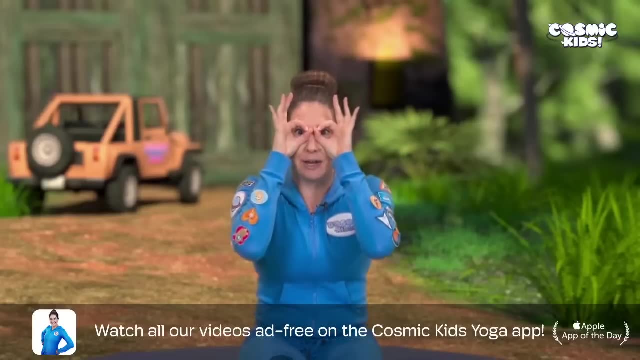 close up from far away. So we get our binoculars, Let's check they work, Joining our thumbs and fingers together, pop them on. Look, you're very close up when I pop these on. Let's see if we can put them on upside down. And what happens then, Turning our hands upside down. 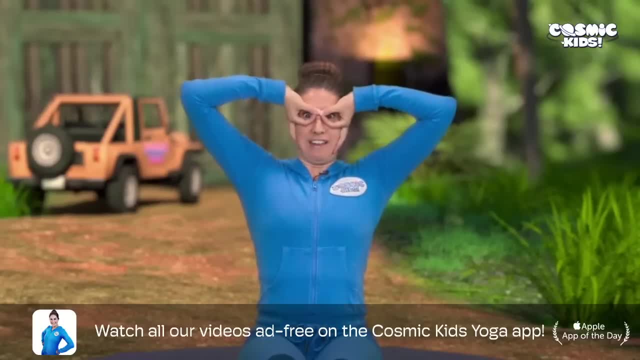 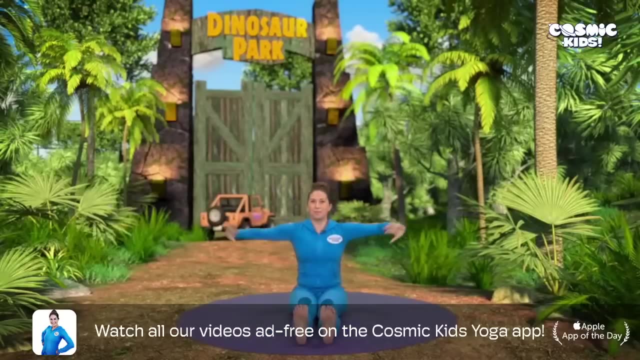 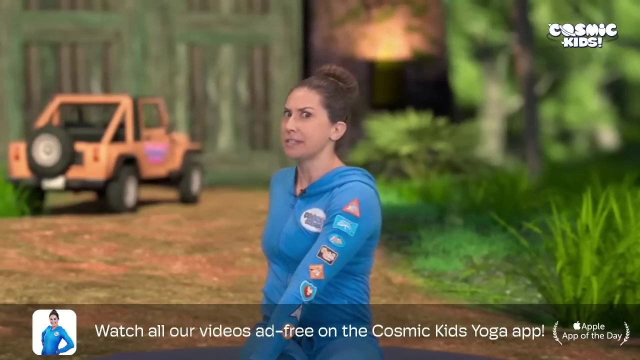 to pop them on, And we twist the other way. Oh, you've gone really far away. now Let's put our binoculars in our backpack Arms, out wide again. We twist the other way and let's get our emergency escape card. Just. 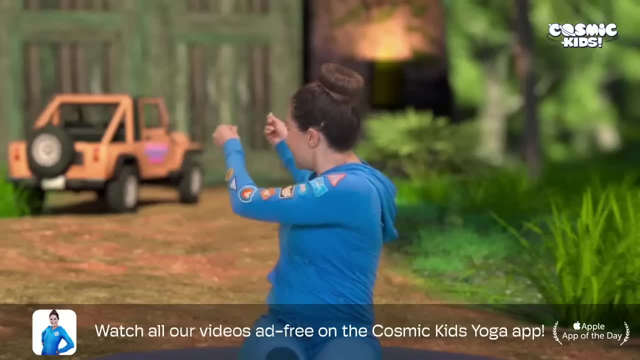 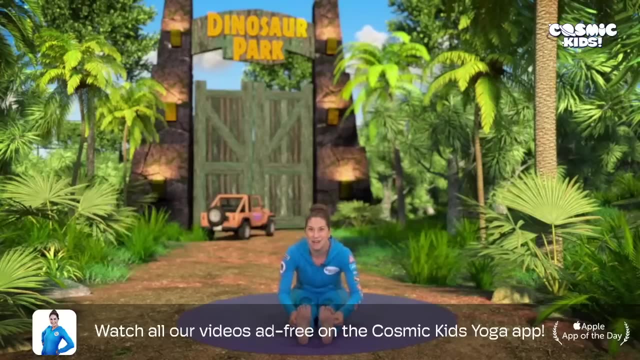 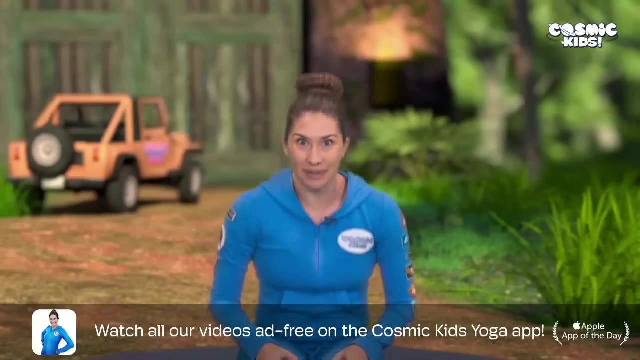 in case we want to go home quickly, Getting our emergency escape card and putting it in the little zip in the top. There we go, Reaching our arms up high, bending our knees a little bit and folding forwards to close our backpack. very good everyone. now let's take a ride in the jurassic jeep and go into the. 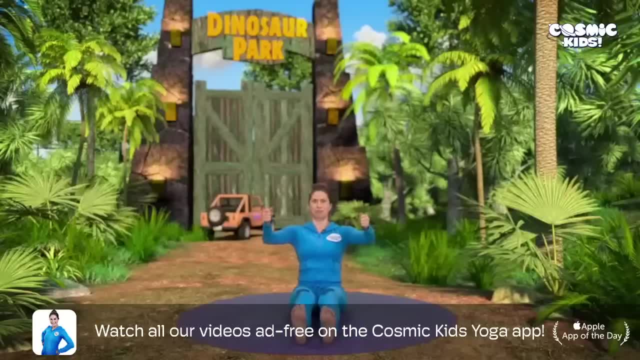 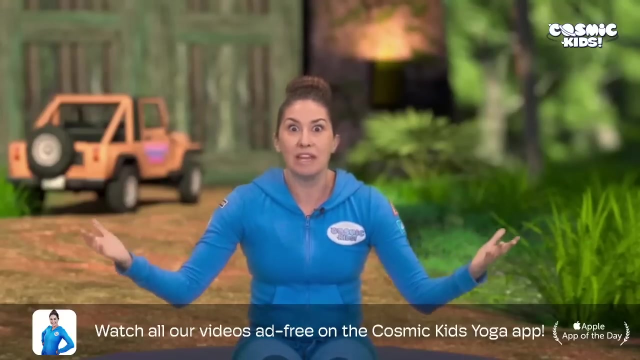 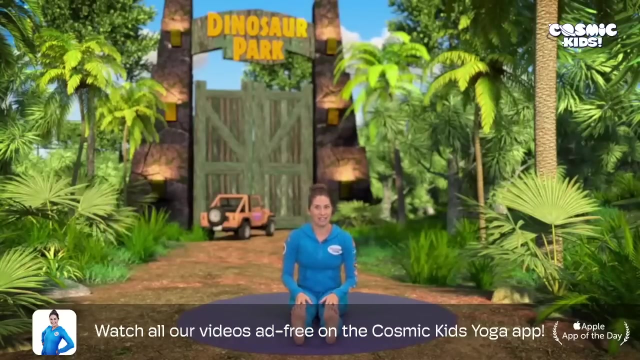 park. let's start our engines. we're going over to one side. we're going over to the other side. we're going down the hill. we're going up the hill, we come to a stop and we've arrived at the most majestic, enormous gates. let's do our gate pose. 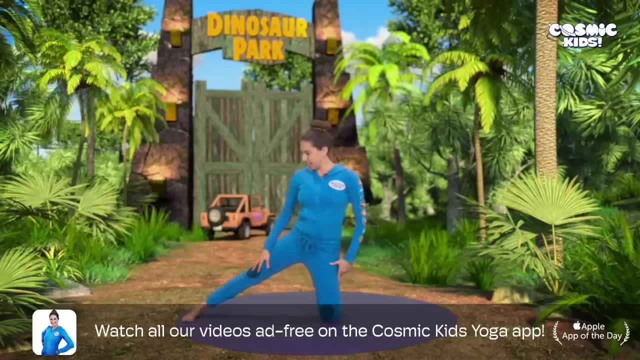 coming up onto two knees everyone. we take one leg to the side and our other arm to the sky. now we open up one gate, leaning to the side, coming all the way back to center. now we need to do the other side, two knees together, leg to the other side, arm to the sky, and let's open up this side. 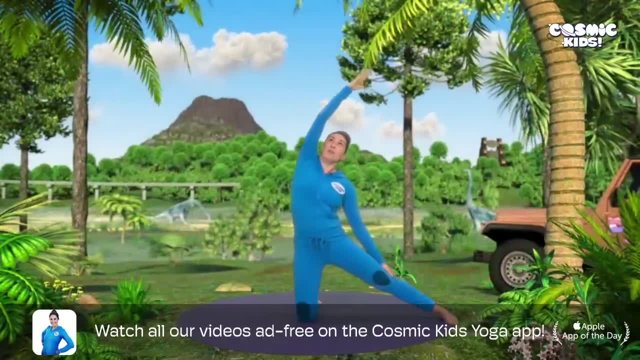 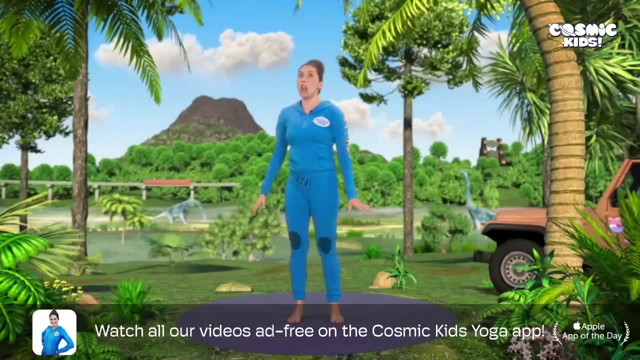 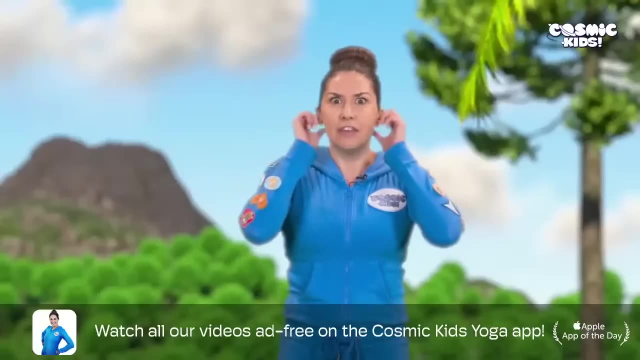 wow, look at it inside, coming all the way up to centre and all the way up to stand. Wow, It's so lush and green in here. It's amazing. Can you hear that Giving our ears a rub? Goodness me, that's a funny sound And look. 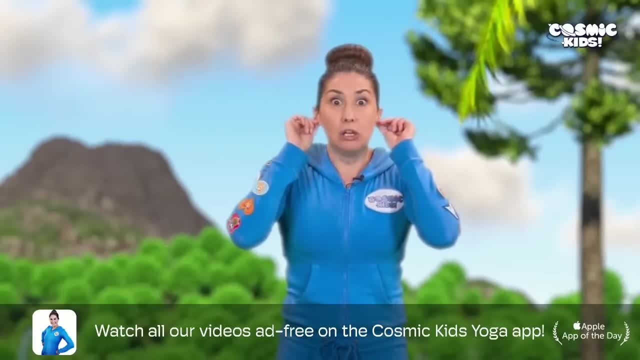 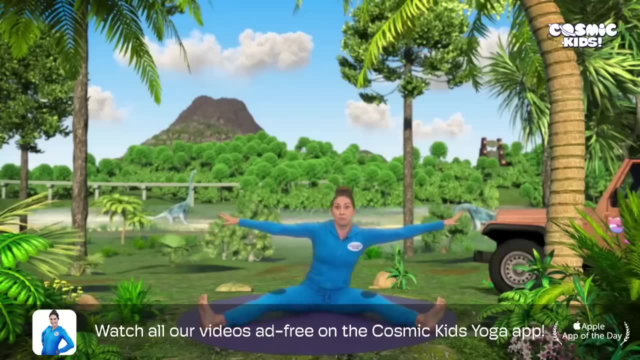 the ground. It's beginning to rumble, Coming to sit on our bottoms, taking our legs out wide. Our knees rumble up and down, arms to the side. Oh, my goodness me. coming towards us is a stampede of velociraptors Folding forwards. let's drum the ground. Here we go. 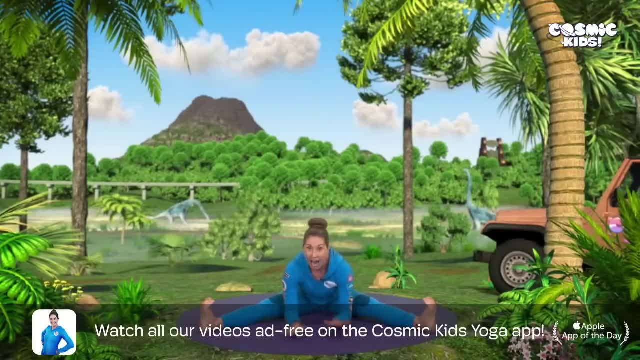 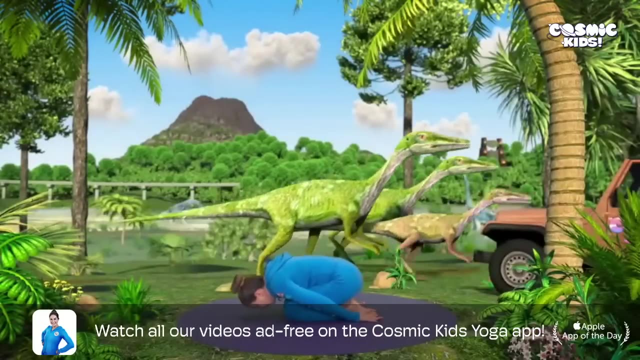 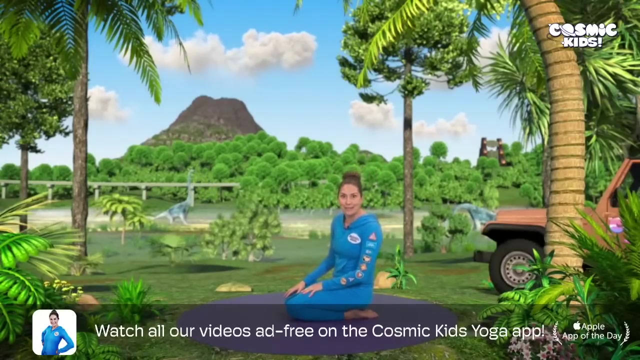 Oh, my goodness, I think we should probably hide. Coming up onto our knees everyone and tucking up, small like a little mouse, Coming all the way up to sit. Phew, I think they've gone. Well, that was exciting, wasn't? 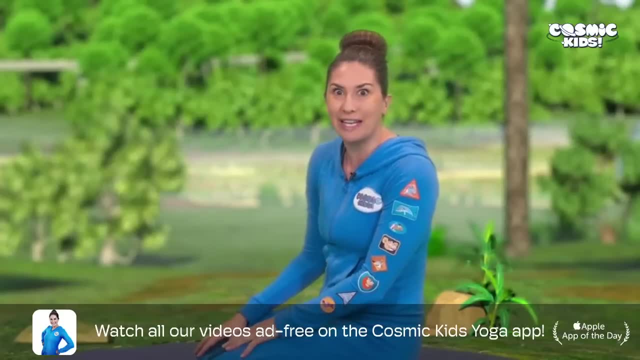 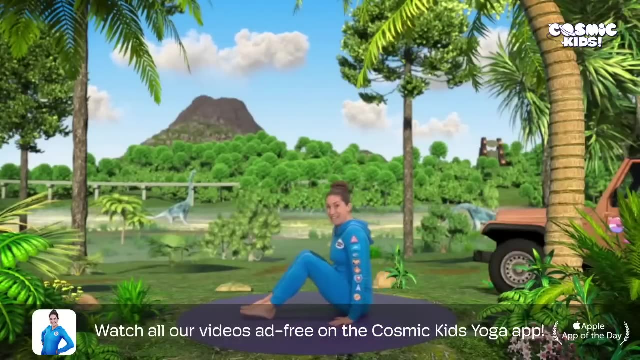 it. Now let's go in and explore the park a little bit further. We go over the bridge. Let's do our bridge pose, Sitting on our bottoms, knees, bent feet, flat hands behind us. we lift up our hips, coming into our bridge pose. 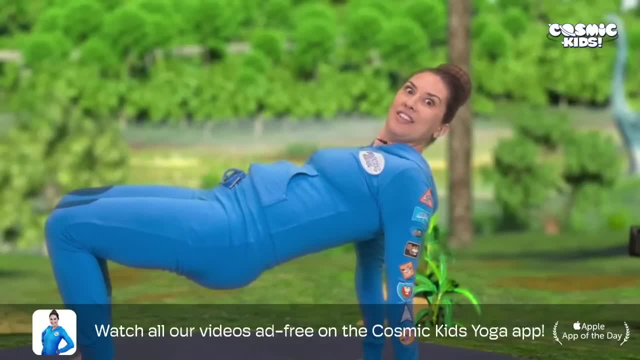 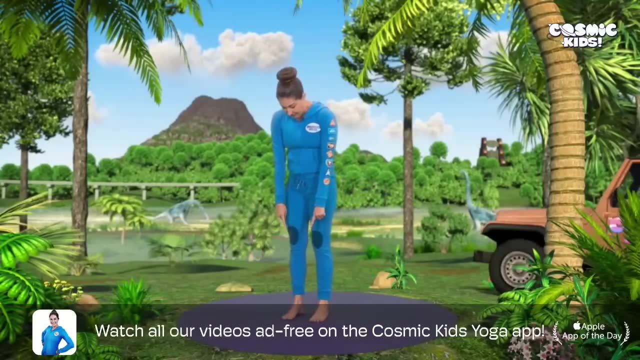 On the other side of the bridge is a zip line. Shall we have a go. Come on everyone Sitting on our bottoms, we come up to stand, We take our feet hip distance and we bend our knees. Now we sweep our arms up high, criss-cross our fingers and hold on as we. 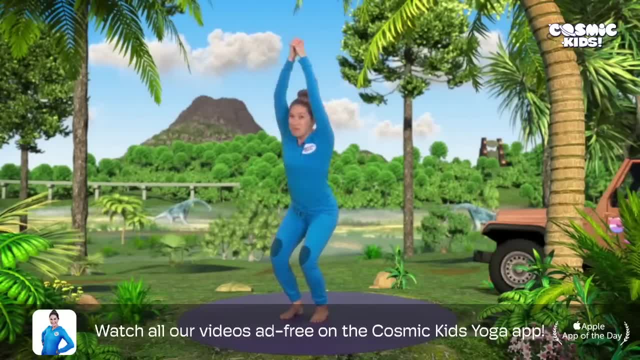 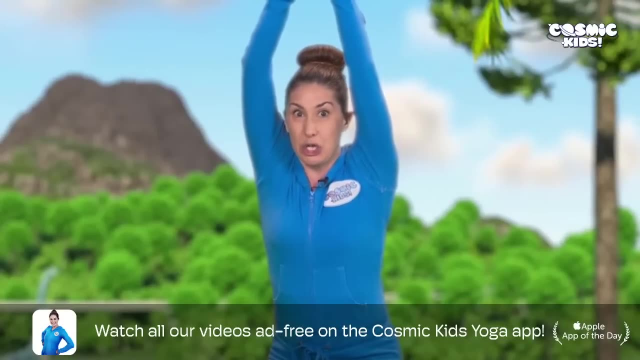 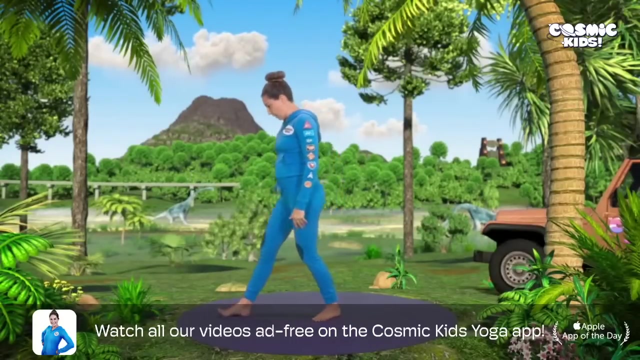 go whoosh and whee All the way through the tree canopy. Wow, it's amazing. up here We can see a Diplodocus. My goodness me, they're absolutely huge. Let's try our Diplodocus pose Coming up to stand lowering our arms. we step one foot forward and one foot back, turning. 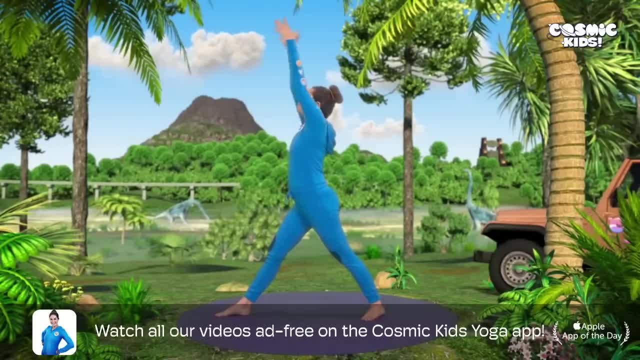 our back toes out a little bit. Now we reach our arms all the way up to the sky and draw our palms together like we're a very tall and long necked Diplodocus. Now, the Diplodocus like to eat vegetables And they love munching the leaves on the trees. Let's fold all the way forwards and do some. 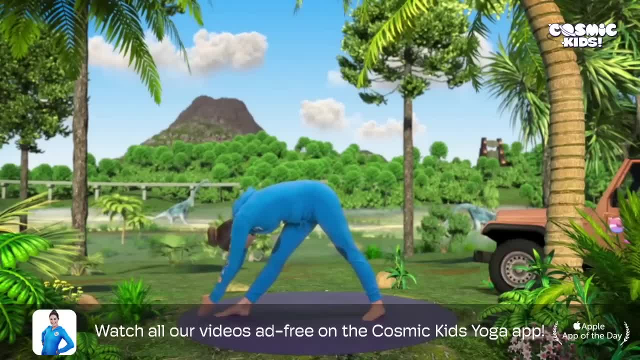 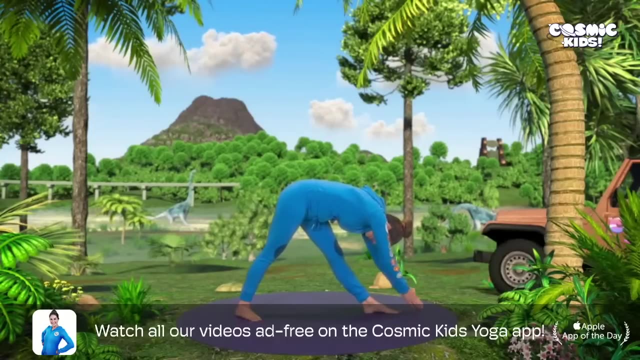 leaf munching Munch, munch, munchity munch, Coming all the way up to stand. Let's try it on the other side, Turning to face the other way now, Reaching up high and folding all the way forwards to munch some leaves: Munch, munch, munch, munchity munch munch. 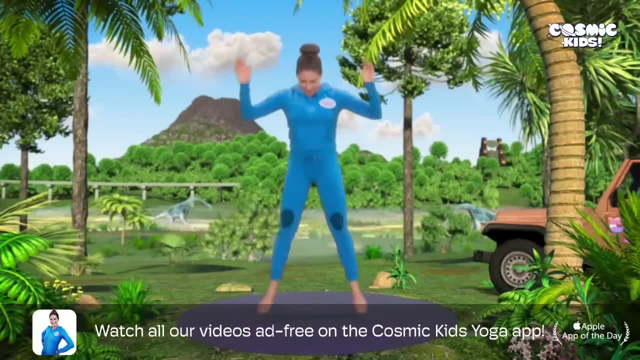 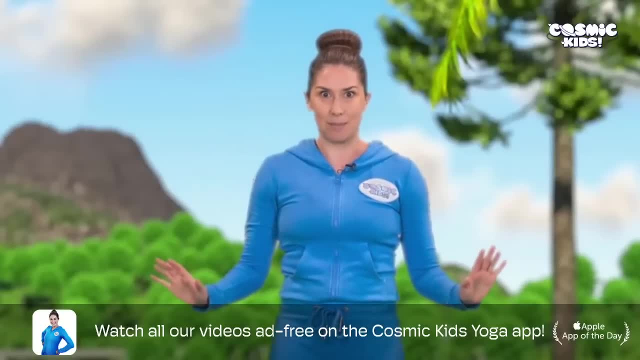 Coming all the way up to stand, Lowering our arms, jumping our feet together. Wow, the Diplodocus are so elegant. On the other side of the zipline, we come to the hatchery, which is where the dinosaur eggs are. Let's. 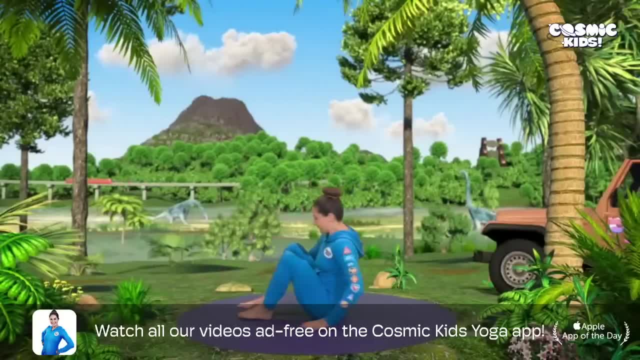 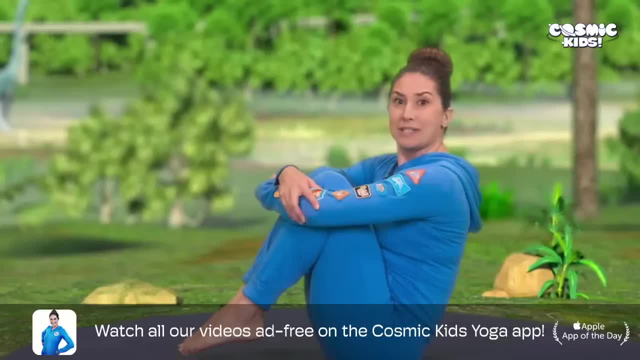 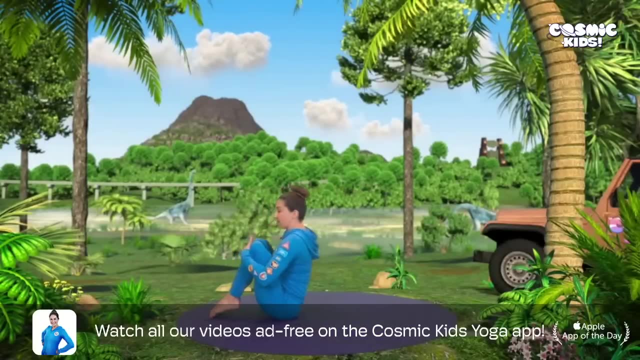 They're beginning to wobble. They're beginning to hatch, Goodness me. they're rocking backwards and forwards. Let's rock back and forwards, like a little egg about to hatch, Sitting up tall, hugging our knees, holding our knees and tucking our chin. After three, let's rock. 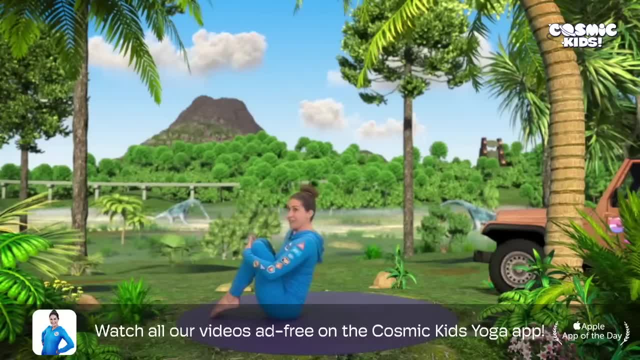 all the way back and all the way up. Here we go. One, two, three, Whoop, whoo. And again One, two, three, Whoop, whoo. Very good, It rocks all the way onto its back. Here we go, Whoop. Then it rocks onto its side, Whoop. 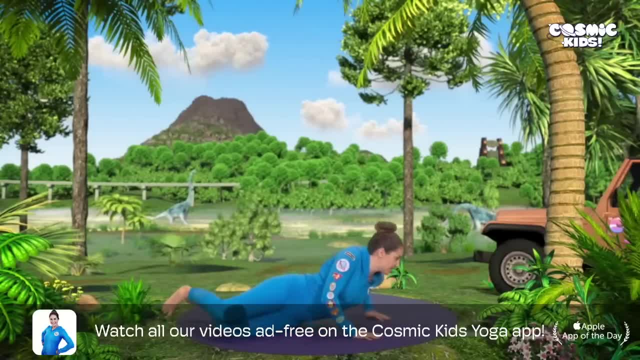 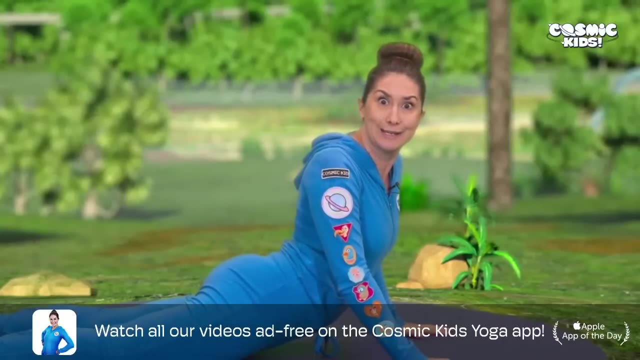 It rolls onto its tummy, Coming onto our tummies, everyone Hands underneath our shoulders and it begins to push forwards with its nose, cracking its shell. Wiggle, wiggle, wiggle, wiggle, wiggle, wiggle And out pops a baby ankylosaurus. Awww. 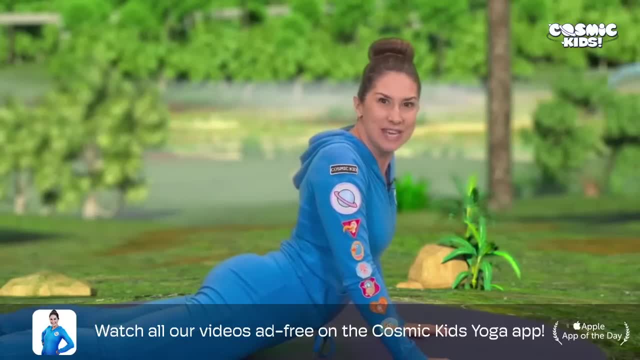 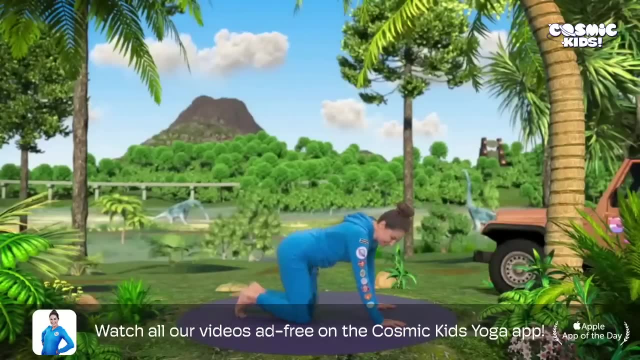 The ankylosaurus are a bit like a turtle, with bony plates and spikes on its back. Let's do our ankylosaurus turtle pose. Coming to sit, we take our legs out nice and wide, bend our knees a little bit and bring our hands down in front of us. Now we slide one arm. 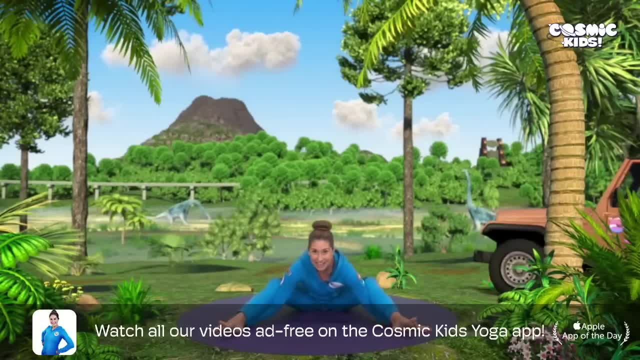 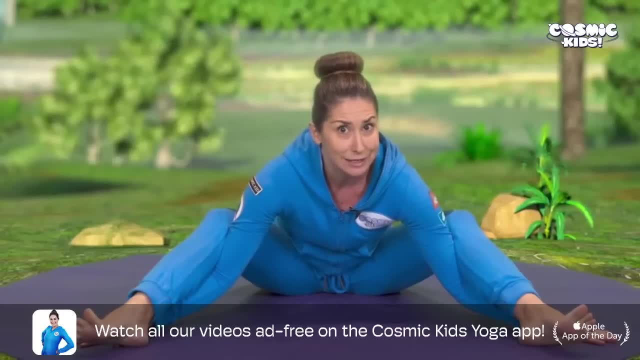 under one leg and we slide our other arm under the other leg. Coming into our turtle ankylosaurus pose. Let's try our ankylosaurus tail. They can do a lot of damage when they swish those around. Let's try our ankylosaurus tail pose. Coming all the way up to stand, We take our feet. 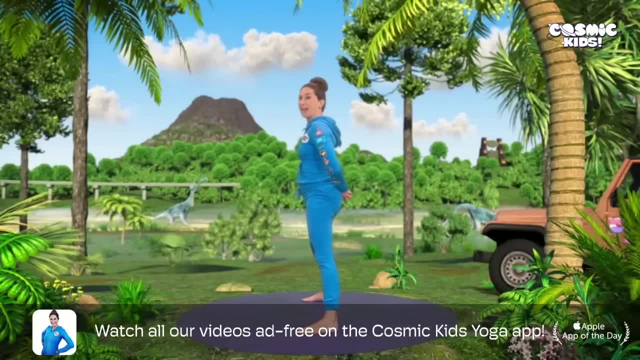 nice and wide criss-cross our fingers behind our back, roll our shoulders back behind us and stretch our arms. Now, after three, we fold all the way forwards with a swoosh Ready: One, two, three, So whoosh. 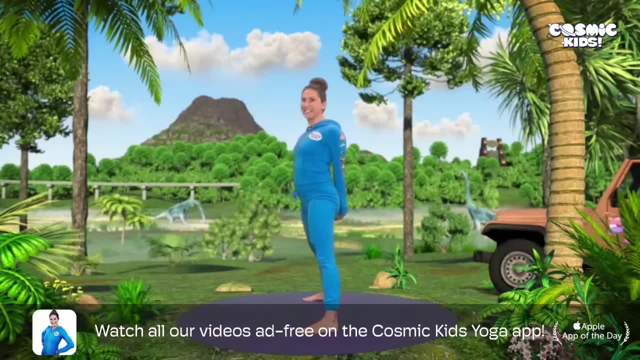 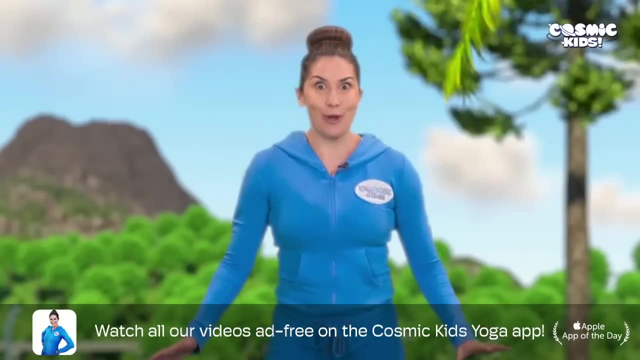 And all the way up to stand. Wow, you better keep out of the way when the ankylosaurus swishes its tail around, Jumping our feet together. coming back to centre, Now, why don't we be really brave and go check out some of the scarier dinosaurs? Let's get. 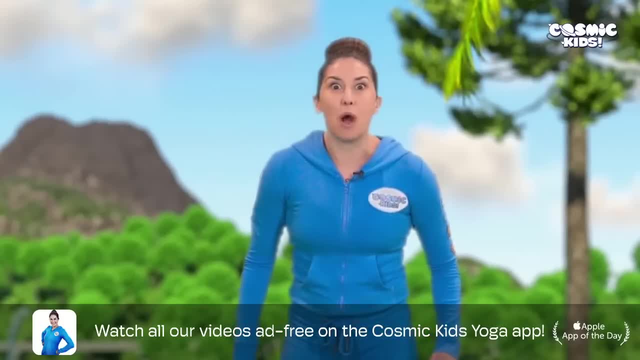 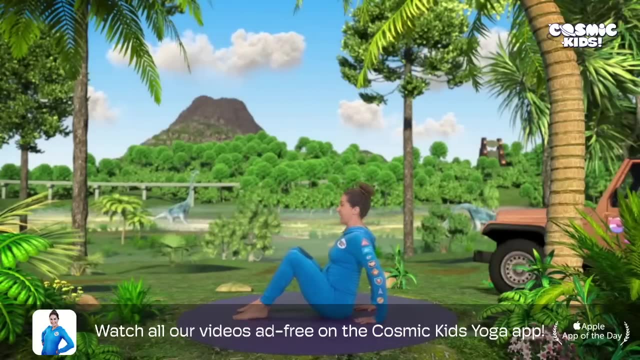 into the little raft boat Coming into our boat. pose: Sitting on our bottoms, knees bent. we keep our hands behind us for balance As we lift up one foot, lift up two, lift up one hand, lift up no hands. And give me a wave: Hi, Very good, everyone Stretching our 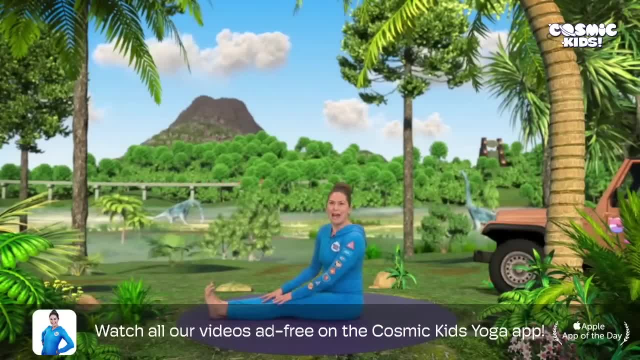 legs out forwards. we row our little raft boat down the Jurassic River, knowing that the dinosaurs are very safe in their habitats. Singing row, row, row your boat, Come on, picking up one of our feet And let's row. 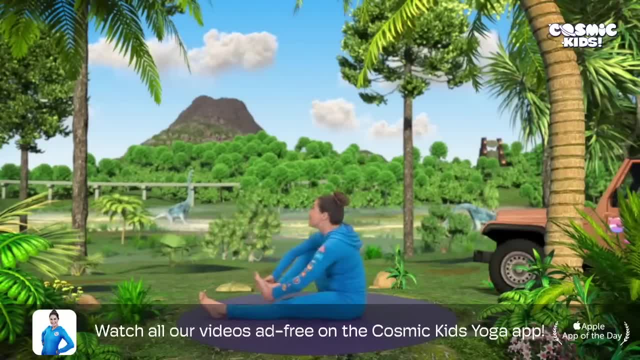 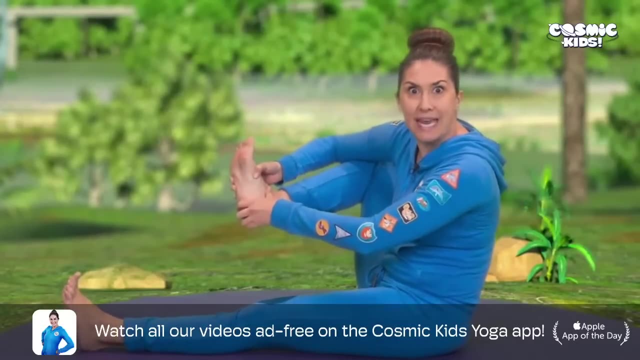 Here we go, Row row, row your boat Gently down the stream, Merrily, merrily, merrily, merrily. life is but a dream. Oh look, That's the walkie-talkie from base camp. Let's answer it. Receiving come in. 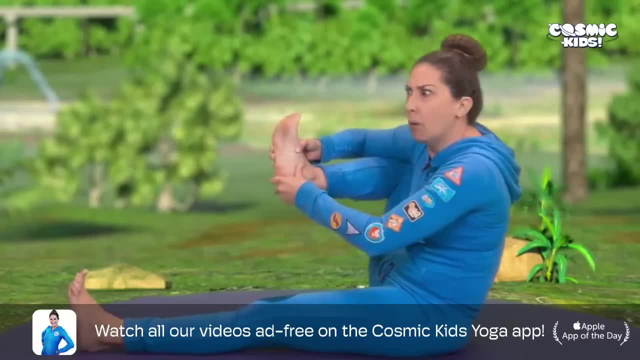 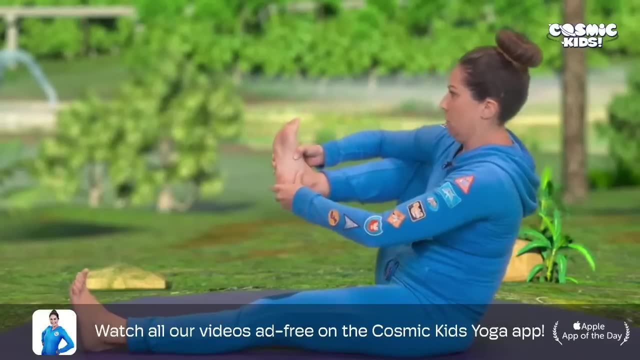 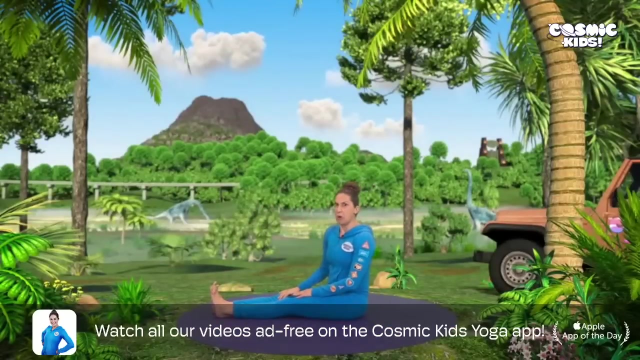 we are on the raft boat. All operatives in the park. the dinosaurs have escaped. Escaped Dinosaurs. Oh, problem. Okay, Oh, it seems to have stopped. Let's put it down. Oh dear, Maybe we should row on a little bit further. Let's pick up the other oar and stay nice and calm as we. 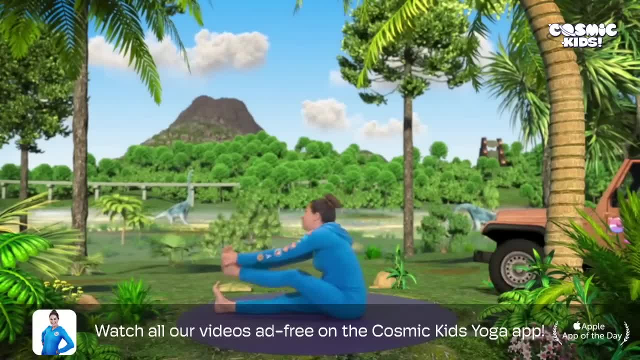 sing our row, row, row your boat song. again, Here we go, Row, row, row your boat Gently down the stream. Merrily, merrily, merrily, merrily. life is but a dream. 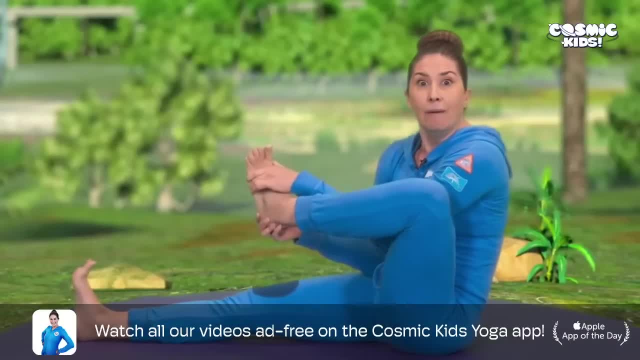 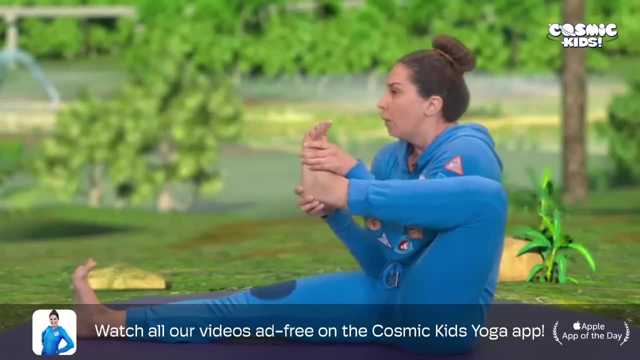 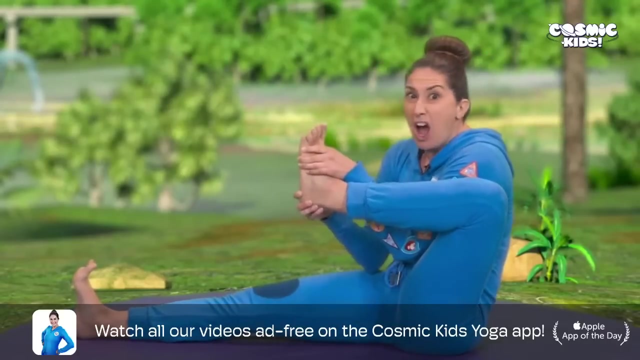 Oh, it's the walkie-talkie again. Let's answer this one, Holding it to our ear. Come in, Roger Receiving. Please make your way to the exit immediately. Exit Immediately. Oh, okay, then Okay, Over and out. Bye, We put the walkie-talkie down. Oh, and it sounds. 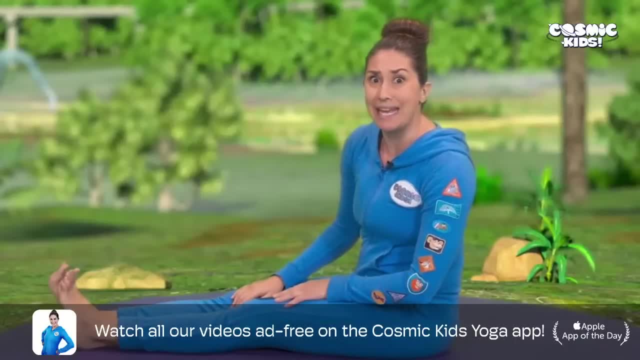 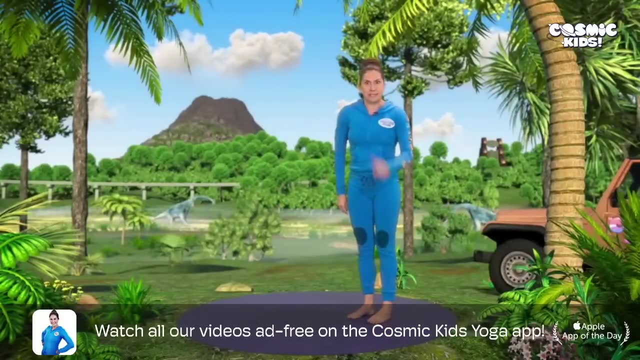 like we need to get out of here pretty quickly. Well, we arrive at the banks of the river, Coming up to stand everyone, And we take big steps into the woods, Standing nice and tall. Here we go, Big step And all. 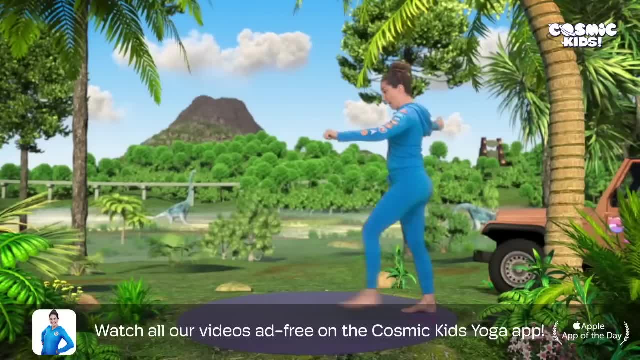 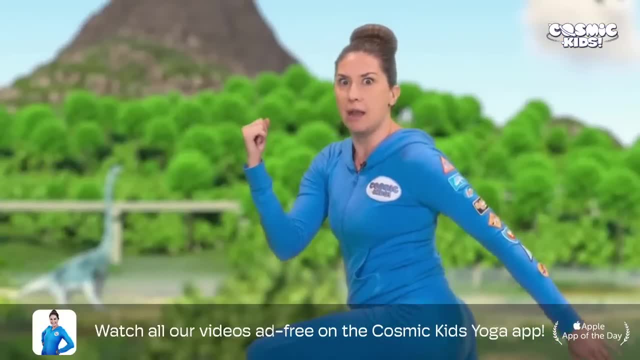 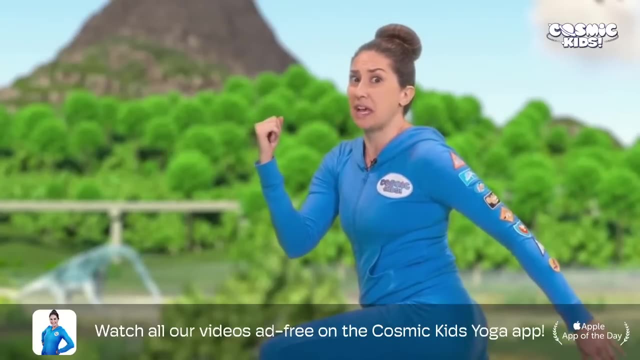 the way back And the other side, Big step, Uh-oh. We can feel the ground trembling again, And this time it's something much bigger and much scarier. Clomping towards us is a Tyrannosaurus rex. 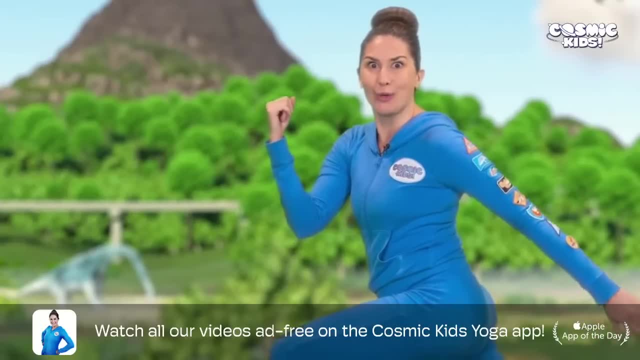 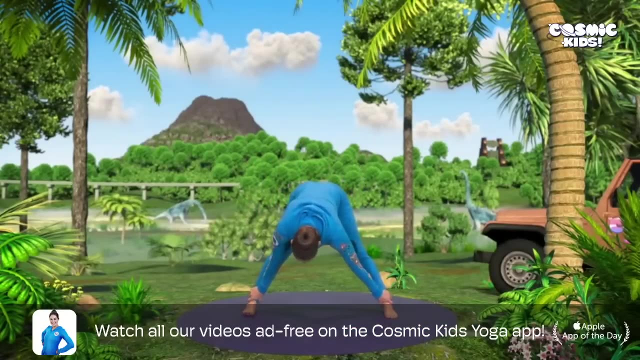 Rex, Let's do our T-rex clomping pose. Coming up to stand Feet, nice and wide, Folding forwards to grab our ankles. We lift them up, one at a time, going clomp, clomp. Here we go, Clomp. 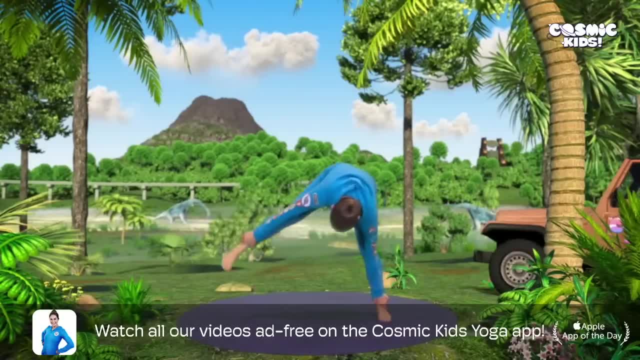 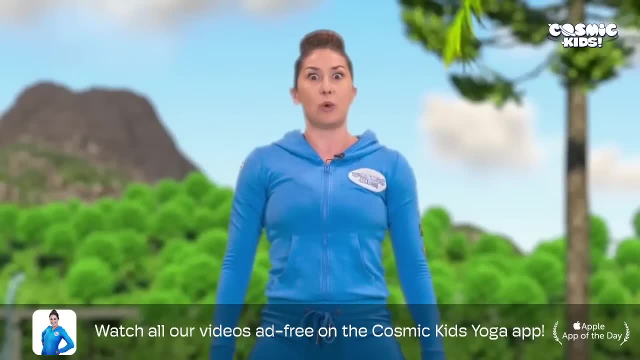 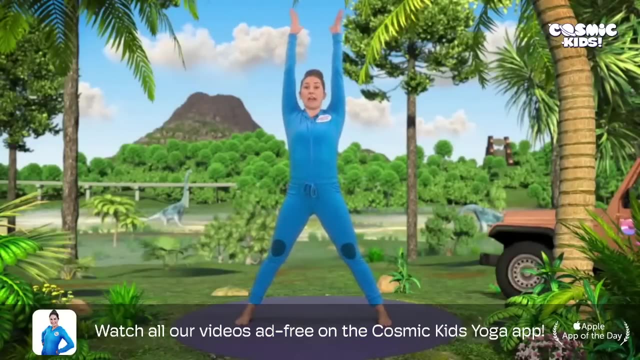 clomp, clomp, Clompity, clomp, Clomp, clomp, Rolling up to stand. Okay, everyone, We've got to think quick. Let's throw our sandwiches for it. Then we can hide Reaching all the way up to the sky Into our backpacks behind us. We grab our sandwiches. 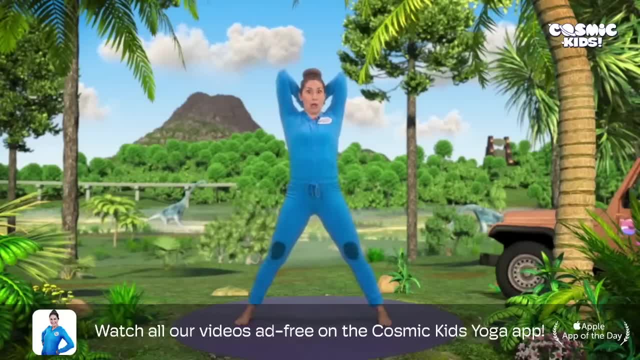 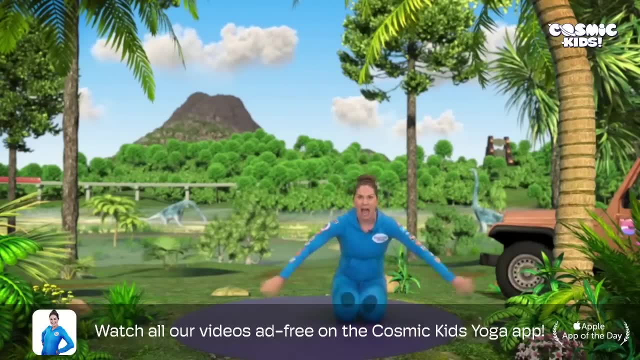 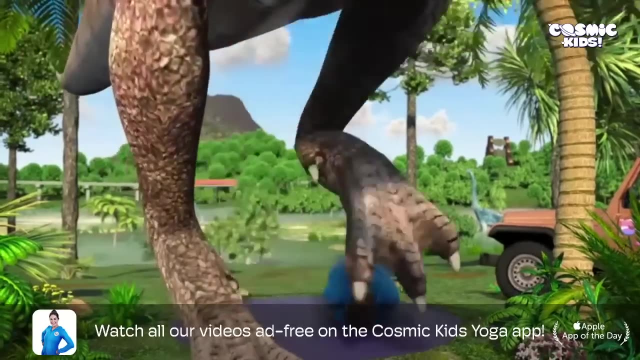 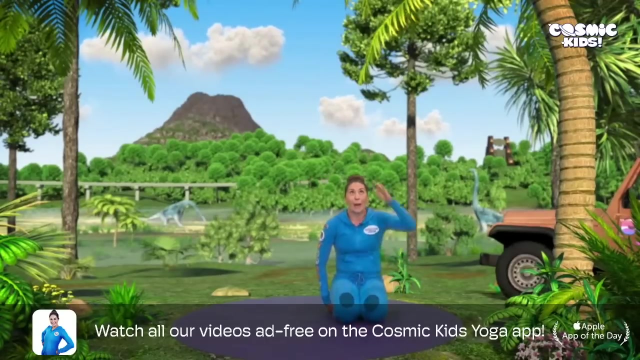 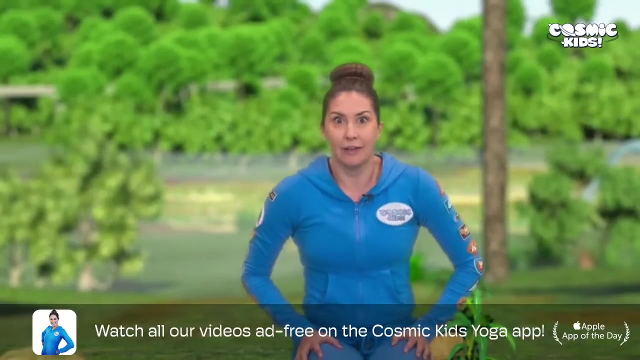 and we throw them for the Tyrannosaurus rex. Here we go, Pee-yoo. Now we need to hide, Coming down onto our knees, everyone And tucking up nice and small. Here it comes for our sandwiches, Coming up to sit for you. Well done It. clearly enjoyed our sandwiches and off it went, That's. 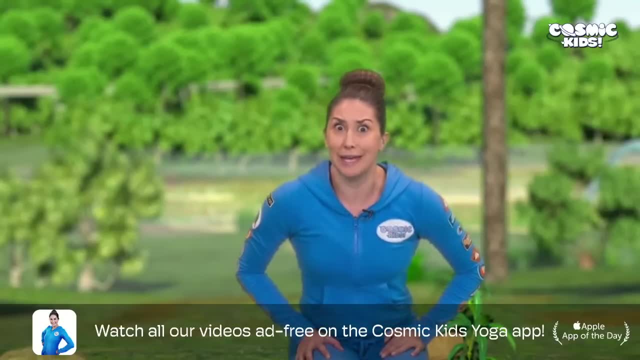 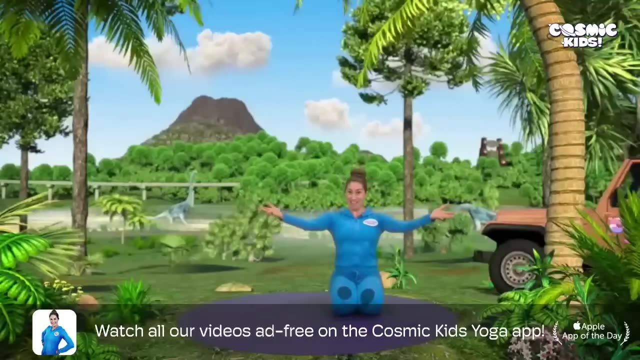 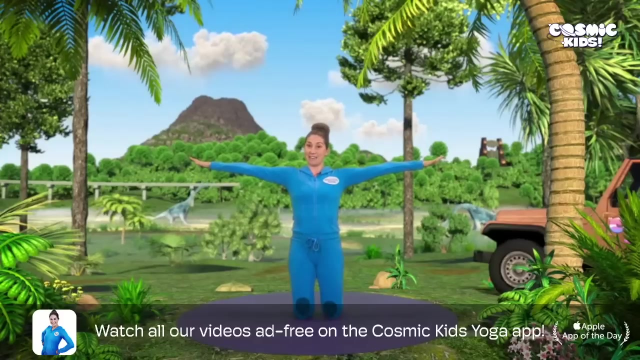 a relief. Well, I think that's about enough excitement for one day, don't you? Let's use our emergency escape card and make the pod plane appear. Here it is. Let's do our pod plane, Pod plane pose, Coming up to two knees. we take our arms out nice and wide, We drop down. 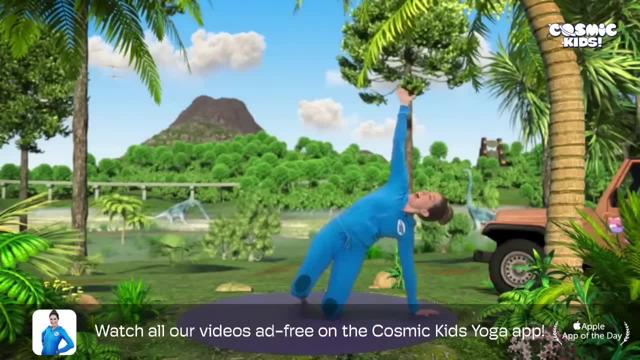 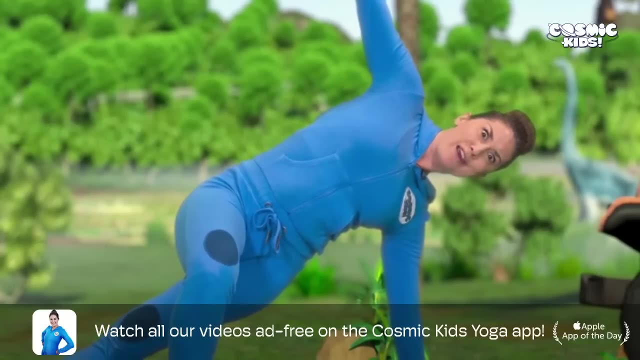 onto one hand and we wave at the sky, Say hi sky, Hi sky. We bring one foot in front of our knee and shoot our back leg out behind us, lifting our hip, And look Up in the sky. we see a whole flock of pterodactyls. Let's wave at the pterodactyls: Hi pterodactyls. 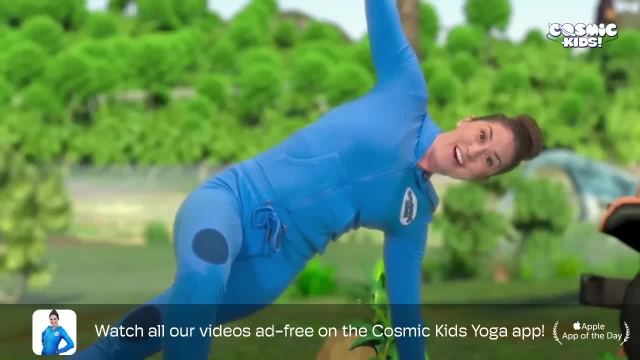 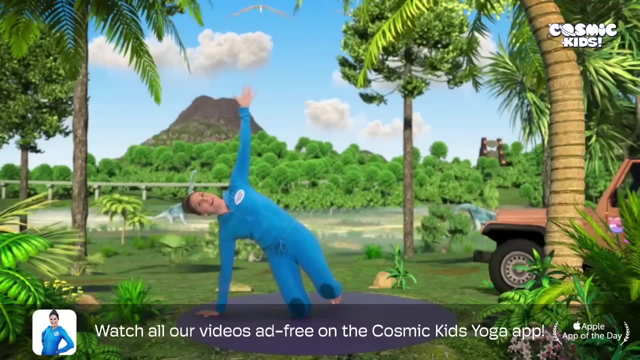 Let's do our pod plane pose on the other side, Coming back to two knees arms wide, We drop down onto our other hand. Let's give another wave to those pterodactyls, Hi pterodactyls. 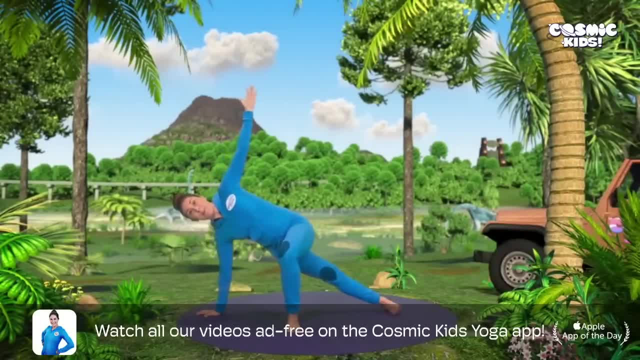 We bring our foot in front of our knee and shoot our back leg out behind us and lift up our hips as we go Flying all the way home. We take a moment to take a deep breath and we take a moment to lie back and relax in our pod plane, Coming to sit on our bottoms. 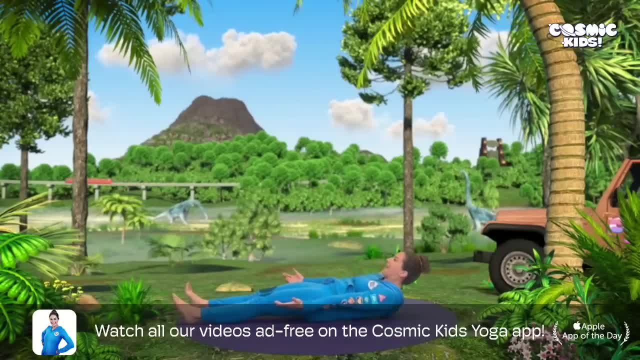 legs long, rolling all the way down onto our backs. Our pod plane will take us home, keeping us nice and safe. It's so peaceful and fresh up here in the sky. What an amazing experience, An adventure. Weren't we lucky and brave to see all those amazing dinosaurs? It's very 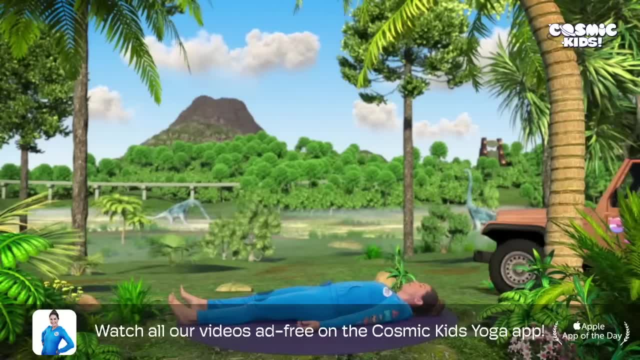 important, whenever we see animals in their habitats, that we treat them with respect. Whether we're in a park like this, we're diving in the ocean or we're just out walking in the woods, We are peaceful and respectful of the other creatures and animals that live there, And 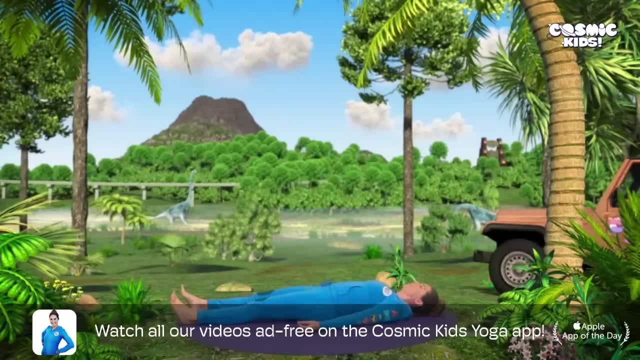 we leave no trace. We always take our litter and our rubbish away. Now we begin to wake up, wiggling our toes, wiggling our fingers, hugging our feet and hugging our knees into our chests as we roll onto our sides and press ourselves up to 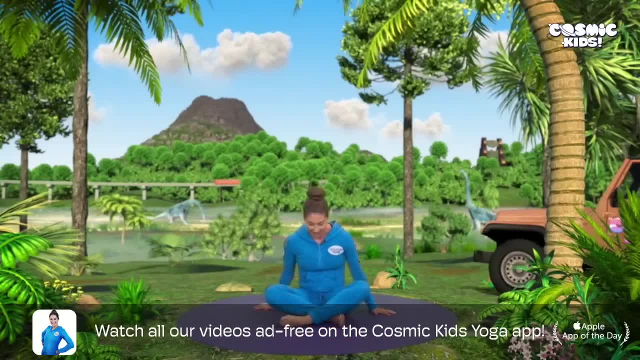 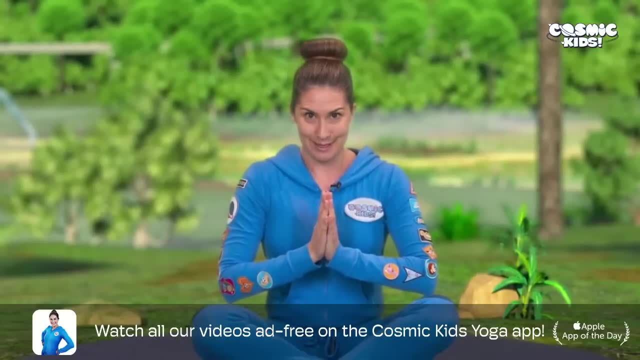 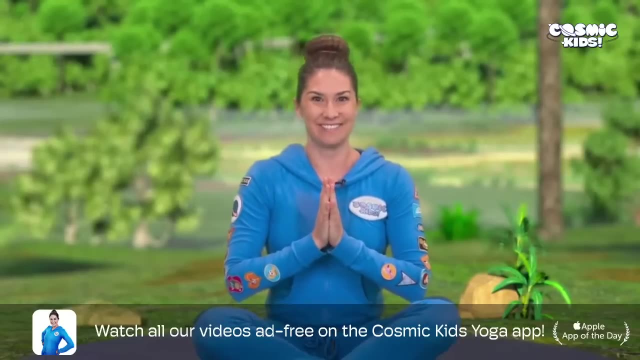 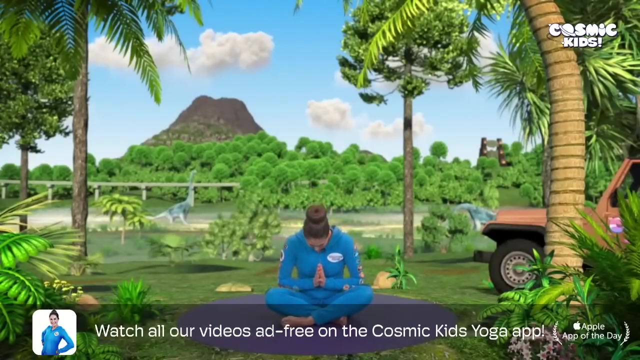 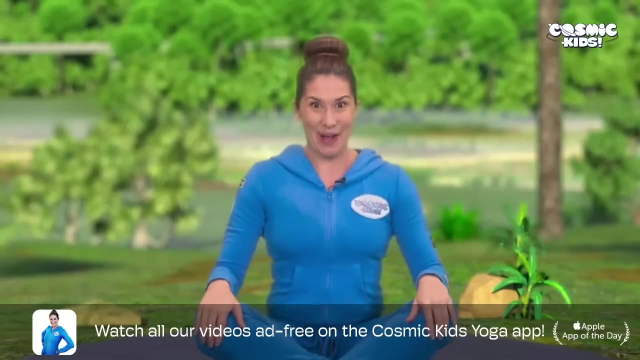 sit with our legs crossed, our hands together at our hearts, to finish just the way we started with our secret Jurassic dinosaur yoga code word, which is Namasaurus, Ready After three: One, two, three, Namasaurus. Wow, You were amazing in the Jurassic dinosaur yoga adventure. I hope you enjoyed it and 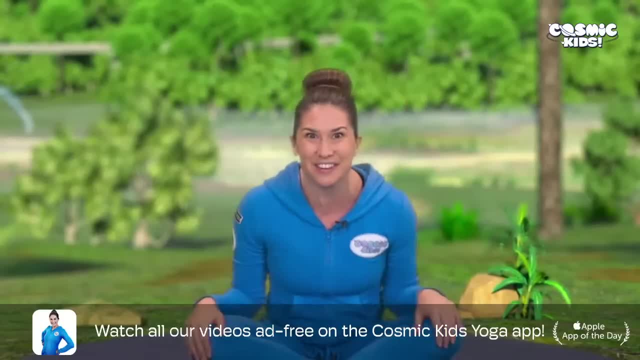 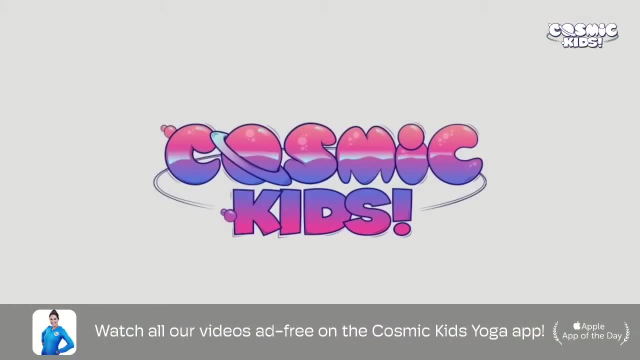 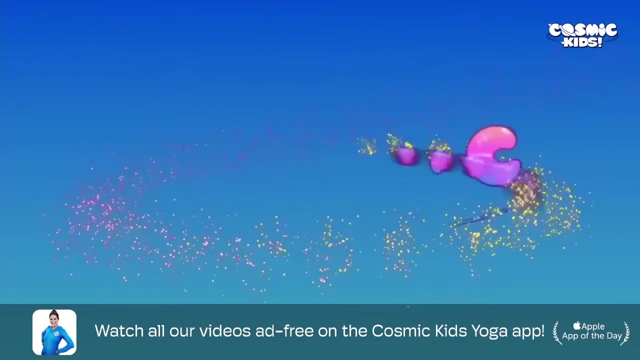 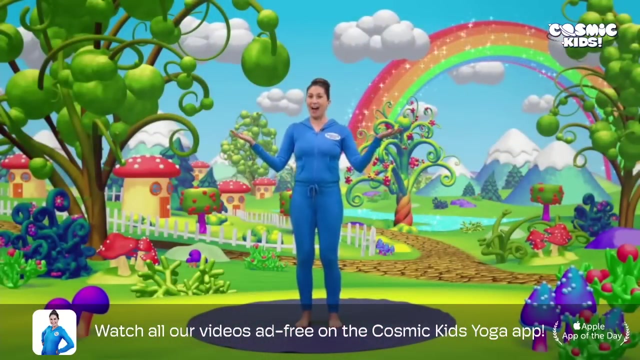 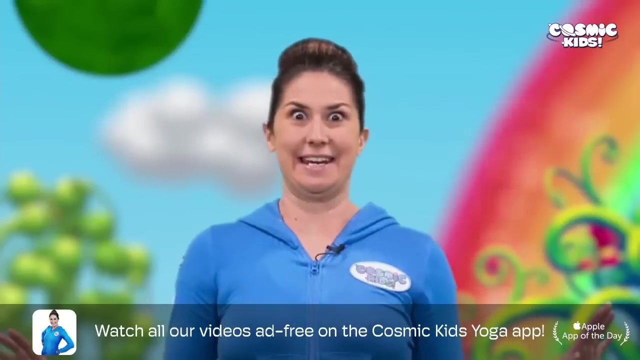 I hope to see you again soon for another Cosmic Kids adventure. Bye-bye, Hello everyone. Welcome to Cosmic Kids. I'm Jamie and this is your place for yoga, stories and fun. It's easy: Just copy the moves I do and enjoy the adventure. Now we always start in the same way. 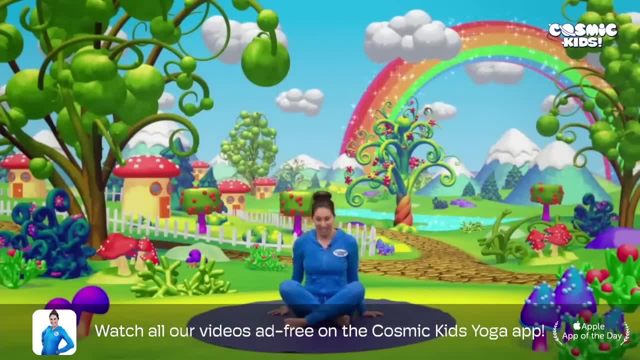 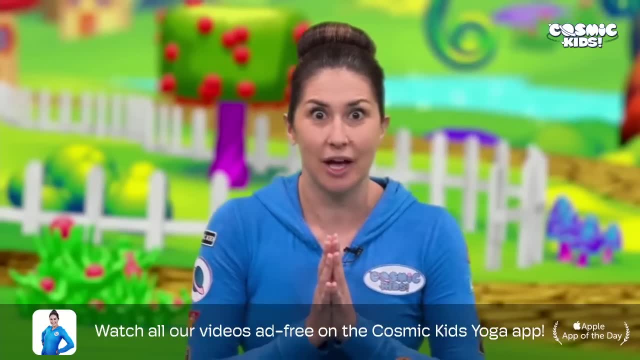 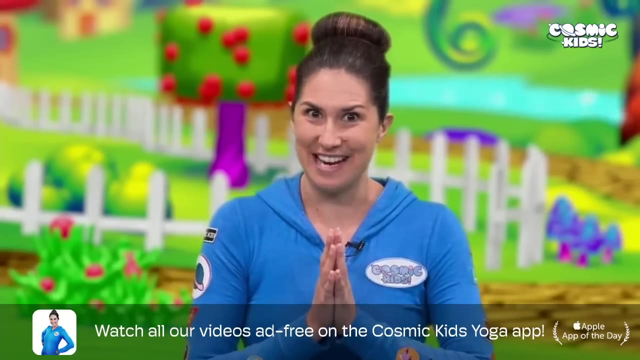 And that's by sitting on our bottoms, crossing our legs and bringing our hands together at our hearts And saying our secret yoga code, The secret yoga code word which is Namaste, Ready After three, One, two, three, Namaste. 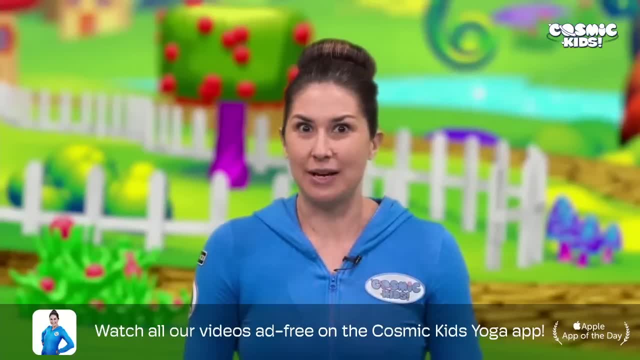 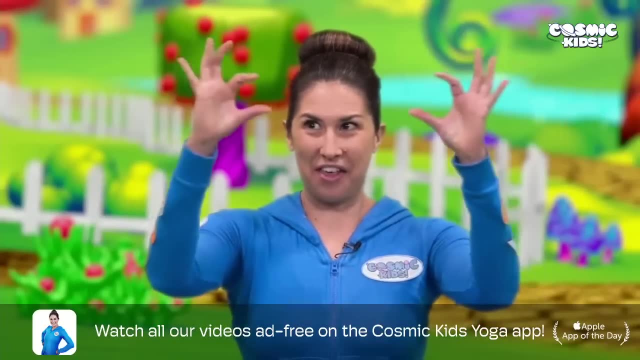 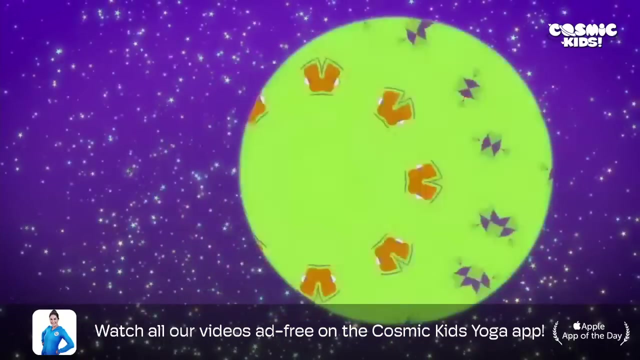 There. Now we're ready to begin. So let's take a look through our cosmonoculars and find out who we're meeting today, Joining our thumbs and fingers together. have a look through, Wow. Look at those colours and those shapes, Those patterns, all swirling and twirling around. 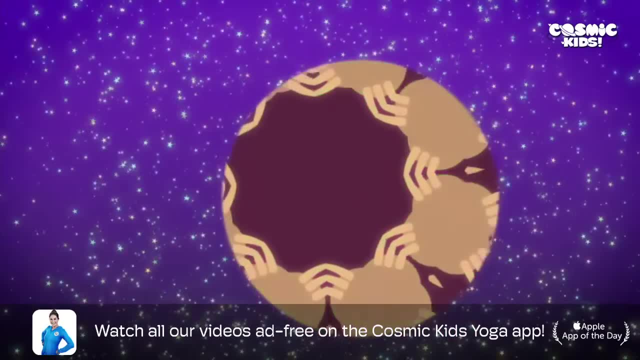 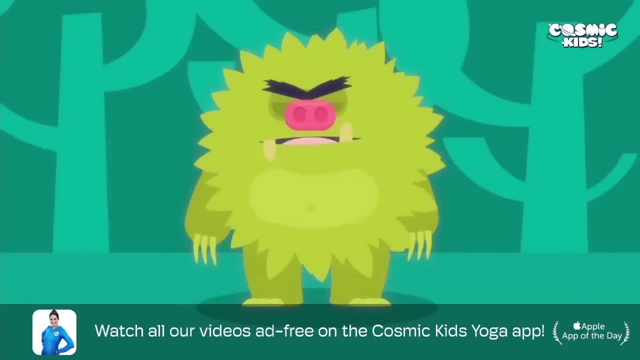 Oh, aren't they pretty. Can you see the picture? It's a monster. It's Biggles the monster. Oh, what's Biggles doing? He's doing yoga. He's doing crocodile pose, Lowering our hands. How cool. 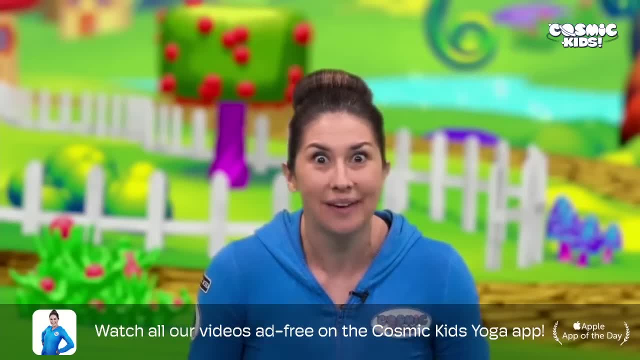 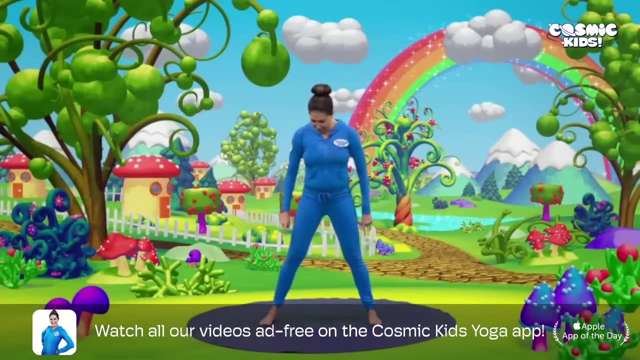 Biggles is a very big monster. So let's begin in our clompy monster pose. Coming up to stand, We take our feet nice and wide, We fold all the way forwards to take our ankles And we lift our feet up and down as we say clomp, clomp, clomp, clompity, clomp, clomp, clomp. 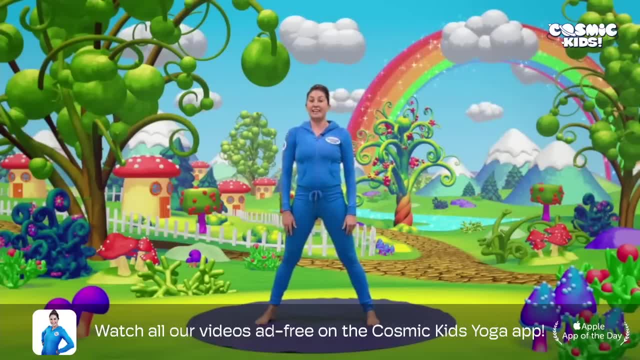 Rolling up to stand. Now. Biggles has spiky green hair that sticks out in all directions. Let's use our arms and legs to be our spiky green hair. Keeping our legs out wide, we stretch our arms out wide as well. 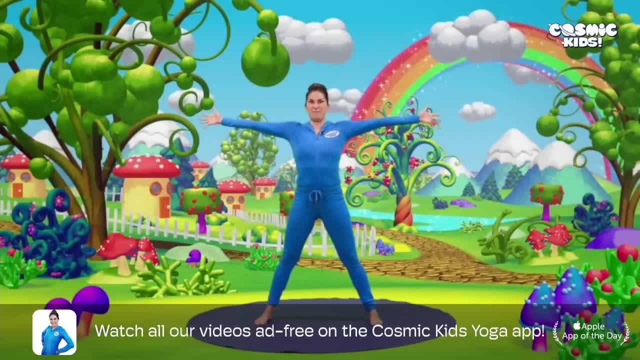 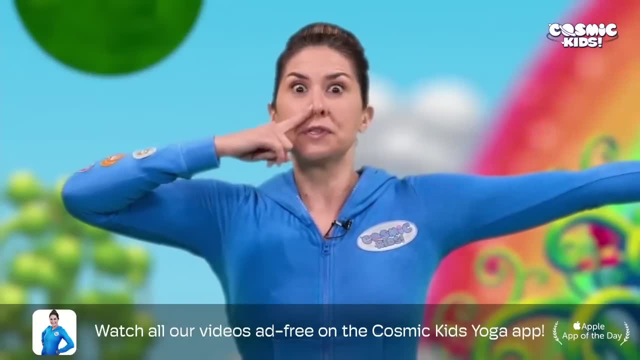 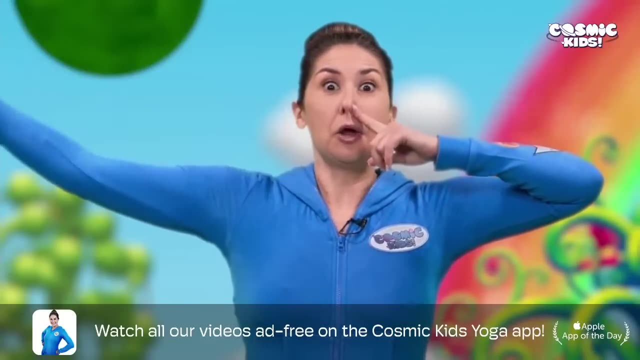 And we wiggle our fingers to make extra spiky bits. He's got a big pink nose. Let's close one of our nostrils And breathe in through the other one. Now we close that one And open the first one to breathe out. 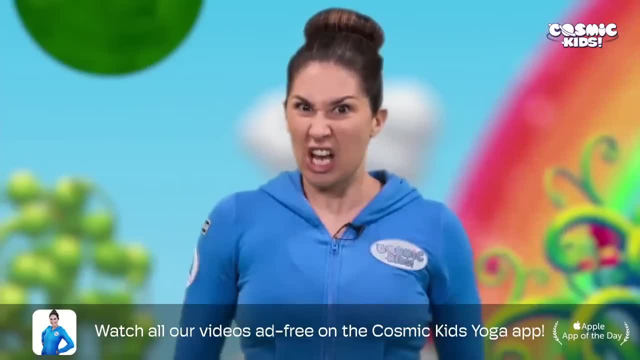 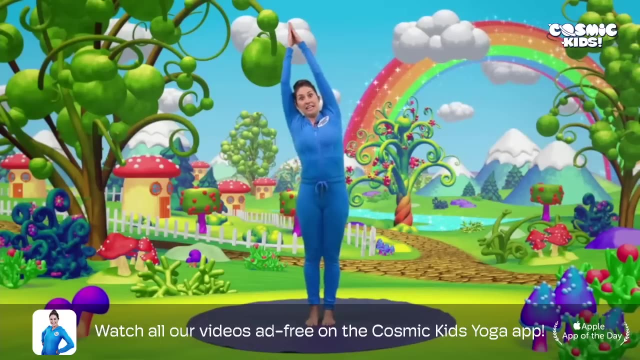 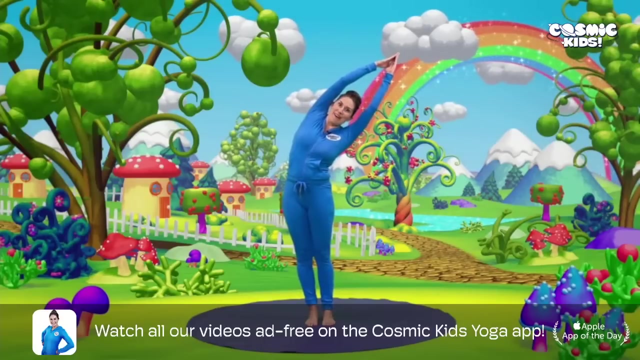 Very good. everyone Biggles' fingers look like bananas, Jumping our feet together, Reaching our arms up above our head. We lean all the way over one way Like a banana And all the way over the other way Like a banana. 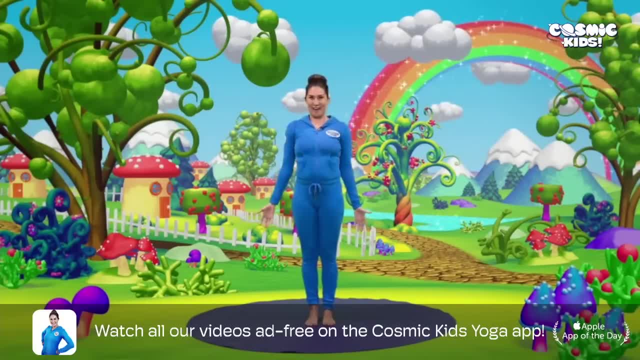 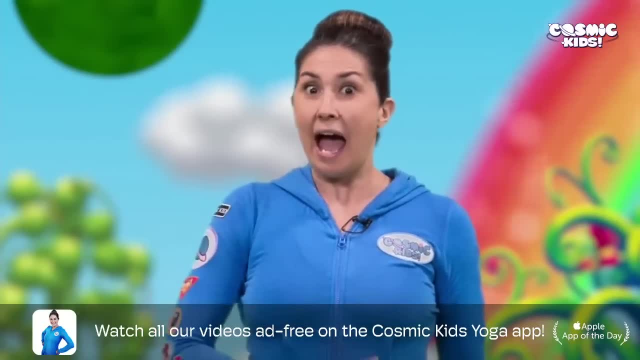 Coming all the way back to the middle And lowering our arms. He has a round tummy- Let's roll our hand around and around on our tummy- And he has short little legs. We walk our feet out just a little bit. 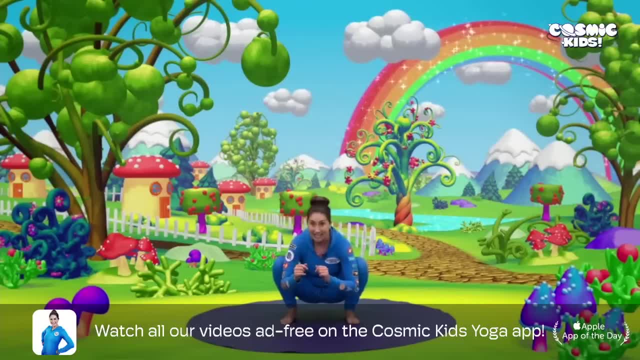 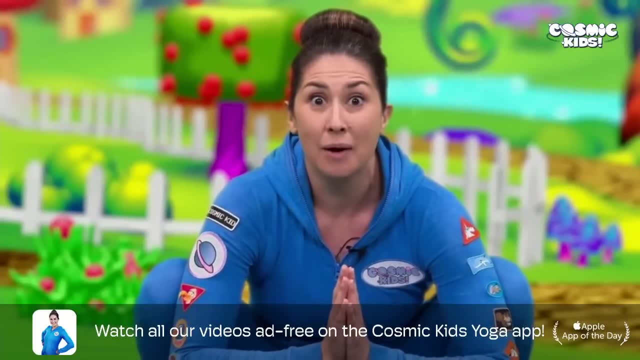 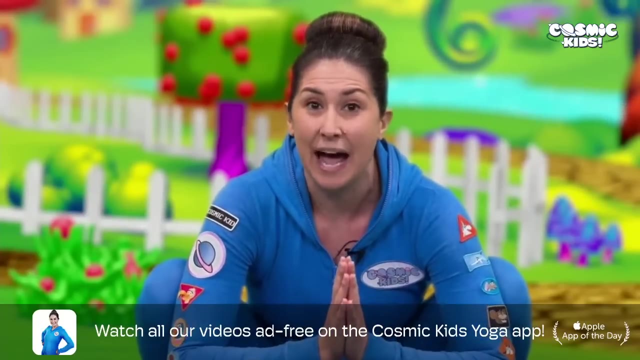 And we squat all the way down, Making our legs look really, really small. Now Biggles only knows one word, Which is Biggles. Can you say that? Biggles, Yes, well done everyone. Now Biggles goes for a walk. 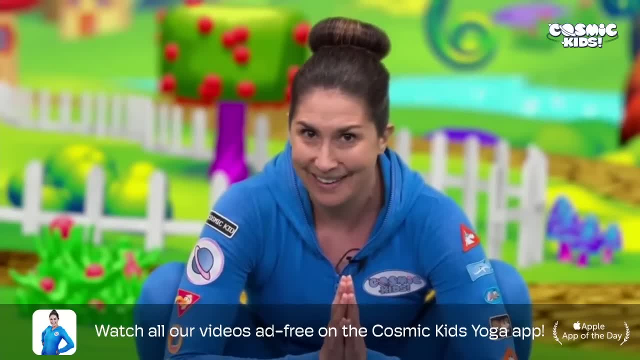 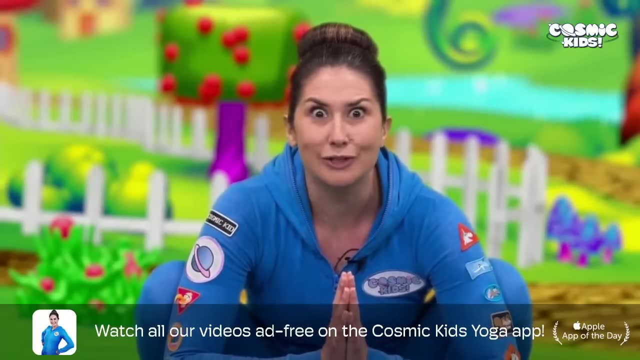 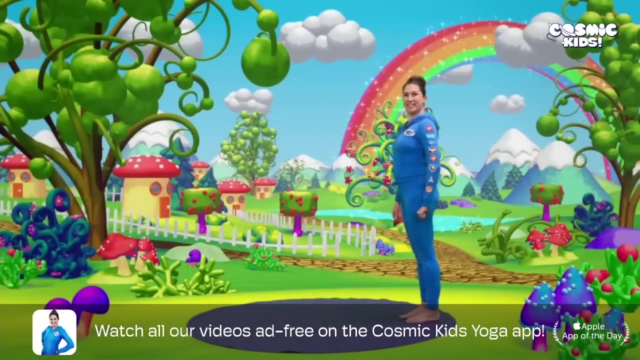 And being a very playful monster, He likes to walk in all sorts of fun and different ways. He likes to take big squelchy steps through the muddy puddles, Coming all the way up to stand. We come to stand nice and tall. 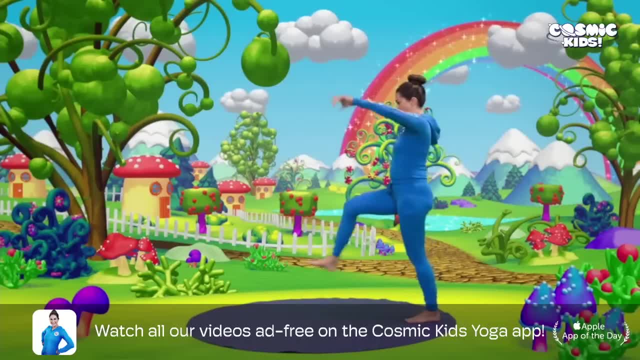 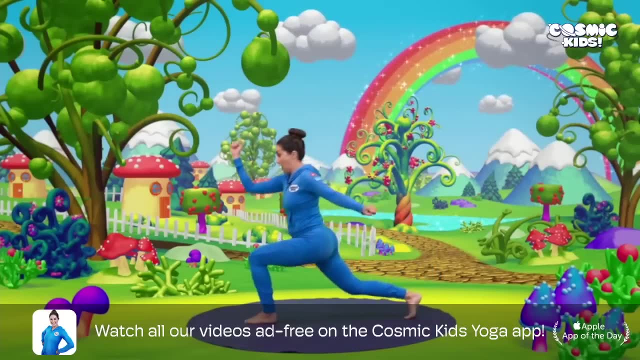 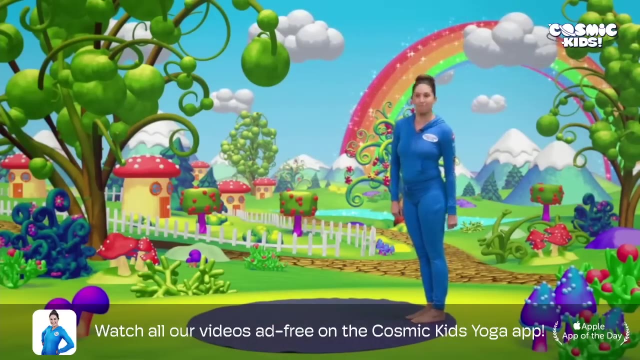 And we take a big step forward Here. we go, Squelch And all the way back. And the other side Squelch And all the way back. Very good. Next he does some skipping: Biggles, Biggles, Biggles, Biggles, Biggles, Biggles, Biggles. 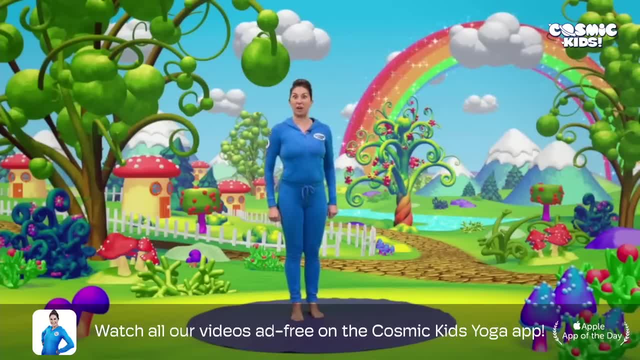 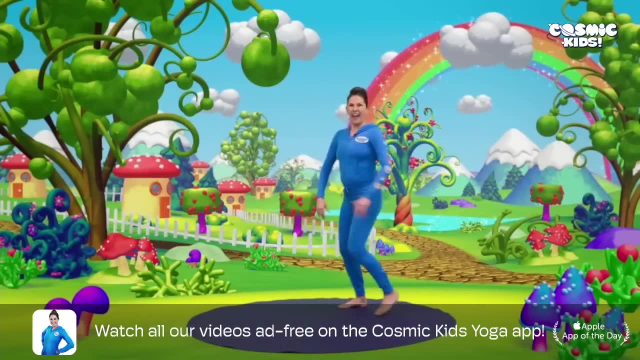 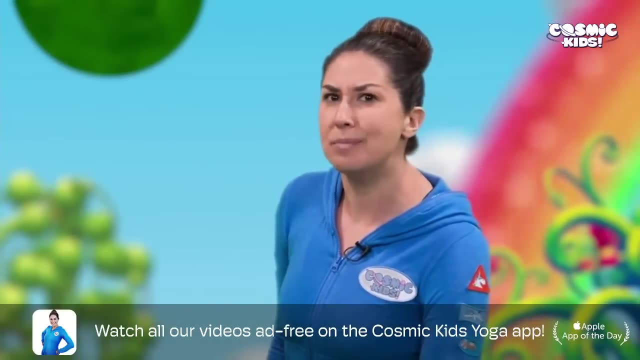 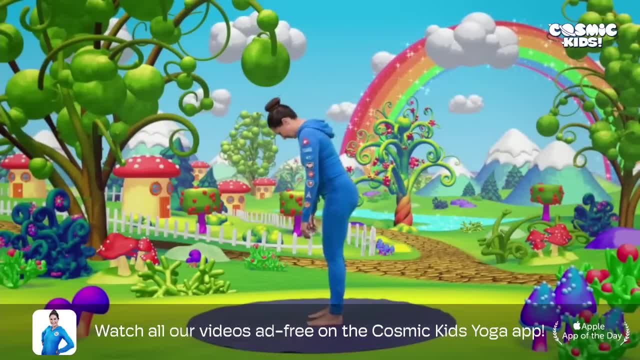 Standing, nice and tall. We drop our chin and we fold all the way down, Luring our hands, Keeping a little bend in our knees. He pops his hands on his shins And he stretches his back, nice and flat, As he takes a big breath in to smell the flowers. 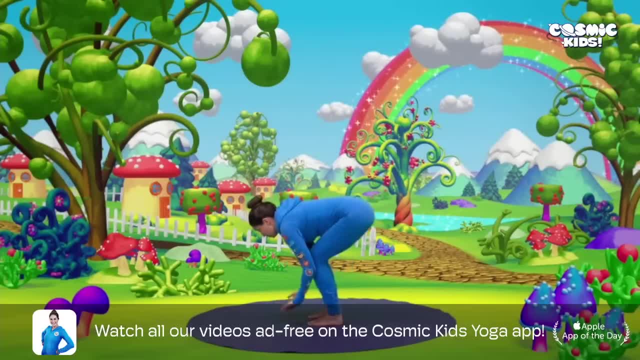 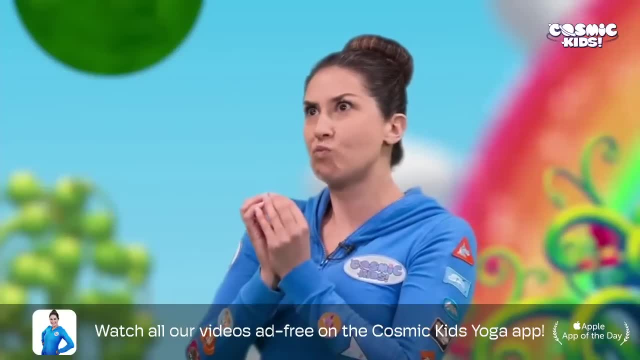 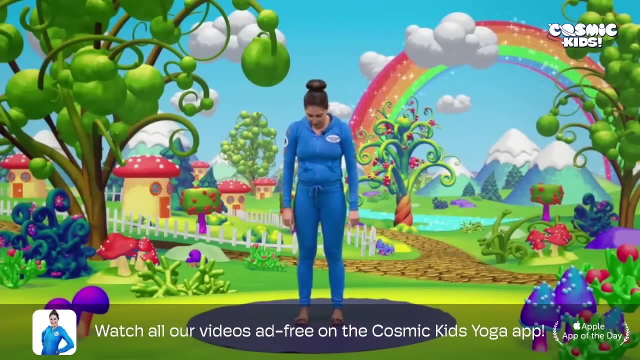 Ah lovely. Next he reaches all the way up to pluck a leaf from a tree And has a little nibble- Hmm, to taste it. He's curious. Then he lifts all ten of his big toes And he squishes them into the lovely soft, smushy grass. 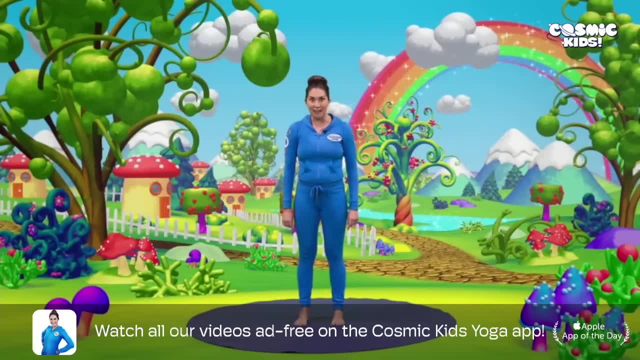 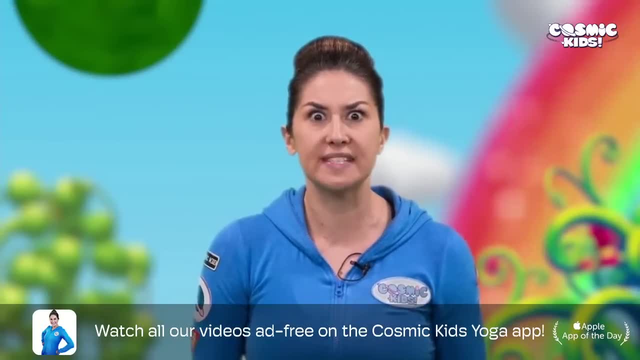 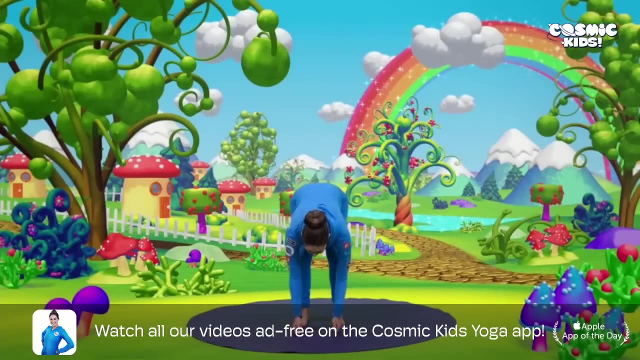 Oh, that feels good. Can you lift all ten of your toes? Yes, very good, everyone. Then Biggles finds two sticks beneath a tree. Bending our knees a little bit, He folds all the way forwards to pick them up. He rolls all the way up to stand. 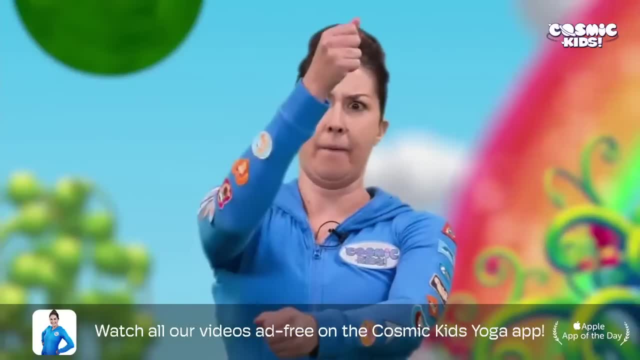 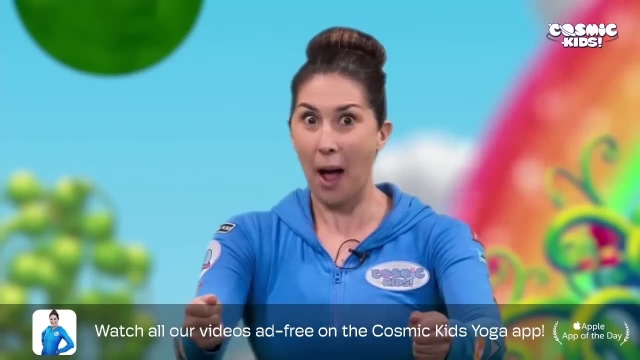 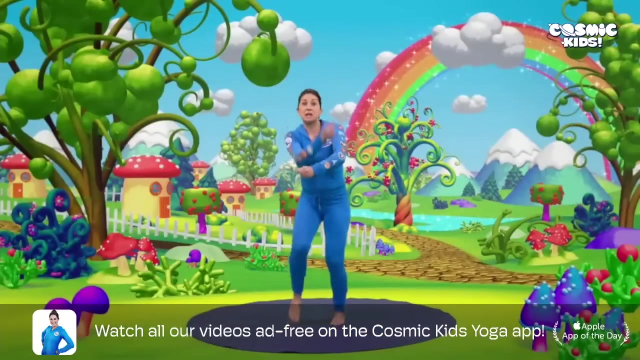 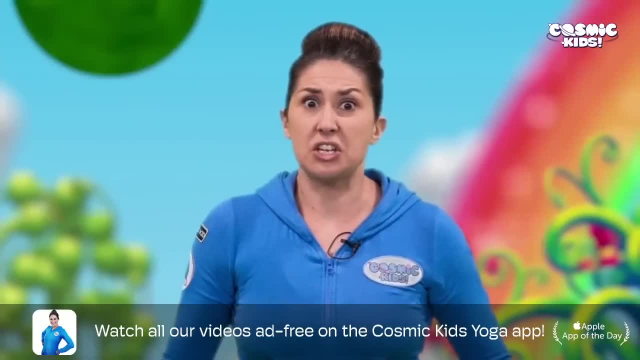 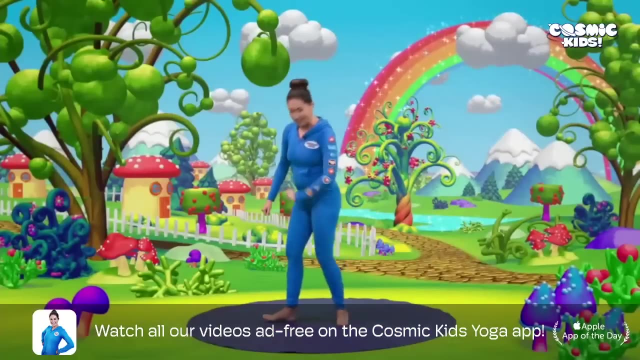 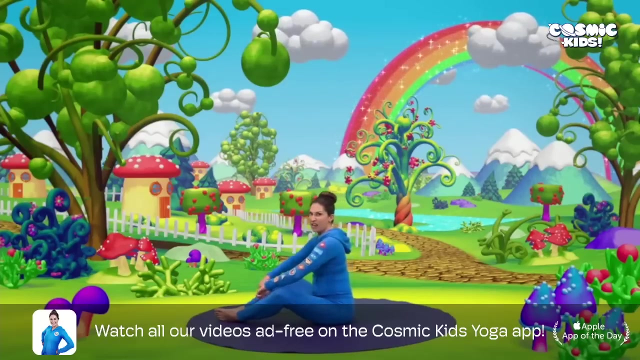 Very good, But he doesn't notice the huge hole in the ground. Let's make the huge hole. with our legs Sitting on our bottoms, We bring the soles of our feet together And keep our legs nice and wide, So they're in a hole shape. 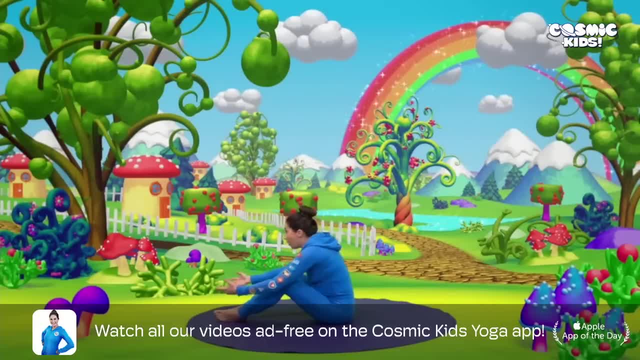 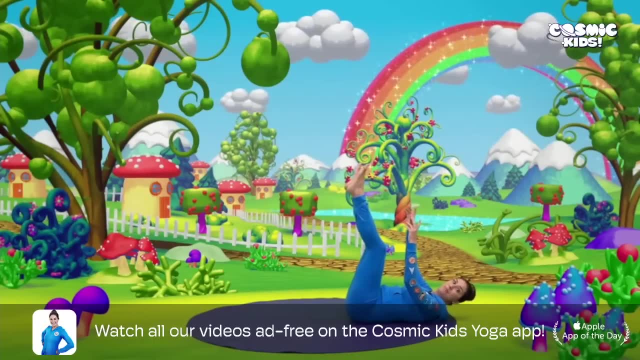 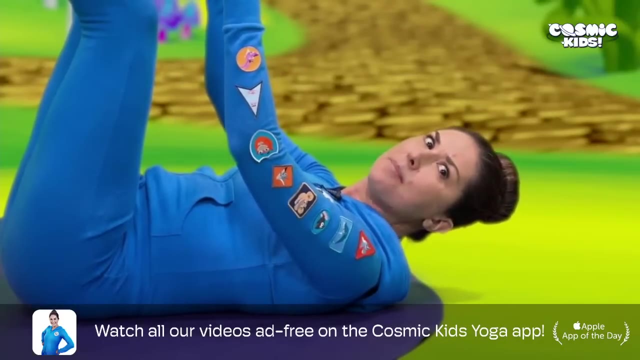 Biggles falls straight down, Rolling all the way onto our backs, Our legs and our arms in the air, And now he's at the bottom of a deep, dark pit. This hole was a trap, Covered in branches and leaves Set to capture Biggles. 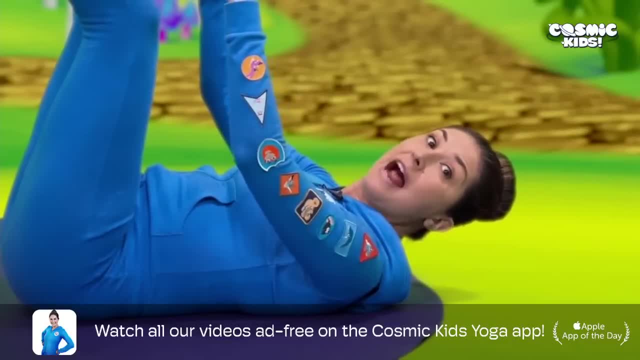 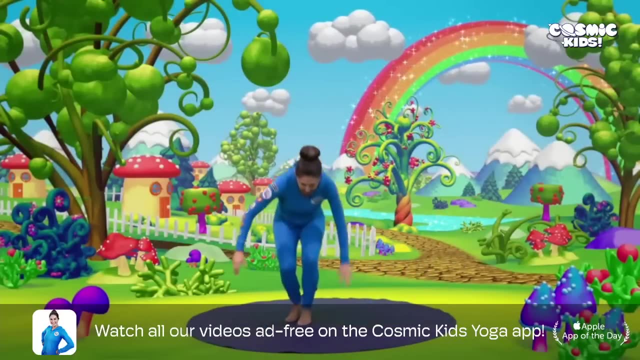 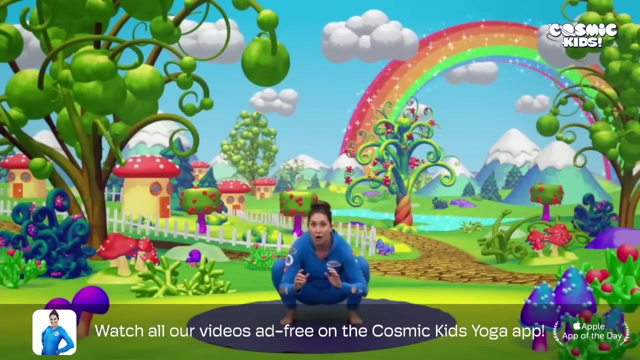 People from the nearby village Gather round the pit. They crouch to point and shout at Biggles Coming up to our crouch position, everyone. We take our feet a little bit wider And we squat all the way down, Snuggling our arms in between our legs. 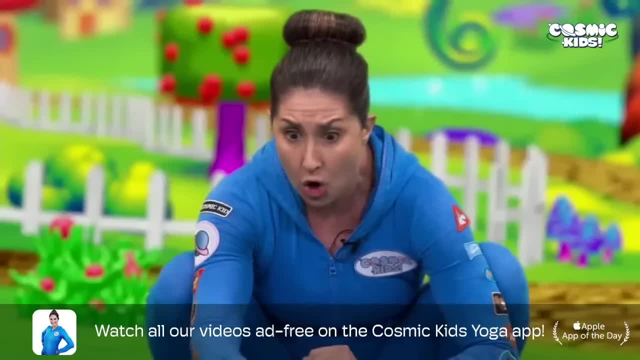 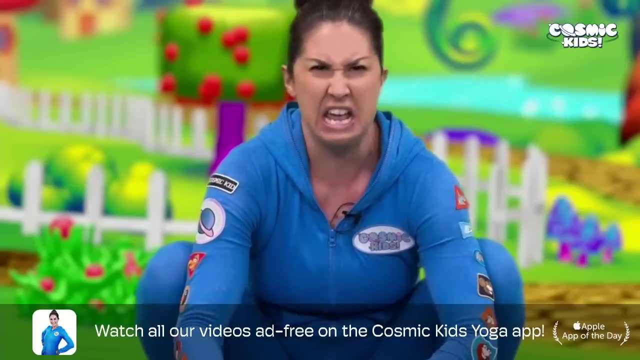 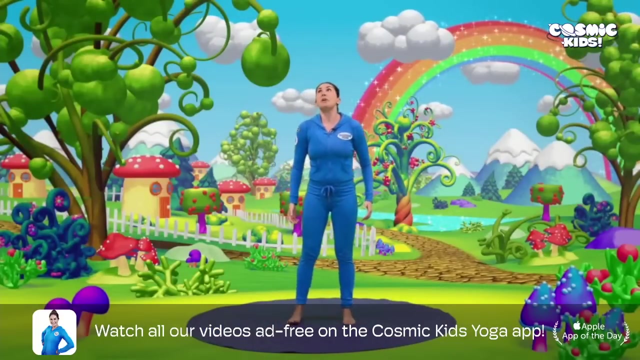 They're pointing and yelling at Biggles. Look, we caught the monster. He's a bit smelly, He looks a bit prickly, He's so ugly. Poor Biggles stands up And he looks up at them With confused and frightened eyes. 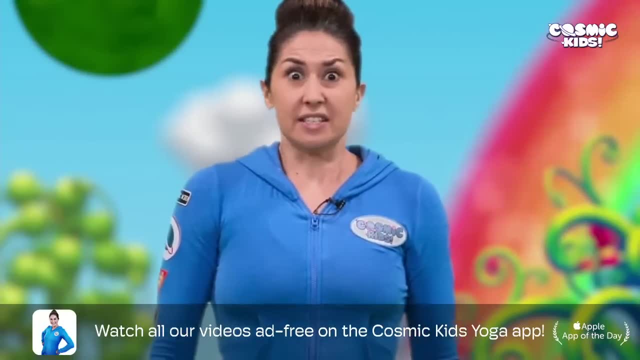 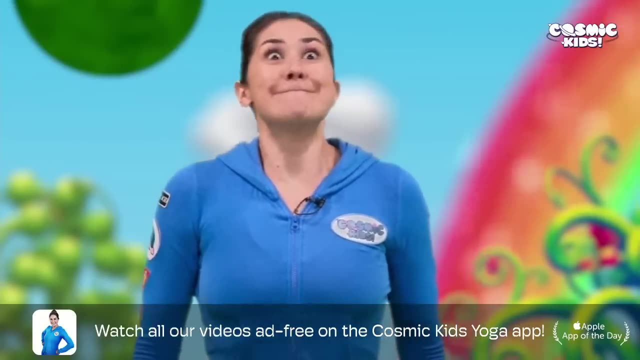 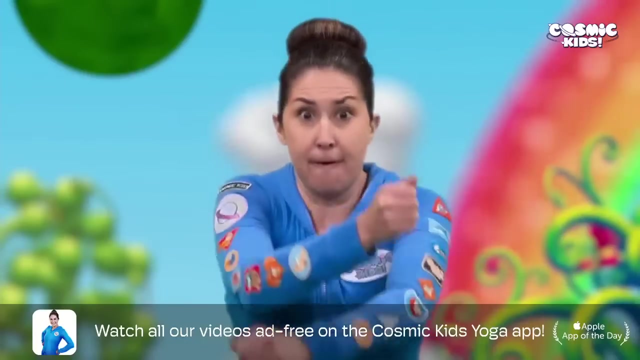 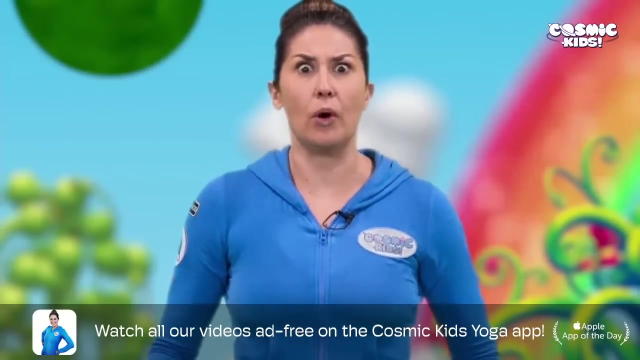 He doesn't know what to do, He doesn't understand them, So he smiles as best as he can And he says his word Biggles, And he knocks his sticks together To show them how lovely that sound is. A little boy lunges. 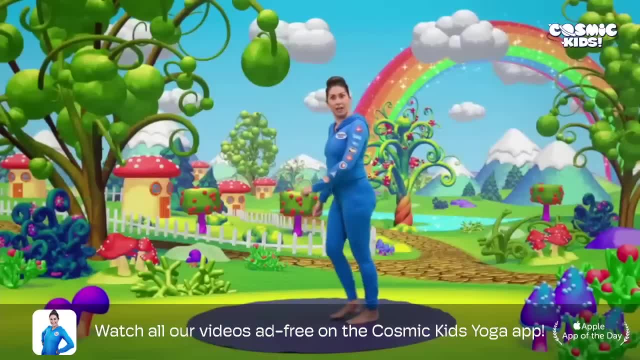 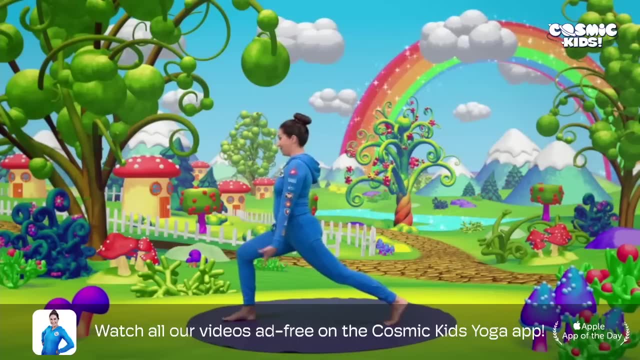 And throws a rotten mango at Biggles. Turning to the side, Stepping one foot forward and one foot back, We bend into our front knee. Now we stretch our arms all the way up, Trying not to wobble As we join our hands above our head. 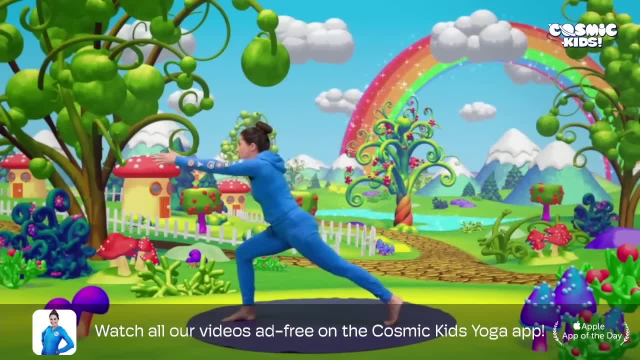 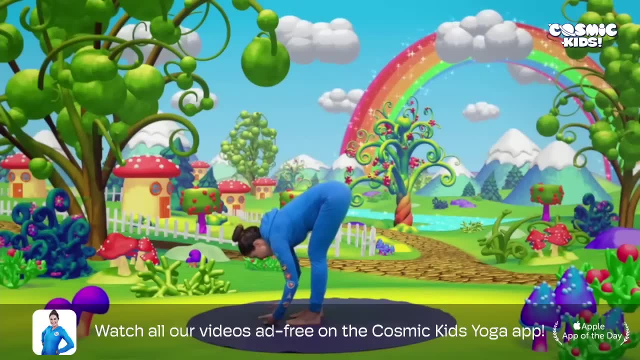 We lean all the way back And whoosh, There goes the mango. Biggles steps forwards And folds all the way down To pick the mango up. Criss-crossing our fingers, He lifts it up And he rolls it around. 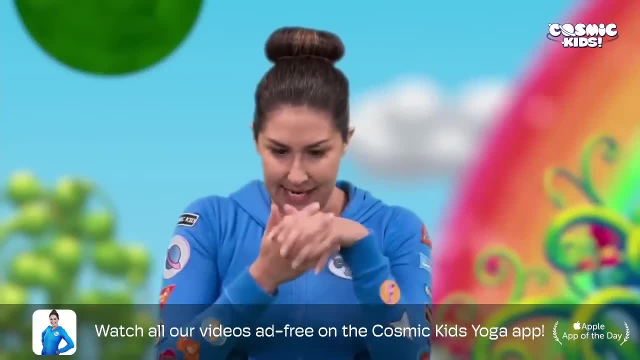 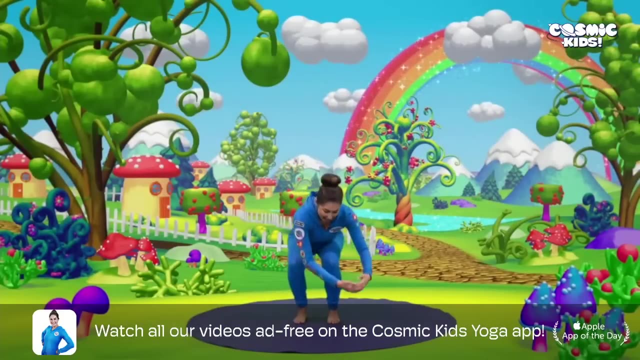 In front of his chest. He smells it. It smells really nice. So he bends very gently And he carefully places it beside him To keep it safe Coming all the way back up to stand. Now the villagers throw even more fruit at Biggles. 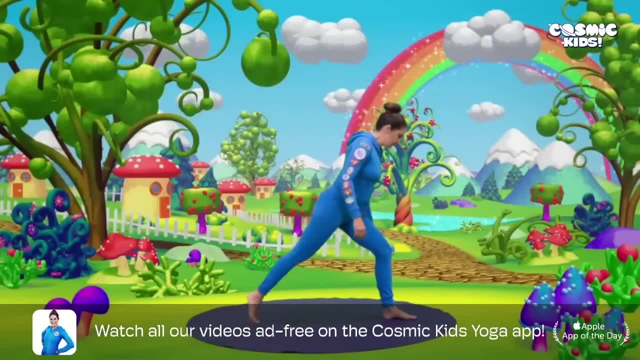 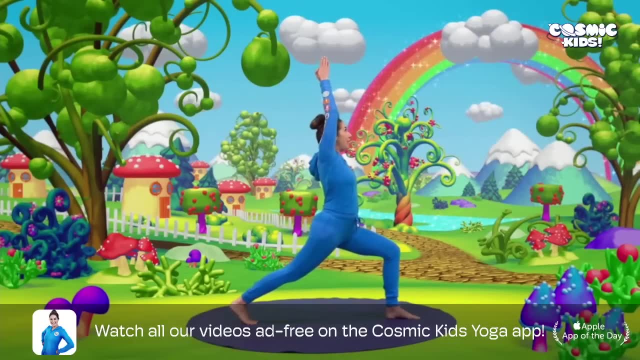 Let's lunge on the other side, Stepping one foot forward, One foot back. We bend into our front knee, Trying not to wobble As we reach our arms all the way up. We lean back And whoosh, Bruised bananas. 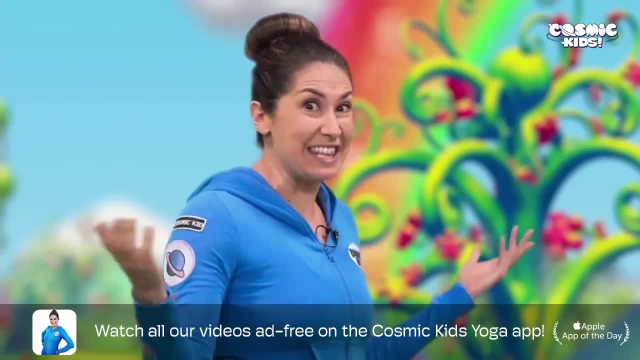 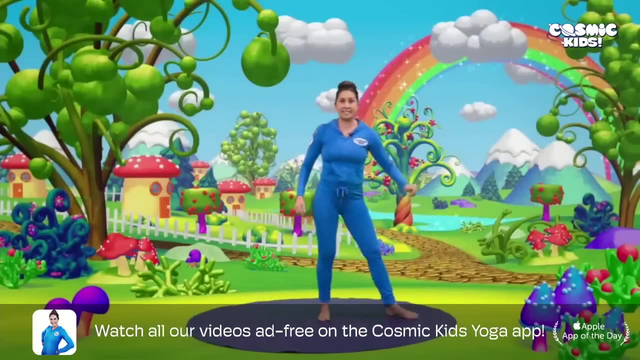 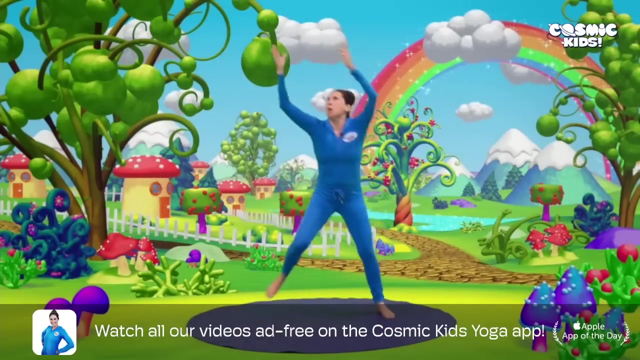 And apples- Poor Biggles, But he thinks they're gifts. So he hops from side to side Trying to catch them Coming up to stand. And let's hop side to side: Biggles, Biggles, Biggles, Biggles. 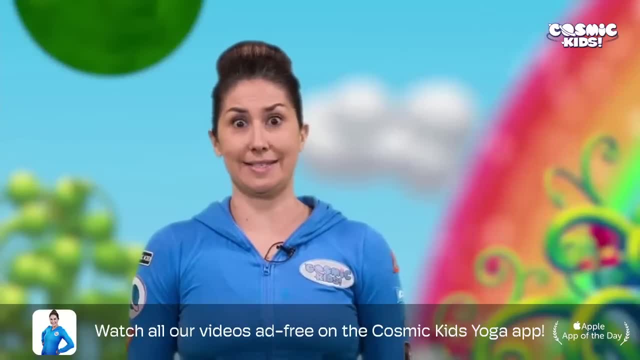 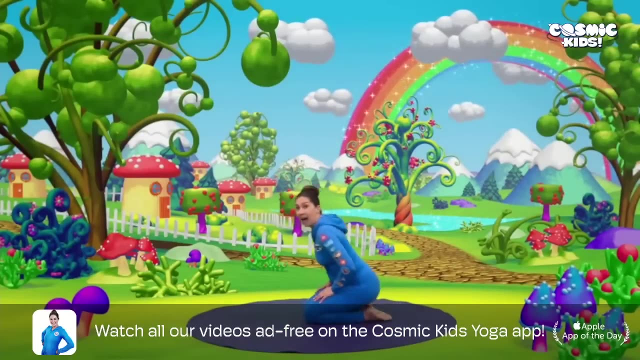 Biggles, Poor Biggles. Next they start to throw rocks at him. Let's do our rock pose: Coming down onto our knees, Untucking our toes, We fold all the way forwards To make ourselves into a little round rock shape. 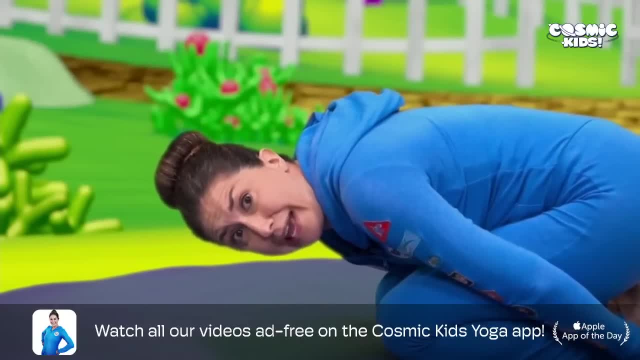 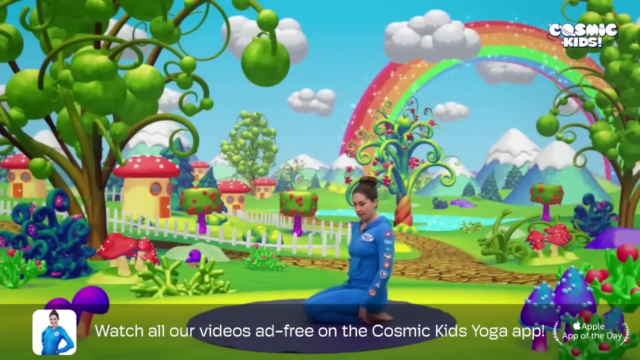 One of the rocks hits Biggles In the eye. He sits up And he blinks. He shudders at the shock of it. Then he picks the rock up, He has a look at it, He rubs it on his chest. 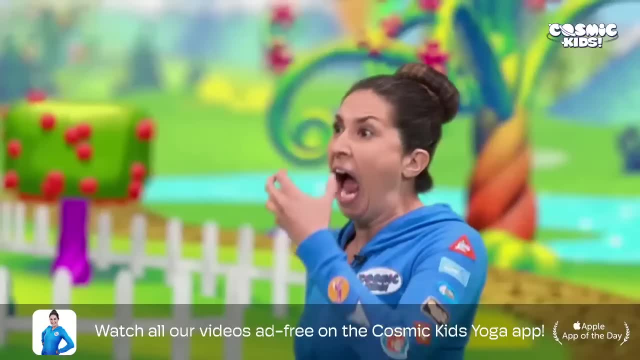 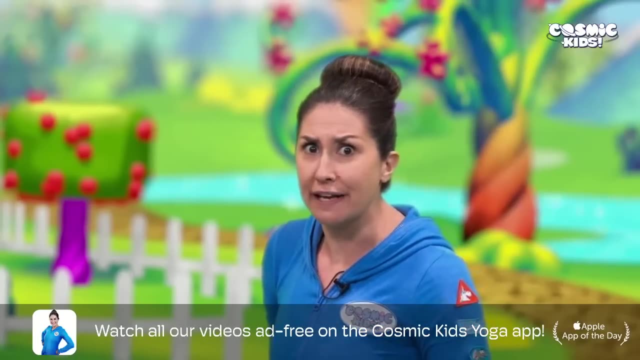 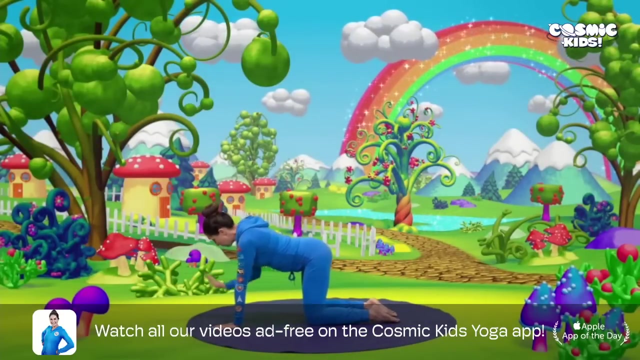 And he tries to take a bite out of it. A little girl is on her hands and knees Pointing and laughing at Biggles Coming onto our hands and knees, Stretching one arm forwards To look at Biggles Putting that one down. 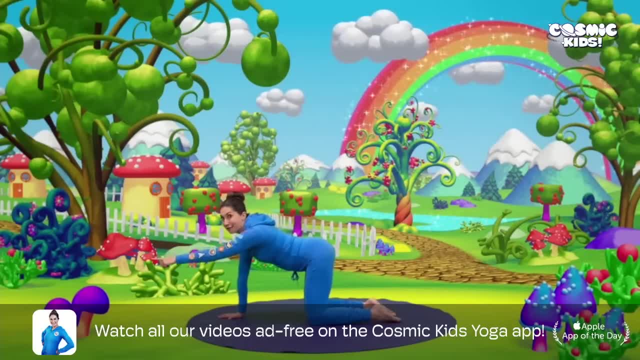 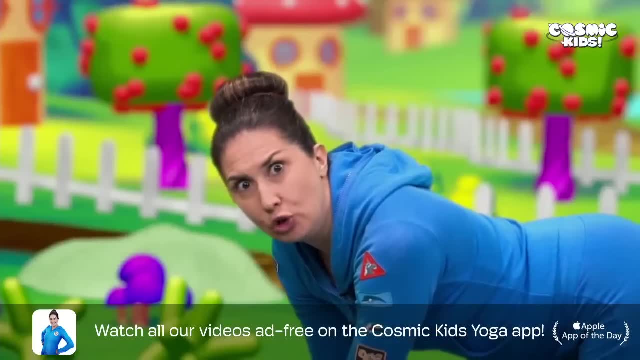 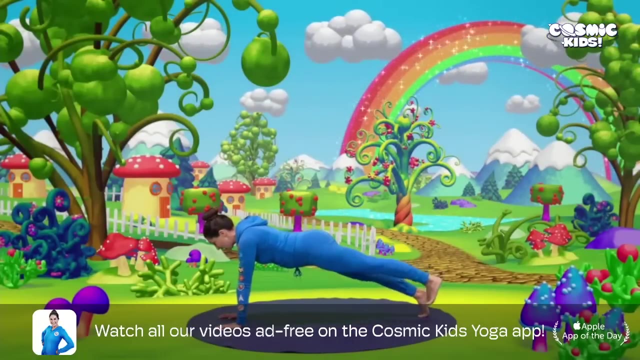 And the other arm forwards. She thinks he's very funny For trying to eat the rock. But she's laughing so much That she slips And she falls down the hole, Landing on her tummy. We stretch one leg back And stretch the other leg back. 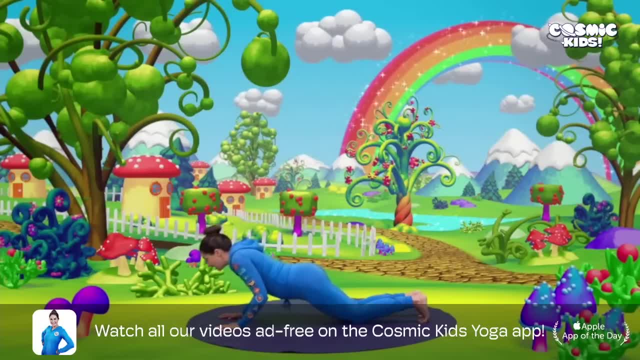 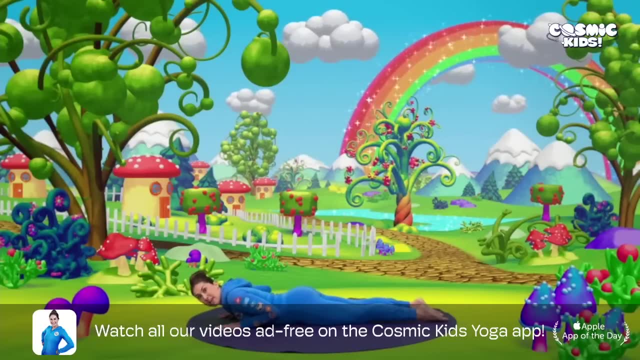 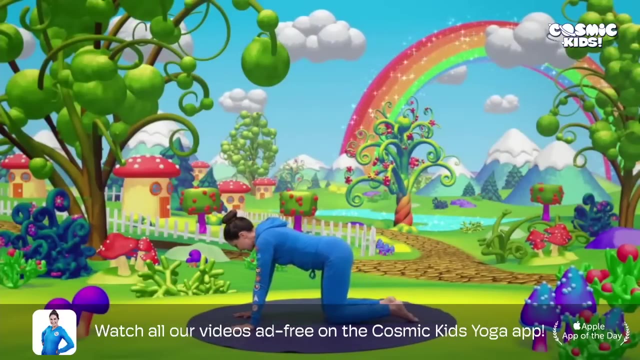 Now we lower our knees And slowly lower onto our tummy. Oh no, Now she's at the bottom of the hole With Biggles. The little girl's mum jumps up And screams, Coming up onto our hands and knees, Tucking our toes. 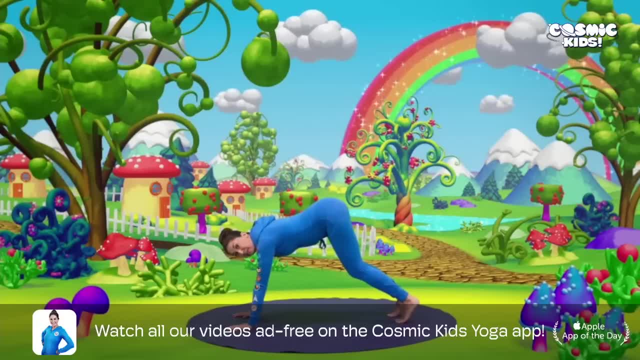 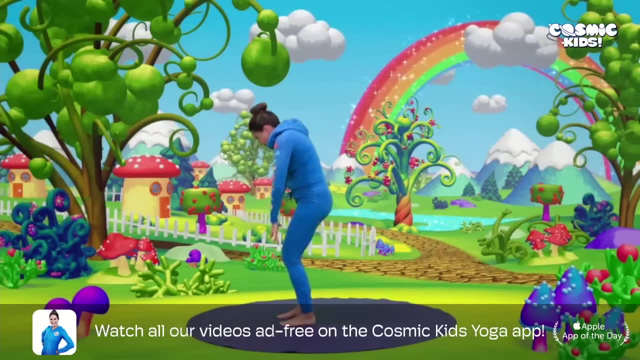 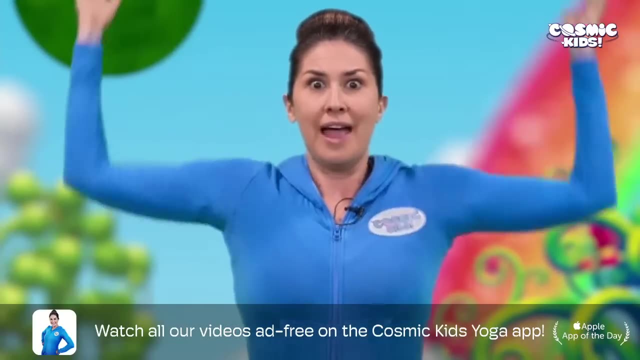 And pressing our hips up. Now we jump our feet forwards Towards, our hands Ready, One, Two, Three Boing Rolling up to stand. She reaches up: The monster has my child. What are we going to do? Everyone goes crazy. 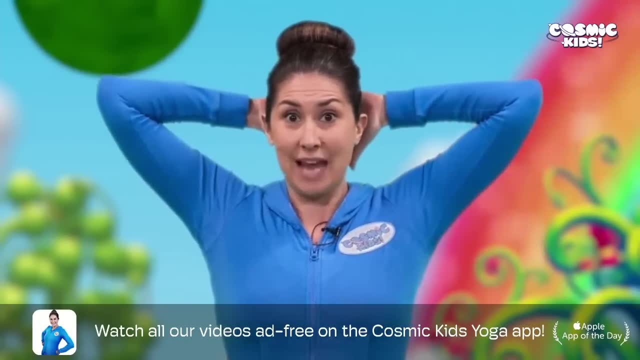 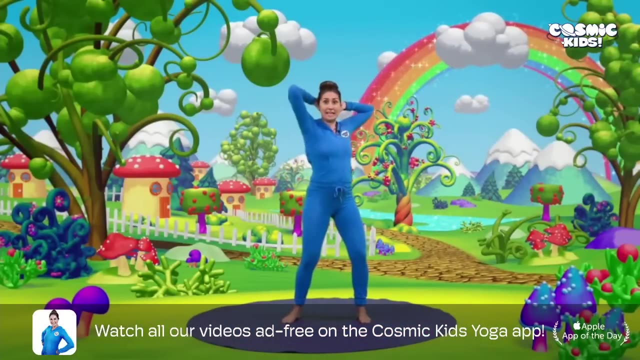 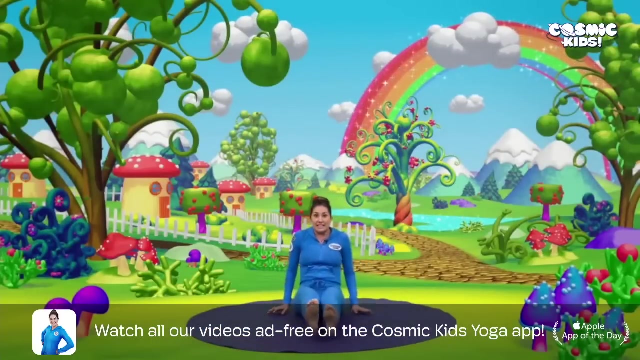 Criss-crossing our fingers, Popping them behind our heads And spinning From side to side. He'll eat her alive, He'll tear her to pieces, But Biggles does no such thing. He sits calmly With his legs out long in front of him. 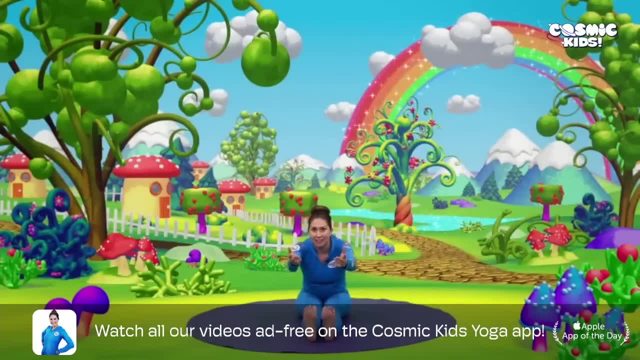 And he reaches forwards Towards the little girl, Checking that she's okay. He picks her up. Let's pick up one of our feet And cradle it in our arms. He's a bit worried about her. That was quite a big fall. 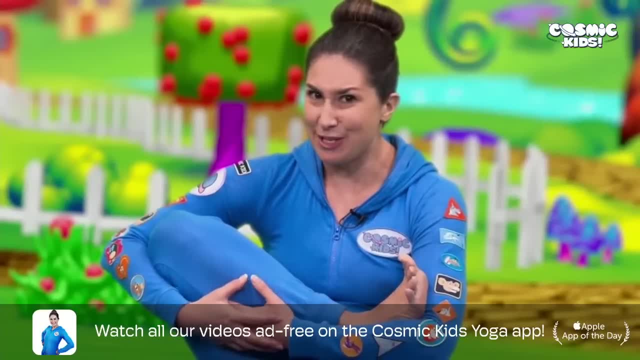 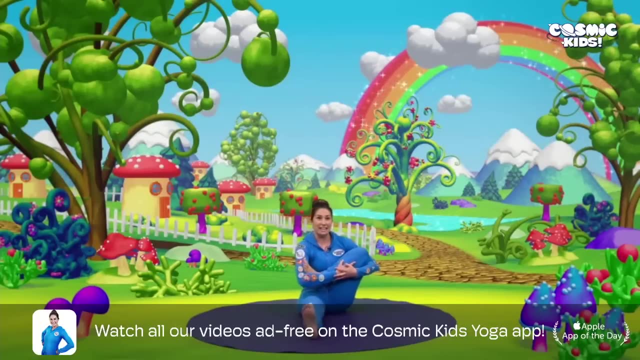 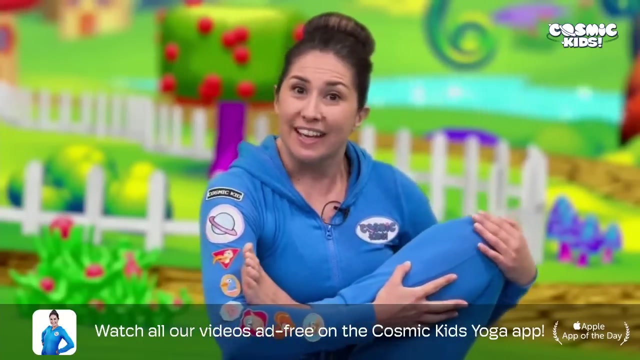 But she seems to be okay. Let's switch sides. Popping that foot down, Picking up the other side, Tucking it into our elbow And cradling on the other side With his big green, hairy hands, Biggles strokes her head. 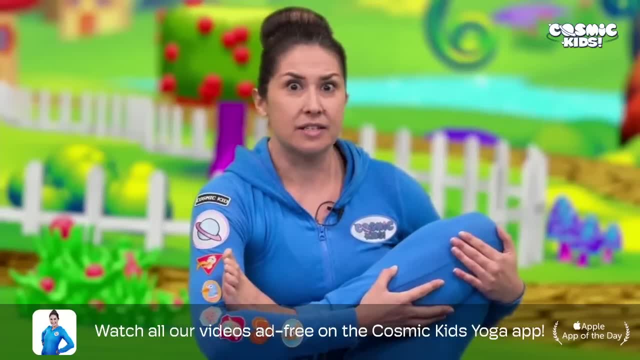 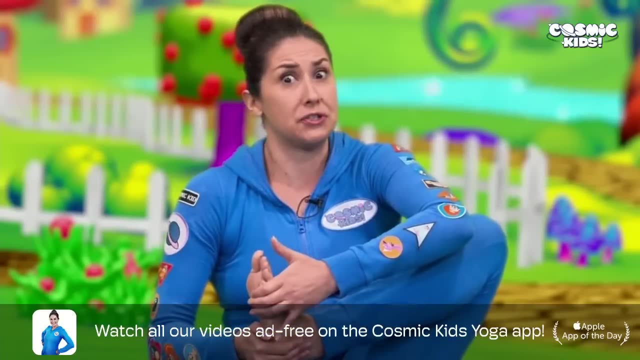 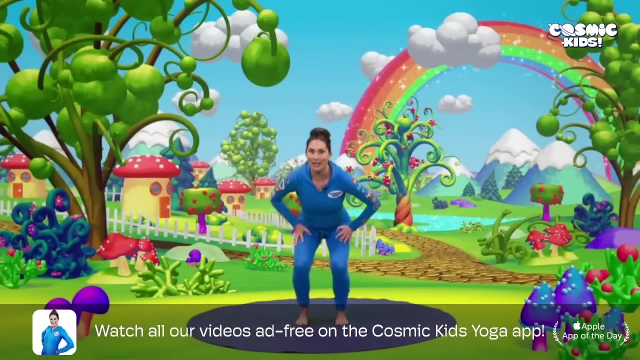 Checking, she's okay. Checking, she's okay. Someone shouts down from the top of the hole: Give her back. Biggles does so, Or tries to, right away Putting that foot down. We come up to stand Now we bend our knees nice and deeply. 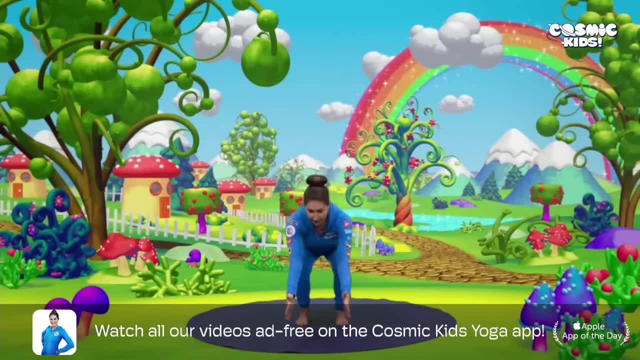 Reach our arms forwards Like we're holding the little girl, And as we come all the way up, He lifts, lifts, lifts Up onto his tippy toes, Trying to get the little girl To the villagers at the top of the hole. 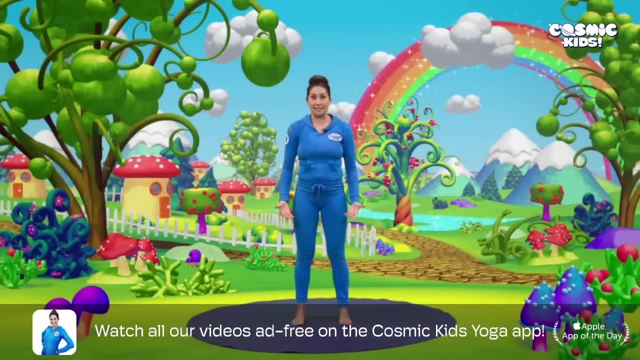 Coming all the way back down Onto our feet. The villagers fold forwards, Folding all the way down, Reaching down towards her To try and reach, But it's just too far Rolling up to stand. Next, someone has an idea. 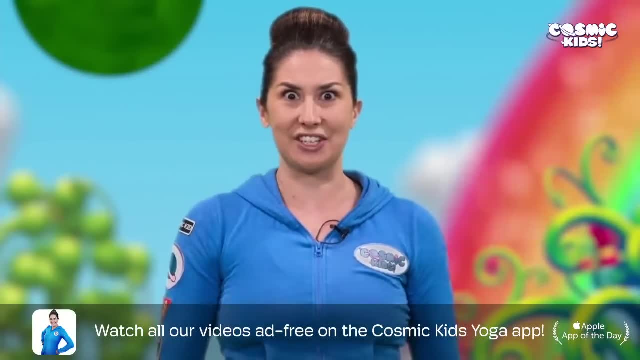 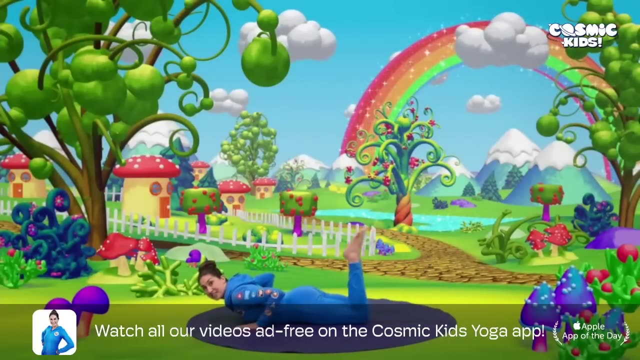 Let's fetch a basket With a rope attached to it. Coming into our basket pose, Coming down onto our tummies, We bring our feet towards our bottoms And we reach around to take our ankles. Now let's breathe in. Kick our feet into our hands. 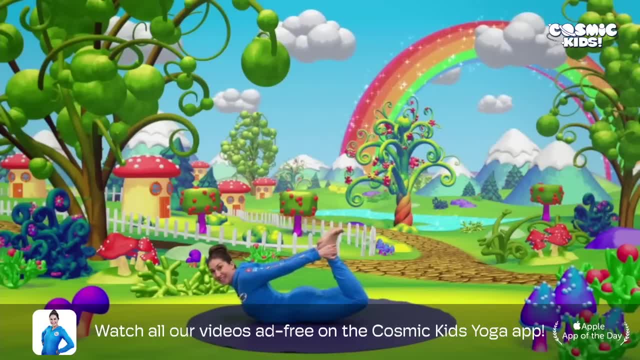 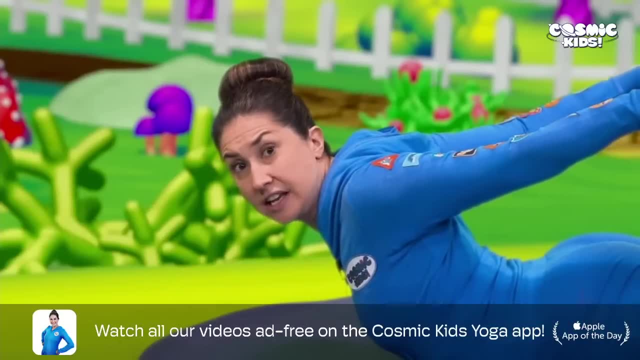 Here we go In our basket pose They're going to lower it down To get the little girl out. But some are worried: What if Biggles leaves the little girl in the pit And climbs up the rope himself? But Biggles does no such thing. 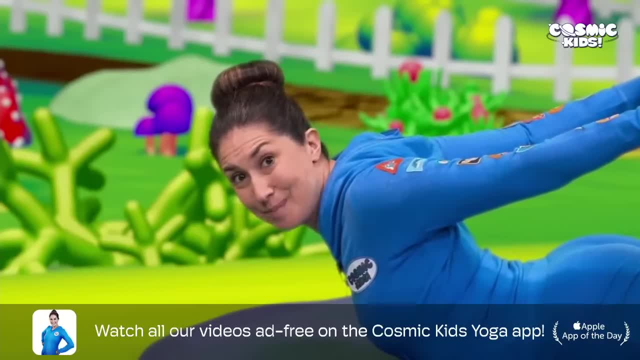 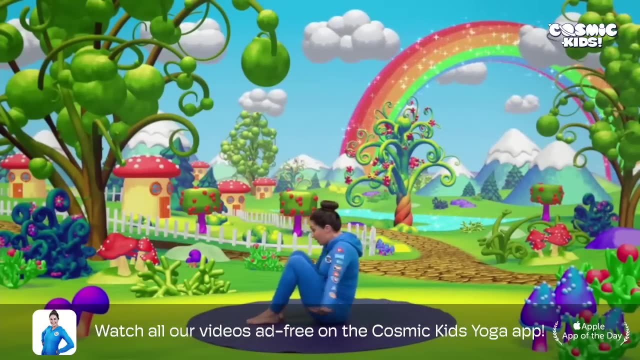 He carefully and gently helps the little girl Into the basket, Coming all the way to sit On our bottoms. We hug our knees into our chest, She snuggles into the basket, Wrapping her arms around her knees, And she's ready to be hoisted up. 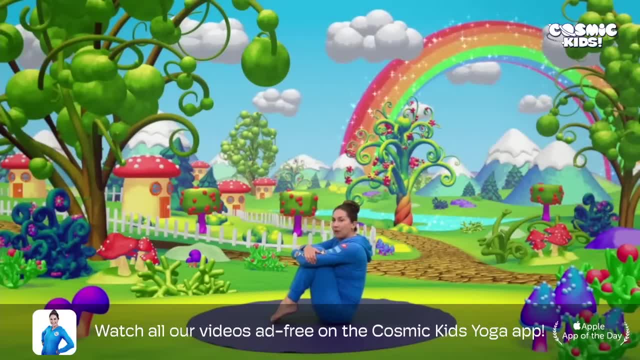 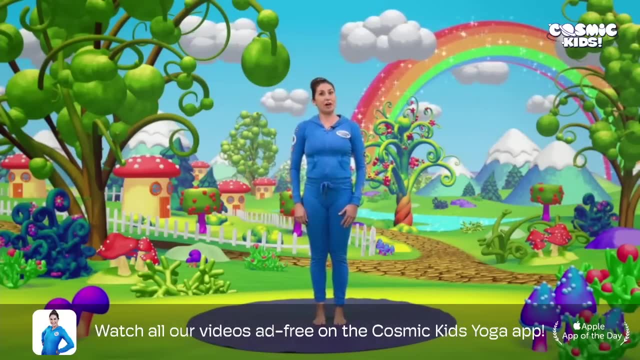 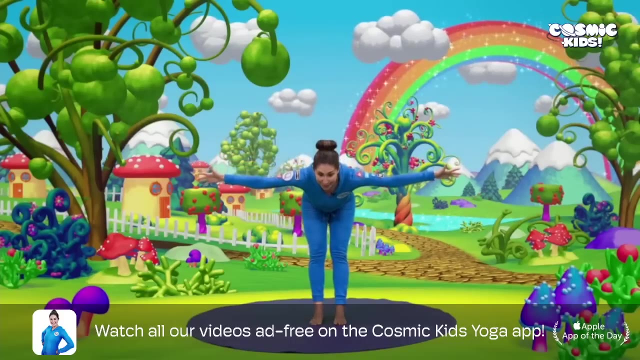 To the top of the pit. Now, once at the top of the hole, The little girl is out And she is safe. But instead of opening her arms out wide And turning to her mother, She folds all the way forwards Towards Biggles. 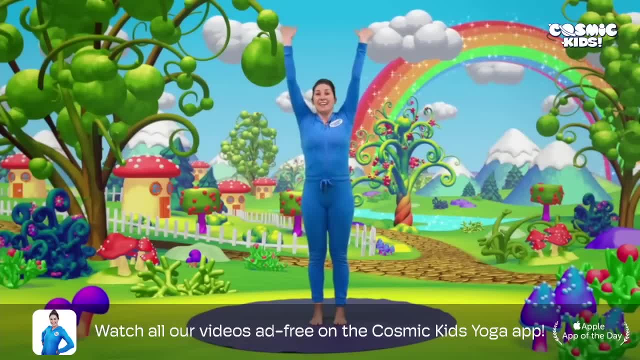 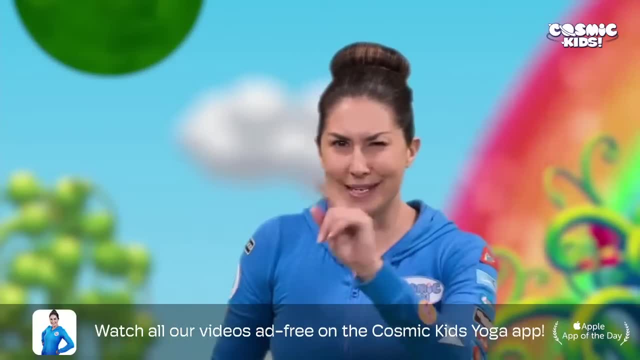 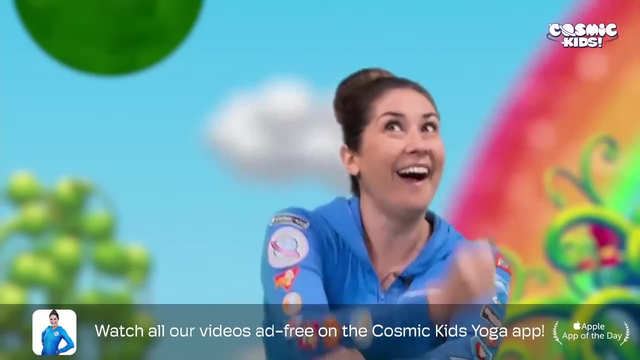 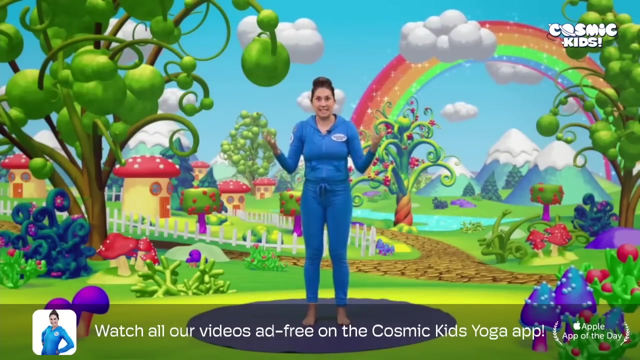 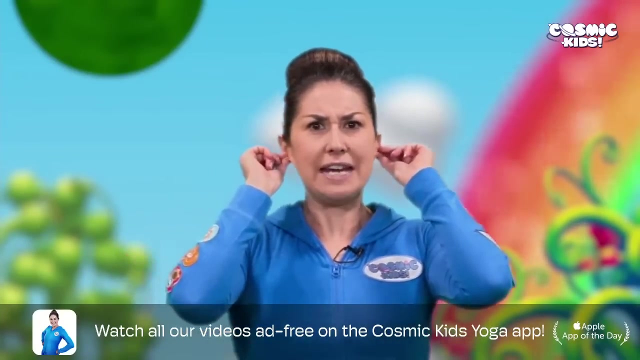 Biggles reaches all the way up And waves at her, Saying Biggles, And he plays his sticks again, This time playing a little tune. The villagers listen, Rubbing our ears. Wow, This monster Is actually very clever. 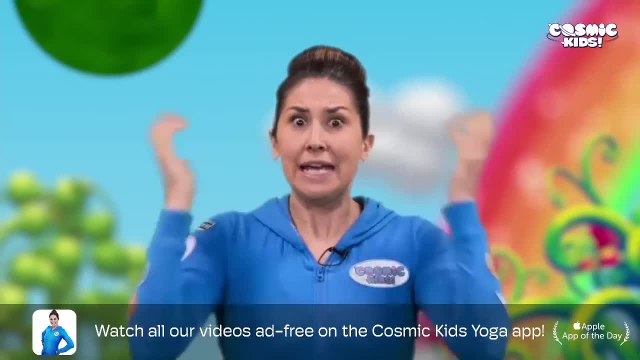 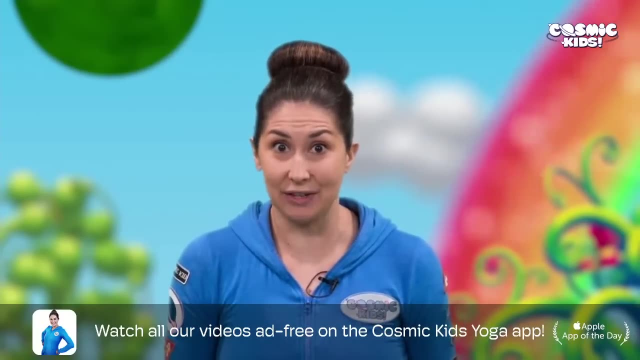 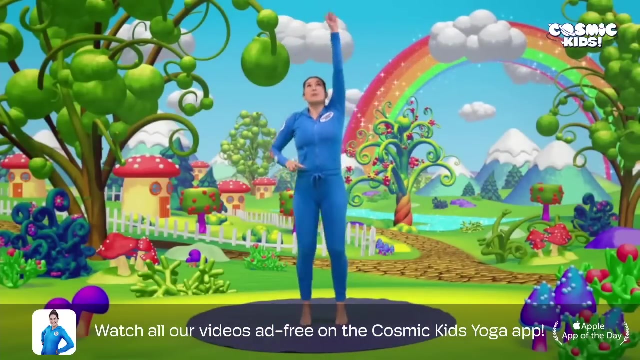 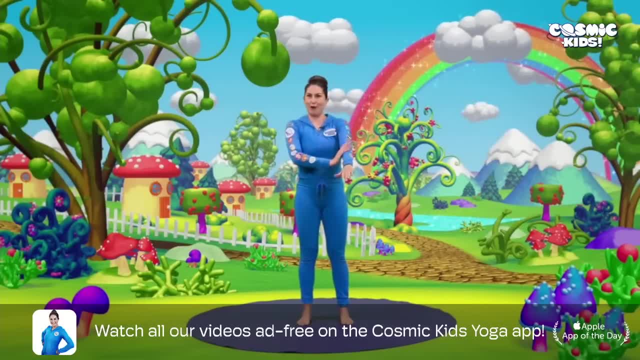 Biggles, Biggles. Once at the top, The villagers stroke Biggles. Let's stroke our arms And stroke our legs. They love his green, spiky hair. Then they give him a big hug, Arms wide, Wrapping our arms around. 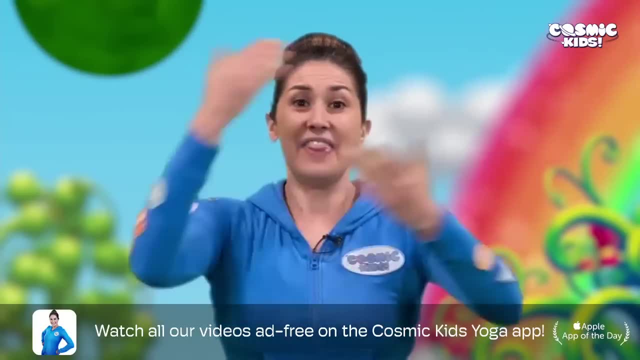 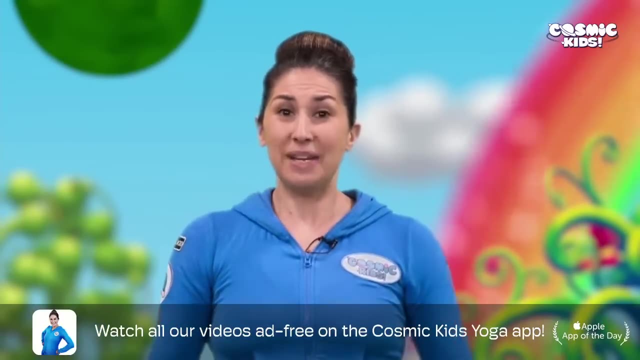 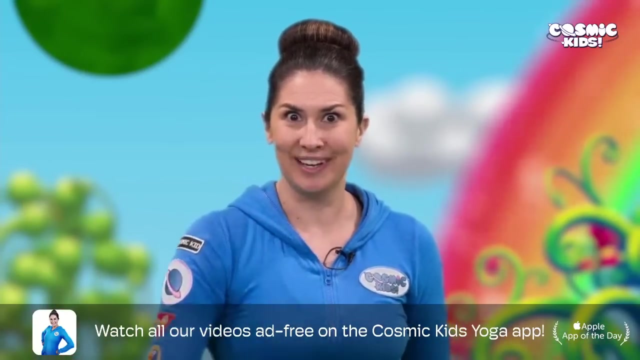 They give him lots of lovely fresh fruit to eat And they welcome him into their community. Now Biggles might look like a monster, But he's kind And thoughtful And sensitive, Just like you. Let's spend a moment now Lying down. 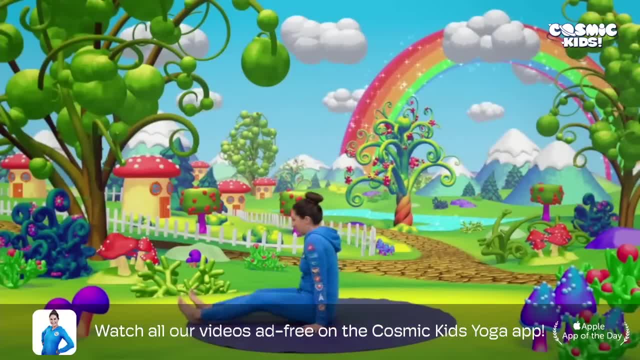 Coming to lie on our backs, Legs long, Arms down by our side, And take a moment to rest, Relax And have a little think About our story, About Biggles the monster. We take a big, deep breath In through our nose. 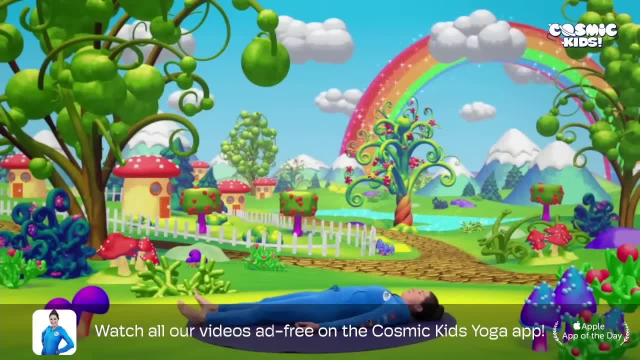 And out through our mouth, And again In through our nose And out through our mouth. What an interesting story. Sometimes, When someone appears Different to us, We might be afraid of them, Unsure, But as we've learnt in this story, 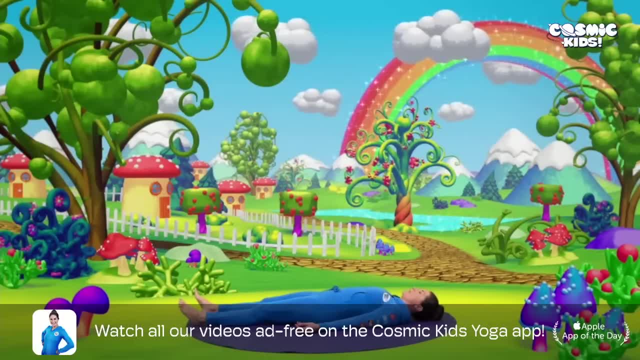 That's probably not the right thing to do. In fact, Just because someone is different Doesn't mean we should be unkind. It means we should be even more kind. We should get to know each other, Learn to understand the world. 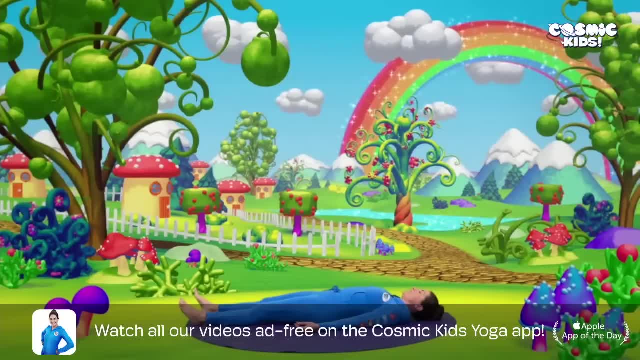 From someone else And to be kind To understand the world From someone else's point of view. In our lives We will meet lots of different people Who are very different to us. Be kind, Be thoughtful And do your best. 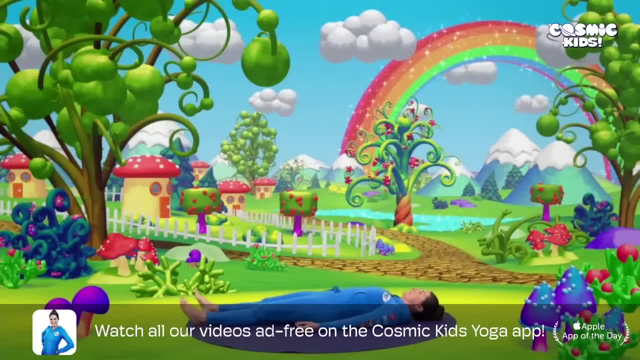 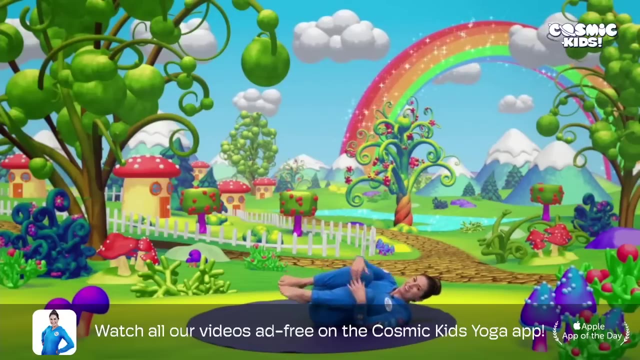 To make friends. Slowly now We begin to wake up, Wiggling our toes And wiggling our fingers, Hugging our knees into our chest And then rolling onto our sides As we open up our eyes And come to sit with our legs crossed. 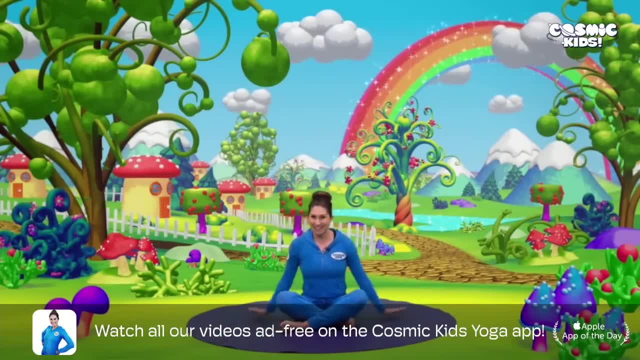 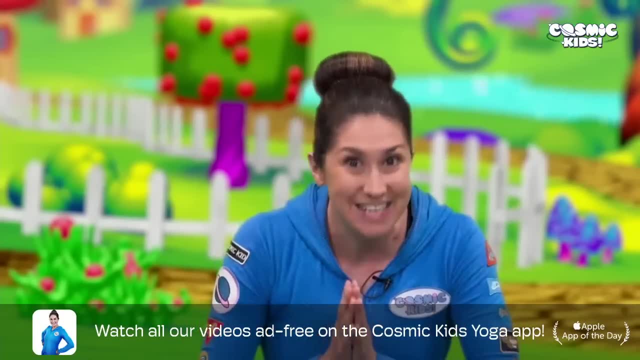 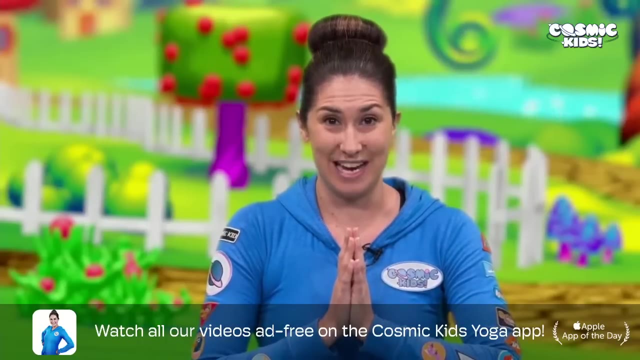 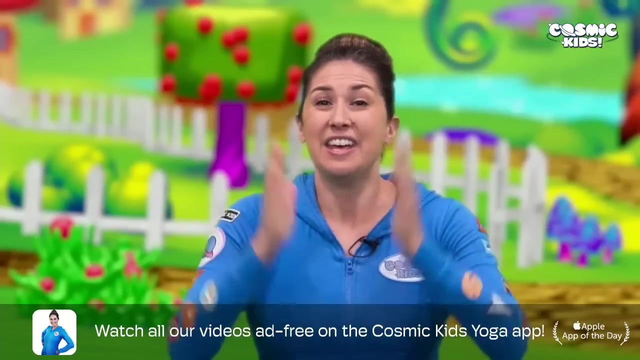 Finishing just the way we started, With our hands together at our hearts And our secret yoga code word, Which is Namaste, Ready After three, One, Two, Three, Namaste. Wow, You were great in the story about Biggles the monster. 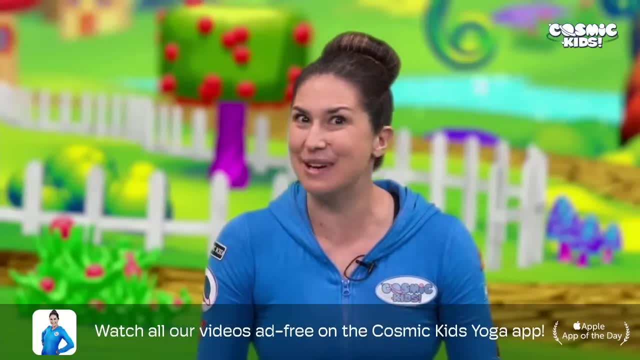 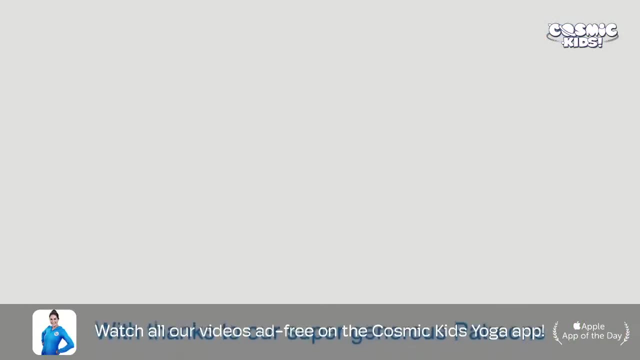 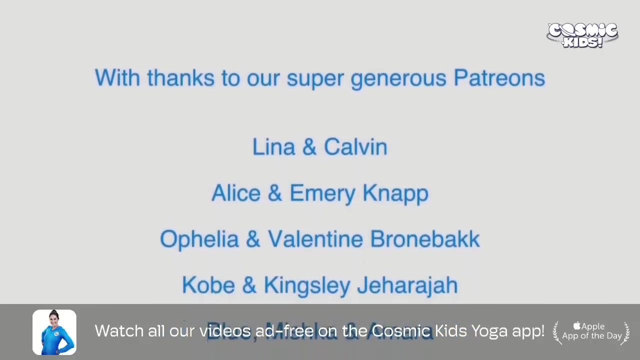 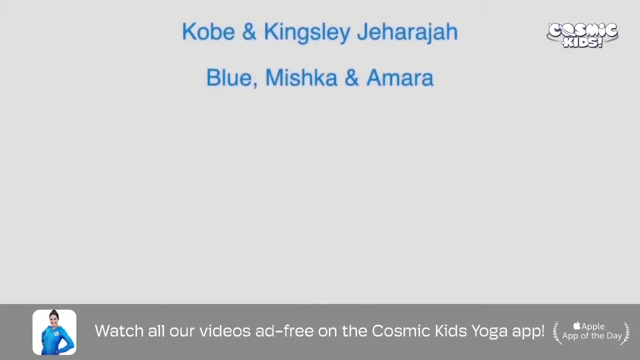 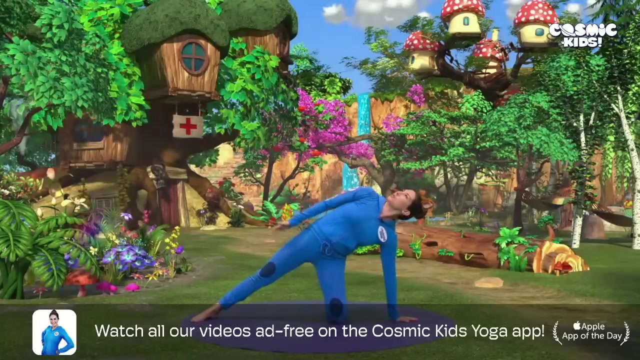 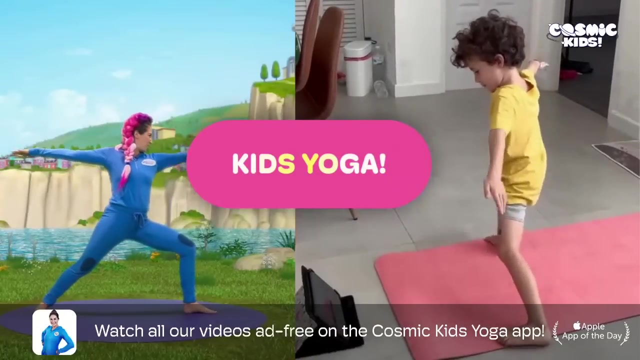 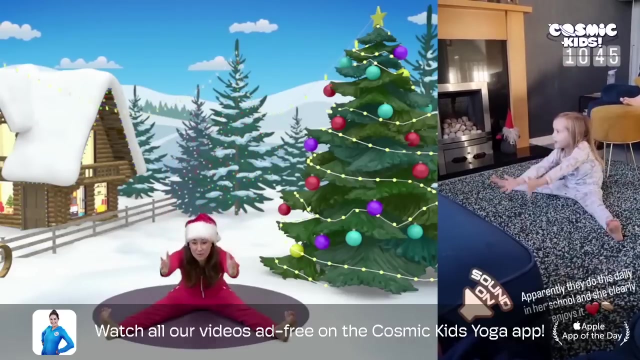 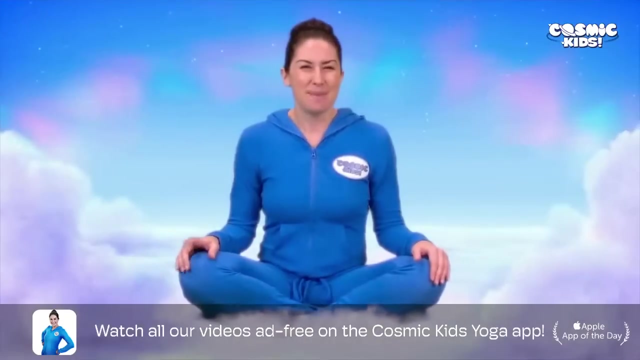 I hope you enjoyed it And I hope to see you again soon For another Cosmic Kids adventure. Bye, bye. Subtitles by the Amaraorg community. So what is it? what is mindfulness? How do we do it? And the best way to make the. I can't thought, go away. 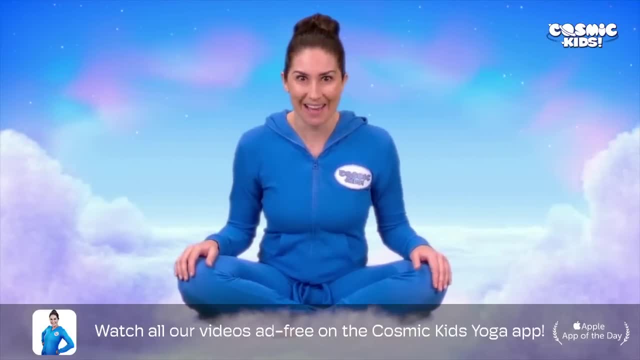 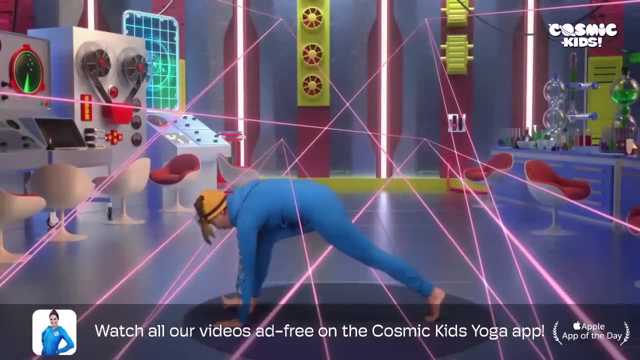 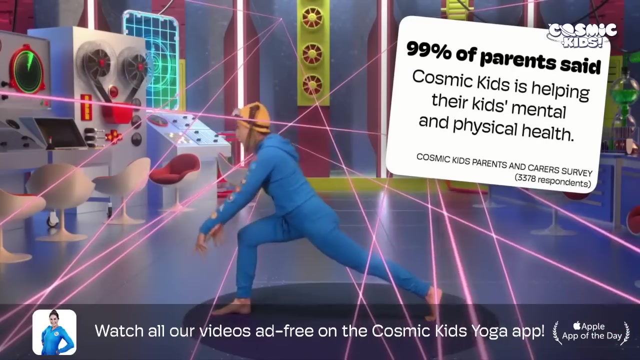 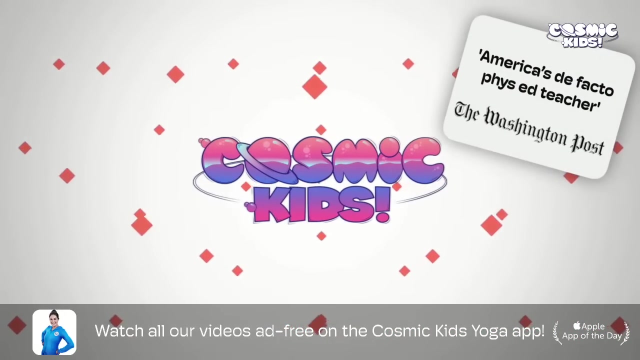 Is to think: Oh, yes, I can We step forward between our hands? Oh, thank goodness, we do yoga Now, making our legs very strong. We lift all the way up, Trying not to wobble, wobble, lifting our arms up to the sky, and then we fold all the way forwards. 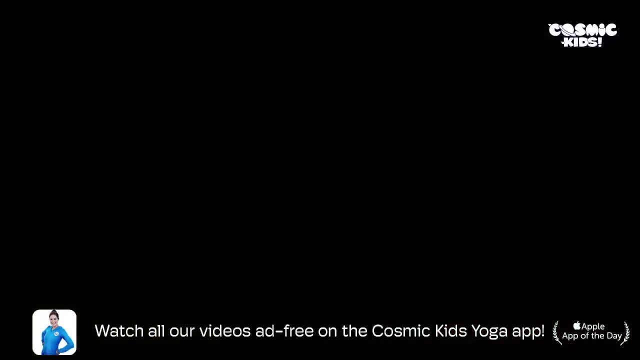 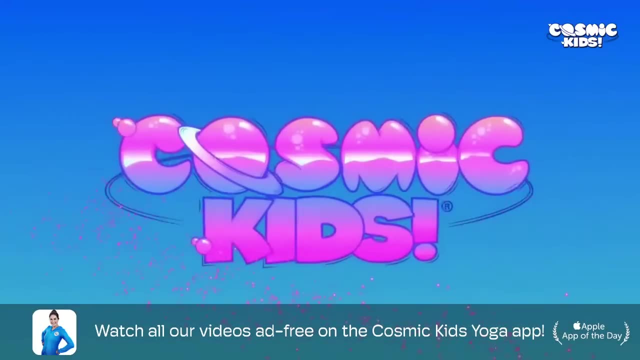 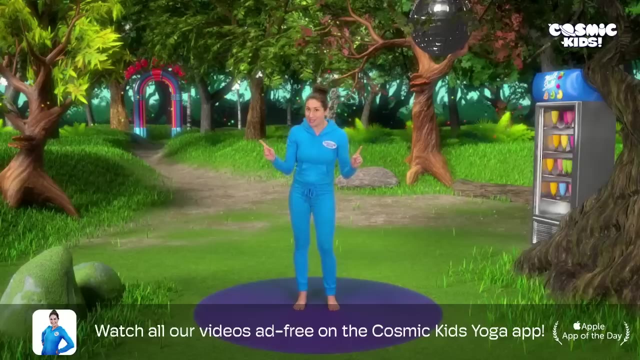 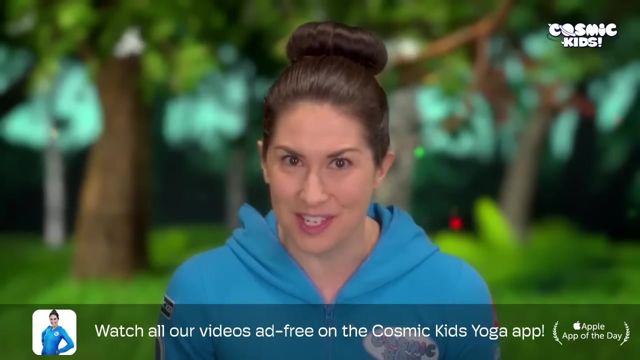 hands come either side of our foot. hello everyone, welcome to cosmic kids. I'm Jamie, and this is your place for yoga stories and fun. it's easy: just copy the moves I do and enjoy the adventure. now, we always start in the same way, and that's by sitting on our 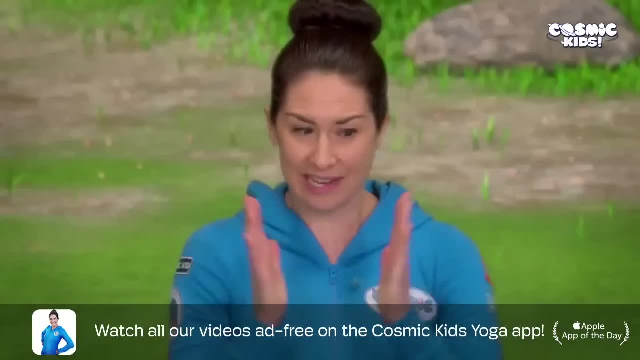 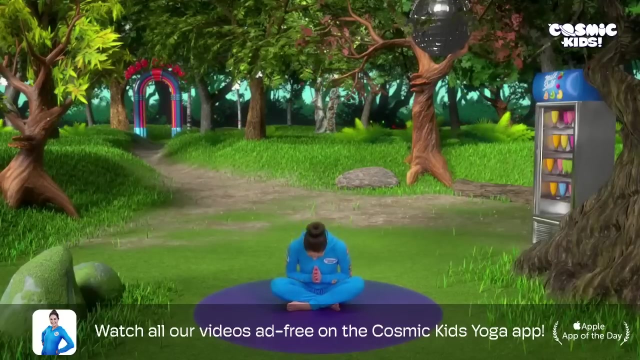 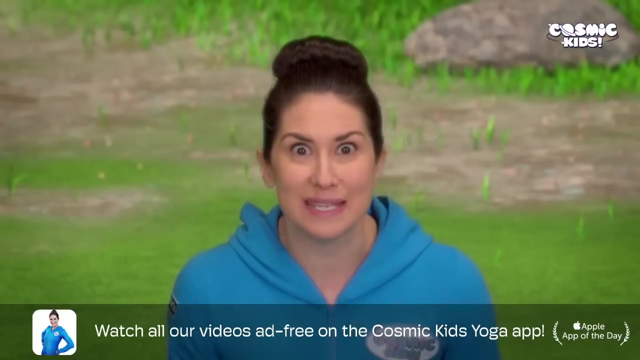 bottoms, crossing our legs and bringing our hands together at our hearts and saying our secret yoga code word, which is namaste. ready after three: one, two, three, namaste. there now let's have a look through our cosmonoculars and find out who we're meeting today. 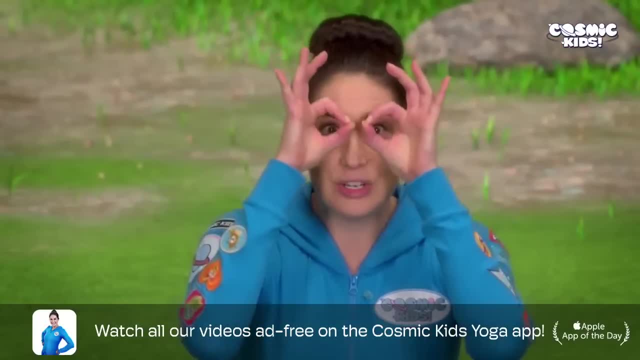 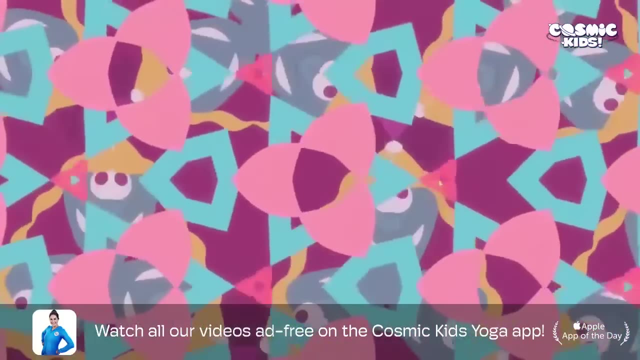 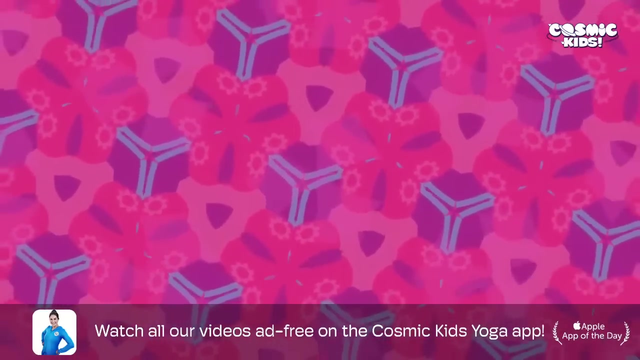 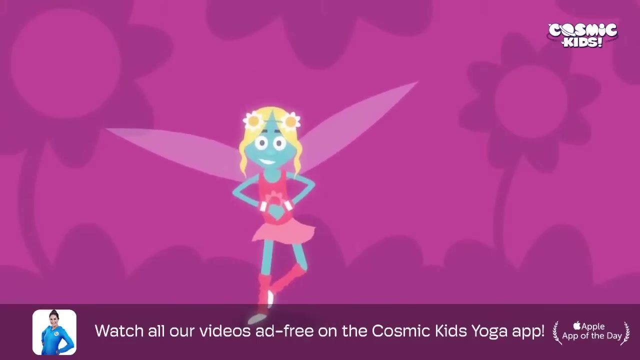 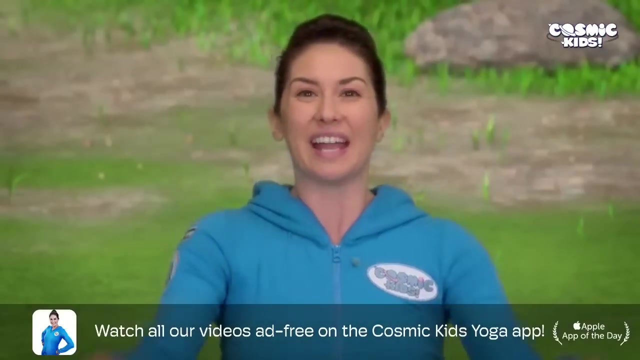 joining our thumbs and fingers together. we have a look through the patterns all going round and round. can you see it, the picture? it's fairy floss. oh, what's fairy floss doing? oh, of course, look, she's doing the floss dance, lowering our hands all the way down. how exciting. we're off to meet fairy floss a. 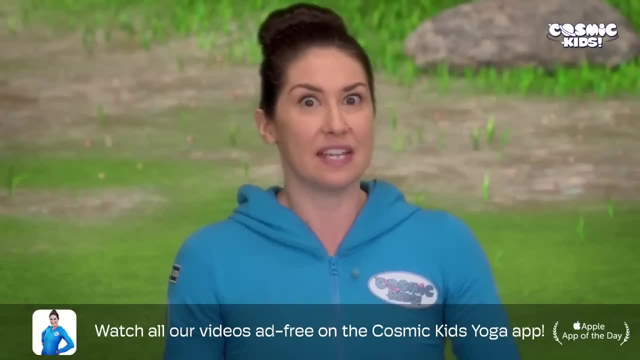 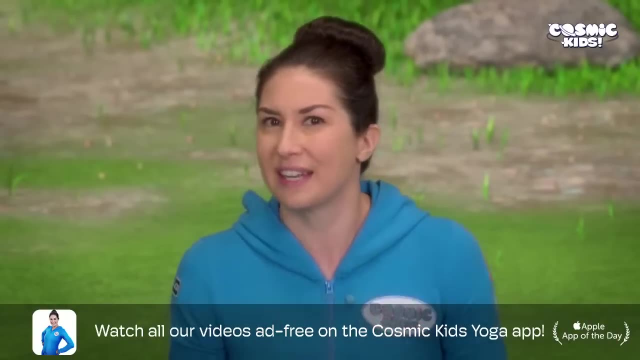 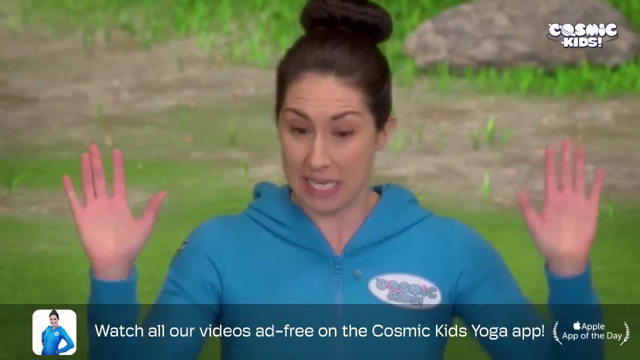 real-life fairy. now, fairy floss lives in pixie patch, which is home to a community of magical folk who love nature and the simple things in life, mostly dancing. let's come up to stand without touching our hands on the floor ready. well done everyone. now fairy floss, as you've already guessed. 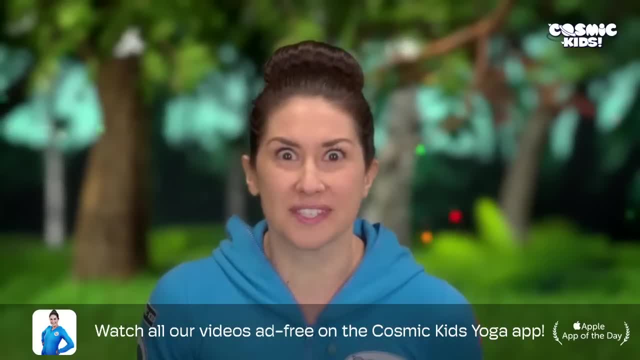 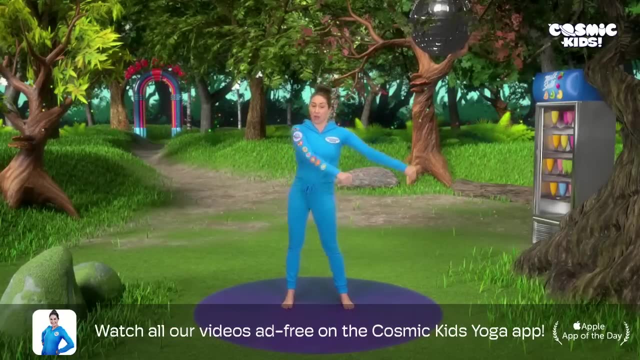 loves one dance in particular: the floss. let's try it. we take our arms down in front of us and make our hands into fists. now we count: one to the side, two to the other side and through front and back. let's do that again: one to the side. 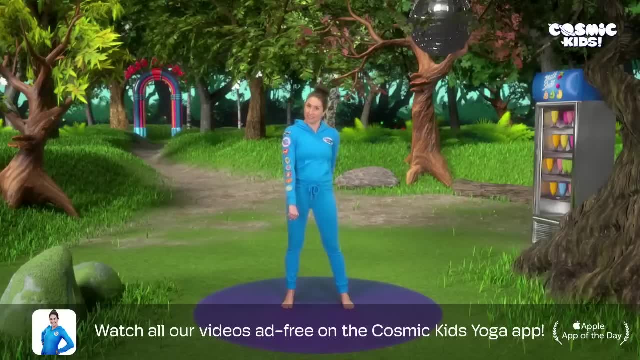 two to the other side and through front and back. and again one, two, three and again one, two through, one, two through, one, two through. yay, we've got the arms. now let's try the hips. let's bring our hands onto our waist and our hips go side to. 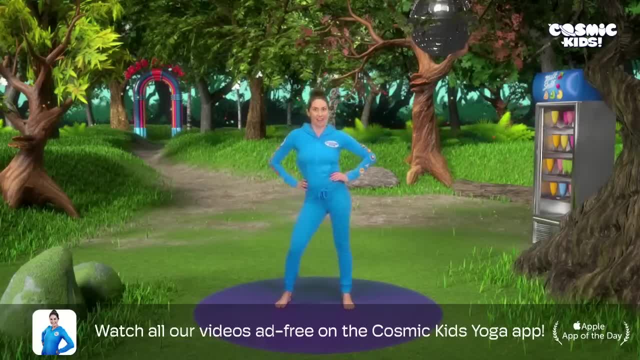 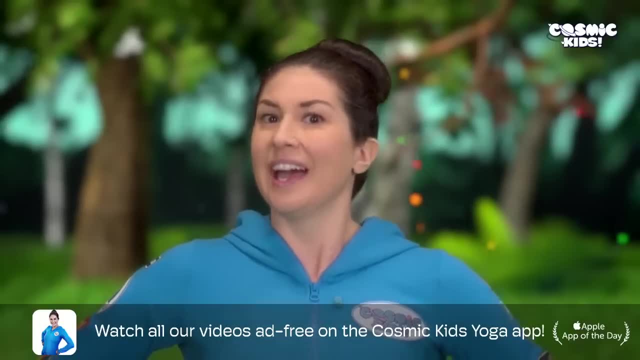 side. we can add a little bend of the knee as well to help. yay, now we're gonna try and put the arms and the hips together. we're gonna start slowly and build up speed, taking our arms down hands into fists. now our arms go one way as our hips. 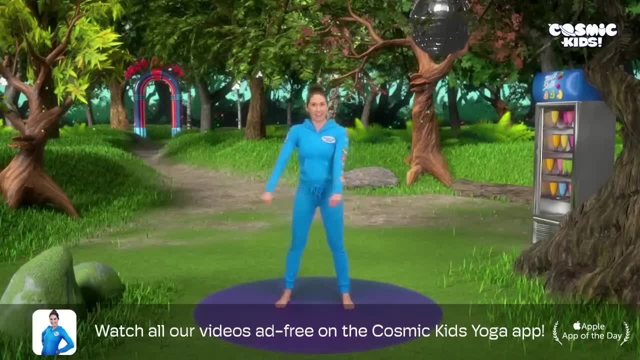 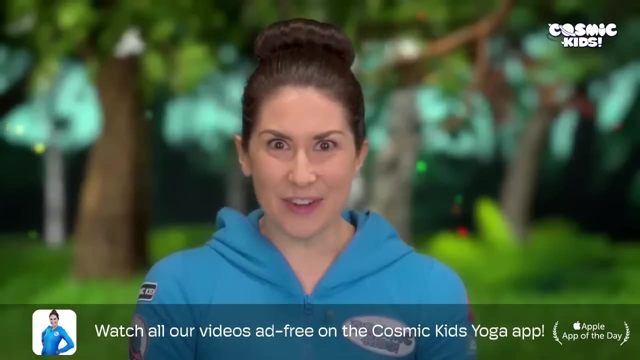 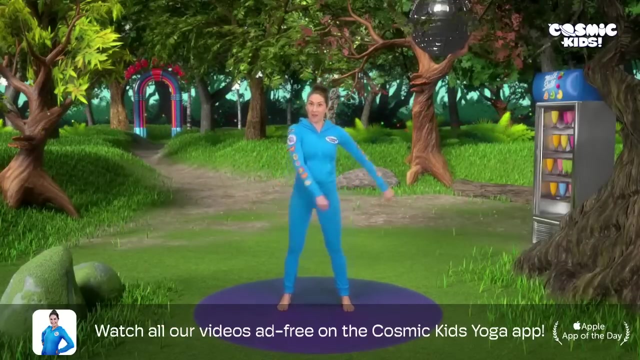 go the other. here we go: one, two, three, and again one, two, three. yea, here we go: one, two, three. one, two, three. let's try a little bit faster. here we go: one, two, three, one, two, three, One, two through. We're getting it. That's it. We're getting it. Keep going. 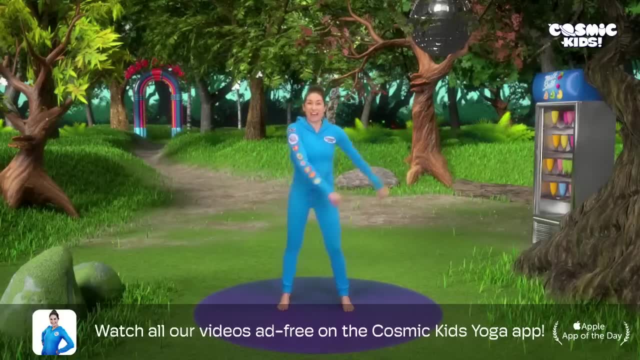 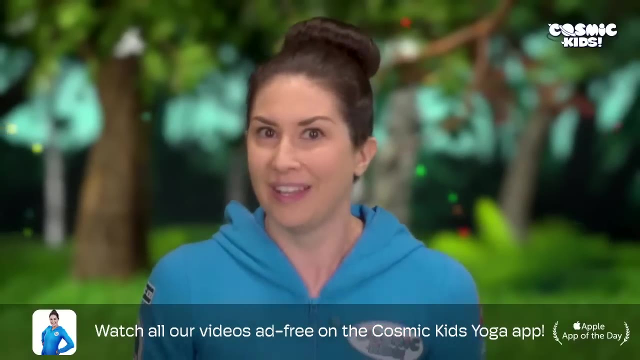 And we are flossing. Fairy Floss, do, do, do, do, do do, Fairy Floss, do, do, do, do, do do, Fairy Floss, do, do, do, do, do, do, Fairy Floss. Woohoo, Now, every week Fairy Floss arranges a big dance. meet up at the brilliant Bubble Club. 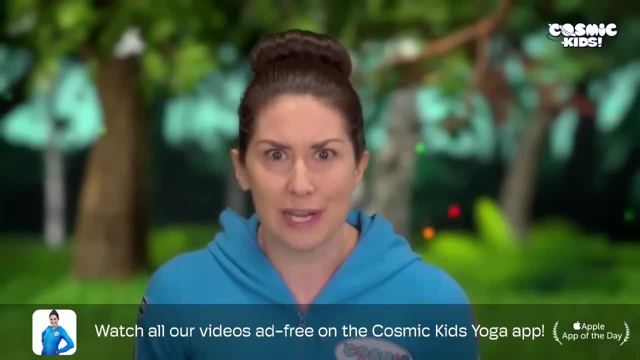 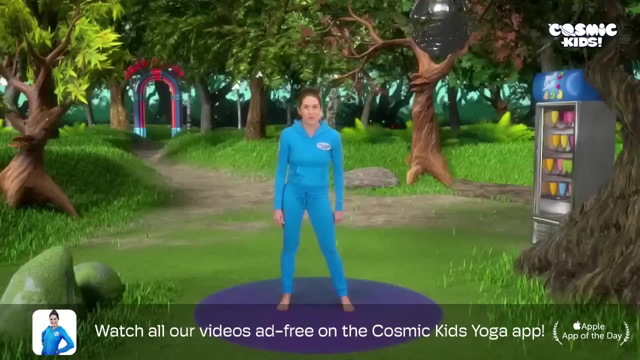 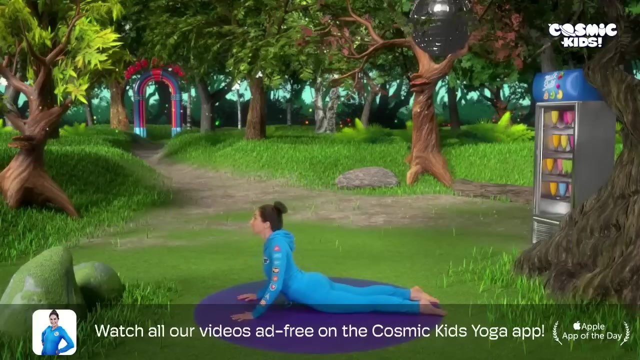 The Bubble Club is a place to dance, to laugh and to drink milkshakes and it's run by none other than Wonky, who is a worm coming into our worm pose. We lie down on our tummies and we bring our hands under our shoulders and we wiggle, wiggle, wiggle, wiggle all the way up like a worm. 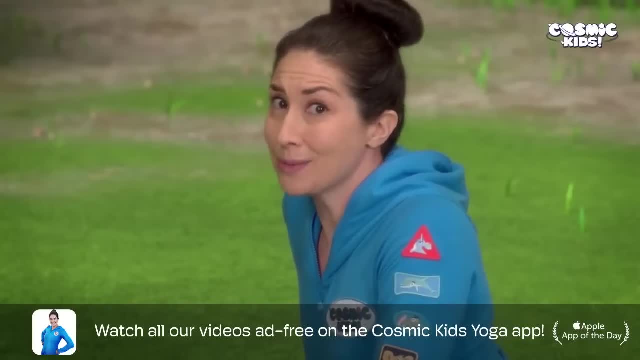 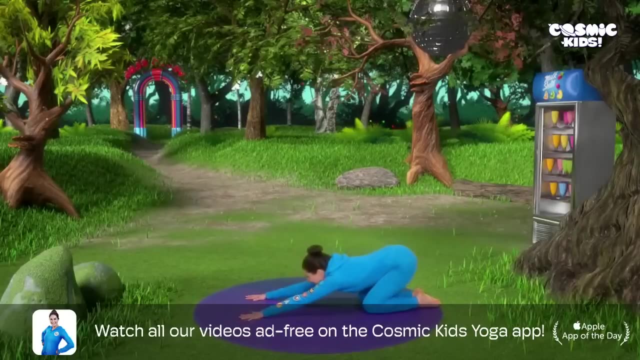 Now Wonky makes a mean milkshake. He's also got his own special dance move, known as Wonky's Wiggle. Let's try, We sit back on our heels, then we slide our body through and we wiggle on up like a worm. 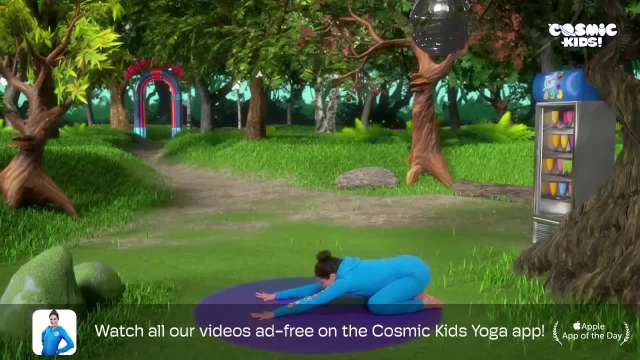 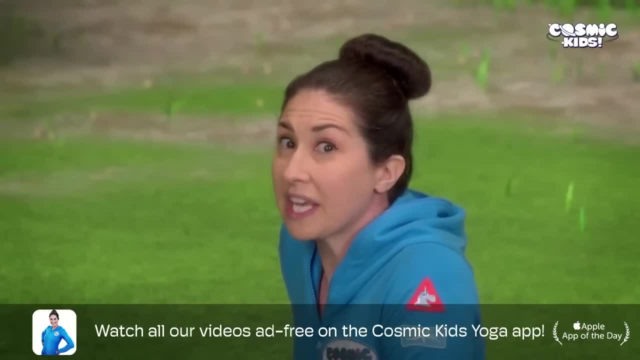 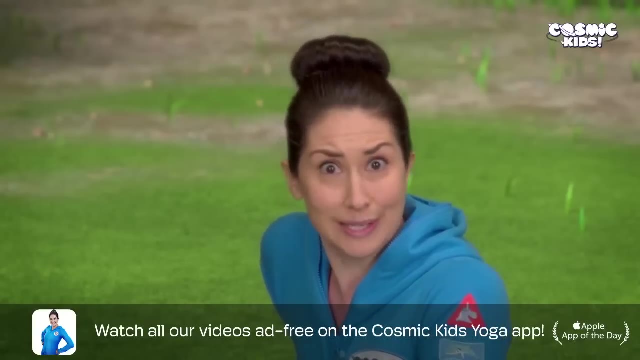 And again Sit back on our heels, slide our body through and wiggle on up like a worm. Very good. everyone Now working alongside Wonky is Dez. Dez is a carrot, a disco carrot. He's also a keen gardener, coming up to stand in our carrot pose. 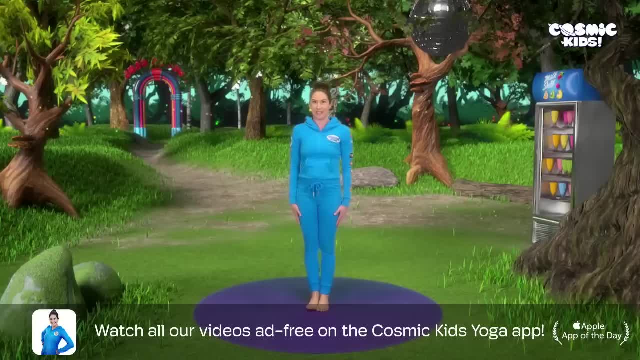 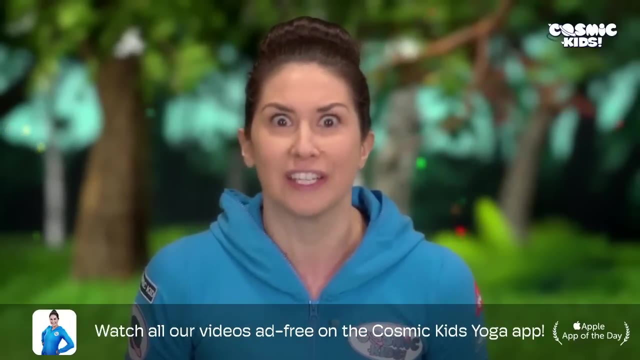 We bring our feet together and our arms down by our side. We go all the way around one way, Yeah, And all the way around the other, Yeah. Now Dez has one job at the Bubble Club and that is to turn on the great big, giant glitter ball. That's it. 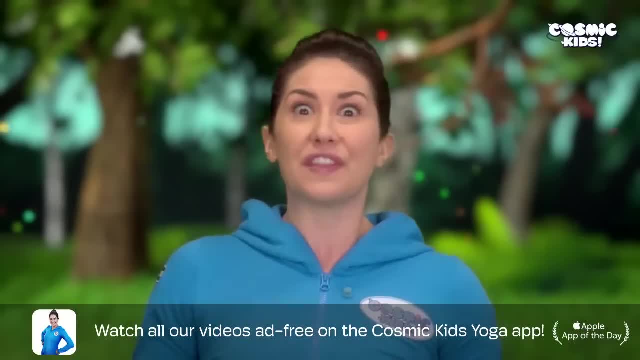 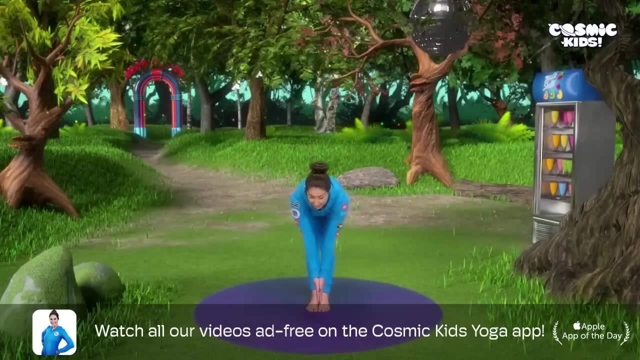 Now, every week, Fairy Floss flies all over the neighbourhood like a bird, inviting everyone to the dance meet, Folding all the way forwards. hands come down, we lift and lower our arms. as we fly like a bird, She never misses anyone out, even inviting Nicodemia the witch, who can't bear dancing. 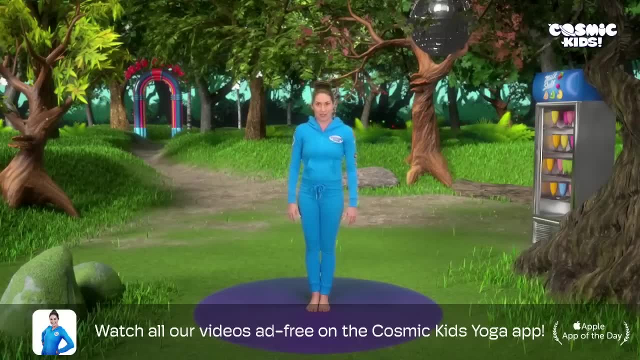 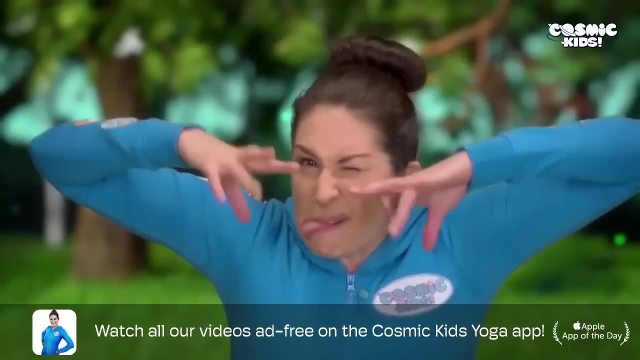 Rolling up to stand, coming into our witch pose. We stand on one leg using our toe for a bit of balance. We make our fingers all craggy, lift up our elbows, maybe close one eye And we stick out our tongue. 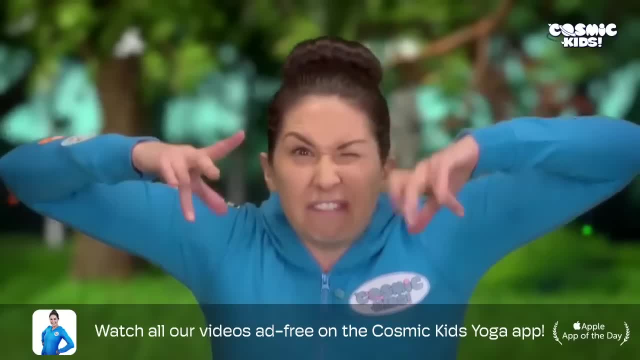 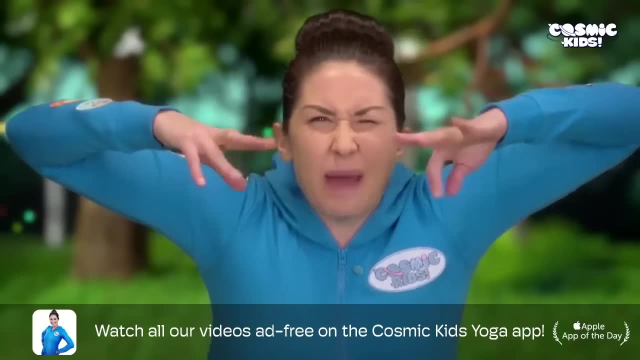 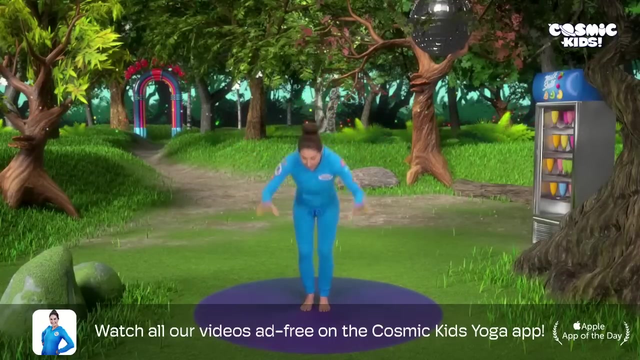 All this dancing, making everyone feel good. If only there were a way I could make it stop. Fungus- where is my spell book? Fungus is a frog Coming into our frog pose. we crouch all the way down, take our knees wide and we use our fingers like little froggy finger pads for balance. 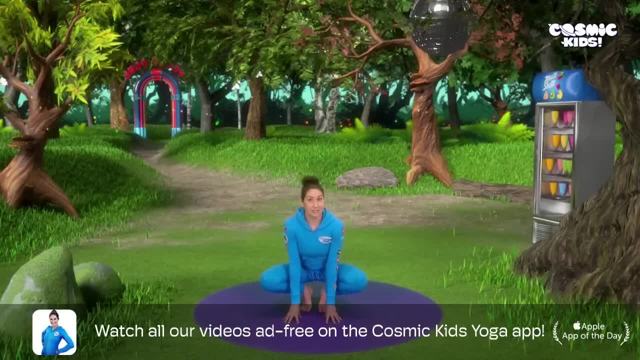 Now Fungus the frog has been servant to us. Fungus the frog has been servant to Nicodemia since he was a tiny tadpole. He hops all over the cottage looking for the spell book. After three, let's do a hop and a ribbit. 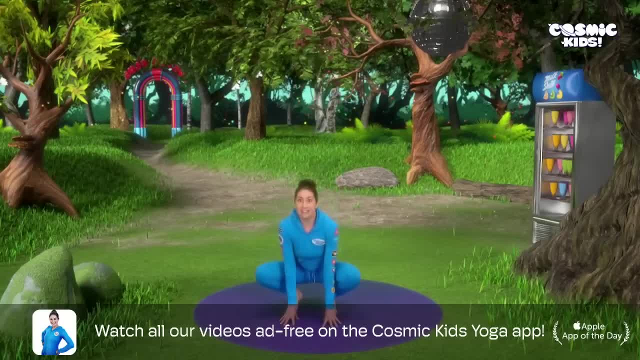 Ready. One, two, three Ribbit, And again One, two, three Ribbit. I found it, m'lady. Just then, Fairy Floss arrives with their invitations for the dance. meet up, Coming down onto our knees. 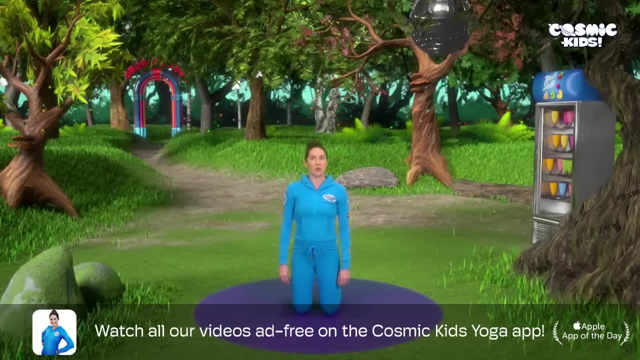 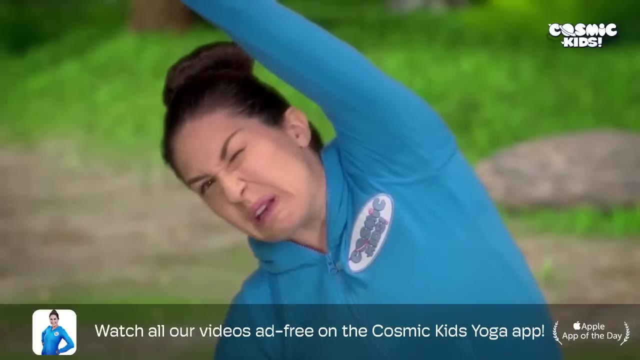 Nicodemia opens the door, Taking our leg to the side, Our arm up to the sky. We open the door, going eeeeee. She stares at Fairy Floss with her grumpy witch face. What do you want, Fairy, Not put off? Fairy Floss stands and smiles. 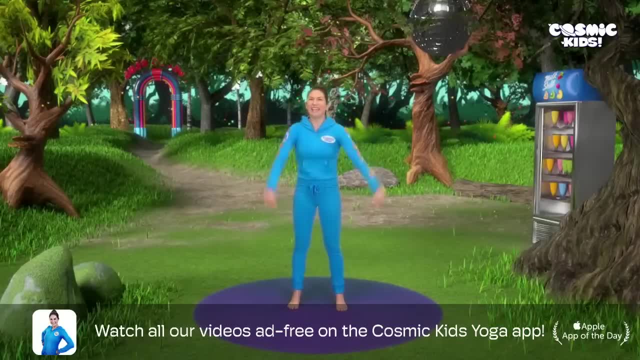 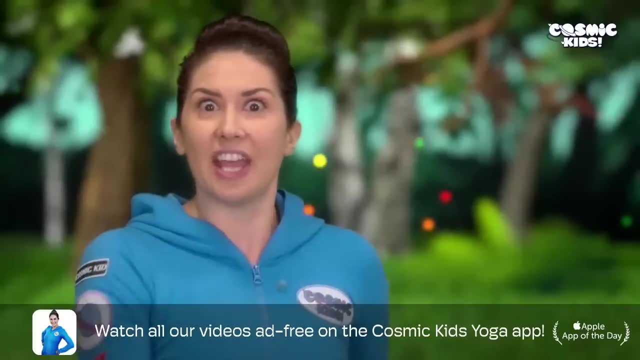 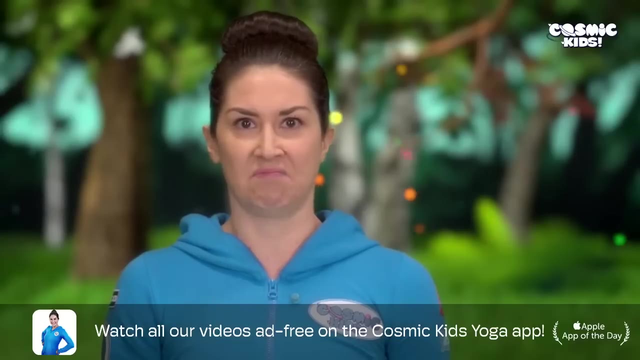 Coming up to stand. Hello, Just popping round to offer you both an invitation To the dance meet at the bubble club tomorrow And to suggest some dance moves that could be fun To try. Nicodemia stares Unimpressed. Fairy Floss continues. 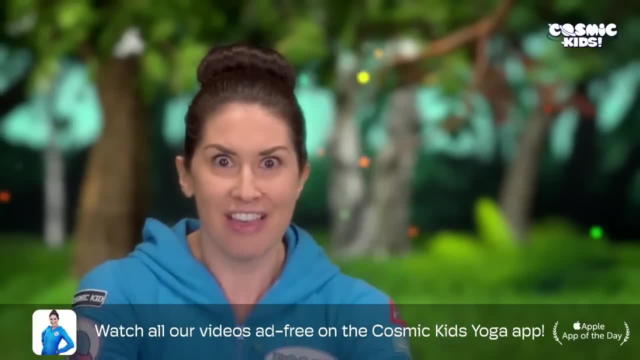 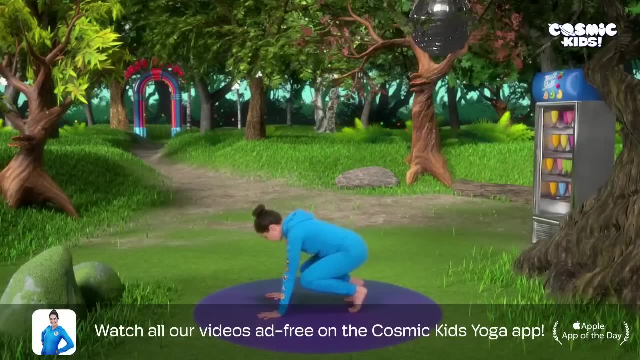 Right now I am loving the bunny bounce. Let's give that a try. You come all the way down. Put your hands flat, Stay high on your tiptoes And lift up your hips. Then you do a little hop Ready. 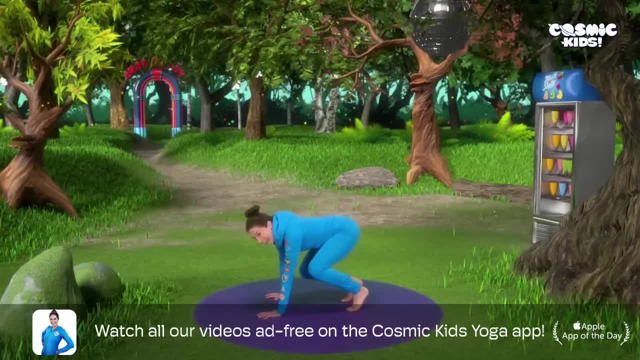 One, Two, Three Hoppity hoppity hop. And again One, Two, Three, Hoppity hoppity hop. No, Okay, Well, there's also the washing machine move Where you sit on your bottom. 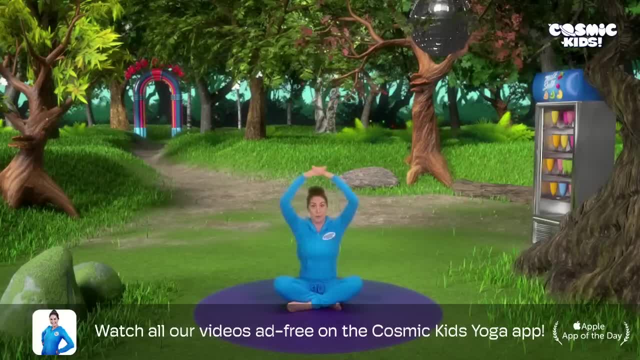 With your legs crossed, Criss-cross your fingers, Put them behind your head, And then you twist From side to side, Saying Wisha washa, Wisha washa, Wisha washa Woo, Wisha washa. 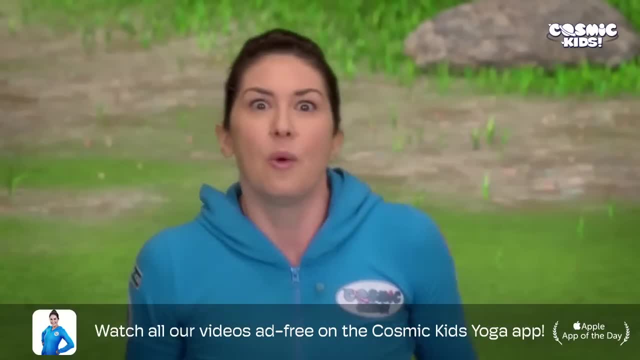 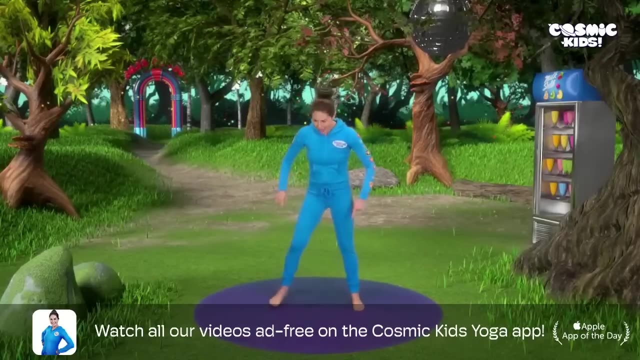 Wisha, washa, Woo, No, Okay. Well, there's also my favourite dance move, The floss. Let's give that a go. You come up to stand Legs a little bit wide. Now your arms go the opposite way to your hips. 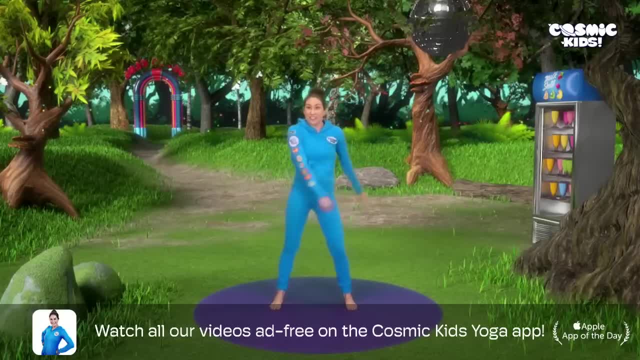 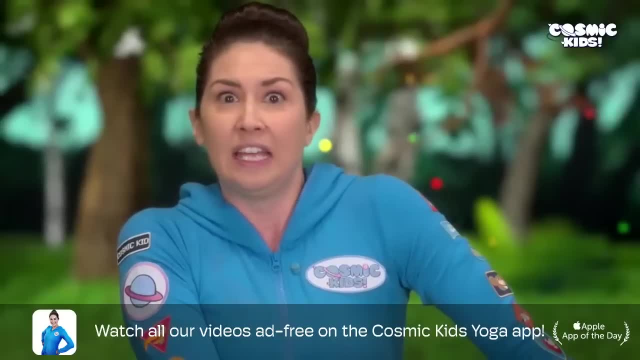 Here we go: Fairy floss, Do, do, do, do, do, do Fairy floss, Do, do, do, do, do, do Fairy floss, Do, do, do, do, do, do Fairy floss. Nicodemia can't bear anymore And she slams the door. 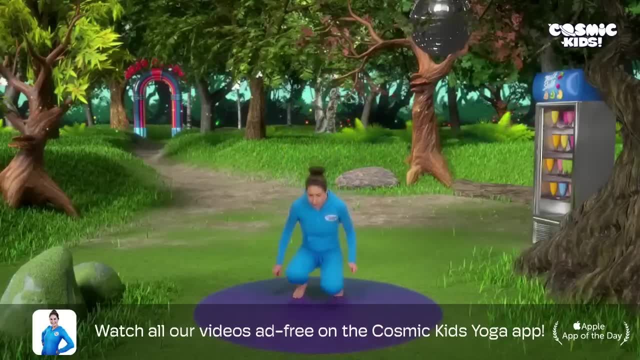 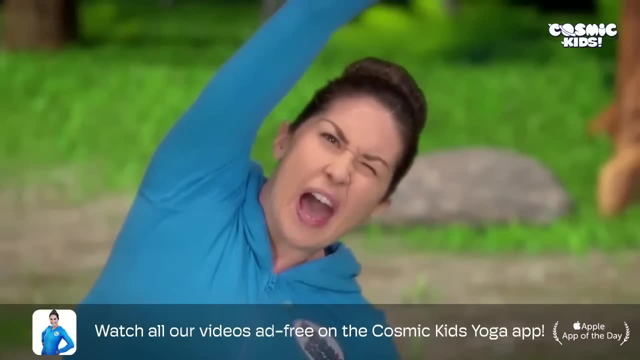 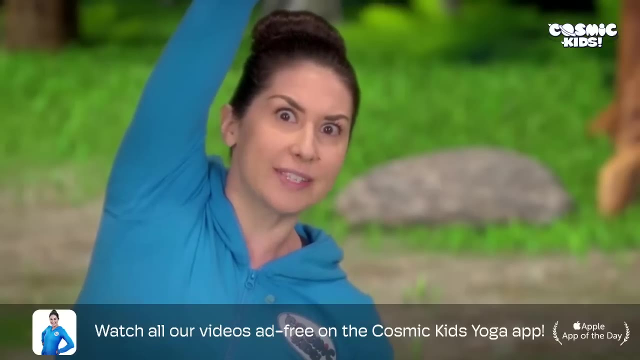 In Fairy Floss's face, Coming down onto our knees, Leg to the side, Arm to the sky, And Salaam. It's time to put an end to all this dancing Once and for all. That night, Nicodemia rides on her broomstick. 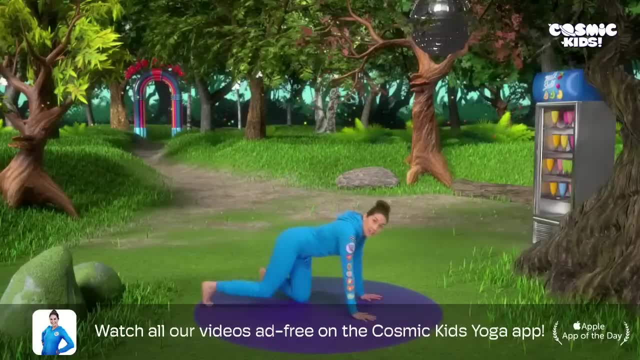 Coming into our broomstick pose. We lie on our tummies, Our arms down by our sides, We lift up our chest, Lift up our feet And we fly Going Whoosh Through the night sky Straight for the bubble club. 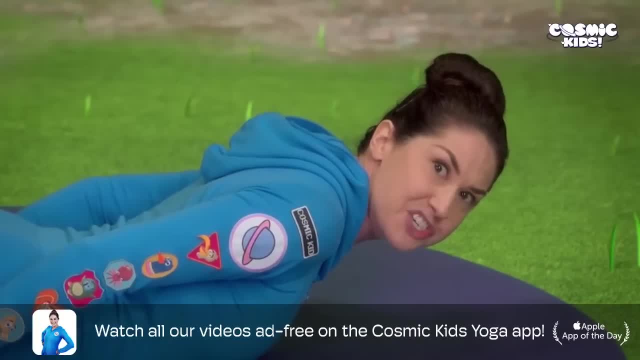 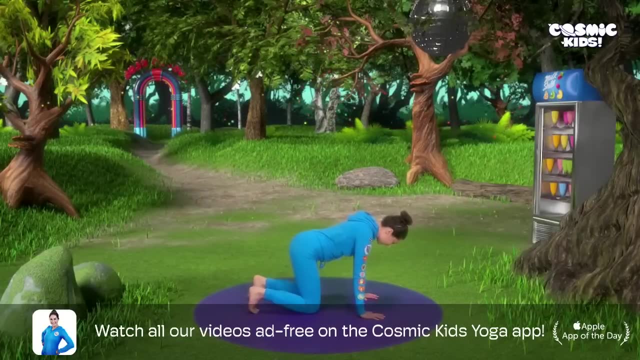 When she arrives, Nicodemia turns herself magically into a cat. Coming into our cat pose Up onto our hands and knees, We tuck our toes And we arch our back Looking into our tummy. Then we dip our tummy down. 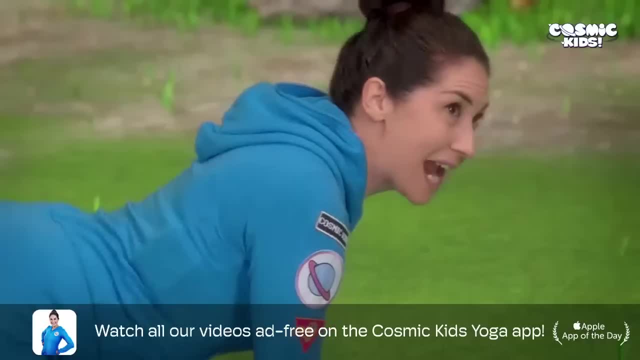 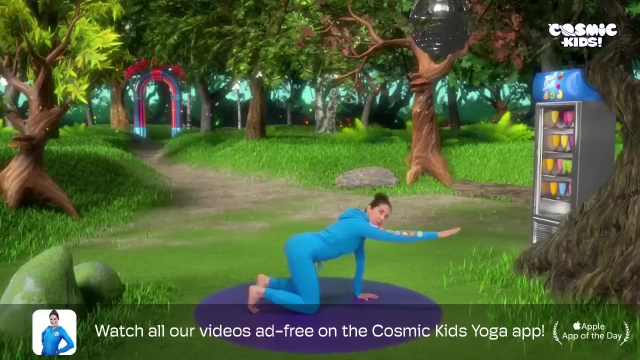 And we wiggle, waggle our tail, Saying Meow Quietly. she slips in through the cat flap, Reaching in with one paw, Reaching in with two, Reaching in with three paws, Reaching in with four. 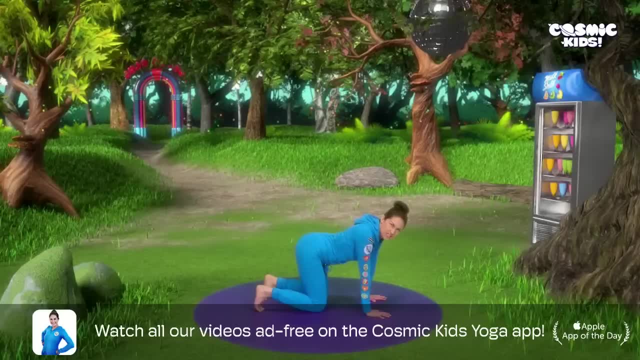 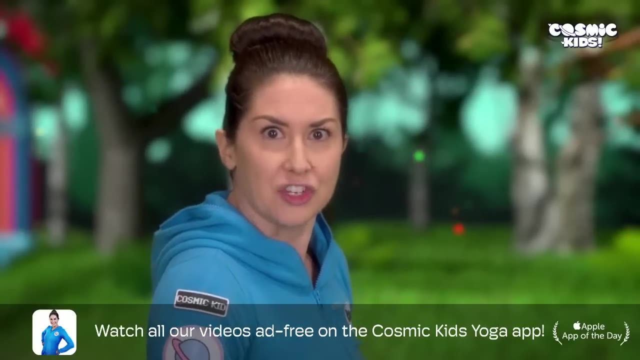 Then she rolls herself back up to her normal witchy self, Walking your hands all the way back And rolling up to stand, Keeping your knees bent, Head to come up last. Then she takes out her wand And she points it straight up at the giant glitter ball. 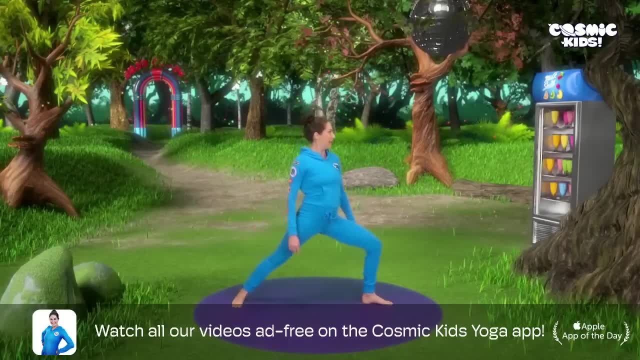 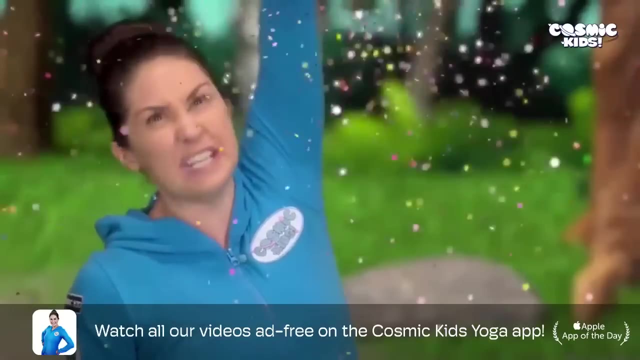 Stepping one foot forward, One foot back, Bending into our front knee, Stretching our top arm all the way up, Making our finger a point Like we're holding a wand. Then she encants her spell, She turns And she does it on the other side. 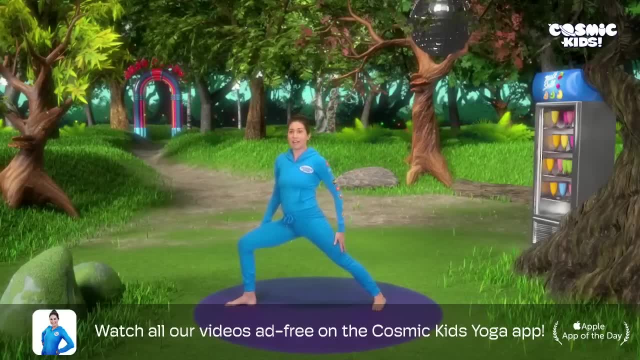 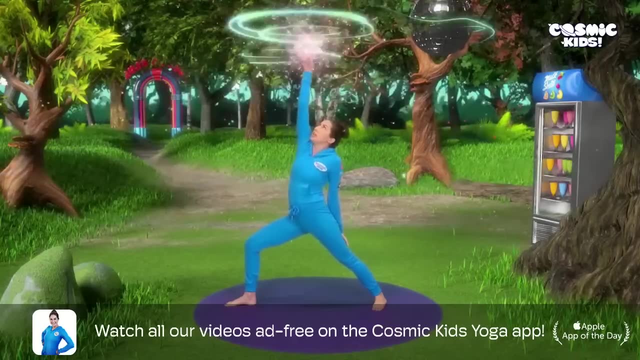 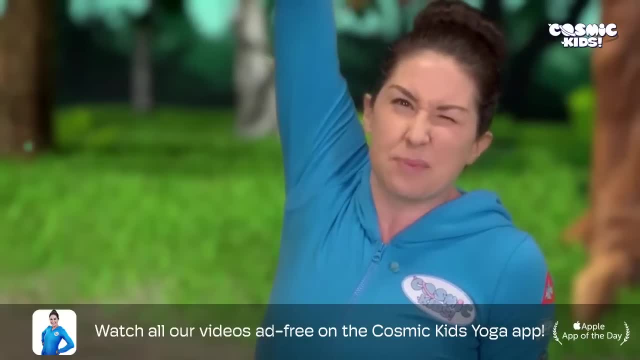 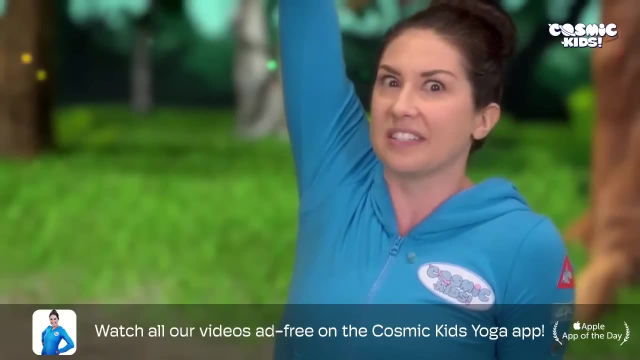 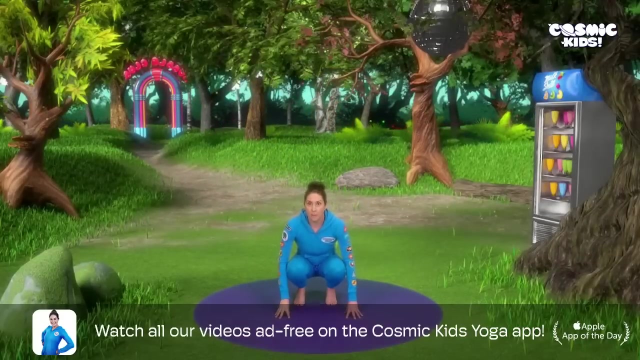 Now, when they all start dancing And their precious glitter ball begins to spin, They will all turn to stone And with that she disappears in a puff of smoke, Coming all the way down to crouch. After three Big jump And a puff. 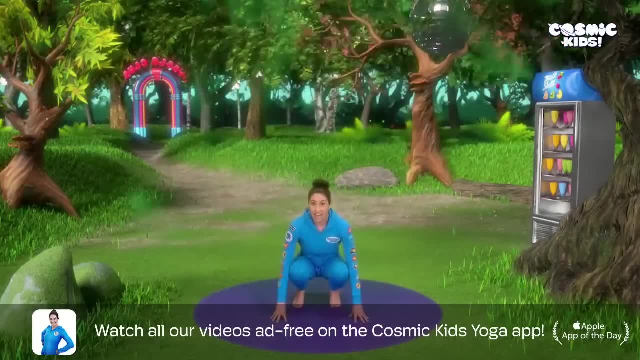 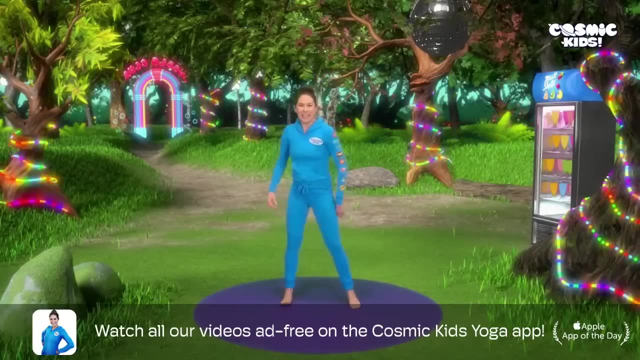 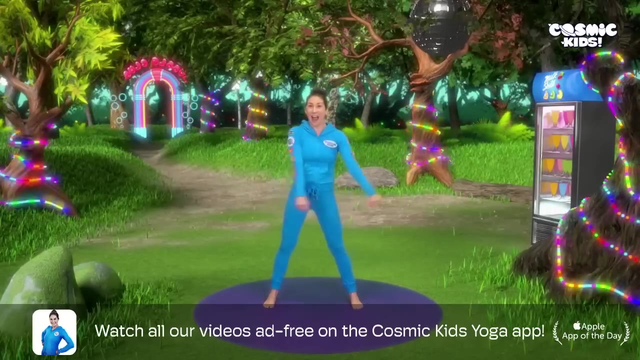 One, Two, Three, Four. The next day is the dance meet, The music starts And the dancing begins. It's led by Fairy Floss, Doing her favourite dance: The floss. Here we go everyone. Yeah, Give it some floss everyone. 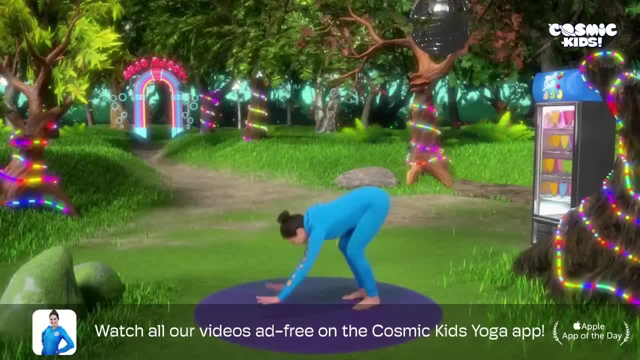 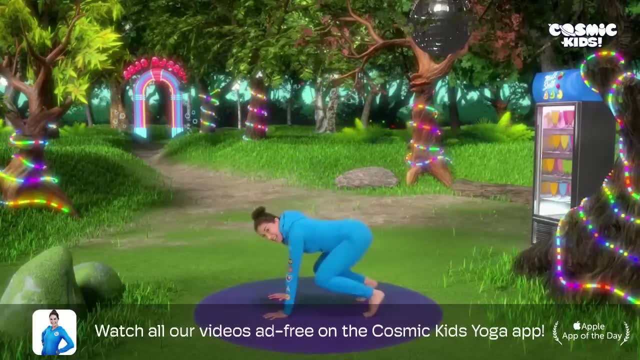 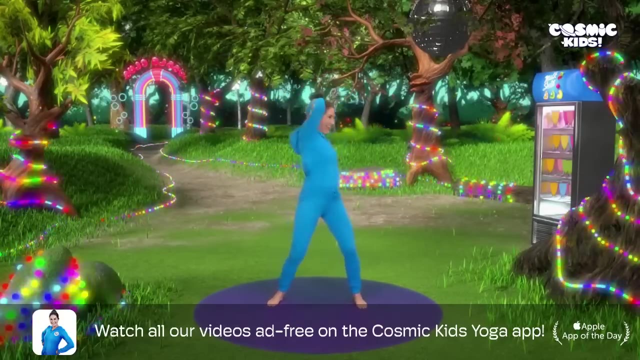 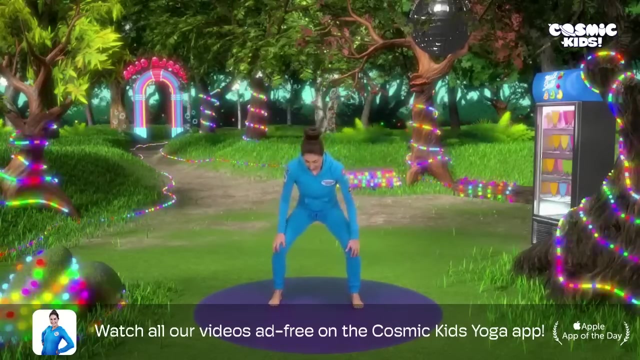 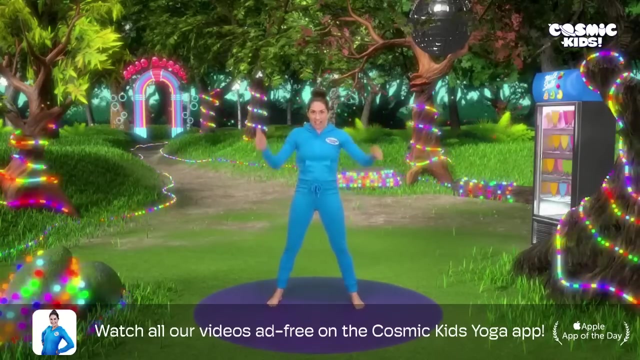 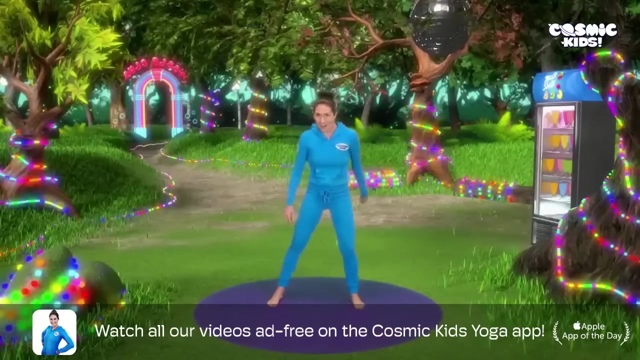 She does some bunny bouncing, Ready to hop, Here we go. And again Last time Coming all the way up Washing machine And a knee cross. One crew is in the fridge getting the milkshakes ready, shapes ready. so Des climbs the ladder, ready to switch on the glitter ball. here he goes. 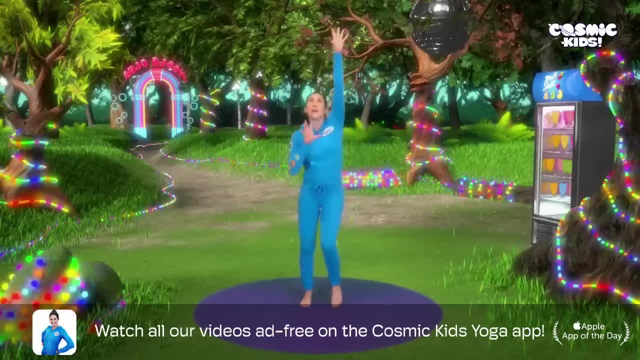 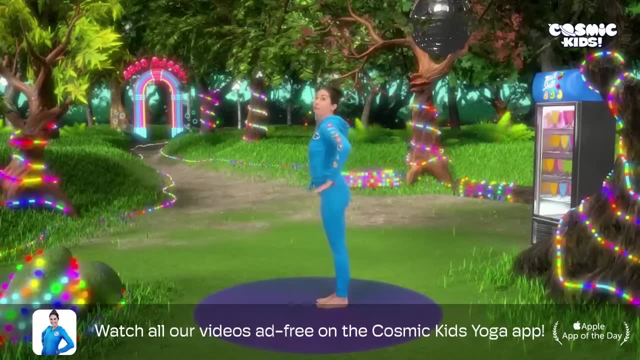 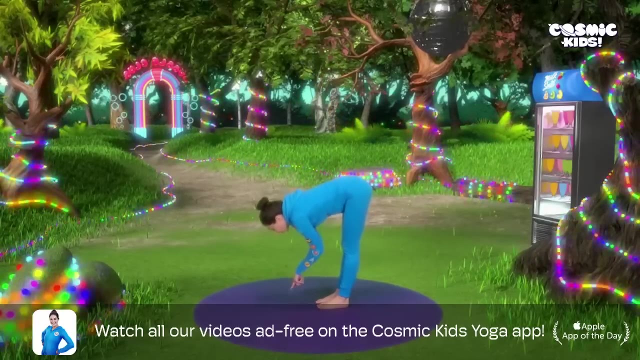 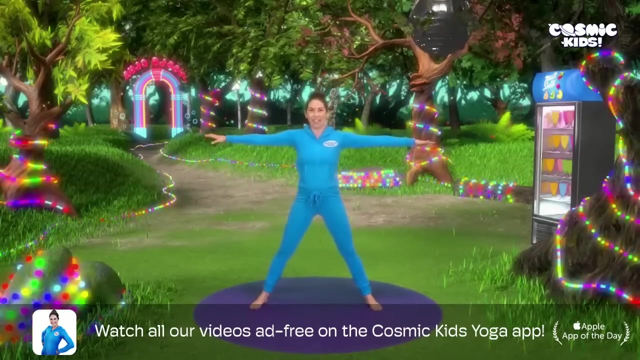 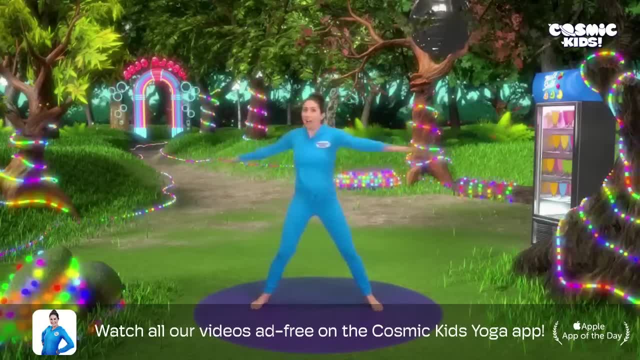 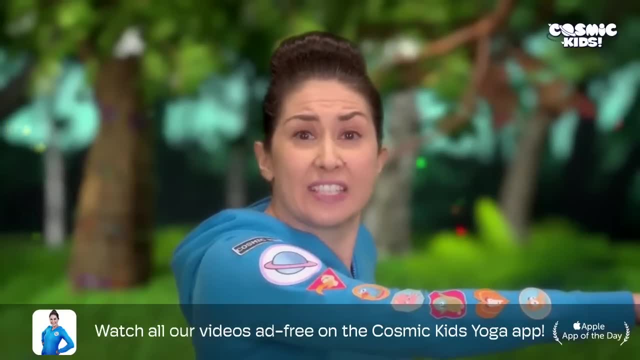 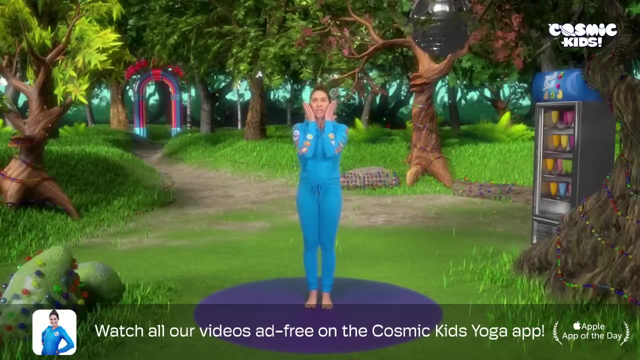 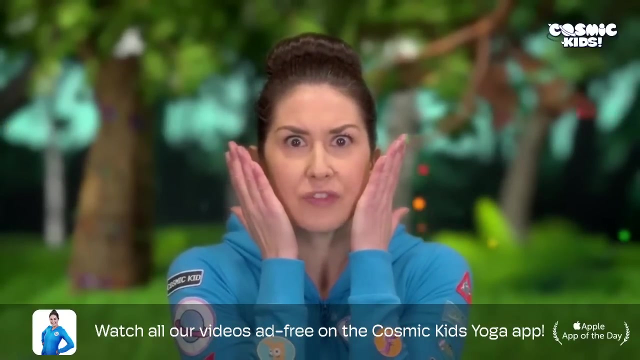 as soon as it does, Nicodemia's spell is activated. everyone freezes because everyone has turned to stone. jump your feet together, hold on to your face, Des the disco carrot is horrified, no, and then he spots someone hopping out of the bubble club. it's fungus, the frog. 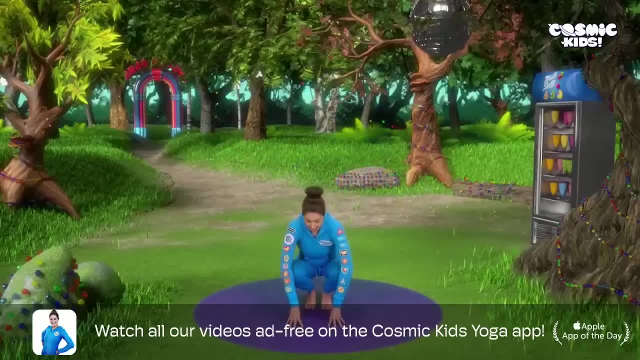 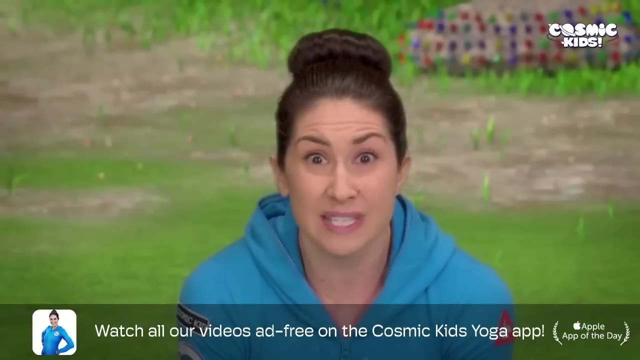 coming into our frog pose, crouching all the way down knees, come wide, balancing with our froggy fingertips. after three, let's do a hop and a ribbit. one, two, three ribbit, and again one, two, three ribbit. wonky, the worm comes out of the fridge and he sees him too. 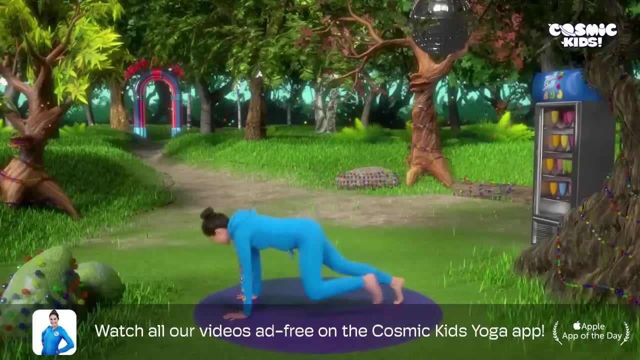 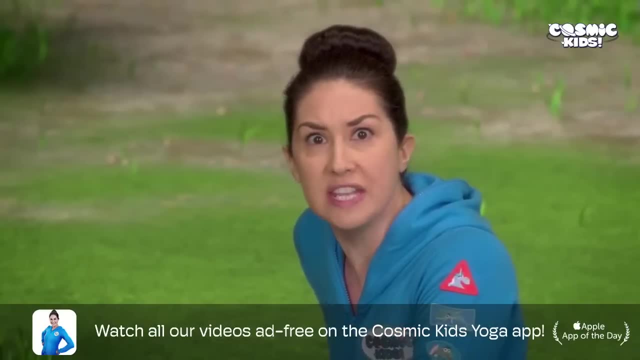 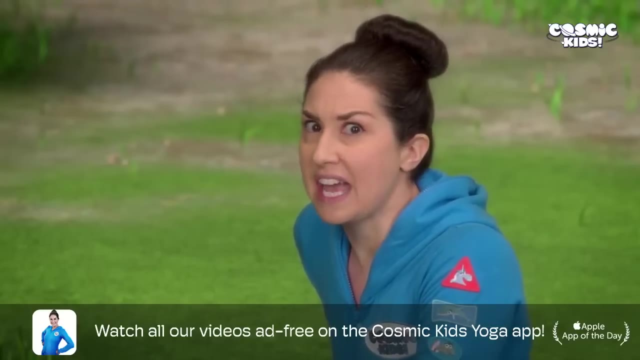 into our wonky the worm pose, lying on our tummies, hands under our shoulders, wiggle, wiggle, wiggle, wiggle all the way up. now we know who's behind this Des: it was Nicodemia. we've got to find out how to break the spell, and so wonky and Des go to Nicodemia's cottage, coming to sit on our heels. 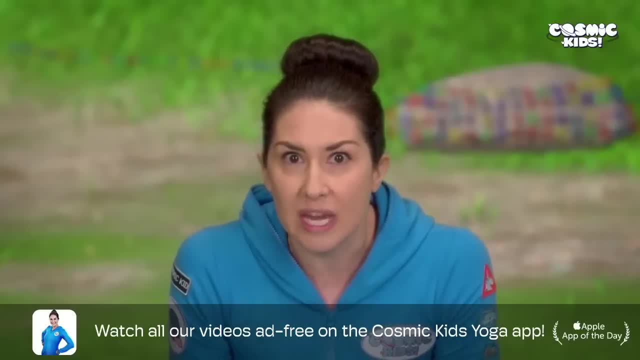 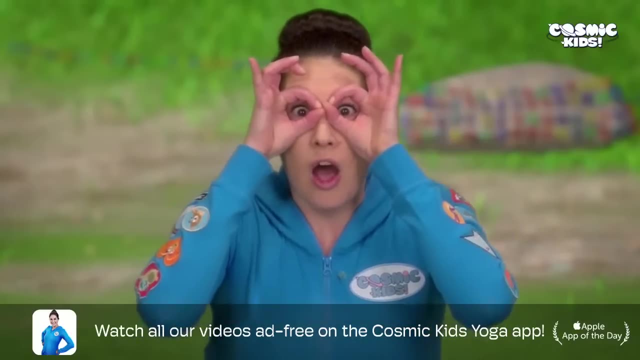 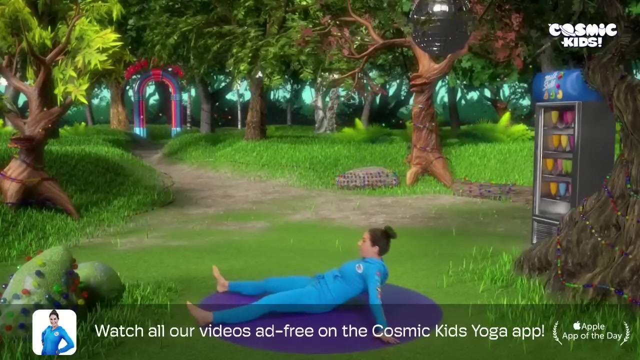 when they arrive, wonky and Des peep in through the window using their cosmonoculars, joining our thumbs and fingers together. have a look through. there. she is lying on the couch, coming to lie down, everyone legs wide, arms wide. she's asleep and she's snoring loudly like a witch. 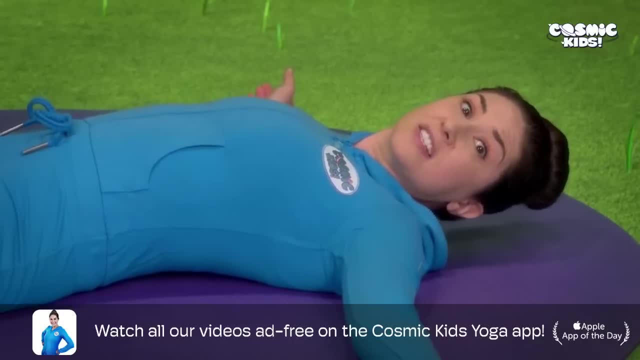 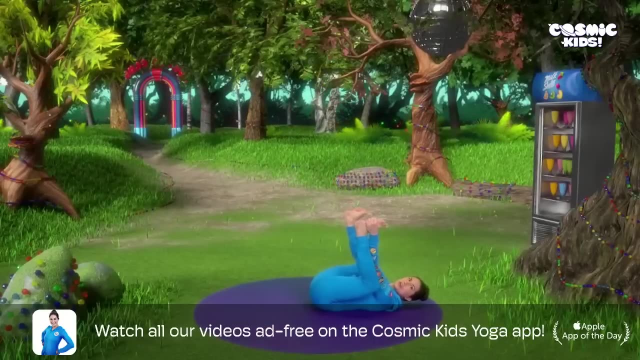 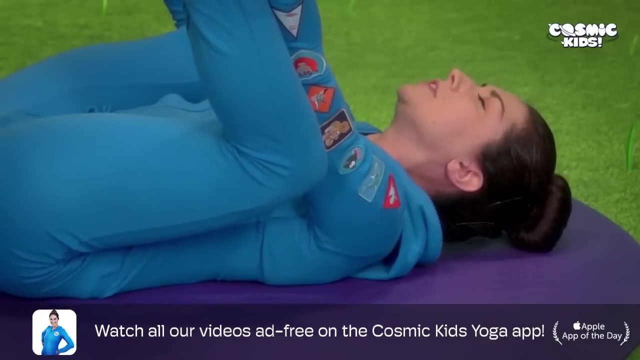 in the corner in his frog basket is fungus the frog. he's also lying asleep, but with his legs in the air, lifting our legs up, holding onto the soles of our feet. he's also snoring loudly, but like a frog. ribbit. ribbit Des keeps a lookout and does a bit. 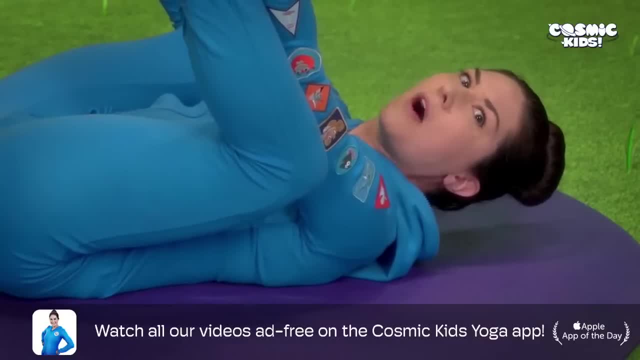 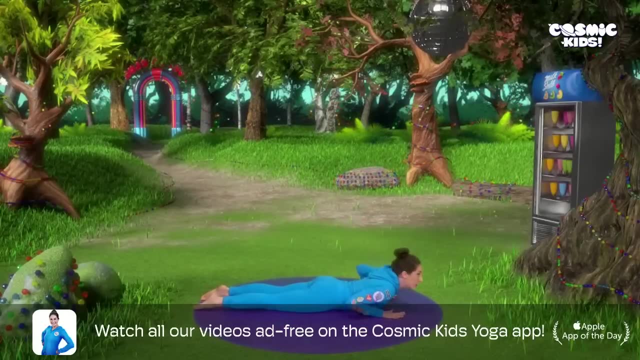 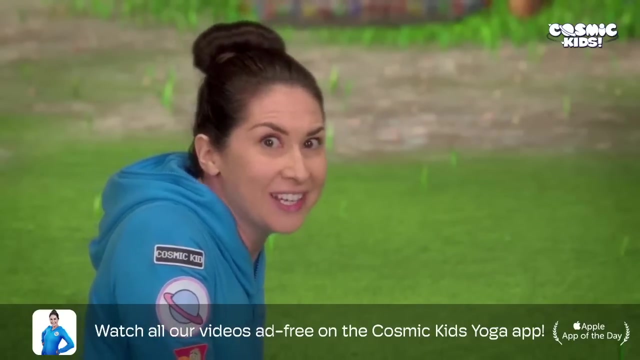 of weeding in the garden while wonky wiggles inside bravely coming onto our tummies. everyone hands under our shoulders. that's wiggly, wiggle, wiggle, wiggle, wiggle, wiggle, wiggle. he finds Nicodemia's spell book coming into our book pose. 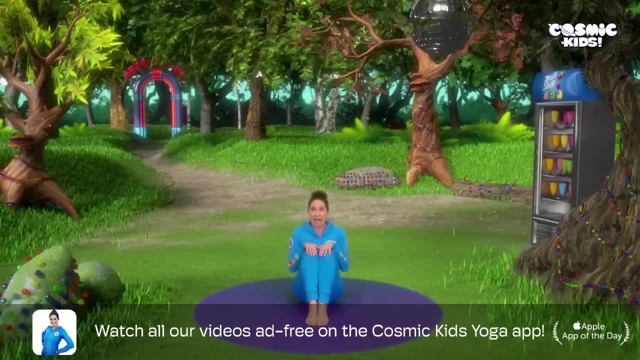 sitting on our bottoms, knees, bent feet, flat hands on our knees. the book is still open, lowering our knees down to the side. the page is titled how to stop dancing. wonky reads down the spell and at the bottom is a note that says how to break this spell. 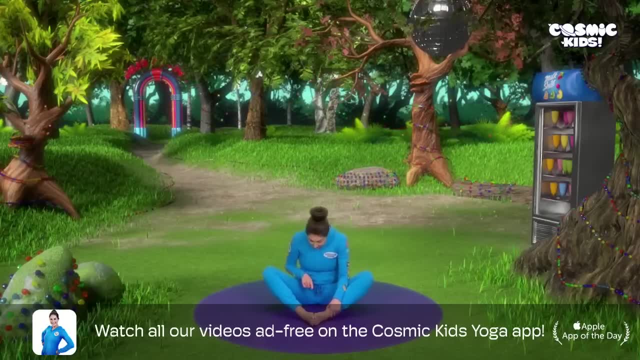 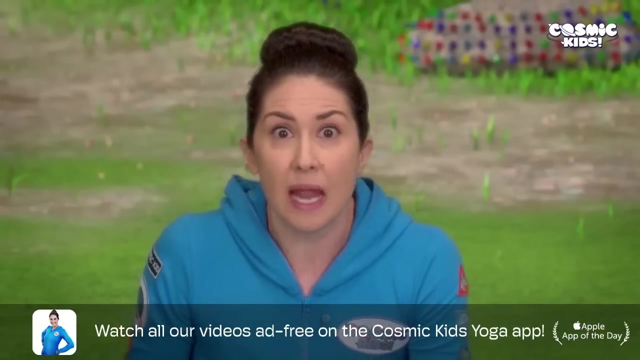 it reads: find as many people not under the spell to dance, dance, dance until they hear a bell. when the spell is broken, a new curse shall begin for the one who cast it: to forever dance like a chicken. chicken, it says chicken, so so this means, when the spell is broken, Nicodemia will. 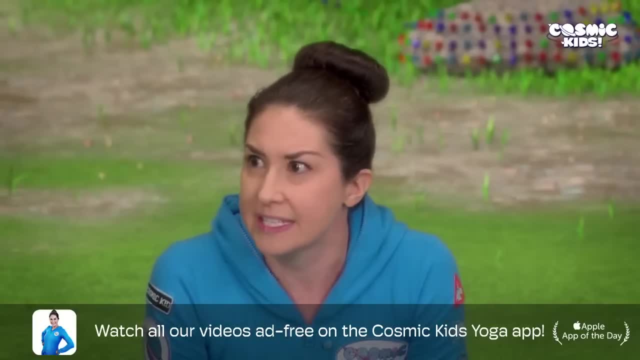 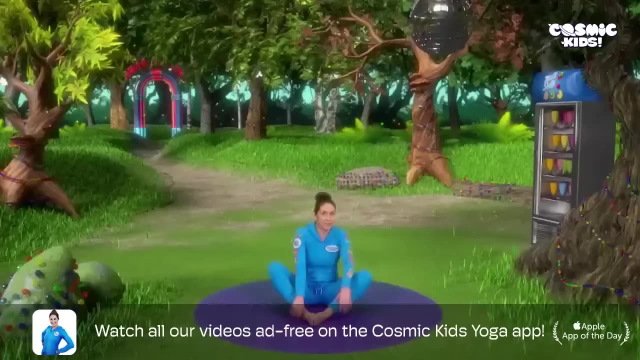 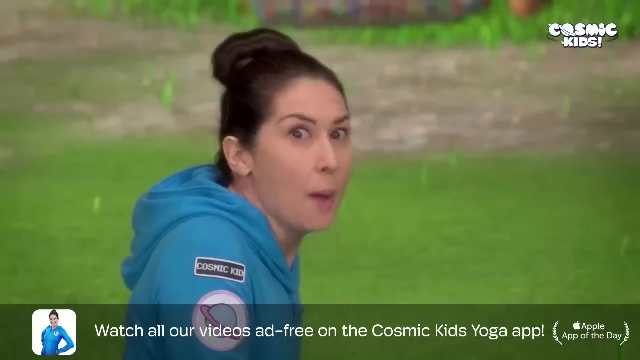 forever dance like a chicken. that is something wonky quietly, silently wiggles out, trying not to disturb Nicodemia and fungus coming back onto our tummies, hands under our shoulders, wiggle, wiggle, wiggle. back at the bubble club, wonky and Des start phoning round everyone they know sitting on our bottoms. 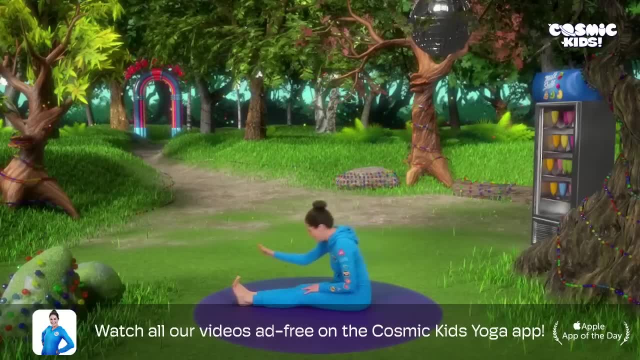 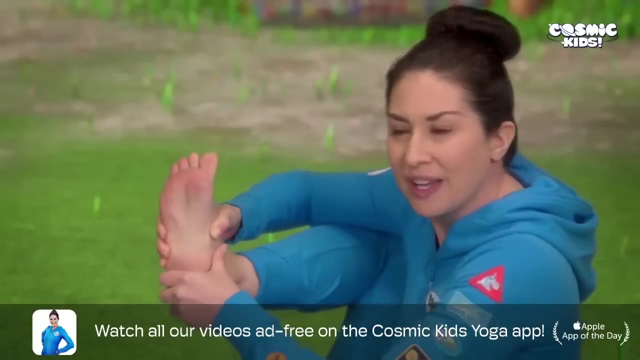 with our legs out long in front of us. they pick up the telephone, lifting up one of our feet and number: Oh hi, Bob. Yeah, it's Wonky and Des here from the Bubble Club. How are you? Oh good, How. 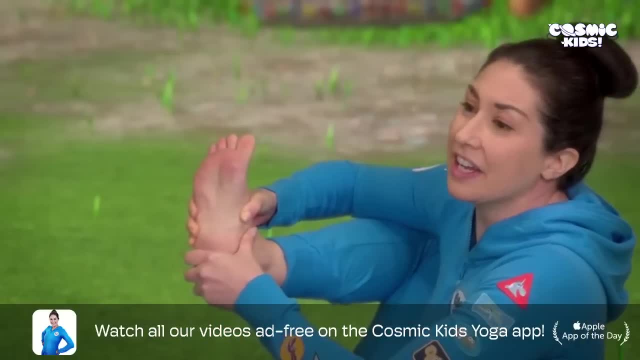 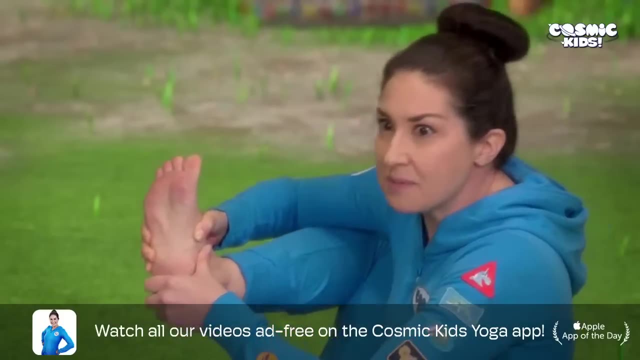 are all the gnomes? Yeah, they all. okay, Excellent, Look, we've got a favour to ask. Would you mind gathering as many gnomes as you can? Yeah, all your gnome friends, Bring them to the Bubble Club. 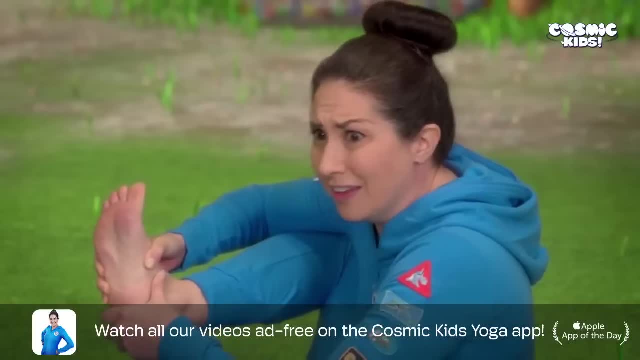 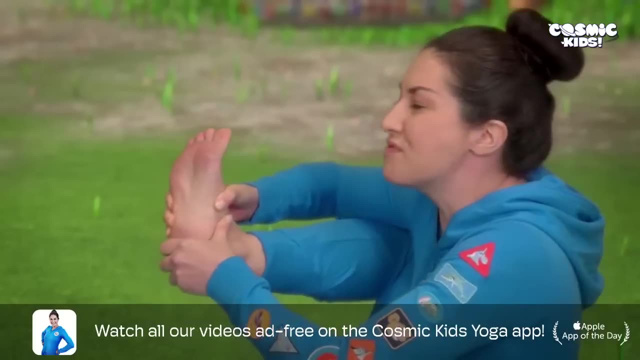 because we need you to dance. Yeah, we've got to break this spell. Nicodemia, she's turned everyone to stone. I know it's awful. Oh, you'll come. Yeah, you'll bring them all. Oh, brilliant You're. 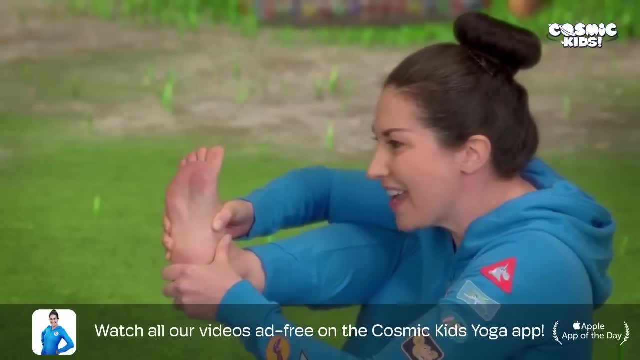 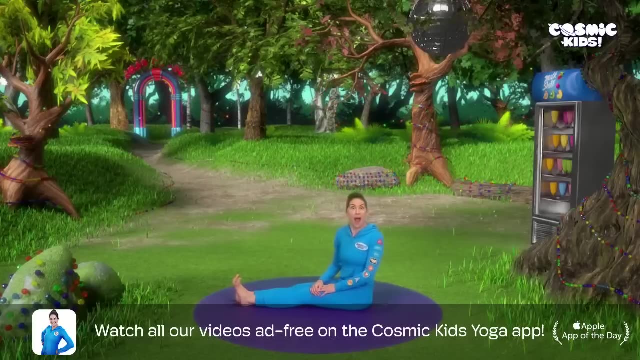 a star, Bob. We'll see you in a minute, Okay, bye. They put the phone down and the next thing we know our telephone is ringing. Let's answer it. We pick up the phone. Hello, Cosmic Kids here, How can I? 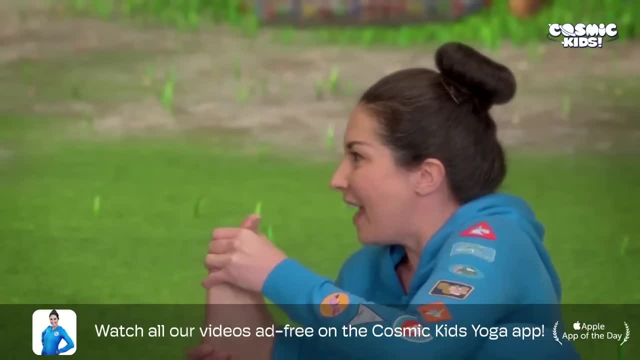 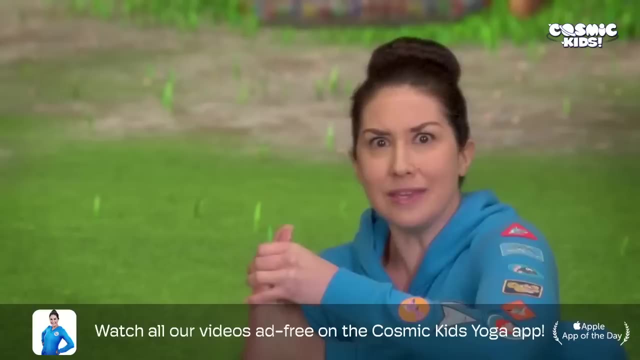 help you. Oh, hi, Wonky, Hi, Des. Yeah, we heard all about it. Dreadful business, Nicodemia turning everyone to stone, Awful. Yeah, we can do that. We can come to the Bubble Club. Yeah, we can dance. 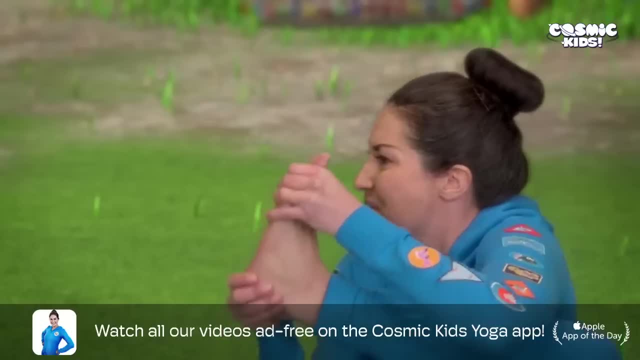 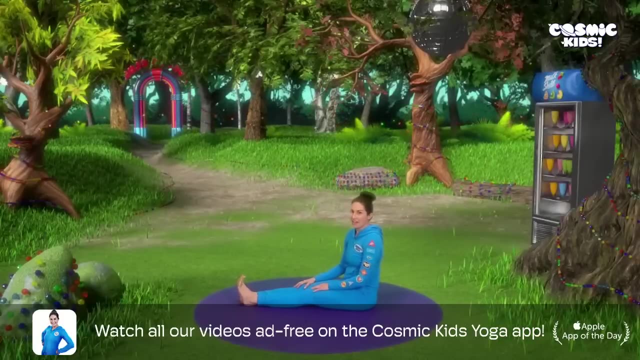 Yeah, Cosmic Kids are awesome at dancing. Easy, Yeah, okay, We'll be there in a minute. All right, Wonky Bye, Oh yeah, Yeah, love you too, Des. Okay, bye, Bye. We put the phone down and we get. 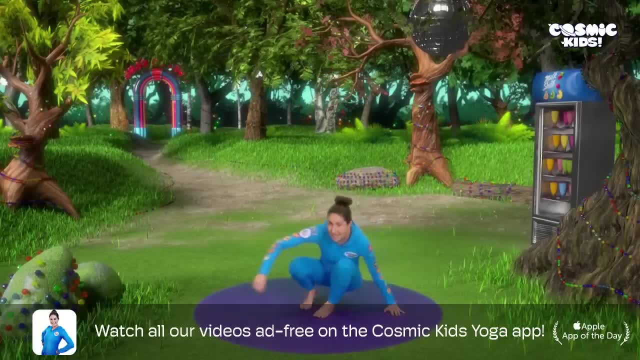 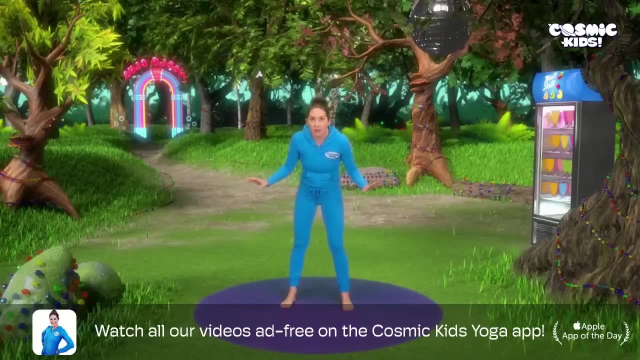 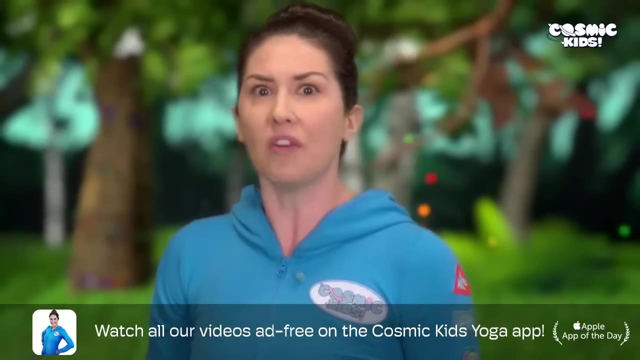 ourselves down to the Bubble Club Coming up to stand everyone. When we get there, the place is packed full of people and thousands of gnomes. It's time to unfreeze our frozen friends and start the dancing. Wonky cues the music and the dancing. 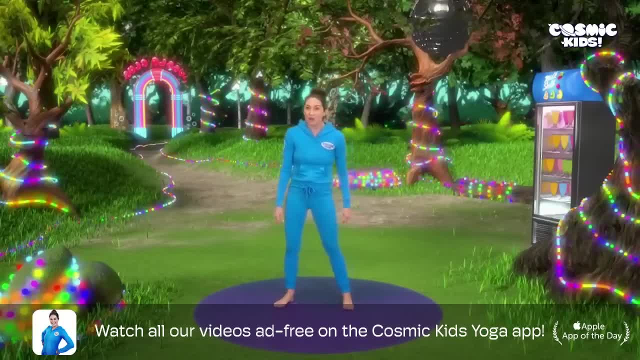 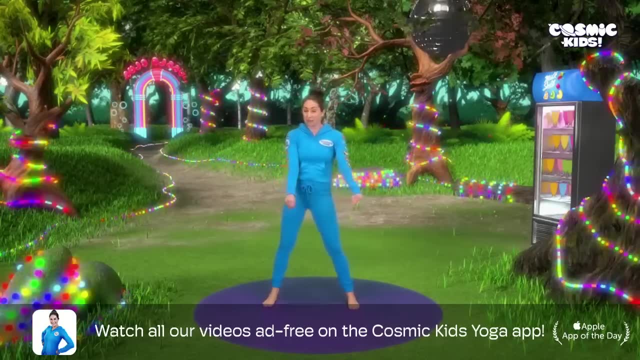 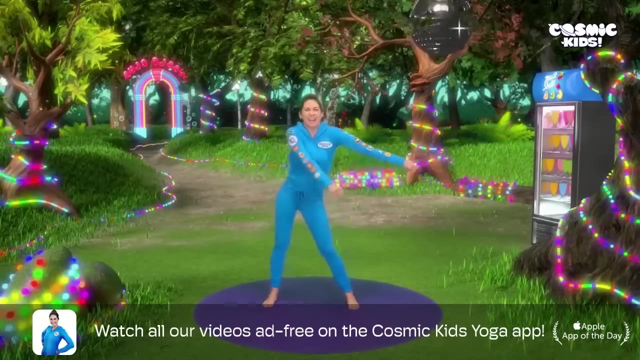 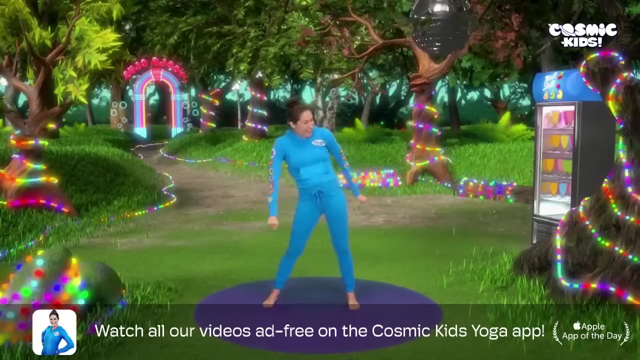 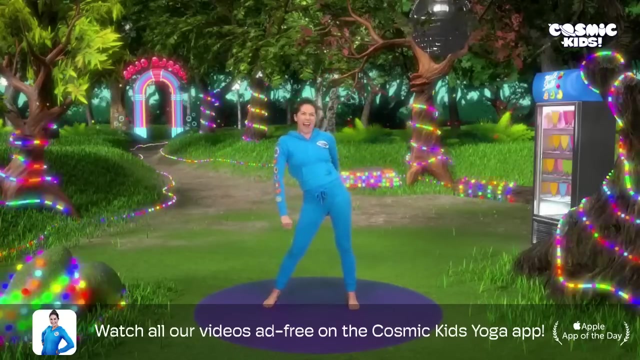 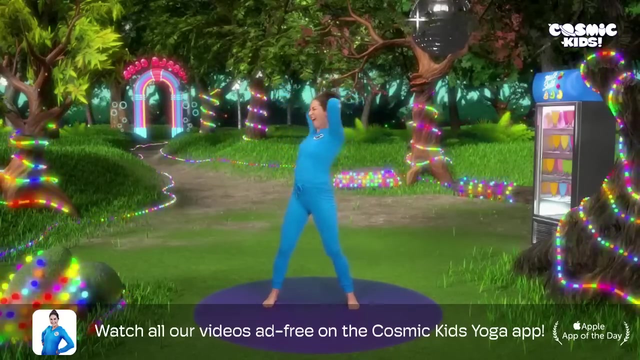 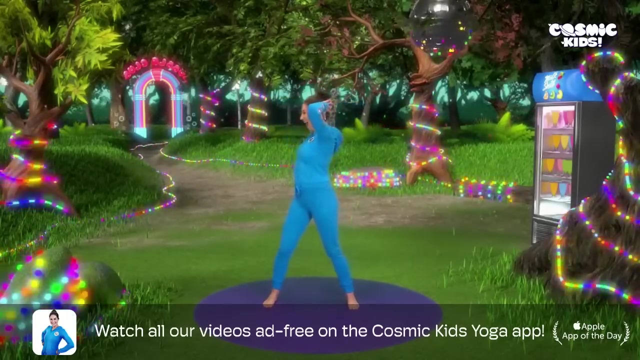 begins. We dance in slow motion, starting with a slow motion floss dance. Are we ready? Arms down, opposite way, with arms and hips. Here we go, Ready, We do slow-mo washing machine, Slow-mo knee cross. 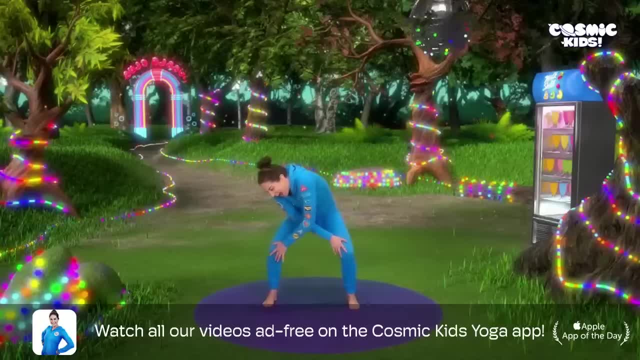 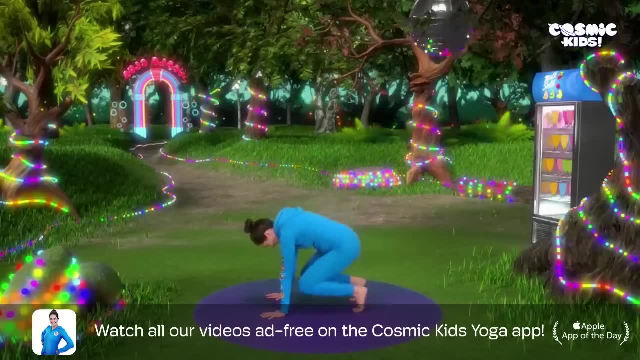 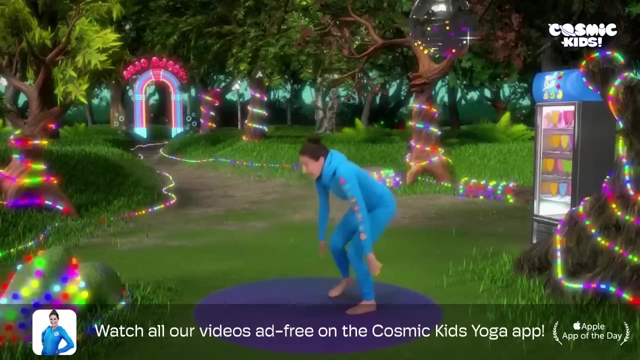 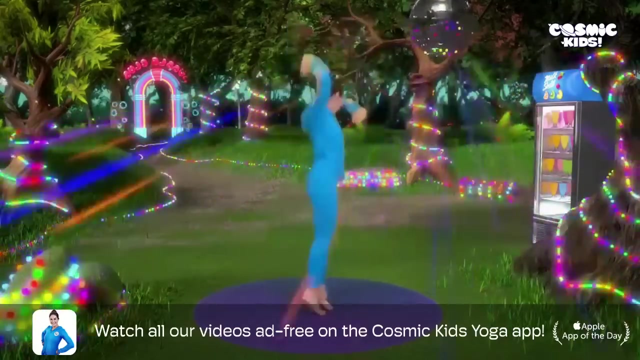 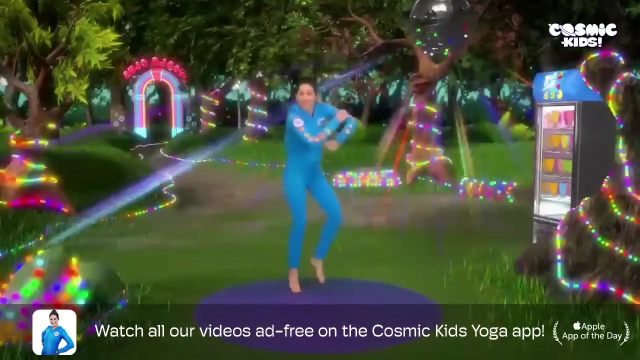 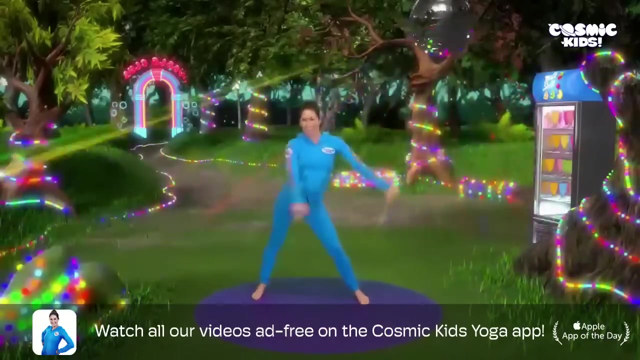 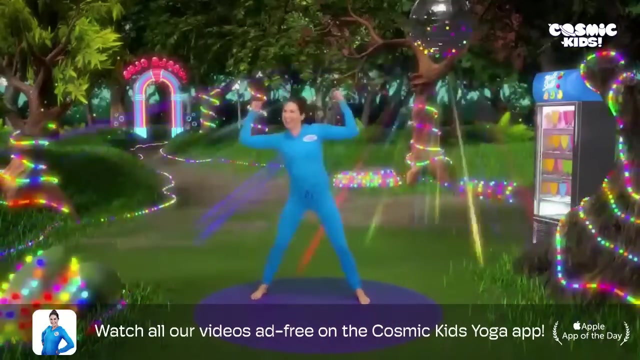 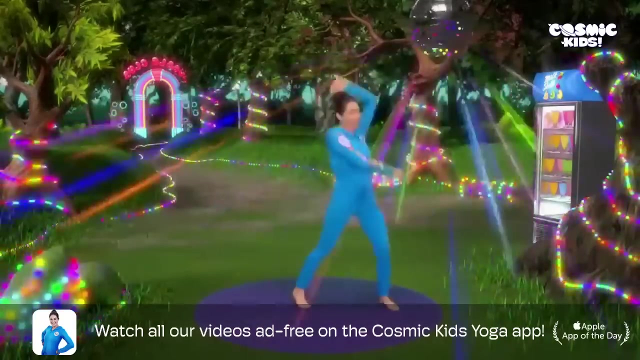 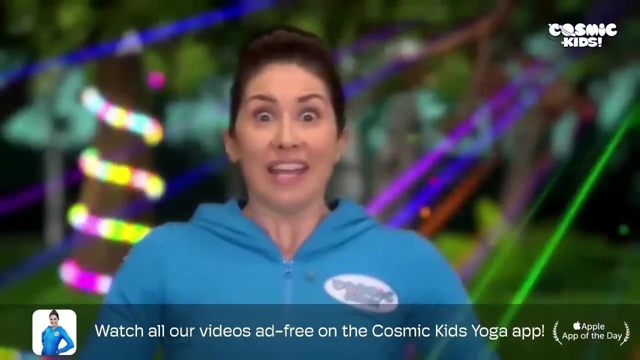 Slow-mo bunny bounce. Then we stand up, put our hands in the air and we dance. Here we go, We keep dancing, everyone, until we hear the bell. You know what to do? Keep dancing. Did you hear it? Yes, we heard the bell, It's. 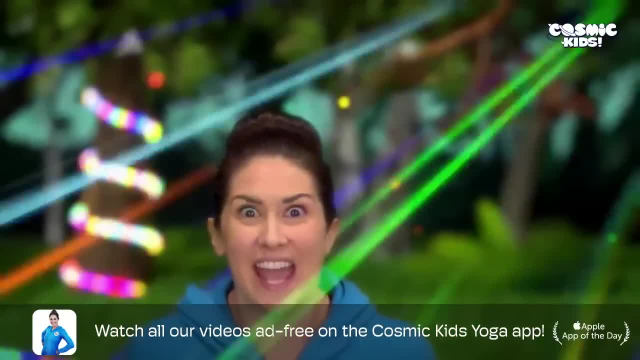 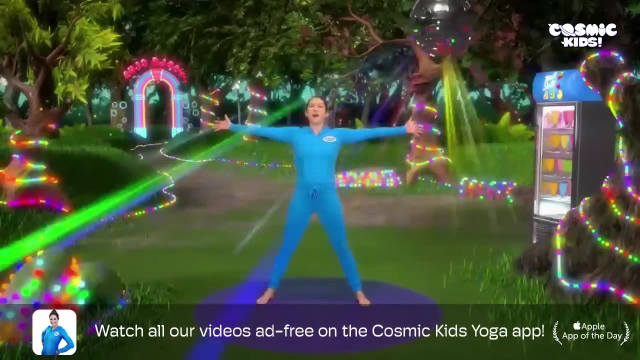 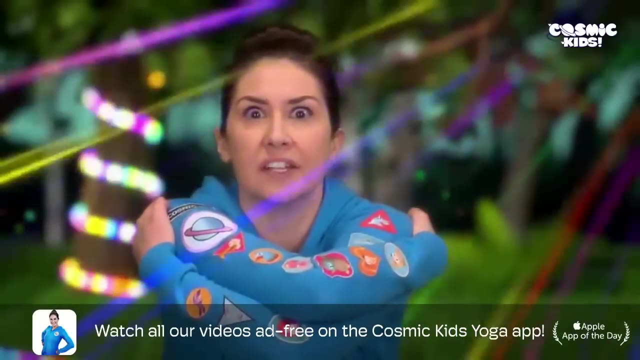 worked. Everyone who was frozen is dancing again. Fairy Floss comes running over and she gives us a ginormous hug, reaching our arms wide, wrapping us up. Oh, you've done it, Cosmic Kids, You saved us with a dance. All of a sudden, there is a puff of green smoke coming all the way down to Crouch. 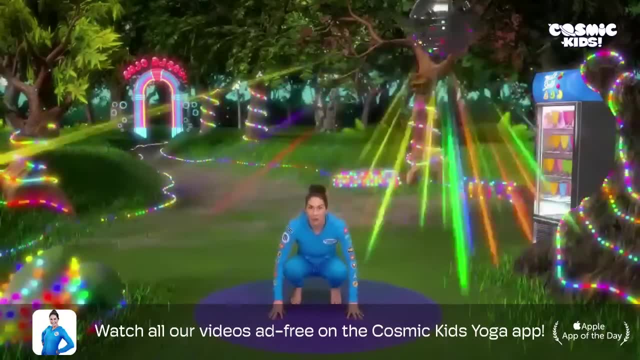 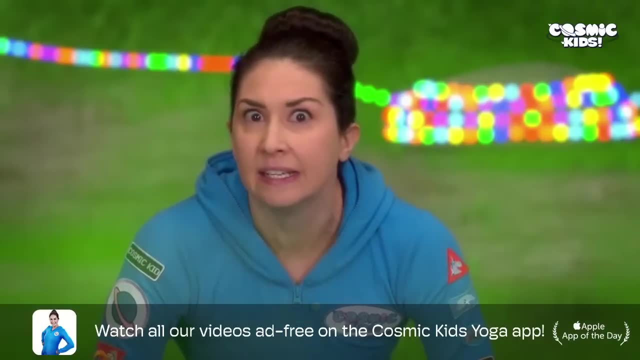 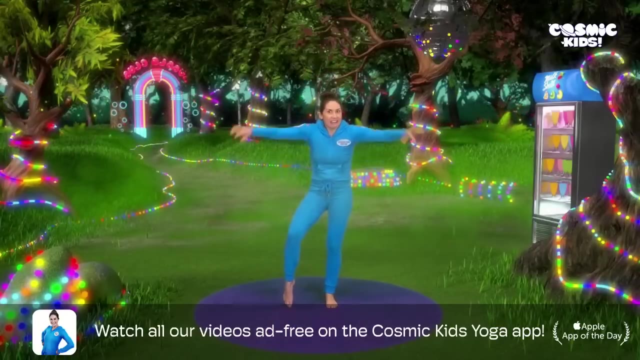 After three, let's do a big jump and a puff. One, two, three. Appearing before us in the mist is Nicodemia the witch, coming up to stand in our witch pose Onto one leg, craggy fingers, lifting our elbows, closing our eye and sticking out our tongue. 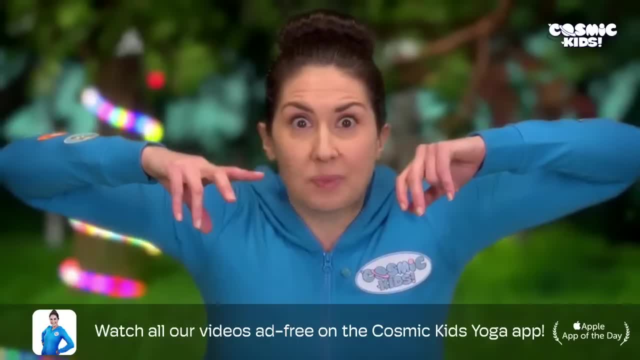 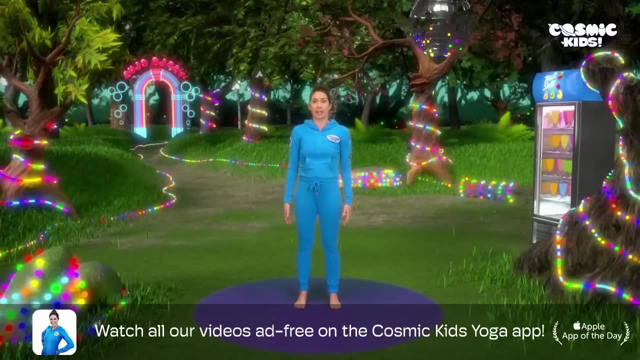 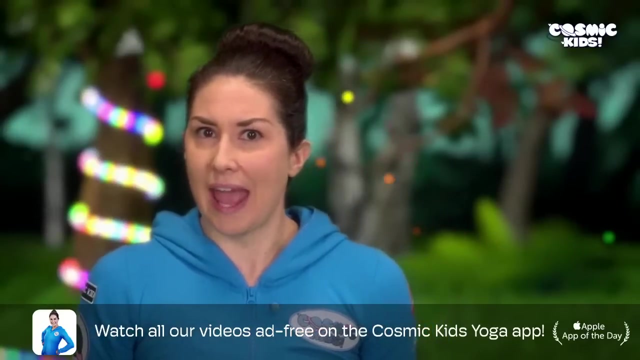 Everyone stops as still as mountains to stare, standing with our feet, hip distance apart, arms down by our sides. Shocked to see her here for the first time. But as the music starts again, Nicodemia begins to dance, unlike anyone could ever have imagined, 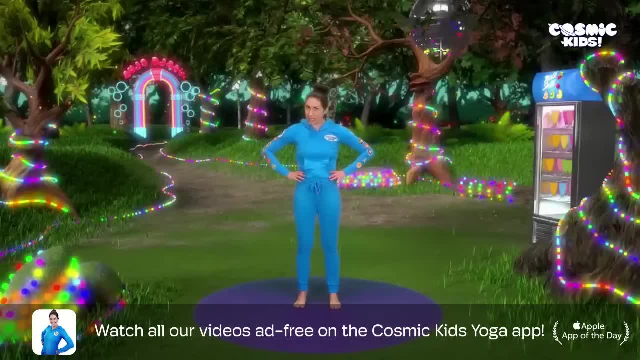 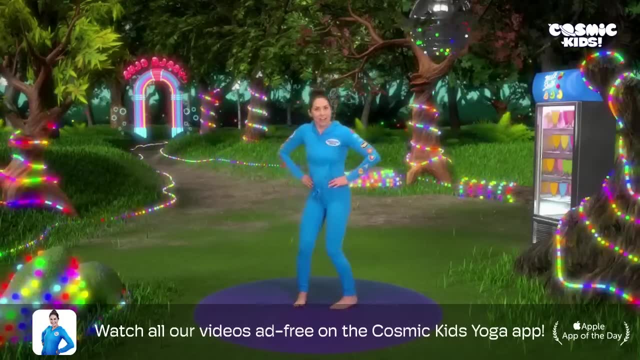 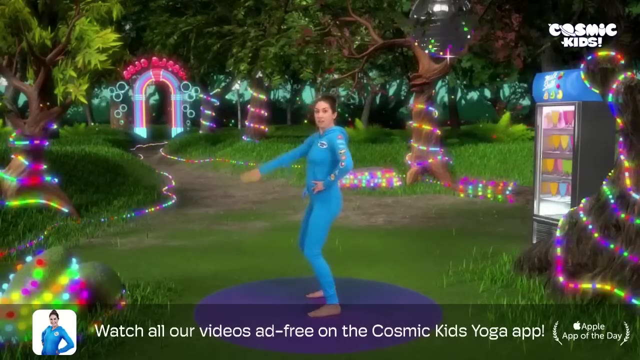 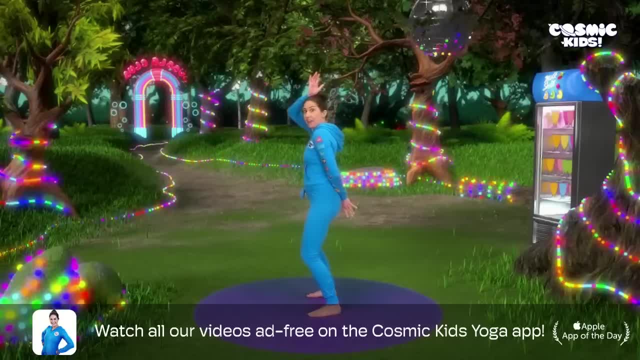 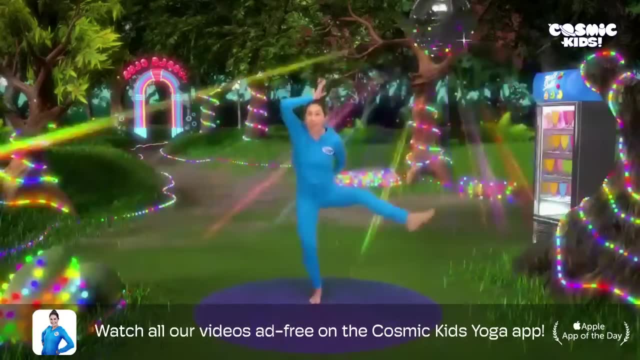 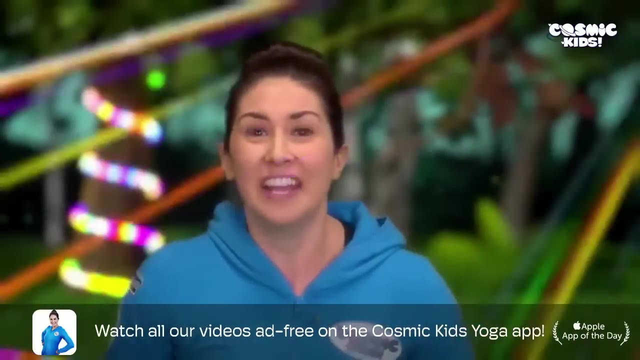 She even makes her head go back and forth. She even makes a comb on her head and a little tail feather with her hand And she kicks her legs up high to the side. Nicodemia is having fun. She is loving the dance. 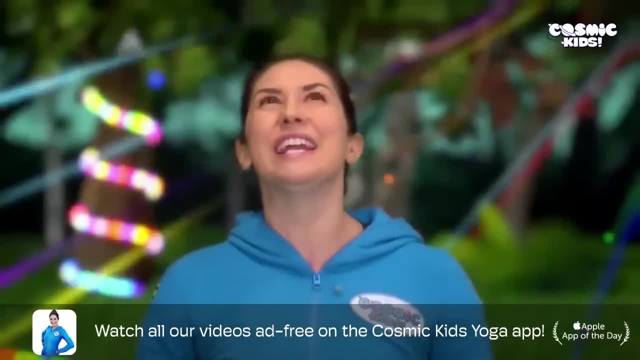 And so is everyone else, as we all join in dancing together. As we look around, we take a moment to step back. As we look around, we take a moment to step back. As we look around, we take a moment to step back. 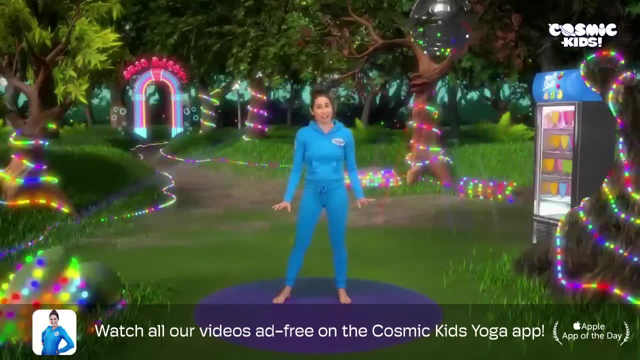 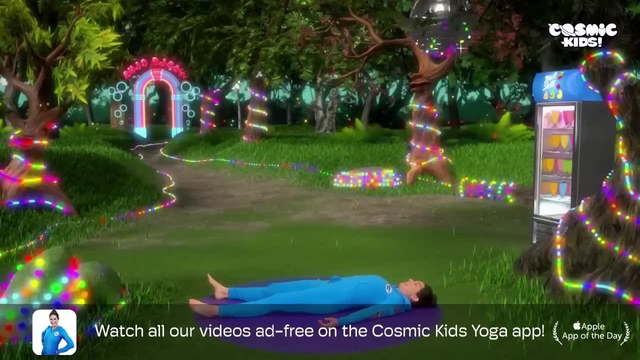 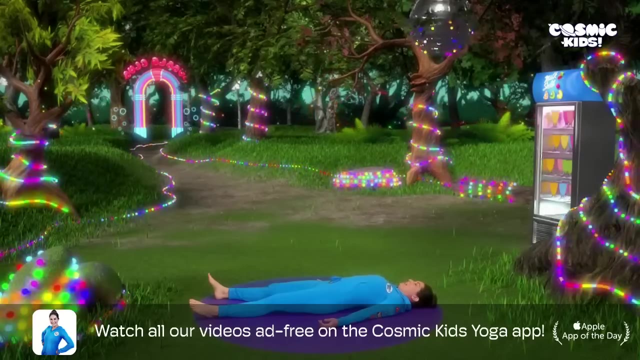 And we take this moment to lie ourselves all the way down on the ground. We stretch our legs long and our arms long And we let our bodies rest, allowing our breath to come back to normal. Wow, It's amazing just to notice how you feel in your body after you've been dancing. 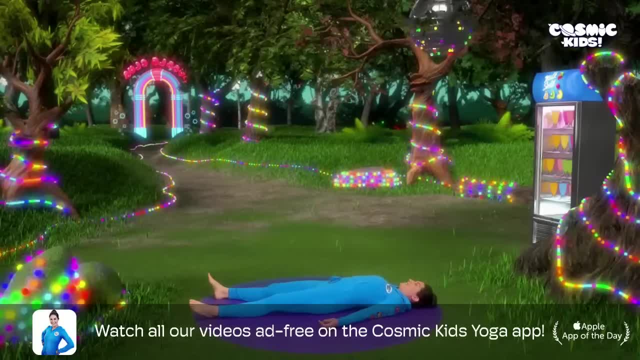 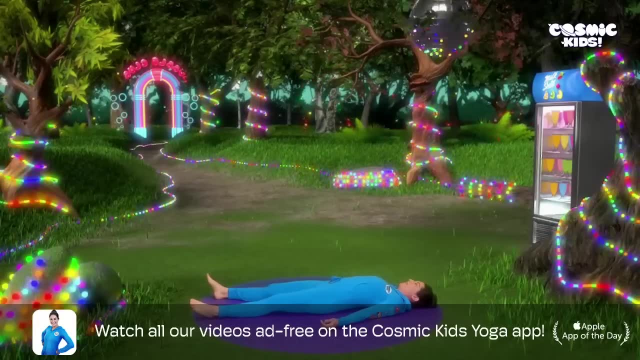 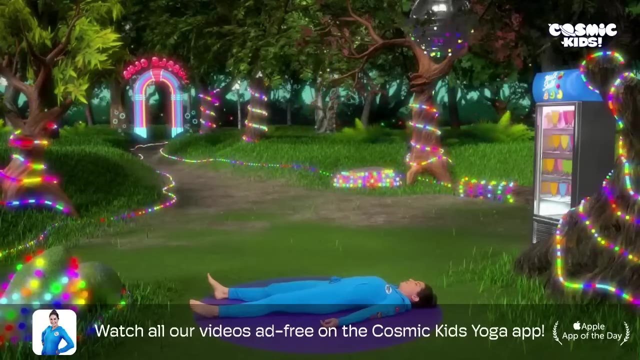 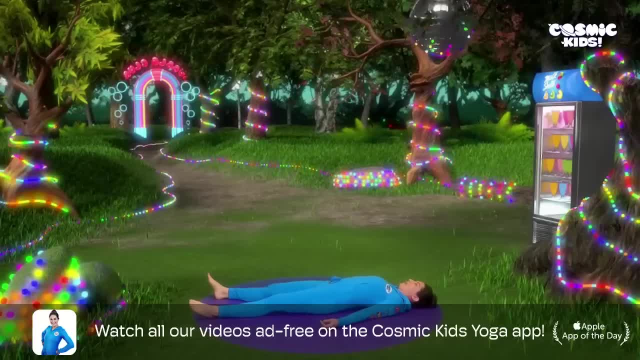 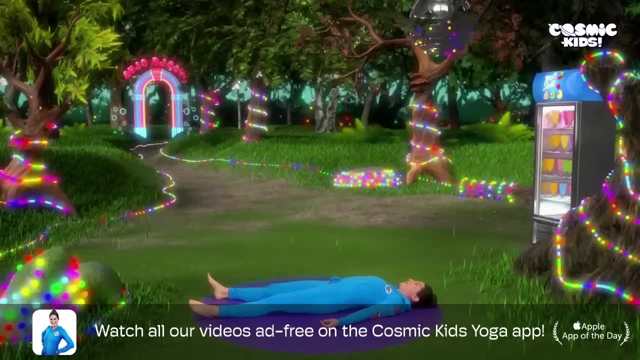 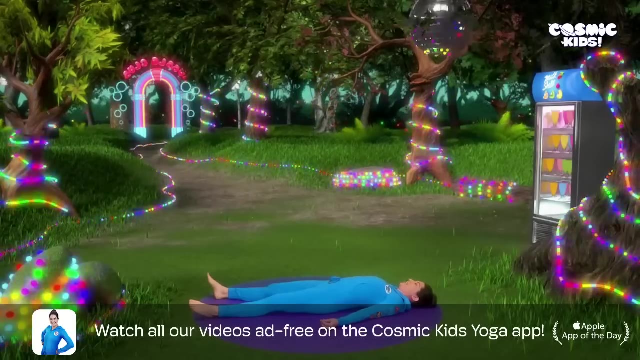 You make yourself feel good. It's a powerful thing like that, And when we dance together, when we dance with others, something very special happens. We create an amazing bond, A bond of trust, A bond of trust, A connection When we trust those around us enough to dance freely. 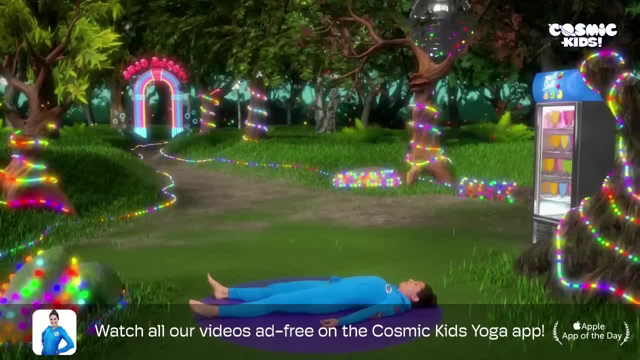 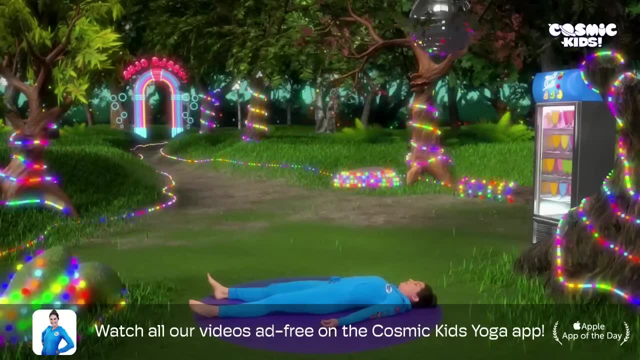 When we trust those around us enough to dance freely, when we feel that safe, we are stronger than ever. We are stronger than ever. We are open, We are free, We are able to learn And ready to listen, Ready to receive. 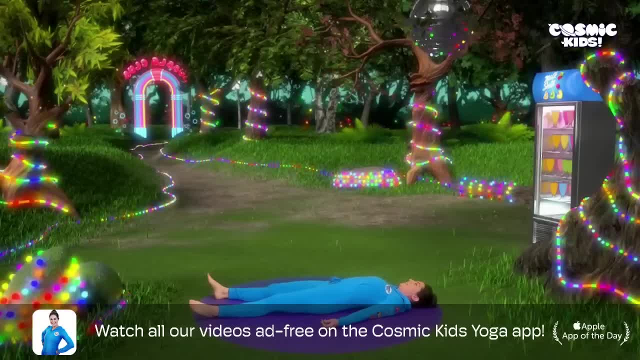 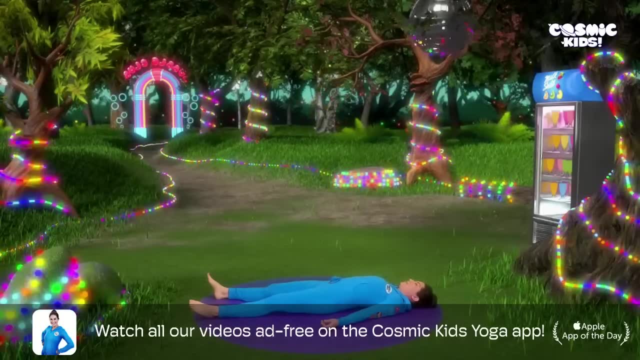 And ready to listen, Ready to receive. We're going to dance whenever you can And when you get a moment to share dance And when you get a moment to share dance with someone else, do it. You will only grow Slowly. now we begin to wiggle our fingers. 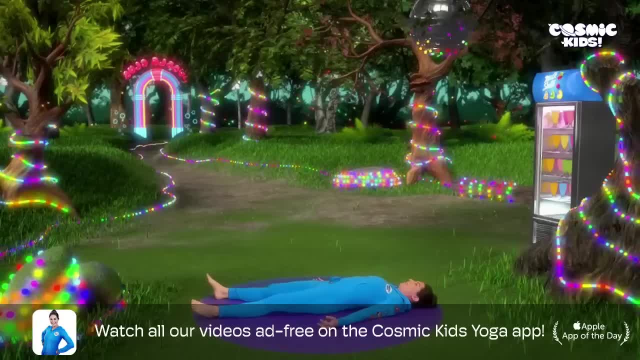 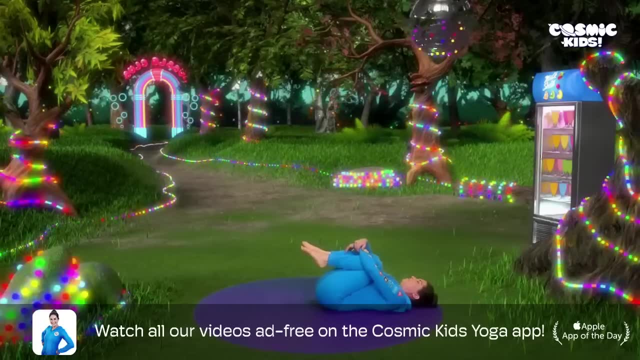 Slowly now we begin to wiggle our fingers and wiggle our toes. We hug our knees into our chest. We hug our knees into our chest, giving them a nice big squeeze, and then we roll onto our side, opening our eyes to press ourselves up to sit. 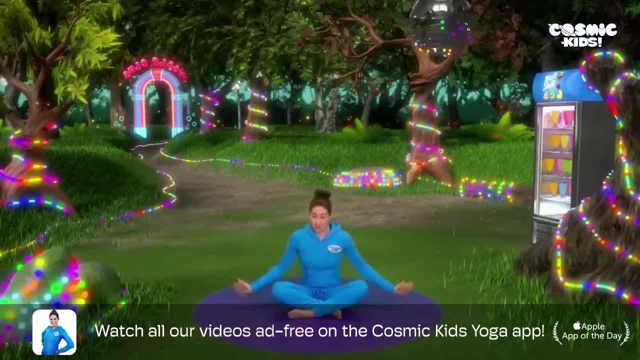 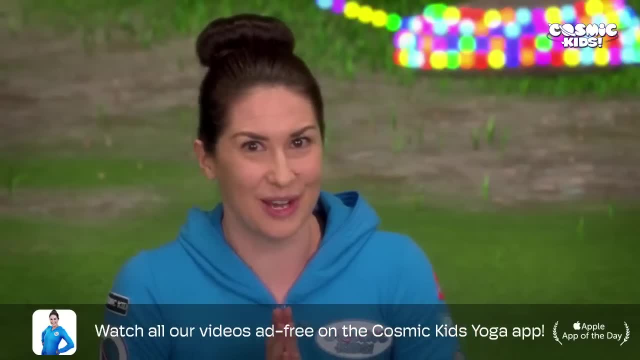 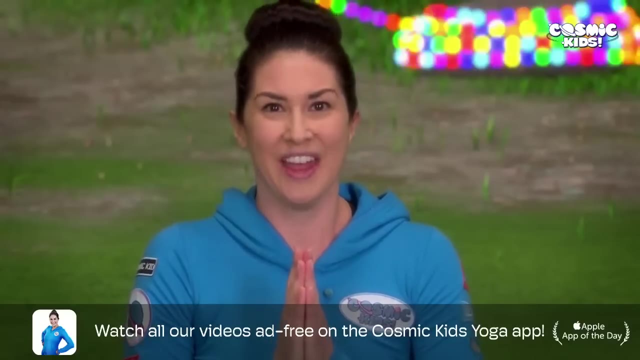 We cross our legs, We cross our legs, We cross our legs and we bring our hands together at our hearts and we finish just the way we started with our secret yoga code word which is Namaste, Ready After three. One, two, three. 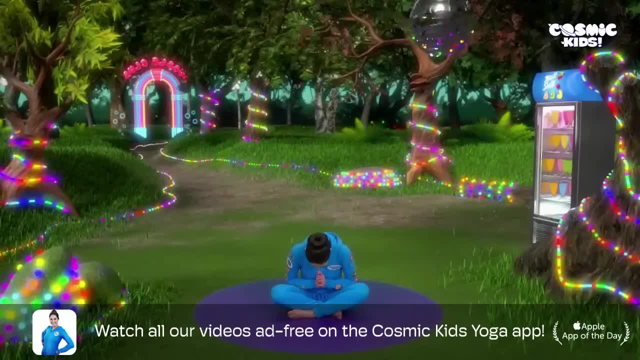 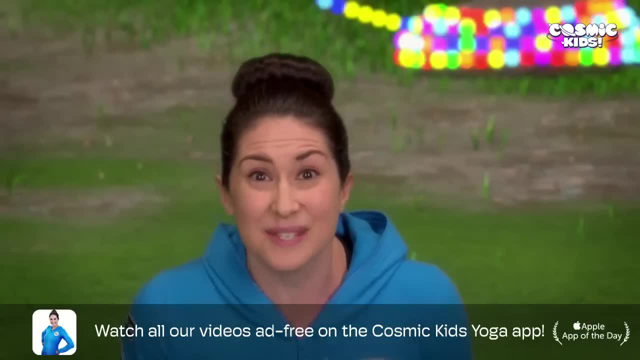 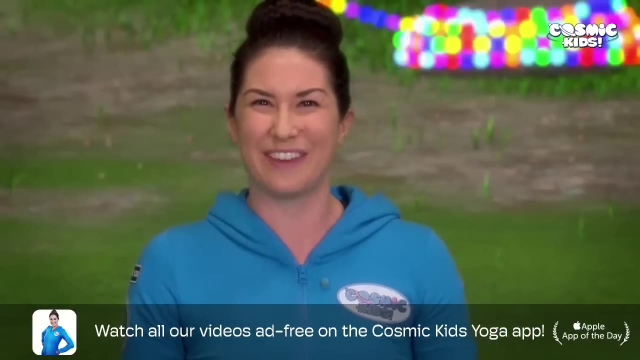 Namaste. Wow, Well done everyone. That was amazing. You were brilliant at dancing. Thank you so so much. I hope you enjoyed the Fairy Floss adventure and I hope to see you again soon for another Cosmic Kids adventure. Bye, bye. 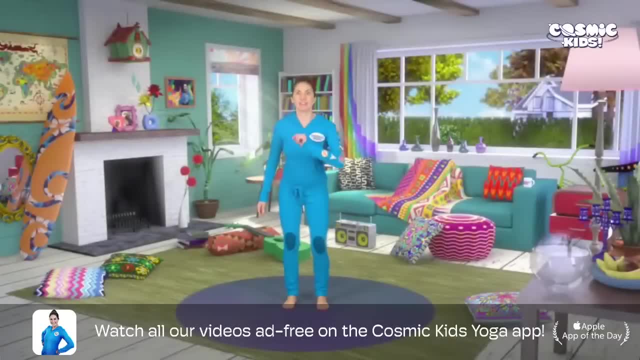 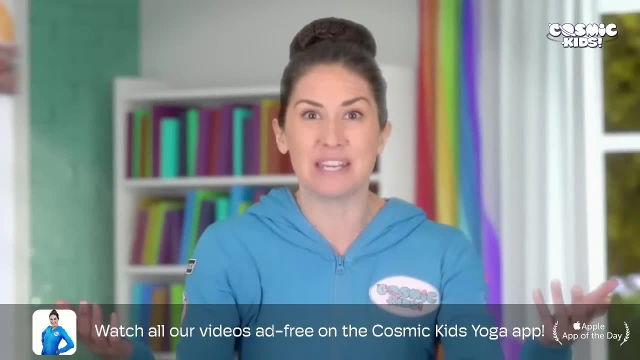 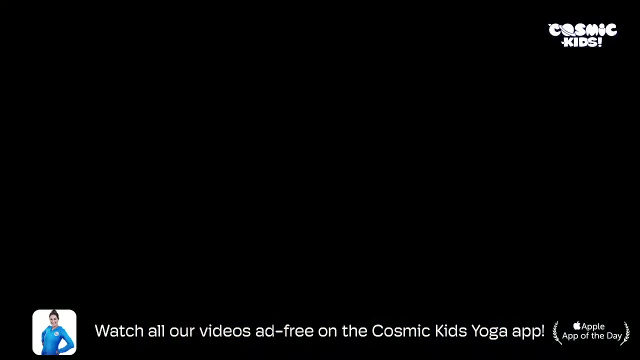 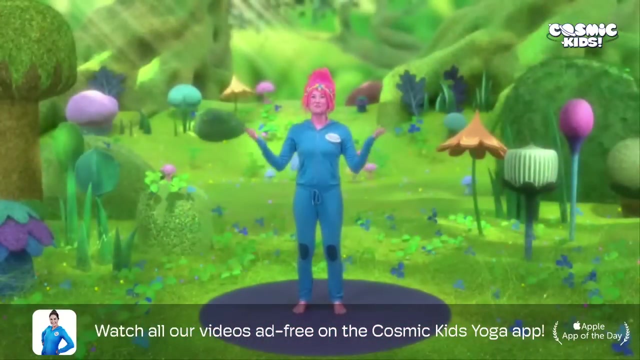 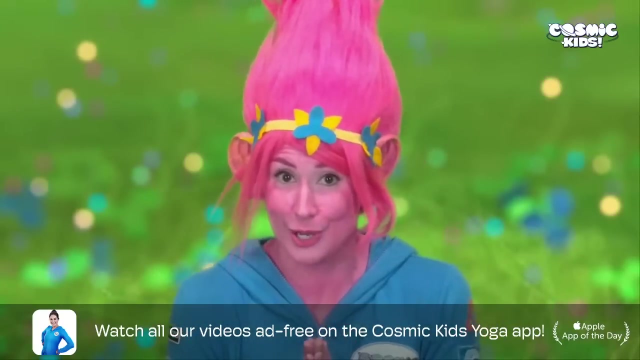 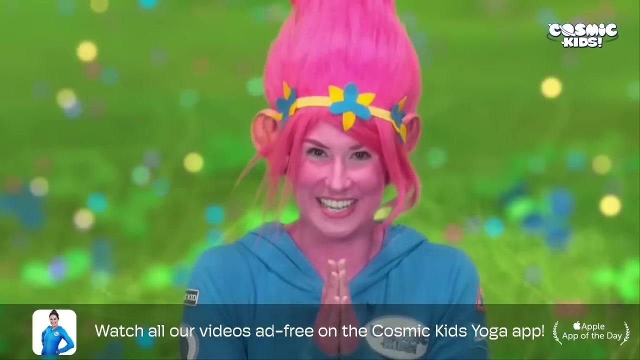 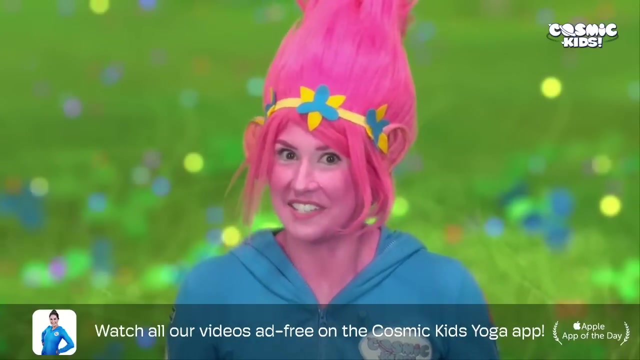 Don't forget to join me on Saturday morning for Saturday morning yoga. Get everyone at home together and enjoy some family time. Remember, subscribe and hit the bell so you never miss one. I'll see you Saturday, Bye, bye. Today we've got a special adventure. 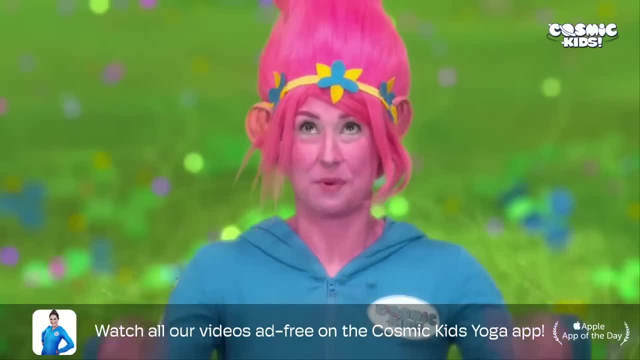 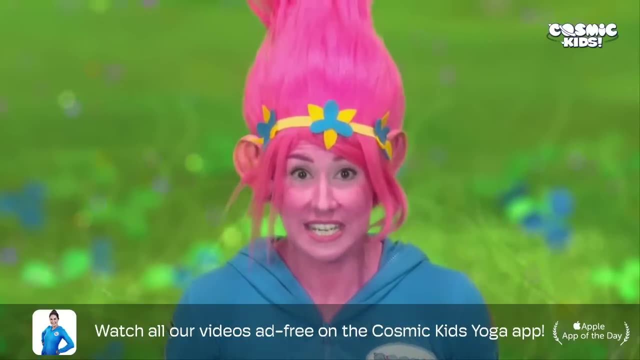 inspired by the Dreamworks movie Trolls. That's why I've got my pink poppy hair and my pink poppy body. Very exciting. Now our story begins 20 years ago in the happy forest, in the happy tree, So let's come up to stand. 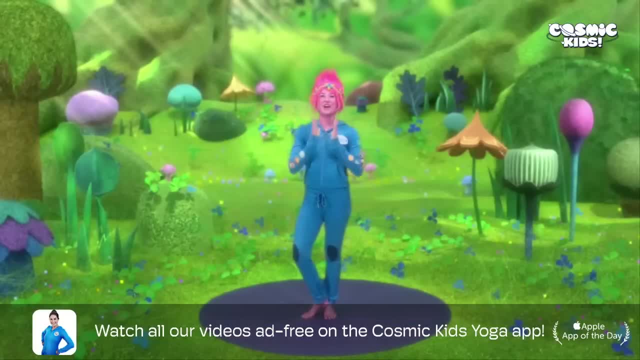 and do our tree pose, Bringing one foot on top of the other, our hands together at our hearts. Let's grow our tree up nice and tall, and open our branches and let's sparkle our fingers because we're a very happy tree. Yes, Now can we do our tree pose. 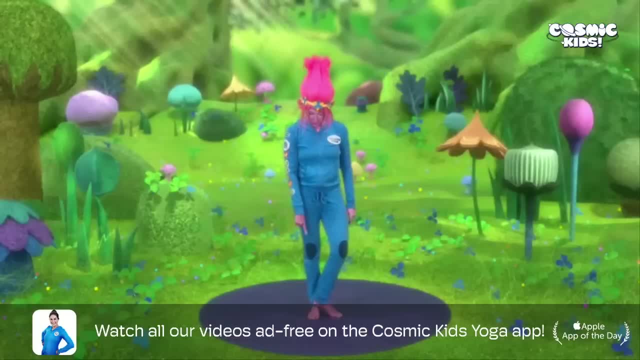 on the other side. Let's try. Bring your other foot on top now, using your heel. Bring your hands together at your heart and grow your tree up, nice and tall, opening your branches wide, sparkling your fingers and how about a big smile Ding? 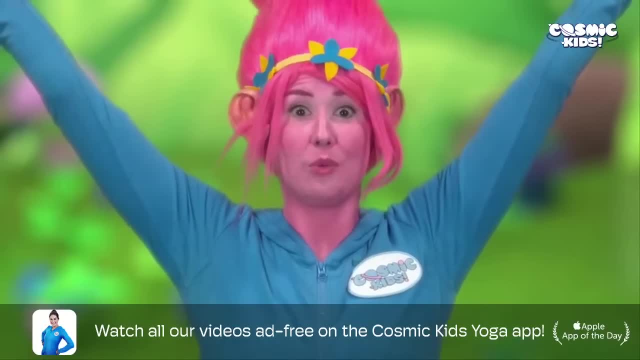 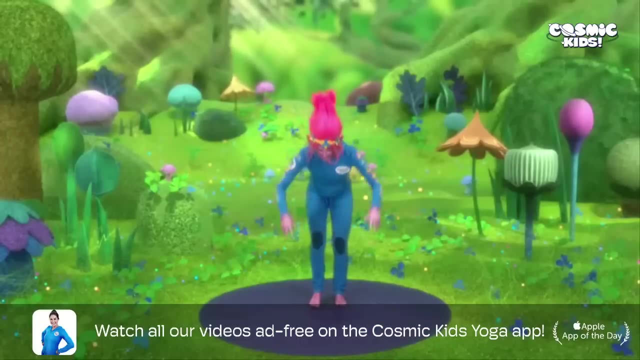 Yay, We're happy. trees Now living in the tree were trolls, Tiny creatures with big, colourful hair. Let's come into our troll hero pose Coming down on top onto our knees. Now take your hands forwards, take your feet wide and snuggle your bottom down. 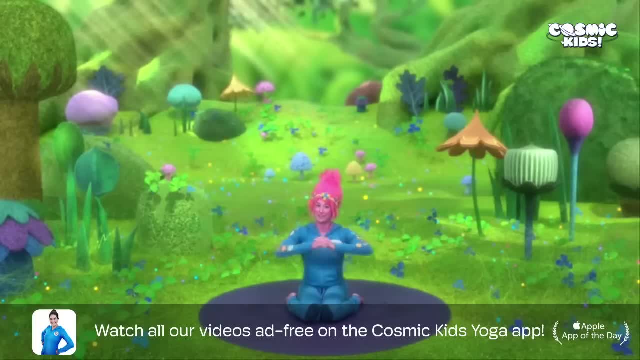 in between your ankles. Yes, Criss-cross your fingers, turn them inside out and lift your arms above your head, coming into your troll hero pose. Now, if that's a bit ouchy on your knees, you can lift your bottom, scoop your feet underneath. 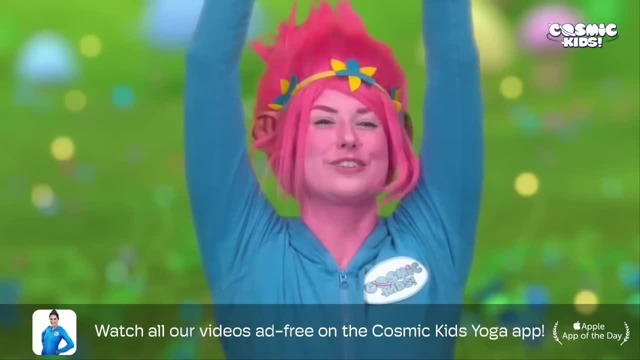 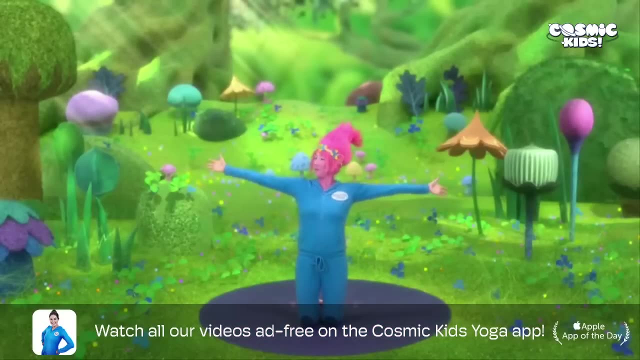 and sit back on your heels. Yes, Now, the trolls love to sing, to dance and to hug. Let's come up into a hug pose, Sitting up tall arms wide. wrap yourself up in a big, beautiful hog. Oh, it's wonderful Life for the trolls was full of glitter showers. 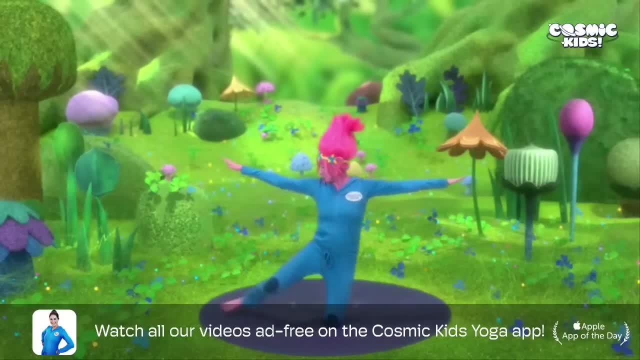 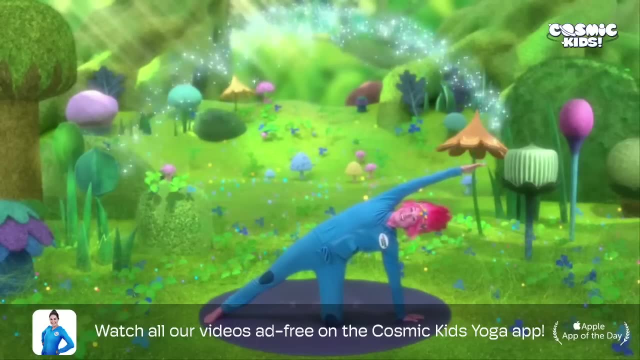 Let's come into our glitter shower pose Taking your arms wide, take your foot to the side and drop down onto one of your hands and sweep your arm up and over your ear. Yes, Making a glitter shower appear, It was also full of rainbows. 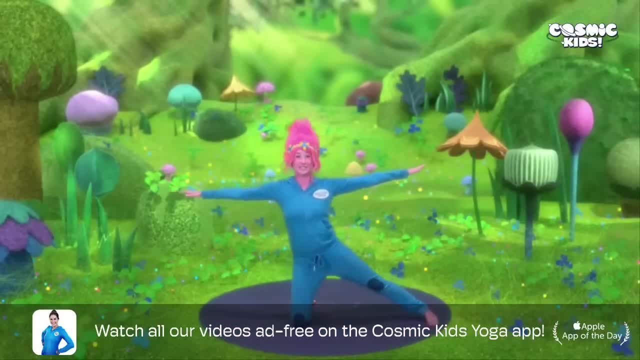 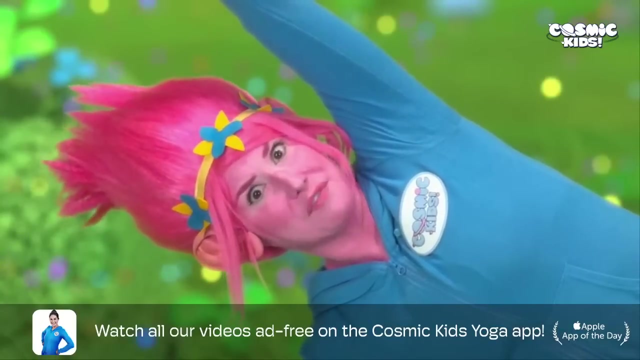 Coming back to two knees, arms wide, leg to the side, drop down onto one hand and sweep a big, beautiful arcing rainbow over your head. Wow, how lovely. Now the Bergens were the exact opposite of the trolls, always feeling sad and clomping heavily around Bergentown. 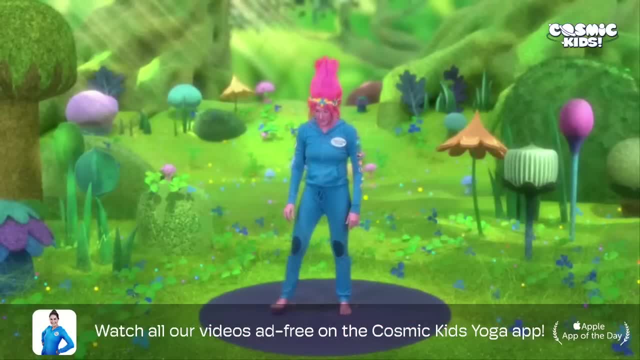 Coming up to stand in our clompy Bergen pose, Feet nice and wide, fold your body forwards, holding onto your ankles, and let's clomp. Here we go: Clomp, clomp, clomp, clomp, clomp, clomp. 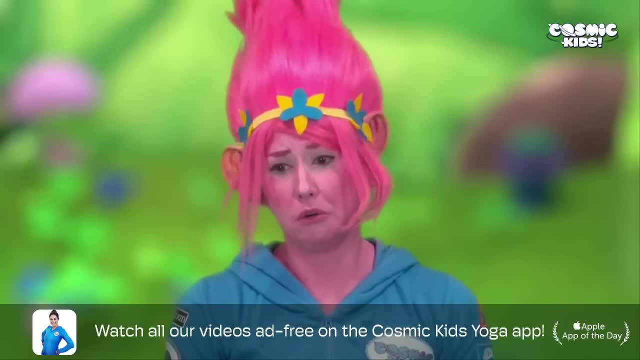 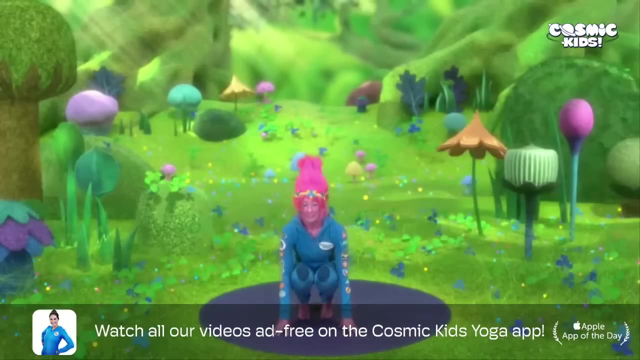 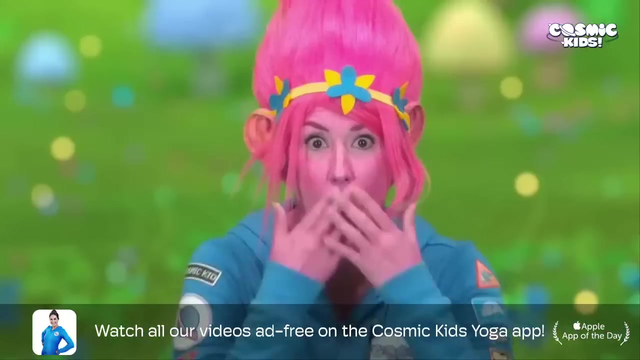 Rolling up to sad stand. Oh, to be happy like a troll, That's all they wanted. Then one day coming down to crouch fingers to balance a Bergen ate a troll, Seeing if you can balance with your fingers off and gobble a troll. 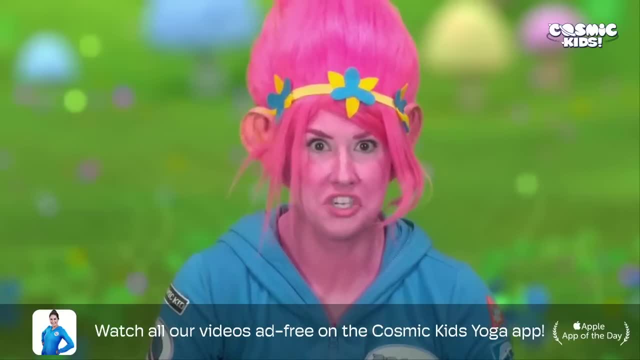 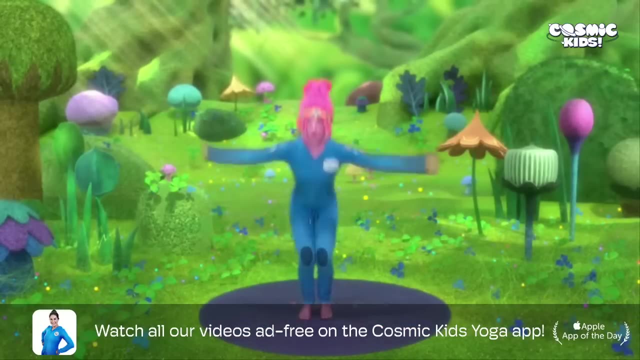 It made him smile And then it made him jump for joy with a big woohoo. After three, let's do a big woohoo. jump in the air, One, two, three woohoo. So this is the secret to happiness. 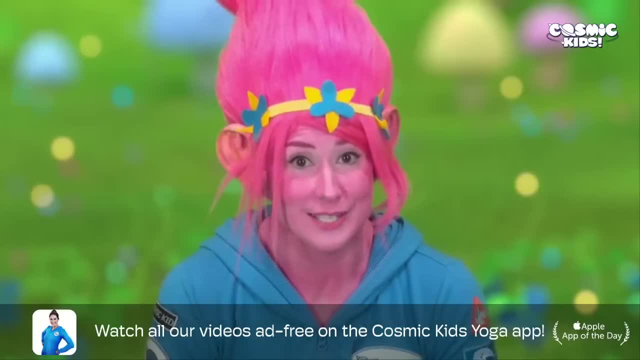 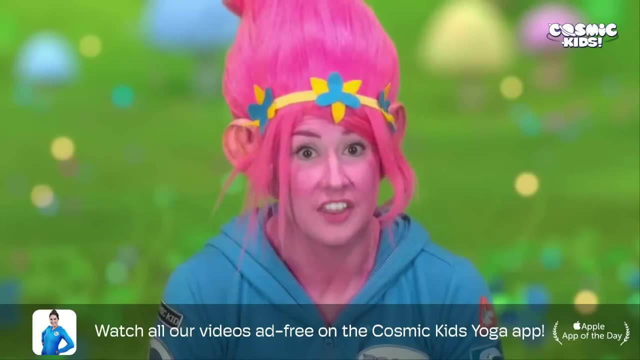 Eating trolls. And so they hold a festival each year, Trollstice, where they feast on trolls to be happy for one day One trollstice, the young Bergen prince, Prince Gristle, is lying in his bed, Coming to lie on our beds everyone. 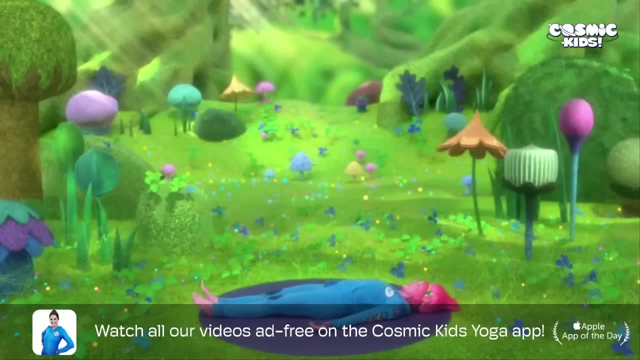 Legs out, long arms down by our sides and closing our eyes. It was time to wake up, so we open our eyes, He sits all the way up and he stretches excitedly. Today's the day he gets to eat his first troll, And no ordinary troll. 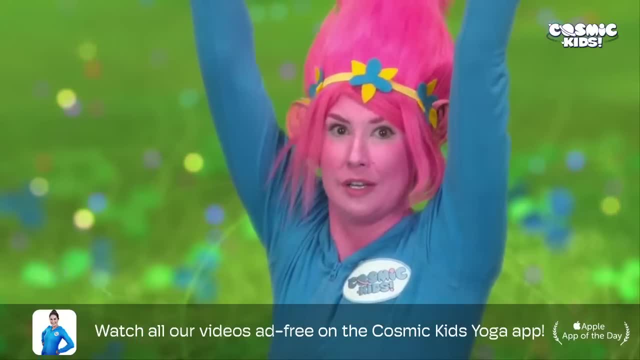 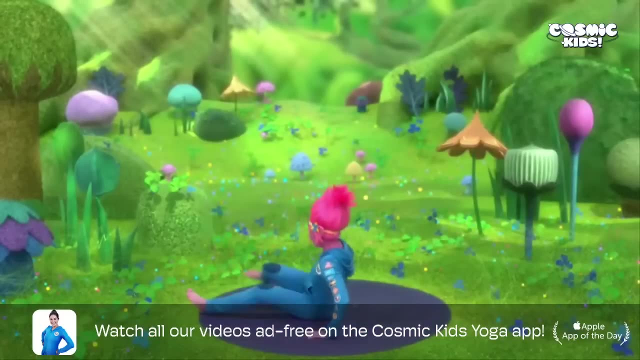 Princess Poppy, the special baby troll. But come feast time all the trolls escape down the secret tunnels. Coming into secret tunnel, pose Onto our hands and our knees, Tuck your toes and lift your hips all the way up to the sky. 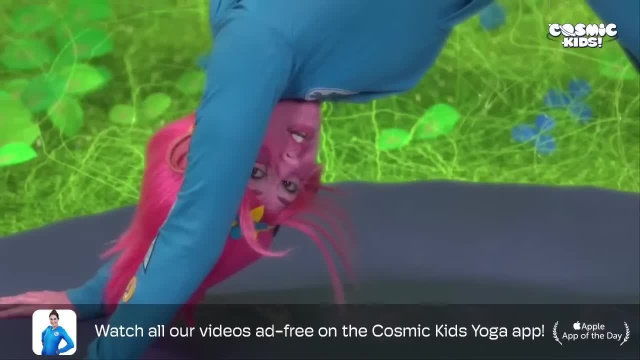 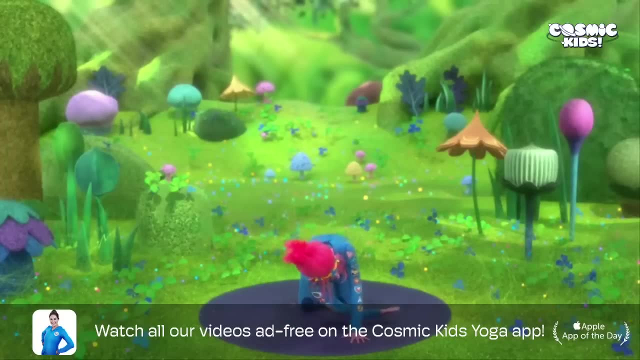 They're escaping And the Bergens reach down after them with their hands, Coming onto all fours again. everyone Now scoot your hands through the gap between your arm and your leg and see if you can rest on your shoulder, Reaching for a troll. 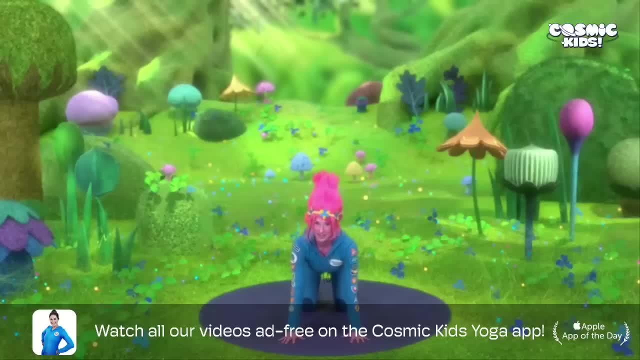 Ah, Coming all the way back up, Let's do that on the other side. Scoot your hand all the way through the gap and reach for a troll the other way. Nope, they can't get them. Coming all the way up to stand. 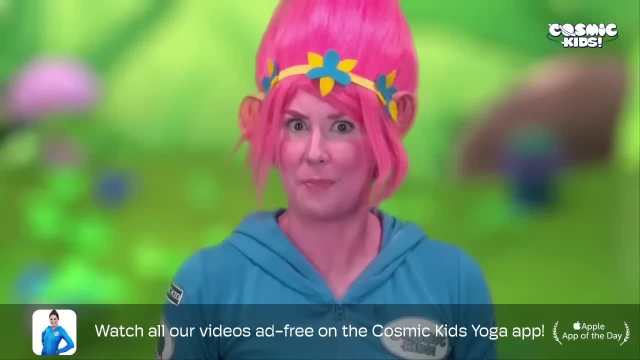 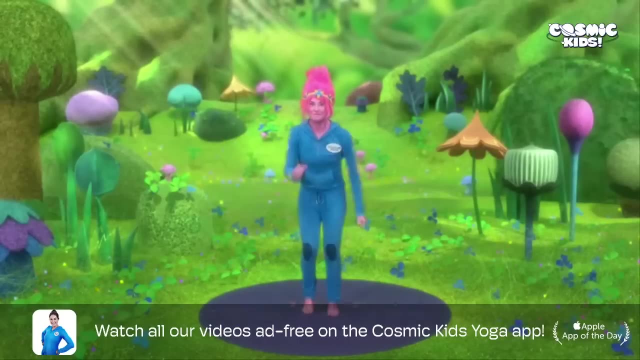 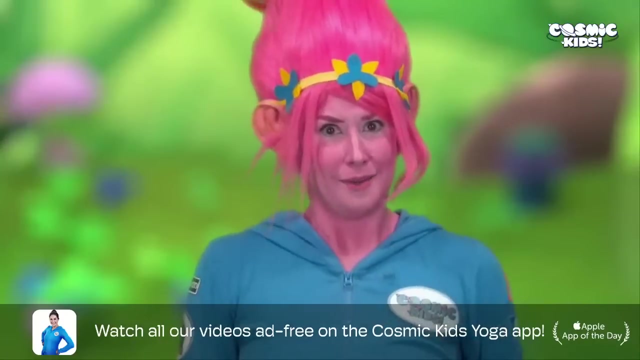 That's because the troll king King Peppy marches. his people to safety, Let's march, He chants. No troll left behind, No troll left behind, No troll left behind. Back in the Bergen Palace, the king King Gristle sits sadly in his throne. 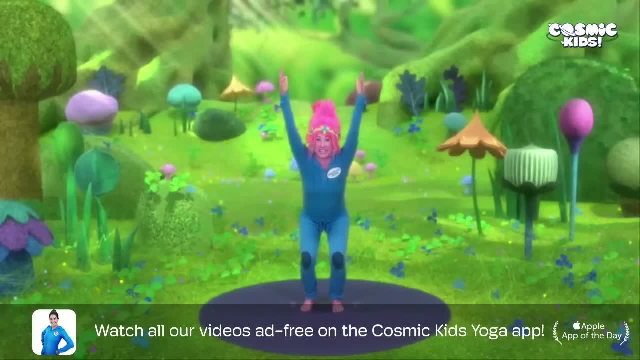 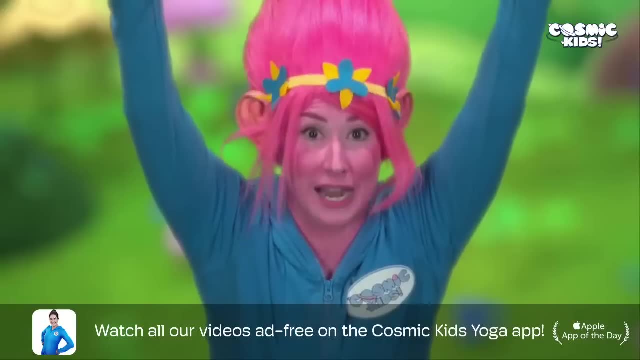 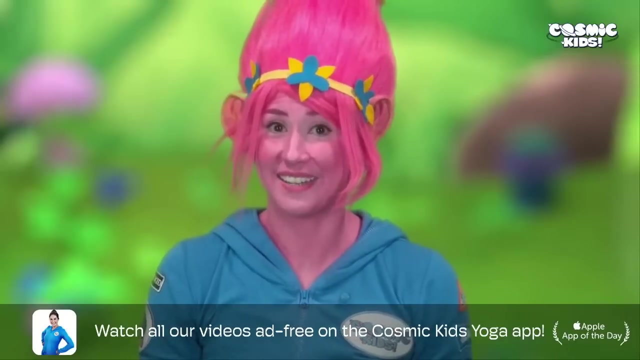 Bending your knees, sweeping your arms up by the side of your ears, Coming into your throne pose, He tells his young son that he will never be happy And he banishes Chef for letting the trolls escape. Coming up to stand Now, 20 years later. 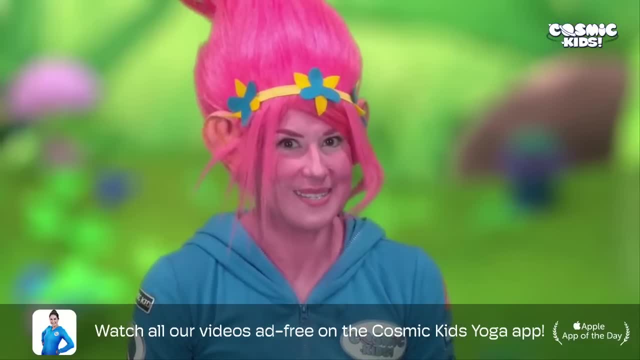 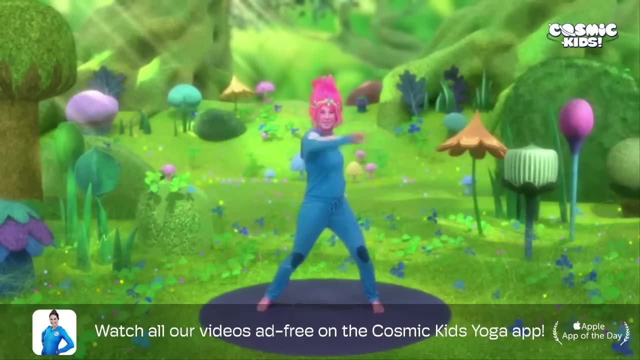 in the new troll kingdom, Princess Poppy decides it's time for a party. Jumping her feet wide, Taking her arms wide, She begins to spin And she sings, inviting everybody: move your hair and feel united. Oh Branch, the grey troll crouches down. 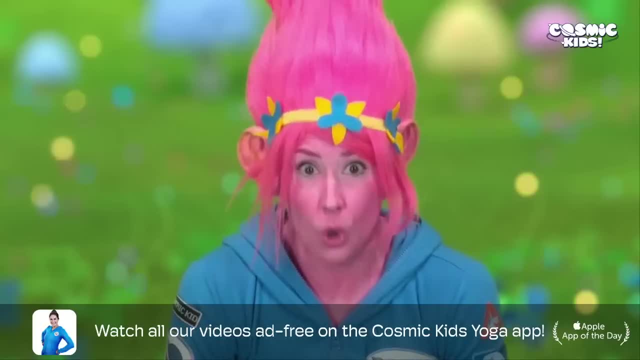 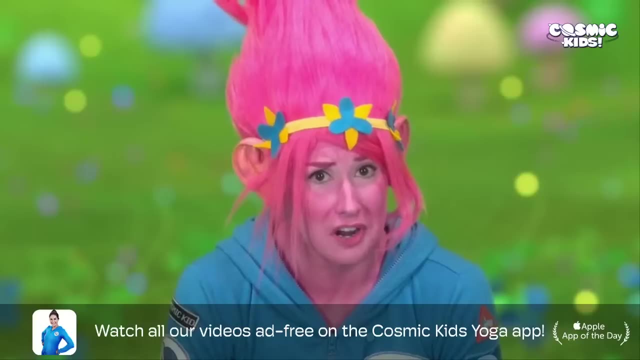 going: Shhh, Too much noise. Too much noise, and the Bergens will hear. You'll lead them straight to us. And then creak. The yogi troll arrives with a Namaste Sitting on your bottoms, crossing your legs. Bring your hands together. 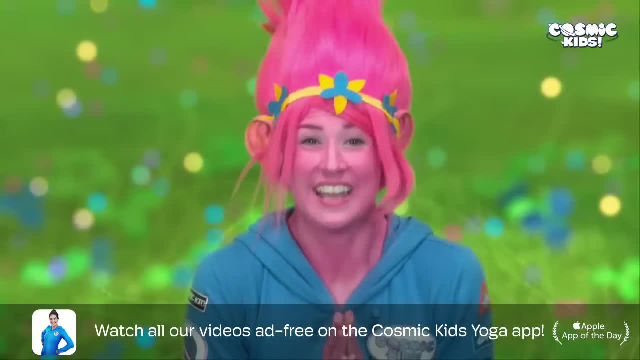 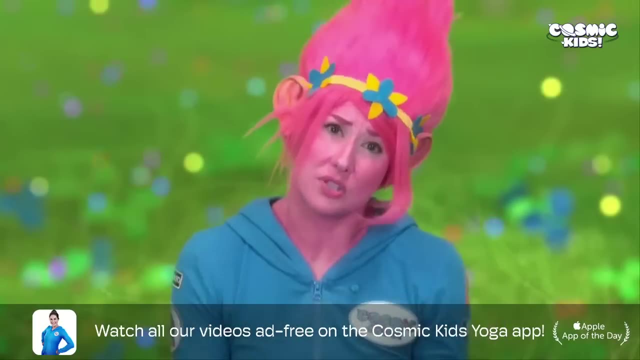 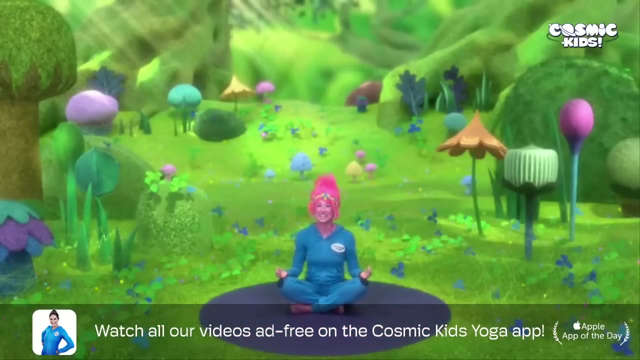 After three, let's do a Namaste: One, Two, Three Namaste. He encourages Branch to channel the positive energy And together we do an Om, Just to do that, Bringing our thumbs and fingers together, Resting them on our knees, And let's Om. 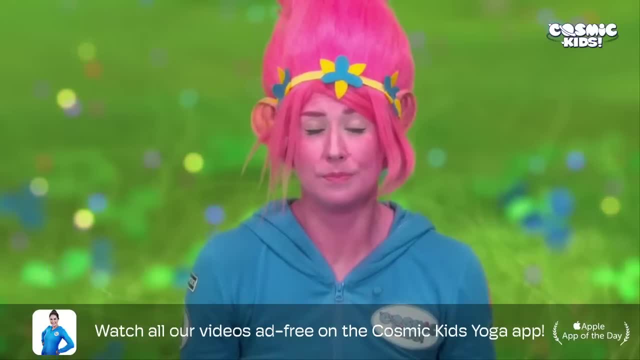 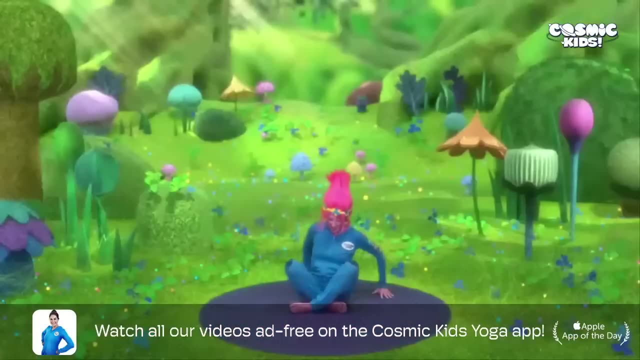 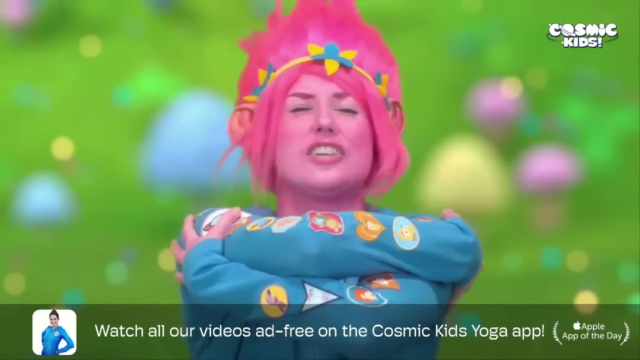 Om, Opening our eyes, Bing, Oh, look at the time, It's hug time Coming up onto our knees, Arms wide, Let's hug, Oh, wrap it in, Oh, yes, I could squeeze you forever Now, despite Branch's warnings. 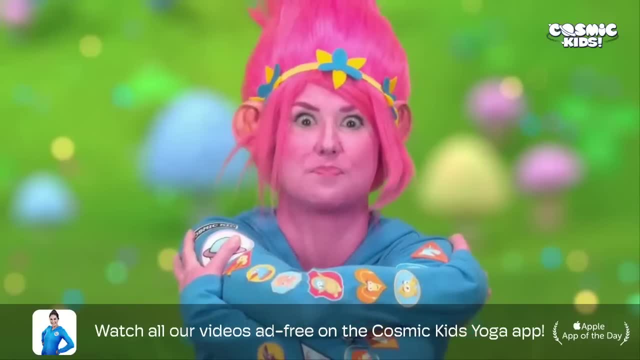 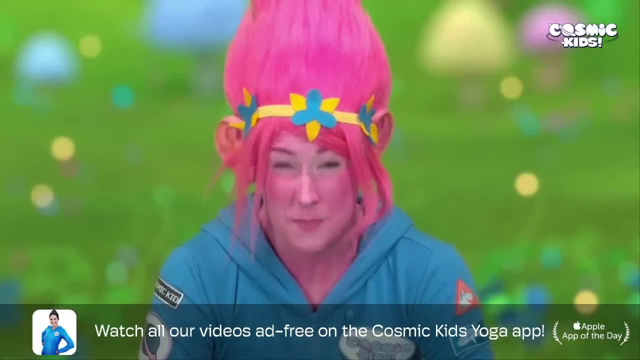 the party happens. There are glitter cannons Popping. Let's come into our glitter cannon pose, Up onto our tippy toes. Now we're going to jump in the air after three with a big pop of glitter. One, Two, Three Pop. 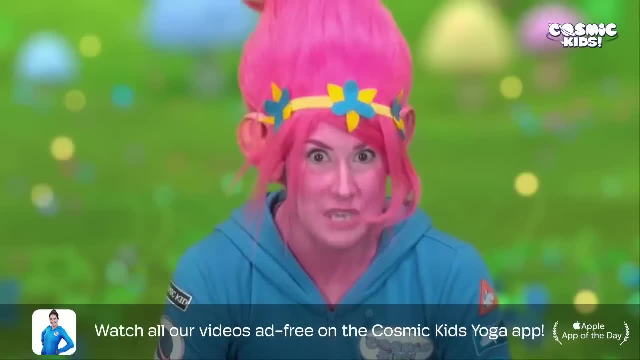 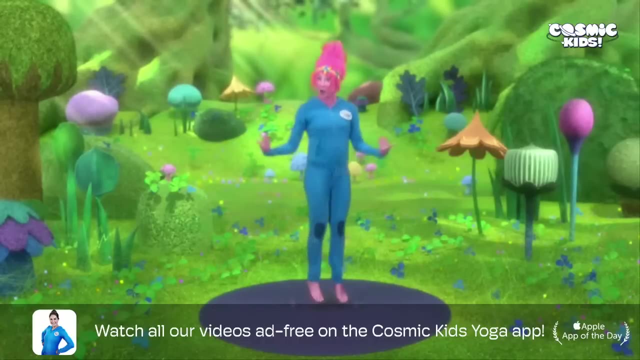 Yay, There's jumping to the music, Coming up to stand and let's jump, And there are light volcanoes exploding everywhere, Coming into volcano pose Down onto our knees, Up onto our toes, Up onto our toes, Up onto our toes. 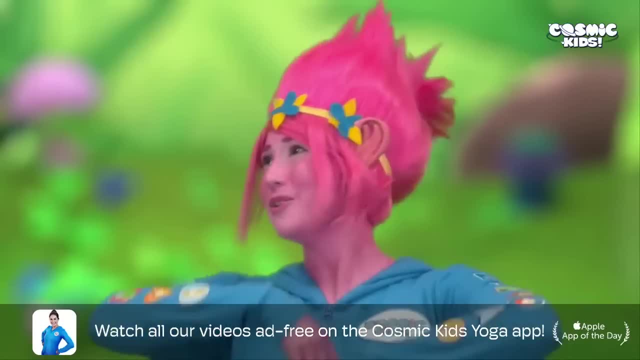 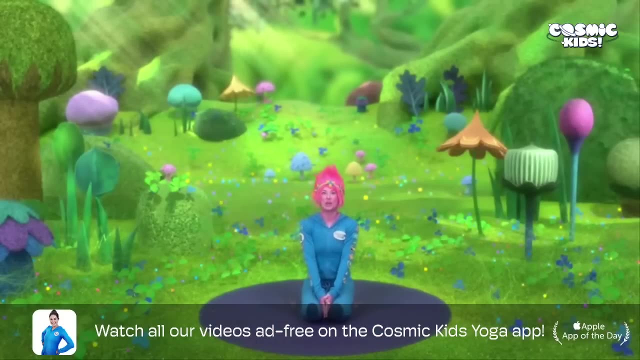 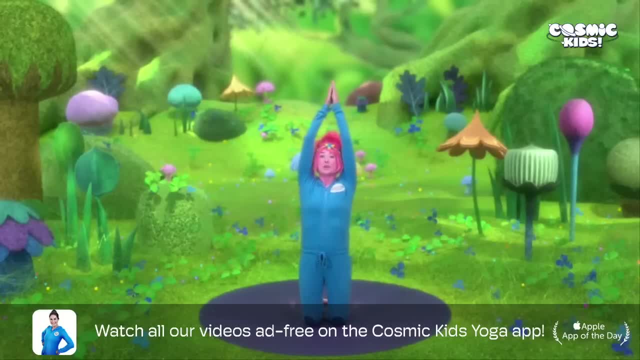 as we lift up, Here we go, And then we're going to blow a light volcano to the sky. Woosh, Breathing in. lift up, Whoosh And whoosh. a light volcano to the sky, Whoosh. Let's do a few. 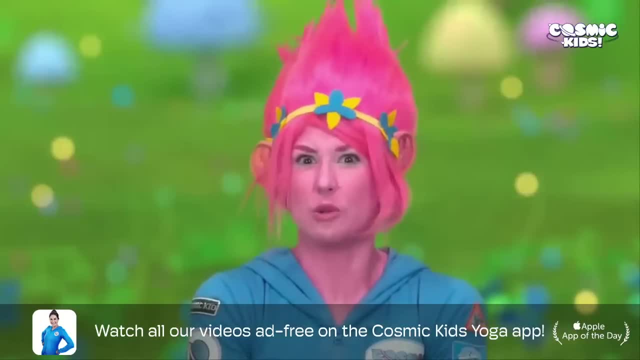 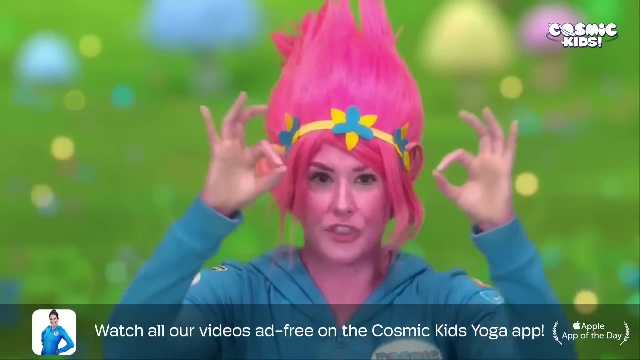 little ones: Pop, Pop, Pop. Wow, It's amazing. It is loud, So loud that the Bergen chef is loud. There is a little itty bit of them. She looks through her cosmonoculars, Joining your thumbs and fingers together everyone. 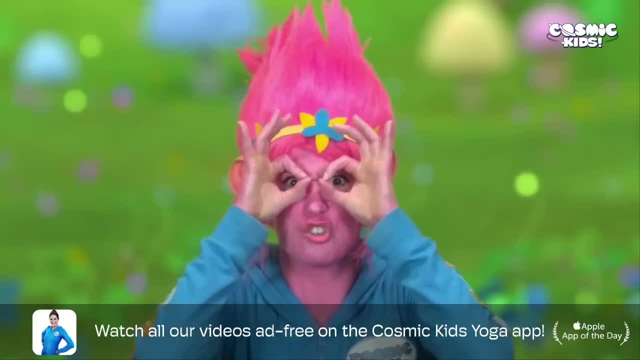 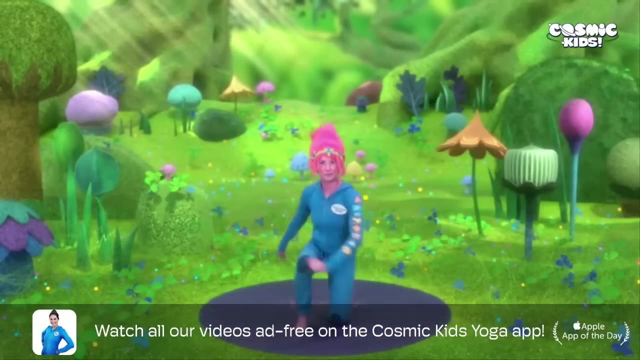 Have a look through. There they are The trolls. She sees them Lowering her hands. Here she comes, taking big steps, Coming up to stand everyone. Let's take a big step forward. Here we go, Big step. She reaches all the way forwards to grab a handful of trolls. Then she steps. 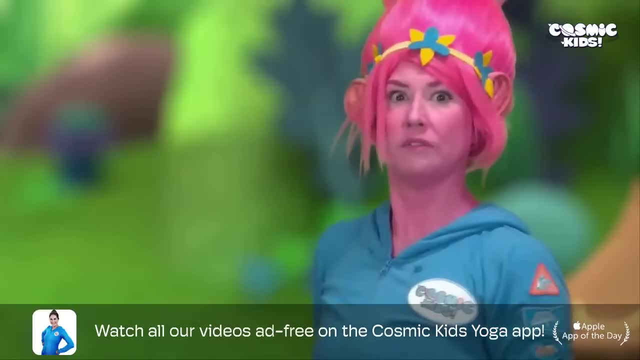 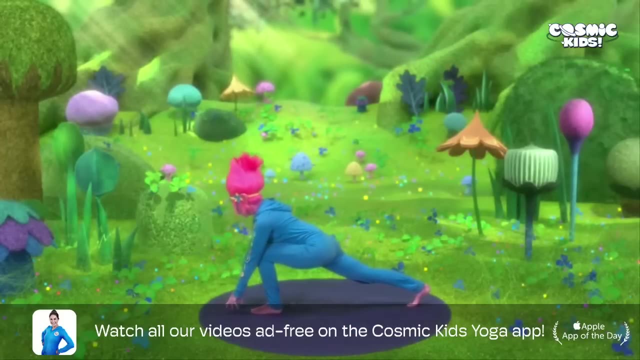 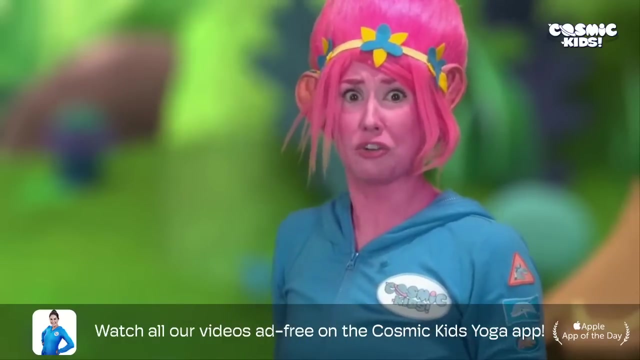 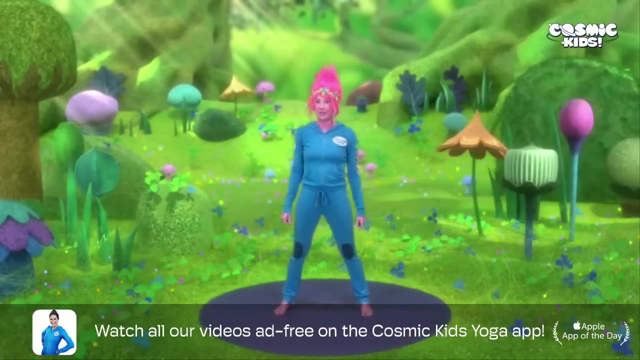 all the way back to put them in her pouch. Then she steps forward on the other leg, Big step. She reaches all the way in to grab those trolls And she steps all the way back, Whoop, To put them in her pouch. Oh no, The trolls run in all directions. Help King Peppy and 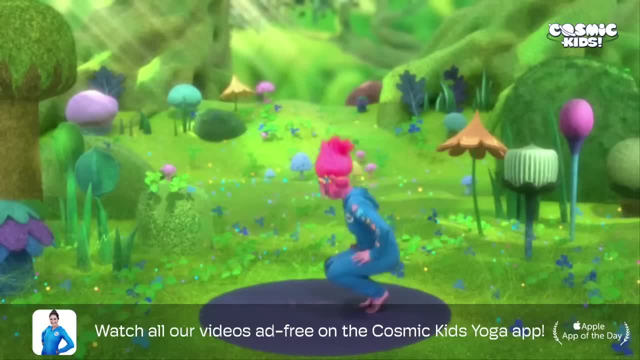 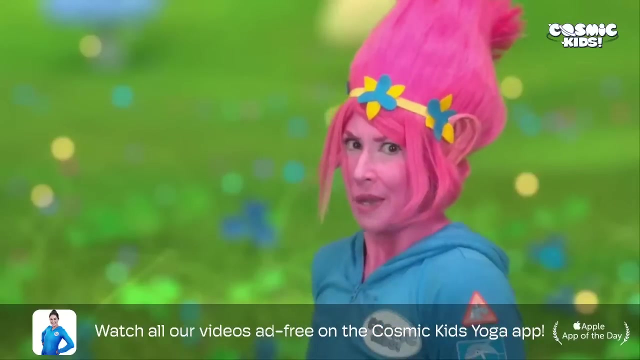 Poppy hide. Coming into hiding, pose Down onto our knees, Untuck our toes And then we tiptoes, Folding our heads all the way forwards To be very quiet as we hide under our hair, Coming up to sit. When the coast is clear, Poppy decides she needs to save everyone. 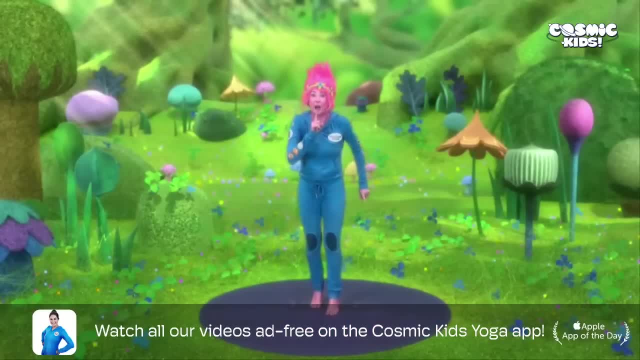 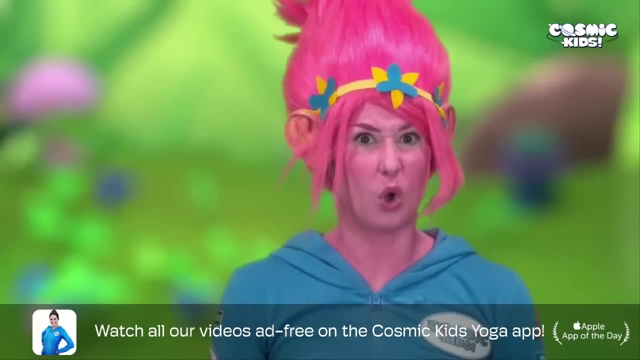 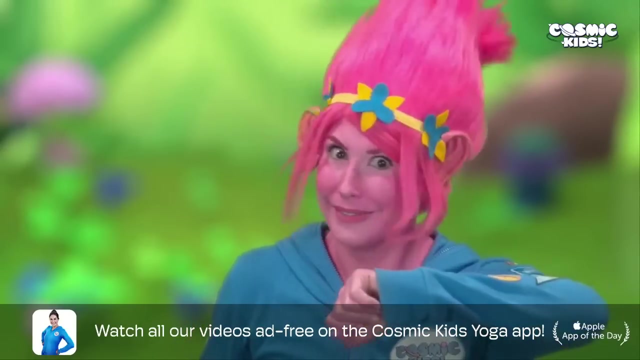 And she gets up quietly. She tiptoes down to branch the grey troll's bunker. She asks for his help, But he doesn't want to. And so Poppy brings all the other trolls down to hide With him, Just in time for Ding. Hug time, Arms wide, Wrap yourself up in that big, beautiful. 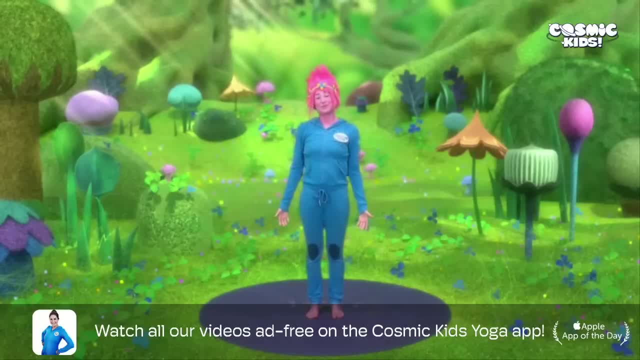 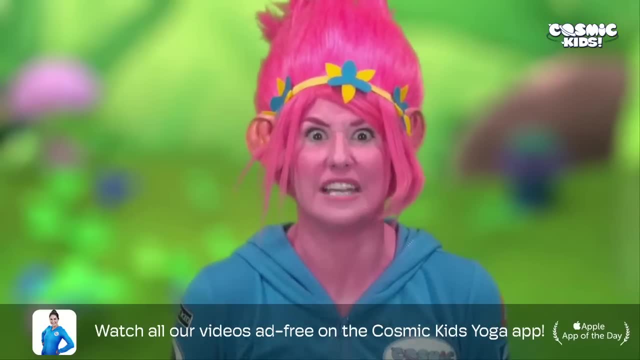 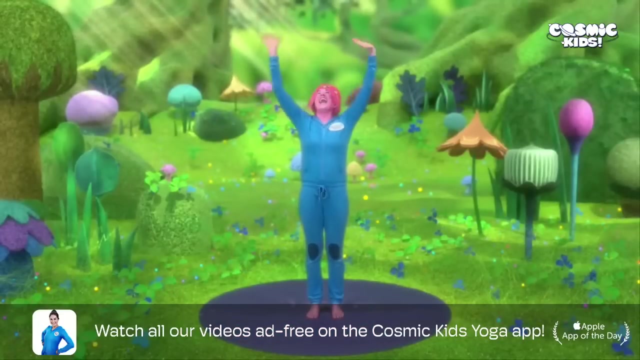 troll hug, Ah, Lowering your arms all the way to the side. And so Poppy sets out on her journey alone Into the scary forest, To feel brave. she sings about the sunshine Reaching up to the sun. Give it a wave and say Hello, sun. She sings about the butter. 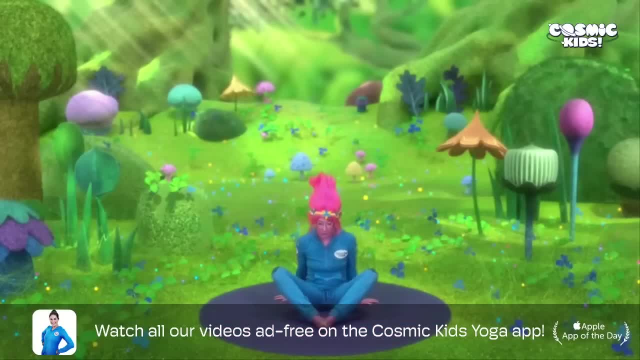 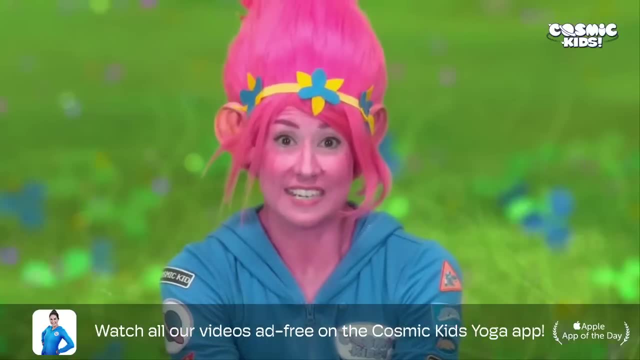 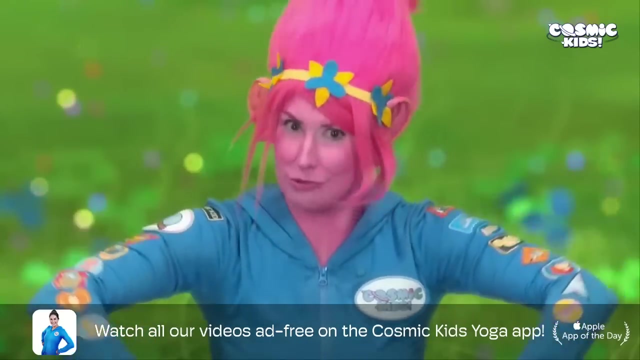 flies, Coming to sit in butterfly pose, Soles of your feet together, Holding onto your feet And fluttering your butterfly wings- Yes, Lovely, Even getting soaked by the rain, Using your fingers to pitter, patter your head And your face All the way round. Maybe your 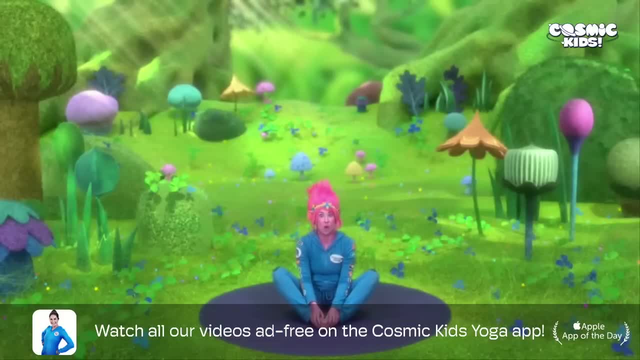 legs, Yes, And she gets chased by the wiggly wormy monsters. Coming into our wiggly wormy monster pose Onto our tummies. everyone Hands underneath your shoulders. Now wiggle, wiggle, wiggle, wiggle, And then We're back to our normal. We're back to our normal, We're back to our. 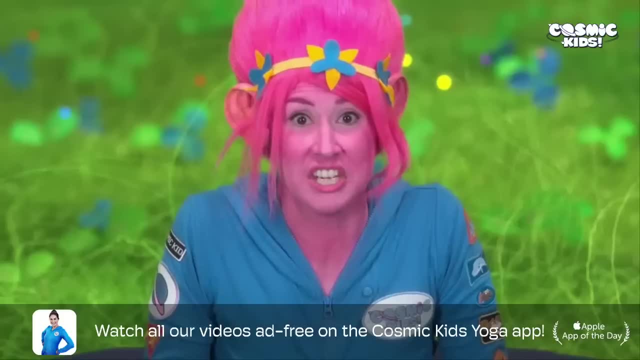 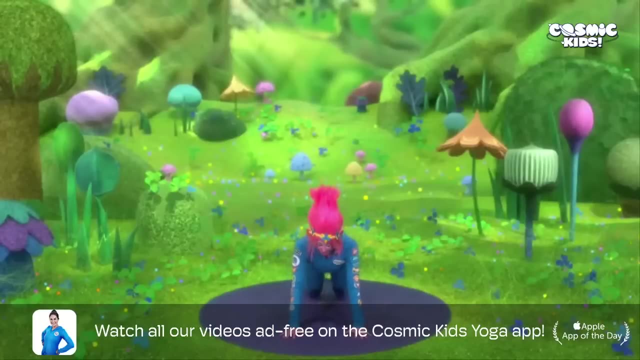 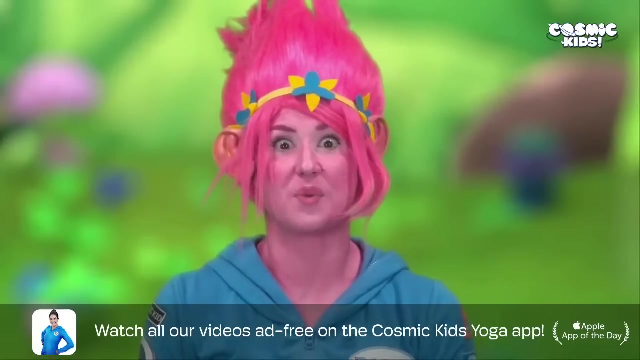 normal Giggle all the way up, Making yourself into a wiggly, wormy monster. She sings: I'm not giving up today. And about getting up again, Tucking your toes Up onto all fours, Walking your feet forwards And rolling up to stand. Then comes the spiders web Jump. 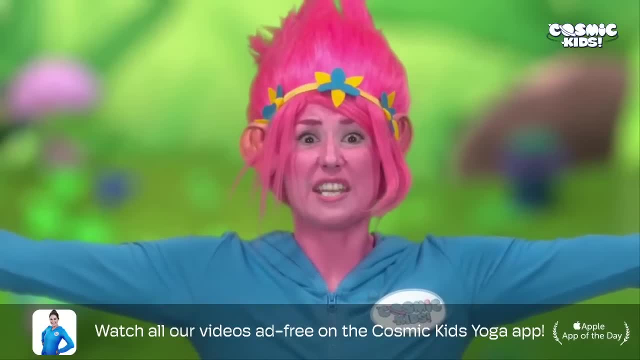 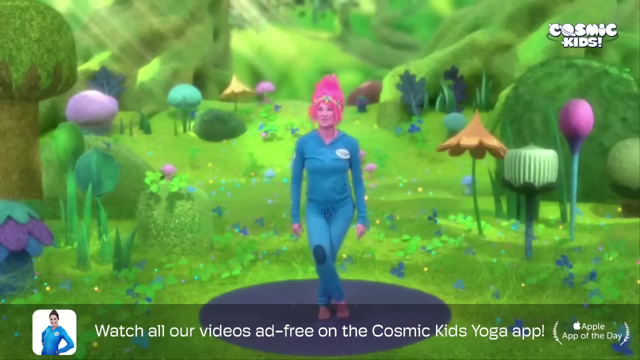 your feet wide. Take your arms wide. Oh no, She gets wrapped up in a sticky cocoon, Bringing your feet together Now, crossing one leg over the other and bending your knees. Arms like arms wide. scissor your arms. wave with your underneath arm and twizzle them. 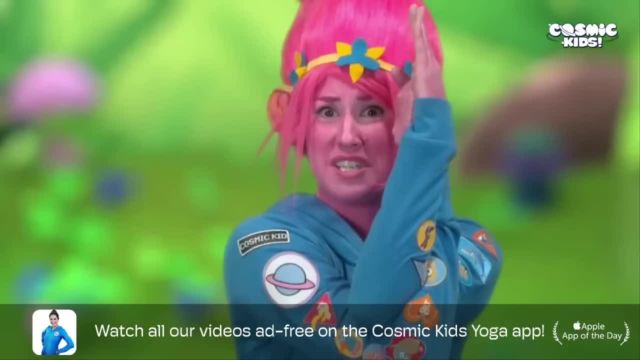 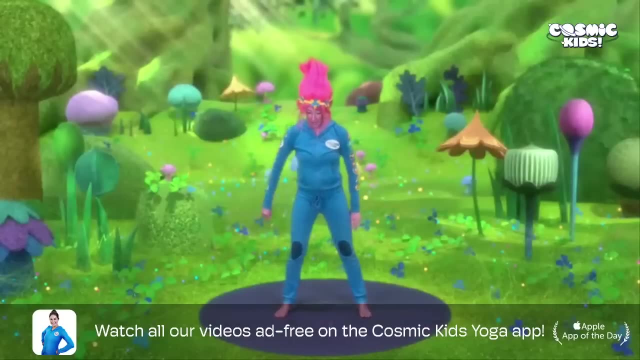 round, sitting yourself down a little bit lower. oh no, she's in a real sticky cocoon. and here come the spiders scuttling along to gobble her up, taking your feet wide, coming into spider pose, bending your knees, hands going between. 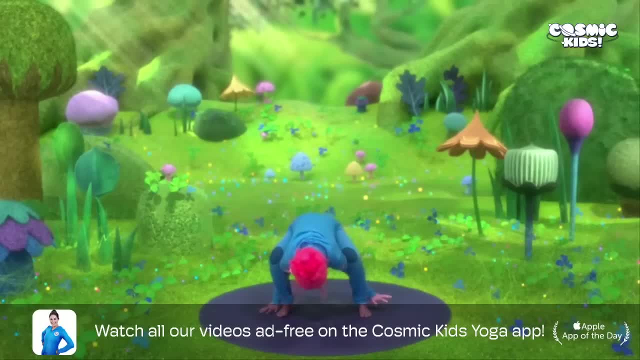 your feet now ticker, ticker, ticker your fingers round the back to the ins outsides of your feet and walk your feet all the way in coming into your spider pose. oh no, but just in the nick of time, who should appear but Branch the grey? 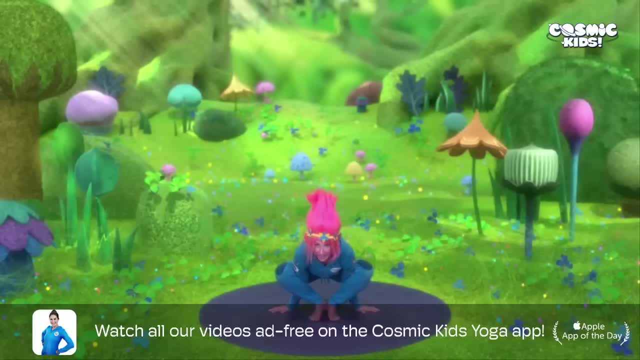 troll using his hair like a warrior to shoo them away. coming up to stand into our warrior, pose one foot forward, one foot back, bend your knee, sweep your arms up high and open them wide. let's shoo those spiders. 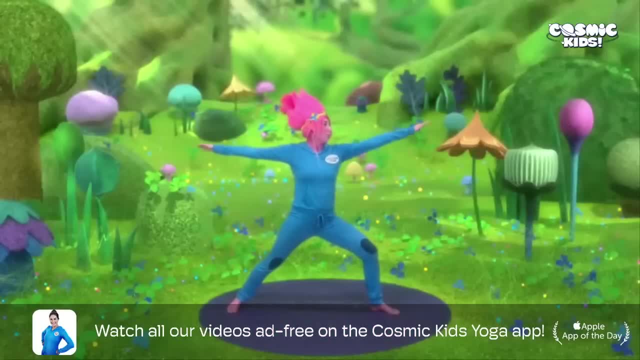 and jump the other way. Branch has decided he will help Poppy you together that night. they make a campfire, sitting on our bottoms with our legs crossed, bringing our elbows forward and wiggling our fingers like they're the flames of the fire crackling away. it's time to go to sleep, and so Branch. 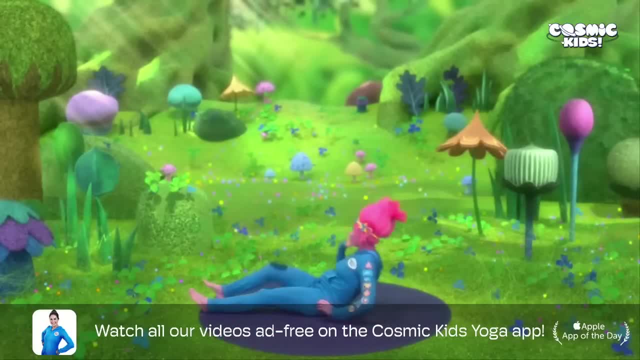 and Poppy lie down, lying down with your legs long and your arms down by your sides. Poppy can't really get to sleep and she looks up at the starlit sky. she sings: stars shining bright above me. Branch rolls over, taking your arms. 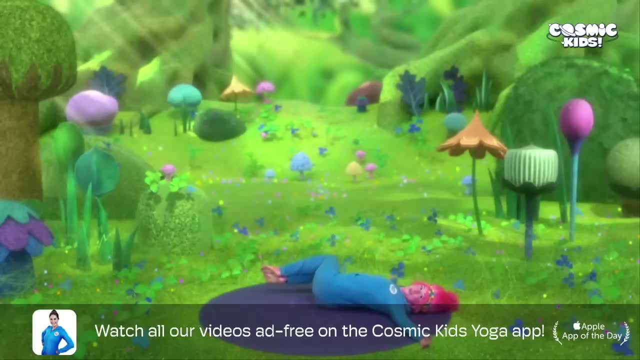 wide, bringing up your knees, taking them over one way and your head over to the other. he looks at Poppy and he goes shhhh. then he rolls over the other side, lifting up your knees, going to the other side and your head to the other side. Poppy sits up and she takes out a ukulele. 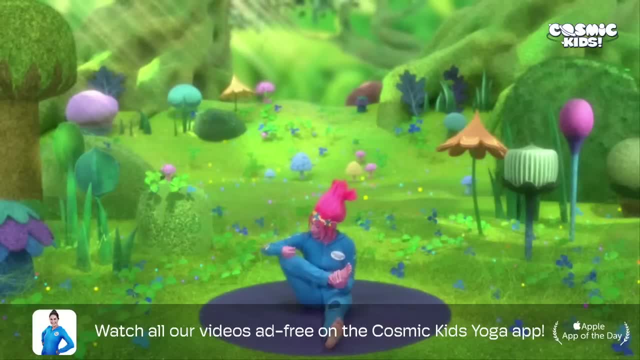 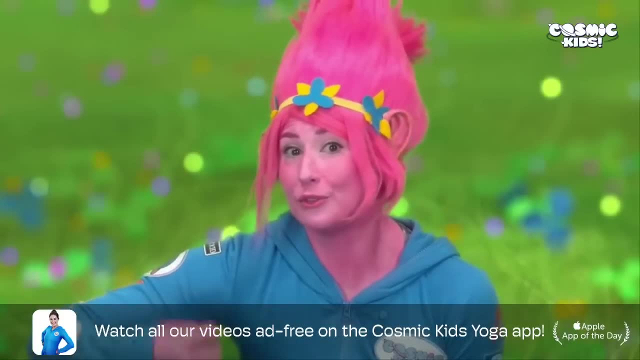 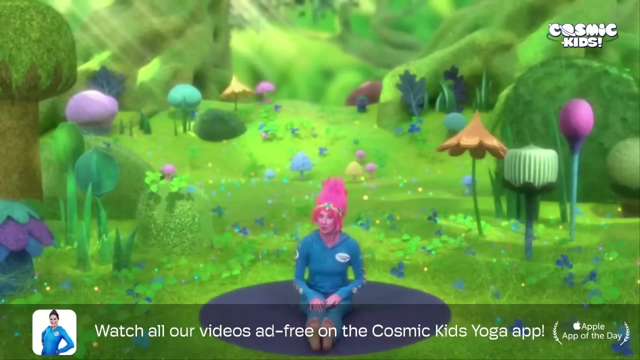 hold of your foot, bringing it to your body and strumming it like a ukulele. She begins to sing to Branch: Hello darkness, my old friend. Branch sits up, Poppy puts the ukulele down, Branch picks the ukulele up, picking up the other foot and he's going to play it, but before he does he throws it. 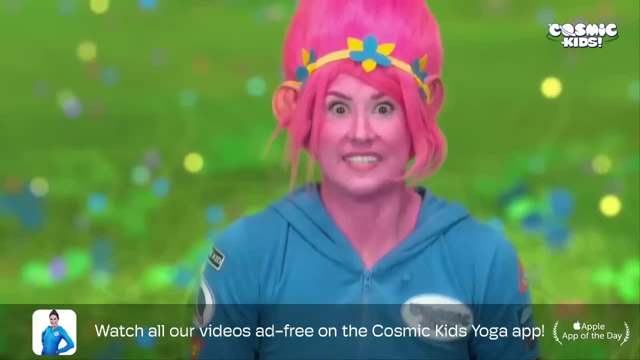 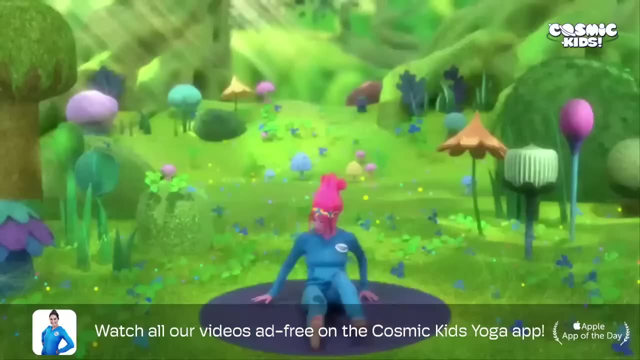 on the fire. Now, the next day, they arrive at the secret tunnels which take them down to Burgantown. Let's come into our secret tunnel, pose onto our hands and our knees, Tuck your toes and lift your bottoms to the sky. There are so many holes to choose from Which one will lead them. 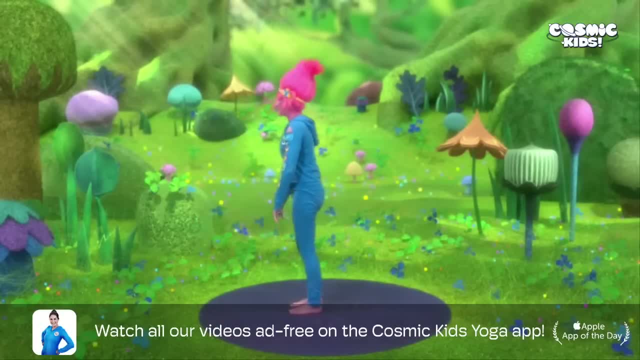 there, Walking your feet all the way forwards, rolling up to stand, and then Cloud Guy arrives. Coming into Cloud Guy pose, bringing your feet together And turning your toes out to make them a v-shape, Cupping your hands around your mouth and we're. 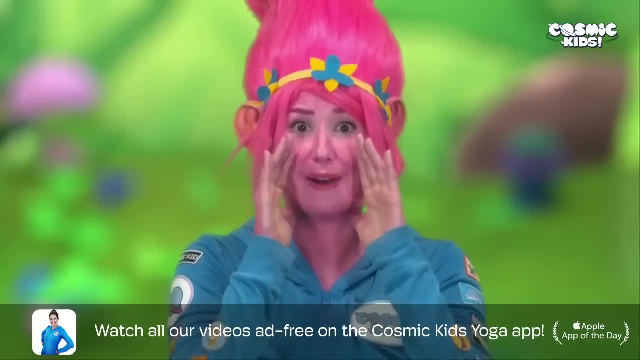 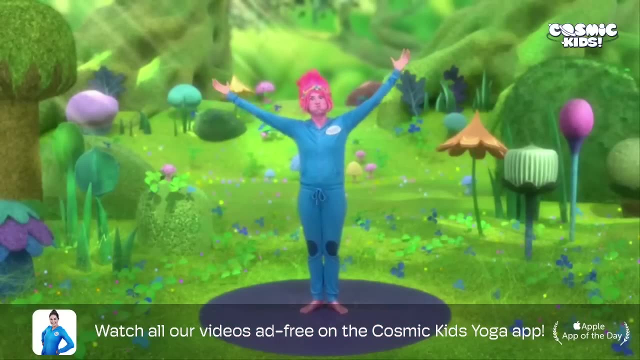 going to do a big blow, to blow up a big puffy, fluffy cloud. Here we go. Cloud Guy tells Poppy and Branch that one of the holes will lead to Burgantown, The other hole will lead to Saturn Death. And then he opens his arms wide and he invites little Branchy Wanchy in for 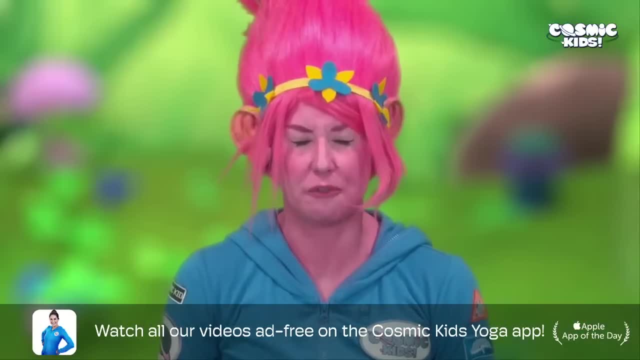 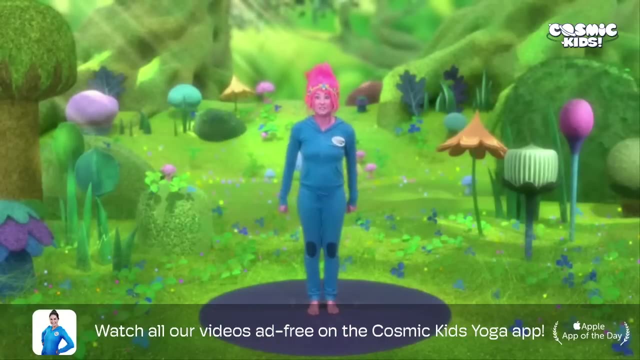 a hug. Wiggy Wuggy Branch has had enough of hugging and he chases after Cloud Guy Come back. He dives down one of the holes after him, reaching your arms all the way up and folding all the way forwards following Cloud Guy down the hole. Luckily it leads them to Burgantown, Rolling all. 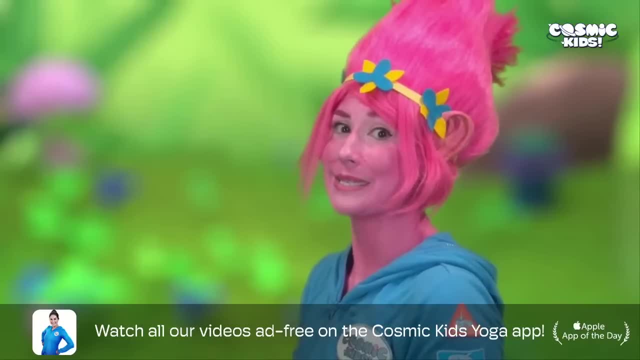 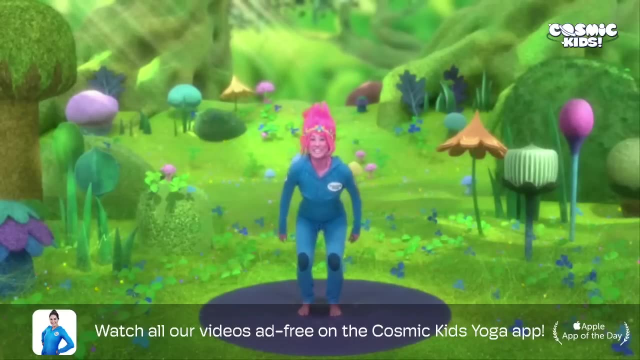 the way up to stand. Now sitting in the palace is the young Burgon King, King Gristle, Coming into throne pose Feet hip distance. Bend your knees, Sweep your arms up by your ears and sit yourself down like you're sitting on a throne. He's with his pet crocodile Barnabus, Coming into crocodile pose. 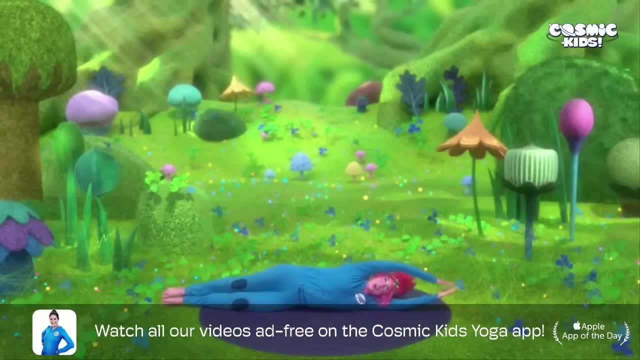 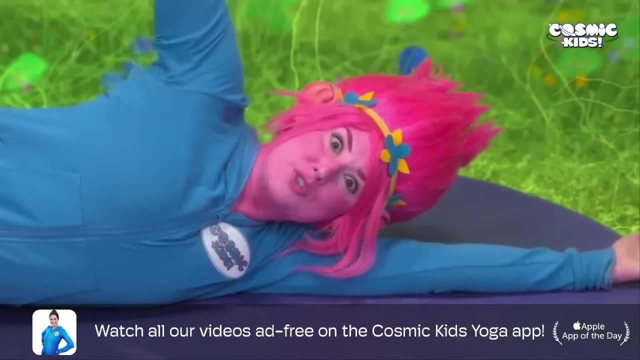 Lying on our sides, Arms long above our heads, And then opening and closing your jaws by lifting and lowering your arms. Very good, everyone In comes. Chef, looking very proud and pleased with herself Coming up to stand, She puts her hands on her hips. 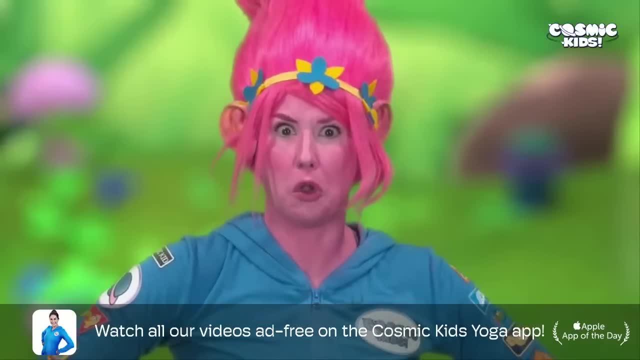 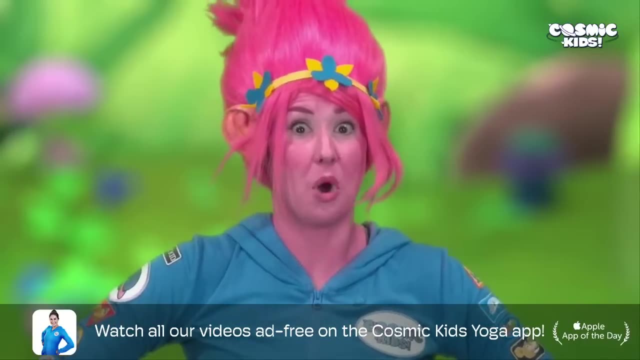 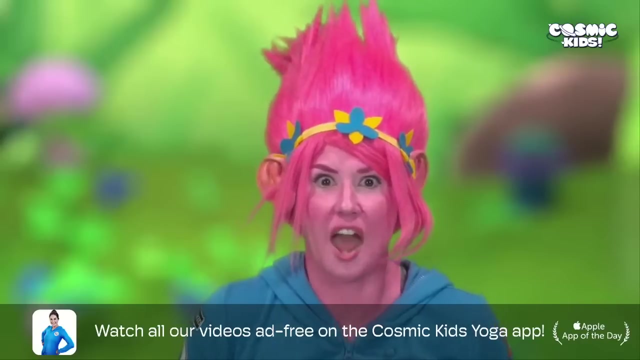 And she tells King Gristle that she has captured the trolls and it is time for Tralstice again. Just at that moment, Poppy and Branch tiptoe into the palace, Just in time to see Chef making a sandwich wrap out of their friend Creek, The yogi troll. Coming into sandwich pose Sitting on our bottoms, Legs out long. Chef rolls out the wrap. Let's abdomen, respondedI on a qualified assimilated action. Let's start the hanging. Chef rolls out the wrap. Let's wrap the hanging from the eatable cling film. and he's going to Med��. who's his sponsor? with his prestamate now. 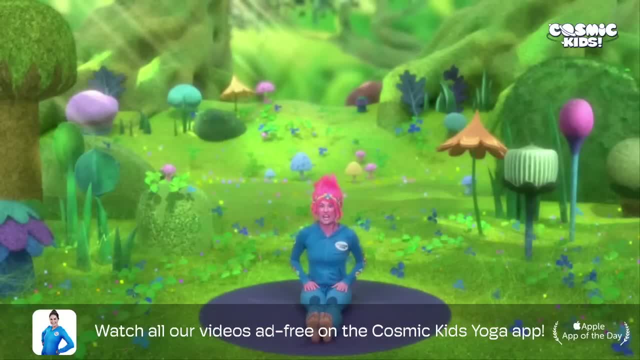 The game calls Life is a PRO. that's all it's got. And about TikTok and Iата For real. it's pouch time. Among other간ättut Kroovesy gonna be looking for the. let's rub our legs here we go. roll out the wrap. roll out the wrap. she takes her arms wide. she. 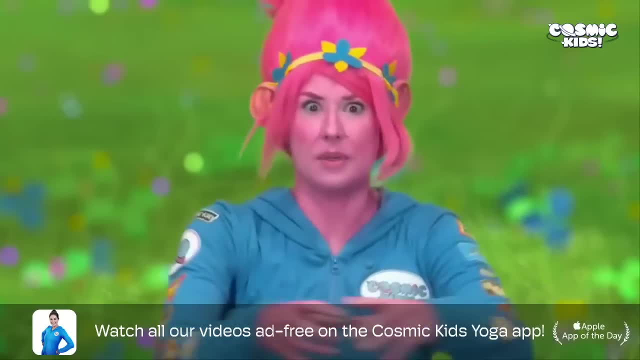 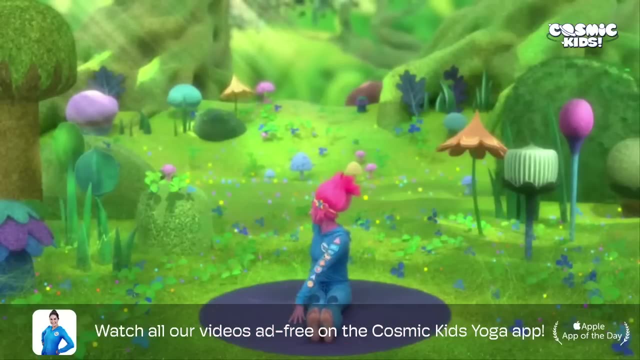 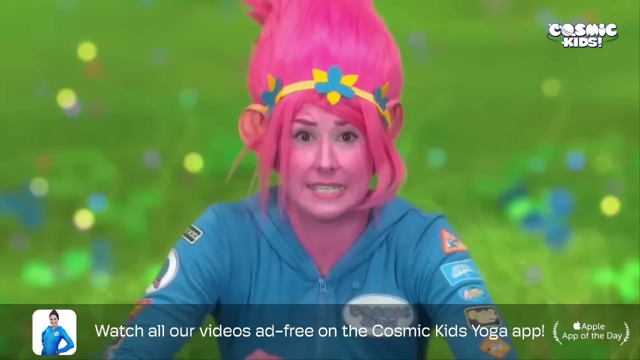 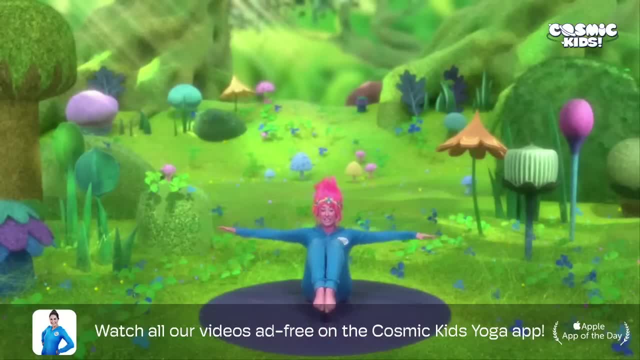 wide. now see if you can bring your knees all the way in lifting your feet, hugging them in. she shoves the whole lot into king gristle's mouth, but before he can swallow, she slams the door. coming into door, pose up onto two knees, leg to the side, arm to the sky, and let's slam it this way: slam. 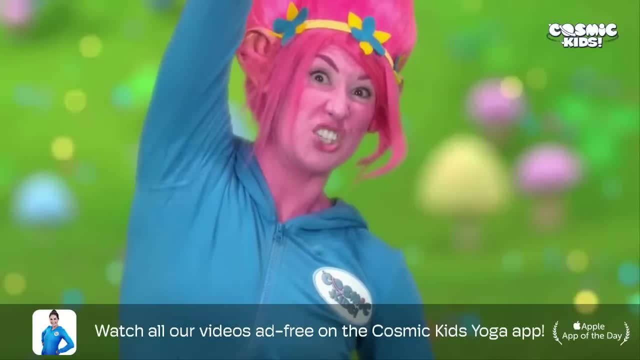 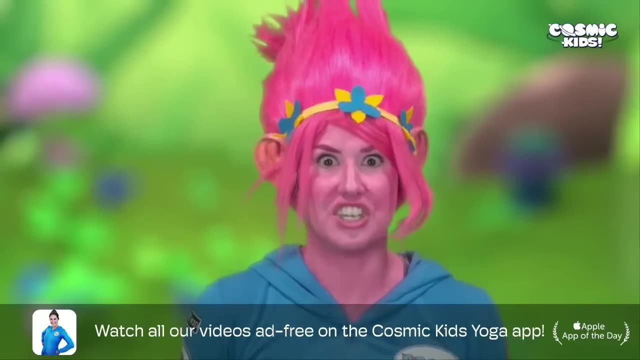 poppy feels. sure, creak must still be alive, but first she needs to save the others. coming up to stand, she and branch jump onto the apron strings of bridget, the bergen scullery maid, bringing your feet together, taking your hands up above your head, bringing your hands to touch. 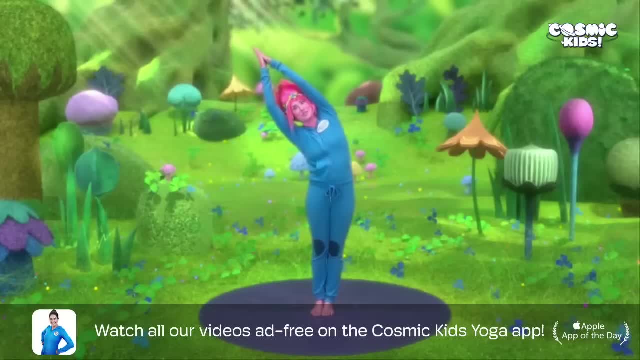 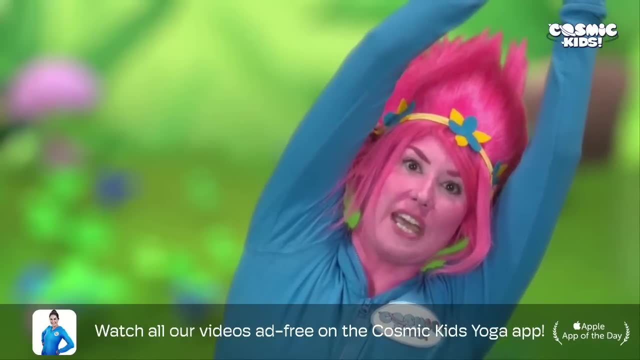 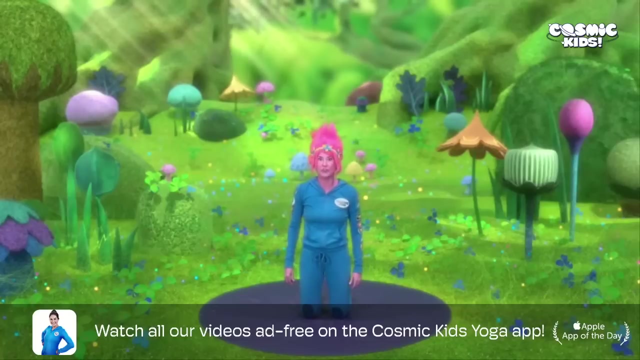 now lean over one way, holding on tight to those apron strings, and lean over the other way. oh, bridget's taking them into her room to guard the trolls, and when she gets there she comes to her knees and she sings a song about her secret love. of king gristle, bringing your hands up. 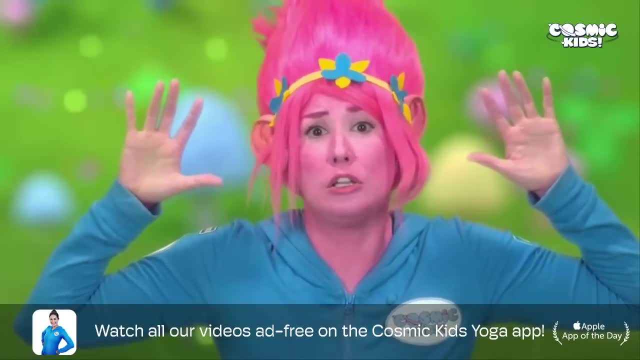 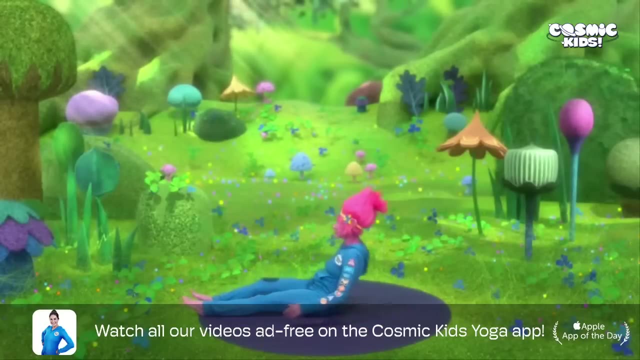 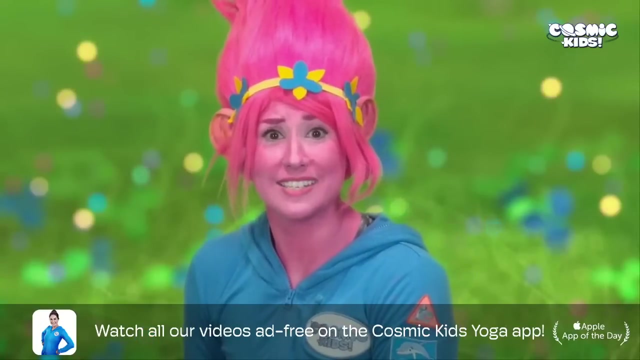 she says, hi, hi, hello, is it me you're looking for? and she lies down on her bed, feeling sad, arms down, legs down, crying and sleeping, opening your eyes, coming up to sit. oh, this is so sweet. poppy thinks bridget's in love with king gristle. oh, that's the loveliest thing. 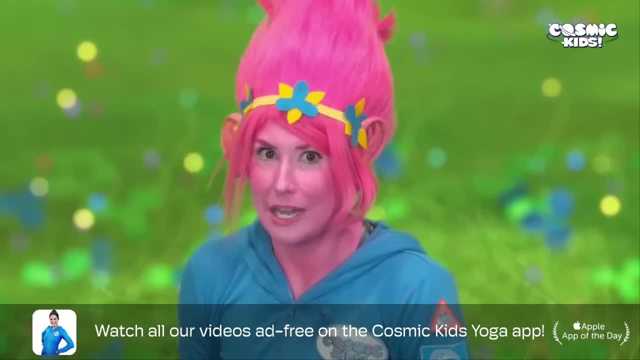 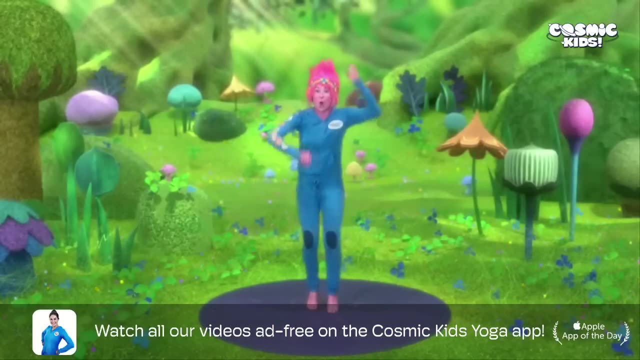 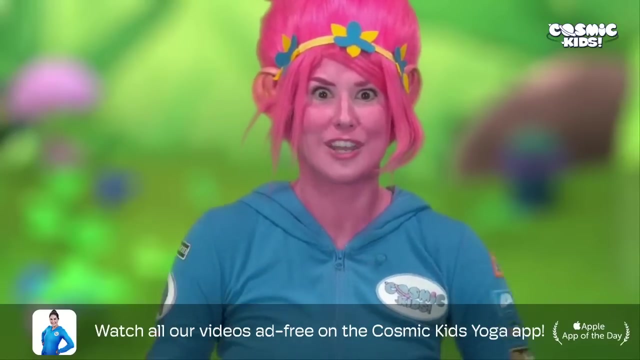 needs to save her friends. so she and Branch climb silently up to where they're kept in the cage, Coming up to stand. let's climb silently Up, we go up, we go up, we up, we, up, we go. When they get to the top, the trolls are so happy to see Poppy and Branch. 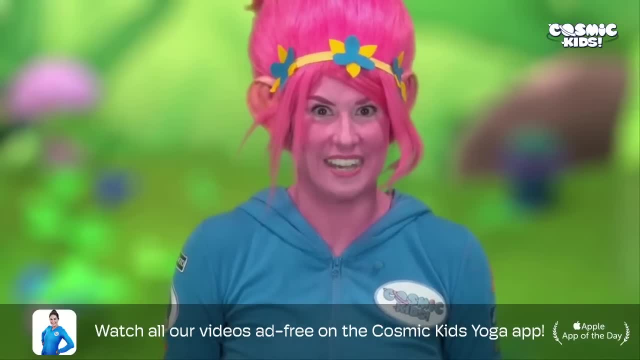 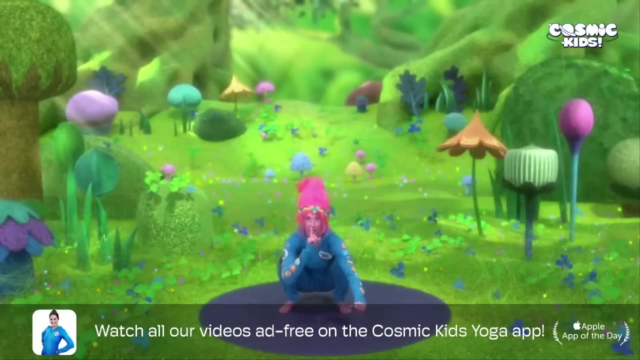 They do a happy dance and they sing about having a party again. Celebrate good times, come on. But we need to be quiet. so we crouch down and we shhh: Now they're free from the cage, it's time to save Creek. 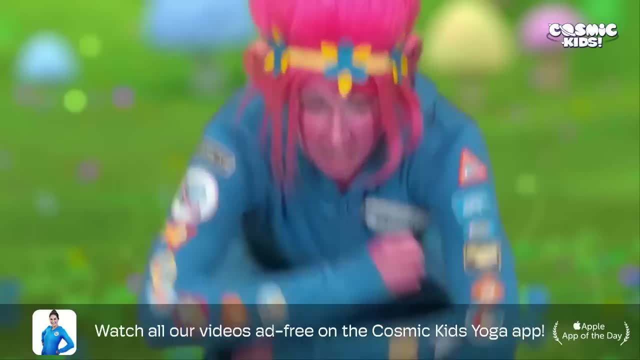 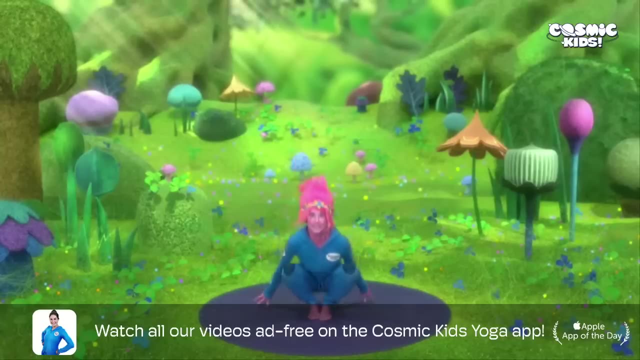 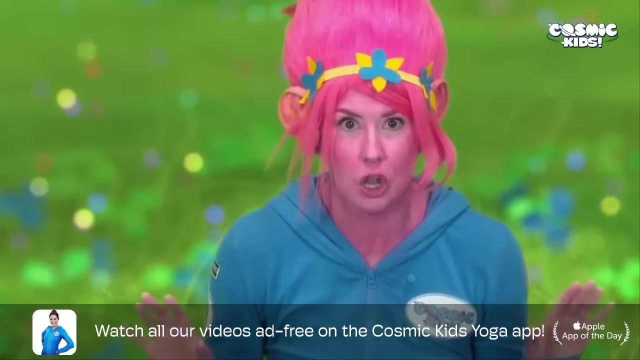 But just as they're escaping, Bridget jumps up in star pose. Stop, Poppy needs to make a deal with Bridget and so sits calmly with her legs crossed. She suggests to Bridget that she and the trolls will turn her into a total babe so that she can get a date with the king. 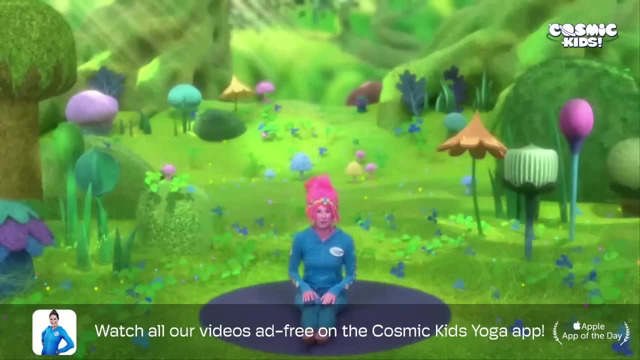 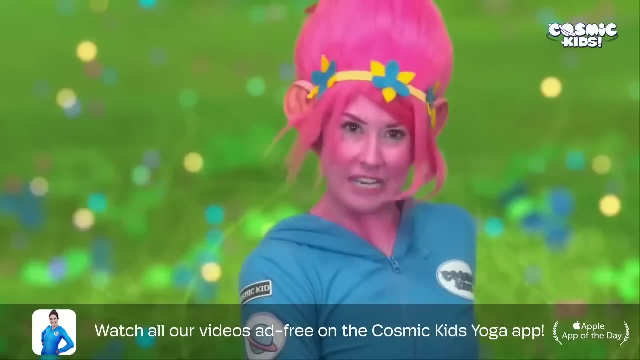 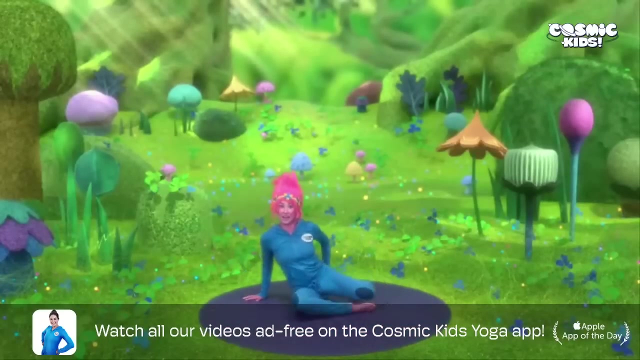 Coming into total babe pose, taking your legs out long, sweeping them round one way, putting your hand on your knee, your other hand behind you, looking over your shoulder back to the front and going ooh la, la, Then let's do it on the other side, sweeping your legs round the other way, hand on your knee, hand behind you. 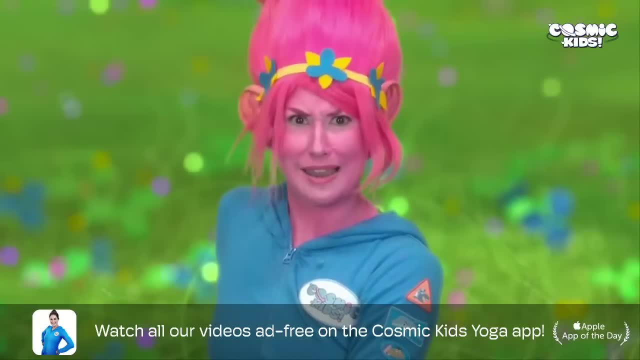 looking over your shoulder, looking back to the front and ooh la la. In return, they ask Bridget to help them get Creek the yogi troll back. After some time Bridget is back in the cage. She asks Bridget to help them get Creek the yogi troll back. 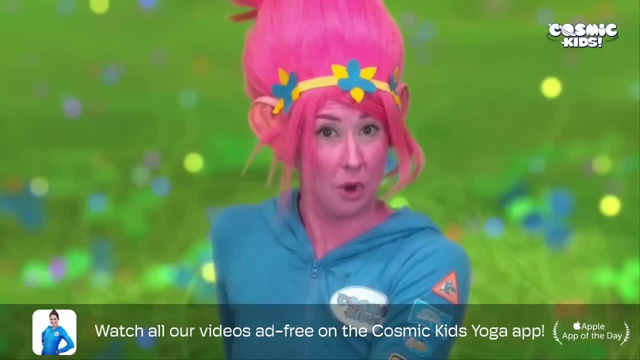 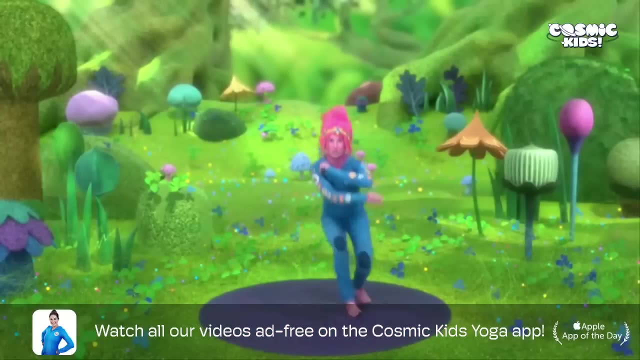 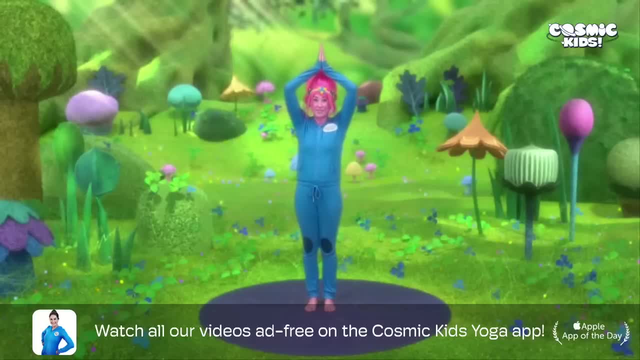 Then they jump on her head, bringing your hands above your head, palms to touch, Stretch your arms up high, like your hair's growing very long, and they're opening it wide, Making that big, beautiful wiggle, beautiful rainbow coloured hair. From here the trolls can give Bridget the word she needs. 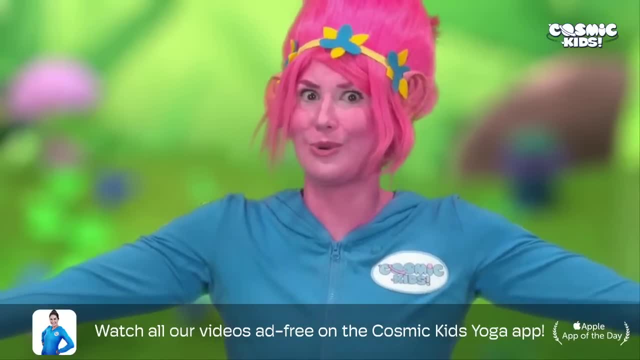 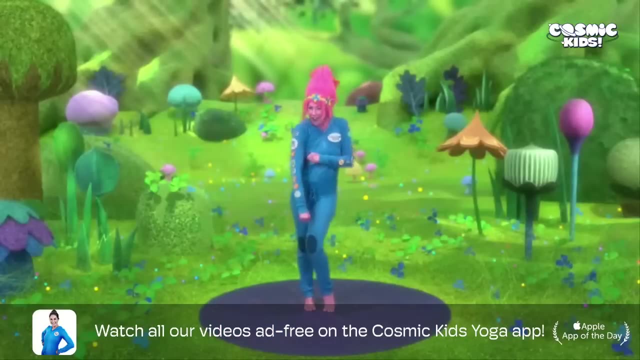 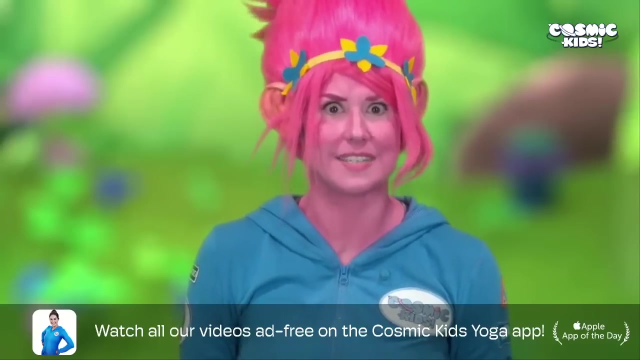 because they're standing on her head, just in case she gets stuck. when she's talking to King Gristle, Bridget steps out feeling rather awesome and confident I'm coming out. I want the world to know. Got to let it show When King Gristle sees Lady Glitter. 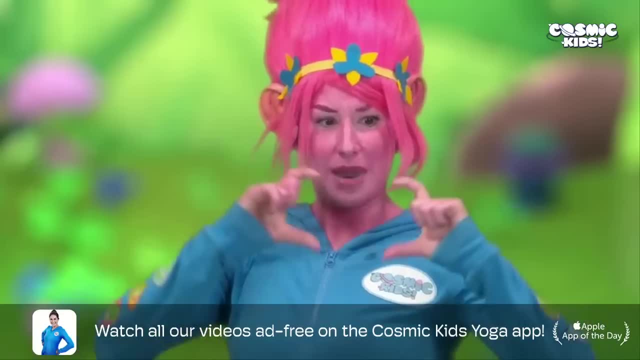 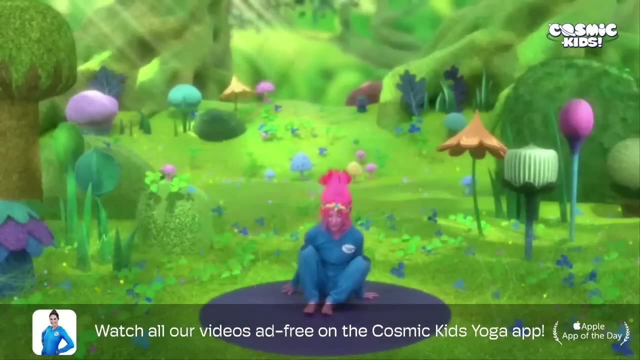 Sparkles. he is in love Seeing if you can make a heart shape with your fingers. Oh, yes, Together they go and eat some pizza. Sitting on our bottoms, crossing our legs, we rub a hand on our tummies and we pat our heads at the same time. Isn't this amazing? They. 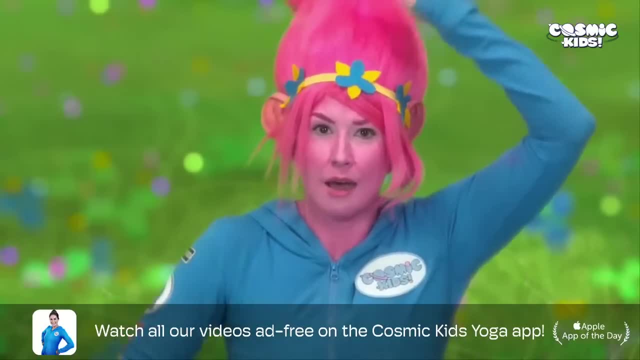 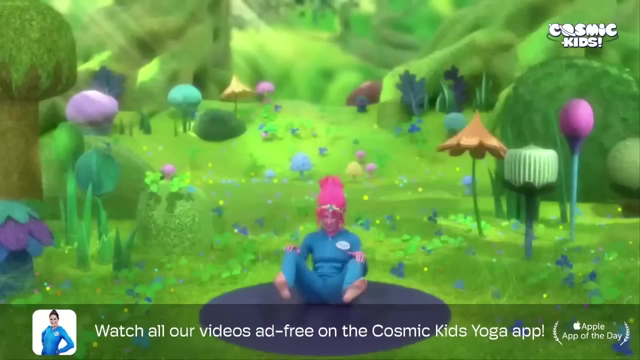 are happy without eating trolls. King Gristle decides to show Lady Glitter Sparkles his gem locket. Coming into our gem locket, pose soles of your feet together, holding onto your feet now, folding your head all the way forwards. We're going to lift up our head. 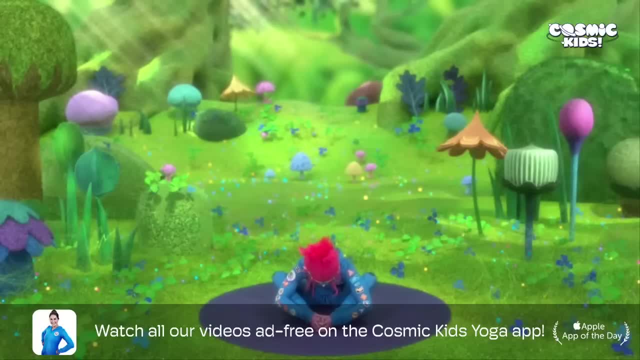 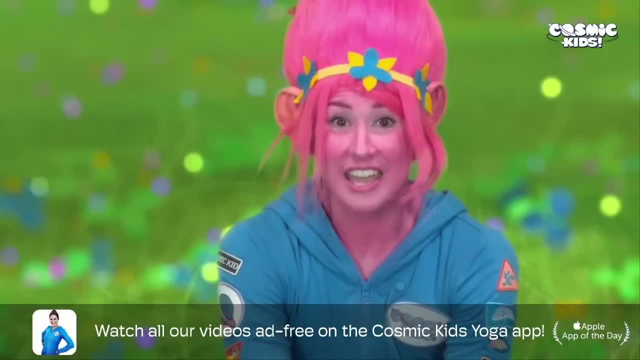 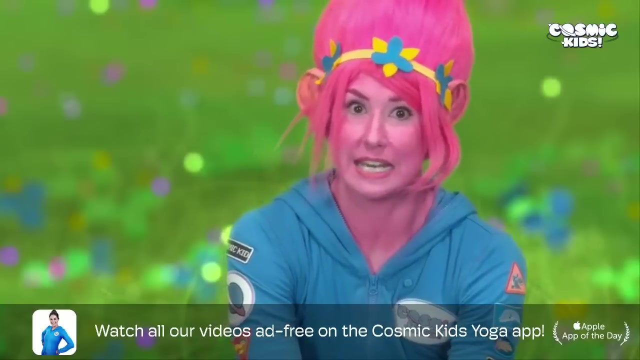 after three to open your eyes. Open it up. One, two, three, Whoop. Inside is Creak the yogi troll. He's alive. Even Mr Dinkles said something. Oh, snap King. Gristle asks Lady Glitter Sparkles whether she will. 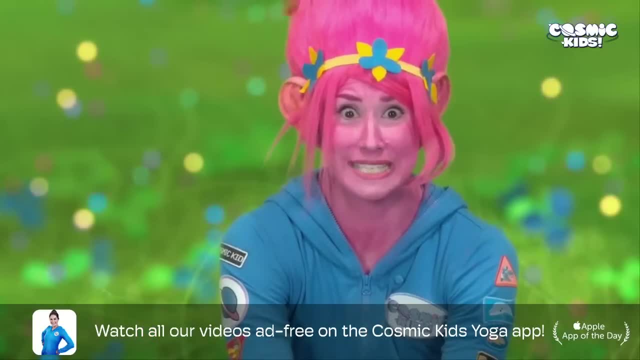 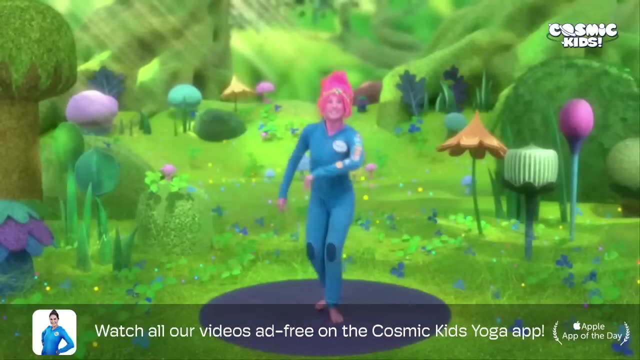 be his plus one for Trollstice. and she says, yes, Now they go roller skating. Coming into roller skating, pose Up to stand, everyone Turning to the side. Now we're going to lift up one of our legs and take our arms wide to take our leg back. 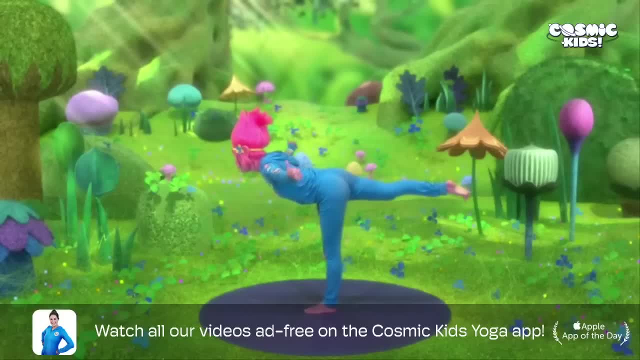 behind us in our roller skating pose. Woohoo, Coming up to stand. Should we try that? the other side, Yes, I think we should. Standing, nice and tall, lifting up one of your legs Now, arms wide, Take it all the way back behind you, nice and strong, We're roller skating. Coming up to stand. They're having such a wonderful time. And then Chef arrives. Look where are you from我们从文字机去大混入中国后 veio 富翘出海。 Da Nang students, thank you very much. 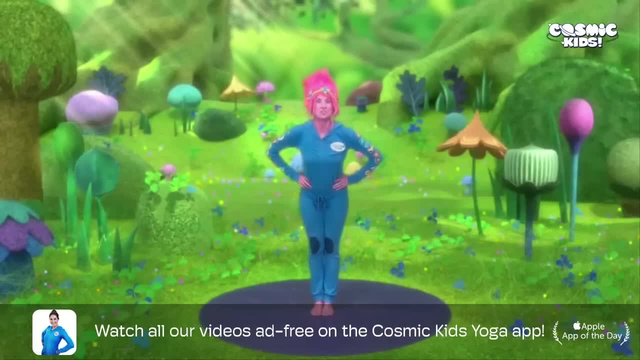 She has her hands on her hips and she folds halfway forwards to get a closer look at Lady Glitter Sparkles. She recognises that it's Bridget and Bridget knows she needs to get out of there. Coming up to stand, putting one foot forward, one foot back, bend your knee, arms wide. 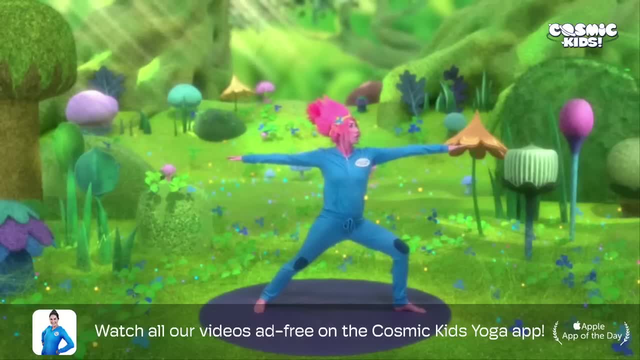 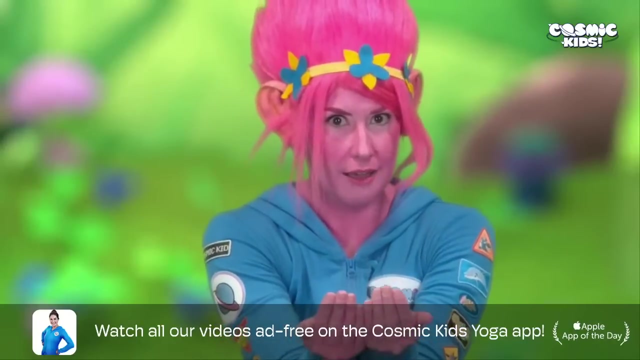 She skates as fast as she can, But she leaves a roller skate behind. Coming to stand, King Gristle is delighted. Folding all the way forwards, he scoops up the precious roller skate. Will she be his Cinderella and come to Trolstice? 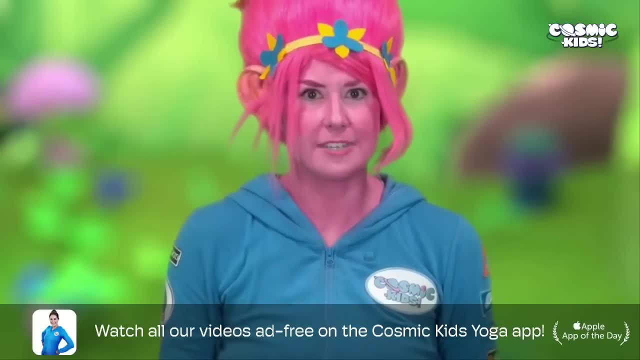 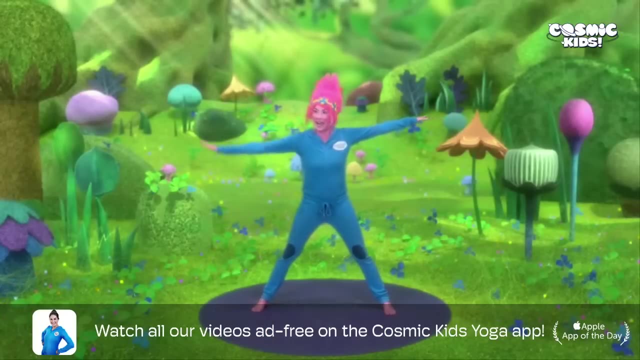 He hopes so. He decides he needs to get fit, and so he starts exercising. Jump your feet wide, take your arms wide. Let's do some windmill pose. Take your hand across to your opposite foot and reach your top arm up to the sky. 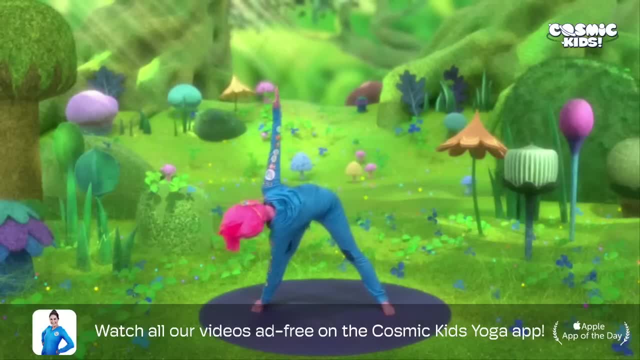 Now let's switch sides. Take the other hand across And your other arm to the sky. Now let's see if we can do eight switching sides. Here we go, And one and two, and three and four, and five and six and seven and eight. 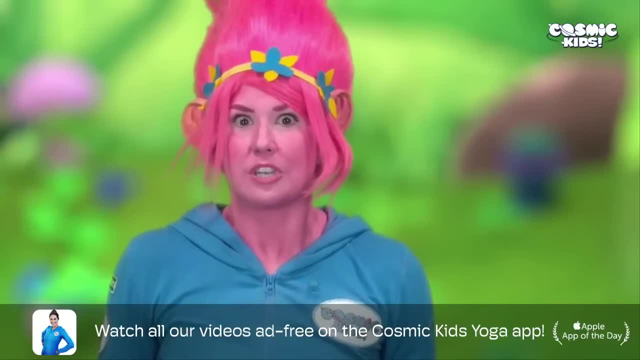 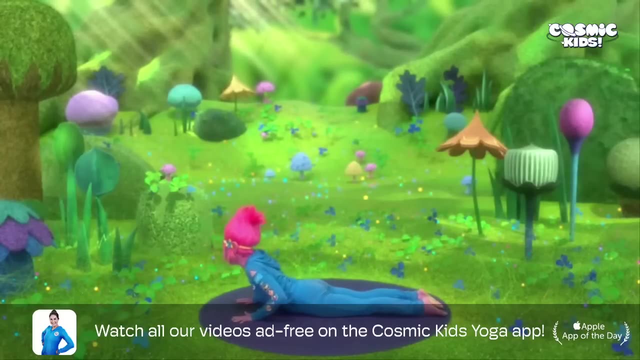 Rolling up to stand. This is their moment. The trolls wiggle in under the rug, Coming onto your tummies. everyone Hands underneath your shoulders and let's wiggle, wiggle, wiggle, wiggle under the rug. They're looking for the gem locket with Creek inside. 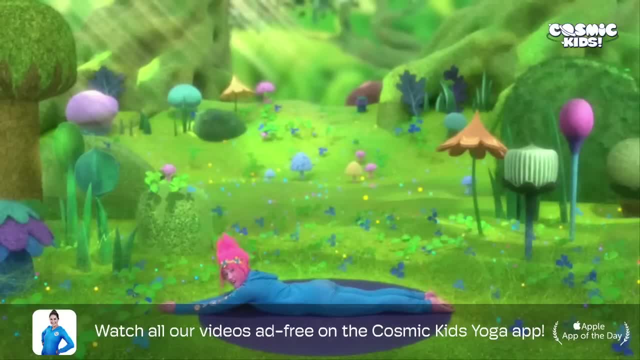 There it is, Lying all the way down, reaching forward with your arms to grab it. They've got it, But just as they do, Barnabus the crocodile sees them Rolling onto your side and opening and closing your crocodile jaw. 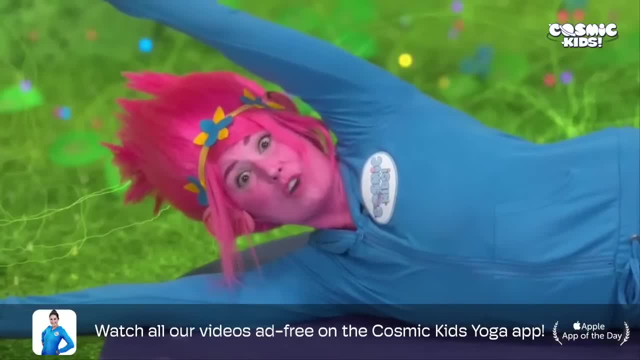 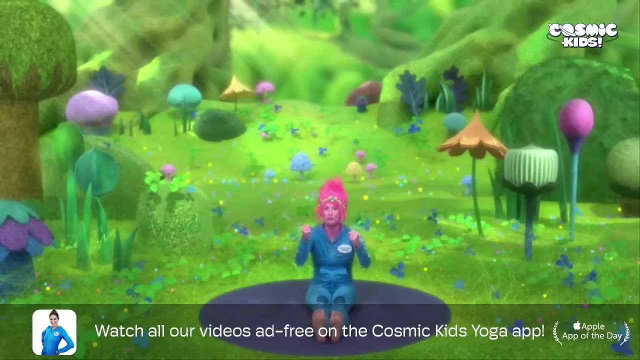 Oh no, he's chasing them. The trolls jump on the roller skate sitting up legs out long, and they drive it out of there Holding onto the laces. they go forwards really fast, Then they sit up really tall. 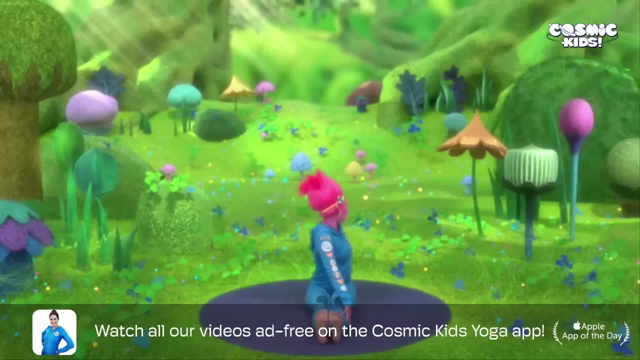 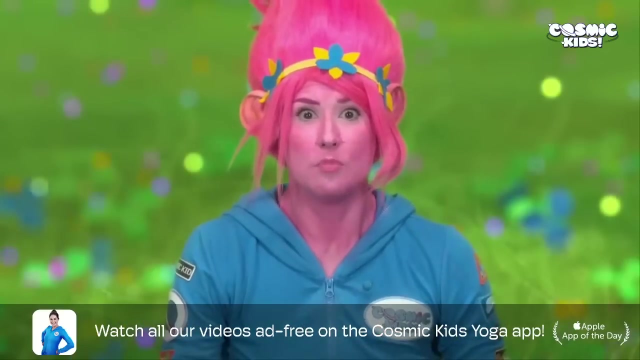 And Guy Diamond, the wonderful glitter troll, twists to the side and he blows Barnabus with his glitter And the other side, turning to the other side, blows some more glitter. They think they've got away, But then the locket flies up into the air. 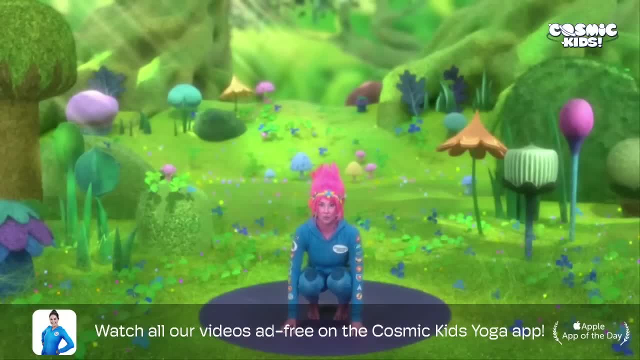 Coming up onto our tiptoes everyone. After three, let's jump in the air like with a locket. One, two, three, It pops open, sitting on our bottoms, soles of the feet together, bringing your head all the way forwards. after three, lifting it up. 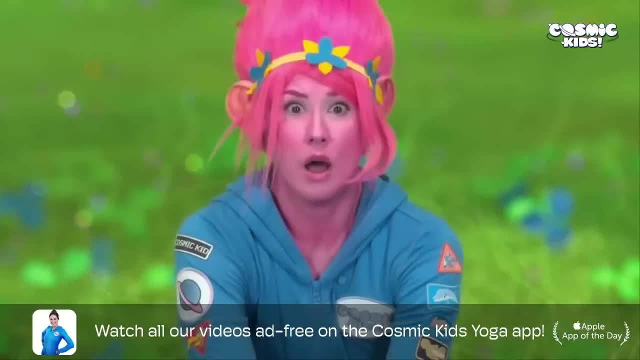 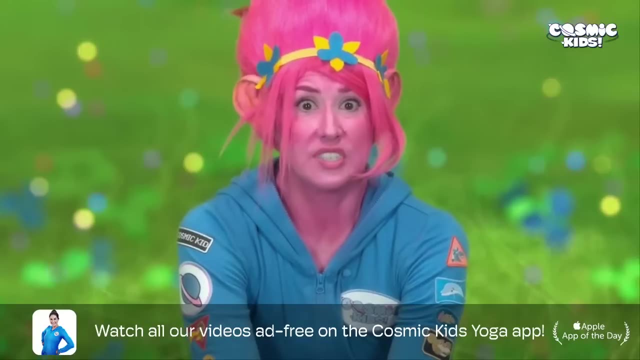 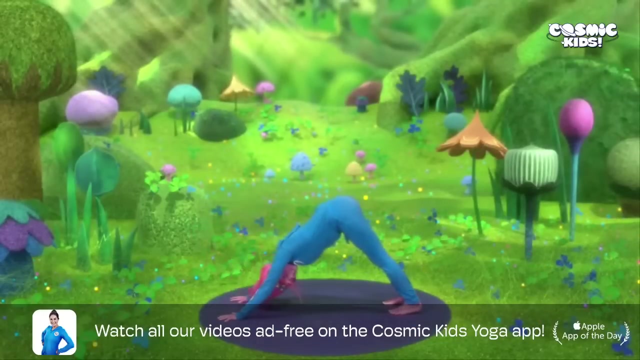 One, two, three, But Creek isn't there. He's disappeared. Just at that moment, Chef arrives and she puts down a cage on top of them all, Coming onto our hands and our knees, tucking our toes and lifting our bottoms to the sky. 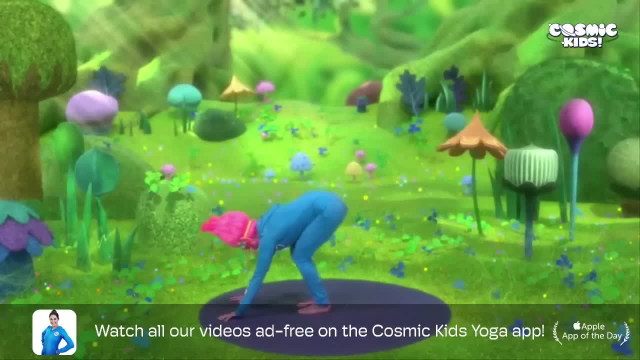 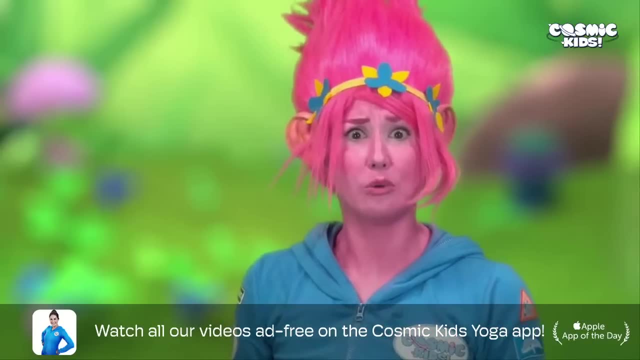 But who's this? It's Peering, Walking your feet all the way forwards, rolling up to stand It's Creek, the yogi troll. He's sold them out. He's agreed that he will ring Poppy's cowbell three times and lead Chef to where all the other trolls are hiding. 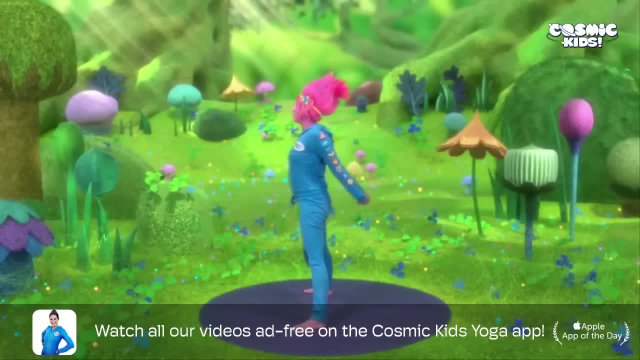 Take your feet wide, crisscross your fingers behind your back, stretch your arms out. Now, after three, let's fold forward and ring Poppy's cowbell. One, two, three Ding And up. One, two, three. 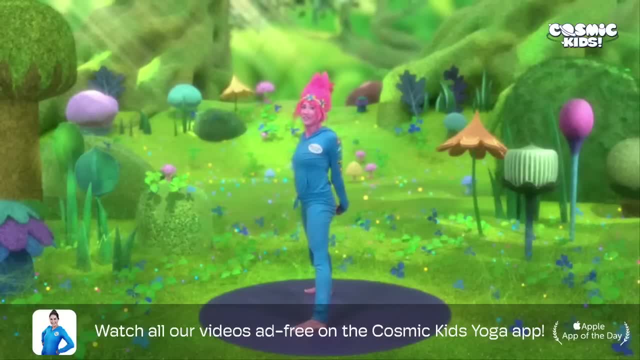 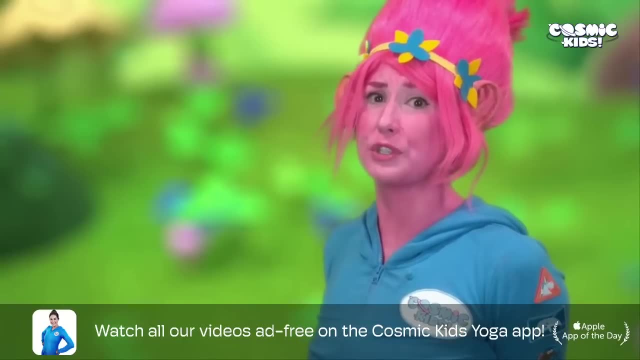 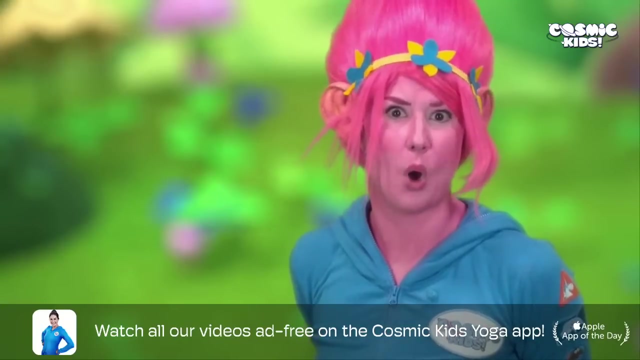 Ding And up. Last time. One, two, three Ding And up. This is so. there'll be enough trolls for Trollstice. Come the day of Trollstice, Chef puts all the trolls into one ginormous pot. Coming into pot pose lying on our tummies. everyone, bring your feet towards your bottom. 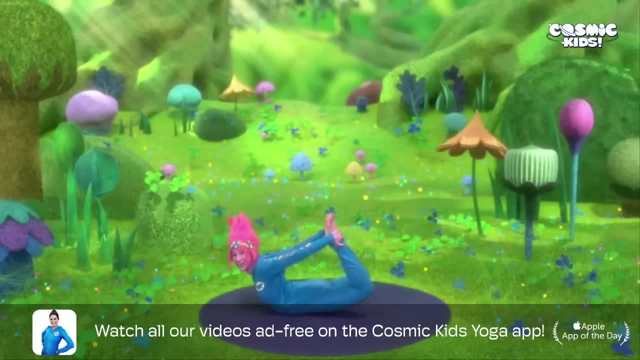 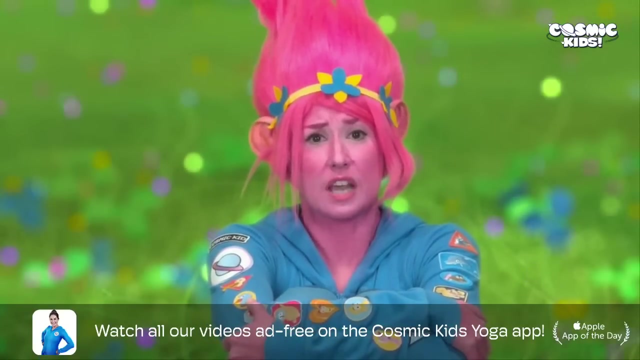 Reach round to grab your ankles and kick your feet into your hands, lifting yourself up into your pot. pose Poppy's feeling sad, Sitting up. she hugs her knees. She feels like she's let everyone down. She feels like she's let everyone down and all of the positivity and hope leaves her. 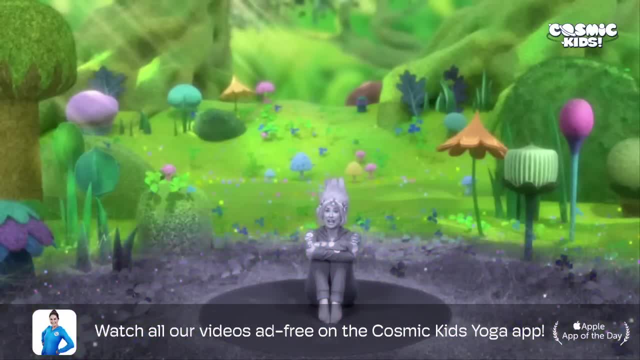 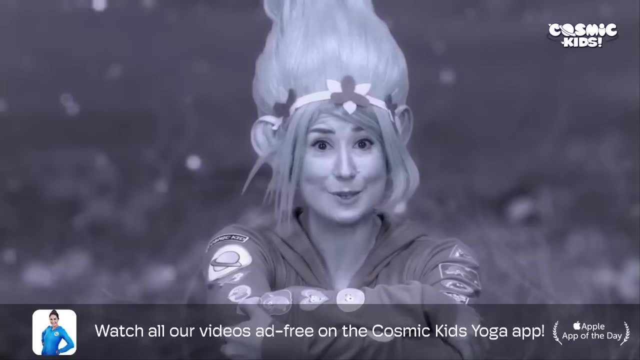 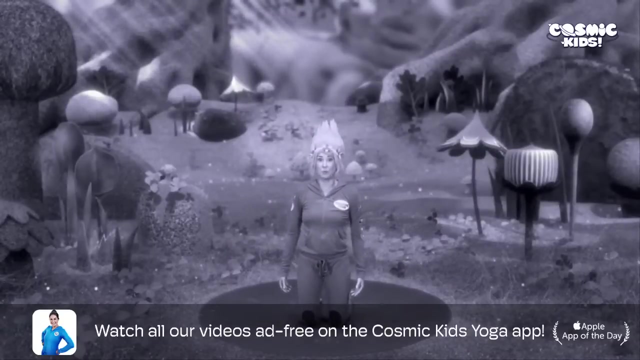 Her colour drains away and she is left grey. It then drains away from all the other trolls. Then, for the first time since losing his grandma, Branch comes forwards, Coming up onto our knees, everyone. He sings to Poppy. He tells her that he thinks her true colours are beautiful, like a rainbow. 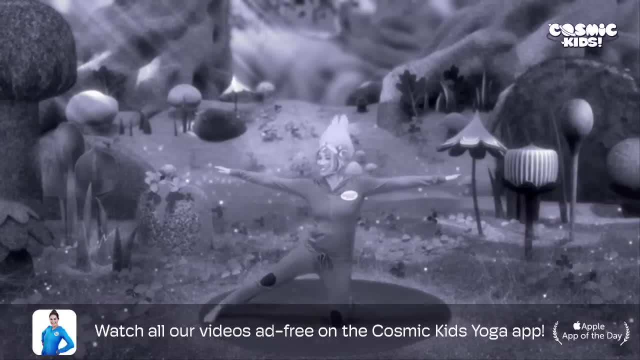 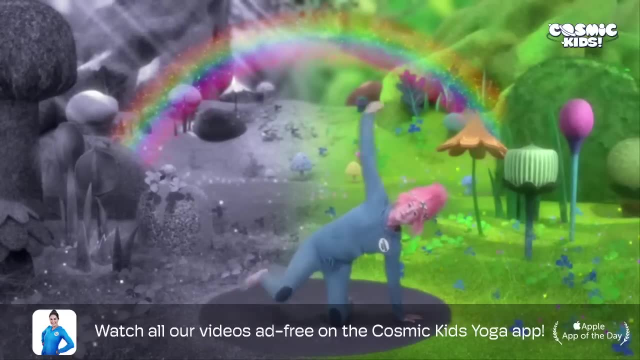 Let's do our rainbow. pose: Arms wide, leg to the side, drop down onto one hand and sweep your arm up and over your ear, making your big, beautiful rainbow Coming to two knees again. arms wide leg to the side, drop down onto one side and 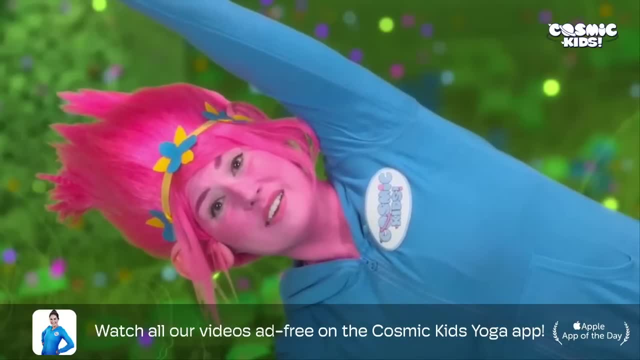 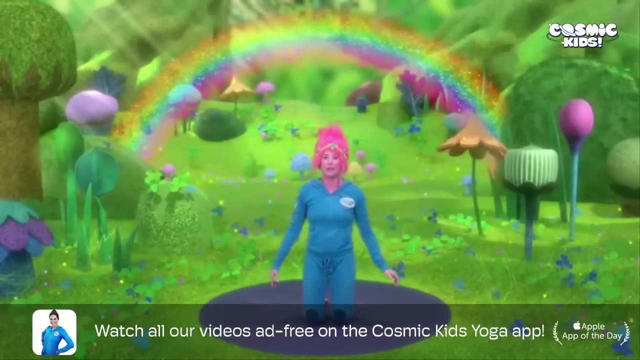 sweep your rainbow up the other way. He sings to Poppy And that's why I love you. Poppy comes up hearing this, hearing this Hope again brings hope flooding back to her And she and Branch open their arms wide and share a big, wonderful hug. 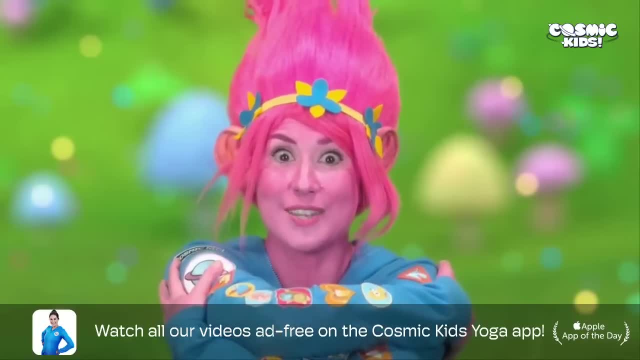 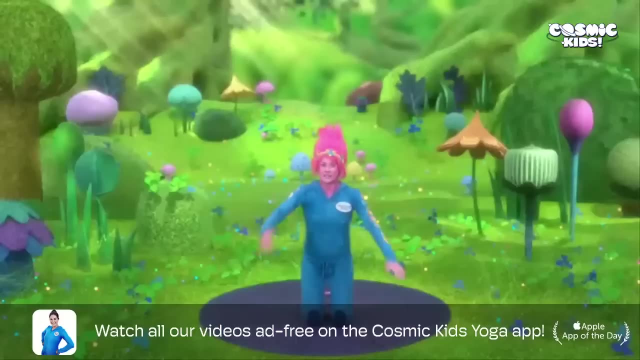 All of the colour comes back to the rest of the trolls and to Branch, who isn't grey but is blue. Now the lid of the pot gets opened. sitting on your bottoms, legs out, long, bending our knees, touching our toes, After three let's lift our arms up to open the pot. 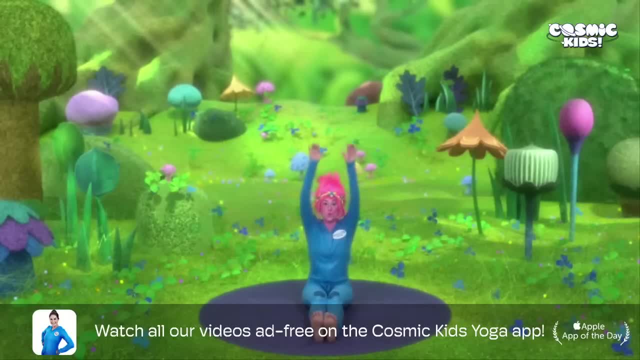 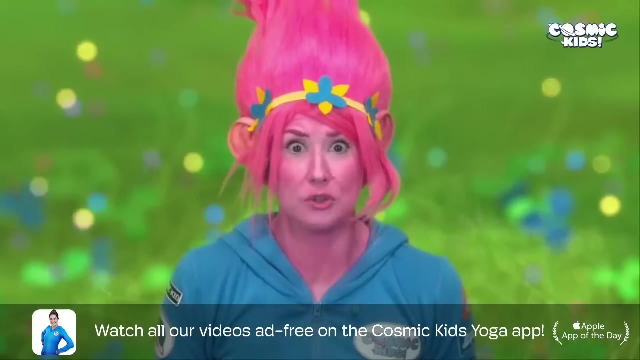 One, two, three. It's Bridget. She's letting them all escape. She wants to thank Poppy for helping her find true happiness. But now Bridget is in some serious trouble for letting the trolls escape, Coming up to stand one foot forward. 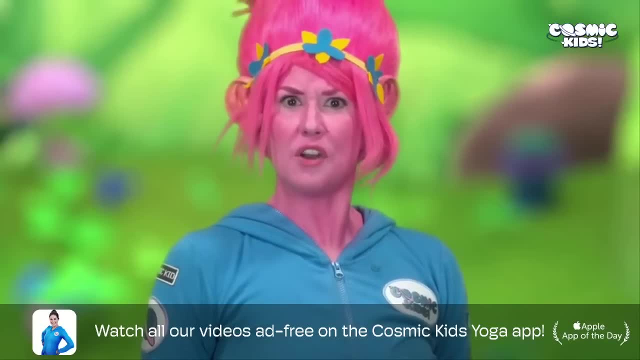 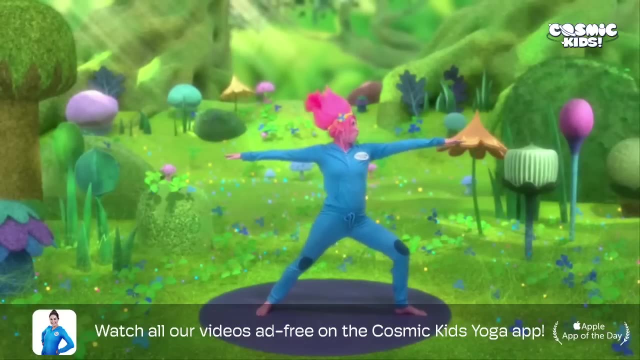 one foot back. Poppy's not going to leave Bridget, nor are the other trolls, And they whoosh in on the roller skate to save her. Sweep your arms up, bend your knee and let's whoosh, Whoosh- They jump back on Bridget's head, turning her back into Lady Glitter Sparkles. 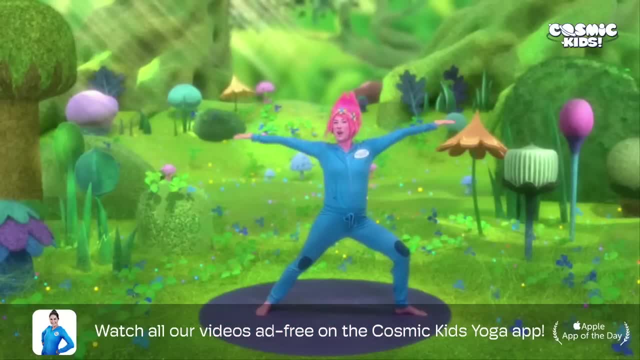 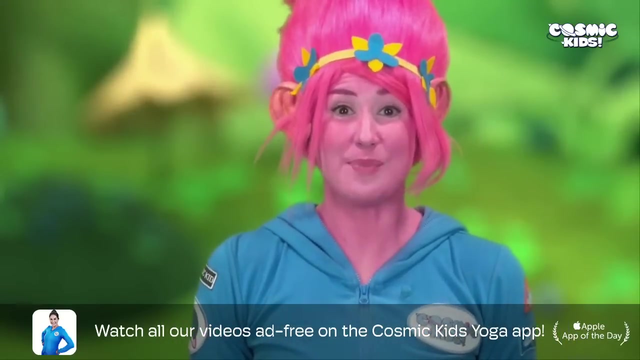 Hands together above your head, sweep your arms up and open them wide. King Gristle is delighted and stands in star pose to protect his Lady. Glitter Sparkles Poppy steps forwards, She reveals herself and she explains: you don't need to eat trolls to find happiness. 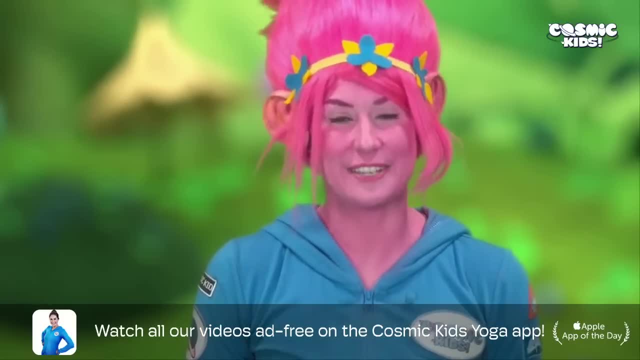 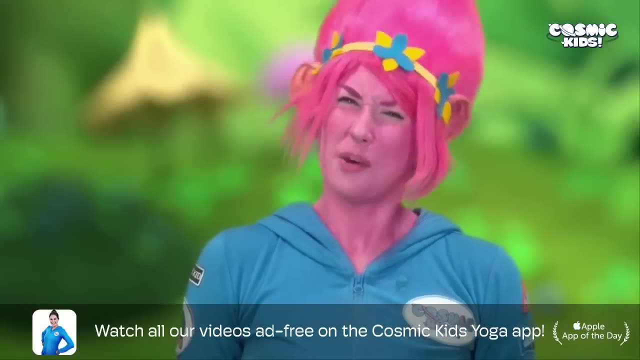 It's in each and every one of us. We just need to find it. Look at King Gristle and Bridget: They had a lovely time and they didn't eat any trolls. The Bergens start to realise that this is true. 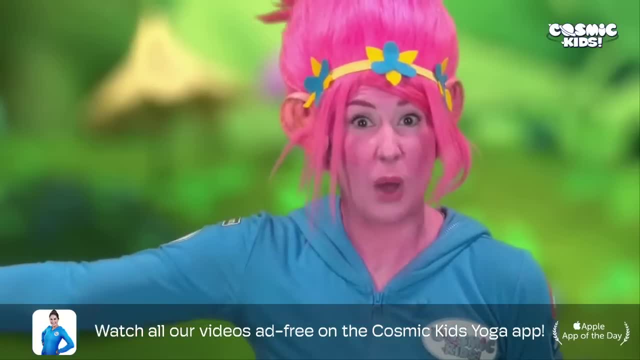 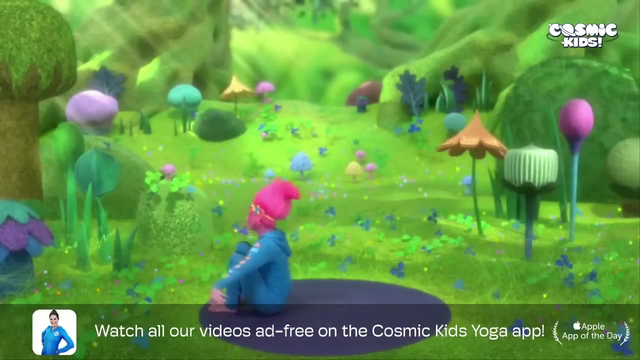 And they banish the chef once again, sending her out of the palace, rolling down the hill in a burning hot tub, And she says: you know what, I'm going to give you a hot pot? Coming into our roly poly burning hot pot pose, sitting on our bottoms, hugging our knees. 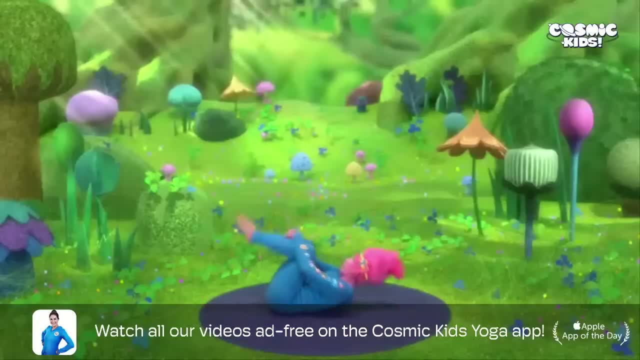 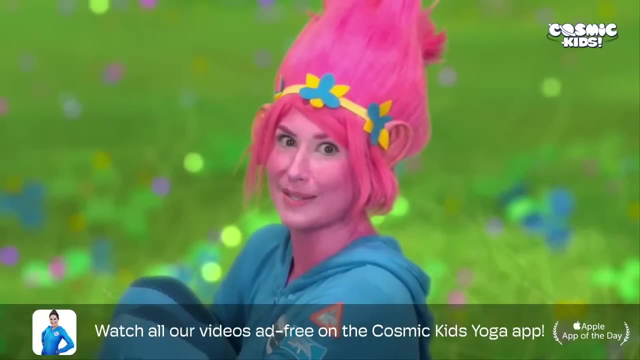 Now we're going to tuck our chin and rock all the way back and all the way up After three: One, two, three, Whoop Wee. One, two, three, Whoop Wee. Now, this last time, can we rock all the way up to stand? 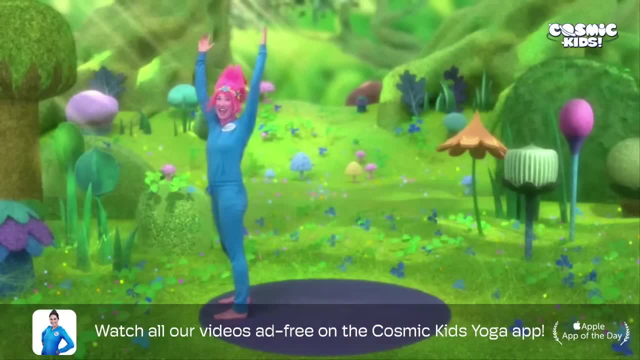 Let's try Ready: One, two, three, Whoop, Kick your legs And up we go. Yay, From that day on, Bergentown blooms again, bringing your hands together, Grow your arms up nice and tall and open. 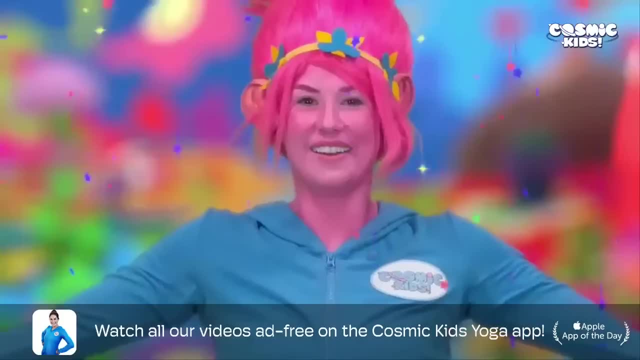 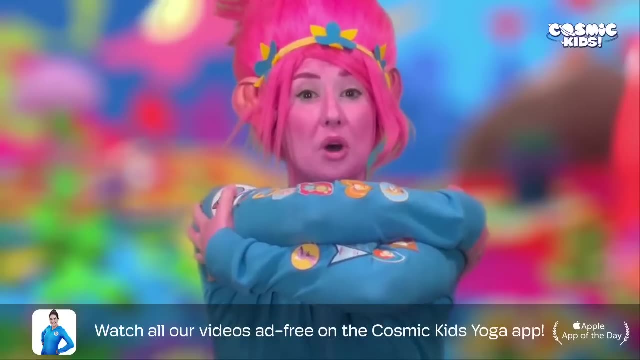 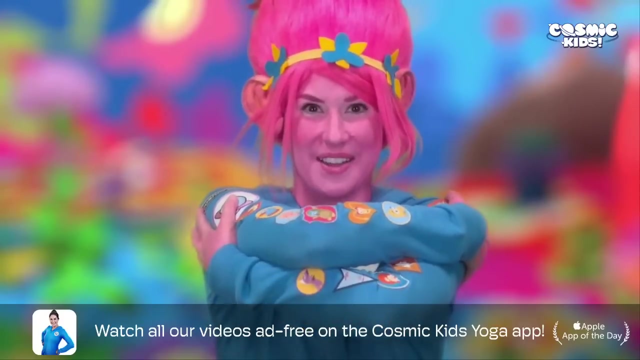 your arms spreading beautiful rainbow colours all over Branch and Poppy share a big hug, arms wide, Wrap yourself up in that wonderful hug. And Poppy is now the queen. She makes a new law: that hug time is all the time. 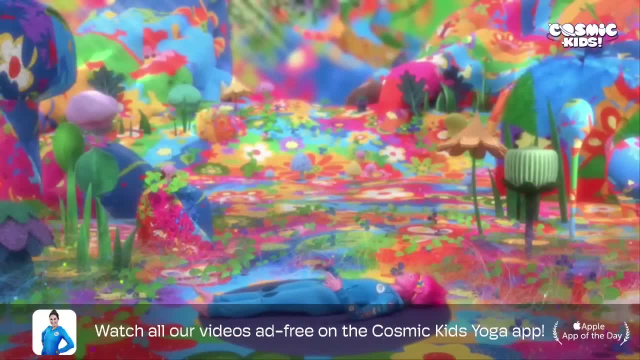 Coming down to lie in our relaxation, pose our legs long and our arms down by our sides. We close our eyes and let ourselves relax here for a few moments, Enjoying this peace and this calm, Letting all of the glitter and the sparkle settle in our hearts. 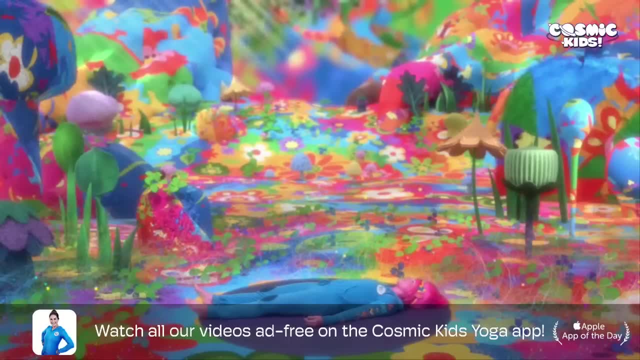 So often we look for happiness outside of ourselves, To things that we own, things, that we buy, stuff, When actually real happiness lives inside each and every one of us. We just have to find it And the time that we share with loved ones, with friends and families. 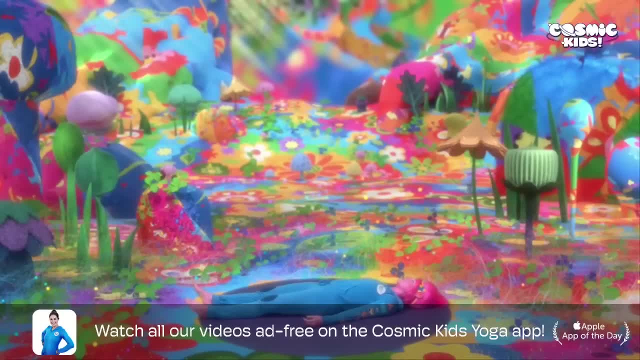 we can double, triple and maybe even quadruple our happiness by sharing just that special time with them, And the happiness we feel from a hug is so special and so strong. Look for the happiness in the little things in life, And that means life will be full of glitter, showers and rainbows. 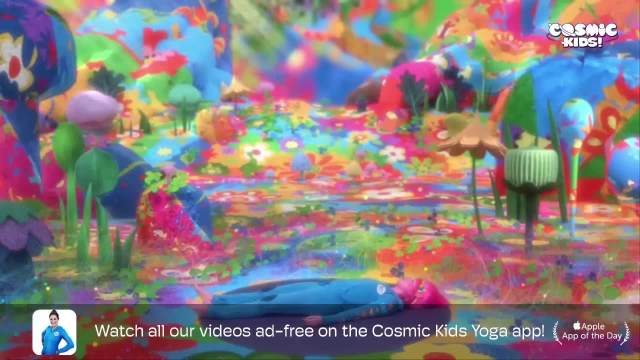 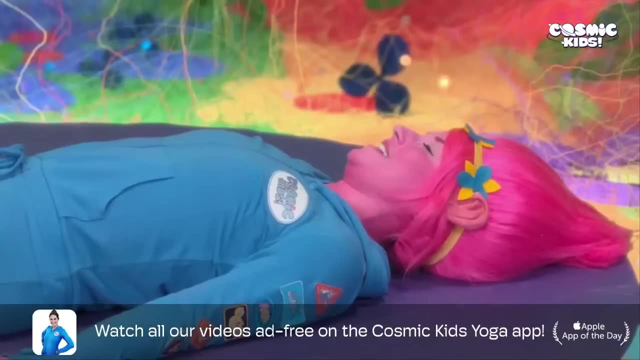 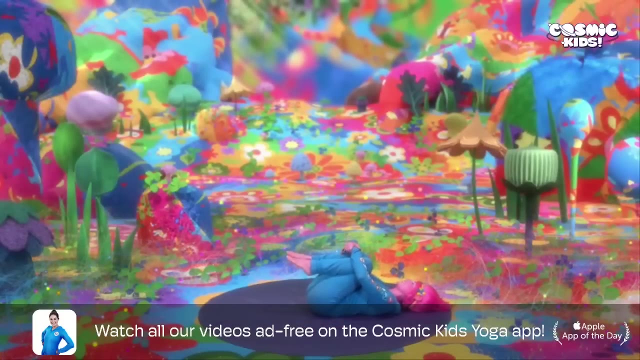 just as it is for the trolls. And now it's time to wake up. We wiggle our fingers and our toes, We bring our knees into our chests and give them a nice hug. We roll onto our sides, pushing ourselves up to sit. 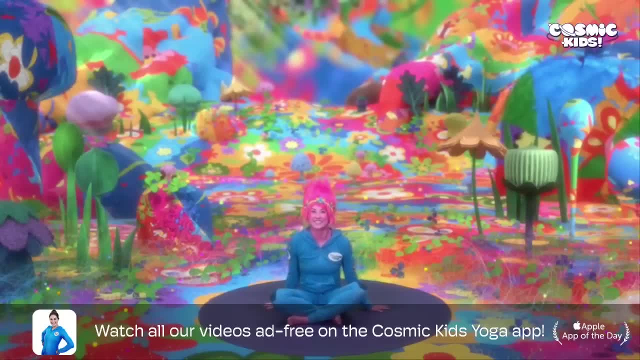 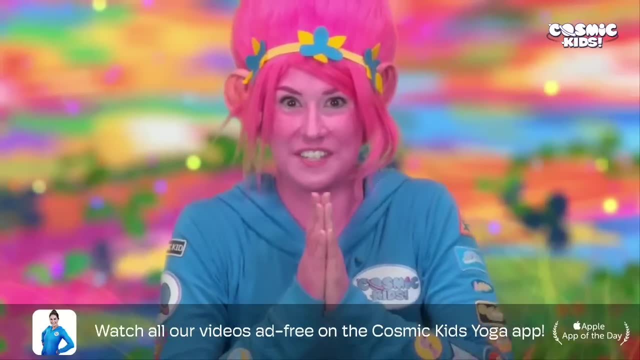 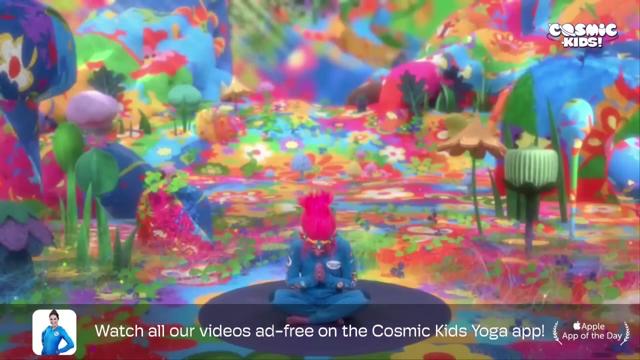 opening our eyes and crossing our legs. We finish just the way we started: with a namaste. So we bring our hands together at our hearts And after three, let's say it together: One, two, three, Namaste, Wow, well done everyone. 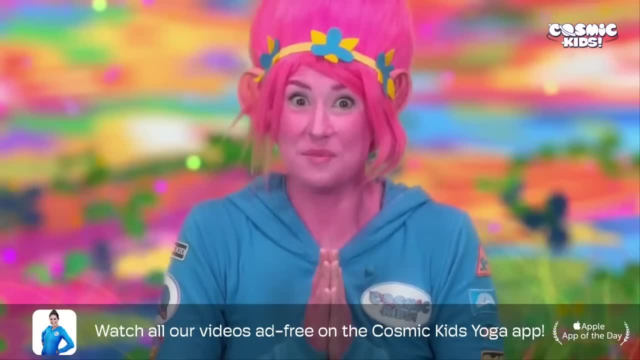 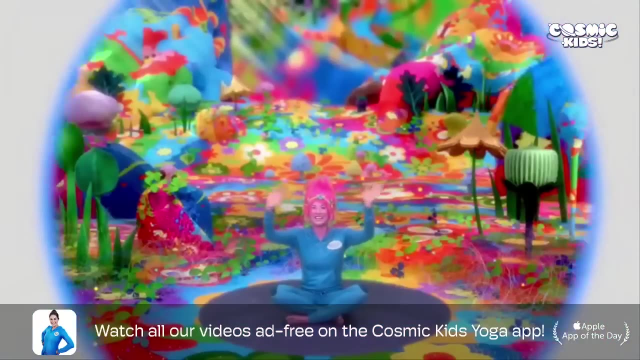 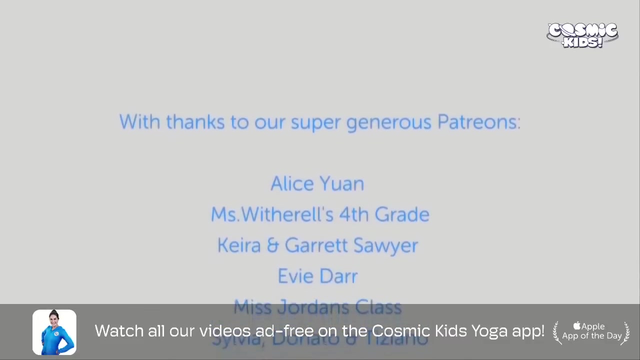 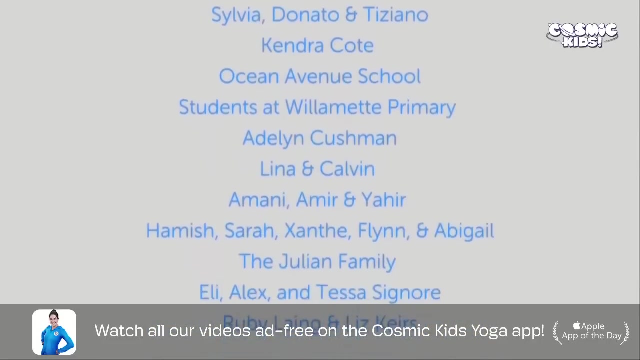 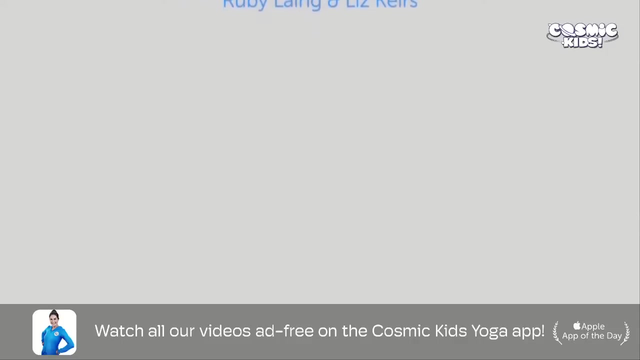 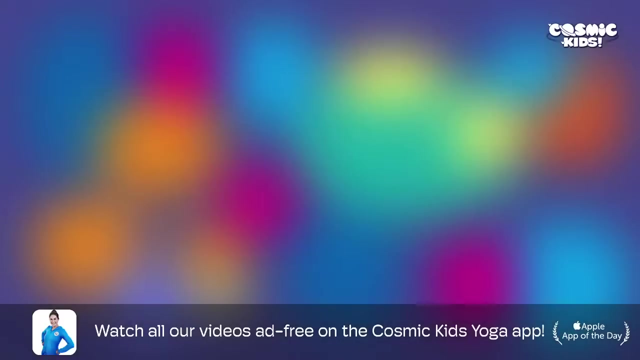 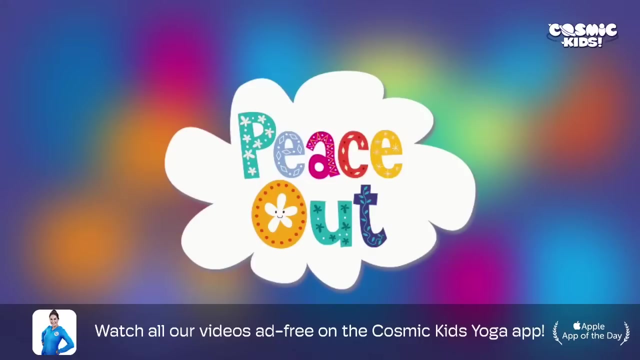 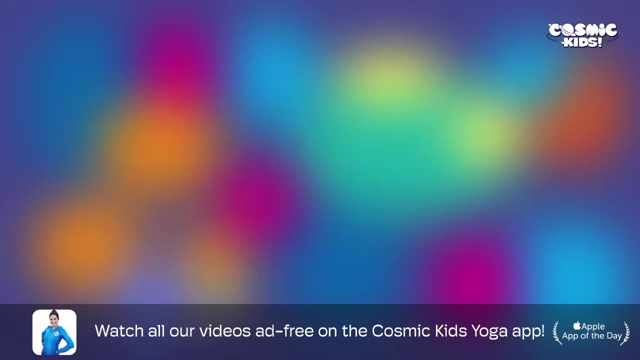 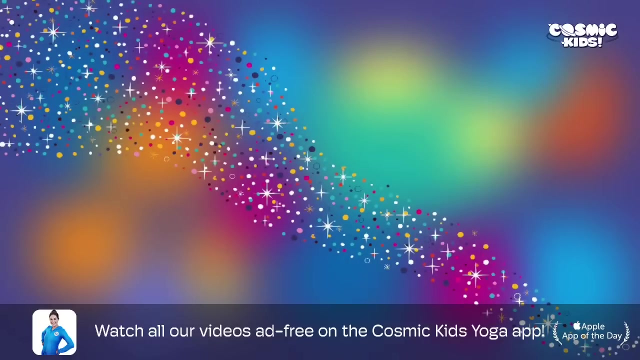 That was super cool. You were amazing. I hope you enjoyed the Trolls Adventure and I'll see you again soon for another Cosmic Kids adventure. Bye, bye, I love you. Peace out, Tickle Pixie. Hello, Jamie here. 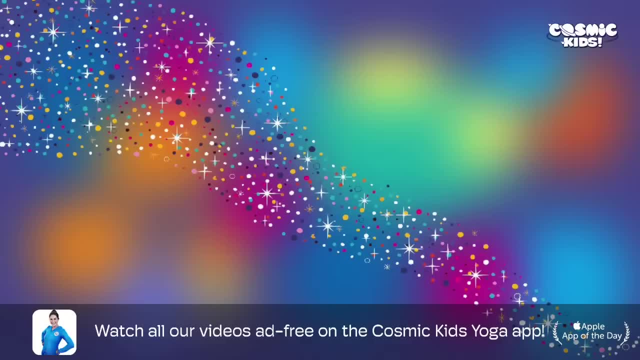 Welcome to peace out. It's time to turn the lights on on in your imagination and enjoy your amazing mind. So do what you need to do to get lovely and comfy, Find a space and lie down on your back, with your arms down by your sides or 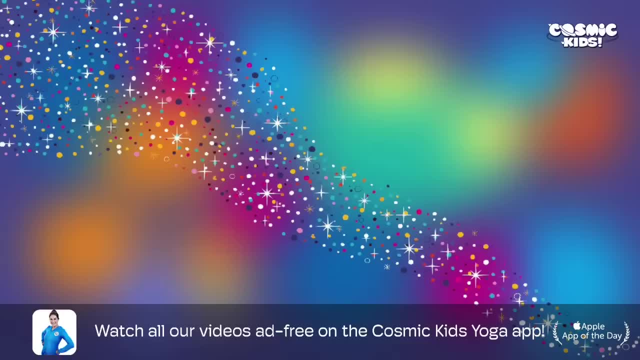 on your tummy, making a pillow with your hands to rest on. You decide which feels most comfortable. Now get settled. Do a wriggle and a fidget to make sure your body feels really happy and comfy. You don't have to be completely still. You can breathe and blink as normal, Just see. 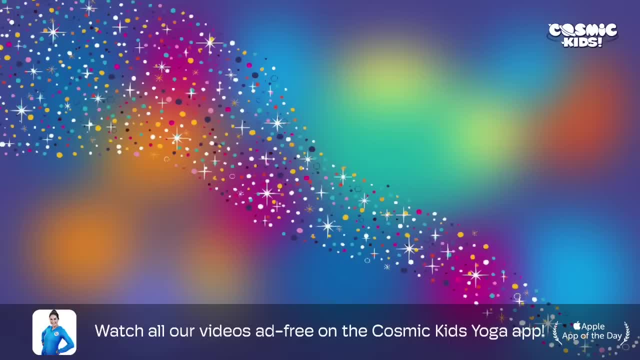 if you can keep your body nice and still Your eyes are open. Now that you're still, can you notice your breathing? Maybe you can feel it a little bit in your chest, maybe your tummy, at your nose and mouth Can you hear it too. 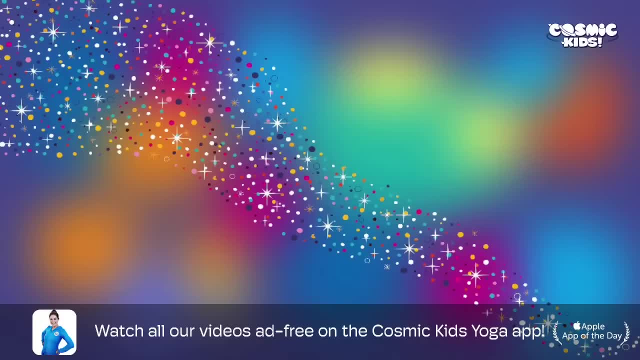 Not really a big problem to keep breath down. deal with the sound of breathing. If you don't want to breathe, take a deep breath in and out. It might be very, very quiet, Like a tiny whisper sound. See if you can hear it. 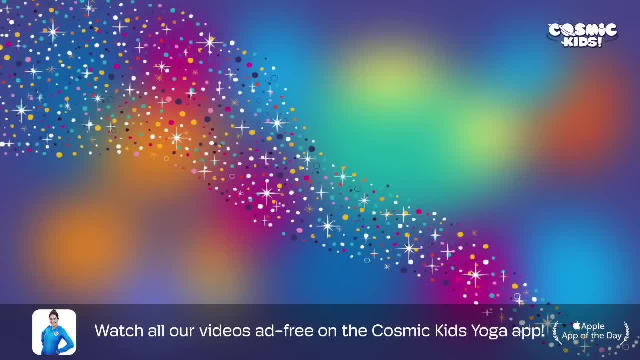 I'll be quiet, so you can try. That's it, Gentle breaths coming in through your nose and out through your mouth. In through your nose and out through your mouth. This next time, as you breathe out, let your eyelids softly close. 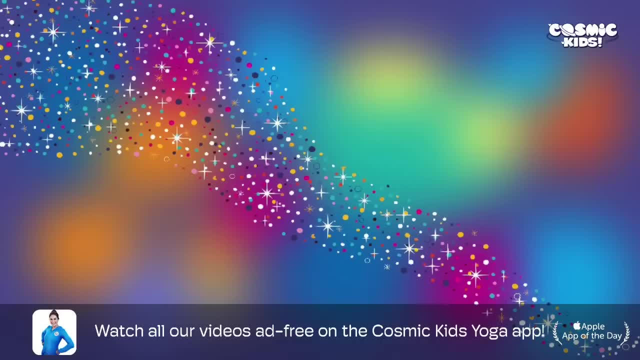 Well done. Now you have a big blank screen in your mind. See if you can imagine a little pixie standing right in the middle of it. That's right, a pixie, a small, fairy-like creature. Think about how it looks. 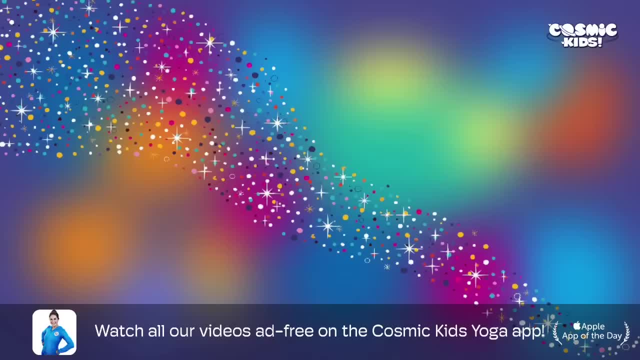 Does it have wings? What colour are its eyes? What's it wearing? What's it wearing? It may be a girl pixie or a boy pixie, or an animal pixie. You decide how your pixie looks. One important thing, though, is that this is a friendly pixie. 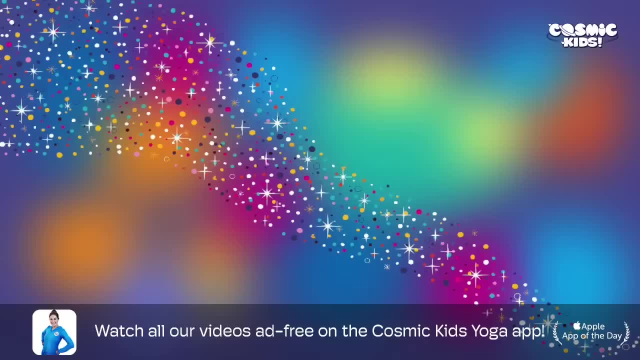 It's a good one. This pixie loves using pixie dust for tickling. not the kind of wriggling, giggling and jiggling tickles, Just a light, fuzzy tickle. that kind of feels nice and relaxing. The tickle pixie sprinkles magic pixie dust on our body and we feel it because of the. 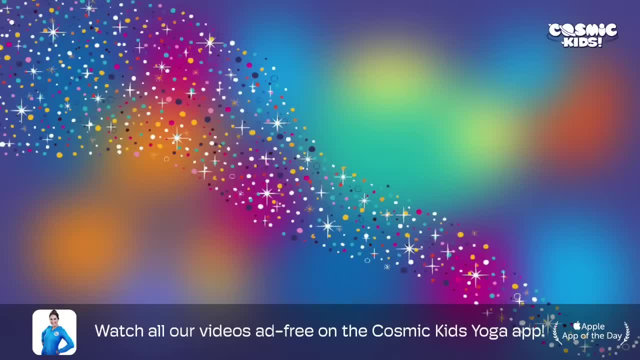 slight tickly feeling. that happens where it's been sprinkled. It's not a good thing. I have a pixie where it's been sprinkled. Let's see if we can notice the feeling when the tickle pixie sprinkles the magic pixie dust on us Ready. OK, Let's be as still as we can and see if. 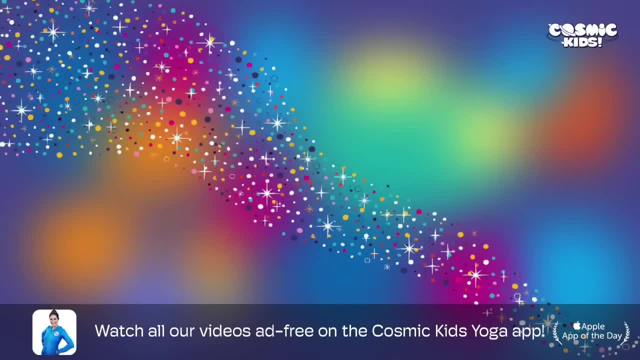 we can feel the little tickles, Here we go. The tickle pixie starts by sprinkling our feet. There's already a little tingle in our toes. Can you feel it? A slight fizzy feeling. It's moving all the way up through our feet. 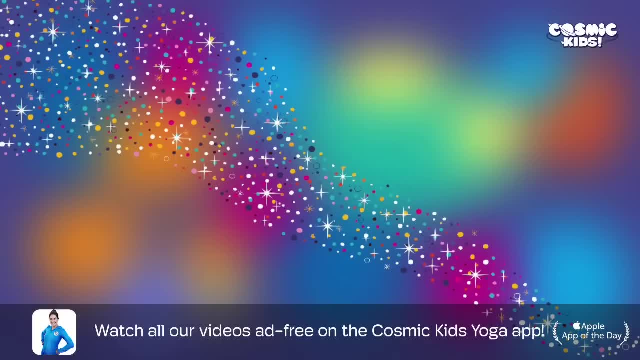 And around our ankles, The pixie moves up, sprinkling the magic dust on our legs. Ah, Now the warm, tickly tingles are happening in our legs, Moving up over our knees And into the tops of our legs. They feel all warm and sparkly. 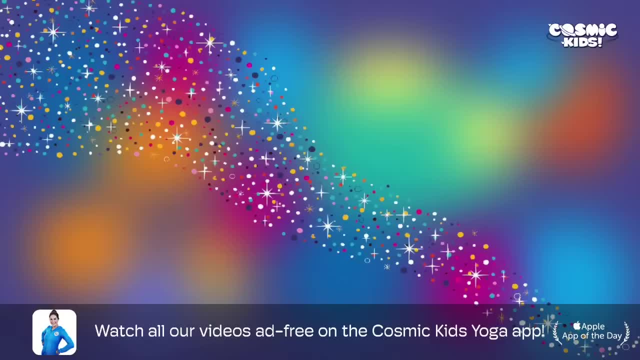 We begin to smile as we notice the tickly feelings. Now the pixie sprinkles the magic tickle dust over the middle of our body, our hips on our tummy and up across our chest. Our body feels the fuzzy tickles like we are full of twinkle lights. 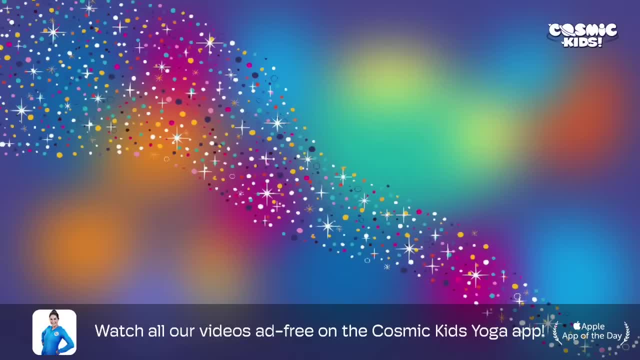 The tickle pixie carries on with the sprinkling. Now we feel the tickles travel all the way down our arms right to the very ends of our fingertips And now coming back up our arms again and over our shoulders. Now the fizzy feeling tingles through our neck and up into our head. 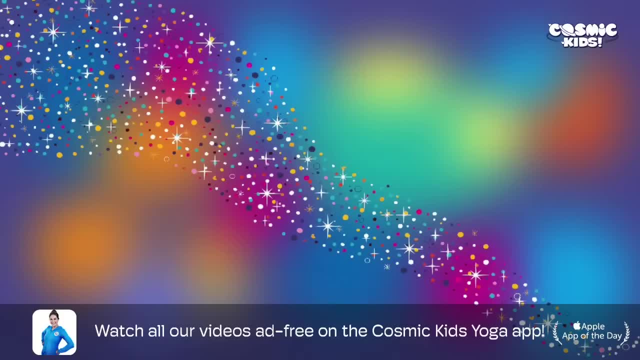 We feel our face tingle with the tickly dust. It may even make our nose wiggle. Wow, What a magic feeling. Our whole body is tingling with sparkling, tickle pixie dust. We feel fizzy and sparkly all over. 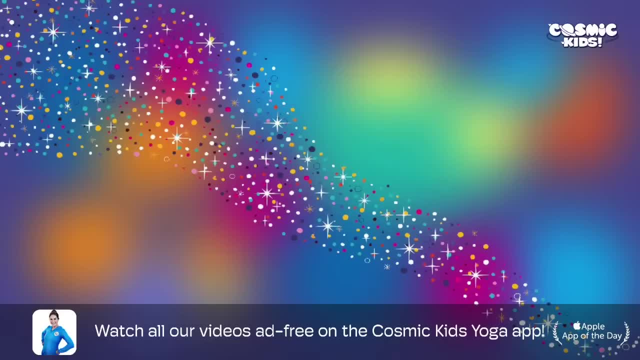 The tickle pixie has done its job. You see it in your mind, smile at you And blow you a sparkly pixie dust, kiss goodbye. It disappears in a puff of magic dust And the screen in your mind is once again blank. 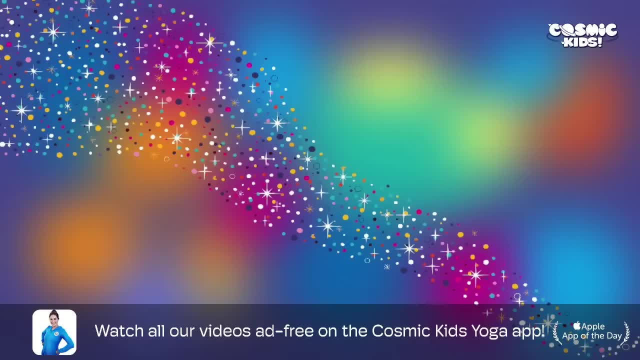 You smile, feeling happy that your body has felt the magic of the pixie dust And without saying the words, you think: a big thank you to your little pixie. It's time to return now. We come back slowly. See if you can notice the sounds around you. 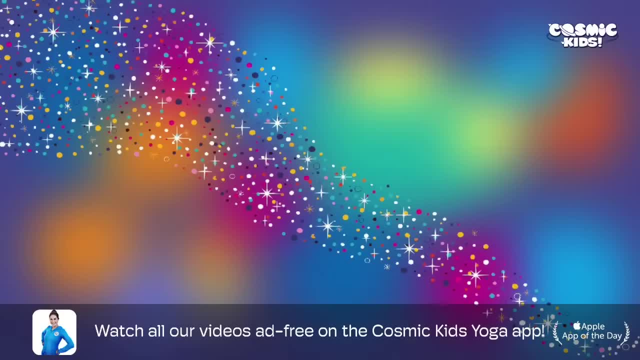 Feel where your body meets the ground. Have a good stretch Making your body long like spaghetti. Take a nice big breath in, Let your stretch relax and sigh out of your mouth. Gently open your eyes And now just sit Or lie where you are for a minute. 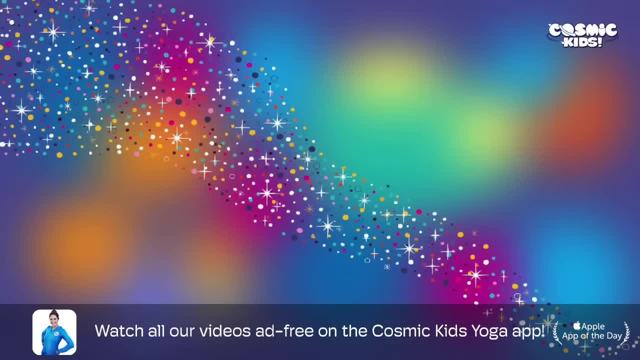 How was that? Having the pixie dust sprinkled all over you? Maybe you can still feel it a little. Well done for giving yourself this time To stop breathe and feel your body, from top to toe, Tingly with magical, sparkling pixie dust. 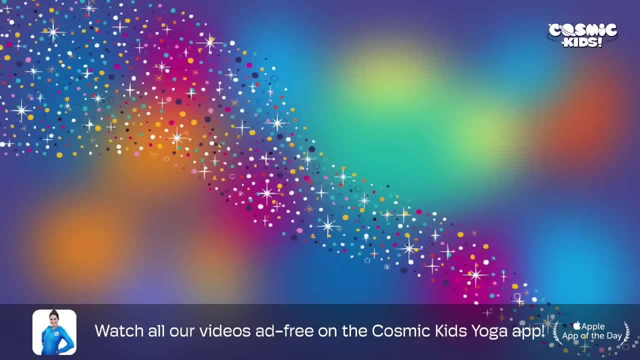 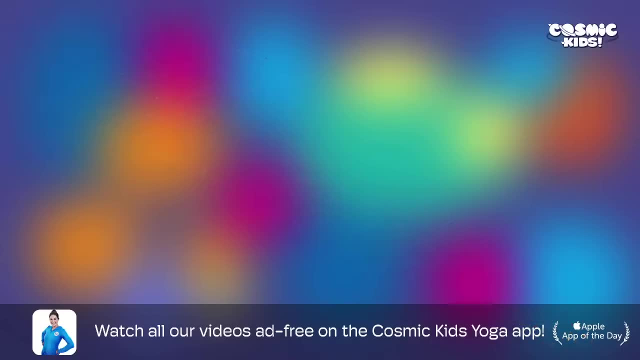 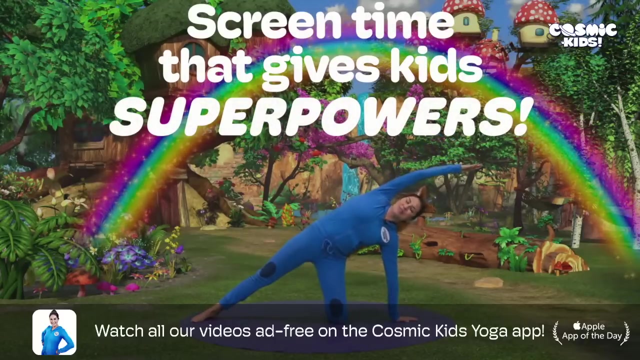 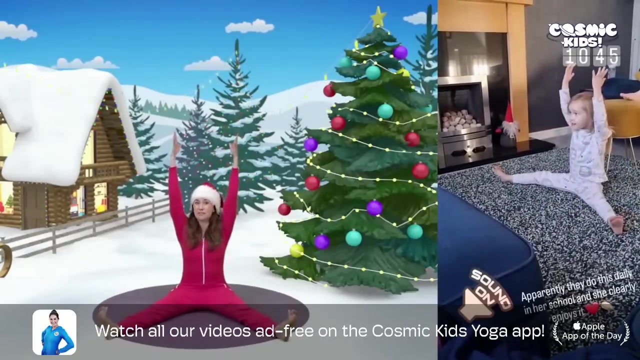 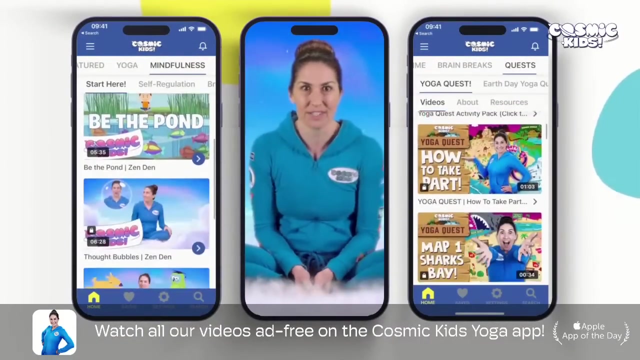 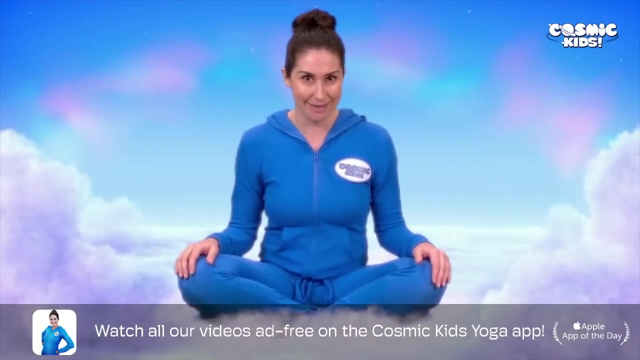 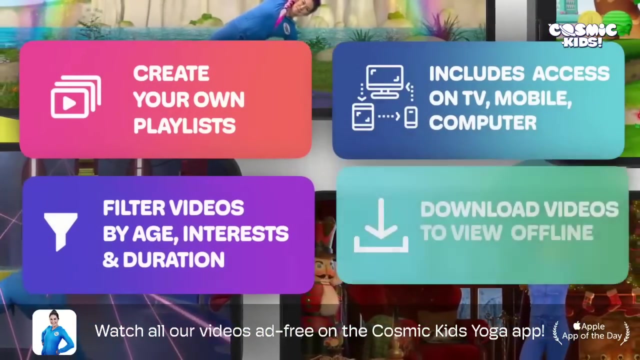 I hope you come back soon. This is Jamie saying peace out. 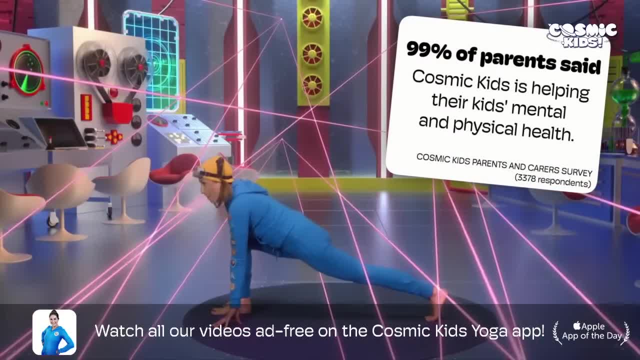 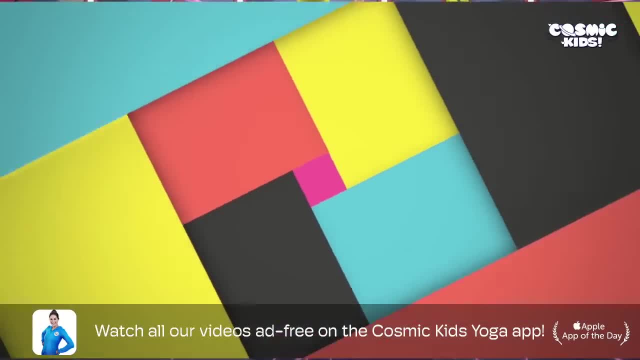 between our hands. Oh, thank goodness, we do yoga Now, making our legs very strong. we lift all the way up, trying not to wobble, Lifting our arms up to the sky, And then we fold all the way forwards. Hands come either side of our foot. We step. 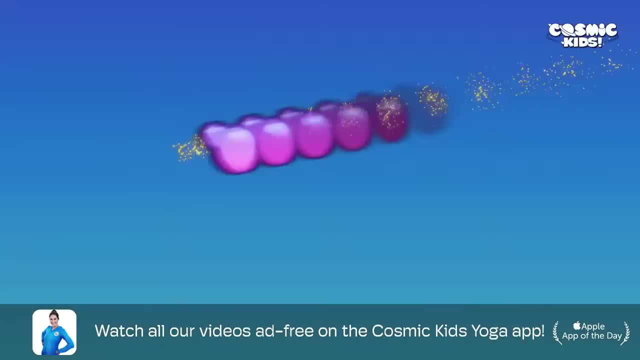 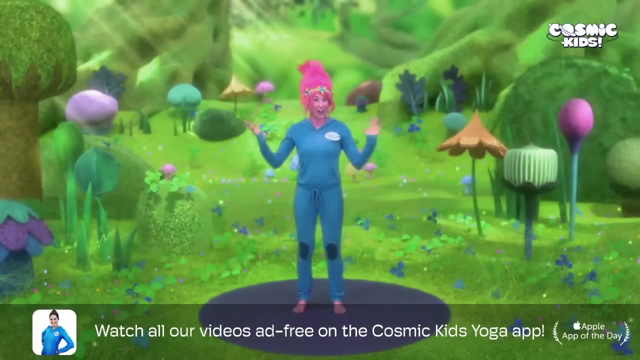 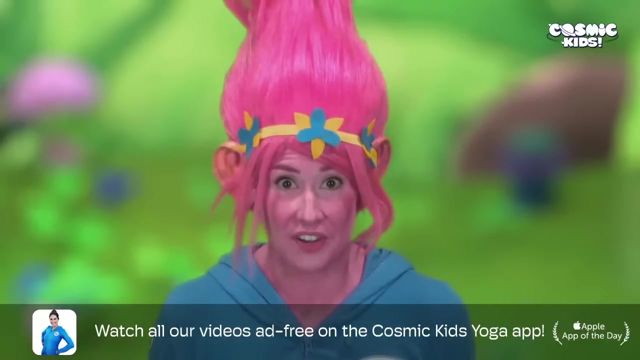 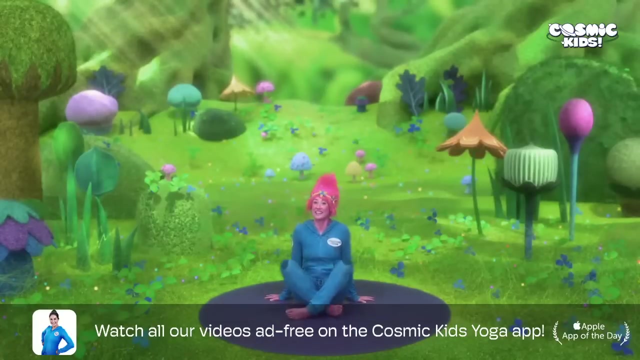 Hello everyone, Welcome to Cosmic Kids. I'm Jamie and this is your place for yoga stories and fun. It's easy: Just copy the moves I do and enjoy the adventure. Now, we always start in the same way, and that's by sitting on our bottoms, crossing our legs and bringing 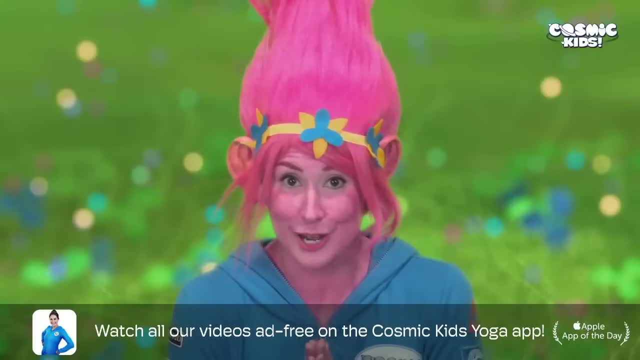 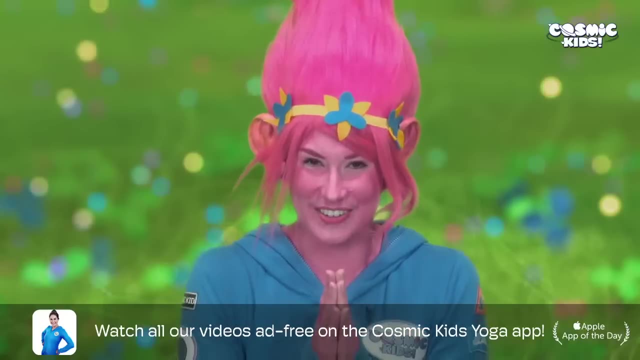 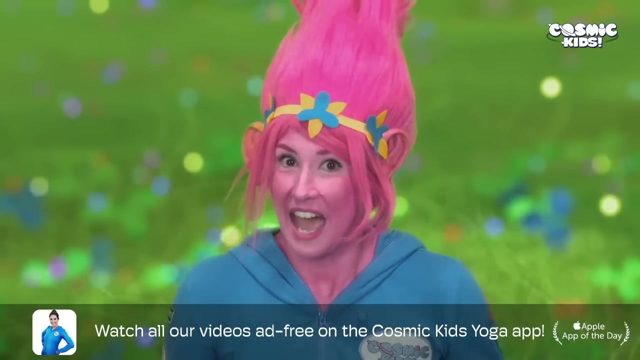 our hands together at our hearts and saying our secret yoga command Code word, which is Namaste, Ready After three, One, two, three, Namaste There. Now we're ready to begin, And today we've got a special adventure inspired by the Dreamworks. 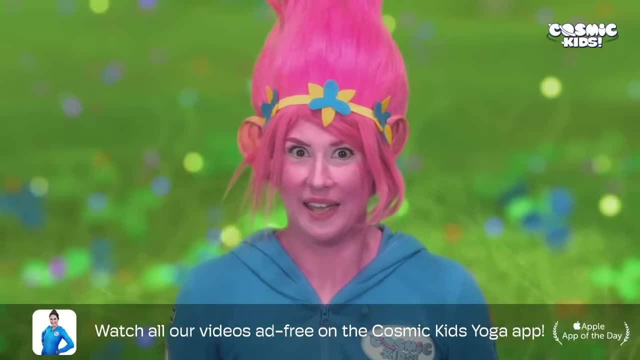 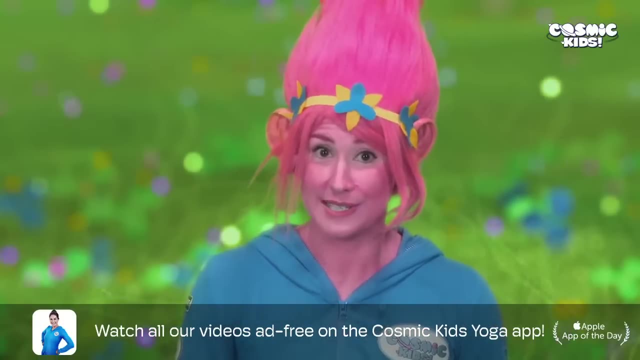 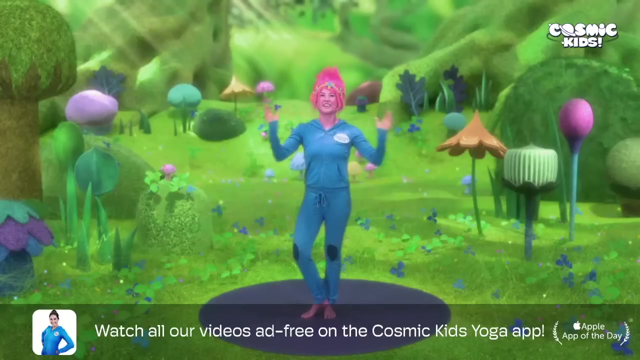 movie Trolls. That's why I've got my pink poppy hair and my pink poppy body. Very exciting. Now our story begins 20 years ago in the happy forest, in the Happy Trolls. So let's come up to stand and do our tree pose, bringing one foot on top of the other. 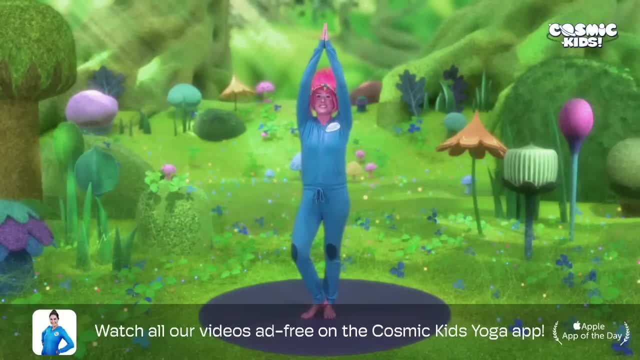 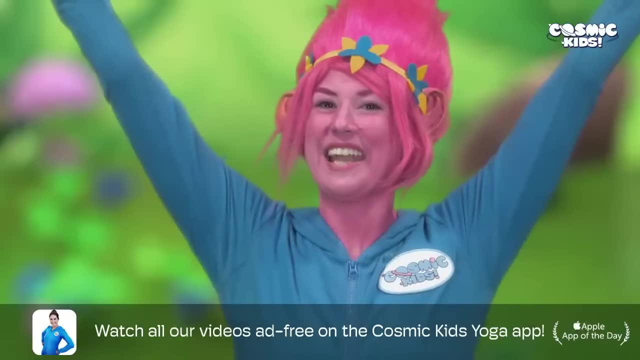 our hands together at our hearts. Let's grow our tree up nice and tall and open our branches and let's sparkle our fingers because we're a very happy tree. Yes, Now can we do our tree pose on the other side. Let's try. Bring your other foot on top now using your heel. 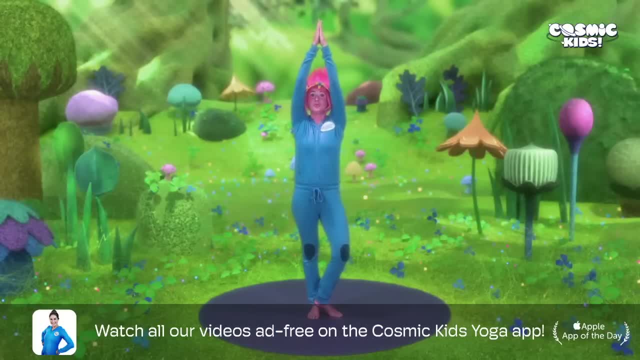 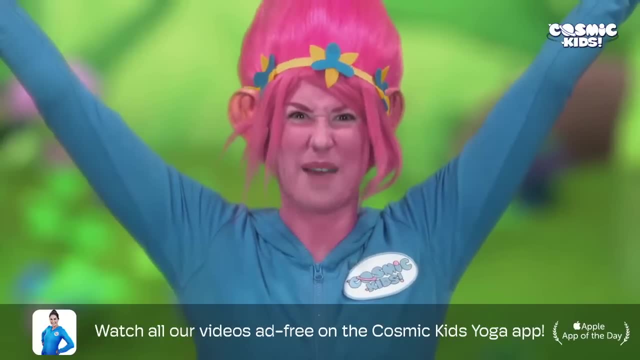 Bring your hands together at your heart and grow your tree up nice and tall, opening your branches wide, sparkling your fingers, and have fun. How about a big smile? Ding Yay, We're happy trees Now. living in the tree were trolls. 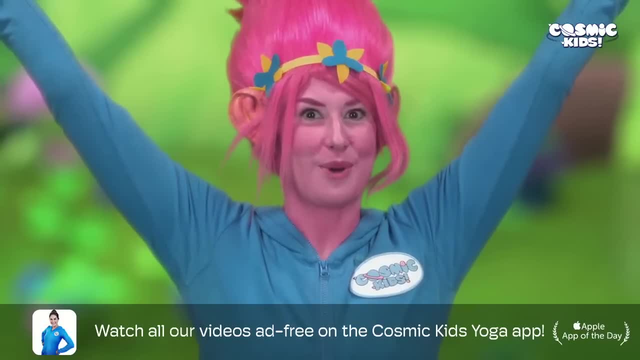 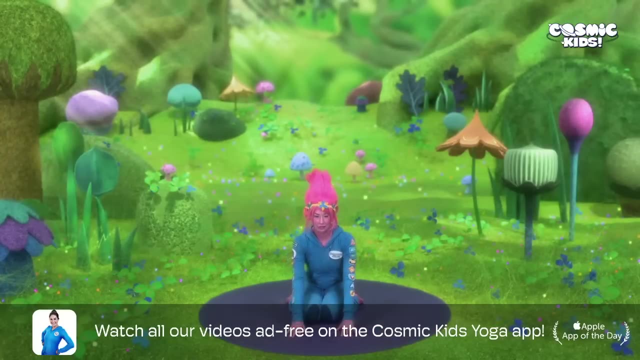 tiny creatures with big, colourful hair. Let's come into our troll hero pose, Coming down onto our knees. Now, take your hands forwards, take your feet wide and snuggle your bottom down in between your ankles. Yes, Criss-cross your fingers, turn them inside out and lift. 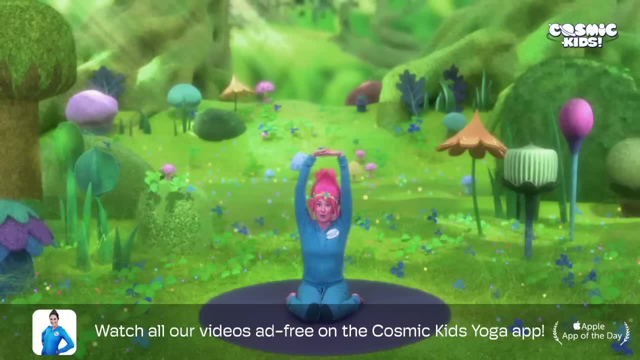 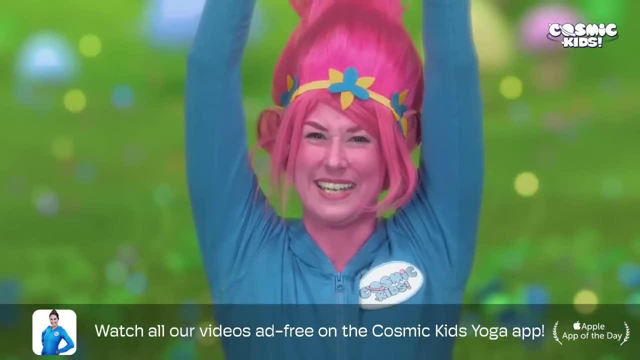 your arms above your head, Coming into your troll hero pose. Now, if that's a bit ouchy on your knees, you can lift them up, Lift your bottom, scoop your feet underneath and sit back on your heels. Yes, Now the trolls. 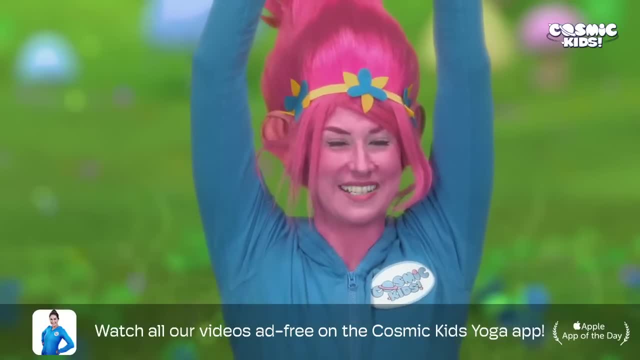 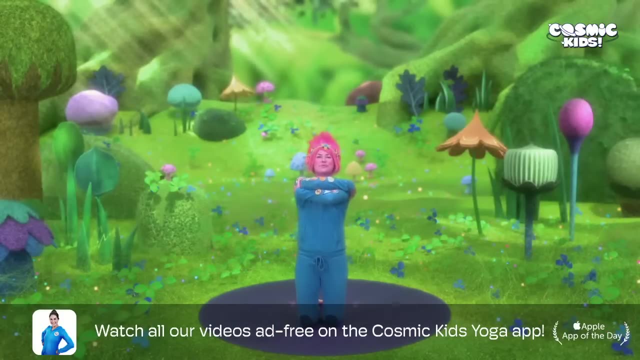 love to sing, to dance and to hug. Let's come up into a hug pose Sitting up tall arms wide. wrap yourself up in a big beautiful hug. Oh, it's wonderful. Life for the trolls was full of glitter showers. Let's come into our glitter shower pose Taking your arms. 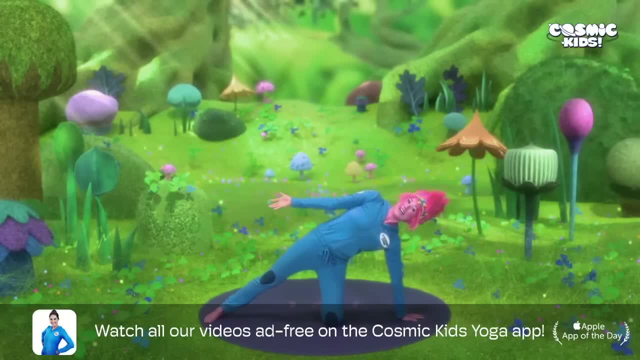 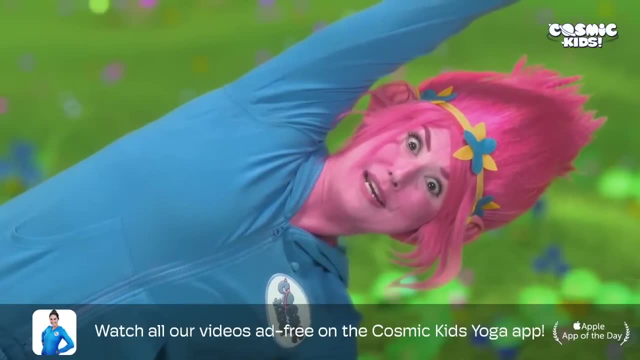 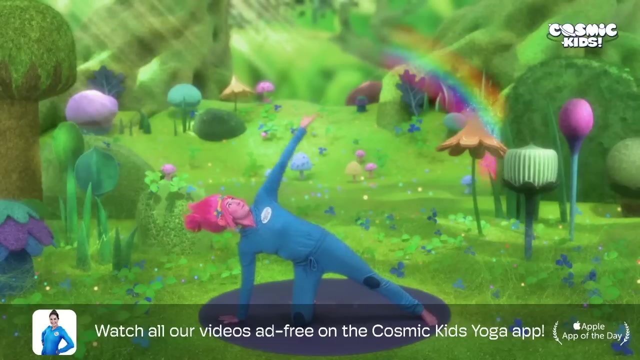 wide. take your foot to the side and drop down onto one of your hands and sweep your arm up and over your ear- Yes, making a glitter shower appear. It was also full of rainbows. Coming back to two knees: arms wide, leg to the side, drop down onto one hand and sweep a big, beautiful arcing. 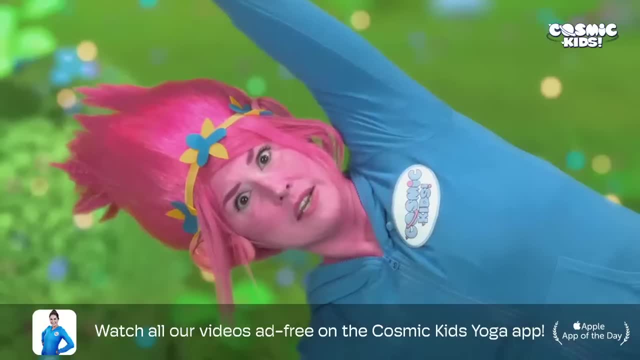 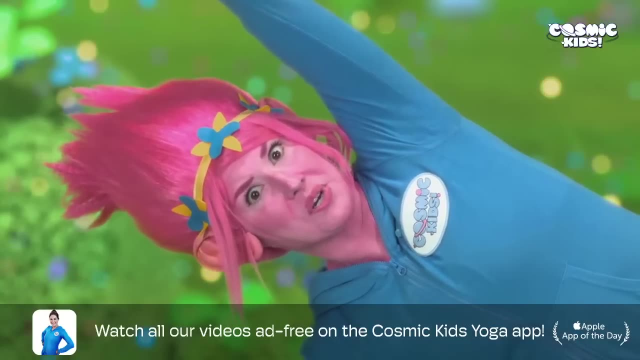 rainbow over your head. Wow, how lovely. Now the Bergens were the exact opposite of the trolls, Always feeling sad and clomping heavily around Bergentown, Coming up to stand in our clompy Bergen pose Feet nice and wide. 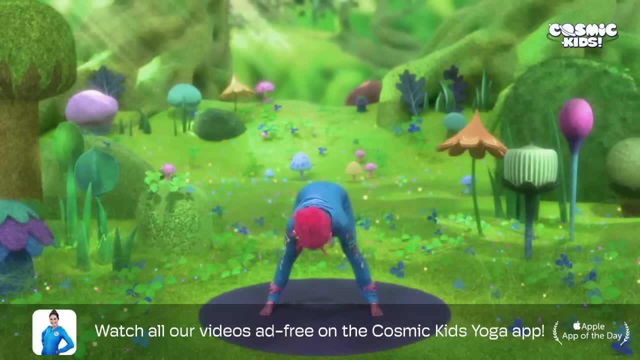 fold your body forwards, holding onto your ankles, and let's clomp. Here we go, Clomp, clomp, clomp, clomp, clomp, clomp, clomp, Rolling up to stand. Oh, to be happy like a troll. That's all they wanted. 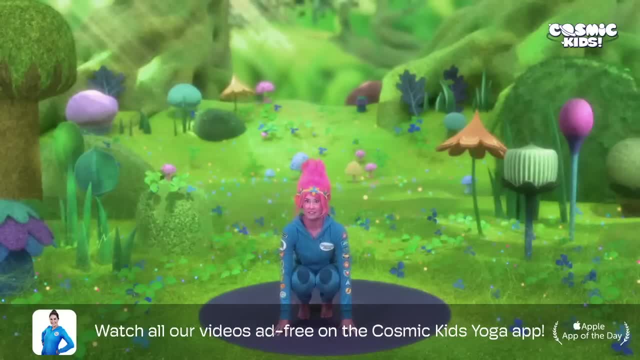 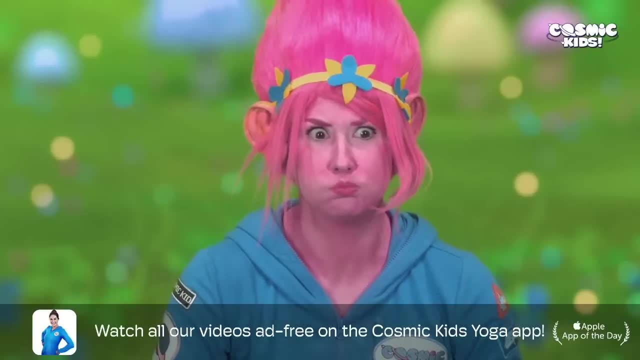 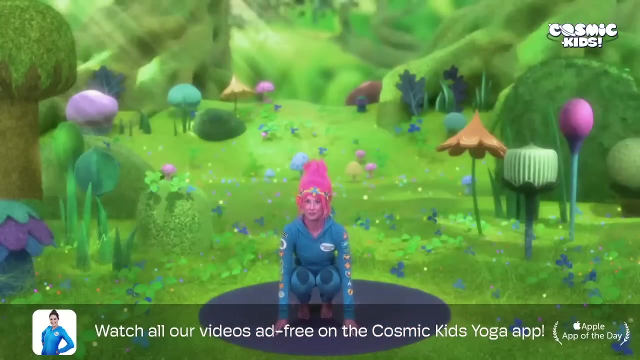 Then one day coming down to crouch fingers to balance a Bergen ate a troll, Seeing if you can balance with your fingers off and gobble a troll, It made him smile And then it made him jump for joy with a big woohoo. After three, let's do a big woohoo, jump in. 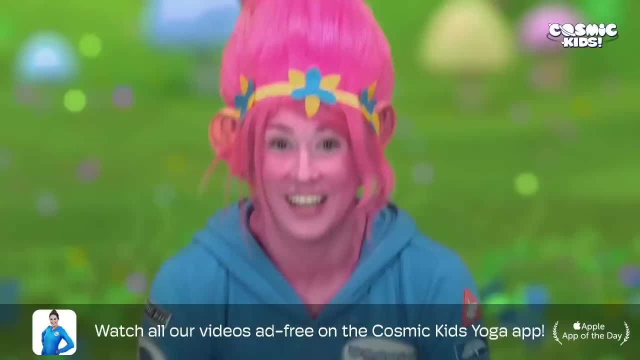 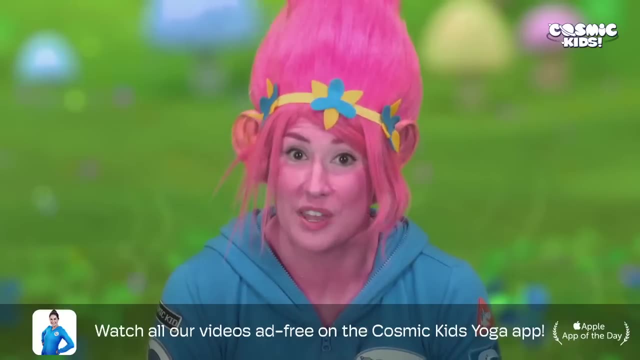 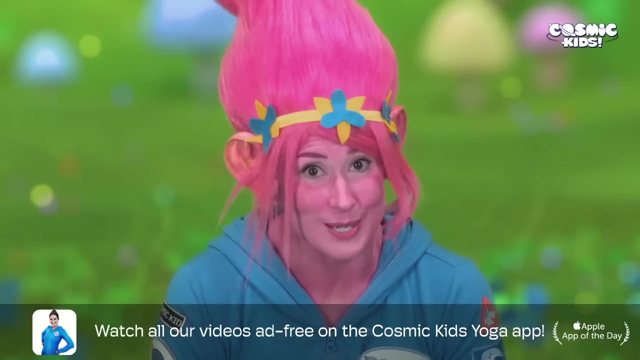 the air: One, two, three, woohoo. So this is the secret to happiness: eating trolls. And so they hold a festival each year, Trollstice, where they feast on trolls to be happy for one day One Trollstice. the young Bergen prince, Prince Gristle, is lying in his bed. 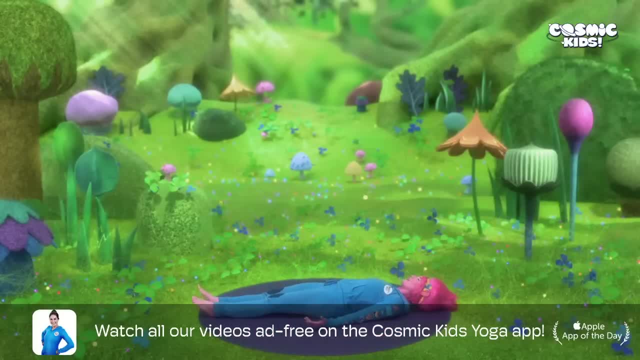 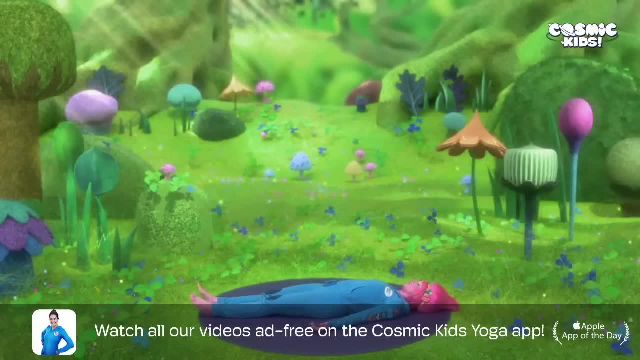 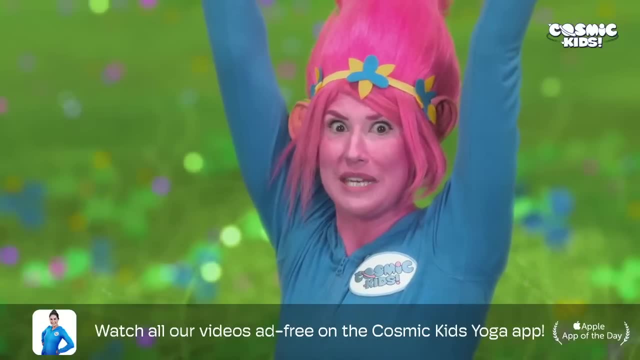 to be happy. We're going to be happy. We're going to be happy. We're going to be happy Closing our eyes. It was time to wake up, So we open our eyes. He sits all the way up and he stretches excitedly. Today is the day he gets to eat his first troll, And no ordinary. 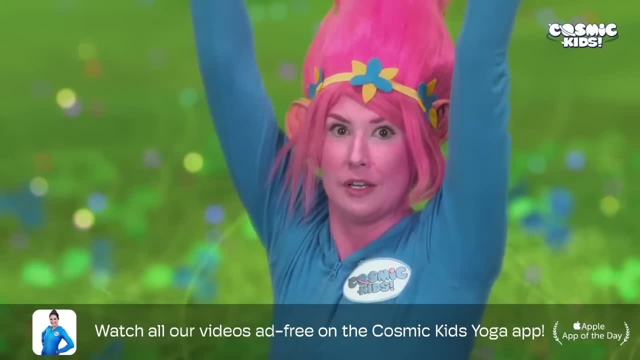 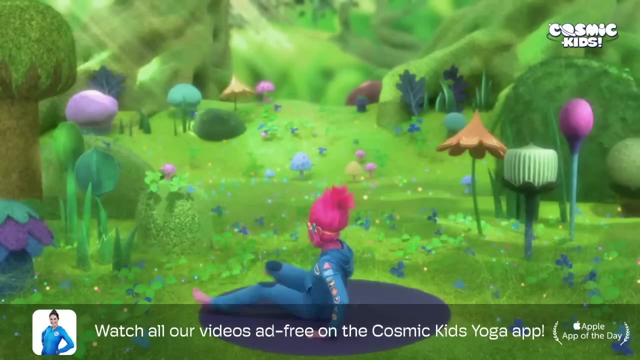 troll, Princess Poppy, the special baby troll. But come feast time all the trolls escape down the secret tunnels. Coming into secret tunnel, pose On to our hands and our knees, Tuck your toes and lift your hips all the way up to the sky And we're going to be happy. 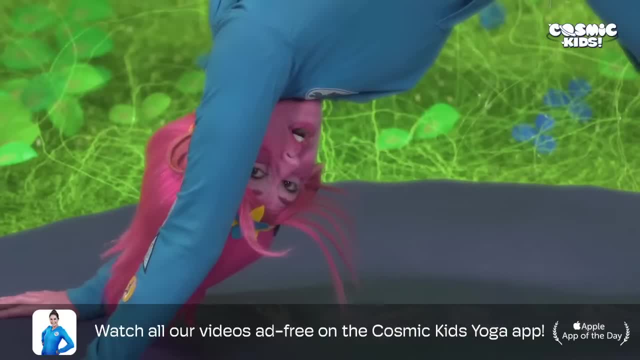 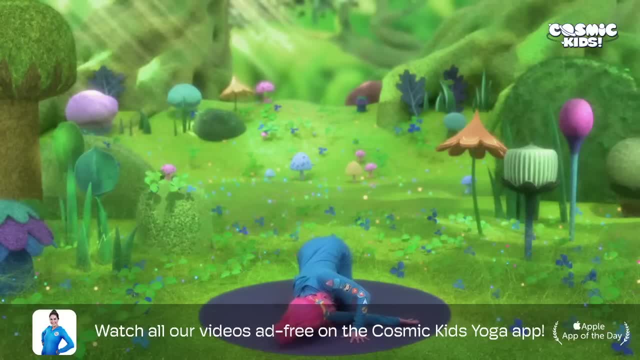 Now scoot your hand through the gap between your arm and your leg and see if you can rest on your shoulder reaching for a troll. Ah, Coming all the way back up. Let's do that on the other side. Scoot your hand all the way through the gap and reach for a troll the other way. 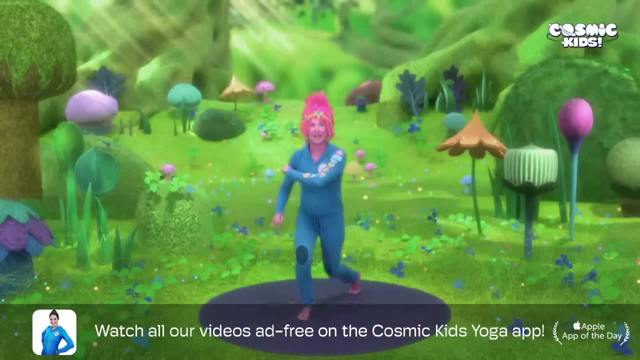 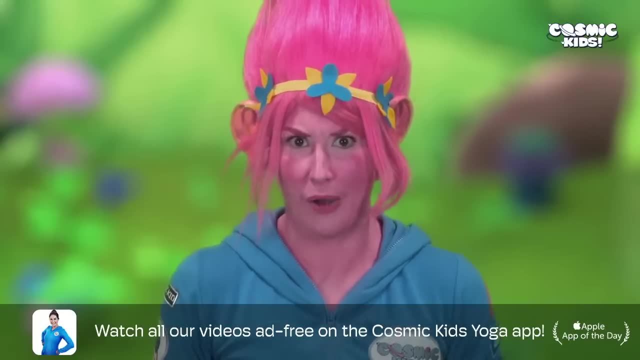 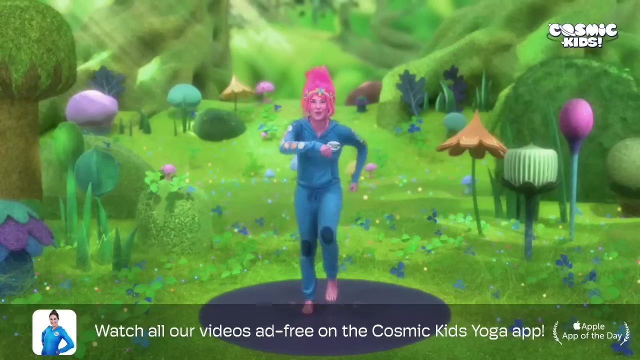 Nope, they can't get them Coming all the way up to stand, And that's because the troll king, King Peppy, marches. his people to safety, Let's march, He chants. No troll left behind, No troll left behind, No troll left behind. 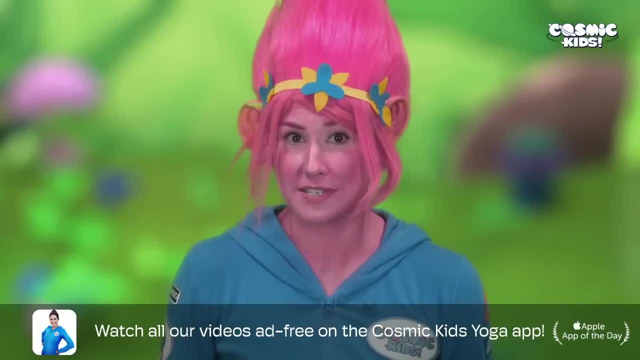 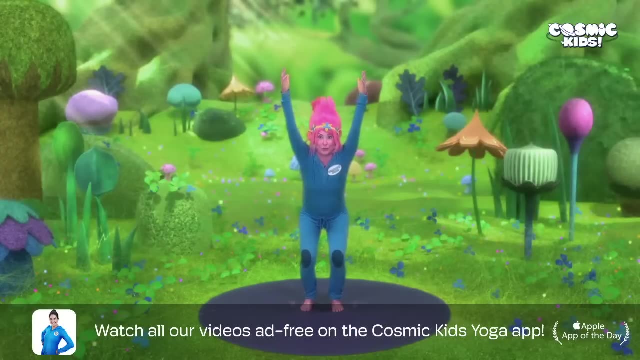 Back in the Bergen palace, the king, King Gristle, sits sadly in his throne, Bending your knees, sweeping your arms up by the side of your ears. coming into your throne pose, He tells his young son that he will never be happy. 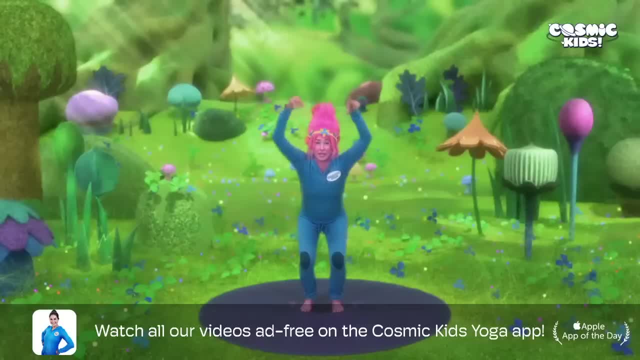 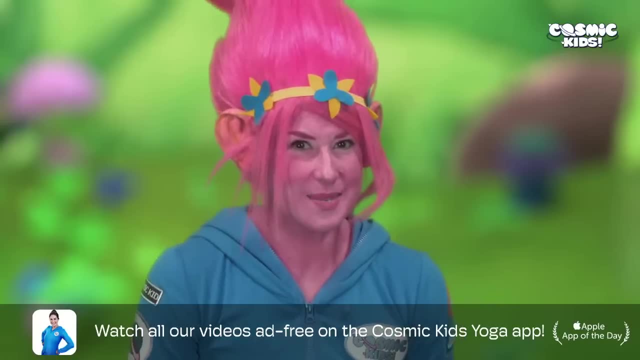 And he banishes Chef for letting the trolls escape Coming up to stand. Now, 20 years later, in the new troll kingdom, Princess Poppy decides it's time for a party, Jumping her feet wide, taking her arms wide. 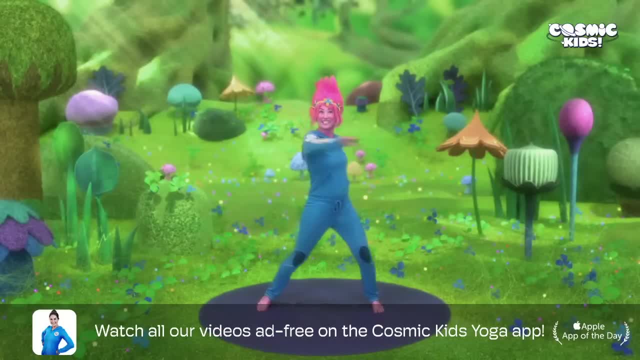 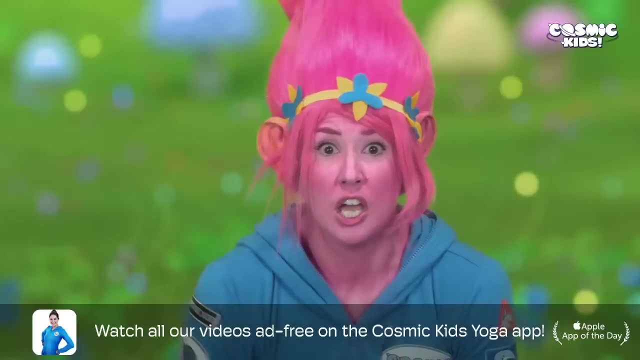 she begins to spin And she sings, inviting everybody: Move your hair and feel United. Oh, Branch, the grey troll crouches down, Going shh. Too much noise and the Bergens will hear. You'll lead them straight to us. 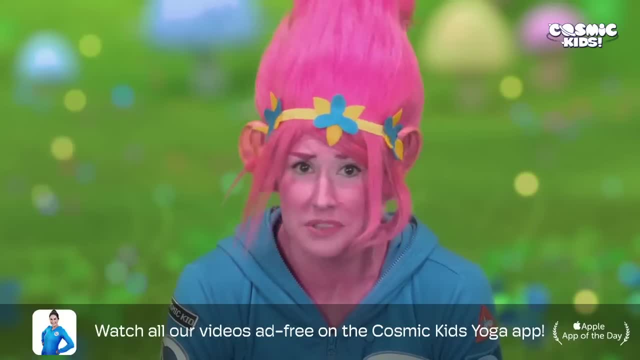 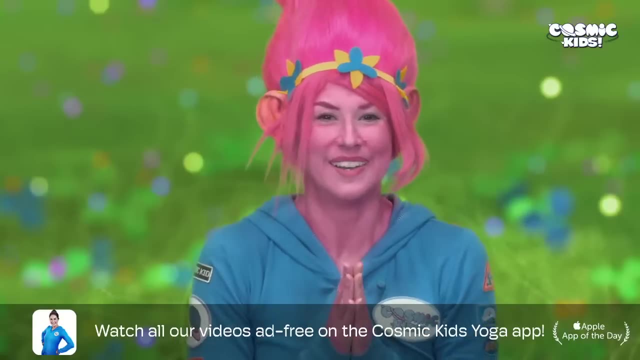 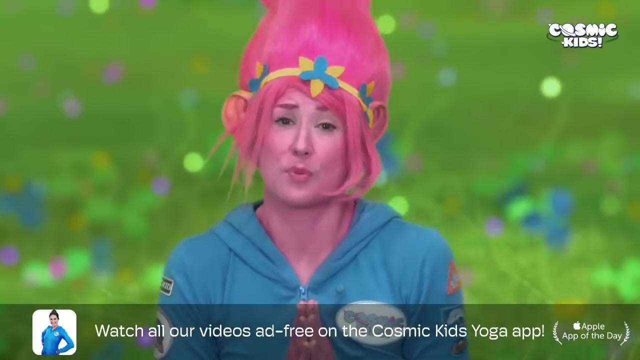 And then creak. the yogi troll arrives with a namaste Sitting on your bottoms, crossing your legs. Bring your hands together. After three let's do a namaste. One, two, three Namaste. He encourages Branch to channel the positive energy. 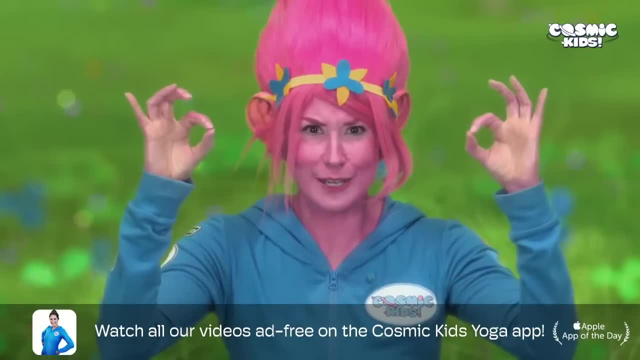 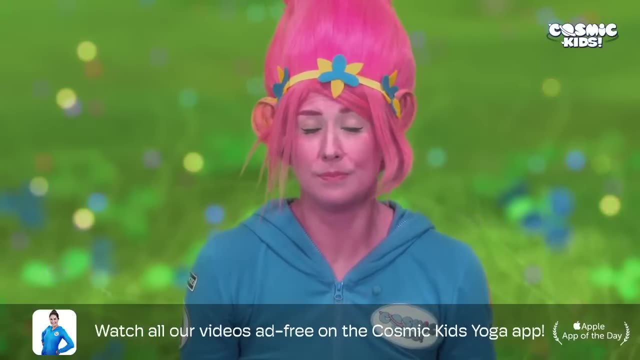 And together we do an om just to do that, Bringing our thumbs and fingers together, Resting them on our knees, And let's om Om, Opening our eyes. Bing Oh, look at the time, It's hug time. 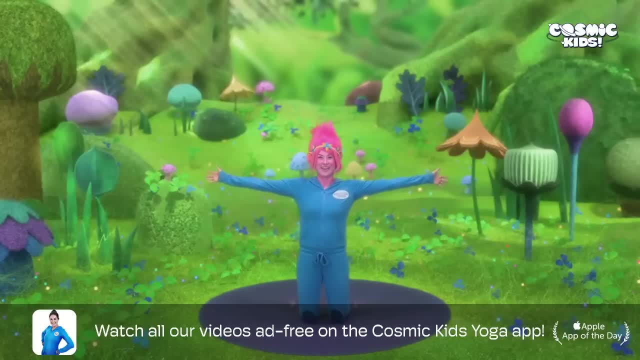 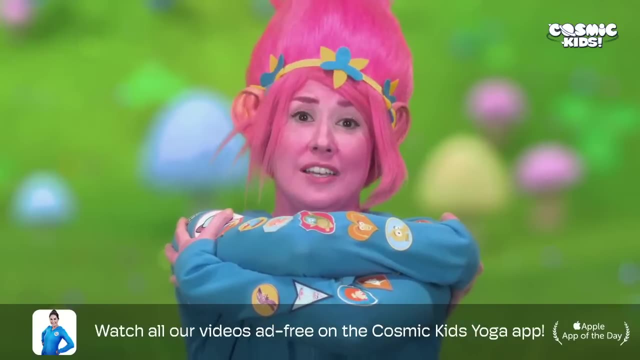 Coming up onto our knees, Arms wide. Let's hug, Oh, wrap it in. Oh, yes, I could squeeze you forever. Now, despite Branch's warnings, the party happens. There are glitter cannons popping. Let's come into our glitter cannon pose. 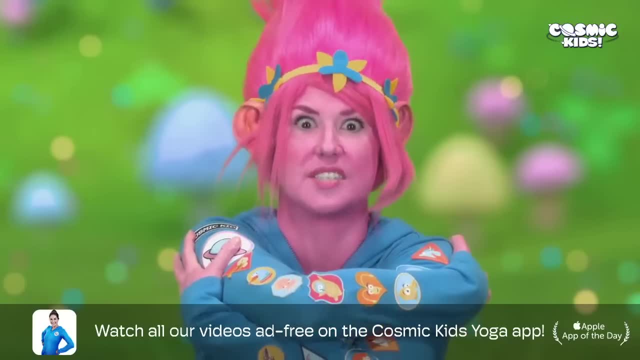 Up onto our tippy toes. Now we're going to jump in the air after three with a big pop of glitter. One, two, three Pop, Yay, There's jumping to the music. Coming up to stand And let's jump. 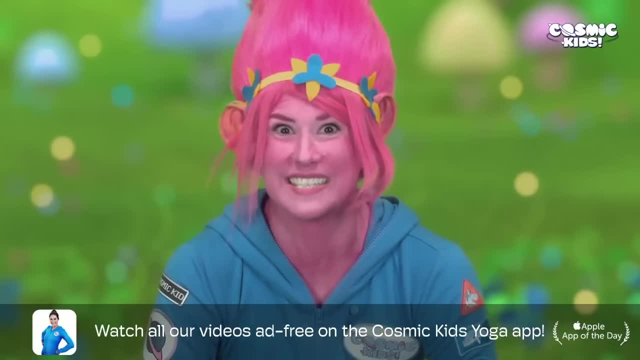 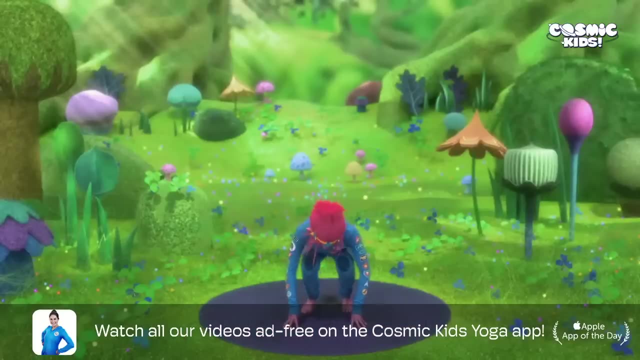 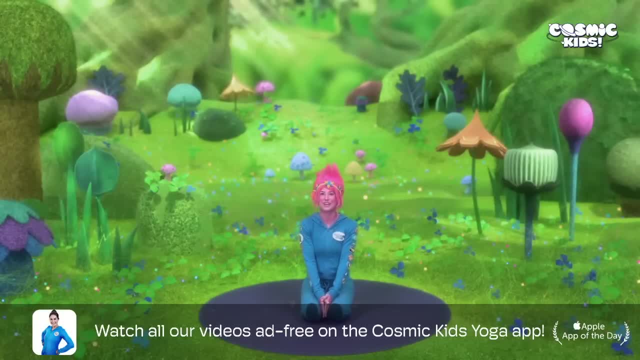 Bringing your hands down in between your knees. We're going to breathe in as we lift up. Here we go, And then we're going to blow a light volcano to the sky. Woosh, Breathing in, lift up And whoosh- a light volcano to the sky. 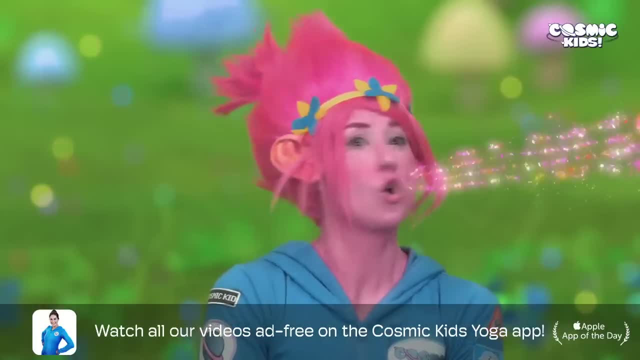 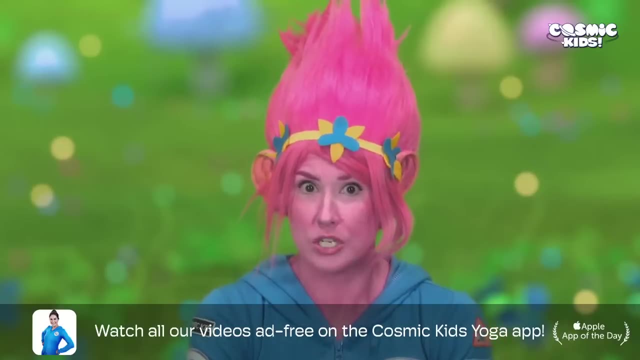 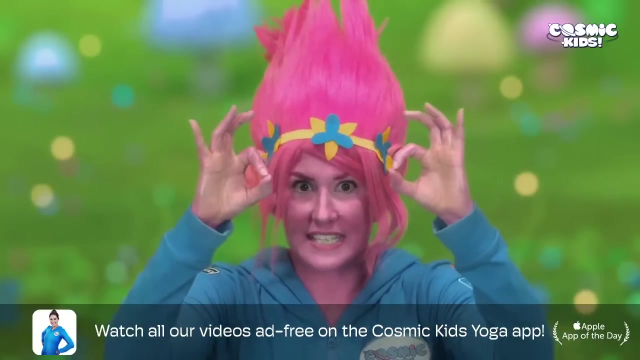 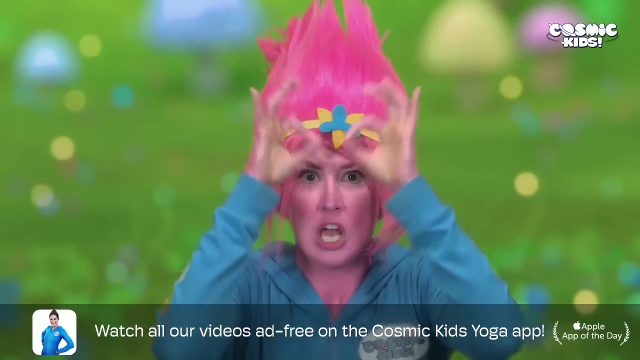 Woosh, Let's do a few little ones. Whoosh, Whoosh, wow, it's amazing. it is loud, so loud that the Bergen chef hears them. she looks through her cosmonoculars, joining your thumbs and fingers together. everyone have a look through there. they are the trolls. she sees them lowering her hands. 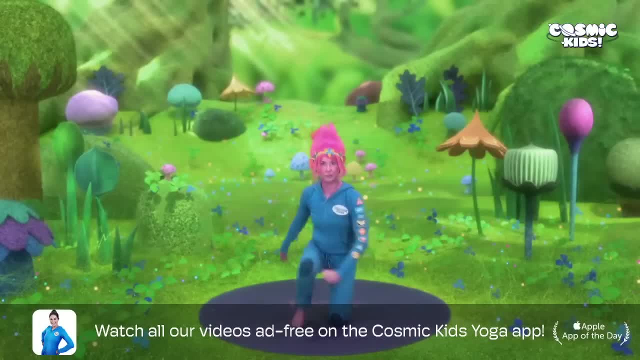 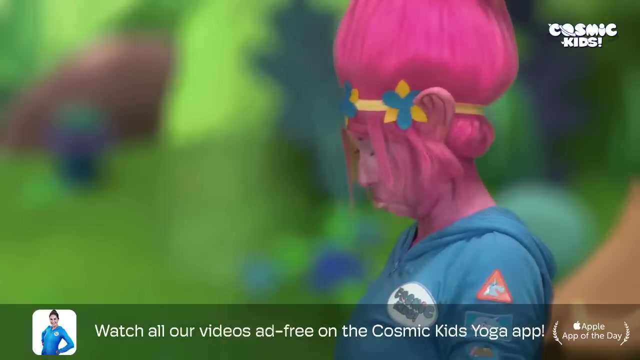 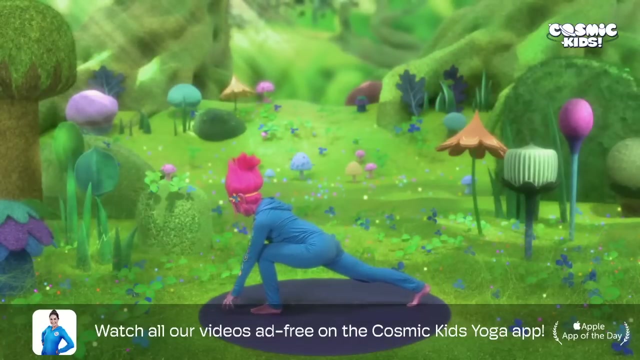 here she comes, taking big steps, coming up to stand everyone. let's take a big step forwards. here we go, big step. she reaches all the way forwards to grab a handful of trolls. then she steps all the way back to put them in her pouch. then she steps forward on the other leg- big step. she reaches all the way in to grab. 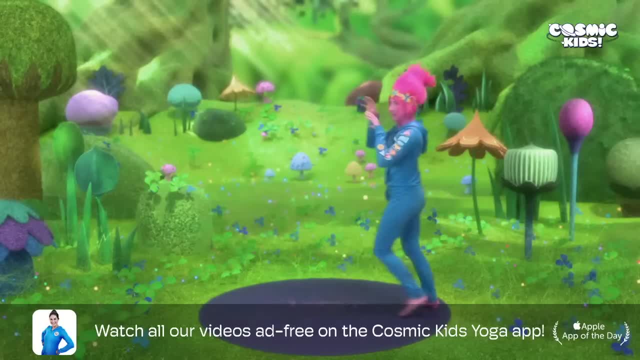 those trolls and she steps all the way back to put them in her pouch. oh no, the trolls run in all directions. Queen Poppy shouts- God help me, aeeeeeeee, clicks. King Peppy and Poppy hide, coming into hiding, pose down onto our knees, untuck. 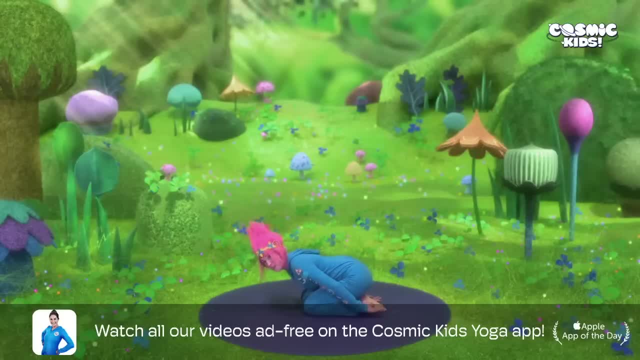 our toes, folding our heads all the way forwards, to be very quiet as we hide under our hair. coming up to sit when the coast is clear, Poppy decides she needs to save everyone and she gets up quietly. she tiptoes down to branch, the gray trolls bumbling. Пальп anac shoulderуска 謝謝. 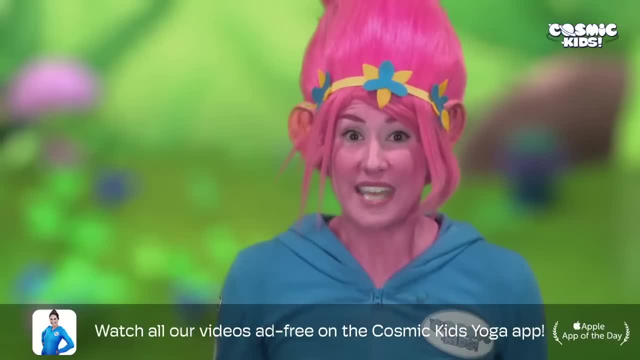 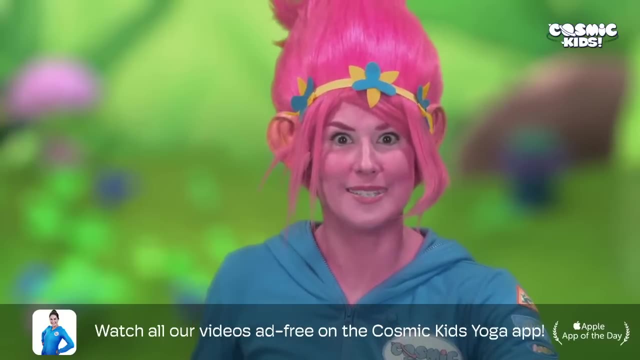 nom paddy tagging along. that was a lesson on learning the elections hunger. Shh, shh, shh. She asks for his help, but he doesn't want to, And so Poppy brings all the other trolls down to hide with him just in time for ding. Hug time Arms wide. 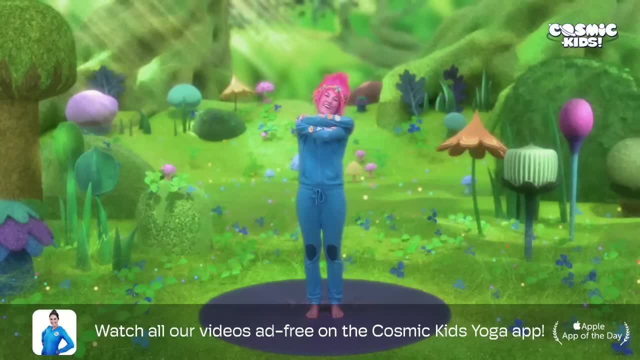 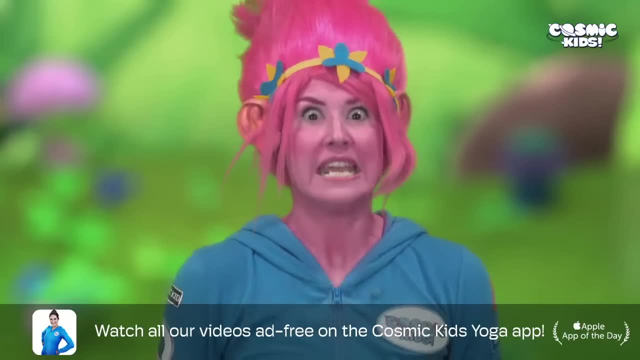 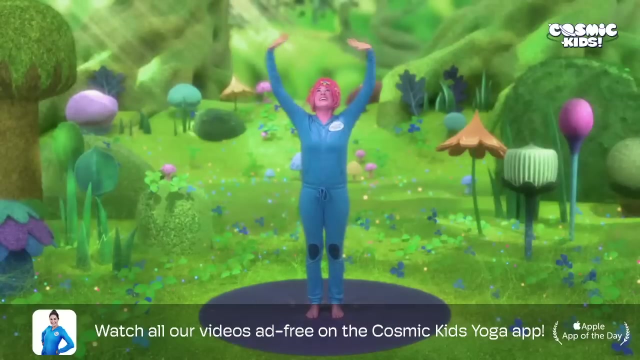 wrap yourself up in that big beautiful troll hug, Ah, lowering your arms all the way to the side. And so Poppy sets out on her journey alone into the scary forest, To feel brave. she sings about the sunshine Reaching up to the sun. give it a wave and say hello sun. 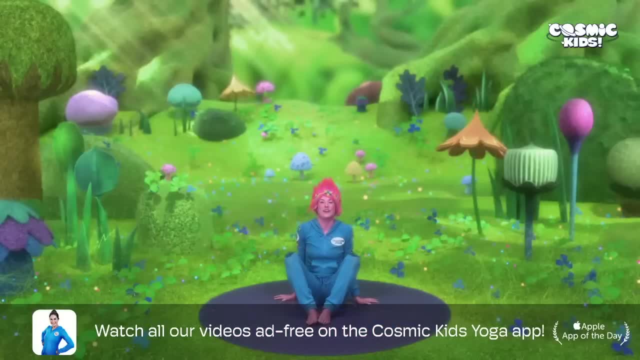 She sings about the butterflies coming to sit in butterfly pose, Soles of your feet together, holding onto your feet and fluttering your butterfly wings. Yes, lovely, Even getting soaked by the rain, Using your fingers to pitter, patter your head and your face, all. 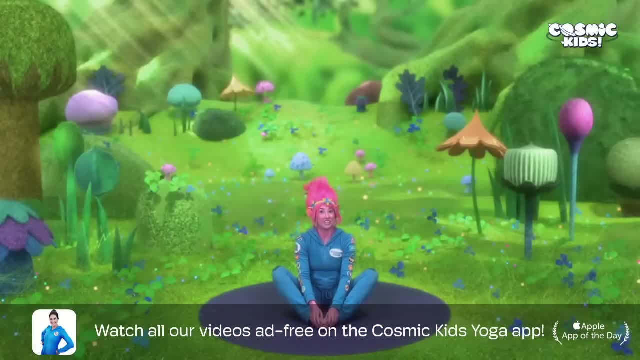 the way round- Maybe your legs, yes. And she gets chased by the wiggly, wiggly, wiggly wormy monsters. coming into our wiggly wormy monster, pose Onto our tummies, everyone Hands underneath your shoulders. Now wiggle, wiggle, wiggle, wiggle all the way up, Making. 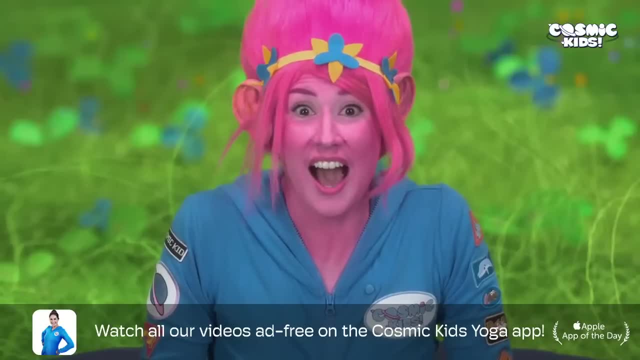 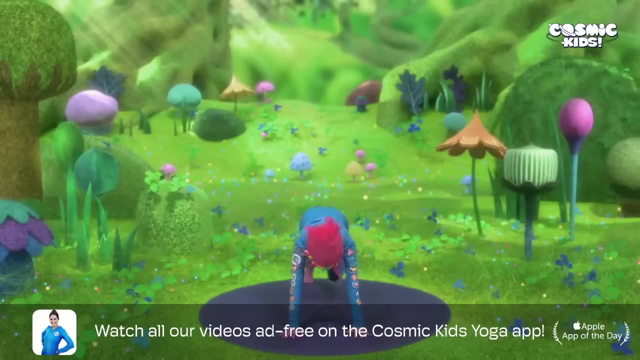 yourself into a wiggly, wormy monster. She sings: I'm not giving up today. And about getting up again, Tucking your toes up onto all fours, walking your feet forwards and rolling up to stand. Then comes the spider's web: Jump your feet wide, take your arms wide. 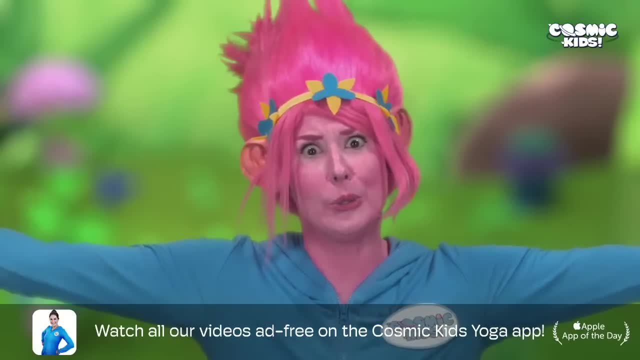 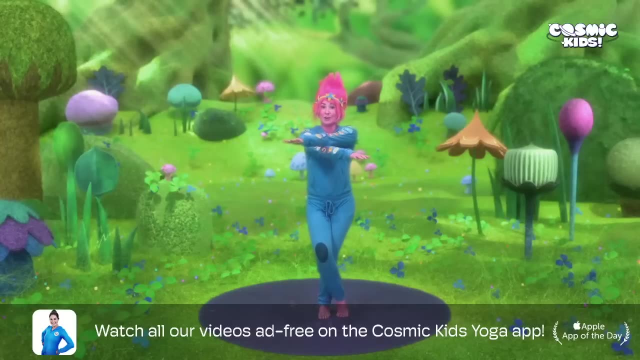 No, she gets wrapped up in a sticky cocoon, Bringing your feet together now, crossing one leg over the other and bending your knees. Arms wide, scissor your arms, wave with your underneath arm and twizzle them round, Sitting yourself down a little bit lower. Oh, no, she's. 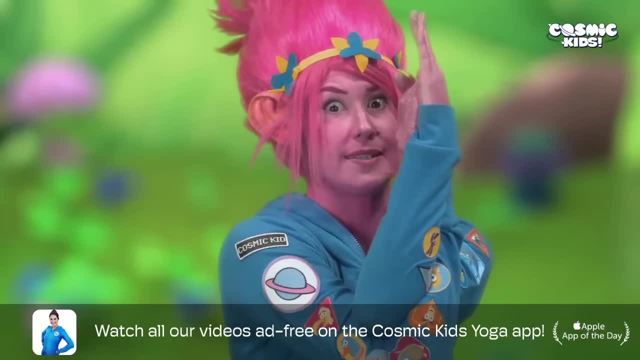 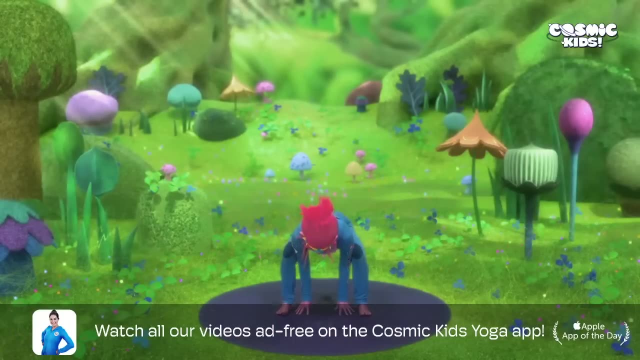 in a real sticky cocoon. And here come the spiders scuttling along to gobble her up, Taking your feet wide, coming into spider pose, Bending your knees, hands going between your feet. Now ticker, ticker, ticker. your fingers round the back to the ins and outsides. 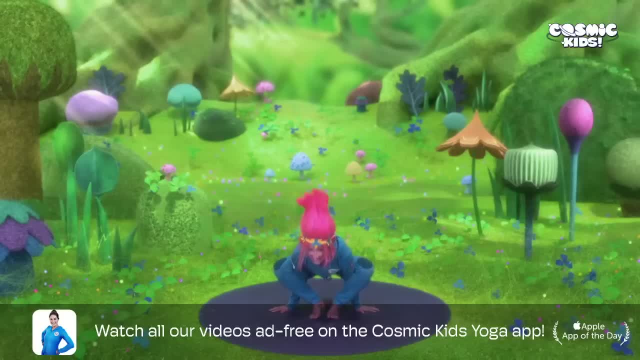 of your feet and walk your feet all the way in Coming into your spider pose. Oh no, but just in the nick of time, who should appear? but Branch the grey troll Using his hair like a warrior to shoo them away, Coming up to stand into our warrior pose One foot forward. 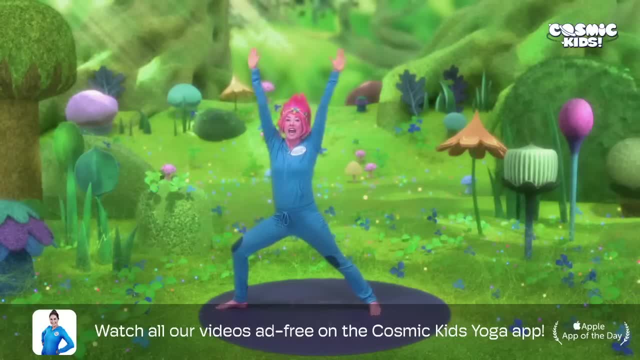 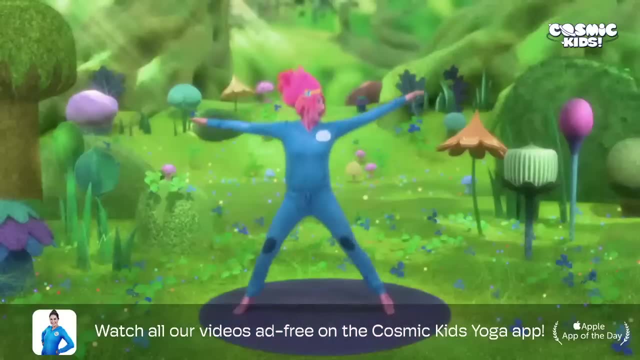 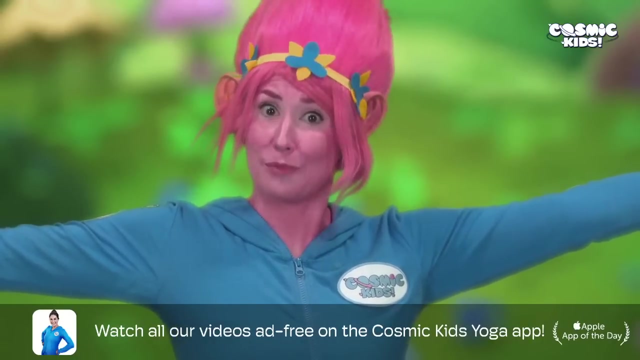 one foot back, Bend your knee, sweep your arms up high and open them wide. Let's shoo those spiders Shoo And jump the other way. Shoo Branch has decided he will help Poppy Together that night. they make a campfire, Sitting on our bottoms with our legs crossed, Bringing our 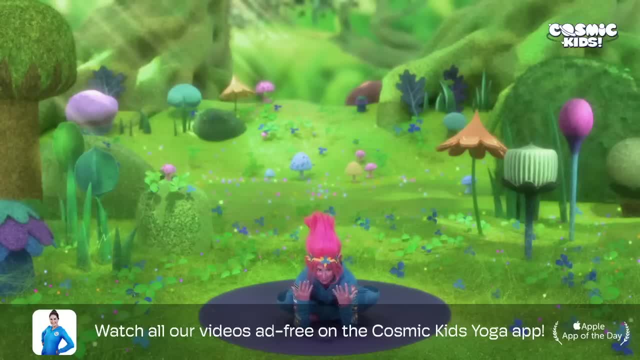 elbows forward and wiggling our fingers like they're the flames of the fire crackling away. It's time to go to sleep, and so Branch and Poppy lie down, Lying down with your legs long and your arms down by your sides. 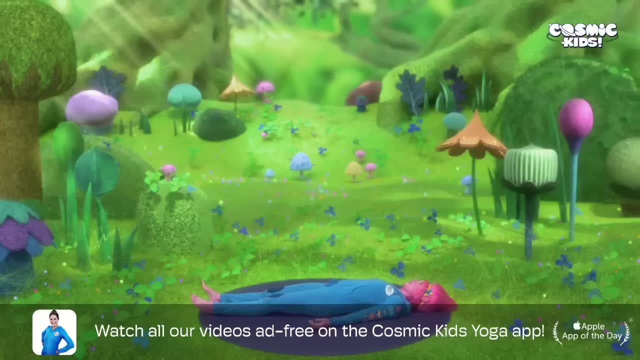 Poppy can't really get to sleep and she looks up at the starlit sky. She sings: stars shining bright above me. Branch rolls over, taking your arms wide, bringing up your knees, taking them over one way and your head over to the other. He looks at Poppy and he goes shh. 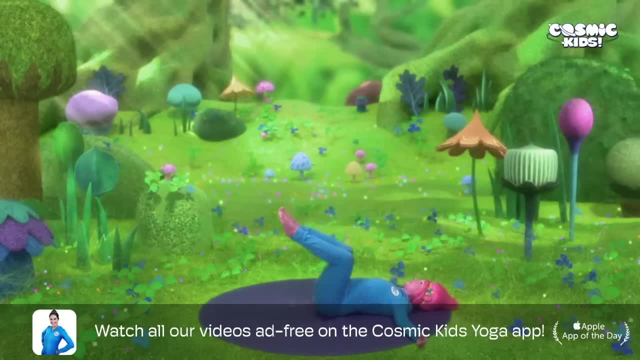 Then he rolls over to the other side, lifting up your knees, going to the other side and along your top row leg, accepting the echo of the anys. Poppy sits up and she takes out a ukelele, Taking hold of your foot, bringing it to your. 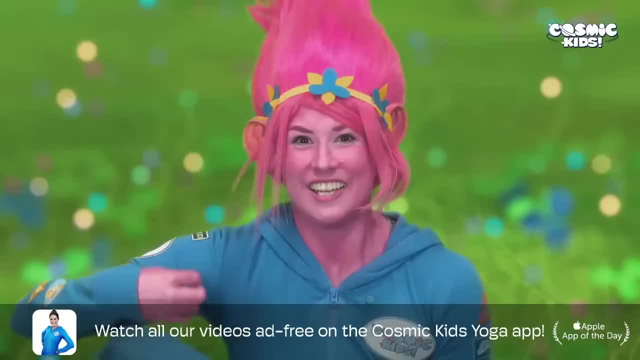 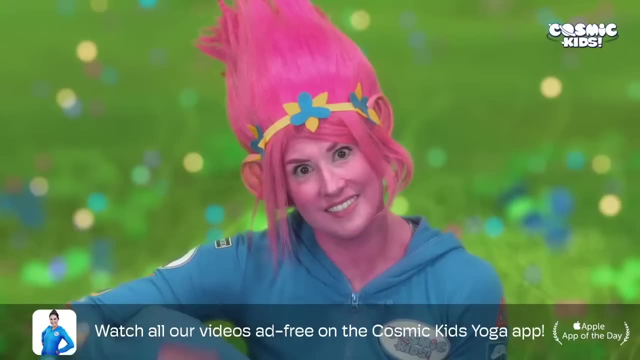 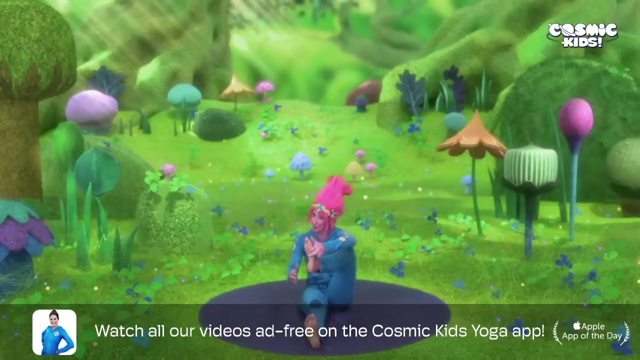 body and, strumming it like a ukelele, She begins to sing to Branch: hello darkness, my old fame. Branch sits up. Poppy put his ukelele down. Branch picks up his ukulele, picking up the other foot, and 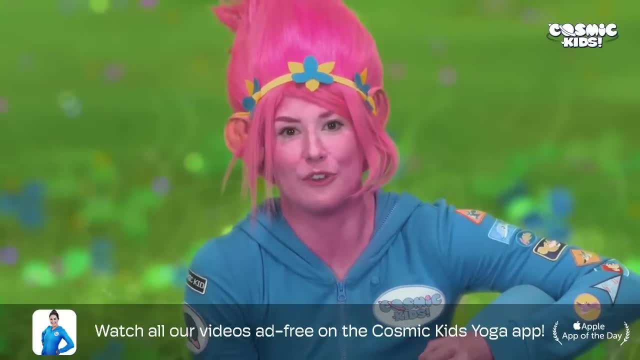 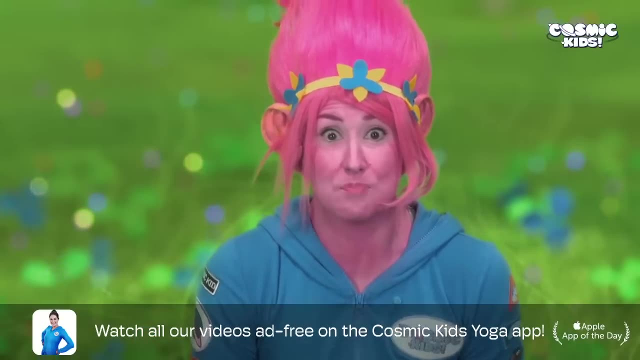 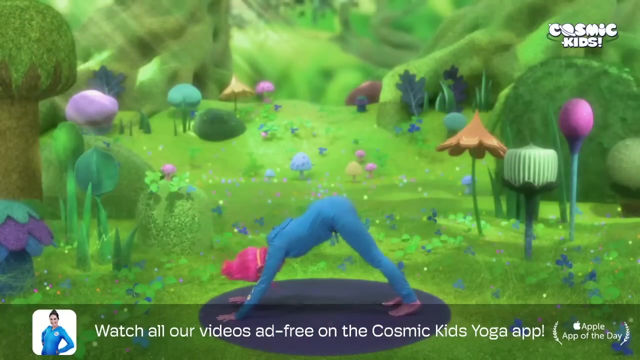 to play it, but before he does, he throws it on the fire. Now, the next day, they arrive at the secret tunnels which take them down to Burgantown. Let's come into our secret tunnel, pose onto our hands and our knees, tuck your toes and lift your bottoms to the 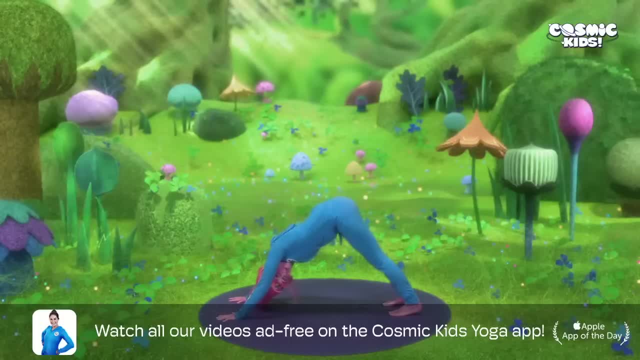 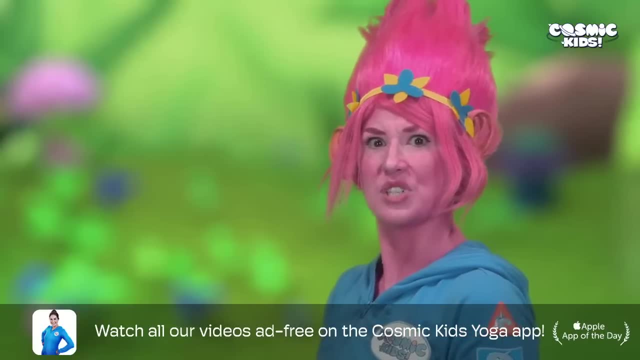 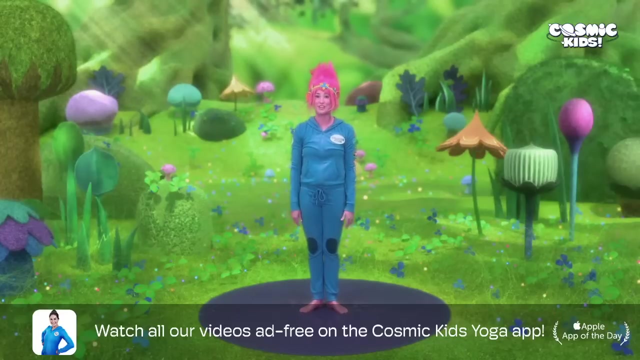 sky. There are so many holes to choose from which one will lead them there, Walking your feet all the way forwards, rolling up to stand, And then Cloud Guy arrives. Coming into Cloud Guy pose, bringing your feet together and turning your toes out to make them a V shape. 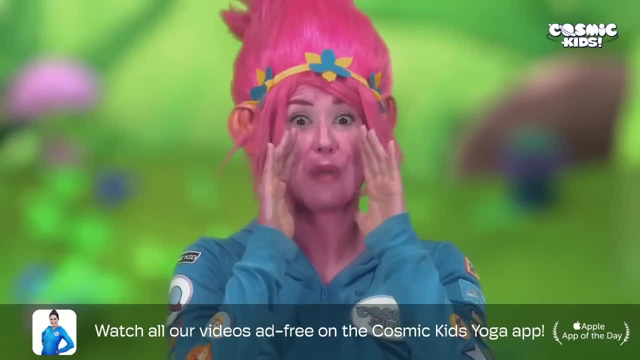 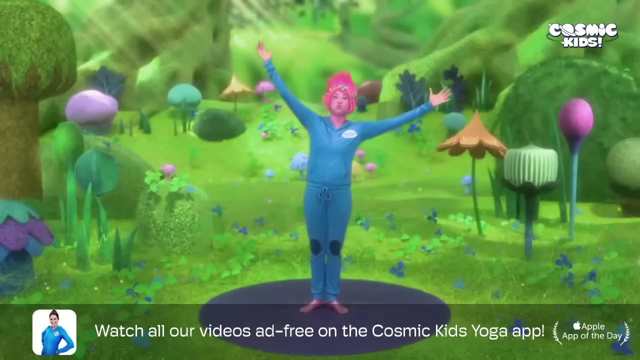 Cupping your hands around your mouth and we're going to do a big blow, to blow up a big puffy, fluffy cloud. Here we go. Cloud Guy tells Poppy and Branch that one of the holes will lead to Burgantown, The other hole will lead to certain death. And then he opens his arms wide and he invites. 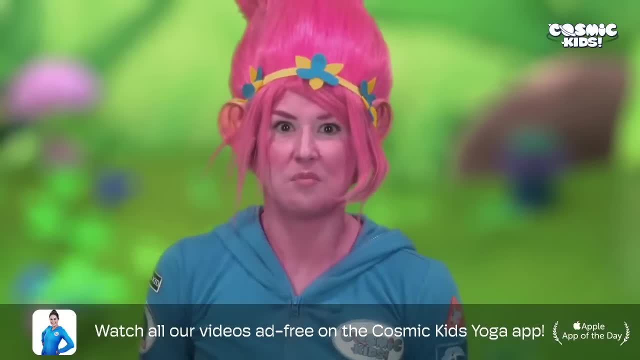 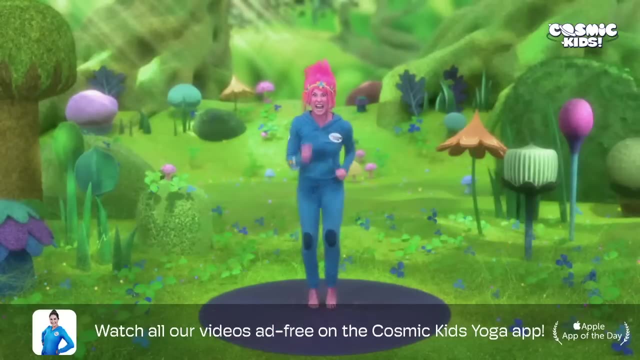 little Branchy Wanchy in for a huggy. wuggy Branch has had enough of hugging and he chases after Cloud Guy Come back. He dives down one of the holes after him, reaching your arms all the way up and folding all the way forwards, following Cloud Guy down the hole. Luckily. 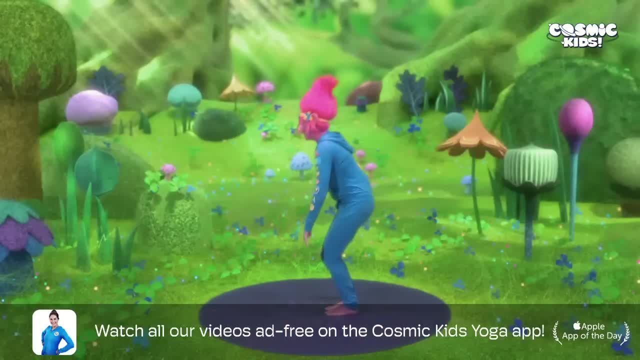 it leads them to Burgantown, Rolling all the way up to stand Now. sitting in the palace is the young Burgant King, King Gristle, Coming into throne: pose Feet hip distance, bend your knees, sweep your arms up by your ears and sit yourself down like you're sitting on a throne. He's with his. 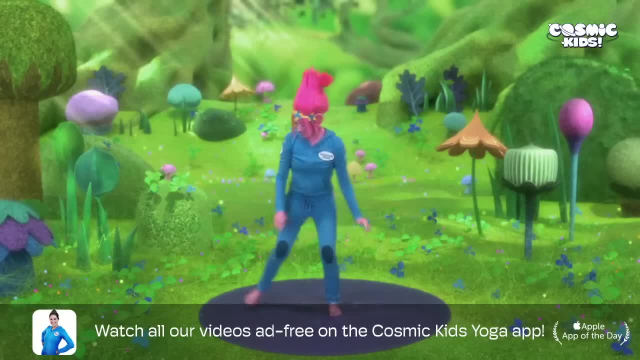 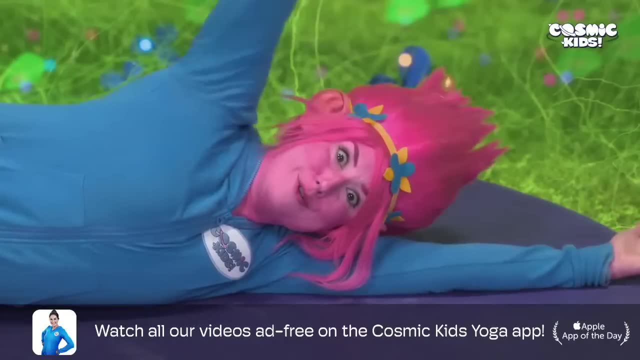 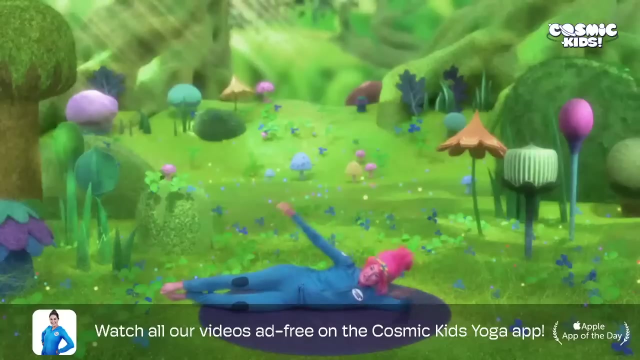 pet crocodile Barnabus Coming into crocodile pose, Lying on our sides, arms long above our heads, and then opening and closing your jaws by lifting and lowering your arms. Very good, everyone In comes. Chef looking very proud and pleased with herself Coming up to stand. she puts: 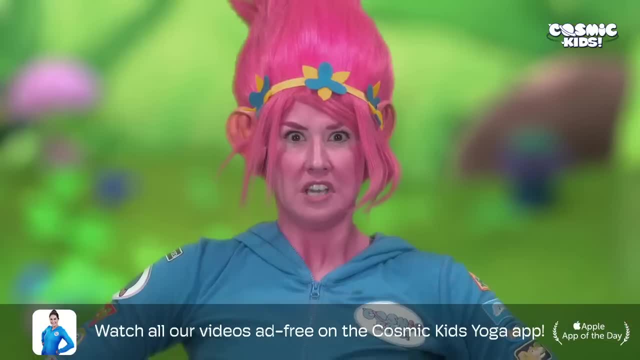 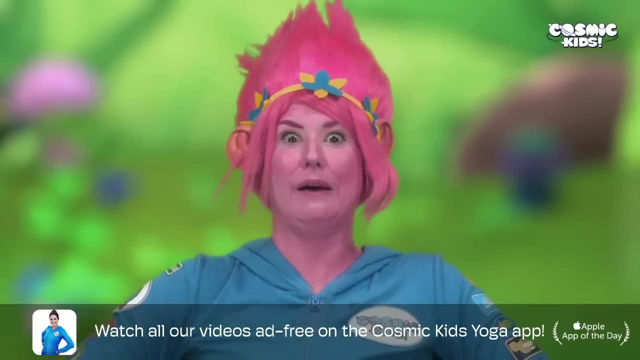 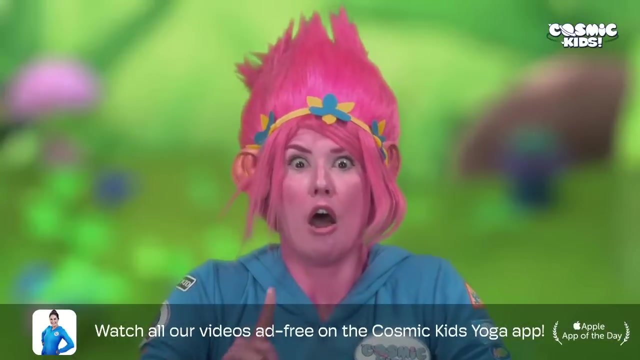 her hands on her hips and she tells King Gristle that she has captured the trolls. and it is time for Trollstice again. Just at that moment, Poppy and Branch tiptoe into the palace, Just in time to see Chef making a sandwich wrap out of their friends. 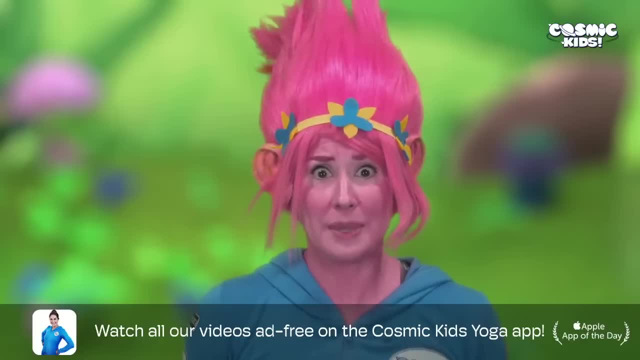 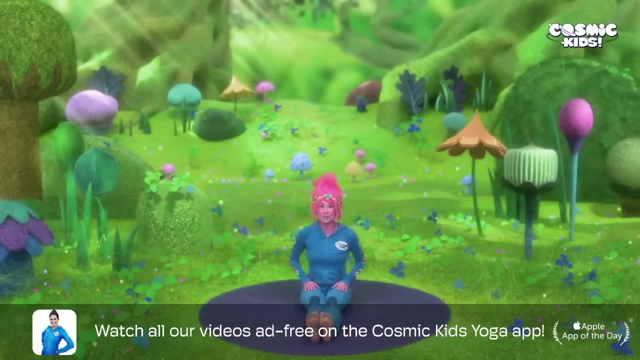 Out of their friend Creak. the Yogi Troll Coming into sandwich pose, Sitting on our bottoms, legs out long Chef, rolls out the wrap. Let's rub our legs. Here we go. Roll out the wrap. Roll out the wrap. She takes her arms wide. She twists one way for Creak. 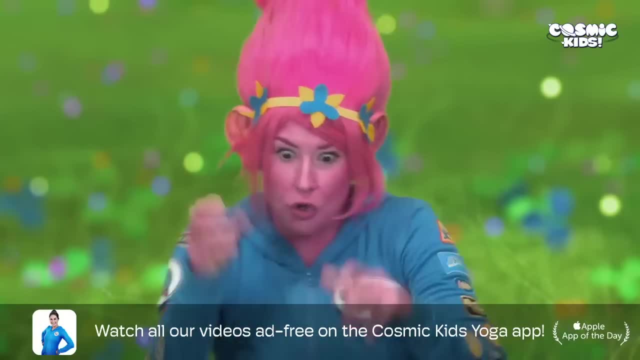 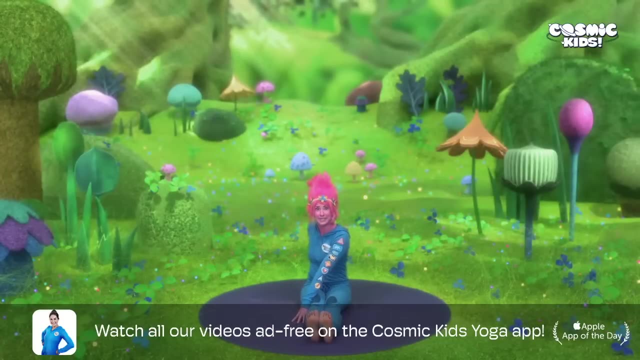 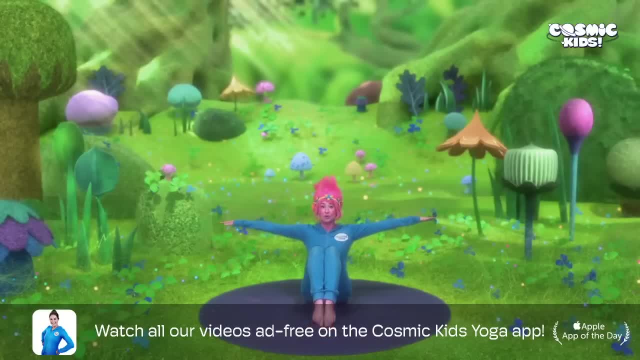 the wrap up Arms wide. Now see if you can bring your knees all the way in Lifting your feet, Hugging them in. She shoves the whole lot into King Gristle's mouth But before he can swallow she slams the door. Coming into door. pose Up onto two knees, Leg to. 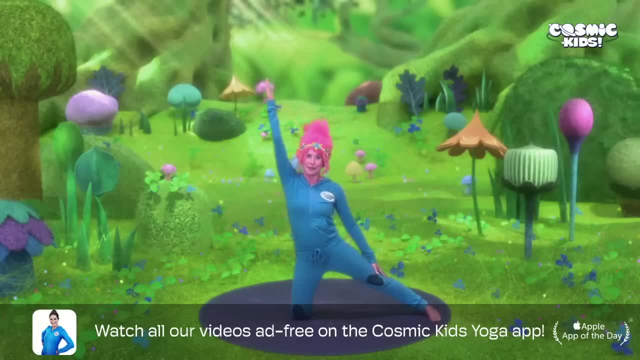 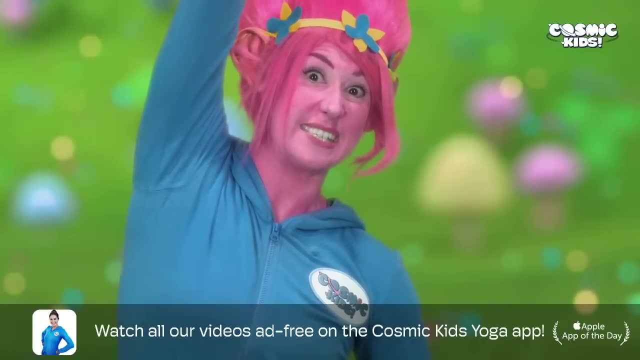 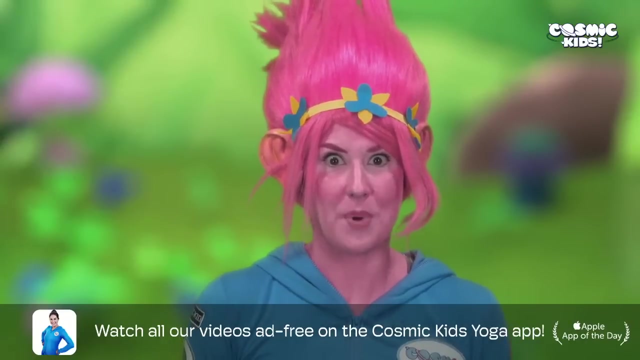 the side Arm to the sky And let's slam it this way: Salaam, Salaam. Poppy feels sure Creak must still be alive, But first she needs to save the others. Coming up to stand, She and Branch jump onto the apron strings of Bridget, the Bergen scullery. 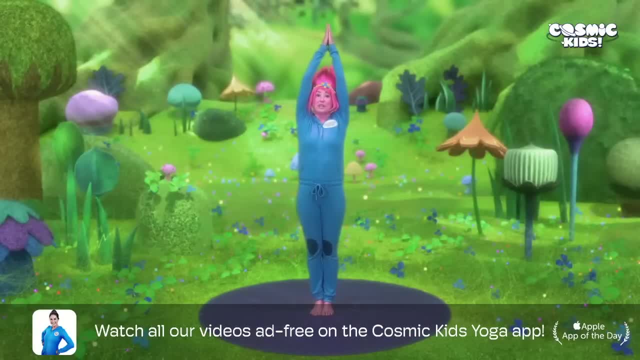 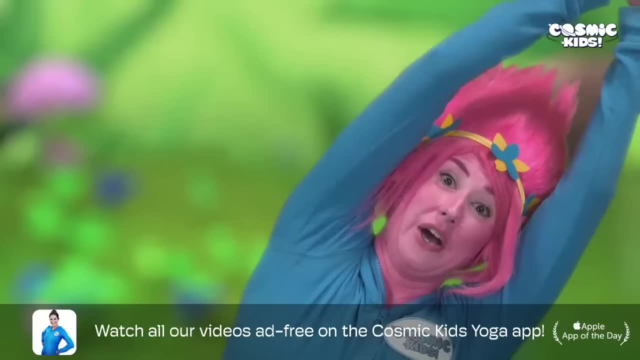 maid, Bringing your feet together, Taking your hands up above your head, Bringing your hands to touch. Now lean over one way, Holding on tight to those apron strings, And lean over the other way, Bridget's taking them into her room to guard the trolls. And when 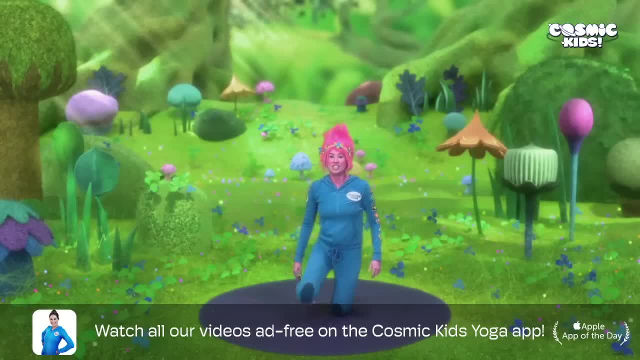 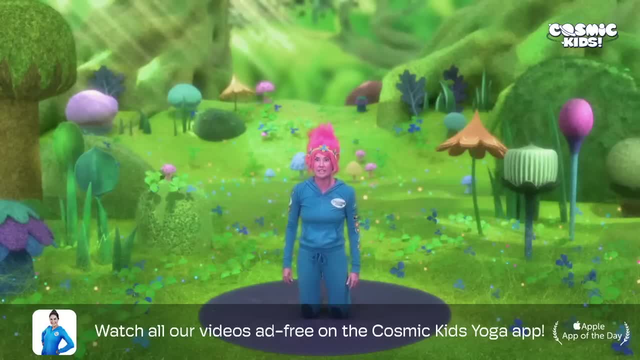 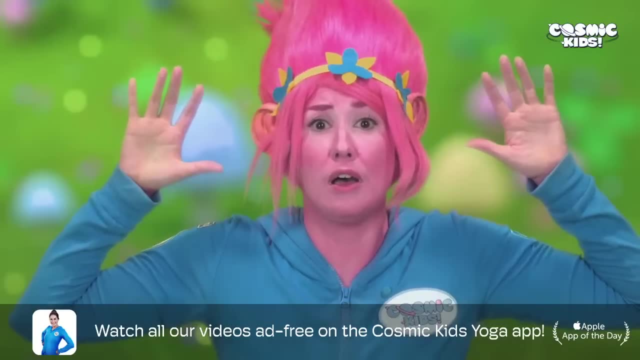 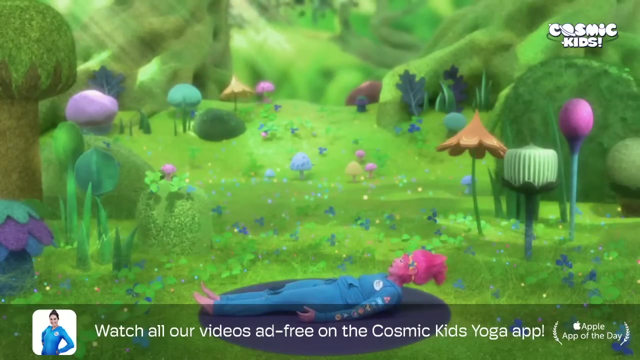 about her secret love of King Gristle, Bringing your hands up- Hello, Is it me you're looking for? And she lies down on her bed, feeling sad, Arms down, Legs down, Crying And sleeping, Opening your eyes, Coming up to sit. 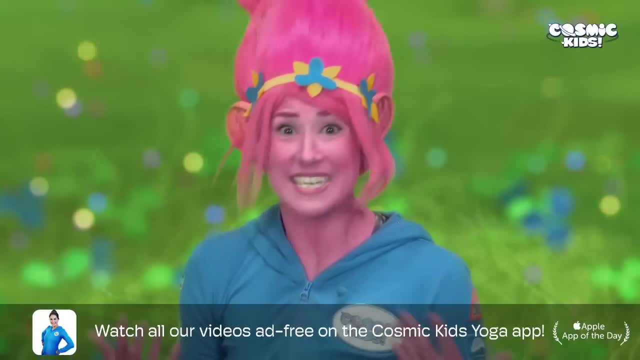 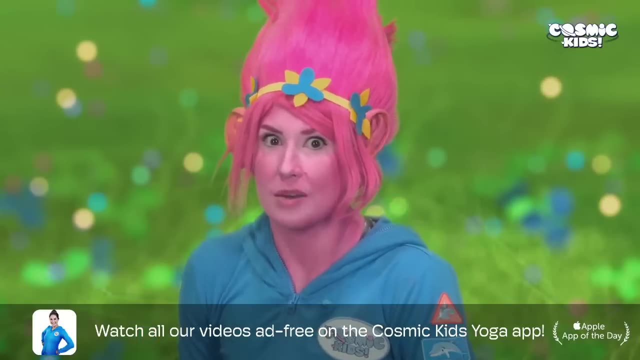 Oh, this is so sweet. Poppy thinks Bridget's in love with King Gristle. Oh, that's the loveliest thing. But she needs to save her friends. So she and Branch climb silently up to where they're kept in the cage. 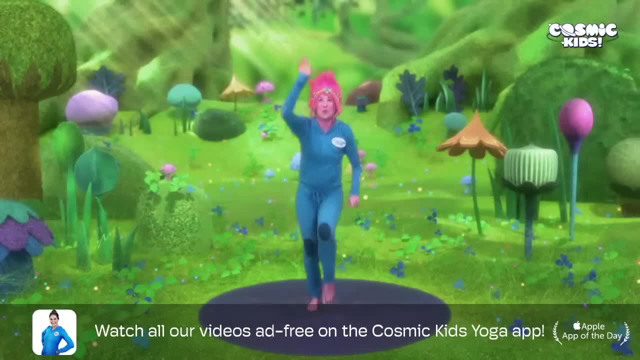 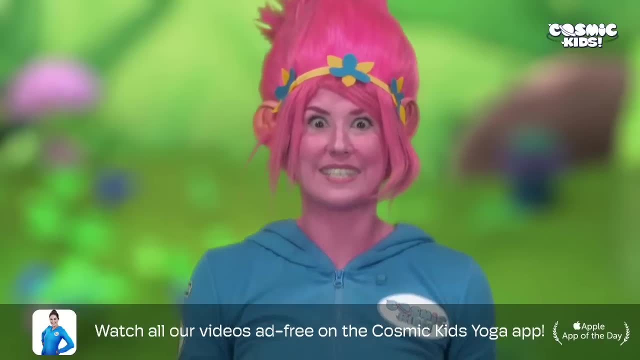 Coming up to stand. let's climb silently Up, we go up, we go up, we up, we up, we go. When they get to the top, the trolls are so happy to see Poppy and Branch. They do a happy dance and they sing about having a party again. 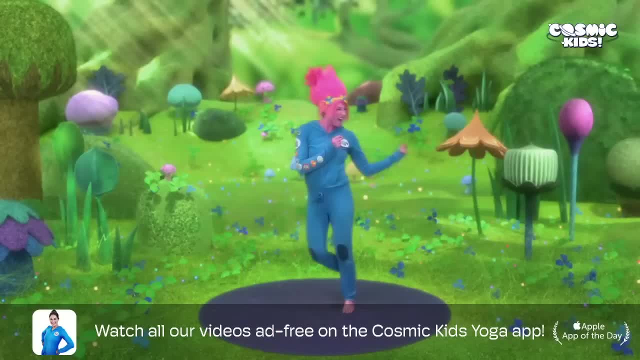 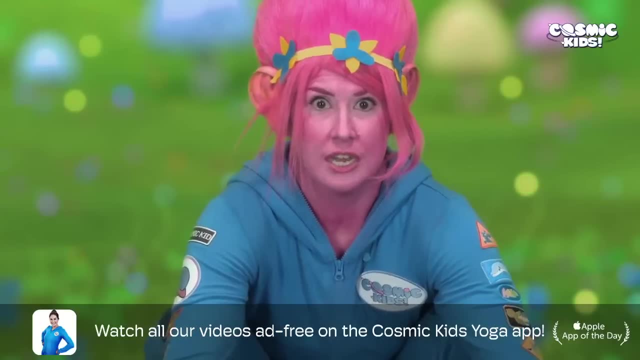 Come on, celebrate good times. come on, But we need to be quiet. so we crouch down and we shh. Now they're free from the cage, it's time to save Creek. But just as they're escaping, Bridget jumps up in star pose. 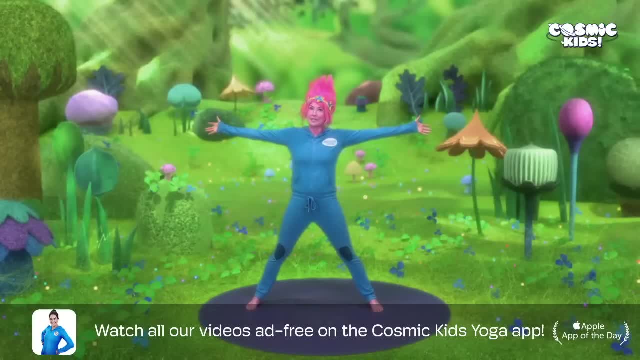 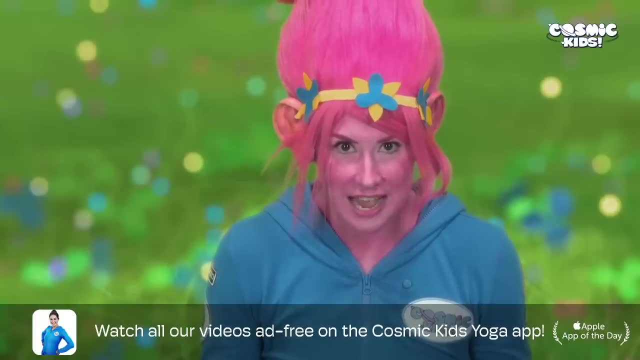 Stop. Poppy needs to make a deal with Bridget and so sits calmly with her legs crossed. She suggests to Bridget that she and the trolls will turn her into a turtle And Bridget will be the total babe, so that she can get a date with the king. 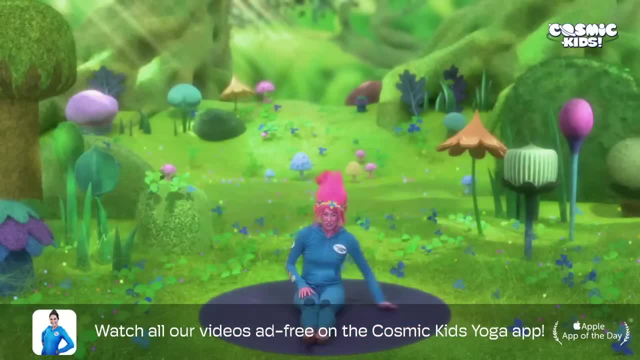 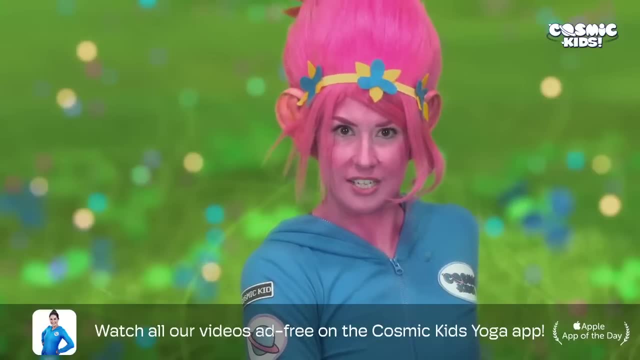 Coming into total babe pose, taking your legs out long, sweeping them round one way, putting your hand on your knee, your other hand behind you, looking over your shoulder back to the front and going ooh la la, Then let's do it on the other side. 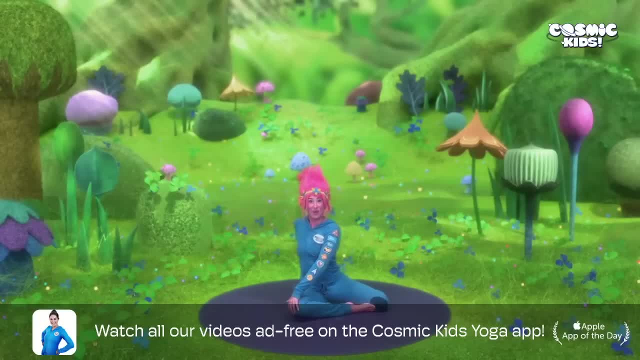 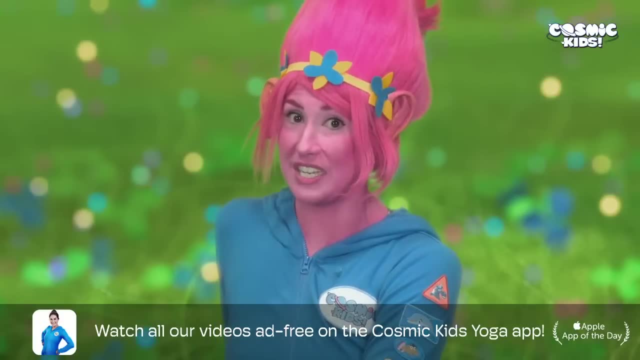 Sweeping your legs round the other way, hand on your knee, hand behind you, looking over your shoulder, looking back to the front and ooh la la. In return, they ask Bridget to help them out And Bridget says no, no, no, no. 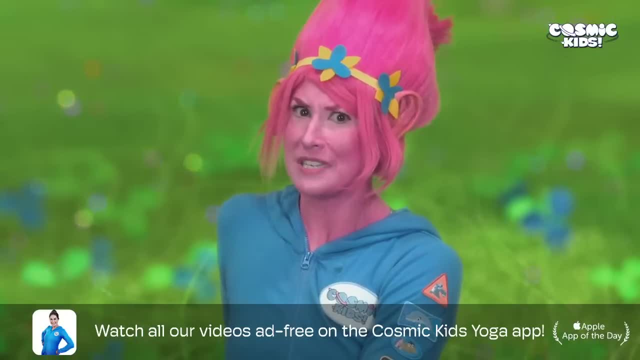 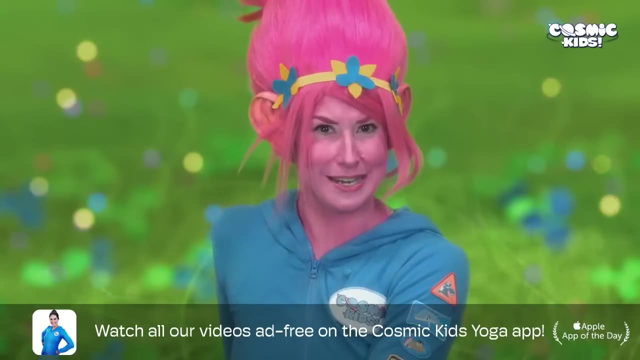 To help them get Creek, the yogi troll, back. After some convincing, Bridget agrees, And so Poppy and the trolls get to work, transforming her into lady glitter sparkles, Coming up to stand everyone. she wiggles into a jumpsuit. 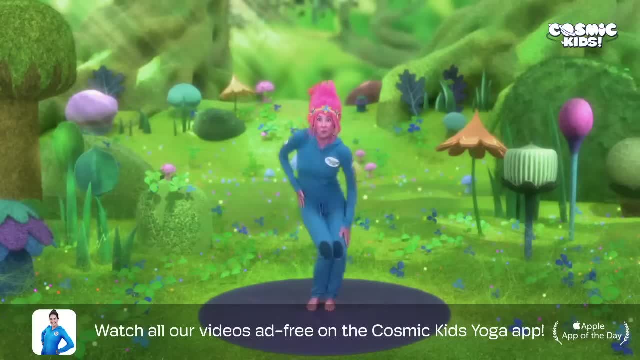 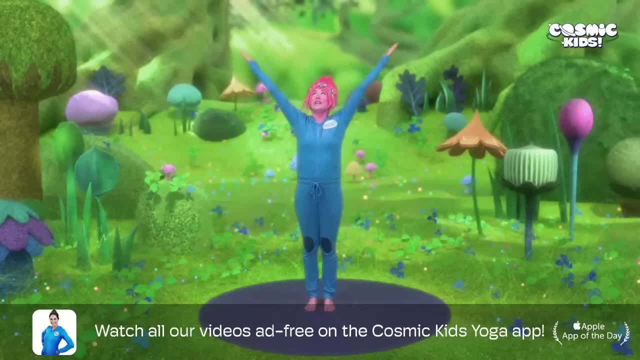 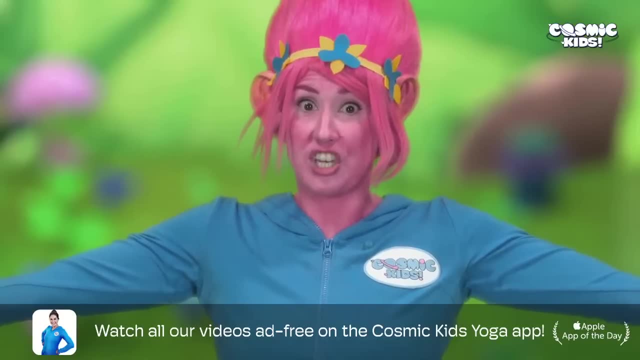 Stretch your arms up high. like your hair's growing very long And they're opening it wide, making that big, beautiful rainbow-coloured hair. From here, the trolls can give Bridget the word she needs, because they're standing on her head. 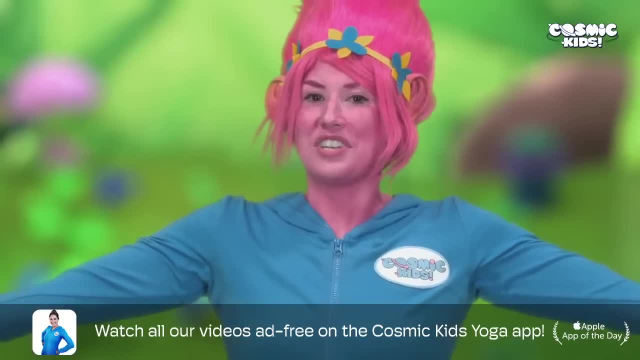 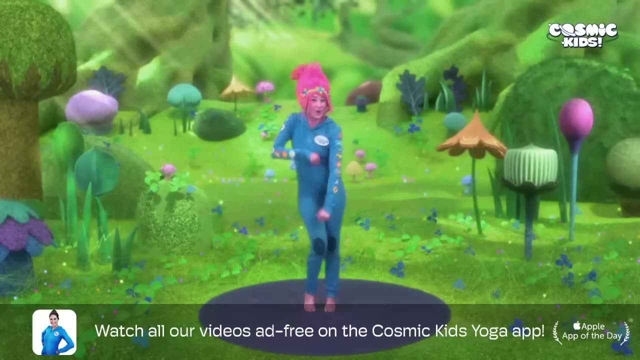 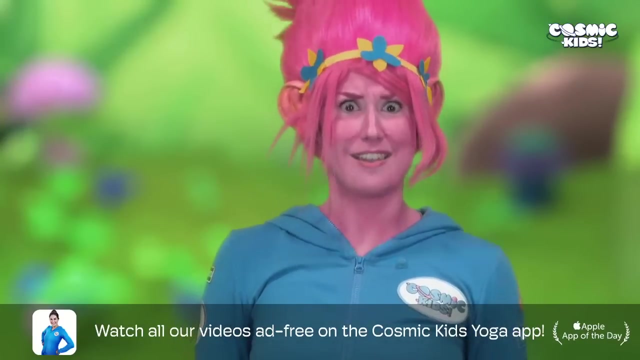 just in case she gets stuck. when she's talking to King Gristle, Bridget steps out feeling rather awesome and confident. I'm coming out. I want the world to know. Got to let it show. When King Gristle sees lady glitter sparkles, he is in love. 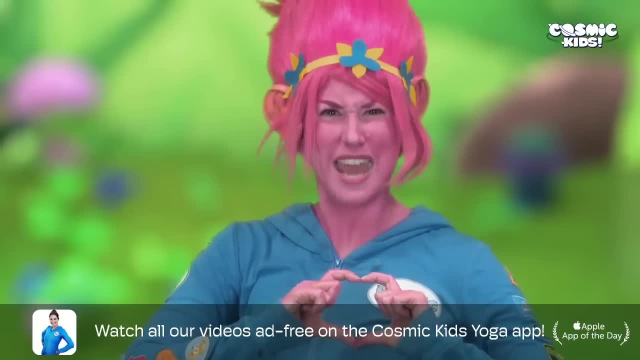 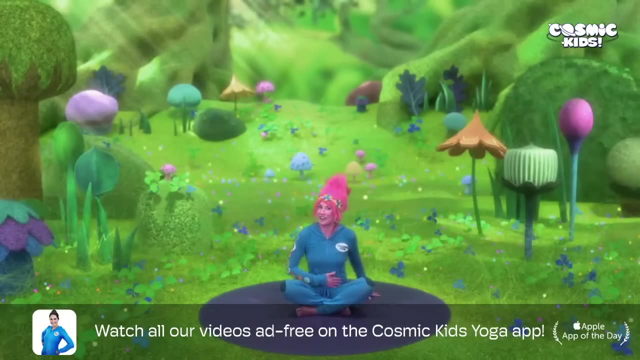 Seeing if you can make a heart shape with your fingers. Oh, yes, Together. they go and eat some pizza Sitting on our bottoms, crossing our legs. we rub a hand on our tummies and we pat our heads at the same time. 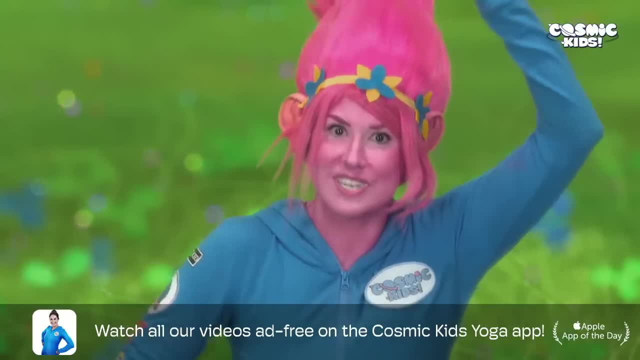 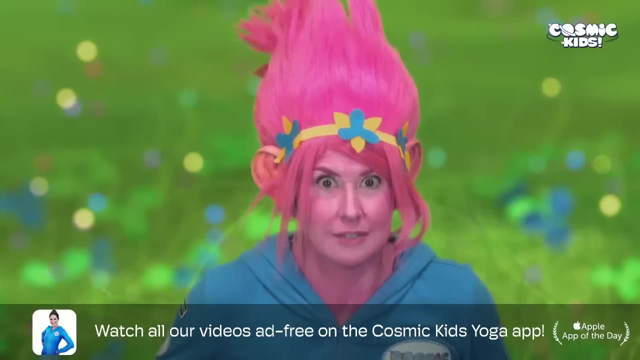 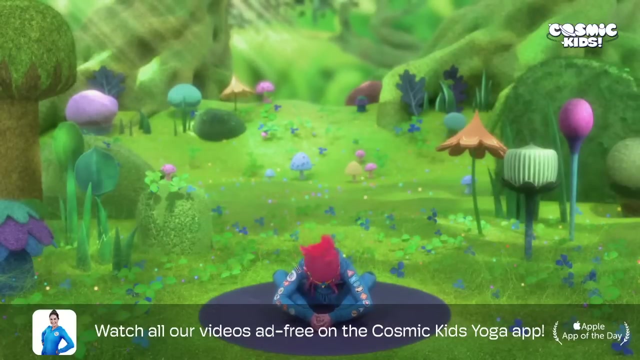 Isn't this amazing. They are happy without eating trolls. King Gristle decides to show lady. glitter sparkles his gem locket. Coming into our gem locket, pose soles of your feet together, holding onto your feet Now, folding your head all the way forwards. 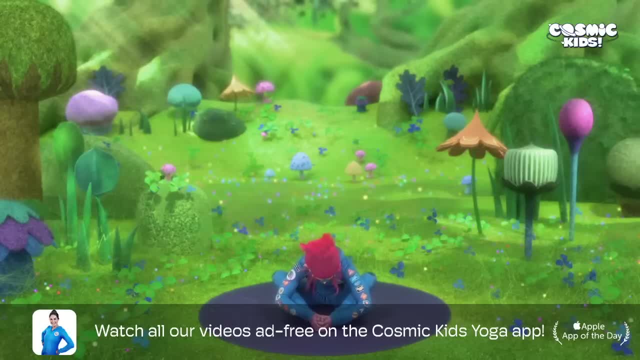 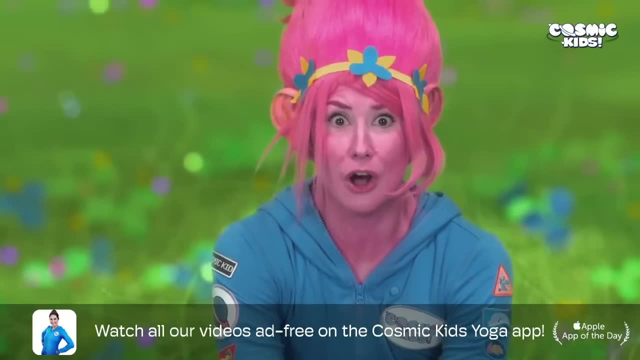 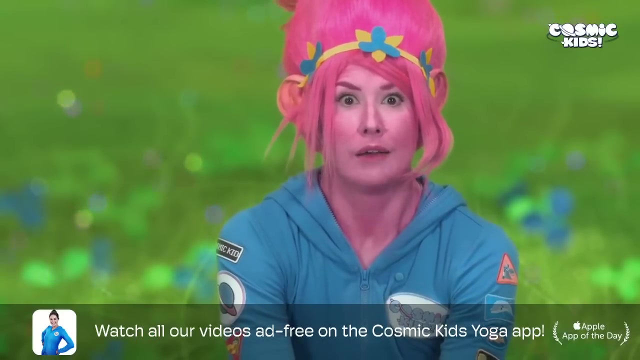 We're going to lift up our head after three to open it up. One, two, three, Whoop. Inside is Creek, the yogi troll. He's alive. Even Mr Dinkles said something. Oh, snap King Gristle asks lady glitter sparkles whether she will be his plus one for Trollstice. 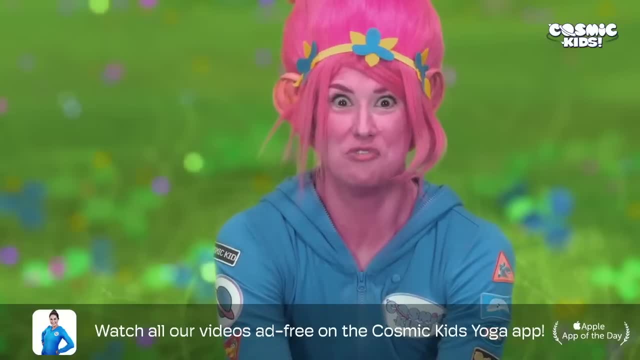 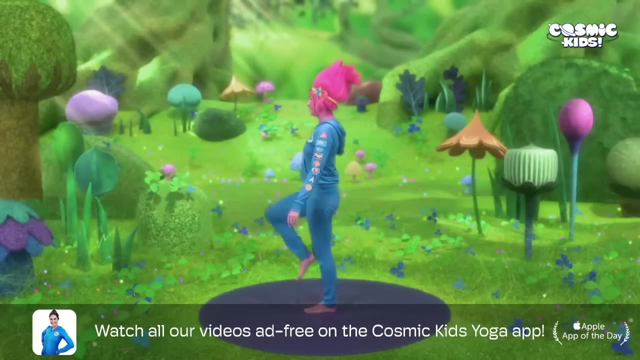 And she says, yes, Now they go roller skating, Coming into roller skating pose: Up to stand, everyone Turning to the side. Now we're going to lift up one of our legs and take our arms wide to take our leg all the way back behind us in our roller skating pose. 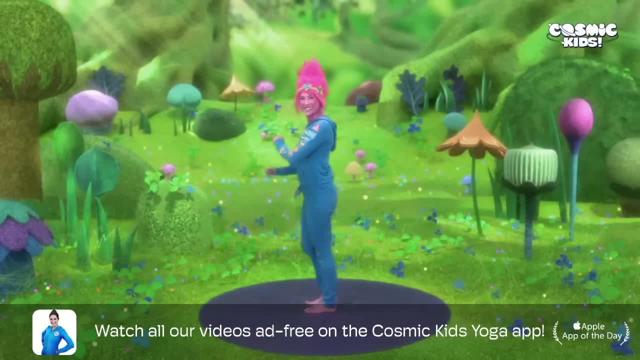 Woohoo, Coming up to stand. Should we try that on the other side? Yes, I think we should. Standing, nice and tall, lifting up one of your legs Now, arms wide, taking it all the way back behind you, nice and strong. 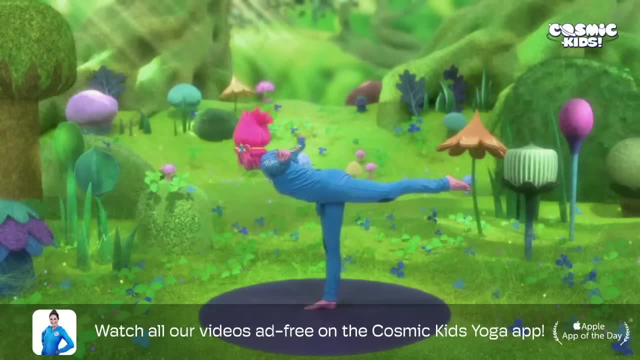 We're roller skating. We're roller skating, Coming up to stand. They're having such a wonderful time. And then Chef arrives. She has her hands on her hips And she folds halfway forwards to get a closer look at lady. glitter, sparkles. 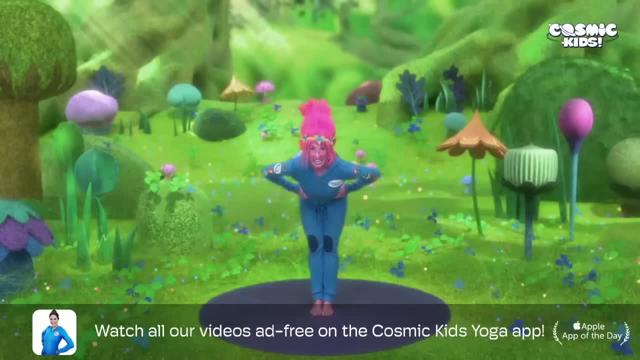 She recognises that it's Bridget And Bridget knows she needs to get out of there. Coming up to stand, Putting one foot forward, one foot back, Bend your knee arms wide. She skates as fast as she can. 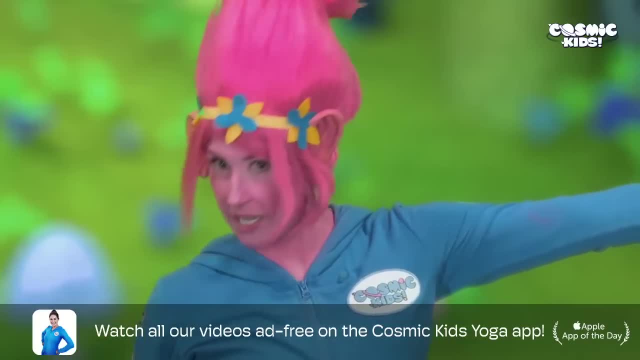 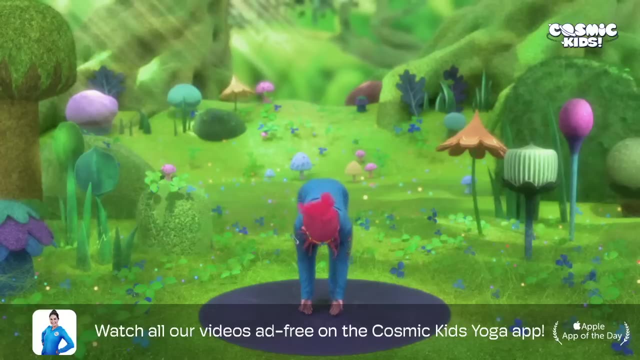 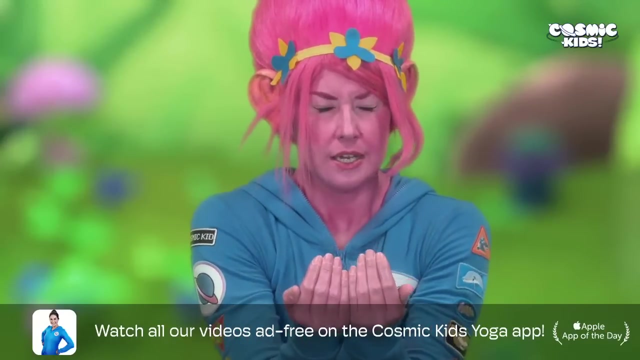 Whoosh. But she leaves a roller skate behind. Coming to stand, King Gristle is delighted. Folding all the way forwards, He scoops up the precious roller skate. Will she be his Cinderella and come to Trollstice? He hopes so. 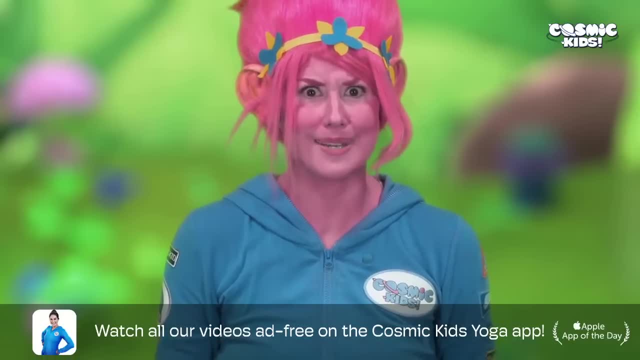 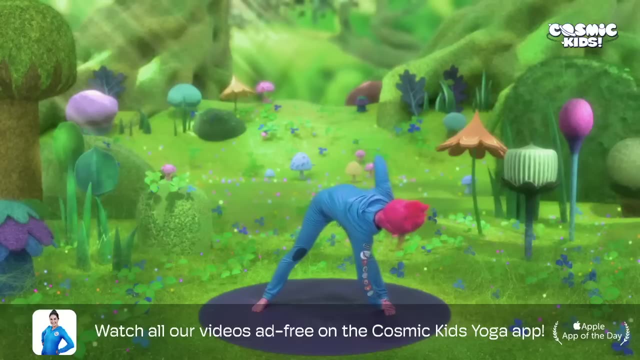 He decides he needs to get fit, And so he starts exercising. Jump your feet wide, Take your arms wide. Let's do some windmill pose. Take your hand across to your opposite foot And reach your top arm up to the sky. 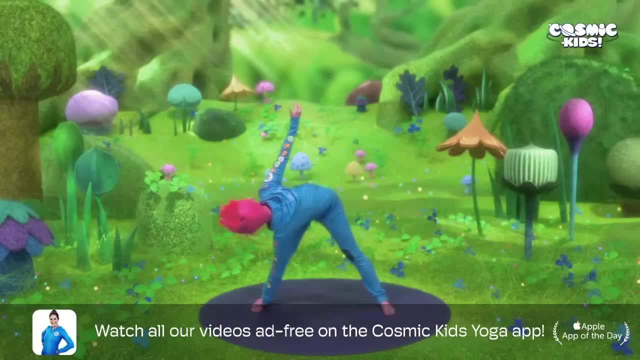 Now let's switch sides. Take the other hand across and your other arm to the sky. Now let's see if we can do eight switching sides. Here we go, And one And two, And three, And four, And five And six. 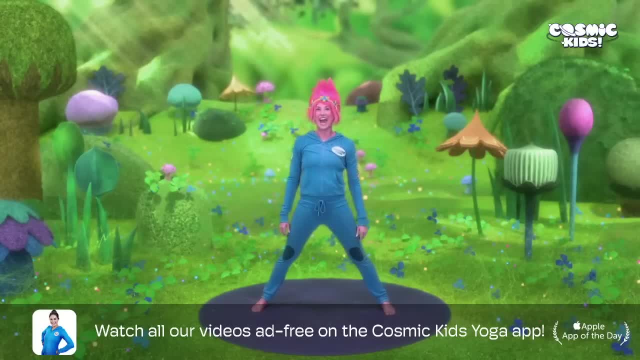 And seven And eight Rolling up to stand. This is their moment. The trolls wiggle in under the rug, Coming onto your tummies. everyone Hands underneath your shoulders And let's wiggle, wiggle, wiggle, wiggle under the rug. 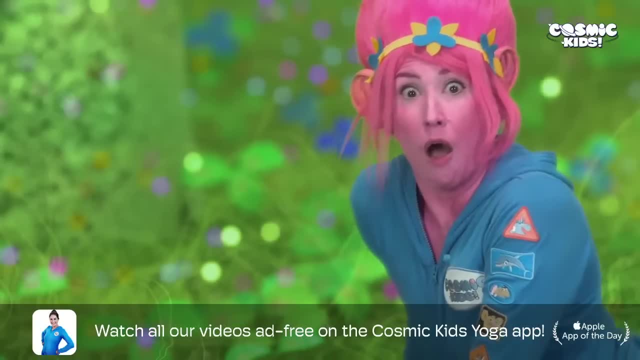 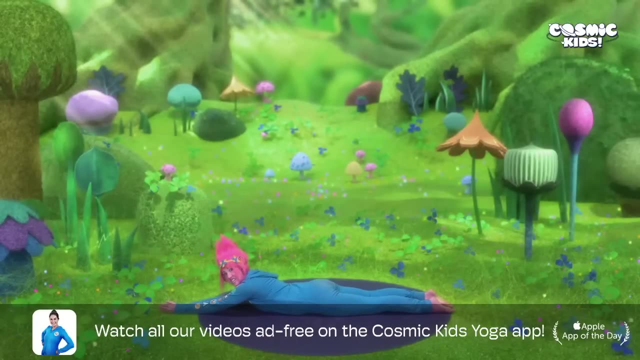 They're looking for the gem locket with creak inside. There it is Lying all the way down, Reaching forward with your arms to grab it. They've got it, But just as they do, Barnabus the crocodile sees them. 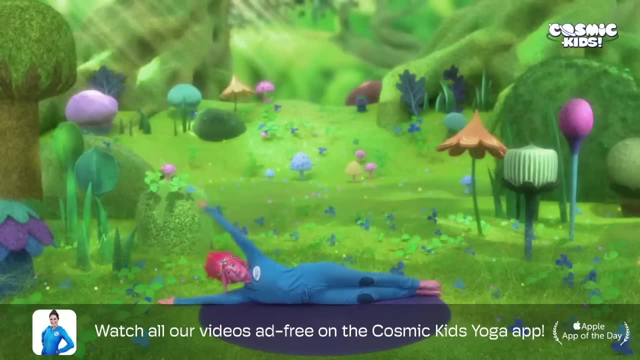 Rolling onto your side And opening and closing your crocodile jaw. Oh no, He's chasing them. The trolls jump on the roller skate Sitting up Legs out long, And they drive it out of there Holding onto the laces. 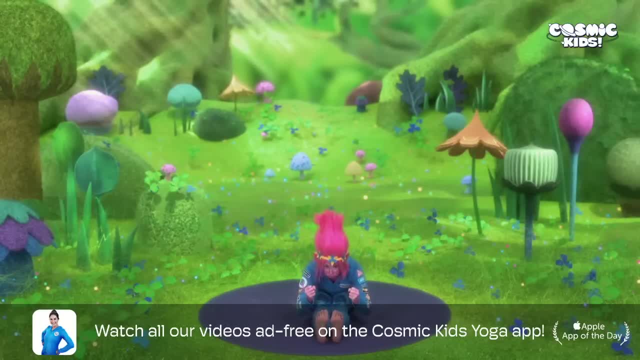 They go forwards really fast. Then they sit up really tall And Guy Diamond, the wonderful glitter troll, twists to the side And he blows Barnabus with his glitter, And the other side, Turning to the other side, Blows some more glitter. 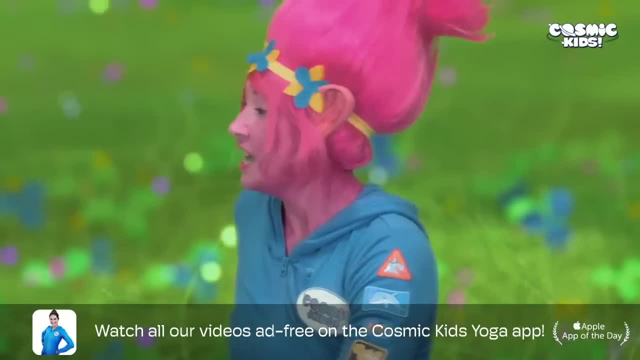 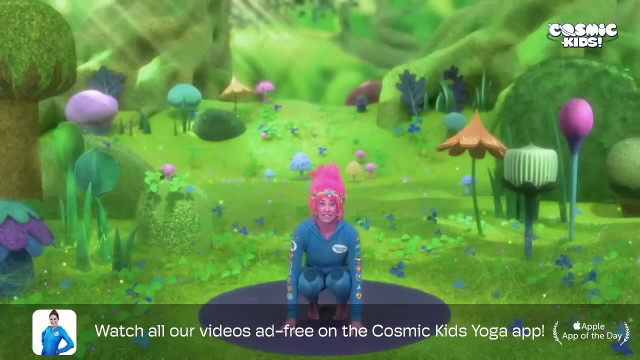 They think they've got away. But then the locket flies up into the air, Coming up onto our tiptoes, Coming up onto our tiptoes, everyone. After three, let's jump in the air, like with a locket One. 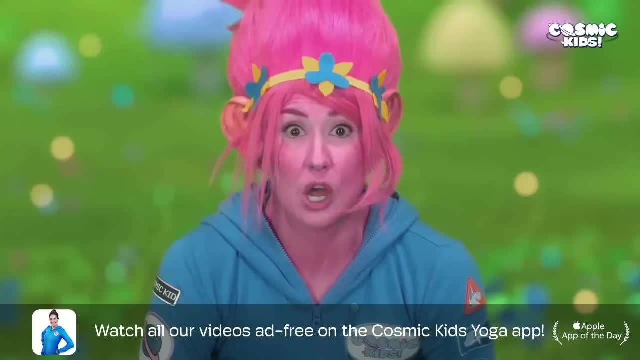 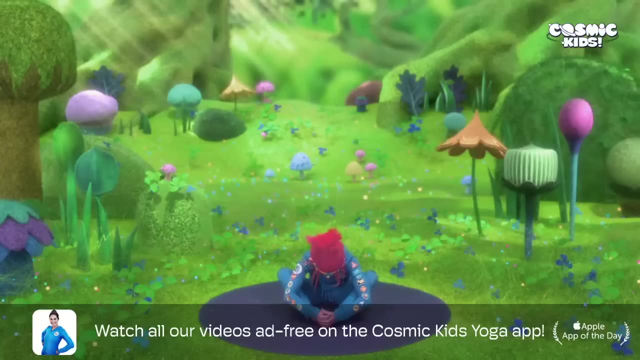 Two, Three, Whee, It pops open, Sitting on our bottoms, Soles of the feet together, Bringing your head all the way forwards After three, Lifting it up. One, Two, Three, Whoop, But Creek isn't there. 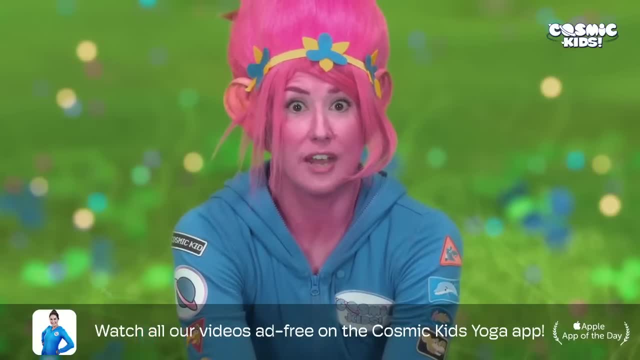 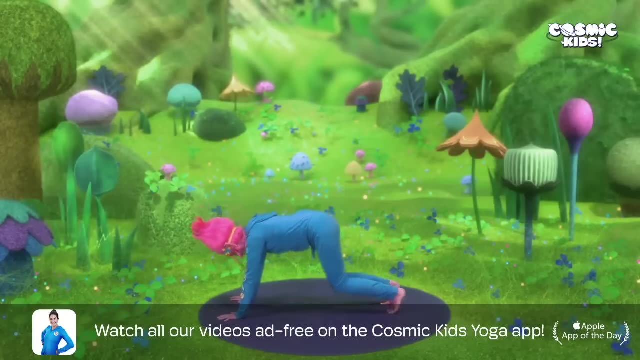 He's disappeared. Just at that moment, Chef arrives And she puts down a cage on top of them all, Coming onto our hands and our knees, Tucking our toes And lifting our bottoms to the sky. But who's this appearing, Walking your feet all the way forwards? 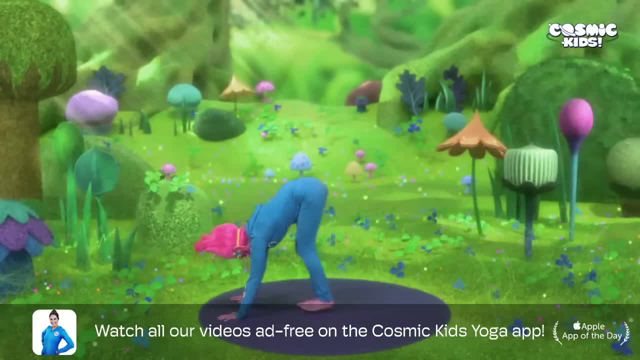 Rolling up to stand. It's Creek The yogi troll. He's sold them out. He's agreed that he will ring Poppy's cowbell three times And lead Chef to where all the other trolls are hiding. Take your feet wide. 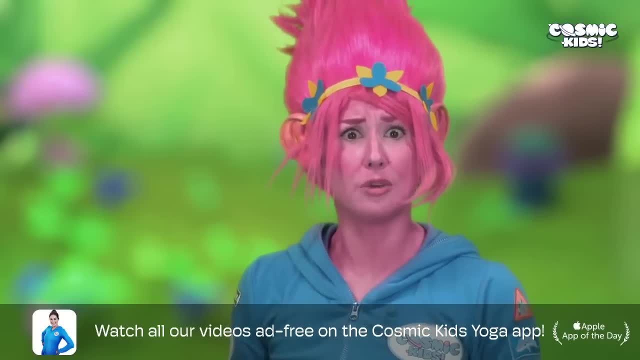 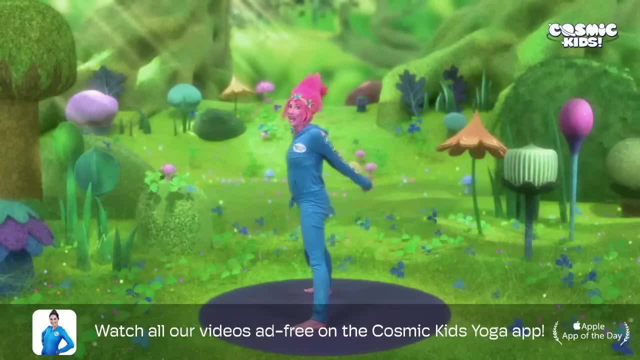 Four, Four, Four Three Two. One Two, Three Ding And up. One Two, Three Ding And up. Last time, One Two, Three, Ding And up. This is so. there'll be enough trolls for Trollstice. 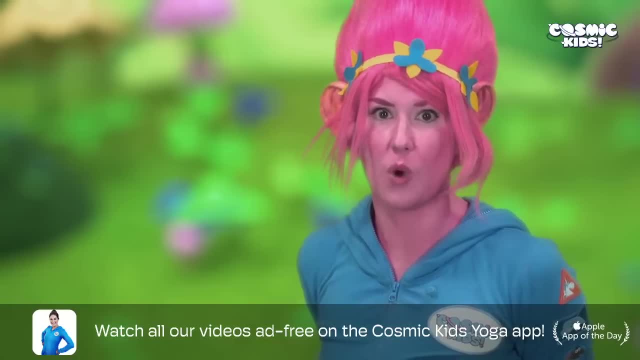 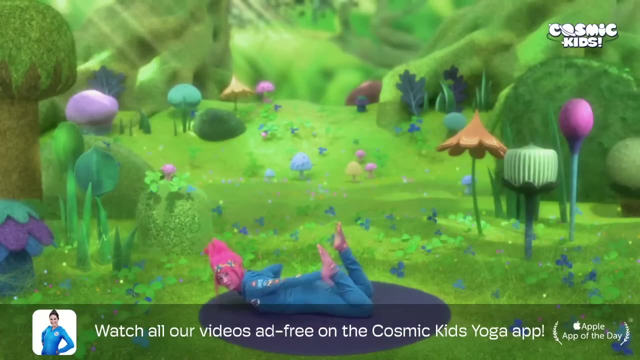 Come the day of Trollstice, Chef puts all the trolls into one ginormous pot. Coming into pot pose, Lying on our tummies, everyone, bring your feet towards your bottom, Reach round to grab your ankles and kick your feet into your hands, lifting yourself up into your pop pose. 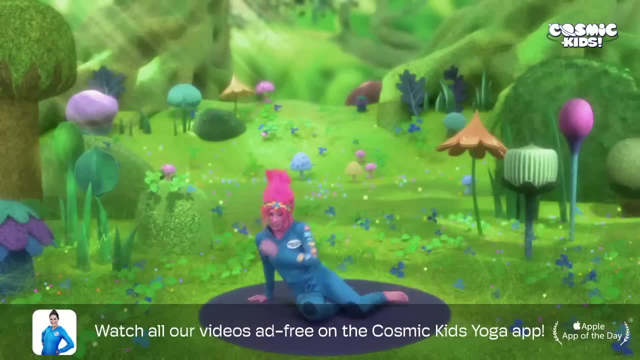 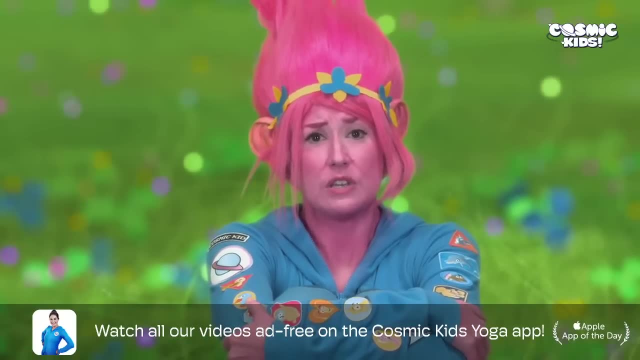 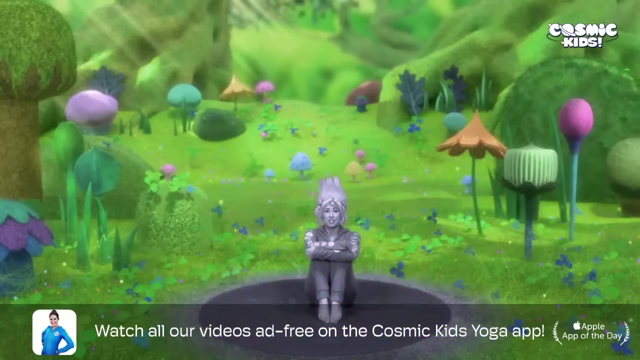 Poppy's feeling sad. Sitting up, she hugs her knees. She feels like she's let everyone down. She feels like she's let everyone down and all of the positivity and hope leaves her. Her colour drains away and she is left grey. 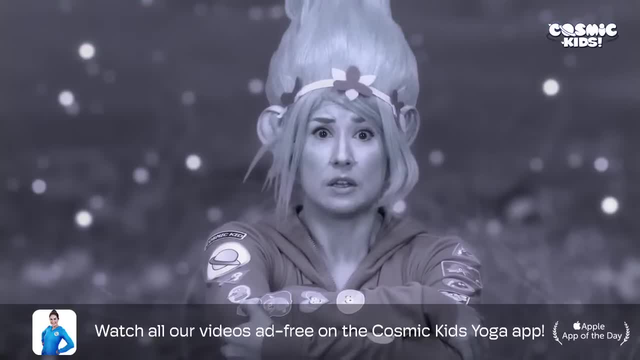 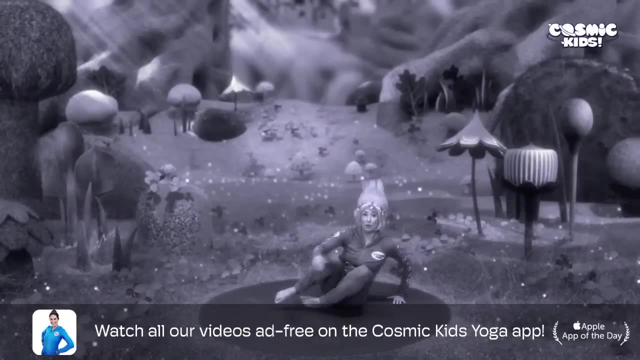 It then drains away from all the other trolls. Then, for the first time since losing his grandma, Branch comes forwards, Coming up onto our knees, everyone. He sings to Poppy. He tells her that he thinks her true colours are beautiful like a rainbow. 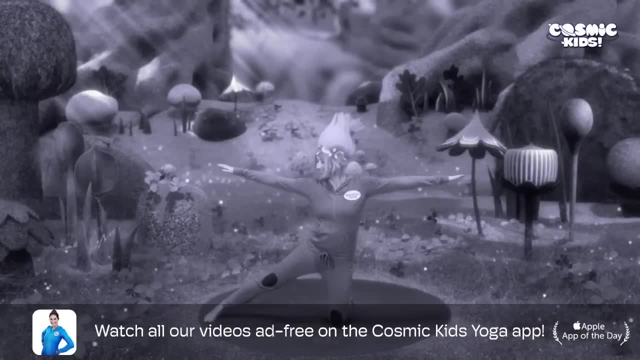 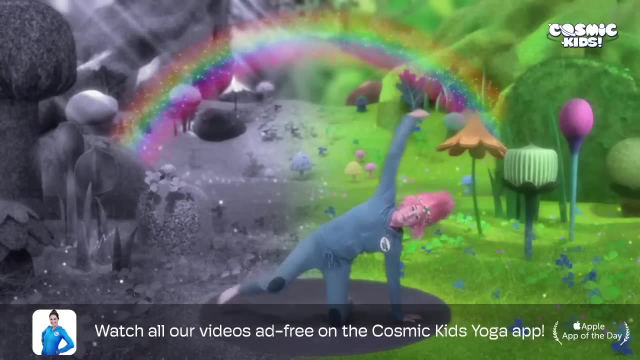 Let's do our rainbow pose. Arms wide leg to the side, drop down onto one hand and sweep your arm up and over your ear, making your big beautiful Coming to two knees again. arms wide leg to the side, drop down onto one side and sweep your rainbow up the other way. 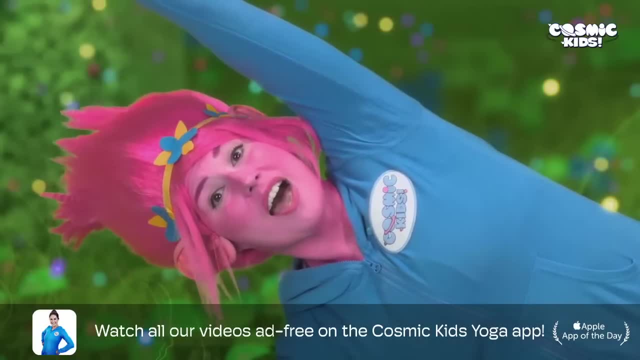 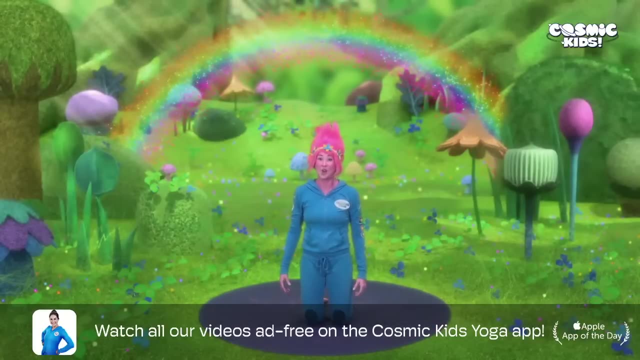 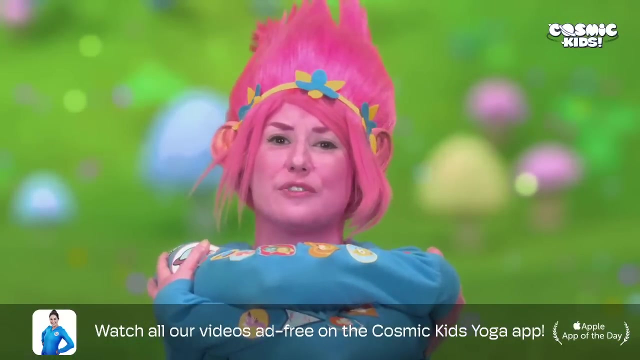 He sings to Poppy And that's why I love you. Poppy comes up Hearing this, hearing this hope again brings hope flooding back to her and she and Branch open their arms wide and share a big, wonderful hug. All of the colour comes back to the rest of the trolls. 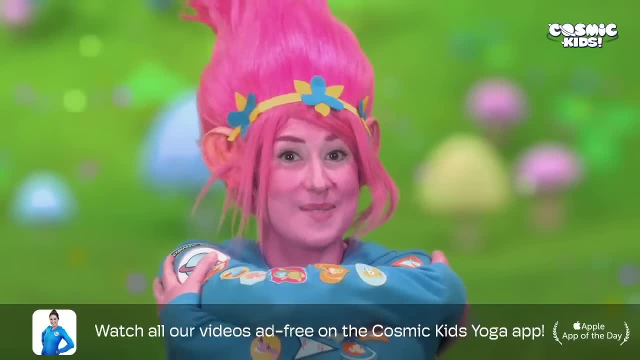 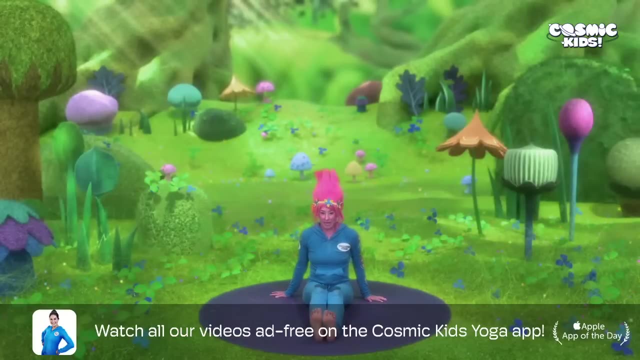 And to Branch, who isn't grey but is blue. Now the lid of the pot gets opened. Sitting on your bottoms, legs out long, bending our knees, touching our toes- After three, let's lift our arms up to open the pot. 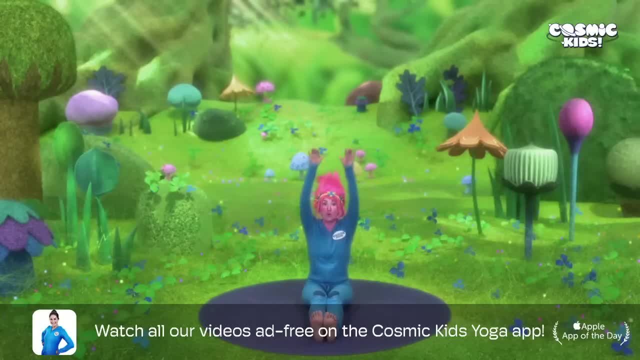 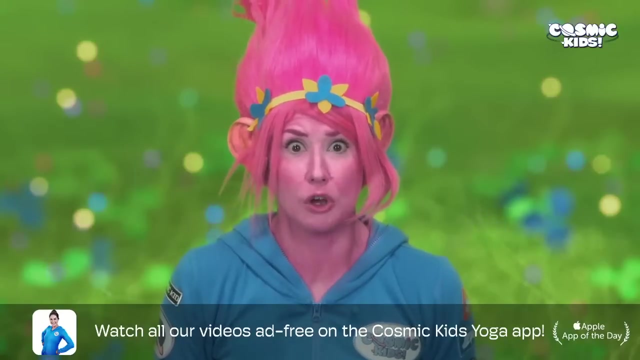 One, two, three. It's Bridget. She's letting them all escape. She wants to thank Poppy for helping her find true happiness. But now Bridget is in some serious trouble For letting the trolls escape Coming up to stand. 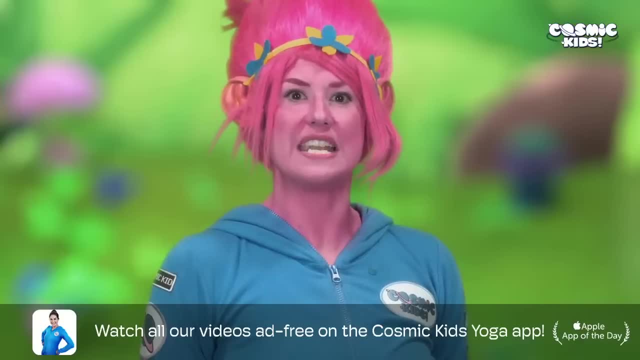 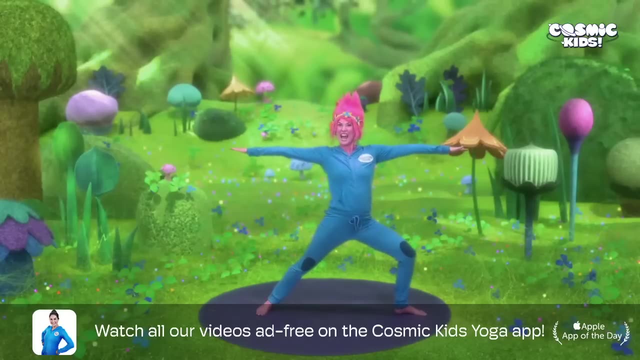 One foot forward, one foot back. Poppy's not going to leave Bridget. Nor are the other trolls, And they whoosh in on the roller skate to save her. Sweep your arms up, bend your knee and let's whoosh. 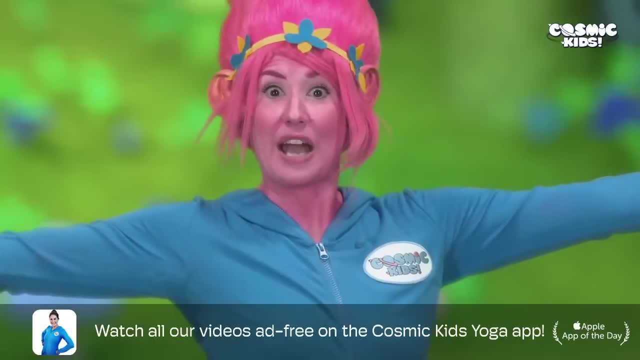 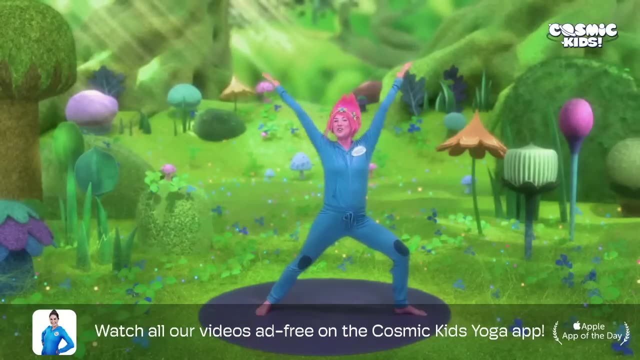 Whoosh, They jump back on Bridget's head, turning her back into Lady Glitter Sparkles. Hands together above your head, Sweep your arms up And open them wide. King Gristle is delighted And stands in star pose. 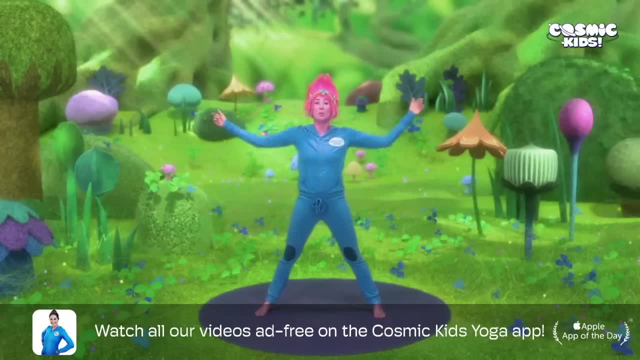 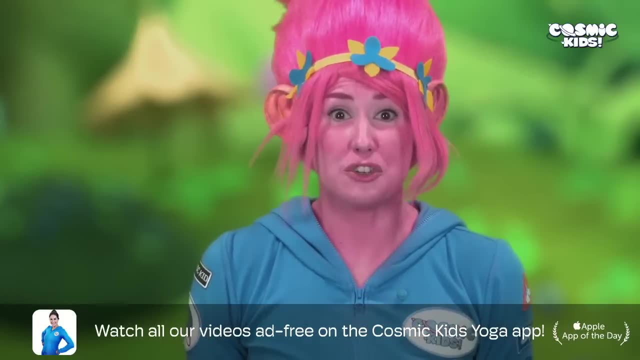 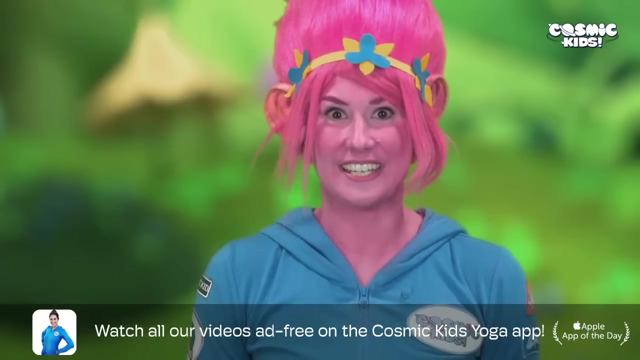 To protect his Lady. Glitter Sparkles Poppy steps forwards, She reveals herself And she explains. You don't need to eat trolls to find happiness. It's in each and every one of us. We just need to find it. Look at King Gristle and Bridget. 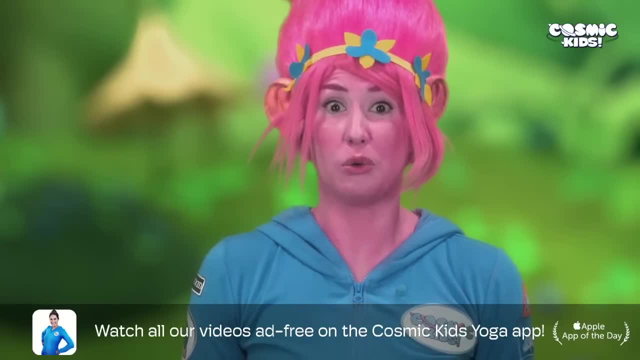 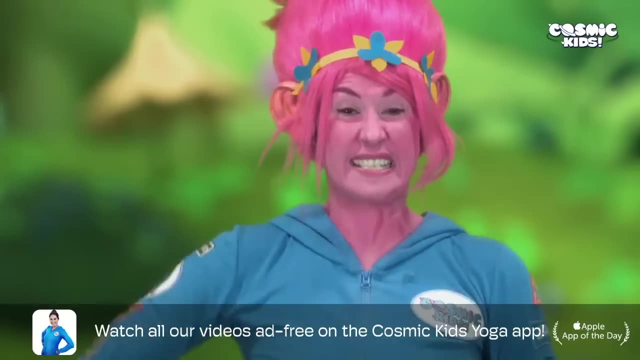 They had a lovely time And they didn't eat any trolls. The Bergens start to realise that this is true And they banish the chef Once again, Sending her out of the palace Rolling down the hill In a burning hot pot. 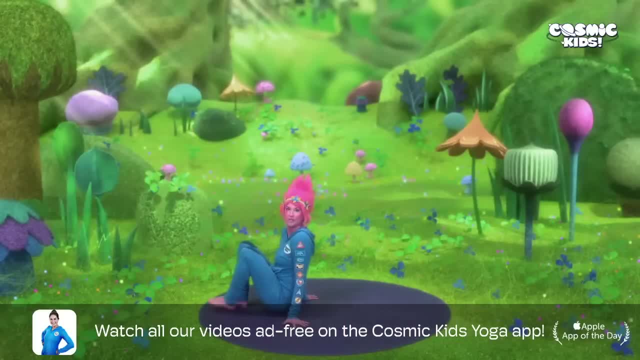 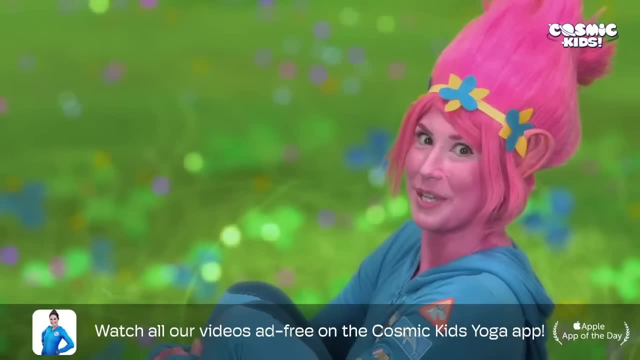 Coming into our roly poly burning hot pot pose Sitting on our bottoms, Hugging our knees. Now we're going to tuck our chin And rock all the way back and all the way up. After three, One, two, three. 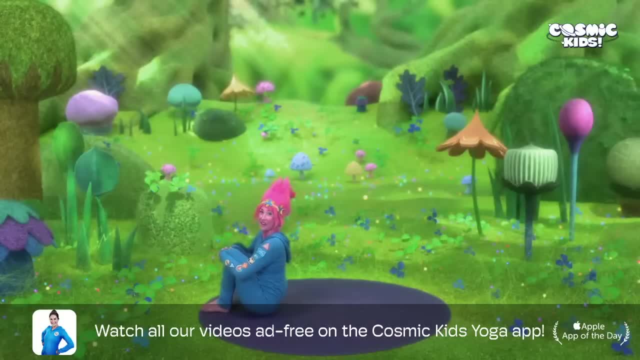 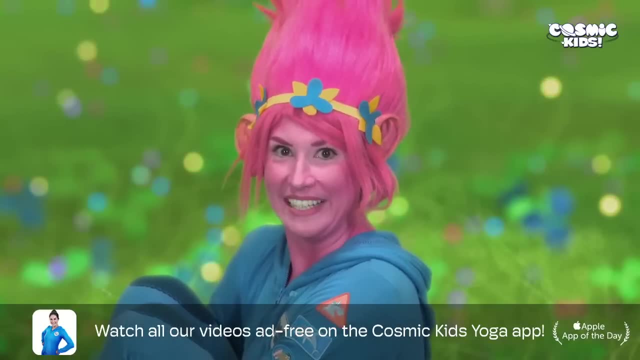 Whoop Whee. One, two, three. Whoop Whee. Now, this last time. Can we rock all the way back? Can we rock all the way up to stand? Let's try Ready. One, two, three. 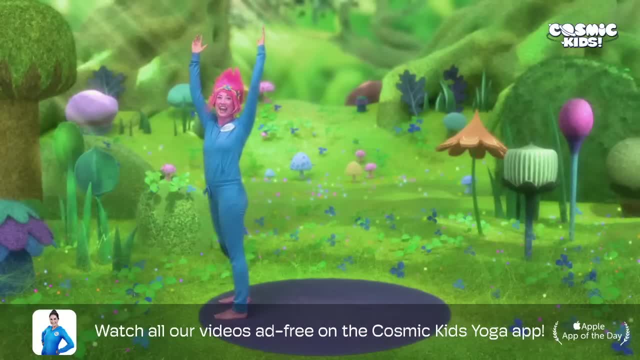 Whoop, Kick your legs And up we go. Yay, From that day on, Bergentown blooms again. Bringing your hands together, Grow your arms up, nice and tall, And open your arms, Spreading beautiful rainbow colours all over. 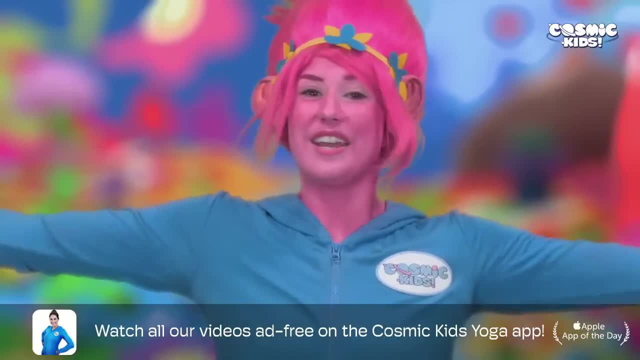 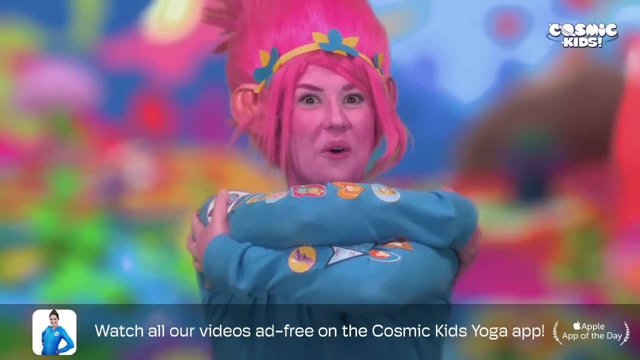 Branch and Poppy share a big hug, Arms wide, Wrap yourself up in that wonderful hug, And Poppy is now The queen. She makes a new law: That hug time Is all the time Coming down to lie in our relaxation pose. 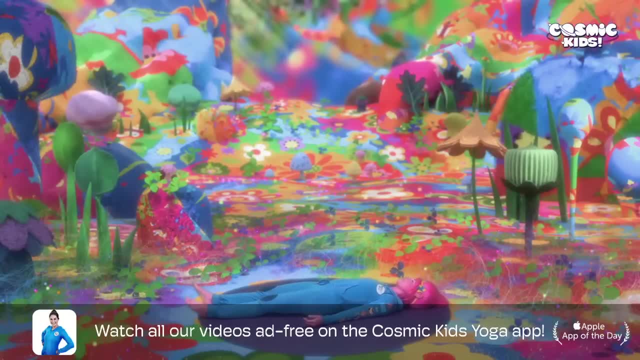 Our legs long And our arms down by our sides. We close our eyes And let ourselves relax here for a few moments, Enjoying this peace and this calm, Letting all of the glitter and the sparkle settle in our hearts. So often we look for happiness outside of ourselves. 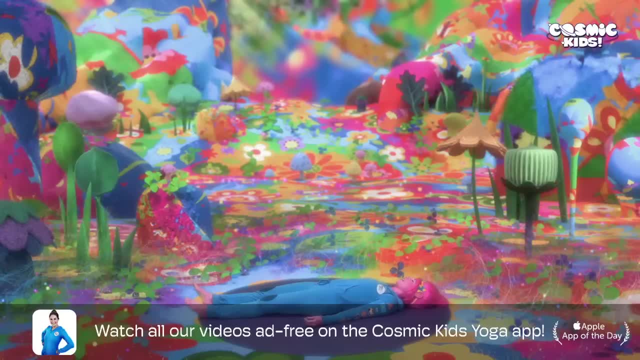 To things that we own, Things that we buy, Stuff, When actually real happiness lives inside each and every one of us. We just have to find it, And the time that we share with loved ones, With friends and families, We can double. 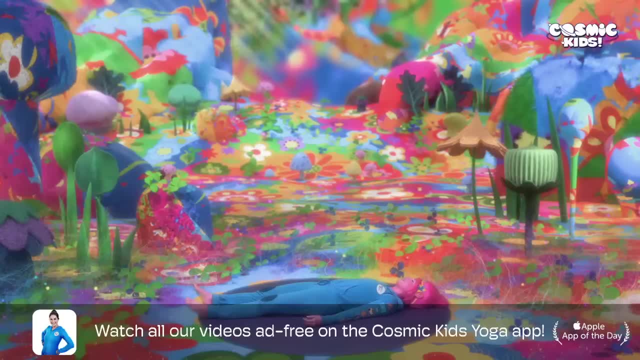 Triple And maybe even quadruple our happiness By sharing just that special time with them, And the happiness we feel from a hug Is so special and so strong. Look for the happiness in the little things in life, And that means life will be full of glitter showers. 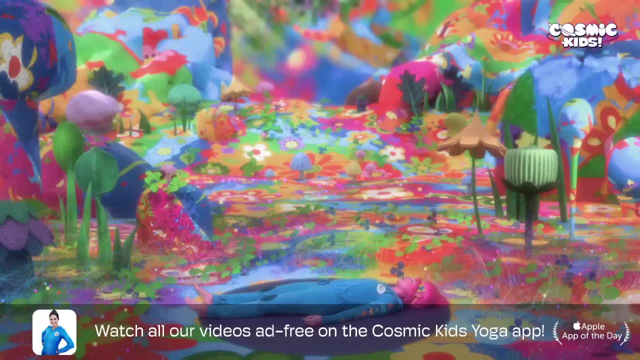 And rainbows, Just as it is for the trolls. And now it's time to wake up. We wiggle our fingers and our toes, We bring our knees into our chests And give them a nice hug. We roll onto our sides. 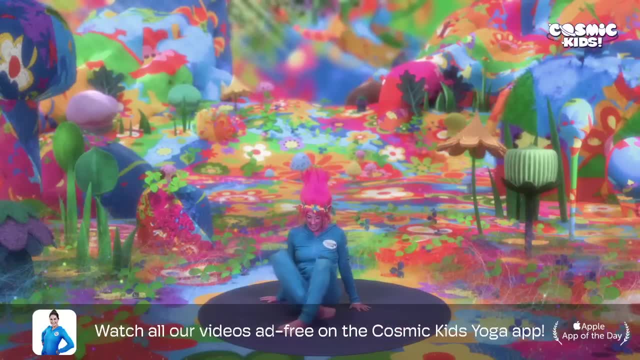 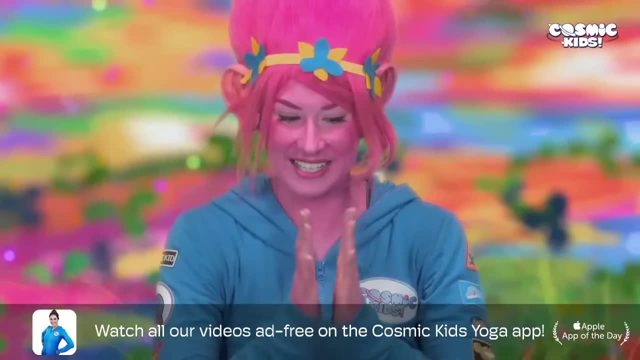 Pushing ourselves up to sit, Opening our eyes And crossing our legs. We finish just the way we started: With a namaste. So we bring our hands together at our hearts And after three, Let's say it together: One: